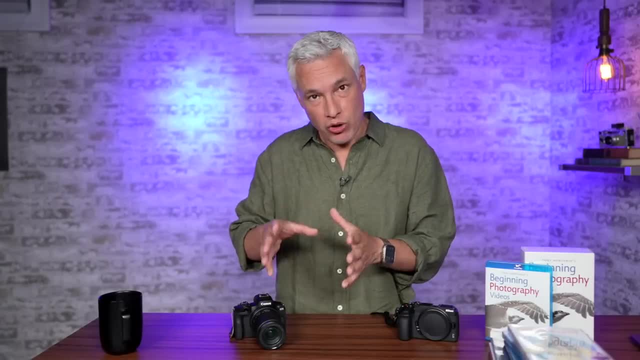 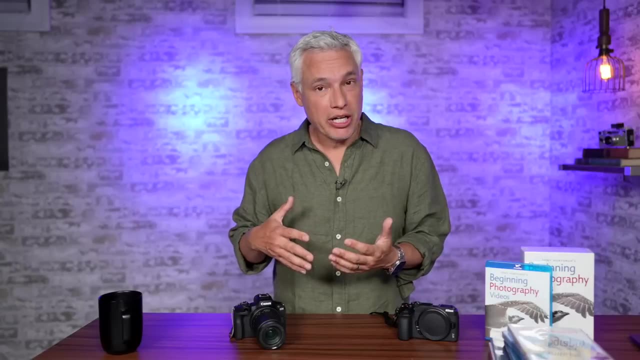 training series because it is structured, it is based on real-world fundamentals and it has practices at the end of each section. So I hope you'll watch it, I hope you'll bookmark it and come back to it because it is a lot And if you like having structured education and you. 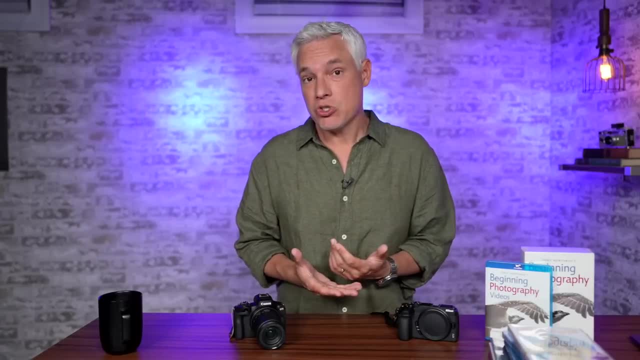 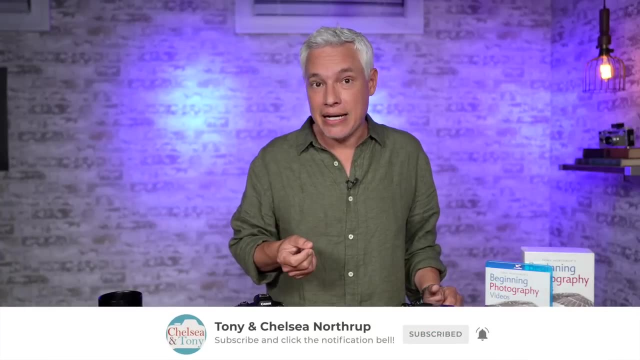 think other people need to learn the fundamentals, then please share it And you can tell the algorithm that people should learn the fundamentals by liking the video commenting: subscribing: Chelsea and I made this content 10 years ago for DVD. Look a four-DVD pack or Blu-ray. 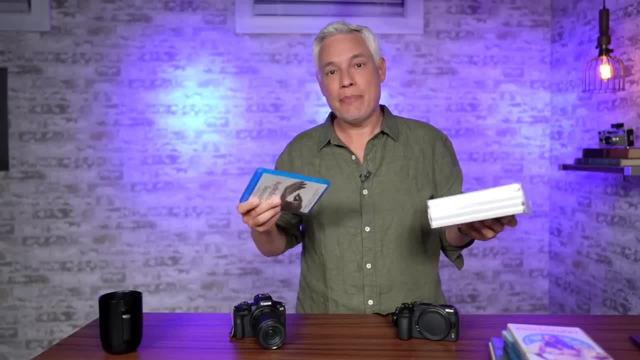 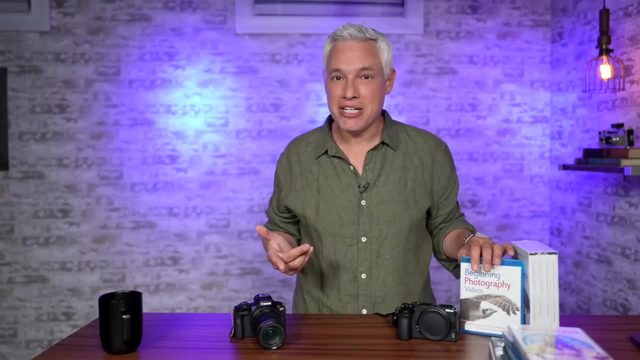 But the fundamentals of photography that we teach: lighting, composition, camera settings. honestly, they haven't changed for a hundred years and they're just as relevant as ever. So I've remastered it, updated it in a few places and here it is for free. Enjoy. Hi, I'm Tony. 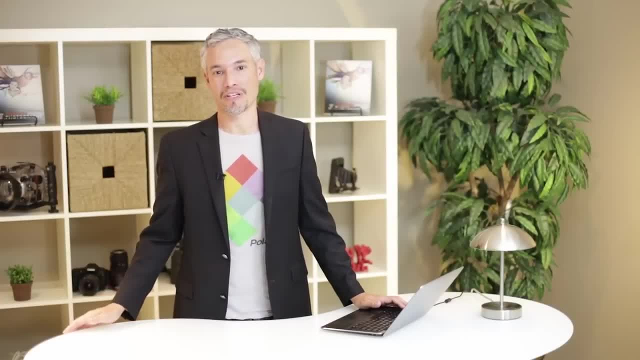 Northrup and welcome to lesson one of my stunning digital photography training series. This is going to cover some really quick tips. We're going to cover lots of quick, kind of bang for your buck tips that we'll get you started really quickly If you're an intermediate or advanced user. 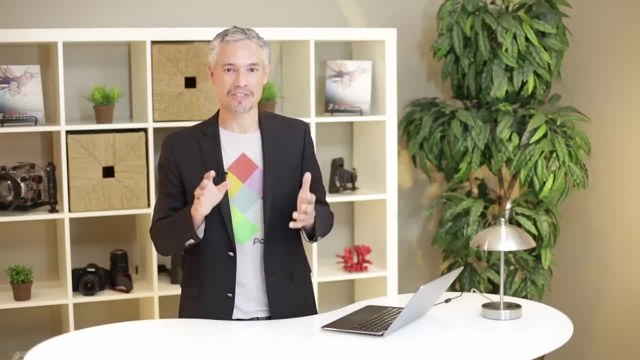 you might think about jumping forward to lesson two, or maybe even jumping straight to lesson six, where we get into specific types of photography. So I'll get started with tip number one, which is to not worry so much about your gear and the settings. I'll tell you what I get. 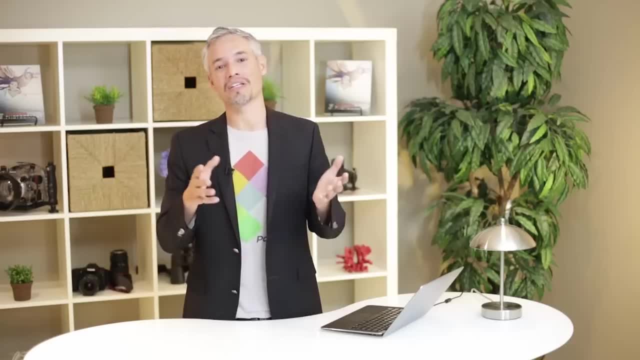 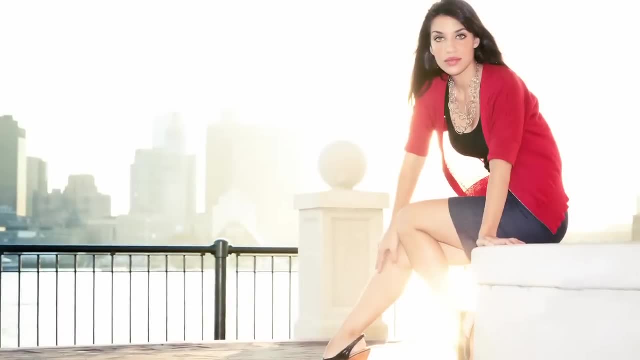 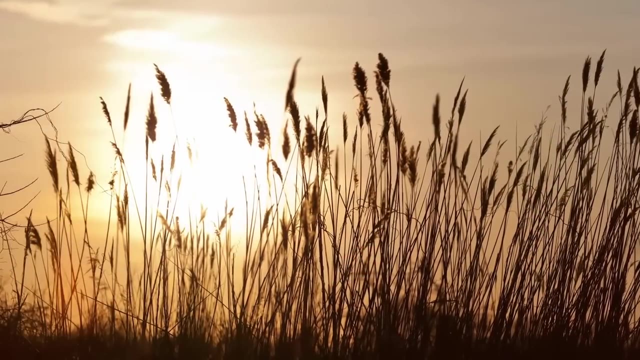 questions from people all the time Like picture, what lens are you using, what's your aperture? but nobody ever asked me: how did you find that location? what did you say to the model to bring out that expression? how did you plan the lighting so that it passed right through? those reads so nicely, and i think those are the far. 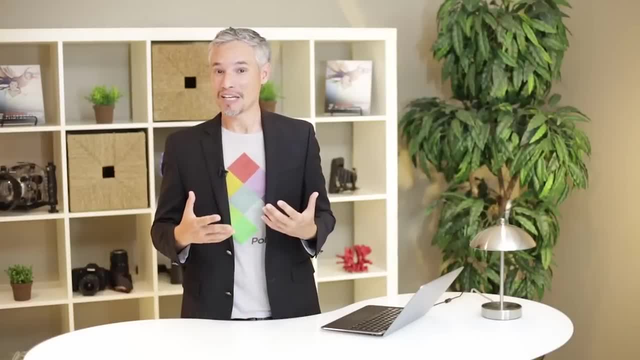 more challenging aspects of photography. but, frankly, guys like me, the geeky types, tend to get really involved in the camera gear and they think that's where all the answers lie. they just need to buy the right camera, the right lens and put the right settings into it and they'll get. 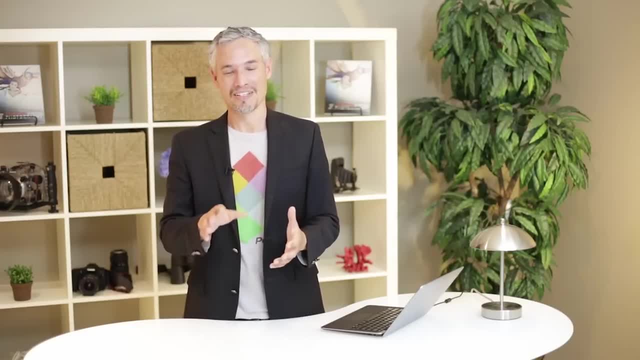 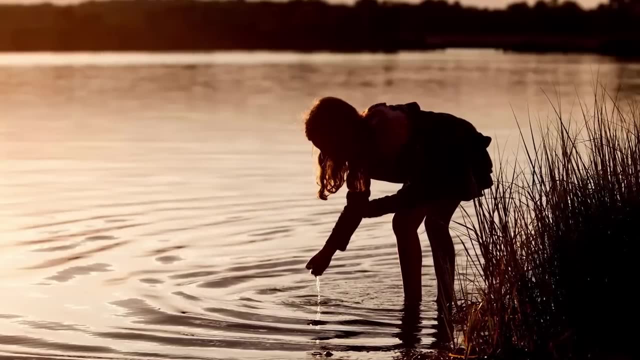 the pictures that they want, but that's not how photography works. let's take a look at a couple of pictures. this is a picture of my daughter that my wife, chelsea, took. now you can see that this is a really nice picture, and it's nice because it captures a really nice moment, and you can see that. 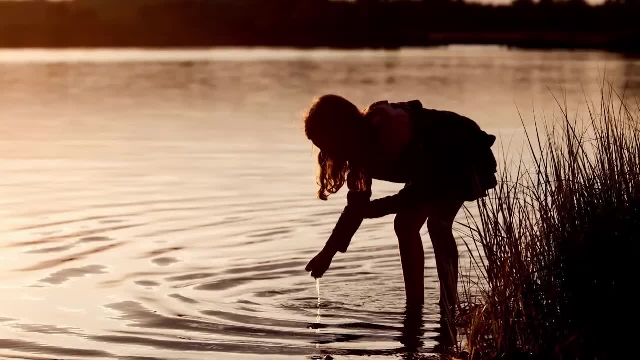 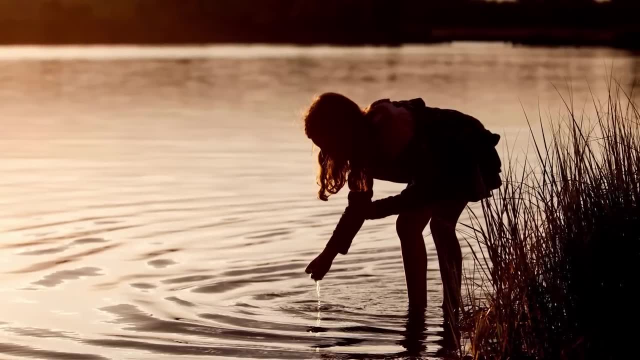 she's pulling something from the water, which is her absolute favorite thing to do in the world, but it's really the lighting that makes it nice here. the sun was really low in the sky and it was reflecting off the water in such a way that you can see all the ripples and chelsea. 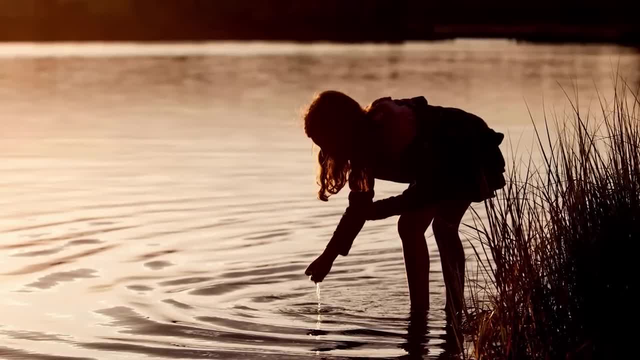 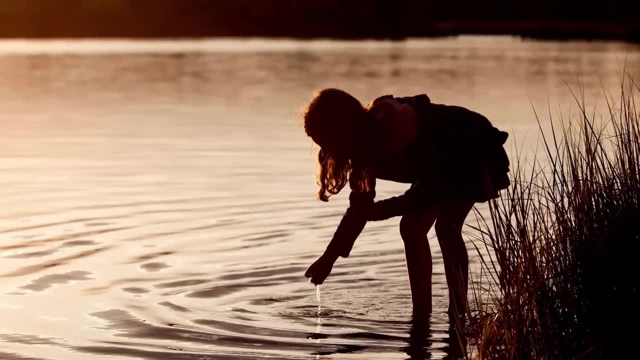 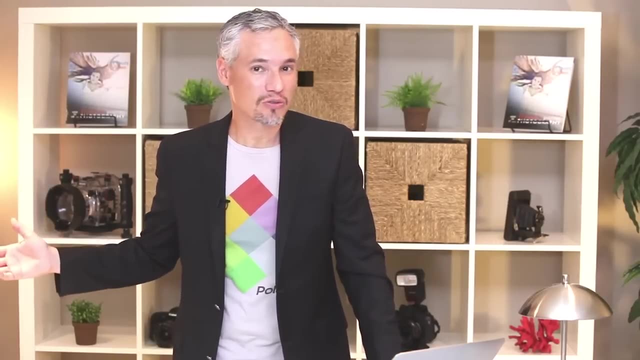 intentionally exposed it to silhouettes. so madeleine and the grasses there are underexposed and it just shows you the very nice shape that they provide without providing a lot of form that would otherwise distract you. and somebody, of course, asked me what the shutter speed of that picture was, and well, the answer is 1, 1500. but you 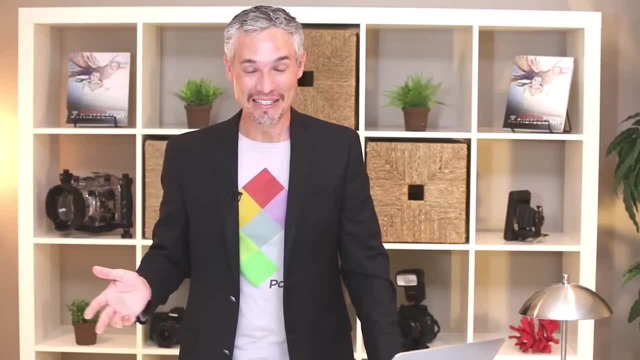 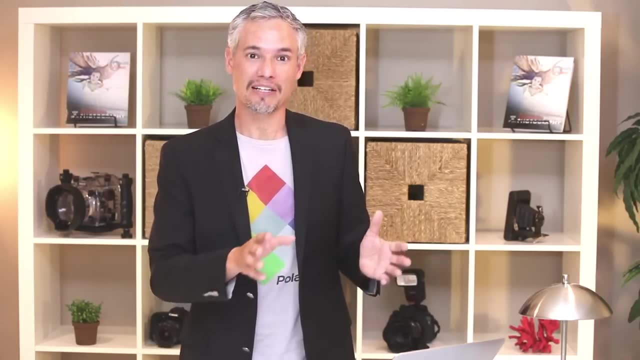 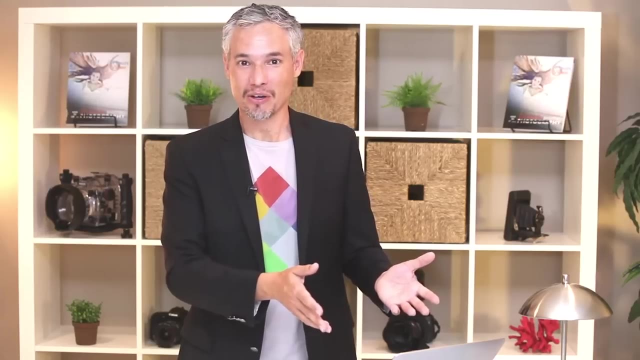 can't just set your camera to 1 1500 and get that picture. instead, you would need to do what we did, which is to think about the lighting, find a day where the sky was going to be clear and find a place where the sun was going to be, and find your subject. and that's what we did, and then we just 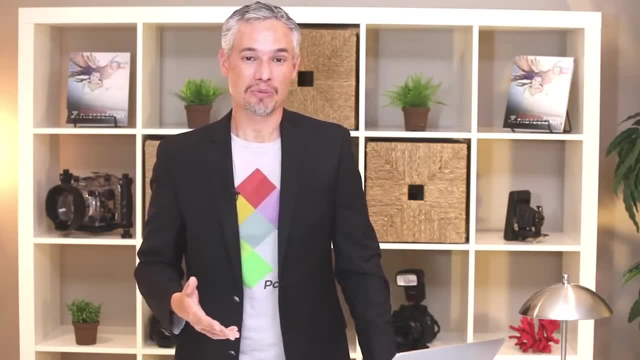 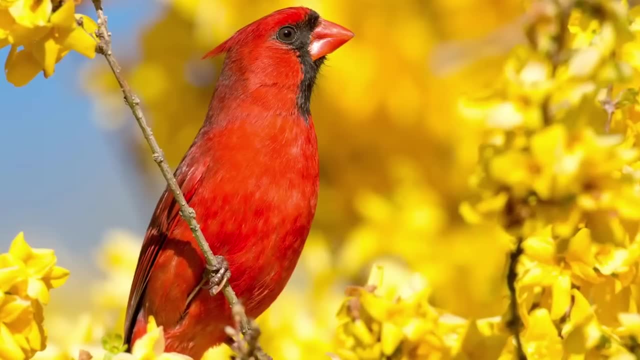 let madeleine go and do what she was going to do anyway, but by planning a nice location i was able to get a great picture out of it, and camera model, lens, camera settings had nothing to do with it. let's look at another picture. this is a picture of a cardinal that i took in my very own backyard. 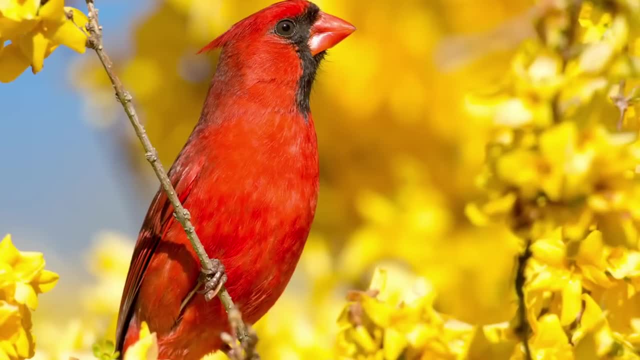 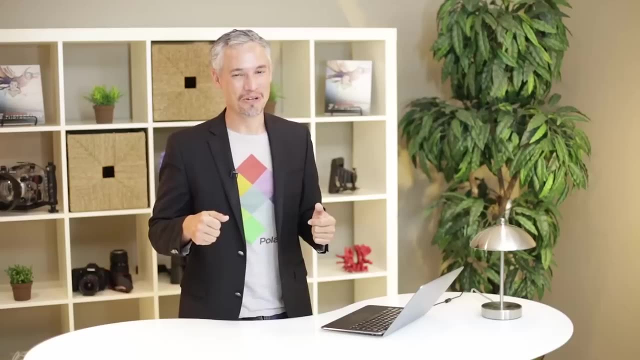 and of course everybody says: what lens did you have? i'm not even going to tell you, because you know what. the lens doesn't even matter. what does matter is that i spent a couple of weeks camouflaged tent with my camera on a tripod and i brought the birds in, i put food out and 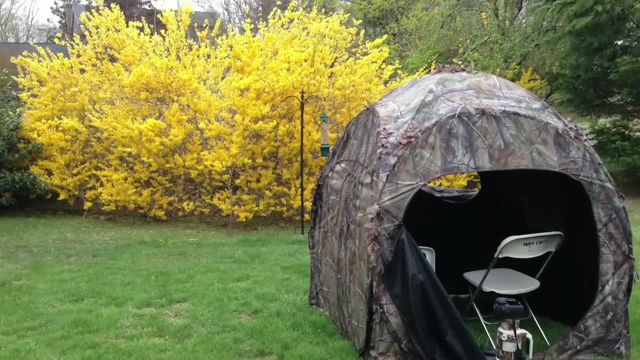 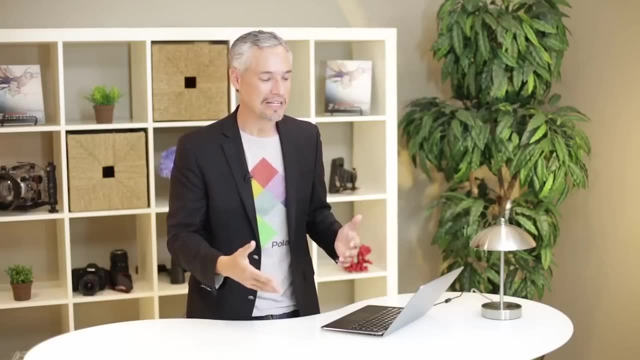 then i used some bird calls and i set up this very nice station near this flowering yellow bush that i had. that i also intentionally planted because i knew birds would like it and i knew it would provide a good backdrop. so an awful lot of planning and preparation and time. 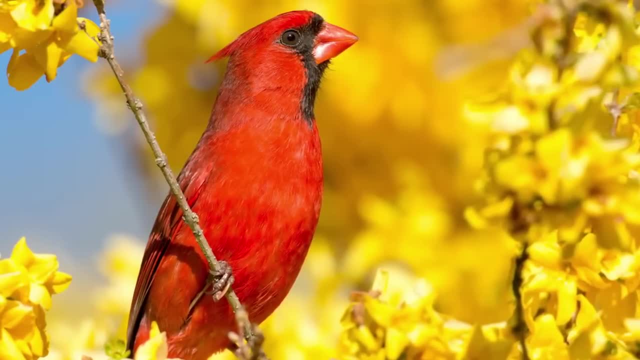 went into this picture and the settings such a small part of it that it is completely insignificant and you don't need to worry about it. so, of course, you should share your photos on your facebook page and share your photos on your facebook page and share your photos on your facebook. 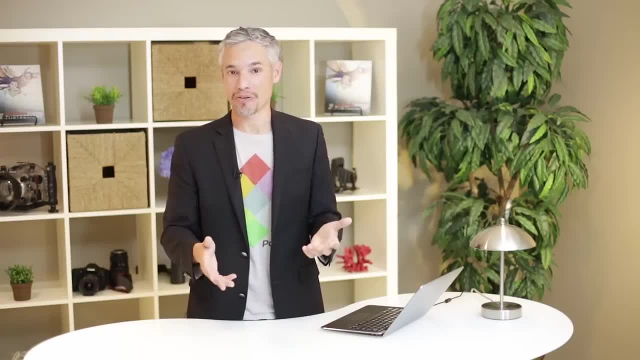 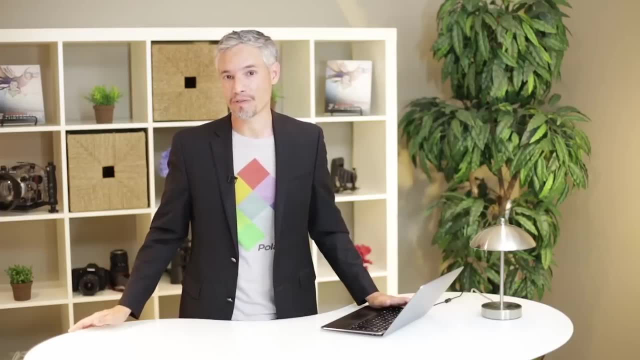 page because that'll give you a good idea of what pictures are better than others. you'll get a certain number of likes or you'll get in certain reaction out of people. but i also recommend setting up a facebook photography page for yourself. you can just call it tony northwood. 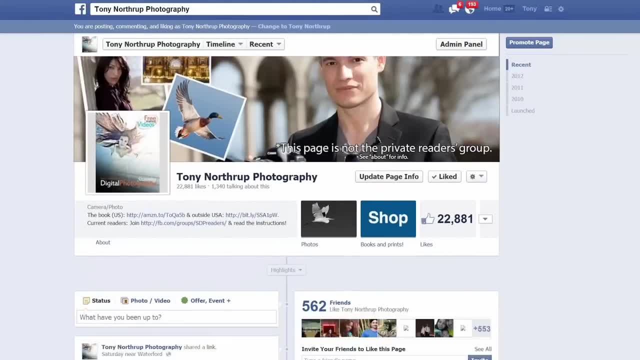 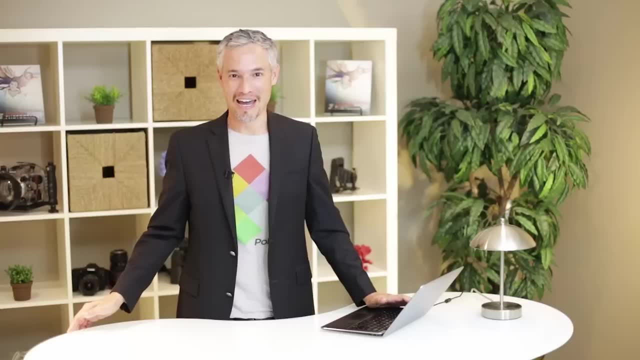 photography, or maybe use your own name, and this will allow people who are interested in your photography to follow you, without you perhaps annoying everybody else with every picture that you take of your cat. but the important thing is that you get out there and you're actually using and sharing your pictures. 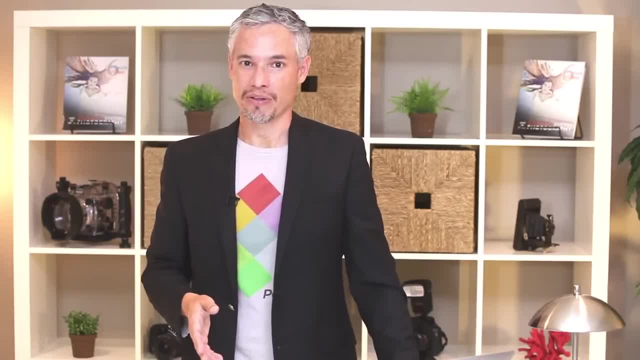 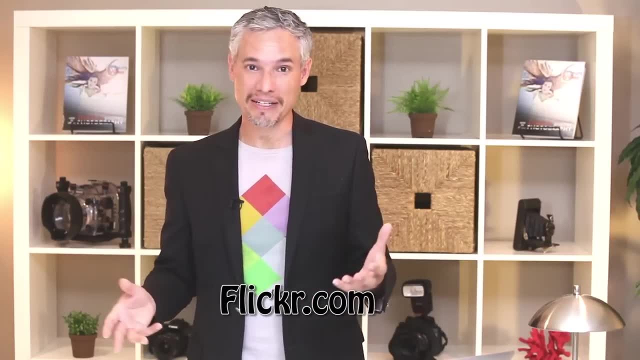 besides facebook, there are a lot of other great photo communities out there. my favorites are flickr, which is just great for sharing photos and allows you to view full-size photos and see other people's metadata. that's also a great way to learn, besides just getting feedback. i also recommend checking. 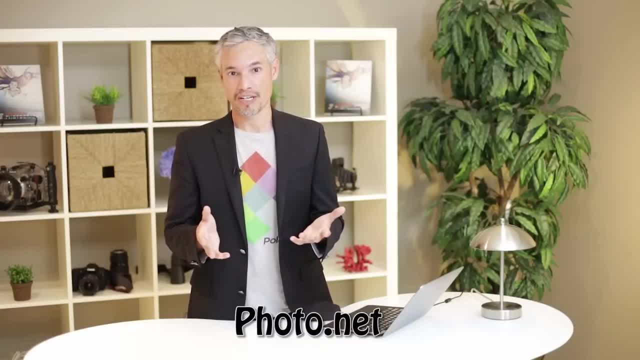 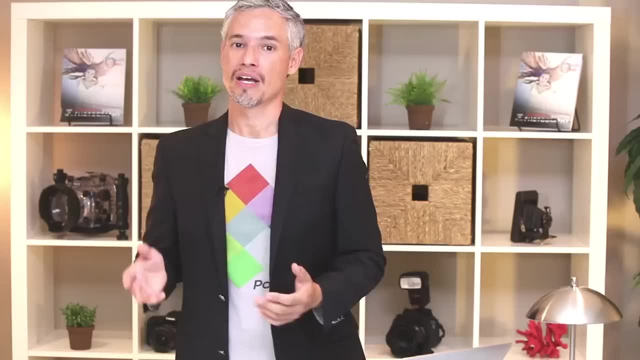 out photonet. photonet is really the original community and it was founded by a friend of mine, philip greenspun, and it's still a great place to share your pictures and get questions answered and, finally, check out deviant art. deviant art leans towards the more 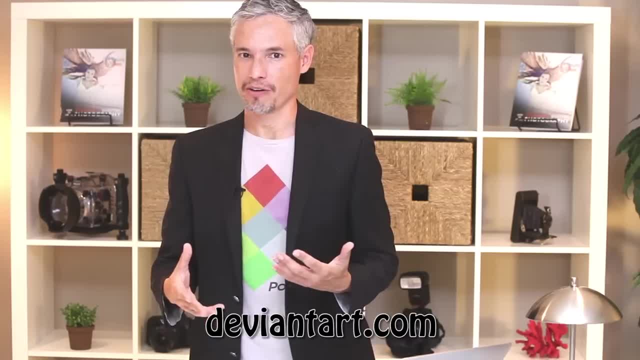 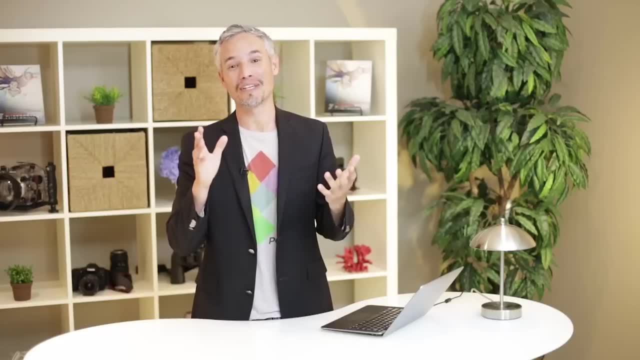 creative side and includes a lot of artists that don't work in photography- painters and sculptors and such- but if you are the creative type, deviant art is a great place to go. now, of course, you don't have to be on your computer to be using your pictures. i highly recommend getting old-fashioned. 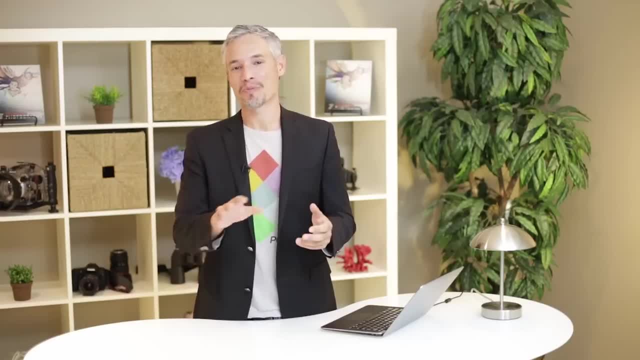 prints and putting them around your house. sometimes people wait until they get like the perfect picture, but don't wait for that. take your favorite pictures that you have now and put them up, even if there are flaws in the picture. you know what? you'll start to see them every day and that 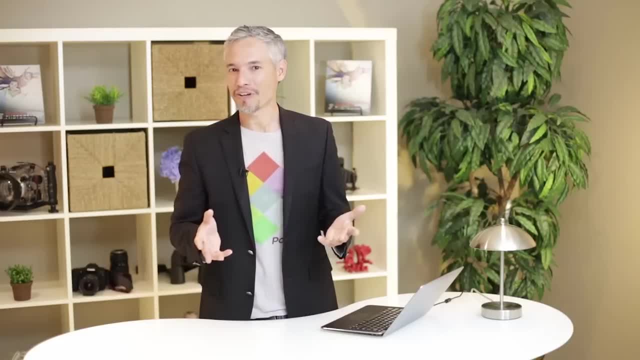 will remind you of how not to make that flaw in the future. and prints are fairly inexpensive and you can always swap them out later. my favorite place to get prints is mpixcom. it's not the cheapest out there, but they do great quality work. here we can see a couple of terrible iphone. 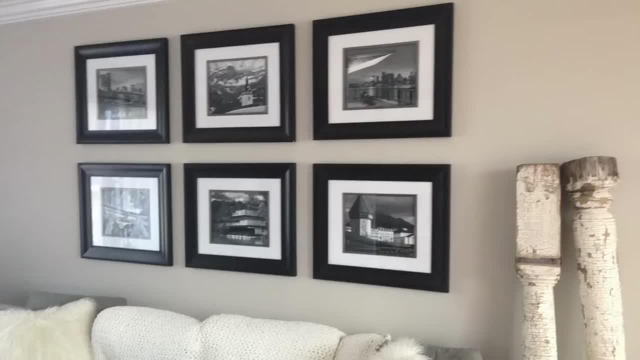 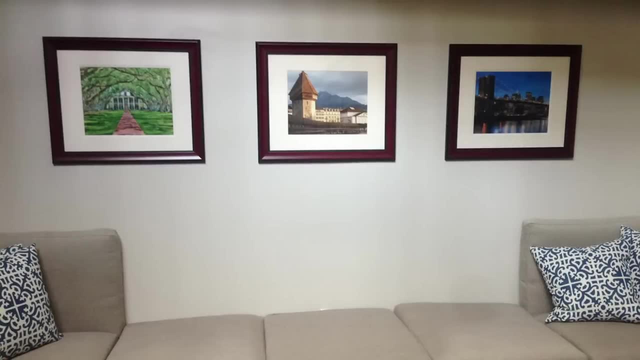 pictures of my own house, but just to show you how i've displayed different pictures, these are pictures from the travels that chelsea and i have taken. here's a series of pictures in the basement of different locations. i just like to see the pictures every day and it just reminds me. oh, that's. 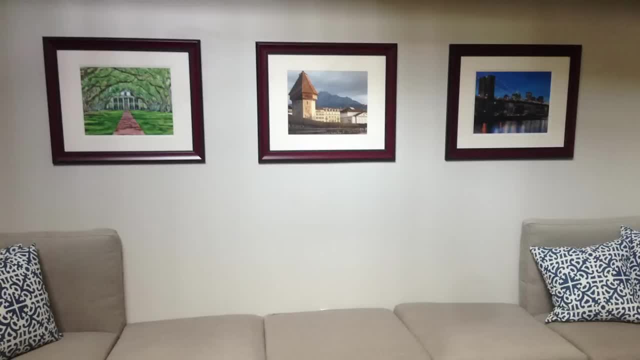 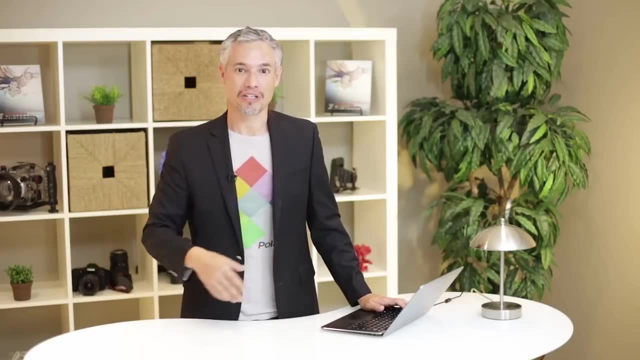 i love taking pictures, but also reminds me of where i was when i took that picture. i also love putting my pictures in galleries, and it's not as hard as you think. my town has a gallery called the hygienic in new london, connecticut, where they allow anybody to put up a picture, and every single year. 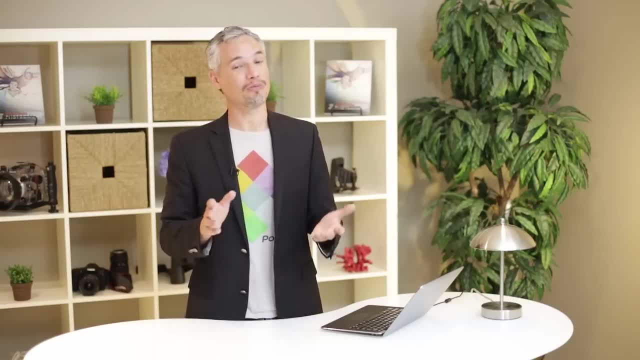 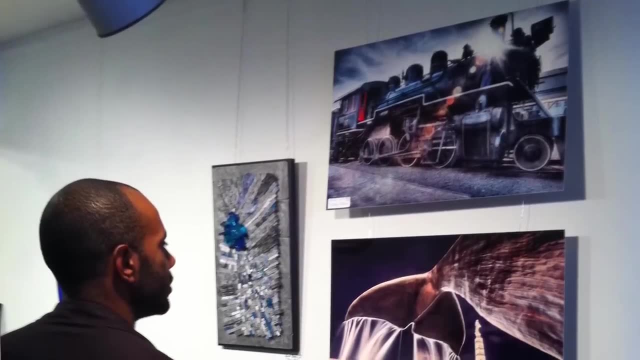 chelsea and i put pictures in and it's a lot of fun and sometimes you sell your picture, sometimes you don't, but you always get some feedback. so here you can see pictures by both chelsea and i. mine's the train on the top there at the local hygienic gallery. my third tip is to know your. 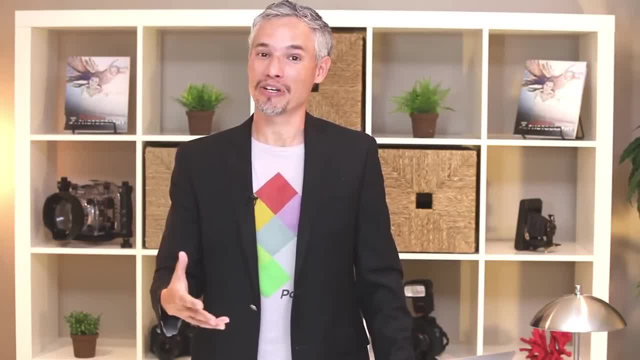 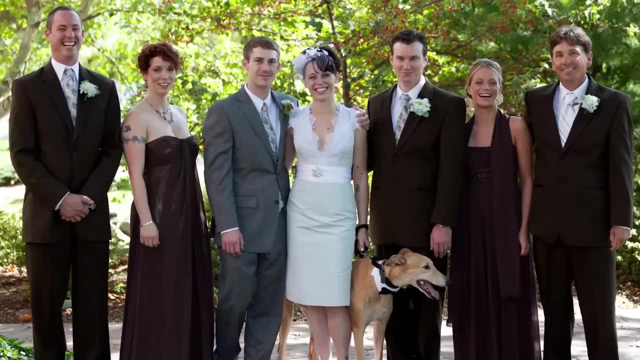 location. the way you take a picture is going to be partially defined by how you're going to use it. for example, if you're going to make an 8x10 print, you need to remember to leave some room on both sides, because 8x10 prints are cropped from the shape of a standard camera sensor. another factor: 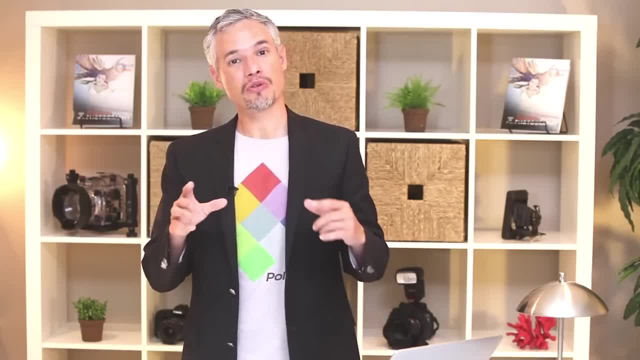 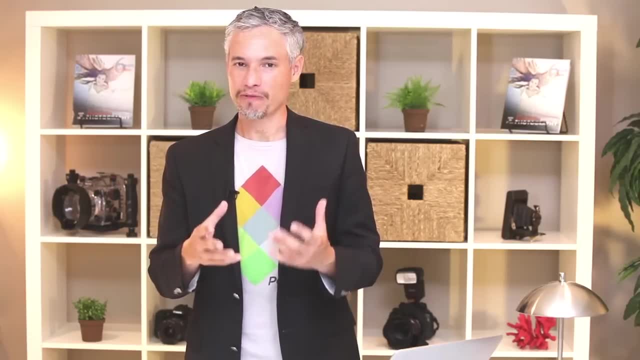 to consider is how the picture is going to be viewed. if a picture is going to be viewed in a small format, you want a very simple close-up picture. a very detailed picture will be far too complex to be eye-catching at all if you're going to be able to take a picture in a small. 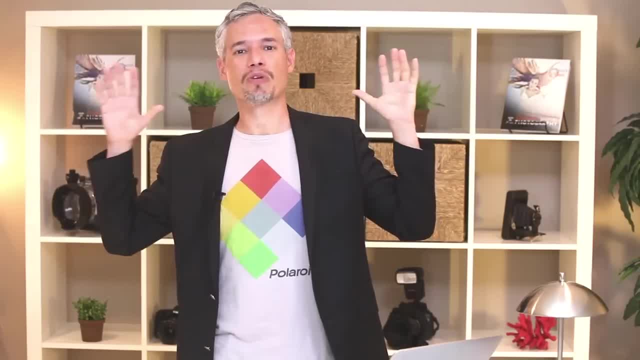 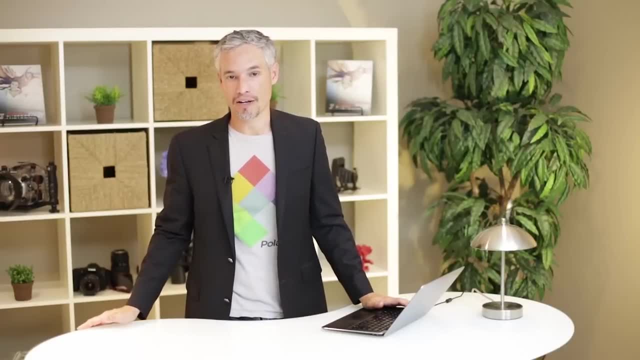 format. you're going to be printing a really huge print. go ahead and take that really detailed cityscape, because people will be able to get close and inspect all the detail. now, if you're going to primarily be sharing your pictures on facebook, something you need to think about is that people 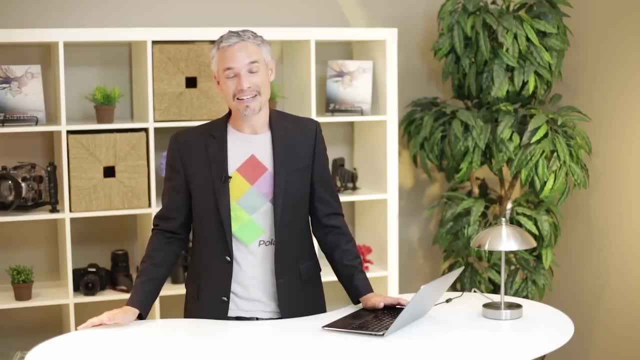 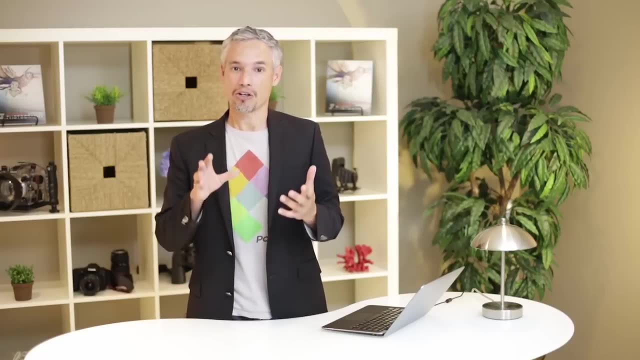 see the thumbnail before they see the full-sized picture. and if you have a really complex picture, that thumbnail isn't going to look like much of anything at all. if you want somebody to actually click a picture, you want to take close-up pictures with very little complexity to them. they can later. 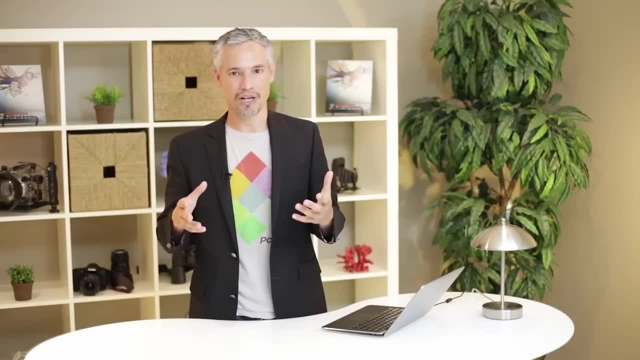 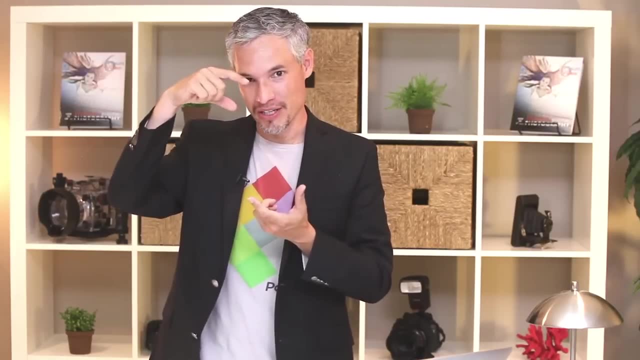 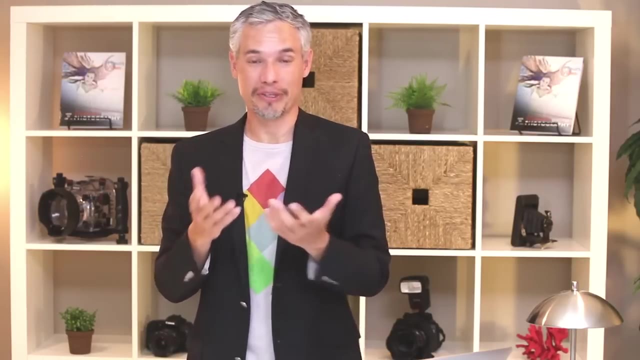 see more detail, but i really don't like to put complex pictures on facebook. crop it down and simplify it. another factor to consider is horizontal shots versus vertical shots. now, most people take horizontal shots because that's just the way the camera fits in your hand most comfortably, and this is the case for me too. probably 95 of the shots i take are horizontal. 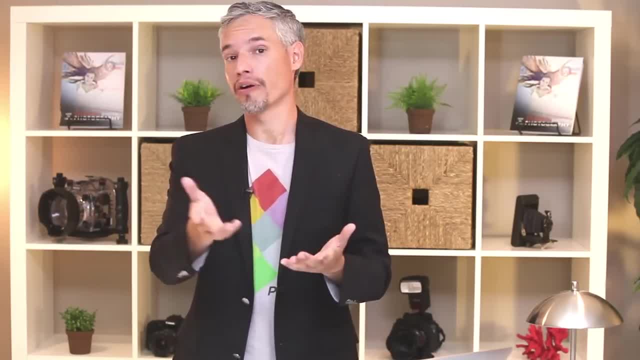 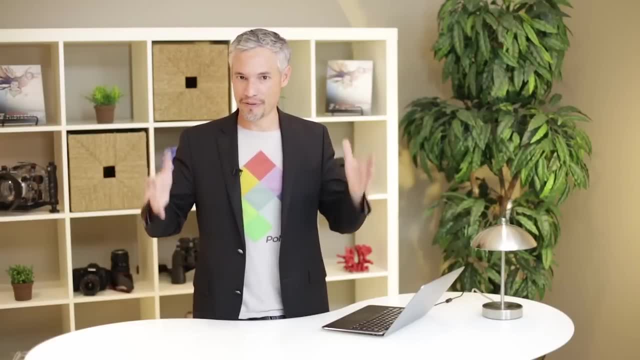 that's also the best way to take pictures for viewing on the web or in video like this. however, there are a lot of great uses for vertical shots too. maybe you're decorating your house and your house happens to have a space where vertical shots would look perfect, or maybe you're a commercial. 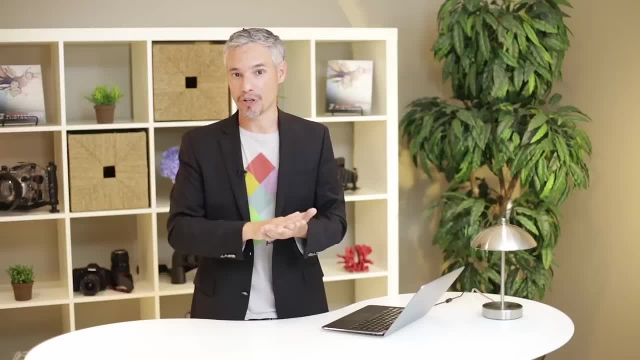 photographer and you need to take a picture for a magazine or a book cover. you need vertical shots for that. anytime you're taking a picture of something and you think that shot might be a winner, go back and take horizontal shots and vertical shots and zoom in tight and shoot wide, because you 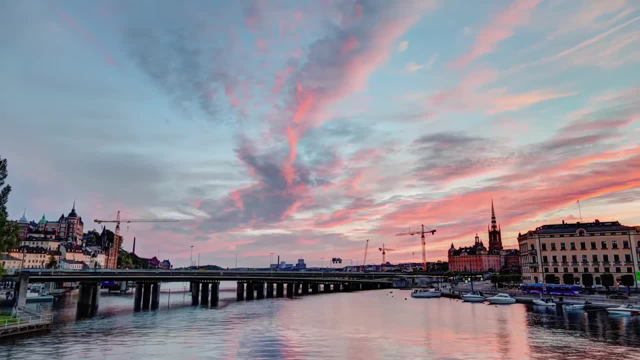 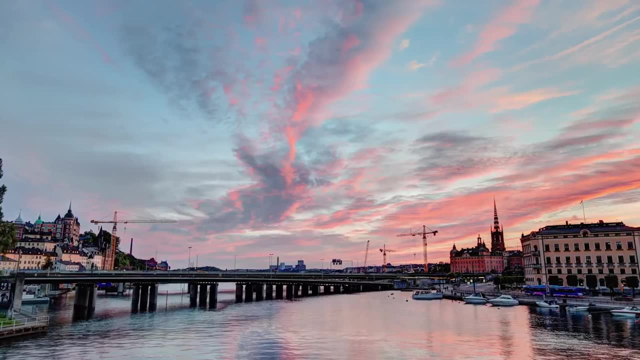 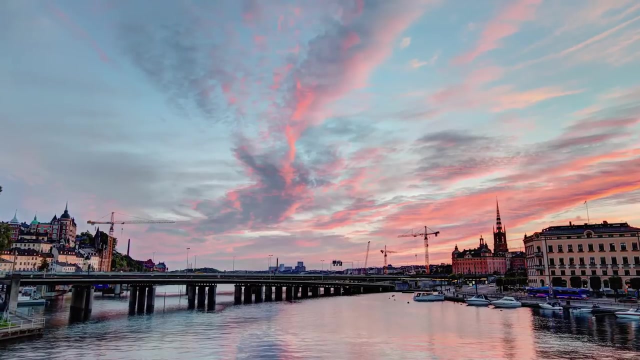 can't take too many shots. here we see a beautiful sunset in stockholm, sweden, where the sunsets literally last all night long in the summer. however, this picture would not be good on the web and in fact i never really shared it, because if you see this at thumbnail size, it just looks like a little mush of blue and red and 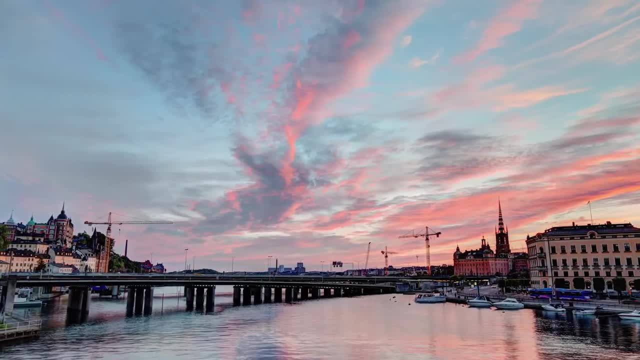 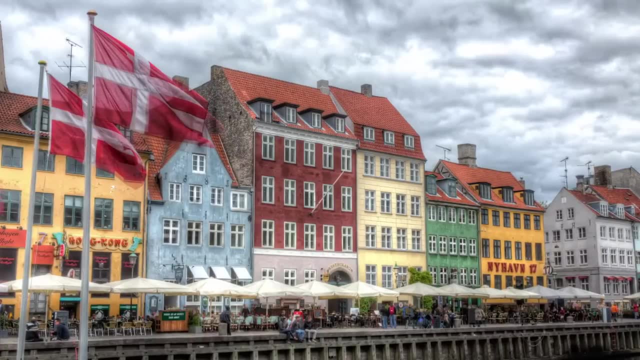 to really appreciate this picture, you need to see it in a large format. so if i were making a wall size print, i would definitely consider this picture, but it's not a good picture for the web. this picture is actually quite a bit better because you can see we're closer to the subject. 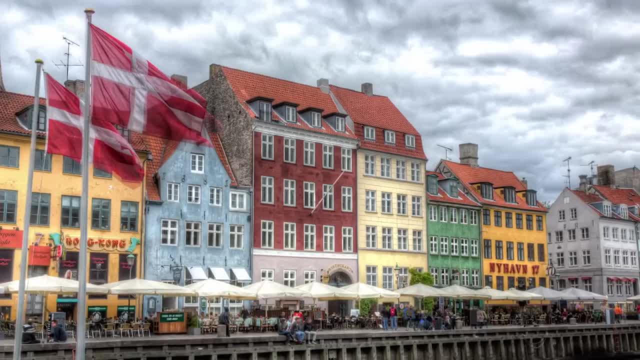 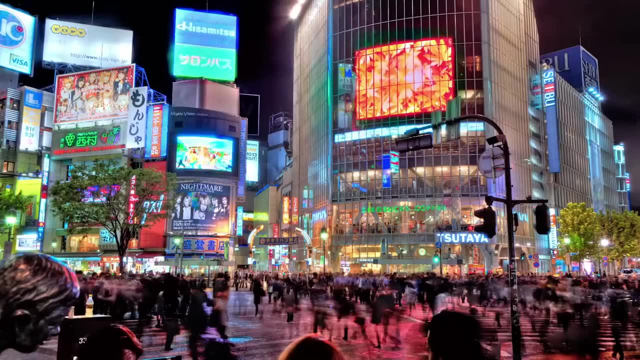 and even shrunken down to a thumbnail, you'll be able to see that it's got colorful buildings and an intense sky and you'll have an idea of what it is and maybe you'll want to explore it a little bit further. here's another picture that is not great for thumbnail or small format viewing either. 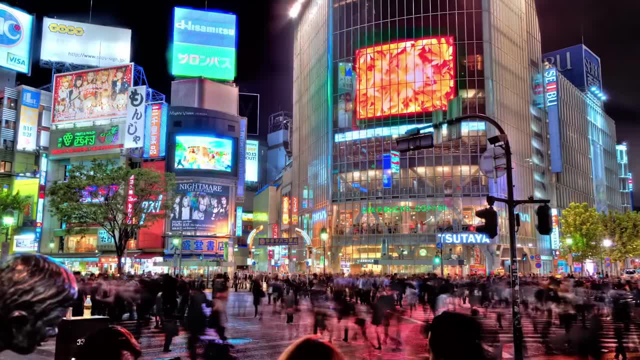 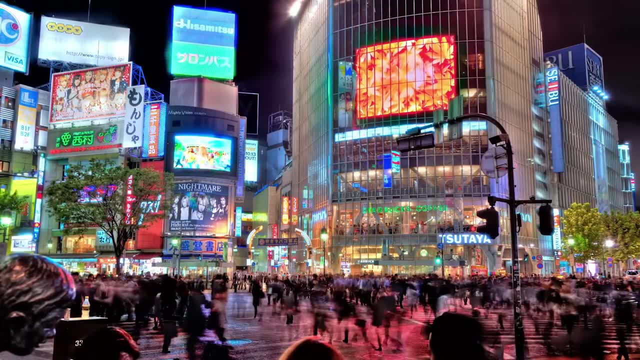 this is shibuya station in tokyo, japan, the busiest intersection in the world, and it's a really great place and i was happy with the way that i captured that hustle and bustle. when you view this on the web in a small format, you can't tell what's going on and in fact, it doesn't have any really bright. 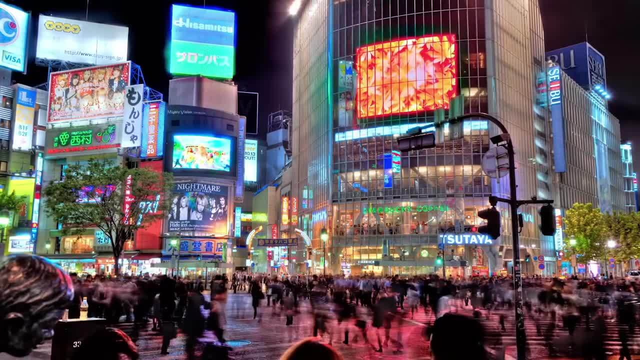 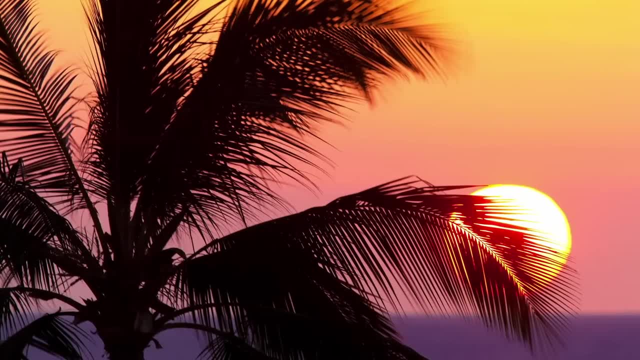 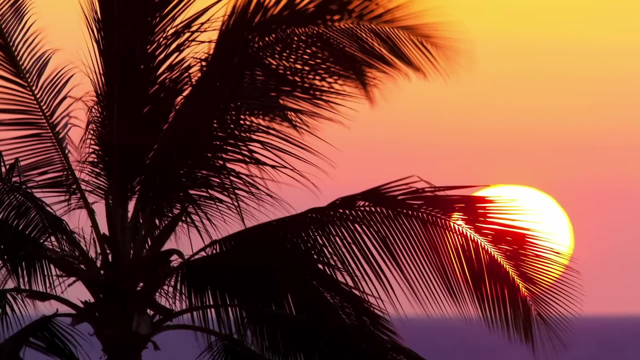 or intense color so it doesn't draw the eye at all. but in person, in a large format, especially in a small format, it really shines. here's a picture that is great for the web. you can see it basically just has three elements: a palm tree, a sun and the horizon. in a thumbnail you can see exactly what. 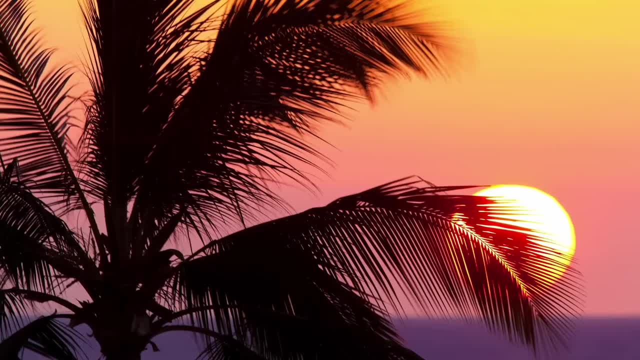 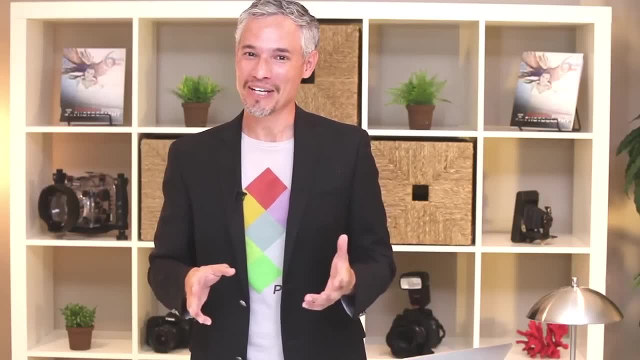 this is going to be, and when you click on it to view it full screen, you get satisfied when you see it. the thumbnail here is really appealing, and a picture like this gets a lot of views and love on the web. my next tip is to get a second opinion on your pictures. we'll develop some. 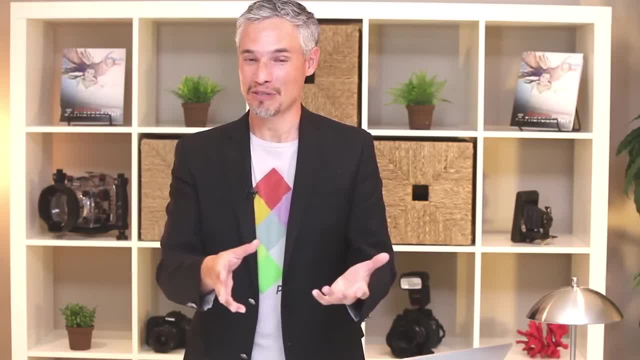 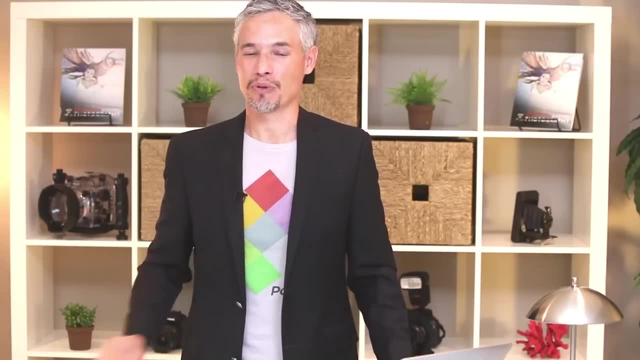 unnatural affection for the pictures that we take, because maybe we love the subject, maybe it's our pet or our child, or maybe we're just proud of the effort that we put into the picture, but it doesn't mean that other people are going to like it. if you want to know if a picture is really good, 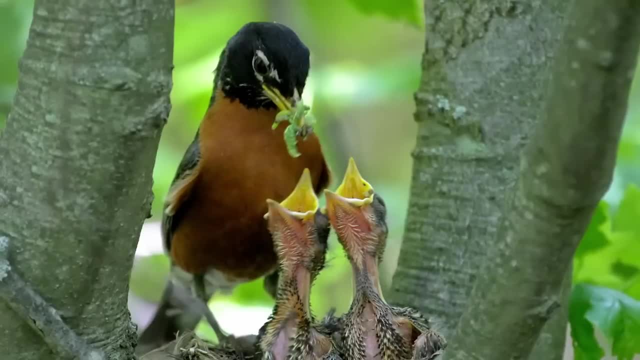 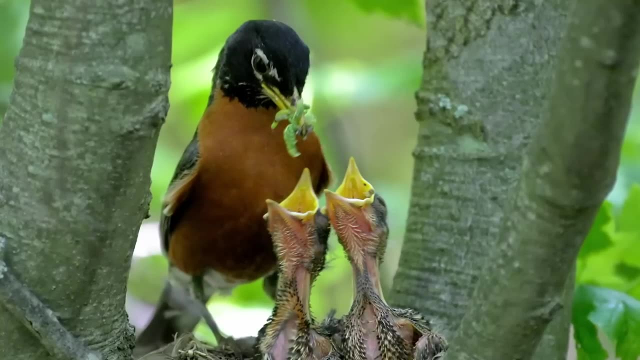 or not, you need to ask someone else. here's an example. this is a picture that i love, because i spent about four hours in the woods holding up a telephoto lens. all my arms ached when i was done, but i finally got the picture that i wanted, which was this mother robin feeding her two babies a 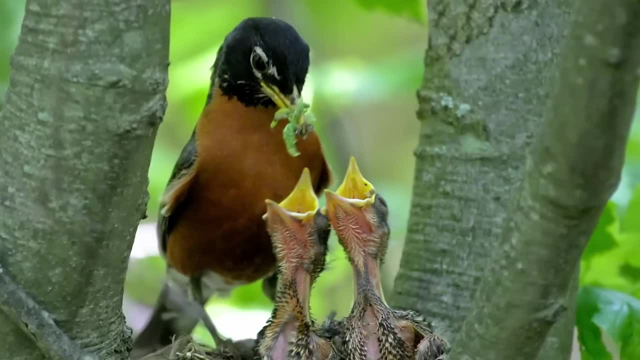 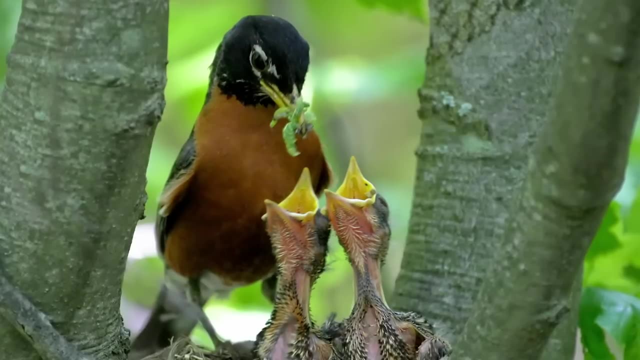 bunch of worms and everybody hates this picture. i love this picture to death. love it because, well, for one, i'm not turned off by the sight of a bird with worms, and it turns out nobody else really likes to see worms being eaten, but two. i also remember being in the woods and the 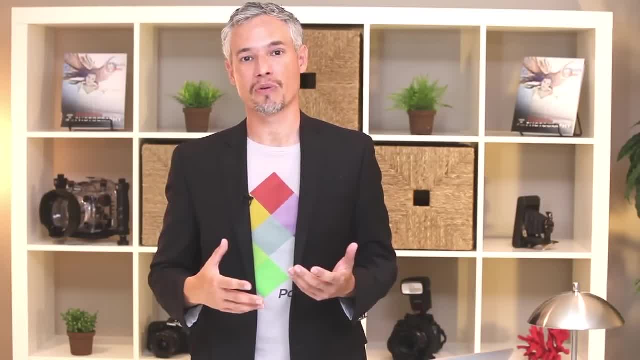 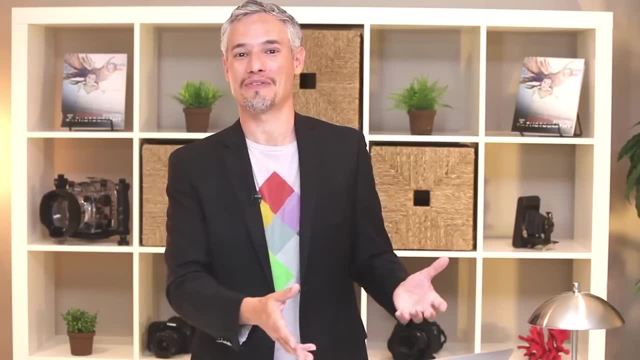 experience of hanging out with the birds and it was a really pleasant experience for me- and those feelings go into the picture when i see it. but other people don't have that same experience, so they just see what they see as kind of a gross picture. here's a picture that other people like. 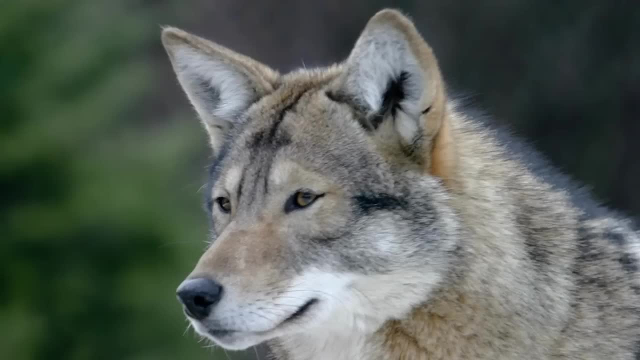 much better than i like it. for a long time this was my top selling stock photography picture and just took this at a zoo. it's a coyote and it's completely boring to me, but it's a popular stock photography picture because it's so simple. it's also really popular on the web because the 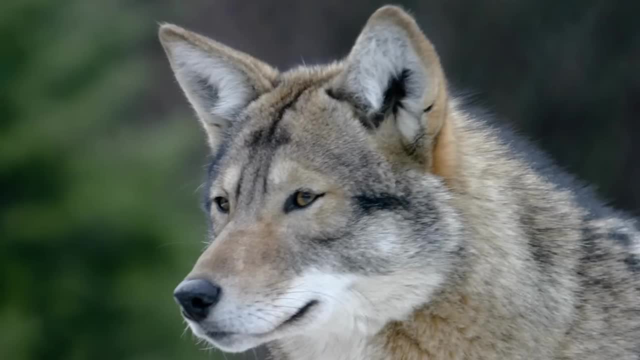 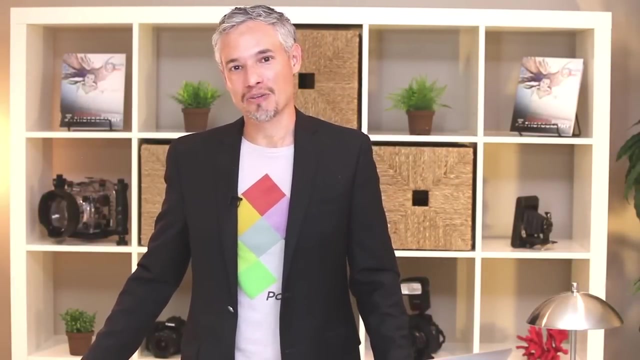 composition is really simple and you can see exactly what it is in the thumbnail. this is actually a better picture than the previous one, even though i have absolutely no feelings for this picture at all, but i really love the other picture. you'll experience the same thing with your own pictures. just ask somebody else and monitor how much you like the picture and 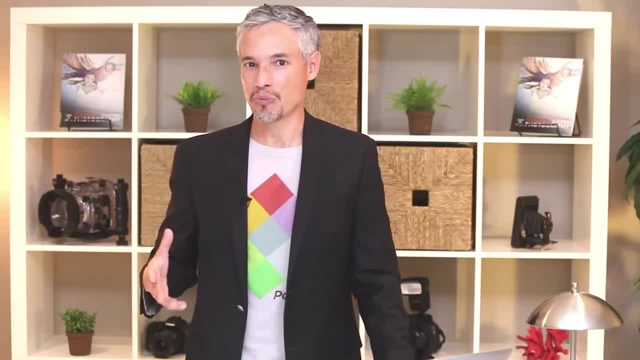 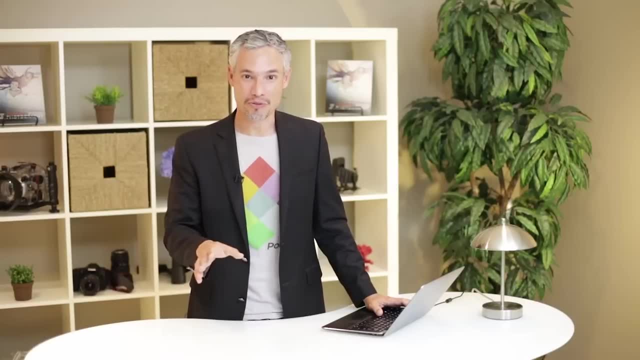 how many likes you get on photos, how many comments you get, and that'll steer you more objectively towards which of your pictures were successful and which weren't as successful. tip number five is: make pictures, don't take them. what i'm saying here is: i don't want to see snapshots from you. 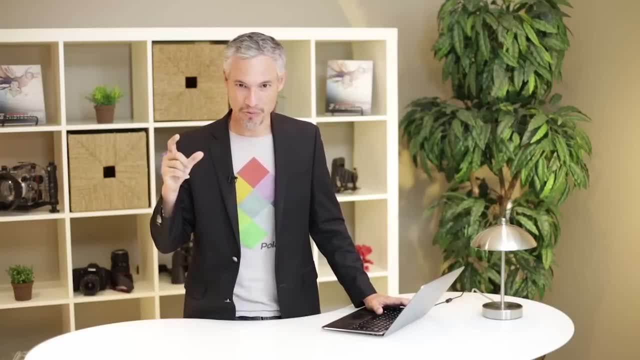 don't just grab your camera and just kind of hold it up and take a picture of what you see. i just want you to put a little bit of thought into it. you don't have to put hours and hours into a project, like i did with that robin picture. you just need to think about the lighting and the. 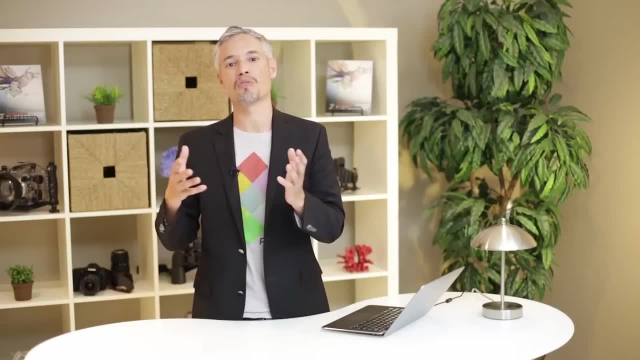 setting and sometimes the difference between the lighting and the picture is that you don't want to get very distant picture between the light and the camera, so that number five is just going to be the same thing, but just look at the picture and your focus on it and the exposure to it. 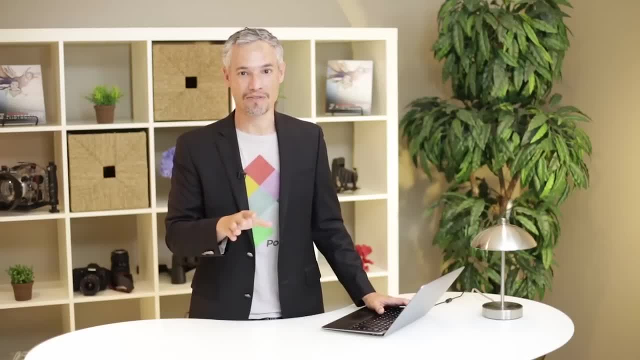 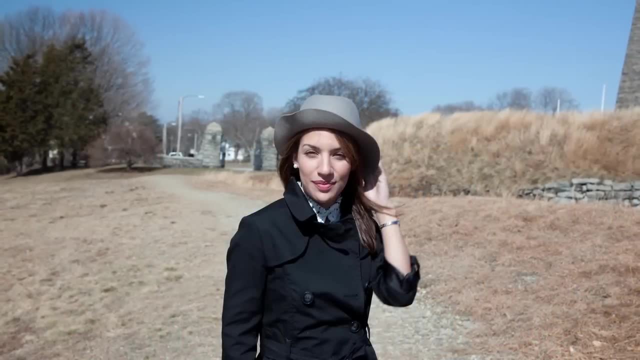 because this is the same picture that you took. in the picture. the only difference between a picture that you take and a picture that you make is 10 seconds. sometimes it might be hours or days, but that extra effort always pays off. let's look at a couple of pictures. here's a picture that i 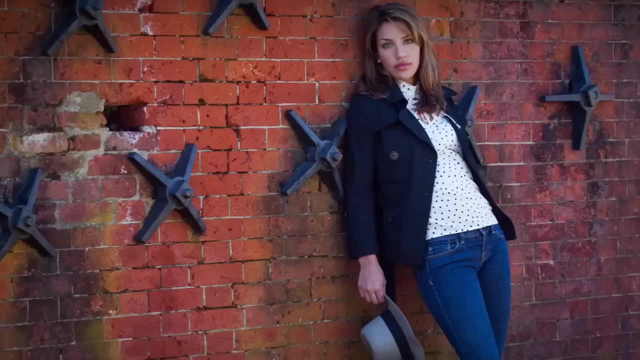 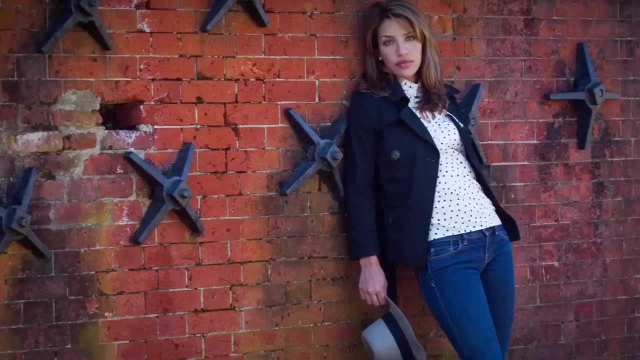 took of chelsea at the park and you can see. it's just a snapshot. she's centered in the frame. the lighting is kind of blinding her a little bit. her hat's falling off. and here's another picture that i She put on a nice expression. 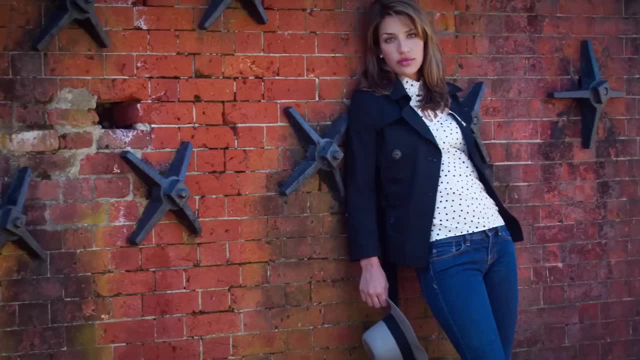 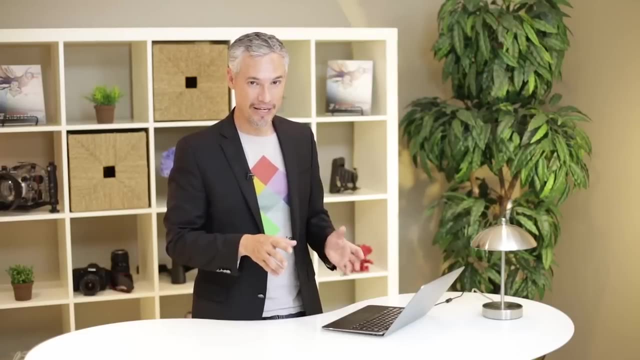 You can see, she went from being in the blinding sun to in the shade, which gave much more pleasing lighting and allowed her to open her eyes a little more naturally. So this is the difference between taking a picture and making a picture. It can be drastic. 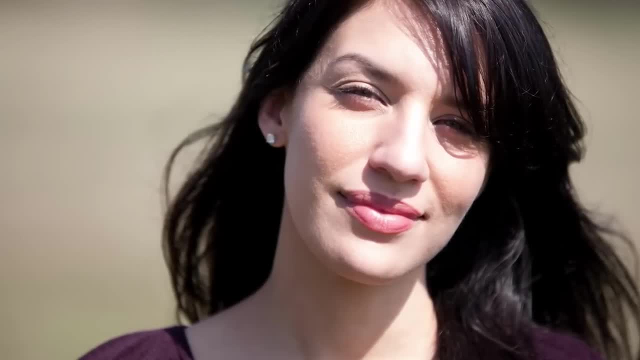 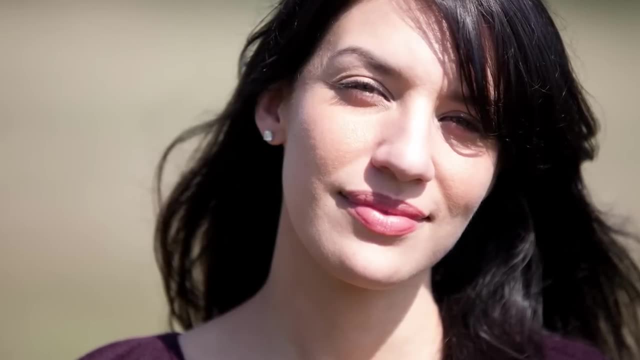 Here's another picture that I simply took of Chelsea. As you can see, there's some of the same situation going on. The lighting here is terrible. She has a decent enough pose, but there's no way this is gonna be a good picture. 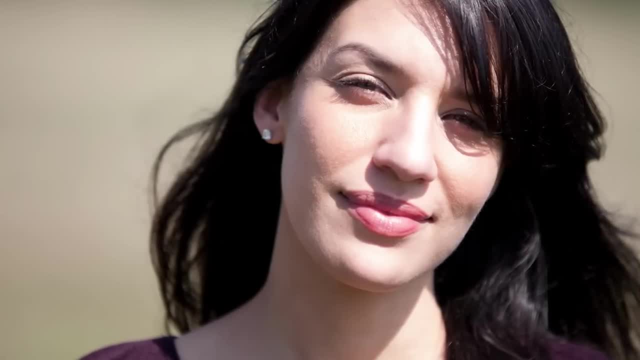 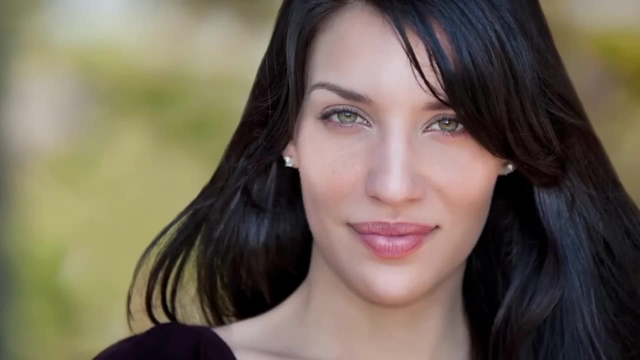 The background is nice and blurred, but it's just gray. Here's a picture that we took just minutes later. I put her in front of a more pleasant background. I moved her into the shade, where she got a nice reflection of the sky. 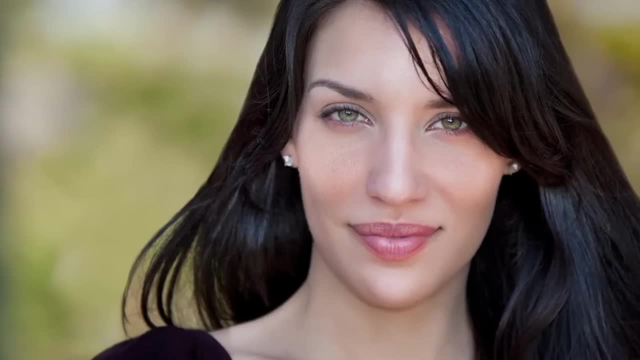 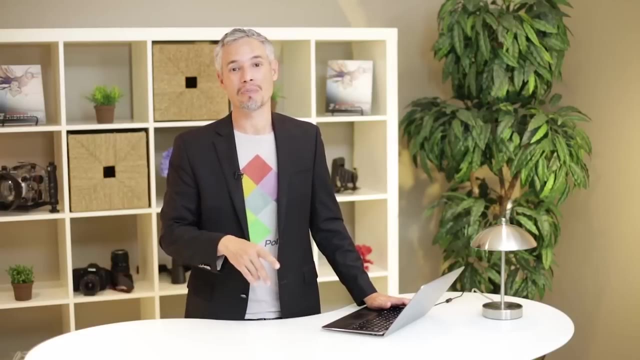 but didn't have the direct light on her face. And then I did a little post-processing too, because that's part of making a picture as well. So remember: make pictures, don't take them and get second opinions If you're looking for another way. 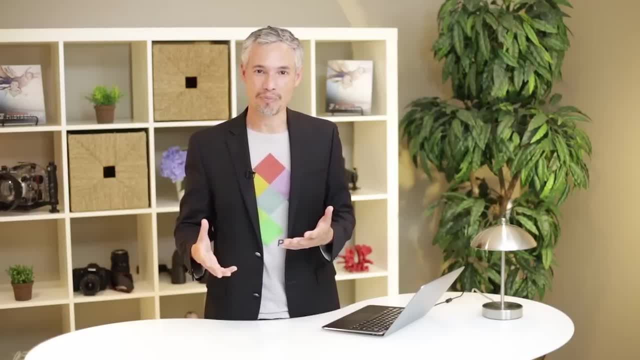 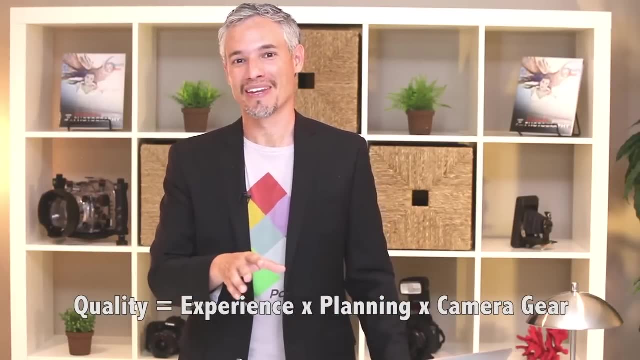 to evaluate your own pictures and know the difference between a good picture and a bad picture, use this formula: Quality is experience times, planning times, the picture Times, your camera gear. What I'm saying here is: you can tell the quality of your picture. 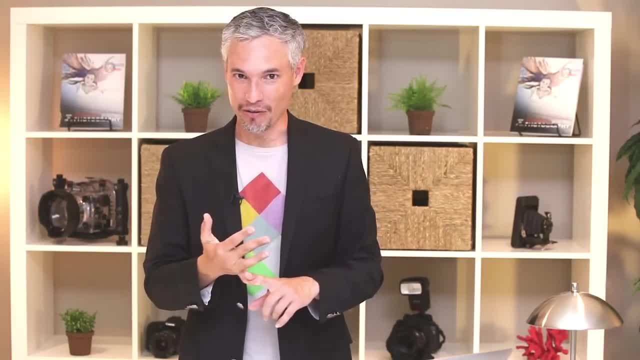 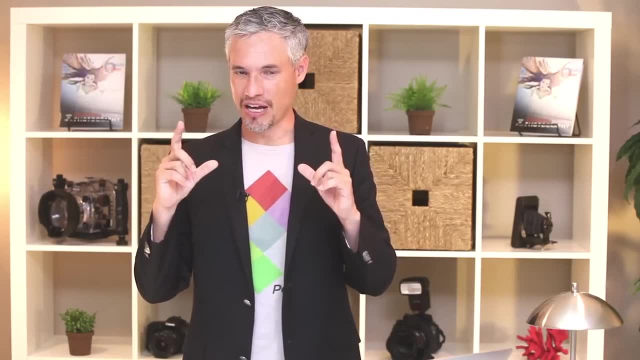 by kind of assessing how much experience you have. Are you a brand new photographer or have you been at it for years? How much planning did you put into that picture, Whether you just picked up your camera and took a snapshot, or did you actually plan the location? 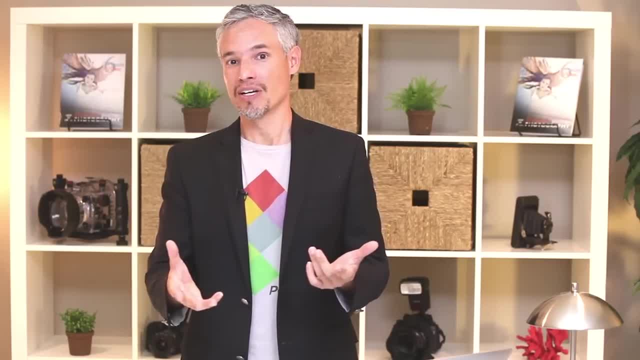 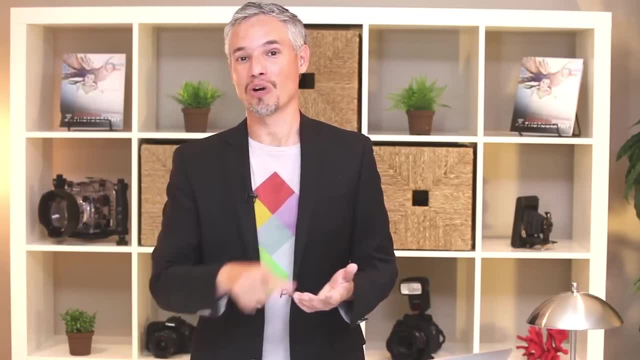 and the lighting and the pose And, finally, your camera gear. You can get great pictures with an iPhone, but you'll definitely get better pictures with better camera gear. Once again, I don't want you to rush into buying better cameras because you don't want to lose your camera gear. 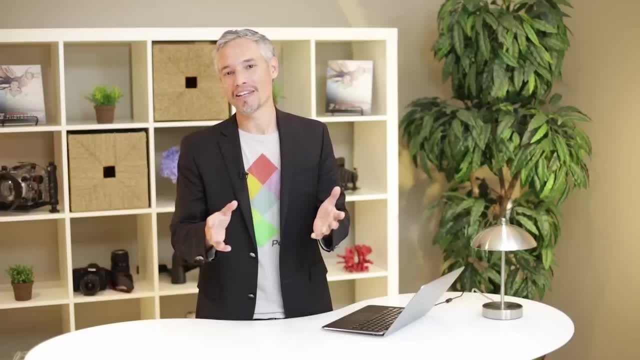 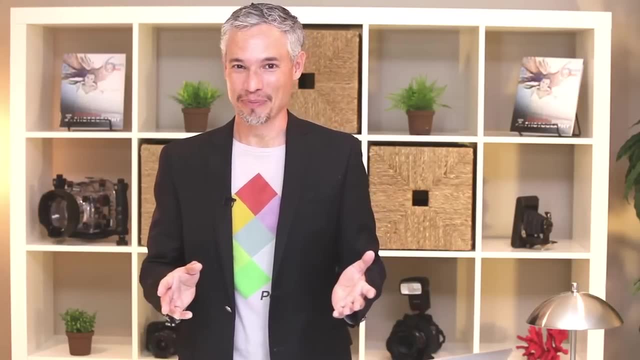 Put most of your energy into the experience and planning side first, And then, when you find that your camera gear isn't keeping up with your experience and planning, that's the time to upgrade. And here's some advice a lot of you are not going to like to hear. 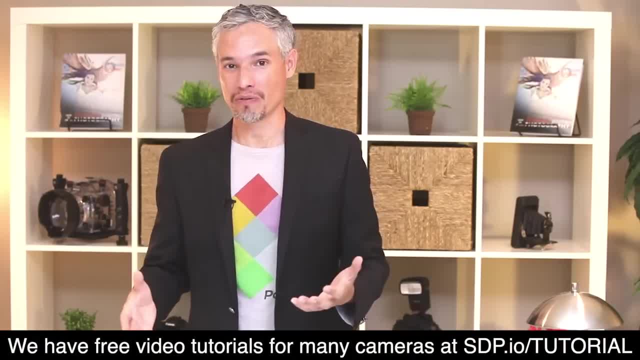 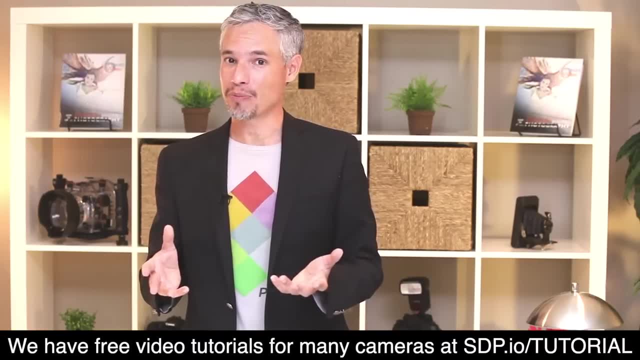 but read your camera's manual. I will teach you general photography techniques, but every camera out there has slightly different controls and menus, and they pretty much all have the same capabilities, but the buttons for them are in different places, so there's no way that I can tell you how to use. 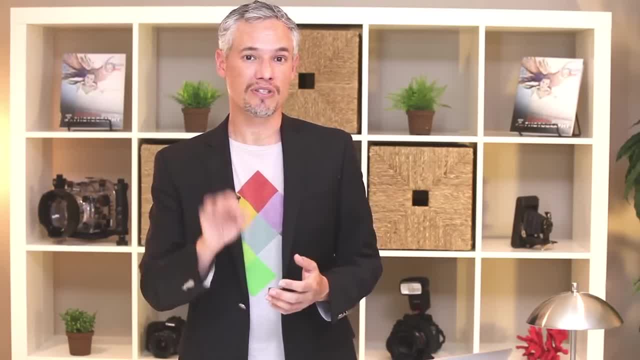 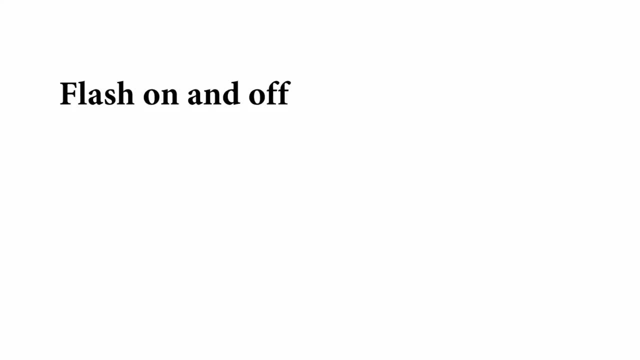 your specific camera. Here are some things that you should specifically look for in your manual. I don't want you to necessarily read the whole thing, but please do figure out these before you get too much further. You should learn how to turn the flash on and off. 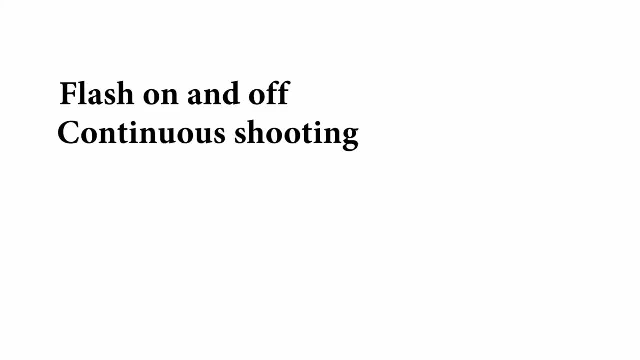 You should learn how to select continuous shooting. You should be able to set your camera's timer to take a delayed shot of a couple of seconds. You should know how to select both aperture priority and shutter priority mode, as well as to change the active shutter or aperture setting. 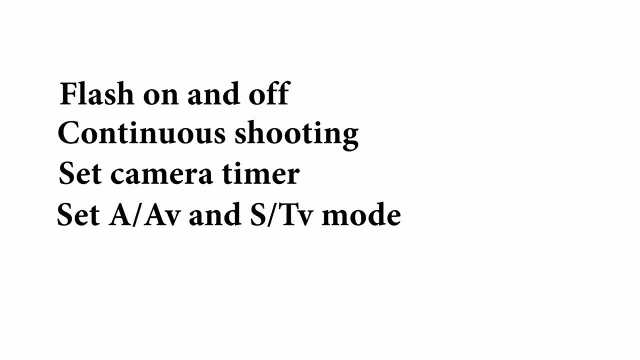 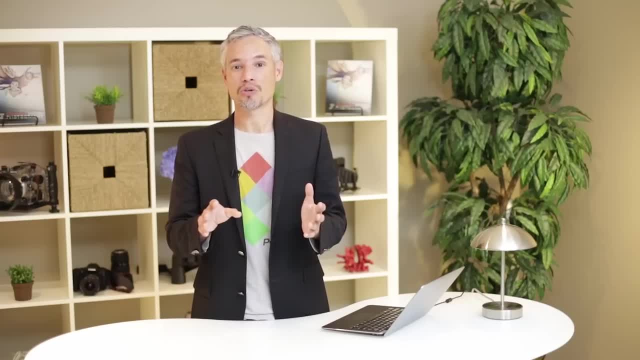 Usually that's just on a main dial that's underneath your index finger, next to the shutter, And finally, you should be able to view the histogram That'll allow you to check whether your pictures are underexposed or overexposed. Now I'd like to show you a video that I originally created. 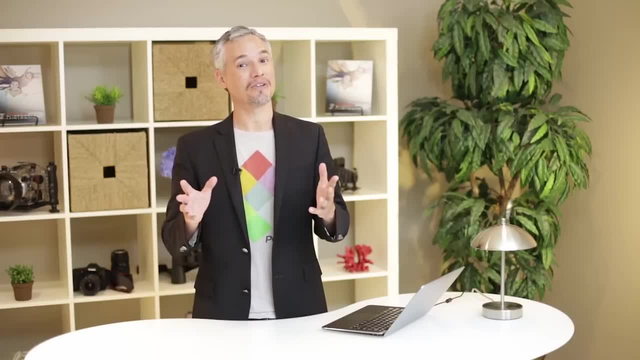 for my book Stunning Digital Photography. You'll notice that I created this earlier, before No Shame. November came along, so I'm not going to have the goatee in here. So let's head into my living room and hook up with my dog Cowboy. 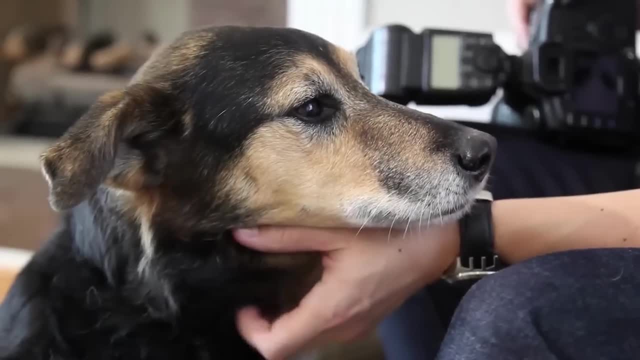 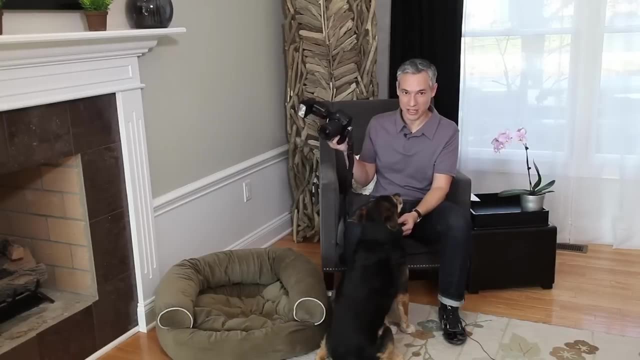 to share a few more tips. The first tip that I have is that I don't carry a camera bag. I don't carry a camera bag around, nor do I use a lens cap. You see, all I have is a camera strap. 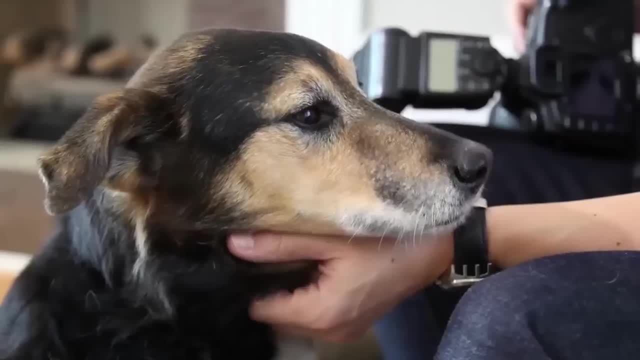 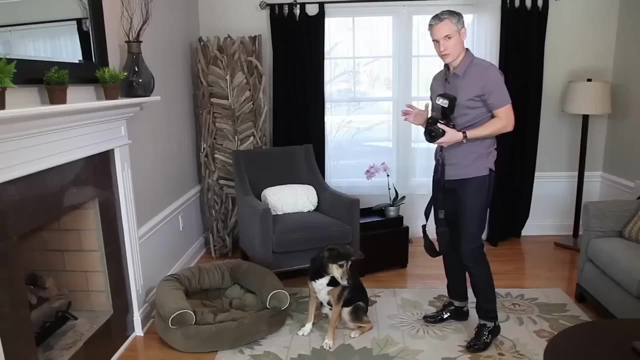 When you carry all that extra gear, it just slows you down. Every time you go to take a picture, you'll have to spend a few seconds digging your camera out, maybe digging through all those different lenses. So here's tip number two. 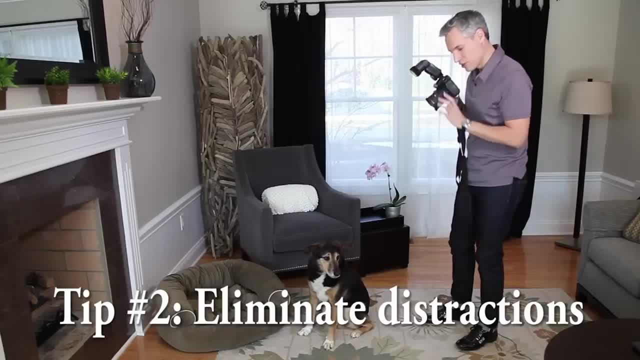 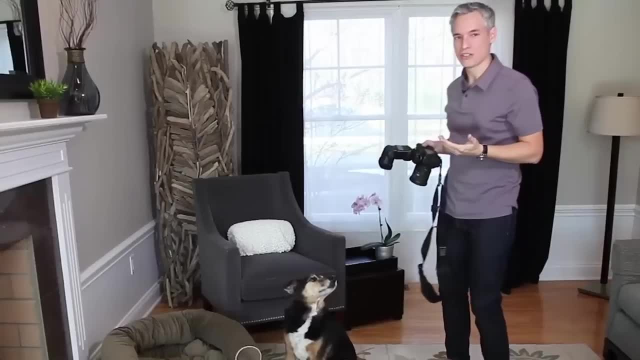 and it's to eliminate distractions. So this is how most people would take a picture. They would just stand at eye level and take a nice wide angle shot. Nice smile, Cowboy. What happens there is: you don't really know what the subject of the picture is. 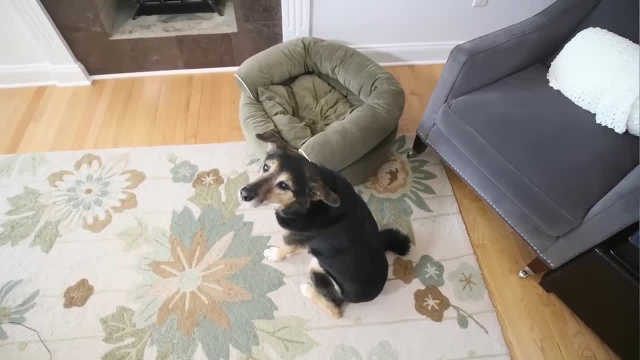 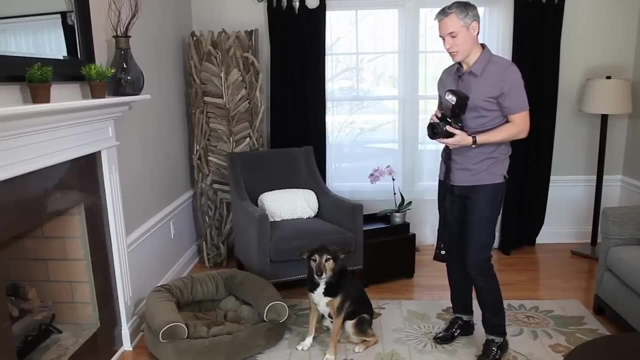 It looks fine when you're seeing it with your eye, but when you look at the actual photo, you see a lot of things in the picture besides the subject. To eliminate distractions, the easiest thing to do is to get closer and to zoom in. 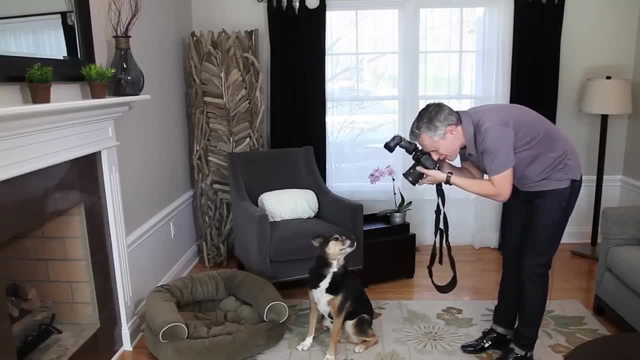 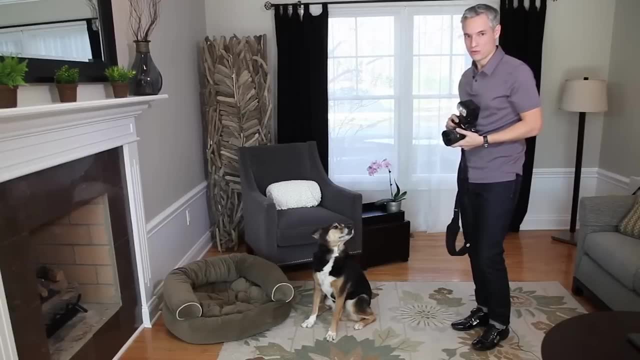 So I'll do that now. Cowboy, look up here, Good boy. Getting closer also reduces the depth of field. It blurs the background a little bit, which I cover in depth in chapter four. The next thing to do, tip number three: 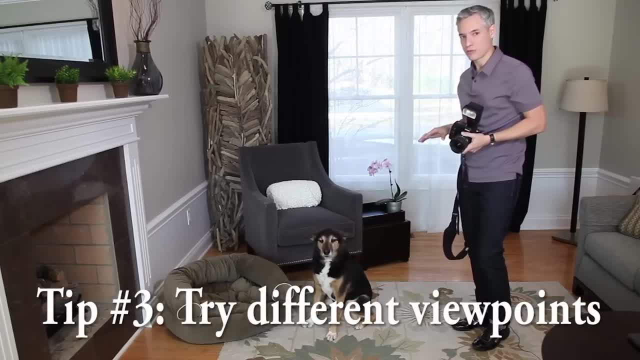 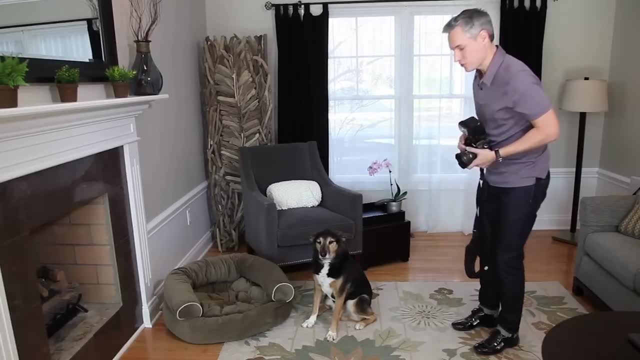 is to try different viewpoints. So I just shot Cowboy from eye level and it's not that flattering For smaller subjects like dogs. you really want to crouch down and get to the eye level. Same thing applies for kids. Good boy Cowboy. 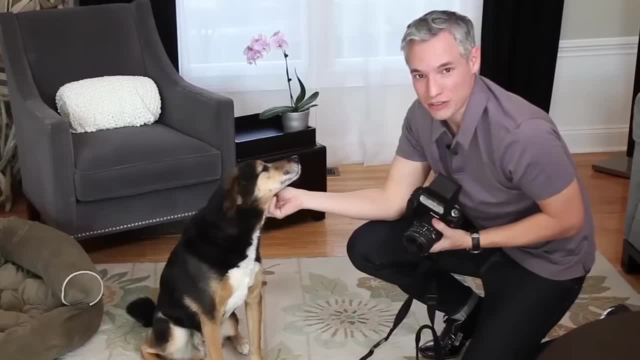 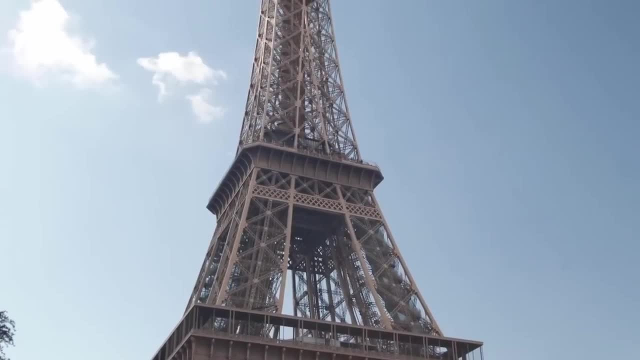 If you're taking pictures of something like the Eiffel Tower, you can move to many different sides of it, get high and get low, get close, zoom in, zoom out. That leads me to tip number four, which is: take lots of pictures. 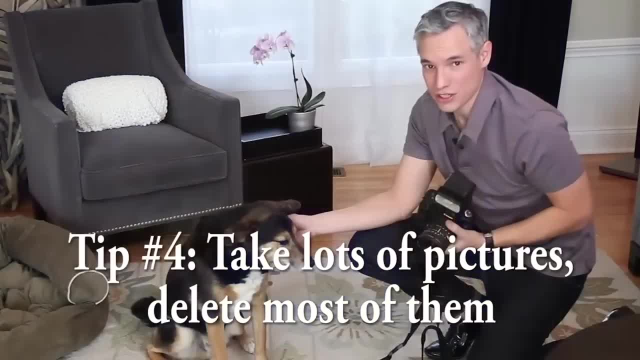 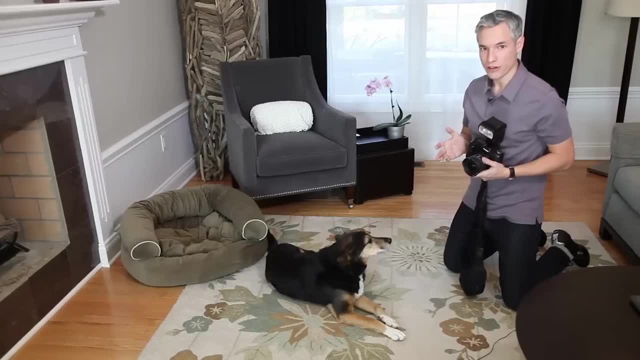 but delete most of them. Don't take too many pictures with digital. It doesn't cost you a thing, But please don't put 150 pictures of the same thing on Facebook. Just pick one. For tip number five, I'd like to talk about flash. 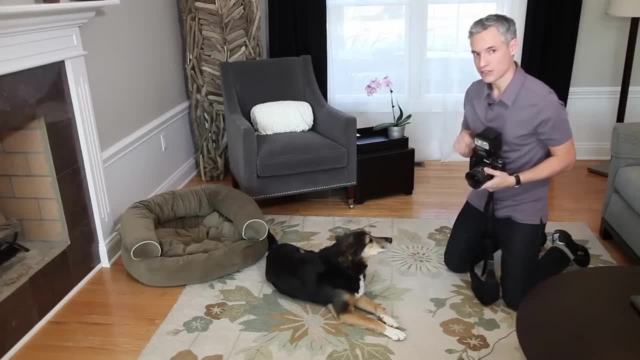 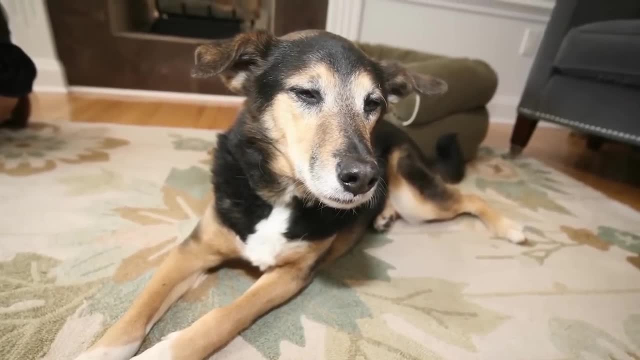 Now, by default, your camera just points the flash directly at your subject, which provides a very flat lighting. I'll take a sample shot now. A better way to do it is to use bounce flash. Many cameras allow you to attach an external flash to the hot shoe. 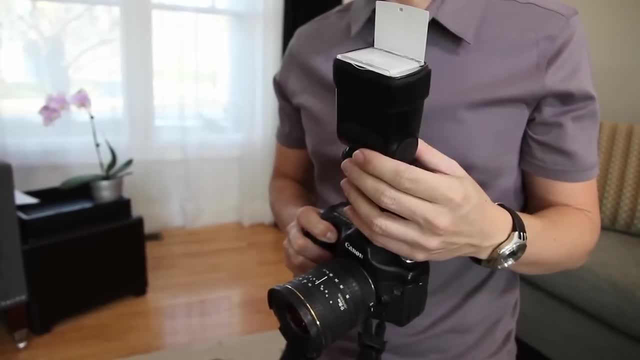 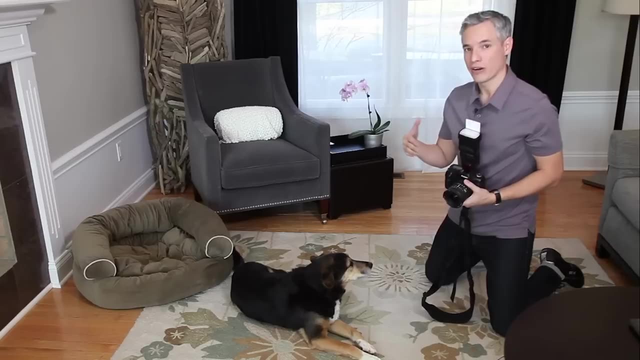 With a bounce flash. you can angle the flash up. Many bounce flashes even have the ability to spread the light a little bit more evenly. Now, as I take a second picture of Cowboy, you'll notice that the lighting is very different. The background has more even shadows. 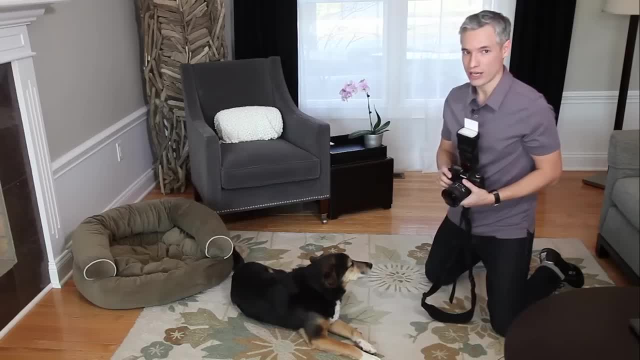 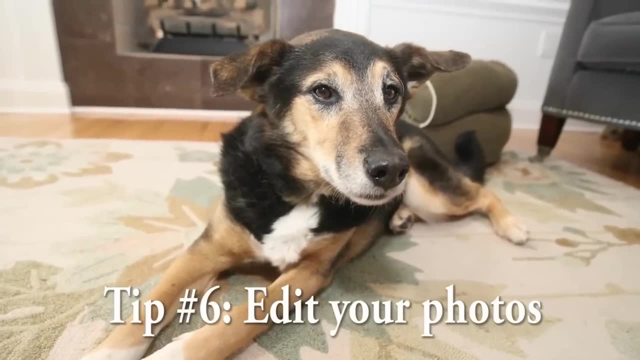 The lighting overall looks more natural, And if he had red eye in the first picture, he wouldn't have red eye in this picture. For my last tip, I want to suggest that you edit your photos. All you need to do is to download. 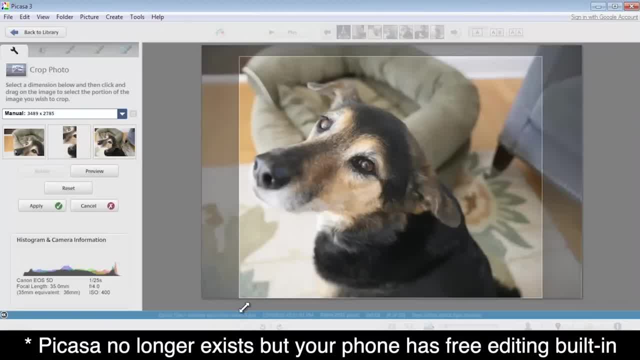 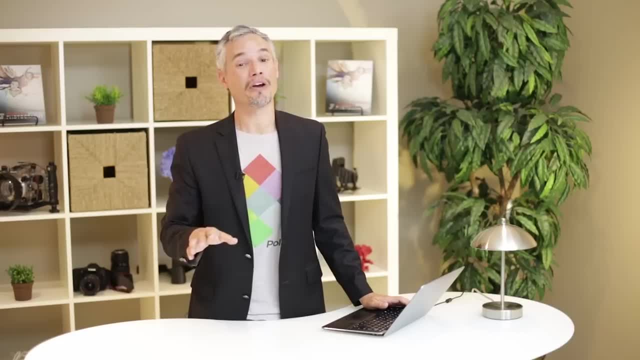 a free application like Picasa and just give it a little crop, maybe adjust the colors and the white balance, and you can edit those settings automatically. I hope those quick tips helped. From here on out we're going to get a lot more intense, so hang in there. 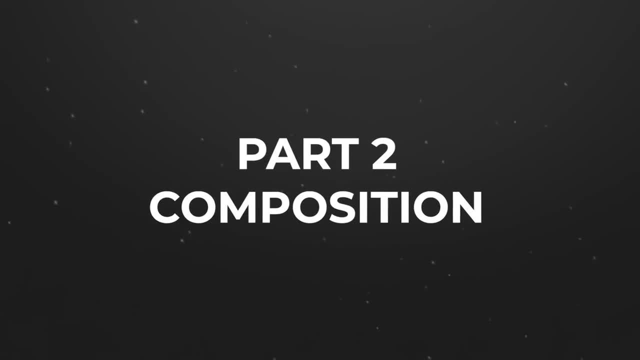 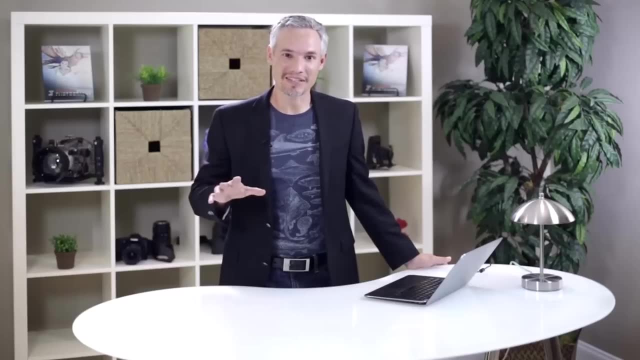 and I hope to see you in the future videos. Thanks Hi, I'm Tony Northrup and in this video lesson we're going to learn about photographic composition. This is the art of placing the subject in the scene compositionally to make for an appealing picture. 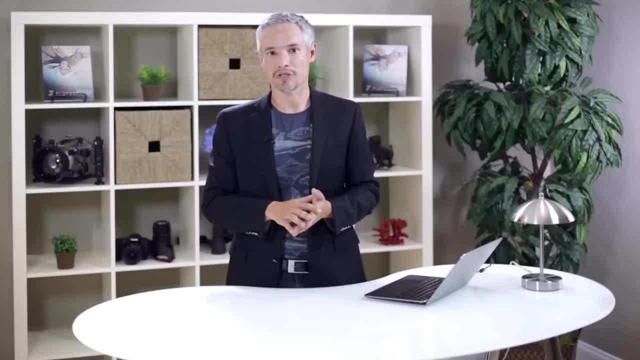 and to communicate whatever it is that you want to convey with your picture. This is a non-technical topic, so you don't have to worry about f-stops or shutter speed or anything like that, and composition applies for just about any type of camera you have. 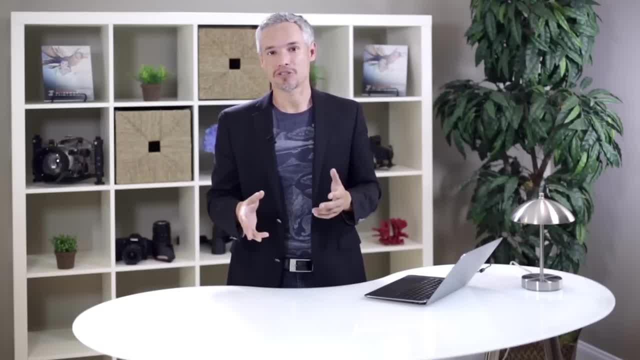 whether it's an iPhone or an expensive DSLR. In fact, most of these compositional techniques have their roots in art and painting, So you don't need high tech to understand all this, but it is really important And, in fact, the photographers 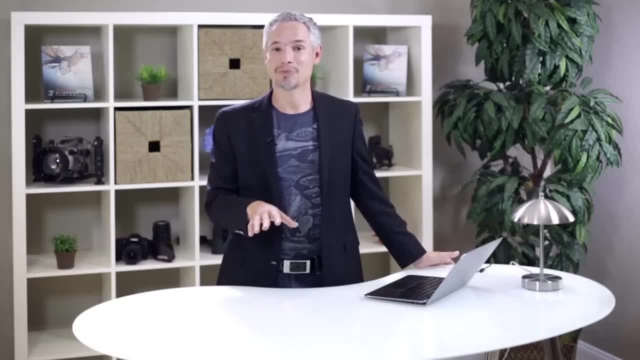 that I know, who decide to focus on the more technical aspects and skip the study of composition end up taking sharp but not artistically pleasing pictures. So this is an important topic for everybody. My first tip is to have a focal point in all of your pictures. 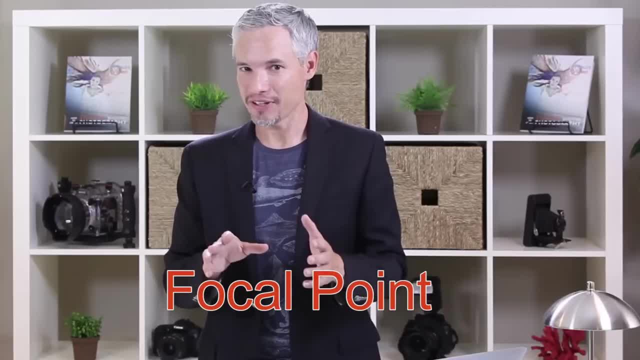 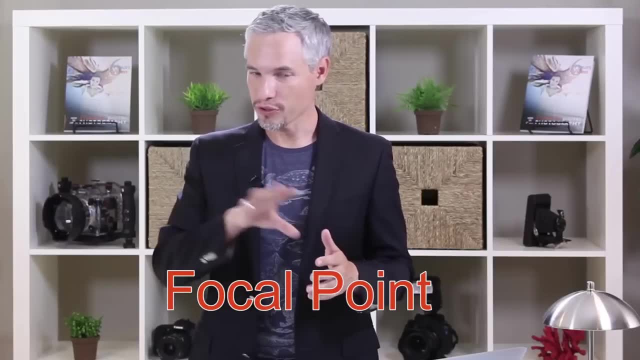 Whenever you're taking a picture of a scene, ask yourself very specifically what it is that you're taking a picture of. If you take a look at a picture and you find that your eye just kind of wanders over the view, well, that picture doesn't have a focal point. 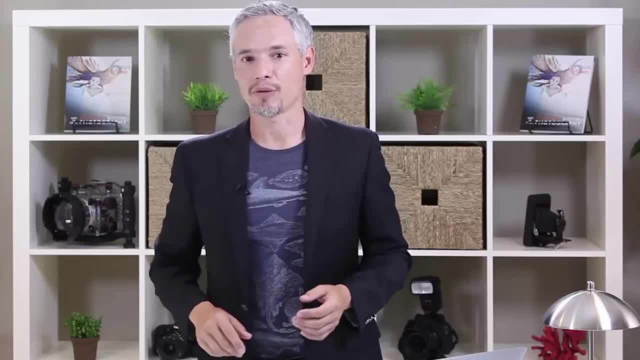 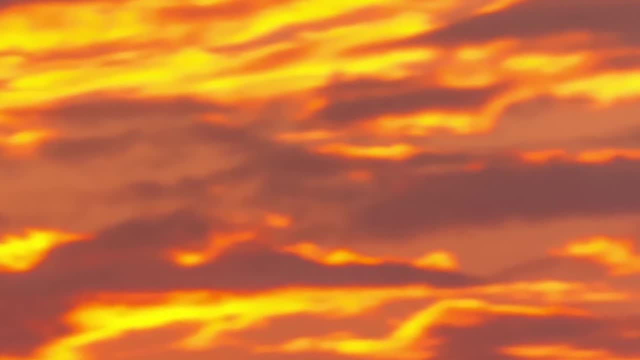 and that's one of the biggest problems that I see with people's photography. So let's take a look at a couple sample pictures. This is a lovely picture of a sunset, but where does your eye rest when it looks at it? There's nothing in particular to focus on. 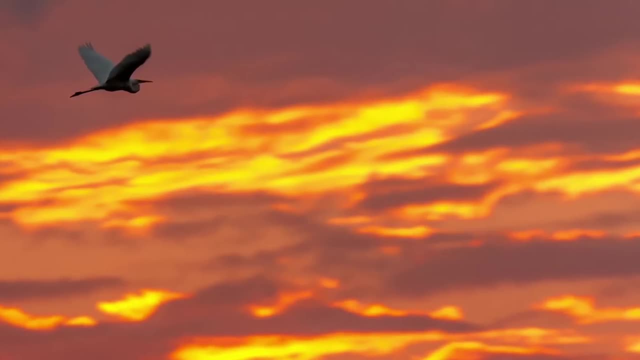 I waited until this egret flew through and put it in the upper left corner, and now, suddenly, you have a focal point and your eye goes right to it. Now, the sunset, the scene still counts and it still makes the picture more beautiful, But that egret makes all the difference. 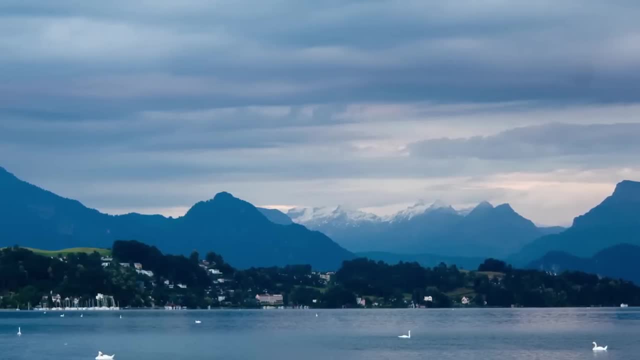 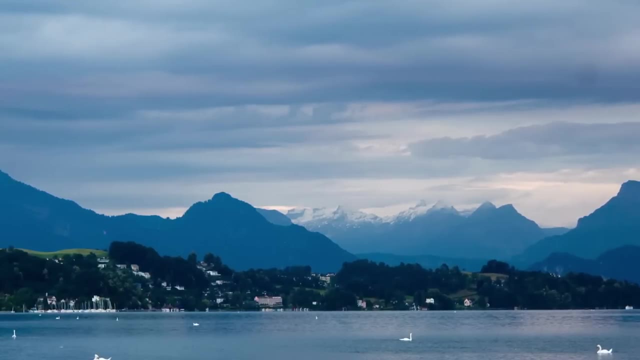 This picture of Lake Lucerne in Lucerne, Switzerland, is nice. The scene is gorgeous with the alps in the background and the swans in the foreground, but again your eye just kind of wanders over it and doesn't rest anywhere. in particular, 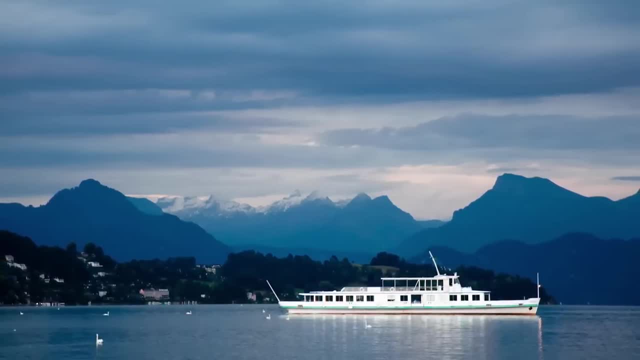 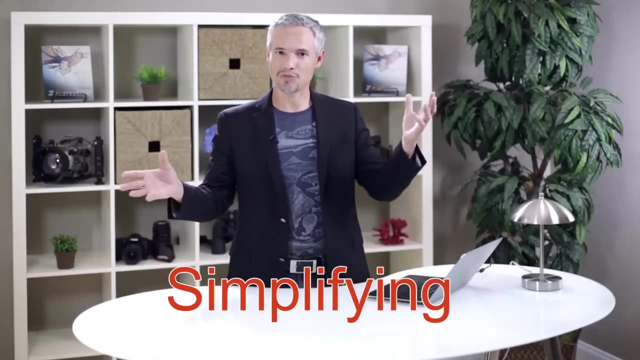 It needs a focal point. A few minutes later, this ferry went through and it made a perfect focal point and, as you can see, that's a much better picture. Now I'd like to talk about simplifying your photography. Often I find people take pictures. 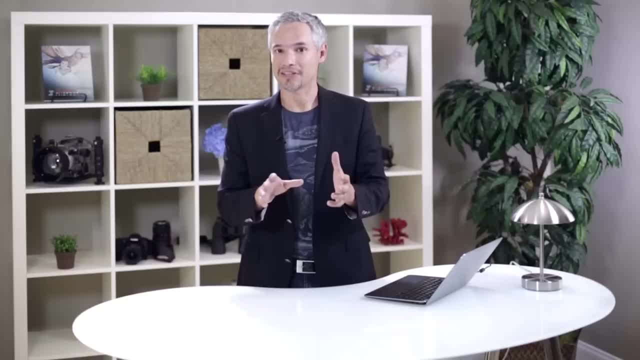 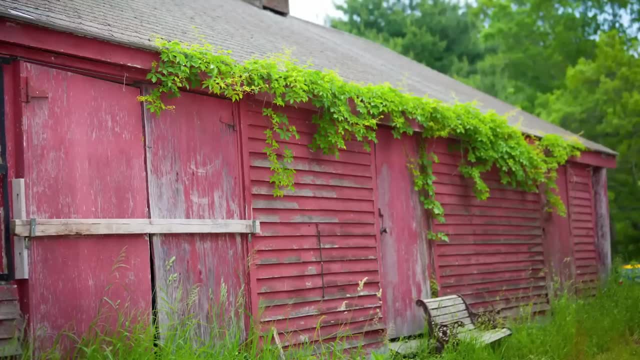 and it simply has too much in it. There can be a lot of distractions and the focus of the picture isn't clear. I might not know exactly what it is you're taking a picture of, So let's look at some examples. I was at this farm in Connecticut. 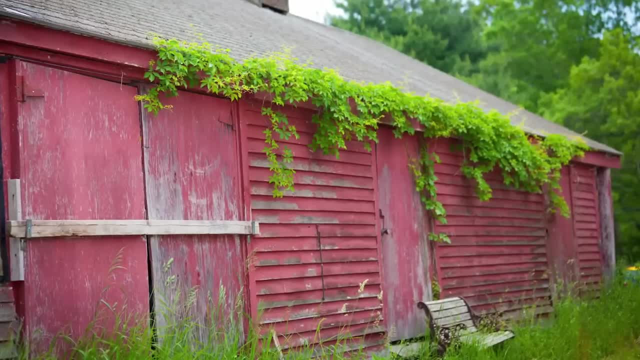 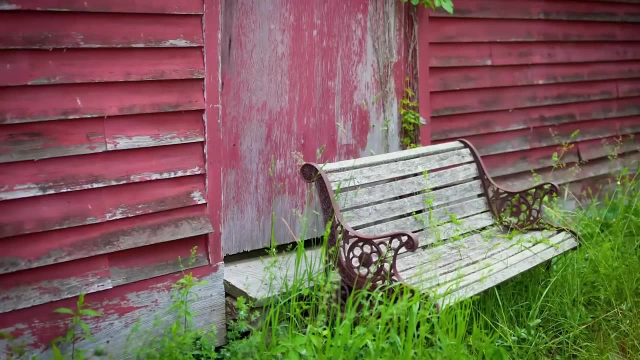 and I saw this rustic barn and this nice bench and the ivy growing over it, but, as you can see, I took a picture of it and it doesn't convey it. That's not a beautiful picture. I decided to close up on my favorite detail. 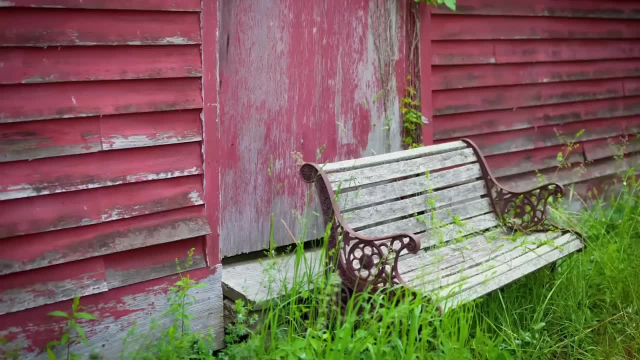 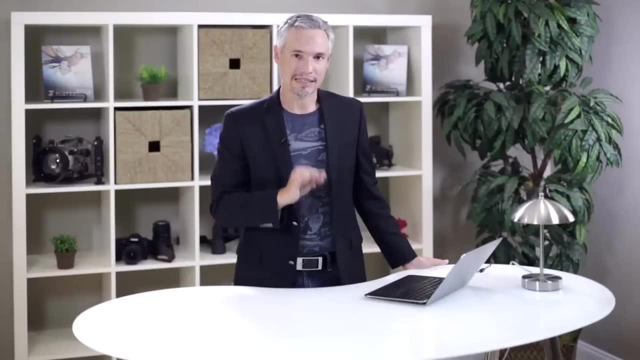 As you can see, I decided to pick this bench with the leaves growing through it and it still includes the rustic part of the barn and that's a much stronger picture because I simplified and I picked a single element to show in my photo. I think everybody recognizes the 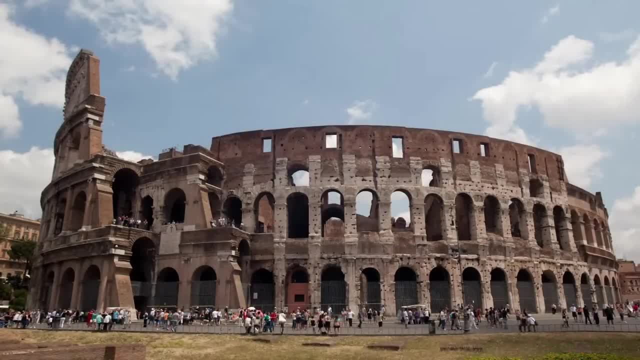 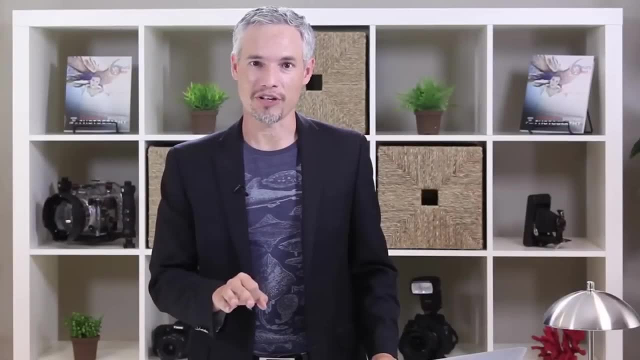 Colosseum in Rome, and it's an extremely important subject to photograph because there are so many tourists there and there are always fences and construction around. Well, what I decided to do was to pick a specific detail that I felt closely conveyed: the interesting part of the Colosseum. 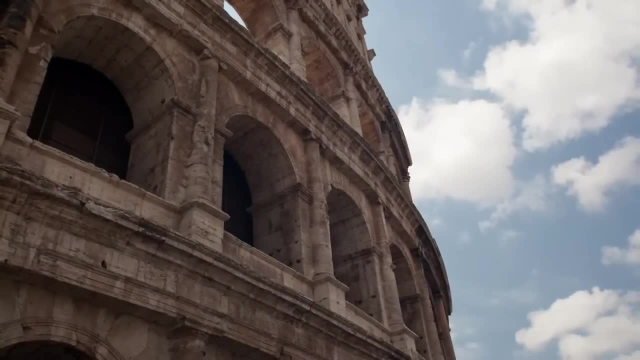 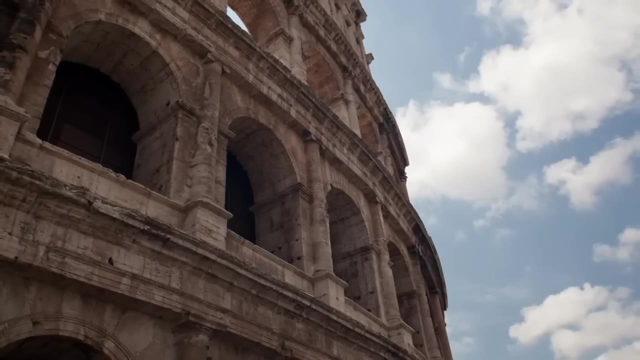 which is the architecture. In particular, the Romans were known for these arches, So I picked a telephoto lens and zoomed in tight and, as you can see, that conveys the Colosseum much better than the wider angle did. Now that doesn't mean you should take only the tight shot. 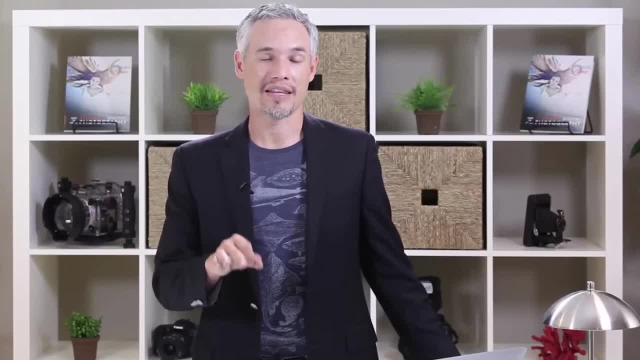 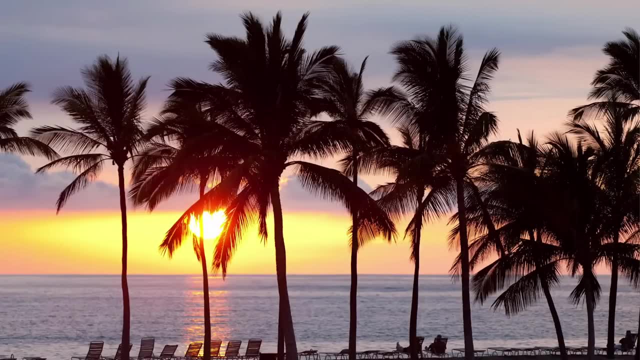 definitely take both, But I did include detail shots that simplify the composition and eliminate any distractions. This is a lovely sunset scene, but it could be even better if you simplified it. So look what happened when I zoomed in even tighter. There we go. 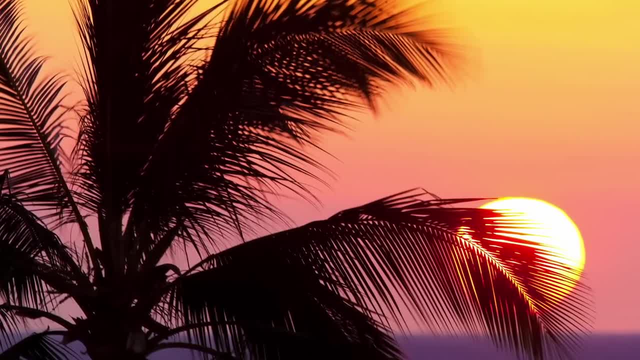 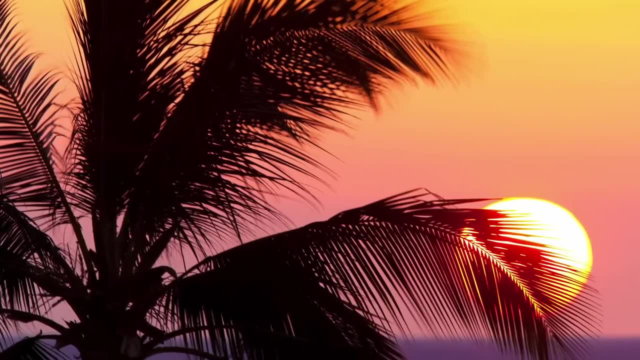 This shot is well suited for use on the web and it could make a great thumbnail because it reduces the previous picture to its bare elements: Palm trees, setting sun, horizon and colors. Here's a picture of a former Nazi headquarters in Berlin, Germany. 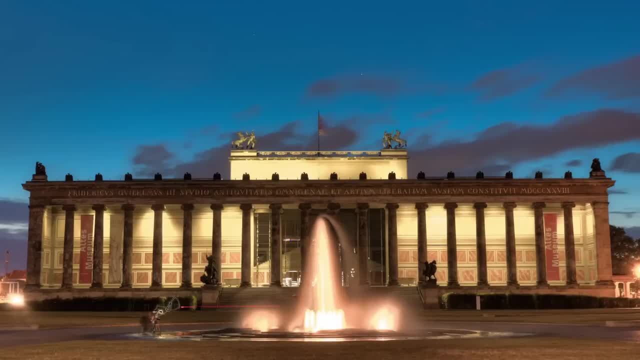 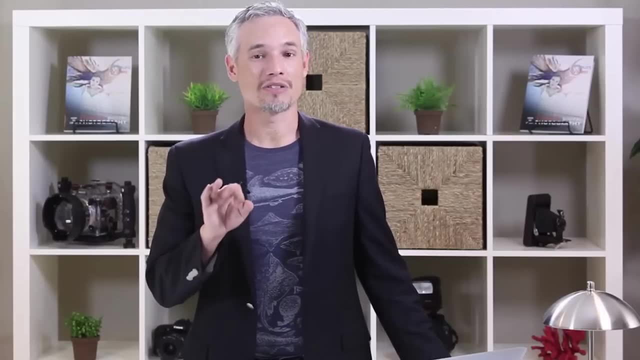 It's a lovely library now and it's an absolutely beautiful scene with this fountain. But there's a lot going on in this picture between the building and the fountain and the sky. Picking a specific detail can lead to a lot more interesting picture. 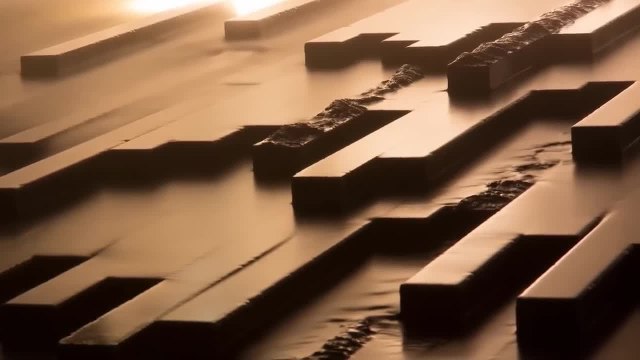 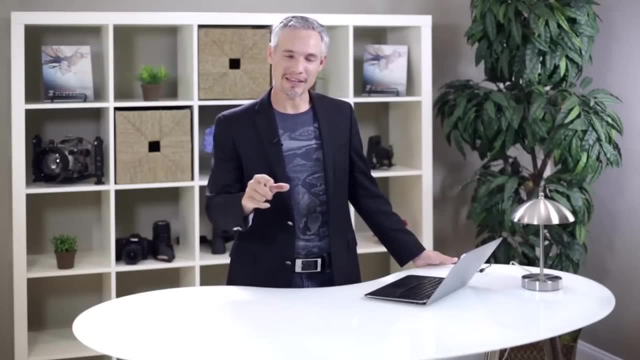 So I zoomed in on the fountain and made this very abstract picture because I thought that was the most beautiful part of the scene. So do take those wide angle detail shots, but also zoom in and pick the part of the scene that you think is the most interesting. 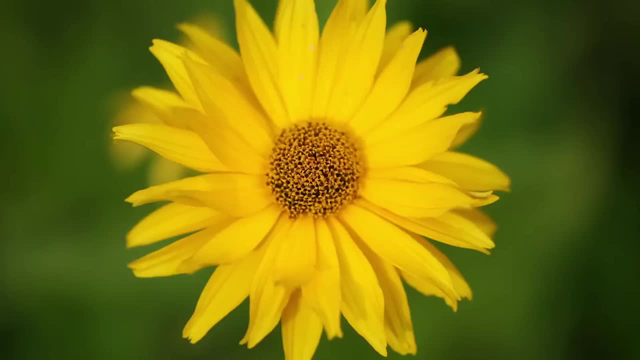 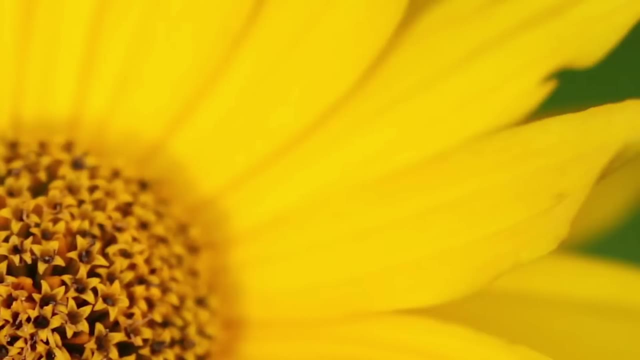 Here's a very ordinary picture of a flower, and you see, people take flower pictures all the time. They think their flowers are beautiful and in fact this one's fairly tight. A lot of people stand much farther back, But this can get much better if you really decide. 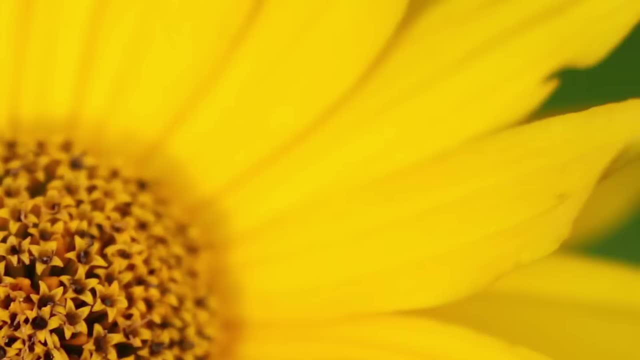 what the key elements of the flower are and you zoom in tight. So, looking at this tight crop, it still conveys everything that the flower is, but it shows it in a much more interesting way. You can see. the composition is more interesting. It also allows you to see more detail. 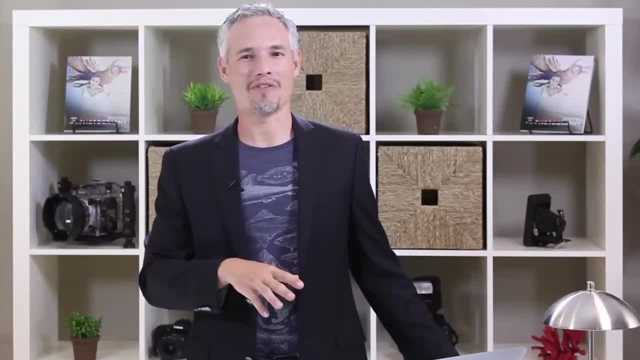 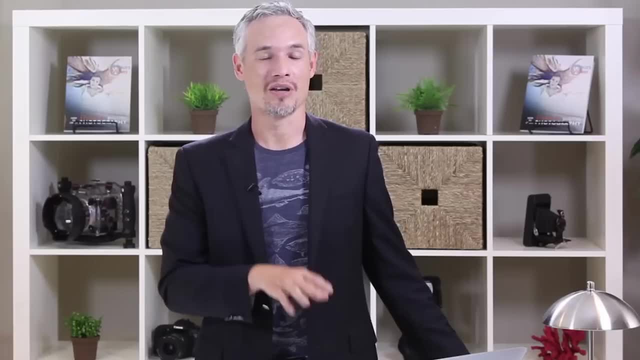 and your brain automatically fills in the rest of the flower. You don't imagine that the rest of the flower has been cut off or is on fire or anything. No, you know that the rest of the flower is circular from just this cross section, but it's a much stronger composition. 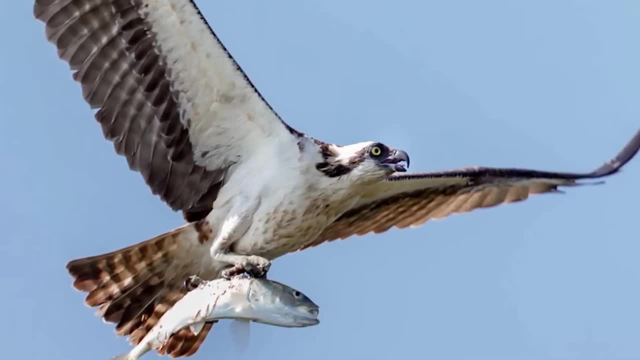 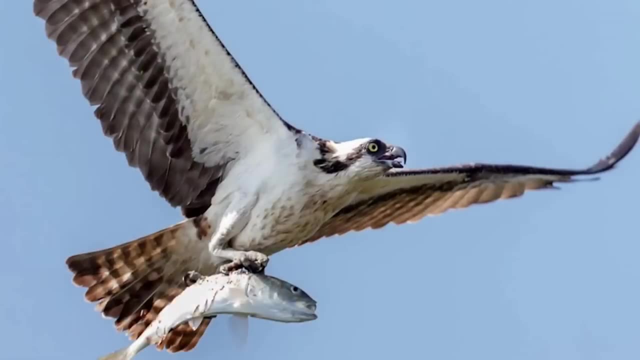 because it's simpler. I threw this picture of my favorite bird and osprey in because it's an interesting crop. A lot of people try really hard to avoid cutting off the edges of anything, but I went ahead and cropped right into the wing because the interesting part of the picture here 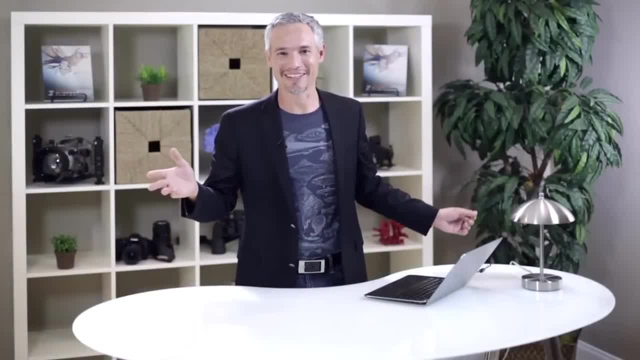 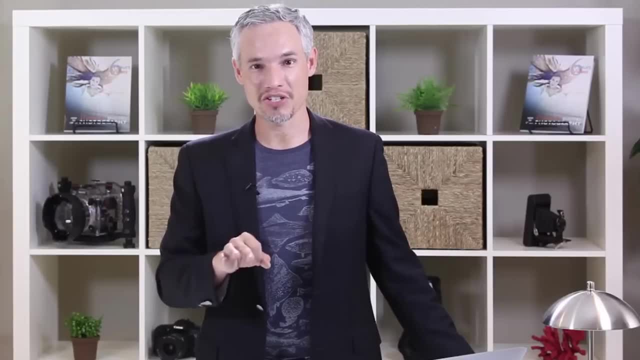 isn't the overall shape of the wing or the bird's wing tips. We know the bird has a wing tip, so it's okay to cut it off. You can also see the detail focusing the viewer's attention on the more interesting parts of the shot. 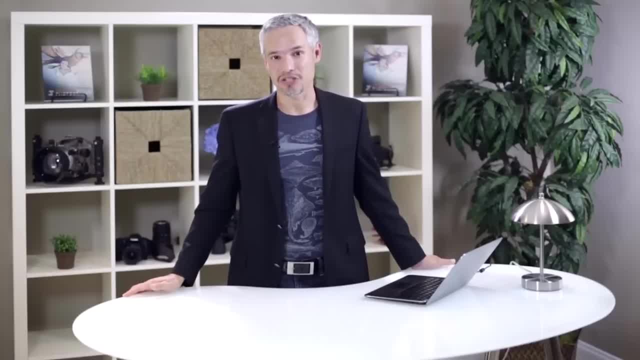 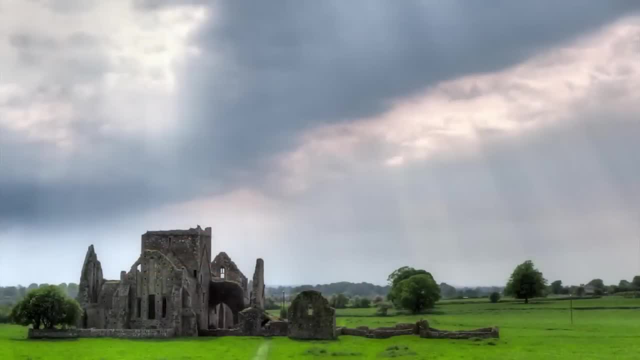 The eye of the osprey and the fish that it's holding. Now let's head into the Irish countryside and I'll show you some tips about taking pictures when you're traveling. This is a beautiful location that I'm at, and when you visit a place like this. 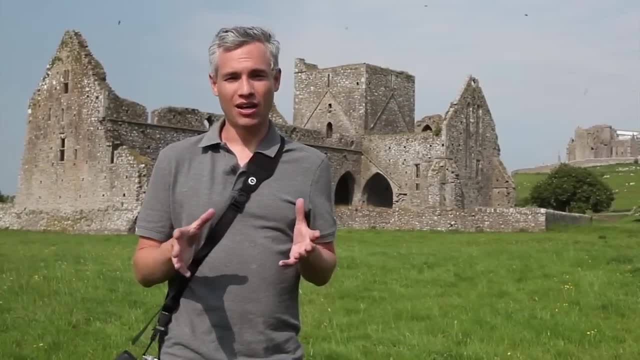 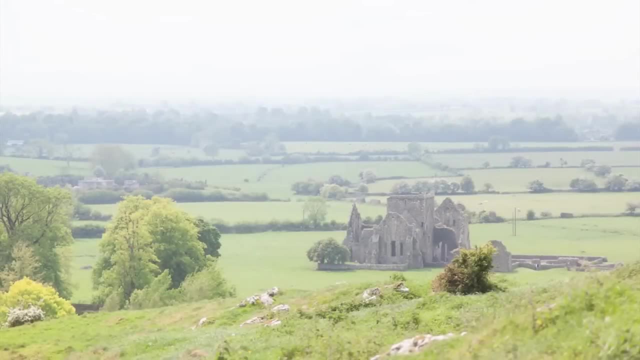 you want to be able to capture it so you can show what it was really like to your friends And, unfortunately, standing back and just taking a snapshot of what you see isn't going to convey it, But you can do it using a series of pictures. 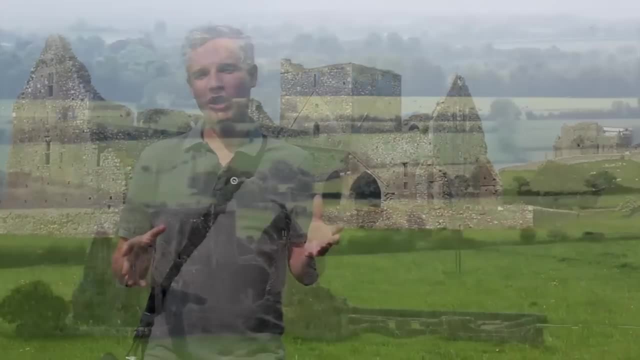 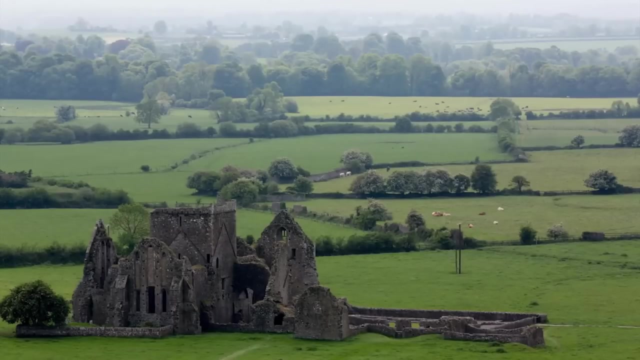 So let's first mix both wide angle and telephoto shots. Use your wide angle to capture the entire scene, So I'm going to show not just the ruins behind me, but also the hillsides and the sheep in the background With your telephoto lens. 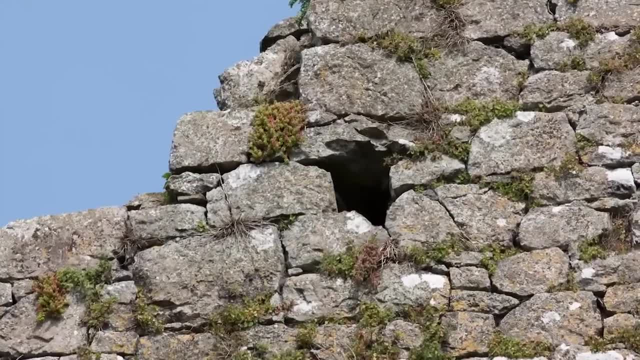 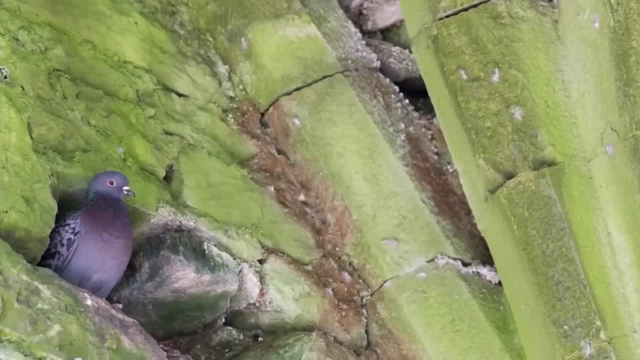 get in tight on the details and close up on the things that you find interesting about the place, Like the way the flowers and the grass are growing within the rocks, Or this bird that was hiding in a crevice of the bricks. These are the types of characteristics 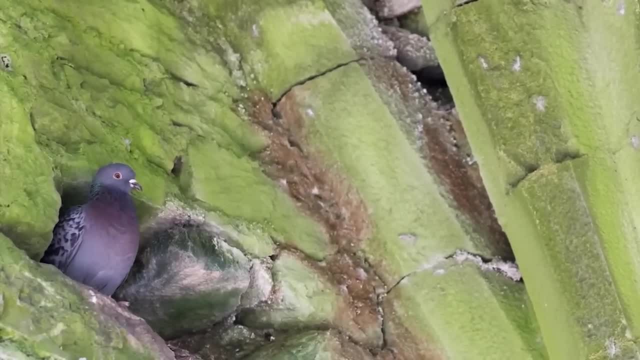 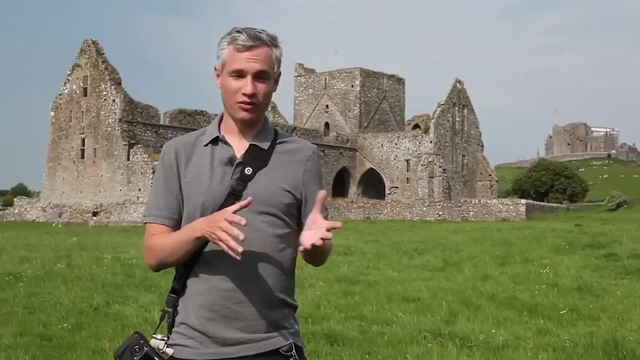 that your brain takes in and compiles into an overall picture of the place. If something is a particularly large scale, like the buildings behind me, you'll need to include something to show that scale. If you manage to get a picture without any people, that's great. 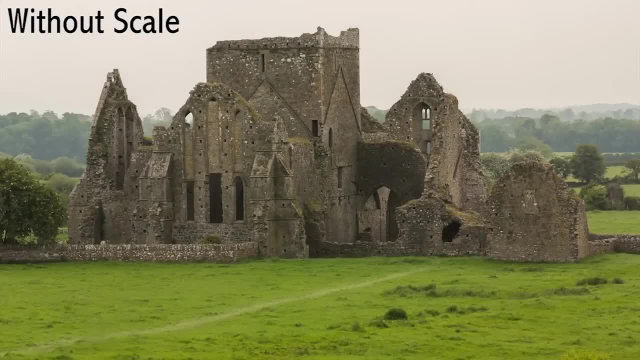 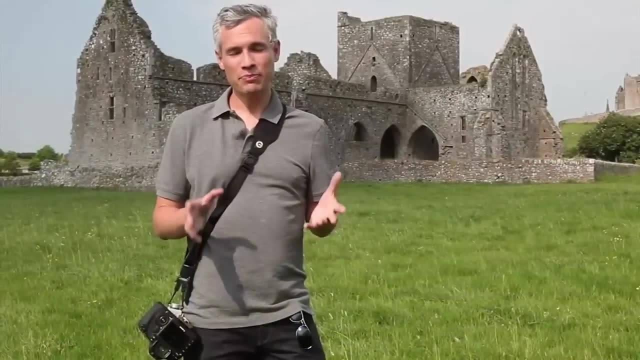 But people looking at the picture won't know how big it is. So take other shots that include people or sheep or anything of known size, so that you can show the scale of the structure. Now one last thing: Be patient about your lighting. When we showed up, we almost left. 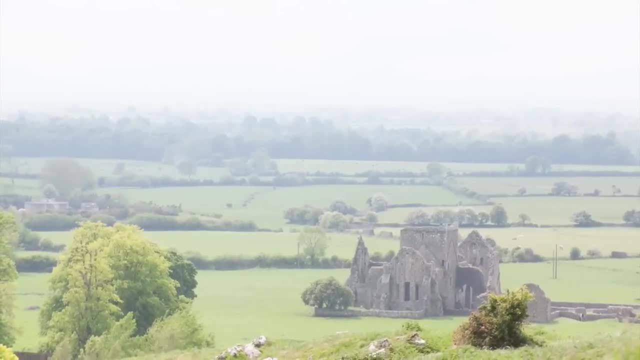 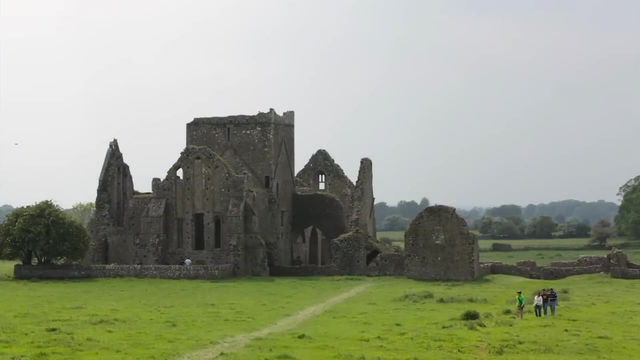 because the lighting was so bad. It was completely overcast and just dark And that kind of lighting doesn't show any depth. If you don't have any hard light, it doesn't form and they become almost a silhouette against the sky And they just look very flat. 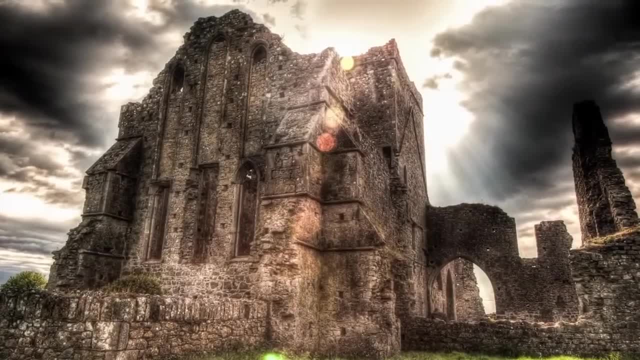 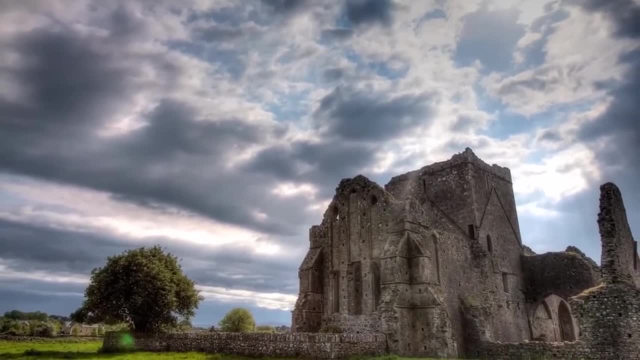 Now I happened to look at the sky and I saw that the sun was about to peak out. We waited around a little bit and we got the beautiful day that you see behind us, And we managed to get some great pictures out of it. Keep those things in mind. 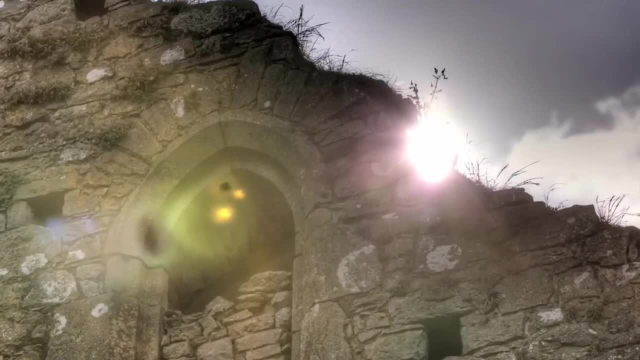 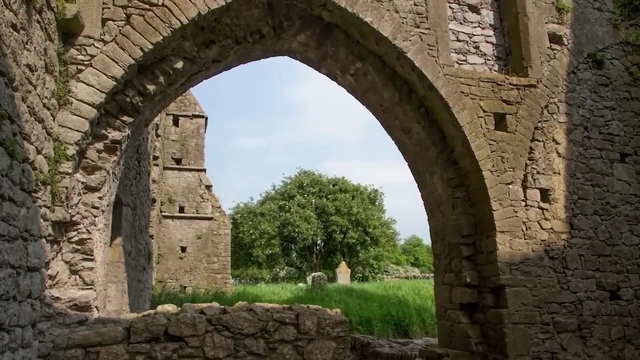 Shoot wide angle and telephoto both to show the surroundings and more important details. Take a few minutes and walk around the building to show different angles. Also, peer through windows and openings so that you can see the view from the building and give context to your pictures. 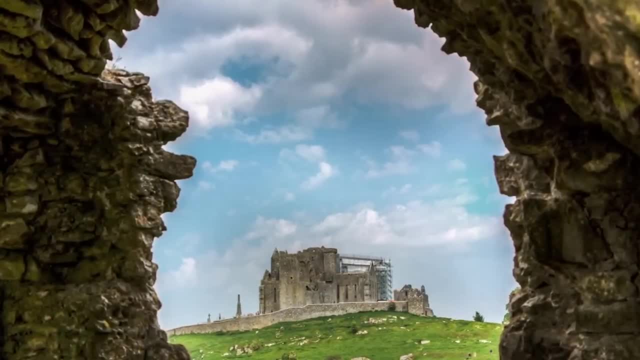 Finally, take a few minutes and wait for nice lighting, and most of the time it's going to pay off for you. And now I'd like to talk about the rule of thirds. This originated in the Renaissance, So this might not be the first place. 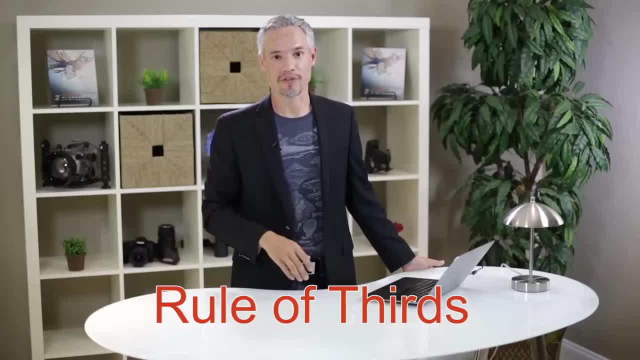 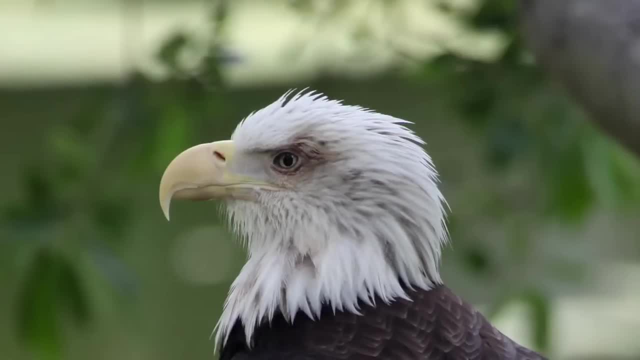 you're hearing about it, but it's one of the most important rules in photographic composition. Let's look at some sample pictures. Here's a picture of an eagle, but it might as well be a picture of a person, because this is the way a lot of people compose pictures. 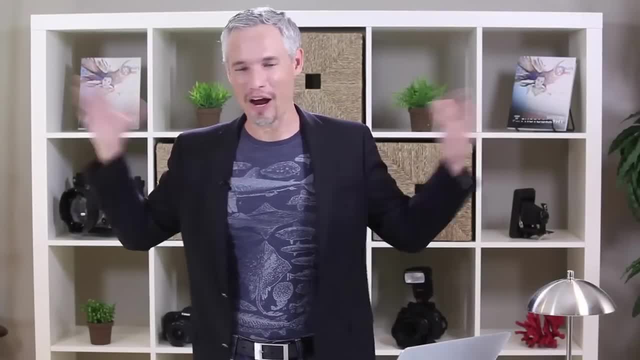 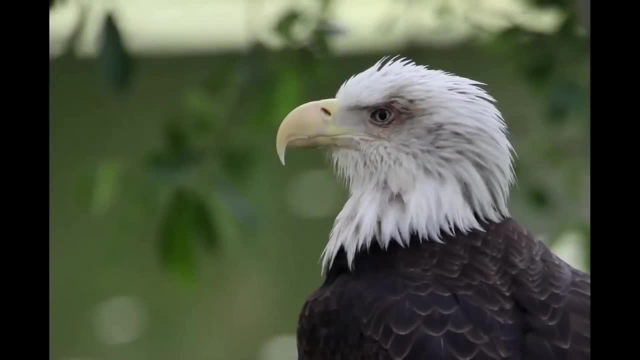 They just put the person's head right in the middle of the frame and then there's a bunch of distracting stuff everywhere. You can make this picture much better by using the rule of thirds, So I'm going to recompose this picture by putting the eagle's eye. 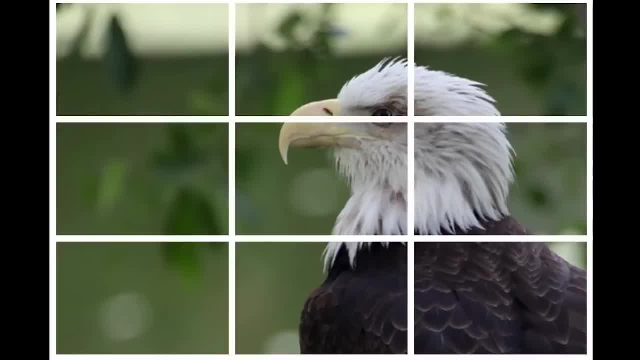 in the upper right third of the frame. Here. let me overlay it for you so you can see exactly where things land. You can see the eagle's body is vertically positioned along the right third of the frame and the eye is very close to that intersection. 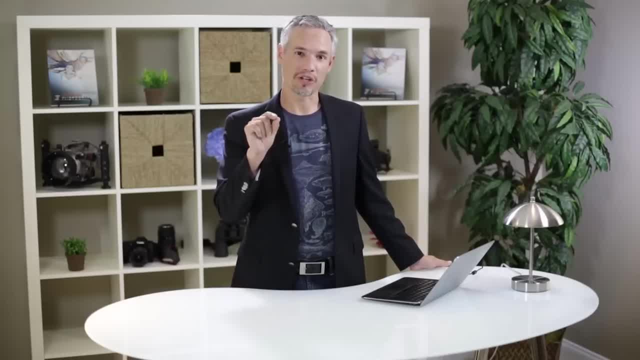 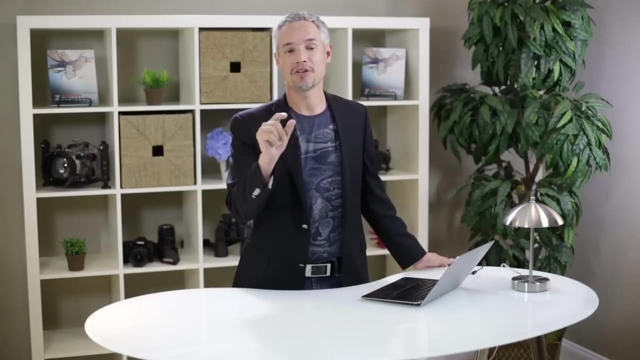 You want to use both those vertical lines and the rule of thirds grid and those points where they cross. Those are magical points. Put your subject on those points, because sometimes your subject isn't the entire person, but it will be the person's eye or the expression. 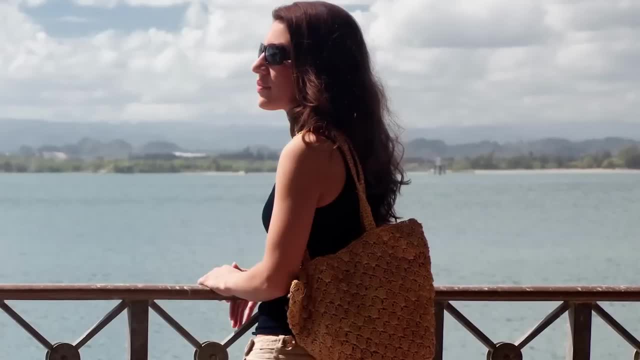 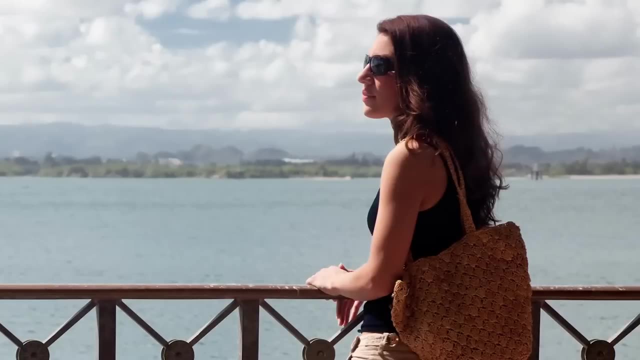 or whatever, the smallest part that still conveys your message is. Here's a picture of my wife, Chelsea, in Puerto Rico, and this is a very common composition. Again, she's just right, smack in the middle of the frame, Applying a little rule of thirds. 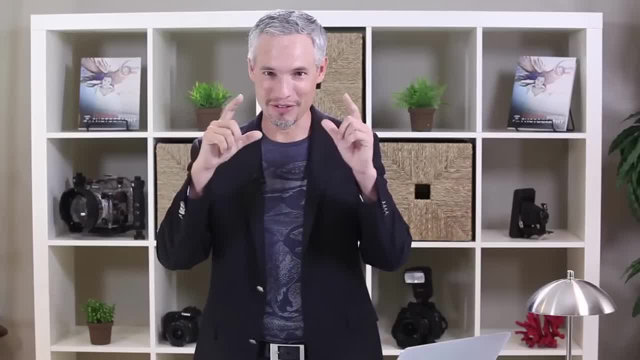 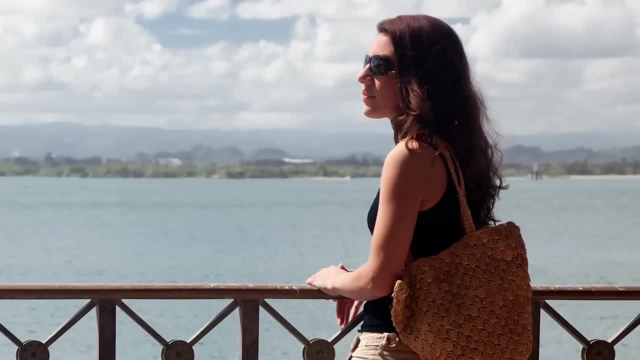 will make this snapshot much more interesting. See, I just moved the camera like that. I just moved the camera to the right a little bit and it got much better already. This image uses the rule of thirds in several different ways. She is positioned along the vertical third. 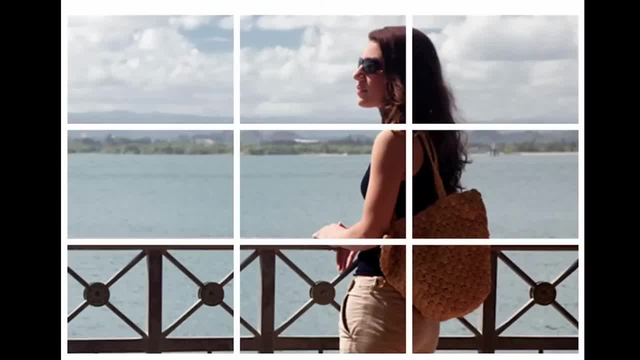 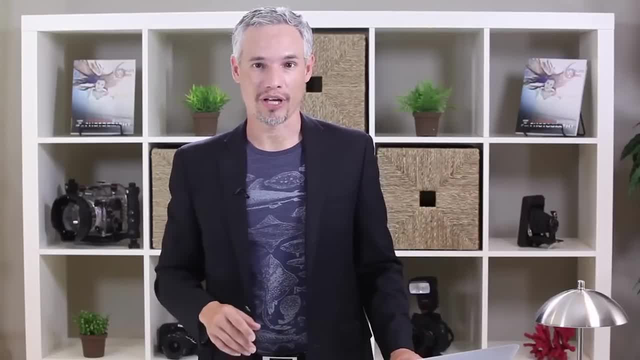 The fence that she's leaning against is along the lower third and the horizon is positioned along the right third, So it's a good example, And though it's a simple picture, not a stunning picture, it still is much improved by relying on the rule of thirds. 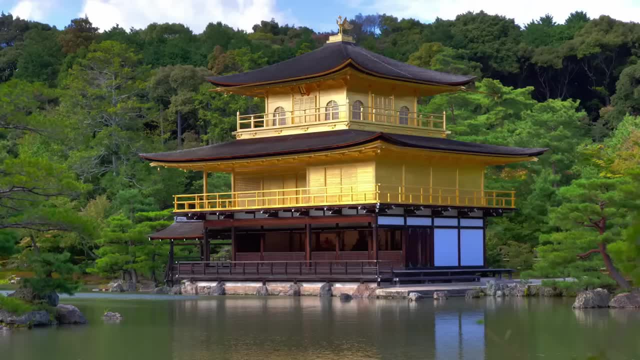 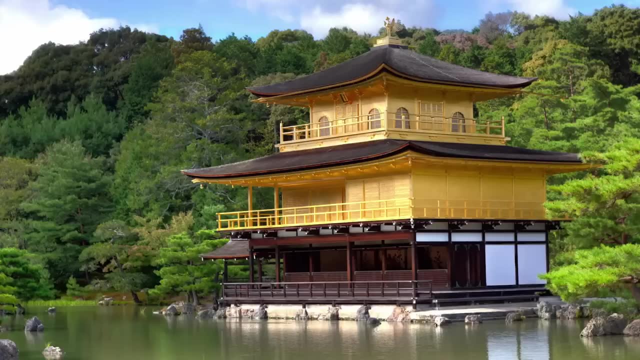 This is the Golden Temple in Japan and it is a beautiful, beautiful sight, but there are a lot of bad pictures taken of it because it's a popular tourist attraction. So if you do visit, be sure to use the rule of thirds Right away. I just shifted it. 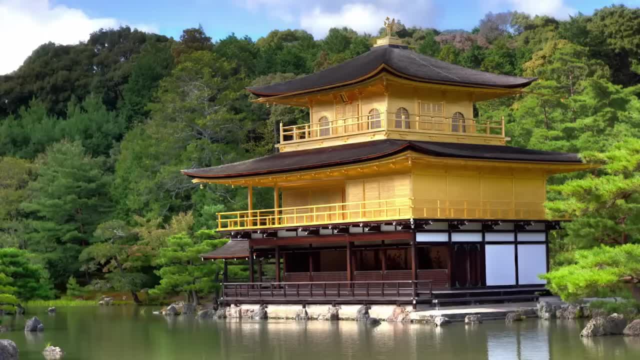 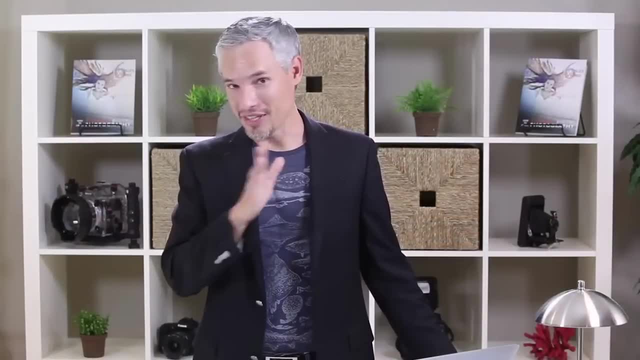 a little bit to the right, but it got much, much better because it's off center and we're just so used to seeing pictures completely centered that we just tune it out because it's just too common. Moving things a little off center can make all the difference in the world. 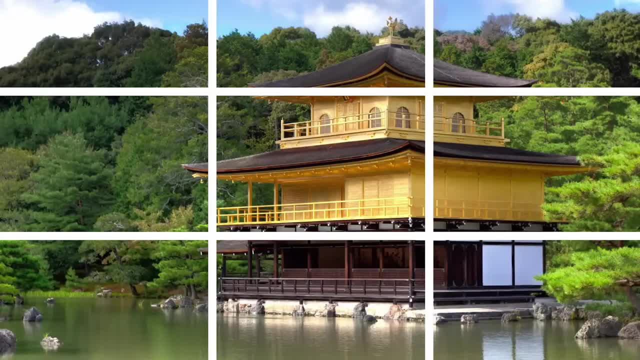 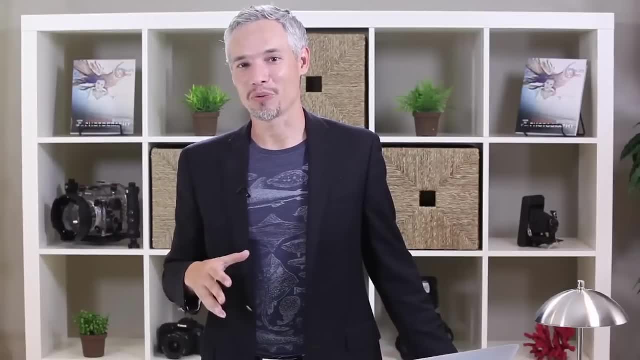 As you can see, with the rule of thirds it doesn't align perfectly necessarily, but you don't have to be too rigid with the rule of thirds. In fact, sometimes it's appealing to put things right against the edge. What I think the most important part of the rule of thirds is. 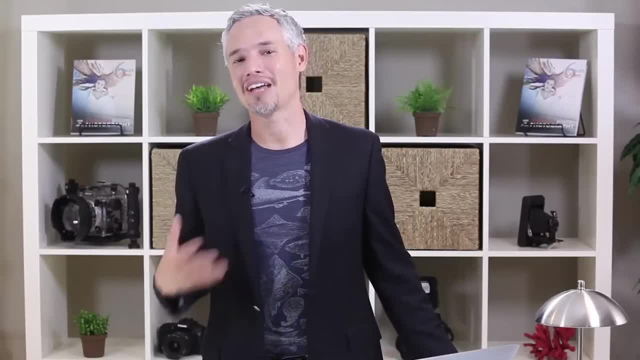 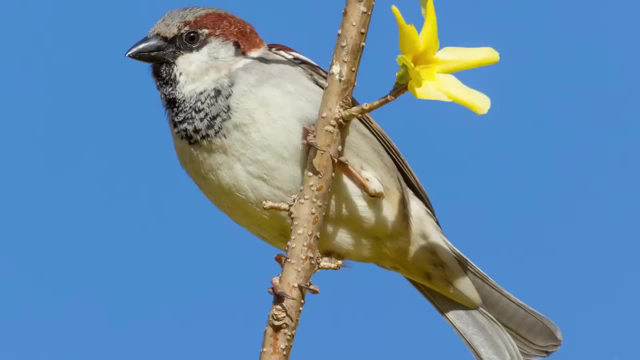 is just to avoid putting stuff off center in the image, because that's a lot of our natural tendency. That is, after all, how we see things with our eye, but it's not what we find appealing in pictures. Here's a picture of a sparrow on a tree branch. 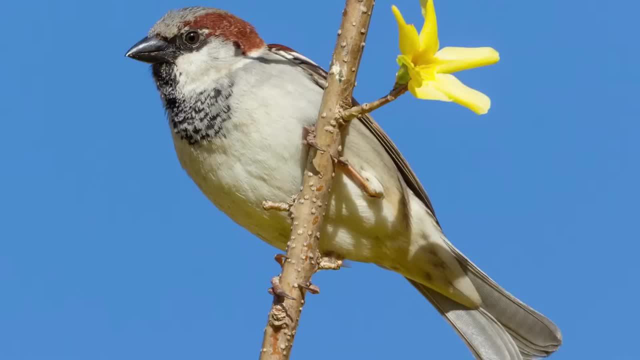 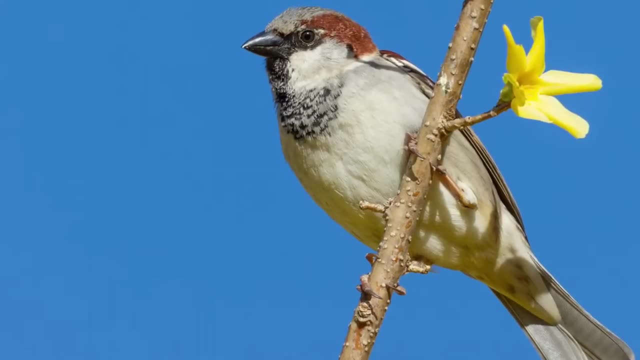 and it's a good picture compositionally because it's simplified. There are no distractions in it. If you move it over to the right third, I don't know that- it gets better. I don't necessarily rely on the rule of thirds when I'm taking wildlife photos. 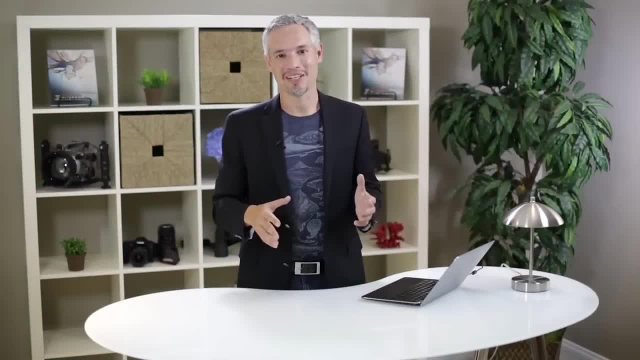 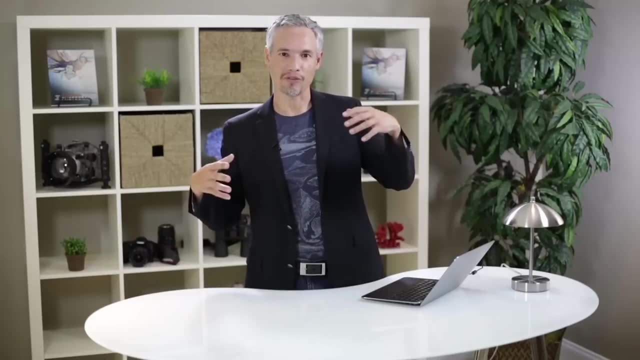 A lot of times with wildlife photos you simply want to fill the frame because the subject is just the animal. There's no detail in the animal. So sometimes you can just forget the rule of thirds and just try to use every part of the frame, leaving just a little border around the frame. 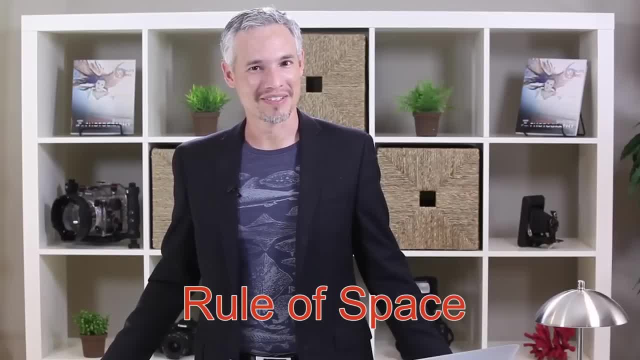 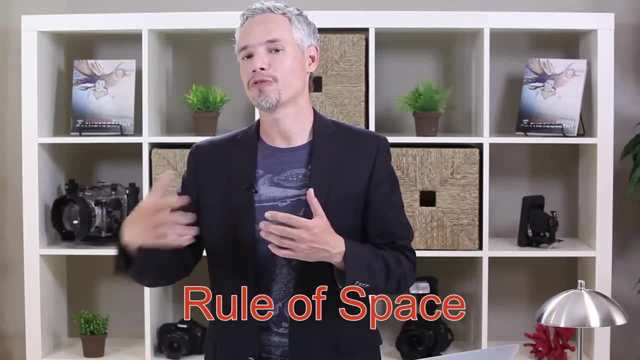 so the subject doesn't feel crowded. Now let's talk about the rule of space. If you have a subject, especially with eyes, but cars too, anything that faces in a particular direction, it's better to leave room in front of the subject rather than behind it. 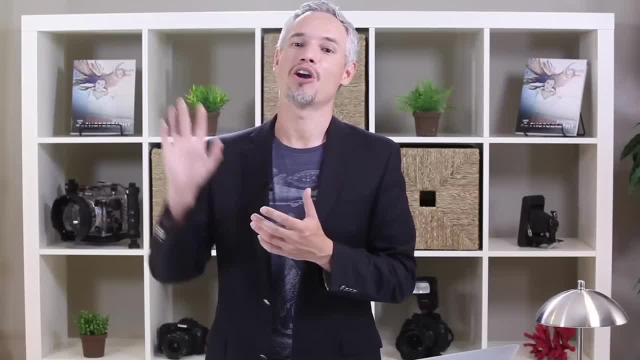 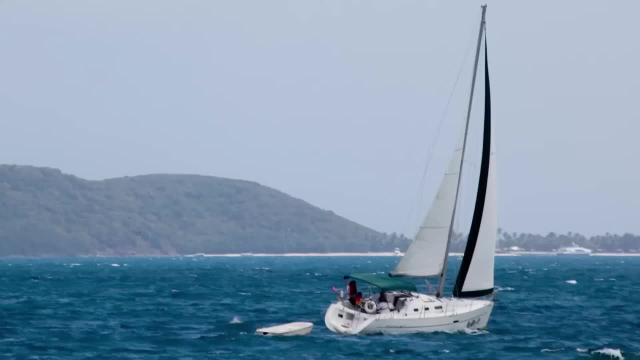 So you might want to use the rule of thirds but position the subject so that it's facing into the open part of the rule of thirds. This will become more clear with some examples. Here we can see a sailboat, and the shot is kind of uncomfortable. 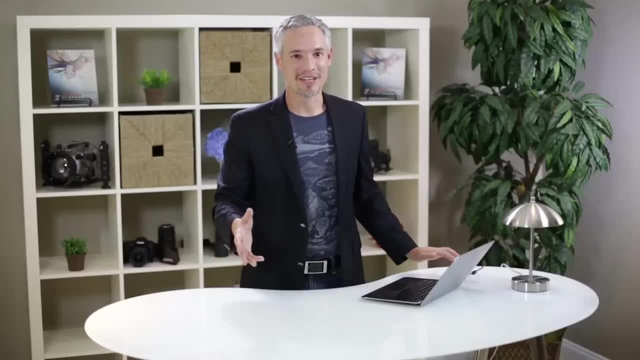 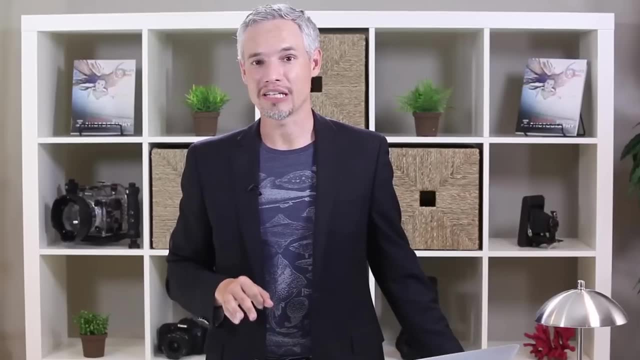 because the boat seems like it's about to soar right off the edge of the frame. Recomposing just a little bit makes this a much more conventional and comfortable composition. The point I'd like to make is that you should leave room for your subject to move into. 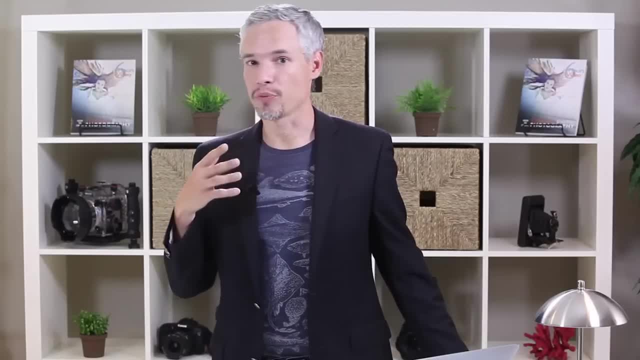 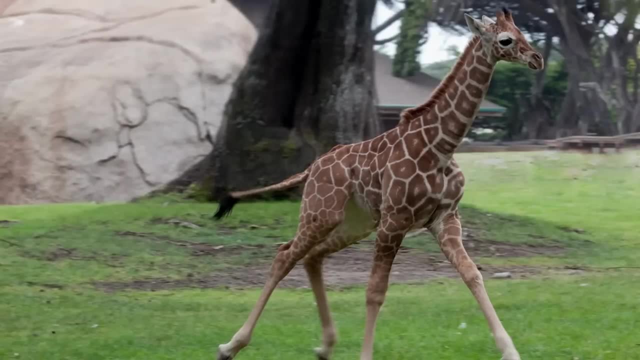 but it's not just movement that you need to worry about. it's also the eyes or whatever way the subject is facing. This giraffe also has an uncomfortable composition because he's about to run into the side of the frame. A simple recrop on this improves the picture. 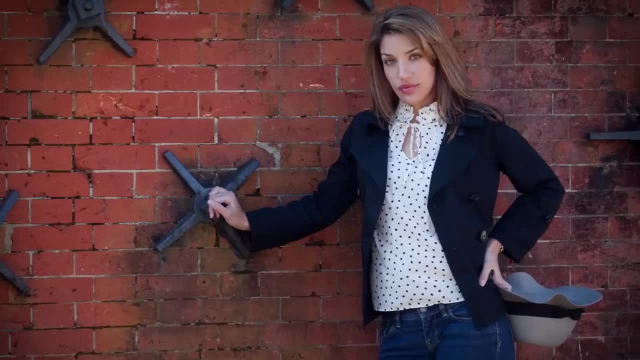 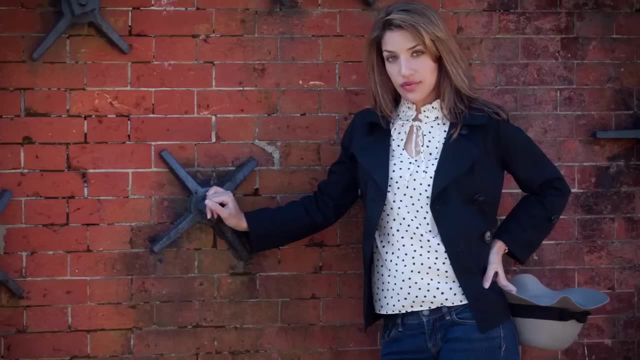 very much. Here's a portrait of my wife, Chelsea, and, as you can see, I've aligned her with the right third of the frame, but I've also left room on the left side of the frame because her nose is tilted to the left, so she's not looking in one direction or the other. 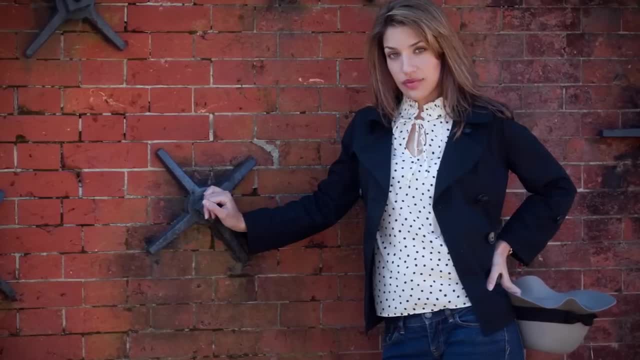 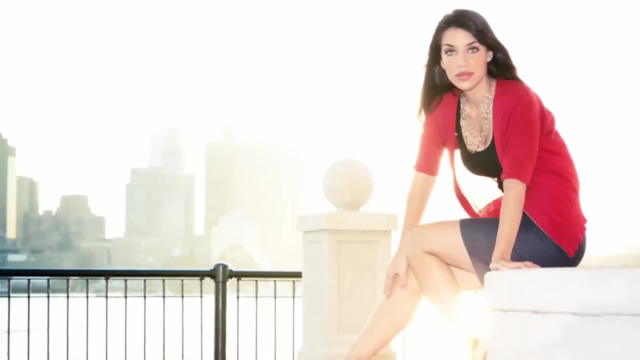 but her head is slightly turned that way, so the more conventional composition is to leave room on that side of the frame. Likewise, with this picture you can see her body is facing to the left, so I've positioned her on the right side of the frame, leaving room in front of her. 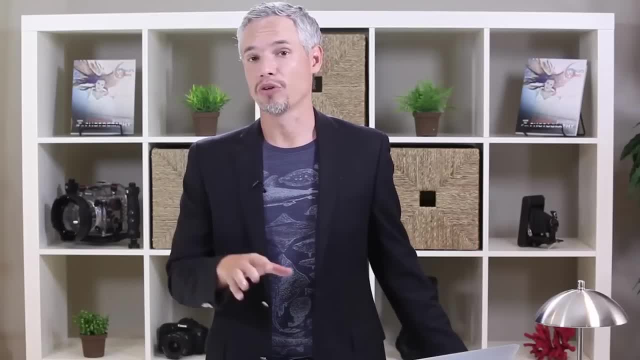 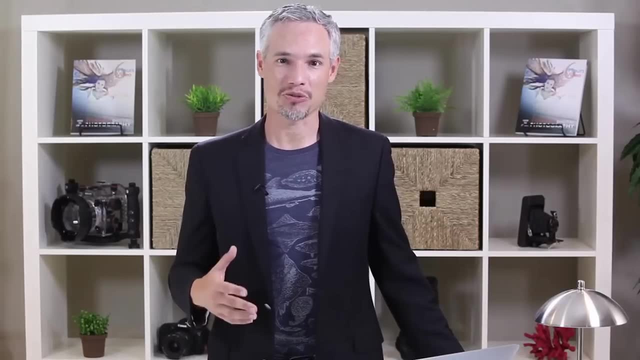 There are also times to break the rule of thirds, and the rule of thirds is so commonly used that sometimes you can use that discomfort a little bit, add a little tension to the picture and make it interesting. I'm fine with that, but I do want you to always be. 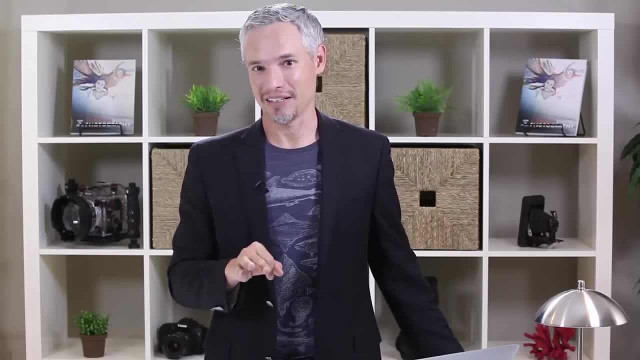 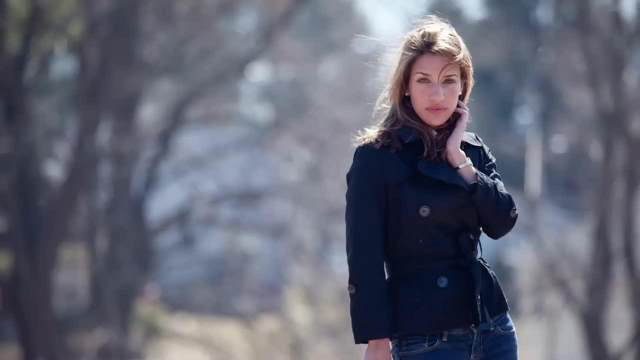 abusing these rules deliberately. Don't do it accidentally. Make a conscious choice to break the rule of thirds. I've done that with this portrait of Chelsea here. As you can see, it's not terribly distinct, but you can see that her body is turned. 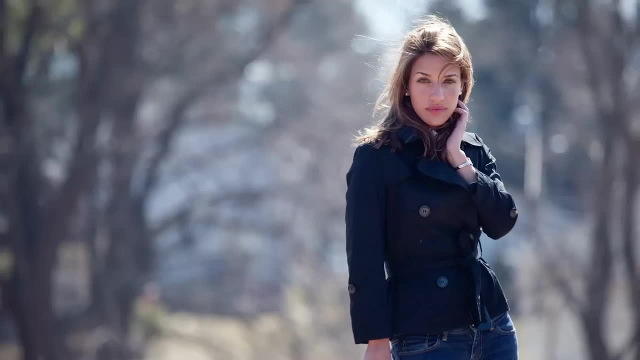 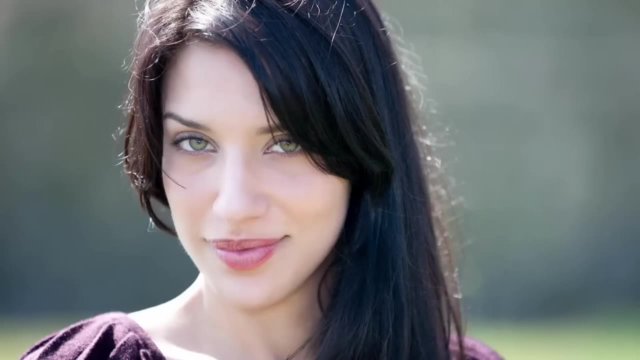 to the right side of the frame, facing the closer edge, and that just adds a little bit of tension and interest to the picture. Likewise, with this headshot of Chelsea, you can see that she's facing off towards the left of the frame and it's not distinct. 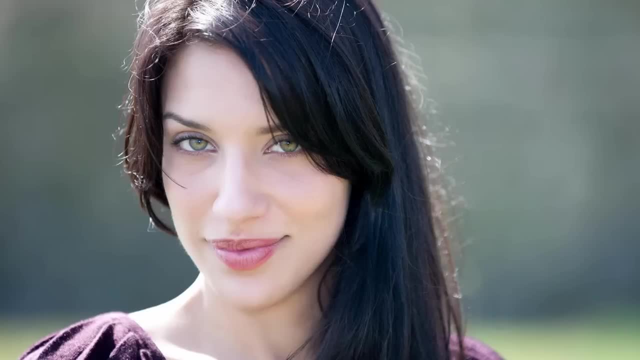 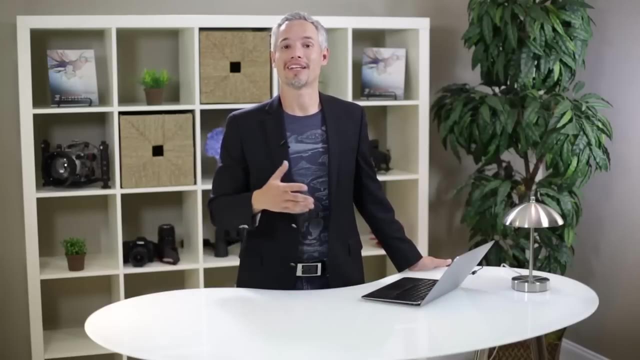 but it is enough to just draw your eye to it a little bit more than perhaps a more traditional composition would. Now let's talk about the angle of view. Every lens has a distinct angle of view that's defined by the lens's focal length. 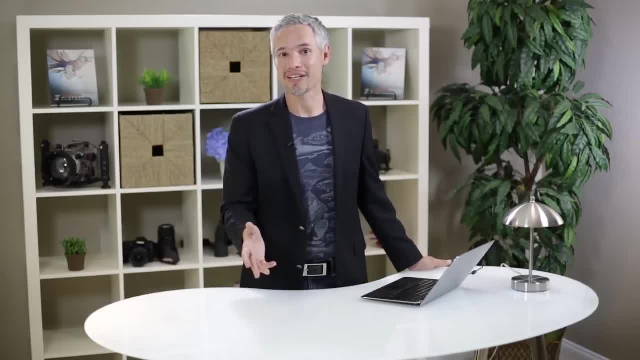 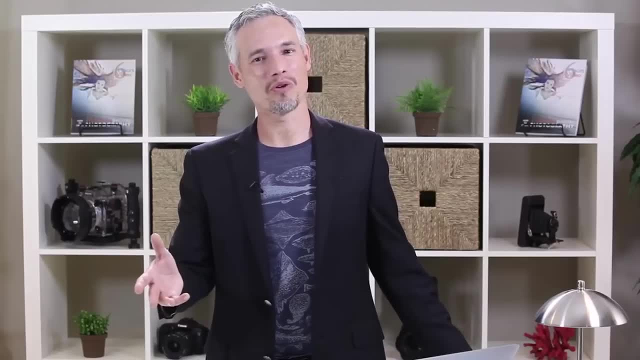 So a wide angle lens such as a 24mm lens, shows a pretty wide angle of view, and that includes a lot of the background. If you want to fill the frame with a 24mm lens, well, you're going to have to get pretty close to your subject. 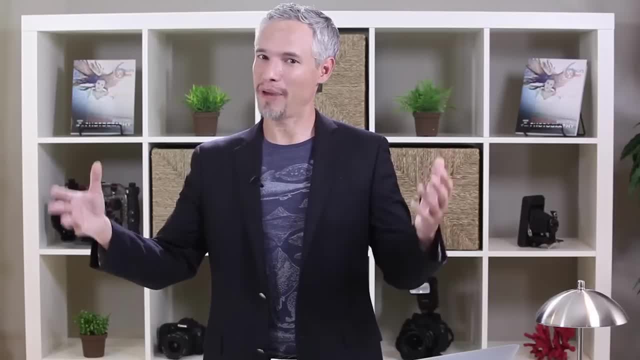 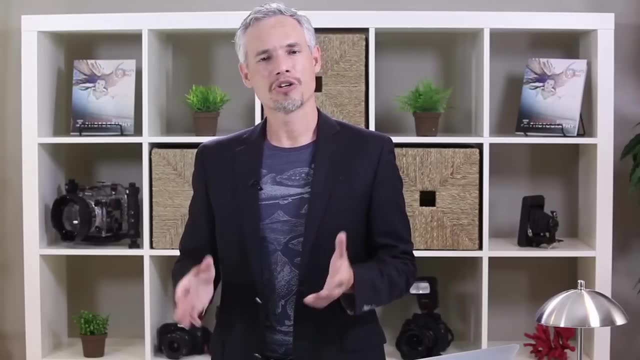 maybe even uncomfortably close, And no matter what, it's going to show way more of the background than the subject does. If you zoom in and use a telephoto lens, such as a 200mm lens, you're going to show much less of the background. 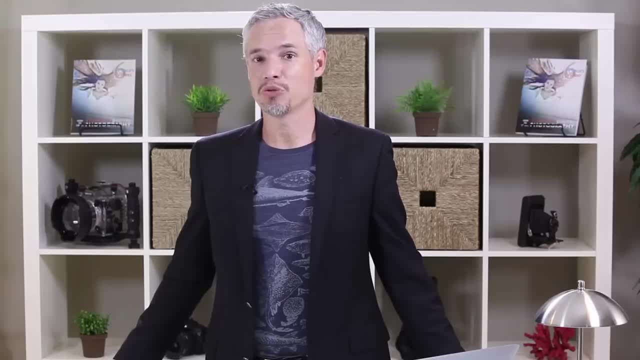 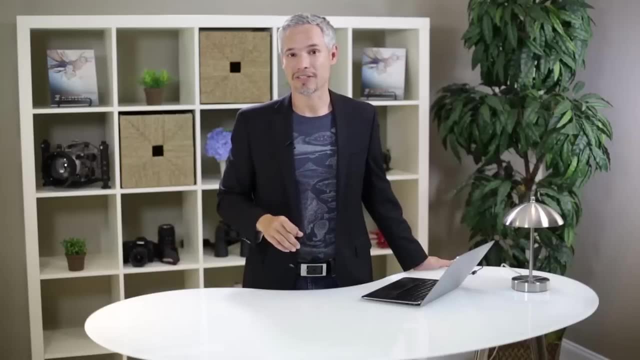 And this is a really important concept to master, because mastering it will allow you to control both the subject and the background, and how big they are in proportion to each other. Using a telephoto lens can allow you to greatly simplify the background, reducing the complexity of your composition. 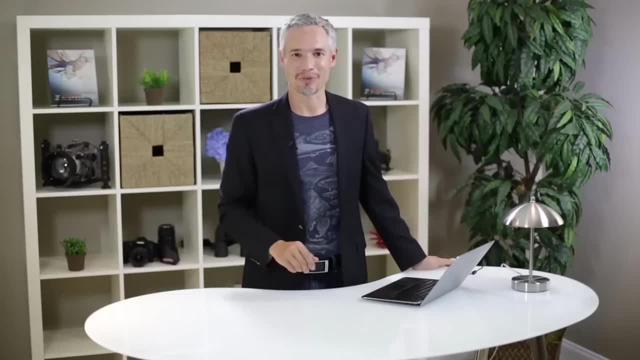 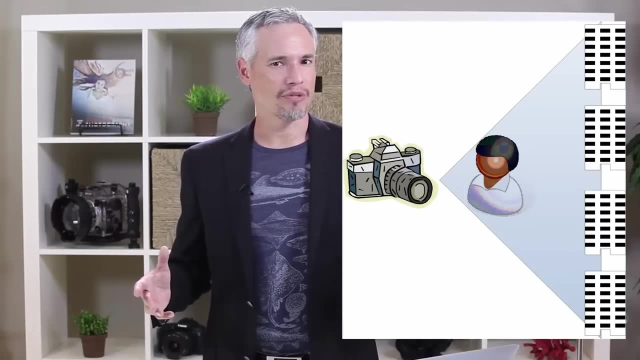 and improving your pictures drastically. So let's look at some examples. This awful diagram shows a wide angle lens being used to photograph a subject in front of some buildings And, as you can see by the diagram, the subject is in the picture, as are all. 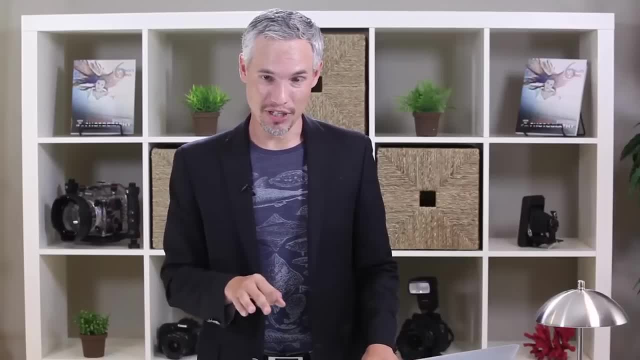 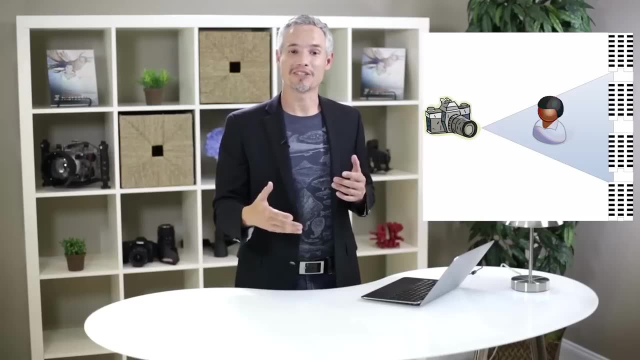 four of the buildings. Now, if the photographer steps back and zooms in a little bit, their perspective changes. This picture shows the subject the same size in the frame, but the photographer zoomed in. So he took a step back and zoomed in a little bit. The subject is still. 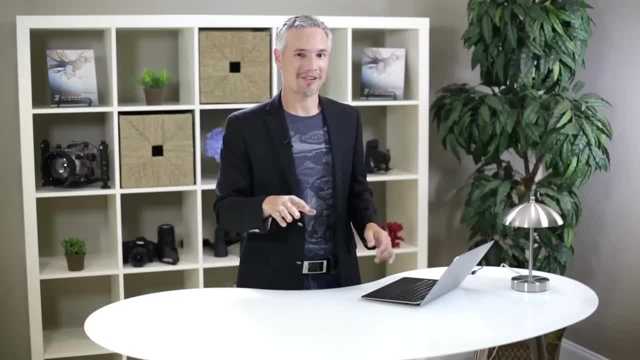 the same size in the picture, but there are fewer buildings in the background. Let's zoom in a little tighter. Here we can see again the subject: the same size, but we see even less of the background. So let's make this real by taking a look at some photos. 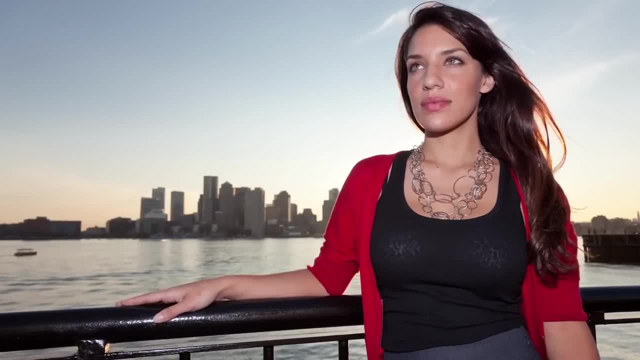 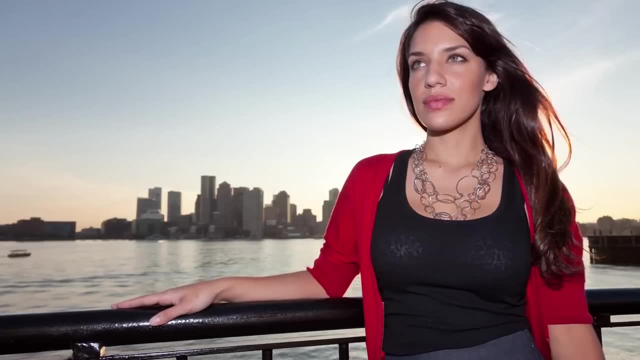 There's my wife, Chelsea, again standing in front of the Boston skyline. I shot this with a super wide angle lens And, as you can see, there's a sweeping cityscape behind her. You can see a whole lot of buildings, So I want you to make note of how many. 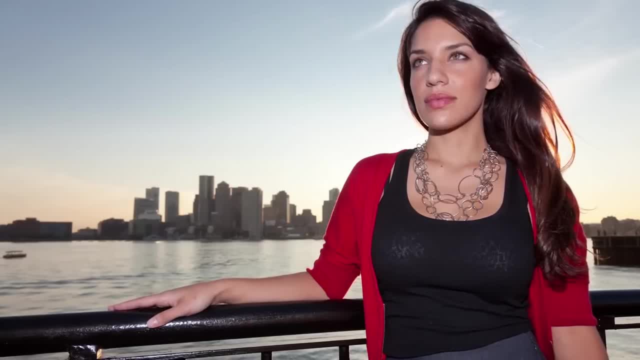 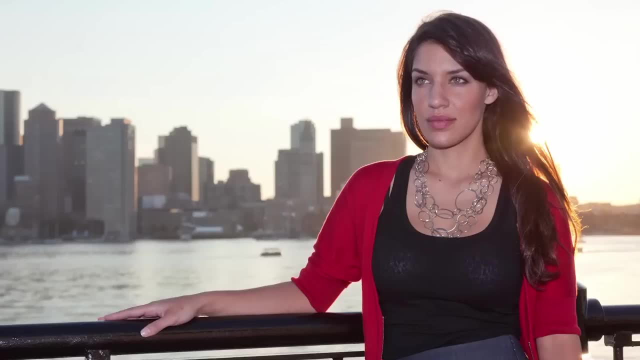 buildings you can see and how tall those buildings are in the frame. Also, note just how much of the sky that you can see. Now I took a step back and zoomed in And, as you can see, Chelsea's size didn't change in the picture, but the size of the 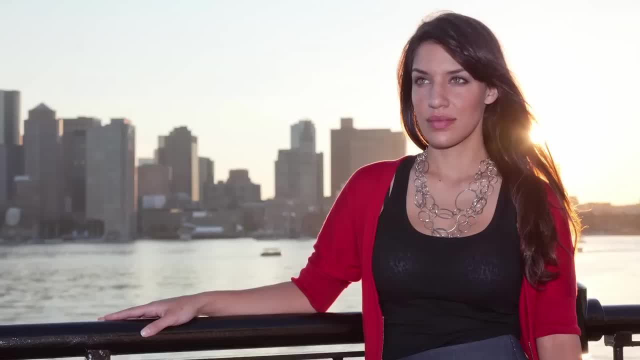 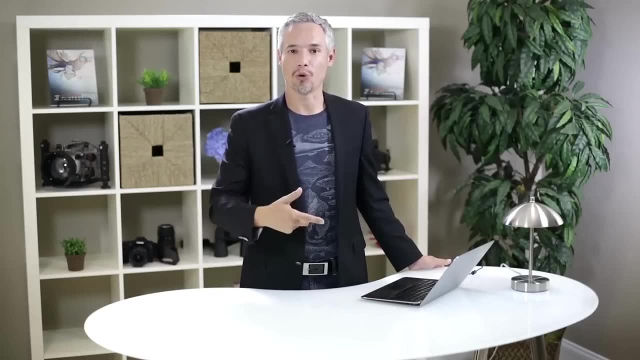 buildings did. You can use perspective and a zoom lens to control the size of the background. You can also control it by using prime lenses. You just have to take the lens off and put on a more telephoto lens. So, as you can see here, zooming in shows. 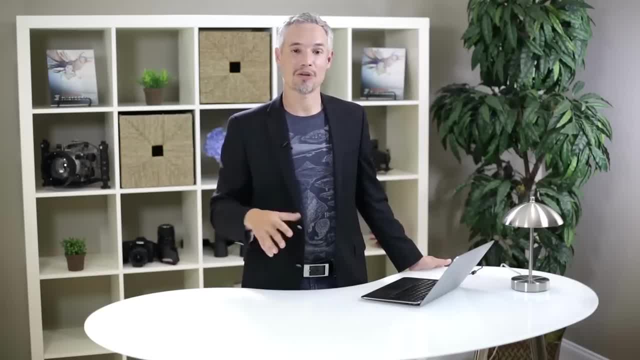 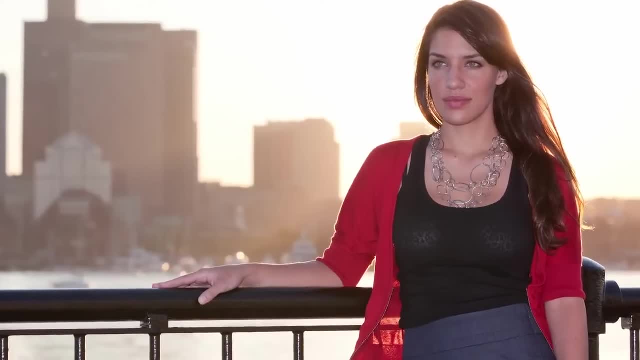 less of the background, but it doesn't necessarily change the size of the subject. If you're willing to move your feet a little bit, let's zoom in even further Now. those buildings are really big. Chelsea hasn't changed much, but the background is getting more and more simple. 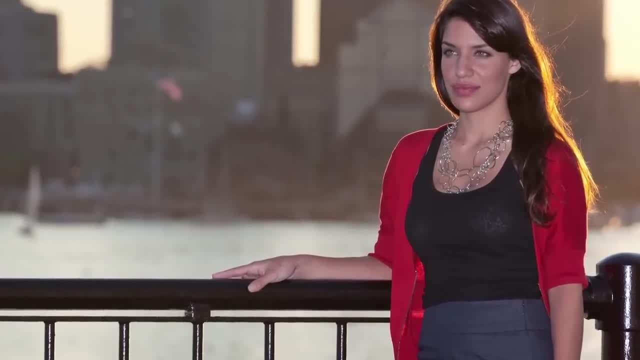 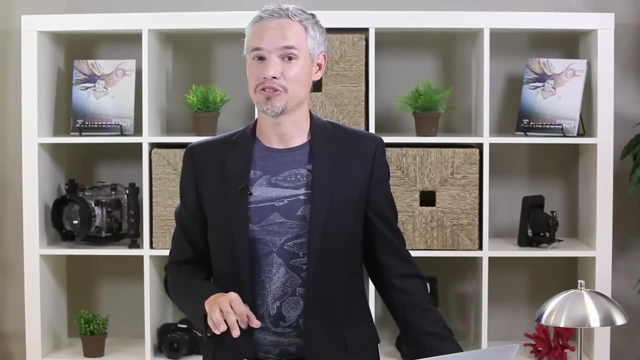 Now those buildings are going off the frame, We can't see the sky at all. That's the power of a zoom lens and switching from wide angle to telephoto. So the next time somebody tells you you just need a single lens, like a 50mm lens. 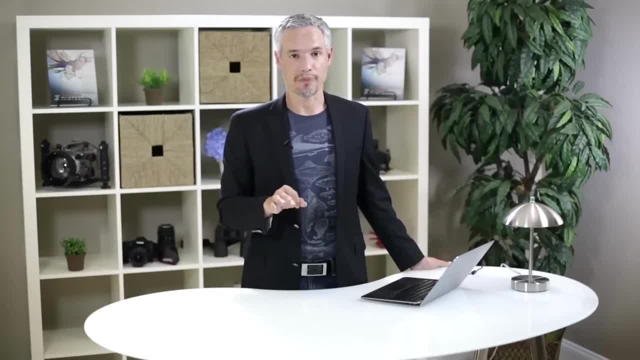 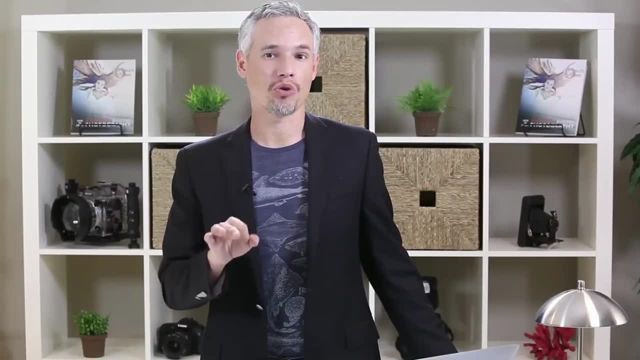 don't believe them. You can do that, but you won't ever be able to control the background. Now let's head to Harkness Park in my hometown of Waterford, Connecticut, to learn how to control the portrait background using zoom lenses and several 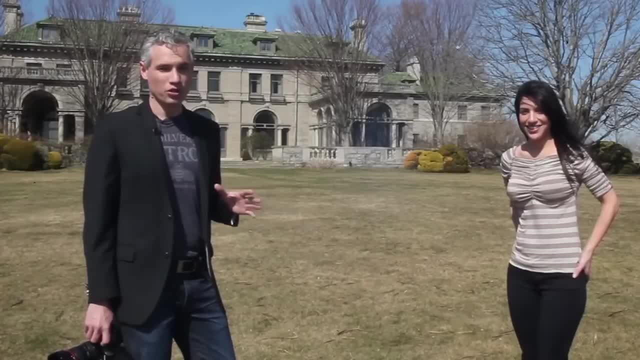 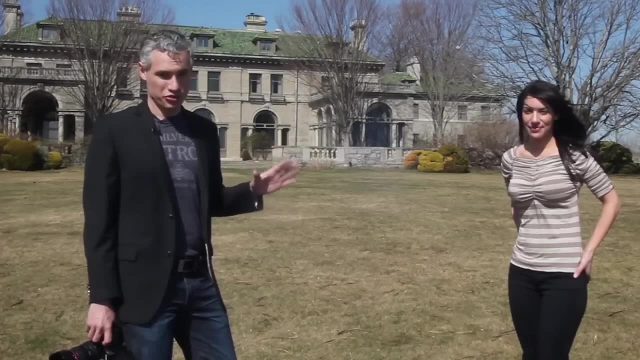 other techniques. The background is one of the most critical parts of composition. People often focus on a subject and find a good focal point, but then have a background that's cluttered or distracting. For this exercise, I'm going to have Chelsea stand in this. 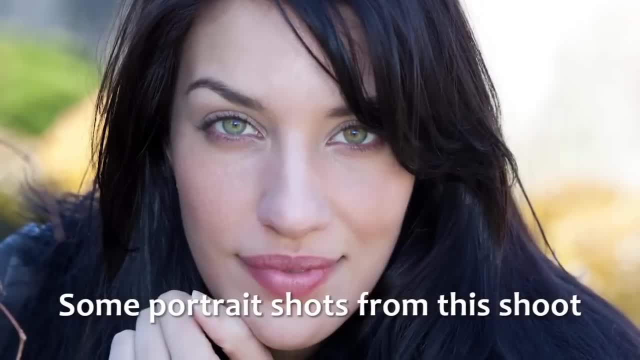 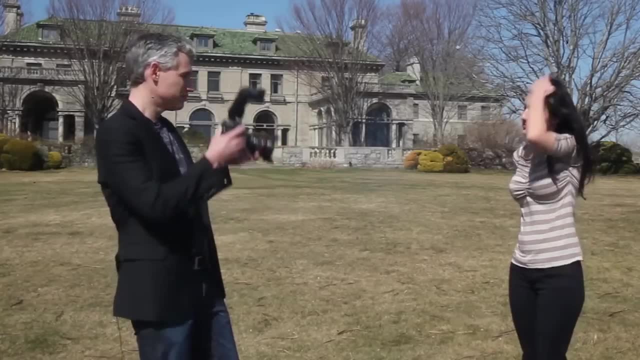 spot and not move from it. I am then going to show you all the different backgrounds that I can choose from. So first I'll do what many people do, which is to take a shot, as I'm standing here. As you can see, it's not a 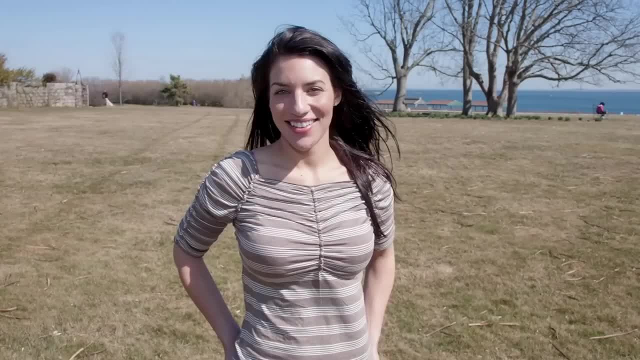 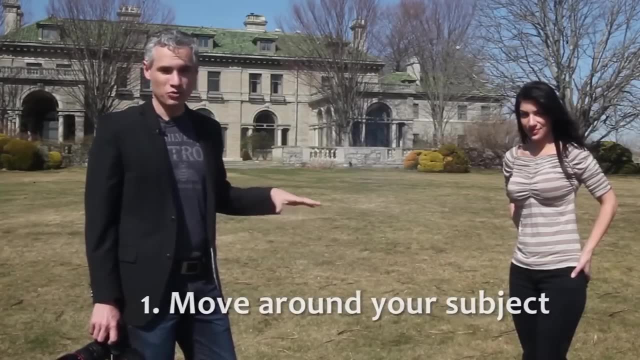 bad shot, but the background is fairly uninteresting. So what I'm going to do is I'm going to move in 360 degrees around Chelsea. She'll rotate to face me, but she won't move from that spot. Wherever you are, you always have. 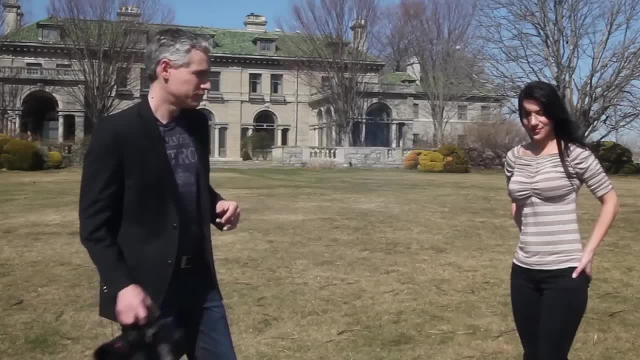 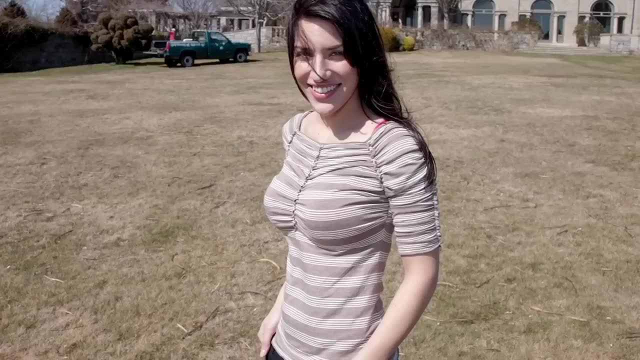 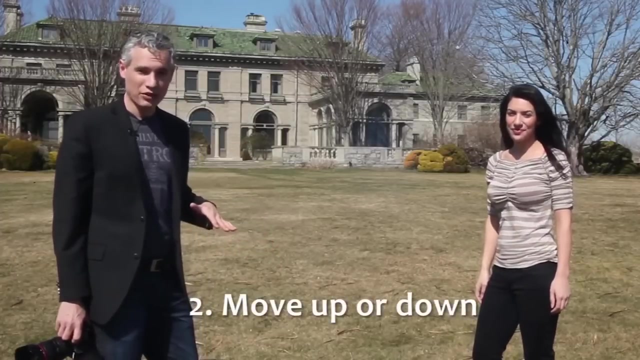 360 degrees of background to choose from if you can move. So you have a lot of different options just by walking around your subject. The second way you can control it is by moving up or down. You don't necessarily need a ladder or anything, You can just. 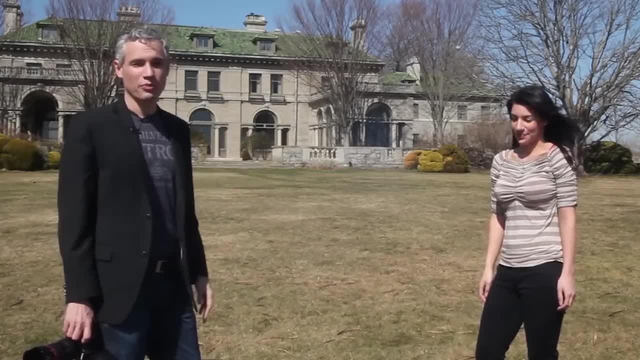 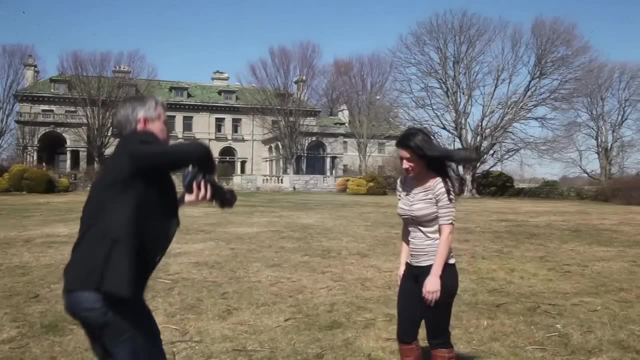 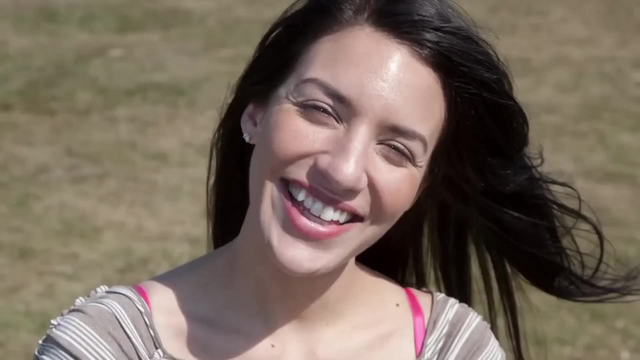 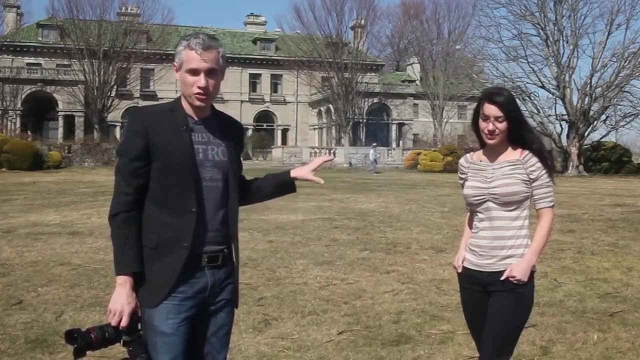 crouch down to get the sky as your background, or lift your camera up to get the ground as your background. Just by raising the camera up and down, I was able to pick between a completely blue sky background, the green grass, or a background that shows the horizon. 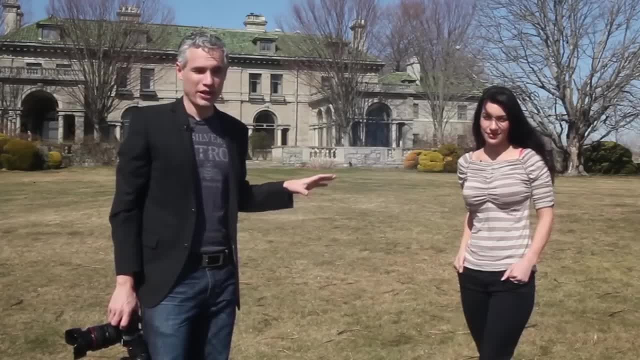 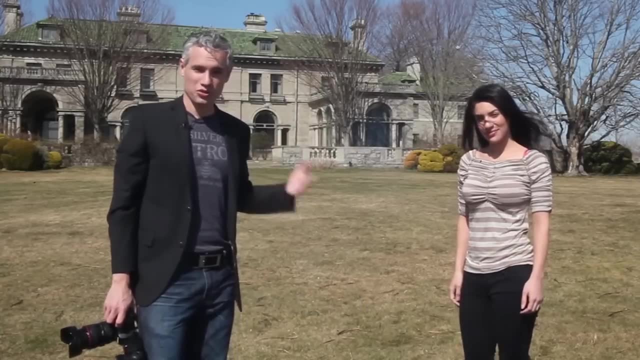 The third way you can control the background is by zooming in and out. You don't necessarily need to make your model bigger in the photo when you zoom in, because you can also step back. So to demonstrate this, I will step forward and away from Chelsea. 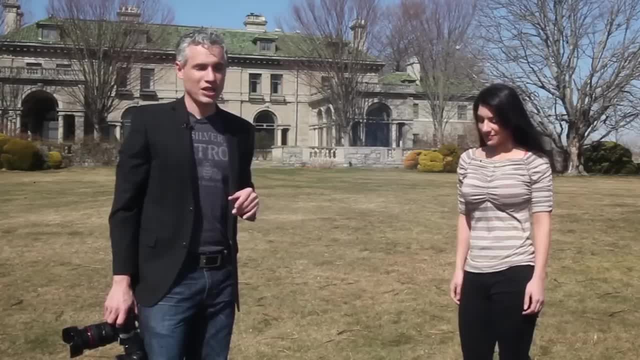 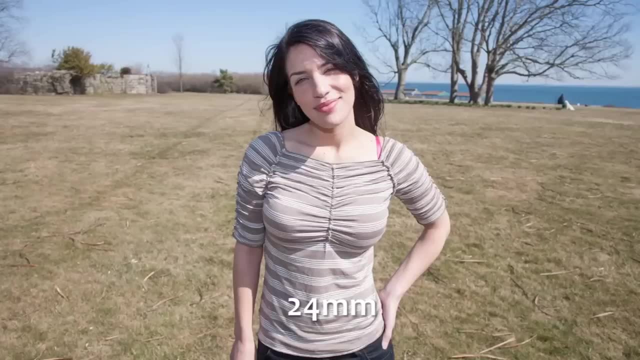 but I will keep her about the same size in the frame and it will show you how changing the perspective adjusts the background. So that's what it looks like when I'm standing fairly close to Chelsea and I'm zoomed way back. Now, if I 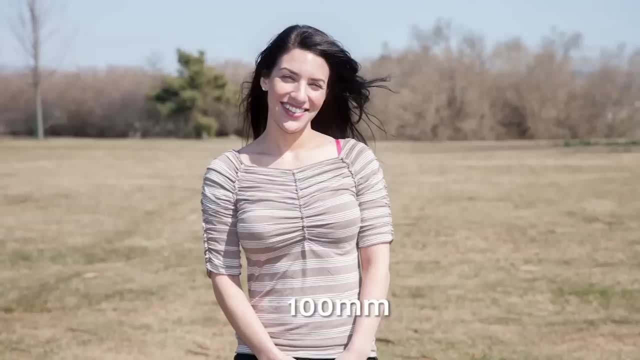 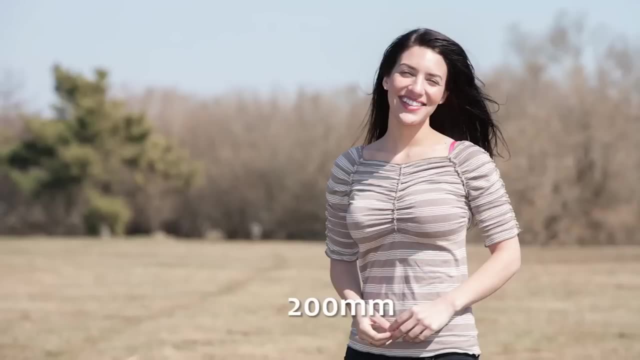 step back and zoom in, you'll see a completely different effect. So in this photo you can see less of the background. That's at about 100mm. If I step back even farther and zoom into 200mm, you'll see the background becomes very. 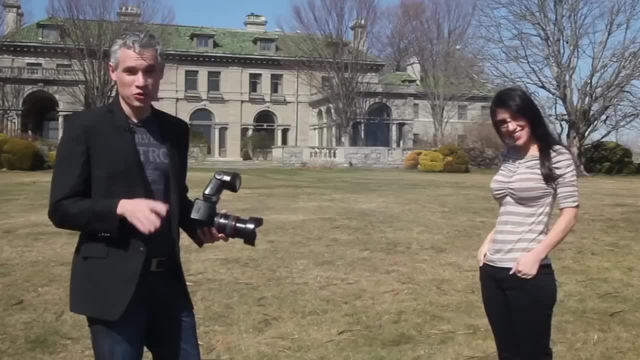 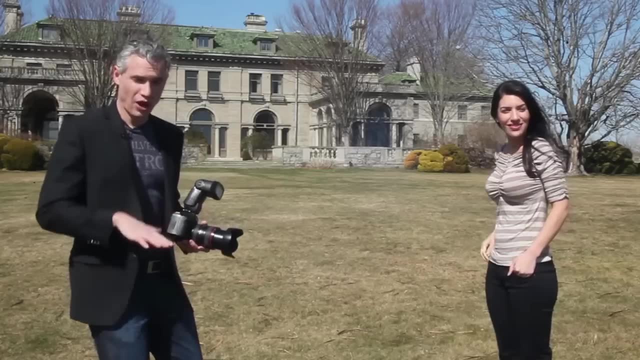 narrow and becomes more blurred. So if you, as the photographer, can move around, those are three things you can do to control the background. Move around your subject 360 degrees. move up and down, or step forward and back while zooming in and out. 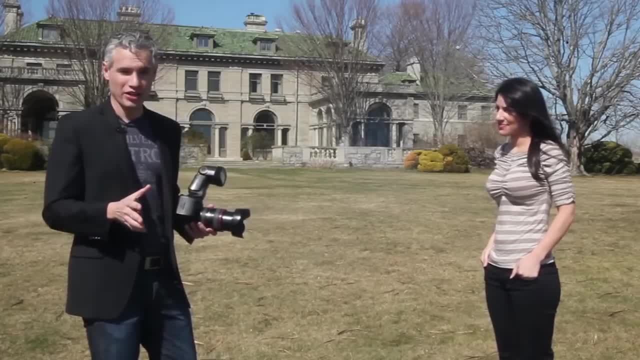 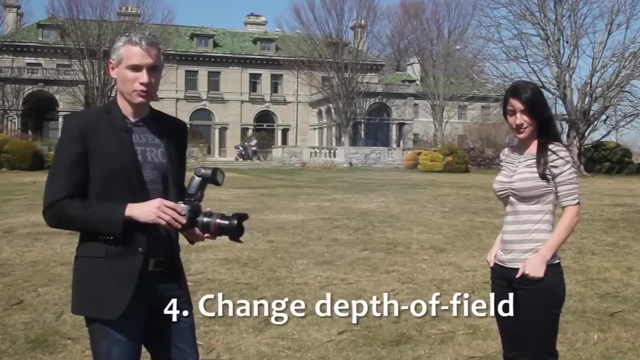 If neither of you can move- maybe you're in a crowded area or, say, a zoo- what you can do is adjust the aperture to change the depth of field. Now, as you'll learn in the book, choosing a lower f-stop number decreases the background sharpness. 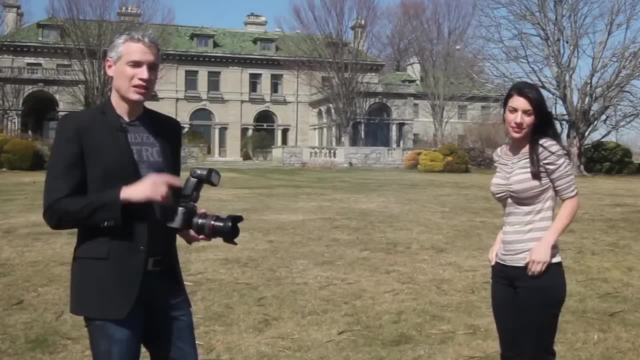 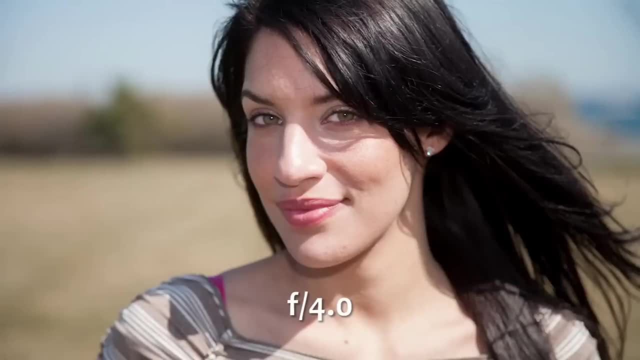 A higher f-stop number increases the background sharpness. Now I'll show you how that can change the effect of a picture. As you can see at f4, a low f-stop number, the background is very blurred Here at f22,. 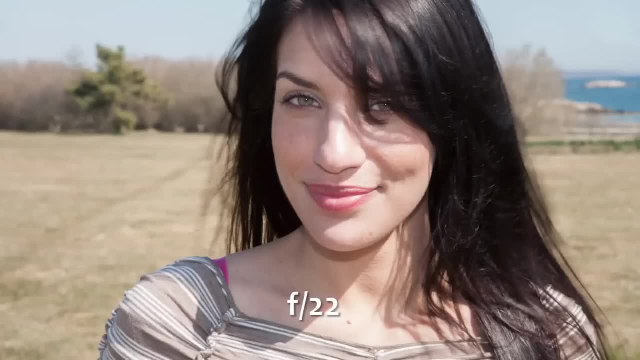 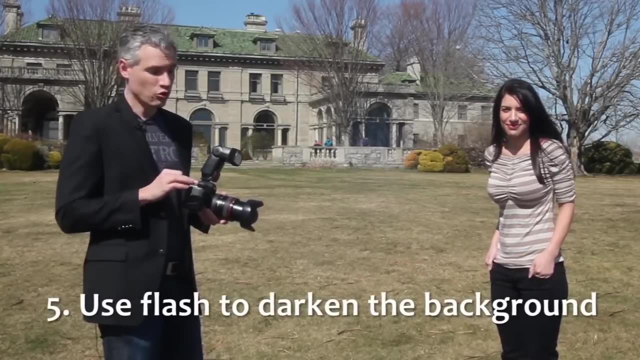 a higher f-stop number, the background is much sharper. There's one last thing you can do to control your background without moving yourself or the subject, and that's by using flash. Normally, your camera will expose the foreground and the background will be at about the same exposure, because 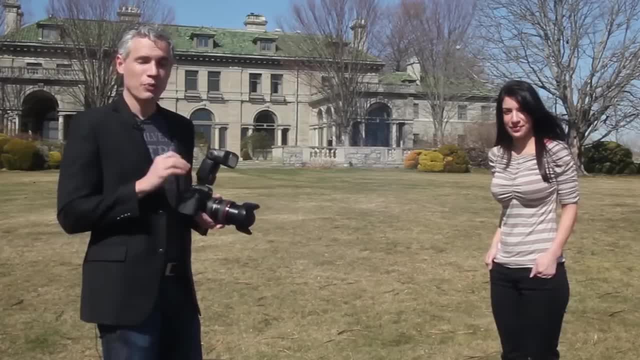 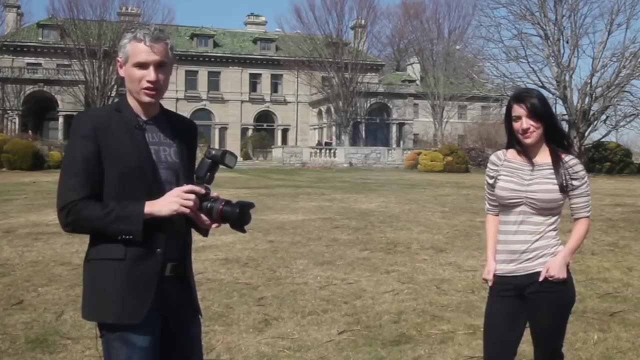 the same light will be falling on your foreground and the background. But if you turn your flash up, that will add light to the foreground and the background, in comparison, will seem much darker. Now it's a little bit hard to do that with. 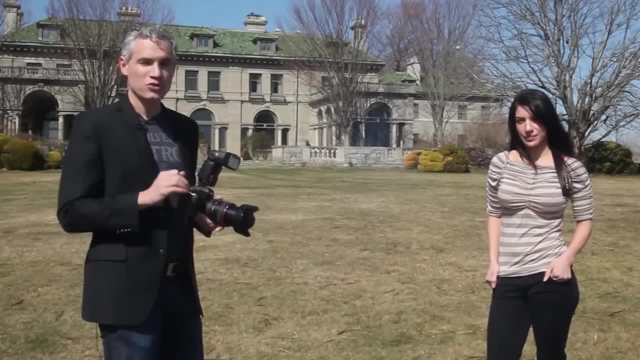 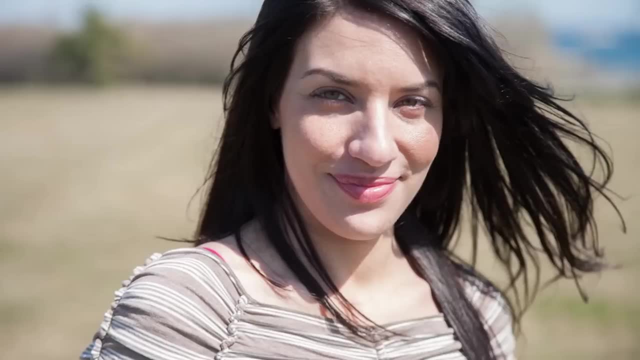 sunlight, but if you have a powerful flash you can still do it. So first I'll take a shot with no flash at all. As you can see here, the background and the foreground have about the same exposure. Next I'll 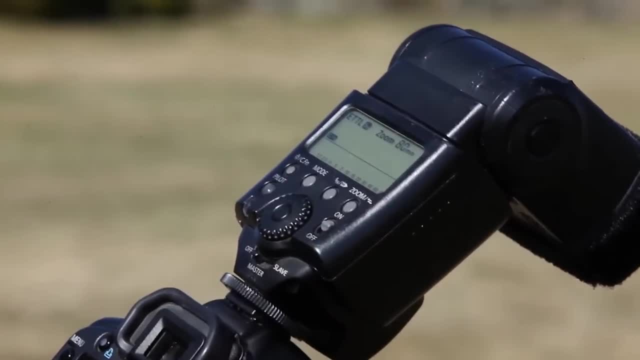 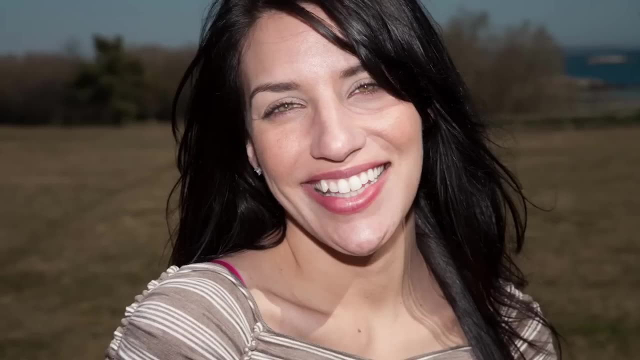 turn the flash on and turn it all the way up so it puts out as much light as possible. As you can see, by properly exposing the foreground, the background in comparison became much darker. Now I'd like to talk about showing scale in pictures. 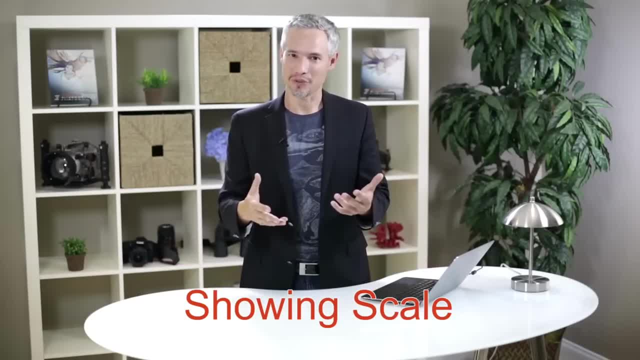 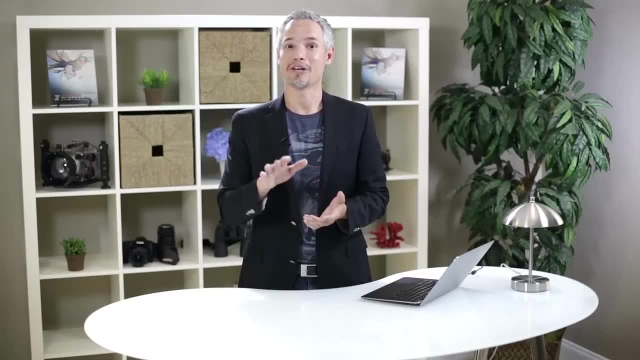 Scale allows you to define the size of something visually in a picture, and if size is important to the subject in the picture, then scale is going to be very important, because if you don't include scale, nobody's going to know how big or small it is. Let's take a look at some examples. 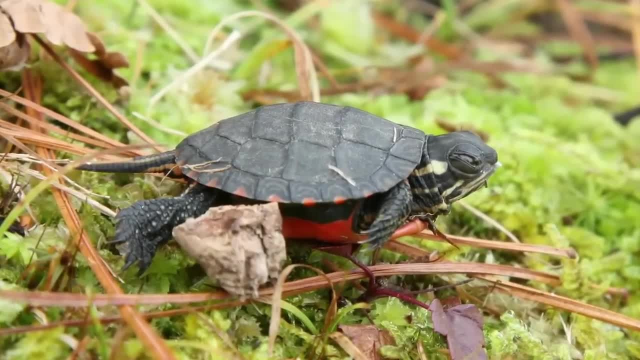 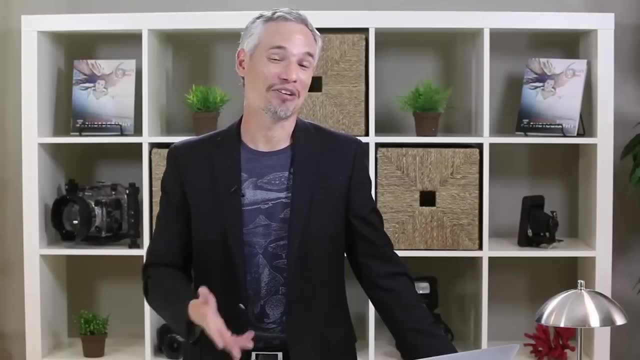 This is a baby painted turtle that I found in my backyard in Massachusetts, and from this picture- well, you don't know- It could be as big as a dinosaur. Okay, you probably wouldn't think that, but you don't have a clear sense for just how tiny. 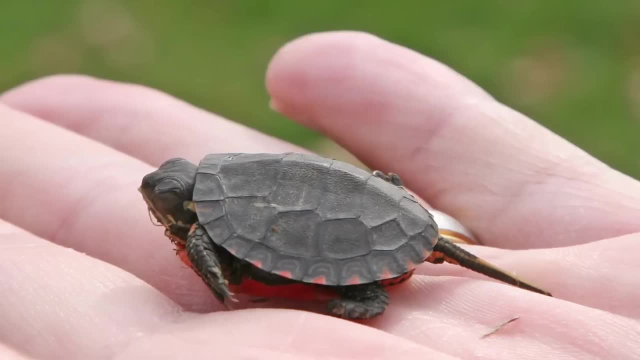 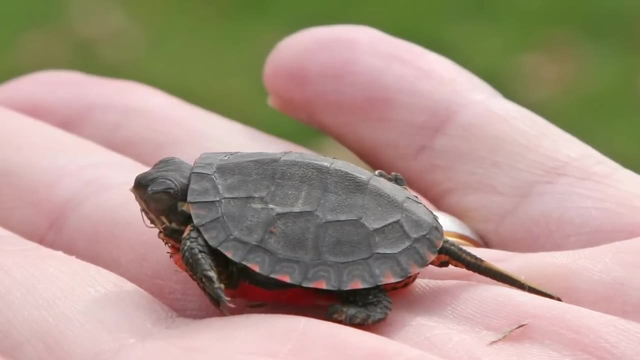 this baby is. so I took a second picture. Now you can see just how tiny that baby turtle is, because you probably know how big a human hand is- right, Unless you think I might have giant hands or something- and it's actually a massive turtle. 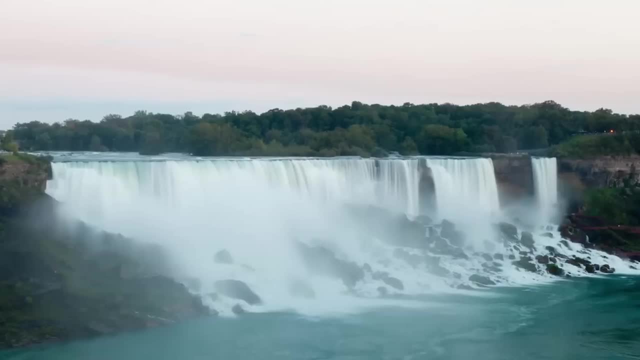 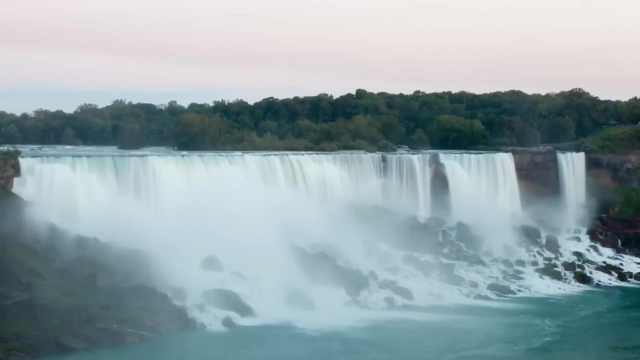 but you do get a much better sense for how small the turtle is here. Here we see Niagara Falls, but you don't know if this is just water spilling over a bathtub, right, You really don't have a sense for how big it is. But 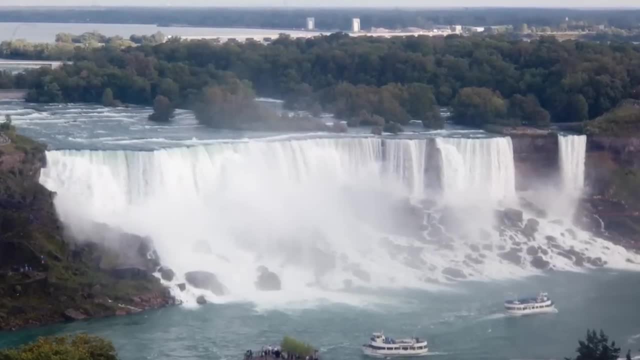 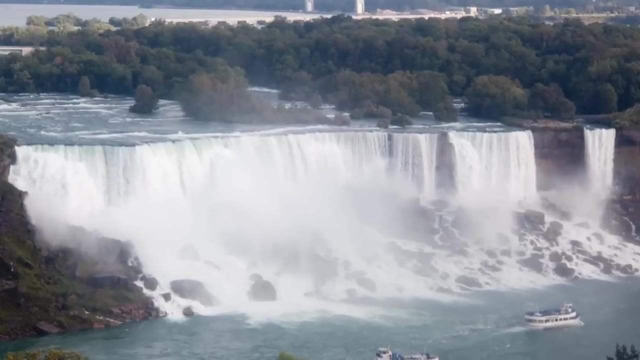 add the two ferries in there and suddenly you know just how massive it is, because you can see these two big boats. You can also see the people collected in the foreground at the bottom there. that give you a sense for just the massive scale This. 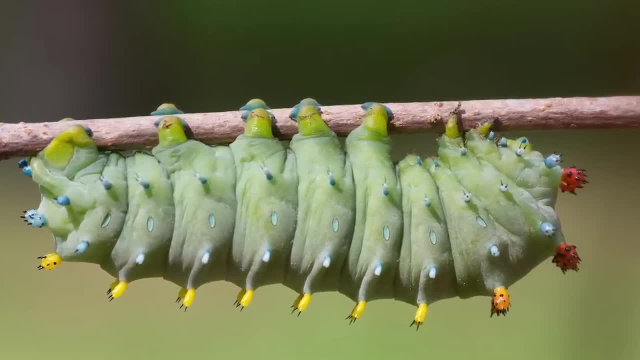 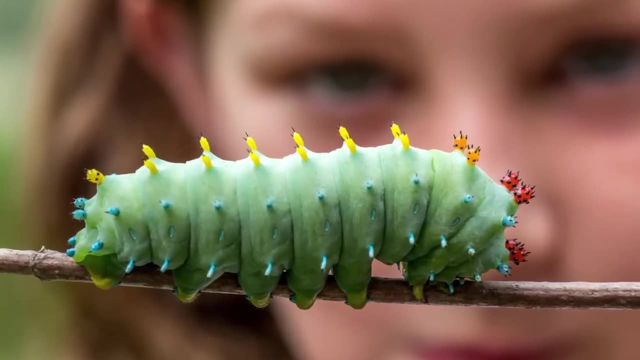 caterpillar is really cool, but until you see something for scale, you really don't know how large it is. You can see the original photo with no particular context. It didn't show you that this was a huge, huge caterpillar. so 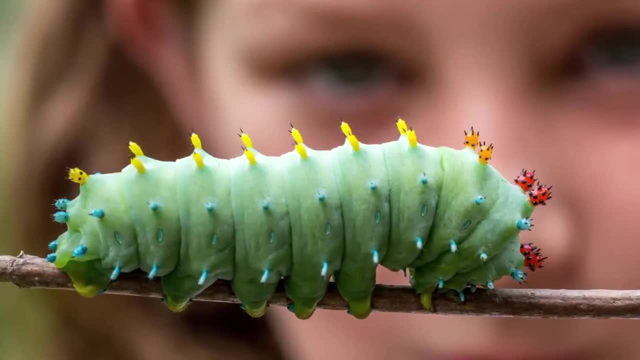 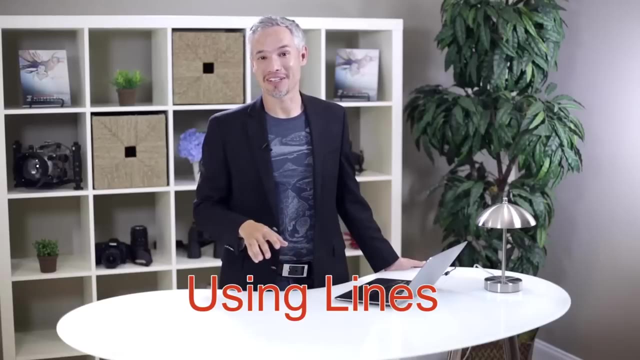 what I did was I just had my daughter hold the stick in front of her face, and her face provided some scale and it also provided a point of interest and perspective. Now I'd like to talk about using lines in photos. Lines are a really powerful compositional 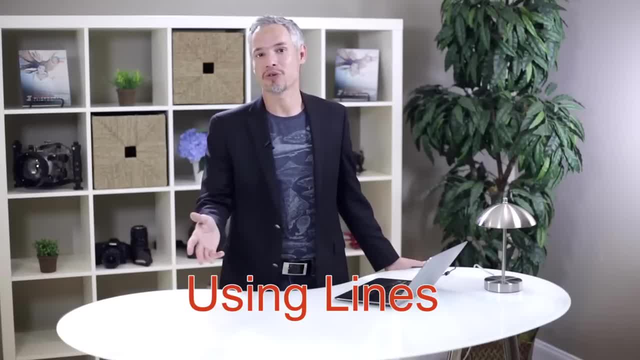 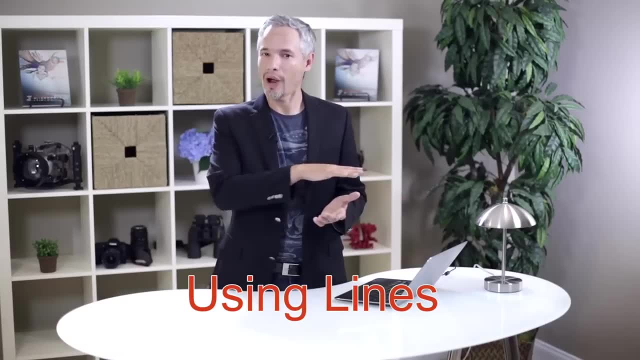 element and lines are everywhere. Of course, train tracks are a common type of line, but any sort of building creates a strong vertical line. If you're on the ocean, well, the horizon of the ocean is going to be a strong horizontal line. So the 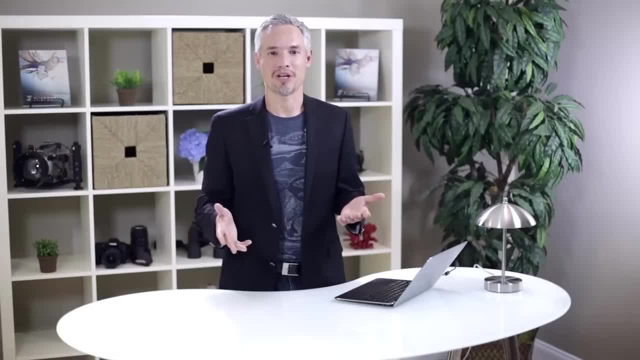 first tip I'd like to give about those lines is: just make sure they're straight. Now, nobody holds their camera perfectly level all the time. That's why you use your post-processing software, Picasa Lightroom. It just takes a second or two. 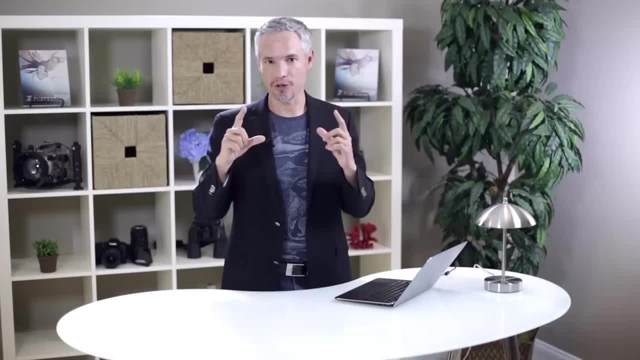 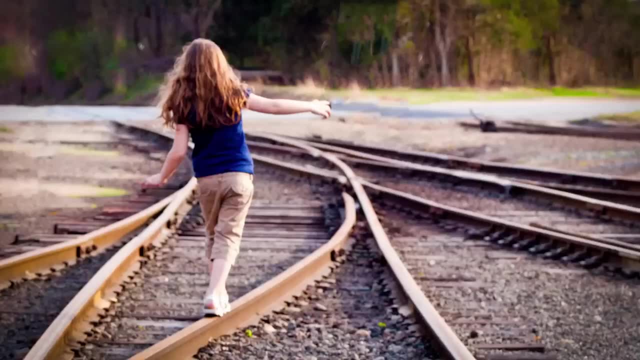 to level it in post, but do be aware and try to get your photo as level as possible when you're actually taking it. Now let's look at a few example pictures that use lines compositionally. Here's a candid shot of my daughter. 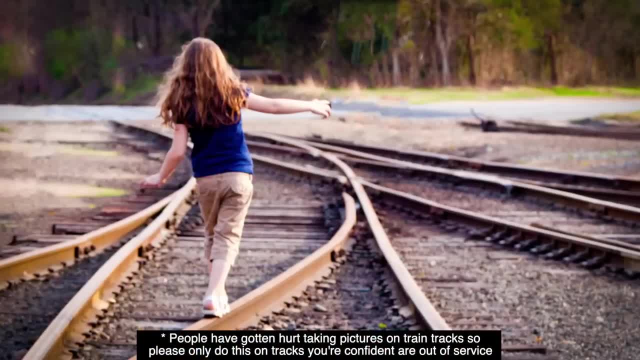 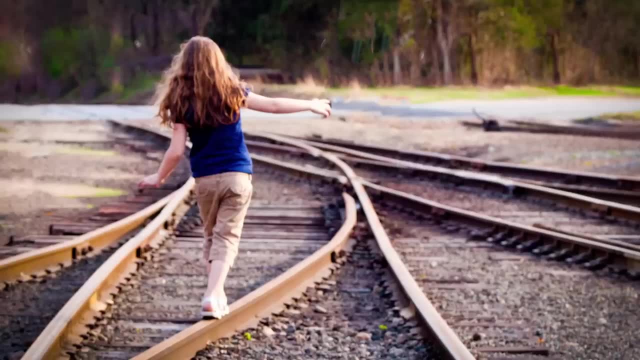 walking along train tracks, and what I like about this photo is the lines. All these train tracks come from the bottom and right part of the frame and they draw your eye to the single focal point where they converge. Now you want a subject. 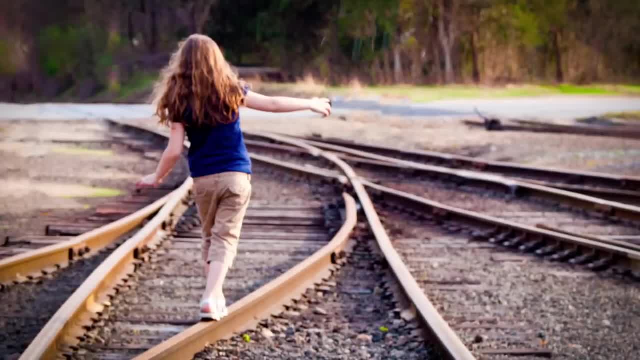 to be at that focal point, because the eye is going to follow those lines and if there's nothing there, well, the eye is going to have nowhere to go and it's just going to wander around. In this shot, my daughter is. 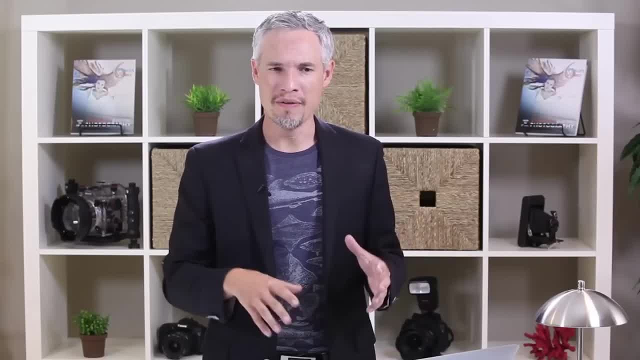 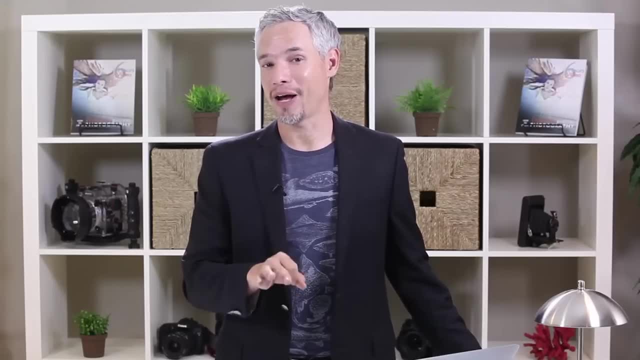 perfectly positioned because all the lines point right to her. So anytime you see strong converging lines in a photo, that's a great place to put a subject and it's also a great spot for a portrait. So grab a friend and put them where those lines. 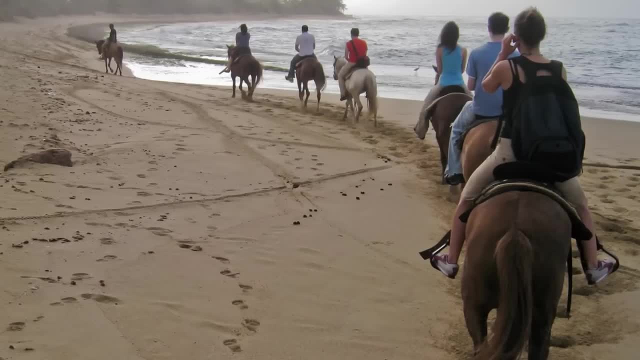 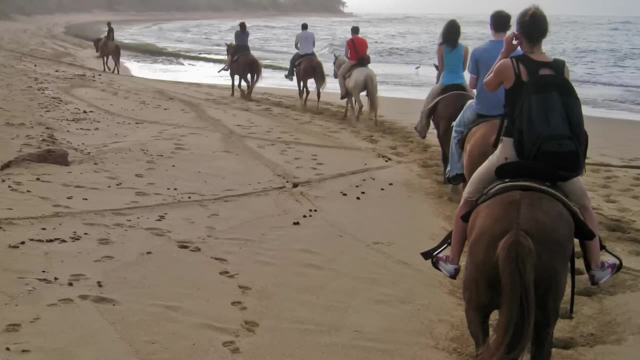 converge. Here's a snapshot that I grabbed on horseback, and you can see Chelsea in front of me there. What I like about this photo is that there are several nice curving lines that go from the bottom right of the photo over to. 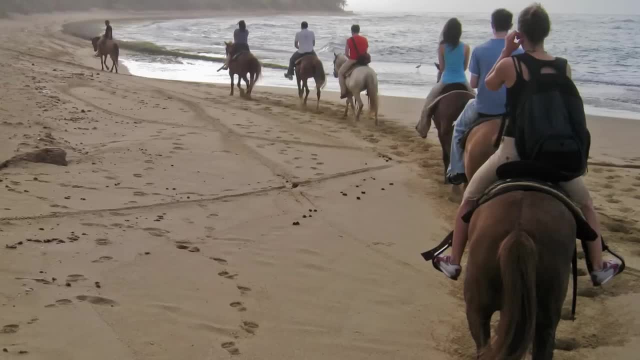 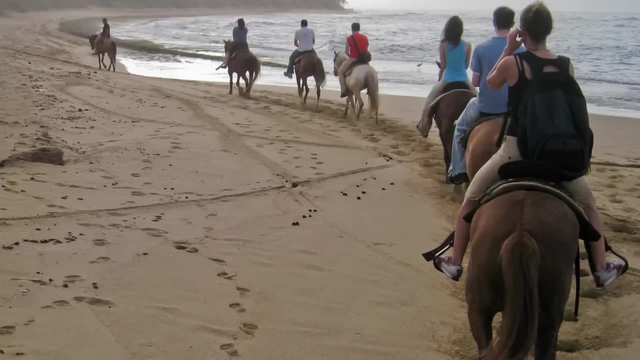 the top left of the photo. The horses themselves form a line, but the beach also forms a nice curving arc that complements the horse line really nicely. This photo is also a good example of using the rule of thirds. This isn't a particularly 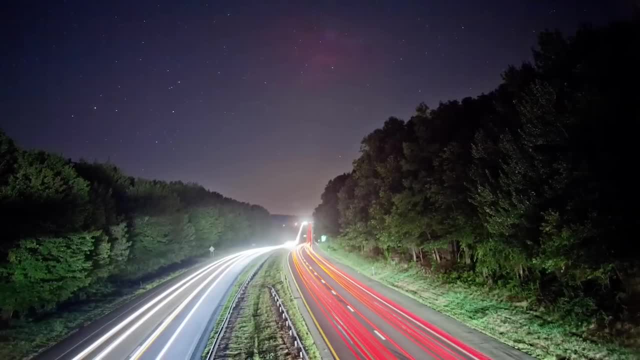 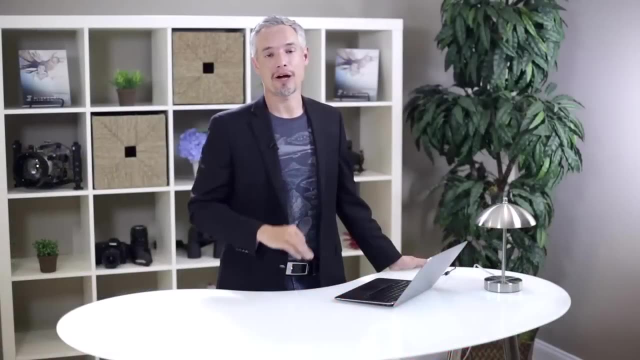 stellar example, but I do want to point out that, with night photography and traffic, the headlights and brake lights of cars are always going to form lines, and you can use this to your advantage as a really powerful compositional element. It can be hard to see because 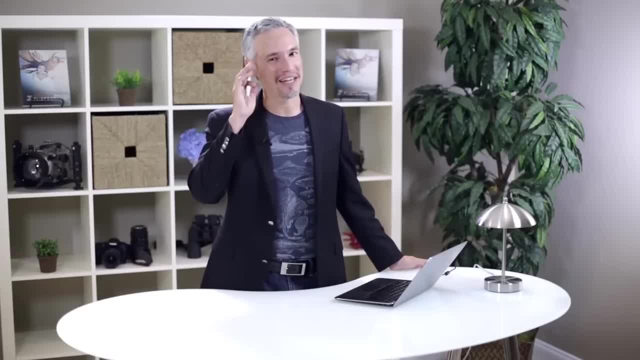 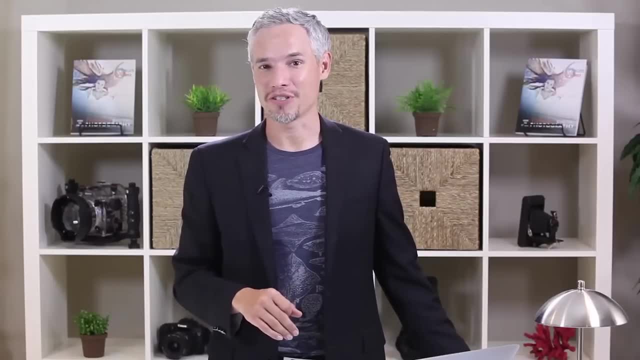 until you take a few night shots, you won't be able to imagine that the cars that you see moving are actually forming long, long lines. There's a whole lesson dedicated to night photography, so do check that out. This photo of the New York City skyline at: 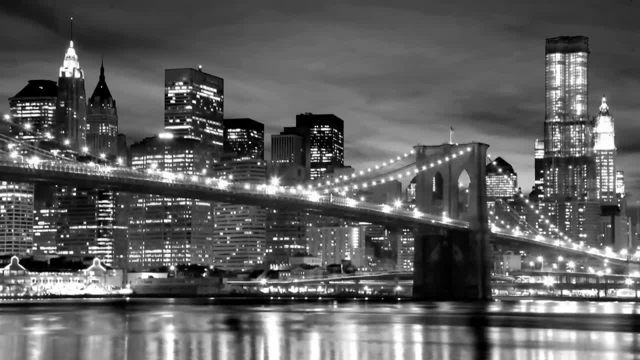 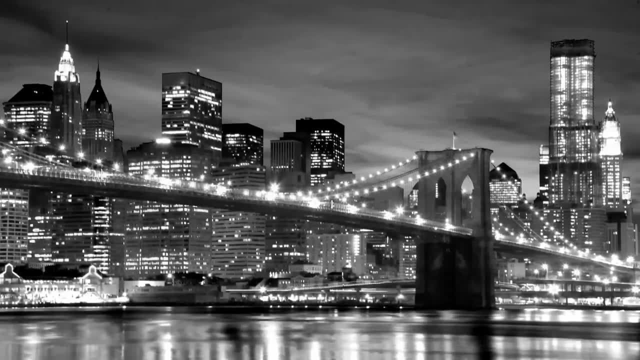 night from Dumbo Park in Brooklyn is all about the lines. These buildings on the skyline form strong vertical lines that draw your eye up from the water. but the most interesting line here is actually a diagonal line, That's the line of the Brooklyn Bridge. 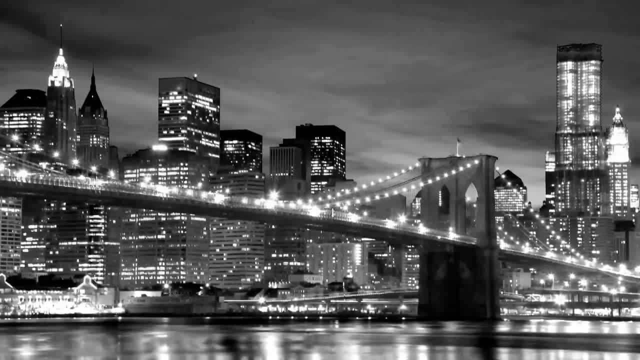 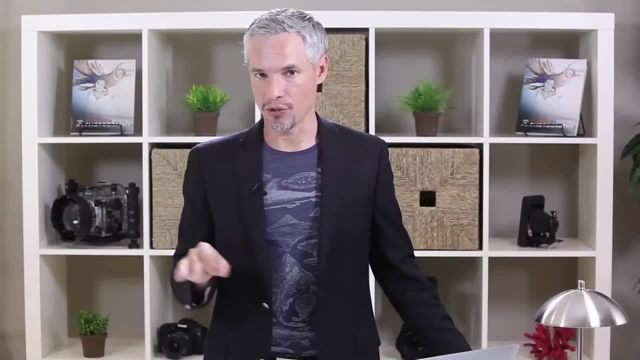 The diagonal line contrasts with the powerful vertical lines and makes the photo more interesting and dynamic. It also helps to bring your eye from the left side to the lower right, As you can see. once again I'm using railroad tracks as lines, And all the lines from the bottom. 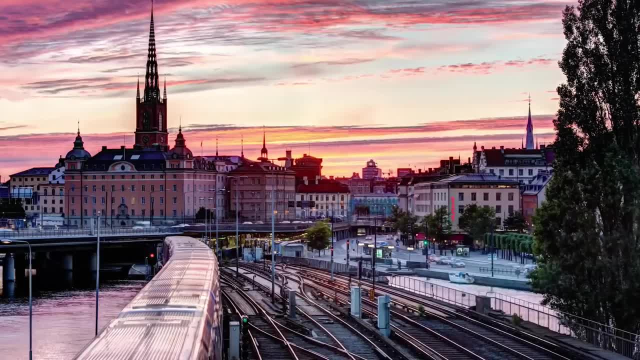 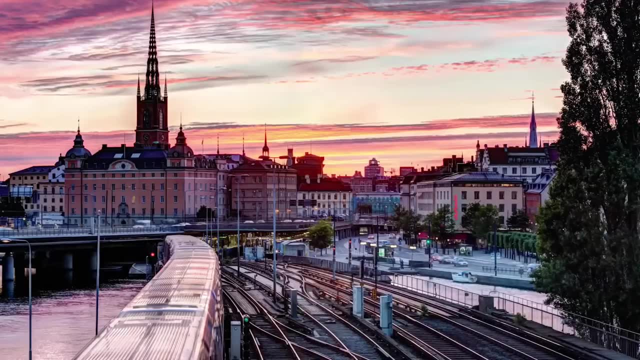 of the frame. converge and draw your eye right to the focal point of the picture, which is that beautiful building, and the steeple, And then the steeple itself forms a line that draws your eye up into the sky, So you can see there are. 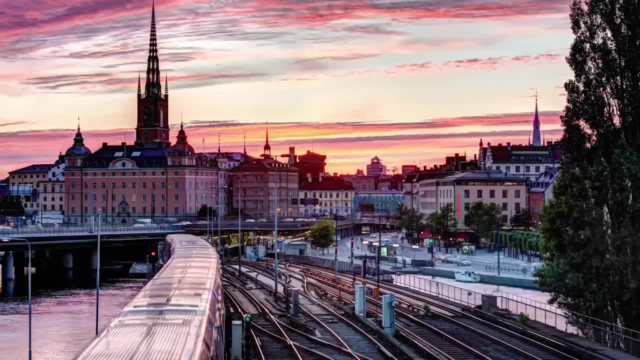 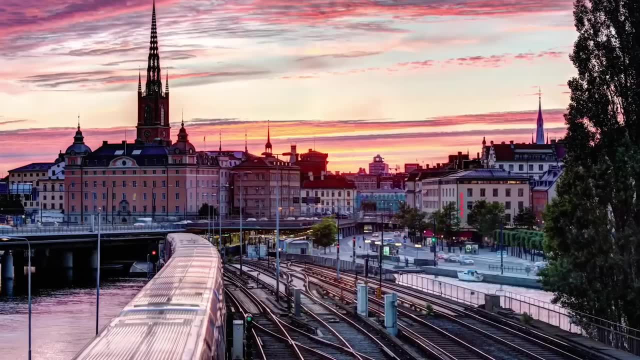 a lot of lines here at work Now to get this picture. it wasn't obvious. I had to go out of my way to get into a position where I was reasonably close to the train tracks. The closer I move to the train tracks, 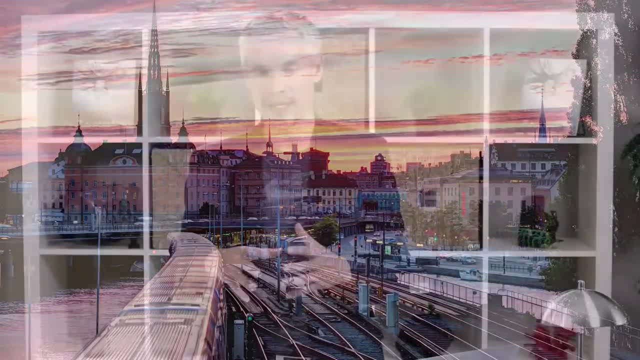 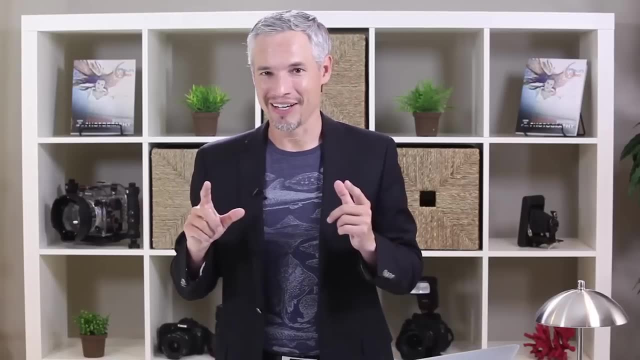 the more exaggerated the convergence is going to be. The higher up I am, the less exaggerated the convergence is going to be. So whenever you're working with lines, move around the lines If you move closer to a fence or a railing. 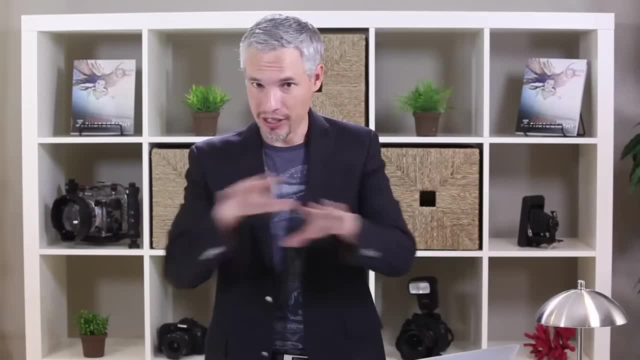 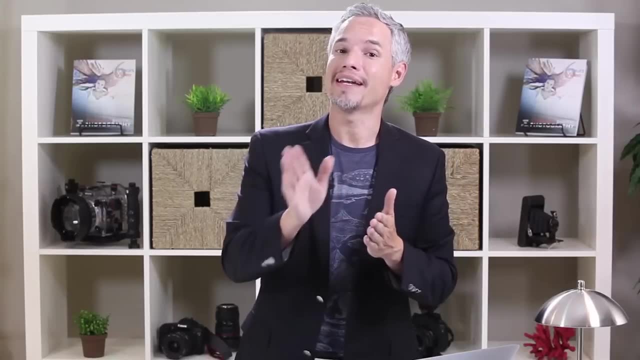 it's going to become more exaggerated If you move square to it. well, the lines are going to be horizontal, But if you turn at an angle to those lines, it's going to add a lot of depth to the picture And with that depth those lines are going to 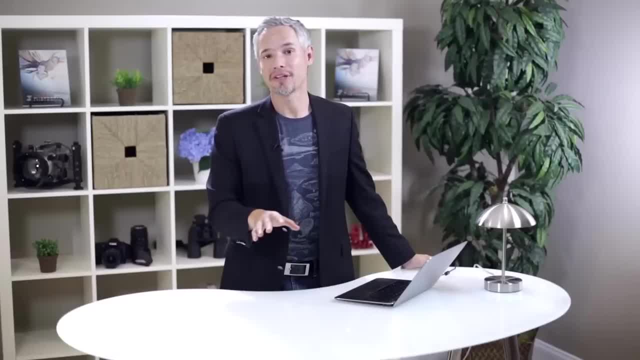 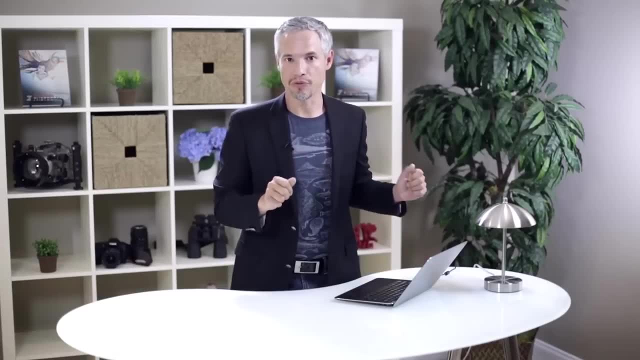 naturally converge and lead the eye through that. So think about the lines in your picture, but also think about the potential lines, the lines that you can move or create by changing your position and moving around. Use those lines deliberately to draw the viewer's eye through your 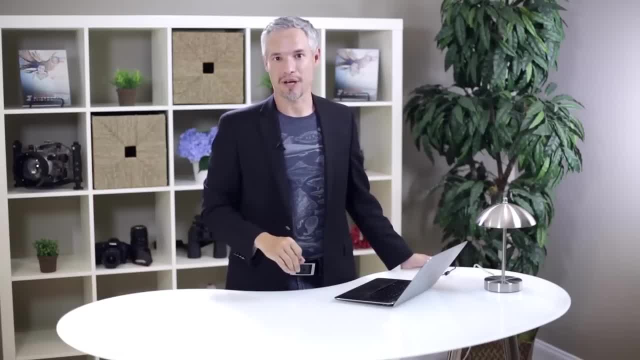 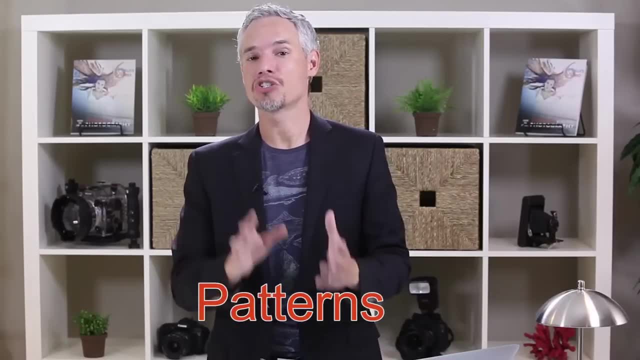 photo and especially draw their eye to the subject matter. Now let's talk about using patterns in pictures. Anytime you have a quantity of an object, you want to show that with your picture, but it can be hard, After all, if you have. 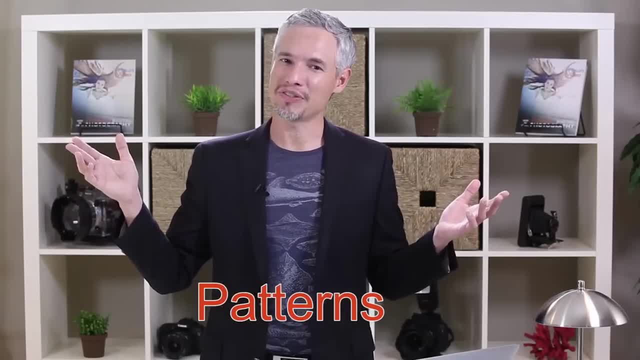 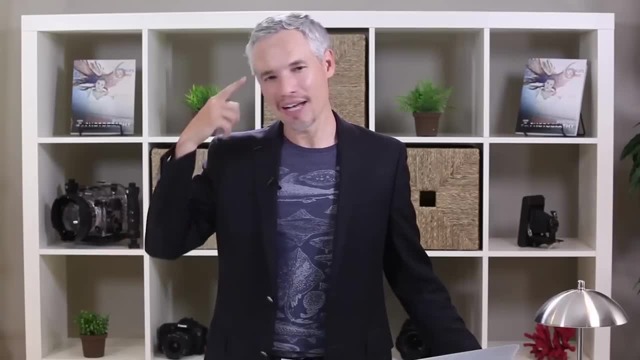 a hundred of something. well, you could step back, but you might not be able to see everything in it. If you use patterns and draw the pattern off the edges of the frame, the mind kind of pieces together that they go on forever. So this: 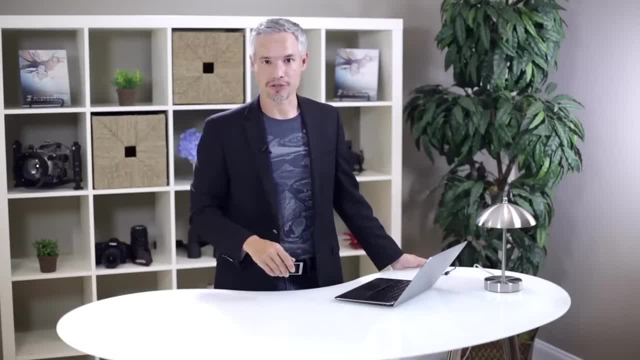 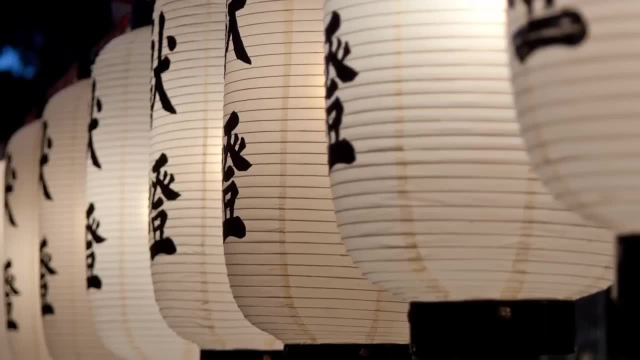 is a powerful compositional element. Let's look at some sample pictures. There's a long line of these lanterns in Tokyo, Japan, And I composed it, not trying to capture the edge of every lantern, but I let the lanterns go. 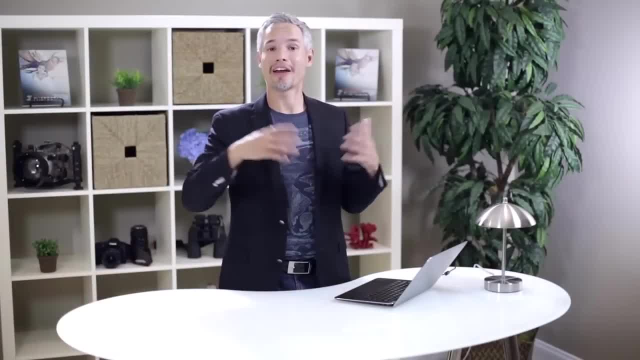 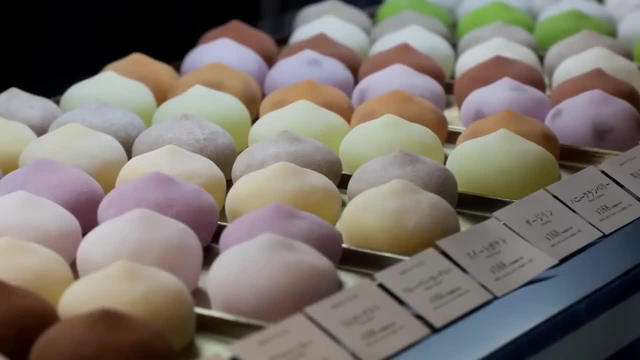 off the frame. This creates a pattern that goes on forever in the mind's eye. Oh, this is making me hungry. This is mochi ice cream also in Tokyo, Japan, And this storefront had just hundreds of these mochi ice cream. 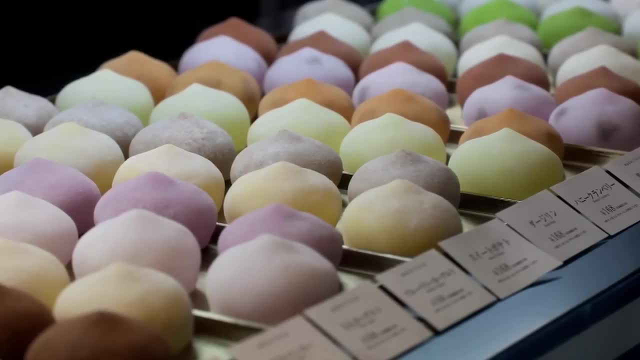 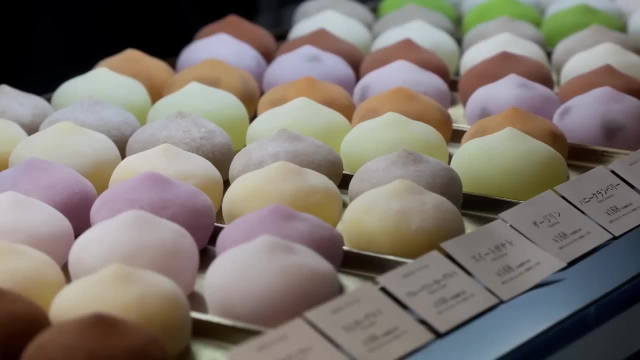 lined up. What I did was I composed the picture at an angle. This created a line from the bottom left to the upper right, And I let the pattern go off the edges of the frame. This gives you a sense that there are a large number of these mochi ice. 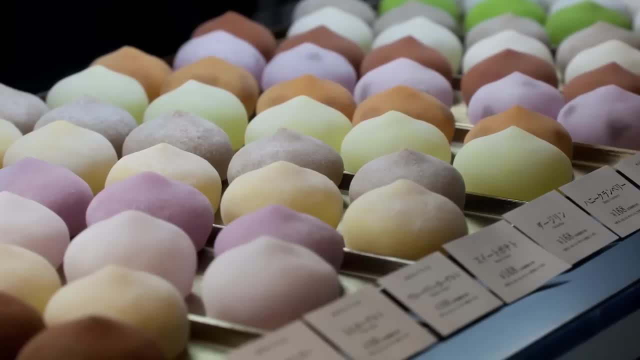 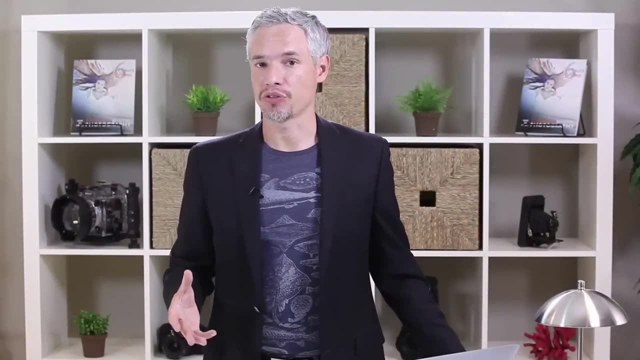 cream and it also fills the frame with the subject. By not shooting the mochi square, I created a much more interesting diagonal composition. Square compositions, as we'll learn later, are a very stately way to compose something. It's very traditional. 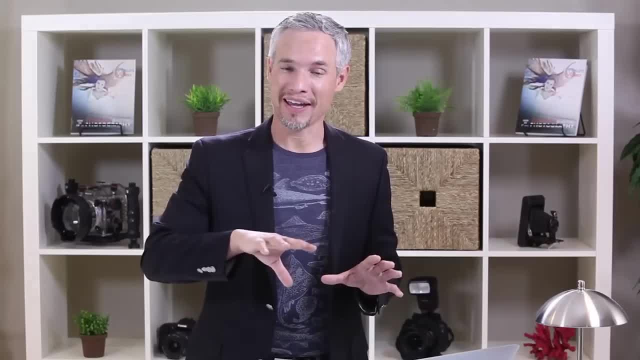 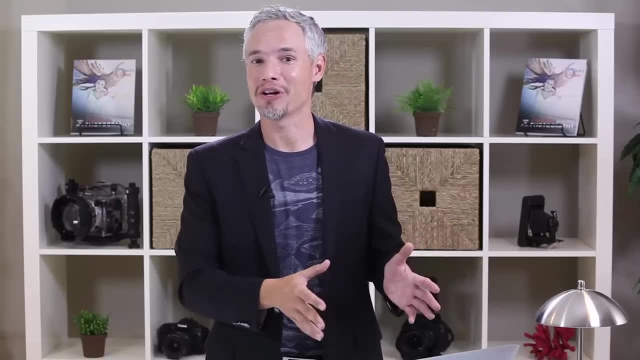 and powerful. But if you move your lines diagonally, as I have here, you end up with a much more dynamic, happy, friendly composition, And certainly with ice cream. I didn't want to convey stately, I wanted to convey fun. Let's look at another. 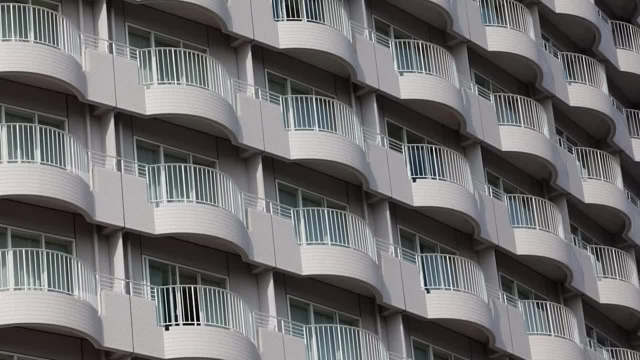 picture. This building is in a little island off of Tokyo And it's just a massive, massive apartment building And I wanted to capture that there seemed to be an unlimited number of balconies. It was easy: I just zoomed in and let the patterns go. 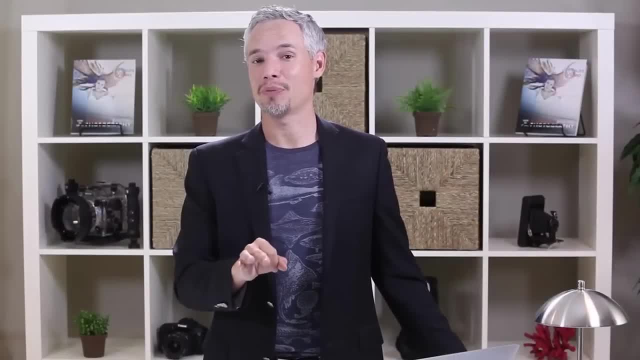 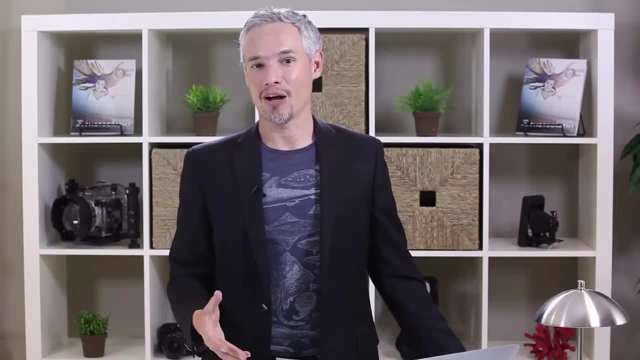 off the edges of the frame. Now, there's a lot of potential with this type of picture by simply including one element that doesn't quite fit in. Unfortunately, I didn't have that opportunity this day, But if there had been somebody leaning over one of the balconies? 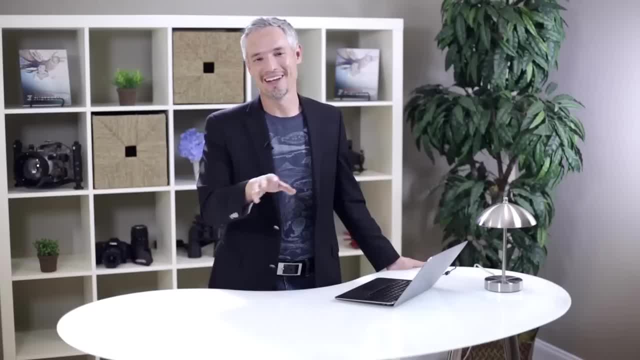 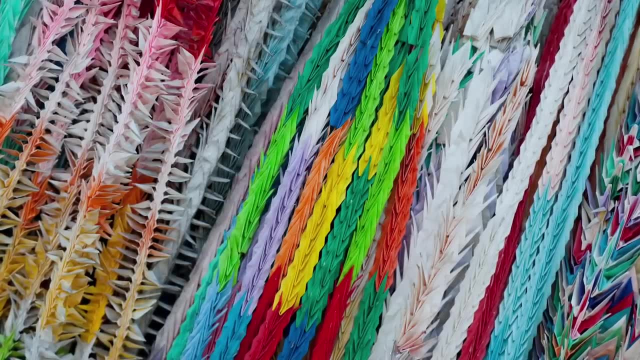 or a scarf that had been thrown over it, it would have been just perfect. I'm keeping my eye open. I'll get that shot eventually. Believe it or not, these are millions of tiny little origami swans. This is a Japanese prayer. 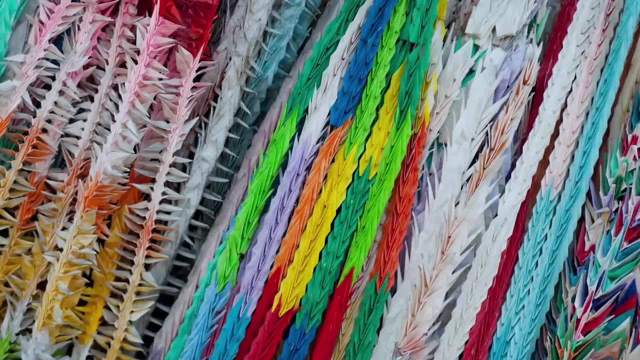 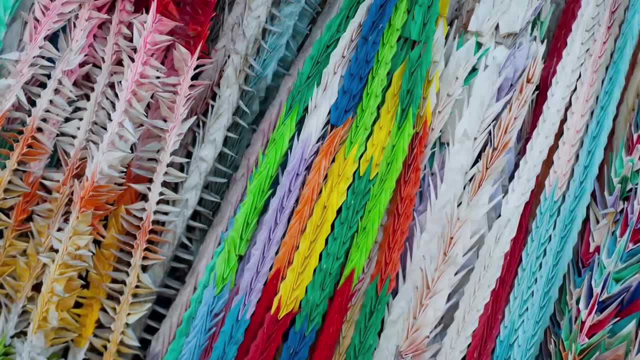 ritual And it was just a beautiful scene. The way I captured it was to zoom in tight so that they went off the edges of the frame And I just created a picture that's filled with color and texture and lines And, as you can see it, 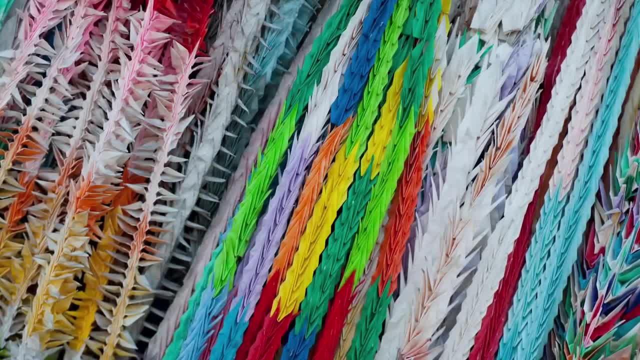 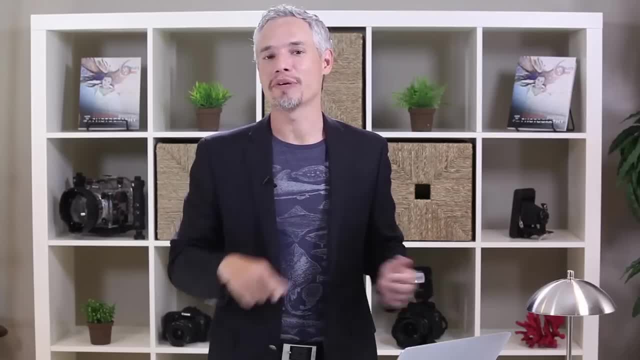 would have been very easy for me to rotate the camera so that the lines would be completely vertical or horizontal in the frame, But instead I decided to go for a slight but deliberate diagonal line- One thing you want to be careful of when using lines. 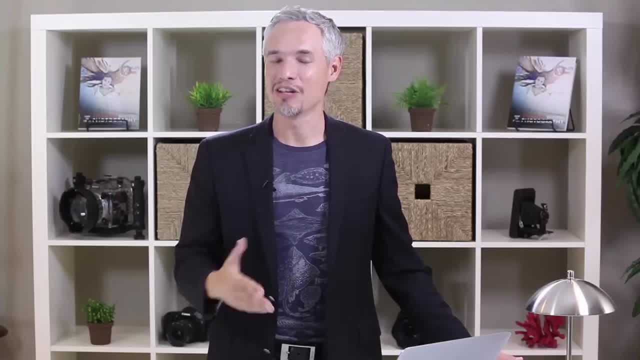 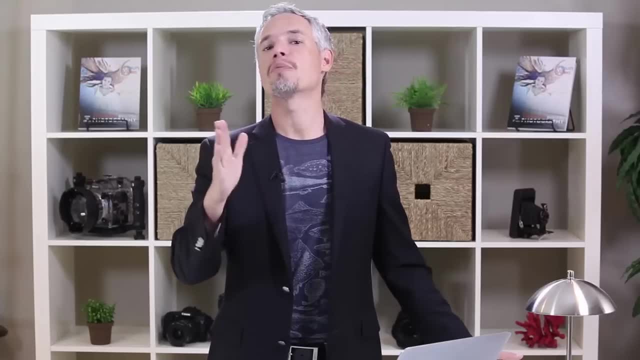 is to make sure that the angle is intentional. You don't want to be just slightly off horizontal or slightly off vertical, You want to be deliberately off horizontal or vertical. So think between 30 degrees and 45 degrees off to make it look nice. The electronic: 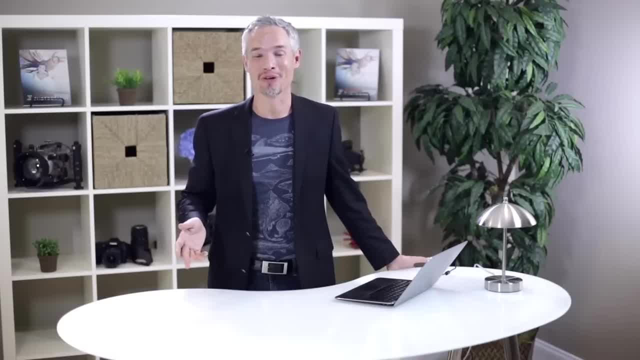 district in Japan is just a nerd's dream come true. They had parts for everything there: Literally billions of tiny little parts in vendor after vendor after vendor. It seemed to go on forever. I thought the best way to capture that would be to zoom in. 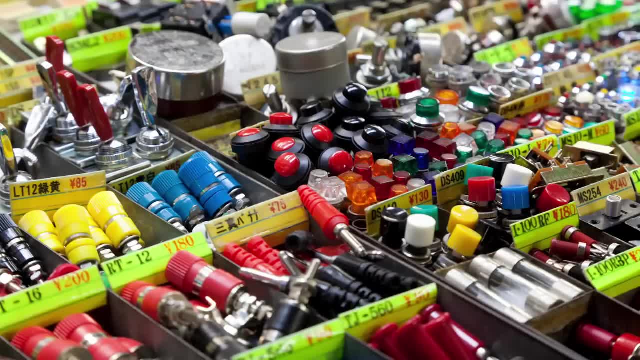 and let the parts go off the edges of the frame. As you can see, I once again threw in about a 30 degree angle there, which makes it a much more compelling composition than if I had shot it completely straight. I could have shot wider. 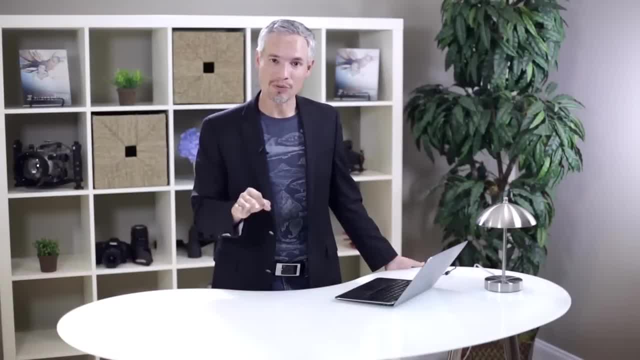 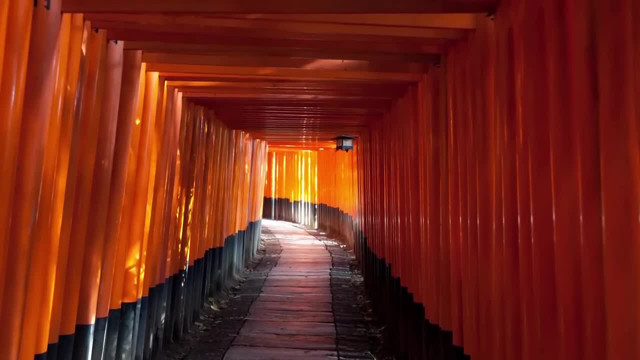 certainly, but I wanted to zoom in tight enough that the viewer could easily see what the subject matter was. Tiny little electronic parts. These are torii gates. in Kyoto, Japan, They have thousands of these torii gates on a particular mountain. Just the massive quantity of them. 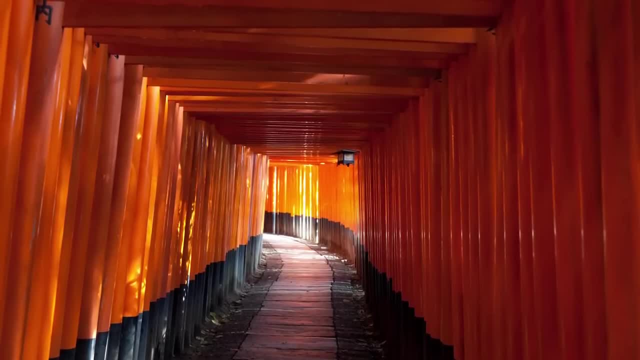 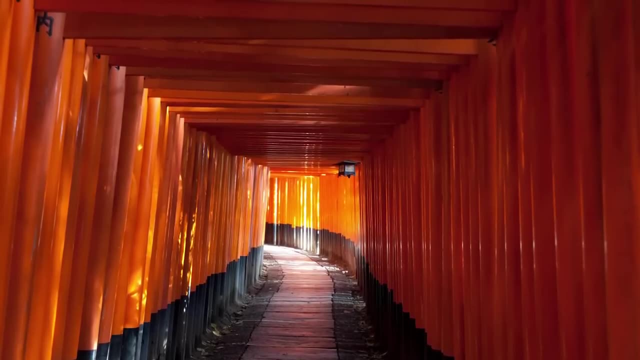 is amazing. It's really a remarkable sight and I recommend anybody visit it, But capturing them is almost impossible because they're winding through these mountains and there's no way that you can simply take a picture of all of them. So what I decided to do was to 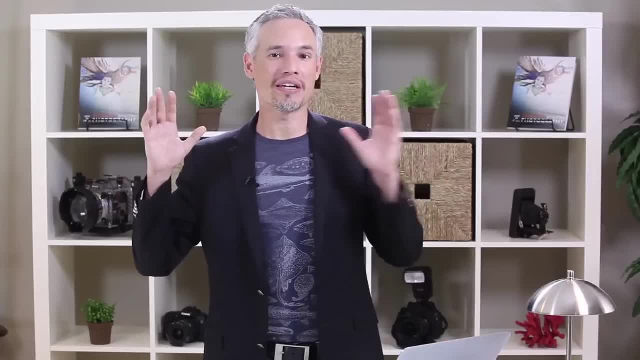 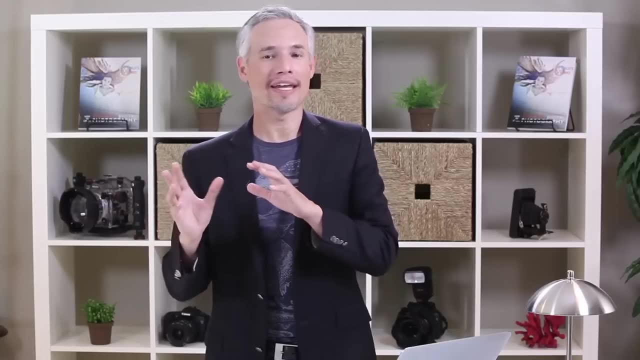 find a framing where I could show the torii gates going off into the distance. So here the pattern doesn't go off the frame, Instead, because it's curving, it actually goes off into the distance in the center of the frame, leading the eye from the 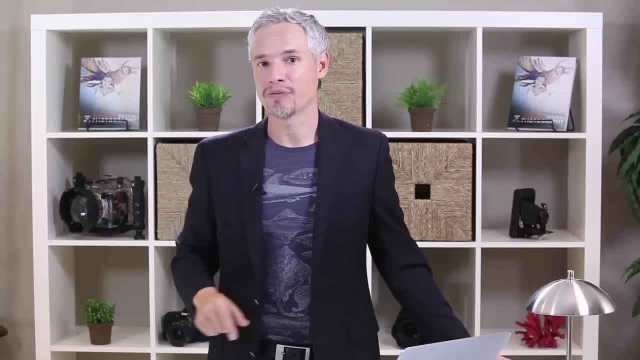 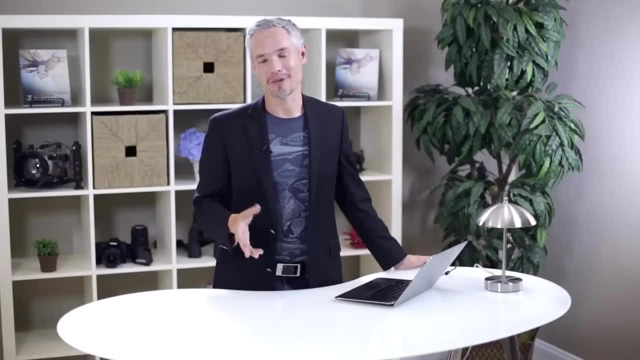 outside to the center of the frame. Now, this would have been an even better composition if I'd put a person in the frame, And in fact I did do that, Unfortunately, because I didn't have a model release from them. there was a serious language. 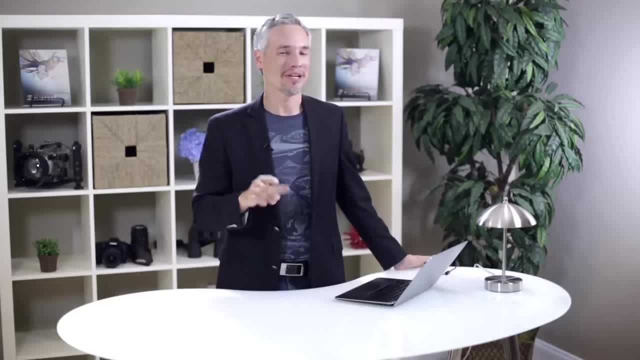 barrier. I can't show you that picture, but keep that in mind. You can use patterns and then throw something that's not part of the pattern into the picture to make it even more compelling. Now let's talk about framing a picture And I'm not talking about making a print. 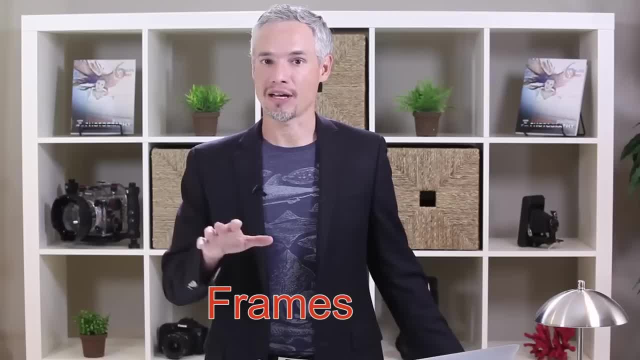 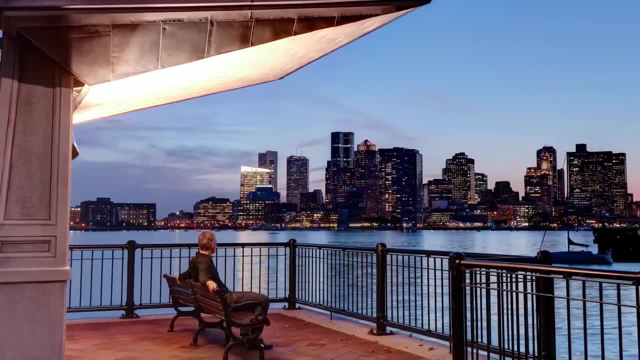 and then sticking it in a frame. I'm talking about using framing as a compositional element. Let's look at some examples. Here's a picture that Chelsea took of me in Boston. Now, this was a very deliberate picture. We were taking pictures of the skyline, but we 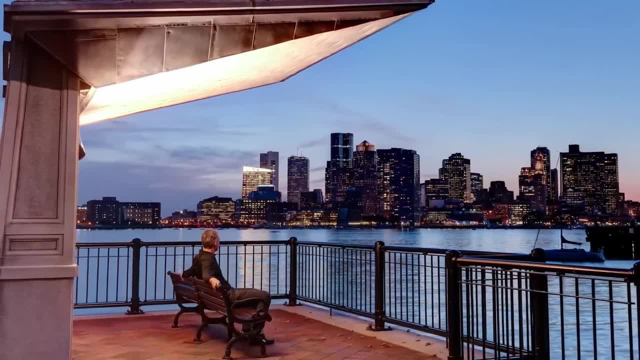 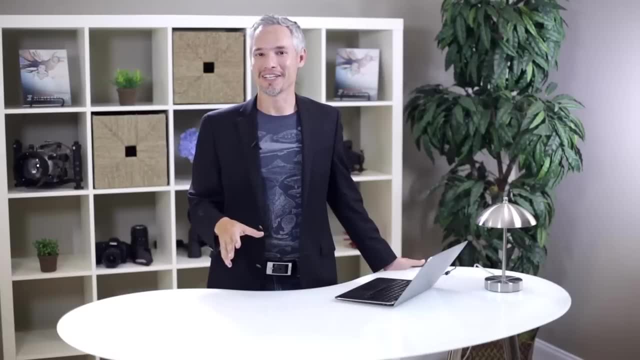 felt like it needed some extra element, And one of my favorite things to do in that situation is to grab a person, whoever I'm with, and put them in the frame as a model. So you can see, my job was pretty easy. I just had to sit on. 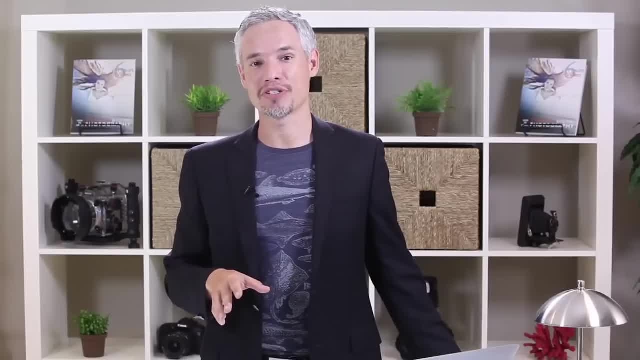 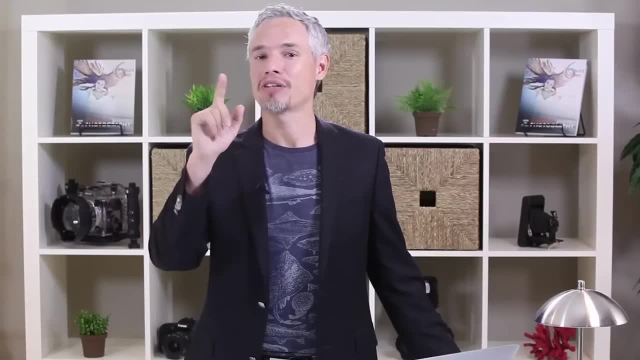 the bench and look at the skyline, But the nice thing about Chelsea's composition is that I'm probably the first thing that you see in the picture, but then your eyes automatically follow the subject's eyes. So because I'm looking off into the distance, your 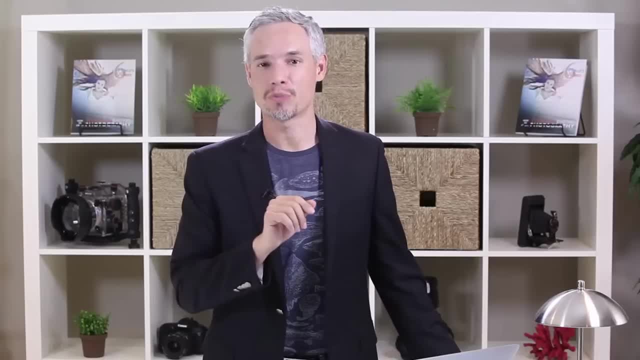 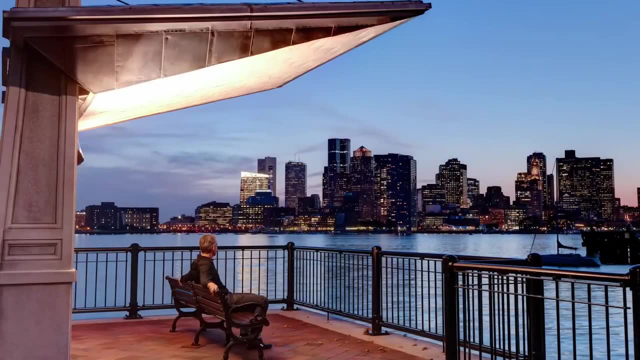 eye then goes and looks at the skyline. But the reason I'm showing this picture here is the use of framing. You can see that Chelsea framed me with that light that goes behind me and over me. I'm further framed by the fencing around me. 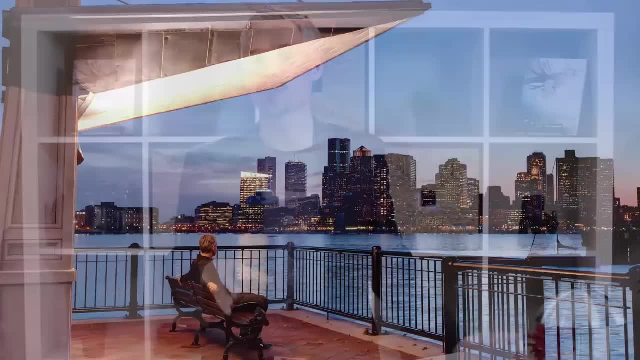 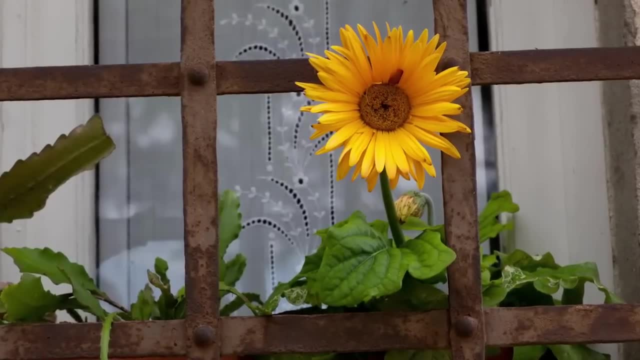 This helps to tie the entire composition together and provide a sense of perspective. Let's look at another example. Flower boxes are everywhere, but I like this picture because of the rusted frame. It's also really nice that the flower is poking through the frame, because that adds. 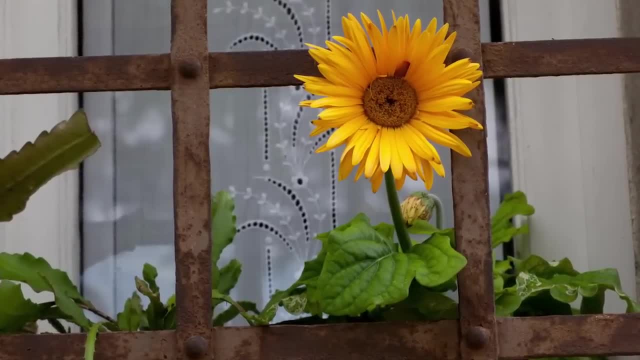 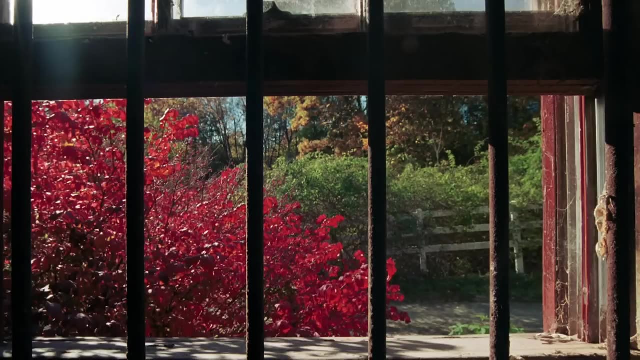 some depth to it. Without the frame, this simply wouldn't be as interesting a picture. Here's an example of using a window frame to show perspective. Now, these bushes and the light were pretty and I could have gone outside and taken the same picture, But by 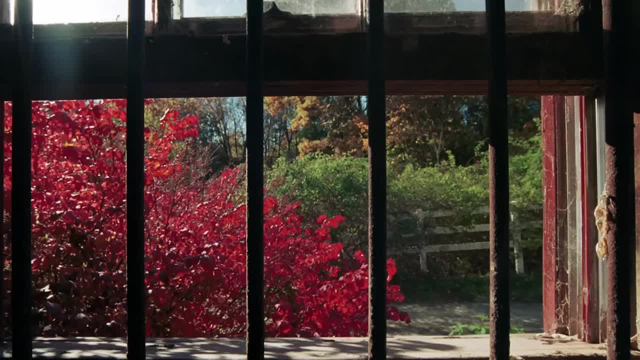 including the frame and the bars in the photo. it gives the viewer a sense of both what's outside and what's inside. They almost feel like they're inside this kind of spider web covered barn, So keep that in mind when taking pictures through windows. Sometimes you just want to take a picture. 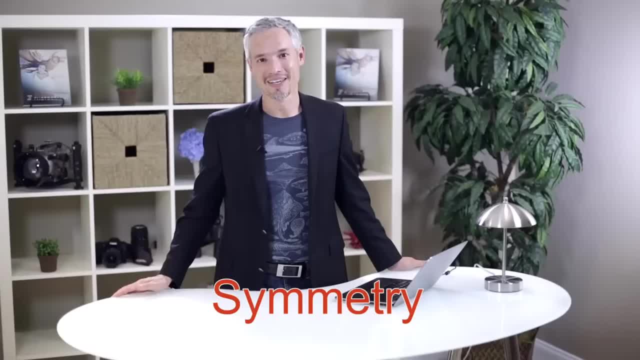 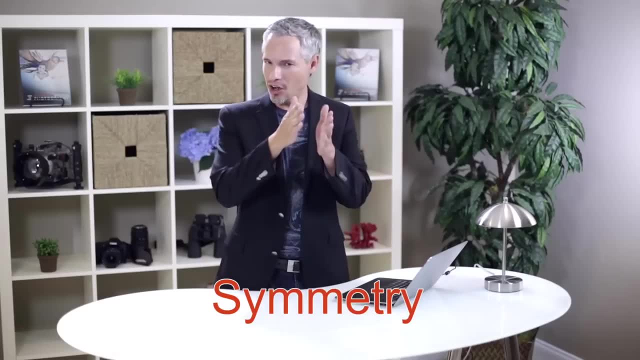 through the window, but sometimes you might want to include the window frame in there too. Now let's talk about using symmetry in a picture. Anytime there's something reflected or some subject that is almost perfectly mirrored from one side to the other, you can use 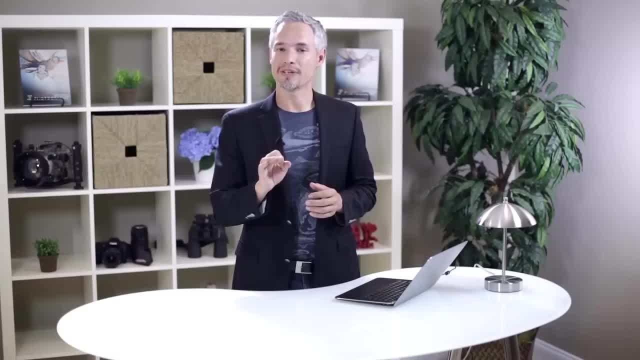 symmetry. Now, when using symmetry, it's really important to be very precise about it. If you're going for something mirrored horizontally, you want to make sure that that center line is perfectly in your frame and that you're not a little bit off to the left. 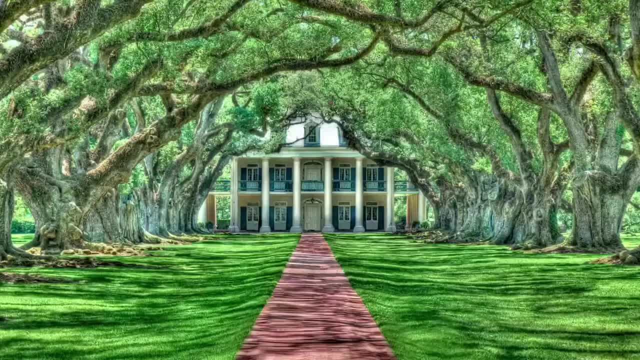 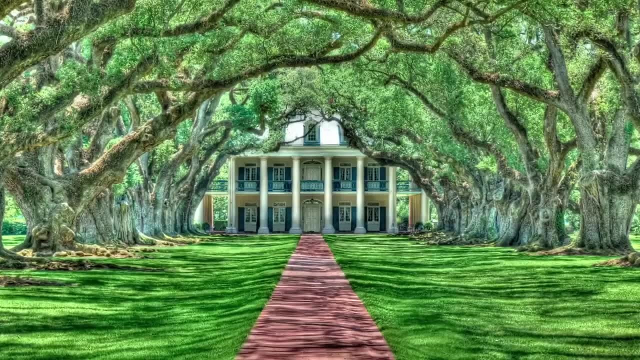 or a little bit off to the right. You want to be really level with it too. This picture is Oak Alley Plantation in Louisiana, and it's just a beautiful sight, And I really spent a lot of time finding the right composition for this picture. Now, one of the nice things. 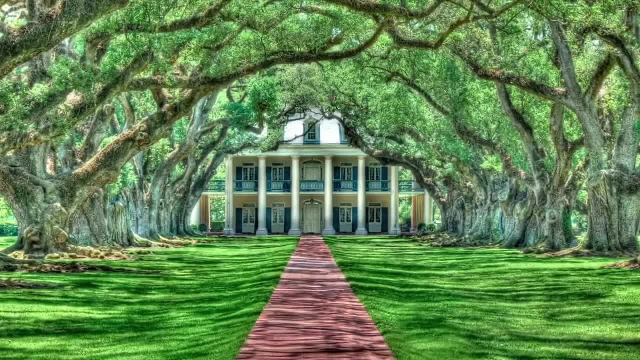 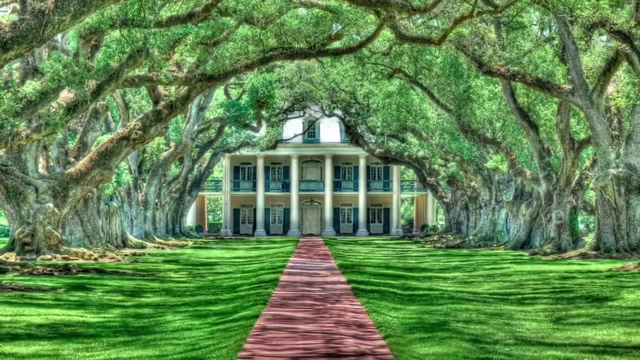 about Oak Alley is that it's a very powerful plantation. It's very stately, with lots of vertical lines in those pillars, And I thought the best way to convey that was by composing a square composition. So rather than showing some depth- which I'll discuss later- 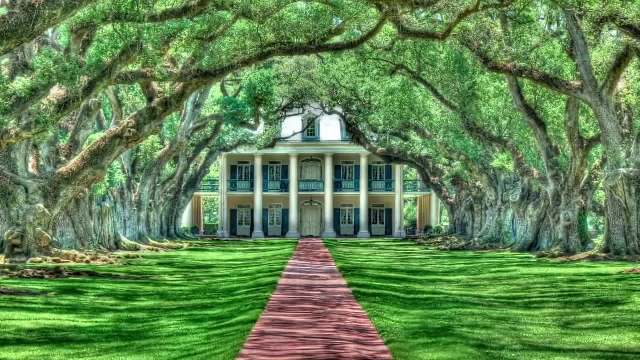 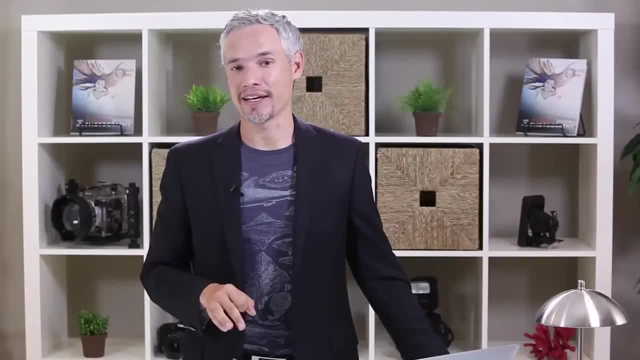 I centered myself on the building and made it look very square. I also used this walkway that was in the middle of it and put myself precisely in the center. Now you might also notice that the color and the lighting here is pretty dramatic. That's because this is a high dynamic. 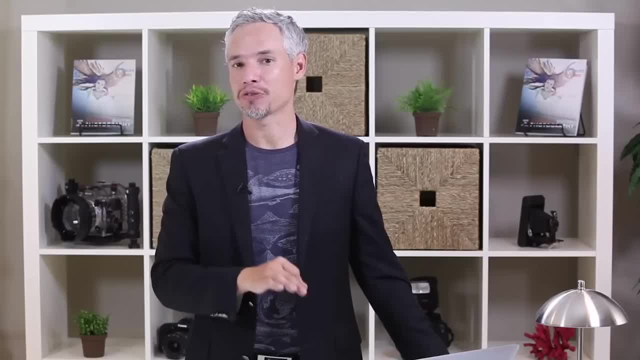 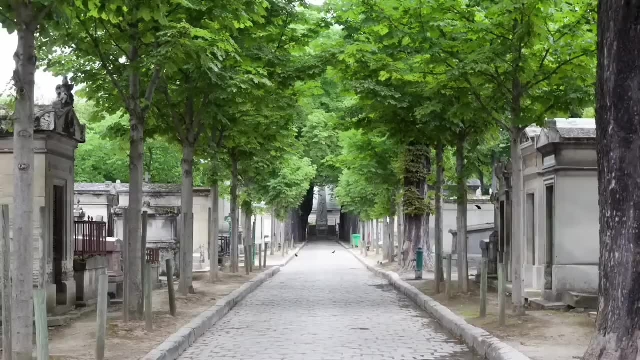 range photo, an HDR photo. I took three separate pictures, bracketed and then merged them together using special software. I'll cover that in a separate lesson, so check that out. Here's another very similar example of symmetry: Anytime there's a walkway surrounded by trees. 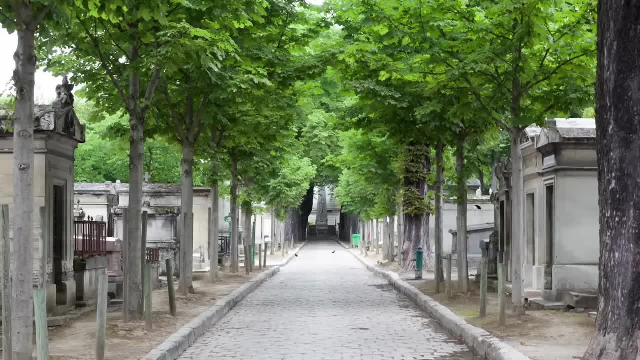 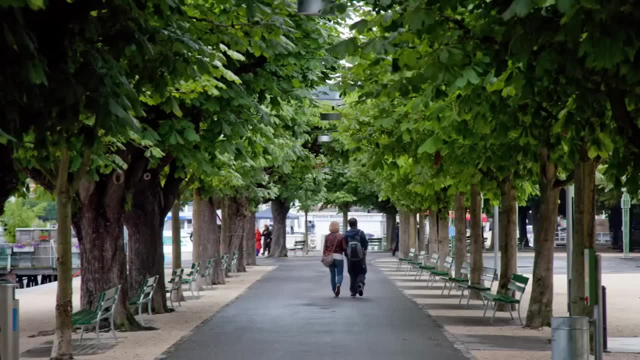 this is an excellent opportunity to use symmetry. Let's look at another similar shot. Here we can see two people walking down a sidewalk. If I had been off to the side one way or another, it would be a much less interesting shot. But 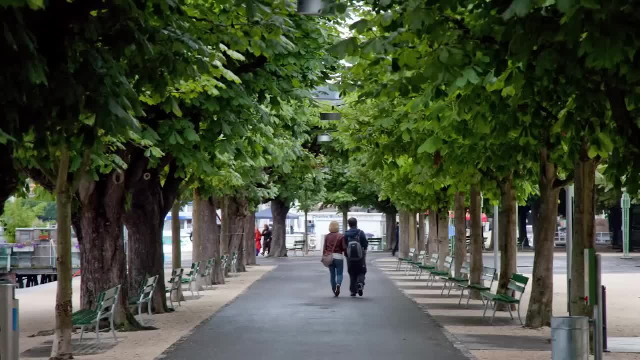 because I went ahead and used symmetry. this shot feels nicely balanced. Now notice that the people aren't directly in the middle, And that's okay, because often when you're using symmetry it's good to throw in one element. that's a little off balance. It makes the photo. 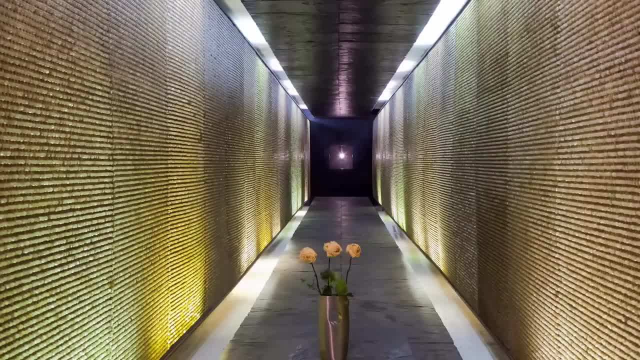 more interesting. Here's a World War II memorial in Paris, And I thought the best way to convey the solemn and serious tone of this memorial was to shoot it symmetrical and allow all those lines to converge on the center point. Those flowers are the only thing that breaks. 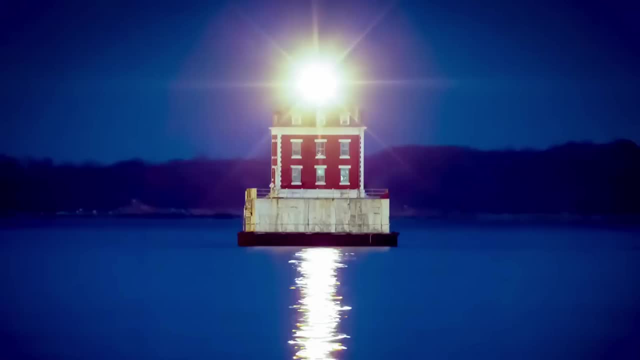 up the symmetry which draws the eye right to them. This is the lighthouse in New London, Connecticut, very close to my hometown, And I composed this shot several different ways. I tried it with the rule of thirds, I even tried it with some depth. But what I 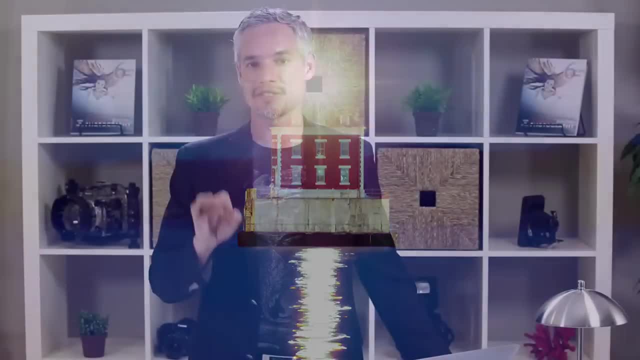 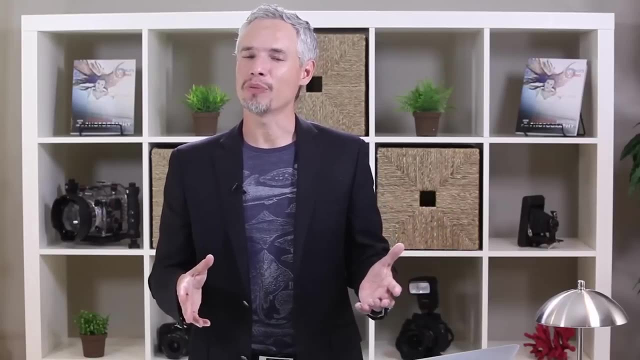 thought worked best was shooting it square and using symmetry. Now I actually used this shot in two different ways. I have a horizontal shot that I'm showing you here because I'm showing a video, But my favorite composition is actually a more vertical shot. 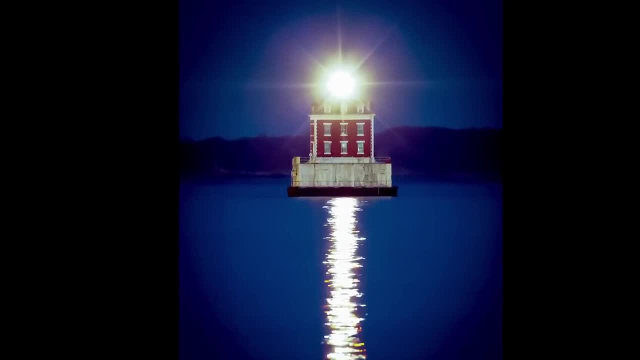 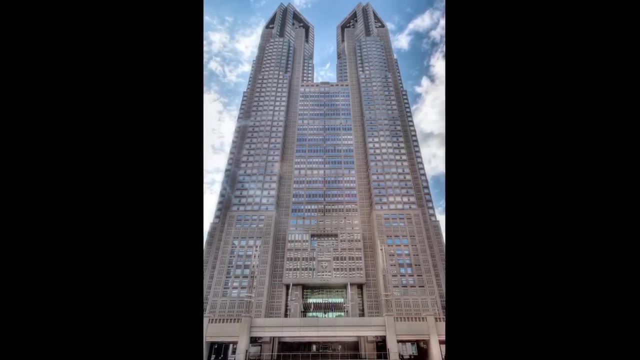 But symmetry worked equally well in both the horizontal and the vertical position of the camera. This building in Tokyo was otherwise unremarkable, but I thought it was so perfectly symmetrical that it would make a perfect picture. So what I had to do was to move myself. 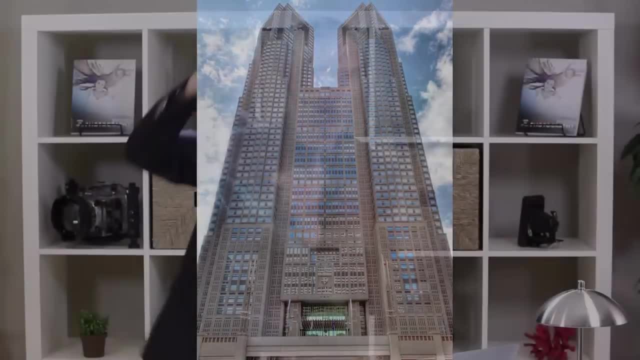 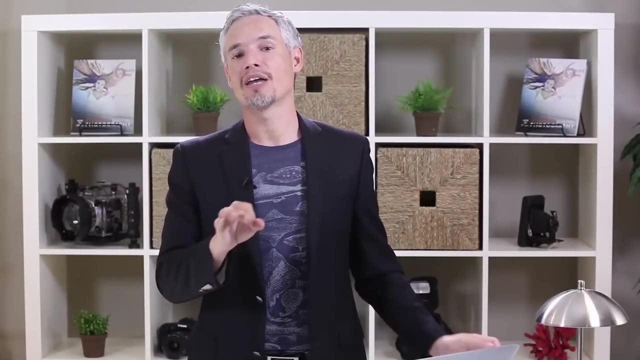 at the exact center line of the building and then angle my camera up a little bit. If I bent off to one side or another, the composition simply wouldn't have worked. So again, whenever you're using symmetry, be sure to align yourself, really. 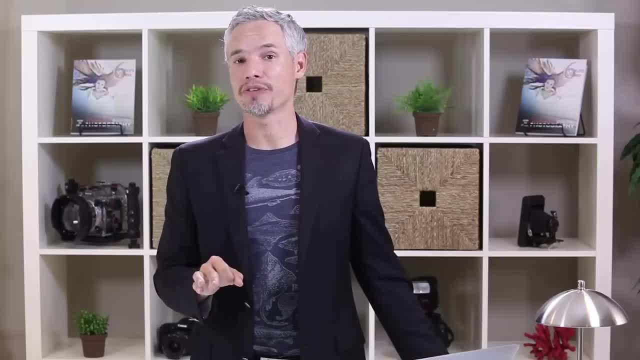 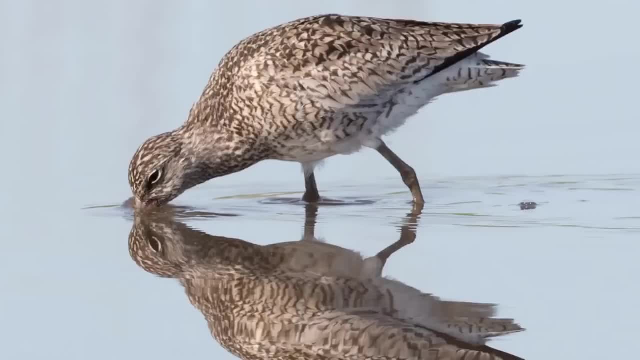 carefully so that that symmetry is perfect. Anytime you see a reflection, and particularly around water, you want to think about using symmetry. Here, this bird is taking a drink of water, and I decided to compose the picture to include the bird's reflection because 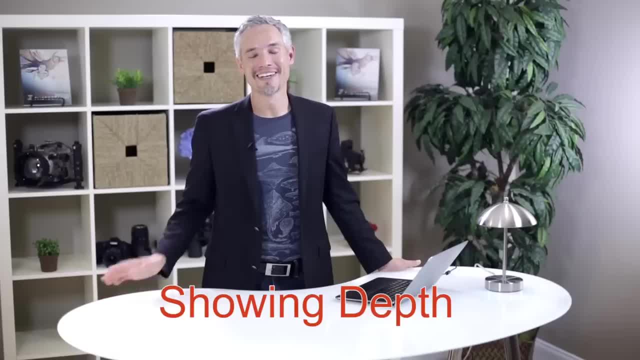 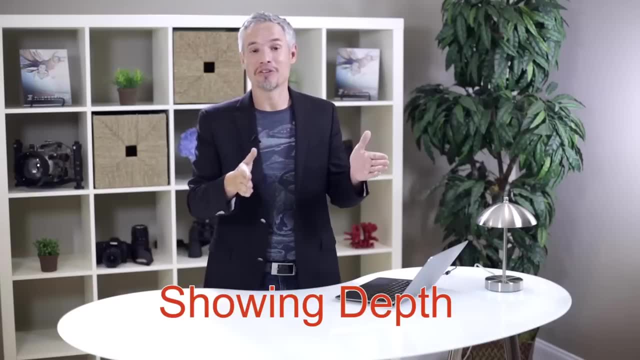 this allowed me to use symmetry as a compositional element. Now let's talk about showing depth. I've discussed it a little bit already. If you shoot something completely square on, well, you're not showing any depth, And that's a good way to make something seem. 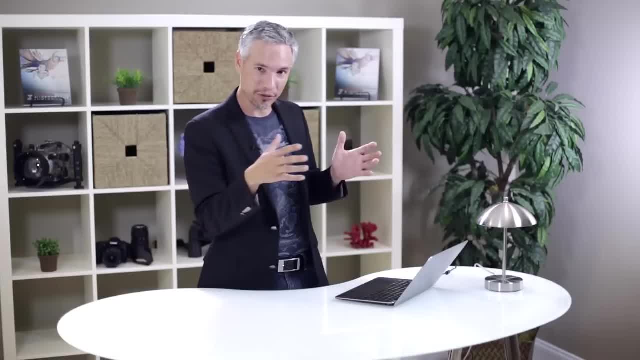 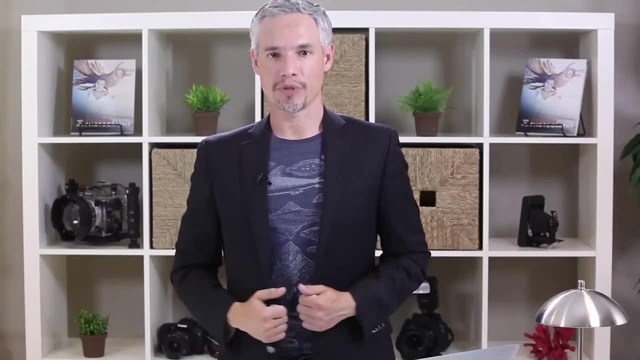 large and powerful and important. If you move off-kilter a little bit, well, it seems more casual and fun. This works really well in portraiture. So if I stand completely straight and square to the camera and face you like this, I seem. 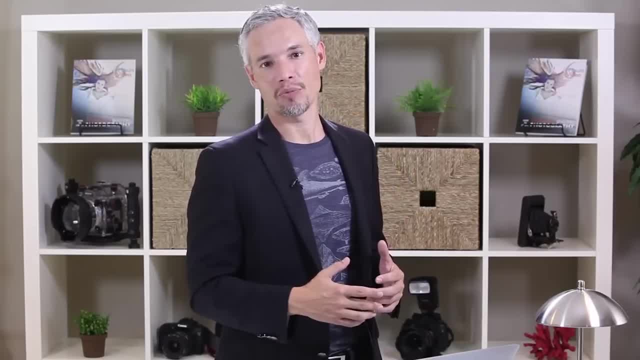 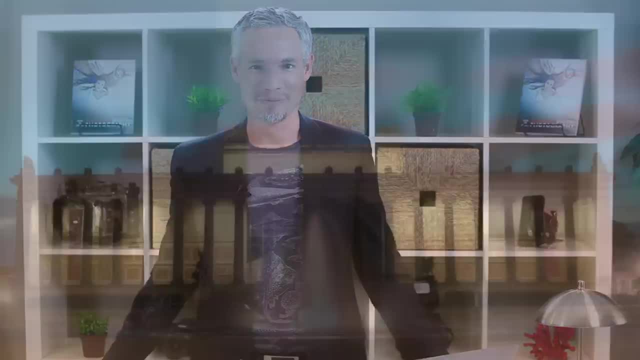 very serious. If I turn my shoulders and maybe tilt my head a little bit, I'm showing a lot more depth in the picture and the picture comes across much more casually. Let's look at some example photos. Here's a beautiful library in Berlin and you can see this photo doesn't. 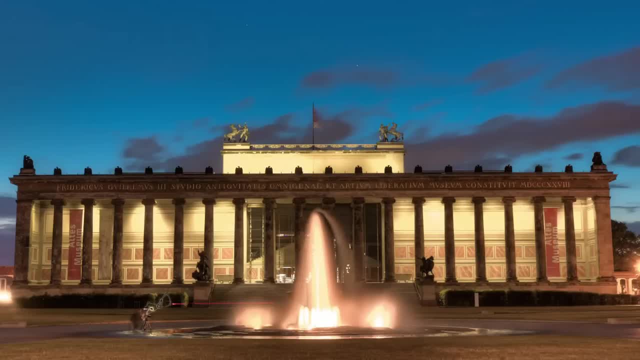 have any depth. I stood completely square to the building. The building is very serious and important. It's a former Nazi headquarters and for that reason I thought the square composition would work best. But let's also look at a shot of it with some depth. 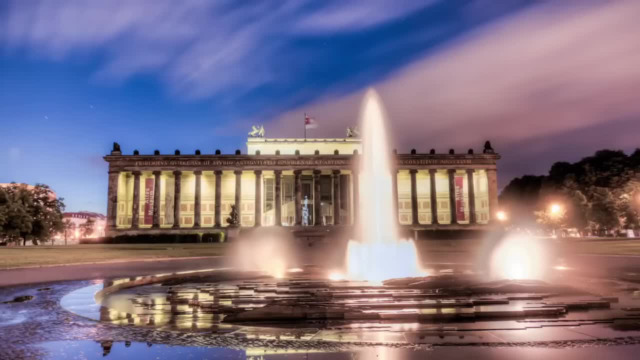 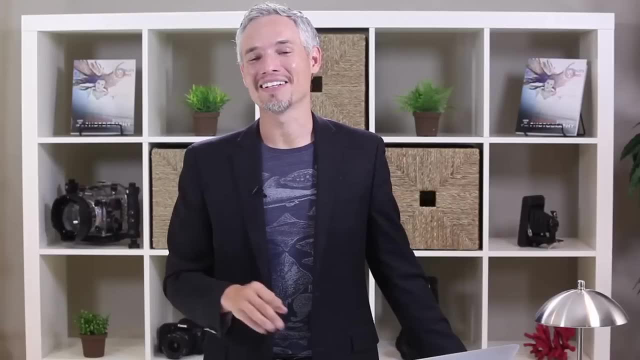 As you can see, moving a little bit off-center shows the building in a very different tone. It now seems much more interesting and less serious. Now let's head to the Niven district in Copenhagen, Denmark, my absolute favorite part of Copenhagen. 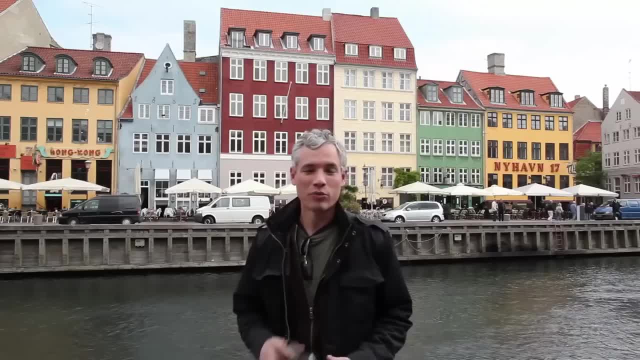 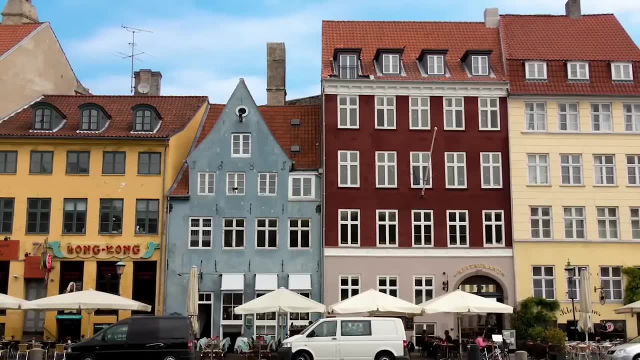 to experiment with depth in the real world. When most people want to capture a building, they tend to shoot it straight on, like they do with this, And that's a lovely picture of a beautiful place, but it doesn't have any depth to it. 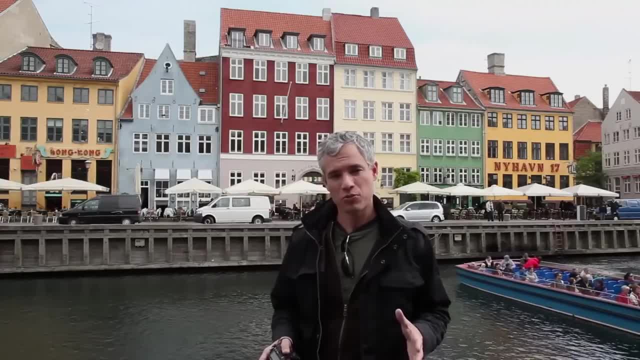 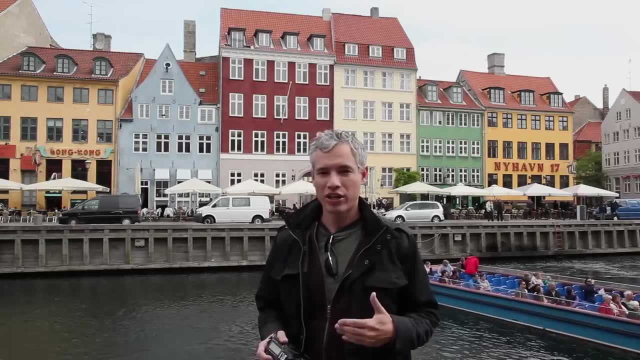 It's a completely two-dimensional picture. One of the things you should strive for when composing pictures is to provide a three-dimensional scene. One way to do that is to show something in the foreground. So I can do that easily here by zooming out and showing a bit of the water. 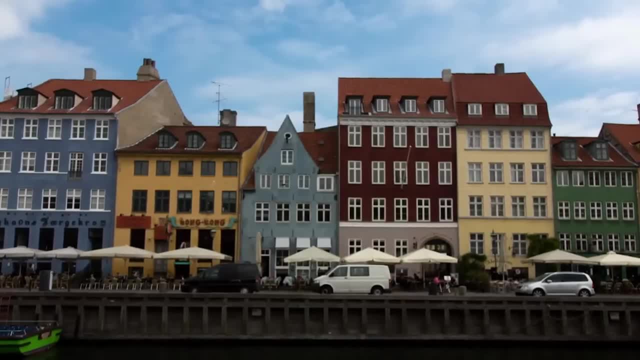 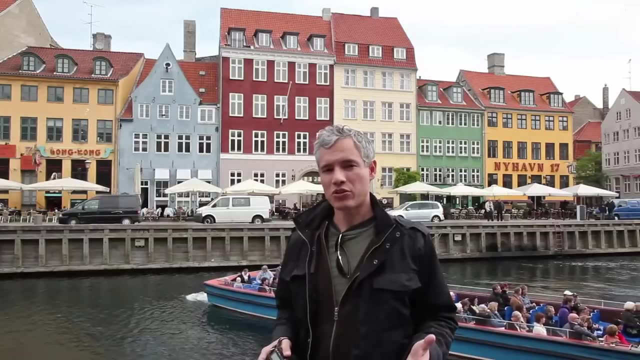 that's in the foreground. So that picture is much more interesting and it shows much more of the area, because it shows the water and the boats as well as just the buildings. But you can make the picture even more interesting by turning at an angle to the subject. 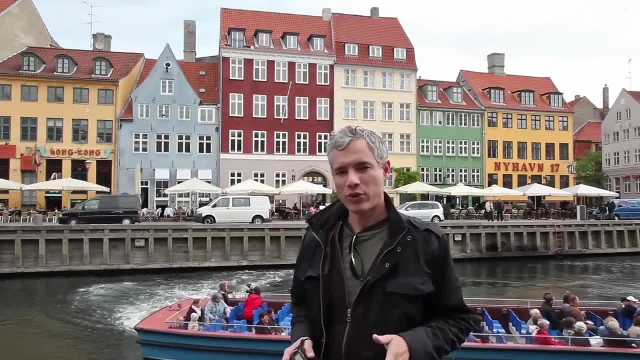 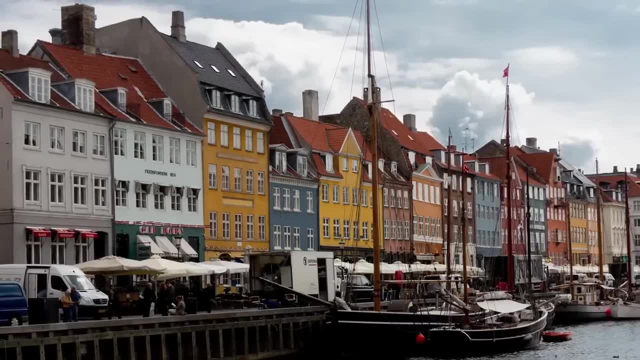 and showing some depth. So I'll take another picture and look down the waterway. Now, as you can see, that picture shows much more of the scene and it's also much more interesting to the viewer because it has depth to it, both a foreground and a background. 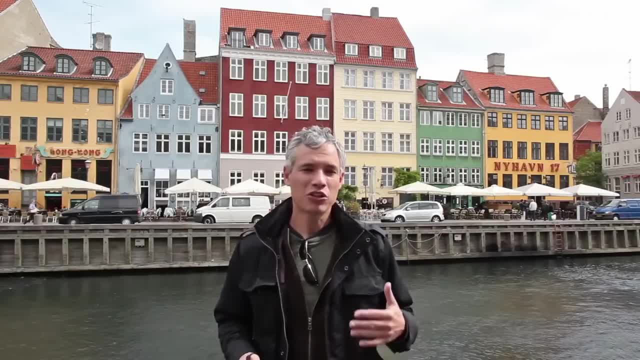 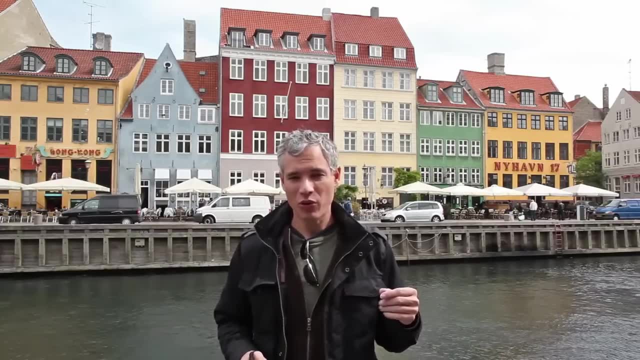 When you shoot a three-dimensional picture like that, however, you add an additional challenge, which is getting everything in focus. The depth of field is the part of the picture that's in focus and it's always in a plane parallel to your camera's sensor. 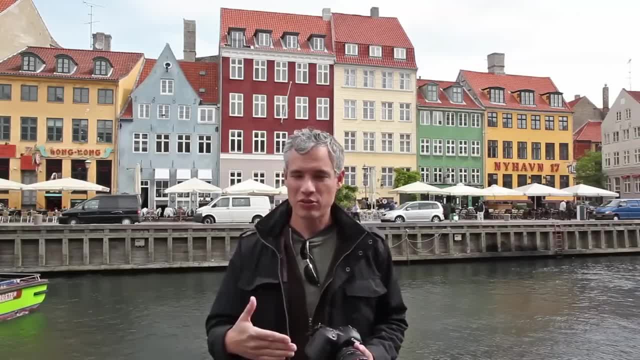 So if you have depth, in a picture like that, only the part you focus on is going to be truly in focus. The rest is going to be a little out of focus. You can fix that by using a higher f-stop number, A higher 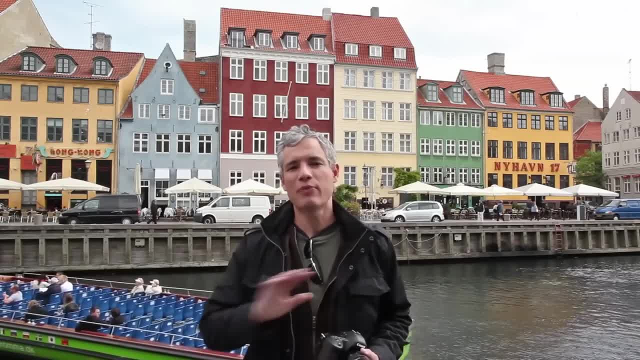 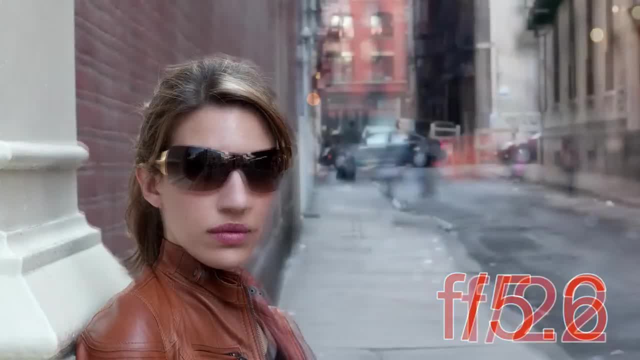 f-stop number increases your depth of field and makes the background more in focus. Remember, the f-stop number controls your background sharpness. So for higher background sharpness, you want a higher f-stop number. You want to blur the background: lower background. 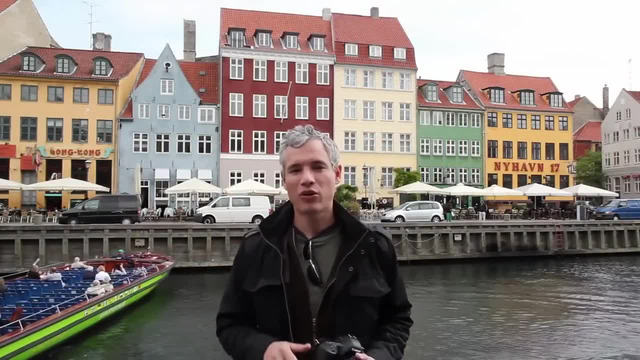 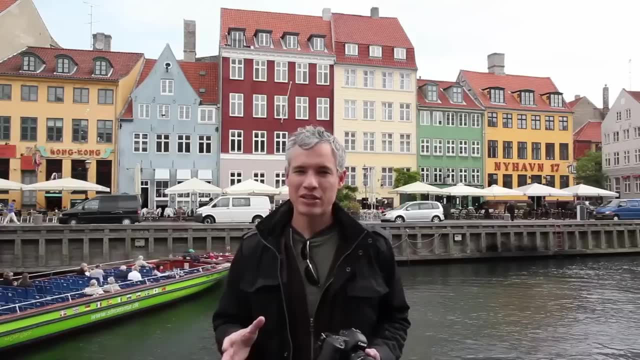 sharpness, lower f-stop number. So let's talk about incorporating foreground elements. to show even more depth, We'll move to a different location so we can show a couple of elements in the foreground of this same scene and see how that impacts the composition. 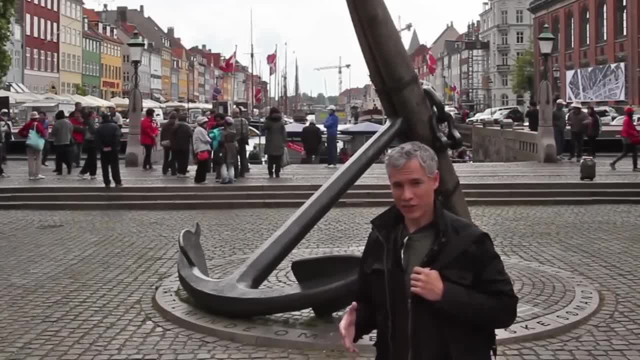 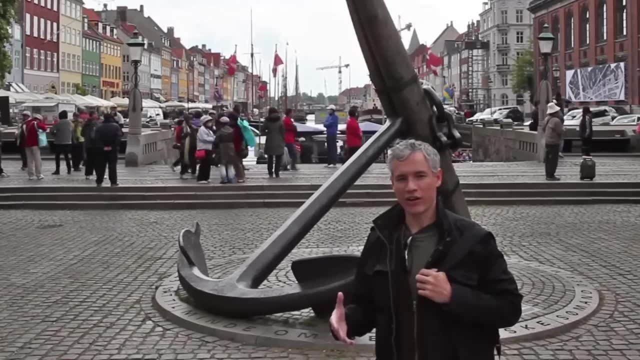 So here I found an interesting foreground element, which is this anchor. It's kind of the symbol of the area, And including it in the foreground is going to increase the depth, provide more context to the area and generally make the picture much more interesting. So let's take a couple of pictures. 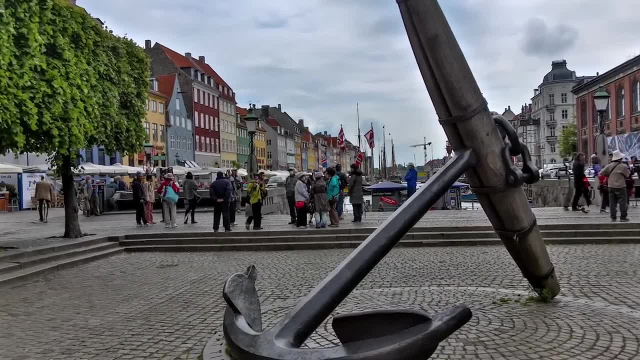 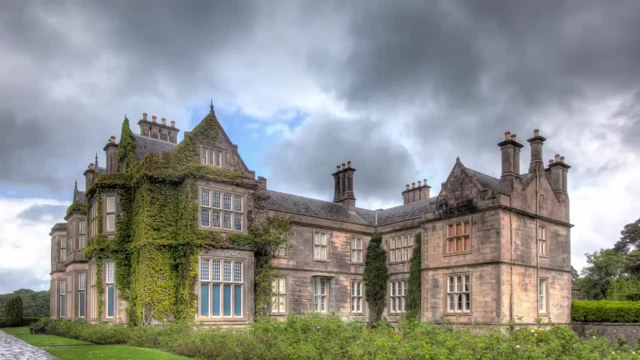 and see what it looks like. So, as you can see, that provides a much more interesting picture And it shows the area better. This gorgeous building in the Irish countryside doesn't really lend itself well to depth. This is a nice shot, but wait until you see the square. 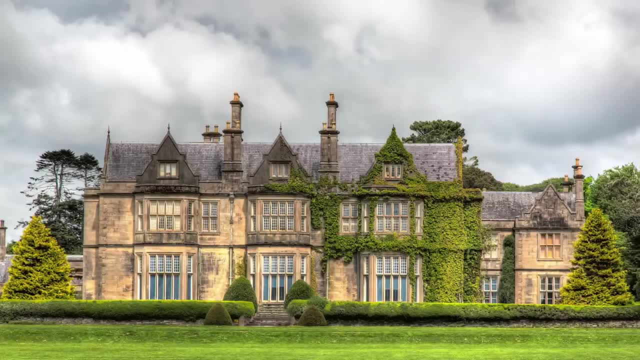 composition. This photo better conveys the real feeling that you get around this building because it was just so proper and stately and formal. Showing this picture with depth doesn't really convey it. I needed to shoot this picture square on Speaking of Ireland. 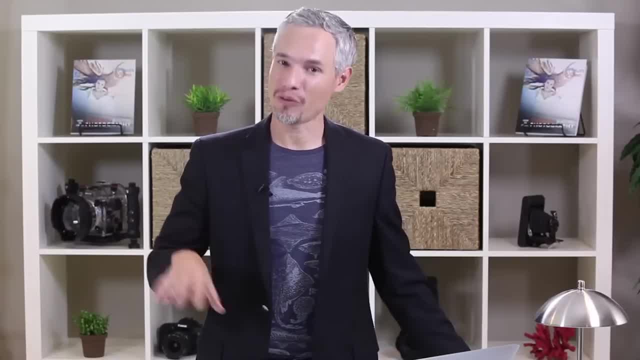 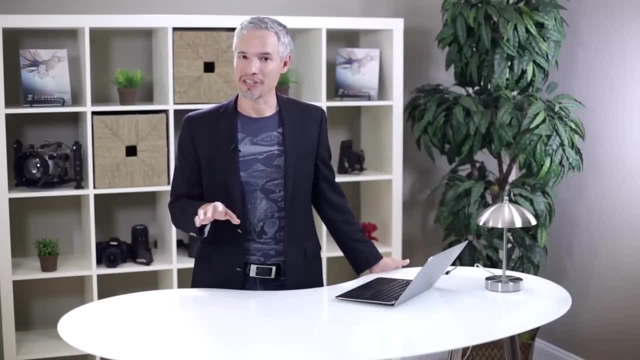 let's head over to Dublin to talk about taking travel pictures and architecture pictures. Especially in older towns like those in Europe, you might see a composition that your camera isn't able to capture because your lens isn't wide angle enough. I think it's really important. 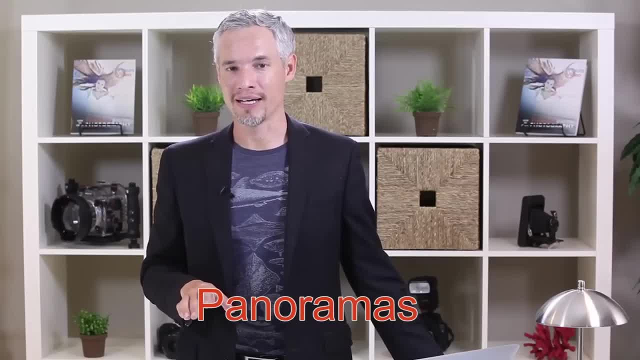 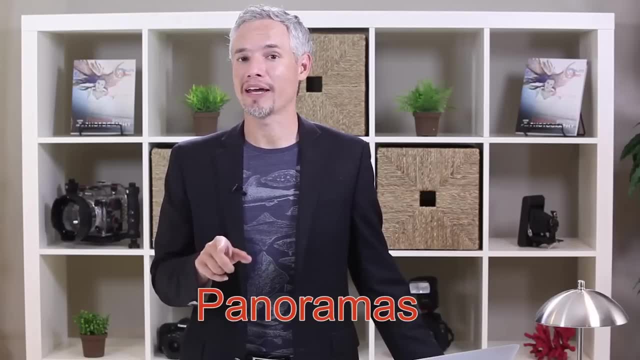 to master the panorama technique before taking a trip like that, And in fact it might save you a thousand bucks on that wide angle lens because you'll be able to use your conventional lens to get super wide angle and high megapixel pictures. I had a similar problem. 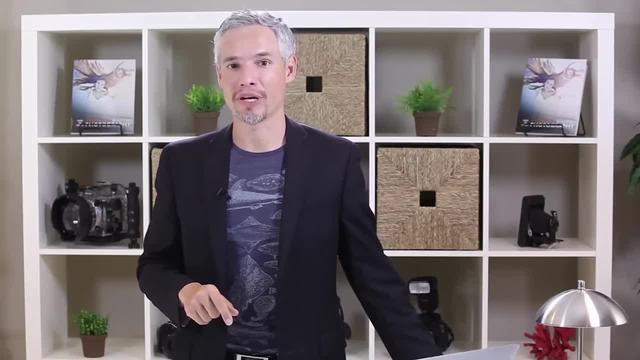 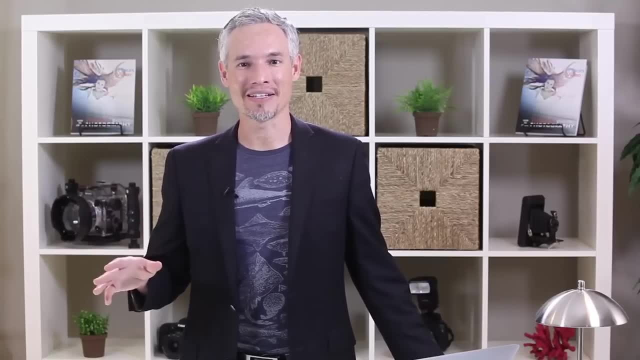 to that when I was in Tivoli, a small part of Copenhagen, Denmark, And there was this beautiful hotel that looked like a palace and it was all lit up at night And I really desperately wanted a picture of it. but there was a massive 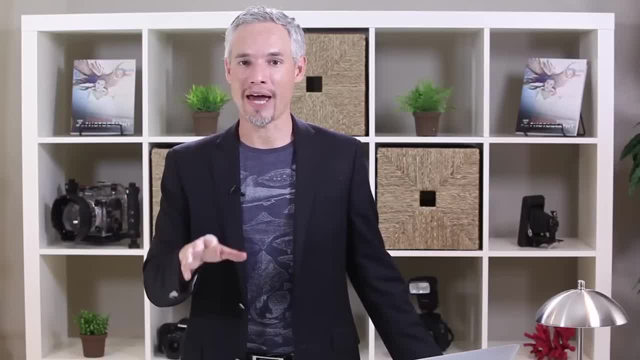 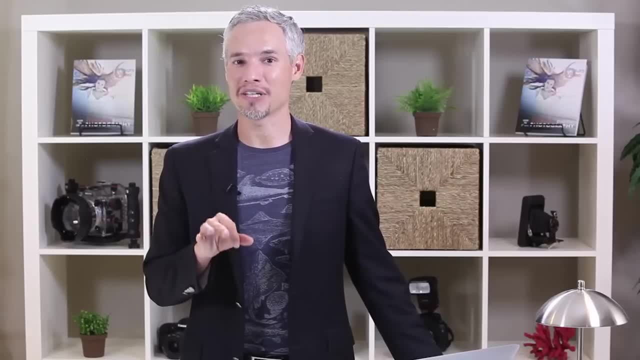 crowd behind me and I simply couldn't take another step back, and I didn't have a wide enough angle lens with me. So you know what I did: I took three shots of the building and then blended them together. So let's look at those. 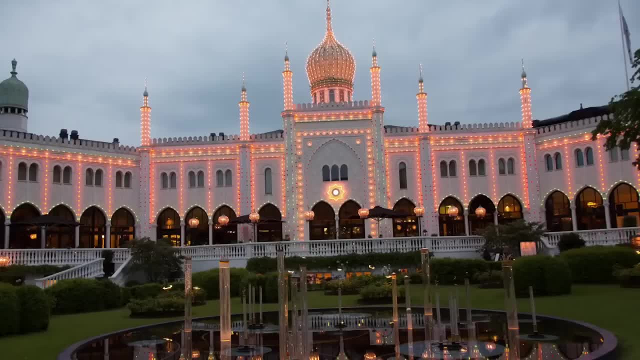 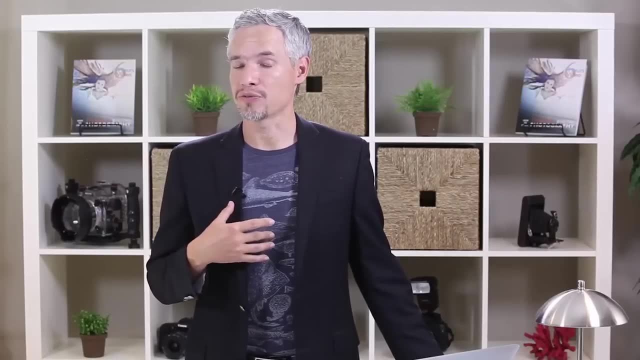 three shots. Here's a shot of the left side of the building, the middle of the building and then the right side of the building. All I had to do was to bring those three pictures into the software I use for panoramas: Microsoft. 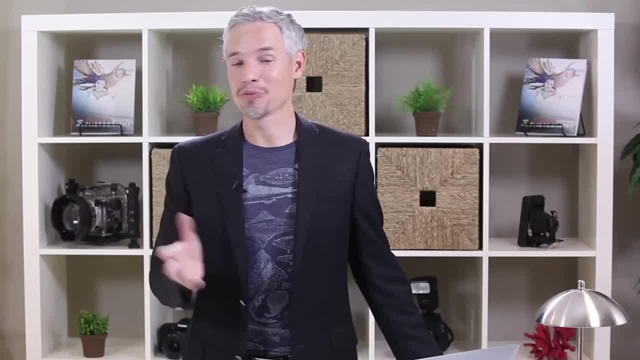 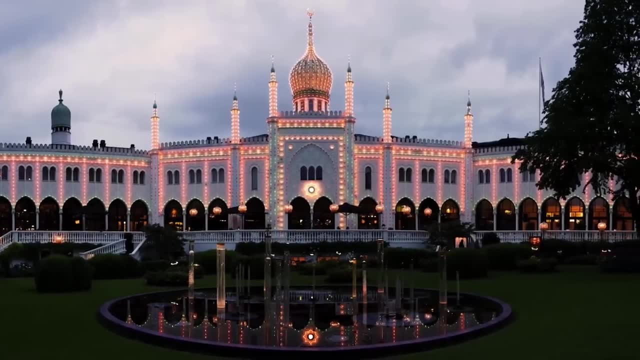 Ice, and it blended them together for me automatically. It really only took a few seconds. I'll demonstrate how to use that in just a moment. Here's what the final result looked like. Now, that's certainly much better than either of the first. 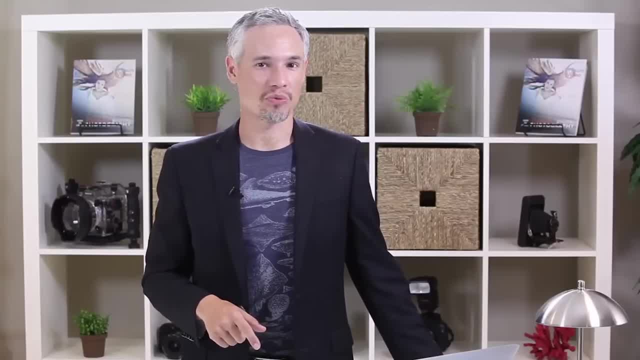 three pictures, right, And looking back at those three pictures once again, you can see that I didn't use a special head. I didn't even manage to keep the camera level between my three shots. Panoramas are really pretty easy to do, You don't? 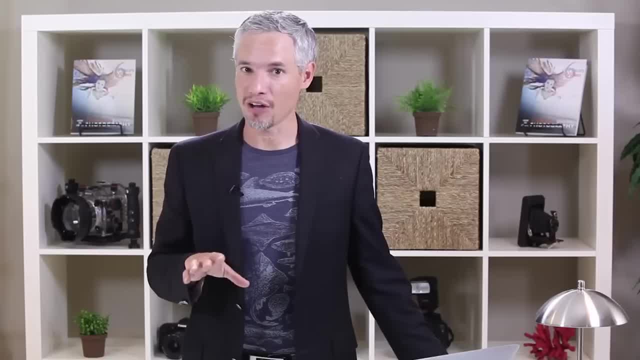 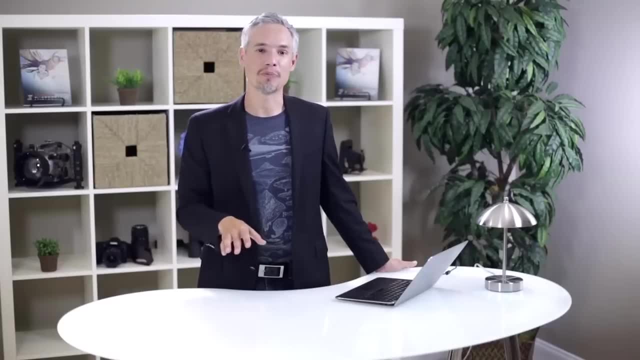 have to be as precise as some people say, because the software- modern software- automatically accommodates for all those little twists and turns of the camera. So now let's head to Berlin, Germany, to combine three of my favorite types of photography: Panoramas. 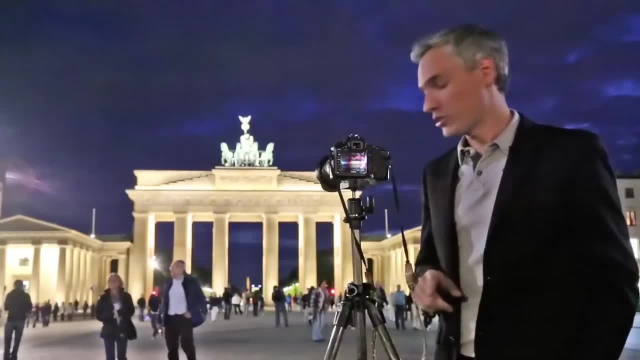 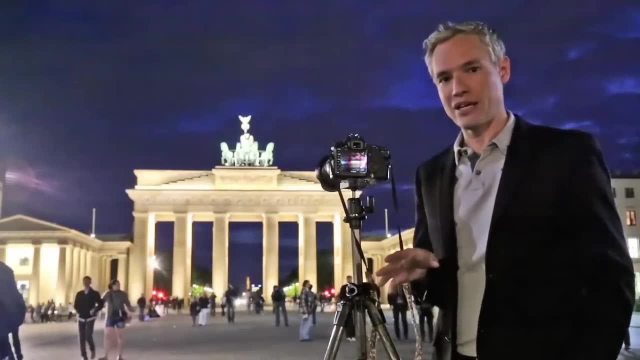 night photography and HDR. The first thing you need is a nice sturdy tripod. The tripod is required only for the night photography part. You can do HDR and panoramas handheld, but because it's night, the shutter speed is going to be really long. 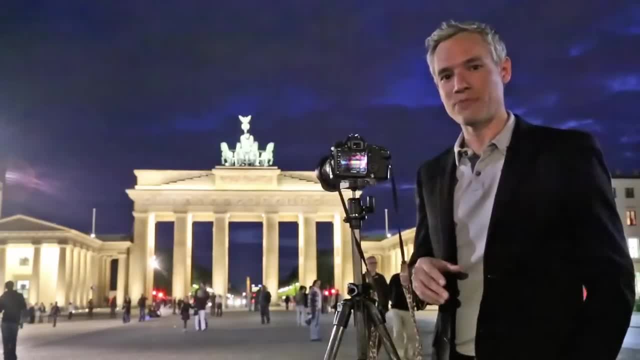 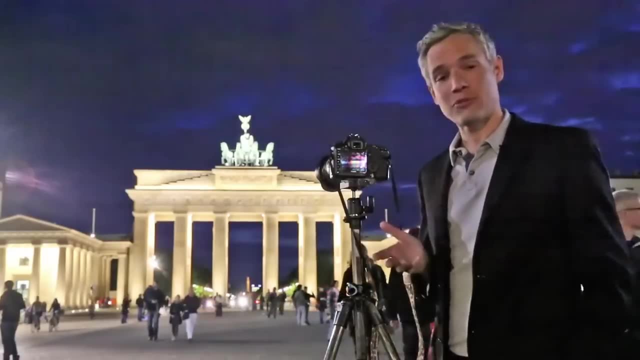 and hand holding. it would mean the camera would end up really, really shaky. I have the camera set to aperture, priority and f8.. That's a high enough aperture that will allow me to get the subject behind me here in focus. I'm using ISO 100. 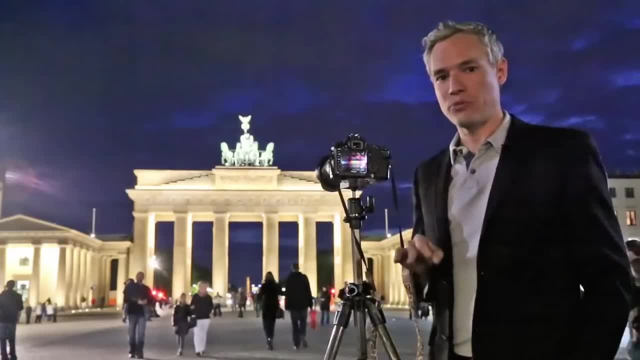 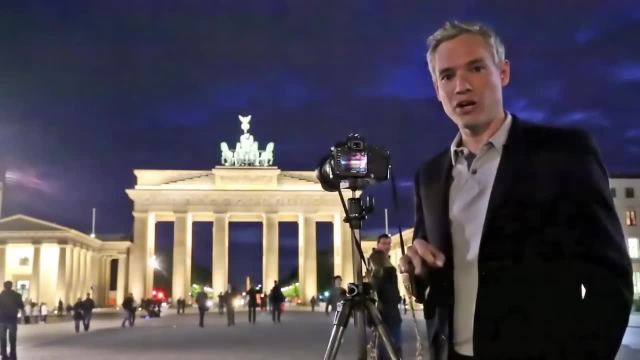 That will reduce the amount of noise that's in the final pictures and because I have it on the tripod, I don't need a higher ISO. So those are the settings I need for the night photography part. For the HDR part I'm going to need to. 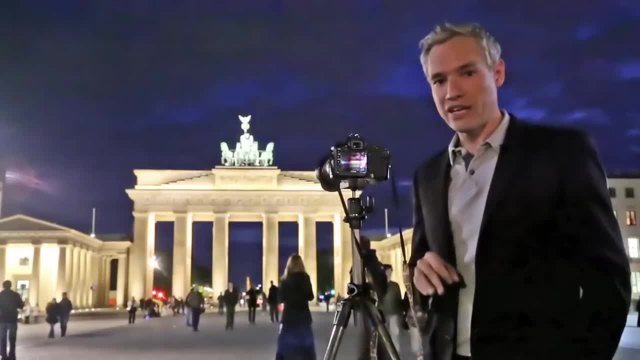 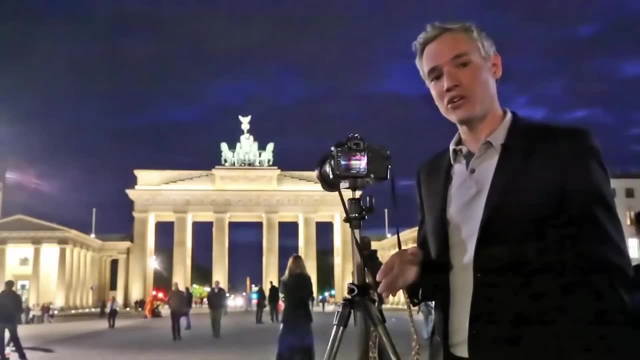 set the camera up for bracketing. If your camera supports HDR natively, you can use that too. So I'm using three exposure bracketing at plus or minus two stops. So each time I press the shutter it will take three pictures: A normal exposed picture, a picture: 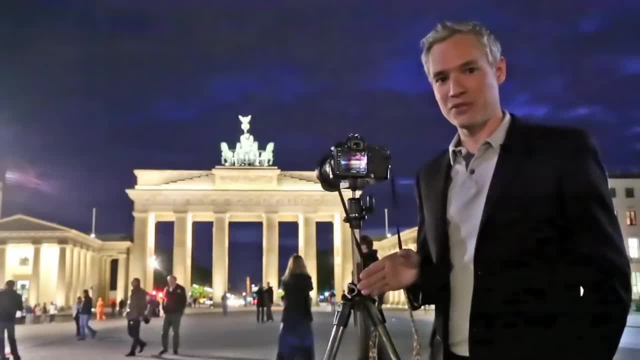 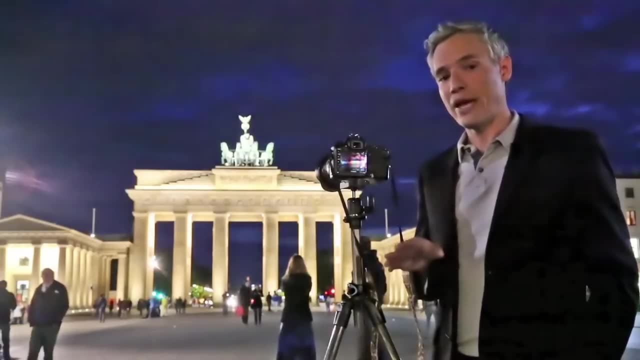 that's underexposed two stops and a picture that's overexposed two stops. So that will do it for the HDR part. The final part is the panorama. This requires some additional settings. Now for a panorama. you rotate the camera in a circle around you. 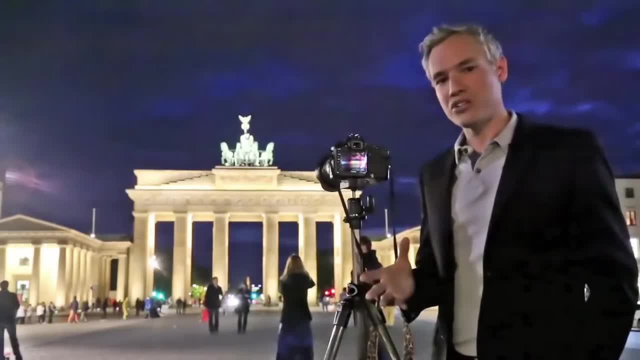 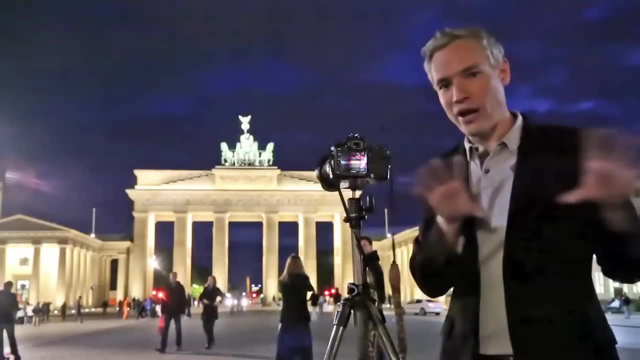 taking pictures of an entire scene. This creates a really large image, even hundreds of megapixels, with just a ton of detail. It also allows you to make a really wide image that you can pan around, and it better recreates an entire scene for a beautiful place like this. 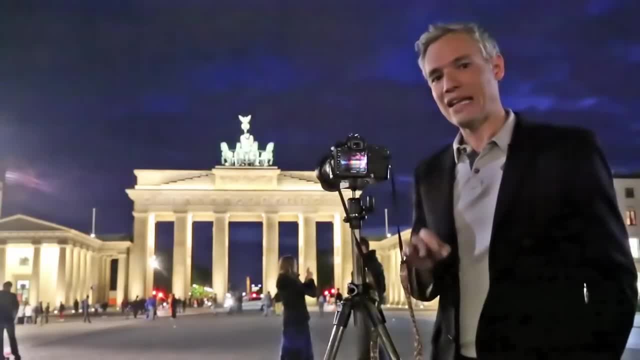 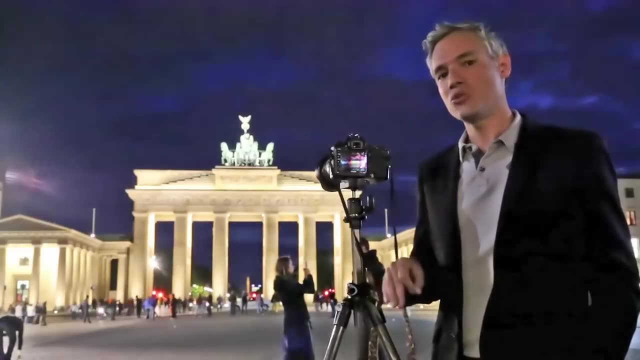 So to make a good panorama, you want to use your AE lock That locks the exposure in. If you don't know where your AE lock button is, you can also take a picture and check those settings and then choose them in manual mode. Either way, so long as your camera 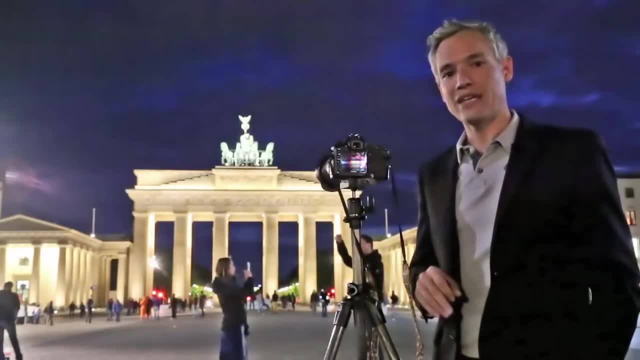 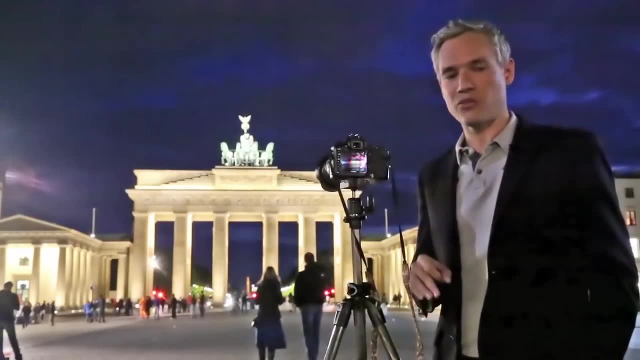 uses the same exposure every single time. So once you have the AE lock set, focus your camera on the most important part of the subject and then switch it to manual focus. This will hold the focus steady throughout the panorama. Next, you're ready to shoot your picture. 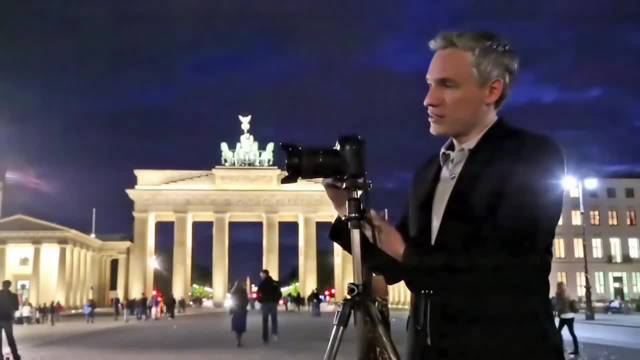 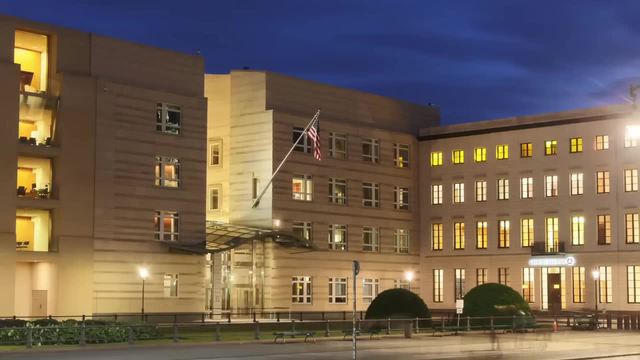 So just loosen up your ball head a little bit and take a picture and then move the picture until about one third of the picture remains. You want to overlap the picture a little bit. This will allow the software on your computer to combine the pictures evenly. 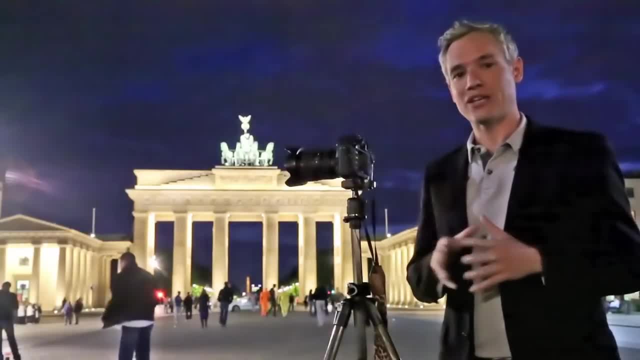 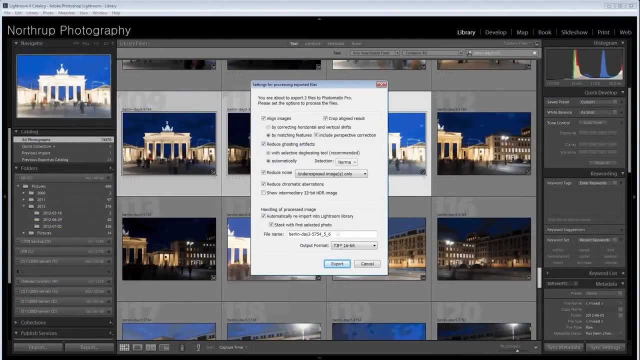 Now, once you've taken the picture and back at your computer, you're going to do a two step process. First, you're going to combine each HDR photo with the HDR software to combine a series of HDR pictures. Next, you're going to combine 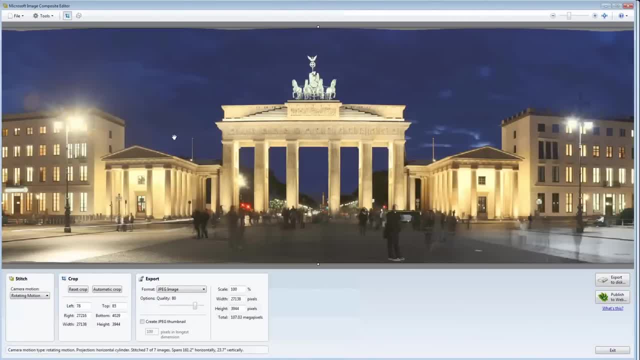 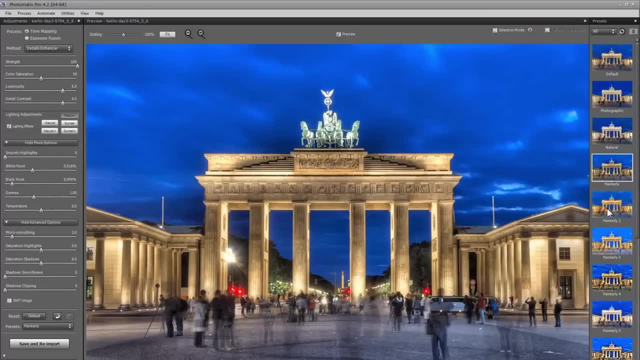 those HDR pictures with your panorama software to make a large panorama. Now my favorite HDR software is Photomatix Pro. It works really well and it's quick and it gives you a lot of creative control. My favorite panorama software is Microsoft Ice. All you need to do. 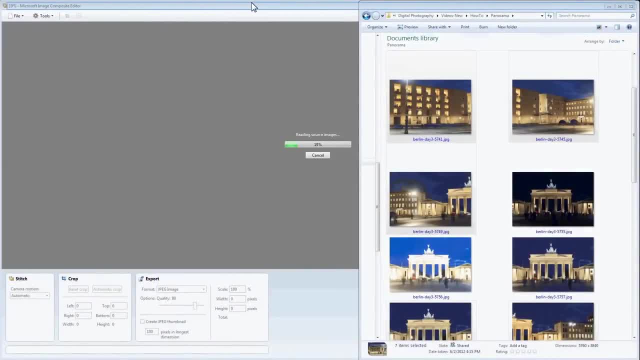 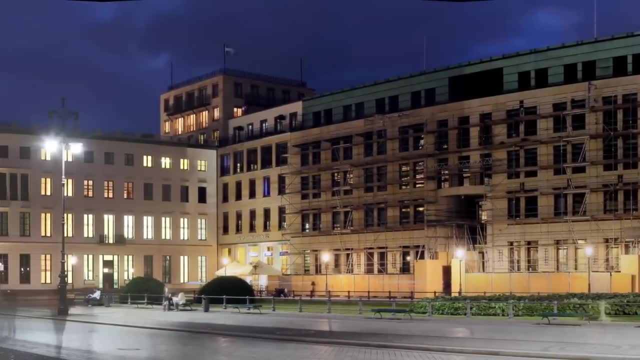 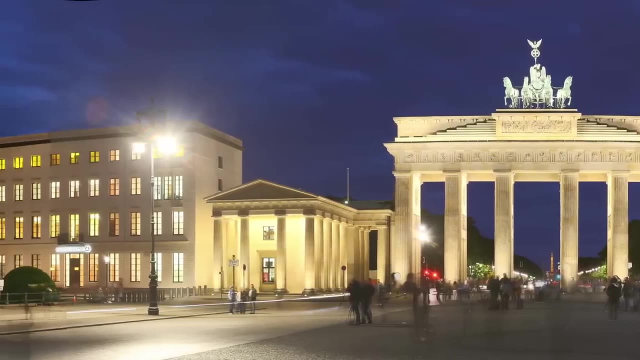 is to drag those pictures from the HDR software into Microsoft Ice and it will combine them for you automatically. Let's take a look at those results. As you can see, you can create really stunning pictures by combining these multiple techniques. Now I'd like to talk about 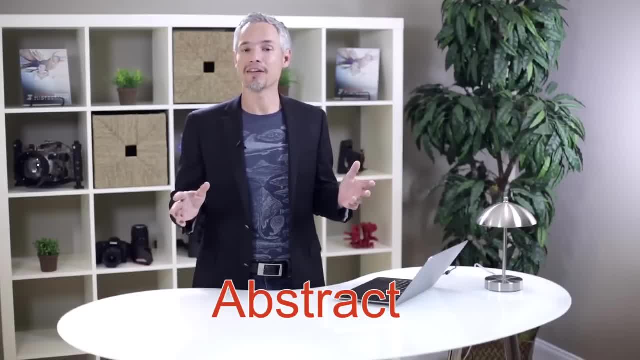 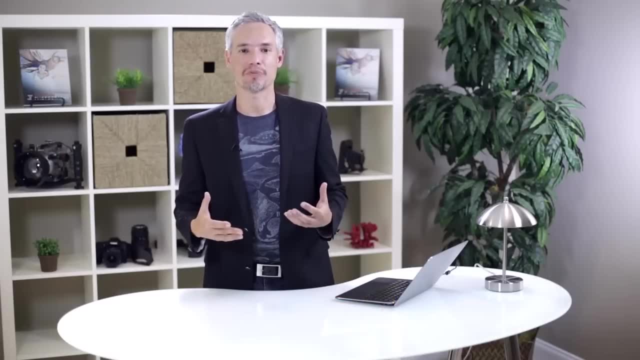 abstract photography. Abstract photography is any photography where the subject isn't completely obvious. Abstract photography is the purest form of composition, because you're not taking a picture of a person or a thing. You're taking a picture of lines and shapes, and colors and gradients. 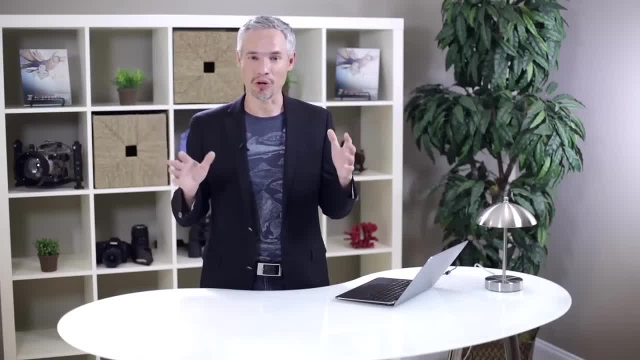 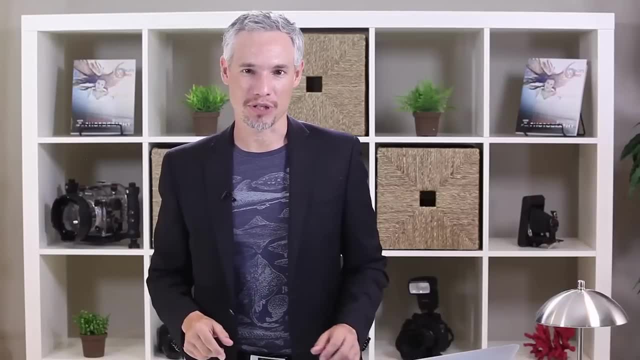 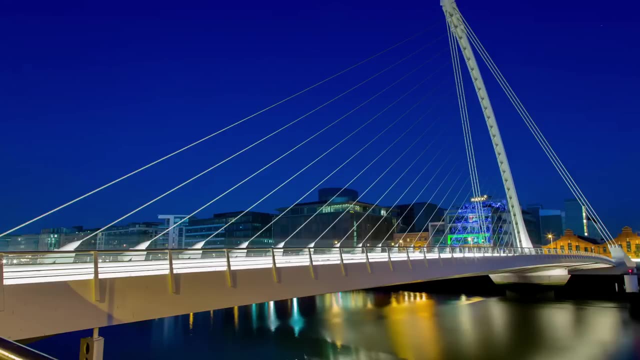 You're completely abstracting anything we know in the real world and breaking photography and art down to its most primitive elements. Let's take a look at a few pictures- This is not of a bridge in Dublin, Ireland, and it's absolutely beautiful. And that's what the bridge looks like. 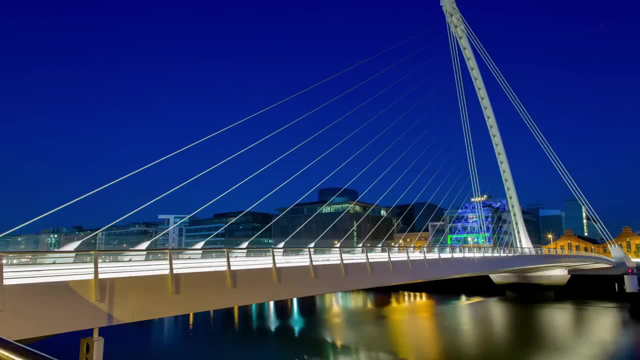 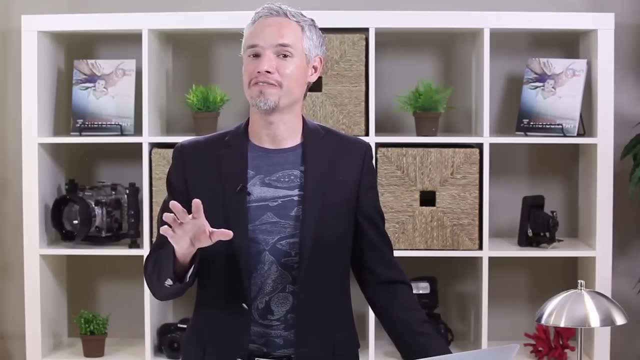 to the eye, But I wasn't happy with the pictures that I was getting. so I did what I always do when I'm not satisfied with my subject: if my pictures aren't turning out the way I like, I zoom in and I try to find abstract. 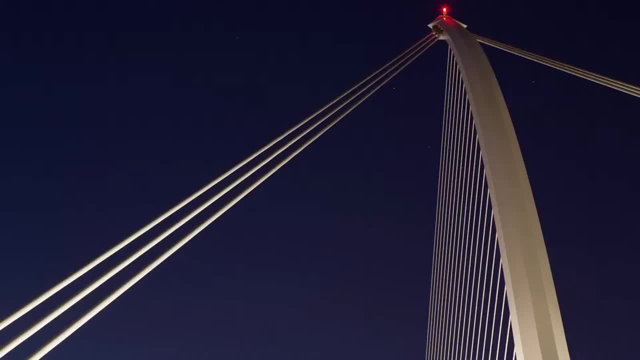 views of the subject. So here's one of my favorite abstract shots of the bridge. You can see by zooming in on a part of the bridge. I broke it down into its core compositional elements: Curved lines and straight lines. Here all these lines lead your eye. 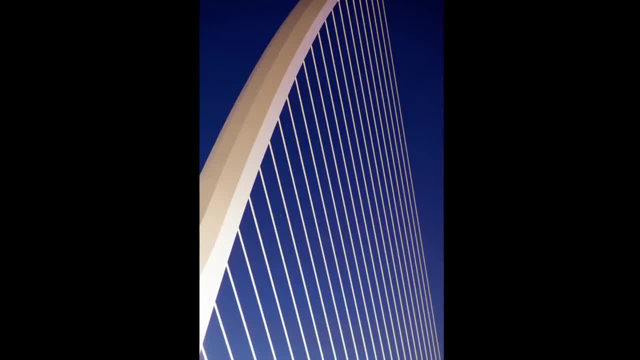 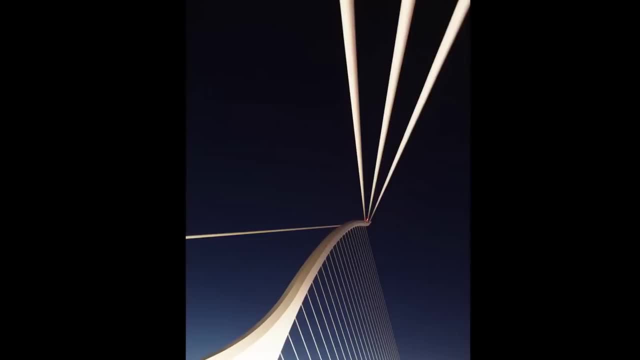 to that nice little red light at the top of the bridge. Here's another abstract shot of it that again just shows that one nice curved line and then lots and lots of vertical lines And finally another shot pointed straight up. Once again: all the lines. 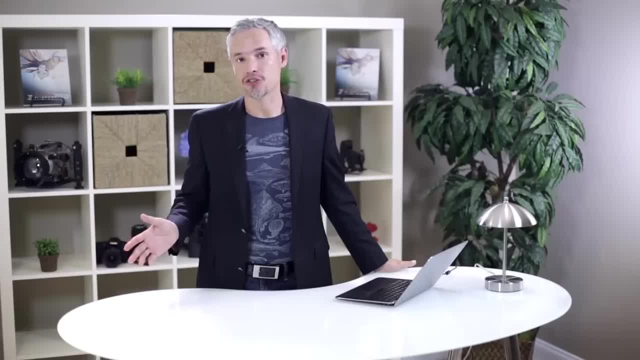 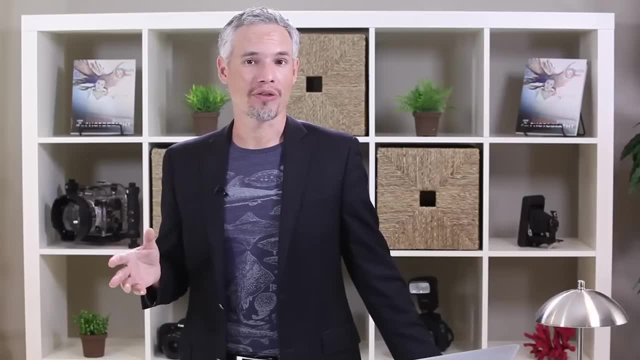 lead you to that focal point in the center of the picture. Berlin in Germany has an absolutely moving memorial to the Holocaust and unfortunately it's in a rather busy district, So there's always people moving in and out, and it's surrounded by other buildings that detract. 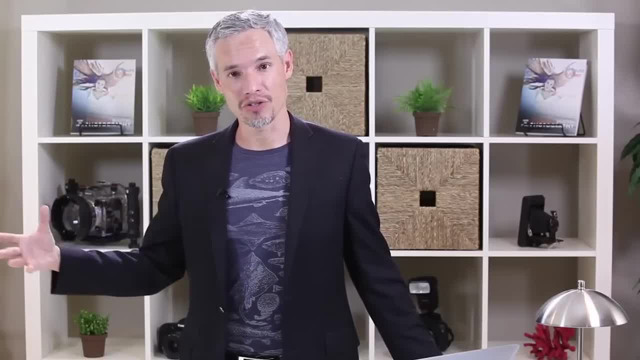 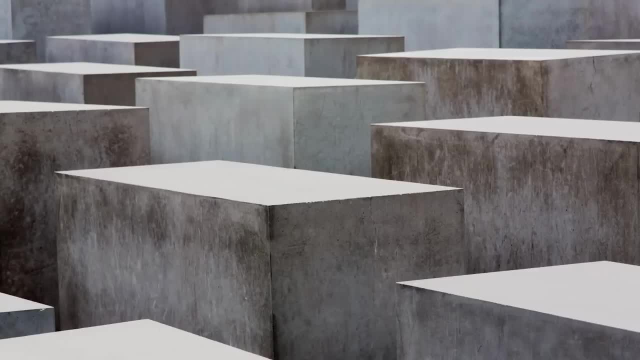 from the picture. So because I couldn't get a picture of the entire large subject, I decided to zoom in and get a couple of abstract pictures. So looking at this first picture, you can see that by zooming in tight on the different concrete blocks. 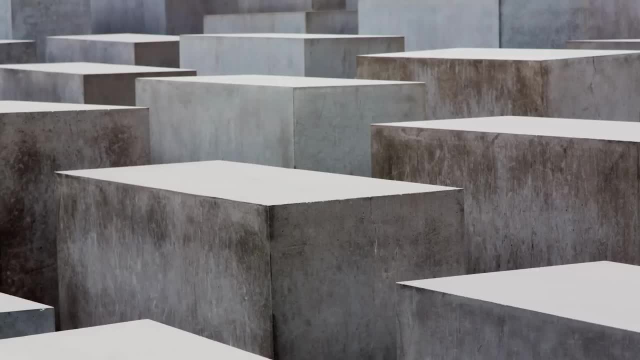 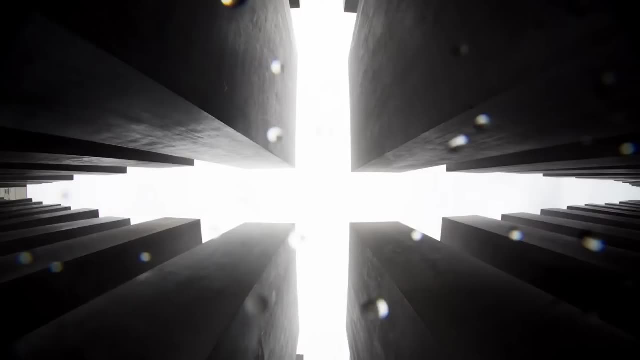 I managed to break it down into the very simple elements of lines and gradients. Here's a picture that I made, laying flat on my back with a fish eye lens pointed straight up towards the sky. It was raining that day, so I let a few raindrops land on the 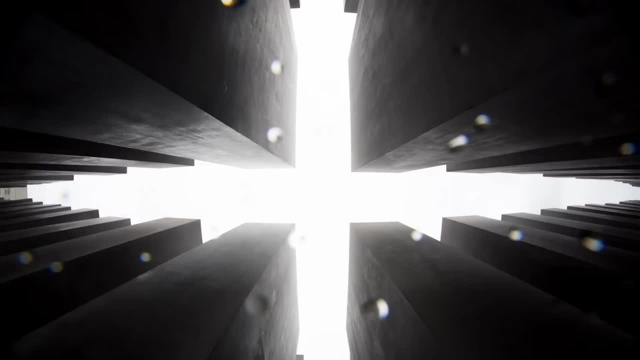 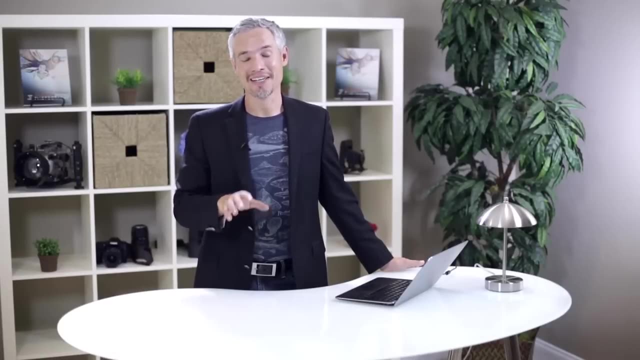 lens, which I felt really supported the somber theme of the memorial. Now I'm going to introduce my wife, Chelsea, and allow her to talk about black and white photography. Yes, even with your colored digital camera, black and white is still very. 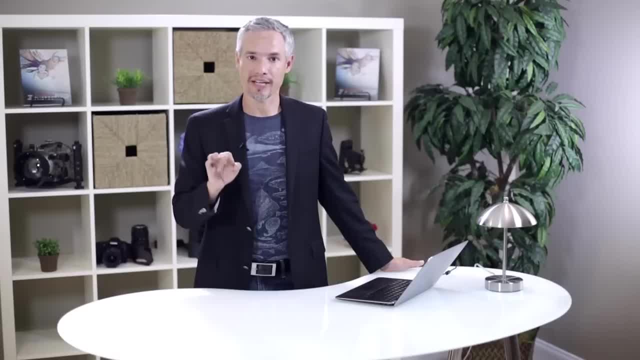 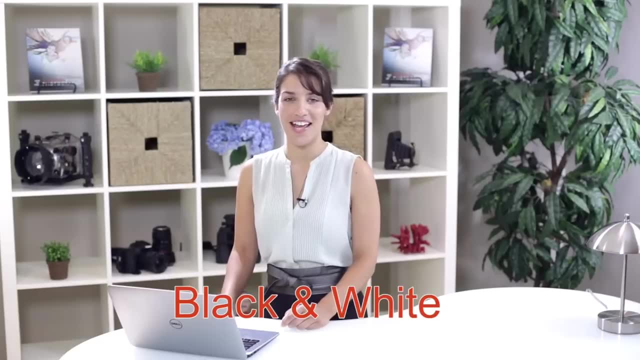 relevant and compositionally. black and white can be an important technique for eliminating distracting colors in the picture, So I'll get out of the way and let Chelsea come in. Hi, I'm Chelsea, and today I'll be showing you how to take and edit black and white pictures. 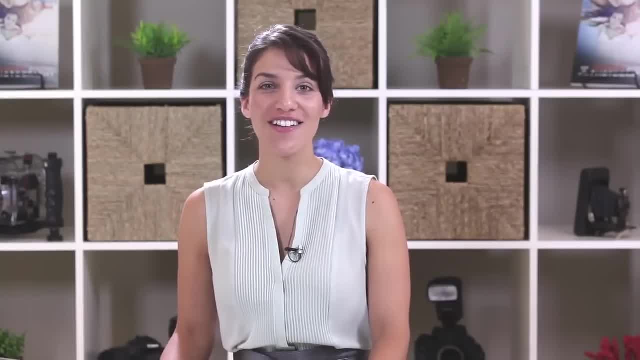 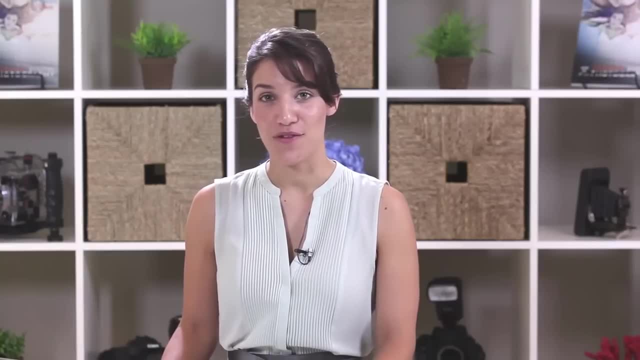 I love black and white photography. It strips away the distraction of color and instead lets you focus on the tone and the textures and the overall forms in the picture. Before you start taking your black and white photos, you'll want to learn to see in black and white, And what. 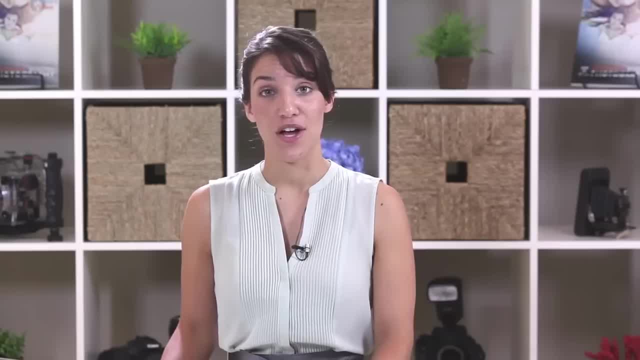 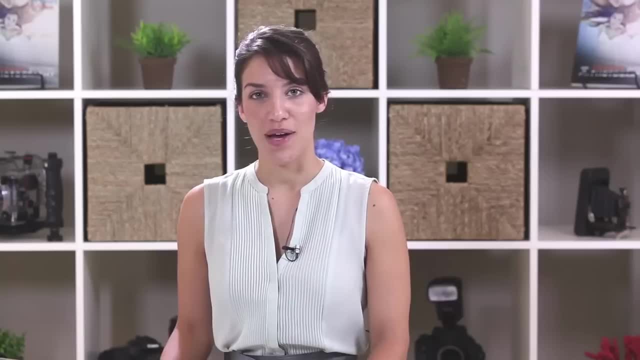 I mean by that is, you want to learn what looks good in a black and white picture before you start looking for a subject. That way you'll know what will end up good once your photo is taken. So before we talk about the overall elements that make 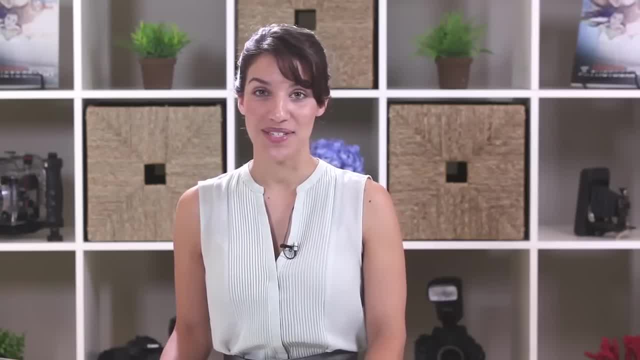 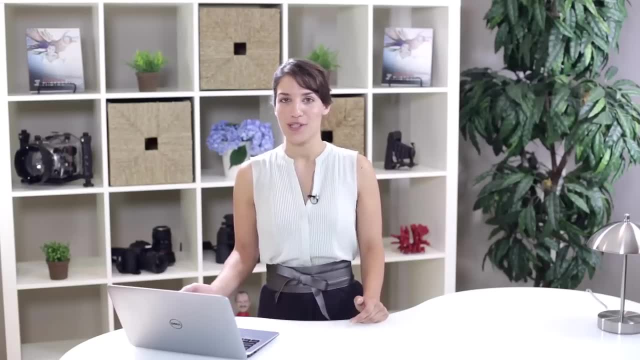 a black and white photo look good. let me give you some tech tips. My first tip is that you should shoot RAW. When people say that they're shooting RAW, they just mean that they're using the RAW file format. When you shoot RAW, it takes. 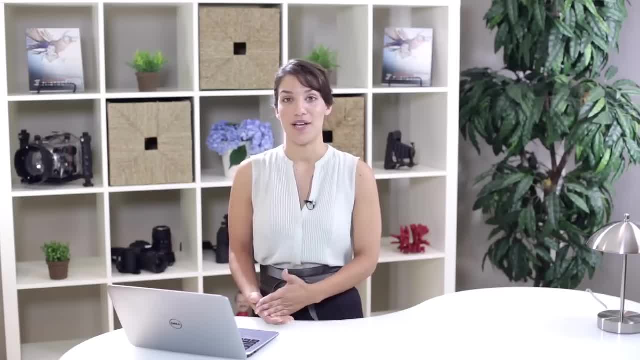 all of the information from your camera sensor and puts it in your pictures. When you shoot in a different file format like JPEG, it can take all the information that you say you need and throw out the rest By having all of the photo information. 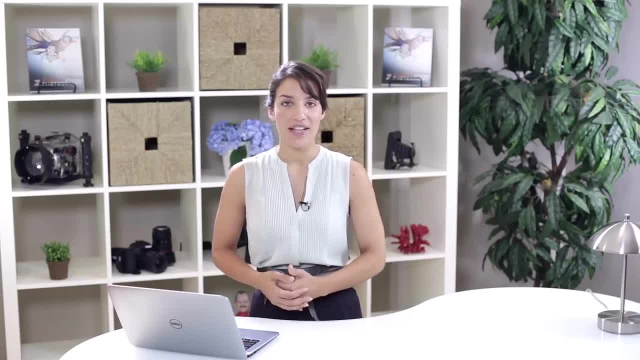 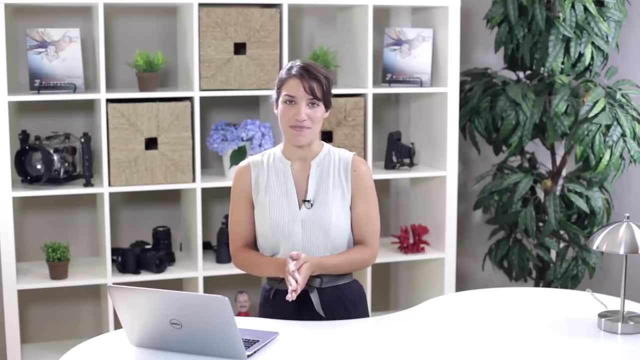 in the RAW format, you can easily recover highlights or underexposed sections of your photos, and it also makes the tonal transitions a lot smoother. Let me show you what I mean by that. In this picture, you can see that there's a very smooth transition. 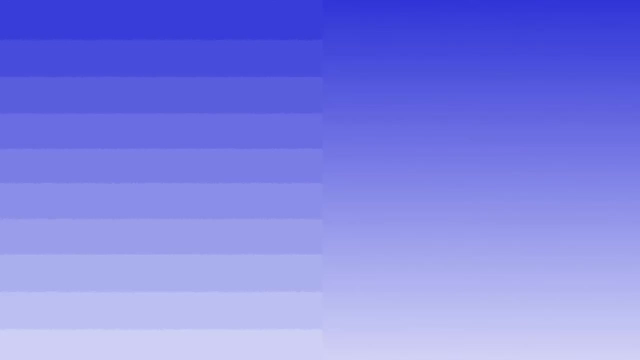 from white to blue on the right And that's what it would look like if you were to use a RAW file And if you had a compressed file, like maybe a JPEG, your tonal transitions from white to blue or black to white, if you're taking 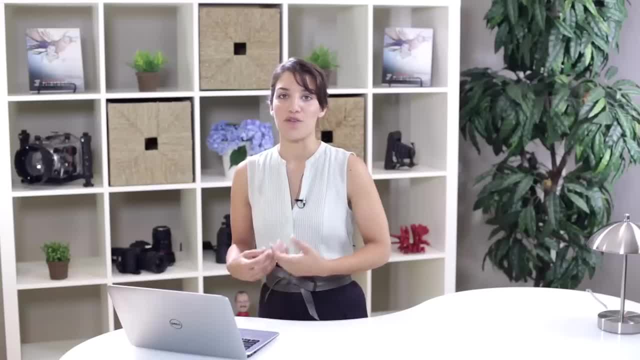 black and white pictures may look a little bit blocky. So for that reason it's really important to use RAW files when you're taking black and white pictures, But I use RAW files when I'm taking any pictures, to be honest with you. 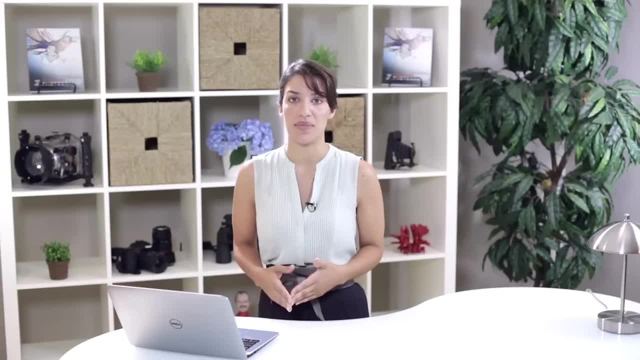 Some people think that the file size is too big. Sometimes it can be two to five times larger when you're using a RAW file. But I really feel that the pros far outweigh the cons And if you need to free up some disk space, you can always. 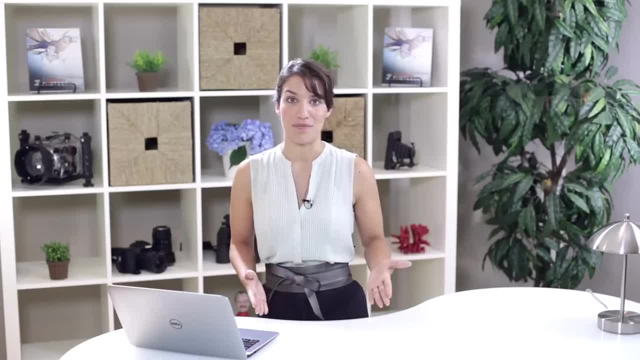 erase the pictures that aren't your favorite. You don't need a bunch of bad pictures laying around on your computer anyway. So I haven't really had a problem with disk space, but I have had problems with JPEG files not being able to recover enough information. 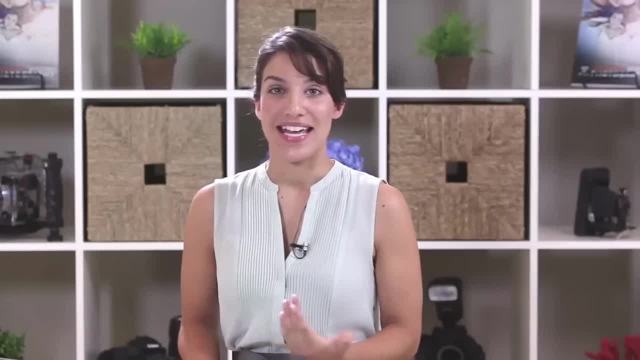 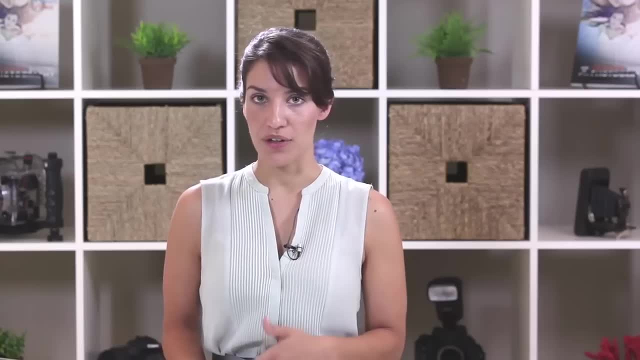 And so I highly recommend shooting RAW. My next tech tip would be to use the monochrome setting on your camera, if it has it. Now I shoot with a Canon Mark II or Mark III, so the setting is built in and it's easy to use. 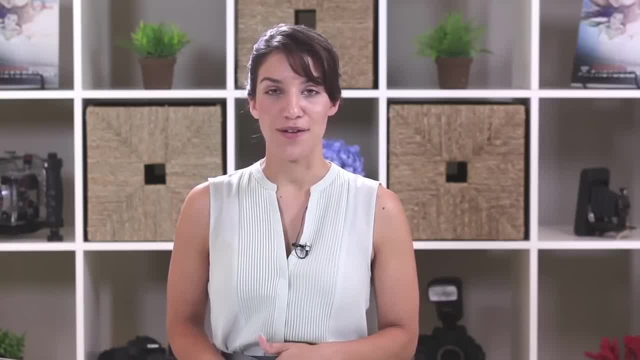 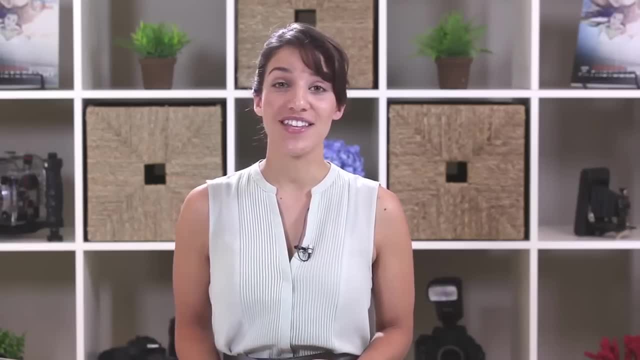 The reason that I recommend it is because it allows you to see what your black and white picture will look like before you get it on the computer. So, like I said, shooting black and white is a little bit different than shooting color. You're focusing. 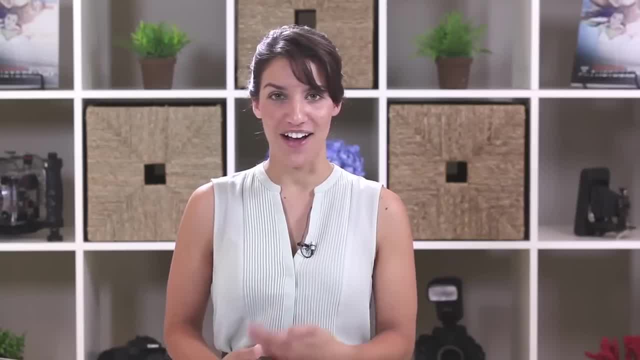 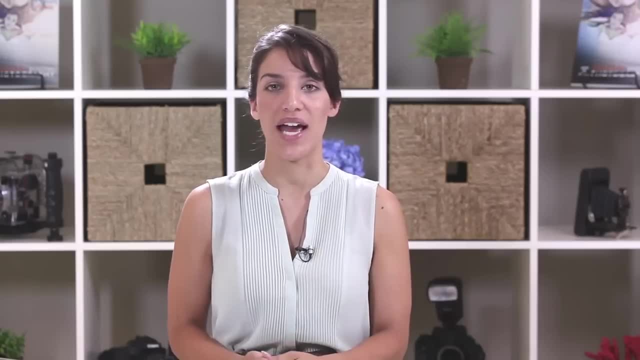 on different things like tone and form, And having it right there on your LCD screens that you can see what your finished product is going to look like is really helpful in teaching you how to see in black and white. Once you upload your pictures onto your computer, into your 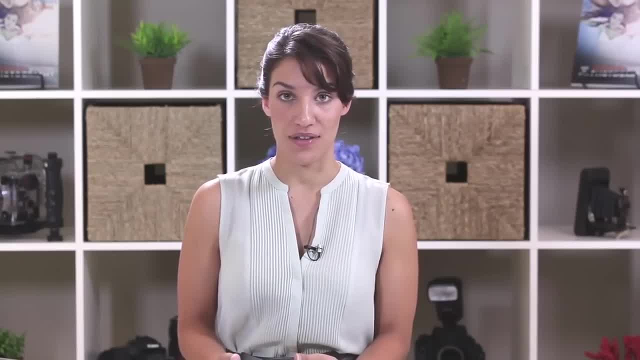 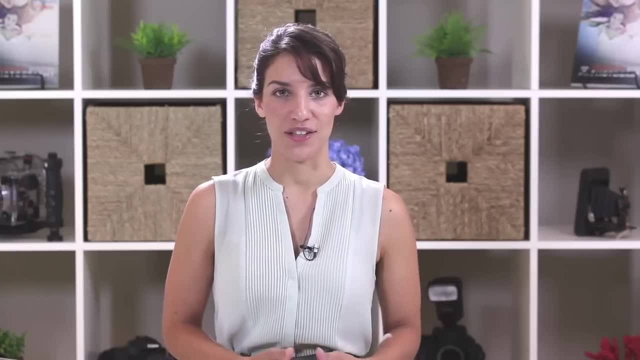 photo editing software. it automatically converts the pictures back to color. You have to go into your pictures and put them in black and white again, But at least you got to see what they looked like on your LCD in that black and white format. My last 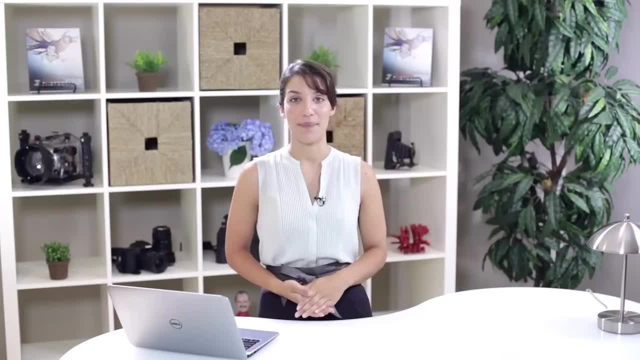 tip when you're shooting black and white is to always check your histogram. Your LCD screen sometimes shows pictures as properly exposed when they aren't really, And that's because the LCD screen is giving off light, So things can seem like they're more exposed than they really are. So check your. 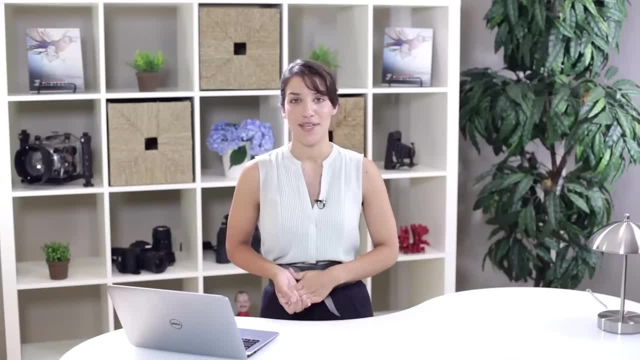 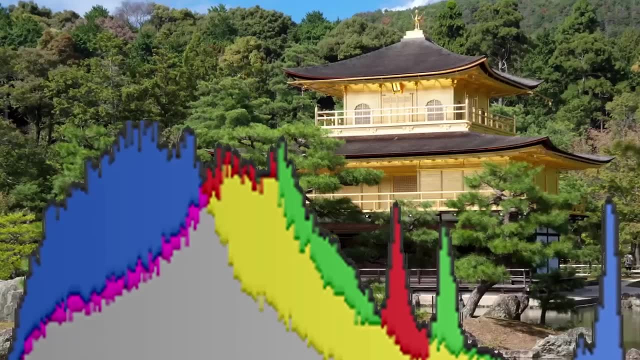 histogram and make sure that your pictures are properly exposed. This means that you'll want the peaks not too far to the right and not too far to the left, but kind of arching in the center. And here I have an example of a properly exposed 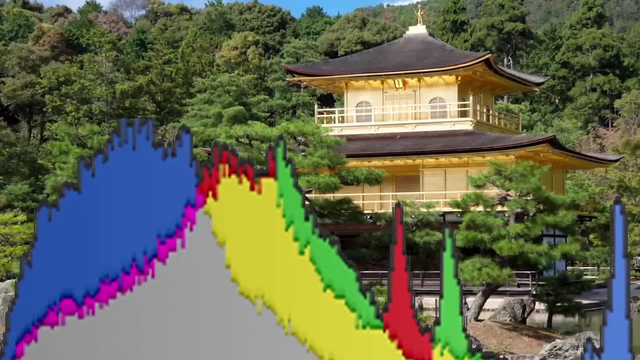 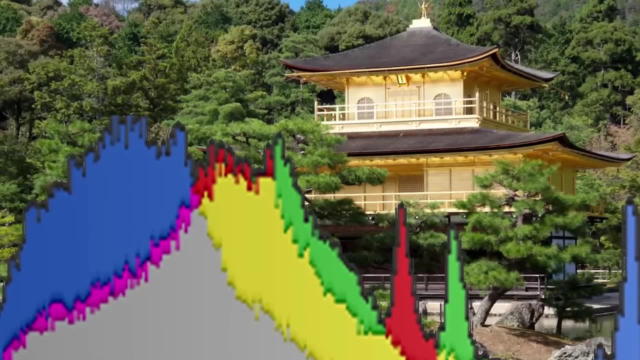 picture and its histogram, You can see that most of the peaks are towards the middle of the picture and there aren't too many big peaks to the right or the left, and that's what your histogram should look like. Now that I have those tech tips out of the way, let's talk about other 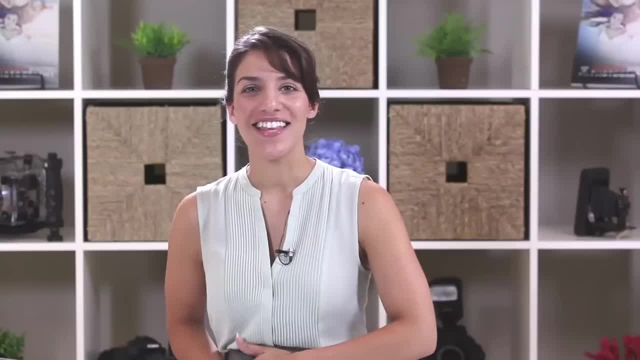 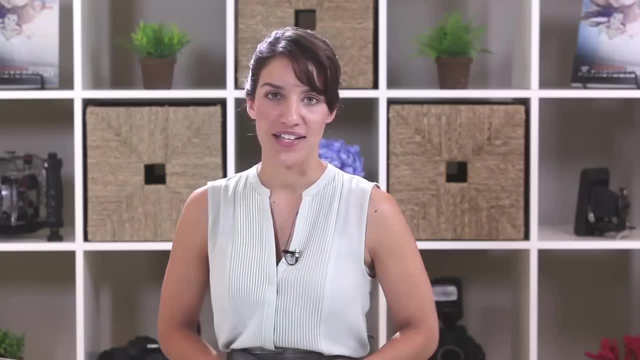 elements that will give you a really beautiful black and white picture. Now, I think that light is the most important part of any picture, but it's especially true with black and white photography. There are all different kinds of light. You have soft light, hard light, directional light. So let's start. 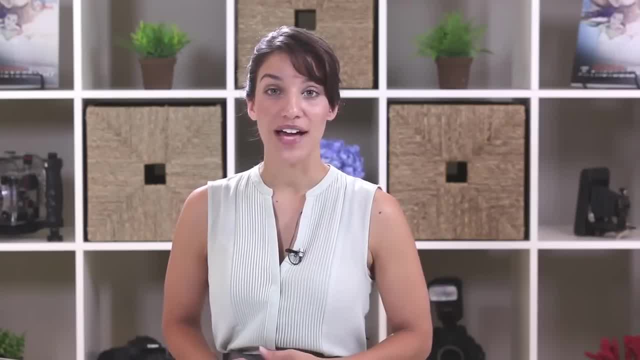 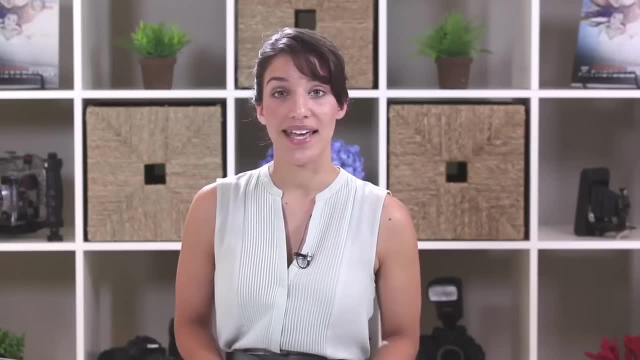 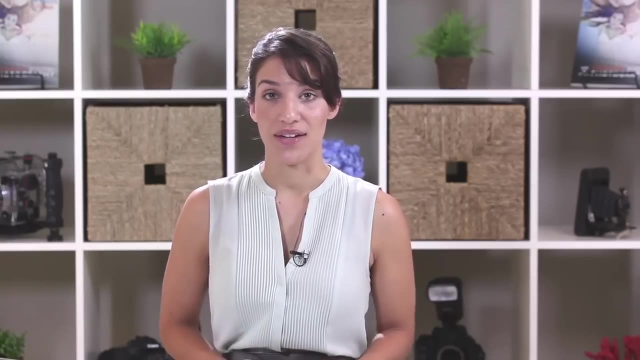 by talking about soft light. Soft light is usually most flattering for portraits because it kind of diminishes details like lines and wrinkles and spots, And you'll get soft lighting in the shade or on a cloudy day or even when there's low light in the sky during sunset or sunrise. 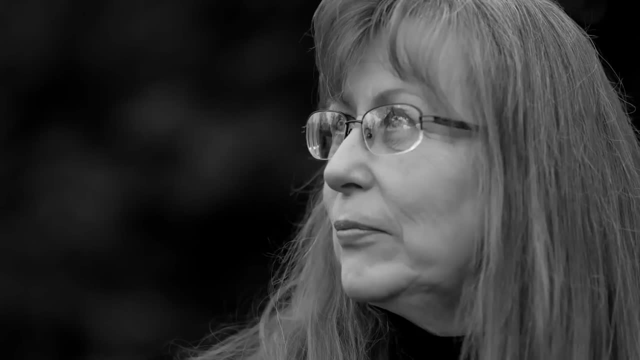 You can see a picture that I took of my friend Hillary using soft light in the shade. There are just really nice smooth transitions in her skin, No hard lines or wrinkles, And it's a really beautiful picture. I think it came out nice. 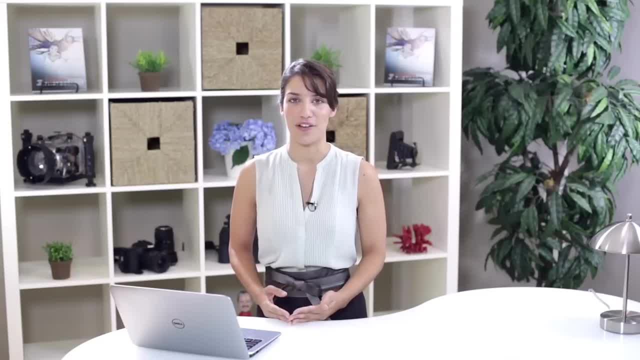 I talk about soft light making a very flattering portrait, but hard light can make a very interesting portrait. If your subject has wrinkles or other defining features that you would really like to accentuate. hard light will do that. So it's really a matter of taste and you'll have to decide if you want a 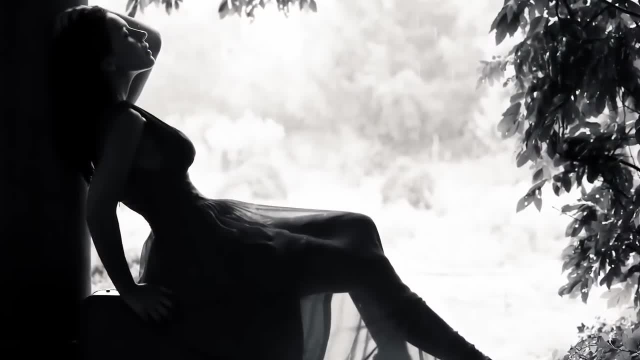 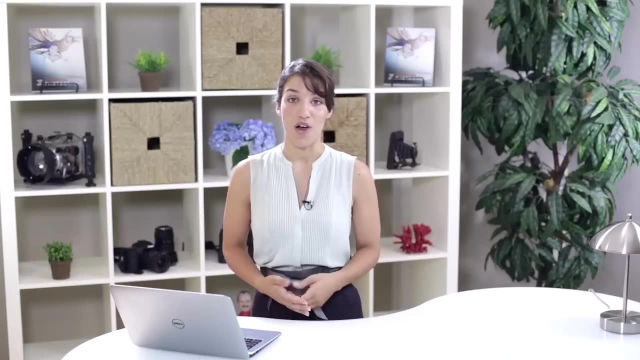 flattering soft portrait or an interesting gritty portrait with hard lighting. So next let's talk about what the light is like when the sun is low in the sky. It tends to be soft, It's during the golden hour and it casts a lot of shadows. 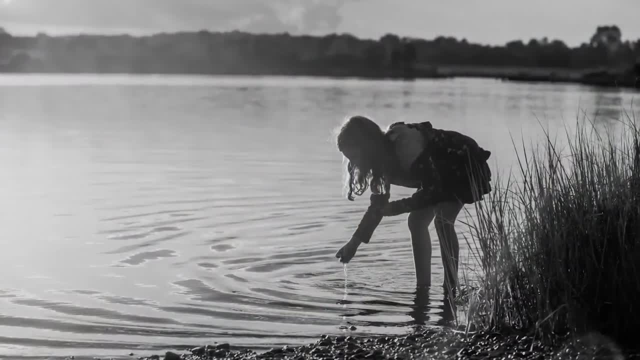 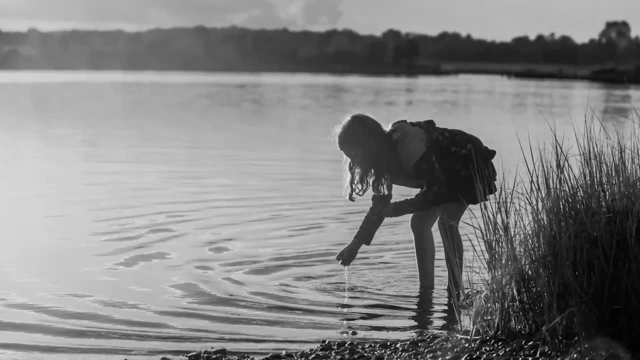 and you can get beautiful silhouettes. So let's look at a picture that I took of my daughter during the golden hour, And you can see that she's backlit by the setting sun And there are a lot of highlights coming off the water and accentuating. 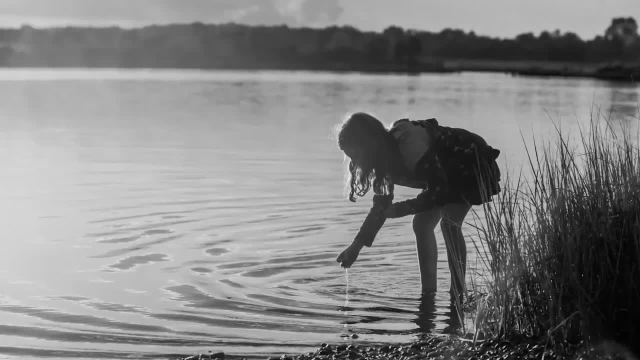 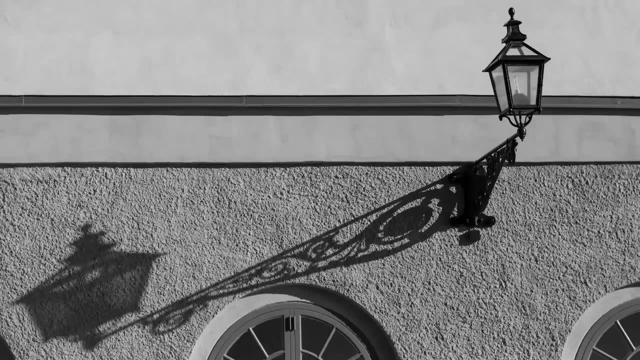 every ripple and casting little highlights on each rock in the foreground, And the light is really beautiful and dynamic in that picture. You can see that in this picture of a lantern that I took in Sweden during sunset The low setting sun casts a very long shadow on this. 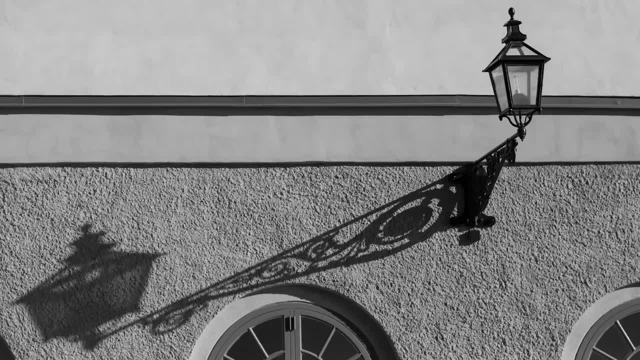 lantern. So without that long shadow it would have been an otherwise boring picture, But seeing all of the details of the lantern shown in the photo here made a very interesting picture. Now I've been talking a lot about soft light and the light that you use. 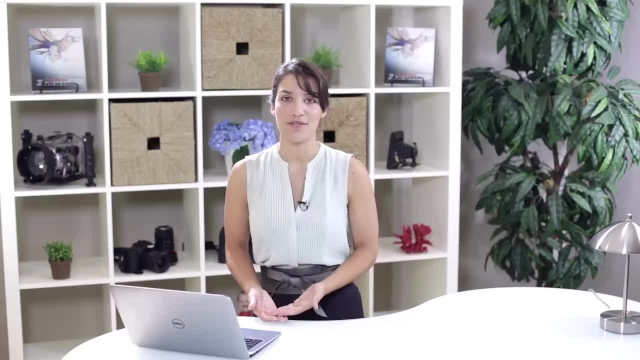 during the golden hour, But hard light during the day isn't really bad either. You just have to use it to your advantage, And I find that it works well when you are taking pictures of structures like buildings, skylines or other architectural. 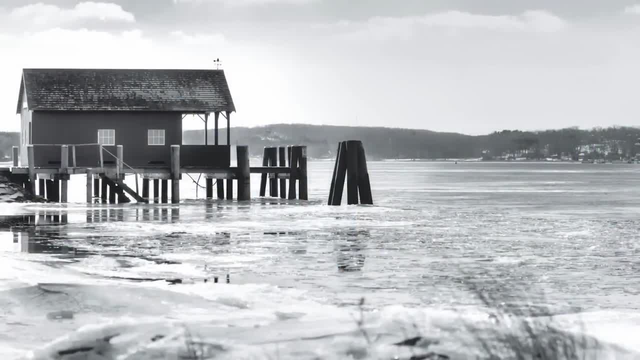 elements, And I'll show you an example of this boathouse that I took in Lyme, Connecticut, And having the hard light directly overhead actually made a very evenly lit picture, So it worked well here And it shows a lot of detail and accentuates a lot of the textures. 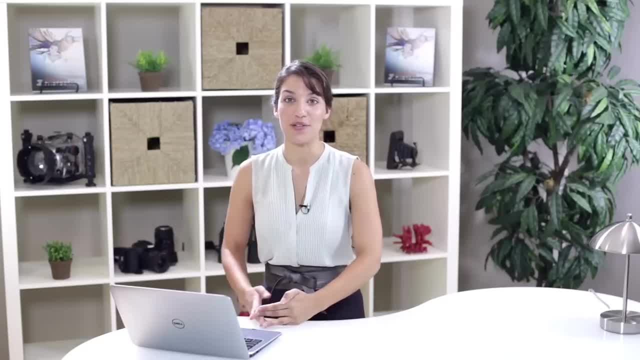 in the photo. Speaking of texture, black and white photography really accentuates the texture in your photo. So if you have rusting metal or weathered wood, it's going to look great in your picture. Let me show you an example of some rustic pumpkins. 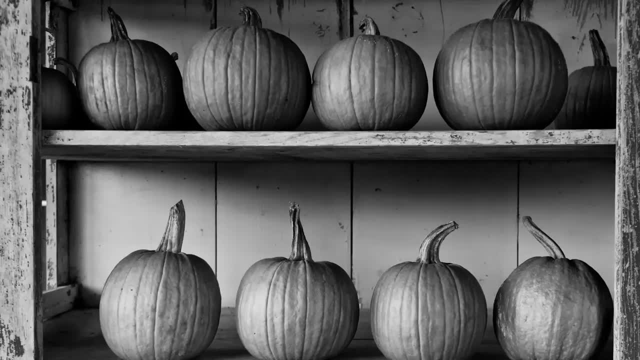 that I took pictures of in Vermont. You can see that they were on this rustic shelf and the light is really casting shadows on every groove of the pumpkin And they're highlighted and it just looks so beautiful And there's a lot of dimension in that picture. Another picture that I 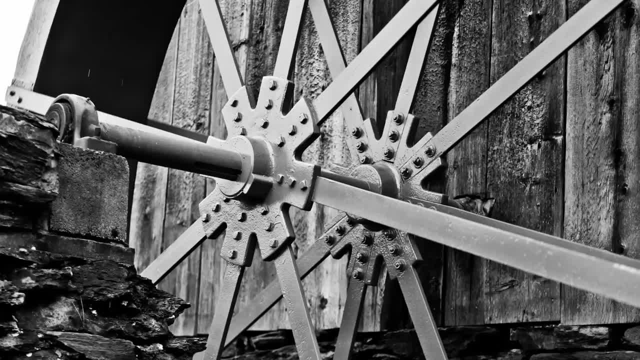 took while in Vermont is of an old mill And you can see it's the same thing. There's metal, but the metal is really brought out Every ribbit. you can see the metal looks luminous and there's aged wood and rocks in the photo. 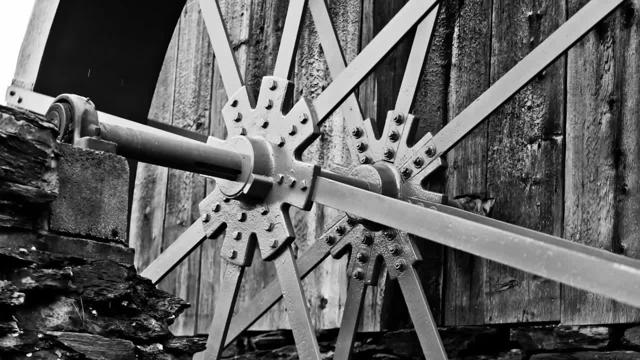 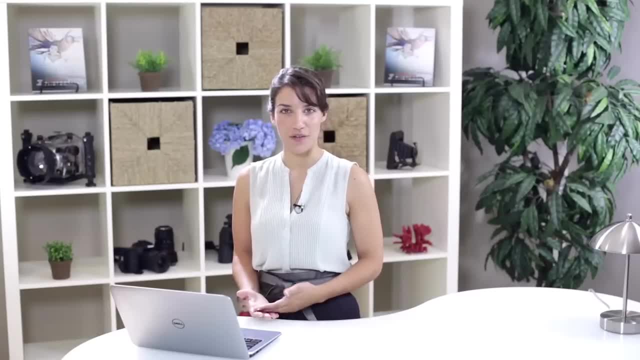 This photo is so full of texture You just feel like you could reach out and touch it. Next let's talk about shapes. Shapes are really important in your picture because they can leave the viewer's eye or they can be the entire subject of your photo. They can be the 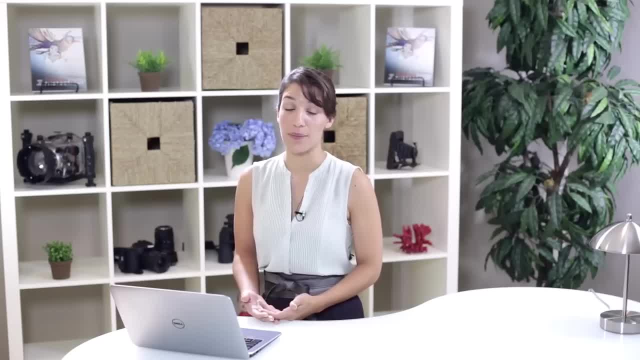 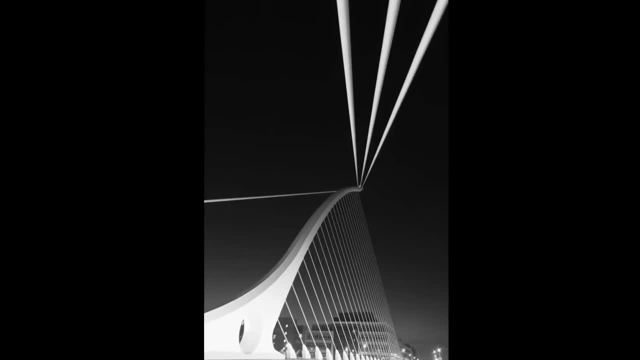 squirrel and a fiddle head, or even the silhouette of a person. So when you're taking your pictures, think a lot about the shapes in your photo. Here's a picture of a bridge in Ireland that I took and I wanted to focus on the shape of the bridge because it 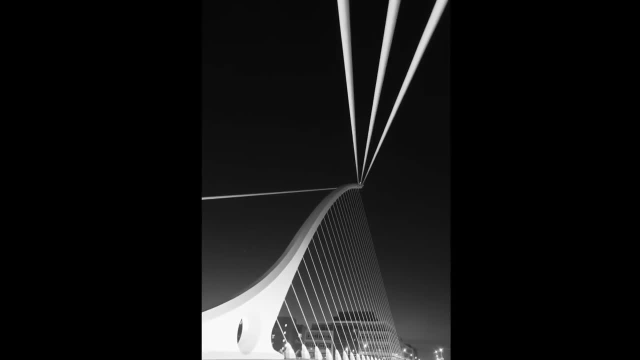 has a really beautiful, graceful arching neck on the bridge and some really interesting cables, And so you can see that the black and white format brings out the shapes of the bridge and you're not distracted by the deep blue night sky that was there or the buildings, kind of, at the 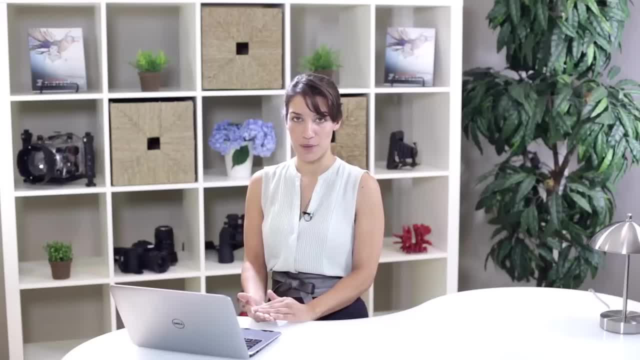 horizon that were brightly lit up. So shape is the two-dimensional form in your picture. So if I were to take a picture of a ball and silhouette it, the shape would be a circle. But if I were to light the ball so that there 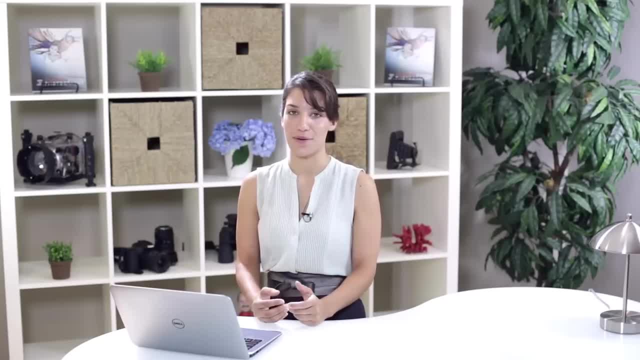 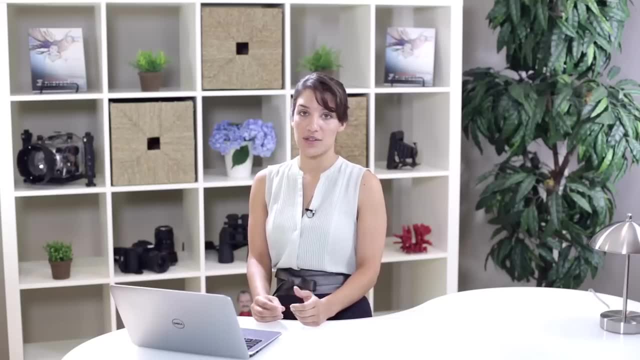 were highlights and shadows, making it look like a sphere. that would be form. And let's talk about form next, because that's very important. Form gives your picture a lot of depth, So let's look at this picture of a fountain that Tony took in Berlin. 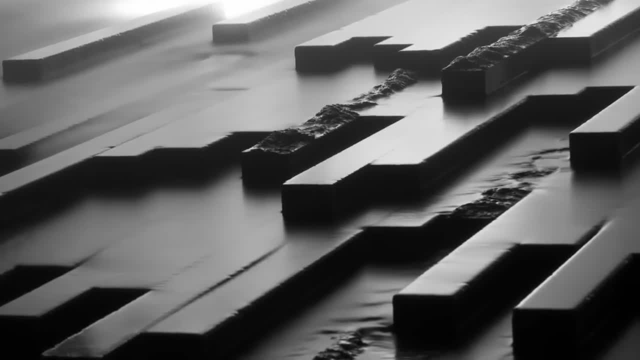 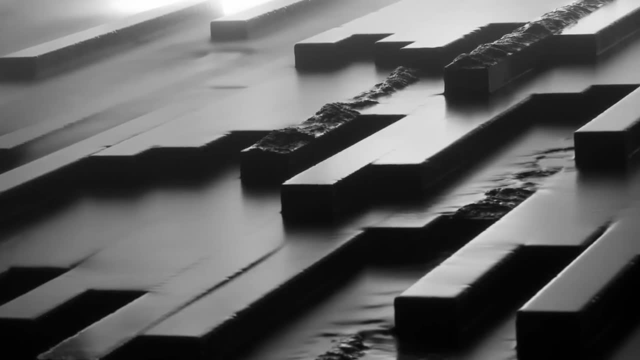 You can see that this picture really plays up the form of the fountain by using light. The top of the fountain is highlighted and all around the edges there are shadows, which gives you a lot of texture and depth and you really feel like you really get a sense of how blocky 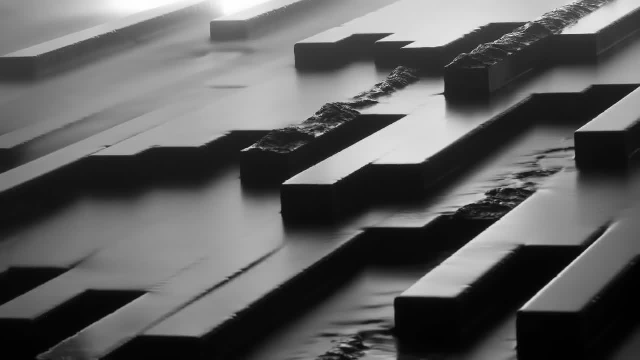 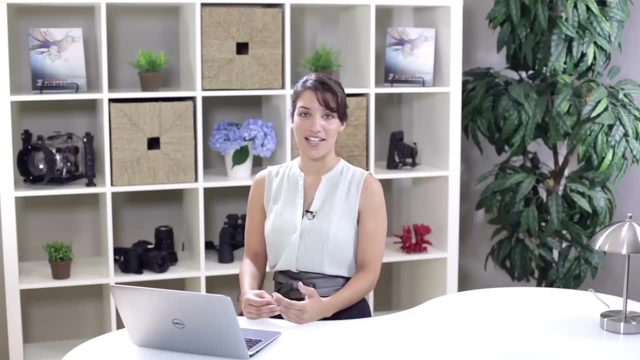 and jagged. this fountain was. Another way to add depth to your picture, other than form, is by using layers, So you can add a foreground, a middle ground, a background, and it gives your picture a three-dimensional feel, even though photos are really taking place in two dimensions. 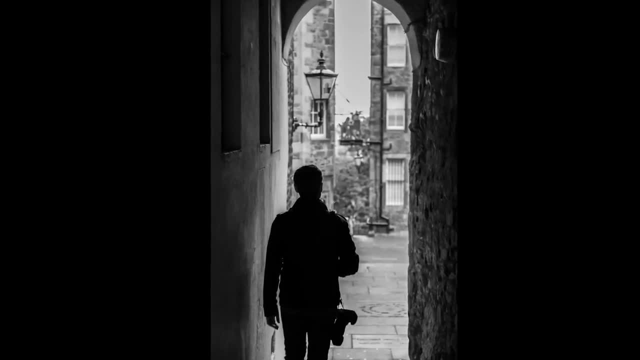 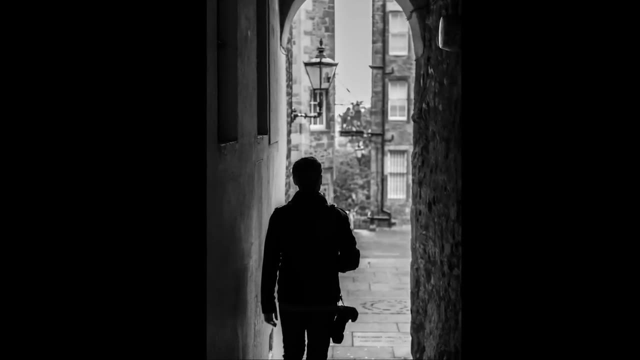 So let's look at this picture of Tony that I took in Edinburgh. You can see that his silhouetted shape is in the foreground, There is an archway in the midground and then there is a background that consists of buildings. There's a lot of depth in this photo. 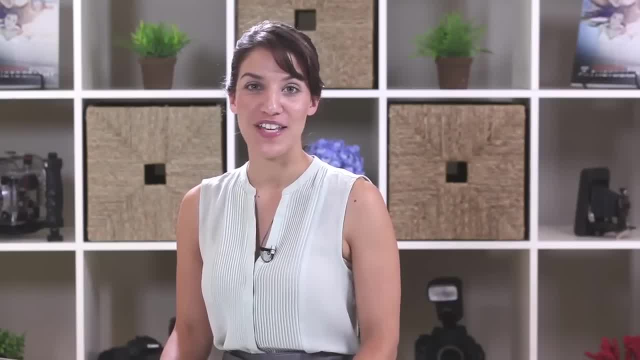 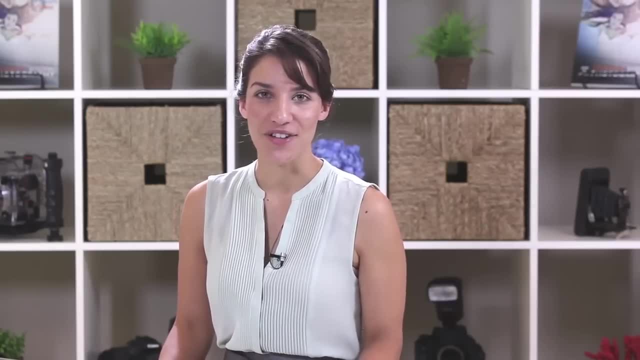 but it's not three-dimensional. One difficult element of black and white photography that you'll have to get used to is the difference between color contrast and tonal contrast. Now, you're used to seeing color contrast every day. That would be the difference between. 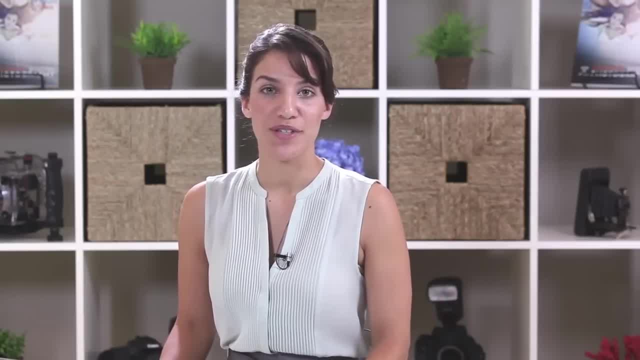 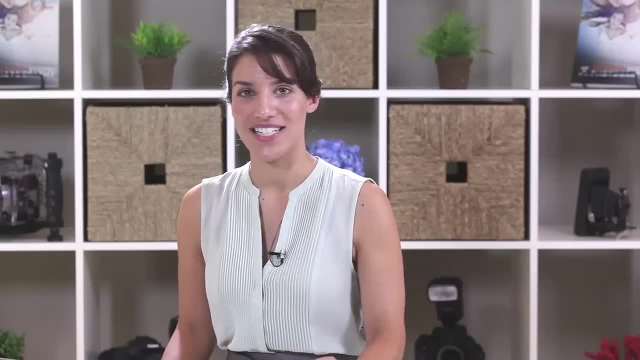 my green shirt and my blue skirt. or sometimes you'll see pictures of a field of yellow tulips with one red tulip popping out, and that's a color contrast. If you were to take that same picture of the tulips and convert it to black and white, you'd have to. 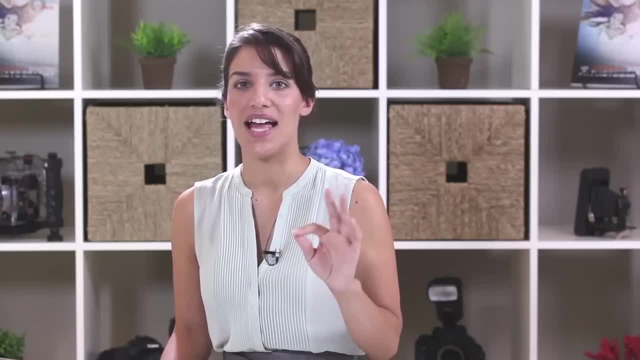 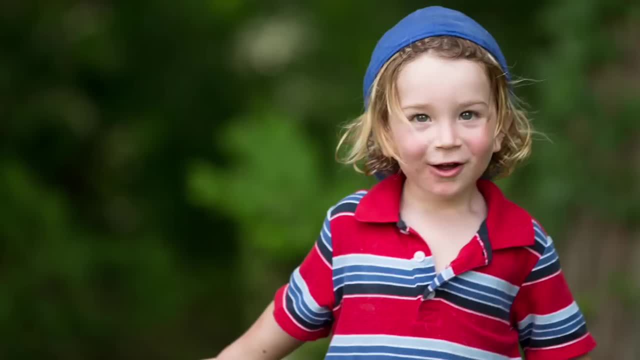 rely on tonal contrast, So the difference between the red and the yellow tulip might not be so jarring at this point. Let me show you a picture of my cousin Lane here, so that you can better see what I'm talking about with the difference between color and tone. 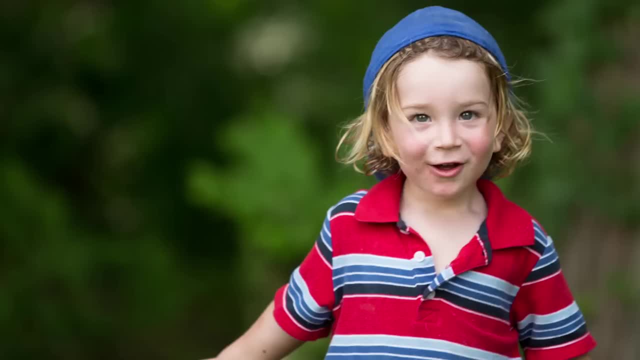 So in this first picture of Lane the difference between his shirt and his hat and the background really pop because they're contrasting colors. You have red and blue and green and the colors really steal the show in this picture If you look at the picture to black and white. 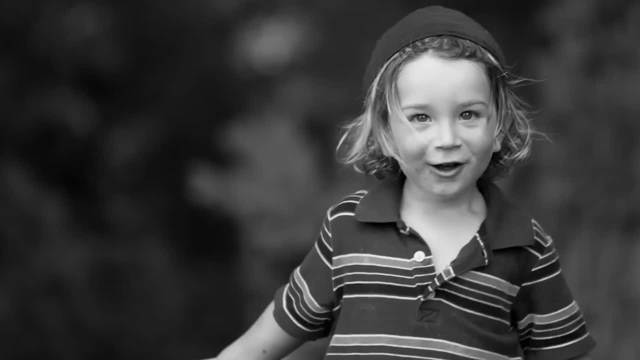 you can see that there's not a lot of tonal contrast between his shirt, the background and his hat. They suddenly fade away and now there's a tonal contrast between his skin and the background, So suddenly Lane becomes the subject of the picture because of the 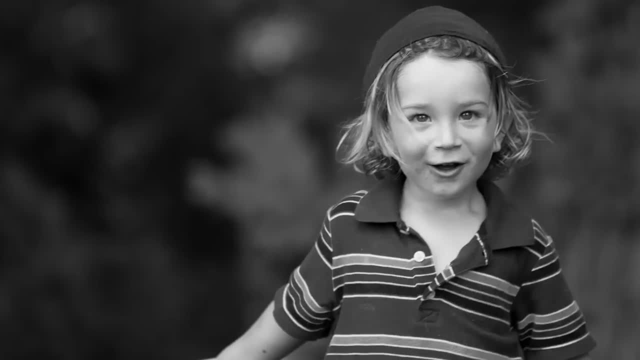 tonal contrast between his skin and the background and it looks really different. I like both photos. I think that the color picture is really bright and sunny for Lane and I think I like that one better. I focus more on his face and his expression. 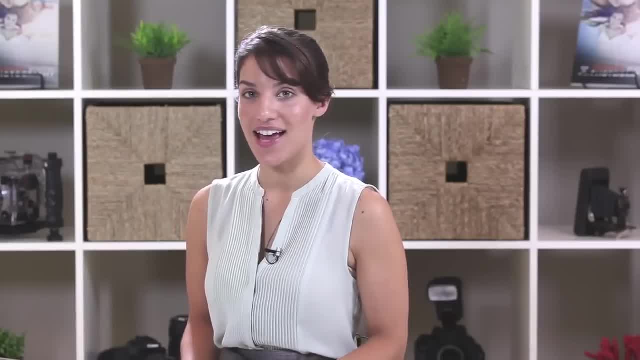 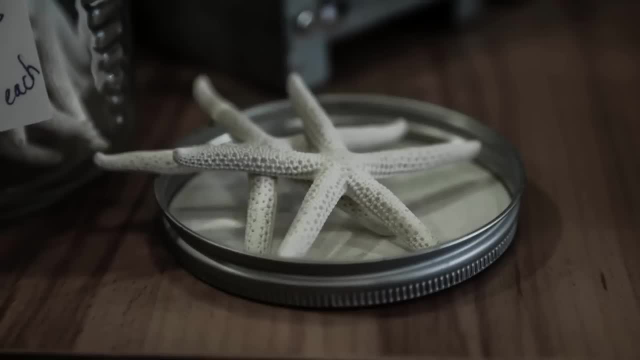 Conversely, a picture that my daughter took of a starfish lacked any kind of color contrast. So you can see here that the starfish and the table they're all kind of beige-y, brown-y tones and there isn't much color contrast. 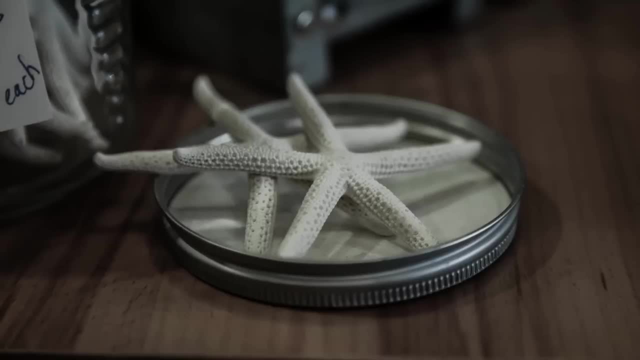 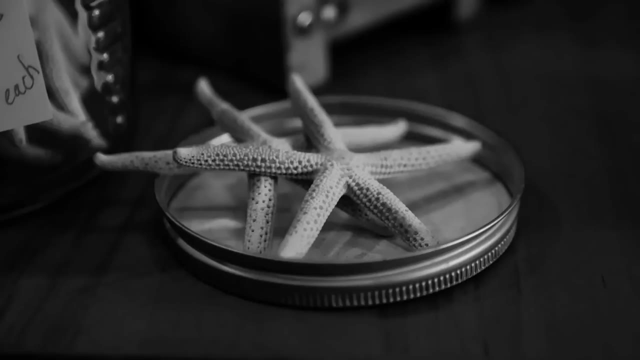 The subject of the picture, which are the starfish, kind of just blend into all of the surroundings. But once I take that picture and I convert it to black and white, suddenly the starfish pop and everything else kind of fades away into the background. So this picture looks: 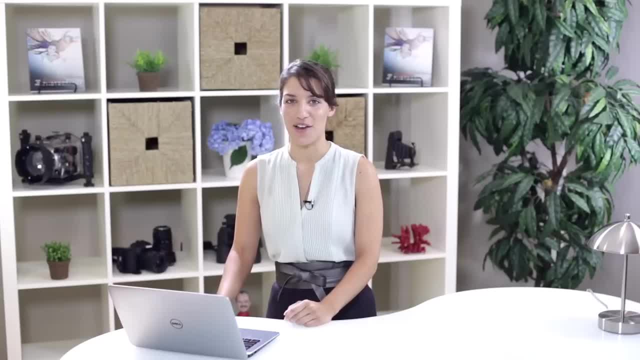 much better in black and white. So, as you can see, there are many elements that go into making a great black and white photo, And now that we have those down, let's go into Lightroom and I'll show you how to start editing your pictures. 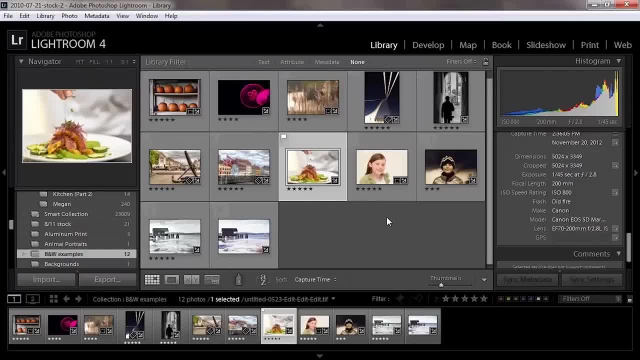 Let's go into my photo editing software and I'll show you examples of a good time to use black and white photography and bad times to use black and white photography. Now I'm using Lightroom 4.. I'm certain there are many other photo. 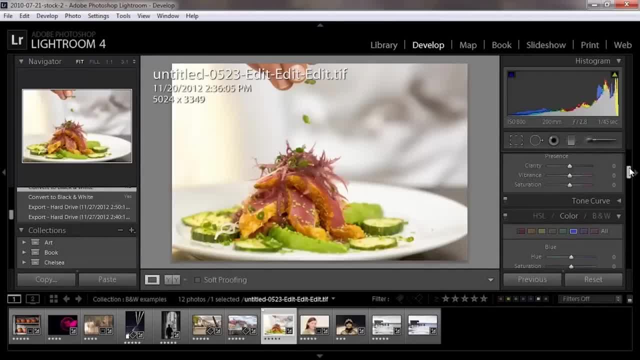 editing softwares that will work just fine As long as they have this option where you can go to black and white and then mix your colors. That's all you'll need. This example is a picture of food, A picture of tuna made by my favorite chef. 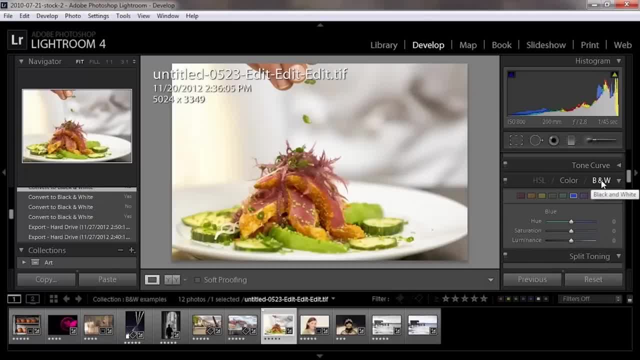 Chris Rao. It looks beautiful in color, It looks appetizing, But as soon as you shift it to black and white, you start focusing on the form in the photo, which is not so appetizing. Another bad time to use black and white photography is: 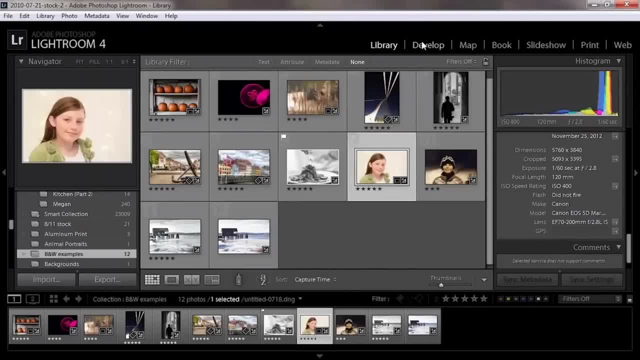 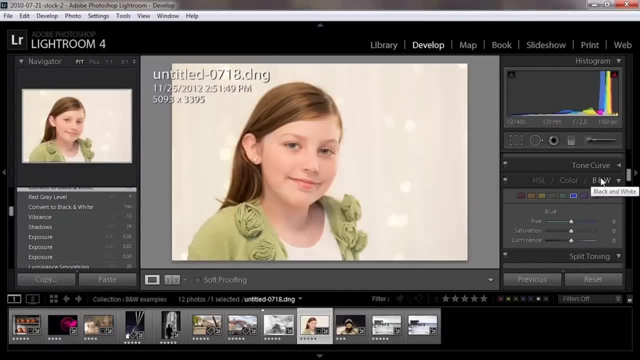 if the soft colors and tones set a mood in the photo, like this Christmas picture that I took of my daughter Madeline, When I convert it to black and white it loses that soft ethereal effect. For me anyway, Maybe some. 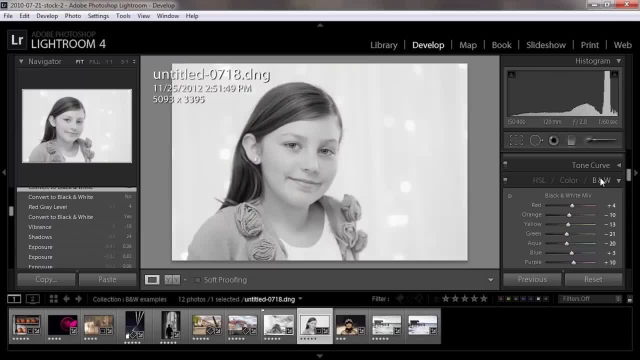 people prefer it, But her skin looks a bit washed out. There's not much contrast and it's a bit uninteresting. Even adjusting the colors doesn't do much. The red channel kind of darkens her lips and her skin and makes it look ruddy. if 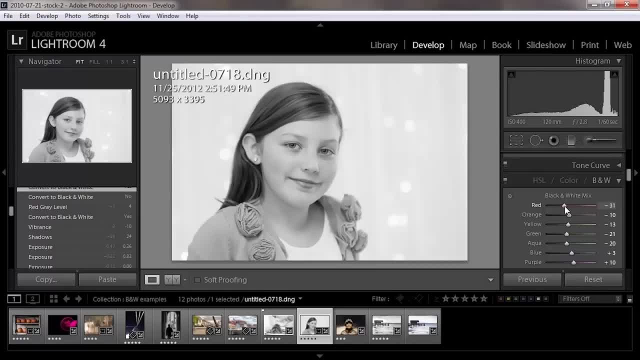 I add too much contrast, The orange will do the same thing. She looks way too tan to be natural there, And when I slide up the slider to create contrast, everything just gets washed away. I prefer this picture in color. Now let's get to a good time to. 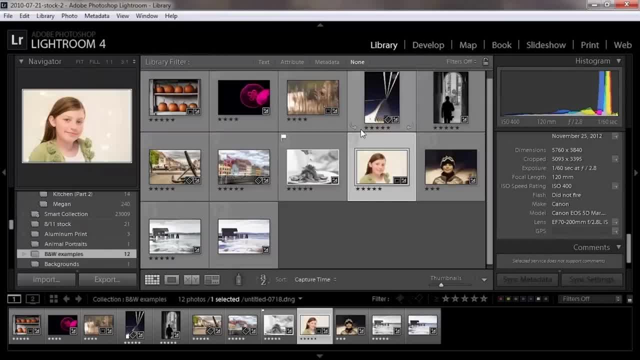 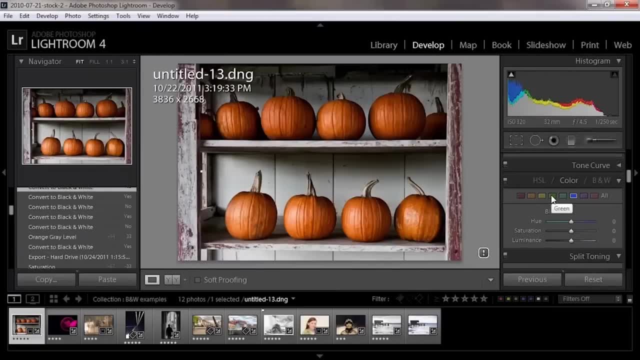 use black and white photography. This picture of pumpkins I took during a little road trip to Vermont. Now you might think that the color looks good, but in my opinion the orange really overwhelms the photo. What I liked about this picture is the rustic. 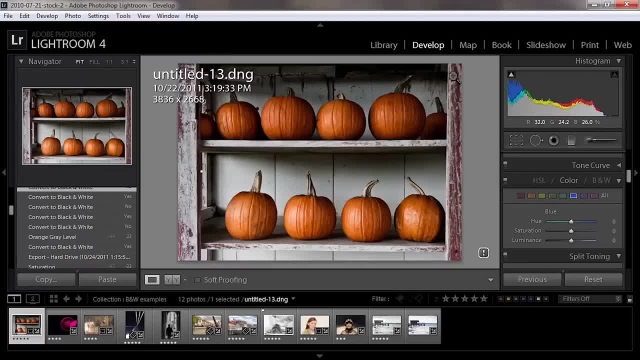 setting. You can see the wood here on the side. It's very weathered and the pumpkins just have so much texture. And when you convert it to black and white and focus on the form of the pumpkins, the picture takes on a whole. 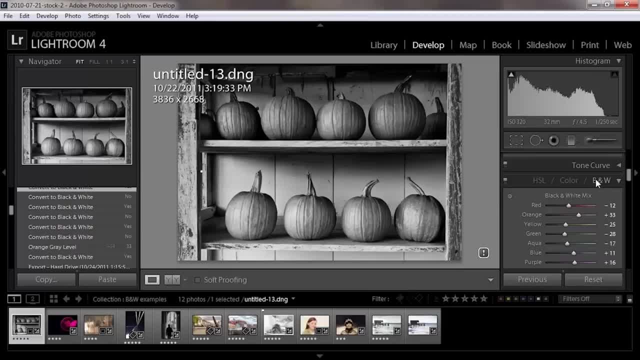 new meaning. One important tip when you have a black and white photo is to make sure that you actually have white in the picture and black in the picture. So you can see, here there's some dark, deep shadows that are black and there are some highlights. 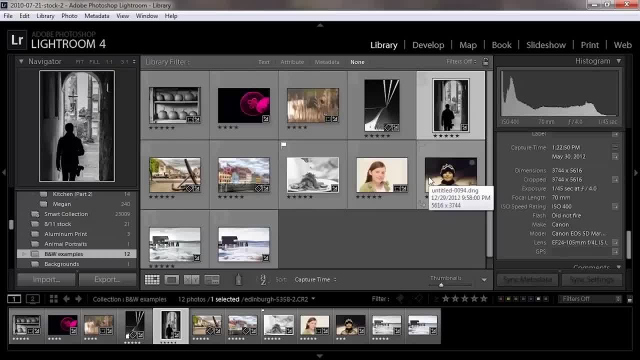 that are pretty much fully white. A picture of Tony in Edinburgh, Scotland, is a great example of how black and white photography can really change a photo. So when I look at it in black and white, I see a silhouette. I see him walking. 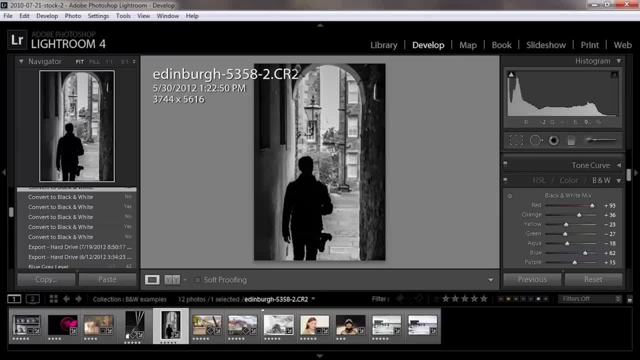 through this beautiful arched doorway and just kind of a vague background. When I convert it to color, my attention is immediately shifted to the green between the two buildings and I notice that there's a person in the background and a sign that seemed to steal a bit of. 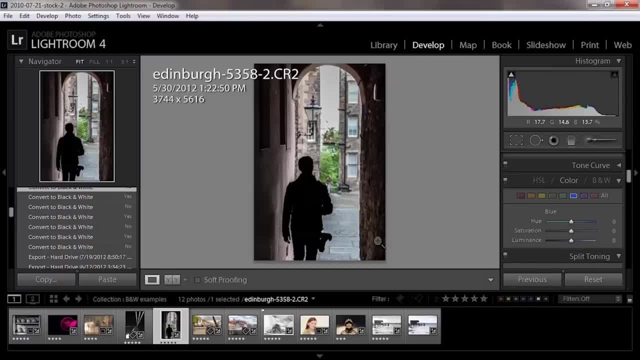 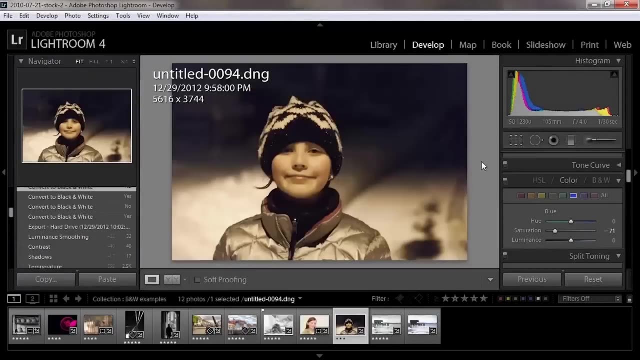 the attention. In this instance, changing the photo to black and white focuses on one form in the picture, making the subject more identifiable. I took this picture of my daughter one night while we were walking in a snowstorm, So my ISO was really high. 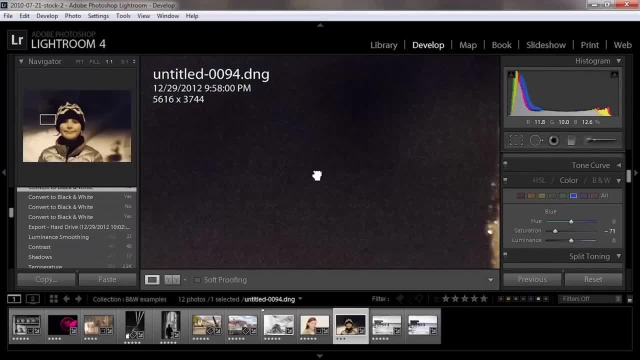 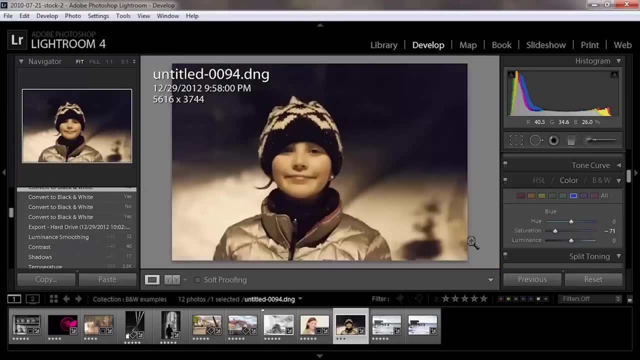 12,800, and this picture is really noisy. It shows it. This is a time when converting to black and white would be a bad idea because, as you can see, as soon as I change it to black and white, the noise becomes even more obvious. 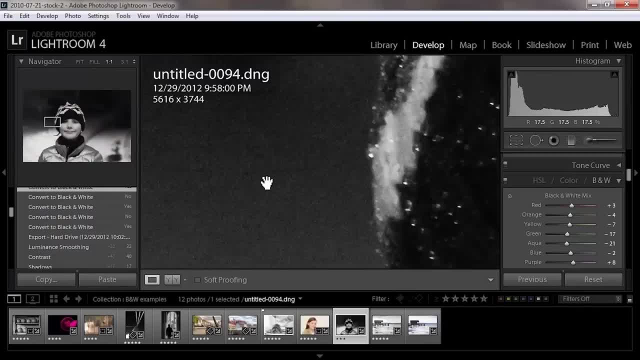 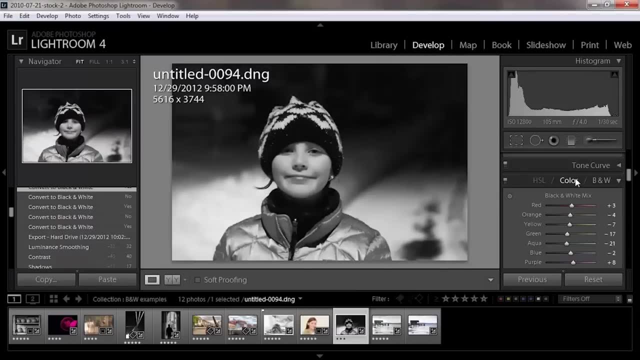 That is a good reason to keep your ISO low, and if you have a picture that's especially noisy, it's probably not a good time to convert it to black and white, unless that's a look that you're going for Now. this picture was taken. 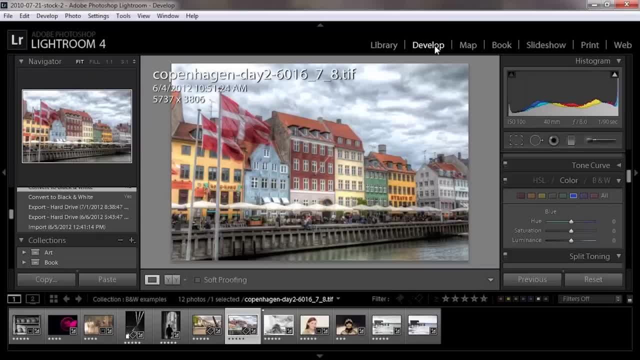 in Copenhagen, Denmark, and it's actually not a picture that I like converted to black and white, but it's a great example to show you how this mixer works. You can drastically change your photo by playing with these color sliders here. You can see that when I change the. 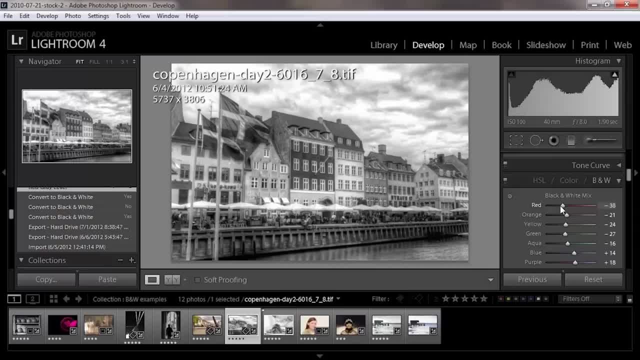 red. I can make it dark or make it lighter. This is important because it creates a lot of contrast in your picture and you have control over making your subject stand out more or less. So if I wanted you to see less of the flags, I would make them. 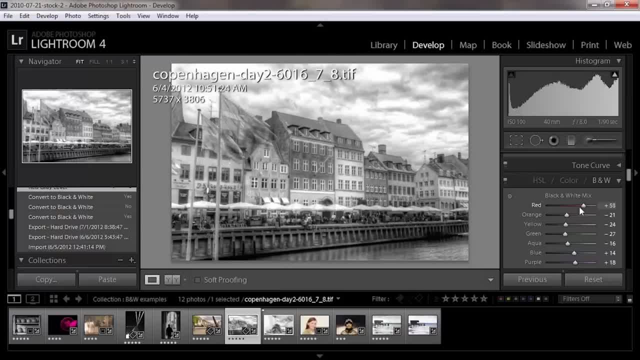 lighter. If I wanted you to see more of them, I would make them darker. Let's play with the orange here and see what that does. The orange channel is bringing out the roof or making it dark Against the light sky. I would probably 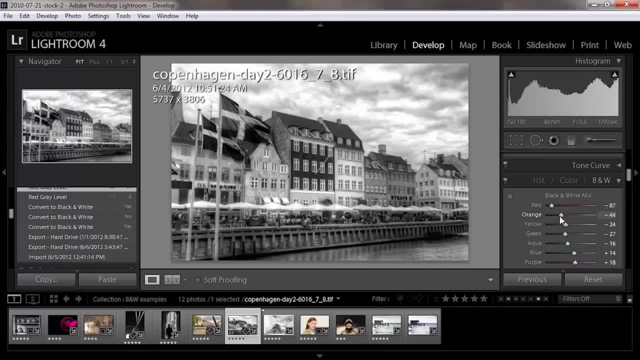 go with the roof being a little bit darker. It brings it out a bit more and it brings out the structure of the buildings. So you can see just by playing with the colors in your black and white photo, or the color channels rather, since they're not color. 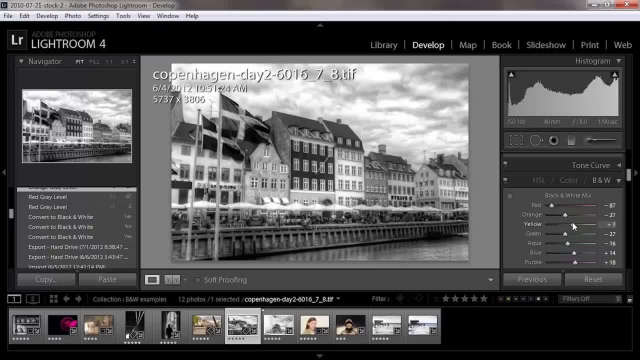 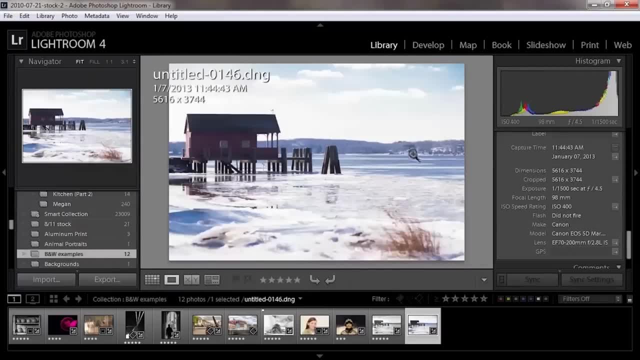 anymore. you can drastically change what your picture looks like. This picture that I took of a boathouse in Lyme is a great example of how black and white photography brings out form and composition. When this picture is in color, I feel like my eyes. 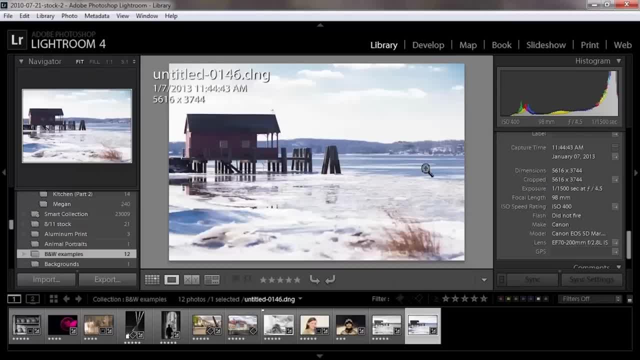 are fighting with it a bit. There's a bit too much going on. We've got this tuft of grass here, the boathouse, the background, the sky. there's a lot going on. My eye doesn't really want to. 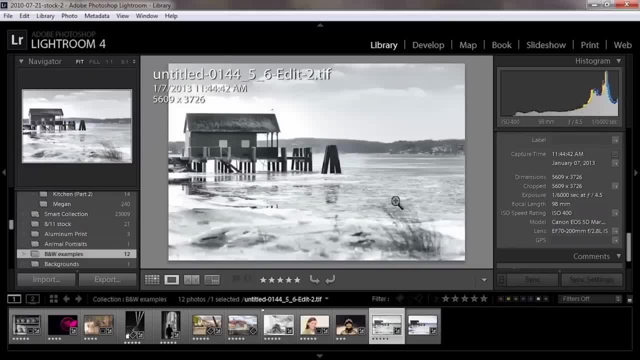 rest on anything. I already converted the photo to black and white and you can see that it anchors your eye a little bit. You've got these two subjects. You're not distracted by the color of the boathouse. The red was a bit. 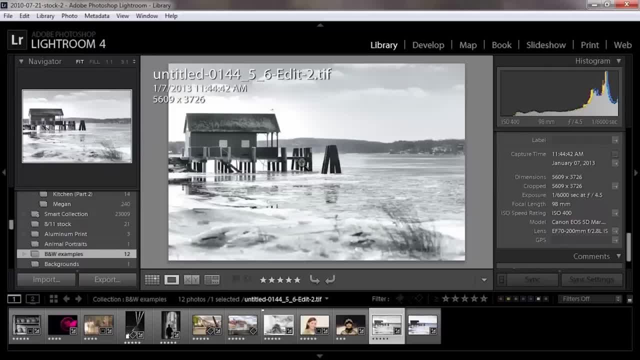 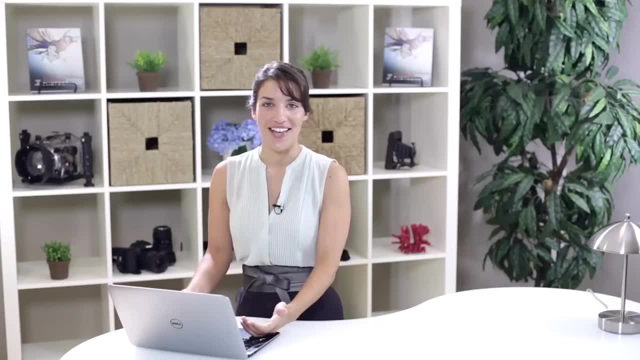 bright and you can really focus on the form, the reflections and just the peacefulness of the scene. So I thought this was a great photo in black and white. So that's pretty much it. Now you know how to take and edit some black and white photos. 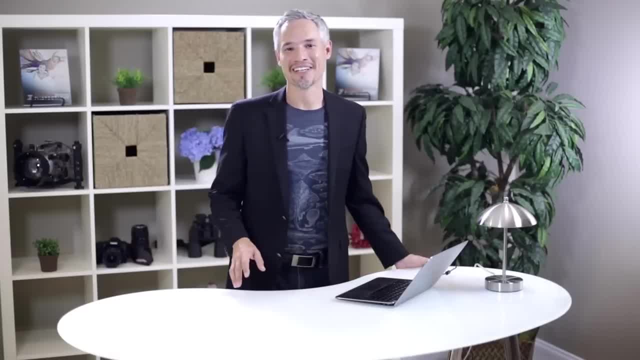 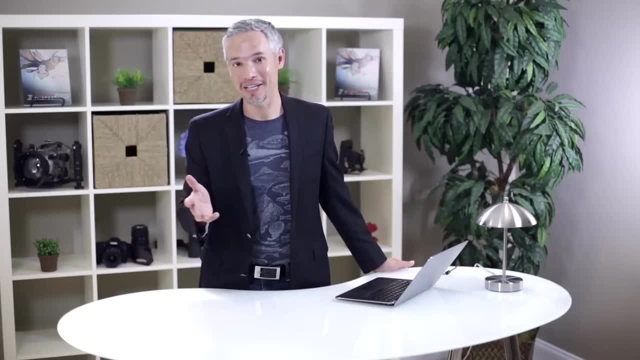 Let's hand it off to Tony and see what he's up to. Thanks, Chelsea. Now I'd like to show you a few practices that you can do on your own to help reinforce these techniques, Because, after all, just listening to me isn't going to make you a great. 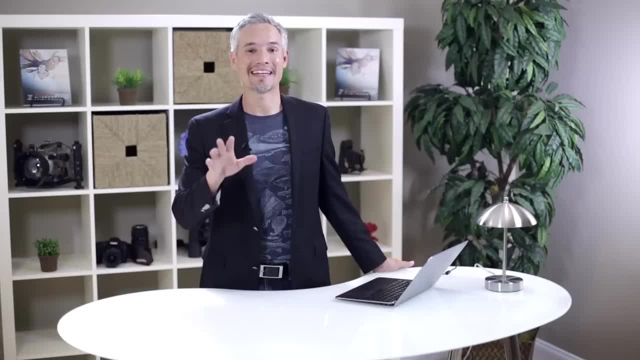 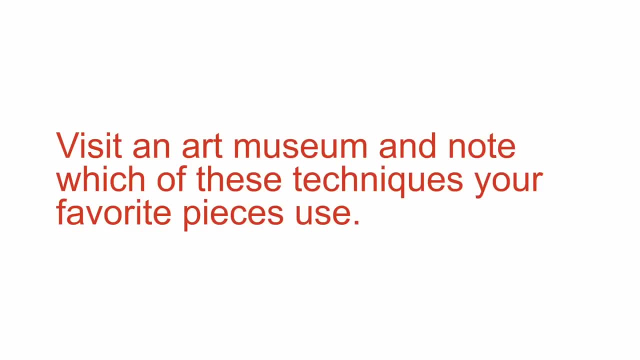 photographer, You've got to get out there with your camera and get it done. So let's look at some compositional practices Up first, I'd like you to visit an art museum, And it doesn't even have to be photography, It can be paintings and 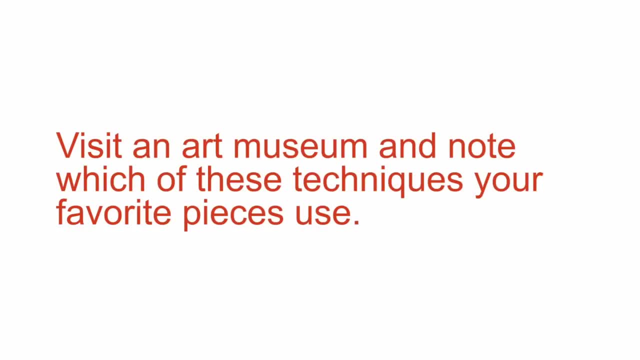 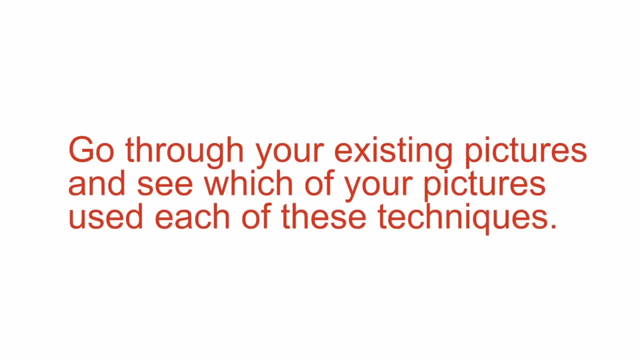 sculptures. As you look at the art, I'd like you to note which of these compositional techniques your favorite pieces use. You can also simply go through your own photo library and see which pictures you have that use these compositional techniques, even if it wasn't. 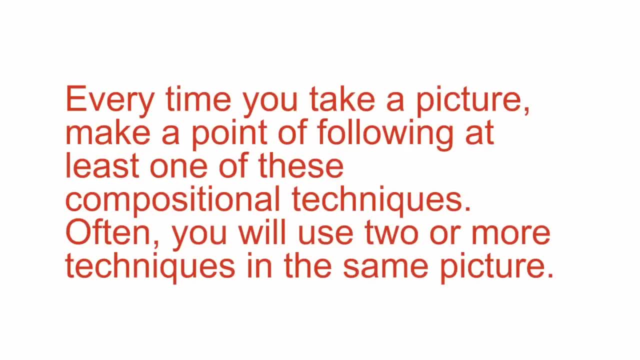 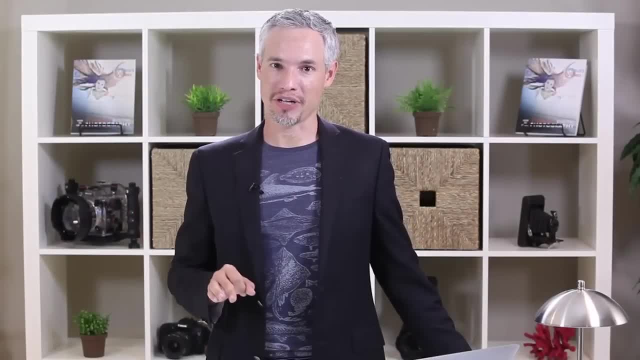 deliberately Anytime you're out taking pictures. I'd like you to make a point of following at least one of these compositional techniques. I use at least one compositional technique in every single picture I take. I bet the rule of thirds is probably the most popular. 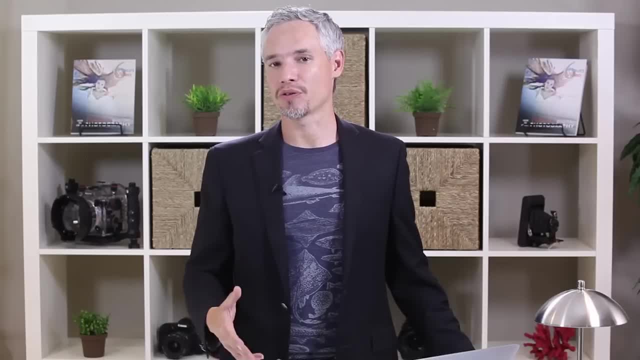 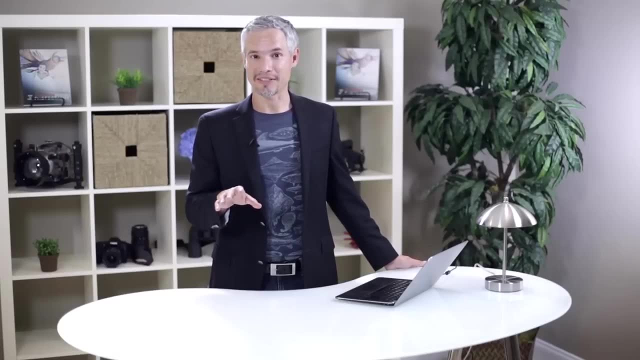 Filling the frame is probably the second most popular. That's important for wildlife, And symmetry is probably the third most popular technique. But it's also great to combine multiple techniques together, So you could use symmetry and the rule of thirds If you haven't used. 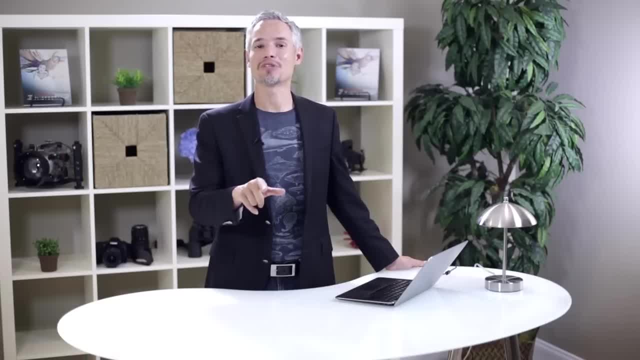 one of these techniques, then I'd like you to seek it out, Find a subject where the technique will work and take a picture of it, Because once you actually use it to take a picture, that's when it's actually going to get burned in your brain. 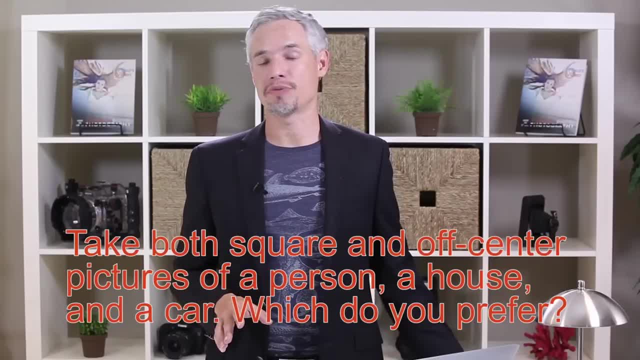 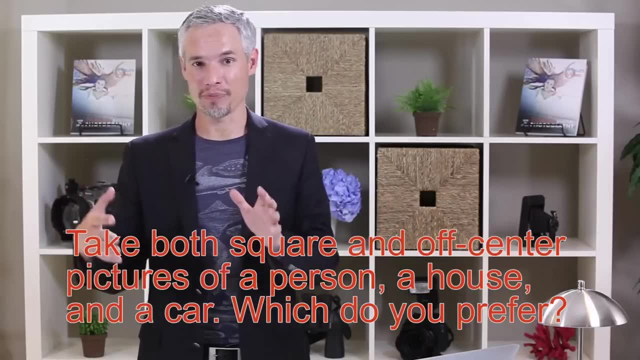 not when you hear me talking about it Up. next, I'd like you to find a subject- It could be a house, a person or a car- And take both square and off-square pictures of it so you can get a sense. 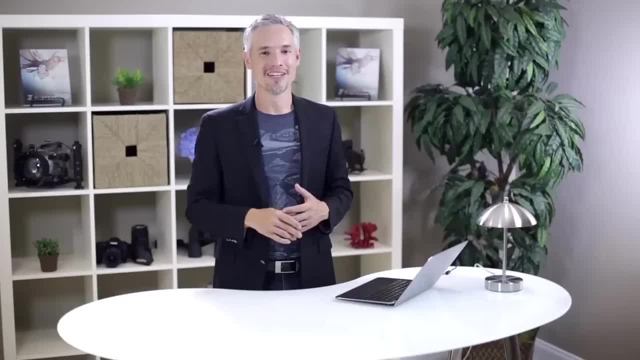 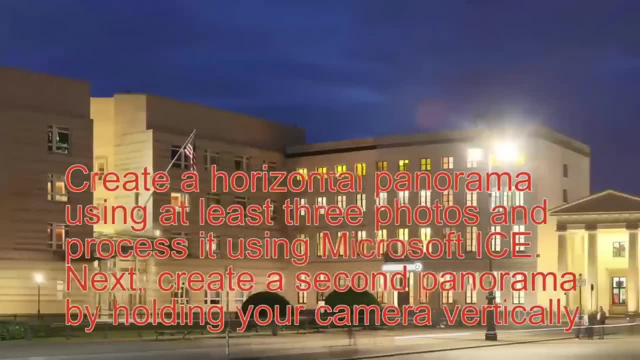 for how it changes your feelings about the subject. So use depth in pictures and see if that changes the tone in the picture. Lastly, I'd like you to get out there and take a panorama, Follow the instructions that I provided in Berlin And just make sure that you know. 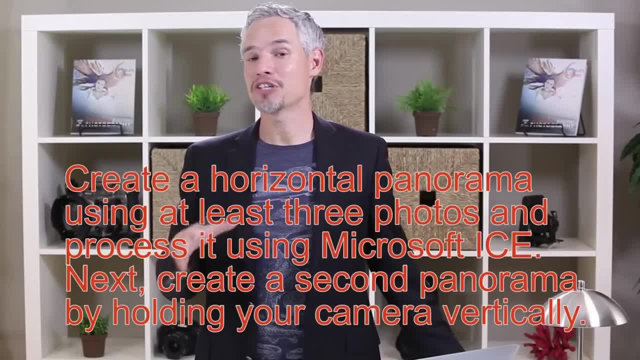 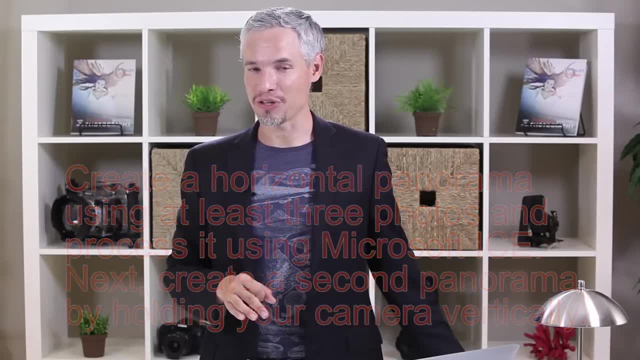 exactly what you're doing and that you have the software ready, Because you never know when you'll need to take a panorama. You could be anywhere and need to take a wide angle shot and not have a wide angle lens with you. With panorama techniques, 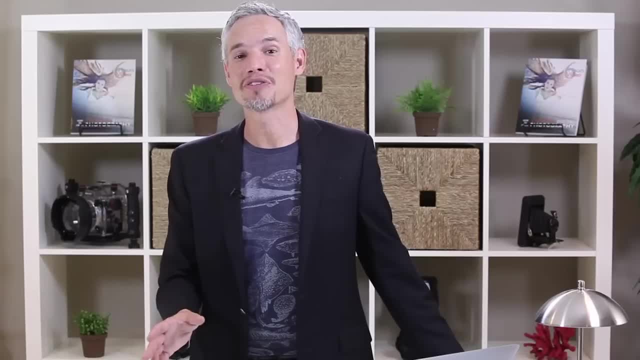 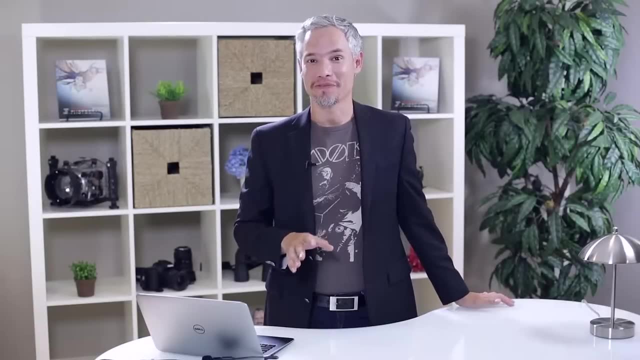 you're always ready to go as wide angle as you need. Thanks so much for watching my composition video and I hope to see you in the next one. Hi, I'm Tony Northrup, and for my stunning digital photography video training series, I'm. 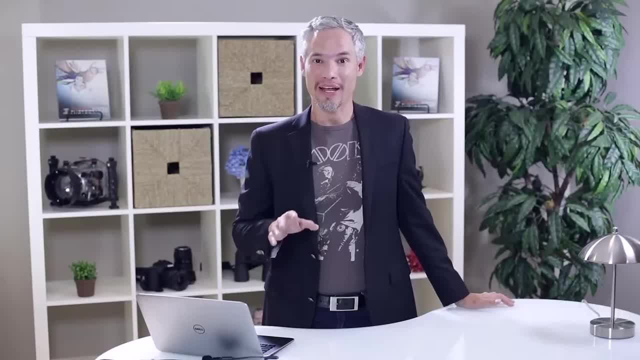 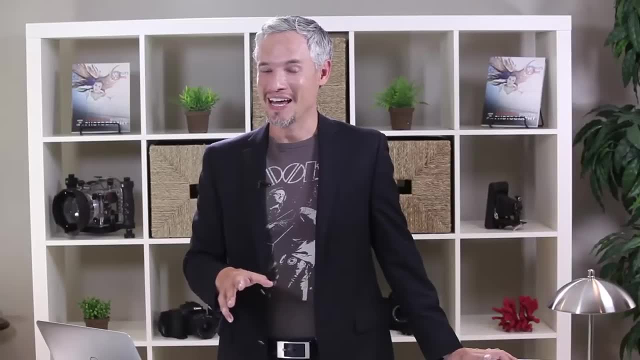 going to talk about lighting. Lighting is one of the most important elements in photography. There's an old saying that goes: no matter what you're taking a picture of, the subject is the same light, And you can treat that philosophically or you can treat it completely. 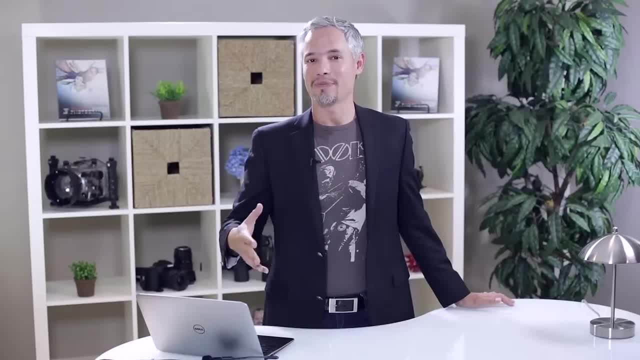 literally and scientifically. Philosophically, light makes your subject come alive, And light is the difference between a boring and flat picture and a dynamic and exciting picture. And if you think of it literally, the camera is just capturing photons that are bouncing off of subjects, just like. 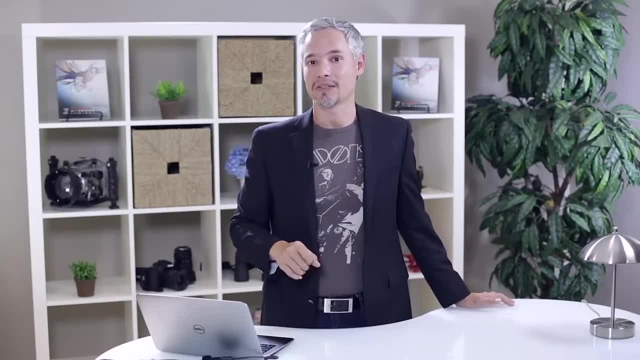 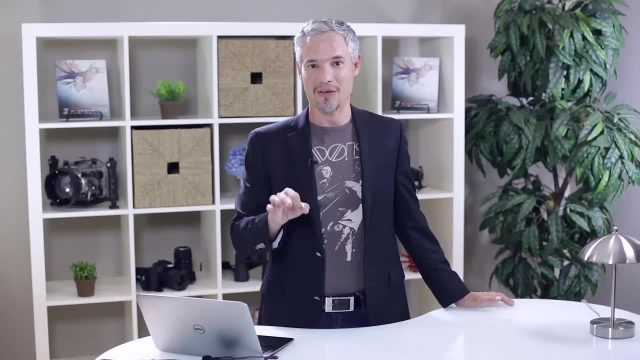 our eyes do. You're literally just capturing the light that's bouncing off of things. That is what we see and that's how our brains process it, and our cameras work exactly the same way. So it's really critical to understand light, even though it's not as 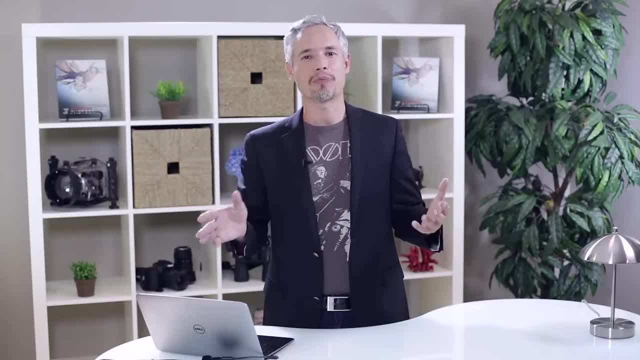 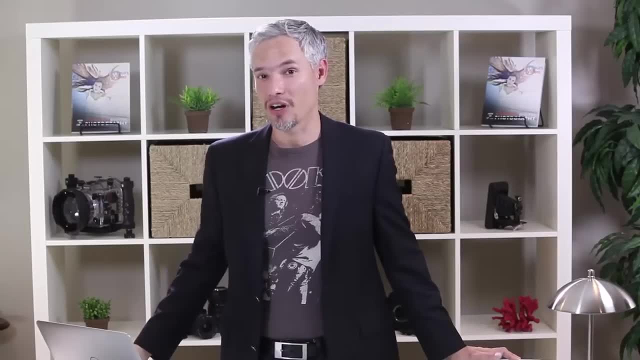 technical as some things like aperture and f-stop and megapixels. Light is the difference between good and great and stunning photos. So let's talk about the difference between hard and soft light. Hard light comes from small light sources that are far away, like 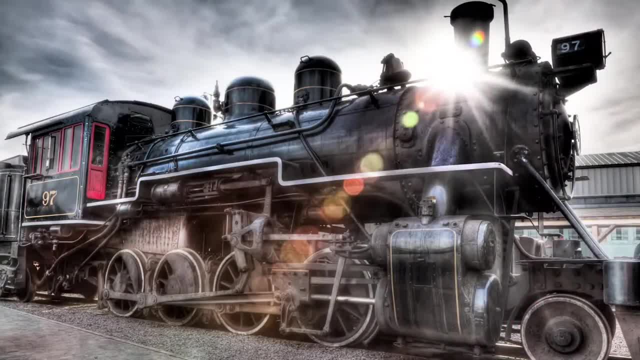 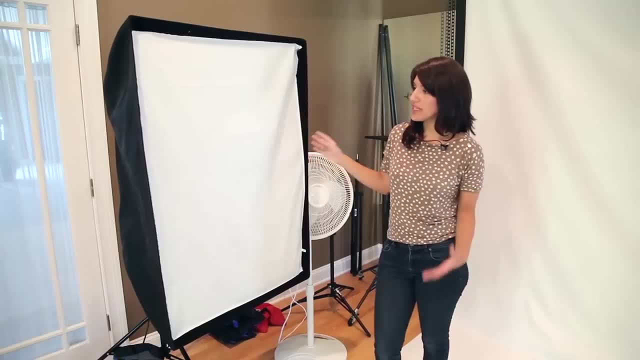 the sun. Well, the sun's not small. The sun is huge, But it's so very far away that it's kind of small to us, especially compared to, say, a big soft box that might be here or even a flash on the camera. Now the quality. 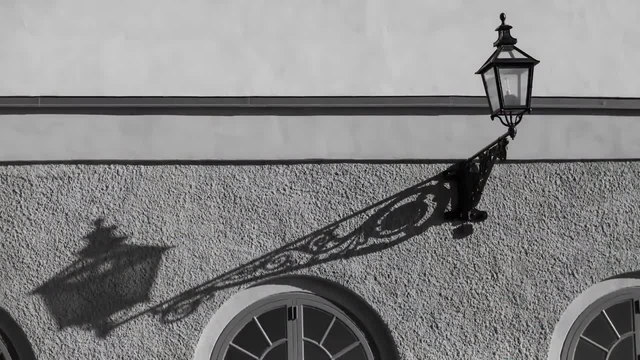 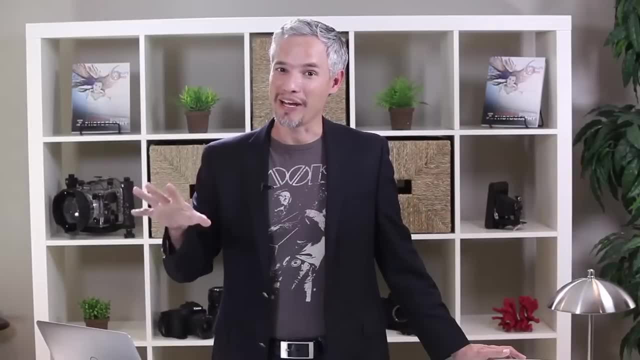 of hard light are really distinct shadows And, if you think about it, a shadow isn't necessarily a black or white thing. There's always a little bit of a transition from the bright areas that are illuminated directly by the light source and the dark areas. 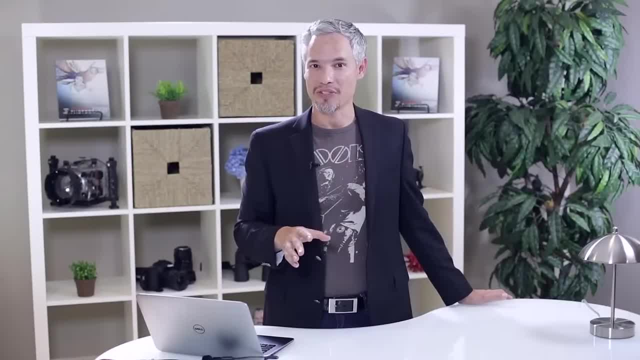 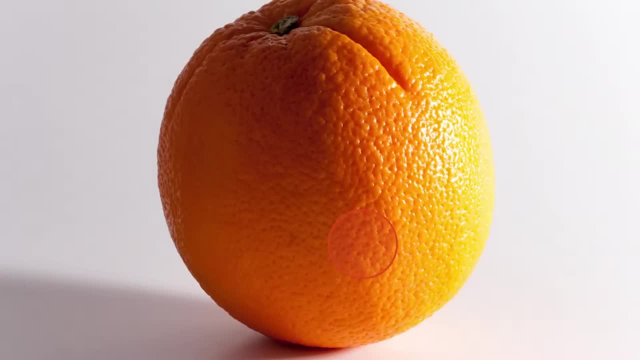 that don't get illuminated. These areas are called mid-tones, And the characteristic of hard light is that these mid-tones are very short. It goes from bright to completely dark very, very quickly. Soft light, on the other hand, is: 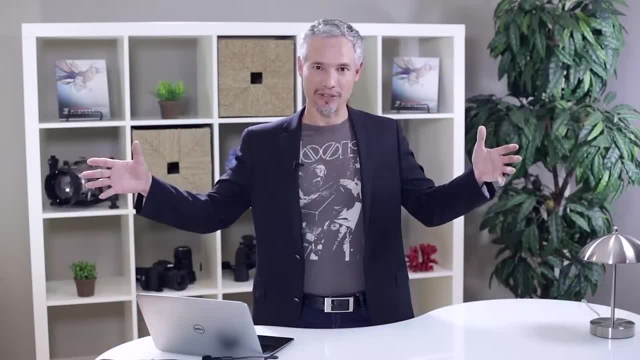 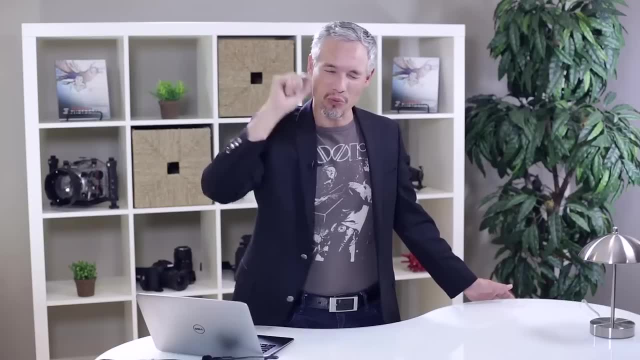 made by light sources that are fairly big and relatively close to you. That means that instead of getting all the light coming from one little point and striking you from this one specific direction, you might get light that's coming from over here and hitting your face here and coming. 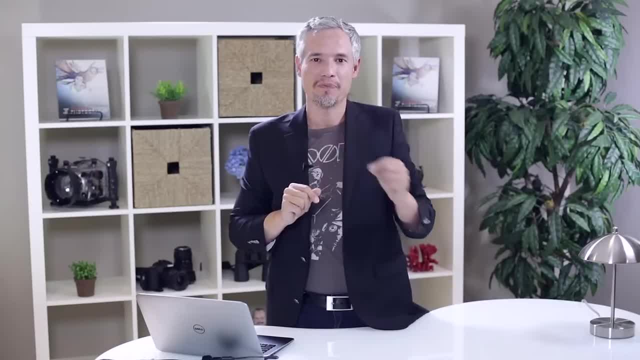 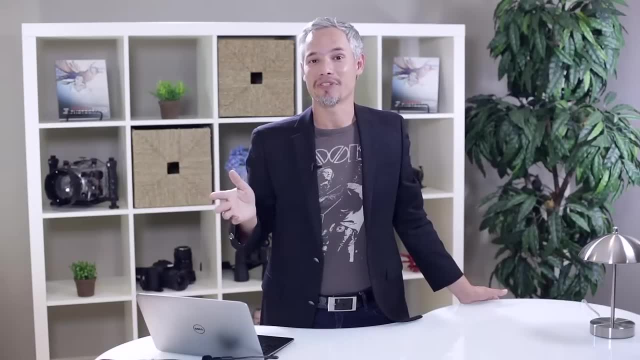 from over here and then coming from this part here and this part here, We see soft light on days when it's bright out but there's an overcast sky, Because you know what happens is the sun hits those clouds in the sky and the sky 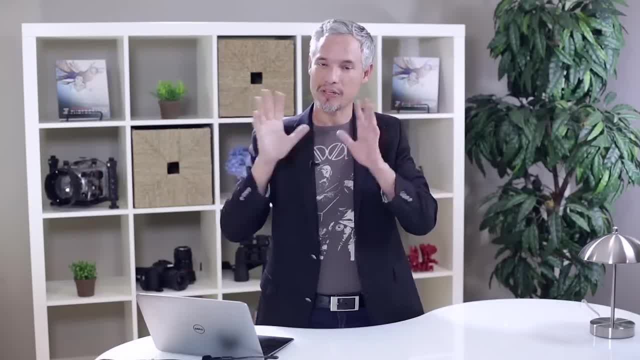 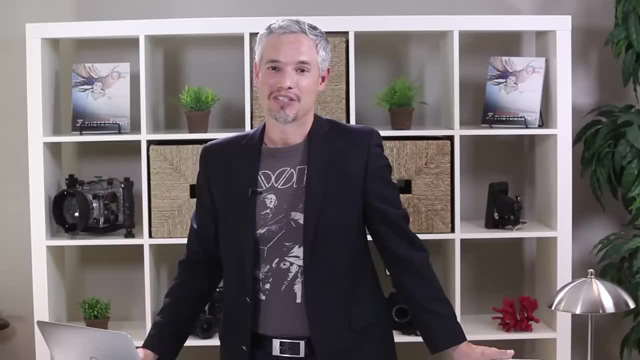 acts as a big diffuser, bouncing the light really from hundreds and millions of little sources, And that's very different than a clear day when all this light is coming directly from the sun. So let's look at a few example pictures Now. the most exciting: 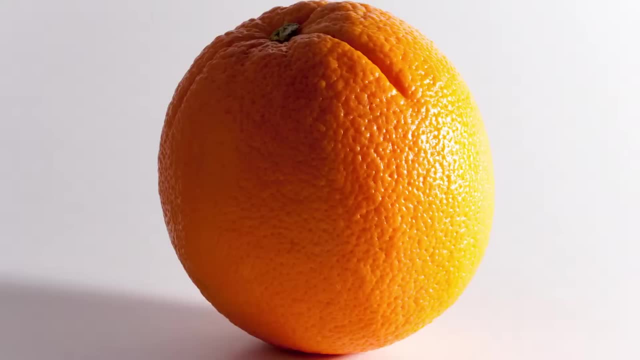 photo. I know This is just an orange, but it's lit from camera right by a flash that's fairly close to it and is a fairly small light source. Therefore it has hard light. Now you can see off the left side of the picture. 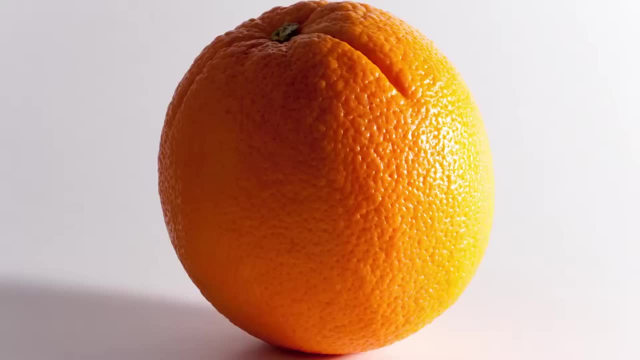 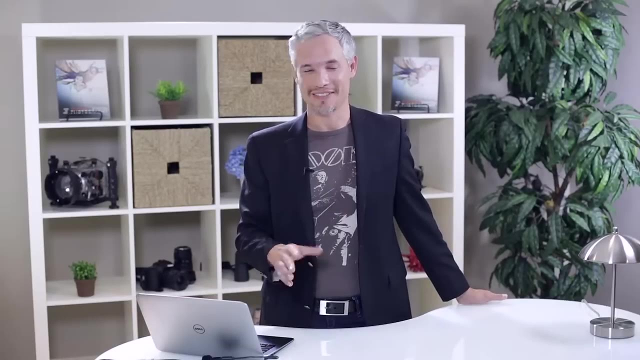 there's a very distinct shadow cast by the orange. You can also see an awful lot of texture in that orange right Now. the reason I used an orange here instead of somebody's face is it wouldn't be flattering light for somebody's face at all. Can you imagine if that was? 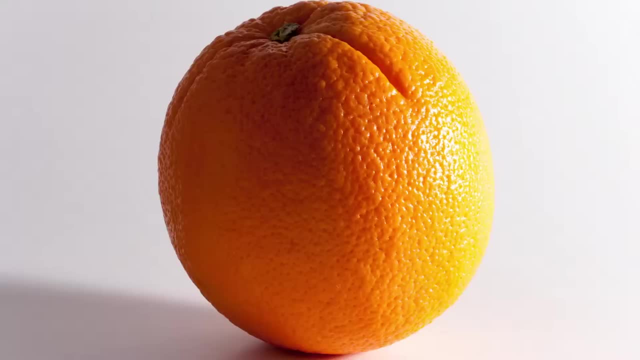 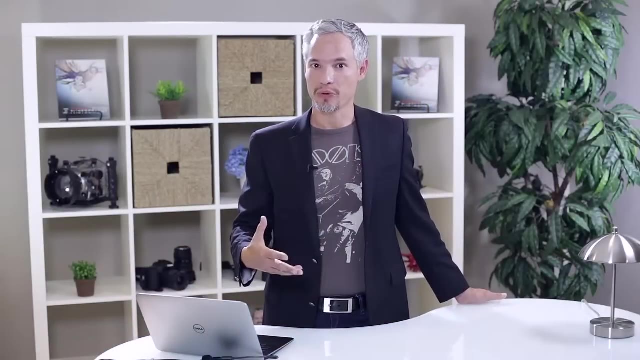 your pores. So I substituted an orange, because I wanted to show you that hard light can be very unflattering to skin. On the other hand, for still life subjects, it helps to really show the texture of it. Here's another example of a photo with: 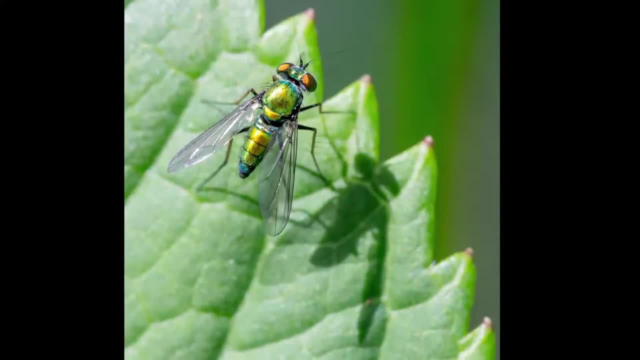 hard light. I captured this fly on a leaf and you can tell that the sun was out and there was not a cloud in the sky, because the shadow of that fly is very, very distinct. That's a quality of hard light: Nice, sharp shadows, And shadows can be a. 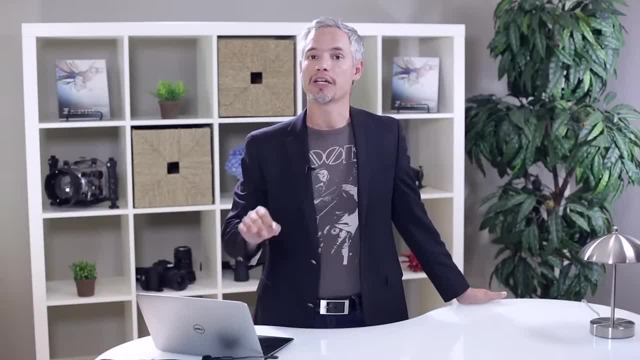 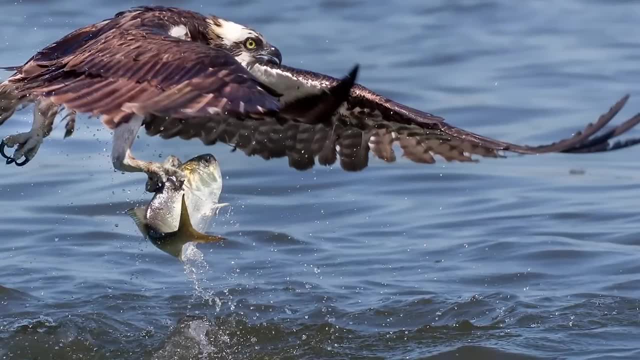 great subject or a great compositional element in your pictures, but you're going to need hard light to do it. Let's look at another photo. Here's a photo that I took of an osprey catching a fish. The sun was behind me and close to the horizon, and 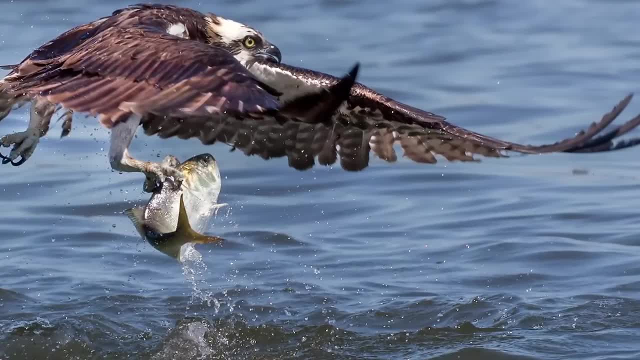 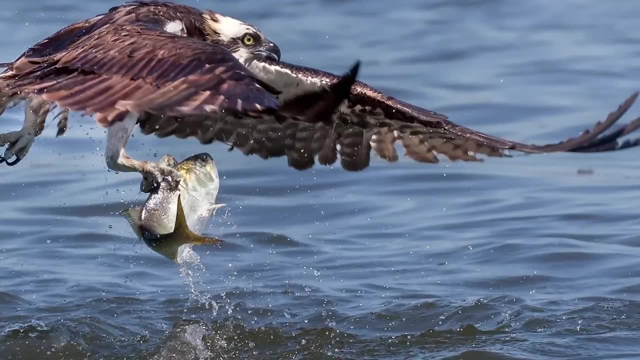 I think you can tell from the picture that it's using hard light First. you can tell by looking at the catch light in the fish's eye, But you can also see fairly hard shadows on the legs and the dark parts of the fish. For a photo like: 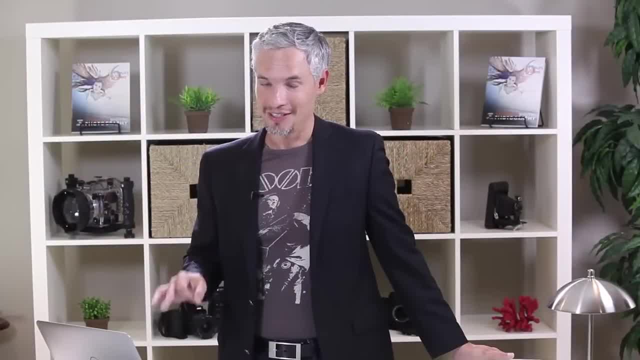 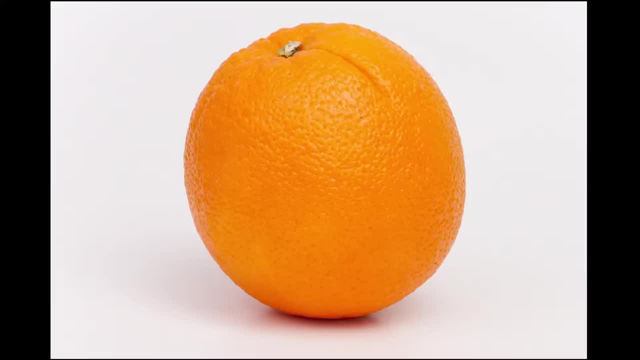 this hard light is great because it shows an awful lot of detail. Soft light hides detail like the pores in your face. Here's that same orange again. I didn't move it an inch. All I did was I turned the flash off. Now this orange is instead. 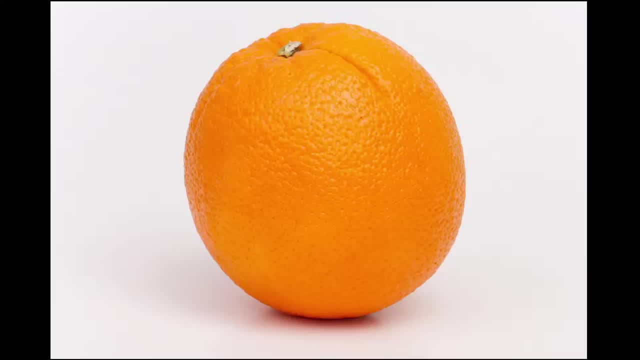 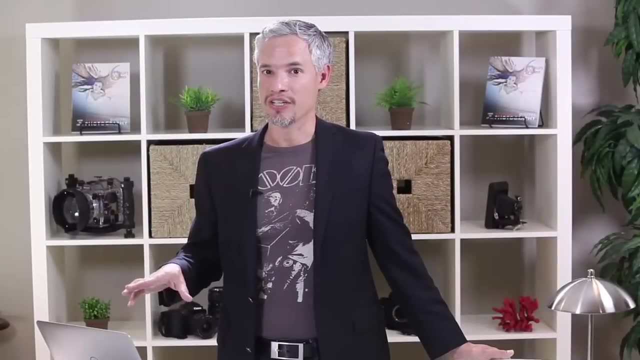 lit by the ambient light in the room and because I just had white ceilings and there was light streaming through the windows, the light was very soft because there was no hard light from the sun reaching the orange. Instead, all the light that was reaching the orange was bouncing off the 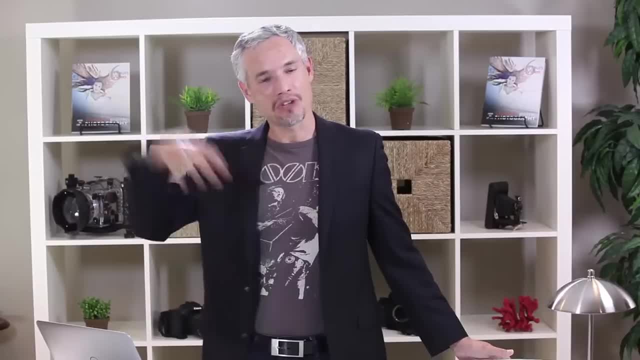 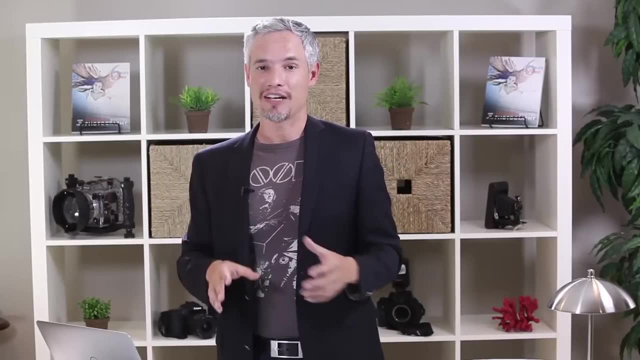 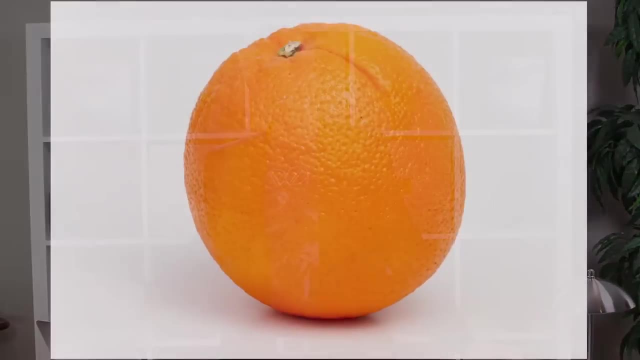 walls and floor and the ceiling of the room, And because all that light was reflected in different ways, it created a perfectly even shadowless lighting for the orange. Now, as you can imagine, this would be much more flattering lighting for a human face. right, You can hardly see any of the 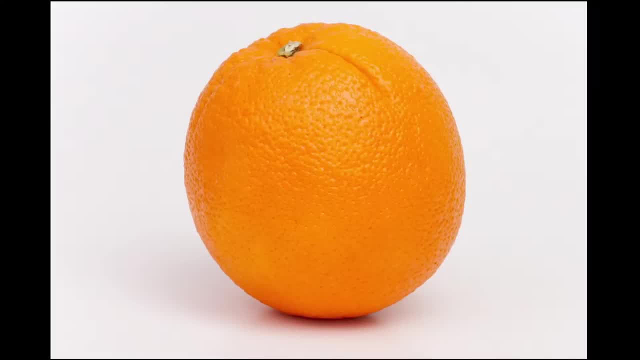 texture in the orange. It might not be as compelling of a photo of an orange, though Now looking at this photo, you can see that your eyes are drawn to the circular shape of the orange. If you look at the photo of the hard lit orange, you'll notice more. 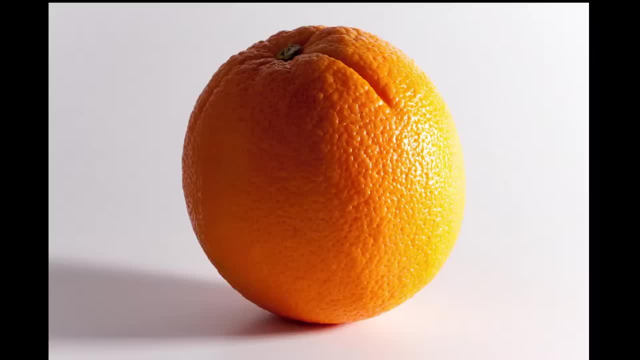 of the three dimensional form. That's because the hard light was coming from the side and casting a shadow on the far end of the orange. Without that shadow there you can't pick up the texture nor the three dimensional form of the orange. So what the soft light gave us was 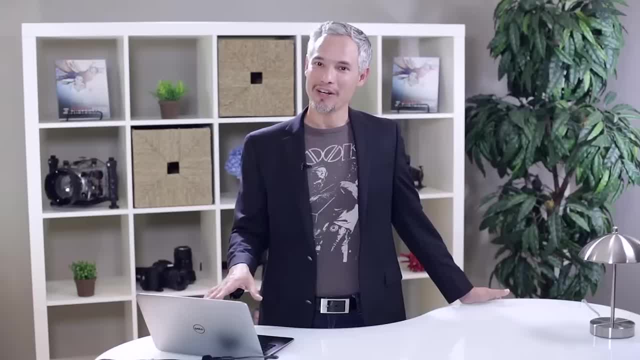 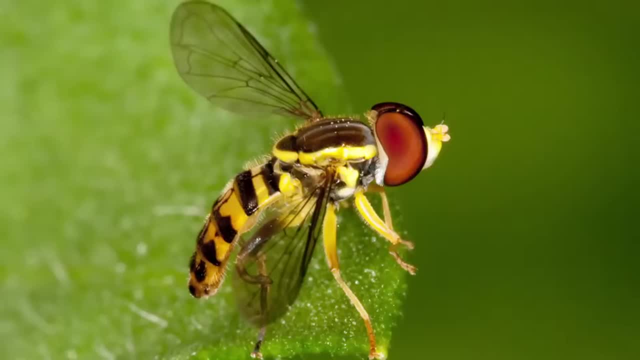 this very formless shape, but for skin it would be very flattering. For an orange, well, you're not capturing the spherical shape of it, so you might have missed the mark a little bit. Here's a soft lit picture of a fly. Now, looking at this picture, you can see it's very 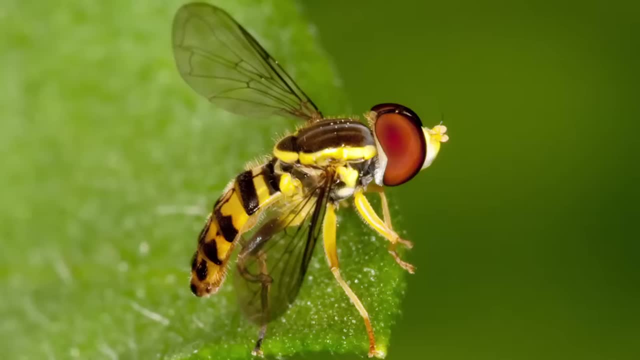 different from the hard lit one. There's absolutely no shadow. There's also not quite as much detail there. However, the lighting itself might be a little more pleasing overall, And here's a soft lit picture of an osprey Again, even though 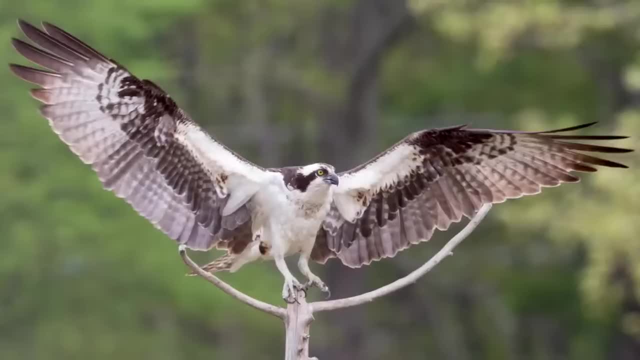 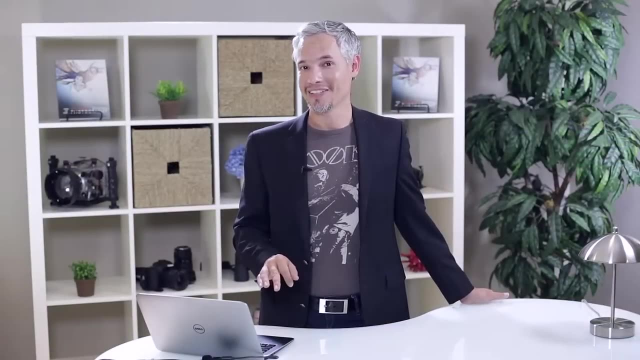 they were taken at about the same distance. you don't see nearly as much detail in this picture, and that's because it's soft light. If you want to capture detail, you need to get that hard light. If you want flattering light, you might want to go with soft light. 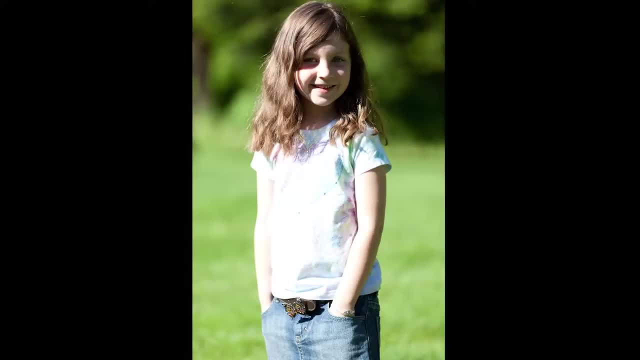 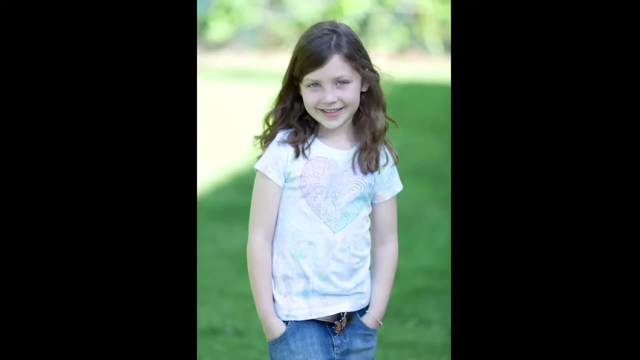 Here's a picture of my daughter. Do you think that's hard light or soft light? Here she is. I just had her step forward a few feet. Now you can see that this one is the soft light and it's therefore much more flattering. 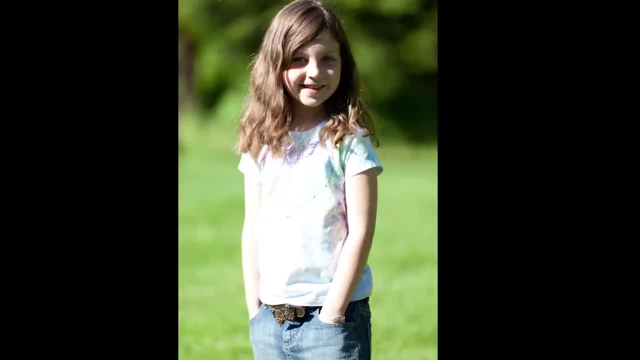 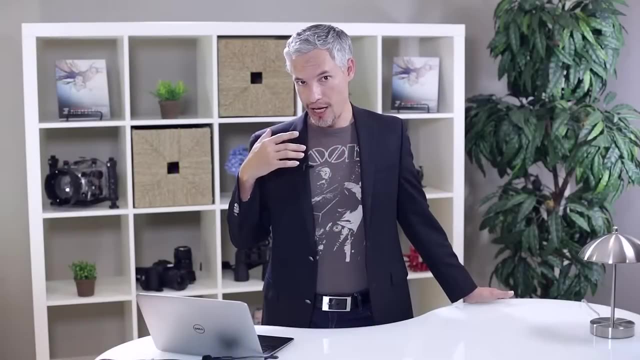 Looking back at that hard lit photo, you can see that she has really distinct shadows on her face, as we call them raccoon eyes. They're cast by the light hitting the brow and then casting a shadow on the eyes, and that's not at all what you want. It does show a lot. 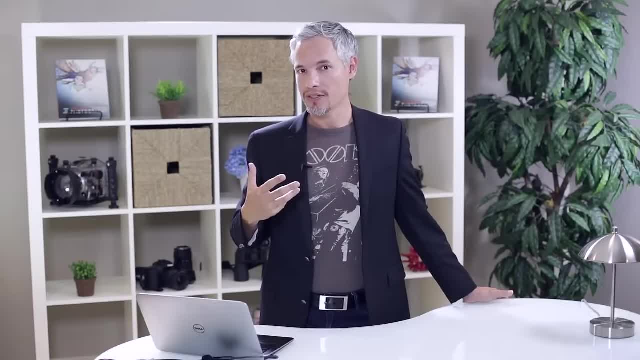 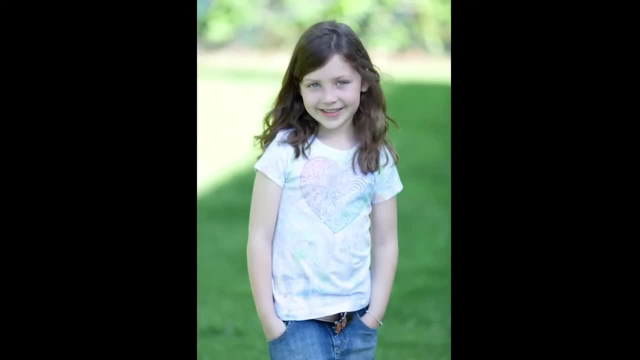 of the form, the 3D shape of the face, but overall it's not especially flattering for portraits. For portraits, you're almost always going to want to try to move your subject into soft lighting. Now, I mentioned earlier that no matter what your subject is, you're always taking a picture. 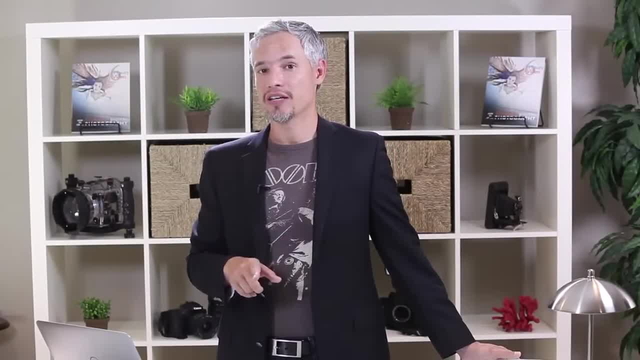 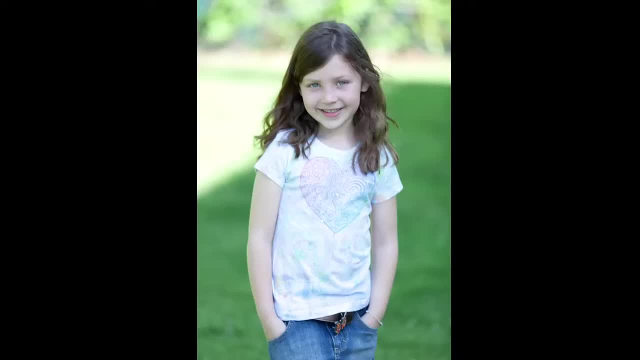 of light and Madeline. even though she's in the shade, she's still being lit by something right, Or else my camera wouldn't be able to expose her and she would be completely black. In this case, she's being lit by light that's being reflected off of everything. 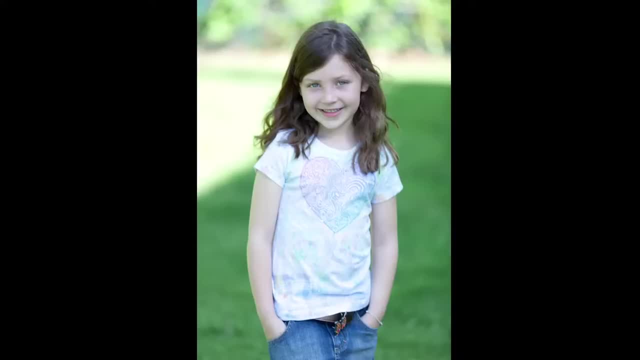 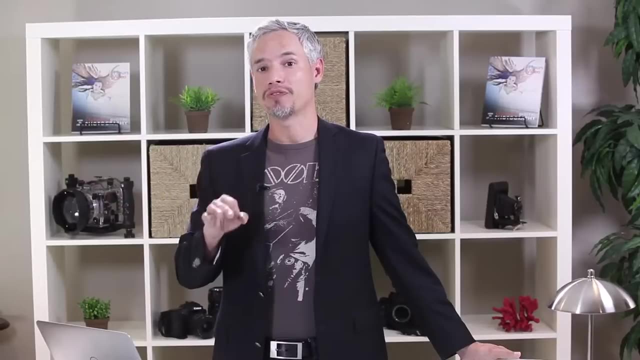 Some of the light is being reflected from the humidity in the sky. That's a big part of the reason there's still light and shadows, and it's not just pitch black. She's also being lit by light that's reflecting off of the grasses. 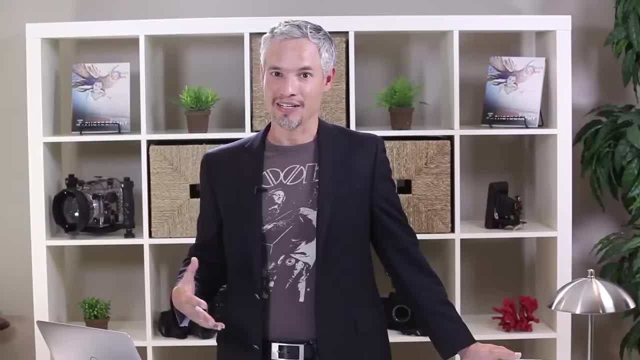 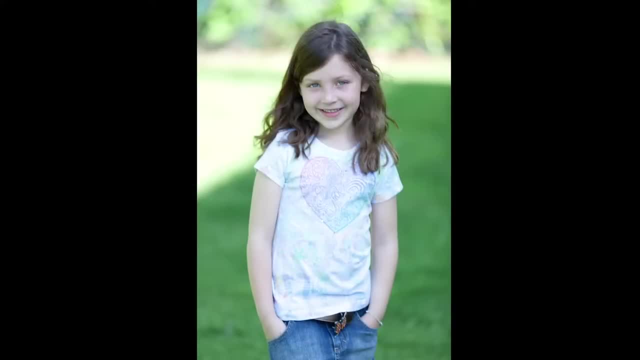 and the surrounding buildings that are in the direct sunlight. So this gets to be pretty complicated because she's actually got hundreds of little light sources around her and each one of those light sources can change the light a little bit, and that makes it a little more unpredictable than. 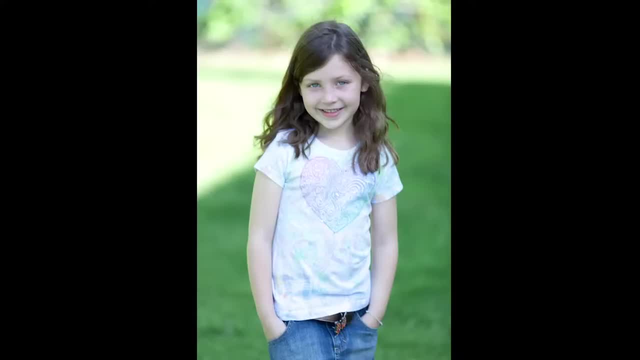 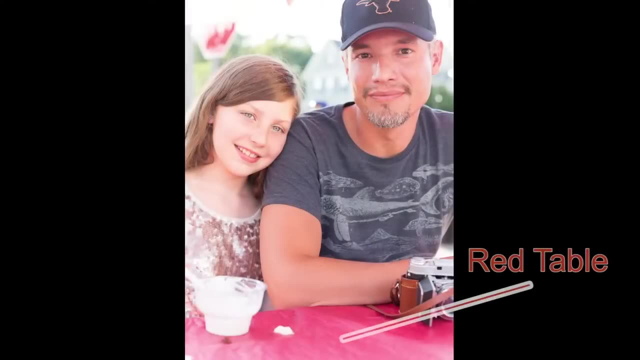 just simple, hard light. For example, the light that's coming off of the grass is going to have a green color to it, And if you look at pictures of people that were taken, maybe laying on the grass or near leaves, you're going to see a green cast of them. 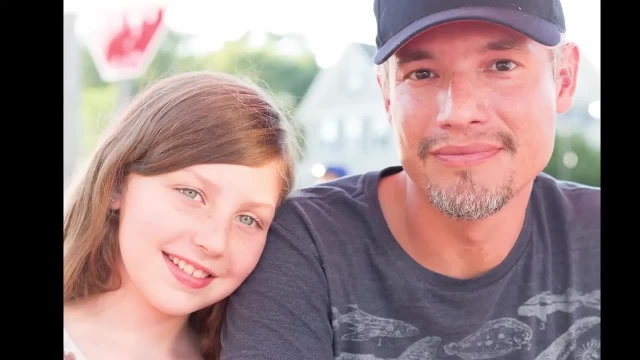 That actually happens and I get a lot of questions from readers and viewers of my video series asking like: why is my subject green? And often the answer is simply: they're standing next to something green. If they're standing next to a red car, they're going to have a bit of red to them. 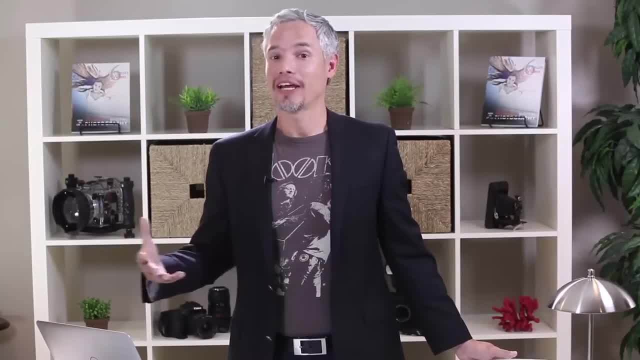 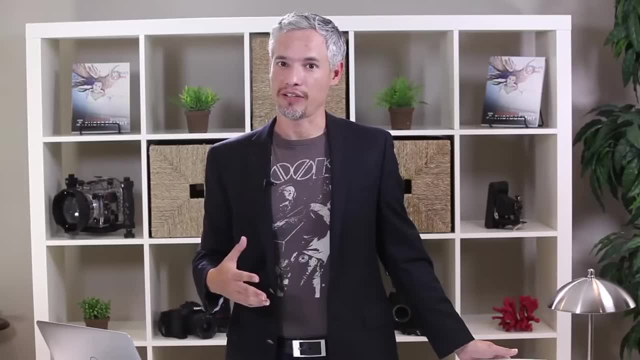 Anytime you're not in direct light, when you're indoors or you're in the shade- your light is actually coming from a million different places, and each one of those things that it's bouncing off of is changing the quality of light a little bit. So take a minute. 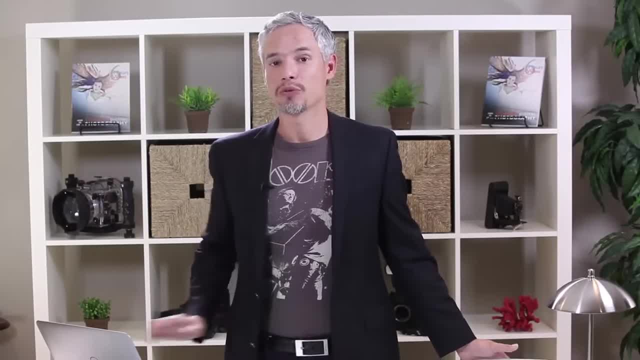 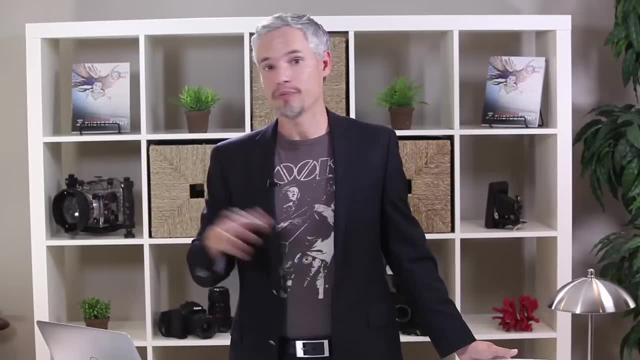 pause the video and look around the room and see where you're going to see different light sources are. Maybe you have the sun streaming through the window and that's a good example of hard and direct light. Or maybe it's completely dark outside and you have the interior lights on. 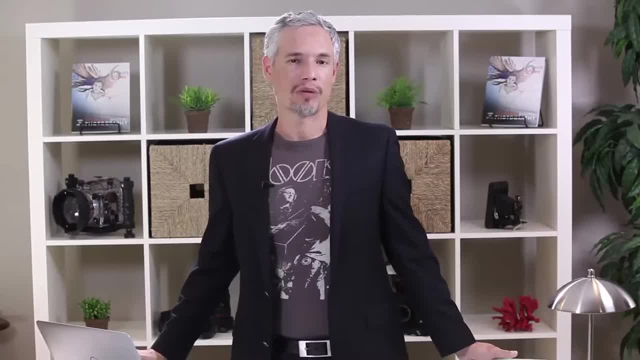 That would mean that you might have multiple different direct light sources, But I bet most of your light is going to be indirect. since you're probably indoors right now, I want you to think about where the light is bouncing off of and how that might impact your pictures. 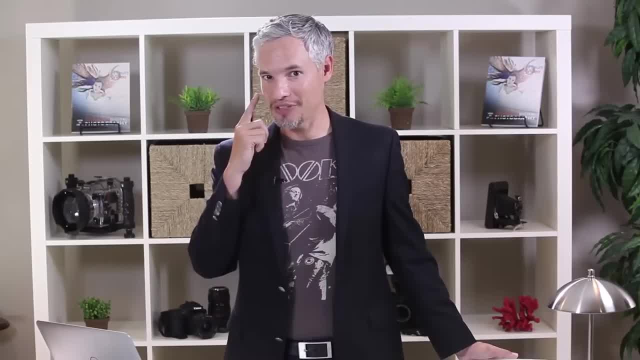 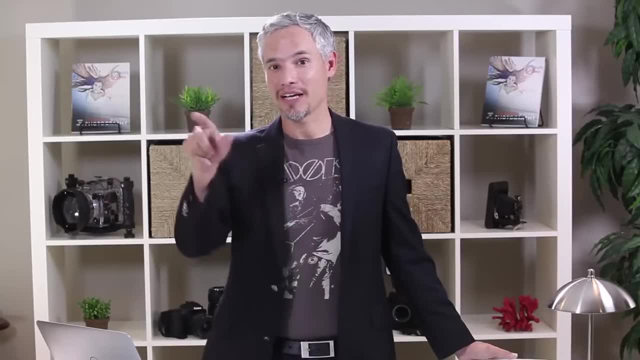 For example, right now I have a couple of lights that are pointed at me, and if you look closely at the reflections in my eye, you can see just where those lights are. But that's not the only light that I have. For example, these lights are also striking this white. 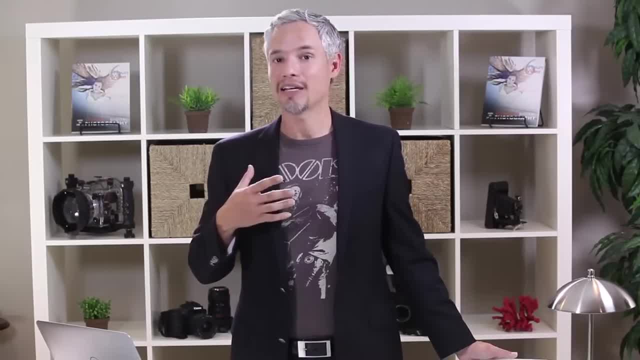 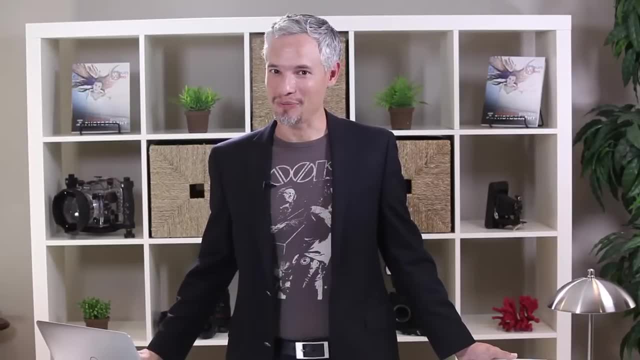 table and that's reflecting light back under me and that's helping to reduce the amount of shadows that I have and add fill. So figuring out your light can be really complicated, but once you get the hang of it you'll be able to diagnose problems in your pictures and 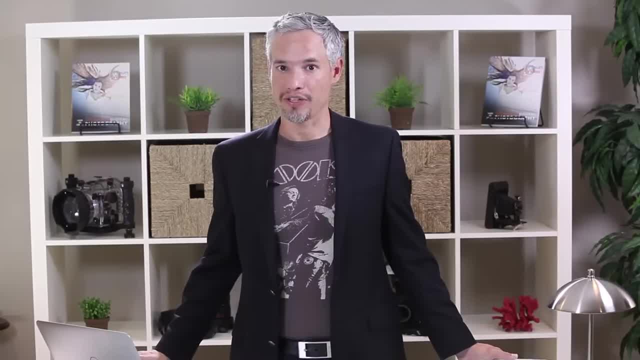 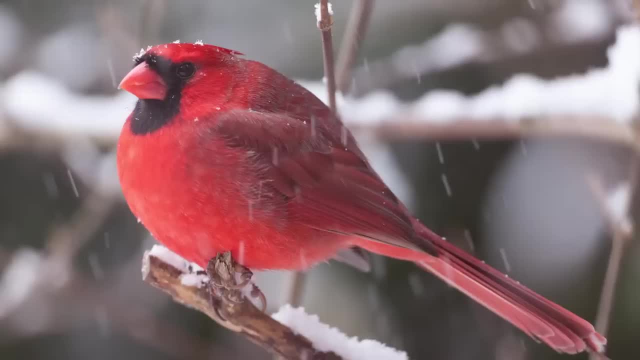 even move your subjects into different locations to get more flattering light. So let's look at some more sample pictures. Here's a picture of a cardinal. What do you think? Is it soft light or hard light? Well, let's look at another picture of a cardinal. 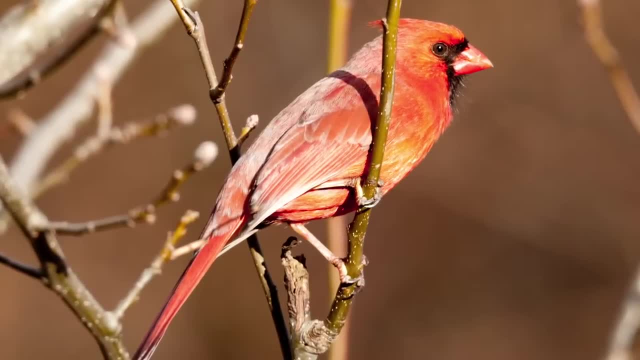 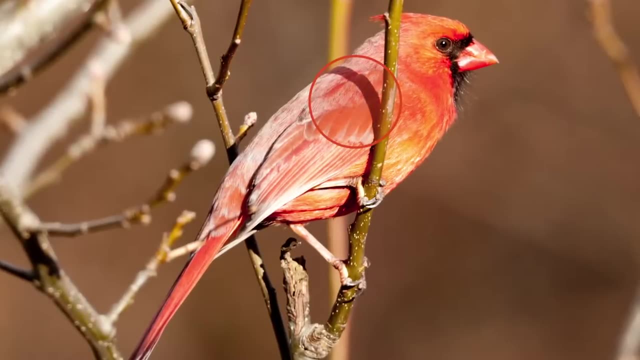 You can see here that this guy is in hard direct light from the setting sun, And if you aren't sure about it, just look at the shadow that's cast by that stick that he's holding. It cuts right into him and is very sharp and distinct, and that would 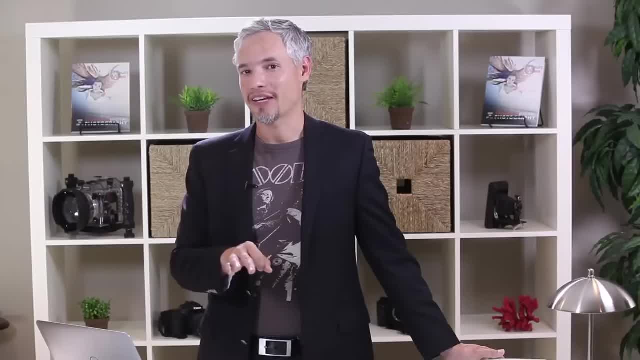 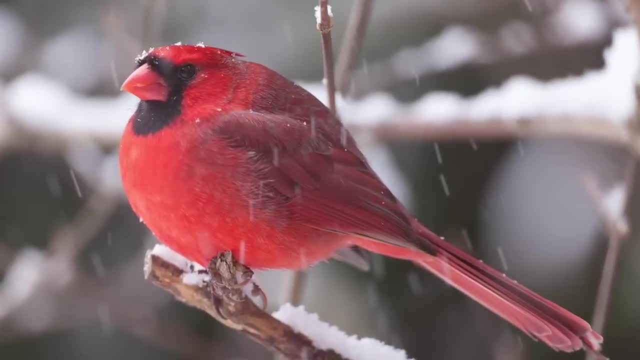 only be caused by a very hard light source. Looking back at that cardinal in the snow again, it's interesting to study the effects of light in snow, because when snow is on the ground, well the whole earth becomes a huge soft box and the light 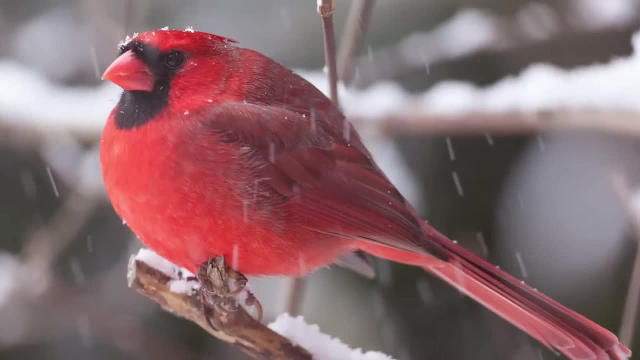 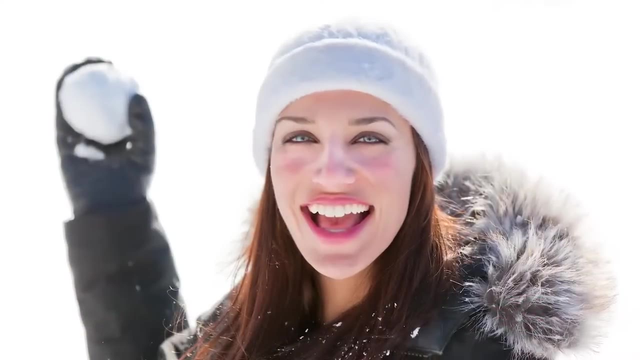 is so soft and even because you have this massive amount of fill. In fact, there are times when I take pictures of people in the snow, when I notice that the light from the snow is actually brighter than the light from the sky, because the snow is just pure white and is a 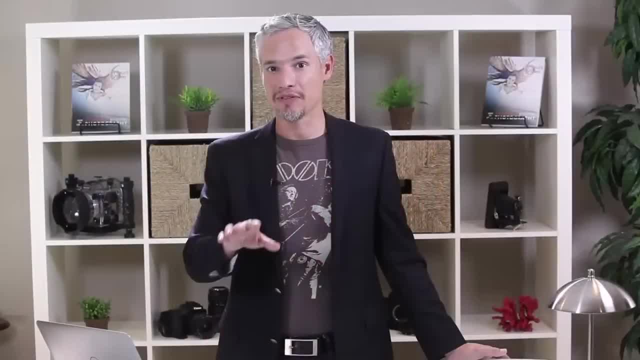 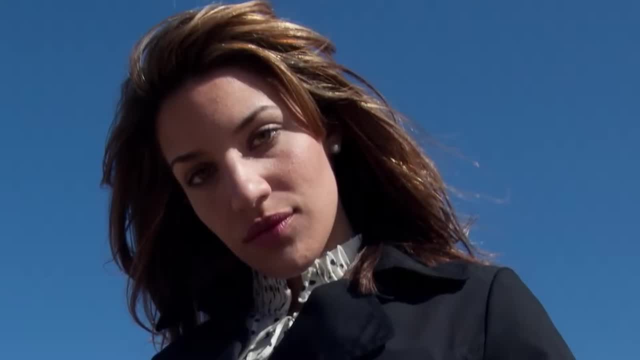 perfect diffuser and it always provides the most even and soft lighting. Let's look at some more pictures. Here's a picture of Chelsea. So what do you think? Hard or soft light? Here's a picture of Chelsea taking pictures indoors, but near a big window. 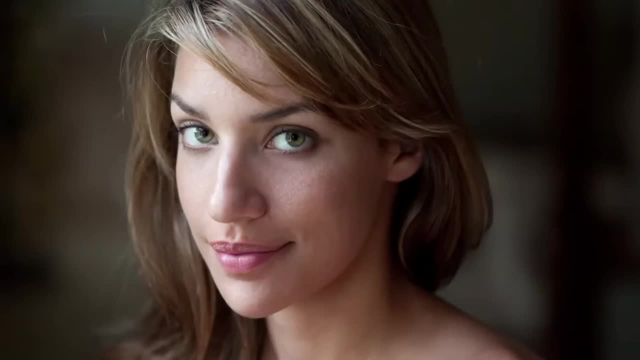 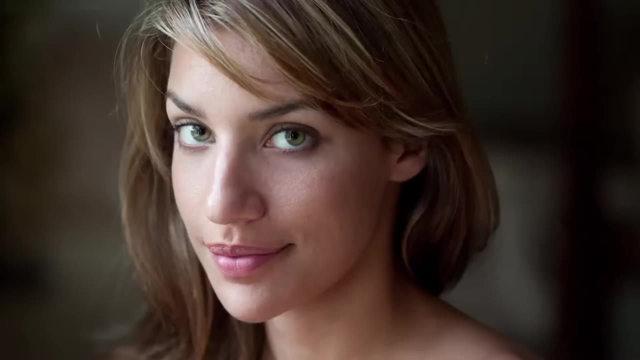 and you can see this is not the softest of light and it's not the hardest of light, but it's much softer than it was in the previous picture where she was outdoors near the setting sun and as a result it's also much more flattering for her. 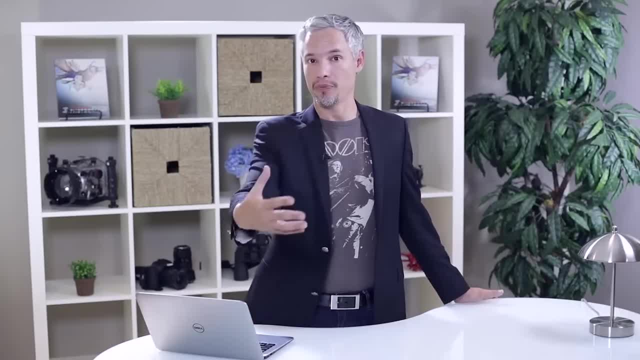 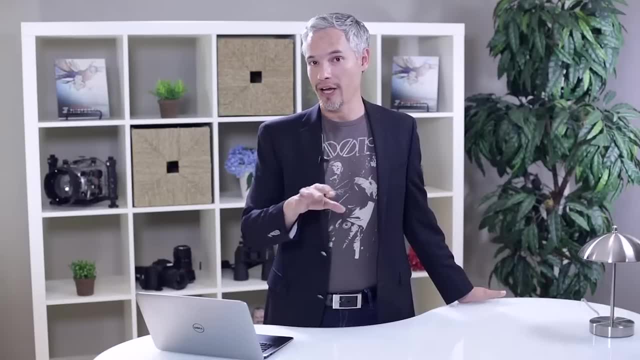 Besides being hard or soft, light is also directional. It can come from the front or the top, or the sides or the back, and learning how to control directional light, either by moving your subject and using natural light, or by adding light using flash, is really critical. 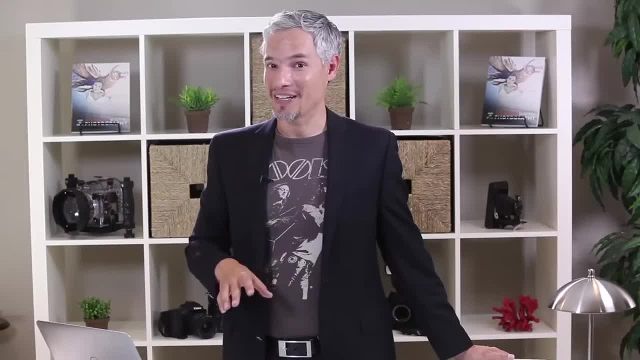 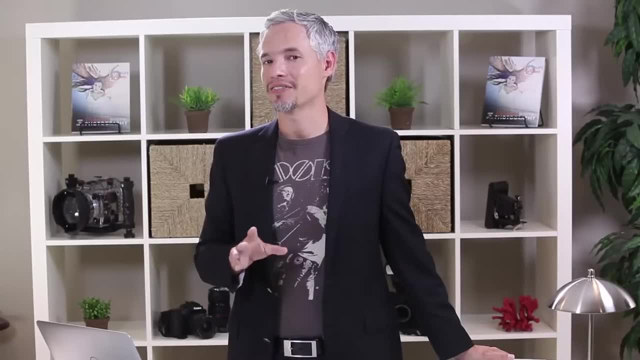 to becoming a good photographer. Anytime it's a sunny day and the sun is high in the sky. you're going to be dealing with top lighting, and top lighting is probably the most challenging type of lighting to deal with. It doesn't tend to be the most flattering. 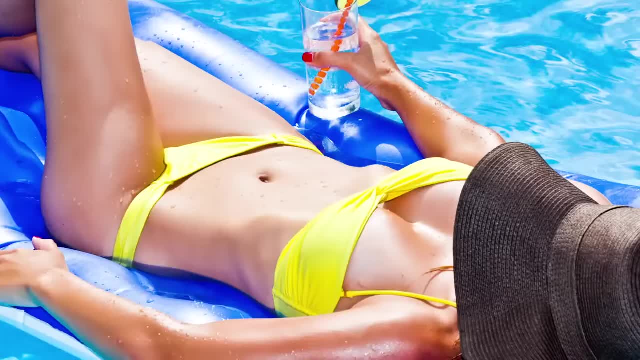 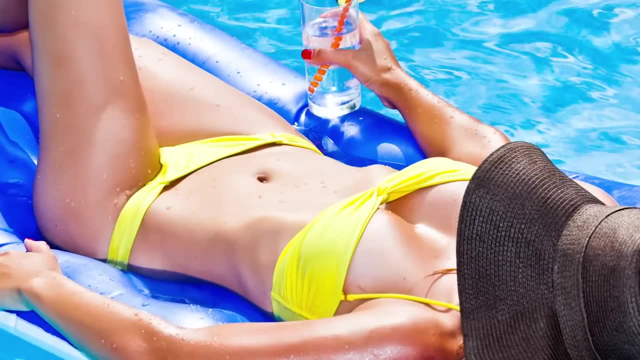 Here's an example picture taken in top lighting. You can tell from the distinct shadows in the photo that it's also an example of hard and direct lighting. That's because the sun was very high in the sky In this case. it's okay, I used that. 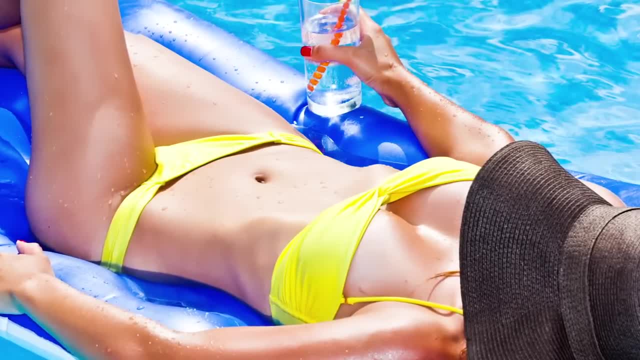 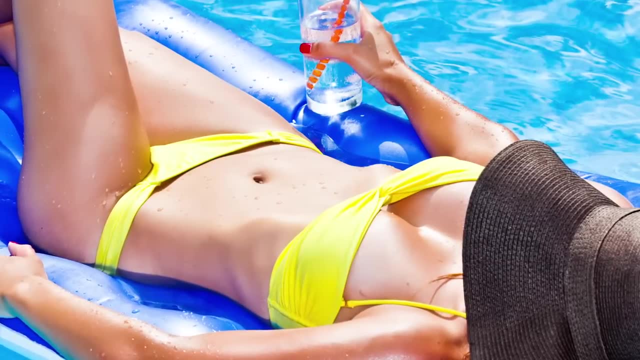 lighting, and the light is reflecting off of the water and adding interest to it. It's also reflecting off of all the water drops and adding a lot of shape to them. But if it were a portrait of a face, it probably wouldn't be as flattering. Here's a picture of a 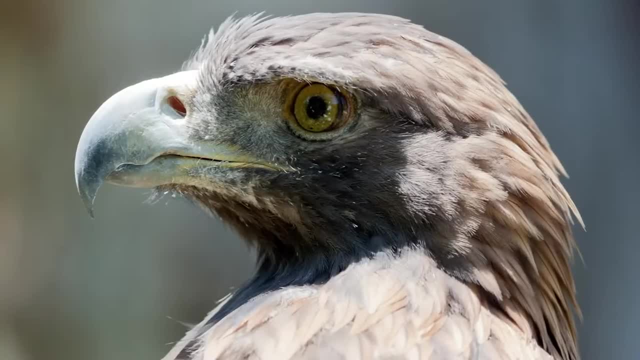 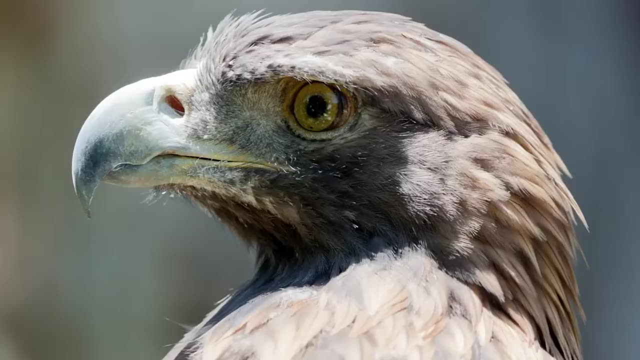 golden eagle, taken while the sun was high in the sky, without a cloud in the sky, and we're looking at hard direct top lighting casting a deep shadow over the bird's eyes. Now the exposure here is very difficult because I needed to expose for the eye. 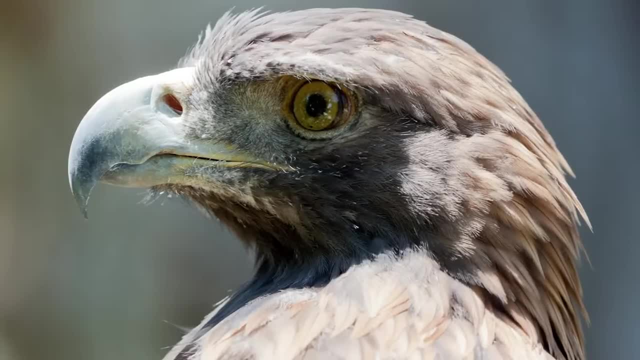 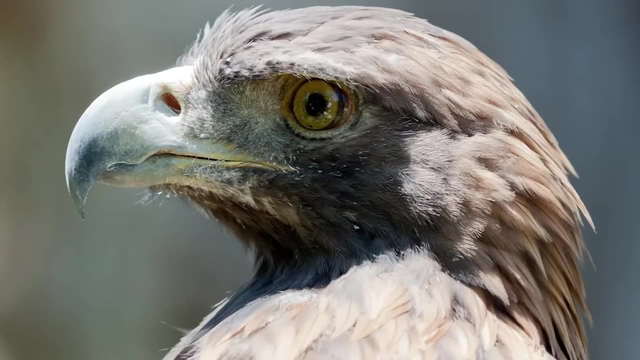 That required me to overexpose the feathers a little bit, and there's not really any one exposure that's going to be right for this situation- And that's one of the telltale signs of working with hard light is the exposure can be very difficult because the difference 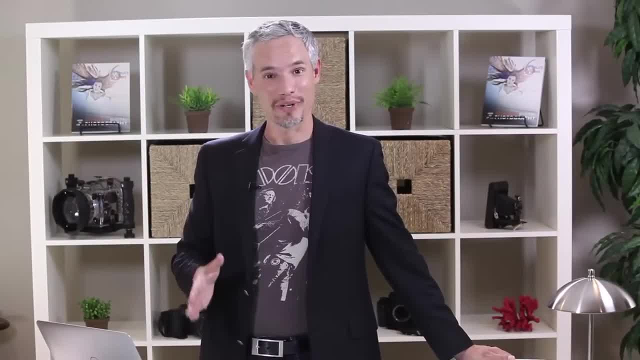 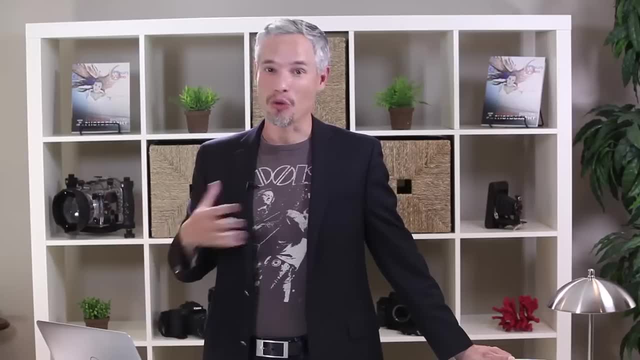 in lighting between the highlights and the shadows is going to be really extreme, And the best you can do is expose the most important part of your subject correctly and then hope that the rest of it isn't too under or overexposed. Here are some people in hard top. 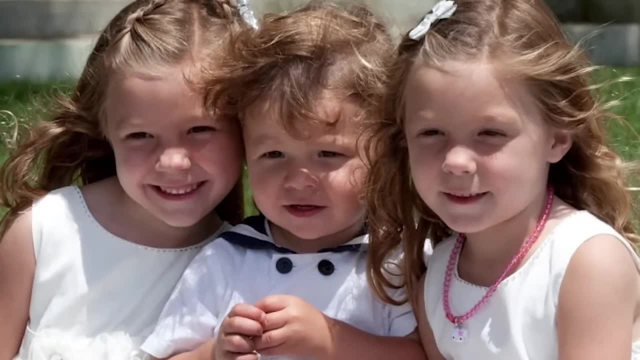 lighting and, as you can see, they have those shadows under the eyes and that's not flattering at all. You always want to move people into some more soft lighting, or at least give them hard back lighting or side lighting, but never hard top lighting. Now let's look at some examples of front lighting. 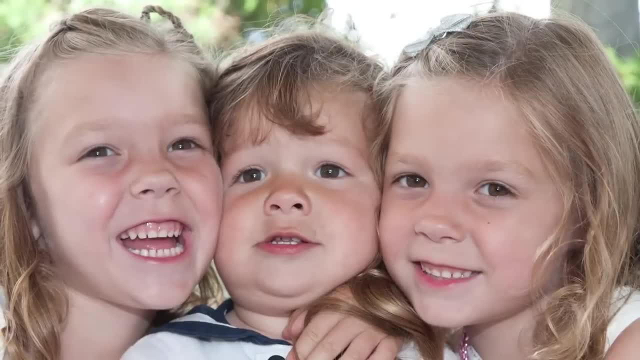 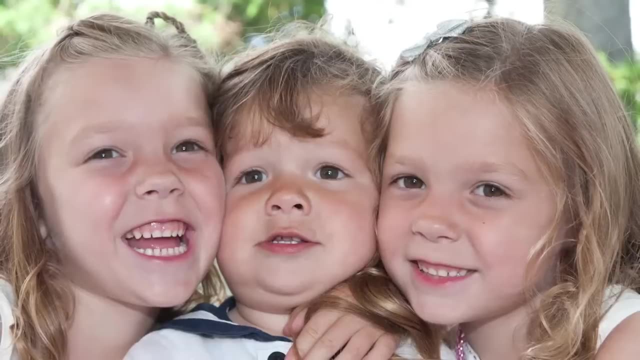 There are those same cute kids again- my nieces and nephew- and here I just moved them into the shadows and added a little bit of flash so you can see the light is much softer Now. front lighting tends to fill in pores in a portrait because it's coming. 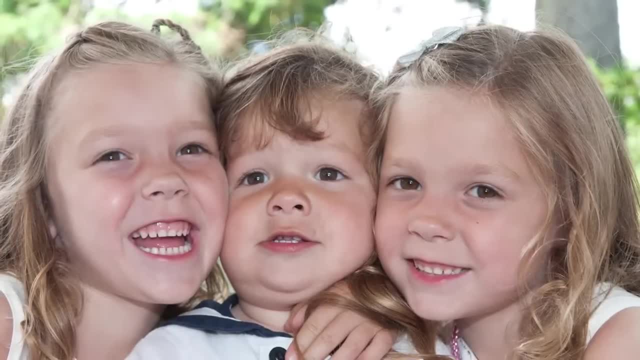 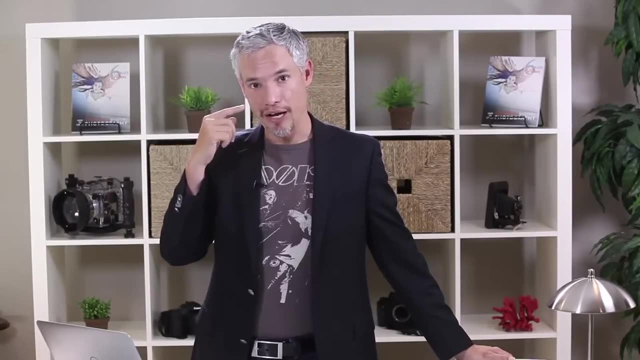 right in through this direction, so your shadow is going to be behind you. Now, if the light is coming in from the side or the top, all of your little pores and your nose and the brow of your eye are going to be casting shadows down or to the side. 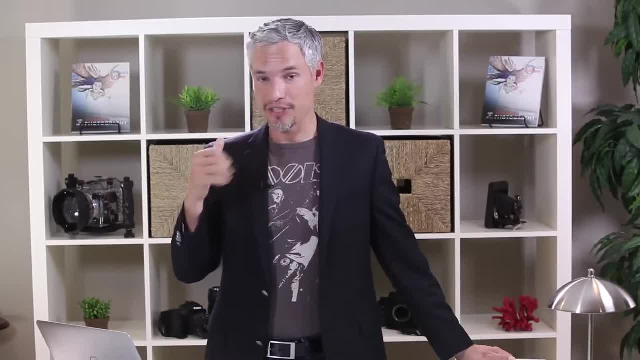 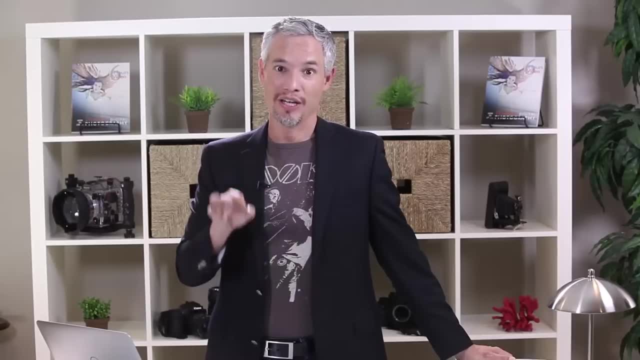 where they'll be visible on your face. Front lighting will still cast shadows, but because it's going behind you, you won't notice it. Working with shadows is critical to portraying texture and form and shape in images, so pay attention to the pictures as we go through them. Here's a picture. 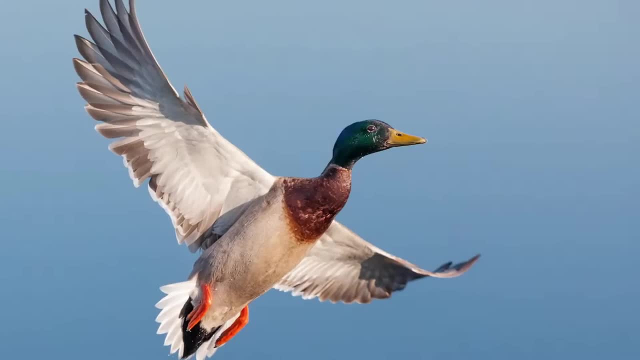 of a duck in the rising sun, and the sun was to my back, which creates nice front lighting when it's low to the sky. This is one of the reasons I'm going to be pushing you to get out there early or late during the golden hours. That's a topic I'll talk about more. 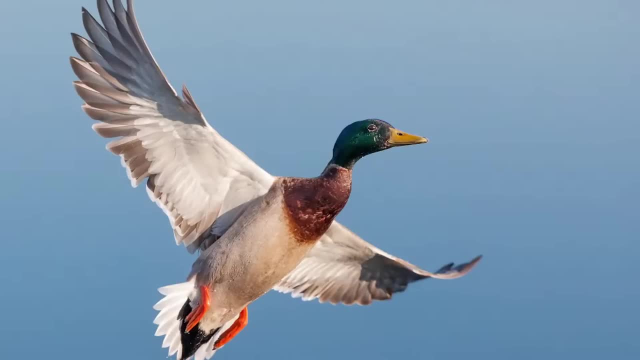 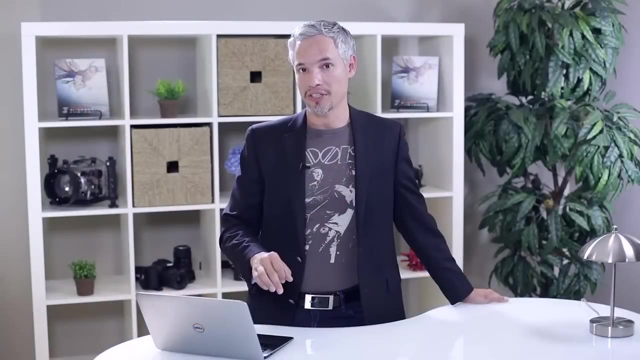 But, as you can see, the hard front lighting shows a tremendous amount of detail in the duck and the shadows that are there, for example off of his wings, are very distinct and hard. Those are tell tale signs that there was no clouds or other type of diffuser between the duck. 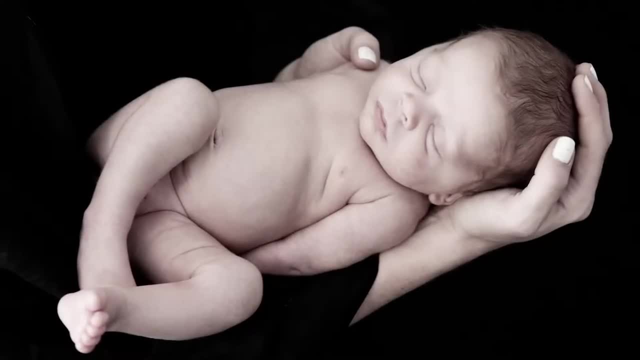 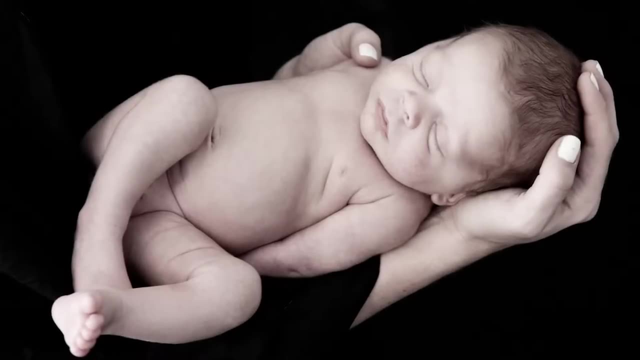 and the light. Here's a picture of a really sweet baby, front lit. Now here the front lighting is very, very soft, So the shadows are also very soft and the mid tones are very smooth and gradual. You don't see any hard or distinct. 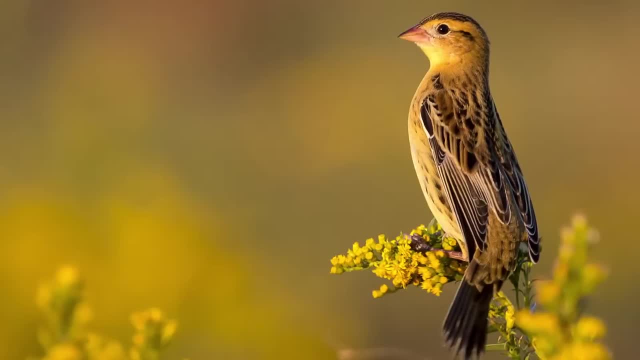 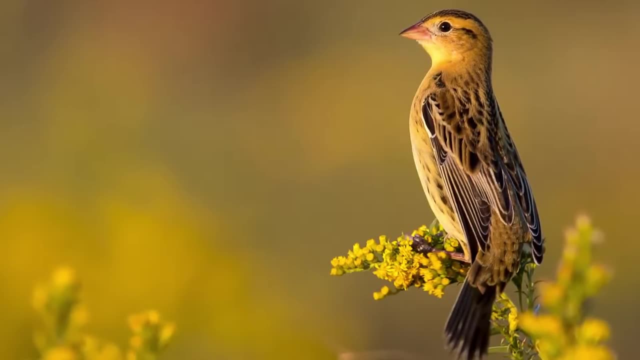 shadows in this photo because the light is so soft. Hard front lighting like this is ideal for wildlife because it really brings out the detail, and it also means you don't have to deal with the shadows and exposure problems that result from that, because, of course, the bird is casting. 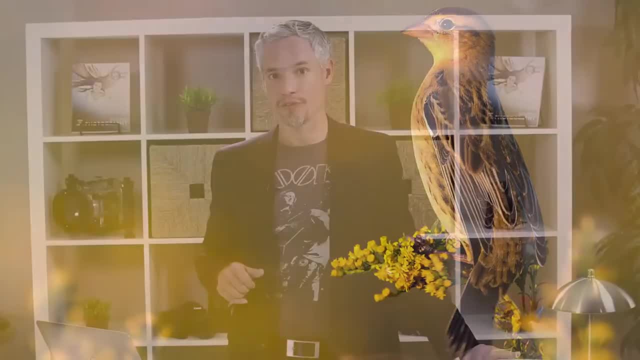 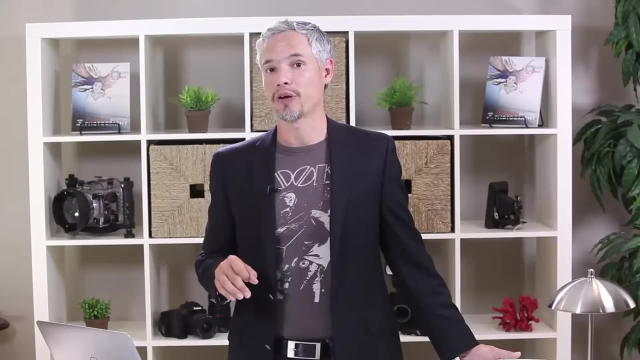 a shadow, but it's behind him and therefore falling outside of the frame. Soft light can also be really nice for wildlife, but myself, when I have a choice, I think the hard light works better, because hard light is excellent at bringing out colors, and while colors might, 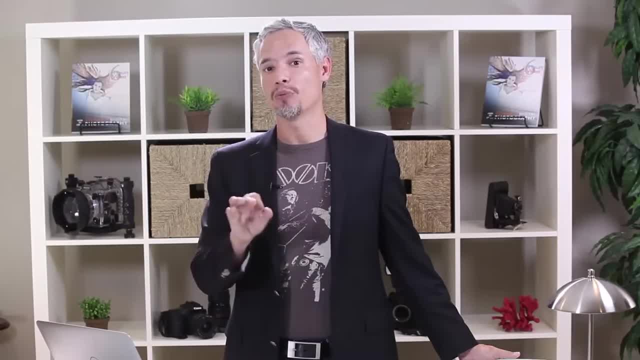 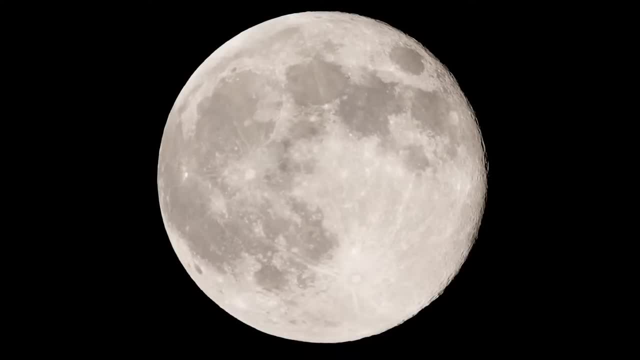 not be something you necessarily want to bring out in a person's face. for birds and animals it's really critical IS the full moon. We don't necessarily think of this as front lighting, but that's what it is. When you're looking at a full moon, that means the sun. 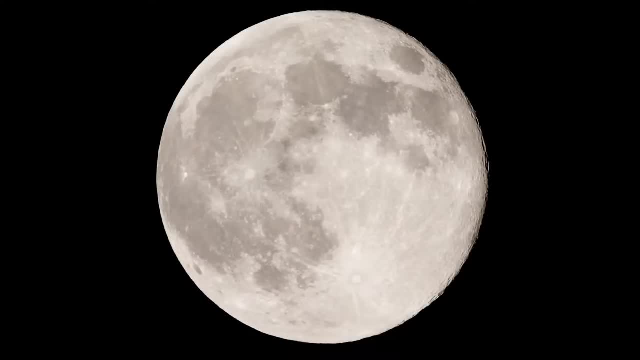 is behind you somewhere, because the sun is still shining on the moon, even if it's night where you are, and I want you to notice the texture in the moon. Of course, we all know that the moon is covered in little craters, but you probably don't see them anywhere on this photo. 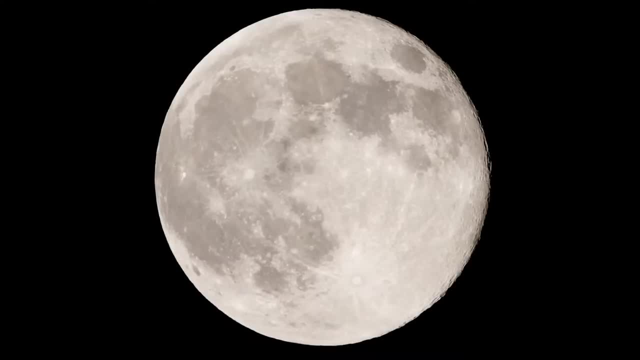 do you That front lighting is? again, it's hiding the pores and craters of the moon, which would be really flattering for a portrait. Now, where do you see the texture in the moon? here I can see quite a bit along the right side of the moon. 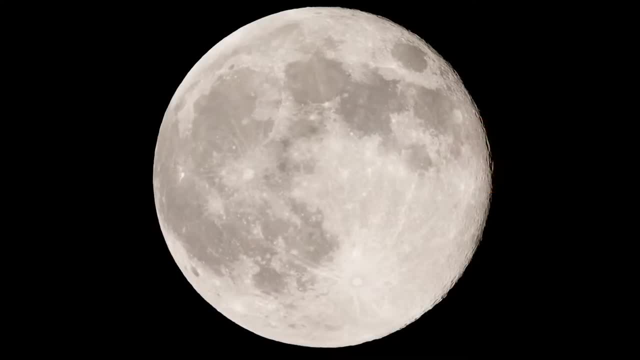 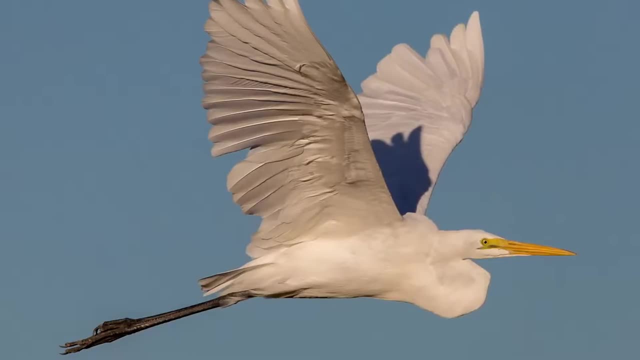 and that's because that right side of the moon is basically side lit by the sun. There were some shadows being cast. Without those shadows, there is no texture. Here's a picture of a great egret, and what do you think? This is definitely front lighting, but is it? 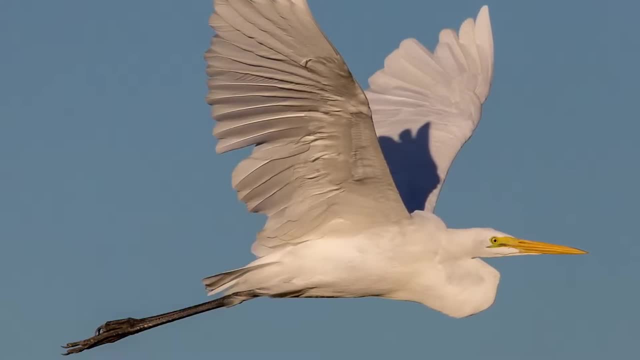 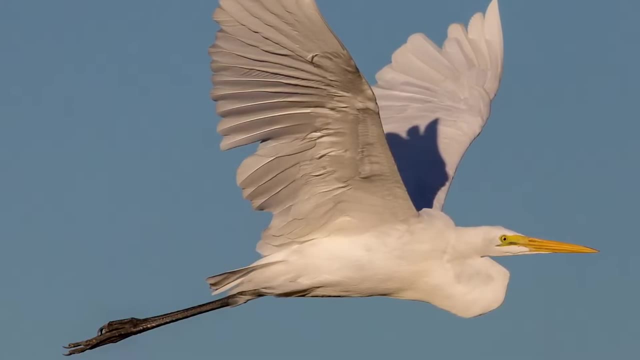 hard or soft. Well, look at that shadow on his wing and you can see that it's very hard lighting because that shadow is almost a perfect copy of his wing. Again, I try to work with front lighting whenever possible for wildlife. Here's a great blue. 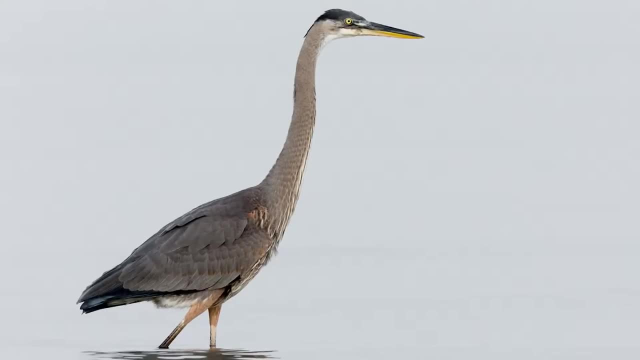 heron, and this is also front lighting, but it's soft front lighting and, as you can see, there are no hard shadows. In fact it was a dense, dense fog, so that's about the softest lighting you can get, because all the humidity in the air is also reflecting. 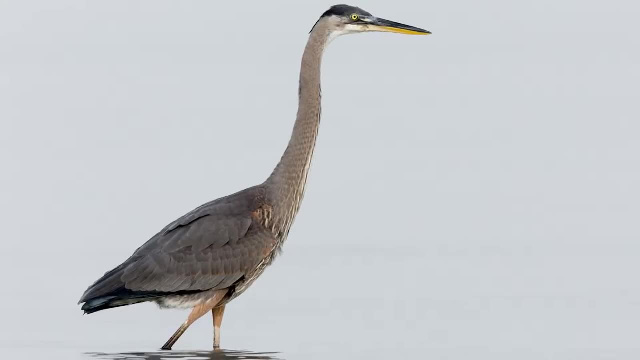 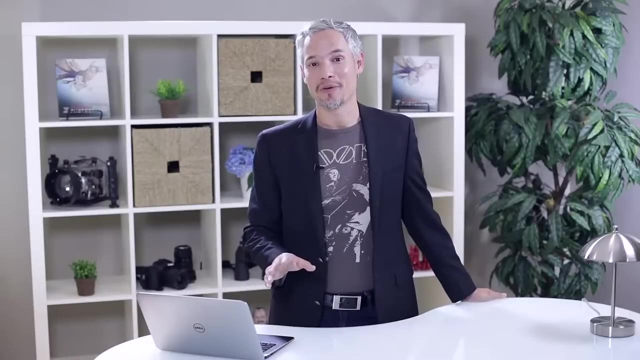 the light Now. this gives the picture a very peaceful tone and it's not nearly as intense. The colors are also really muted, because soft and diffused light mutes colors. Now let's look at some examples of side lighting. Here's a cardinal in. 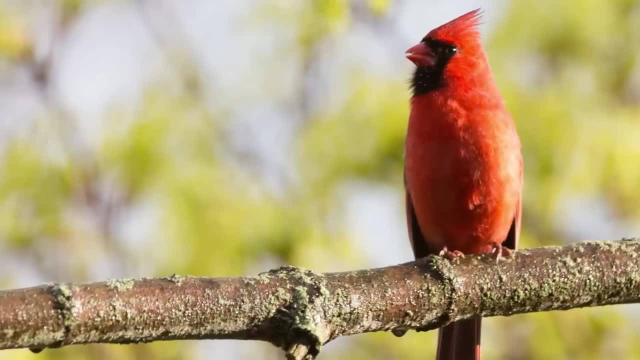 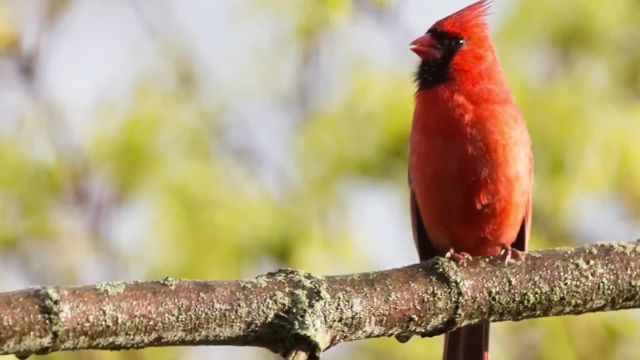 hard side lighting. You can see the shadows are very short, which means it's hard light, and you can see the left side of the bird. the camera left side of the bird is completely in shadow, while the right side is completely bright. Here's a picture of Chelsea inside. 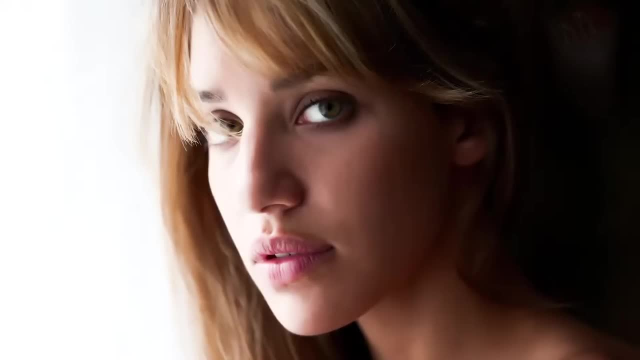 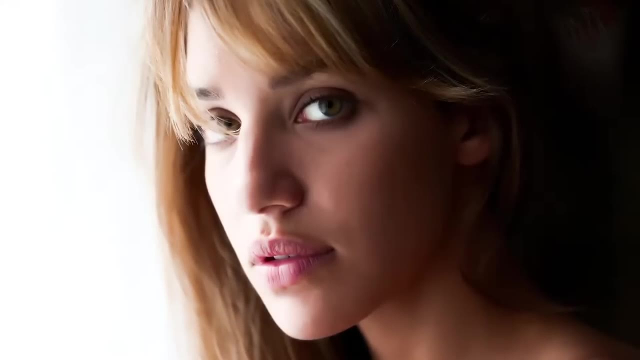 lighting To make this picture. I just positioned Chelsea next to a nice big window on an overcast day, So the light coming through the window was nice and diffused, but it lit the side of her face closer to the picture much better than the other side of her face. 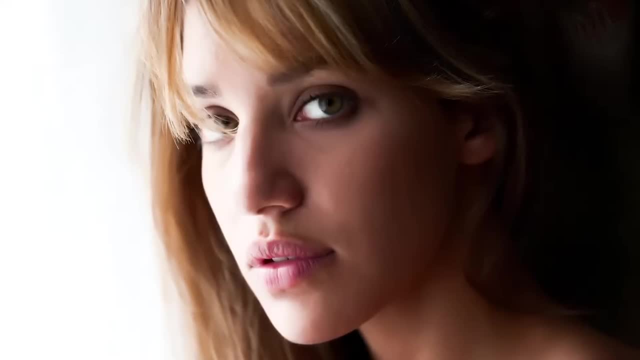 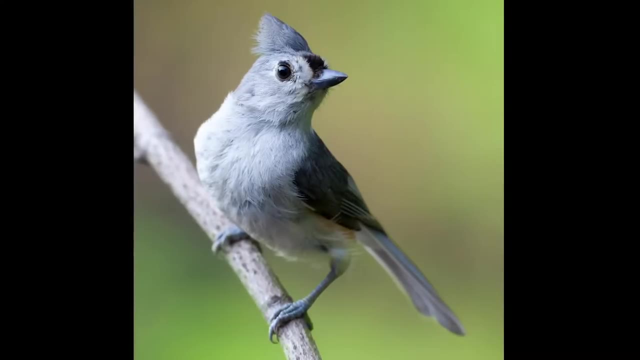 which is basically in shadow, and that created a nice gradient from bright to dark. Here's another side lit bird and one of the things you'll notice about the side lighting here is that it's really accentuating the texture of the feathers in the bird. 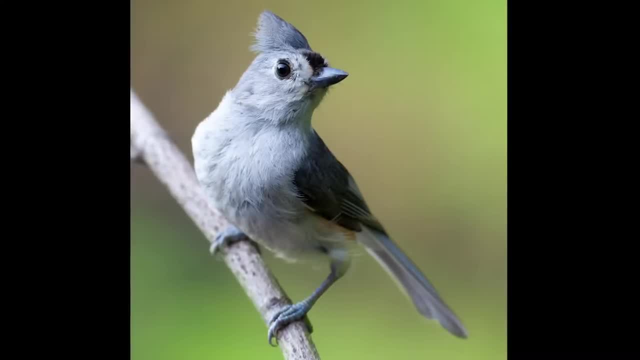 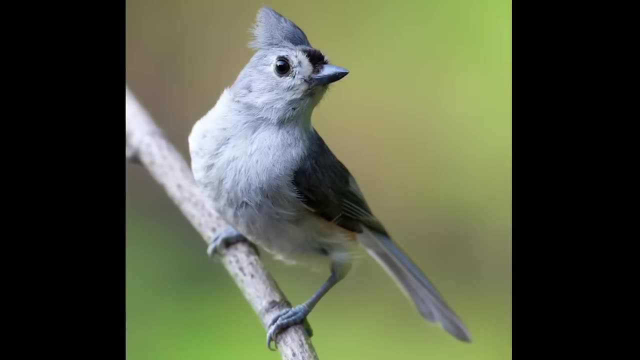 One problem with front lighting again is that it's eliminating any texture because it's hiding any shadows that would give you that visible evidence of texture. Well, side lighting doesn't do that. If you want to show texture, there's no better way than side lighting to do it. So if you 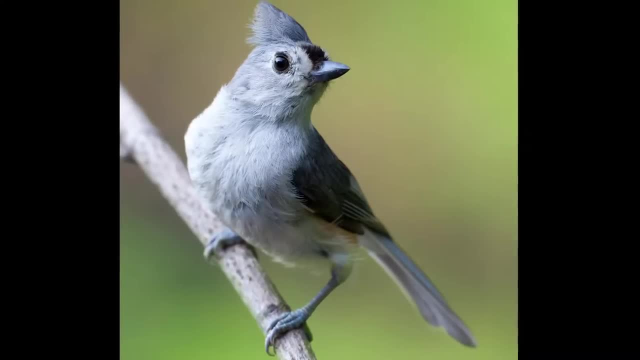 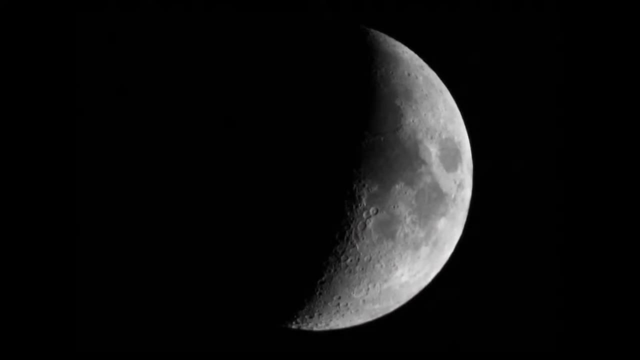 look at the feathers in that bird's belly. you can just see much more detail than you could in the pictures that were front lit. And here's that moon again. Look at how much more detail you can see in the individual craters. You couldn't see any of those. 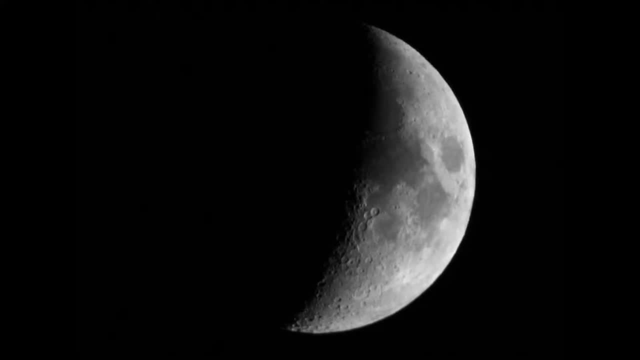 craters, but they were still there. This is, of course, the same side of the moon. We always see the same side of the moon, But this is side lighting, because now the sun is somewhere off to the lower right corner of the frame and even though it's night out. 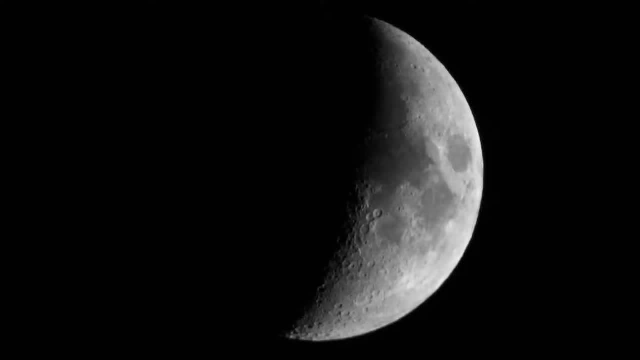 and I'm not seeing the light. the moon is still catching it and reflecting that sunlight back to me. The side lighting allows shadows to form in the individual craters. So look closely at those craters and you can see that the shadows form on the nearer side and the highlights. 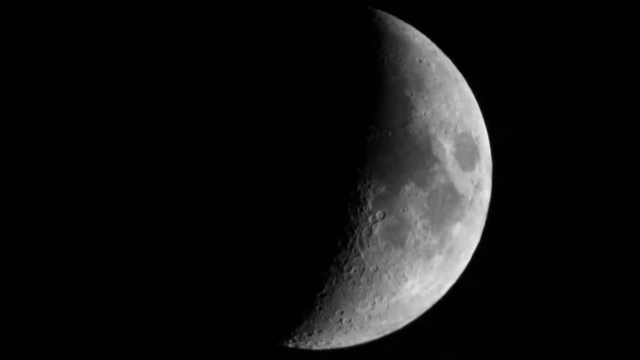 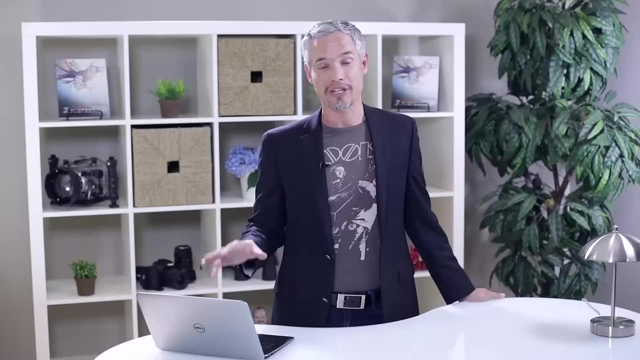 form on the far side of the craters because they're dented in a little bit, and that's what gives us the sense of texture and three dimensional form to the moon, With that front lighting that you get from the full moon. there's none of that, No texture. 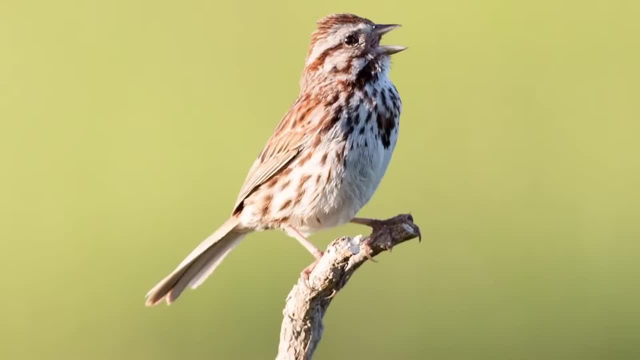 no three dimensional form. Now, here this bird is side lit and even though the lighting is coming from behind the bird, it's still side lighting because you'll refer to it in relation to yourself and really, the camera, And again you can see an awful lot more. 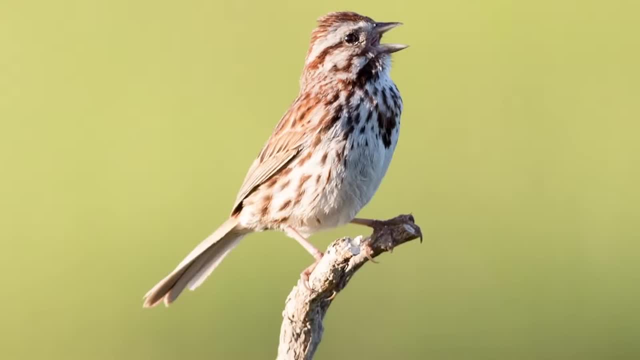 texture in the bird's feathers, especially in the transition from highlight to shadow. there You can tell that this is a very hard lit picture. The sun was setting and there was not a cloud in the sky. Now let's talk about back lighting, and back lighting is one of my favorite. 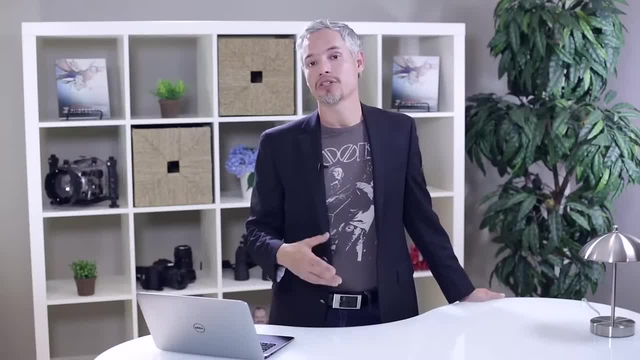 types of light to work with, It can be the most rewarding, largely because it's also the most challenging. And there's this thing in life: the things that are the most rewarding are usually the hardest, and the reason is that most people don't develop the skill. 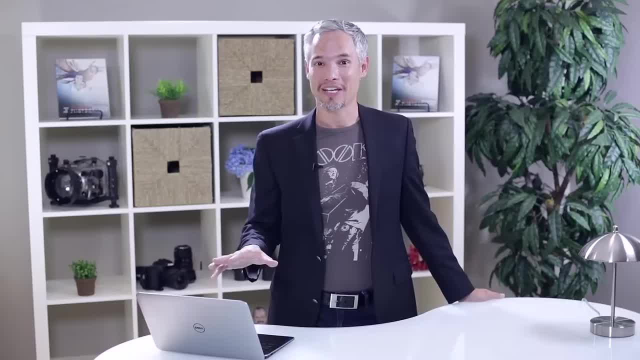 to do something all that hard right. So when you find something and it looks a little bit difficult, that's the stuff you should really dive into, and back lighting is a perfect example of that. So let's look at some back lit pictures. 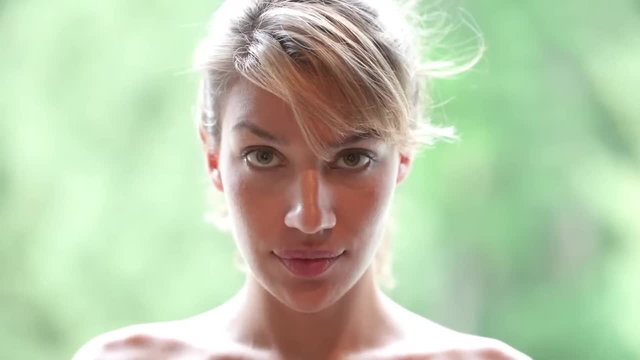 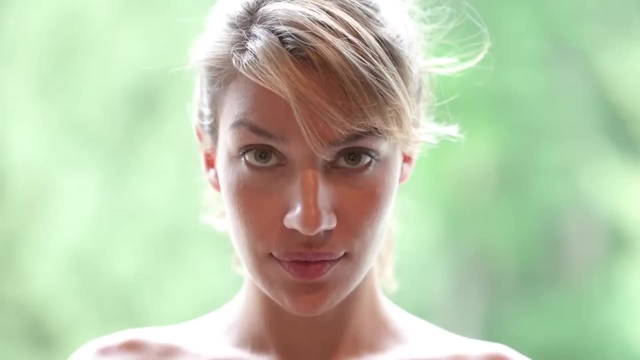 Here's a picture of Chelsea taken at the same moment as that last side lit picture, and what you can see here are the various effects of back lighting. Now look at the top of her head here and you can see. well, there's some crazy flyaways. 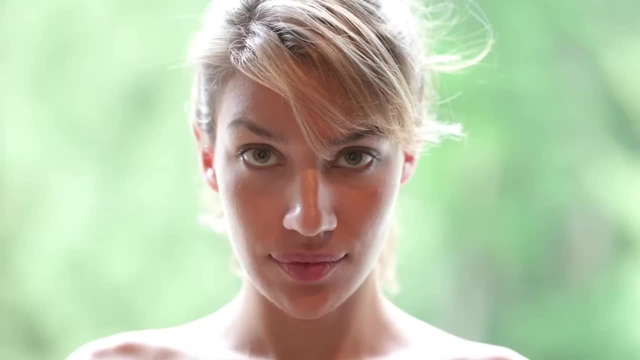 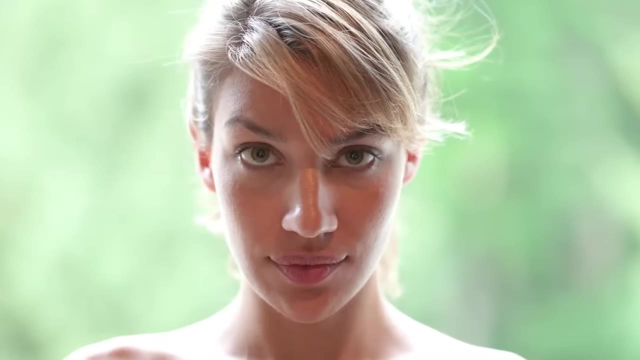 but the back lighting from the sun is casting light through those hairs and those hairs are catching the light and some of the light is passing through the edges of each individual hair. some of it's being reflected and what happens is the hair picks up all that direct light. 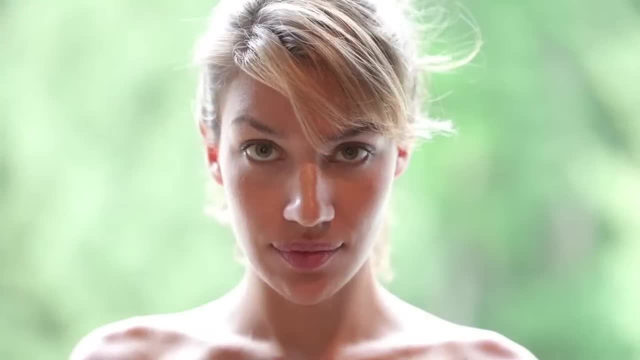 and reflects it, and it creates what we call rim lighting, which accentuates the two dimensional shape of a subject. You can see that same rim lighting on the sides of her face and shoulders and it creates a really dramatic light. Here I'm shooting directly into the sun. 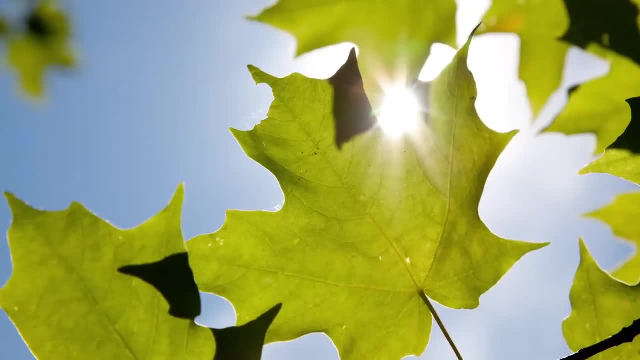 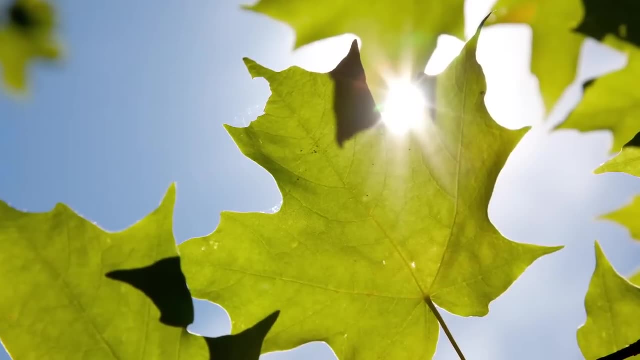 which is always an example of back lighting, and the reason I like this picture is because it shows the quality of light that passes through subjects. Now, there's no direct light for the leaves here. All the light is passing through them and picking up the green color. 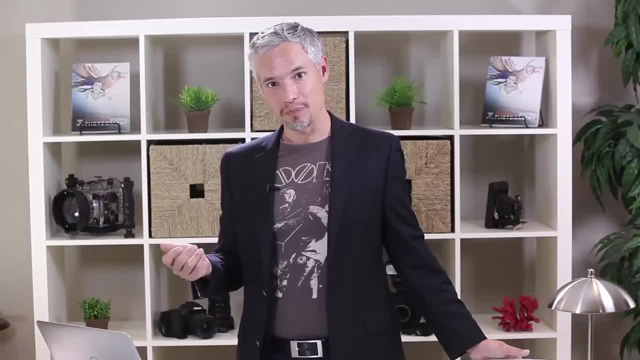 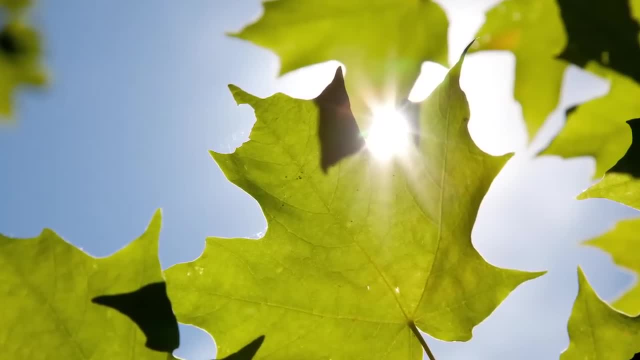 of the leaf and then hitting my sensor, because these leaves are actually partially translucent. Another thing I like about this picture is that the leaves are casting shadows on each other, So you can see that the leaves are absorbing some of the light. That is, after all, their. 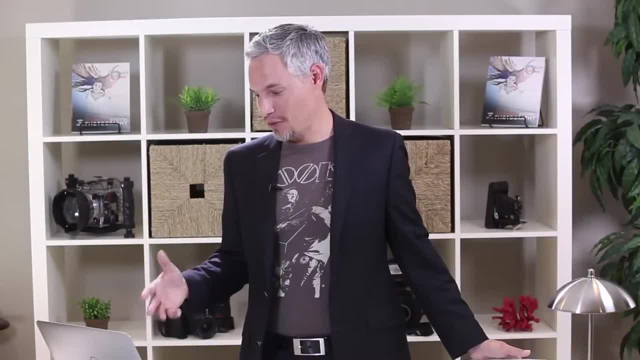 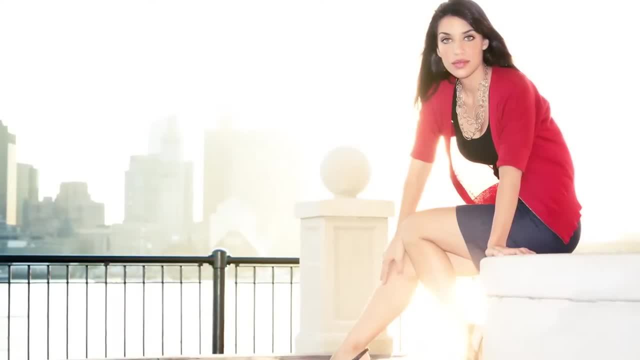 biological job, but some of the light is still passing through. Here's a backlit photo of Chelsea on the Boston skyline. We can see some of those backlit properties. You can see that the back lighting is passing through her sweater, making it appear almost completely white, even though 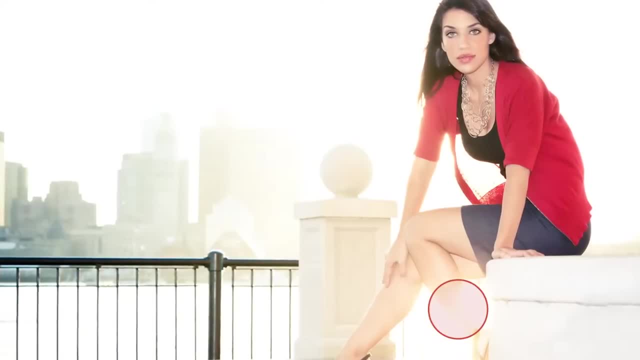 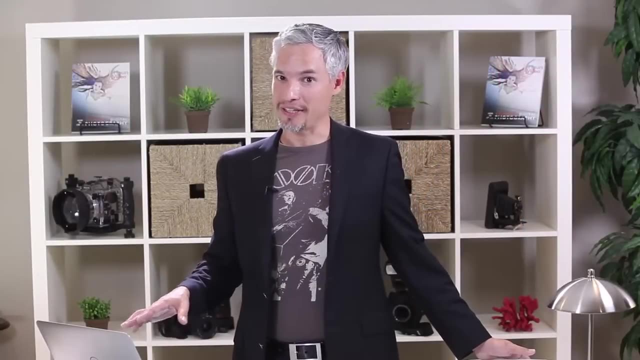 it's definitely there, You can see. it also has somewhat of a thinning effect on her legs because it kind of creeps around them. I'd also like to make a point about proper exposure. with this photo, The hard back lighting meant that the background was much brighter. 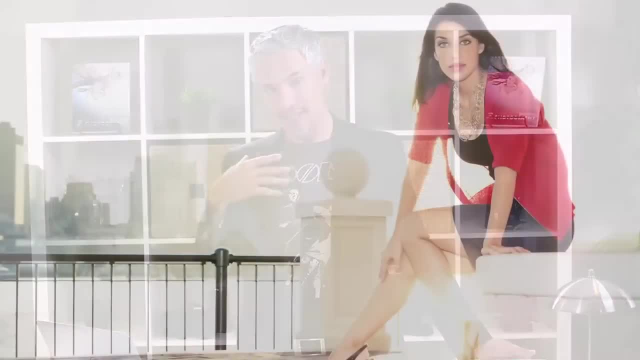 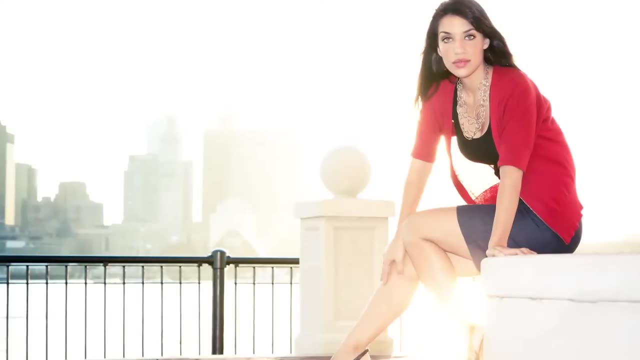 than Chelsea, because she's actually in shade, So her face is mostly lit with diffused light. I had to expose it properly for Chelsea, though, because she's the subject and my camera would have exposed for the background because of all that just hard light coming in, So I actually had to switch my 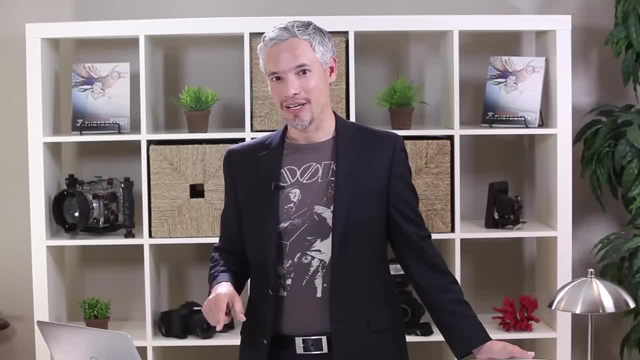 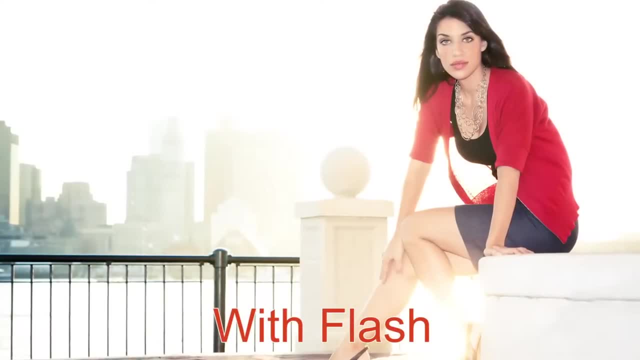 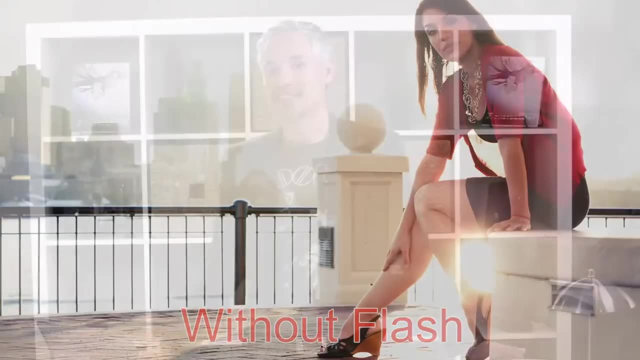 camera to manual mode. I also put a flash on my camera and used that to add some front lighting. That additional front lighting from the flash helped offset this extreme dynamic range that the picture had previously, because I was shooting directly into the sun. So that's a lot to take in. 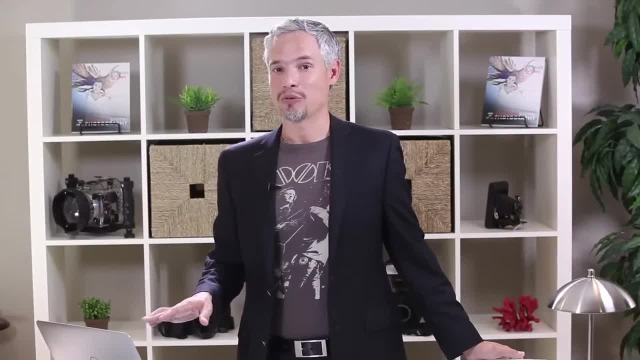 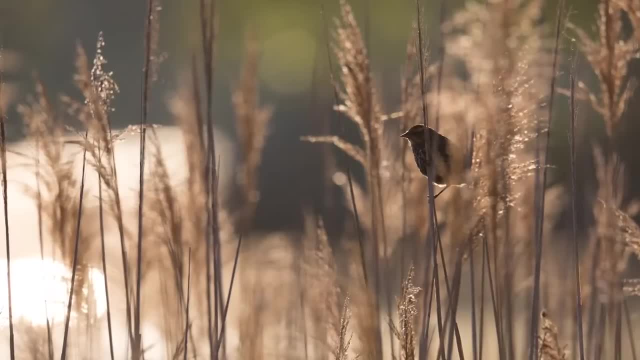 I'm going to discuss flash later in this lesson and I will discuss camera settings and manual mode and exposure compensation in an upcoming lesson. I just love this picture and it's a great example of backlighting. Here the sun is setting in front of the camera somewhere and behind 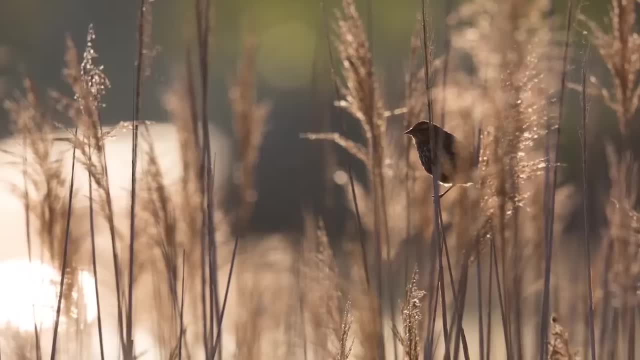 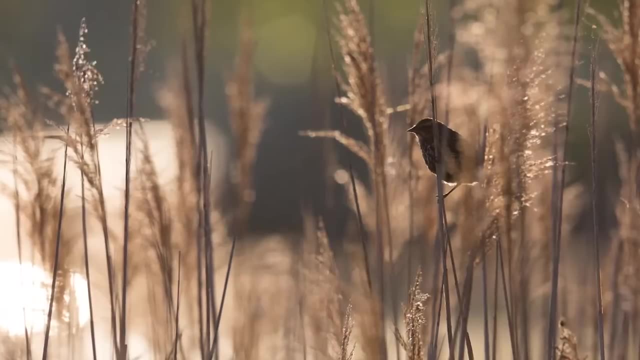 the bird and the light is filtering through these reeds, giving them this bright and glowing color. I also want you to note the rim lighting around the bird. You can see the edges of the bird are just perfectly detailed and because it's all backlighting, 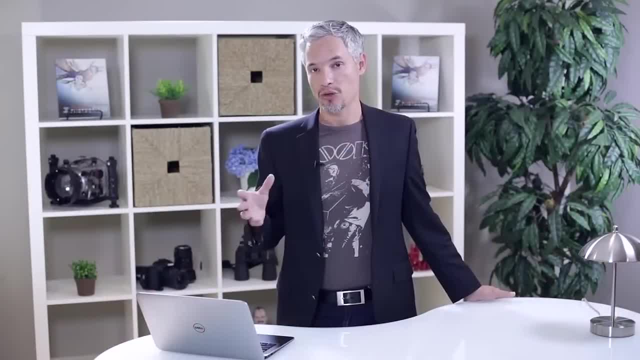 and there is no front lighting. the bird is completely in shadow. So the bird itself is dark. It's actually in its own shadow, And the picture of Chelsea was the same way, except that for the picture of Chelsea I added flash and front lighting and that. 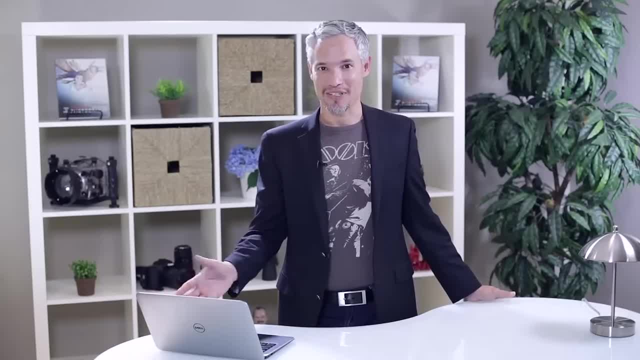 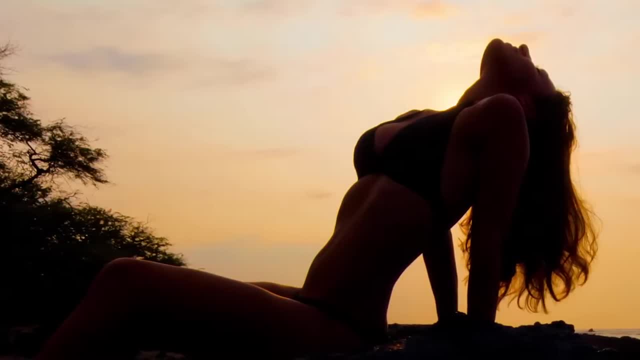 helped illuminate Chelsea a little bit better For this shot. I didn't think it was necessary. Let's look at another picture. There's Chelsea again, and this is a good example of creating a silhouette. With a silhouette, you have most of the light in the background. 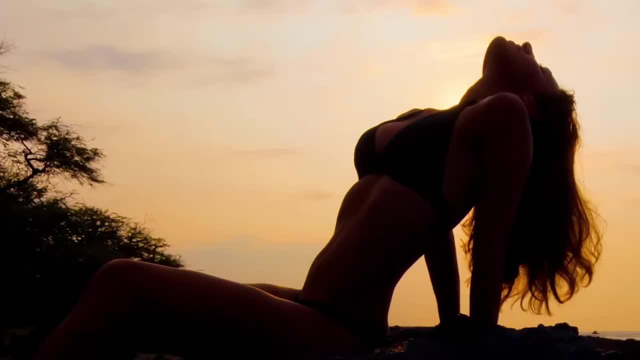 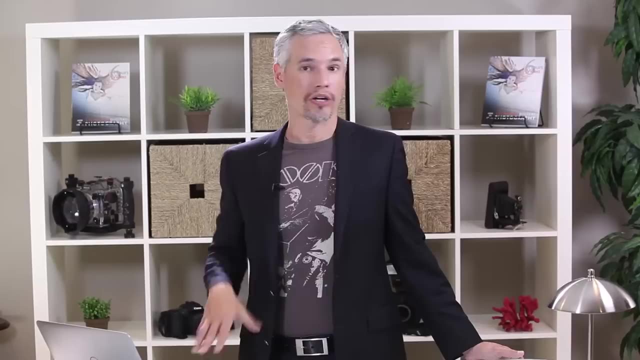 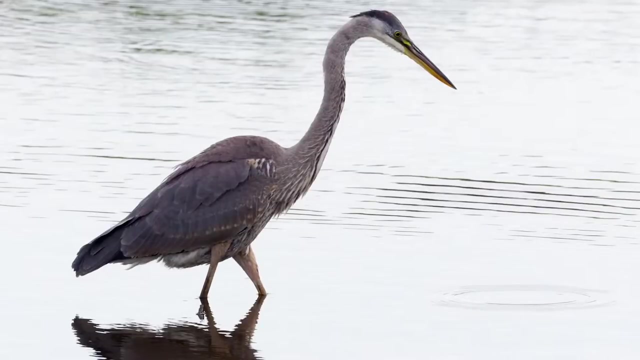 and the subject itself is just in complete shadow. You can create a silhouette by exposing the picture for the background and allowing the foreground subject to become dark and perhaps even completely black. You'll learn more about that when we study exposure compensation in another lesson. Here's another picture of a 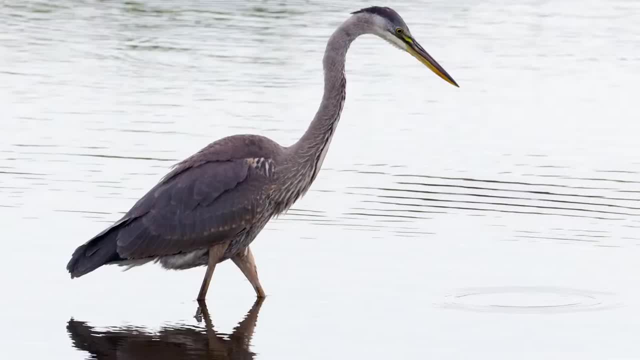 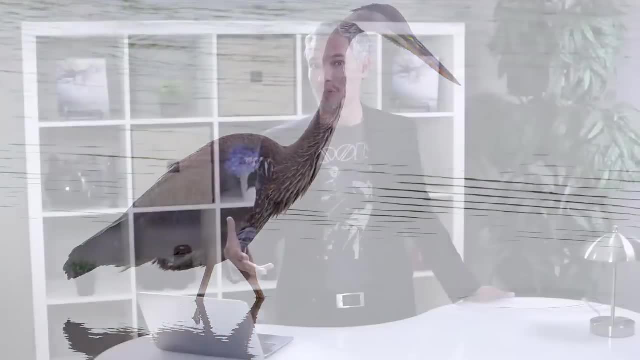 great blue heron, and you can see here that it's backlit because the water behind him is so much brighter than he is. The sun here is in front of the camera and behind the subject, and therefore he's in his own shadow, Meaning that he's going to be much darker than the surrounding. 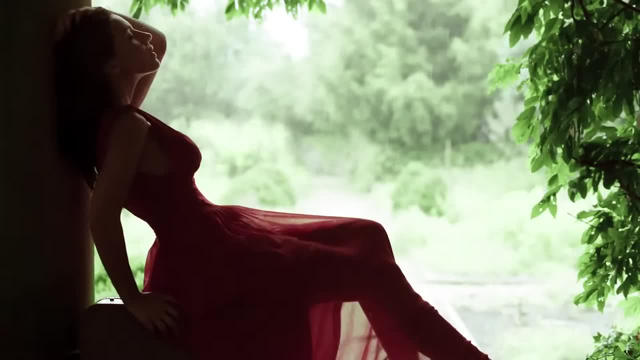 water. Another backlit photo of Chelsea, and this illustrates a lot of the same points. You'll see that in her dress, near her legs. there The light is passing through it. That's one of the nice qualities of backlighting: It shows subjects that 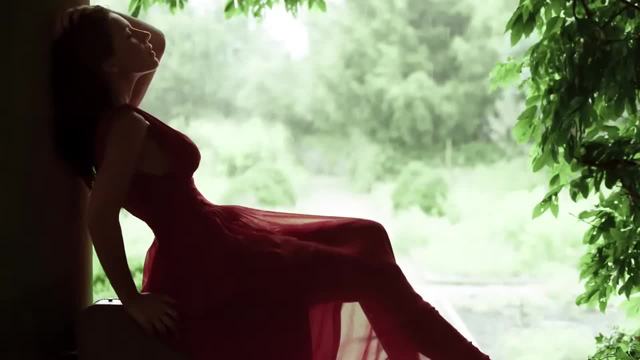 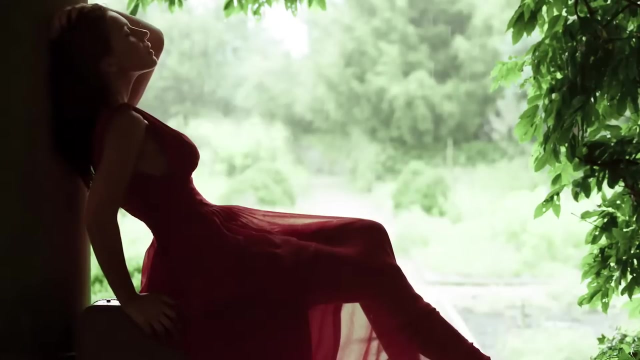 are translucent and highlights their physical properties like that. I also want you to note the nice rim lighting around her forehead, nose, lips and chin. that really helps offset her from the background. We had to carefully position her arm to allow you to see that rim lighting because if her arm 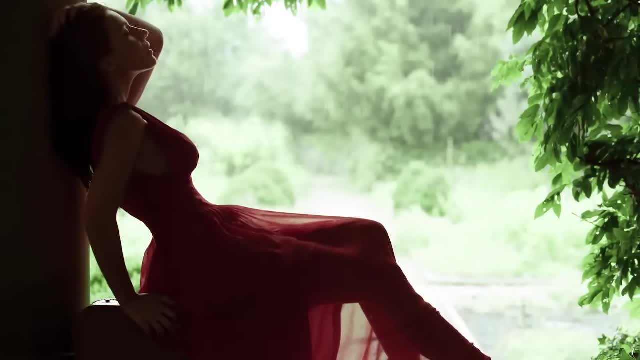 weren't there, she would have just been against a very bright background. What I want you to remember is that with backlighting it gives you a nice rim lighting and that helps to define a two-dimensional shape. This photo is very nearly a silhouette and, as a result, it doesn't have much of a 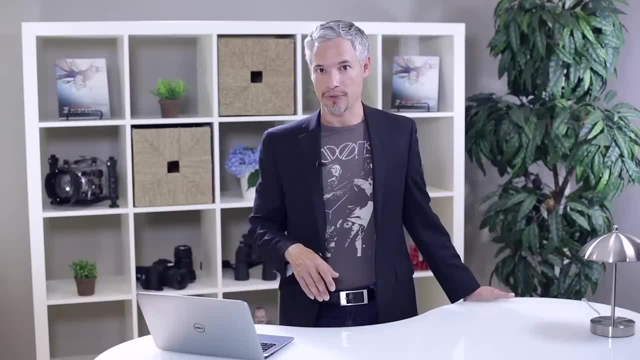 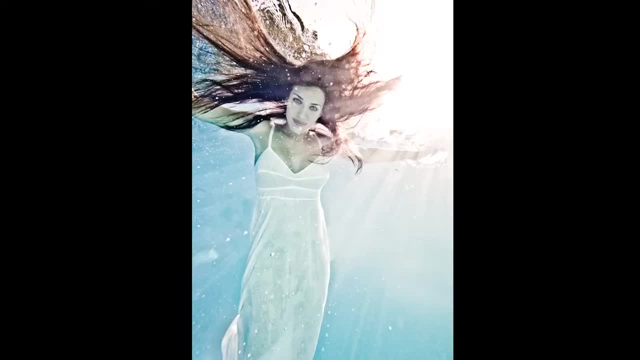 sense of three-dimensional form. Chelsea in this photo is almost completely two-dimensional. Some of you might recognize this photo. This is an underwater photo that I took of Chelsea and she is backlit. She's on the surface of the water pointing down, and I have an underwater camera laying on my back. 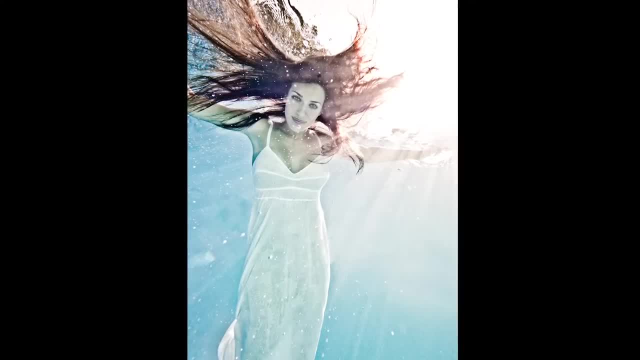 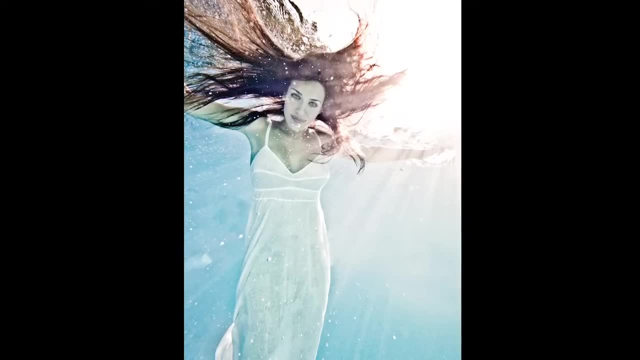 underneath the water pointing up at her, and the sun was high in the sky and positioned behind her. Here, because we're in the water and the water is reflecting some of that backlighting, you get what's commonly known as God Rays. God Rays occur because light is. 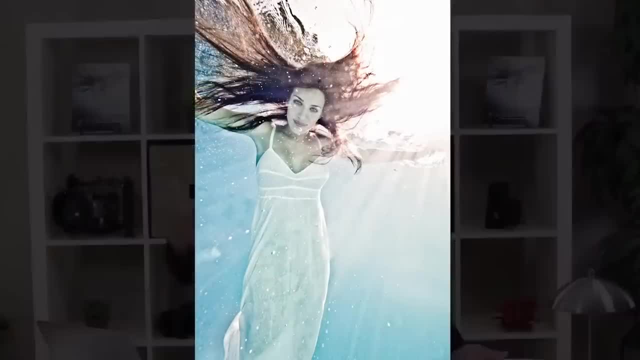 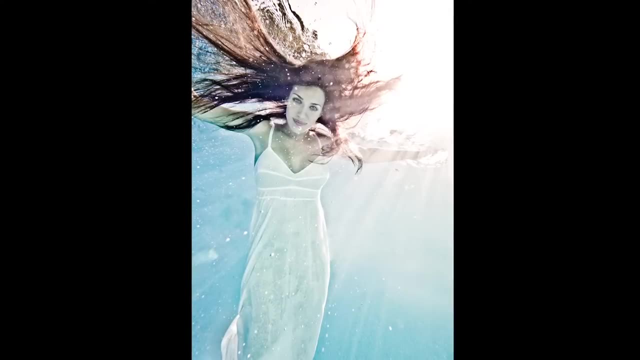 passing through a fairly dense subject that's reflecting the light and it has a dark background- In this case her hair- that allows us to see it. That's another nice property of backlighting. It allows you to work with these God Rays when the conditions are right, And again, those conditions. 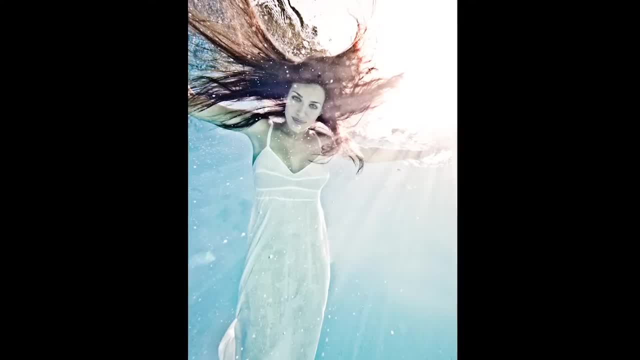 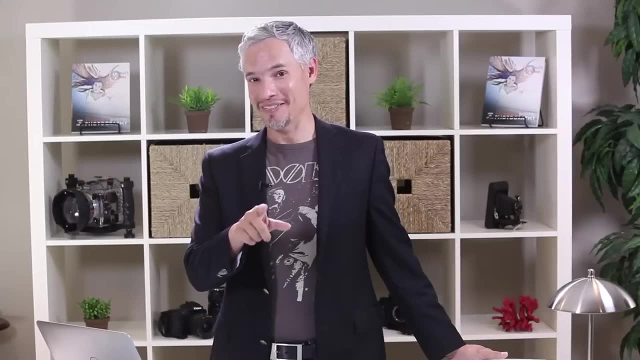 are dense air or water, that will allow the light to refract just a little bit as it passes through it, and then a dark background behind it that allows you to see that light. Time for a quick quiz. I'm going to show you some pictures and I 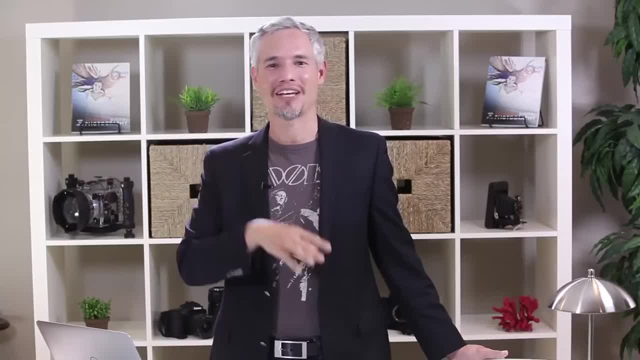 want you to think to yourself whether it's hard or soft light, top light, side lighting, backlighting, etc. Let's look at a picture. Alright, what do you think this is Now? I want you to look at the shadows created. 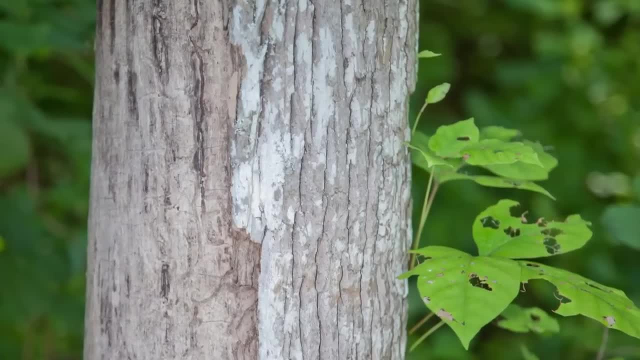 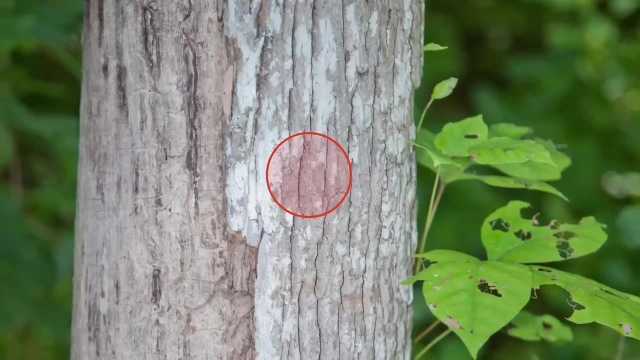 by the bark, because there's an awful lot of texture in this picture, so it gives you a lot of opportunity to figure out where the light is coming from. So we can see some very thin shadows and there's almost no midtones in it. It's almost. 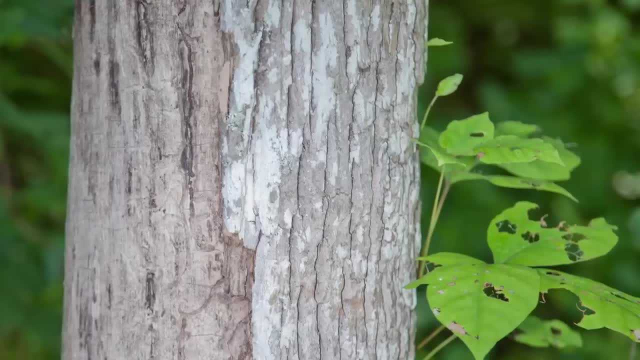 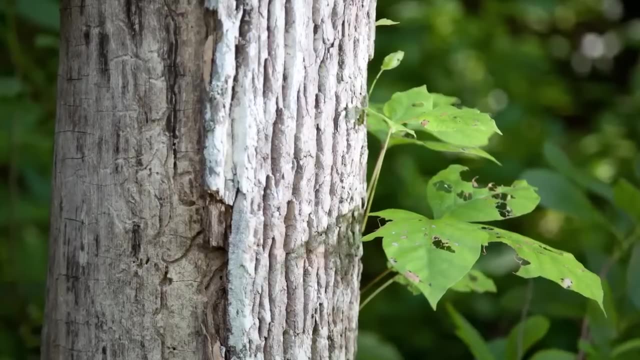 all highlight and black shadows, which indicates that it's hard light, And because the shadows are so short, we can tell it's front lighting. Let's look at another picture of the same subject. Here this is an example of side lighting. We can see so much more texture. 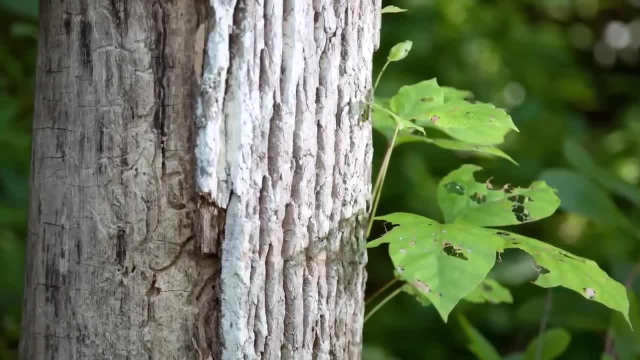 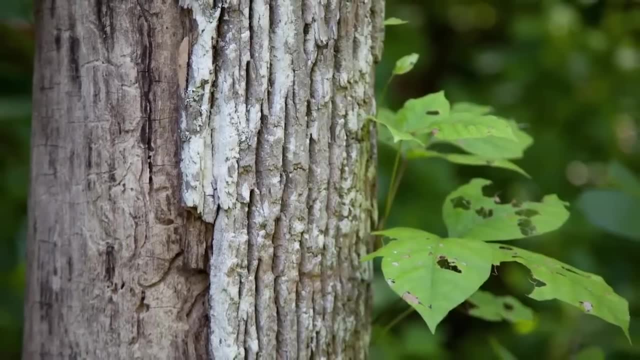 in this picture because the shadows again are so short and distinct, we can tell it's hard lighting rather than soft lighting. Now in this photo, the shadows are much more gradual, much longer. The lighting is still coming from the side, but this time it's. 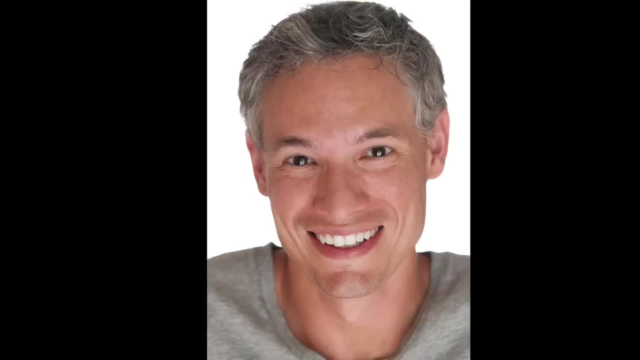 soft lighting rather than hard lighting. Here's a picture of me, and where do you think the light is coming from in this picture? Well, there are actually two light sources. You can see behind me is completely white. That means there was definitely light coming from. 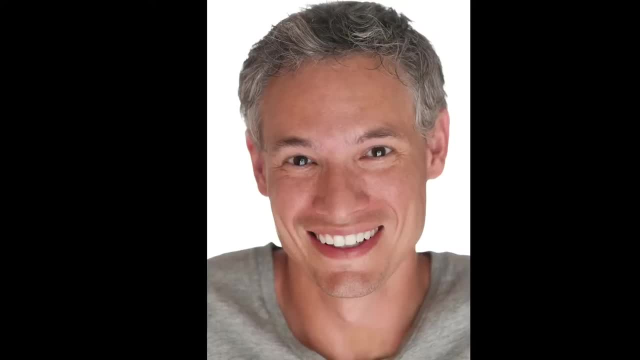 behind me, right Light that's forming the background, But you can also tell that there's some front lighting from the shadows on my face. My face isn't completely in shadow. You can also tell by looking at my eyes where the light source is. So that's a secret. Look at. 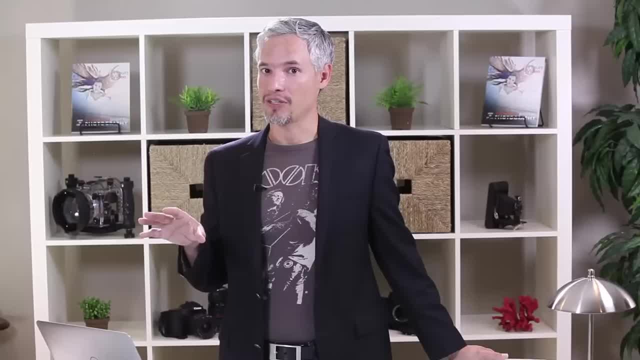 the eyes in a picture and you can often tell how many light sources they are and where they're positioned. Doesn't always work nowadays, because often photo editors will remove the catch lights from a picture or move them around or put in fake catch lights, but often in unedited pictures. 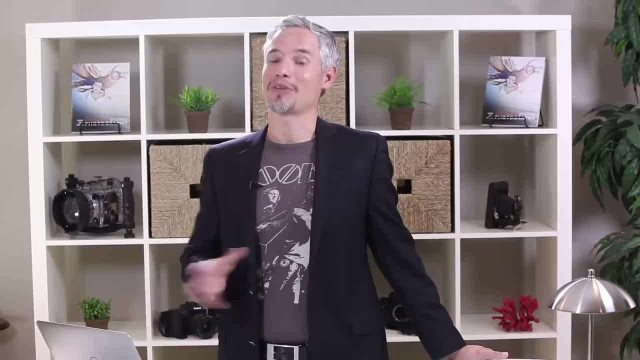 it's a dead giveaway of what the lighting was. That's a good tip to know, because sometimes you see a picture and you think, oh, I wish I could recreate that light. Well, you can kind of reverse engineer their setup just by looking at the eyes. 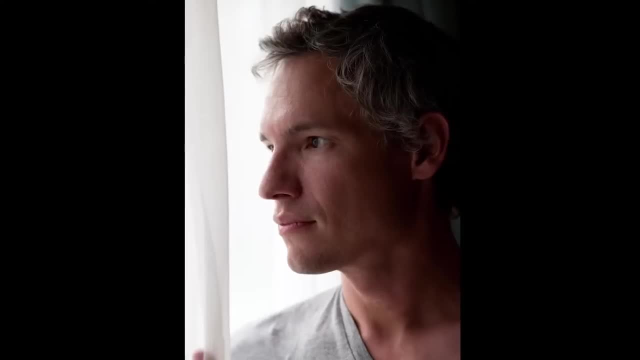 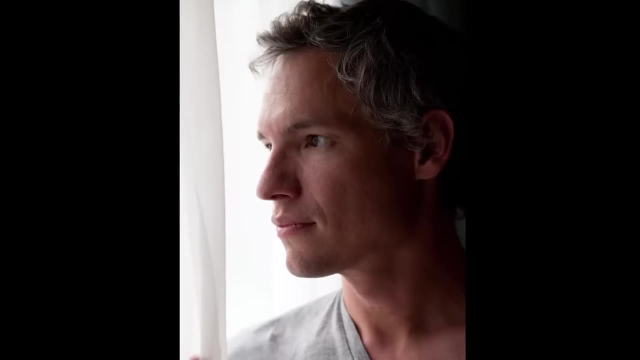 and the shadows and other elements of the picture. So all I did here was I just turned my head a little bit and now you can see it's become more back lighting and side lighting than anything else and it's creating a rim light on my nose. 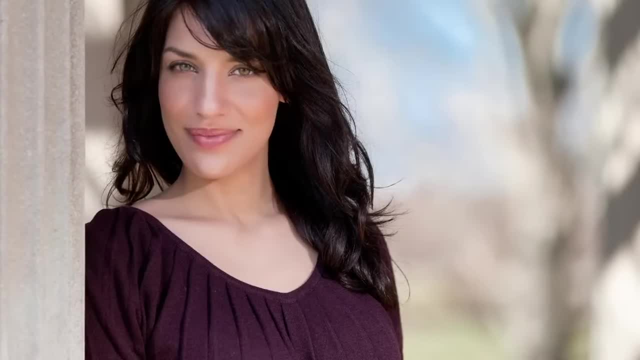 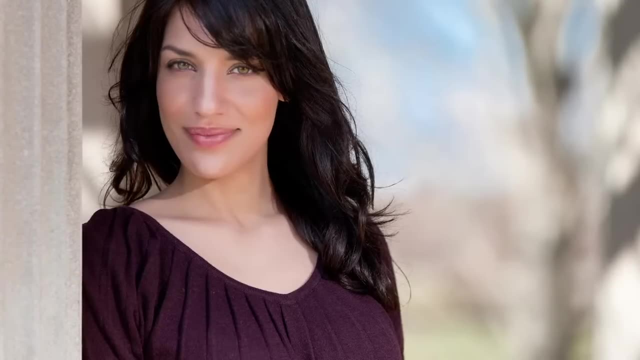 Here's a picture of Chelsea, and for these next few shots I had the flash off camera and I was moving it around so I could really control the light. Now first, hard or soft light on this picture? Well, I'll give you a hint. look at that shadow underneath her chin. 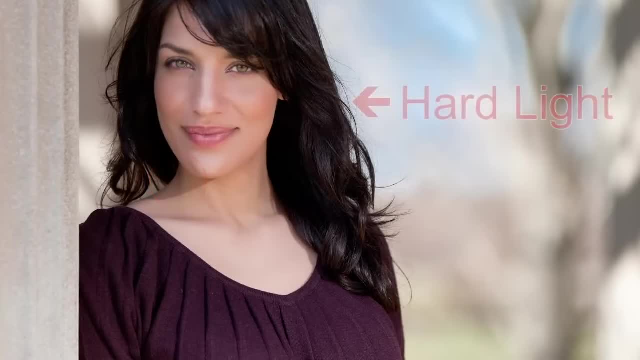 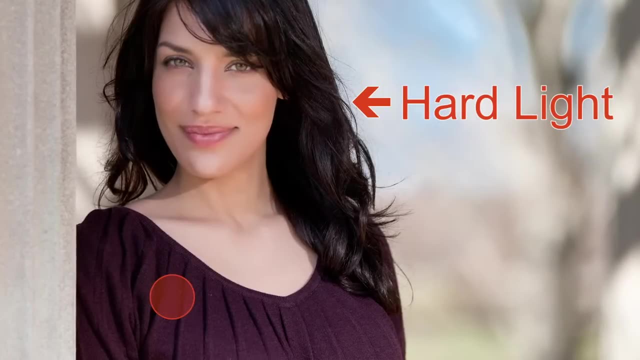 and you can see it's a nice sharp line. that means that it's hard light. That shadow also gives away that it's side lighting and you can see from the shadows on her shirt there that the shadow is being cast to the side- Another good clue that it's side lighting. 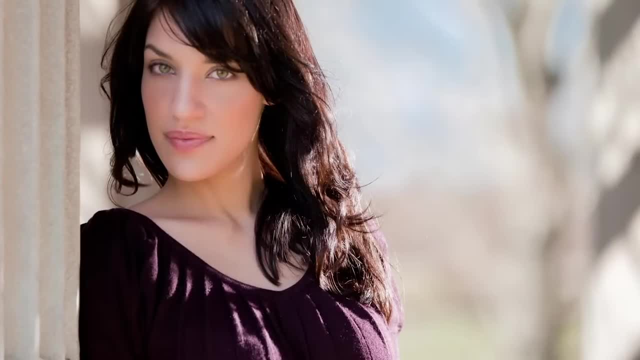 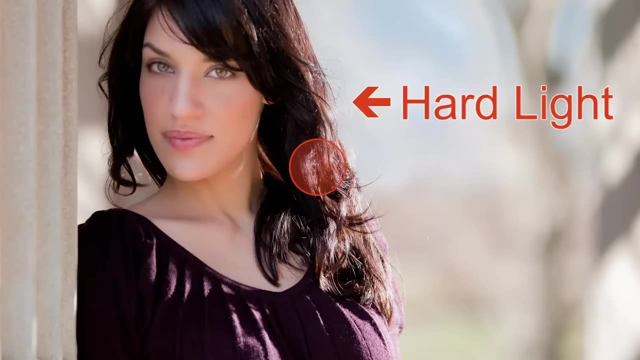 Now, what do you think here? Hard light or soft light? Well, truthfully, it's a mix of both, because there is a hard light source, as you can see from the highlights in her hair and the shadows that are being cast across her shirt. However, her face itself, 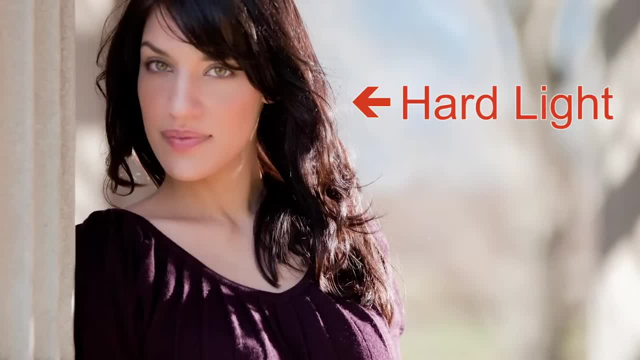 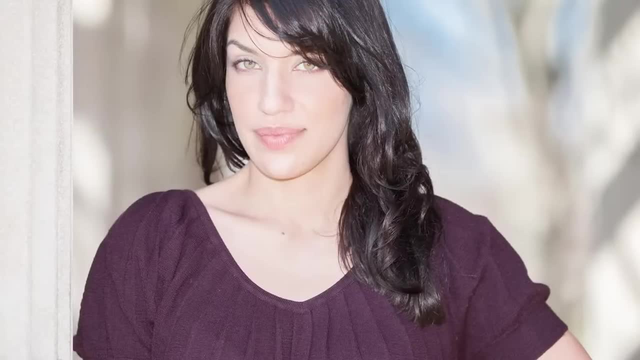 is completely in shadow, So her face has very nice soft lighting, but there's hard, direct lighting behind and to the side. that's illuminating her hair and the shirt. Okay, first, what do you think? Hard light or soft light? Well, I think we can tell it's hard light by: 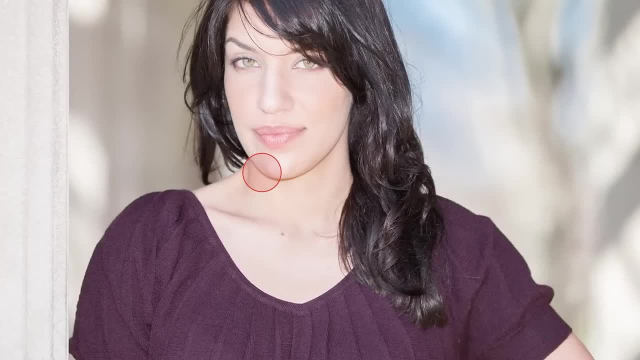 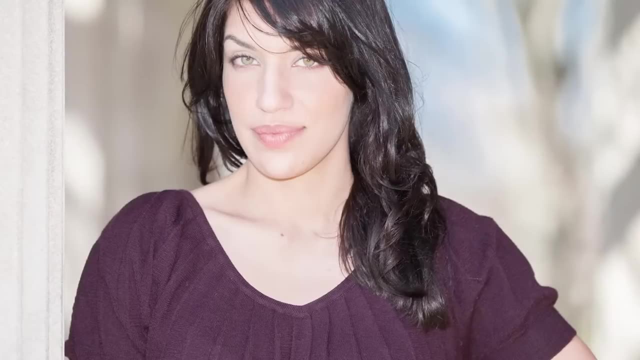 looking at that hard, distinct shadow underneath her chin- Not exactly flattering right. Soft light is definitely better for portraits And can you tell whether it's coming from the side or behind, or from the front? Well, it's definitely coming from the front First. you can see the catch light from the flash. 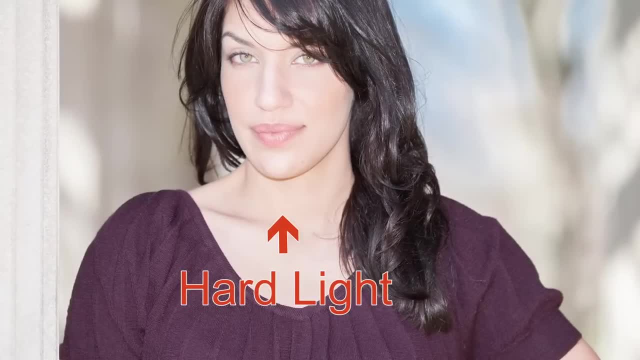 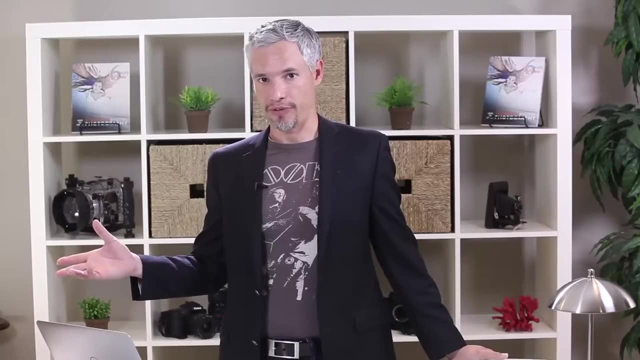 in her eyes, but also the fact that she has a shadow underneath her chin and it's not going to the side or anywhere else and there's no room lighting from a back light, Just simply hard direct front light from a flash, and that's very typical of 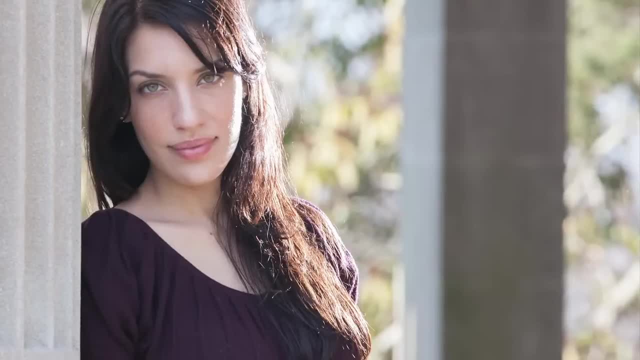 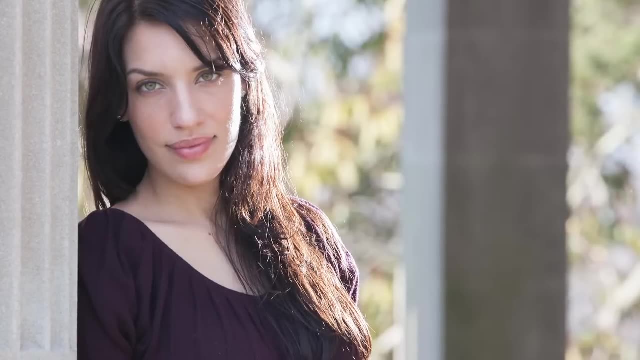 what you'd get from an on camera flash at full power. Again, take a minute and think about whether this is hard or soft light, or maybe some combination of both. Is it front lighting, top lighting, back lighting, side lighting? Well, the answer is. 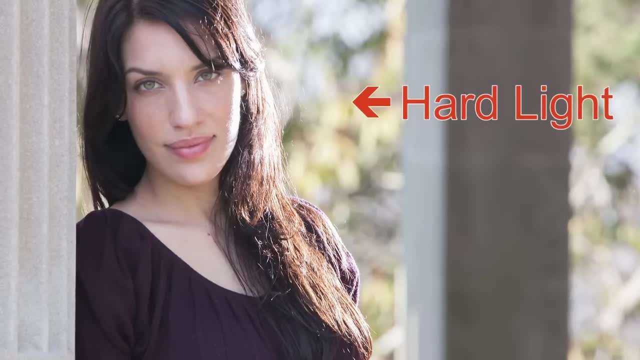 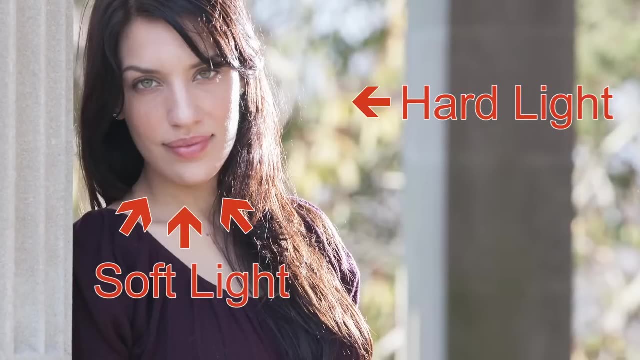 that it's hard side lighting. but because her face is in shadow, her face is being illuminated by just the ambient light in the shadow Light that's bouncing off that pillar next to her and the trees around her. So her face itself has nice soft light. 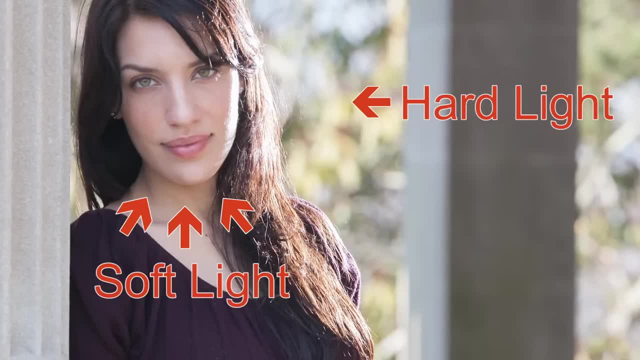 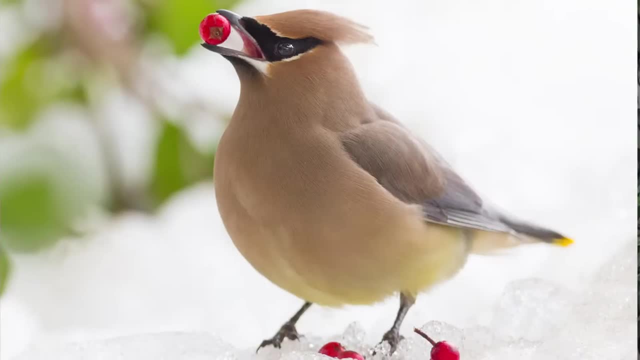 but she's being lit from a direct hard flash off to the side and that's lighting up her hair. Here's a picture of a cedar waxwing in the winter, and I talked earlier about the snow and the effect that it has, So that will probably give away. 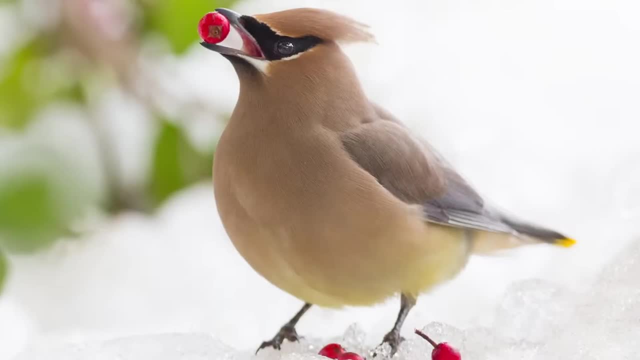 whether this is hard or soft light. right, Anytime you're in the snow, it's probably going to be soft light, Even if the sun is out, there's so much fill coming from the snow that it tends to soften it quite a bit Now, in this case. 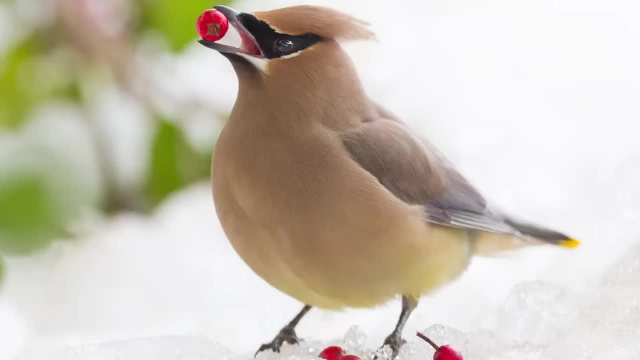 the bird was hiding under a bush, So the only way it's being lit is really from the snow, and we have about the softest light you could. Now, as a side effect of that, you can't see much texture in the feathers at all. You can kind. 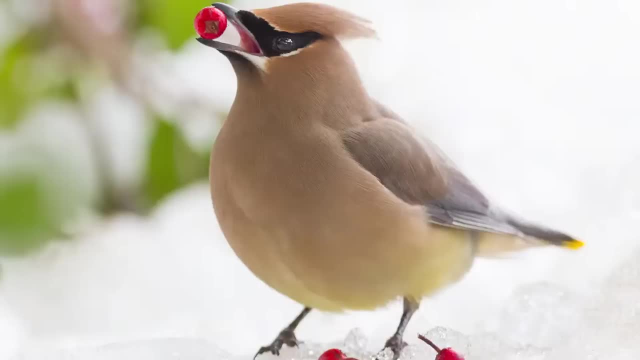 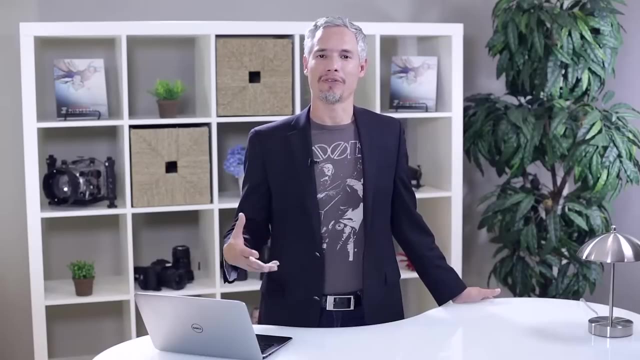 of see them, but there's not nearly as much detail as there would be if there were hard light. Now let's talk about the golden hour. The golden hour is a period of about an hour before sunset and an hour after sunrise, when everything is just way more beautiful. 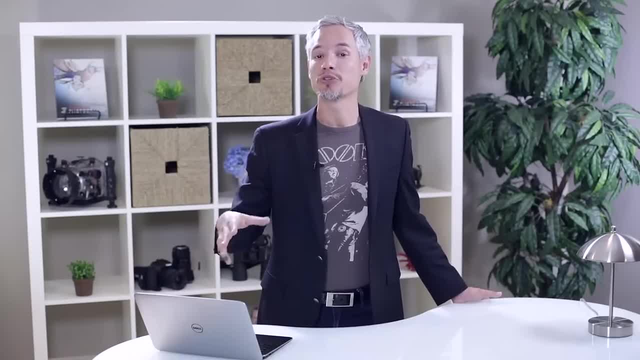 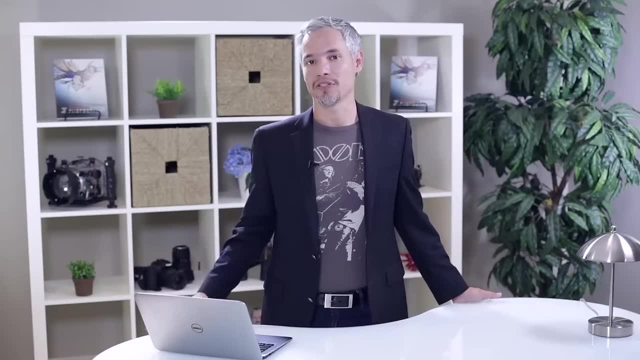 During the golden hour the sun is low to the sky, So what you get are side lighting and back lighting and front lighting, but not that awful and really difficult to deal with top lighting. In the mornings, the sky tends to be especially clear too, because the humidity 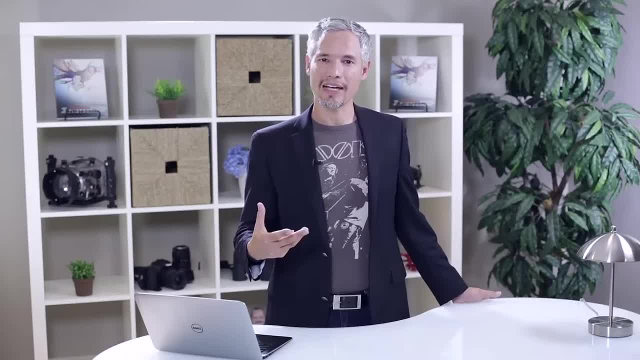 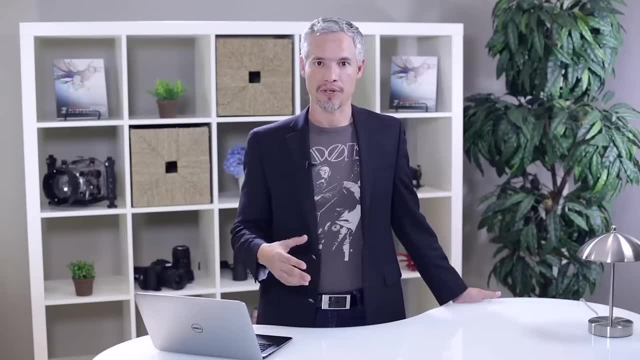 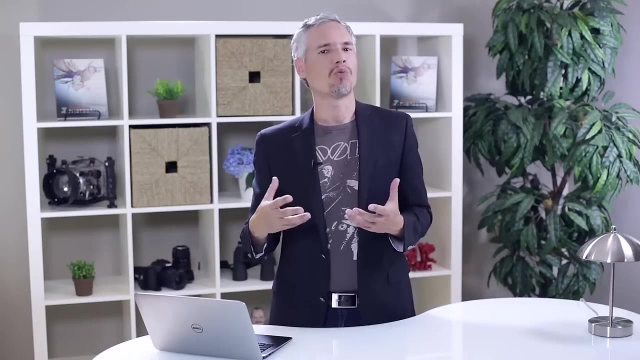 drops overnight, the temperatures are cooler and that clear sky gives you more distinct and hard lighting, which can make really powerful shadows and create more impactful pictures. Because the sun is low to the horizon, it's actually passing through more atmosphere than usual and that gives it a very warm. 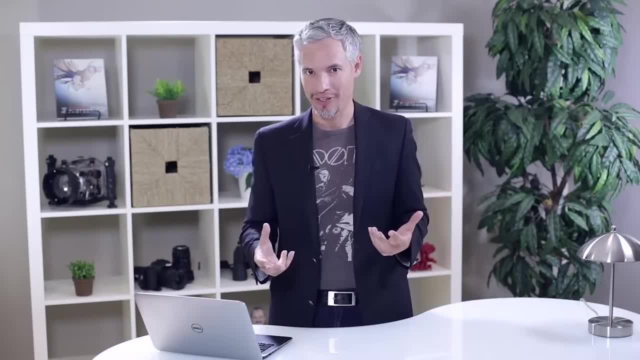 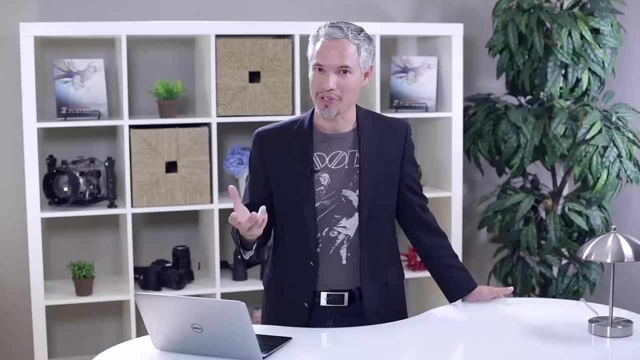 color. That's why the sunrise and sunset tend to be this like golden color, But at the same time, the sky, because it's not being lit by the sun being above it, the sky takes on this deep blue color and because all your shadows are being lit by the 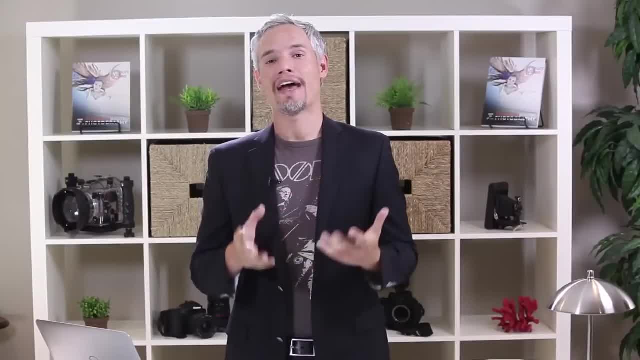 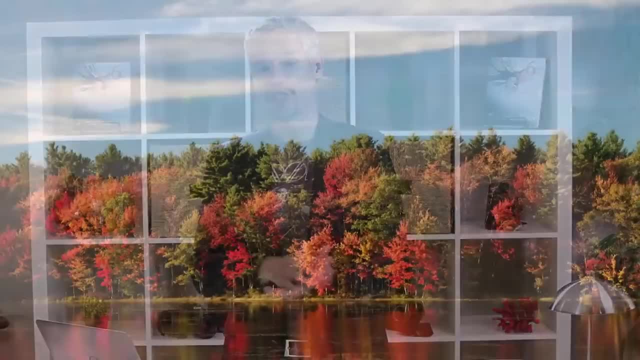 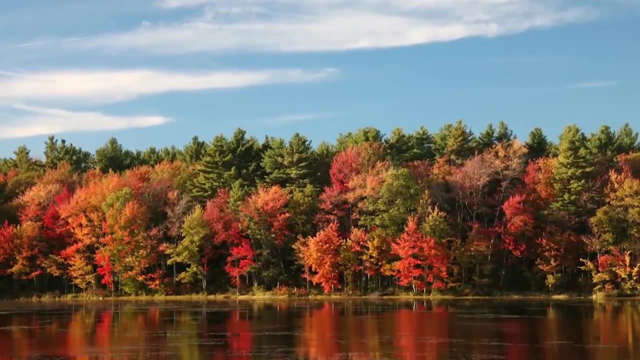 ambient air, they also take on a nice cool tone. So what we have during the golden hour is this gorgeous contrast of warm red and orange is coming directly from the rising or setting sun and the deep blues that we have in the skies and the shadows, and these oranges and blues are very complementary. 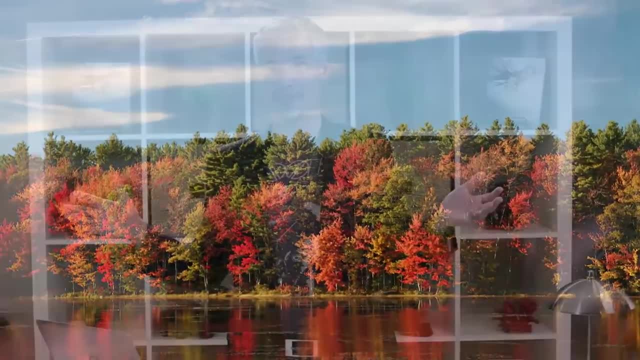 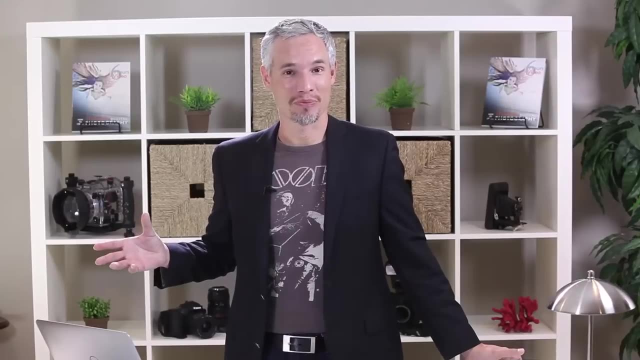 colors. That means that you just have an amazing color palette of light all around you. Now I'm kind of selling the golden hour hard, and it's because I'm not a morning person and usually when the sun is setting I'd rather be maybe having a. 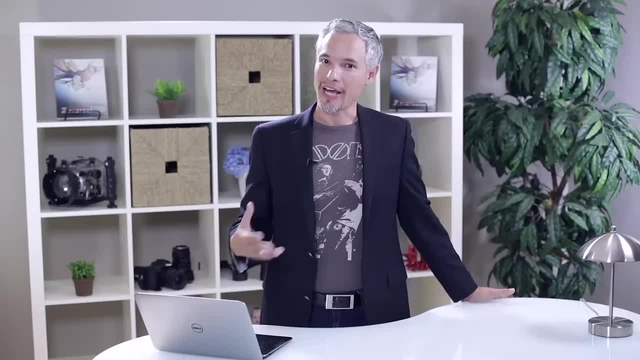 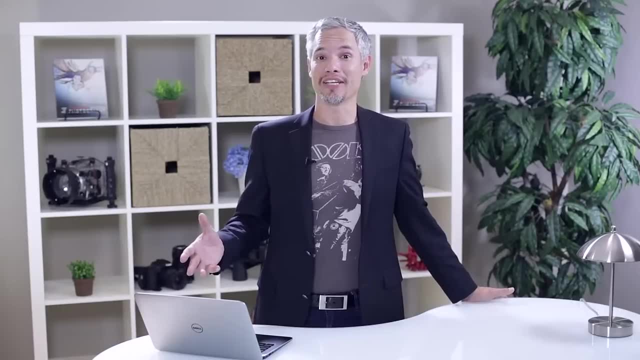 drink or eating dinner. I feel that it's worth it to really plan your photo outings around the golden hour. Now we say the golden hour, but depending on where you are, it could be a golden 10 or 15 minutes, or it could be a whole golden. day When you're on the horizon, like say in Hawaii or in the Caribbean, well, that sun will set so fast You could literally see the sun dropping towards the horizon. It could be gone in 10 minutes- really could Now, if you go really far north. or south, you will see sunrises and sunsets that last for hours, And in fact I was in Sweden recently and the sun never really set in the middle of the summer. I woke up in the middle of the night and it was still completely lit and you could see. 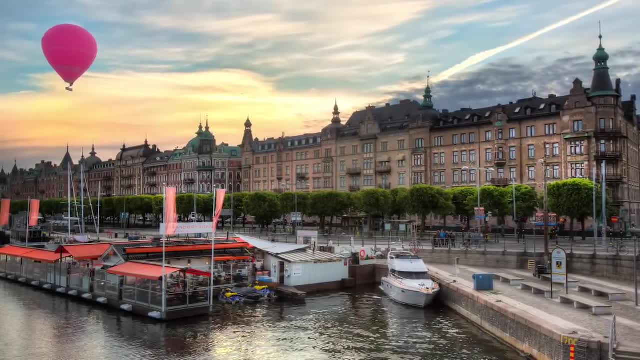 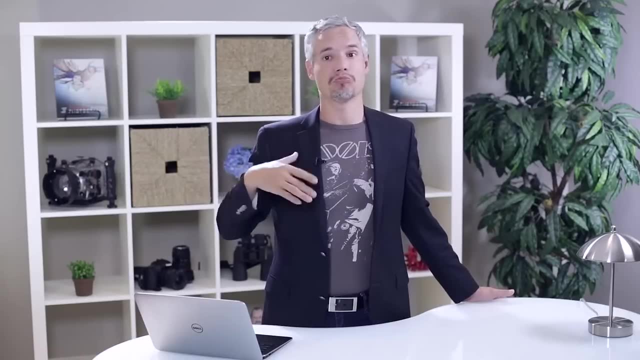 just a glint of the sun on the horizon. When you're at the extremes, the sun just kind of dips below the horizon, but it's still casting that light and for that reason the golden hour can last for 6,, 8,, 10 hours. 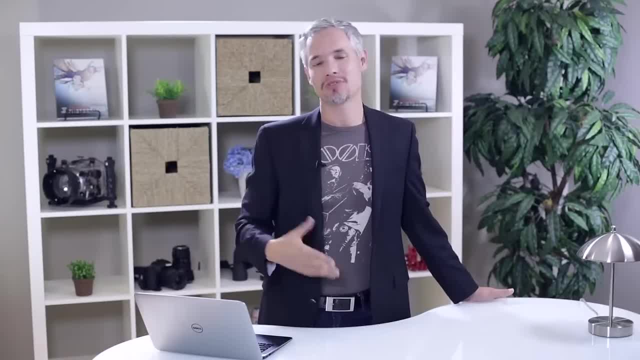 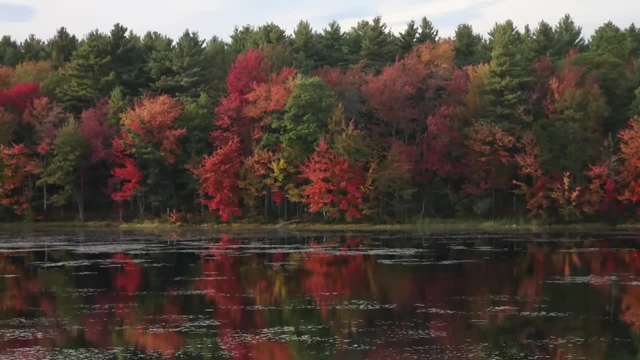 and that means that you have a lot of opportunity in those areas. So just plan accordingly. Let's look at a couple of example pictures Up here. first we have a photo of New England foliage and you can see it's quite beautiful and the colors are very nice. 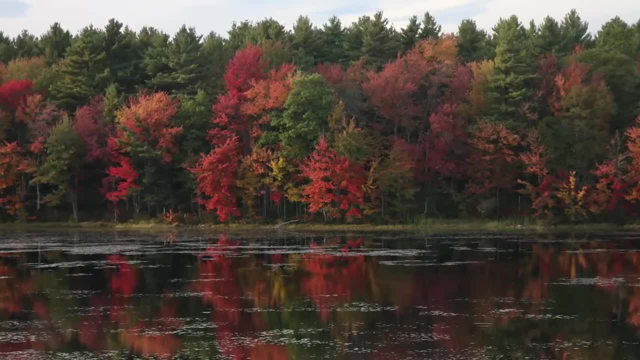 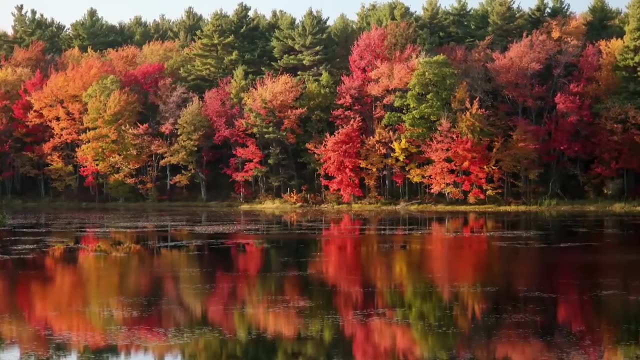 and this has taken I don't know, let's say 15, 20 minutes before the sun set. All I had to do was wait just a few more minutes until the sun got a little lower in the horizon, and we got this Now. 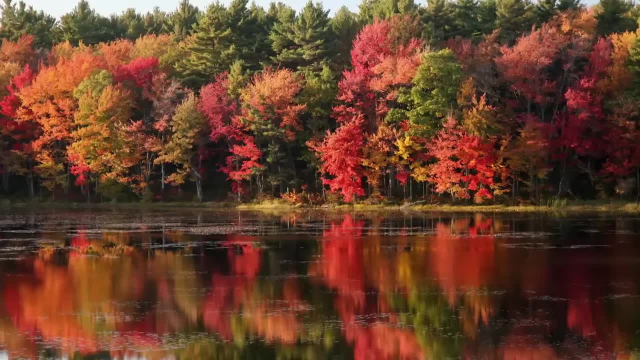 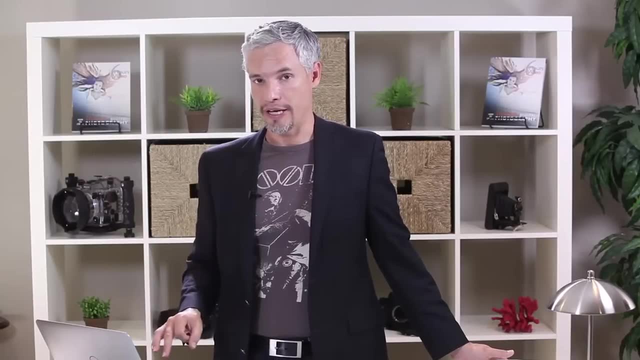 look at that distinct difference. Here the colors are so much richer, and the difference is just that the sun set a little bit more. That's how much of a difference the golden hour can make in your pictures. Let's look at another sample photo. This is Salzburg. 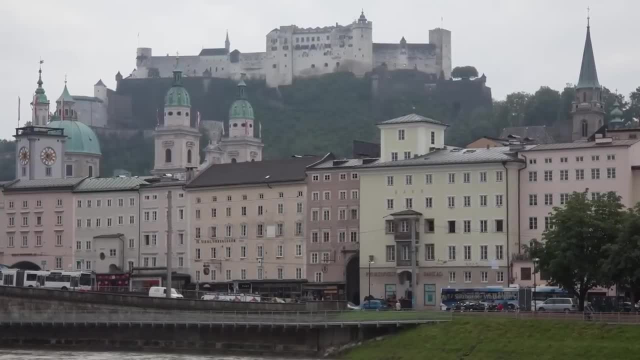 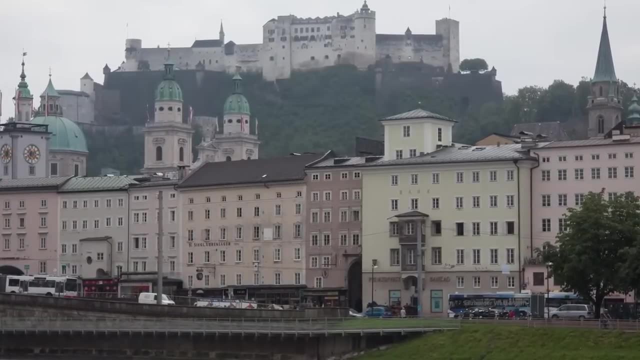 Austria and I took this photo in the middle of the day and it hasn't been retouched at all and, as you can see, it's kind of flat and ugly, because during the middle of the day it was naturally hazy and the lighting wasn't good. but 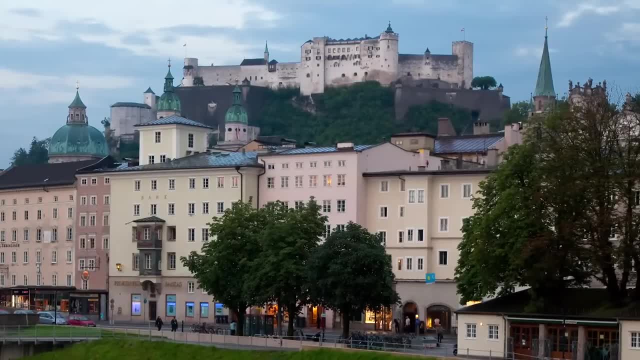 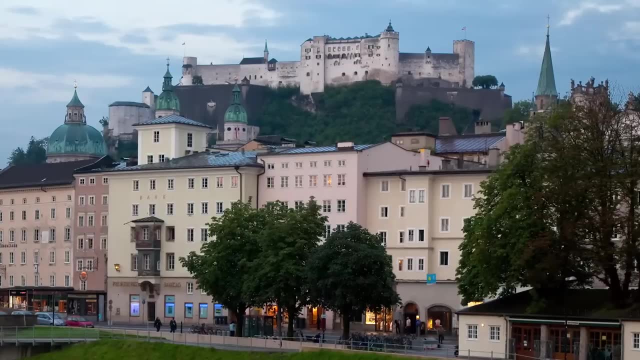 here we are during the golden hour- I think this is in the morning- and the buildings are being lit by nice front lighting from that low sun on the horizon and you can see that sky is a nice deep blue, but the buildings themselves are taking on this nice warm. 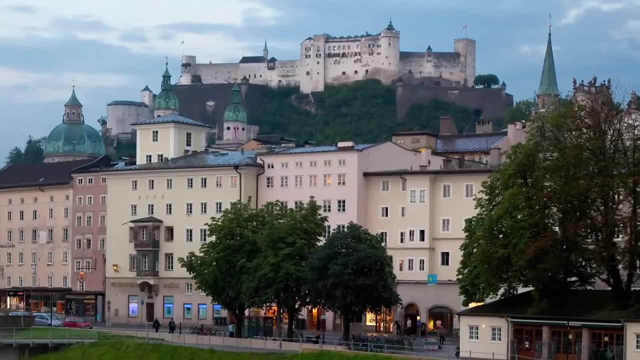 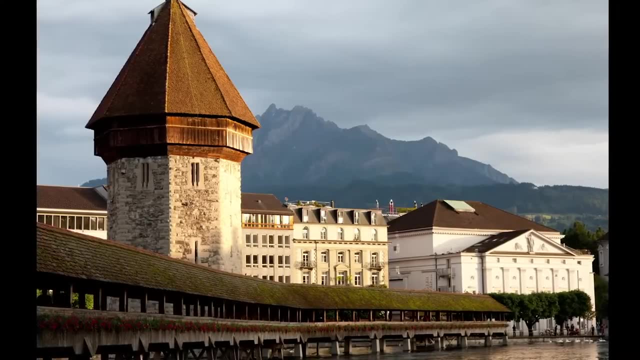 tone, The colors are so much more flattering and the lighting is just so much more nice during the golden hour. This is a picture of the chapel bridge in Switzerland, and I must have taken a hundred pictures of this bridge trying to get it right, but the one that really worked was this. 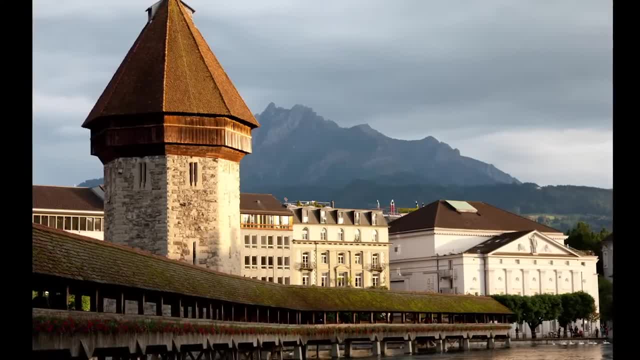 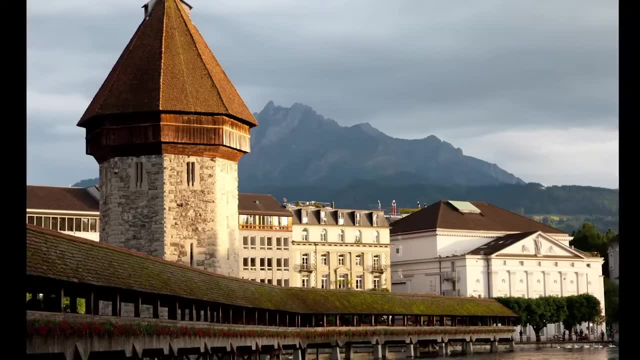 one at sunset, and because the sun is low to the sky off the right side of the picture, it's creating side lighting and that side lighting is showing off the three dimensional form of that tower. With any other sort of light you wouldn't be able to see the differences. 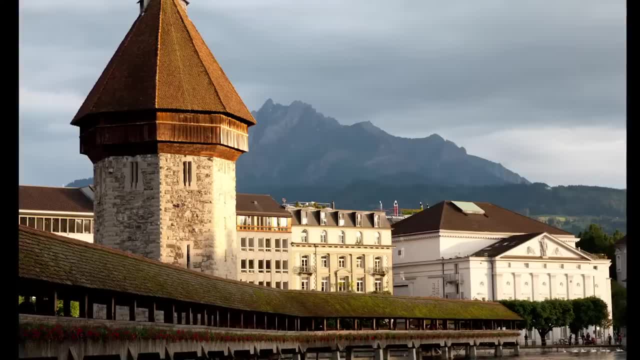 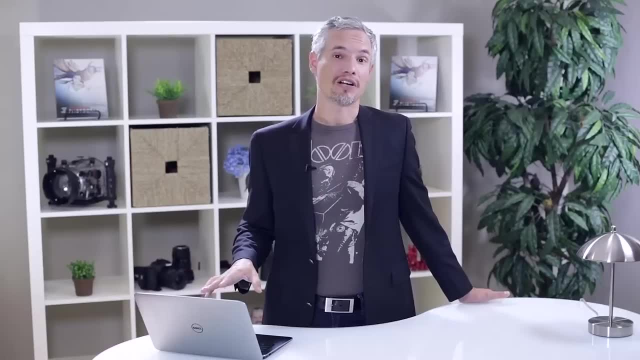 in the facets of the building. It's also creating that nice warm color in the tower itself and the nice cool color in the skies that we see in the background there. Now let's talk about controlling the sun. Yes, you can actually control the sun. You can be a natural light photographer. 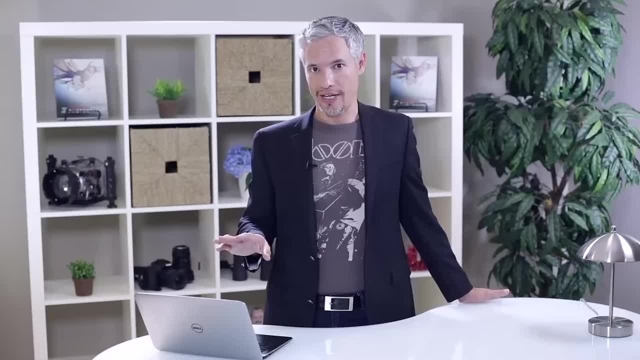 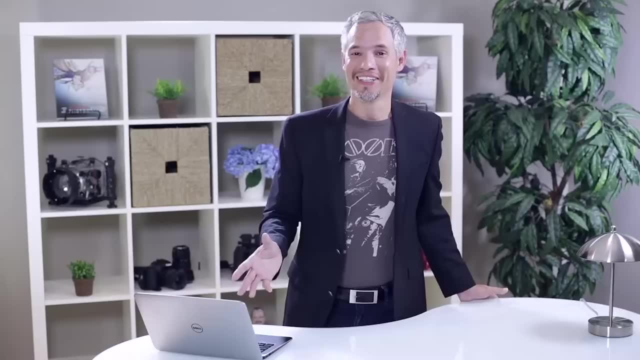 and have near perfect control over your lighting conditions. You just need to do a little bit of planning, and I've hinted at that already by talking about the golden hour: Get up a little bit early, right, and get out there when the sun is rising or when the sun is setting. But there's also a pretty huge difference between sunrise and sunset. After all, they happen in completely different directions. So if you wanted to take a picture of a building, you might want to pick either the sunrise or the sunset, where the lighting was the most flattering. 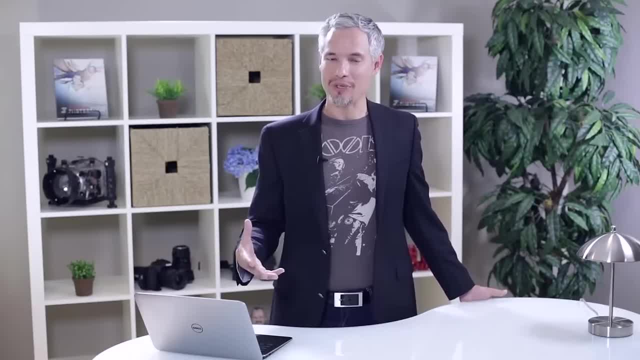 You can do that by just looking at your subject and kind of watching it over time and seeing where the sun rises and how the light hits it. That's great for your own house if you're there all the time, But you can also find some software. 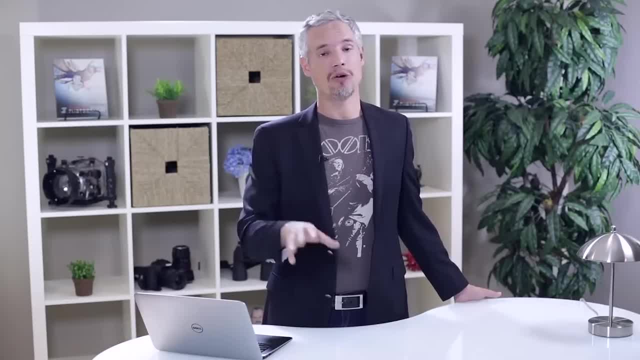 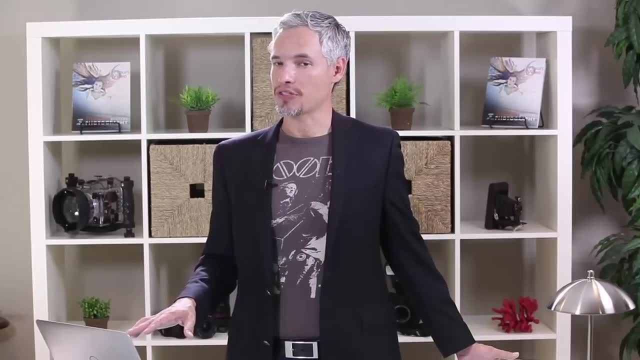 tools that will tell you exactly where the sun is going to be and how it's going to be lighting different subjects. So now I'll jump onto the computer here and we can take a look at my favorite app, which is called the Photographer's Ephemeris. I'm going to be looking at the PC. 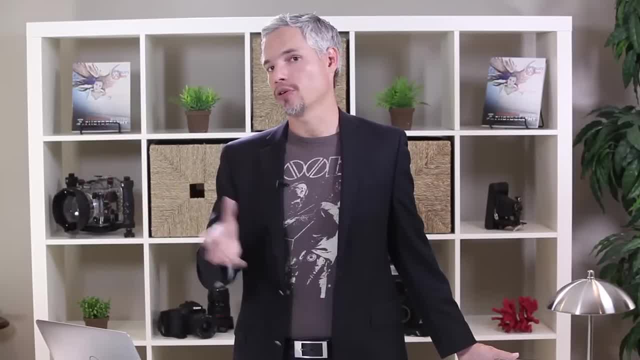 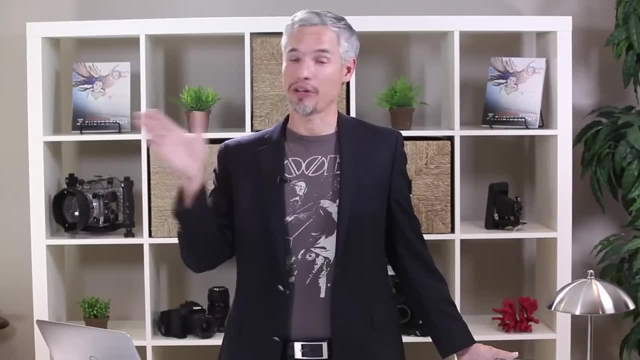 app, but you can also get mobile apps for your iPhone or Android phone, and I find that they're really useful when I'm out traveling, because I can just quickly look up and see exactly where the sun is going to be at any given time of day and when that sun is going to be rising. 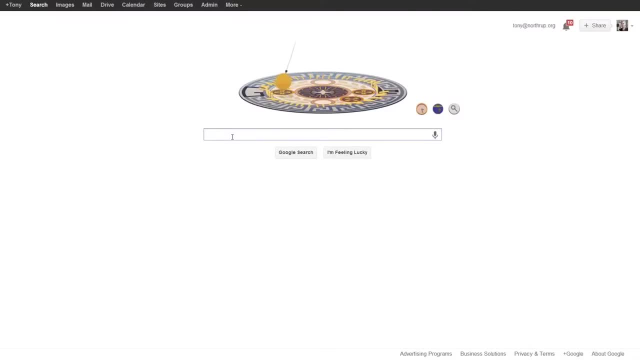 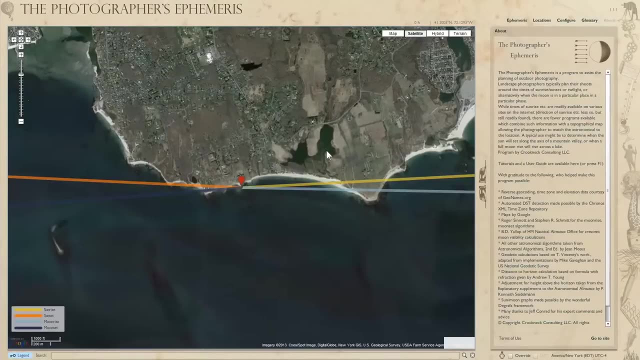 or setting First to find the Photographer's Ephemeris, I suggest you just go to Google and search for Photographer's Ephemeris. You'll see this window and at the bottom here you can search for a particular location. So I'll jump over to. 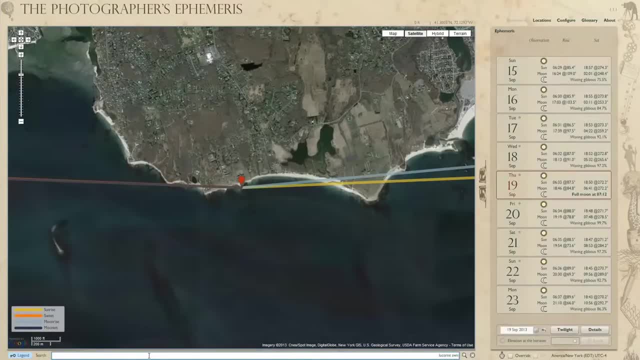 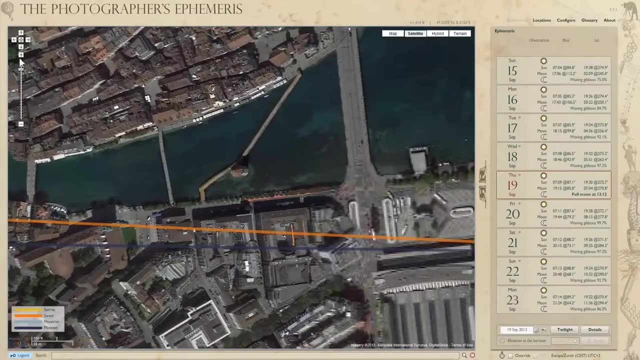 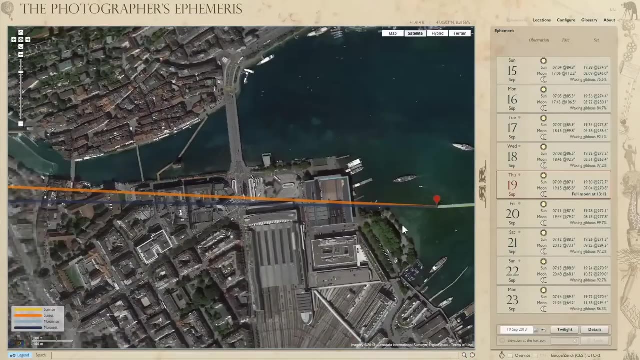 Lucerne, Switzerland, And if we zoom in a little bit here, we can find that chapel bridge that I was just showing you a picture of. Here we go, So I'll take my marker and just drag it right to the bridge, because I want to see how the 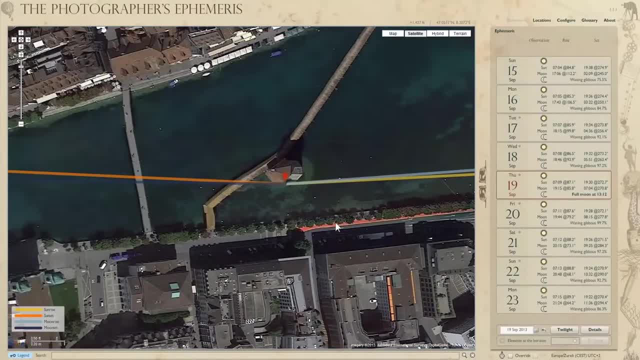 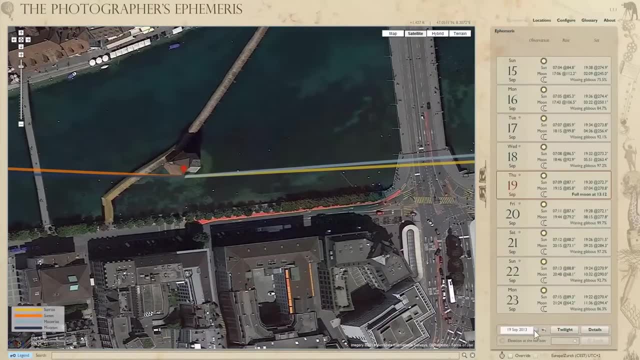 sun rising and setting is going to be striking it. Today is September 19th and we can see that the sun is coming right in from the side. But if I switch to a different time of year, let's say January 3rd, my birthday- 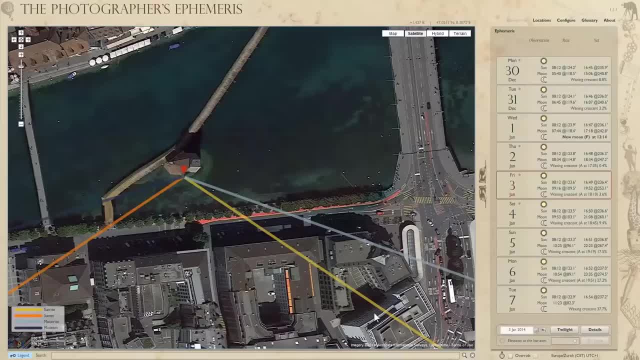 here. we can see the sunset right here, and the sunrise is coming at a much steeper angle. It's going to be coming in almost from this direction, So if I wanted to get that side lighting, well, I'd have to be standing over here instead of over. 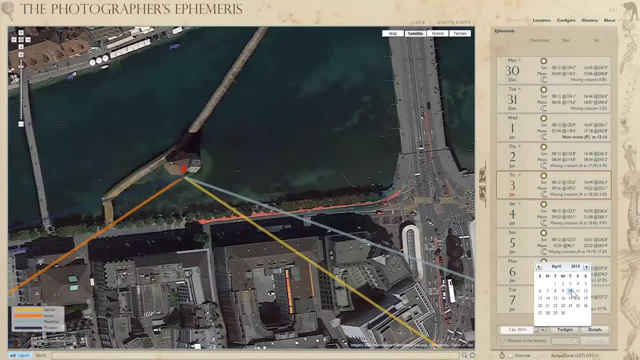 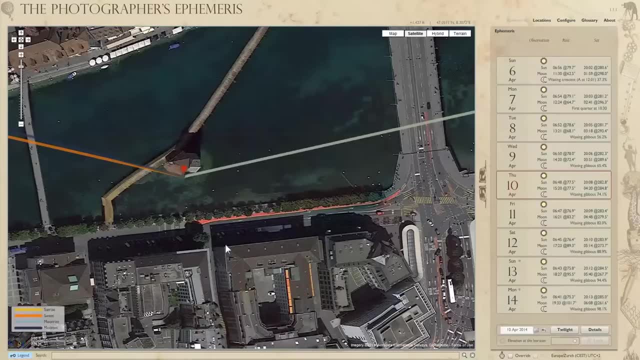 here. If we jump forward a few more months into April, we can see the sun is now coming from just a very different direction. So you can see, I'd have to plan something very different. Now let's head over to New York City. 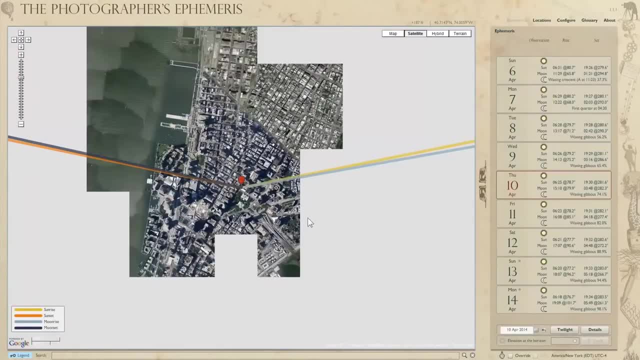 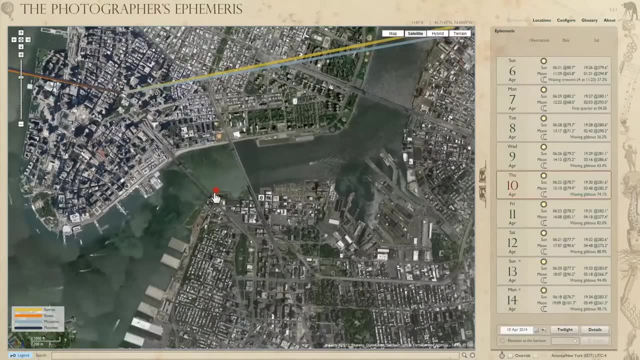 Zoom back a little bit and I'll find one of my favorite spots, which is actually just outside of New York City, in Dumbo Park, right here next to the Brooklyn Bridge. So I'll drag my marker right over here. Oh, you know what? 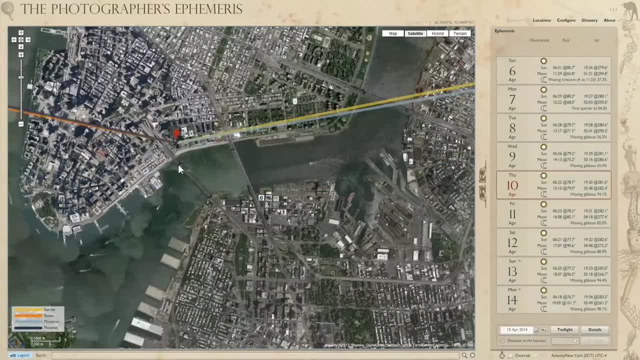 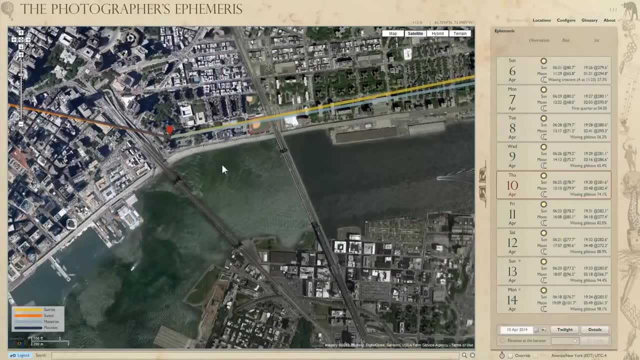 The great thing about it is the view that you get of the skyline. So I'll leave the marker here in the city and we'll just pretend that we're looking at it from here So we can see. I'm still on April here and we can see that the rising 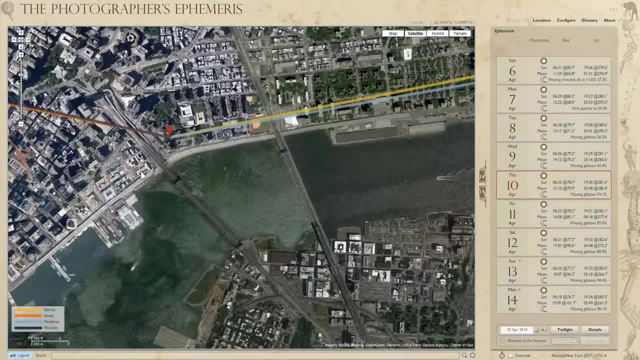 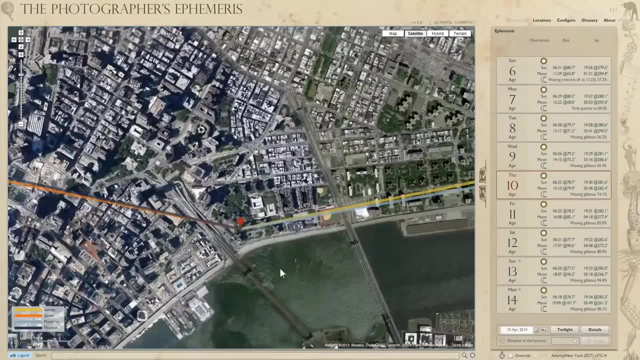 sun is going to be coming in from the right and striking the buildings over here, And the setting sun is going to be kind of behind the city, but also more to the side if you're looking at it from this way, from Dumbo Park down here. But let's see. 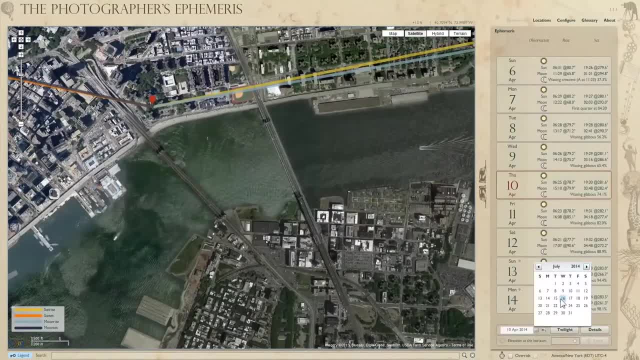 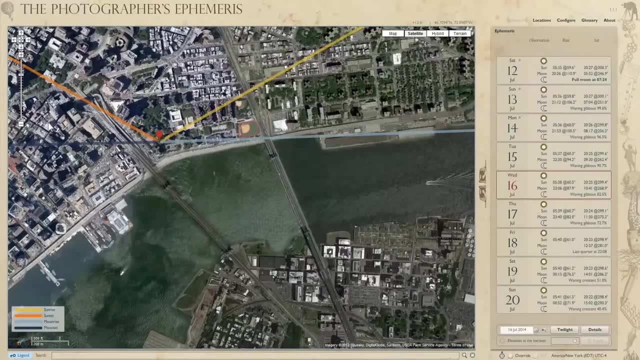 what it looks like in the summer. As we get into mid-July, we can see that both the rising and the setting sun are going to be more behind it, But the sunset is going to be right behind Manhattan. So if you wanted to get the sun, 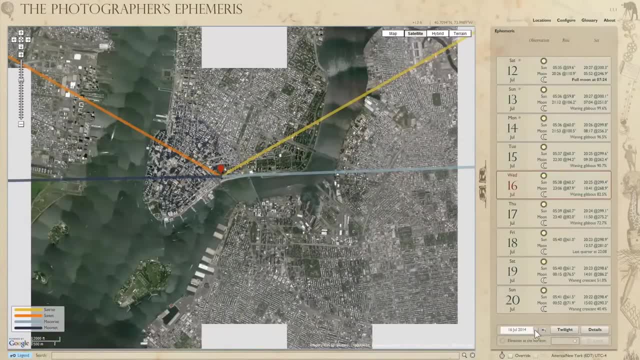 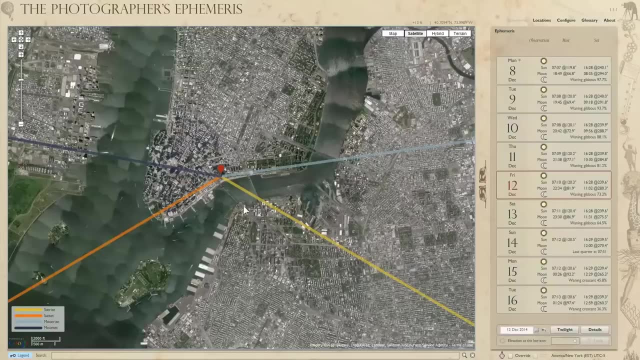 setting behind the city. you could do that in the summer, But you wouldn't be able to do that in the middle of the winter. If you were to visit that same spot in mid-December, you wouldn't see the sun setting behind the city. You'd see the sun setting over. 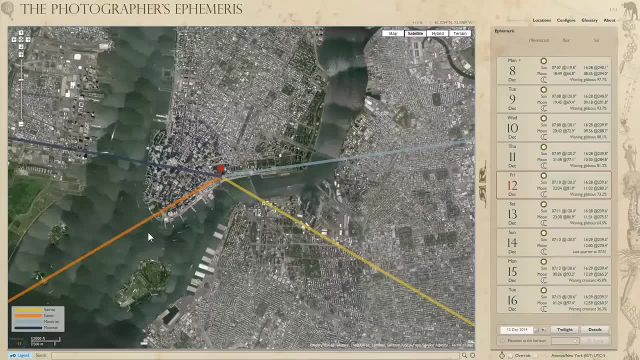 to the side of the city and that would just dramatically change your lighting conditions. However, you could now get the front lit city during sunrise- This is the sunrise here- and it would be to your back- and therefore just illuminating the buildings just beautifully in the middle of the winter. 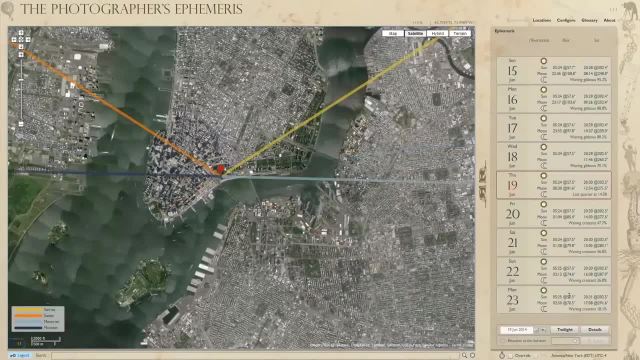 If you were to go during the summer, pick mid-June, the rising sun would not front light the buildings, It would be sidelighting the buildings. So you get a completely different picture. I also want to show you that it's telling you exactly. 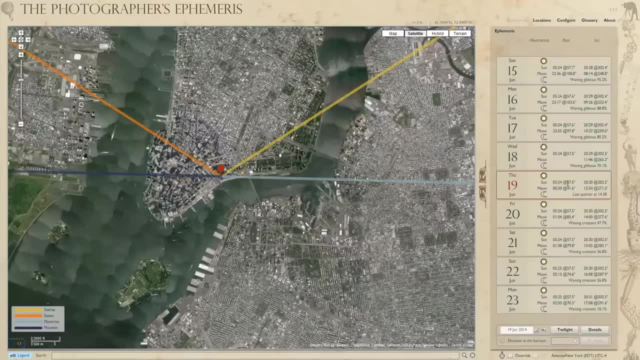 what time of day the sun is rising and setting. So here on June 19th, we can see that the sun is rising at 524 AM and it's setting at 830 PM, And if you're into night photography, you can check. 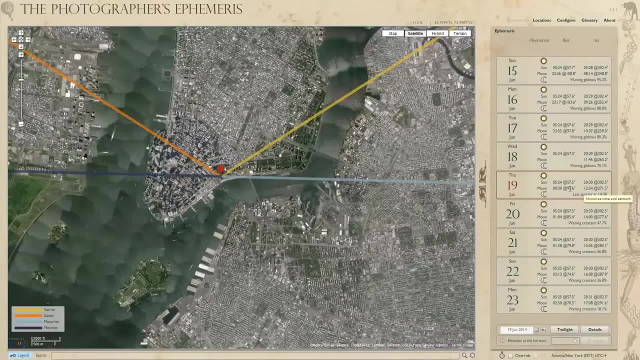 out the moonrise and set times. 0030 here means 1230 at night and the sun is setting at 1254.. So that's when the sun is going to be up. That's particularly important, of course, if you want to take. 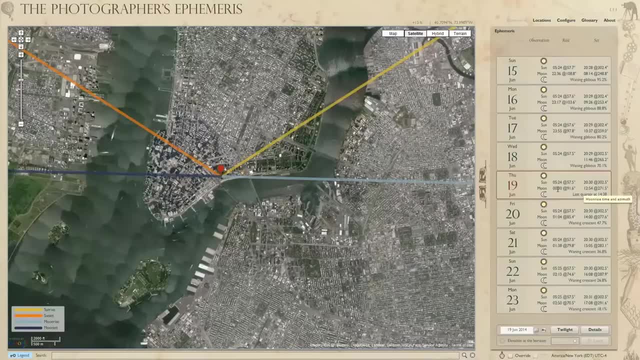 a picture of the moon, You'll need to know what time it's rising and setting. But if you want to take a picture of the stars, you'll also want to know, because you'll want to choose a night when the moon is not up or 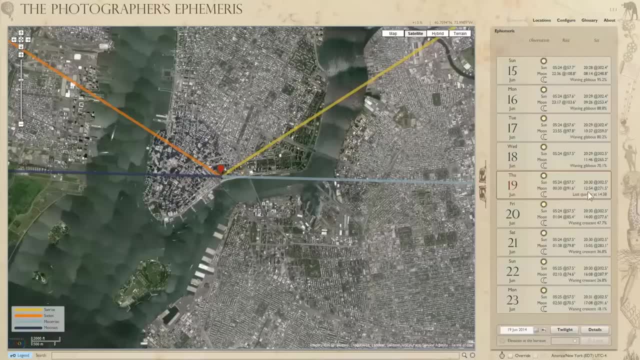 when the moon is almost completely gone. So here we can see it's at the last quarter here, But if we jump forward just a few more days we'll be able to see that there's the moon is almost completely gone, down here at 1.8%, So even 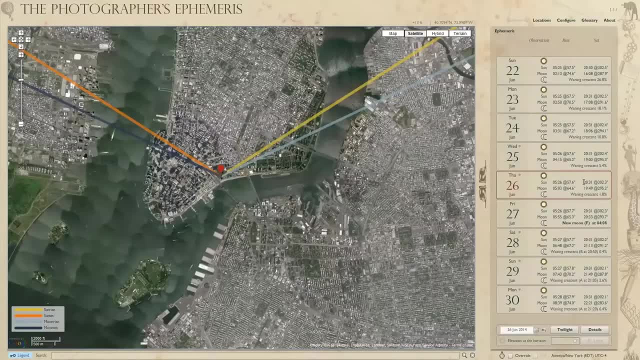 if the moon were up on June 26th here, even if we were out at night, you'd still be able to get some stars, because it's almost completely gone If you were to try to shoot the stars on a night with a full moon. 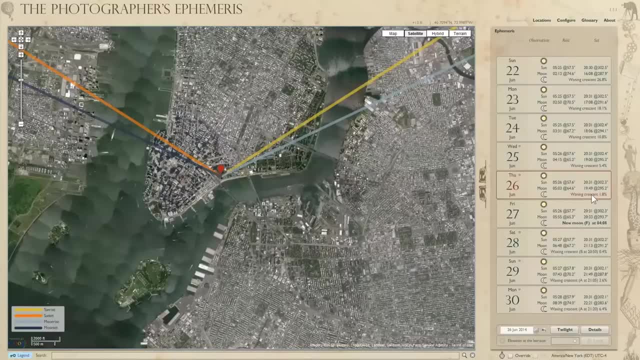 well, the light from the moon would completely blow out your stars and you wouldn't be able to get a clear view. So being able to track both the moon rise and set time is important, as well as being able to check the moon phase. Now, of course, beyond that, you'll also want to be checking 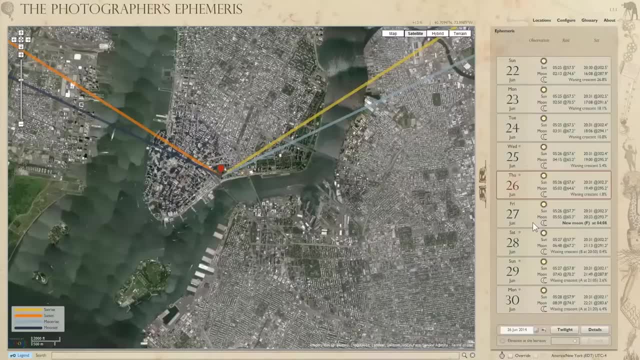 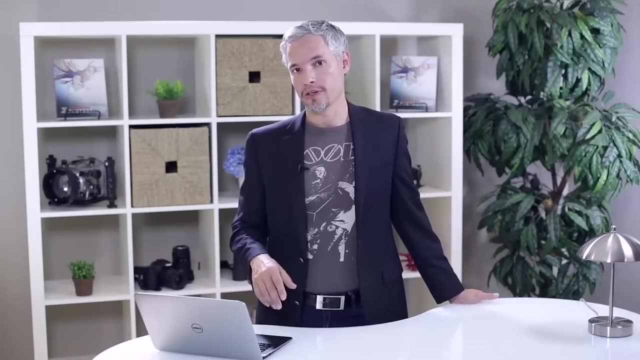 your weather, because you can know that the sun is rising, but if you have a thick cloud cover, you're not going to get that golden hour light that you're looking for. So that's the Photographer's Ephemeris. It's free for the PC and Windows. 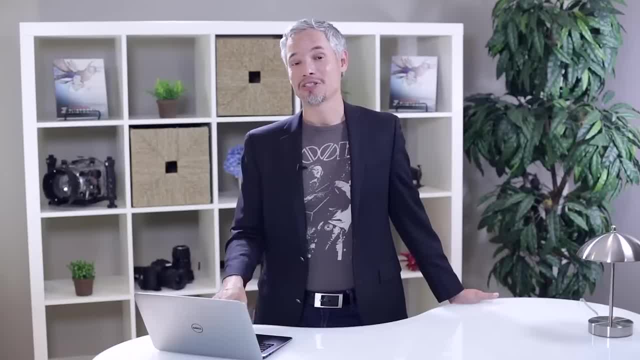 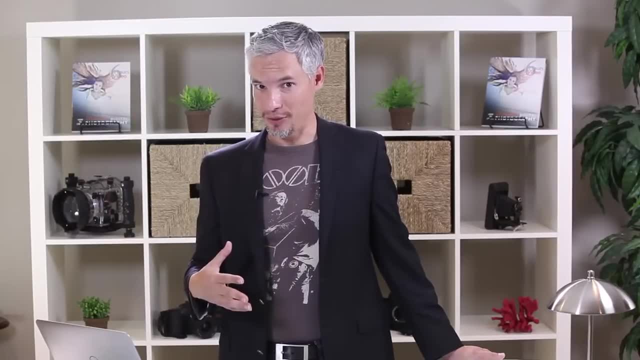 but it costs a little bit. if you want it on your mobile device Now I'll show you an app that's free, no matter where you go, and that's Google Earth. It's particularly powerful when they have the 3D buildings available, like in major metropolitan. 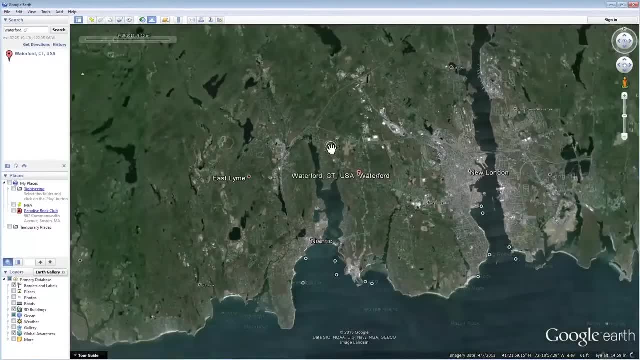 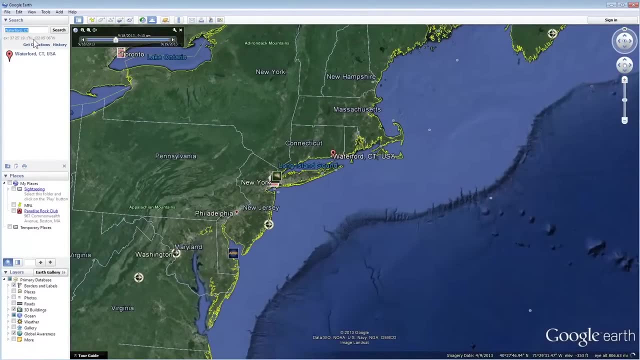 areas. So let's take a look at it now. Here we are in Google Earth and let me zoom back a little bit, and then I will jump over to one of my favorite spots in the world, which is Dumbo in Brooklyn, New York, Dumbo Park basically. 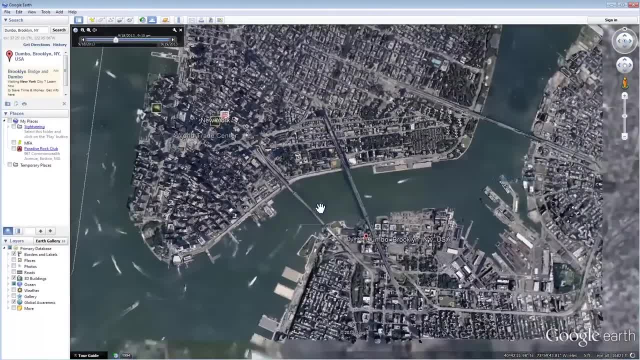 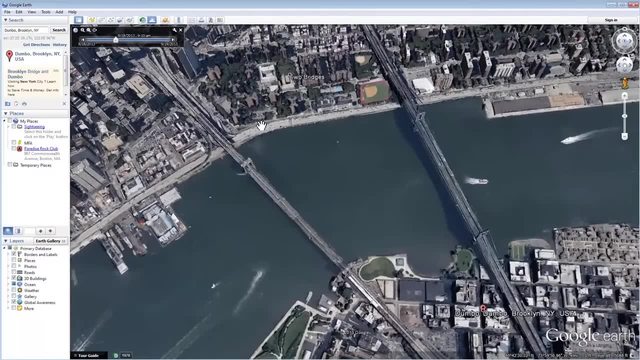 So it's pretty close and, as we can see, this is Manhattan here and this is the Brooklyn Bridge, and that's the Manhattan Bridge and this is Dumbo Park here, And you just get this amazing view of the city. So I'm going to hold down the control. 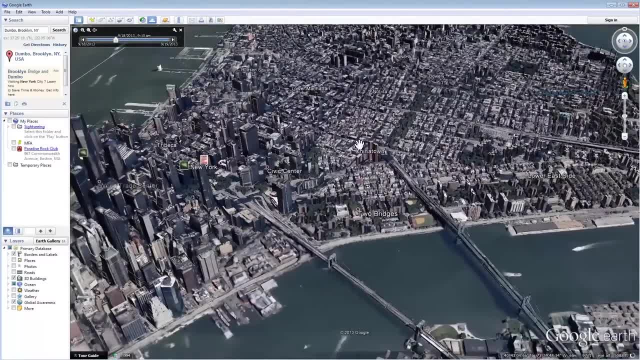 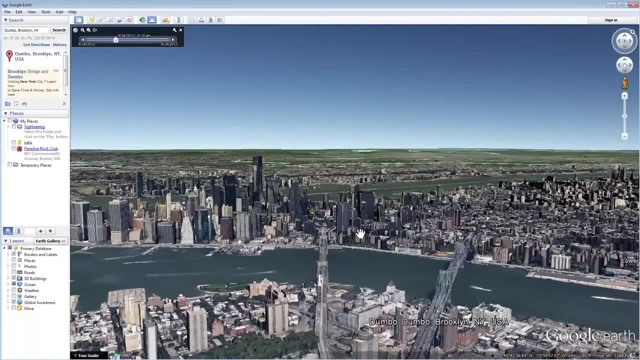 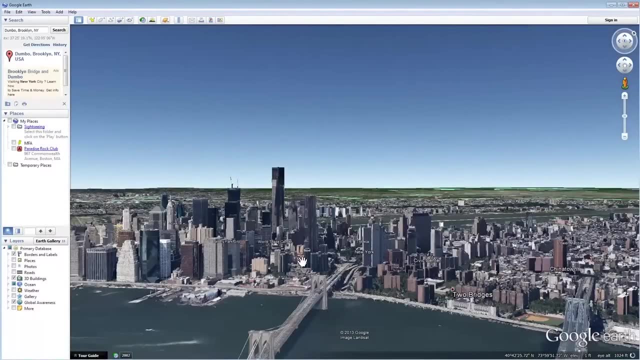 key and kind of pan the whole map back. Now I'm holding down the shift key to give myself a little tilt and I'm just kind of maneuvering the map until I position myself right in Dumbo Park Now. so this is a great way just to find a spot. 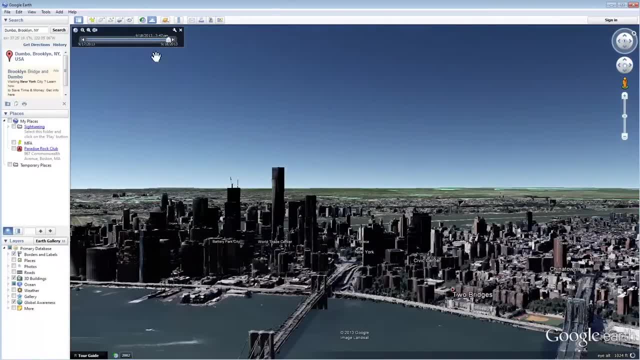 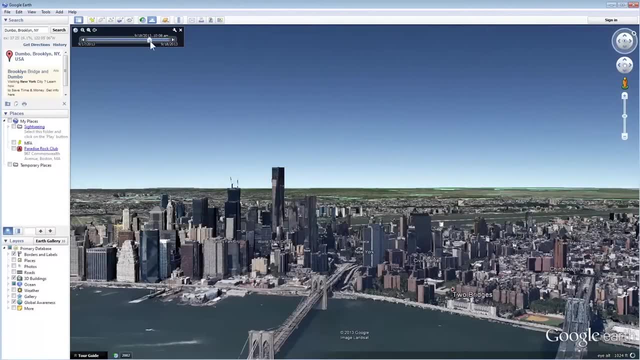 but if you want to see where the sun is going to rise or set, you can click this little sun button here and then it lets you adjust the time. So it's set to the current date, which is September 18th, and, if you can, 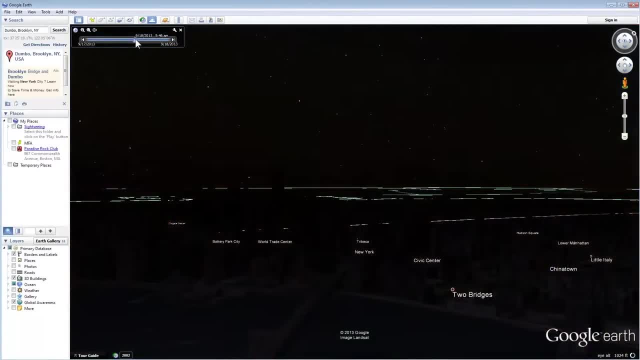 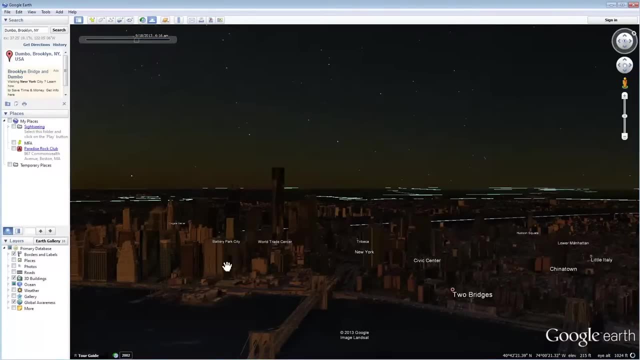 see, I'll go back a little bit before sunrise and so we can see the sun coming up about 616 and you can see that it's actually plotting out how the sun is going to shine on the three-dimensional buildings of New York, which gives you a good idea. 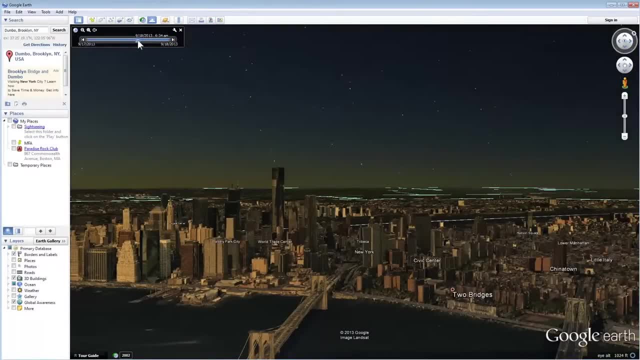 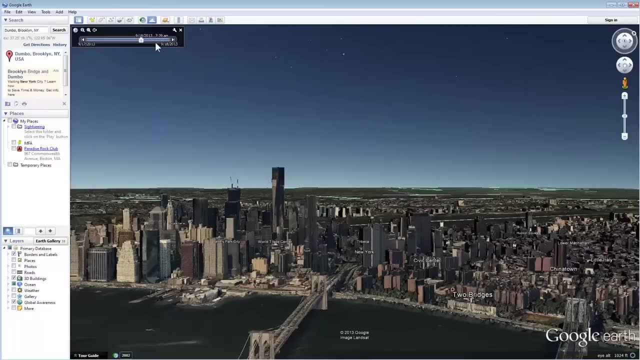 of what the lighting would look like, and that side lighting does look really nice. It gives a real nice depth, and so we can see, by 640 we start to lose some of the beauty. Now the sun's by 740. here the sun is pretty high. 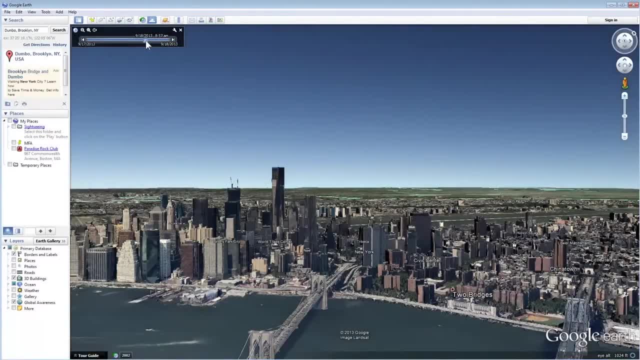 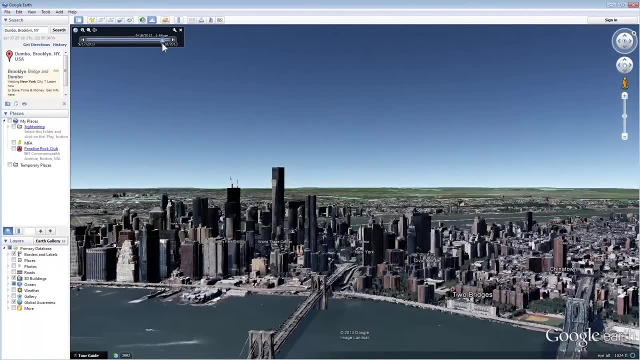 in the sky, so this would give you a good sense of when you actually needed to be there. and then, as we can see as the sun progresses throughout the day, it's pretty boring and flat and doesn't change too much, and you can tell from the lighting that the sun is going. 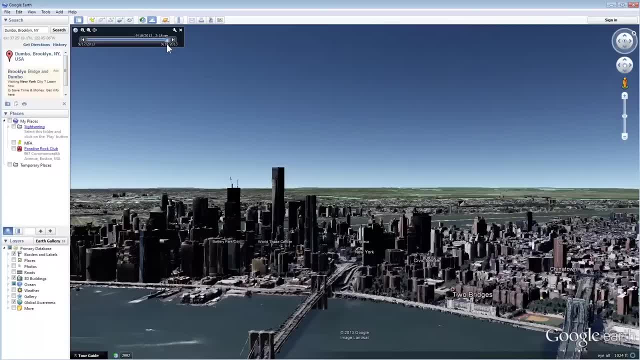 off to the right side of the sky, as it does during the summer, and as the sun is setting after about 3 o'clock here, we don't have any direct light on the buildings, which would mean they'd lose all their color and all their pop. They'd all be in just the 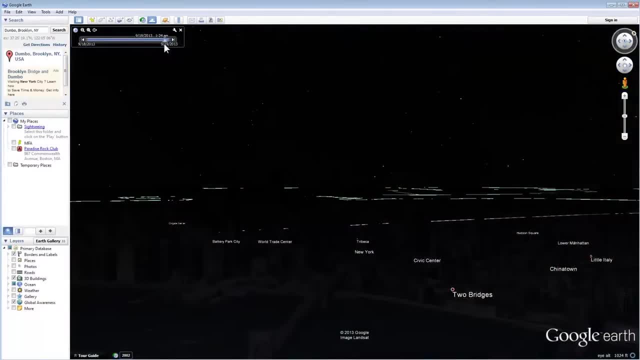 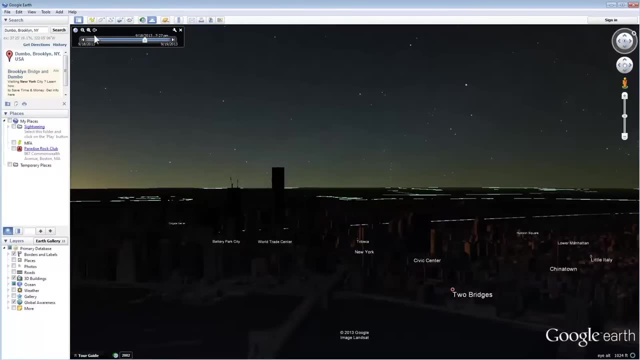 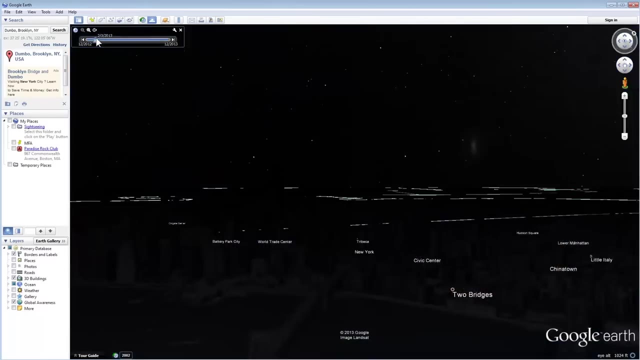 shadow of the sun as it's approaching the horizon. Now, this is what New York is like in September, so let's jump to a completely different time of the year. Let's go into mid-January, right near the winter solstice, and I'm using these 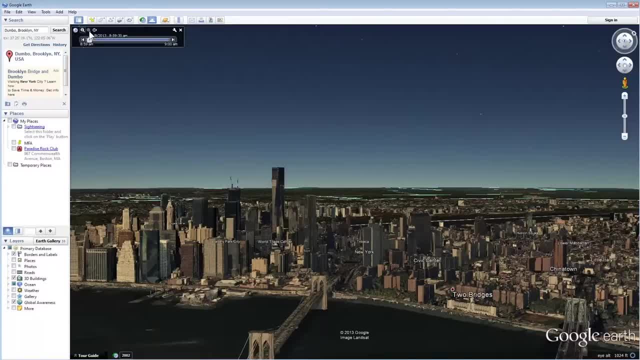 little magnifying buttons plus and minus to kind of control how much detail I see in the timeline. So now it's zoomed in to give me a sense of what it looks like in about one full day, and so this is what the sun would look like. 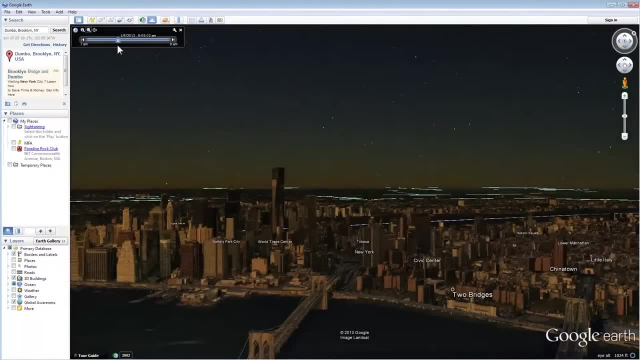 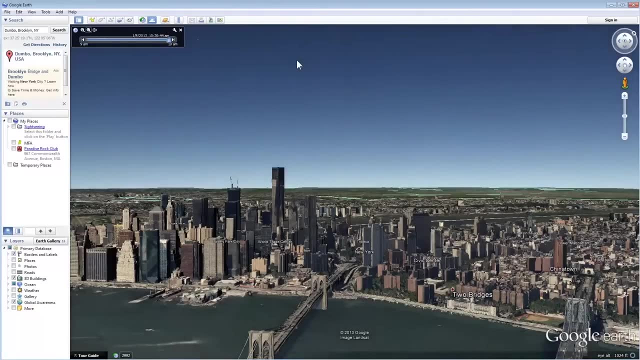 as it was rising in the middle of January and it's not too different from the summer, but as we get closer to the sunset. so now you can see that clock it's about 11 o'clock and this is what it looks like mid-day. now we're at about 1 o'clock. 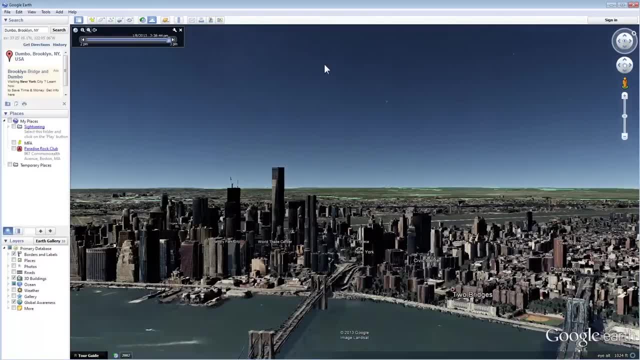 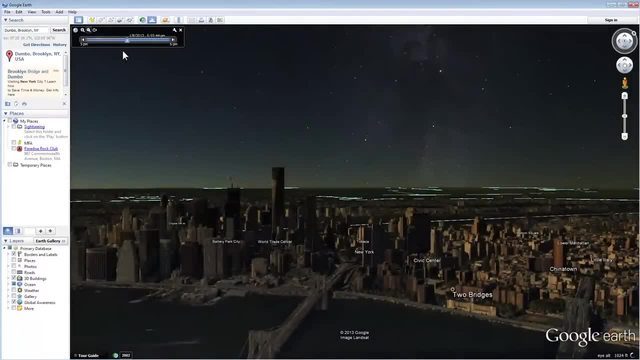 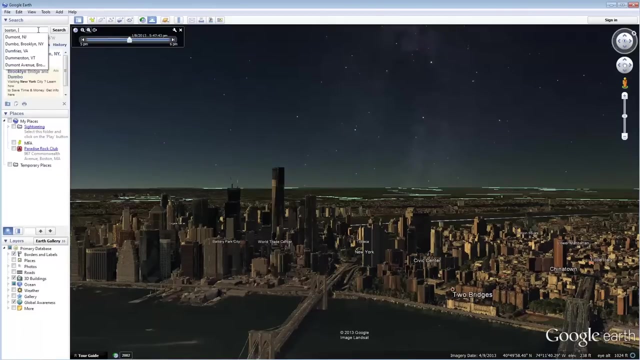 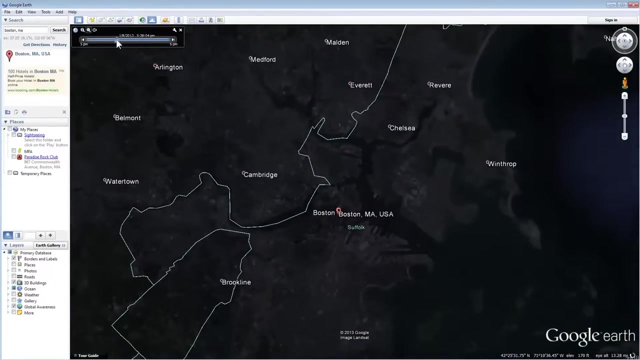 and then about 2 o'clock and 3 o'clock, and here we can see the sun casting everything in shadow once again and the stars start to come out. now let's jump over to Boston to adjust the time so that it's bright once again. I'll turn off the. 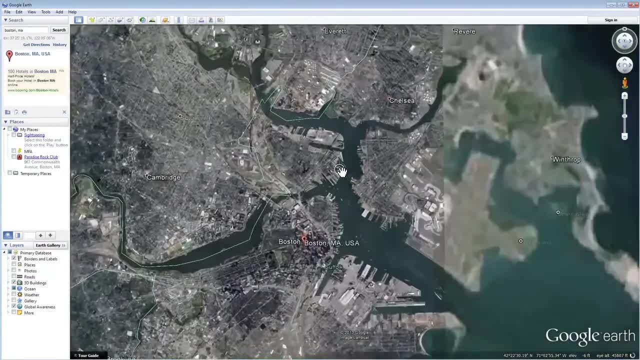 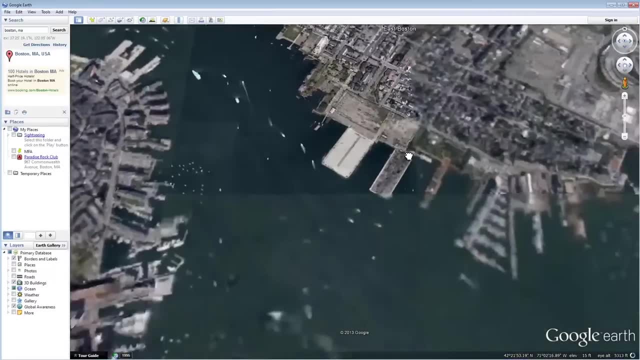 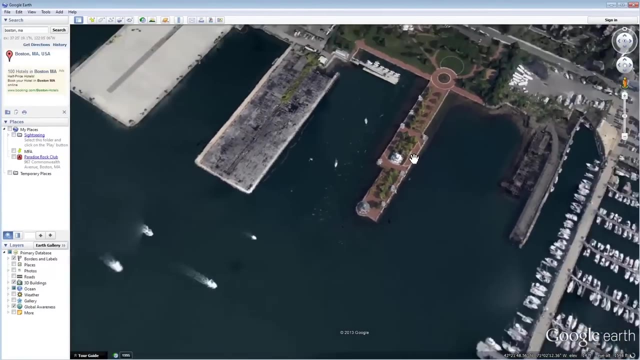 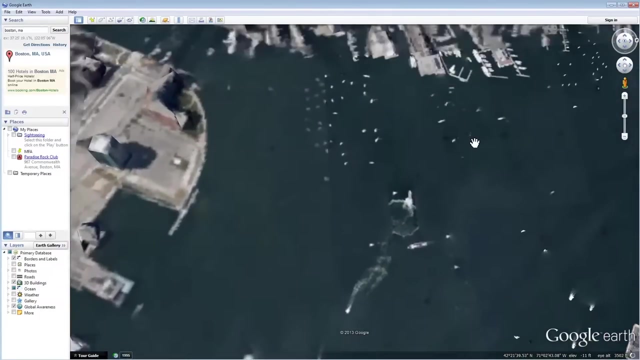 sun and I'll show you my favorite spot to see the Boston skyline. there it is. this is a wonderful little park called Piers Park, and it's just beautiful. so now that I'm zoomed in there, I'll rotate the whole map around as if I were standing at Piers Park. 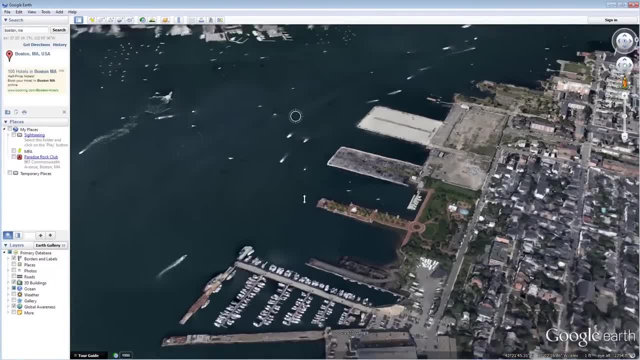 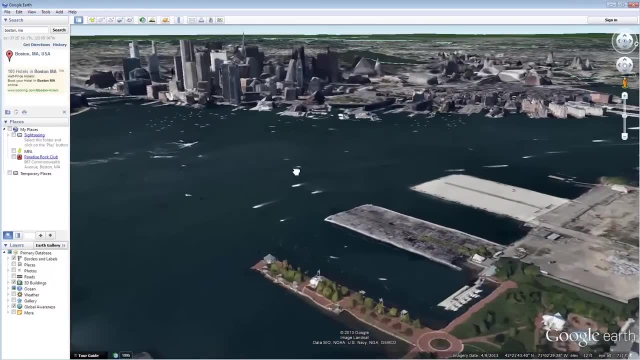 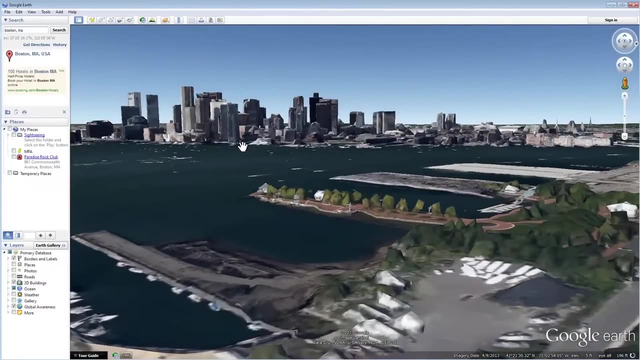 looking at the skyline- and I'm using the shift key now to pan down- and no, Boston hasn't melted. Google Earth is just trying frantically to download all this building data and render it on my poor, underpowered computer. alright, so here I am, right in Piers Park. 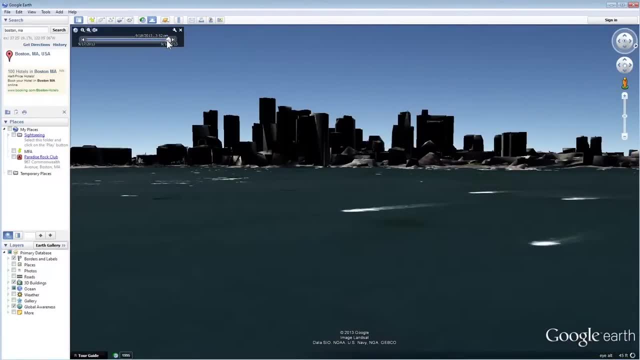 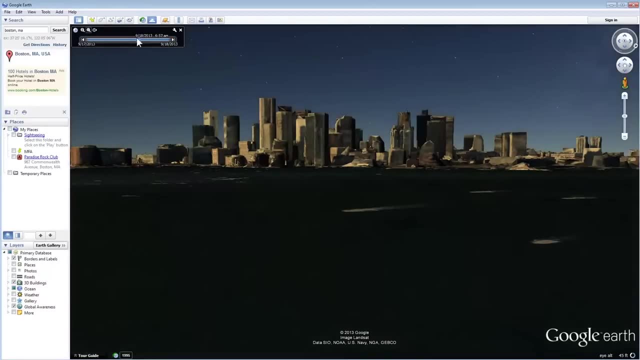 and I'll turn on the lighting effects and just look at the current day and, as we can see, as the sun rose from this view, we had really nice side lighting over here, illuminating these buildings as the sun rose, around 640, and then as the sun got a little. 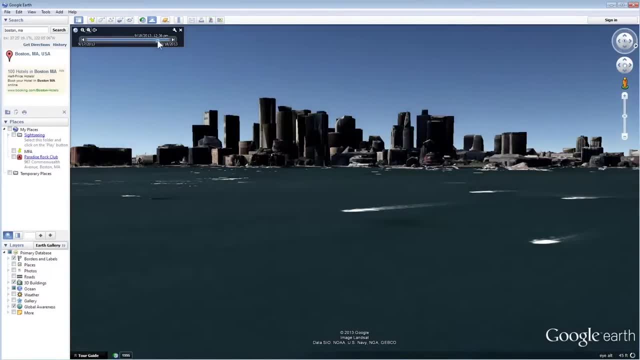 higher in the sky, the lighting got a little less interesting and then we can see the sun moving through the top of the sky there. and then you know we can see that- wow, really past noon, all these buildings are going to be completely in shadow. so you know if you're going to go shoot at this. 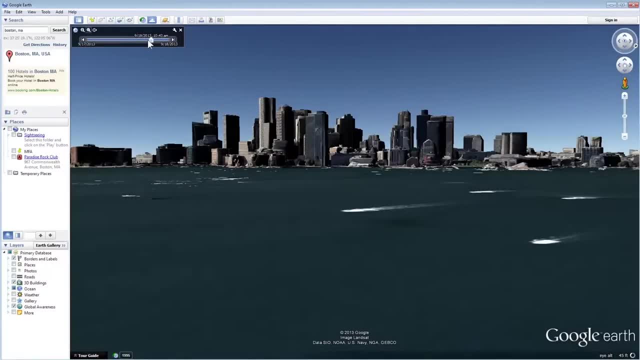 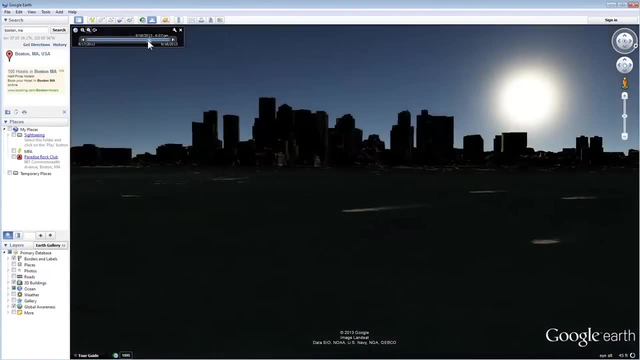 spot on this particular day of the year. well, you better get there in the morning, because in the evening it's completely gone and we can also see exactly where the sun is going to set. you can see that it sets off to the right there, and indeed, this is the exact same experience. 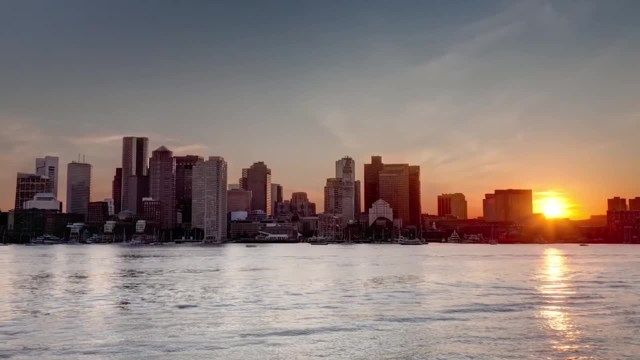 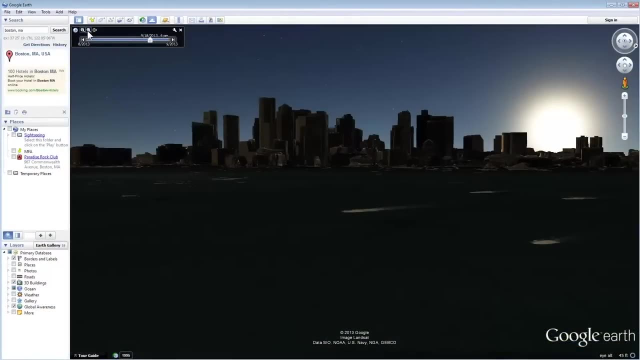 I had when I shot there recently. that is where the sun set now. I shot there a little bit earlier in the year so it was a little closer to the left, but let's zoom back on the timeline here and we'll see what it looks like in. 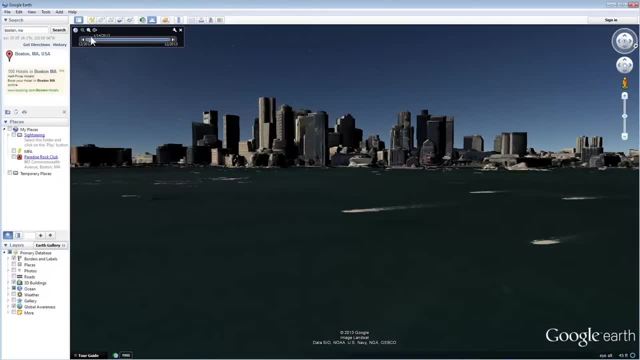 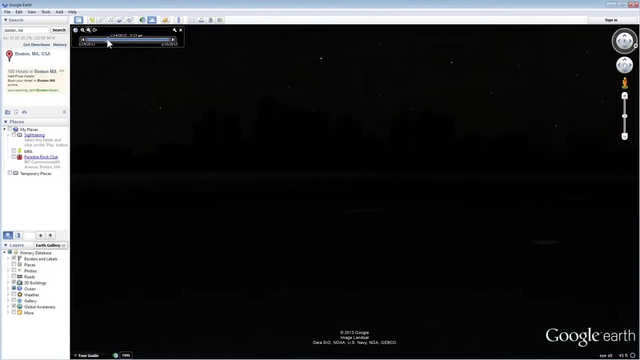 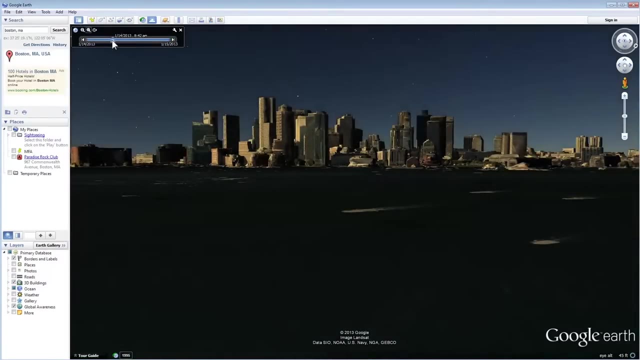 the winter. alright, so let's get right there in the winter solstice so we can see the sun rises. a little bit later now we don't see any light at all until about 750, and then those buildings really light up nicely. now I wonder where the sun is going. 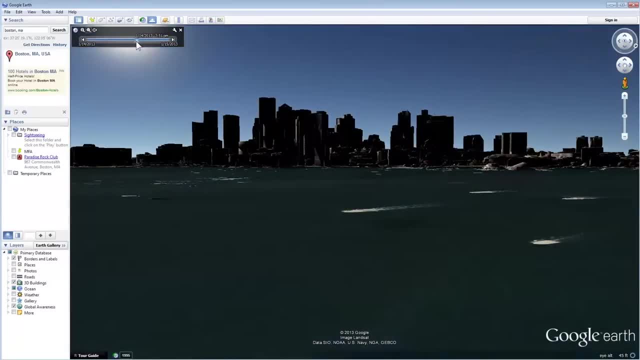 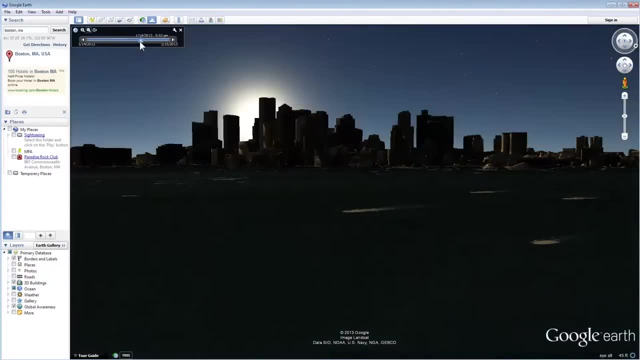 to set in the winter. I'm pretty confident it's not going to be in the same place. oh, here comes the setting sun. now you can see about 420. it's right behind the building, so look at that now. in the summer the sun sets way over here. 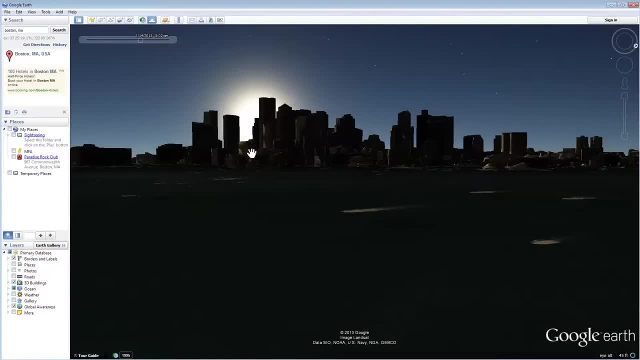 but in the winter you could get a shot of the Boston skyline from Pierce Park with the sun right behind it, and that could make for a really interesting picture. so you can see, if you're planning the perfect cityscape of Boston, then it's going to be really. 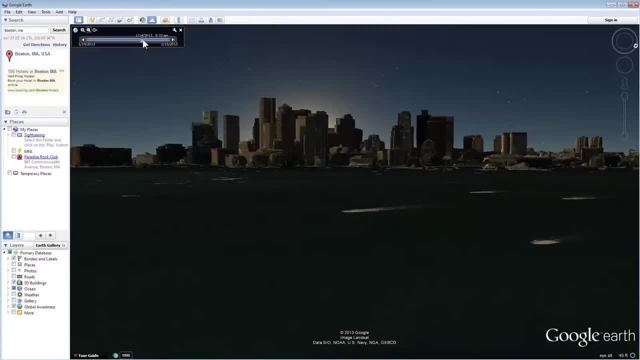 important not just to plan the time of day and, of course, the weather, but also to figure out what time of year you need to be at that spot, because, well, there might be a better spot than Pierce Park, maybe something off to the left here, if you were in the summer. 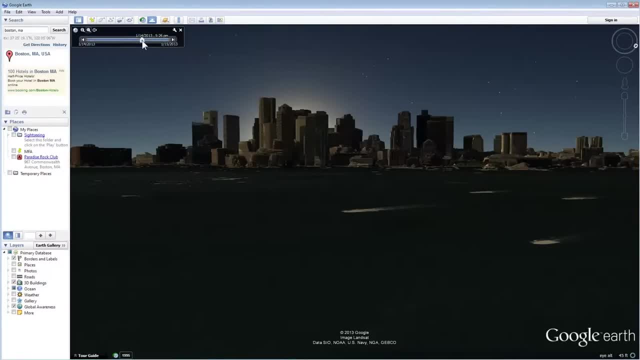 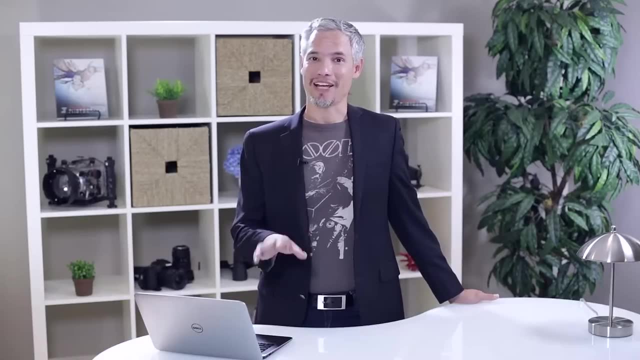 but Pierce Park would be just perfect for the setting sun in the winter. I really love Google Earth. it's such a powerful tool. let's talk about another way that you can control light, and that's by using flash. flash is a really convenient way to control lighting. 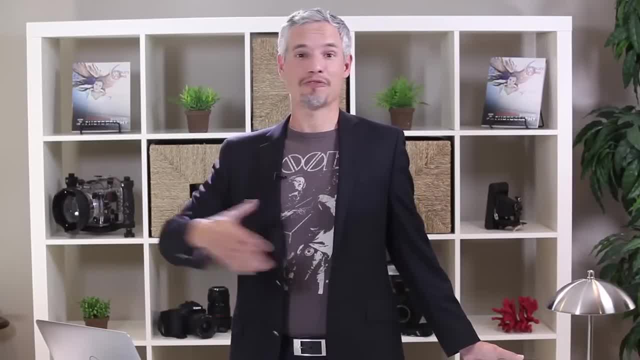 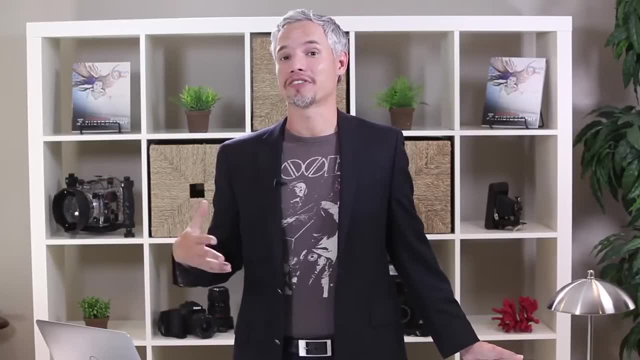 a lot of cameras have a flash built right into them and you can turn it on and get front lighting, no matter where you are. now, flash on camera is usually intended to just kind of fix lighting problems if there's just not enough light to take a picture of somebody. 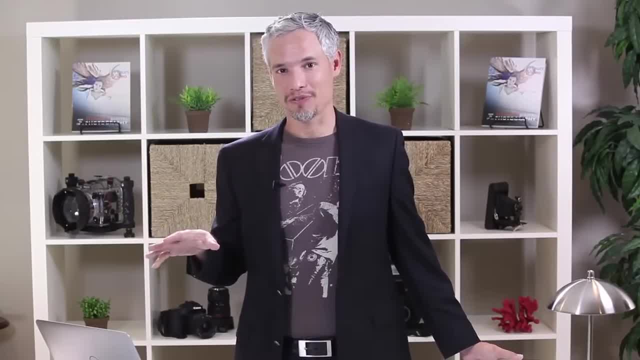 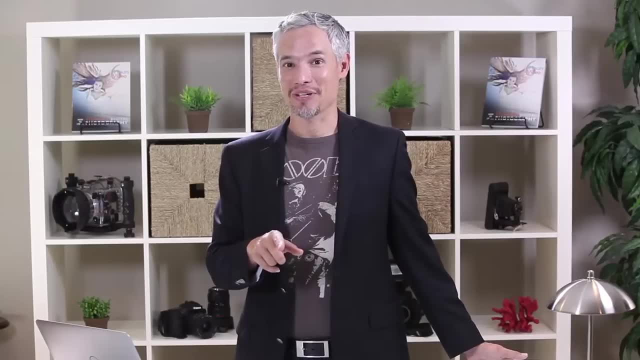 you turn on a little pop up flash and it illuminates your subject for you. however, you can also use flash in ways that aren't terrible, and that's by attaching an external flash to a camera and then controlling the head. so let's look at some examples. here's a photo of 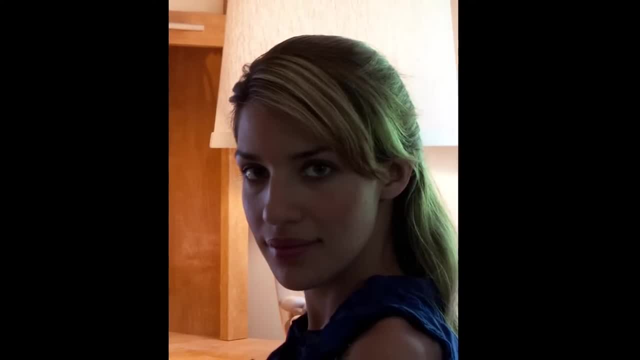 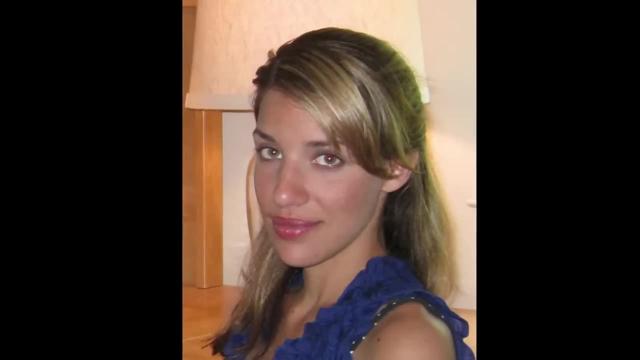 Chelsea indoors with absolutely no flash and you can see, in this particular setting she was completely backlit, which meant her face was in shadow and therefore underexposed. here I just turned on the on camera flash and, as you can see, it created some pretty awful red eye. 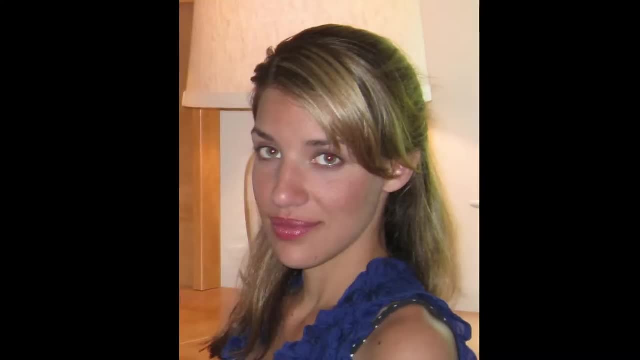 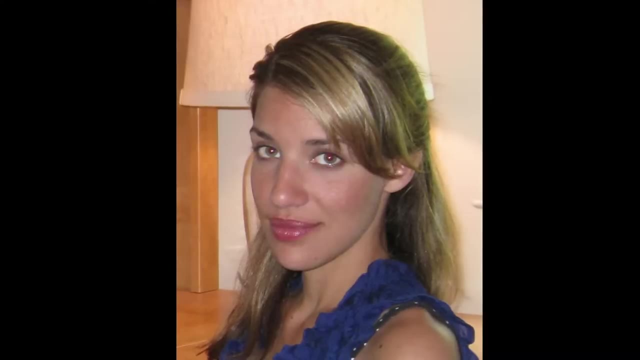 now you can fix that with software and some cameras will even fix the red eye automatically. but either way it's never going to be flattering light because it's so close to the camera itself, it creates these like really hard shadows. now I'll show you what an external flash looks like. 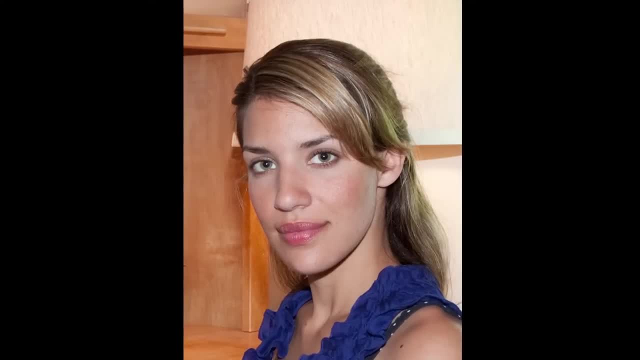 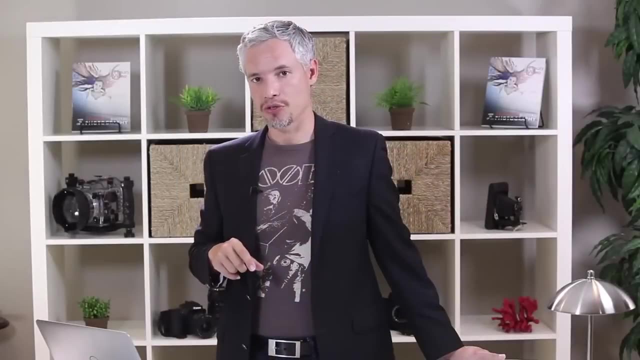 as you can see, it's still hard and direct light. after all, it's just mounted to the top of a camera. however, these shadows are a little less distinct. they go down a little bit farther, and just moving it that extra inch or two off the camera made a big difference. 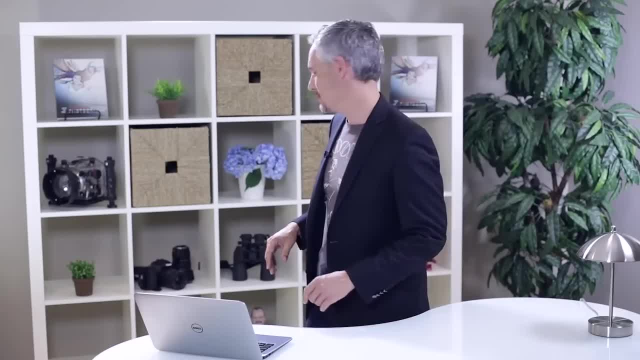 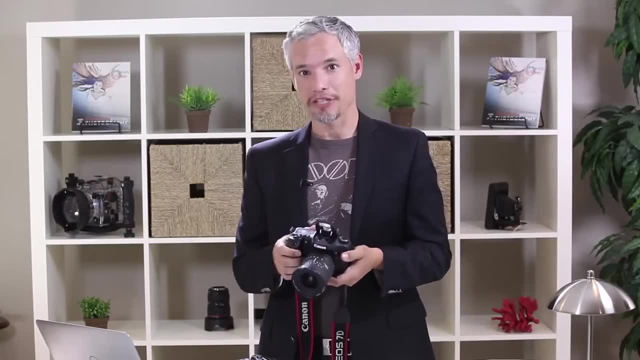 let me grab a couple of cameras from behind me and I'll show you what they do. so this Canon 7D has an on camera flash and I just turn it on by hitting the flash button here and it will create pretty awful pictures. it's always going to create this. 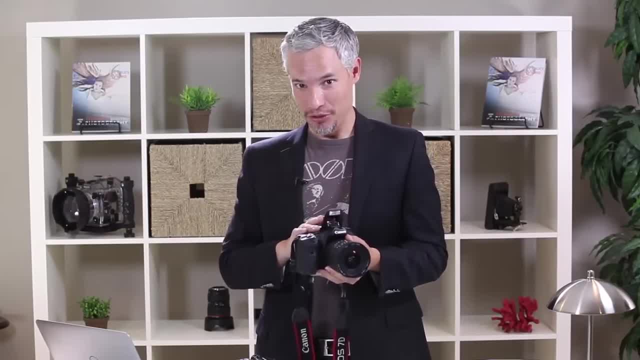 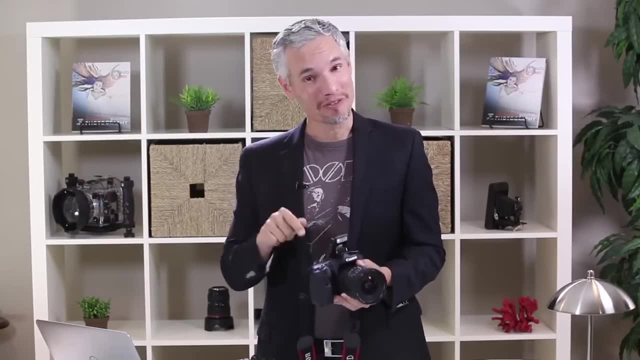 really direct light and I never, ever use this. and in fact, when you look at the pro level cameras, you'll see that they don't even have a built in flash. that's right. you pay way more for the camera and they give you less. they don't give you that pop up flash. 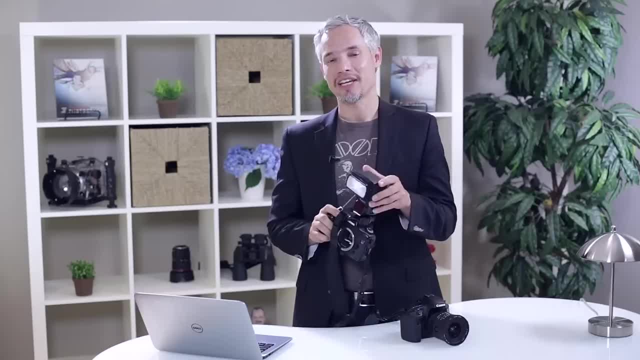 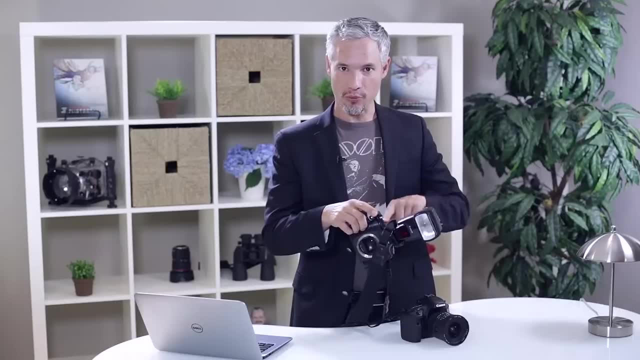 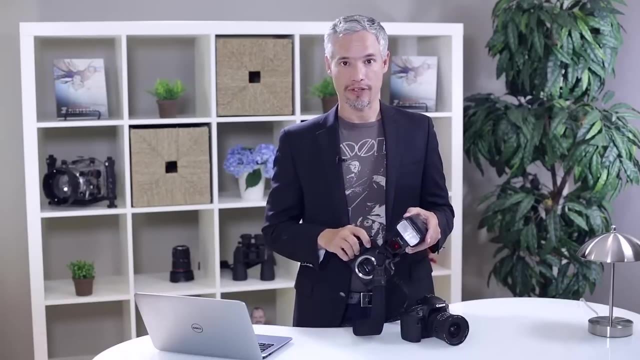 you know why cause? every single pro hates them. now. this external flash has a lot of great features now. first and foremost, most importantly, it simply moves the light farther away from the lens. this extra just couple of inches here makes all the difference in the world, but it also adds a lot more powerful capabilities. 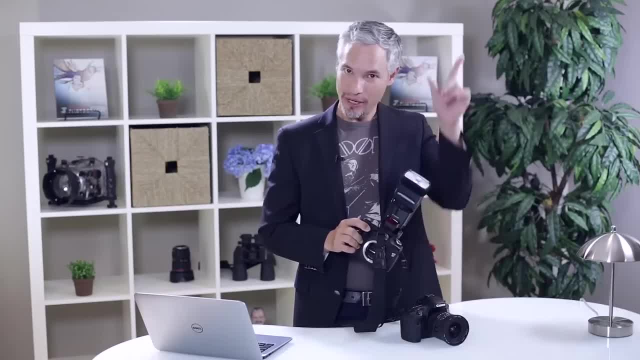 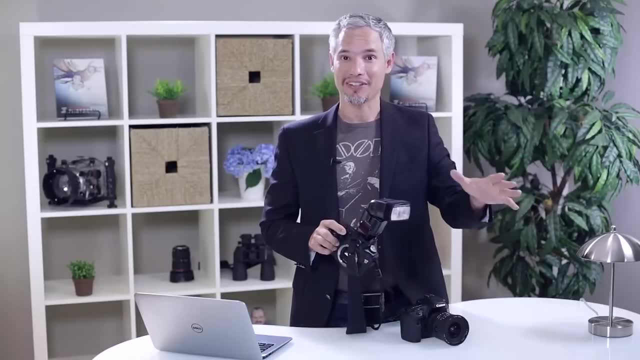 for example, I can rotate the head up like this and then bounce the flash off the ceiling. I can also turn it to the side and bounce the flash off. over here I'm controlling the light, and when you learn to control the light, you'll never want to go. 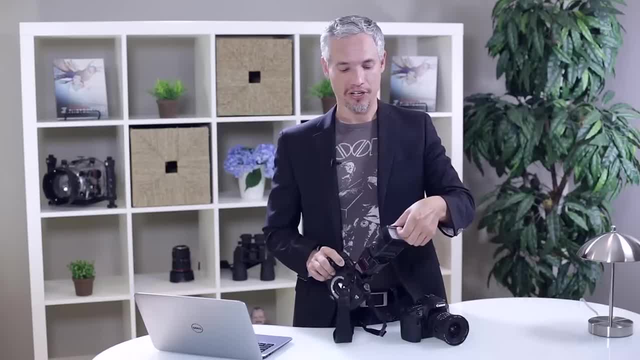 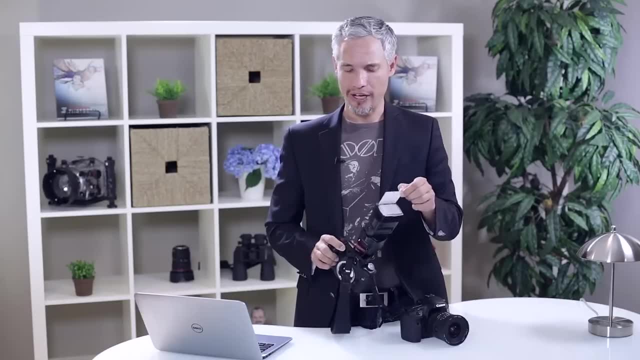 back. this particular flash- and most higher end flashes- also has a built in diffuser that spreads the light around more, creating a softer bounce flash and a little white card here that will reflect the light forward. now let's talk about using fill flash. when you use fill flash, 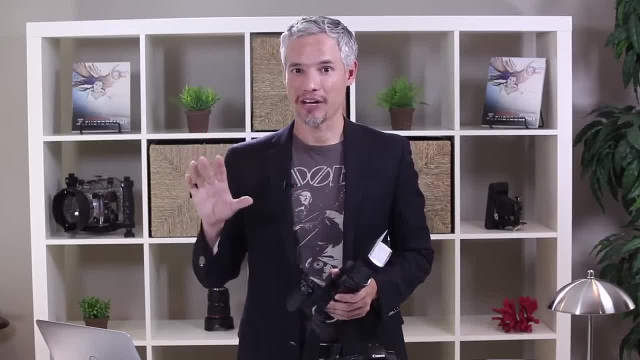 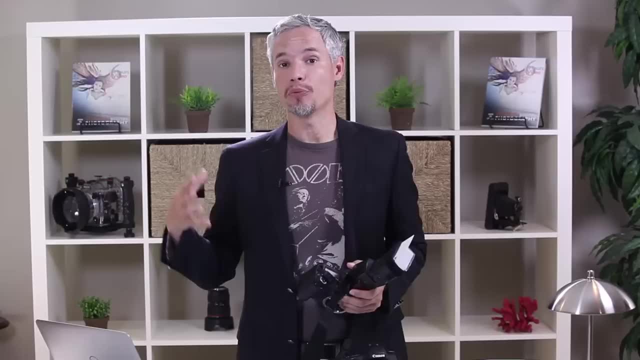 you're using your flash to just add light and fill in shadows, it's not becoming the main light in any given picture. there's always a main light and that is the brightest light source that's illuminating the subject. if you're outdoors, that's almost always the sun. 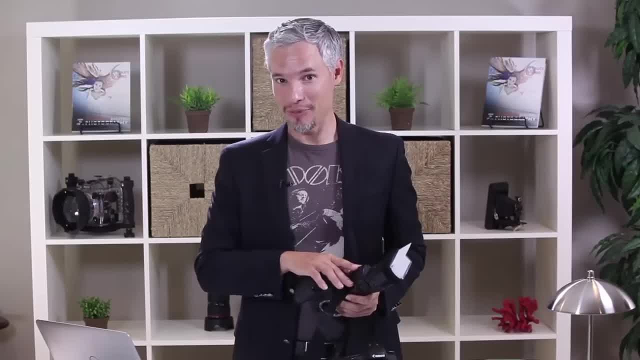 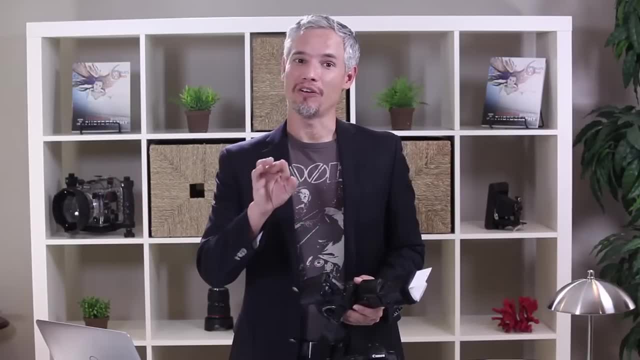 and if you just turn on your flash and fully automatic mode, it's probably going to be your flash. your flash is going to provide enough light to completely illuminate the subject. but if you put your camera in one of the creative modes- aperture priority mode, shutter priority mode- 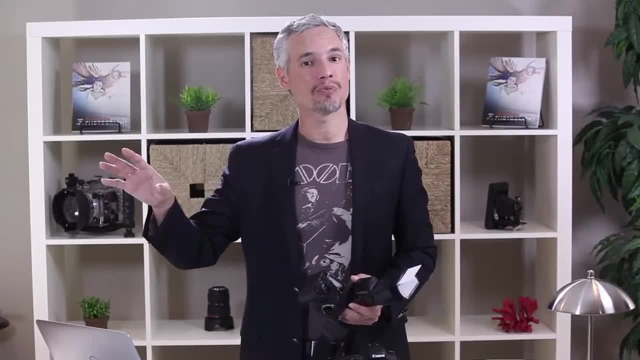 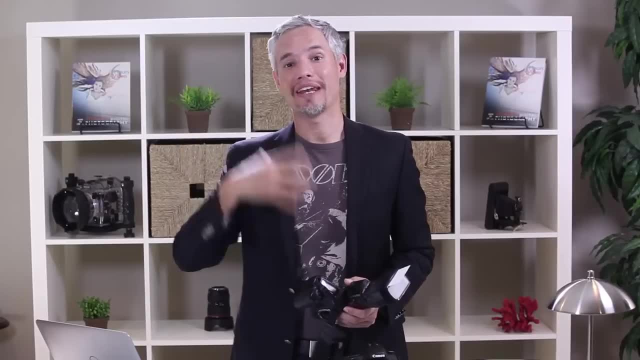 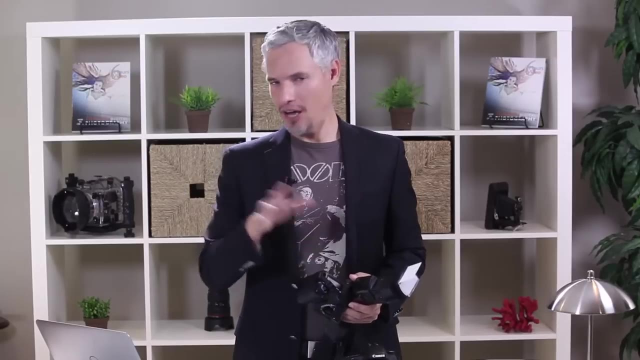 or manual mode, your camera will automatically expose the picture properly without using the flash, and then it will add just a touch of flash to create a flattering light on your subject and fill in some shadows. you can use flash exposure compensation to dial up or down the amount of flash that it adds. 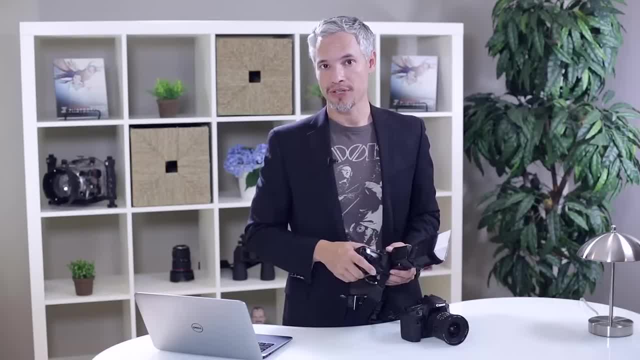 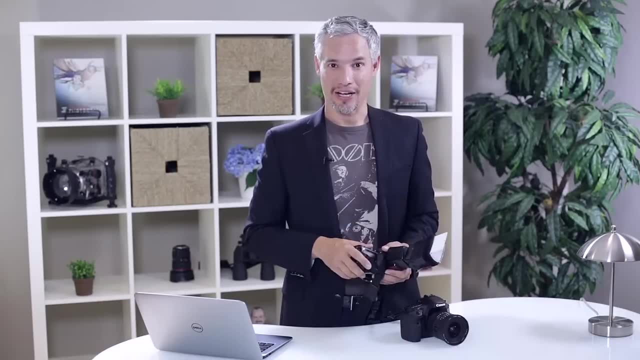 so what i suggest doing for portraits, especially outdoor portraits, is putting your camera into aperture priority mode, selecting the lowest f-stop number possible and then turning on your external flash. if you're outdoors, you should have it pointed directly at the subject. if you're indoors, go ahead and 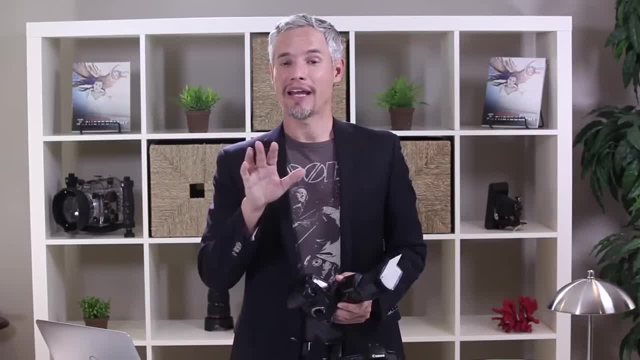 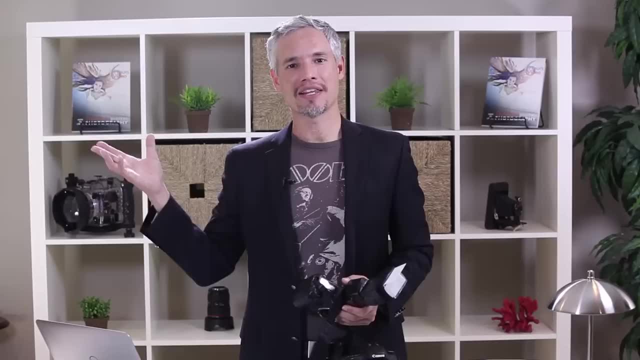 point it at the ceiling and use bounce flash now because we're in aperture priority mode, the flash isn't going to try to be the main light. the main light is going to be whatever your ambient light is- the sunlight or anything else. instead, the flash is just going to try to fill in the 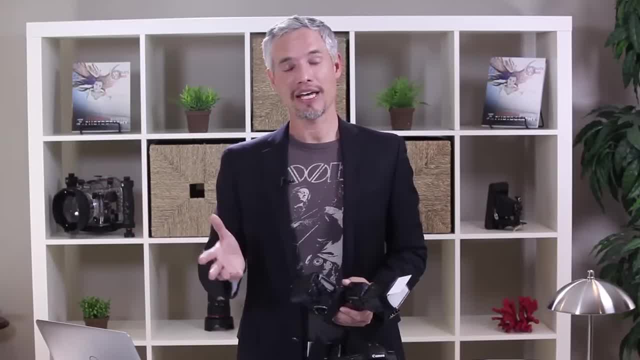 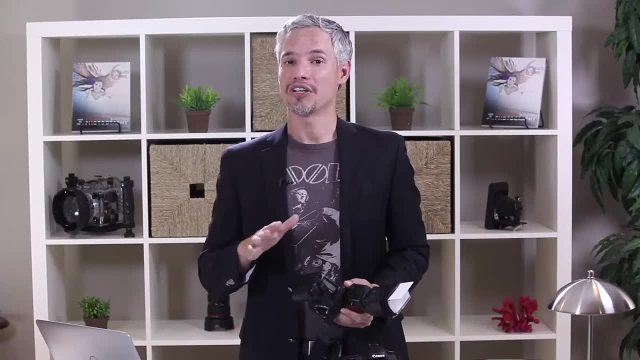 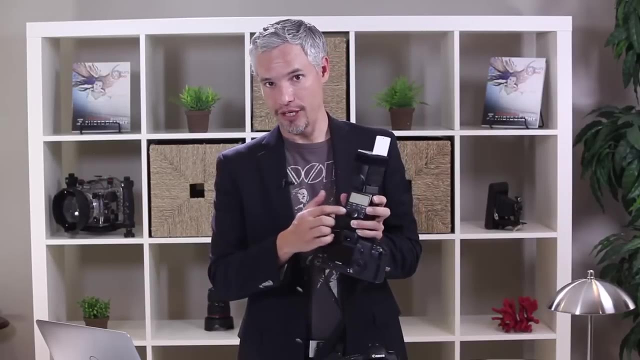 shadows a little bit. now just take a sample picture and look at it. look at the histogram. how does it look? is the flash too much? is it overpowering? if so, then adjust the flash exposure compensation on your camera. sometimes the flash exposure compensation is controllable by the buttons on the 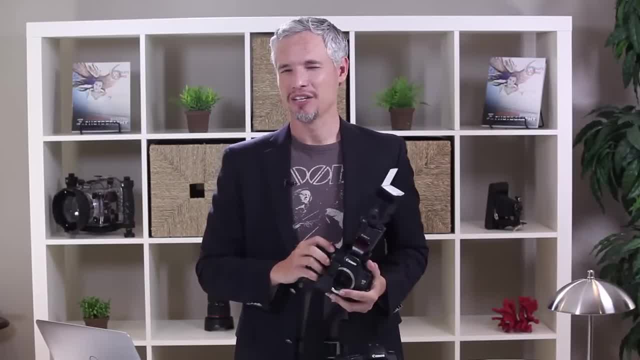 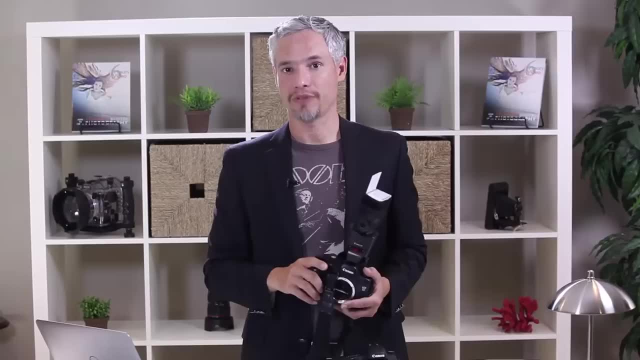 back of the camera and other times you need to press a special button. usually it looks like a little thunderbolt with like a plus and minus sign next to it, but check your camera's manual to learn how to control the flash exposure compensation. unfortunately, i can't tell you specifically. 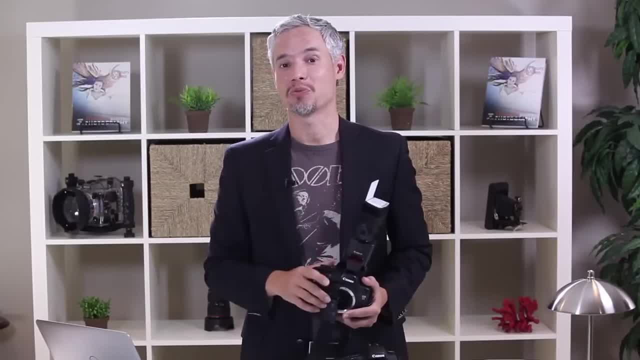 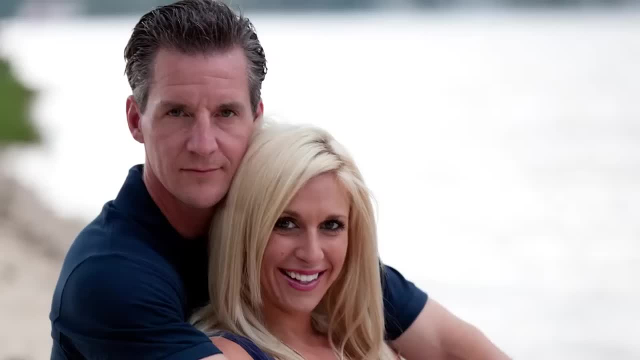 because it's different for every camera, but learning to use what they call the fec makes you a much more powerful photographer. now let's look at some examples of fill flash. here's an outdoor portrait that i took on a completely overcast day, so you can see. 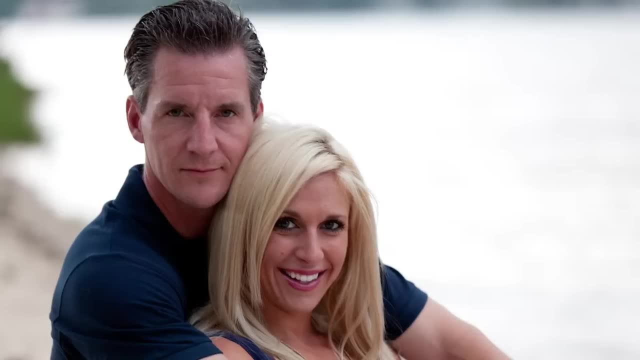 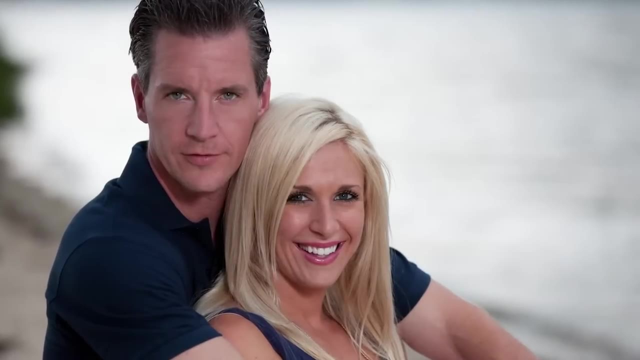 the lighting is soft, but it's top lighting, which means that their eyes are in shadow. they have a little bit of that raccoon eye, even though it's not too bad. here's what it looks like with fill flash and i think it looks much, much better. you can see that their 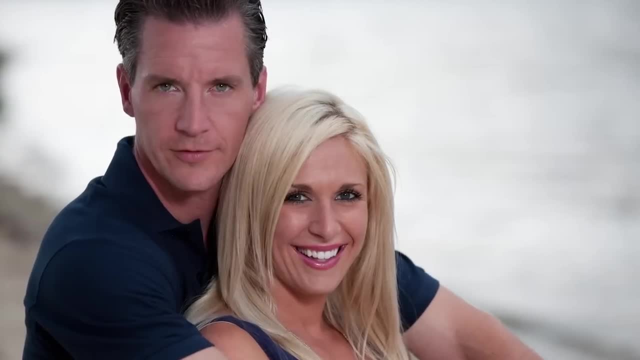 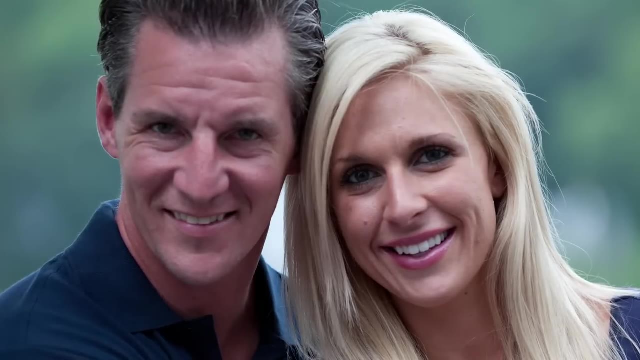 faces now have that hard light that is required to show detail. here's another snapshot of the same models, and again you can see their faces are in shadow because, even though it's a diffused light and the whole sky is lit up well, their brows are casting a shadow on their faces. so i 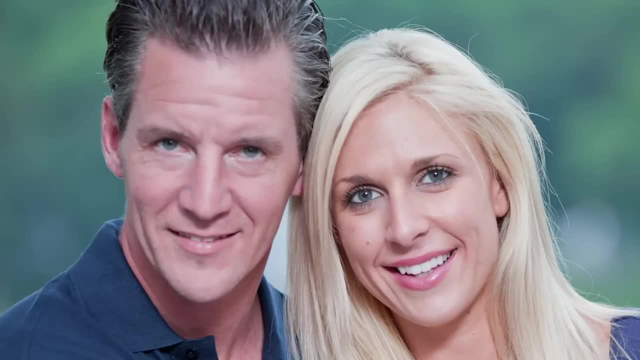 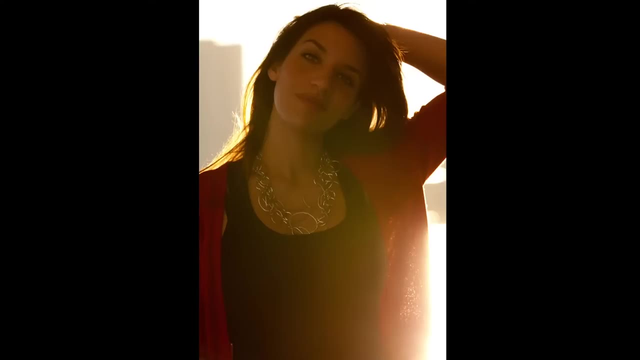 added a little bit of fill flash and you can see it changed the picture completely. here's a heavily backlit picture of chelsea in boston and you can see her whole body is in shadow. but turning on the fill flash changes the picture entirely. now the fill flash balances. 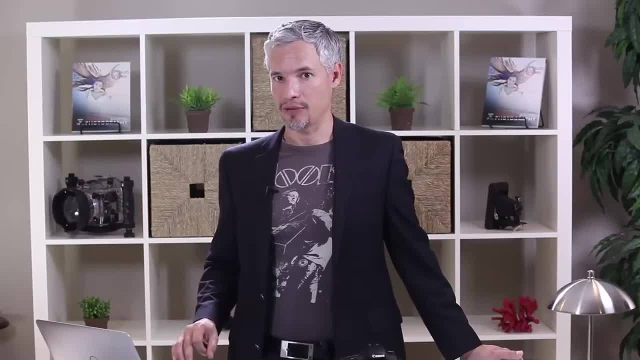 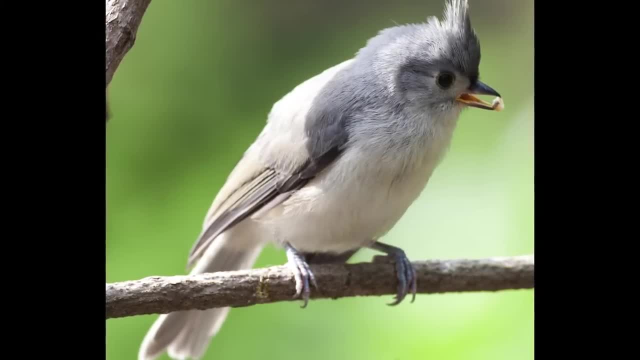 the backlighting and really brings out the color and detail in the subject. here's a tufted titmouse with no fill flash. as you can see, its face and eye are in shadow and with wildlife shots, the eye, and specifically a catch light, is really, really important. 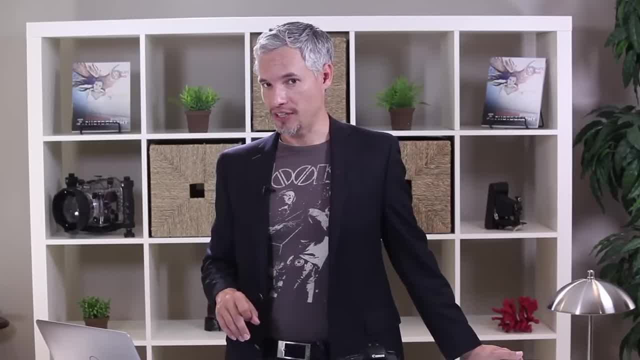 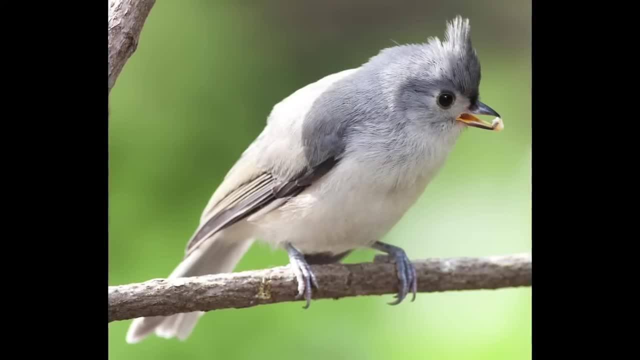 so because i knew the bird wasn't ever going to move into the sunlight for me, i turned on a little fill flash and there you can see it adds a nice and distinct catch light to the bird. i'll cover more of that in the next lesson that covers wildlife photography. 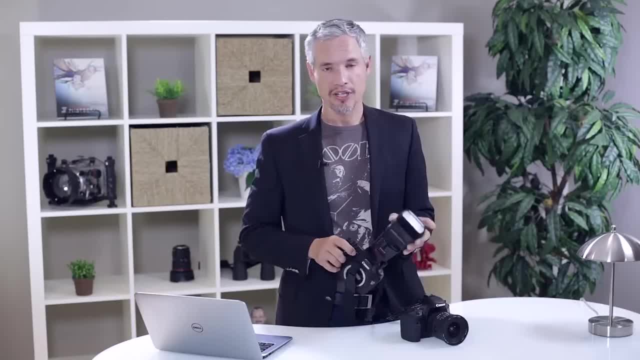 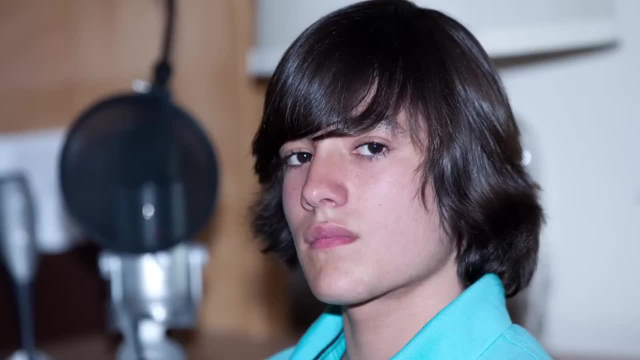 now let's look at some examples of different flash directions. first is just direct flash and of course this creates hard front lighting. as you can see from this photo, the model my producer, tyler, has a very distinct line under his shadow and a very bright catch light in his eye. 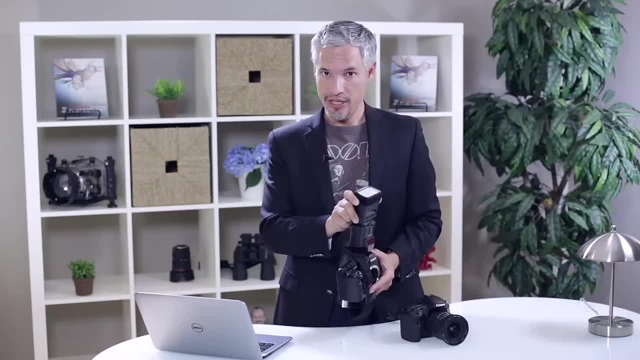 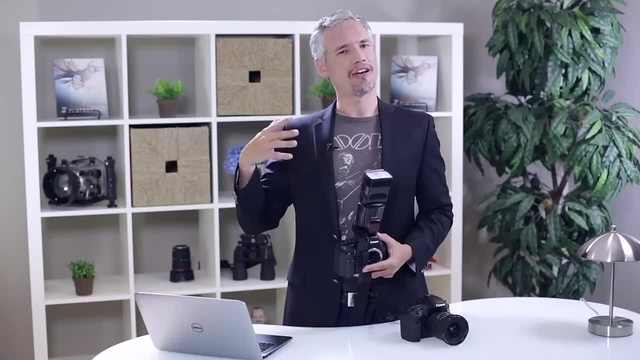 all i need to do is to move the flash head into the upward position and i'll be bouncing the light off of the ceiling. now you have to kind of check out the ceiling of the room that you're in. ideally you'd have white ceilings if you're. 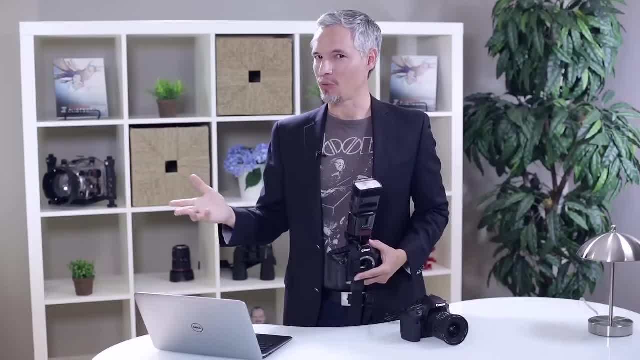 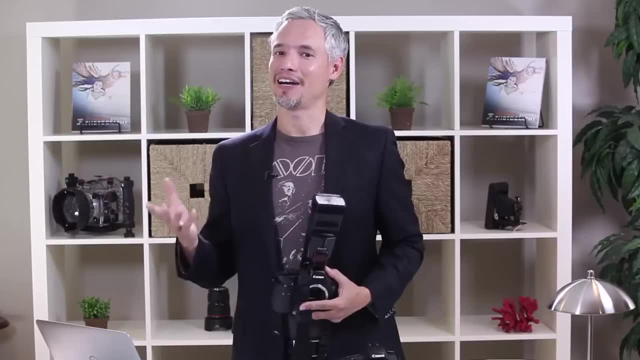 in a room with really high ceilings or if you're outdoors, it might not work at all. for example, if you had red ceilings, well all the light bouncing back from your flash is going to be red. then it's going to be causing an odd color cast on your subject. 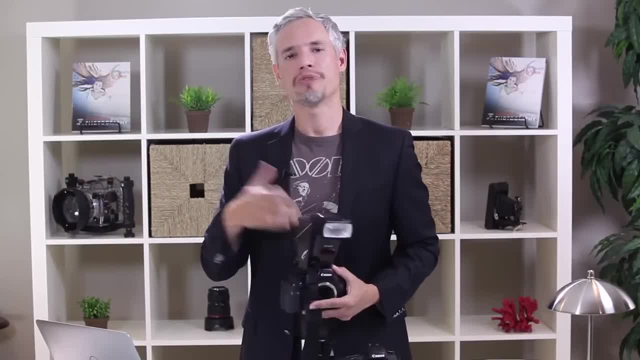 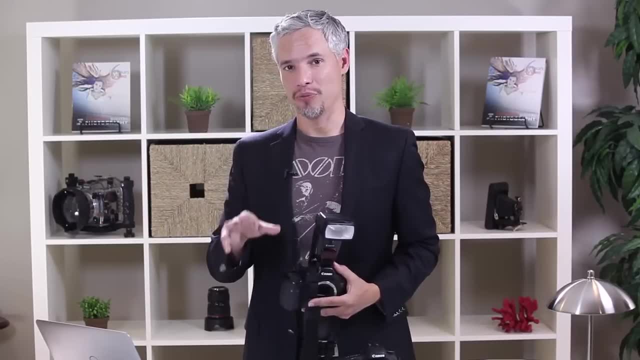 that wouldn't happen if you used direct flash. so these are things that you just need to think about and experiment with. obviously, i can't give you one rule, because it depends entirely on the room that you're in, so let's look at a sample photo of tyler. 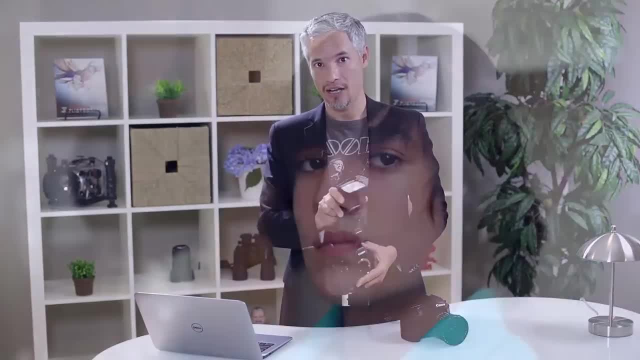 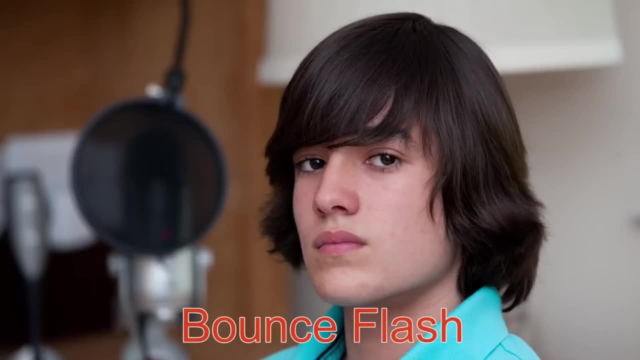 being bounced directly off the ceiling with the flash in the upward position. as you can see, this creates a much softer shadow because, in essence, the entire ceiling is becoming a huge soft box, one big light source, and big light sources create soft light. therefore, the shadow underneath his chin is much softer. 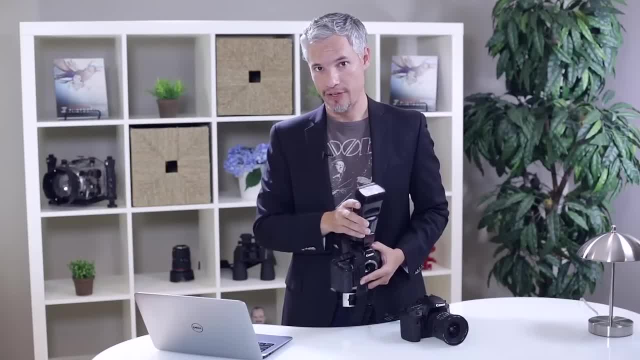 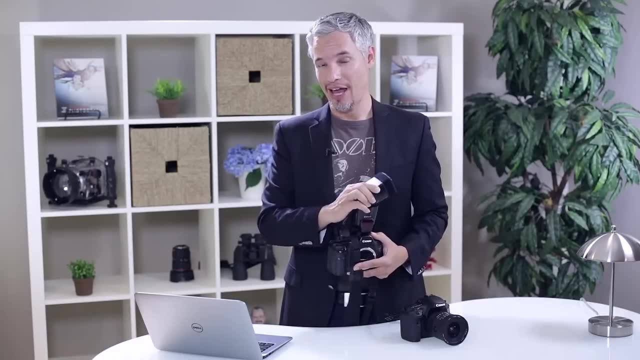 now you're stuck with front lighting or top lighting. when you work with a bounce flash, you can also have it move to the left or the right. so let's look at what happens when i turn that flash head to the left and bounce it off the left wall and ceiling. here we can. 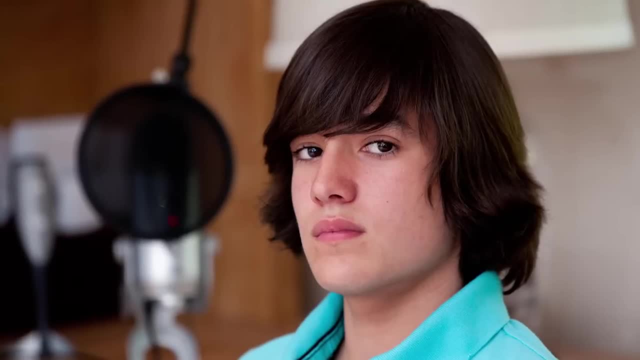 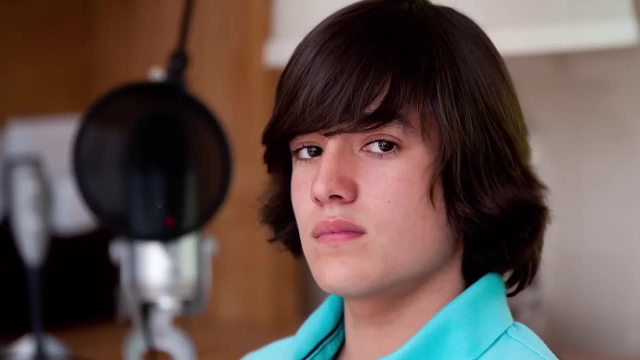 still see a shadow underneath his chin, but because it's coming from the far side of the subject, it's creating what's called narrow lighting. that means that the light is coming from the far side of the subject's face, and this side is brighter than this side, so let's move that flash. 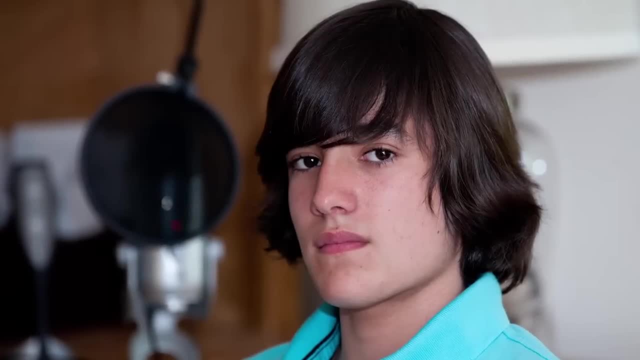 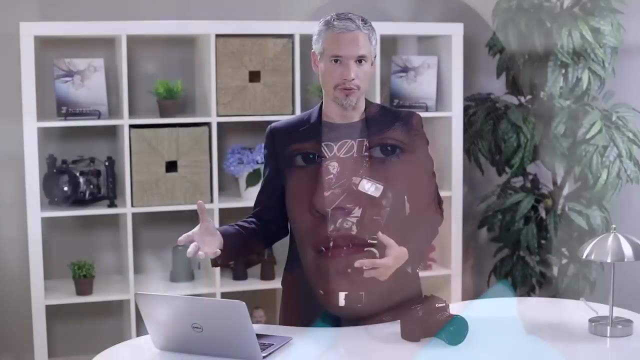 around over to camera. right here we see broad lighting. the flash is striking the closest side of the subject's face and bouncing off the right side of the wall. again, you just kind of have to assess the room that you're in to determine how the flash is going to. 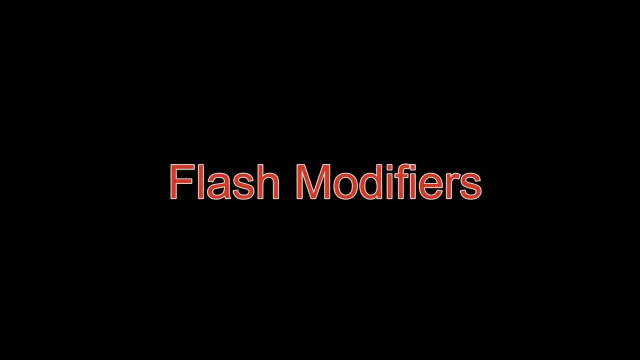 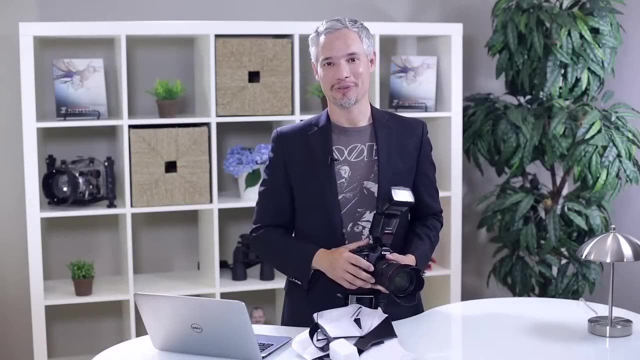 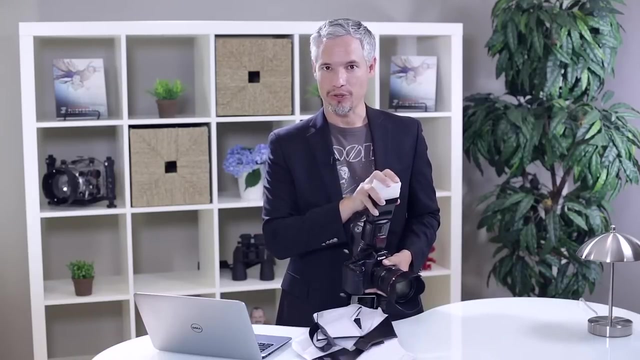 affect it. so now let's talk about a couple of different flash modifiers. you can attach devices to your flash to modify the light and completely change the light characteristics. so my favorite is the very compact diffuser here and it just pops right onto the flash. make sure you buy one that's compatible with your specific. 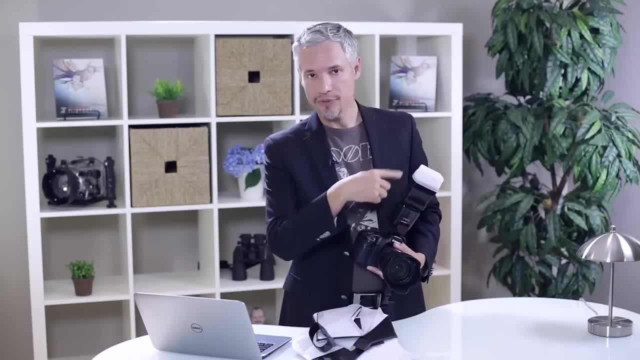 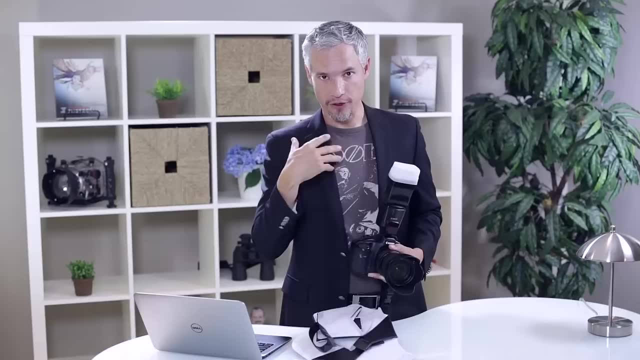 model of flash, though, and what it does is, when the light comes out of the flash, well, it's going to kind of scatter that light everywhere. so some of the light is going to go straight forward and create some front lighting and a nice catch light in the subject's eyes, but then again a 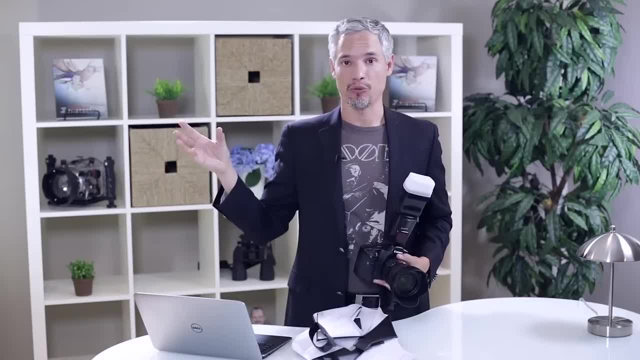 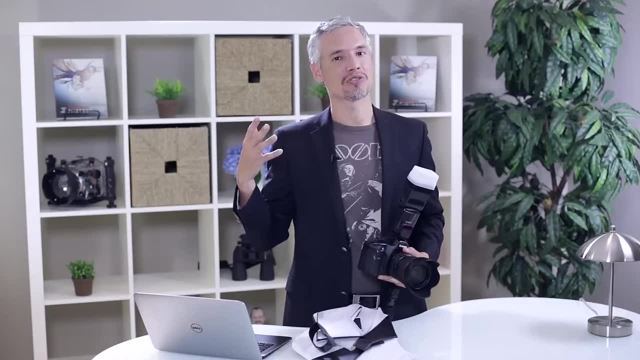 bunch of it's going to bounce up and behind and it's going to be scattered around the room, creating this soft light. so you have a nice combination of hard direct light and diffuse light, which is just great for portraits. if i had to have just one implement. 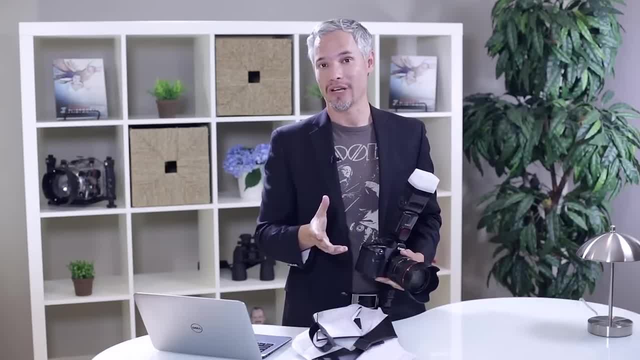 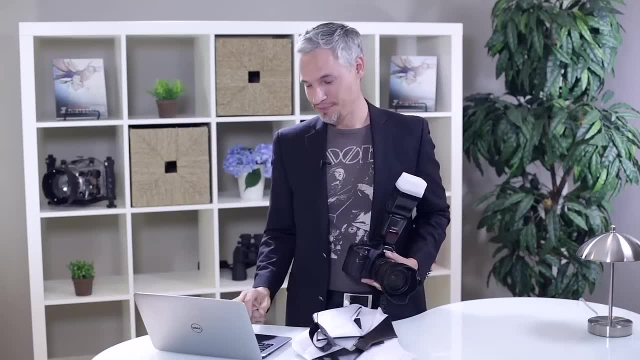 on my flash, it would be this. of course, it's primarily for indoor photography, because so much of it is being bounced around. if you're outdoors, well, it would just be going off into space, right? let's look at a sample photo. here we see tyler photo. 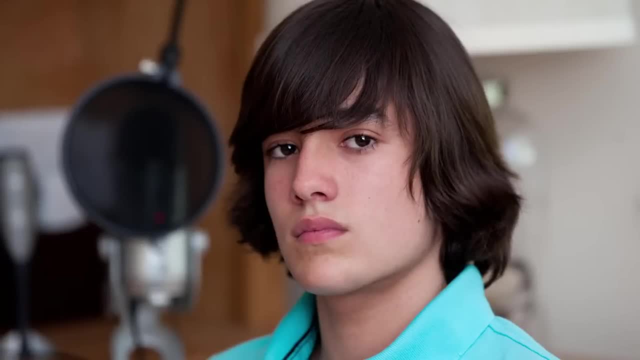 graphed with the diffuser. and again we see those characteristics. we see the nice catch- light in the eyes and plenty of direct light- but we also see that soft light created by having the light bouncing all over the room. now i'll move on to a small soft box, so 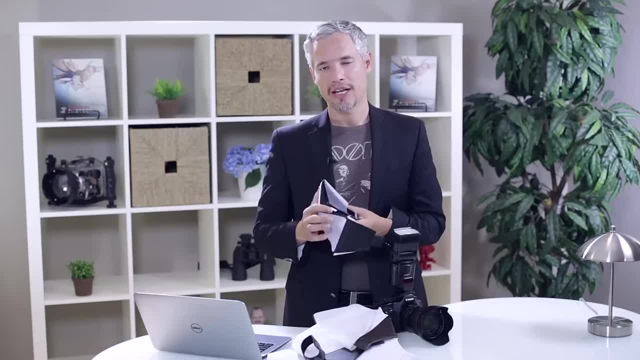 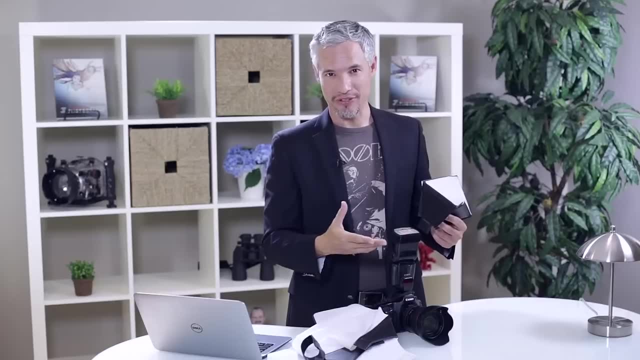 i'll take that off and attach a small soft box. now these devices attach in a couple of different ways, but usually it involves some velcro attached to your flash, and i don't know why they don't come up with some snap on system that works with every different flash, but they don't. 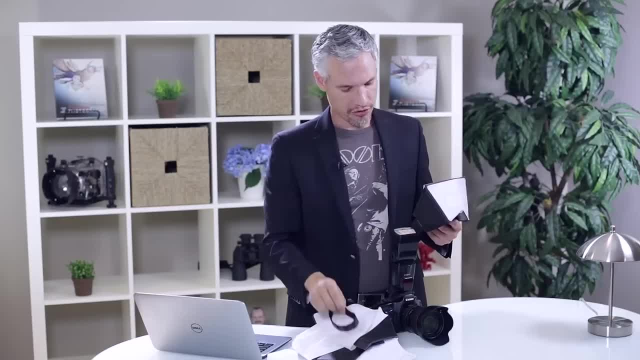 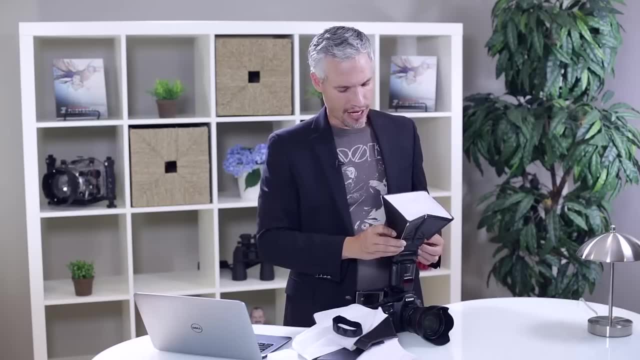 so you end up like putting this sticky velcro on here or using a strap like this to get it attached, but these soft boxes all work in basically the same way, even though there are lots of different models. i have a lumiquest promax soft box, but i'm not. 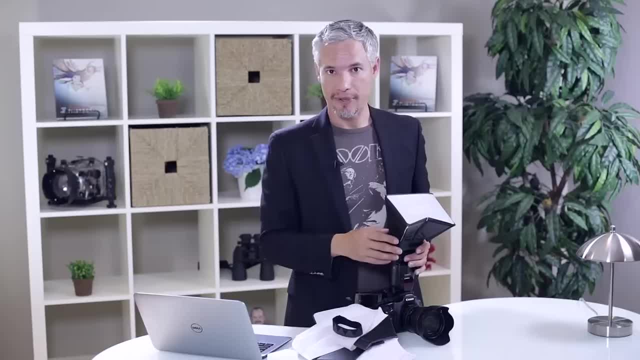 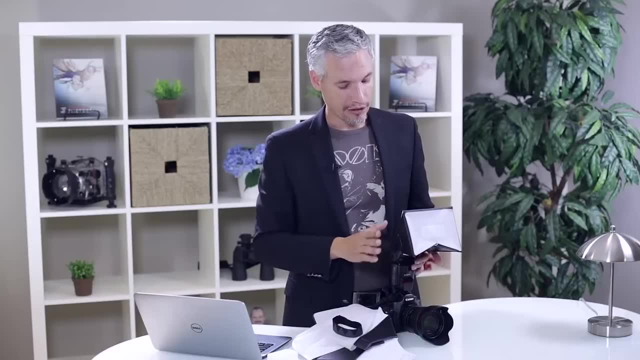 endorsing it. it's fine, it does the job. there are lots of other soft boxes out there that will do exactly the same thing. i mean, basically, it's just a slightly translucent piece of plastic that scatters some of the light. now, you don't typically use this with a. 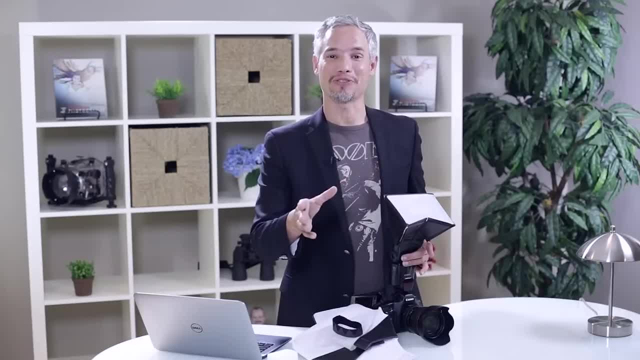 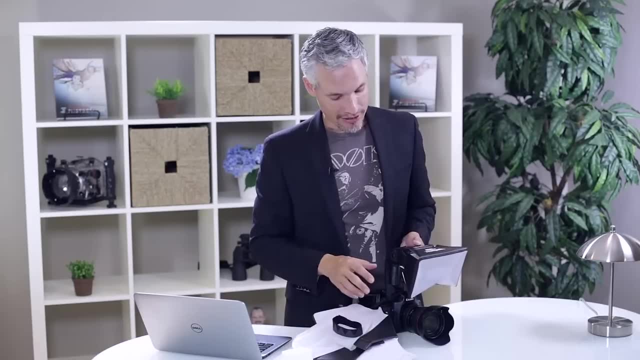 bounce flash. in fact, you wouldn't use this. if you could use a bounce flash, you would just bounce the flash or use a little diffuser like this. use these outdoors or in rooms with high ceilings, because they allow you to go back to using direct flash. all your light is still pointed forward. 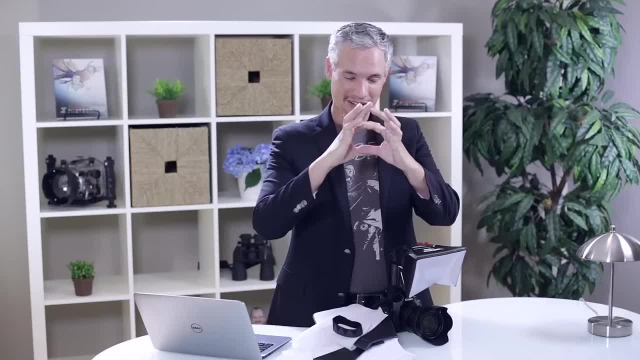 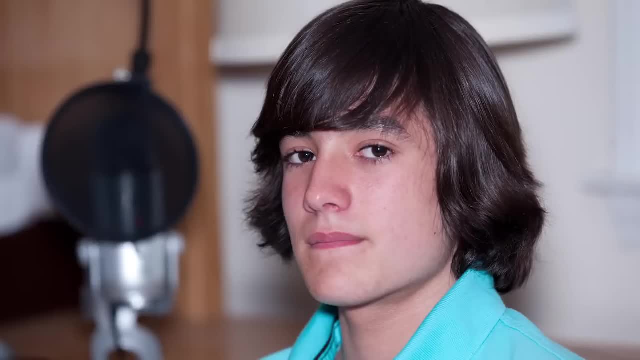 but now, instead of having a light source the size of the flash head, you have a light source the size of the whole soft box. so let's look at a sample photo here. we can see tyler direct lit by the small soft box and it creates a much. 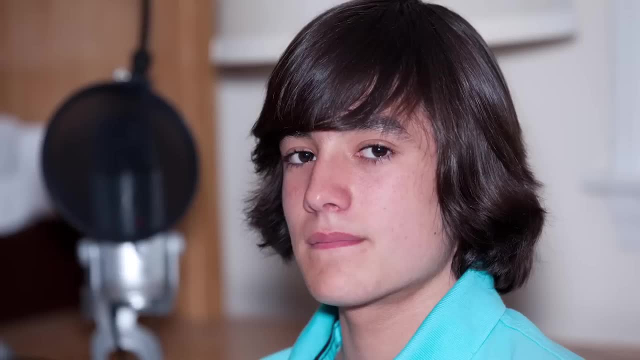 more flattering light than the direct flash did. now it's not as nice as the bounce flash or the diffuser, in my opinion, but again, use the small soft box when you can't use those things when you're outdoors or when bounce flash is otherwise unusable. so now i'll show you the. 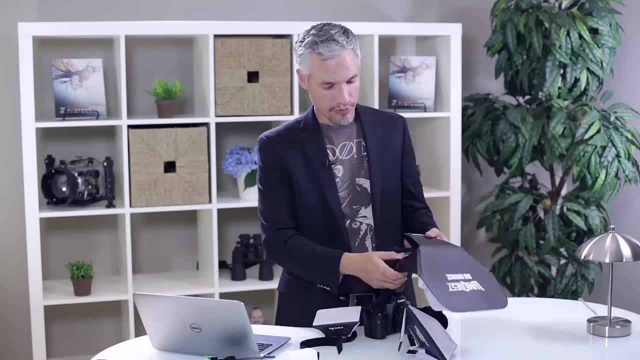 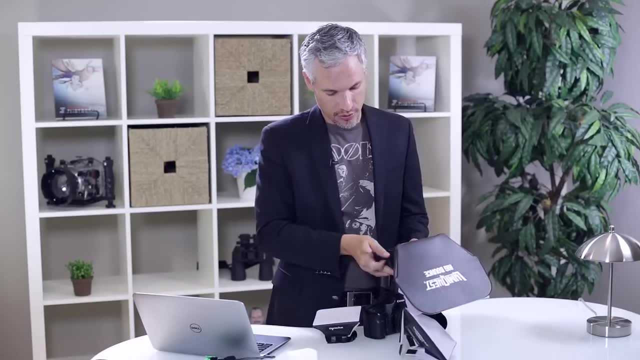 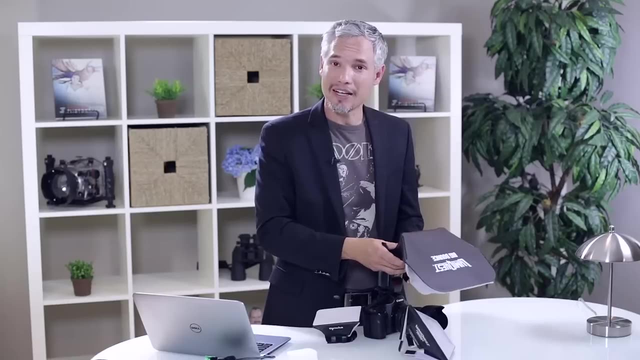 large soft box. the large soft box is much more cumbersome than the small soft box and, besides attaching with velcro, it typically has an additional strap like this that's going to go around the flash and, as you can see, it doesn't go on all that easy. and then when it is on, you know. 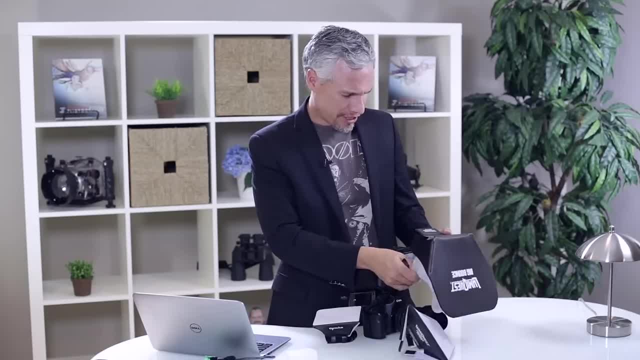 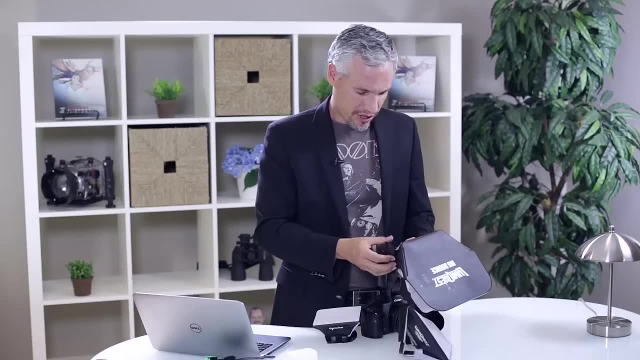 what? it's not all that stable because it's big and floppy and the flash really wasn't meant to hold it. so my clumsiness here kind of illustrates a point. these large soft boxes get to be pretty cumbersome and in fact sometimes they end up flopping off when you 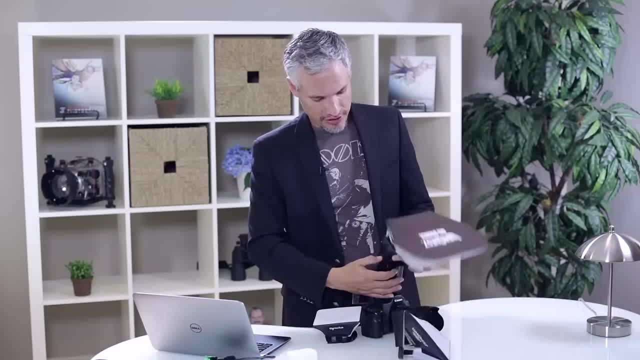 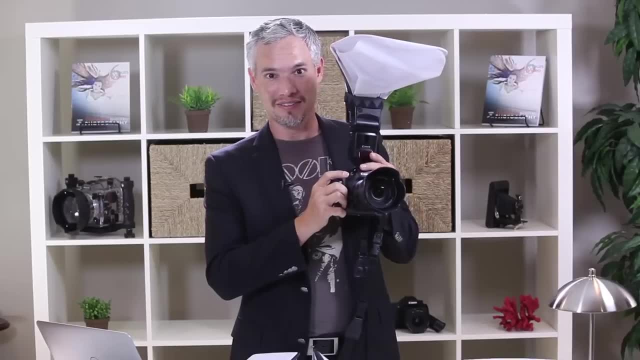 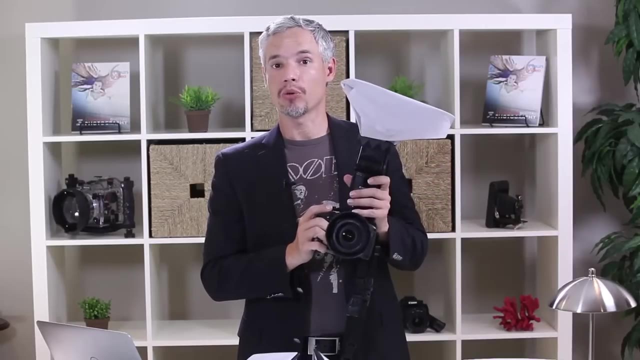 need them the most, which is a real problem. but all right, there we go. once it's attached, you can elevate this and the flash fires directly forward. so i'll demonstrate that now and, as i mentioned earlier, the larger the light source, the softer it's going to be. so if you're outdoors and you need 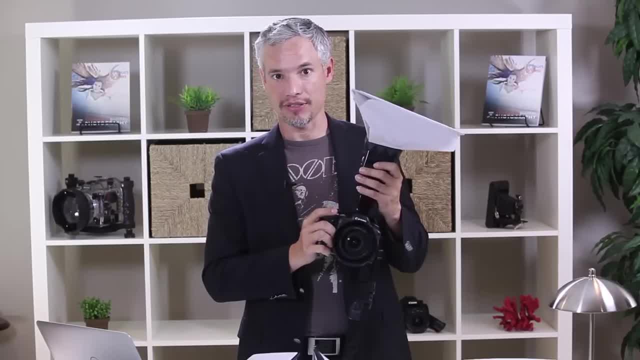 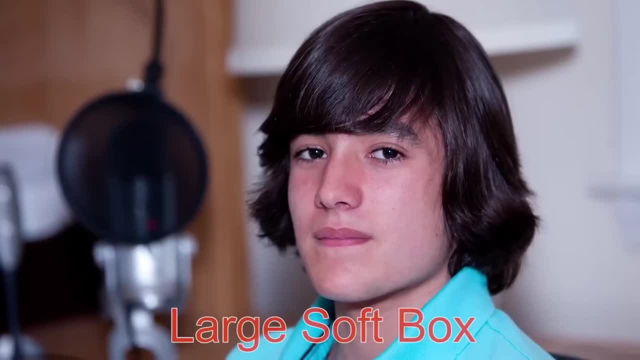 the softest light possible. attach a large soft box like this. let's look at a picture to show you what that'll look like. as you can see, the line under his chin is much softer and in fact the catch light in his eye is higher because the large soft box. 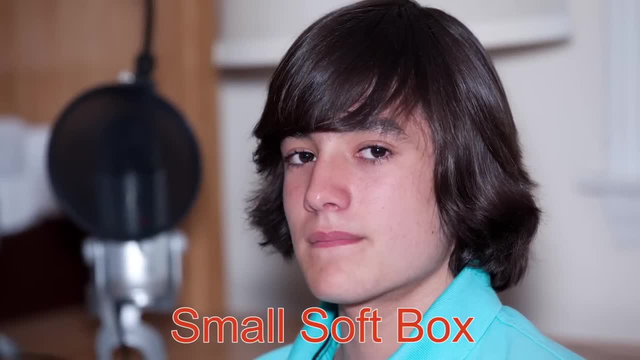 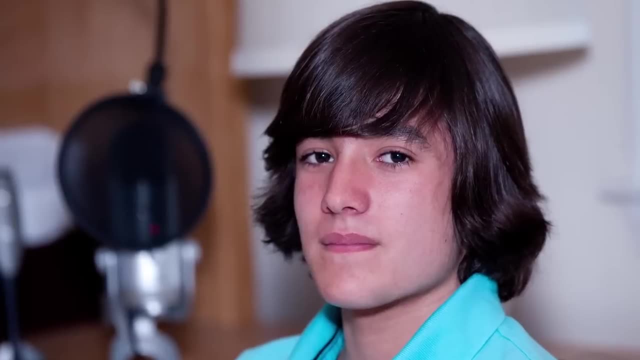 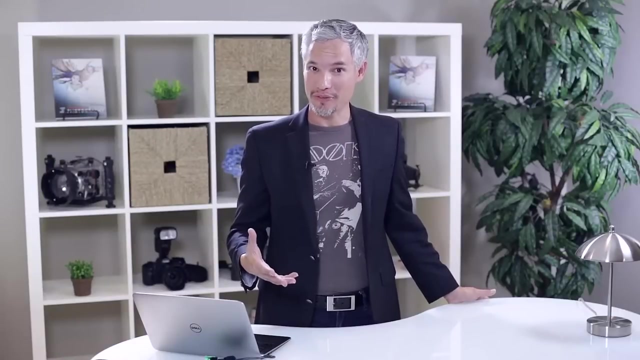 moved the flash farther from the lens. now let's talk about using a high speed sync. by default, a flash occurs over a period of about 1 200th of a second, or 1 250th of a second. the flash seems to fire in an instant in your 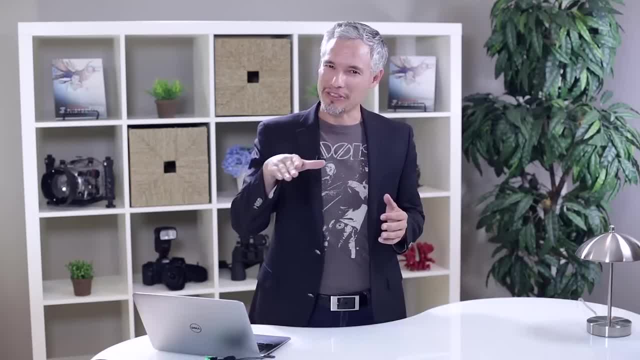 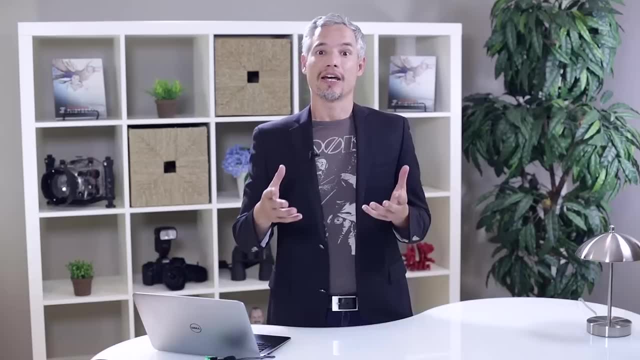 eye, but the flash actually ramps up a little bit. it starts out a little dim and it gets brighter and then all the light falls off and, like i said, that happens over about 1 250th of a second. now what happens if your shutter speed is faster than a quarter? 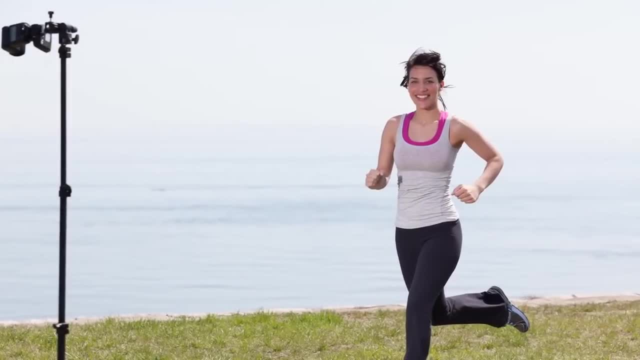 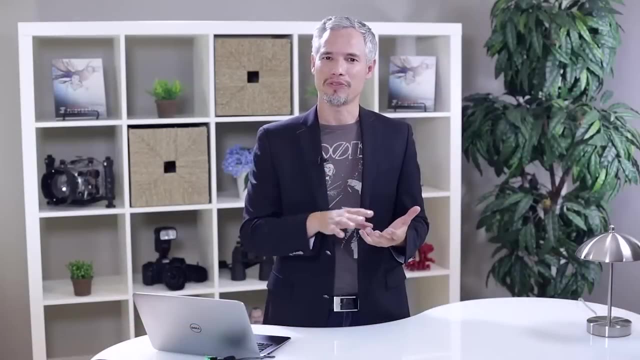 of a second. what if you're shooting sports outdoors? you need to take a picture at 1 1000th of a second? well, you'll run into sync speed problems. now the 200 milliseconds, 250 milliseconds that i mentioned, that's known as the flash's. 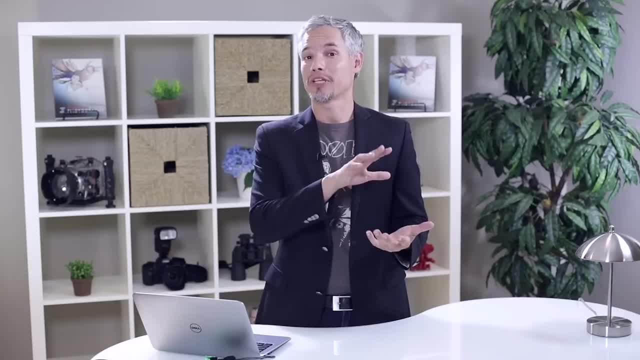 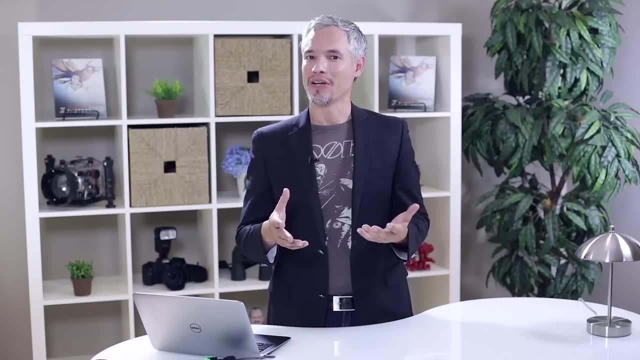 sync speed. it has to match up with your camera, so you have a particular sync speed for the camera model that you have and the flash that you attach to it, and the faster it is the better. but it's not a huge hurdle to overcome so long as you. 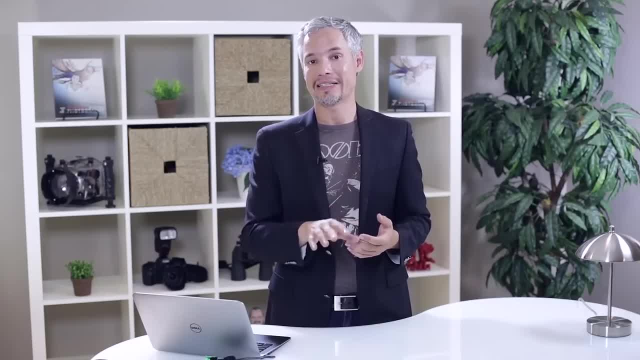 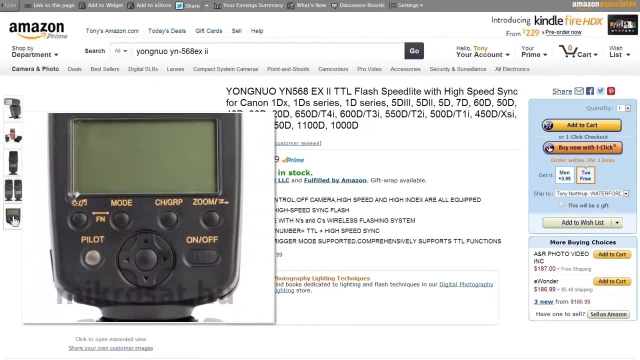 choose a flash that supports a high speed sync, such as the Yongnuo YN568 most cameras. if you try to use a faster shutter speed than your camera and flash's sync speed, well it's simply won't let you do it. it'll stop you from adjusting the shutter. 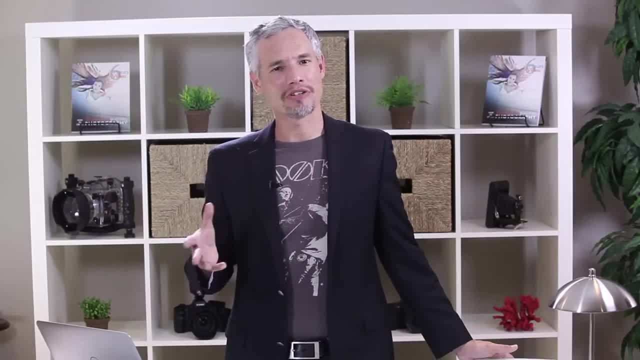 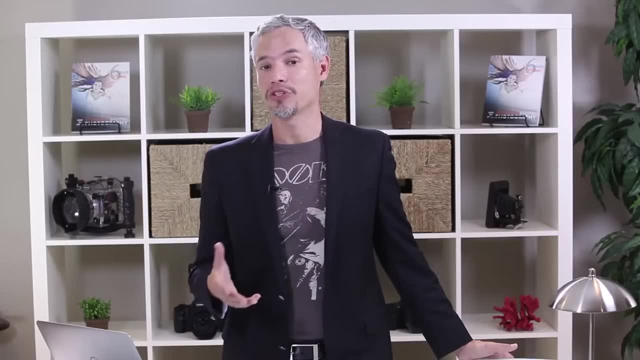 speed past 1 200th of a second or so and, depending on your camera mode, it'll behave kind of differently. so you might end up frustrated because you're trying to pick a faster shutter speed and the camera is just not cooperating well. what you need to do is either change 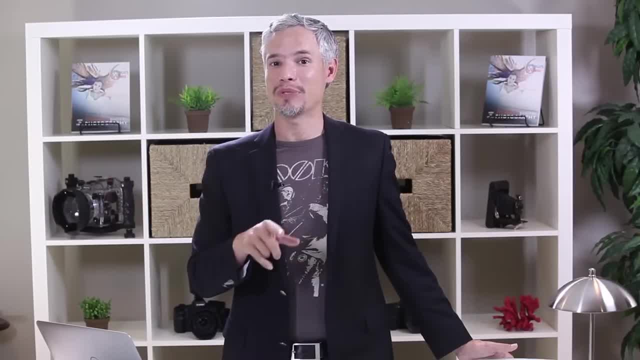 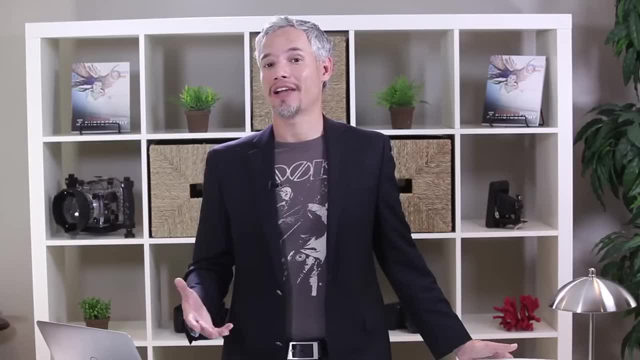 your flash to one that supports high speed sync or turn high speed sync on on your camera. usually there's a switch on the back, though sometimes there's a mode. now you might ask why doesn't the flash automatically turn on high speed sync whenever you need? it seems like you. 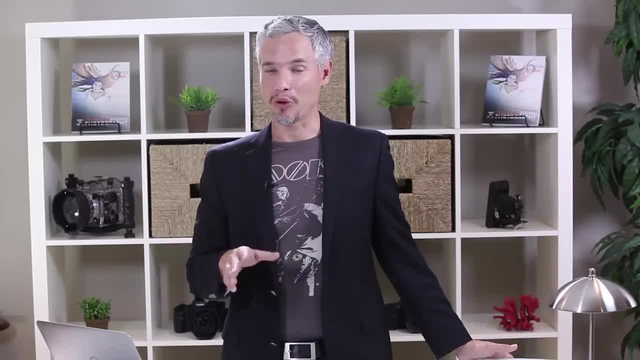 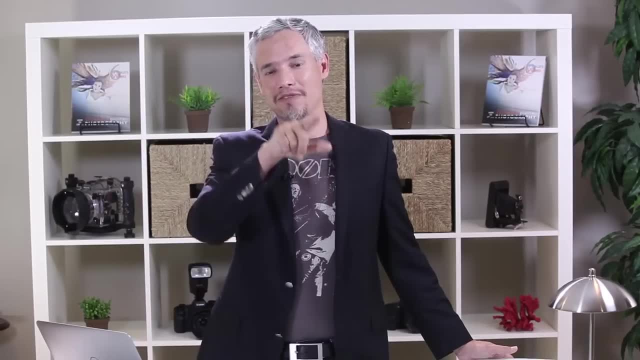 could do that. the answer is that high speed sync uses much more power. the way that high speed sync works is, instead of this kind of gradual ramp up and then a bright light and then it falling off really quickly. the way high speed sync works is it pulses. 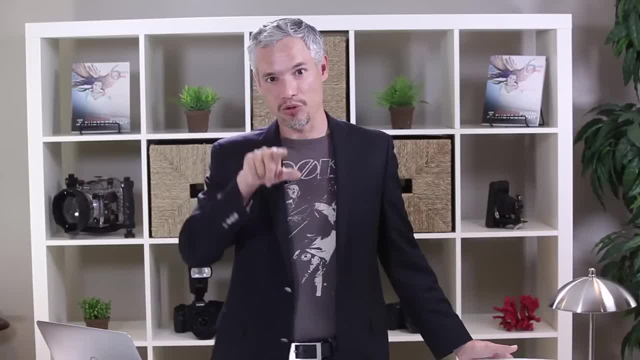 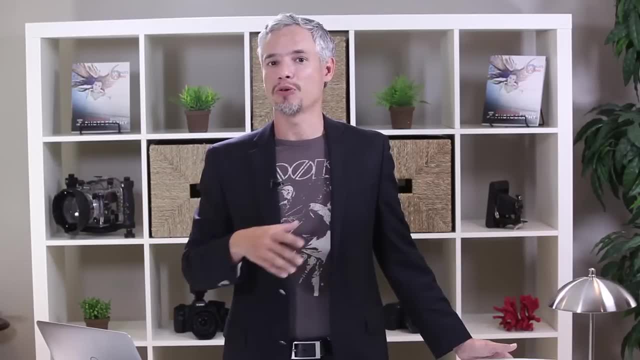 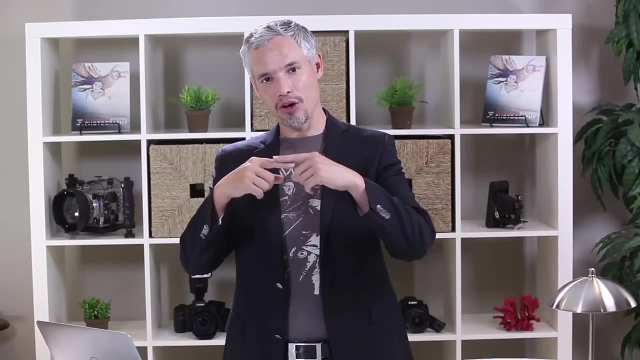 the light. so the light looks like this: it comes in very short waves that are very bright and then suddenly very dark. this allows the entire frame to be exposed more evenly. this happens because when you're using high speed shutters, the camera shutter doesn't stay open the whole. 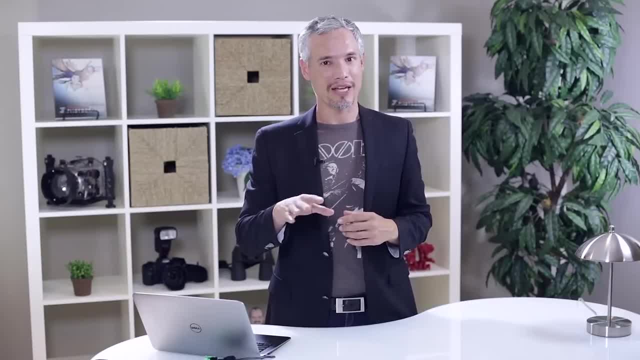 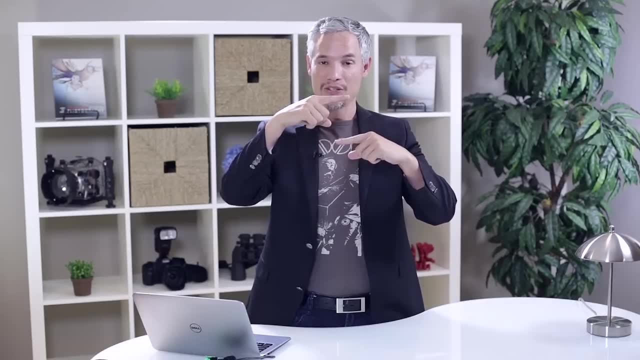 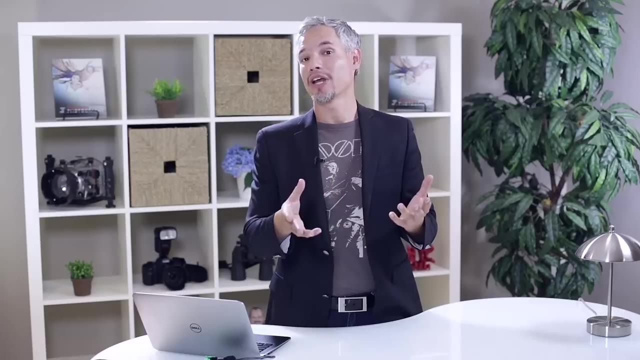 time. here's the way it works: your camera has both a top and a bottom shutter curtain and when you take a picture, what happens is the bottom curtain opens up, shows the entire frame, and then the top curtain comes down after it, covering up the frame. now, if you shoot at 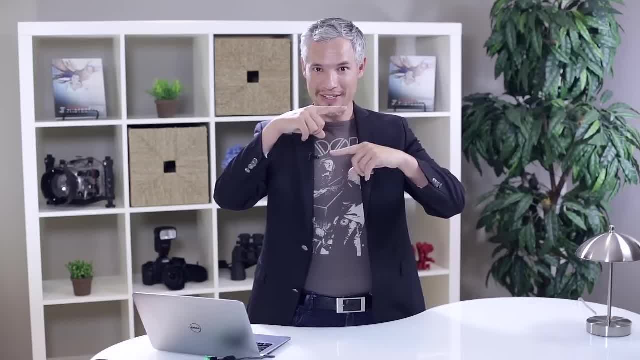 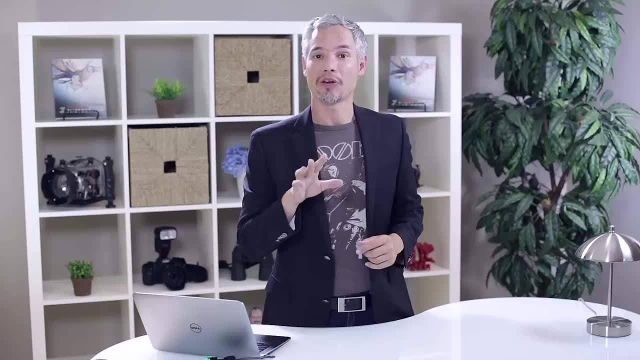 1, 60th of a second. the bottom frame opens up completely, the flash fires, illuminating the entire frame, and then the top shutter comes down to cover it. if you take a really high speed photo, with or without flash, here's what happens: the bottom shutter starts to. 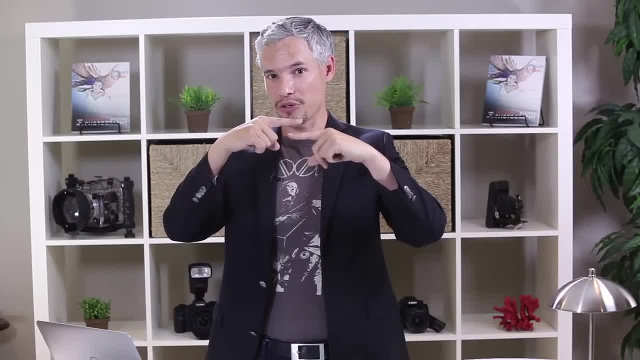 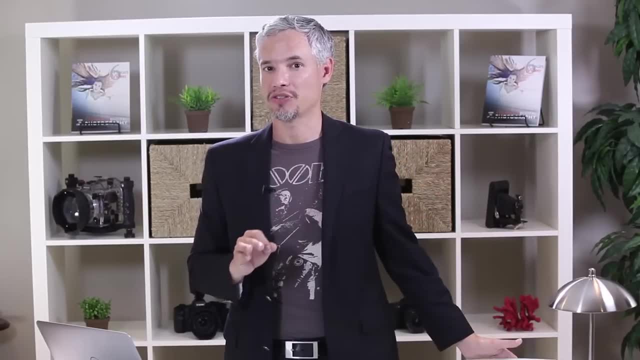 open, revealing just part of the sensor. then the top shutter curtain starts to chase it and the two curtains are kind of chasing each other, revealing just a small part of the sensor at any one point. so as you can imagine if you were to fire the flash when just a small part of that shutter curtain 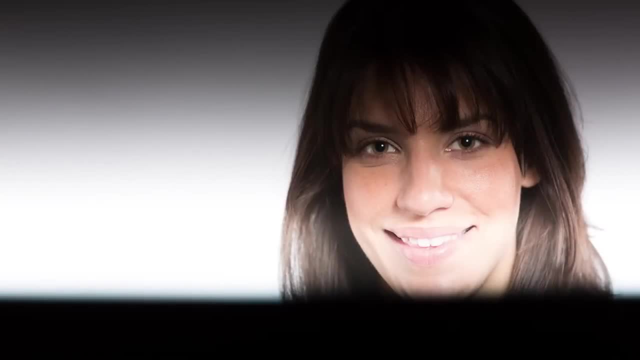 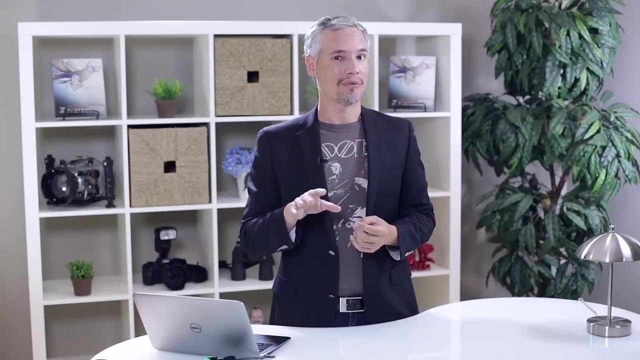 was open, just a small part of the sensor would be illuminated, and that's why your camera is limited to a particular sync speed. now you can overcome this by enabling that high speed sync that I mentioned, but because it has to pulse on and off, it uses several times more power. 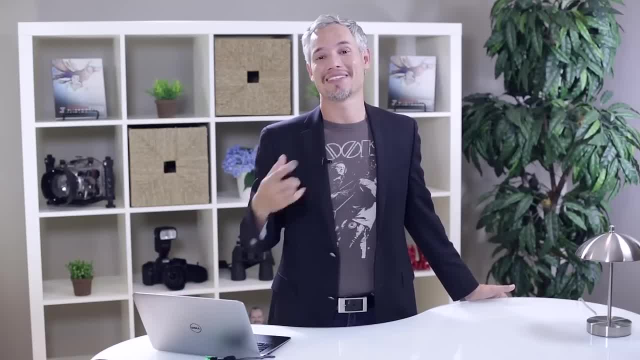 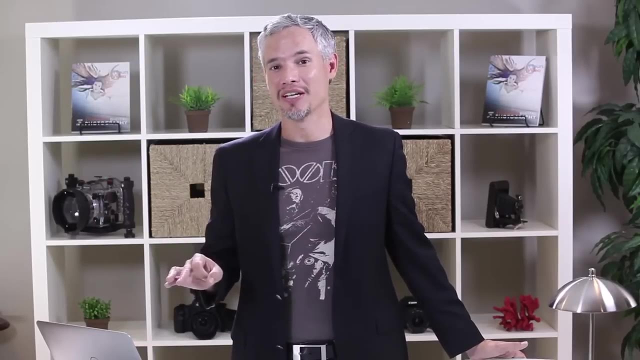 and it increases your flash recycle times, meaning it takes longer until you can take another picture, and it also just burns through your batteries much faster. so that's why high speed sync isn't enabled by default. but high speed sync is really useful for stopping motion. I'm going to take a look at a couple. 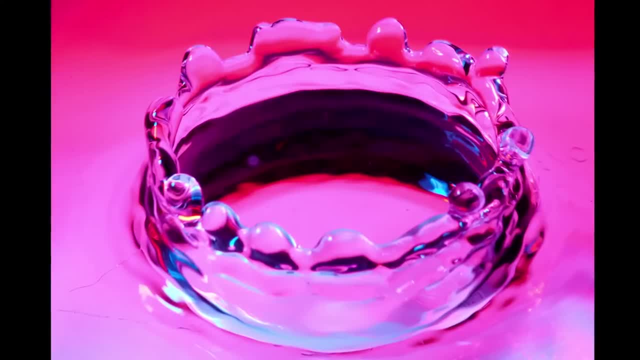 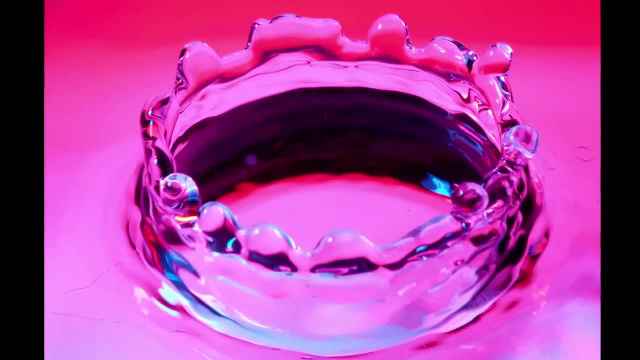 of pictures that illustrate this. here we see a water drop that I captured. now this water drop explodes in just a split second, and if you were to take a picture of this at 1 60th of a second, well, you would just see a bunch of blur. this shot: 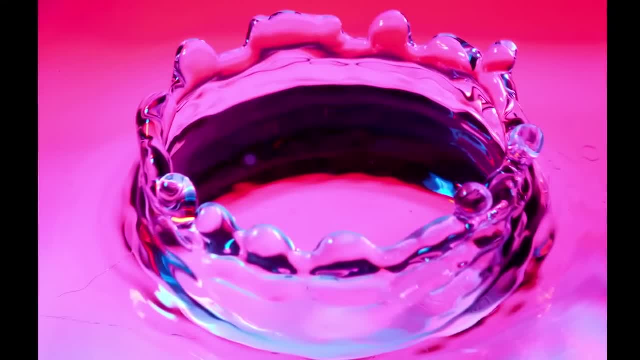 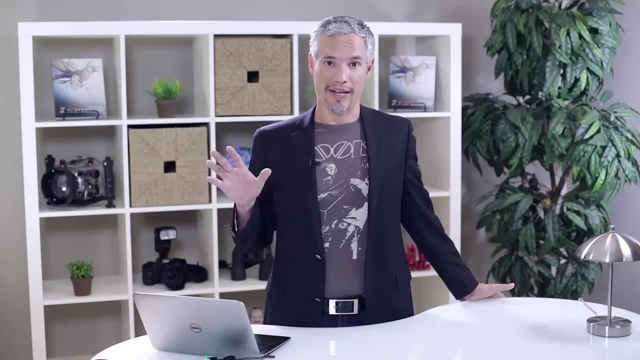 was taken at about 1, 4 thousandth of a second, and that's enough to freeze the action. I don't have enough light to just freeze that water drop in my living room, so I had to use an external flash with high speed sync enabled. let's look at another picture. 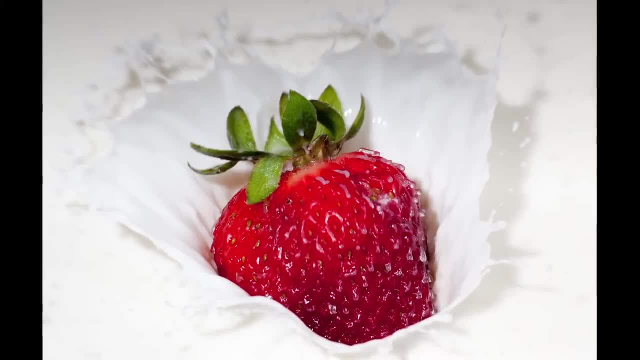 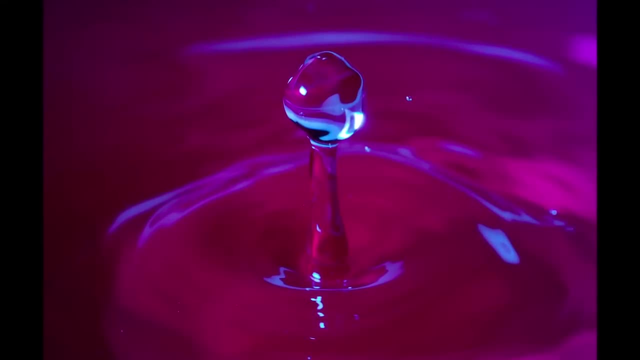 here's a strawberry falling into a bowl of cream and, as you can see, that high speed flash and high shutter speed allowed me to completely freeze the action. here's another water drop and, as you can see, I added some color to the picture if I didn't have any color. 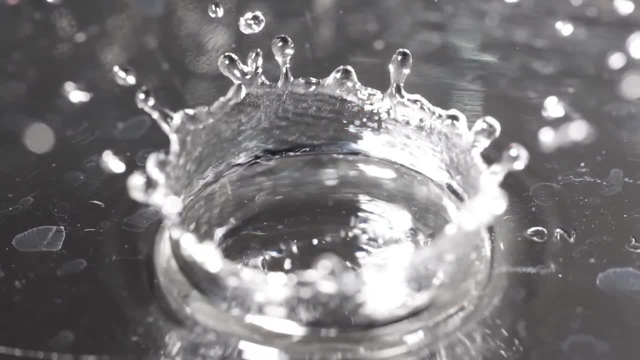 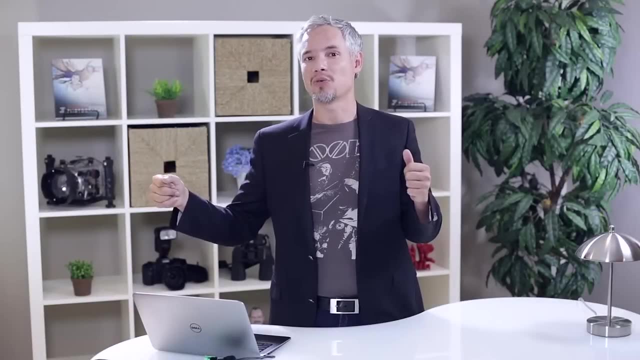 in it. this would just be a clear water droplet and you would see reflections of whatever was in the room around me. so what I did was I put a red gel over the flash and then I set up a blue card to kind of reflect into the water and catch those. 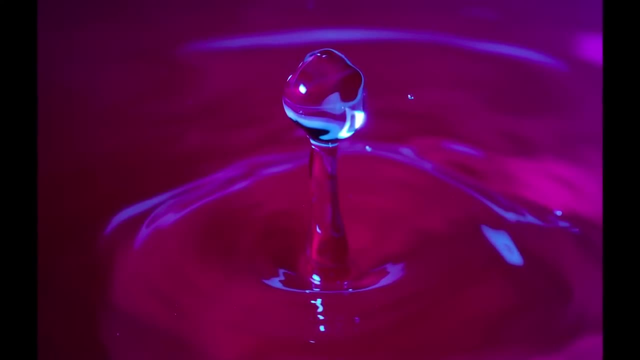 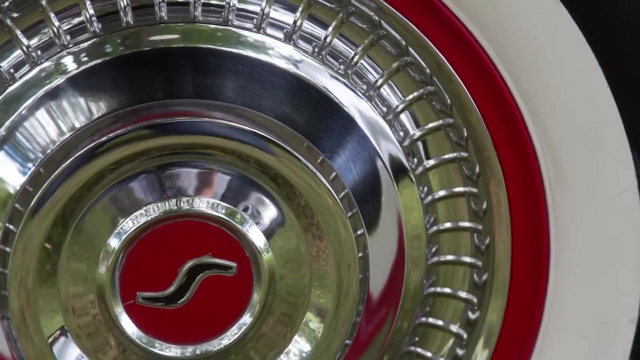 highlights. this also kind of illustrates the way that light is always being reflected around the room. something reflective like a water droplet or a car is going to be reflecting the surroundings. so you really need to think about that, especially if you want to do product photography. let's say you're taking a picture. 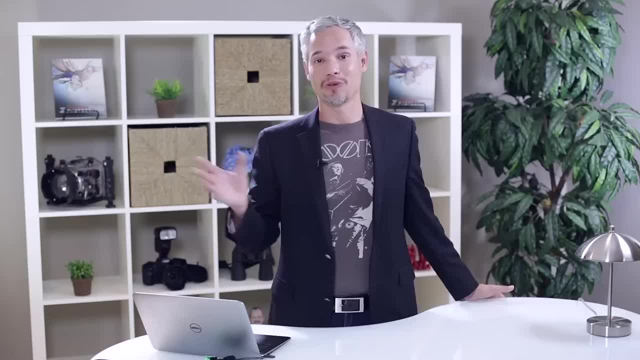 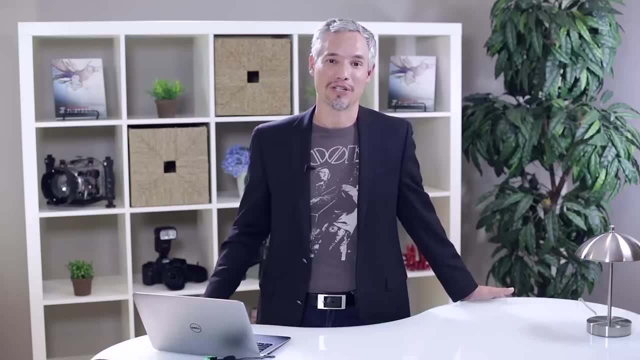 of an iPhone, that front edge is going to capture a reflection of everything in the room, so you not only need to plan out the objects that are in the frame, but you need to plan out the objects in the surrounding area. for something like that, you might even set up just. 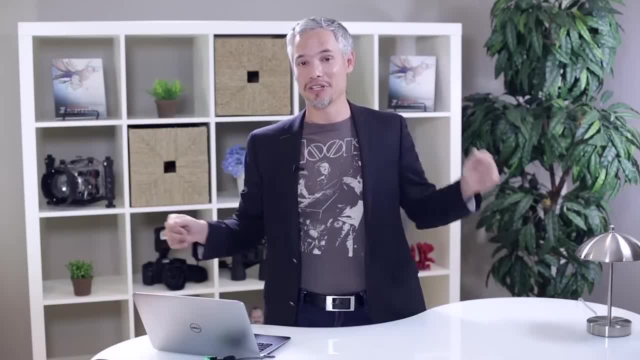 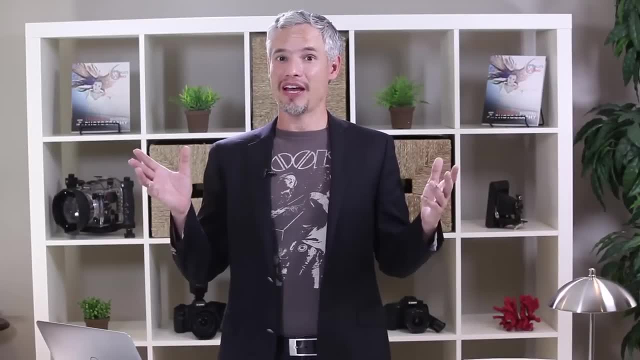 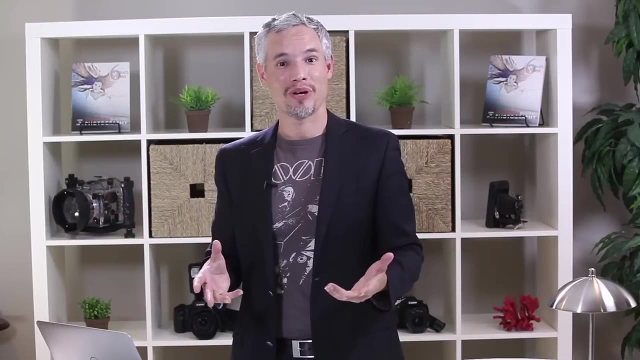 big cardboard cards that are reflected perfectly into it, so you get the exact reflection that you want. another really complex aspect of light is white balance. now, when you're inside under halogen or incandescent lights, everything looks white to you. a white book looks white. the white trim in your house looks white. 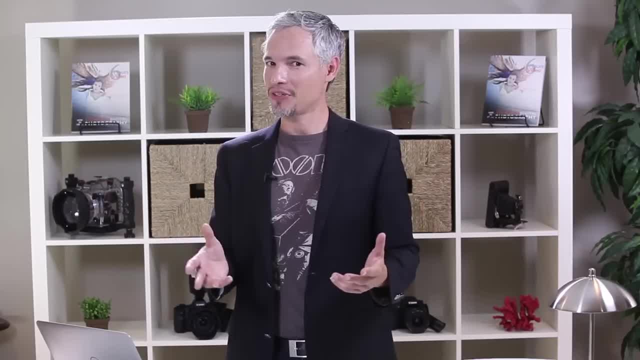 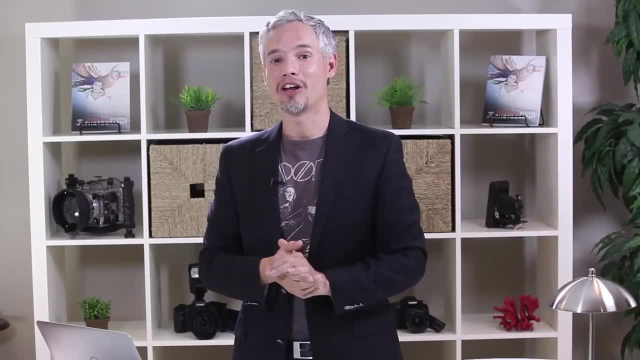 and if you were to open a window and let the sunlight come through, it would still all look white. that's because your brain is lying to you and your camera can lie to you too and automatically adjust for all these things, but it doesn't always do it correctly. 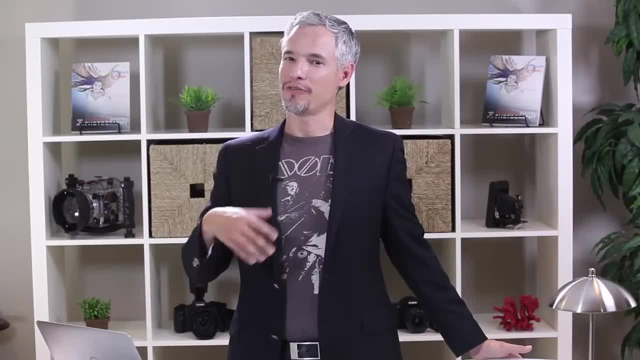 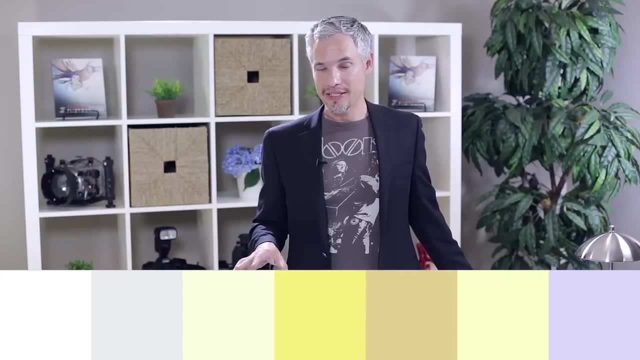 so let's take a look at an example of a white piece of cardboard that I took pictures of in many different rooms. now, each one of these vertical colors is the exact same piece of cardboard, just photographed under different lights. some of these were natural light and others. 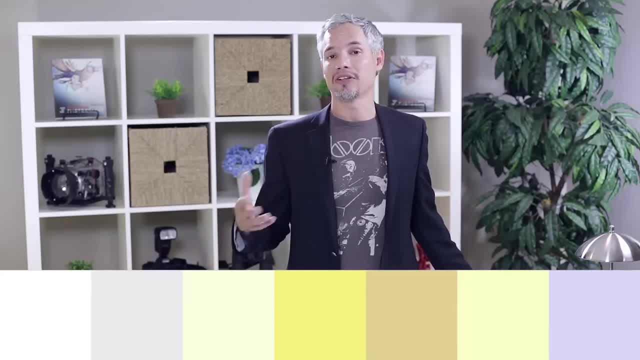 were the incandescent lights in my house, or halogen lights or fluorescent lights. as you can see, it ended up being a range of different colors, even though it's all white. like I said, it's your eye that's lying to you. these things really do have different color temperatures. 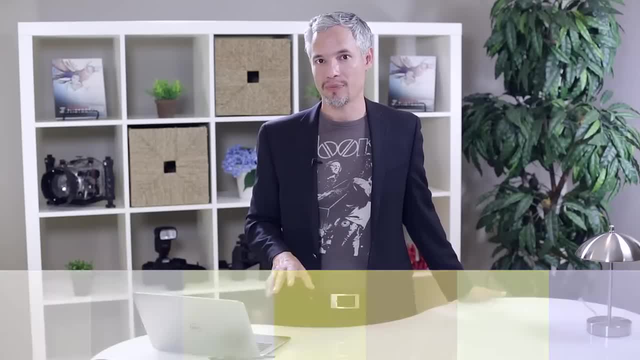 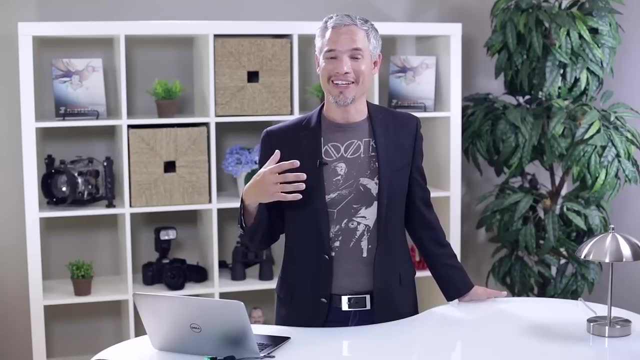 and a white object doesn't necessarily look white to a camera all the time. now your camera is, by default, going to use auto white balance and it will try to detect the incoming light and set the white balance correctly, and that usually works fine and you might never have to worry about the white. 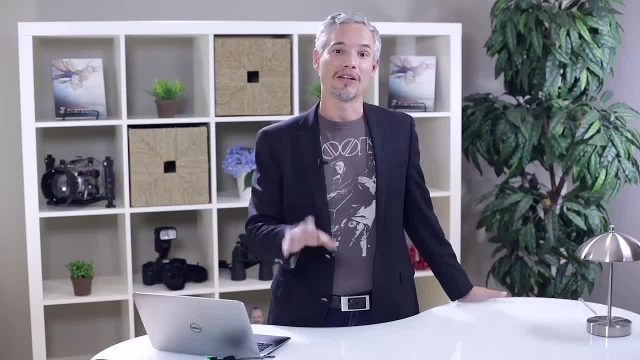 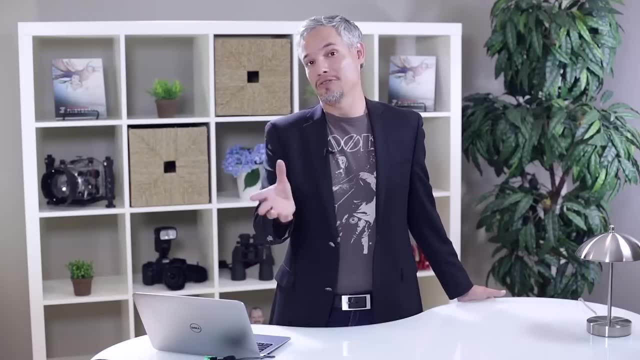 balance. however, if you start getting into night photography or you're taking pictures indoors with multiple different sources of light, well, your camera's not going to be able to figure it out because there is no one right answer and it needs to pick one right answer. so for that reason, it's important. 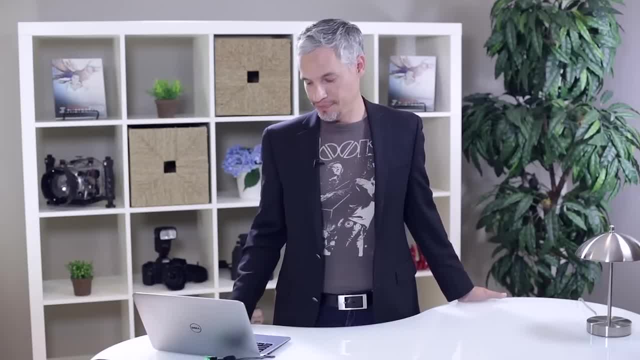 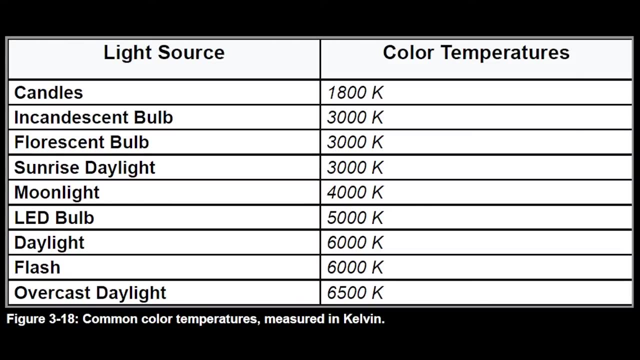 to understand white balance, let's look at a chart. this chart shows a variety of different light sources along with the associated color temperature. now color temperature is measured in Kelvin. that's that big K and, as you can see, at the low end of the Kelvin scale we have really warm. 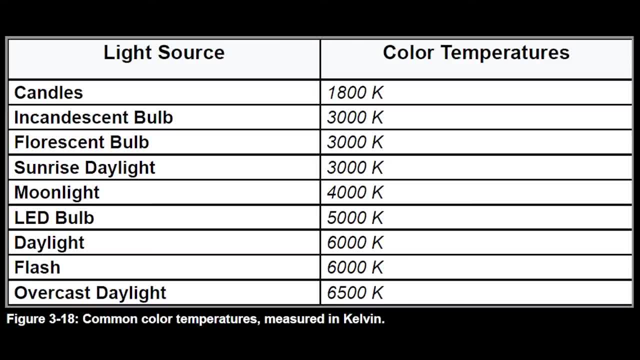 color temperatures, like candles and incandescent bulbs and fluorescent bulbs. to our eyes these all look pretty orange, and below that we start getting into cooler light sources, light sources that look more blue like moonlight, or those new LEDs, D bulbs. now you notice that daylight and flash. 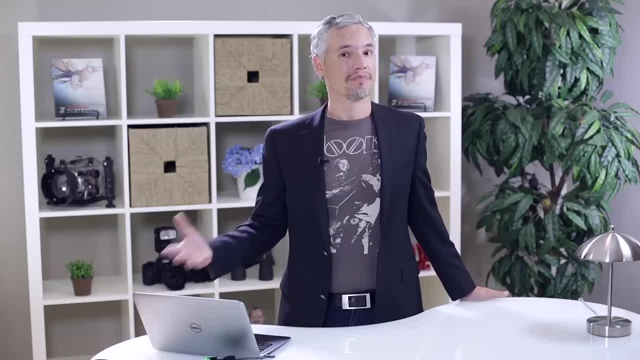 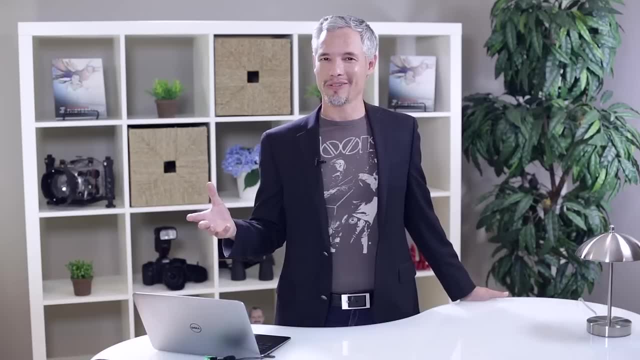 are both 6000 Kelvin. that's because your flash is daylight balanced. your flash is always going to look good mixed with daylight and, in fact, if you're indoors and you're getting some weird colors, turn your flash on, bounce it around the room, because your flash is. 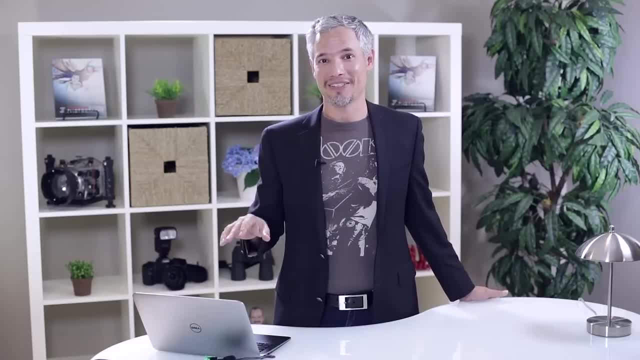 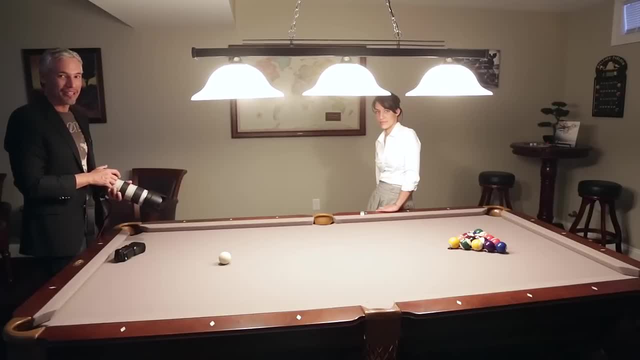 going to fill up the room with perfectly daylight, balanced light, and it's going to solve all your white balance problems for you. Chelsea and I are in the basement to take some sample pictures in a low light environment. we're lit entirely by this artificial light. here I've 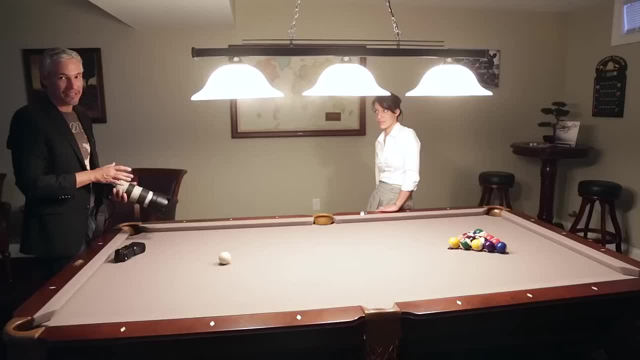 put my camera into aperture priority mode with f 2.8 selected. that's the lowest f sub number this lens supports, and I've selected auto ISO, so the camera will automatically select the shutter speed and ISO to expose the picture properly. so I'll take a picture of Chelsea now. 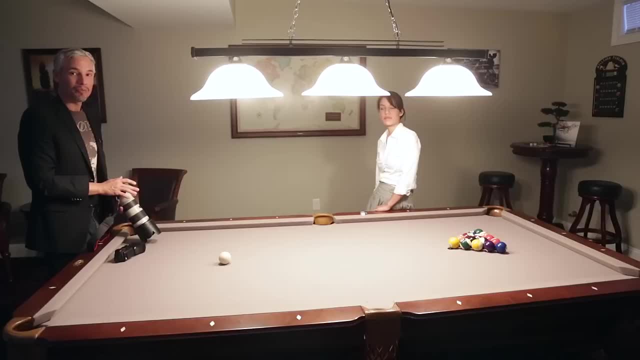 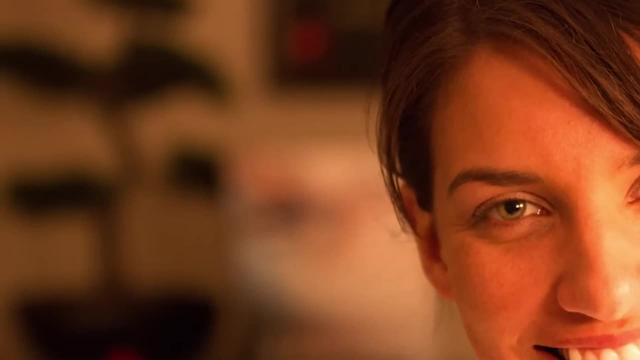 so that's not bad. the camera exposed it properly. but there's a bit of a problem. if you look closely it's extremely noisy. that's because the camera had to select a very high ISO to properly expose in this dark environment, even though Chelsea's pretty close to the light. also, you notice. 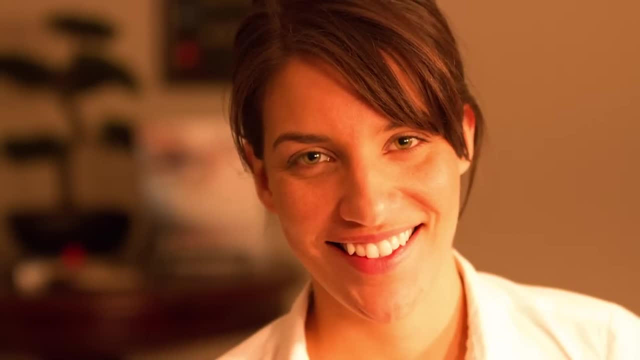 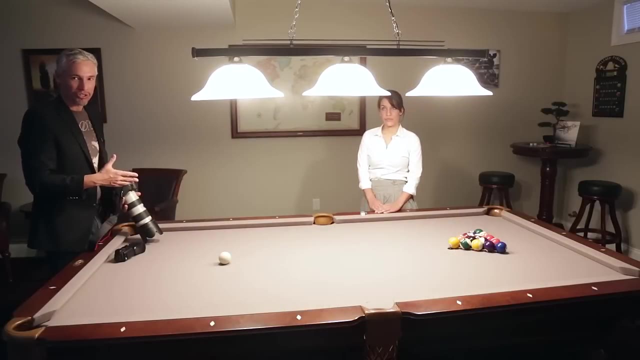 that the color temperature is completely wrong. I have the camera set to auto white balance, but it didn't do a great job of it because these lights are so extremely warm- warm meaning very orange colored. so one way to rectify this is to add my own light to. 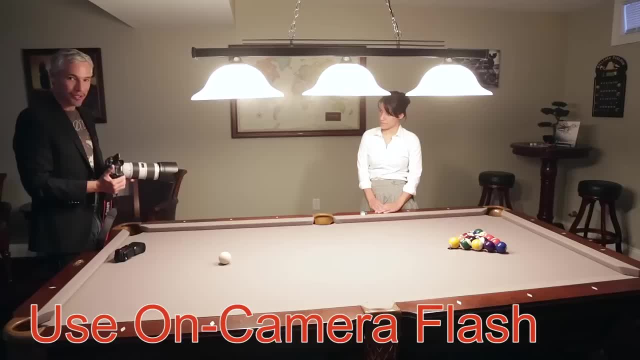 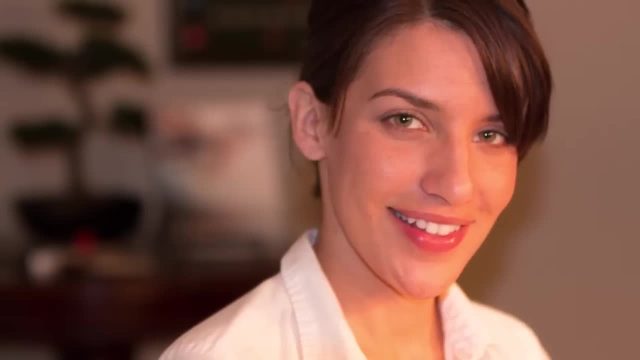 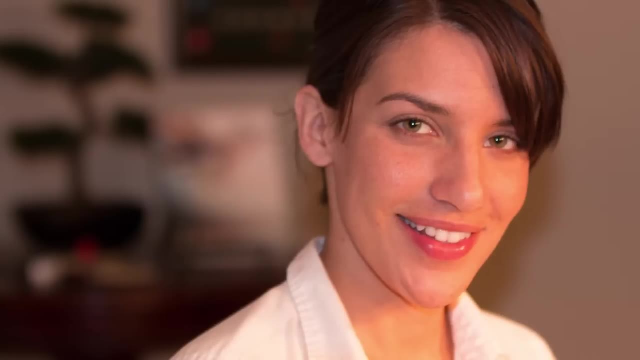 add some flash. so I'll turn on the on camera flash here and take another picture. so that's a big step in the right direction. we dropped to ISO 400, which gives us a much cleaner image, and the white balance is suddenly fixed because the flash here is. 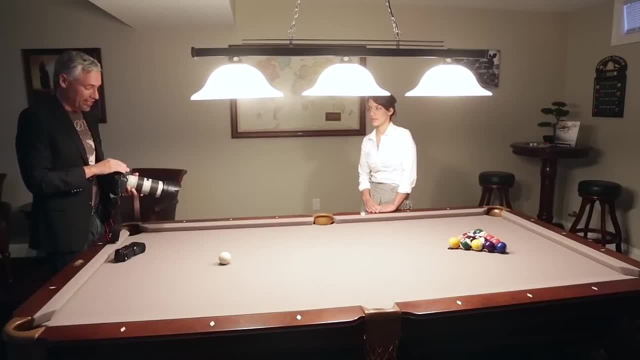 always daylight balanced, but we can do better. having the flash so close to the lens cast these really ugly shadows both on her chin and against the wall, and it's pretty easy to fix with an external flash. now you don't need any kind of fancy flash for this, but I do recommend getting a flash. 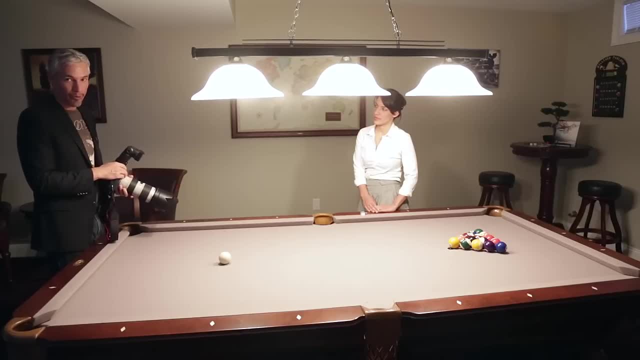 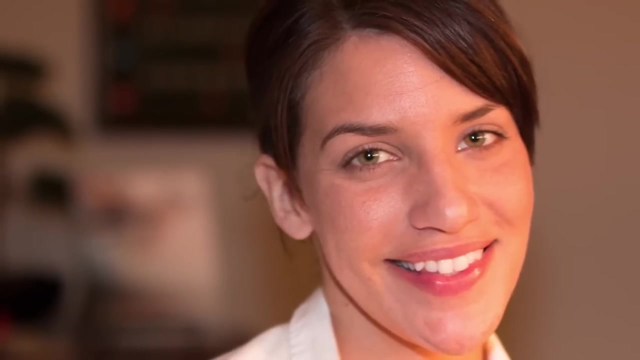 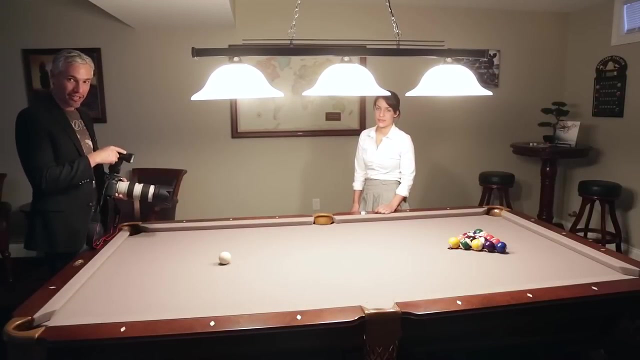 with TTL support for your particular camera model. I recommend looking at the Yongnuo YN468 too. so with the external flash on, I'll take another picture of Chelsea so we can see the difference. so putting the external flash on did a couple of things. the front lighting coming from the flash was moved. 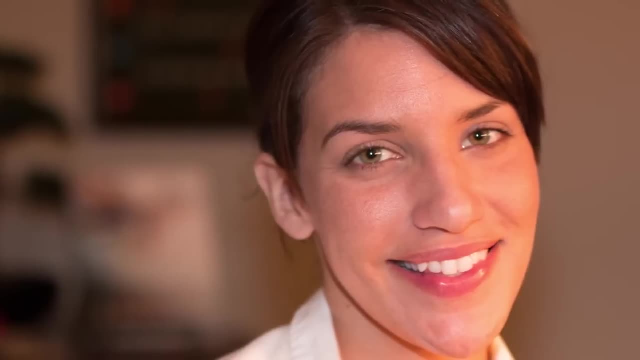 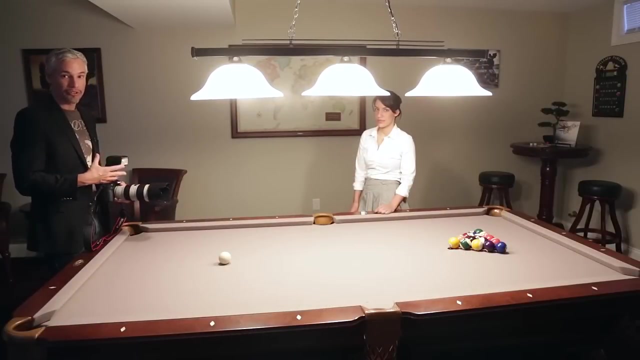 farther from the lens, which cast a little more pleasant shadow, and it also has a bigger surface area. the on camera flash is much smaller than this and a larger surface area casts softer light- still a relatively small surface area- and is still relatively close to the lens, so a really easy way to fix that. 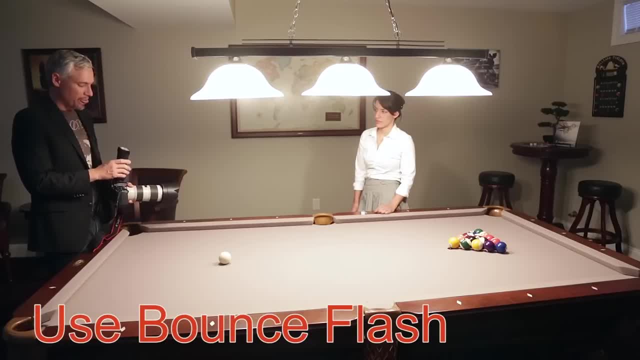 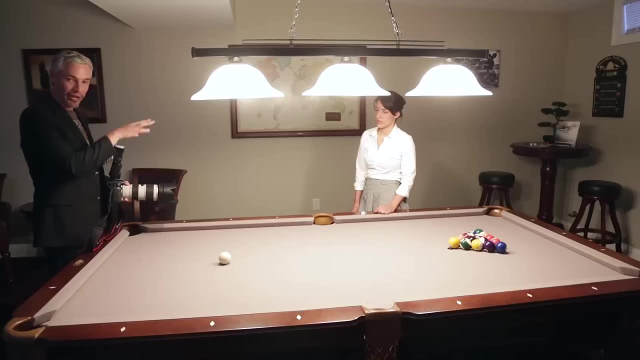 is to use bounce flash instead. so I'll just turn the bounce flash on, and usually what I'll do is I'll pull out this little diffuser and leave this white card up. the white card will catch some of the light and reflect it directly at Chelsea. 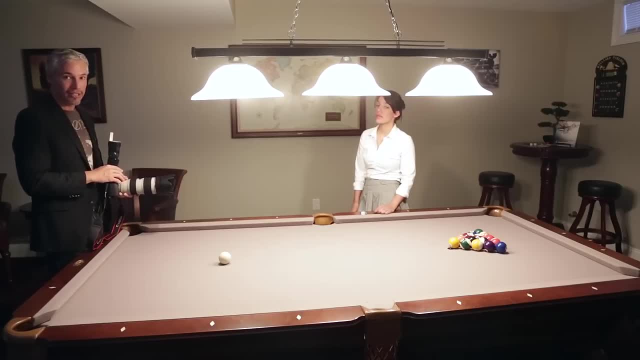 so most of the light here is going to be bouncing off this low ceiling, but some of it will be bouncing off this white card and that will give her just a little bit of a catch light. it's a really nice effect and it's also really easy to do because this is built into 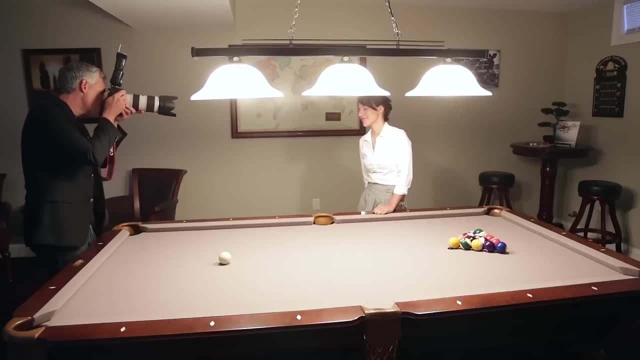 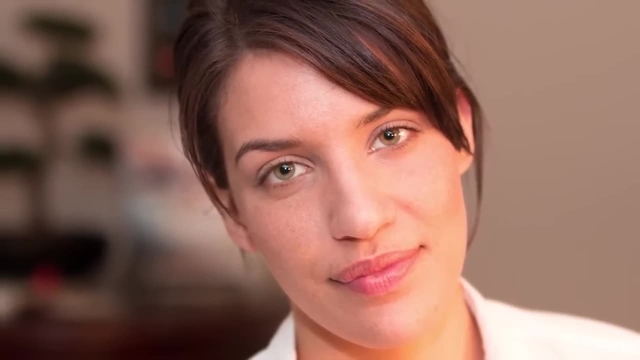 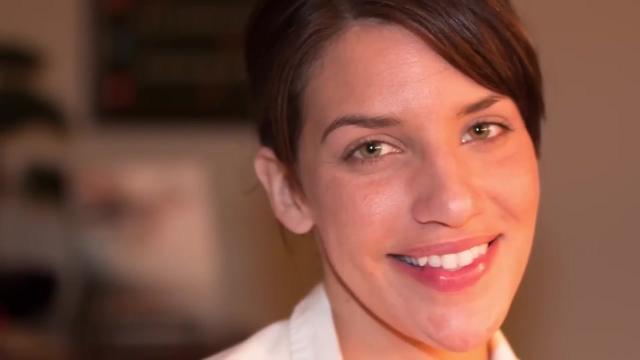 most modern flashes. so I'll take another picture. compared to the other pictures, the picture with the bounce flash has the background much more evenly lit, because when the flash is direct, when it's pointed directly at Chelsea, the light falls off behind her because she's so much closer. 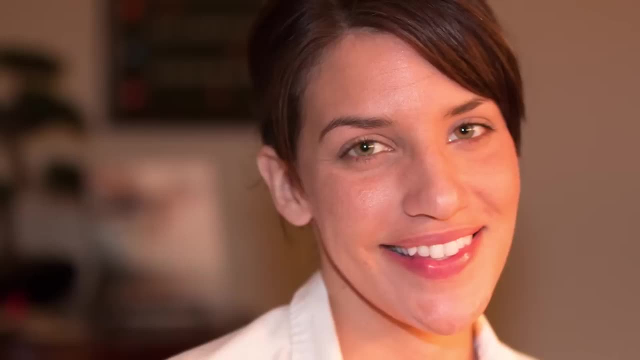 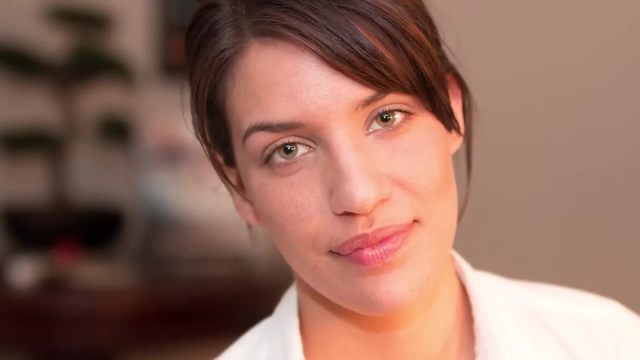 to the flash. therefore, the subject is always going to be much brighter than the background. however, by bouncing the flash straight off the ceiling, more of the light is reaching the background and it's more evenly spread across the foreground subject. it's still a little darker, but the balance is much better. 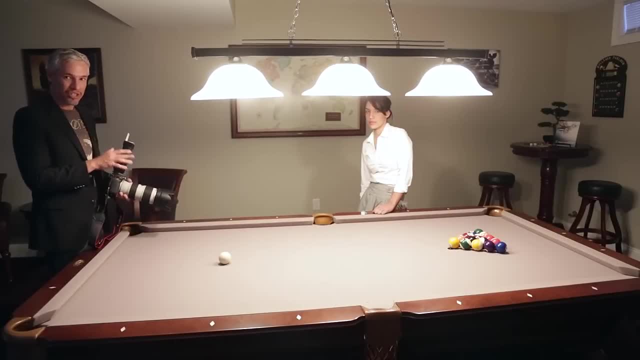 now I'd like to talk about how changing your ISO can change the effect, because it requires more or less light from your flash. so I've been shooting at ISO 400, which is a good compromise. ISO 400 provides a reasonable amount of noise while not requiring 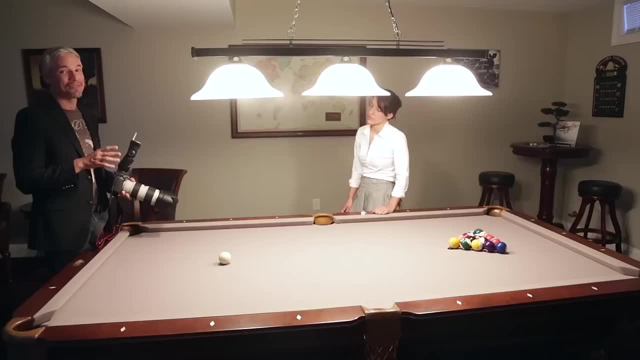 your flash to do too much work. ISO 100, though, provides a much cleaner picture, however, because it's two stops brighter. I'm going to need to turn my flash up by two stops now, because this flash supports TTL, it'll automatically compensate by putting out two stops more light four times. 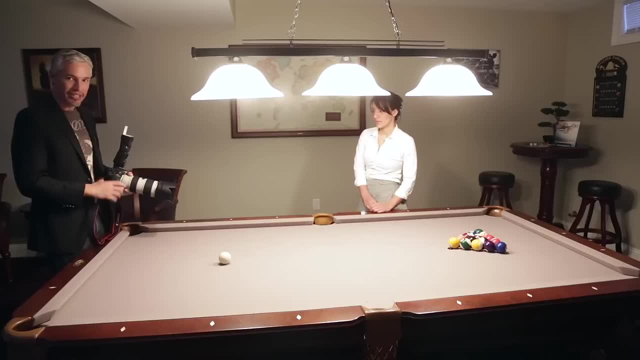 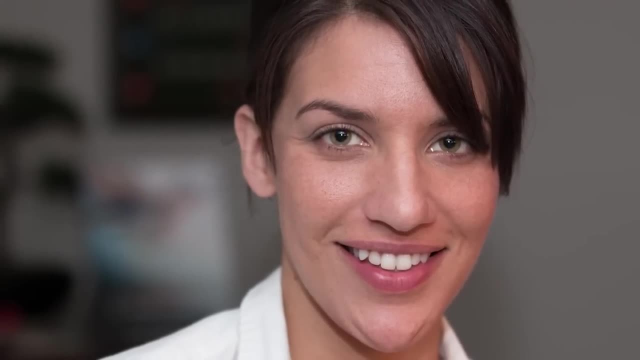 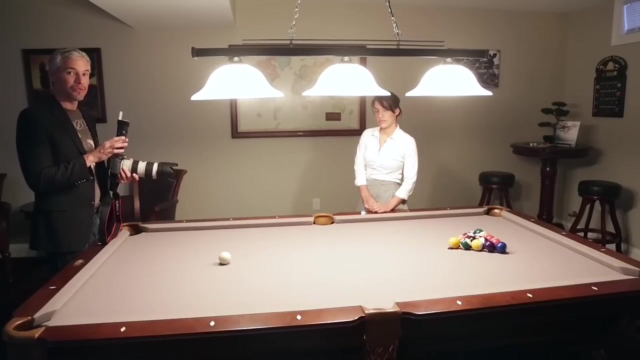 more light, so I'll put my camera into ISO 100 mode and take another shot. besides putting my camera into ISO 100, I put it into manual mode and set the shutter speed to 1, 60th of a second, otherwise it would try to expose the. 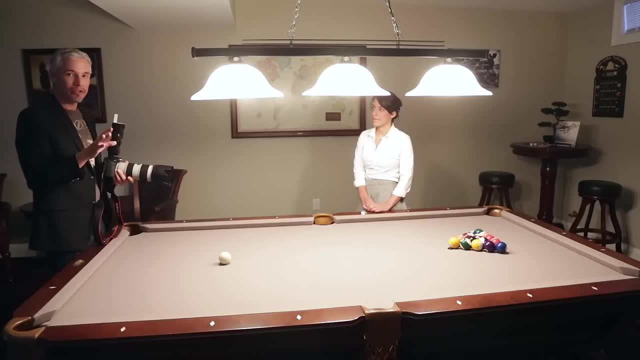 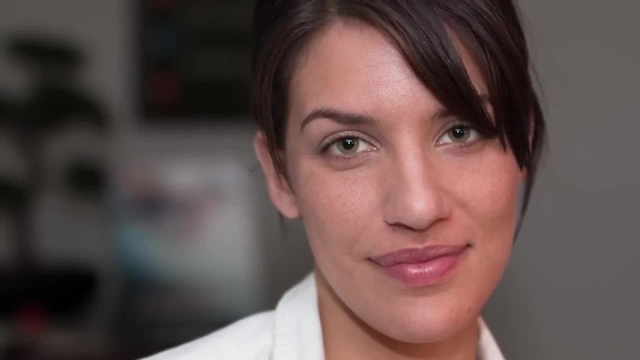 ambient light properly. but because I'm using bounce flash, I don't even need to worry about the ambient light. I know the flash is going to overpower it. well, looking at those pictures, they look pretty good and ISO 100 looks okay. but listening to my flash, I noticed 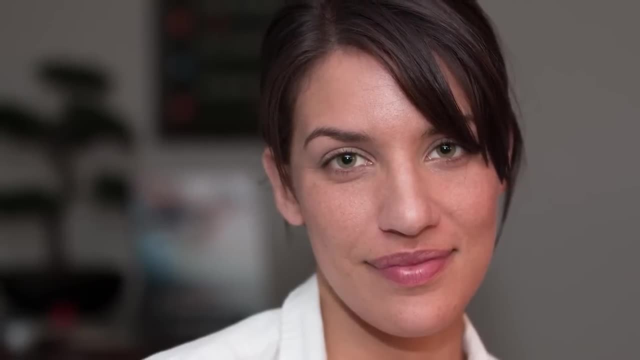 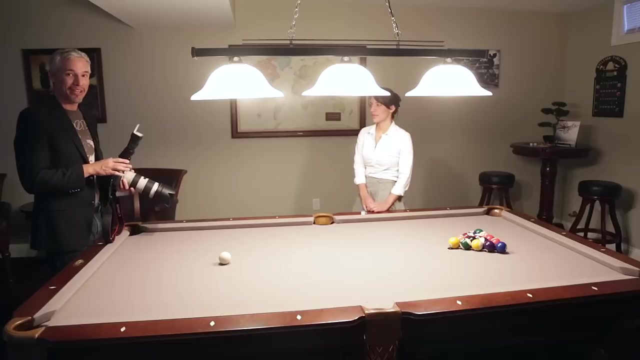 it was working a lot harder. it made a louder noise and it took longer to recharge. you know you kind of hear that like winding up sound that it makes. it took longer because at ISO 100 it needs to put out four times more light than ISO 400. 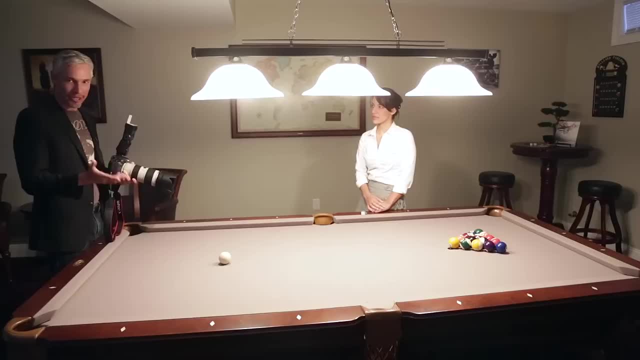 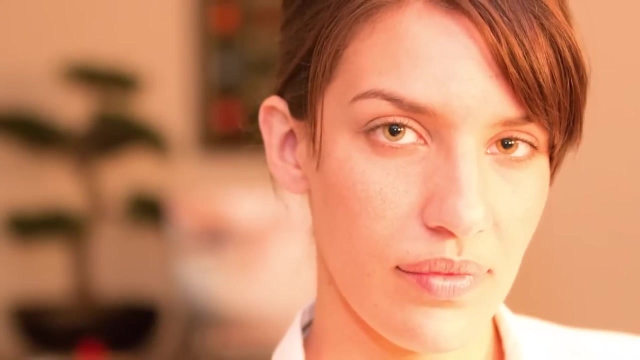 so to compare it, I'll raise the ISO all the way to ISO 3200. now, compared to the ISO 100 shots, the effect is very different. you'll notice that the color went from being perfect to suddenly being very warm, very orange and very brown. that's because 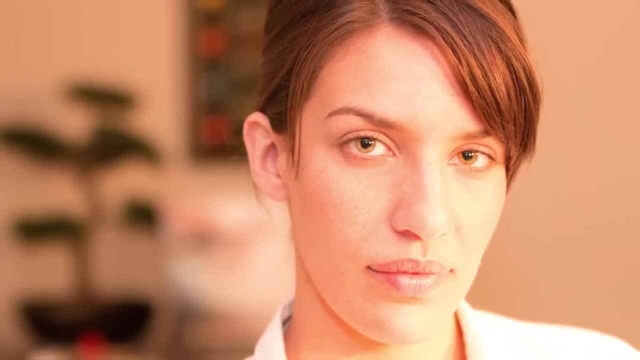 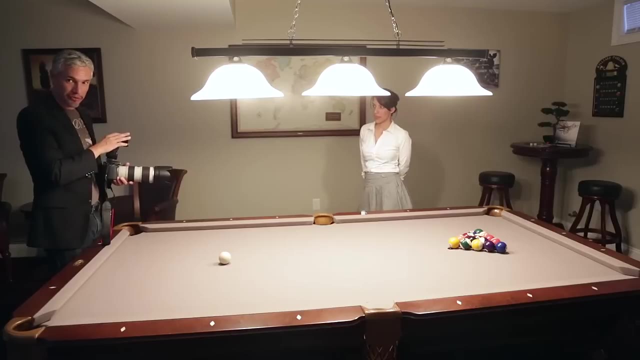 at ISO 3200, the camera's TTL system needed to put out much less flash. now you can get into situations indoors where the ambient light is a different color from your flash. that's what I've been dealing with here and that's why we've seen these struggles. 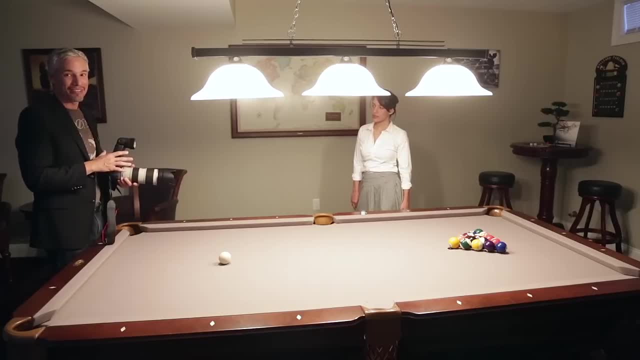 between an orange white balance and a very natural white balance. sometimes, if you want to use the artificial lights to light up the background or to partially light your subject, the easiest thing to do is to adjust the color of your flash to match that of the light. so what I find I like to do is 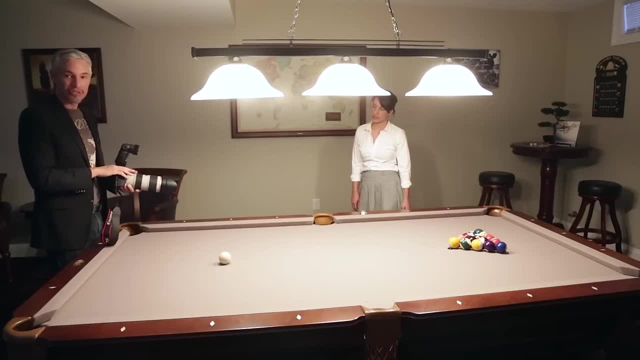 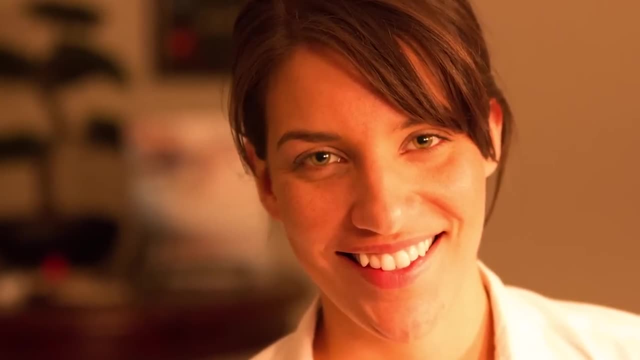 take a picture of something white, with the white balance here set to daylight and, as you saw in those pictures, that results in a picture that looks very orange if you look at Chelsea's shirt. now what I want to do is to make my flash the same color as these lights. I want to make my flash. 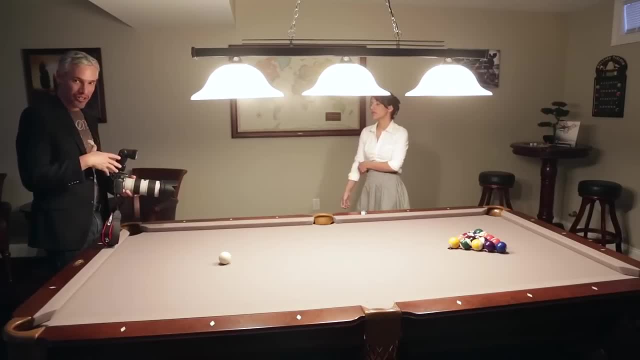 orange, and that way I can adjust the entire picture to be more blue and the color will be consistent between the foreground that's lit by the flash and the background that's lit by the ambient light. so I'm going to add an orange gel to my flash now. 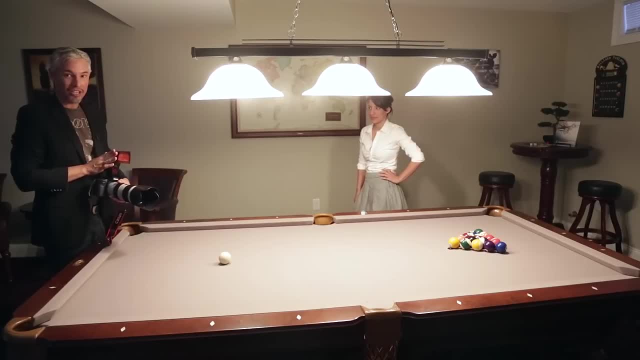 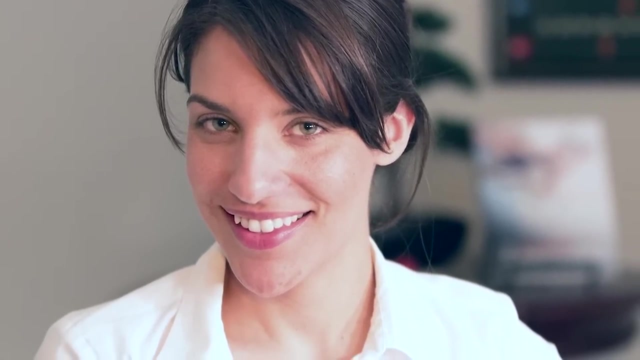 so now that I have the orange gel attached to the flash, it will come out the same color as these lights here, according to the camera, so I'll take another picture of Chelsea. it actually looks really weird when you're looking through the camera, because you'll see this orange flash coming out. 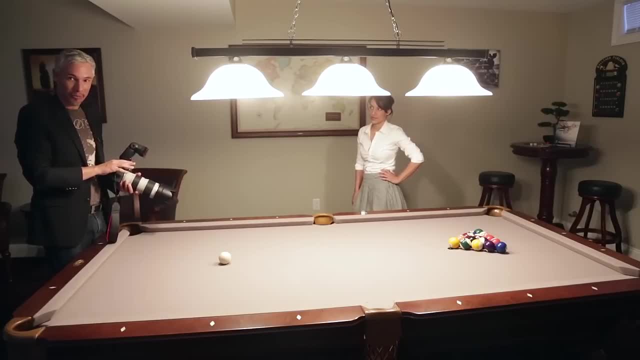 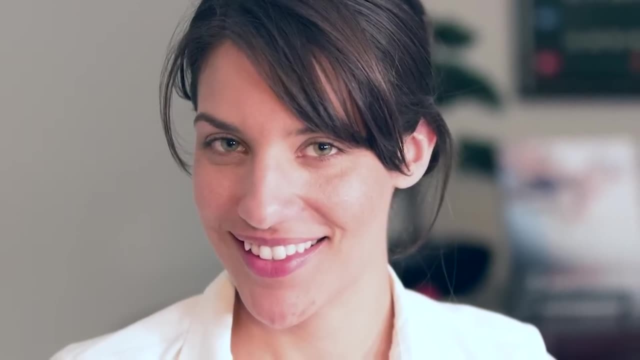 and you think your pictures are going to be ruined. but if you have the white balance set correctly on the camera, then everything looks completely natural, because the camera is going to pull everything towards the cool side, back to blue, so the color from the flash perfectly matches the 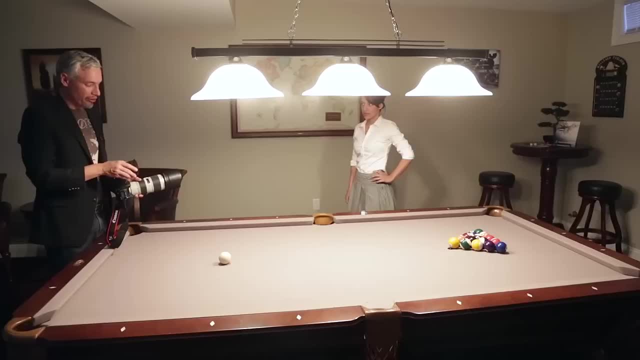 color coming from your ambient lights. it's a good thing to do to carry around a bunch of gels like this if you're going to be shooting indoors and you think you might want to add a little bit of fill flash, because it's impossible to adjust. 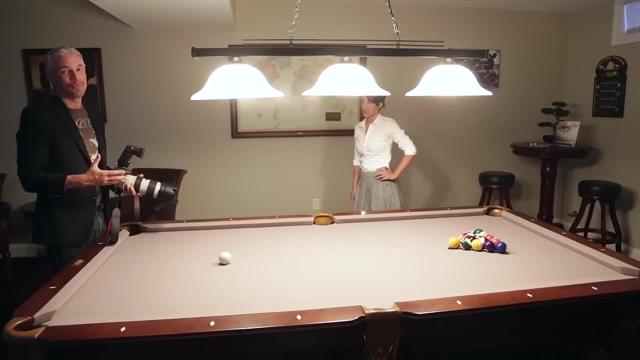 the white balance. when you have different colors of lights in your pictures. you know, if you shoot raw then you can adjust the entire picture towards blue or towards orange to fix any color problems. but when you have multiple light sources, like a fairly blue flash and a fairly orange light here, 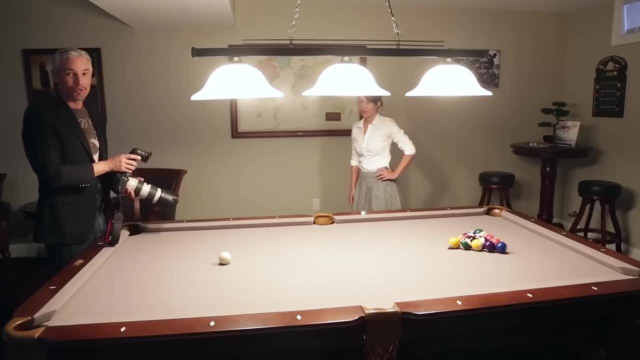 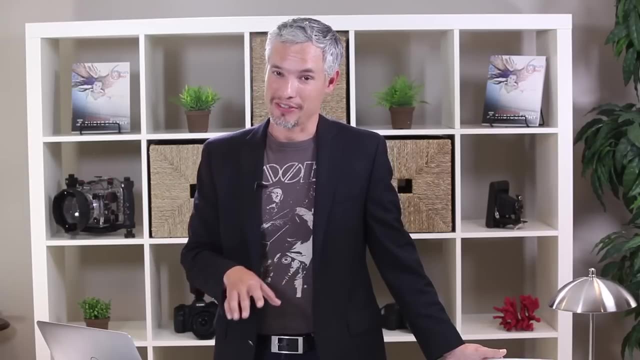 it's really difficult to fix that, so it's better to do it at the time you're shooting, by adding a gel to your camera flash. another way you can easily solve your white balance problems is by shooting raw instead of jpeg, and we're going to go into this in more detail in another lesson. 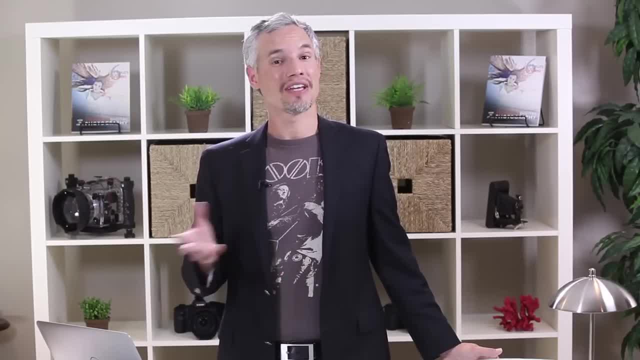 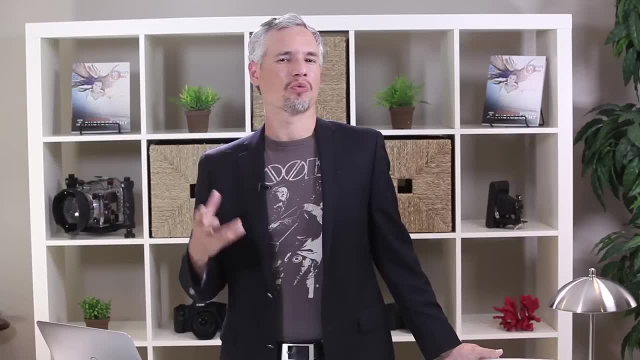 but my advice to you now, especially when you're still learning, is just enable raw on your camera. if you still want that jpeg, you can shoot. jpeg plus raw raw captures- just the raw data that's collected by your camera sensor and it doesn't process it in any way. normally, your camera 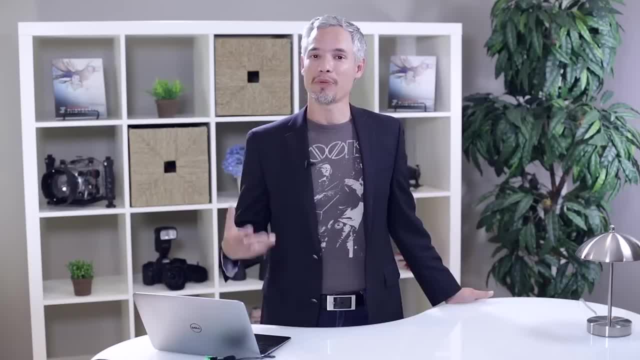 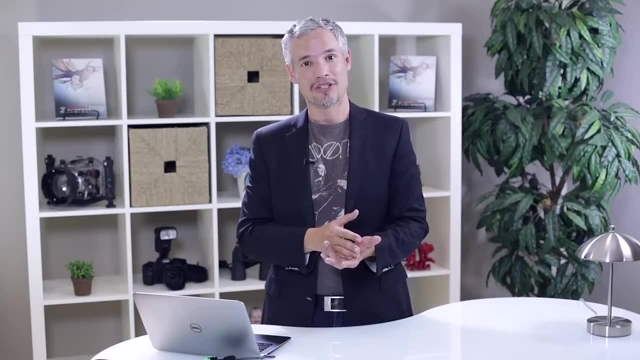 processes that raw data and turns it into a jpeg, and part of that processing is deciding on the white balance, figuring out what set of colors is going to make pure white on the image. so it's doing that in real time instead of allowing you to do it. 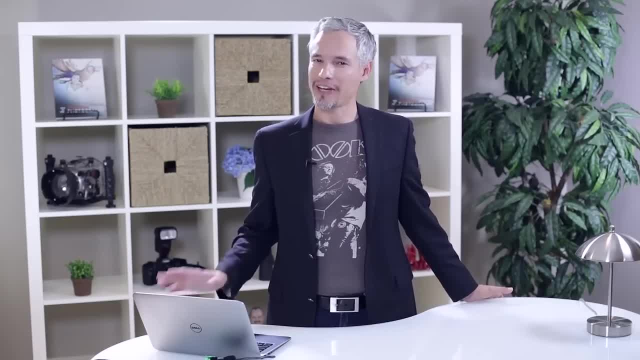 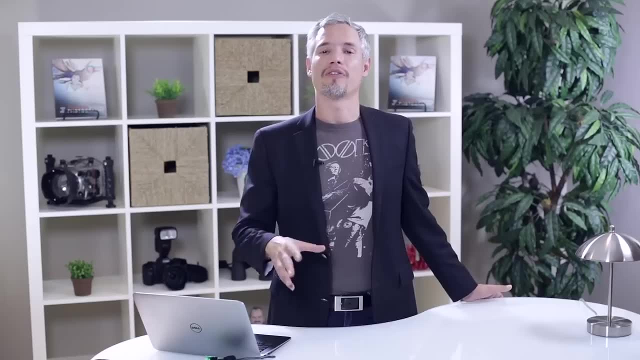 later. don't worry, if you have shot jpeg pictures and you find that the color is a little off, if it has an orange tint or a blue tint, you can probably still fix it. however, if you shoot raw, you'll have a stronger ability to fix it and you'll be able to fix it more. 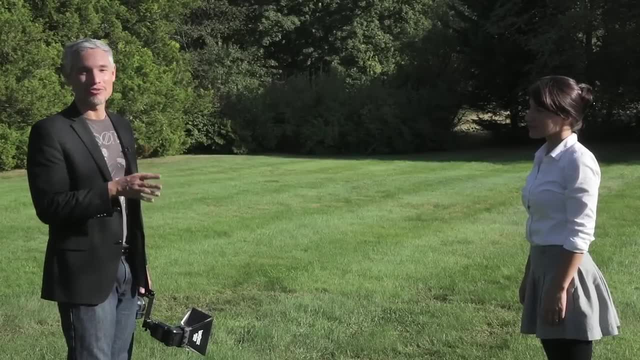 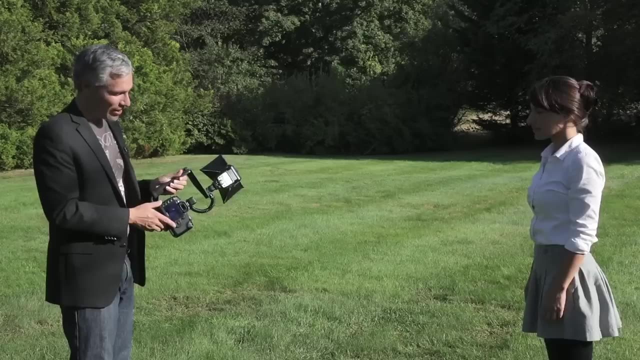 perfectly. now we're outside to talk about some of the challenges of taking pictures in the sun, especially with flash. so i have this fancy get up here which is kind of my standard outdoor flash setup. i just have a like a $12 bracket and a $10 flash cord. 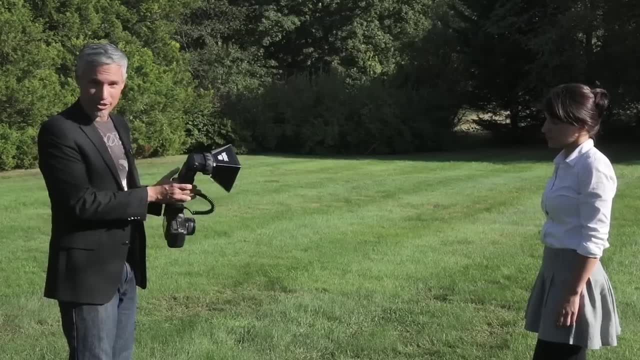 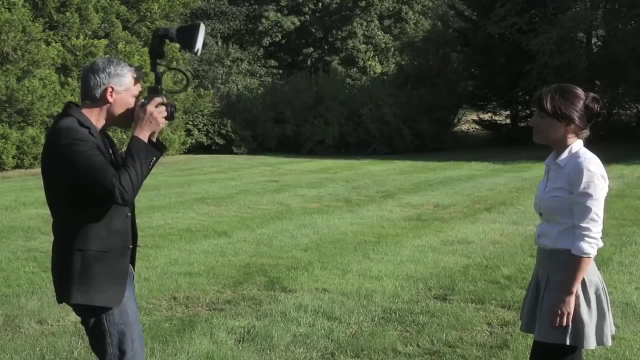 and then a $10 little softbox on top. but for now i'm going to keep the flash turned off and i'm just going to take this picture of chelsea in automatic mode so we can see what the natural light is like. so those pictures are okay, but there's a real. 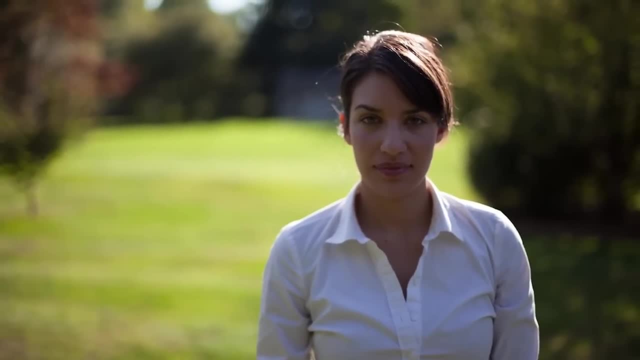 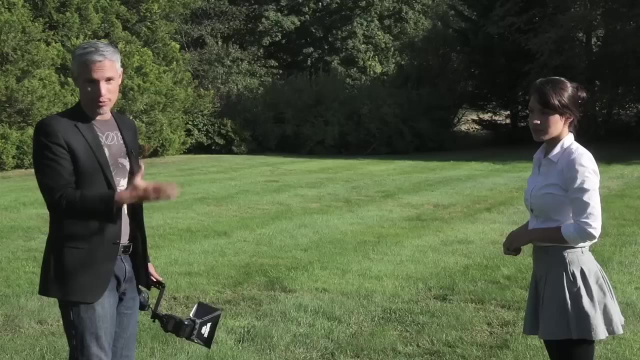 problem in that her back is to the sun, so her face is completely in shadow. the background is really really bright and her face is really really dark. and i have a couple of choices. i could expose the background properly, even though she'd be dark. it doesn't look good. i could raise the. 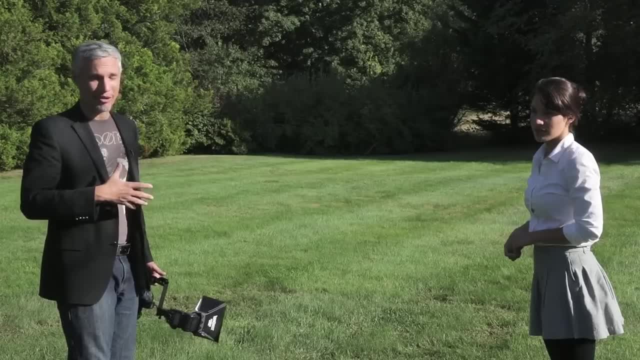 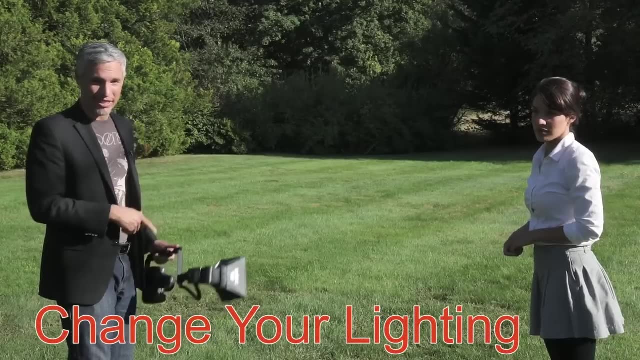 whole exposure so that her face is nice and bright, but then the background is going to be completely blown out. there's no great answer except for changing the light, and you can do that really easily with the flash. so i'll just turn my flash on in fully. 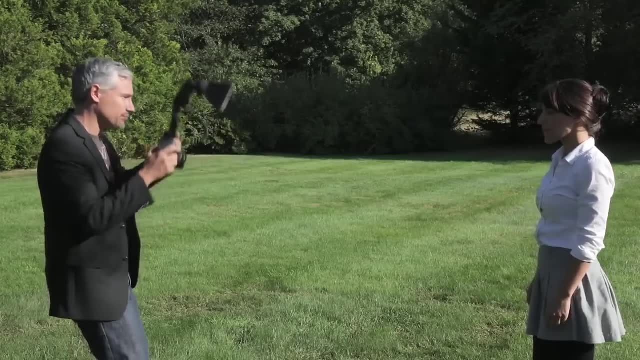 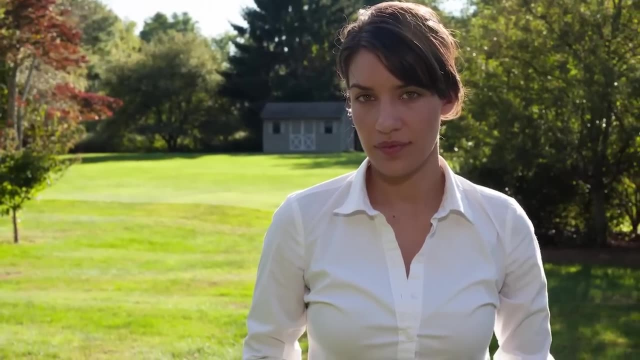 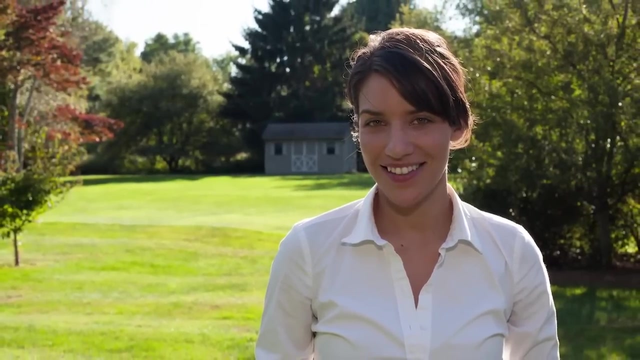 automatic mode and we'll take another picture. so in fully automatic mode, the camera properly balanced the foreground using flash with the ambient light in the background. it's pretty amazing what TTL can do. the flash puts out a little bit of light and the camera reads it as it's coming back. 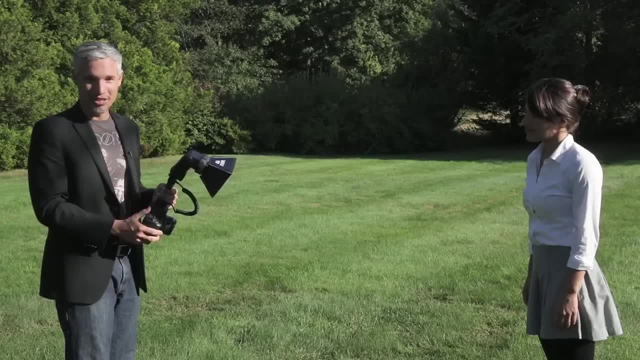 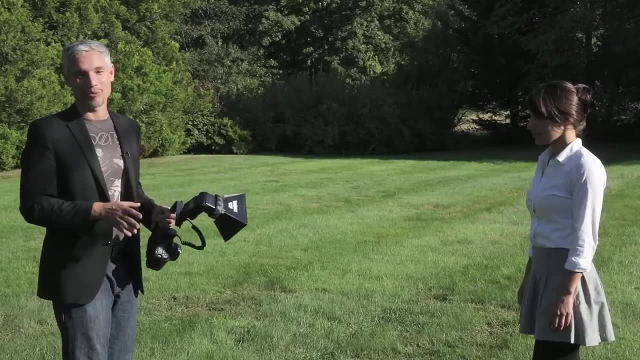 through the lens. this all happens before you actually take the picture and then the camera balances the background light from the sun with the light from the flash, properly exposing Chelsea and the background. pretty cool. but there is a problem you'll notice if you look at the background. 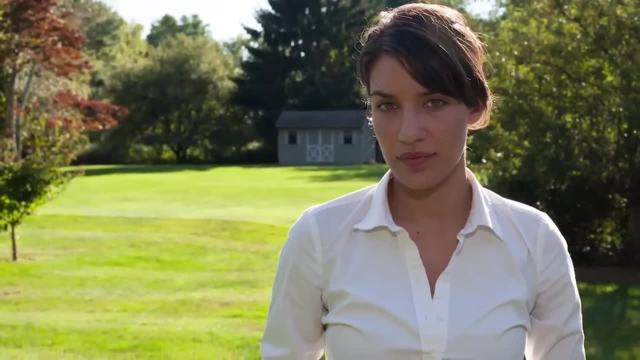 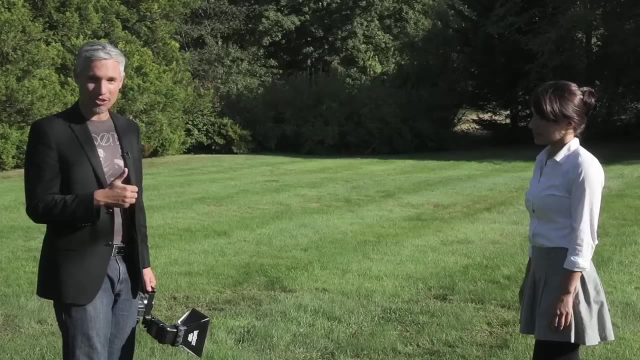 in the first picture i took versus the background in the automatic picture. suddenly my neighbors shed became completely sharp and in focus. that happened because the camera in automatic mode raised my aperture. i started out at f1.4, which is a really wide aperture, a really low. 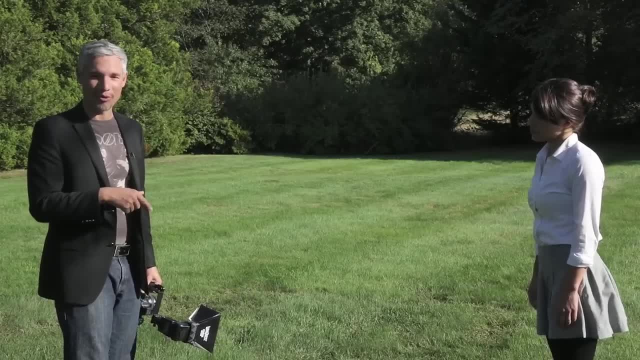 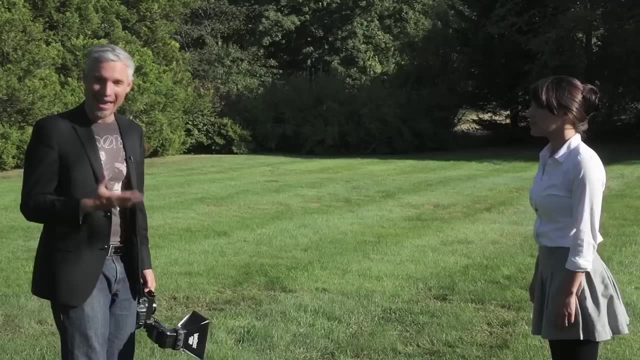 f-stop number to blur the background. remember, a low f-stop number means low background sharpness and i do want that background blurred. now, when i put it in automatic mode, it had to change my settings. it had to raise the f-stop number in order to sync. 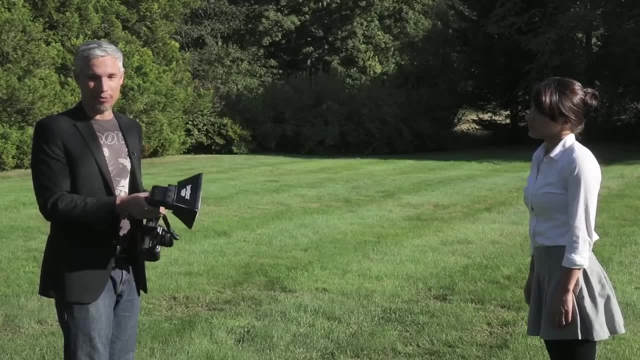 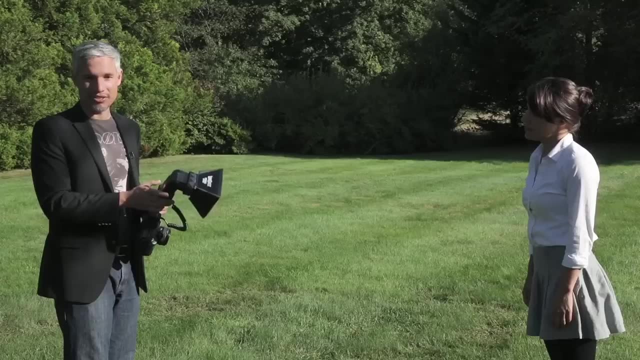 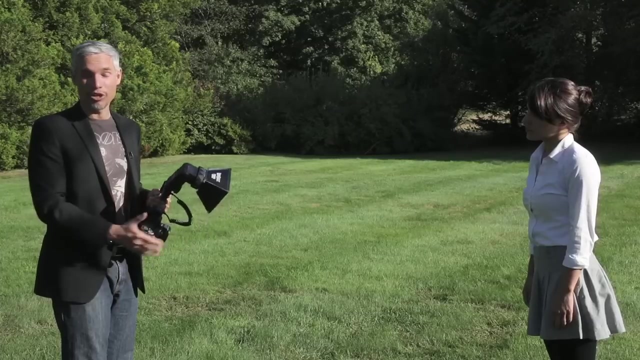 with this flash. every flash has a maximum sync speed and that's the fastest shutter speed you can use with the flash and this camera and flash combination can sync at 1 200th of a second. but in full daylight that's a fairly slow shutter speed. it was shooting. 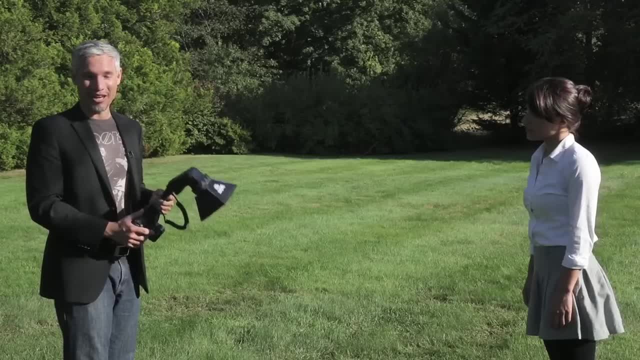 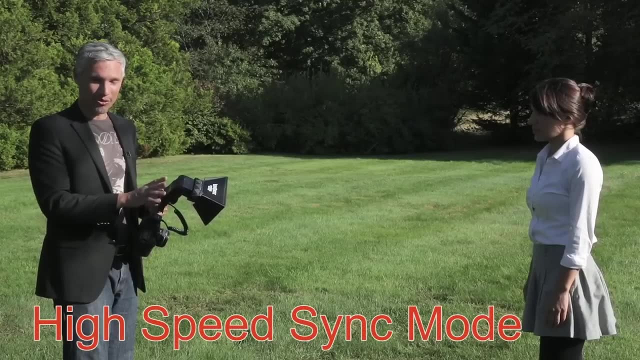 at 1 3000th of a second without the flash turned on. so if i'm going to shoot at that fast of a shutter speed with flash, i need to turn on high speed sync. so i'll do that now and take another picture of Chelsea at 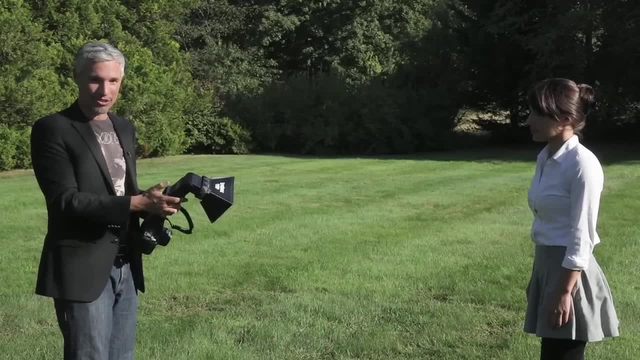 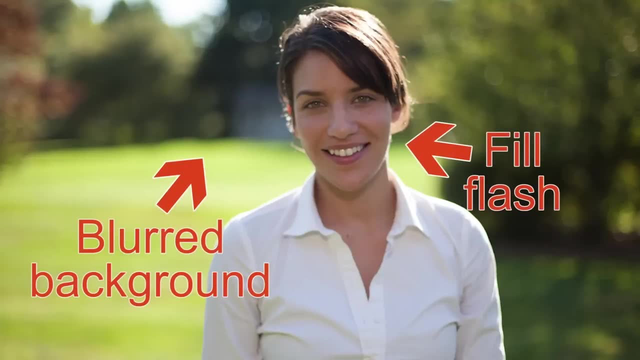 1, 3000th at f1.4 and with the flash in high speed sync mode. now, looking at that picture, it looks pretty good. the house is nicely blurred in the background, Chelsea's exposure is good and that couldn't happen without high speed sync. 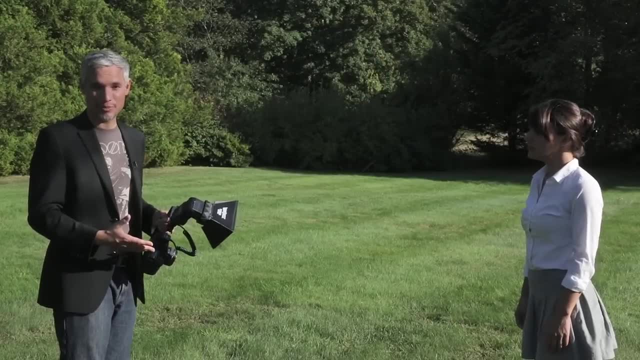 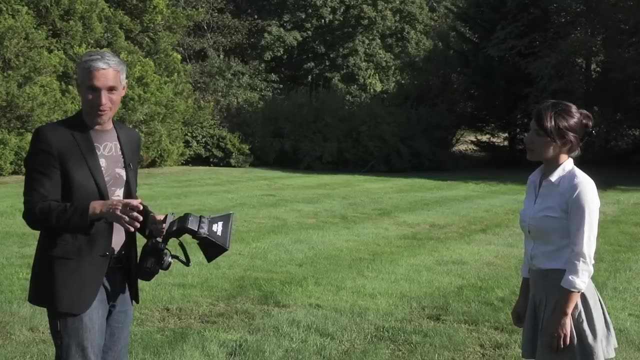 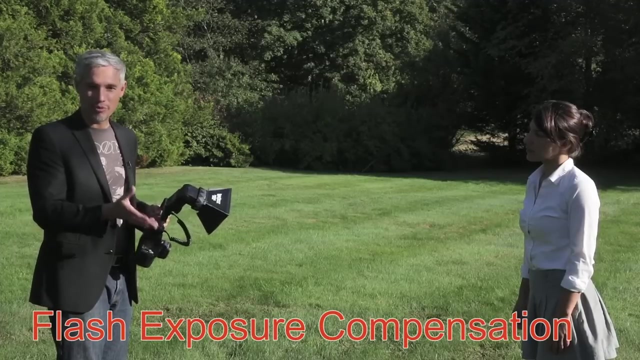 i also want to demonstrate using flash exposure compensation, because the flash is illuminating Chelsea and the sun is illuminating everything else. now i can't turn the sun up or down, but i can control the foreground lighting here with flash exposure compensation. so what i'll do is i'll add three stops. 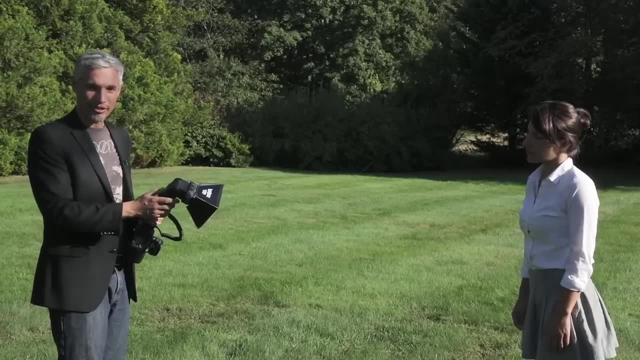 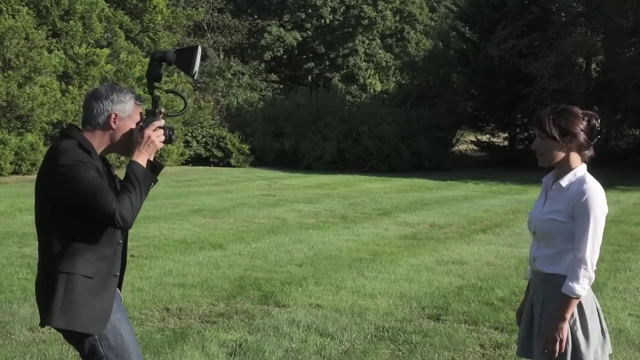 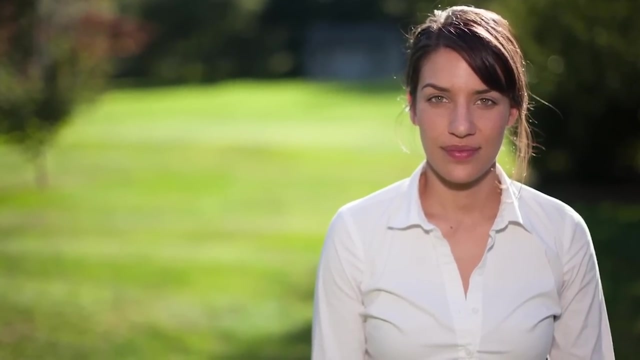 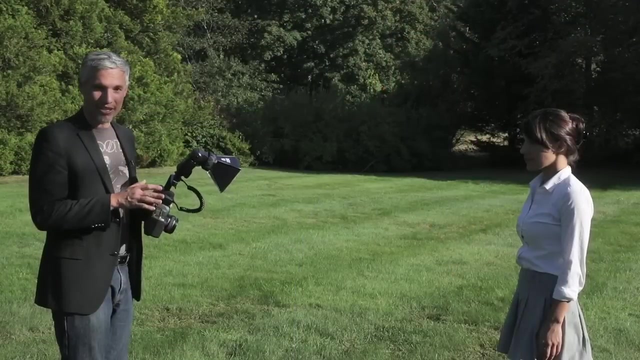 of light to illuminate Chelsea and then let the camera automatically expose the background. so i'll turn on flash exposure compensation and add three stops here and then take another shot. i switched my camera into manual mode and set it to 1 6000th of a second. this under. 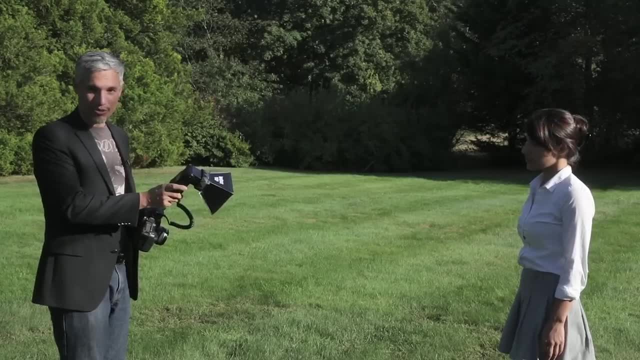 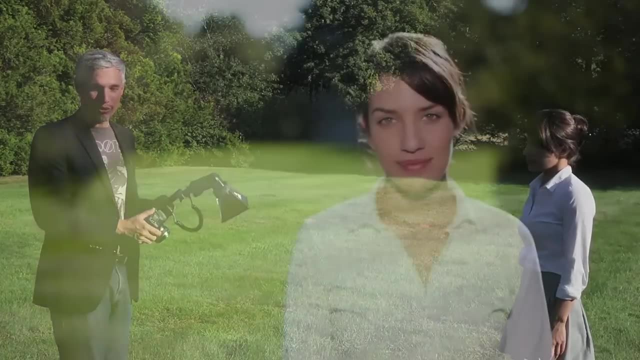 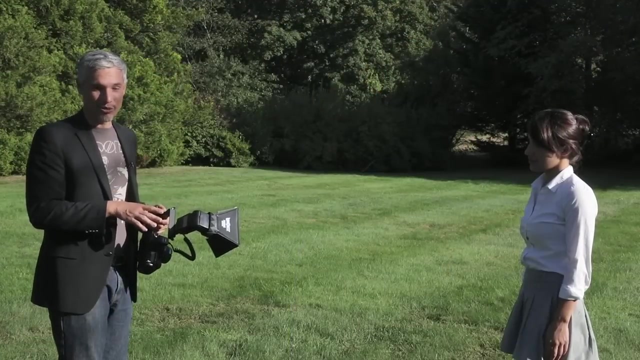 exposed the background by a stop. i then added flash exposure compensation to the flash so it was putting out more light. this properly exposed Chelsea, despite having an overall lower exposure. the way it adds up is the background became darker and Chelsea's exposure stayed the same. so in this way, 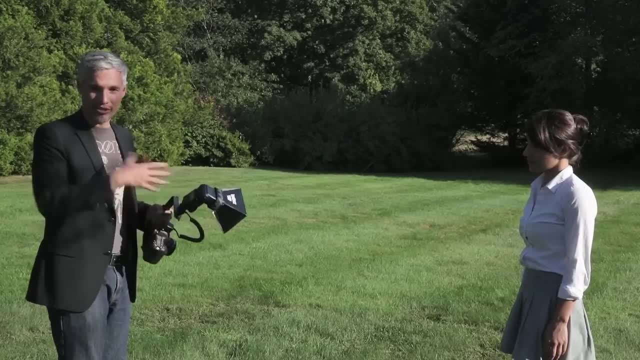 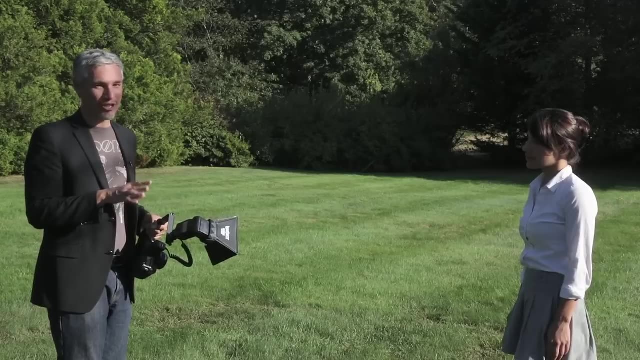 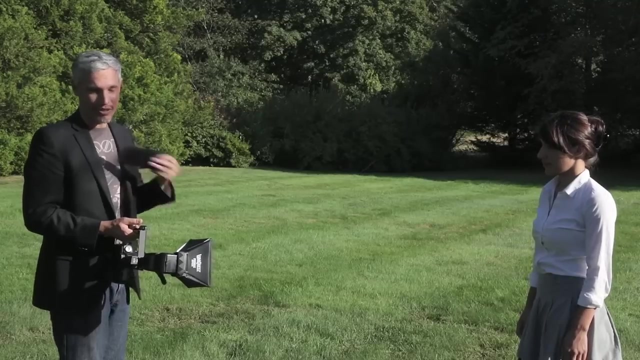 you can use flash exposure compensation outdoors to control the relative brightness of your foreground subject to your background subject. now i'm going to show you one more kind of fun trick that you can do using the same technique, by adding colored gels to your flash. so i'm going to pull out these. 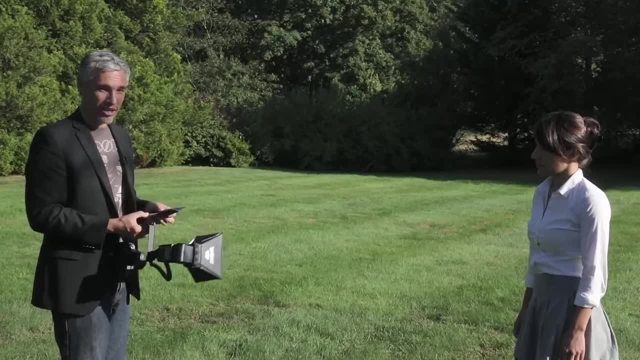 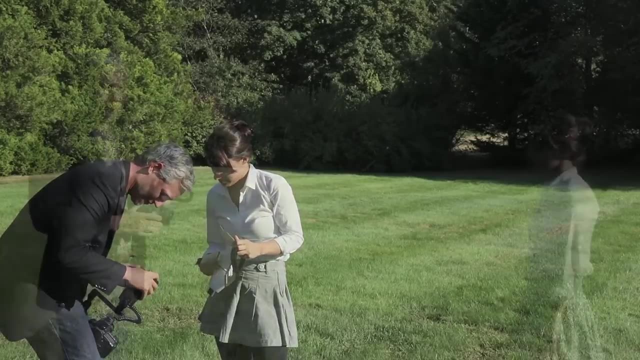 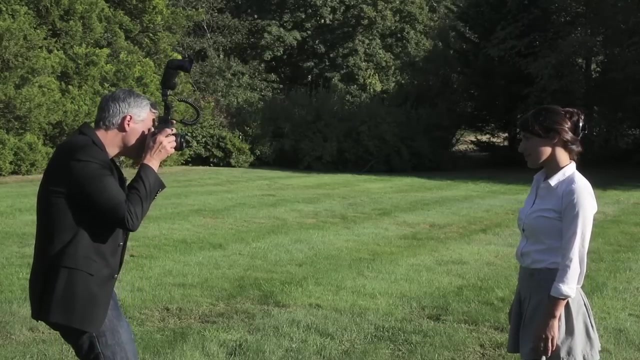 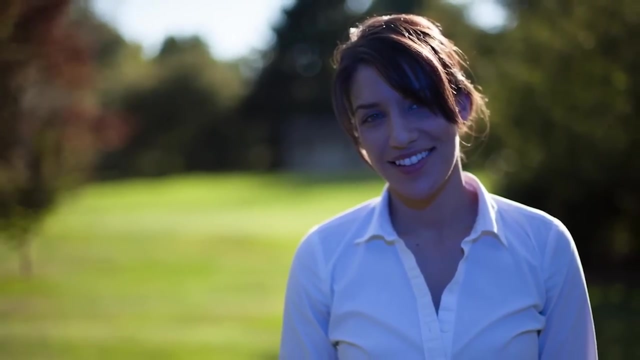 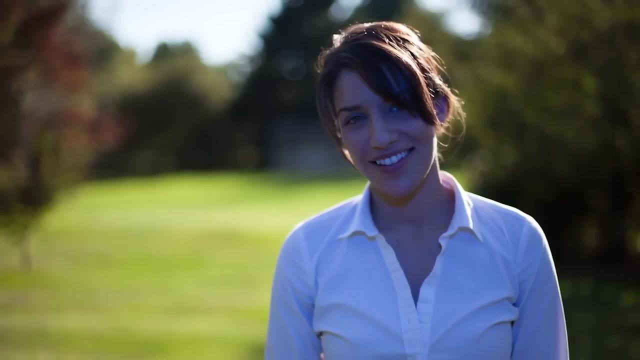 gels here and put a blue gel on the flash so you can see the effect with the blue gel attached. i'll take another picture of Chelsea, alright, so she looks suddenly very smurfy. right, she's very blue, and that's ridiculous. why would you want to do that? 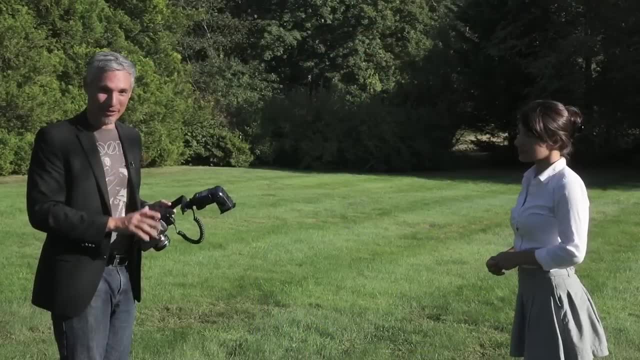 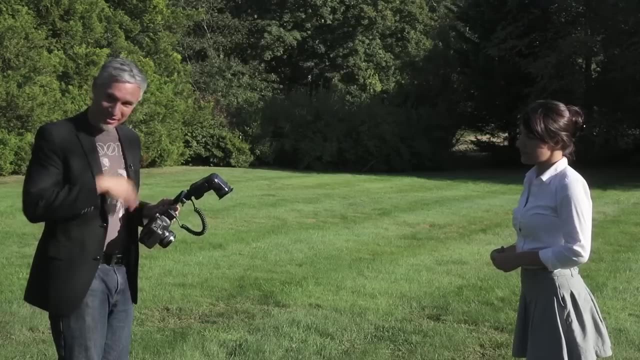 it can be a cool effect, though, because i'm going to correct for that blue color in camera by changing my white balance. so what i'm going to do is i'm going to select the coolest white balance, i'm going to go past the cloudy scenes and all the way to the coolest. 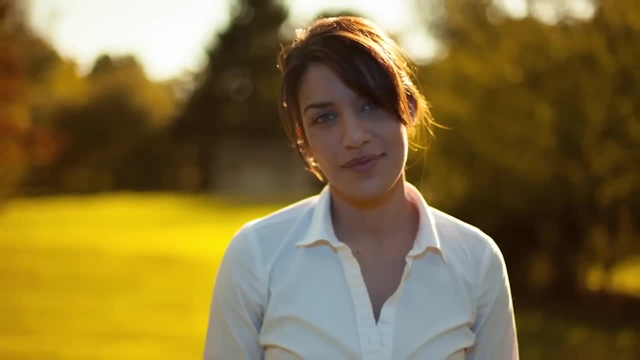 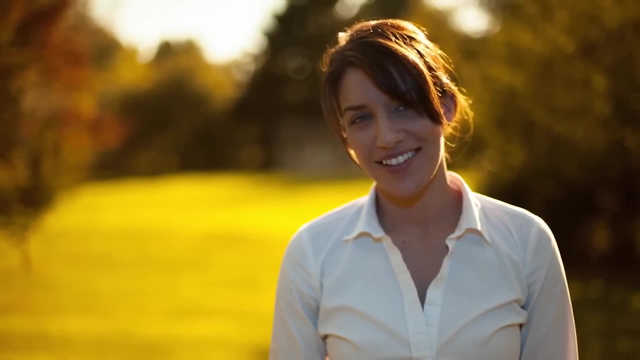 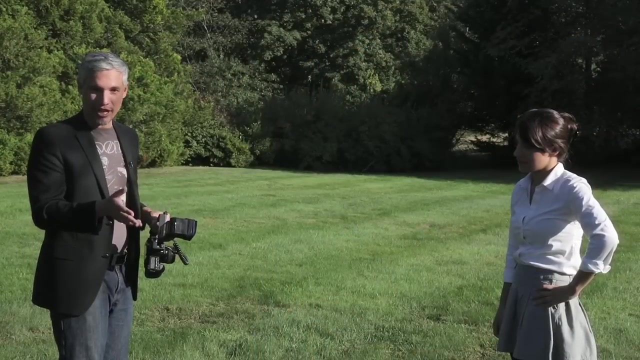 setting that it allows. with the white balance correction in camera and a little adjustment in post, Chelsea's skin tone will be back to normal, but that leaves the background completely warm and bright. you can reverse this by putting an orange gel or a red gel on the flash. 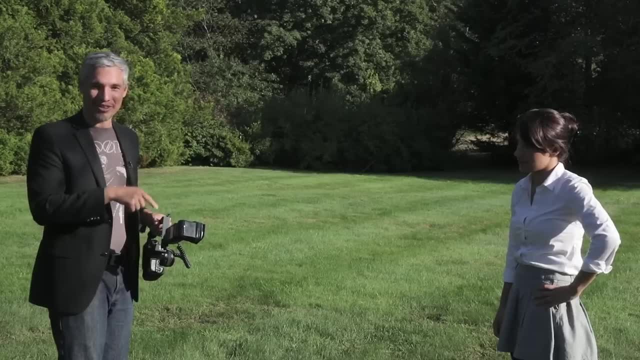 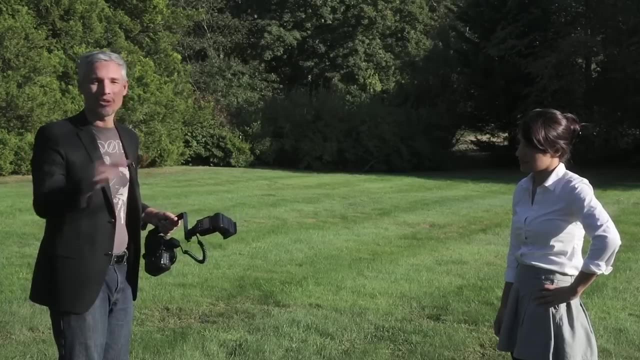 your foreground subject will be lit with that odd color, but you can correct that later or correct it using the white balance setting in your camera and then completely change the color of the background so you can have completely warm or completely cool backgrounds. whatever the effect is you want, it's not something you'll be doing every day. 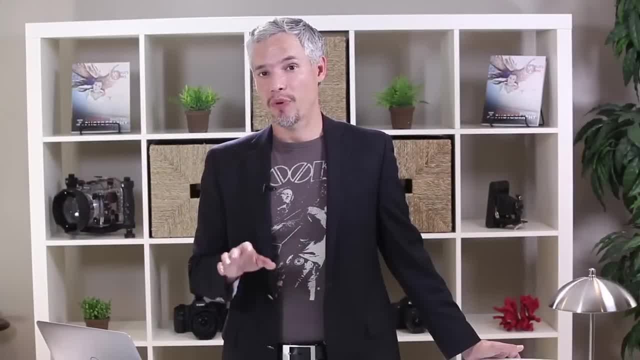 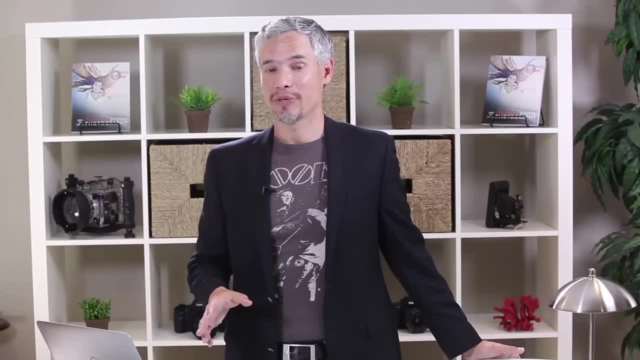 but it's a fun trick to try out once in a while. now i'm going to share some practices that i think you should try out on your own, because, after all, i can talk all day, but it's never going to be the same as getting out there with your. 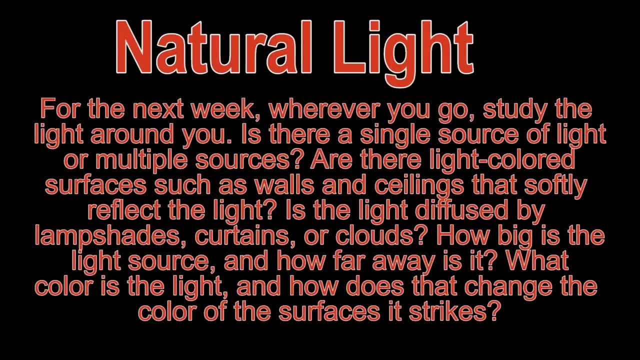 camera, so let's give these a try. the first practice is working with natural light for the next week. wherever you go, i want you to study the light around you. is there a single light source or are there multiple light sources? are there light colored surfaces such as walls? 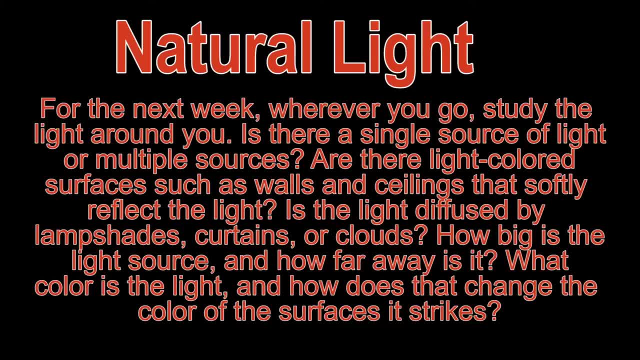 and ceilings that softly reflect and diffuse the light. if there's light that's diffused by lampshades, curtains or clouds, what effect is it having on the lighting in the room? how big are the light sources around you and how far away are they? are they? 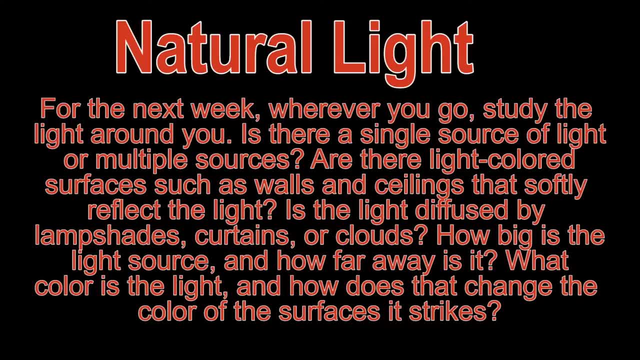 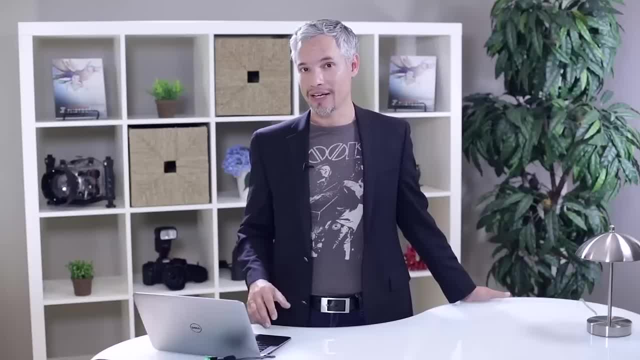 leading to the light being hard or soft. what color temperature is the light, and how does that change the color of the surfaces that it strikes? how might your eyes be adjusting for that? next, let's talk about understanding lighting and photographs. i want you to go back and look through your older 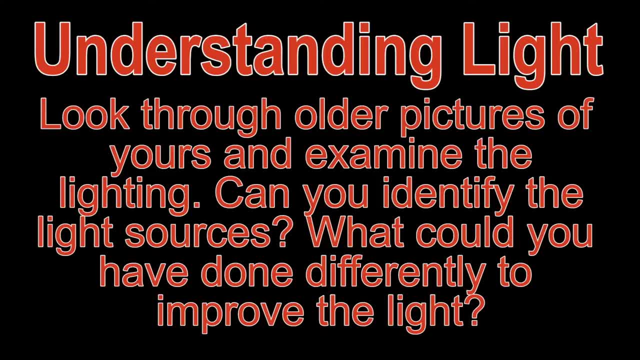 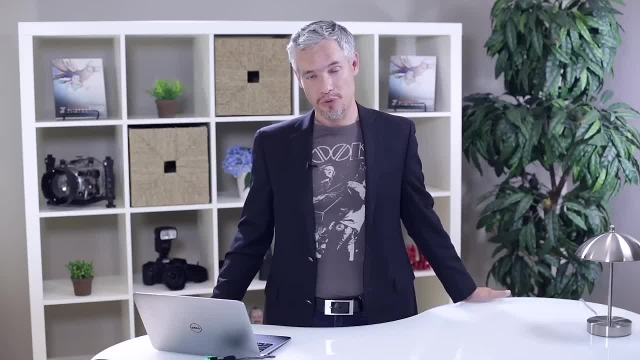 pictures and examine the lighting. from just looking at the pictures can you figure out what the light sources are? retroactively, hindsight is a 20- 20, of course. what could you have done to improve that lighting? now let's talk about hard and soft light. on a sunny day, take a picture of 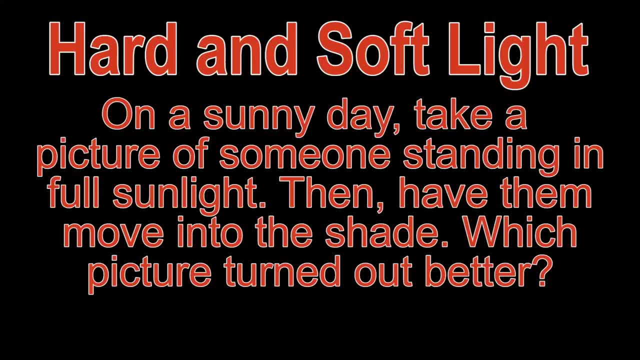 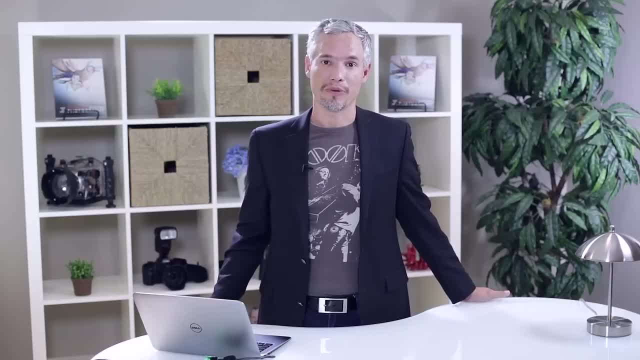 someone standing in full sunlight, then have them move into the shade. which one of those two turned out better? i'm going to go on a limb and guess the one in the shade, but it's important for you to experiment with that and learn for yourself. up next, i'd like you to practice using 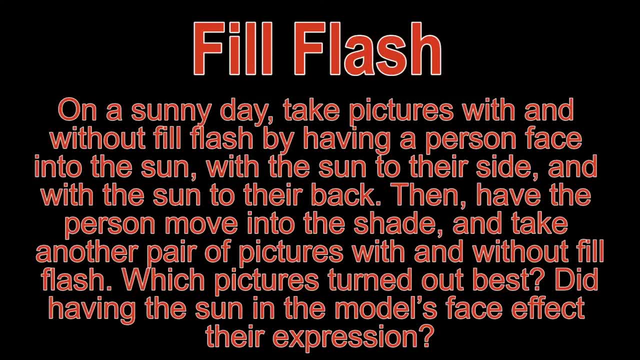 fill flash on a sunny day. take pictures both with and without. fill flash by having the person face into the sun, with the sun to their side and then with their sun to their back. then if the person moved into the shade, and take another pair of pictures, both with and 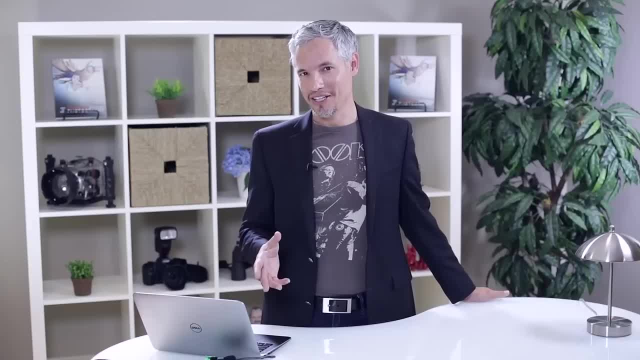 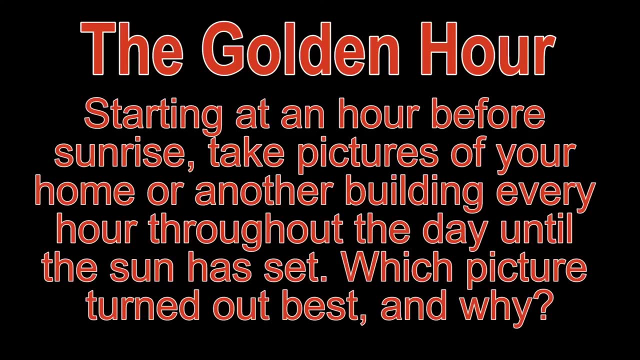 without fill flash. which pictures turned out best? did having the sun in the model's face affect their expression? might have made them squint a little bit. it's hard to look into the sun. now let's talk about the golden hour. i'd like you to start an hour before sunrise and take 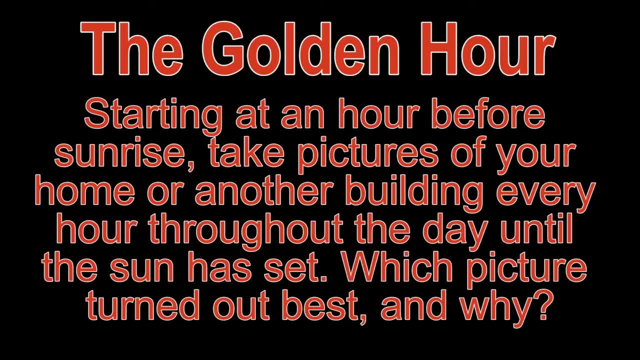 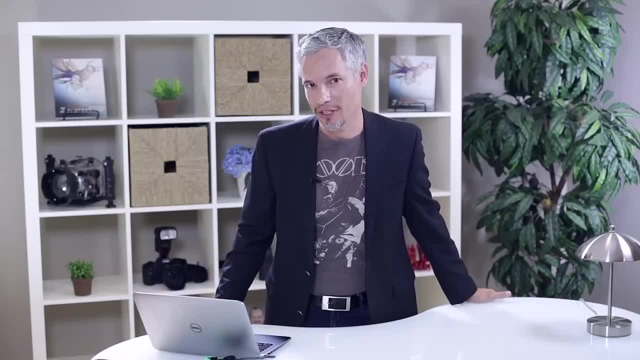 pictures of your home or another building every hour throughout the day, until the sun has set. which pictures turned out best and why? no, i don't expect you to go stand in the parking lot or the street all day, but if you do get up a little early, go take a picture. 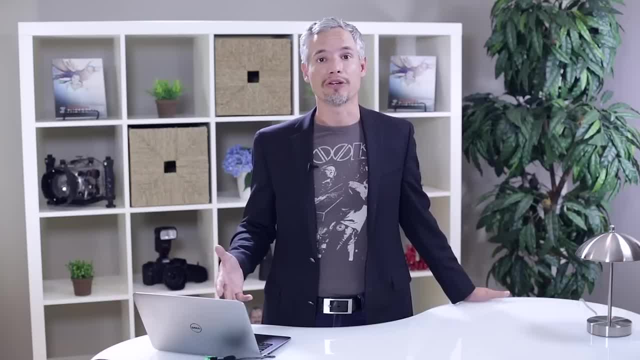 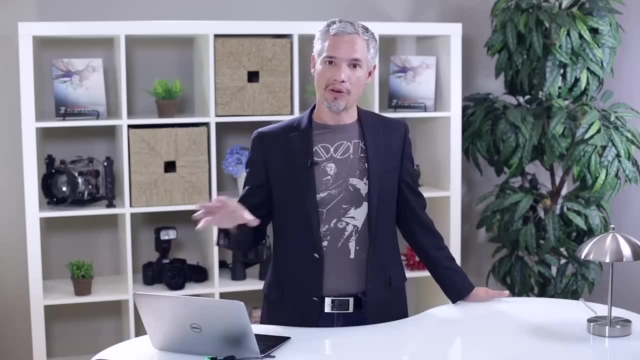 of the front of your house and then throughout the day, every hour or two, set a reminder to yourself. just run outside and take another picture. doesn't have to be the exact same spot, but you can flip through later and see how the lighting changed throughout the day. go through the whole. 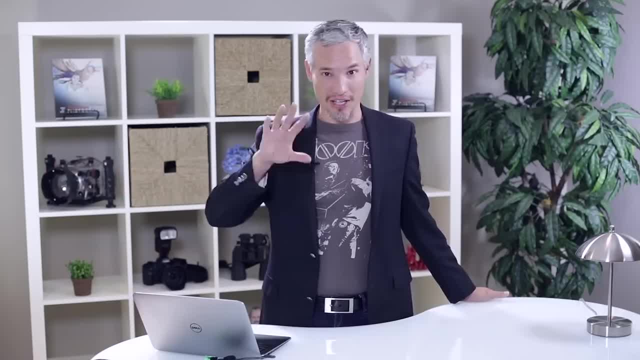 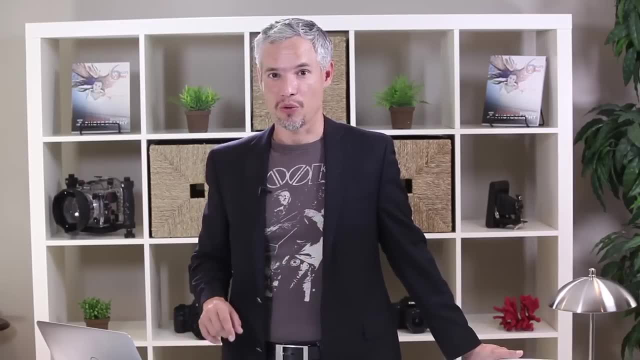 day, because sunrise and sunset are similar, but the sun is in different positions, so you're going to get different shadows, different textures and an entirely different feel. now here's a practice for using white balance. i'd like you to override your camera's automatic white balance by. 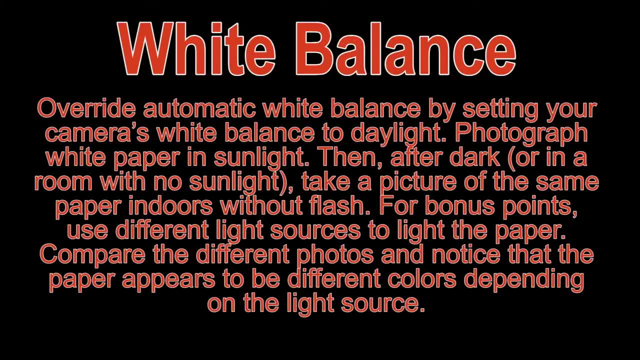 setting it to daylight. you have to check your camera's manual to learn precisely how to do that. now go outside in the sun and take a picture of white paper. now go into a room with no sunlight and take a picture of that same paper without using flash. 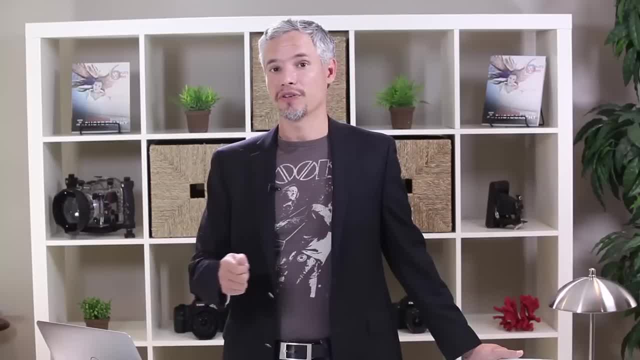 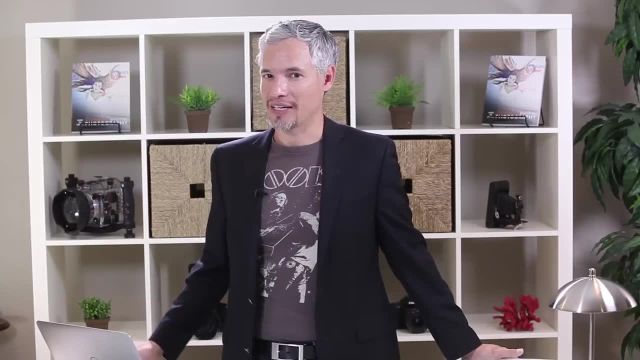 take that same paper and move into different rooms, put it under different light sources, try to find an led light and an incandescent light, a fluorescent light, a halogen light and, with your camera- still on daylight- white balance, see how that color of the picture changes. i bet you'll recognize. 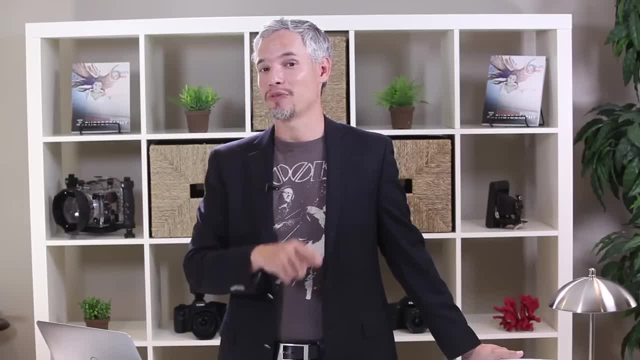 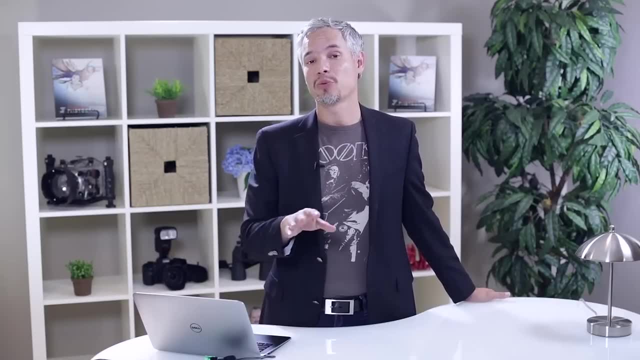 that odd color tint in some of your older photos taken before you understood how white balance worked. now i'd like you to head to a museum. it could be a virtual museum on the internet. i just want you to look at some paintings. in particular, i want you to research the paintings of: 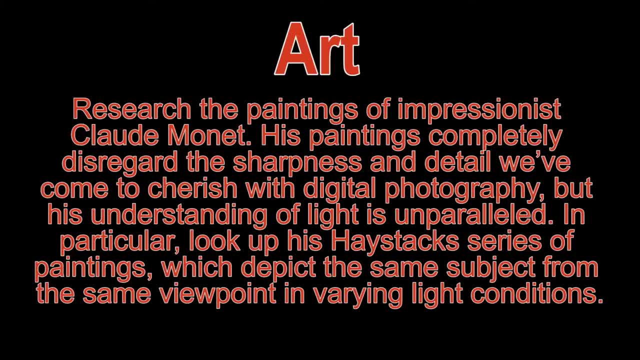 impressionist claude monet. i love claude monet because he has absolutely no regard for detail, and i think that's something a lot of digital photographers pay way too much attention to. in particular, i want you to look up his haystacks series of paintings you can. 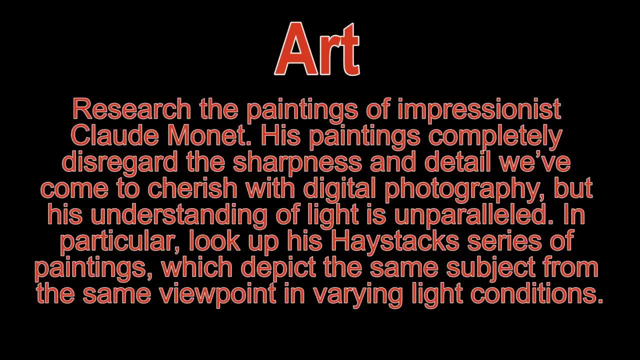 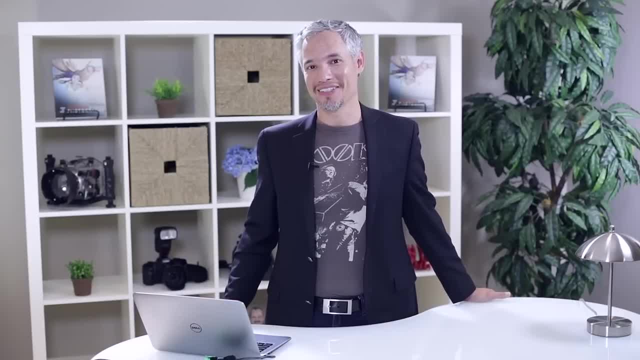 just google it and it'll come up. they depict the same subject from the same viewpoint in varying light conditions, and it's a really interesting study. it's oddly similar to that practice i just suggested for you. now here's a practice for working in outdoor light. i'd like you to pick a. 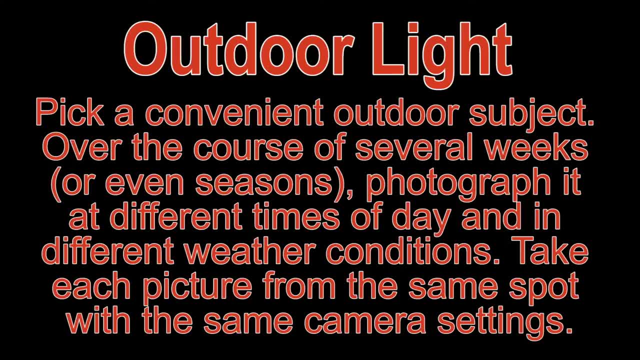 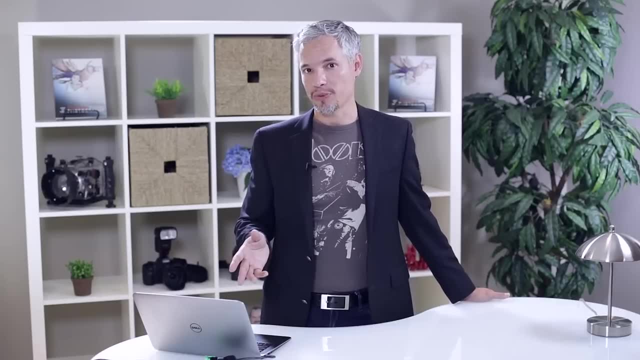 convenient outdoor subject such as your house, and, over the course of several weeks or even throughout an entire year, multiple seasons, photograph it at different times of day and in different weather conditions. take each picture from the same spot with the same camera settings. you can allow auto exposure to work. 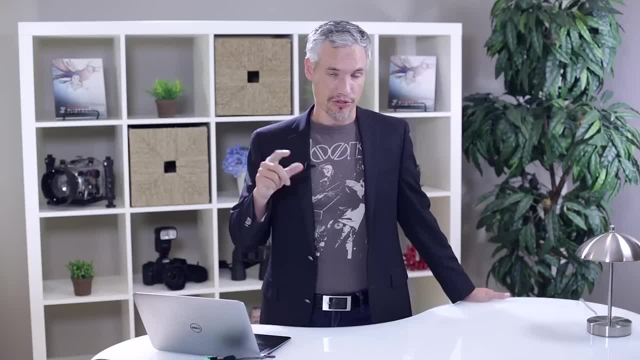 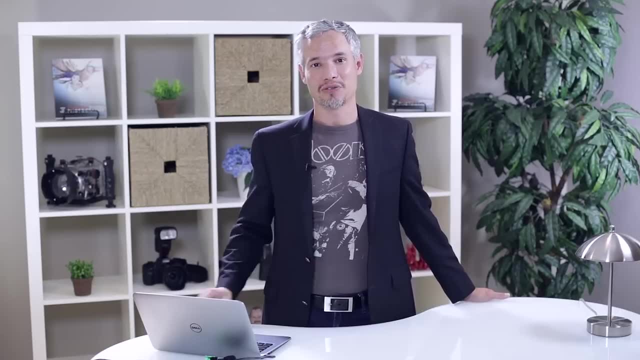 i would just suggest using aperture priority so that your camera doesn't change the depth of field. all this is going to do is give you a sense for how timing changes the conditions around you. thanks so much for joining me in this discussion of light, and i hope to see you. 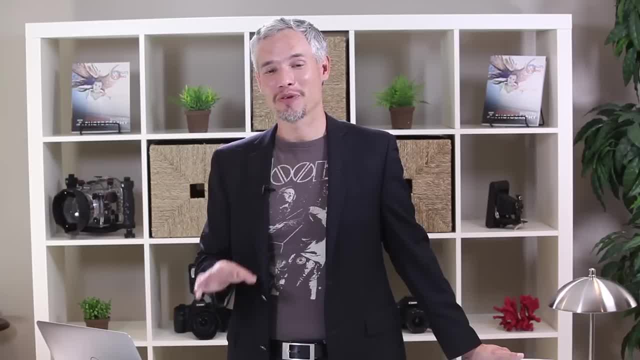 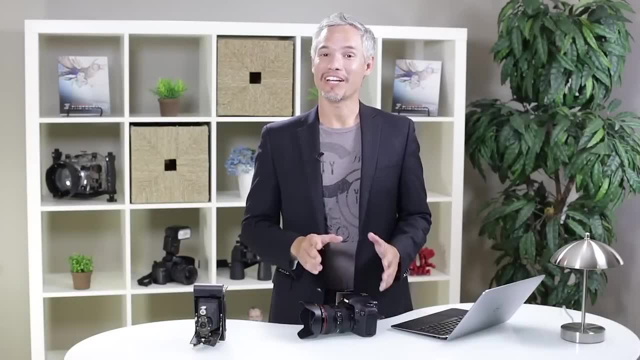 in future videos. once again, i'm tony northrup for the stunning digital photography video training series. hi, i'm tony northrup and for the stunning digital photography video training series. i'm going to talk about controlling your camera and i'm going to start by going over the 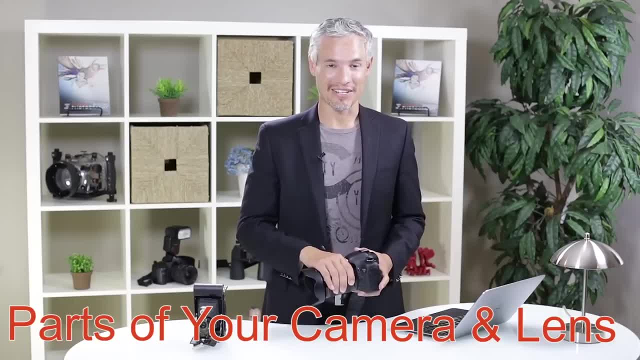 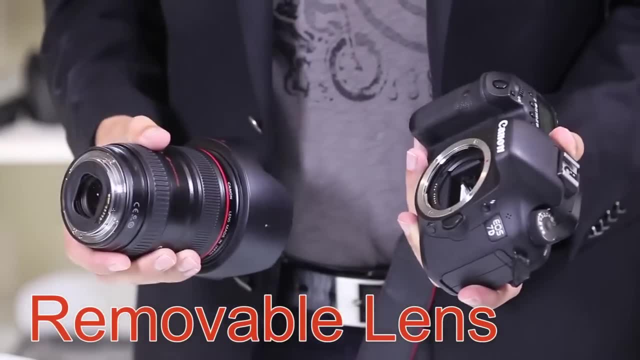 major parts of the camera and lens. so, like with any interchangeable lens camera, slrs have a removable lens, and this is one of the most powerful features, because you can take off the kit lens that comes with your camera and put on a telephoto lens for wildlife. 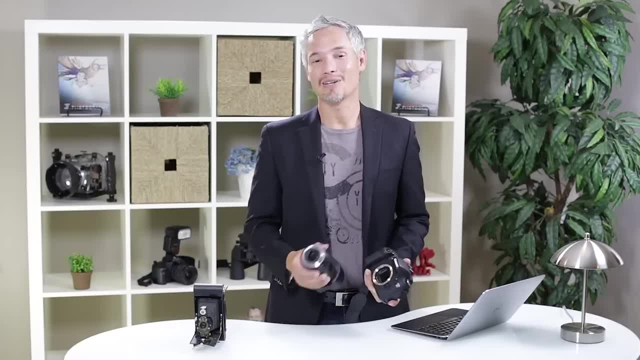 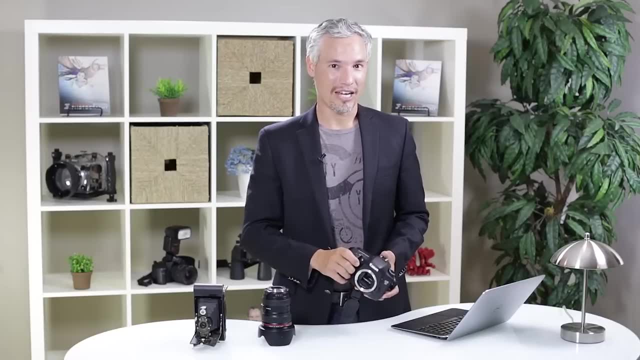 or a portrait lens for taking pictures of your family. the possibilities are really endless. so i'm going to take off this lens and we can go over some of the individual features on the outside of the camera body up. first, we have the mode dial here, and different cameras will have different 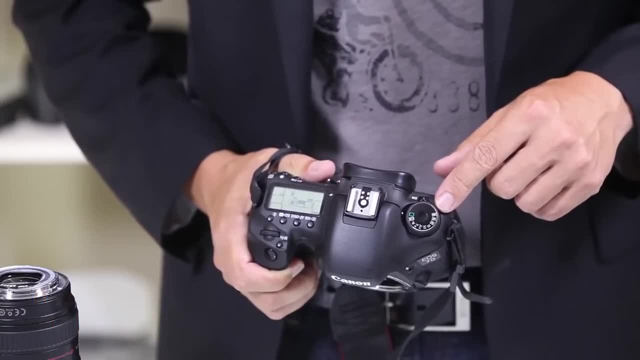 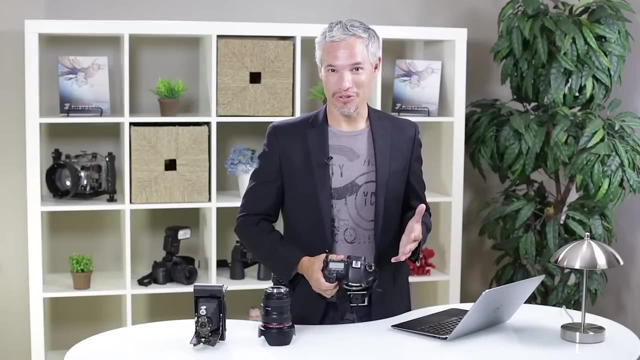 modes available. this is the fairly high-end camera, a canon 7d, so you can see it doesn't have the little running guy that indicates a sports mode or the portrait phase that you're supposed to use for portraiture. no, it's limited to the creative modes. 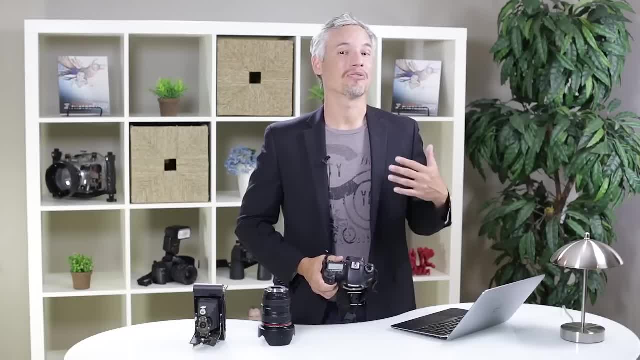 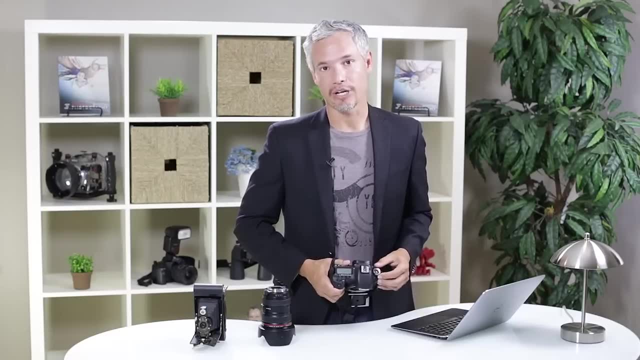 and these are the modes you're going to be spending all your time on, now that you know how to use the camera, how to use your camera. so the major modes are usually a green box of some kind, which indicates the camera is operating in fully automatic mode. 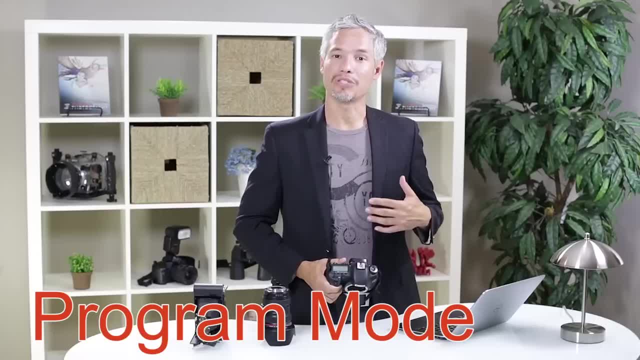 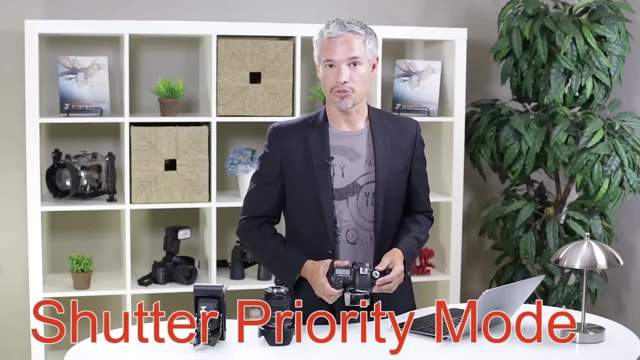 and then there's usually a program mode which allows you to take some control but still allows the camera to make most of your decisions. then you'll have shutter priority, which allows you to control the shutter speed by using the main dial. here the main dial is right next to the 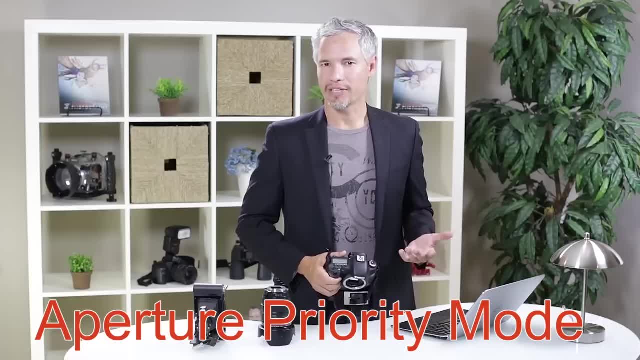 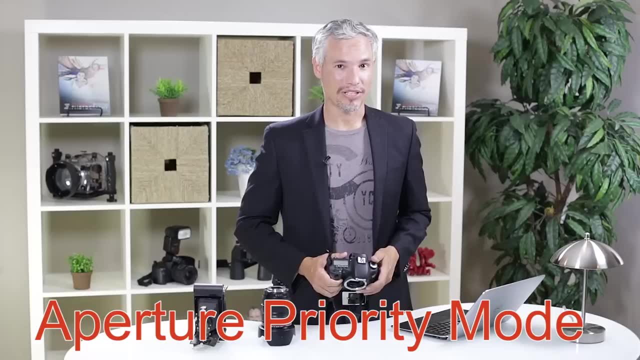 shutter button up. next you'll have aperture priority. on canon cameras, this is av, and on nikon's and the it's. simply a aperture priority gives you control over the aperture and lets the camera set the shutter speed automatically. aperture priority lets you control the depth of field, and it's. 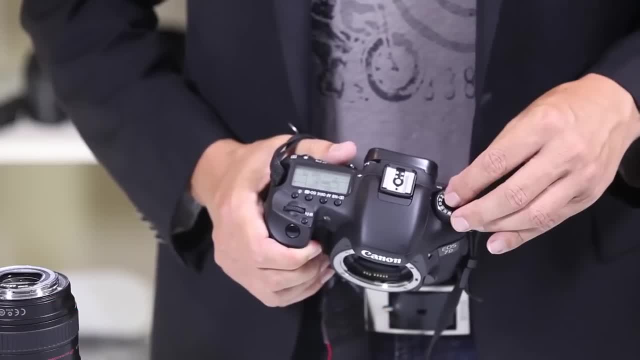 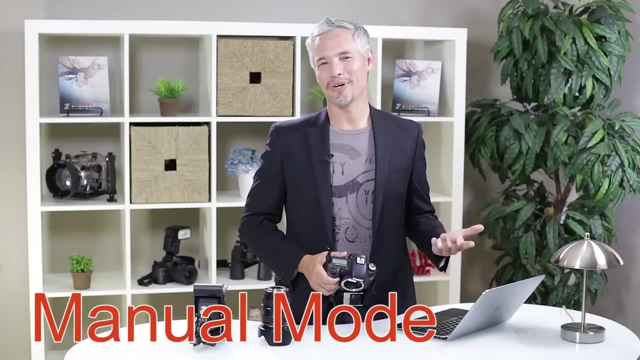 the mode that i use almost all the time. the last major mode is the manual mode and this gives you complete control over the shutter speed and the aperture. manual mode is this kind of like bougie mode that artistic people talk about using all the time, but realistically. 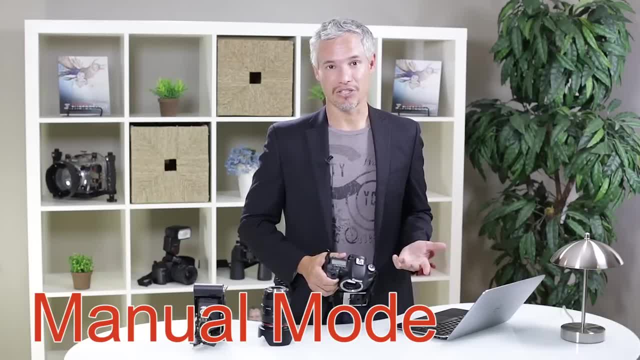 pros use shutter priority or aperture priority, depending on the conditions. one nice thing about modern cameras with manual mode is you can use them with auto iso, which lets you auto exposure pictures even when you take complete control of both the shutter and the aperture. i'm giving you a lot right. 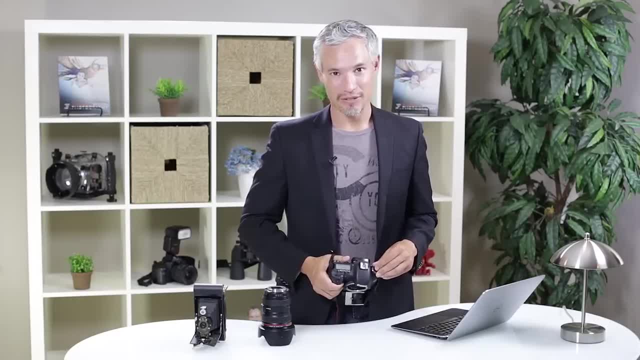 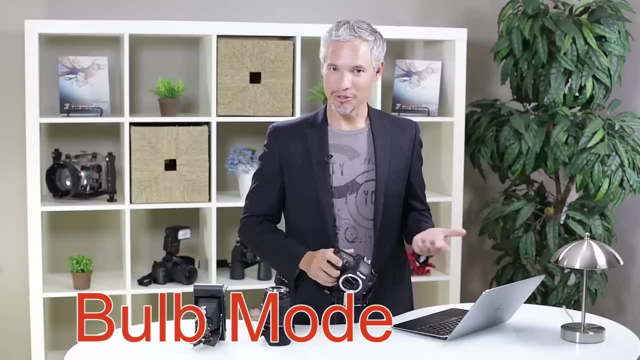 now, but don't worry, i'm going to demonstrate all this a little bit later on. the next major mode here is bulb mode, and bulb mode keeps the shutter open for as long as you hold the shutter button down, so you could take a 30 minute exposure if you wanted to. 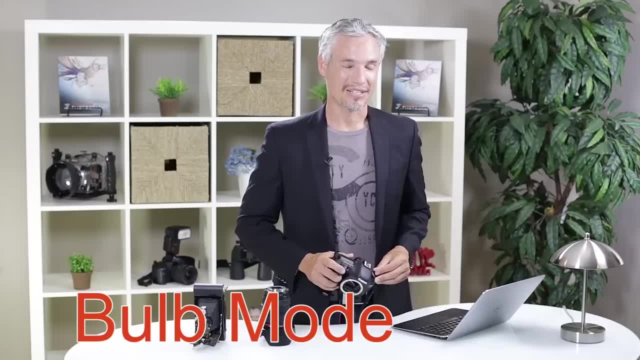 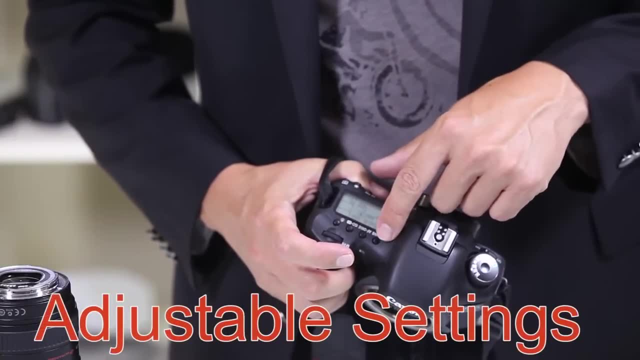 you'll usually use that in conjunction with a remote shutter release, but we'll cover that in the night photography live video lesson. this particular camera has controls for setting the metering mode, the white balance, the shutter speed, the iso, the flash exposure compensation and a few other things right on top as 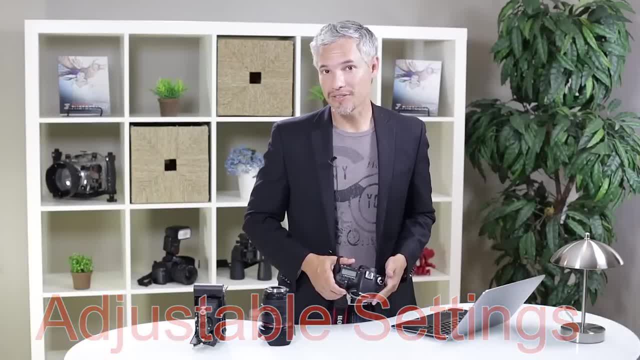 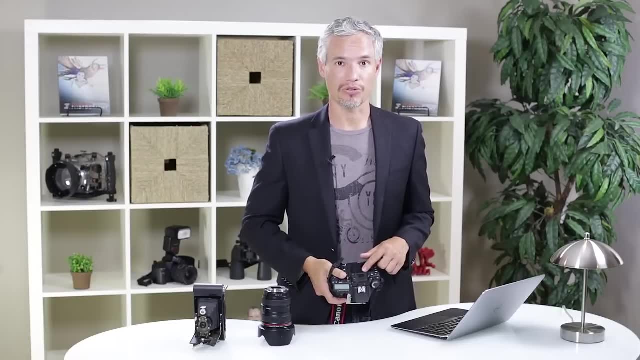 well as a display, but different cameras will have these settings in different places. there might be buttons for them, there might be dials, there might be a menu system that you have to navigate on the back of the camera to control those settings. so i can't tell you what your camera looks. 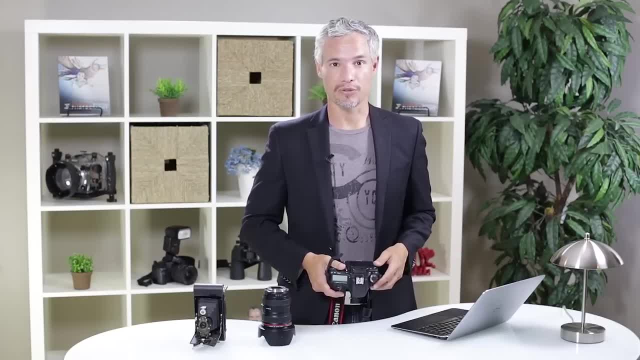 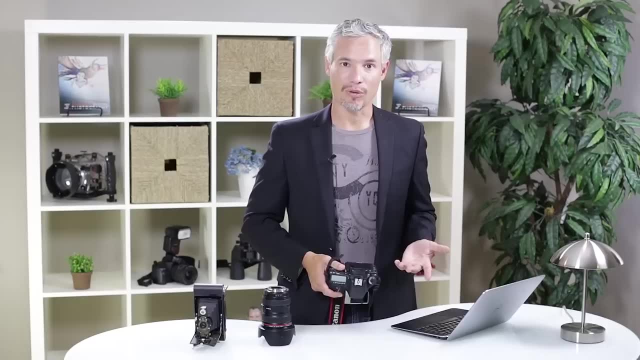 like, because there are too many cameras out there. so do check your camera's manual for the specifics of it, but rest assured, all major cameras, both mirrorless and dslr cameras, have these same capabilities that i'm going to be covering in this lesson. another feature that i want to point out: 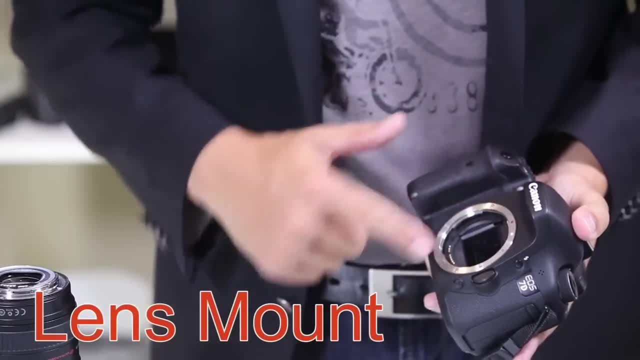 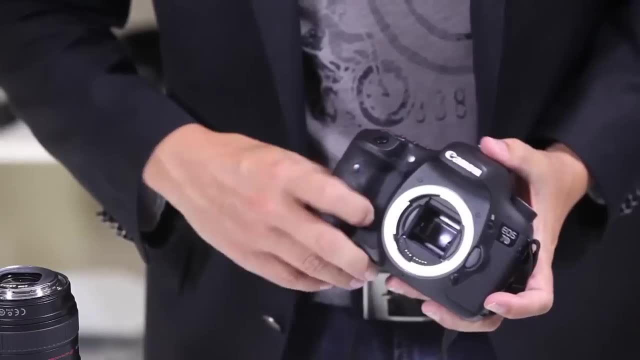 is the lens mount. here we're starting to look at the inside of the camera, but there's always a button on the side of the camera that releases the lens, so you hold that down and then twist the lens. the lens mount is made of plastic on the 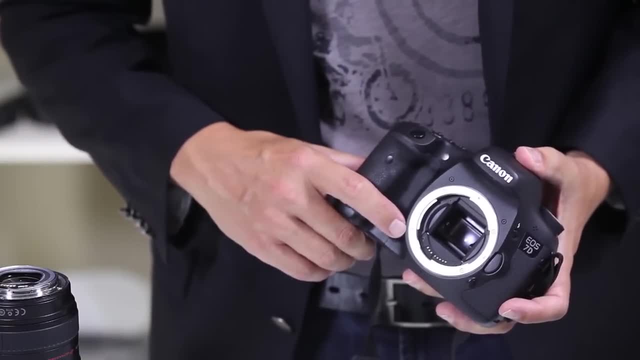 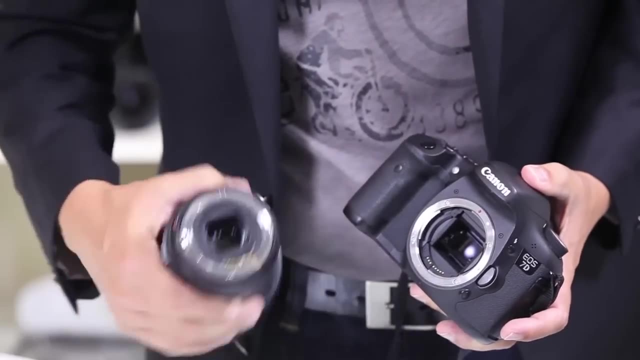 less expensive cameras and metal on the more expensive cameras, and it holds the lens firmly in place. you'll notice that it has markings- and to allow you to properly line up the lens, so the red dot here will line up with the red dot on the lens, allowing me to fit them together. 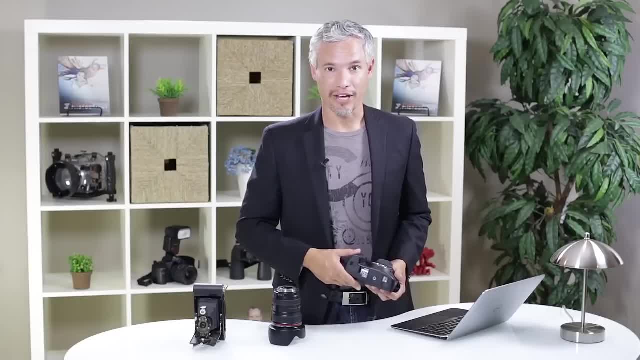 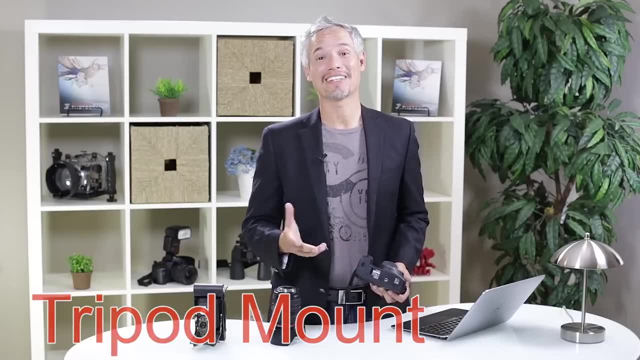 with a twist. another feature on the outside of the camera is the tripod mount. just about every modern camera has the tripod mount and they're threaded exactly the same. it's one of the few things that they've all managed to agree upon. so if you have a canon or a nikon or a 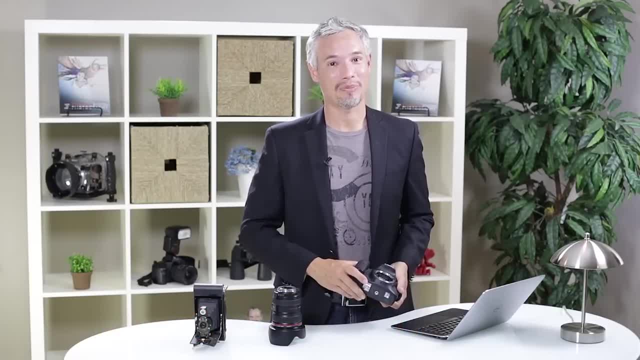 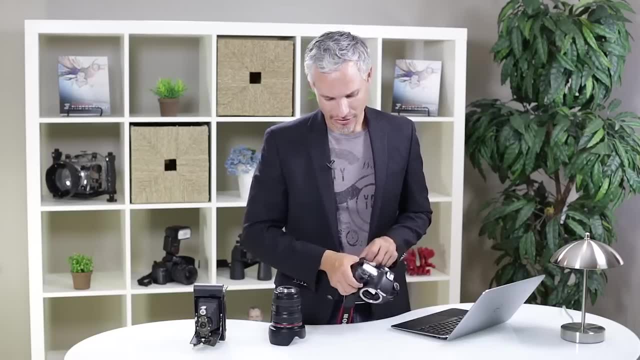 sony or olympus or whatever, you can use the exact same tripod, thank god. i wish they could do that with like lenses and flashes and stuff, but really it's just the tripod that fits universally. even the camera straps here can vary in width a little bit though. 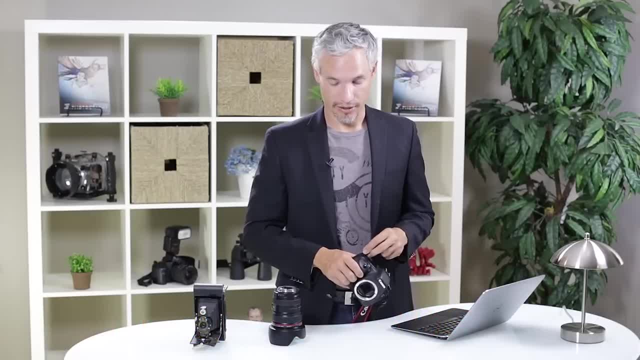 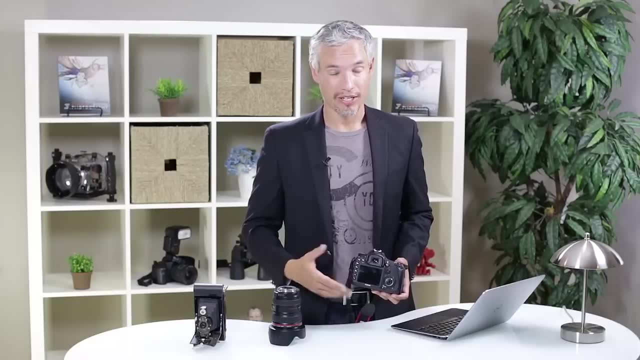 there are a lot of universal camera straps that you can buy that work just fine. the back of the camera tends to have quite a few different controls that you can use too, but again, this varies largely based on the camera model that you have. less expensive cameras will probably have. 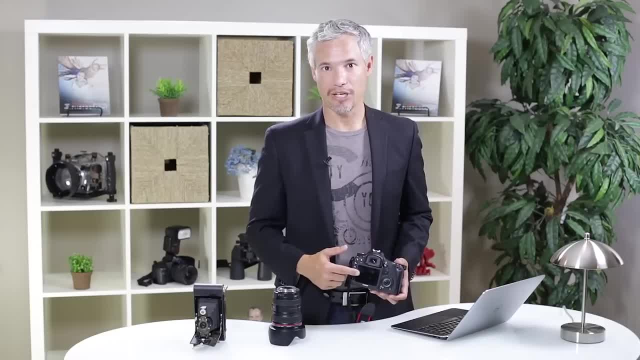 fewer controls and they'll require you to do more things by navigating the menu system. this is one of the big differences between the higher end cameras and the lower end cameras. the higher end cameras are just giving more buttons because they know that you'll want to adjust your exposure compensation by 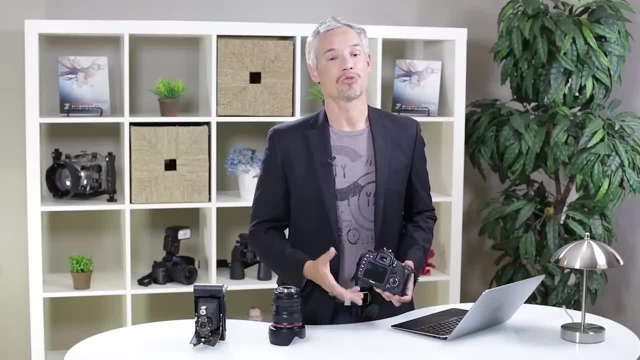 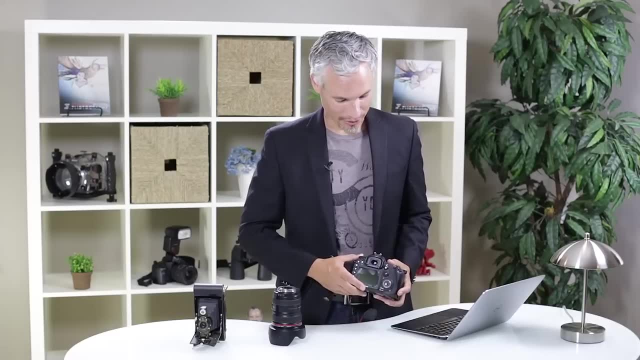 just moving this dial here. if you get a base model camera, you can still control your exposure compensation, but you'll need to press a couple of buttons and navigate a couple of menus to do it properly. so these higher end cameras: they simply allow you to get the settings that you need quicker. 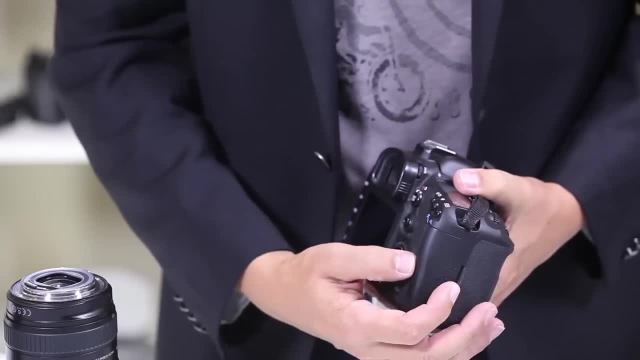 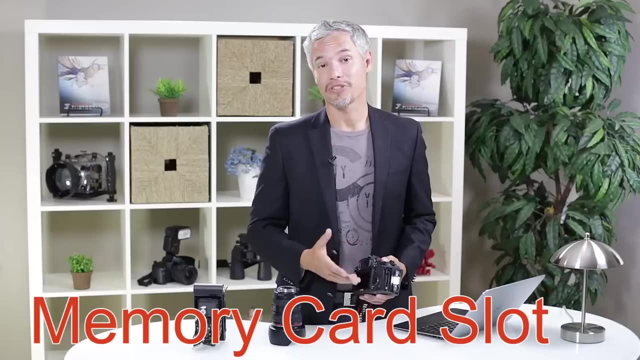 and they do it by providing more buttons. before we go to the inside of the camera, i'll just point out that every camera has a slot that stores the memory card, and some cameras will have multiple memory cards. there are different types of memory cards that you might use. this particular 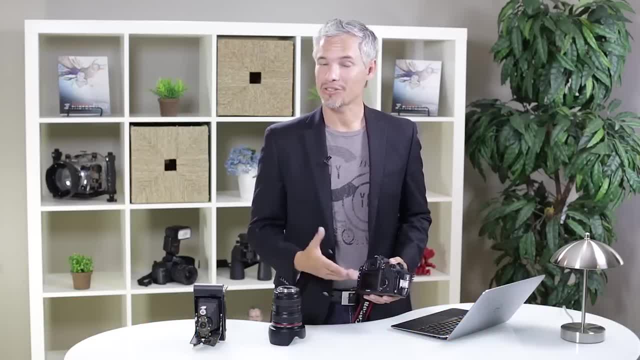 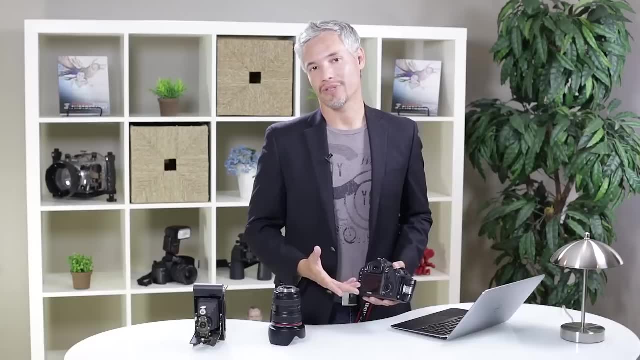 camera uses a cf card, which is a larger and faster card. it's a little more powerful, a little more durable. the lower end cameras will have sd cards or even micro sd cards, but truthfully, it doesn't matter that much. the point is that you can take out the. 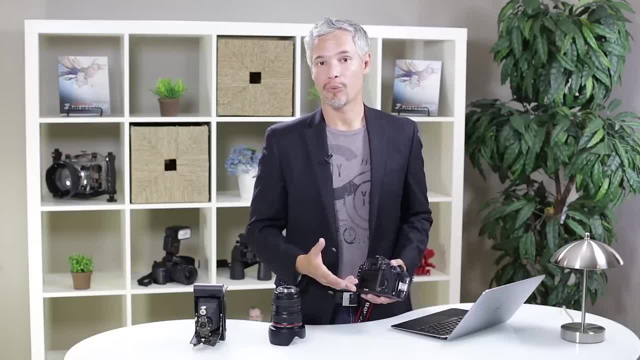 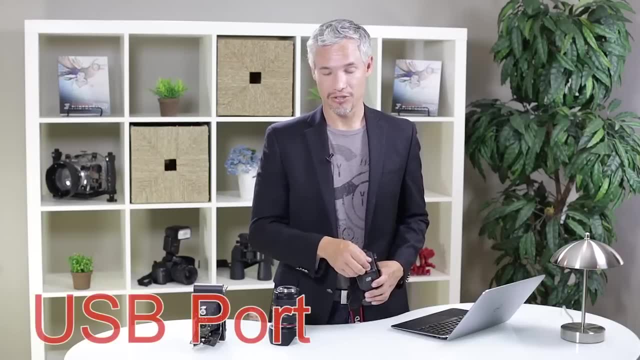 memory card and put it directly into your computer or a dedicated memory card reader to unload your pictures. another way to unload the pictures from the camera is to connect a usb cable directly to it. this usb port is often covered under some sort of plastic cover like this: 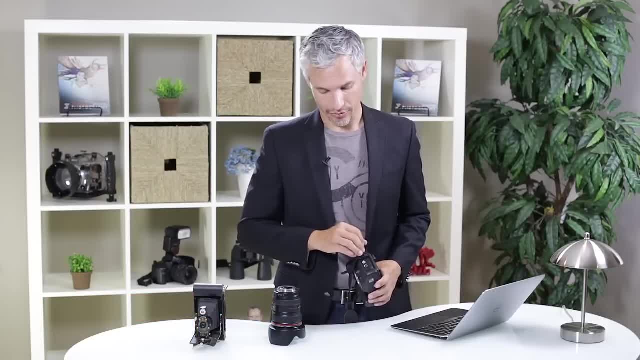 and that just prevents the rain and water from getting in, in case you take it out in the rain. so you can see the usb port here and it could plug a usb cable in here to unload the pictures or remotely control the camera. now the unique feature about slrs and 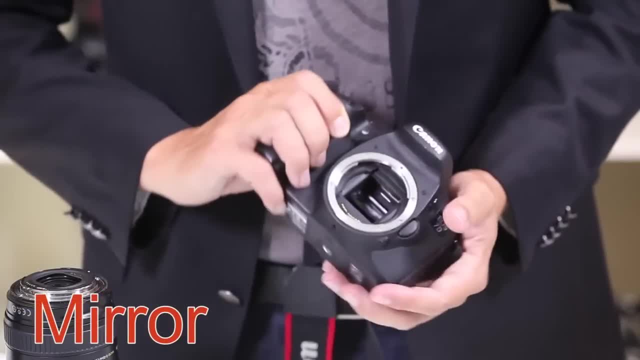 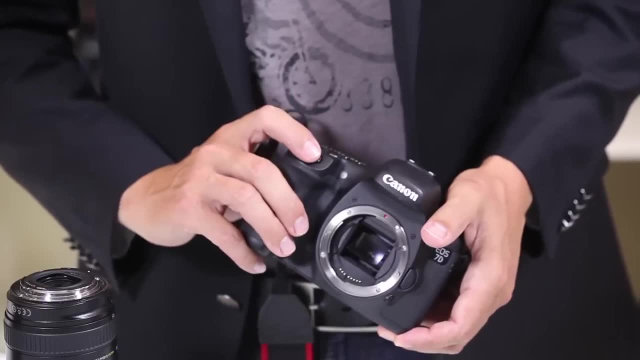 dslrs like this is the mirror in there, and so what you'll see here is this angled piece, and i'll move it up now when i press the shutter button. that piece that's moving is the mirror, and the mirror is the best and worst in the world. 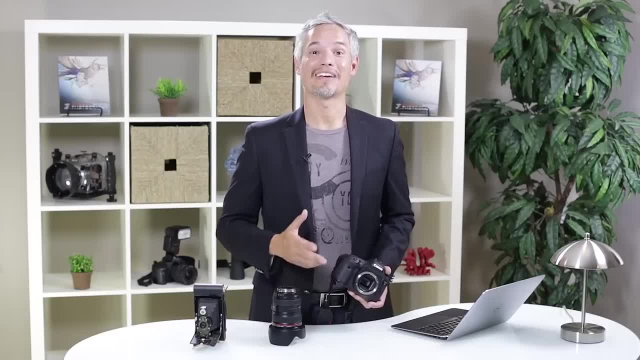 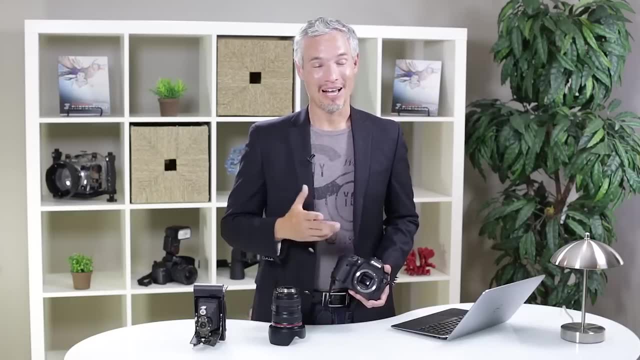 part of an slr. it's such a big deal that they created a whole line of cameras called mirrorless cameras that are exactly like slrs, except they lack that mirror. i personally, i love that mirror, but you can see just how much space it takes in there and that makes the 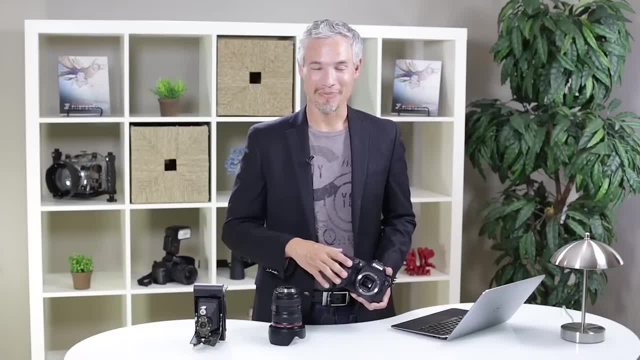 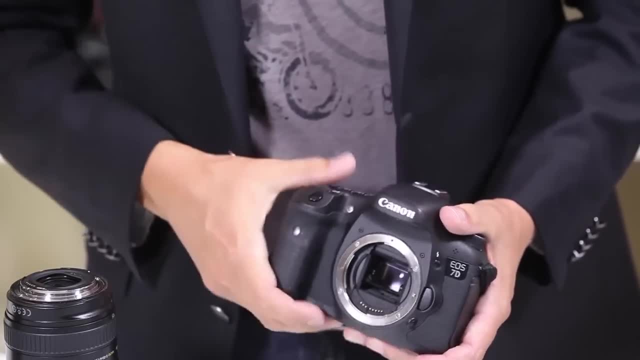 whole camera get bigger because you have to wedge this mirror in. what the mirror is doing is it's taking light that's coming in from your lens and it's bouncing it up into the viewfinder here. now, as i angle this down, you'll see what's called the prism here and the 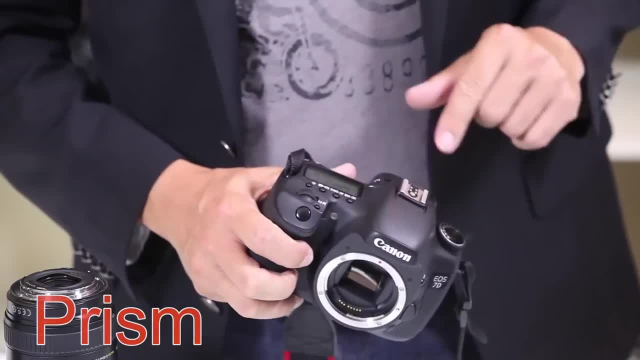 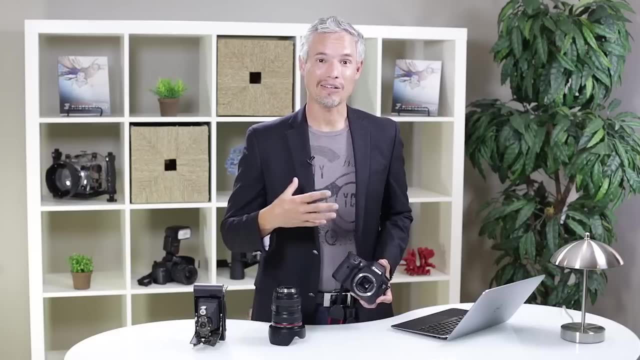 prism bounces the light up into this piece and then towards your eye. this is the unique feature about dslrs: you see what's coming right through the lens. you see exactly what your camera's sensor is seeing. now i'm going to move the mirror out of. 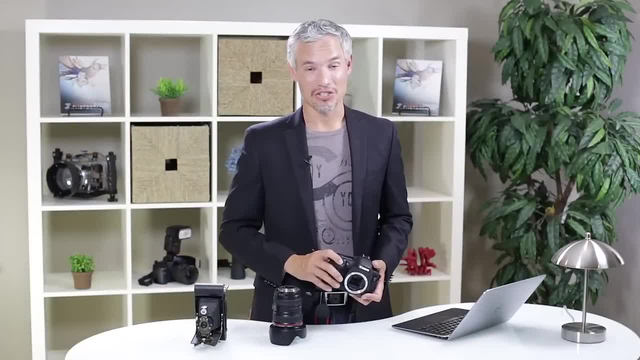 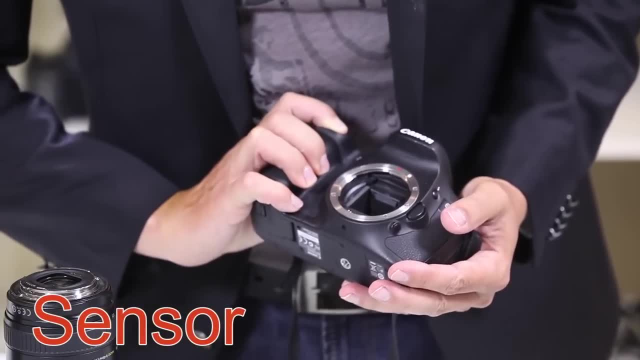 the way and show you what's hiding underneath, and that's a couple of different things: the shutter and the sensor. as i pop this up, you'll be able to see the camera's sensor, and this little guy is quite an expensive part and it's is responsible for capturing all the light that comes through your lens and recording it. 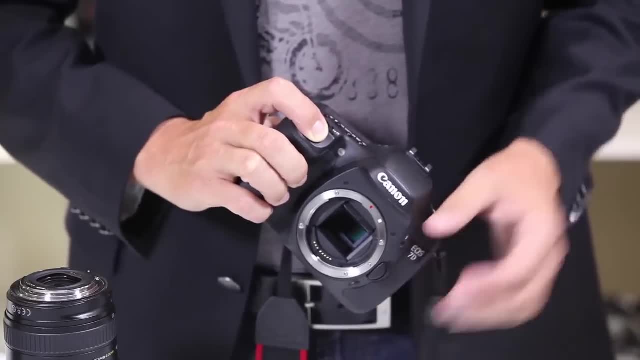 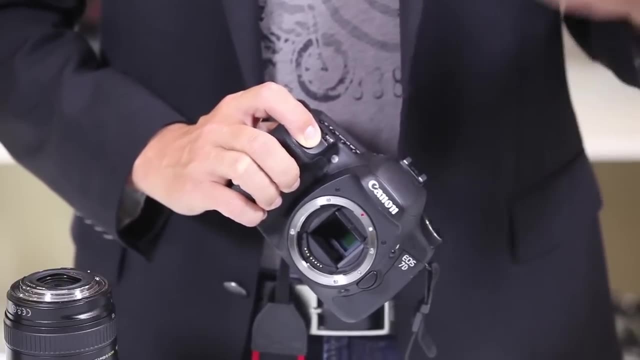 So light comes in in the form of lots of little tiny photons and this has little cells that capture that photon and basically records how many of different colors of photons that it captures. And you know, with 2 million of these, 20 million of these, it can put together a decent picture. 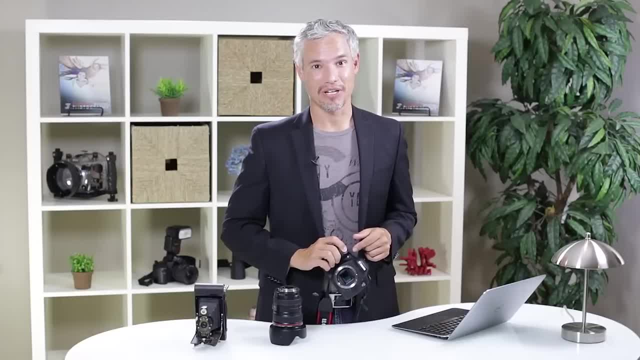 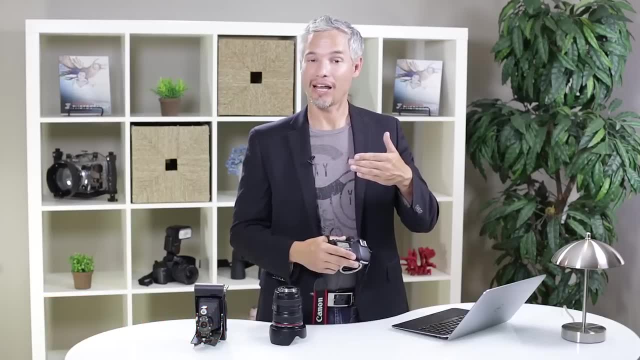 for you. But there's something in between the mirror and that sensor and that's the shutter. The shutter is this two-piece component that slides down to reveal your digital sensor and allow the light from the lens to hit the sensor. And then there's another piece that comes down and 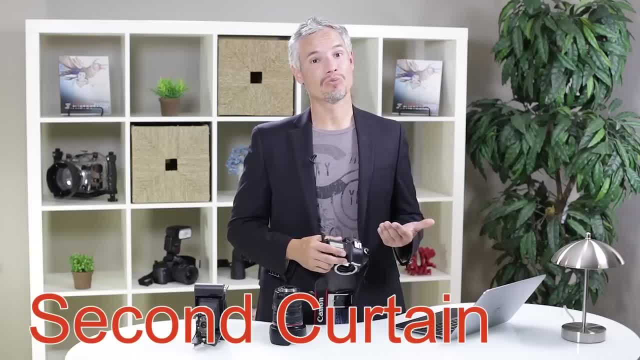 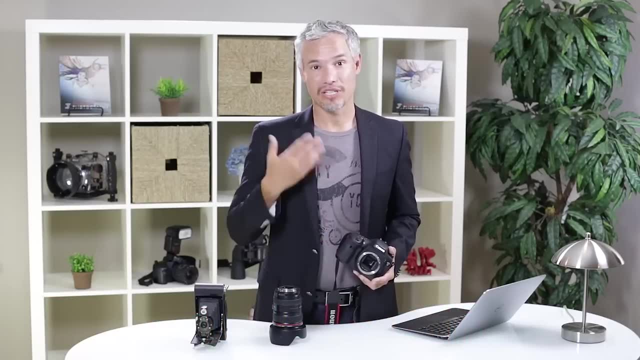 covers it up the second curtain. Now, this moves really really fast. A camera like this can take six to eight frames per second, So, as you can imagine, the shutter is getting out of the way in just a fraction of a second, And so I can't easily show it to you in action, but I happen to. 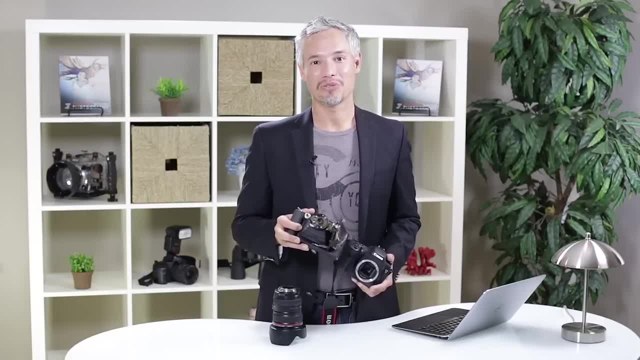 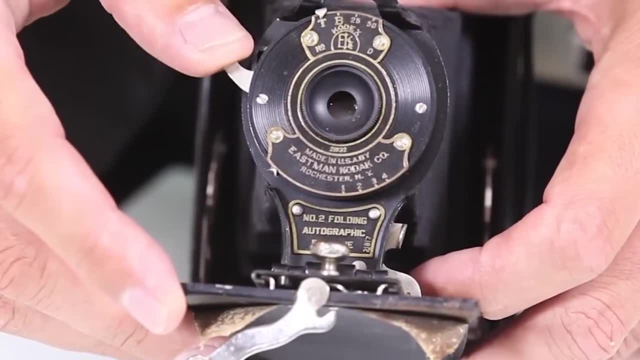 have this really old camera here that will allow you to see the shutter And the aperture in action, So let's take a look at it. So the first thing I'll do is I'll open the shutter just by pulling this down, and we can see that it just opens up like your eyelid, And so I'll close. 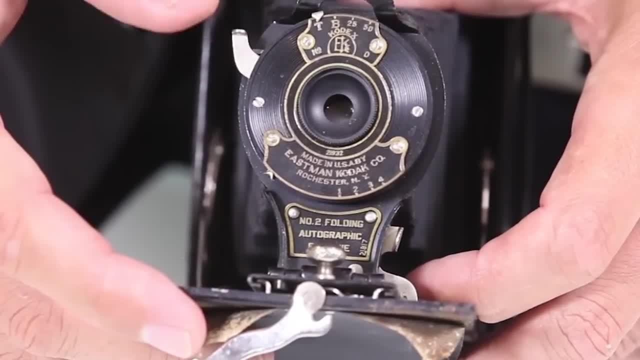 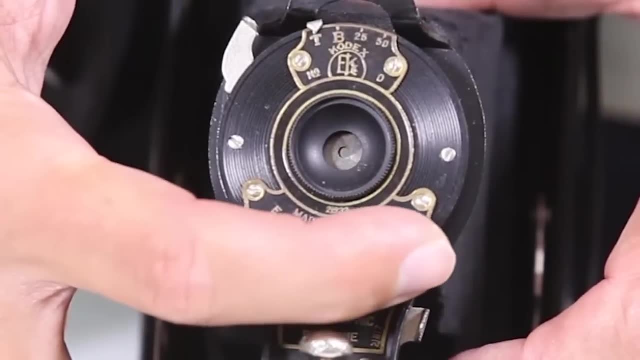 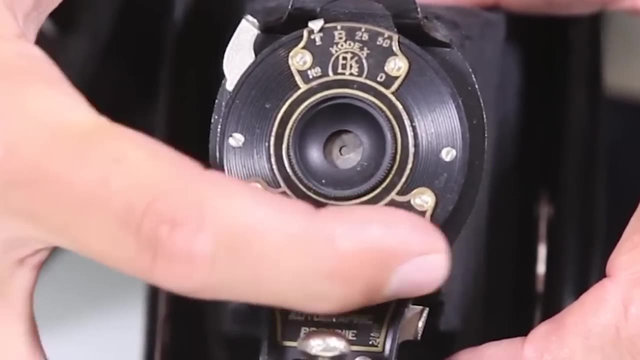 it back up and you can see it just opens and closes, just like it does in a modern camera. Now I'll adjust the aperture down As I pull this dial here you can see the iris closing. There it is at the smallest possible aperture, and then I slide it back. it gets wider and wider. Works exactly. 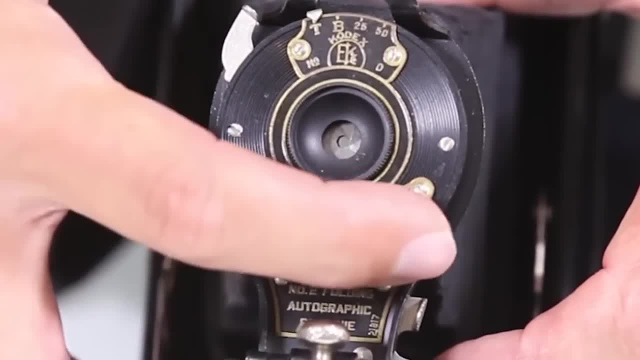 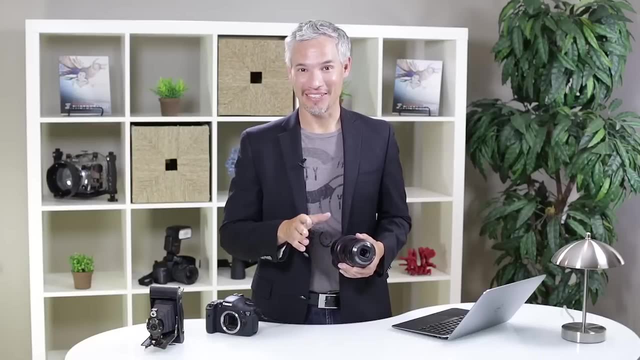 that way for modern cameras Lenses too. The difference is that modern lenses are typically controlled electronically by the camera, and it might not be as easy to see. So now let's talk about the parts of a lens. At the back of the lens we have the camera mount, and this obviously attaches to the lens mount on the back. 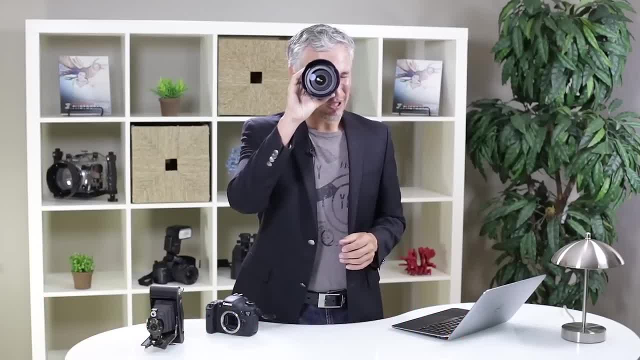 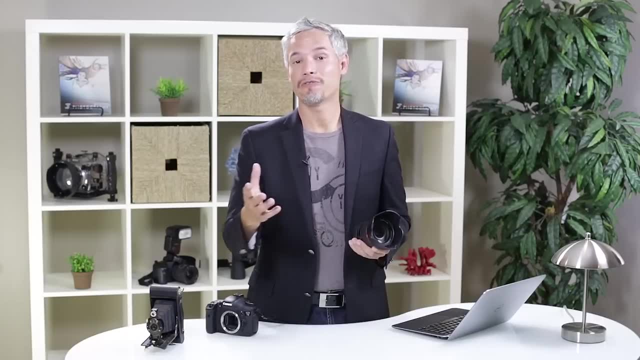 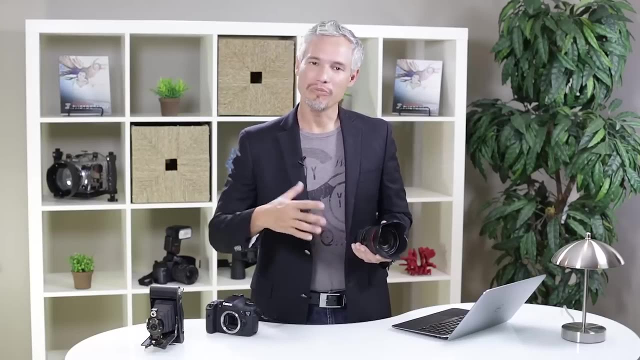 of the camera And then inside there you have a bunch of optics. There's very carefully formed glass, many different pieces of it that take incoming light and focus it perfectly so that it's nice and sharp when it hits the sensor. These optics are also shaped to minimize distortions and chromatic aberration, and 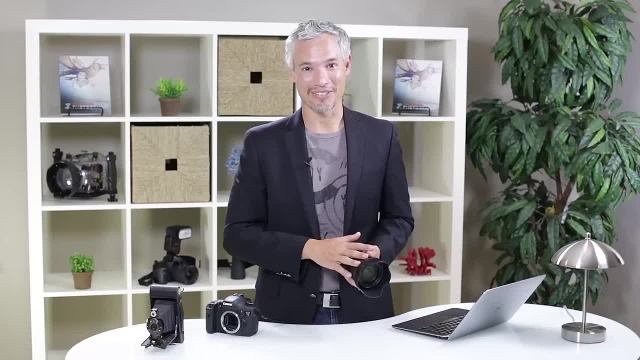 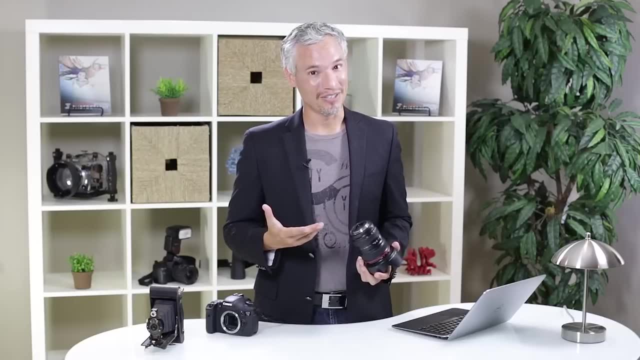 all this technical stuff nobody except the lens designers really understands. I guess the point I'm trying to make is the insides of lenses are really complex and some people, including myself, get kind of gung-ho and they want to like clean the inside of their 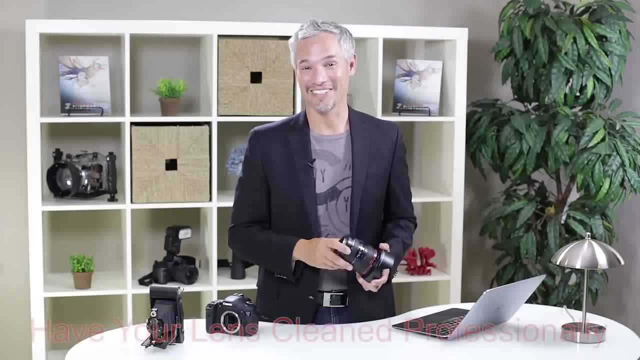 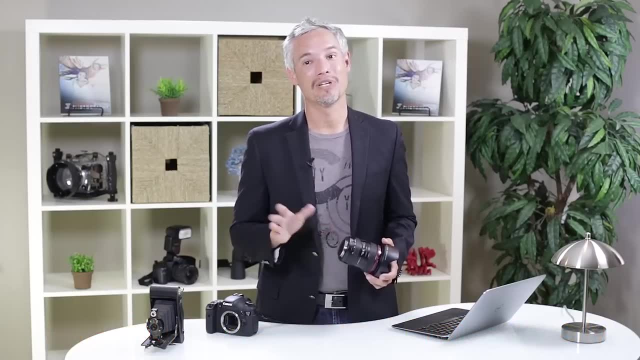 lens or repair it or something. Don't do that. Send your lens off to Canon or Nikon or wherever your camera manufacturer is, because it gets a little hairy inside of there and if you mess something up, your camera's never going to work right. So don't do that. 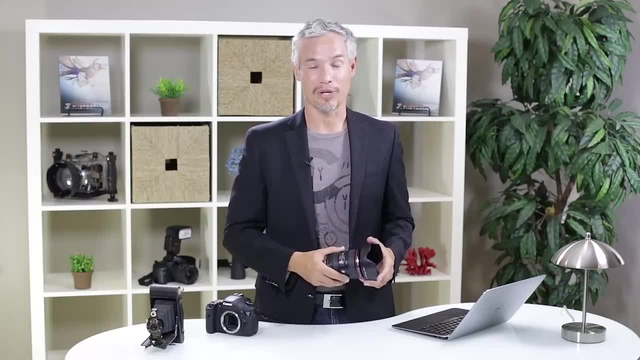 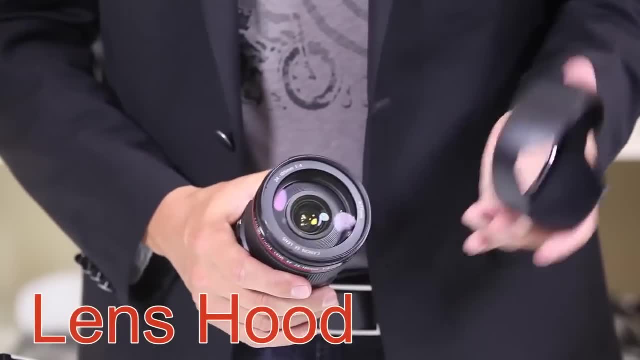 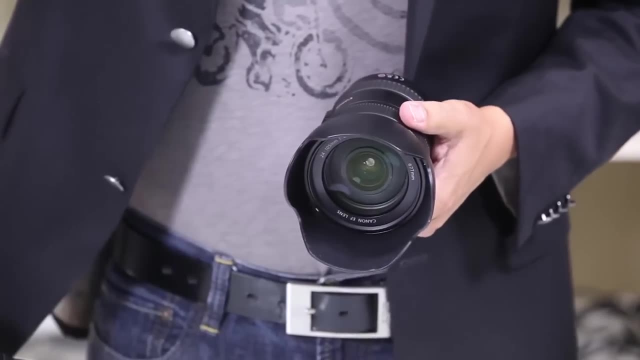 Again. so lenses are not really meant to be serviced, but we can take a look at some more of the external components on it. On the front here we have the lens hood, and this does very little optically except block stray light from coming in If the sun, for example, is up here. 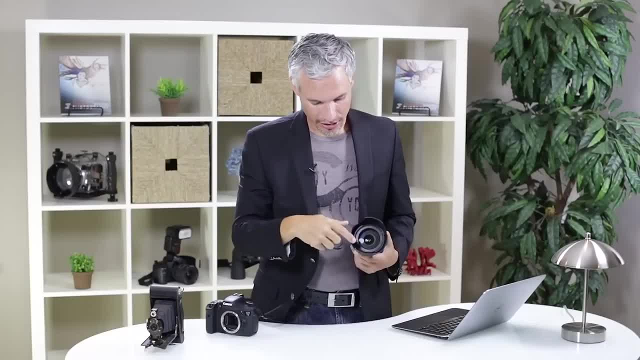 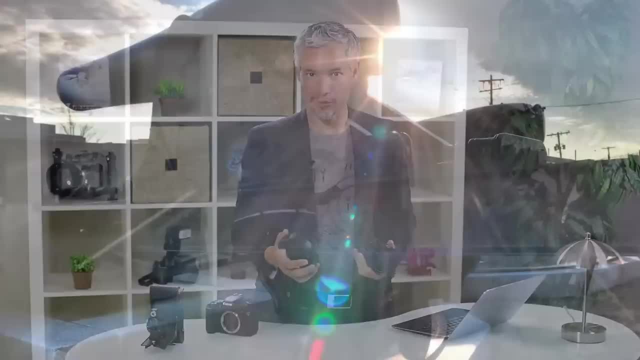 it might not be in the frame, but the sunlight could hit the front lens element and bounce around inside the lens. That would produce a condition called lens flaring, which are odd spots that you might see in your picture. Some people end up thinking that they're ghosts. It's not something. 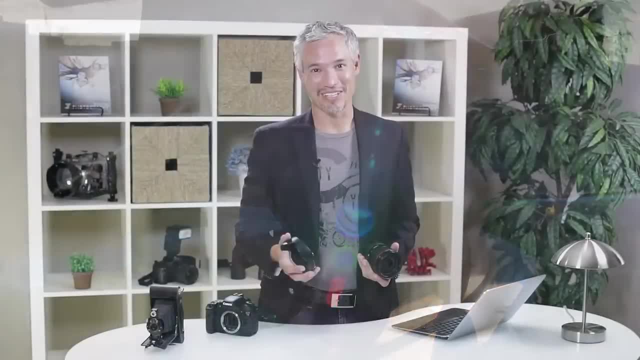 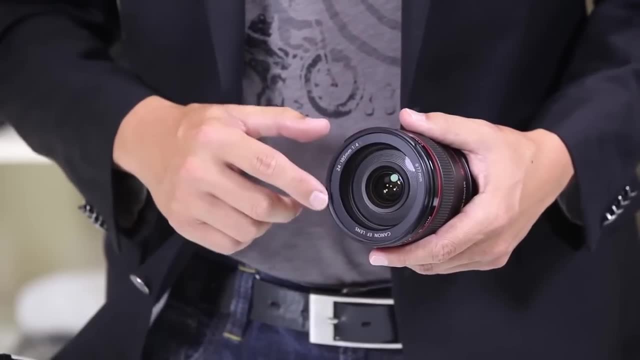 from another world. in your picture It's just stray light from bouncing in and you can kill those ghosts with just a lens hood. You'll notice that the front end of the lens is threaded like a screw. You can screw a filter on there. A filter is just another optical element that you put in. 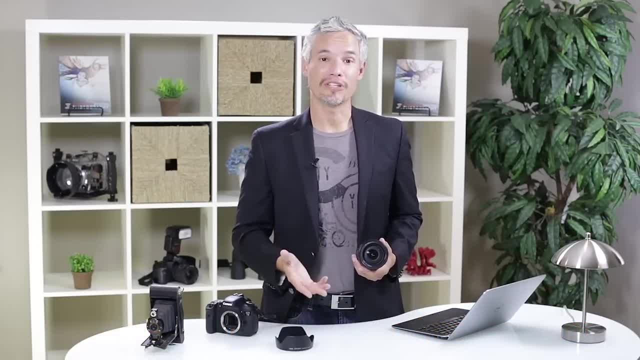 front of your lens and they do a few different things. Some people use UV filters. They're just clear filters that help to protect your lens. I'm not a fan of UV filters. They make your pictures a little less sharp and generally your front element is pretty durable As long as you have the lens hood on there to protect it from. 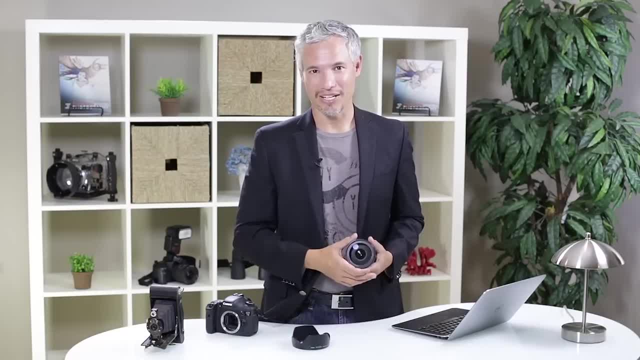 impacts, you should be a-okay. You'll get some dust on it. Just clean it off with a nice soft cloth. Another type of filter is a polarizing filter, and polarizing filters do have some optical qualities, like they block stray light and they can make your skies nice and blue. 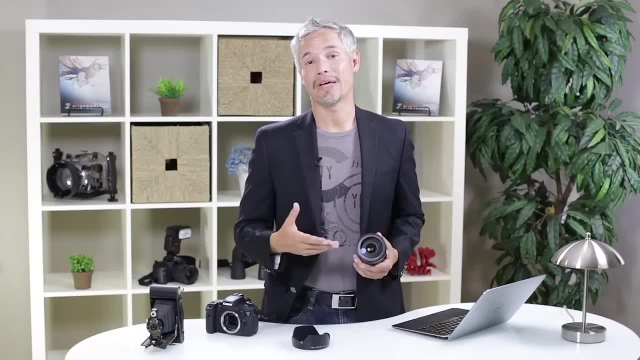 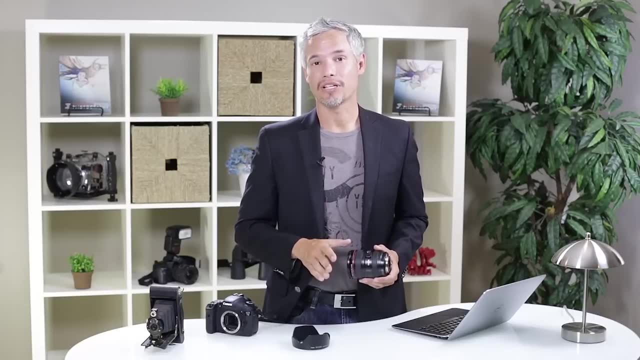 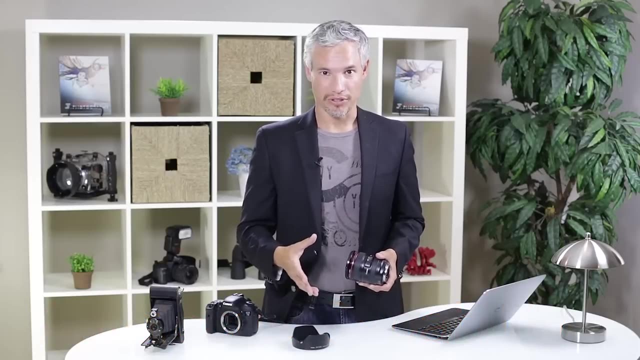 They can help, but again, they can also reduce your sharpness and they can be kind of a pain to use and often things like darkening skies are better done in post-processing. anyway, Most modern lenses are autofocus lenses, which means they have a motor built inside of them to allow them to adjust the focus electrically. And if it is an 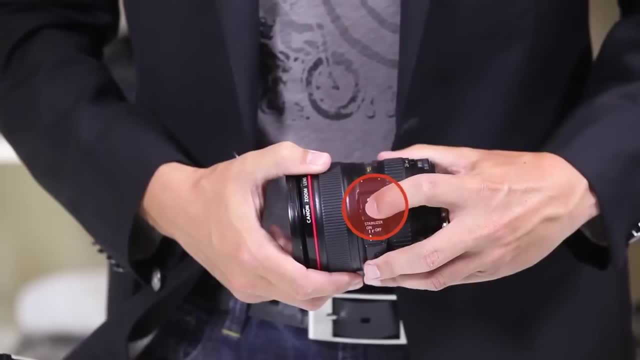 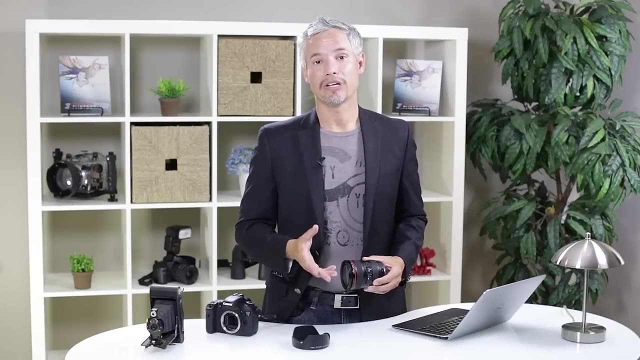 autofocus lens. you'll see a switch here for switching between manual focus and autofocus. Most lenses nowadays allow you to adjust the focusing ring here, even when you're in autofocus mode. But if the camera is annoying you by trying to autofocus, you can just switch it over to manual focus and not have to worry about it. 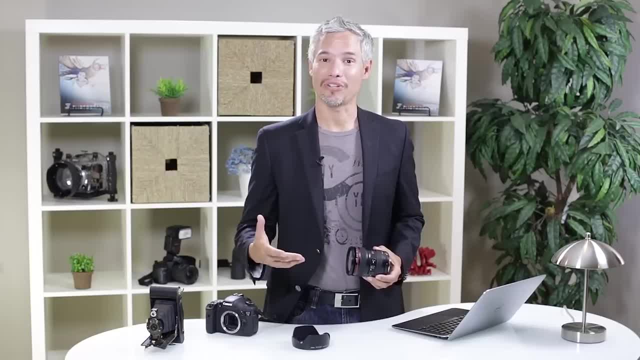 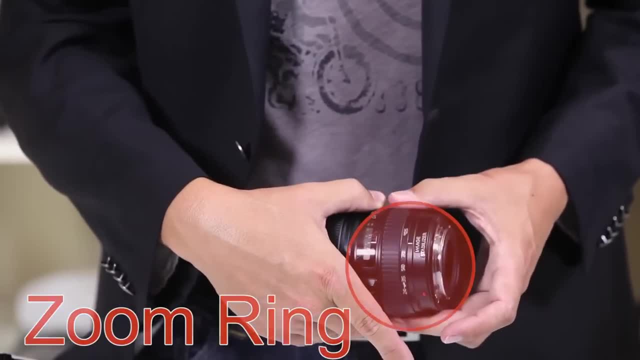 This lens is not a prime lens. If it's a zoom lens that allows you to change the focal length and zoom in optically closer, it'll have a zoom ring on it. This lens allows me to zoom from 24 to 105 millimeters. You'll notice, as it does it also changes the physical length of the barrel. 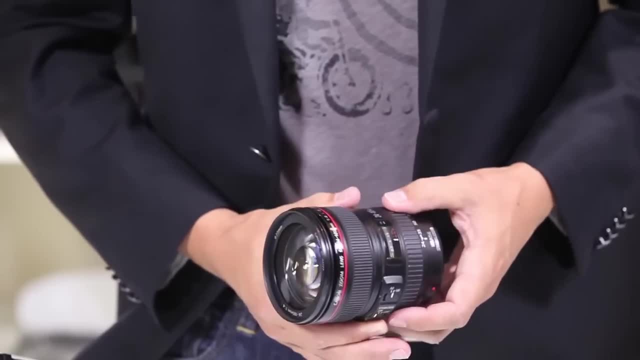 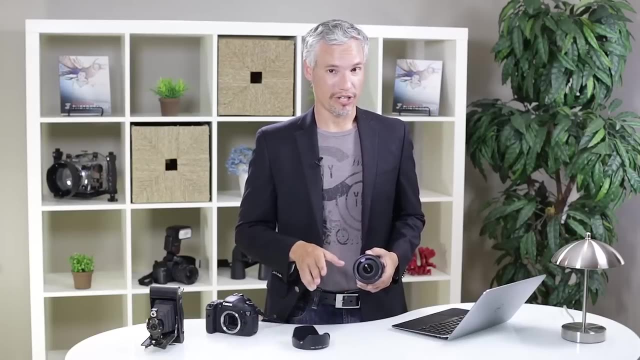 so it tends to be shortest at the shortest focal length when you're zoomed all the way back. A couple other features on some lenses. Many lenses have some useful information written on the front of them. This is helpful if you pick up somebody else's camera or another. 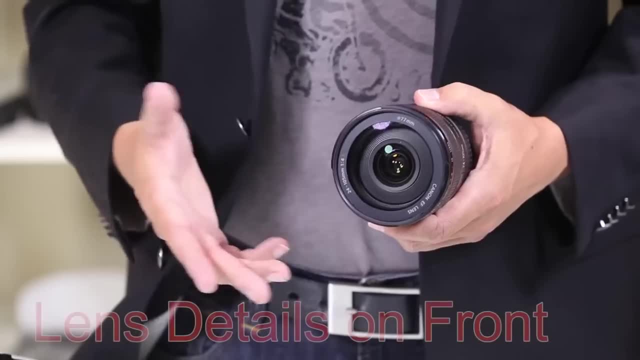 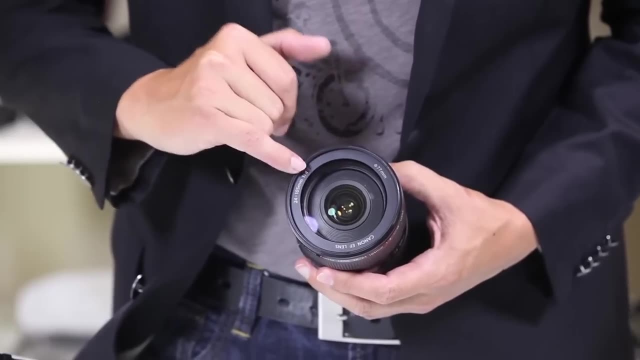 lens, or if you're just not sure which of your lenses is which, They'll usually have the focal length written right on the front here, So you can see this one says 24 to 105, 1 to 4.. The 24 to 105. 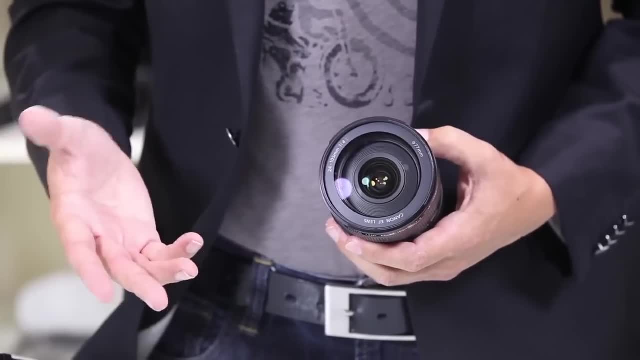 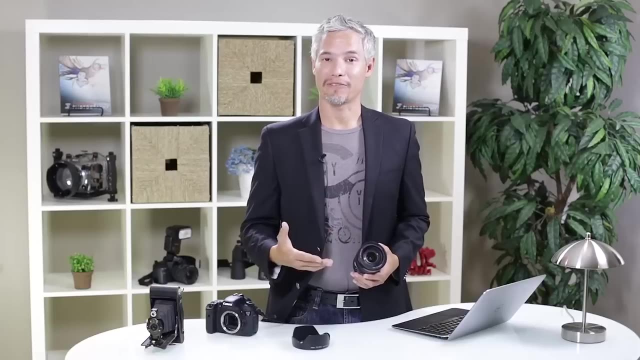 is the focal length. That's 35 millimeters, so 24 is pretty wide and 105 is fairly telephoto. The 1 to 4 is the maximum magnification. That's how close I can focus to a subject, and we'll learn more about that in the macro video lesson. 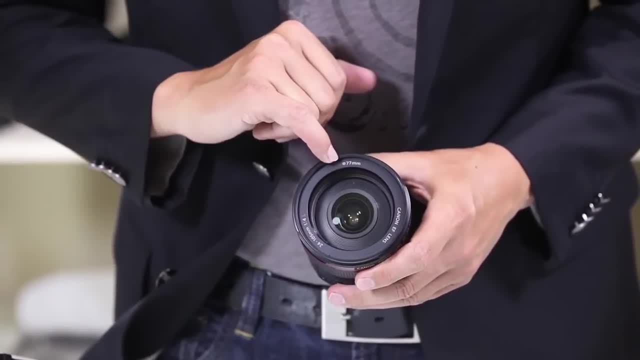 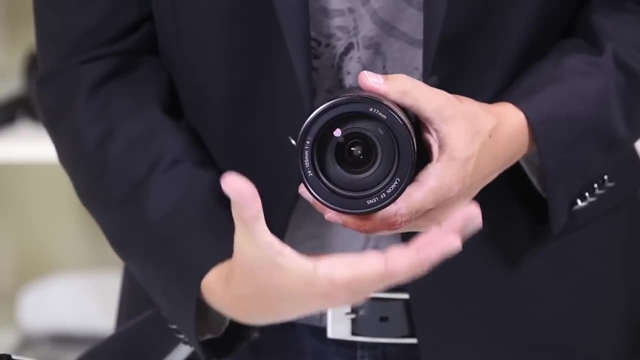 Another number that you'll see here is this funny Greek sign, and then followed by 77 millimeters, and that's the filter size. So different lenses have different filter sizes. Some are really big and some are much, much smaller. If you buy a filter for your lens, you'll need to make sure. 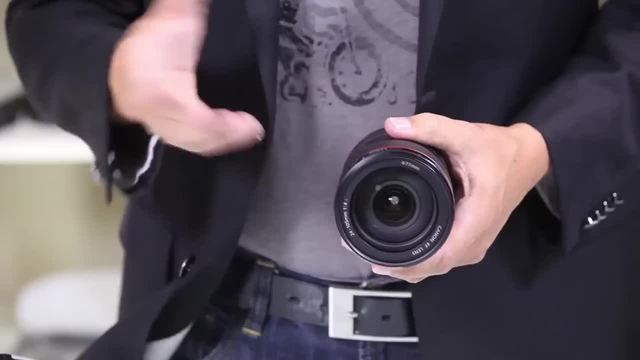 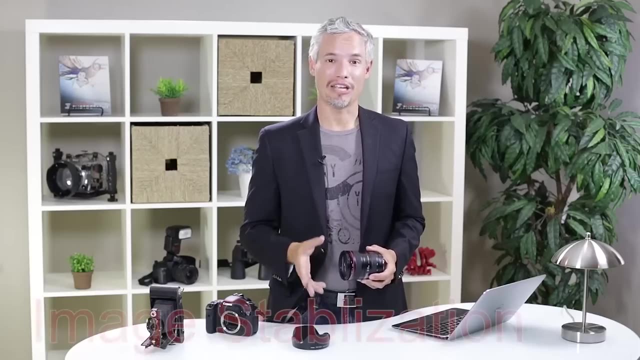 that it matches the filter size written on the front of the lens. If your lens doesn't have this written on the front, you'll just need to search for it on the web and you'll be able to look it up, no problem. Many lenses nowadays also have image stabilization and if they do, you'll have a. 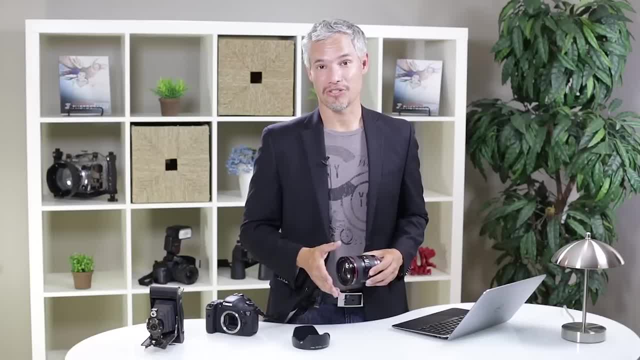 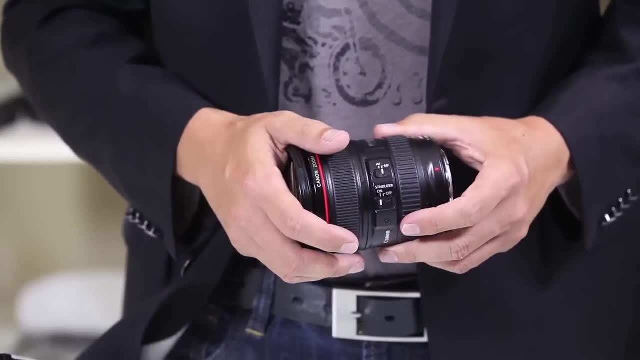 filter on the lens that is not even on the front. There might also be a second switch to allow you to adjust the image stabilization mode from standing still to panning, to being on a tripod. This lens doesn't have another switch. Now I'd like to go over the parts of the camera one more. 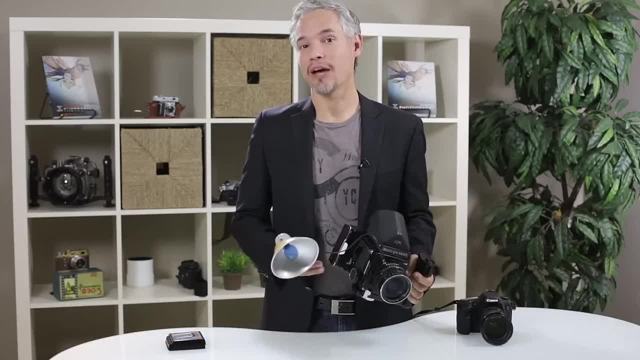 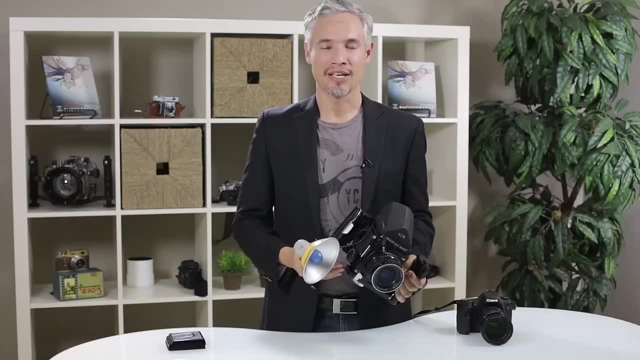 time using this old system camera. A system camera is a camera that allows just about any component to be replaced and taken off and repaired and serviced, and that means that it's a lot easier for me to show you what goes on on the inside This camera has. 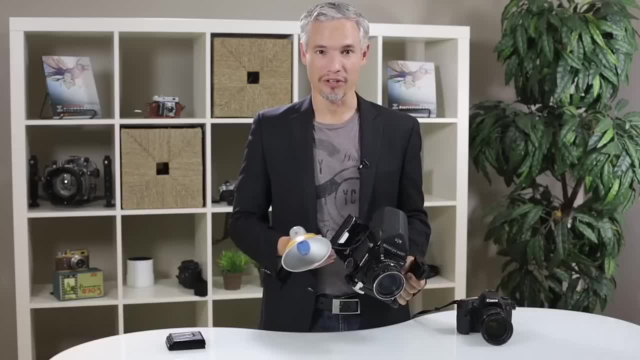 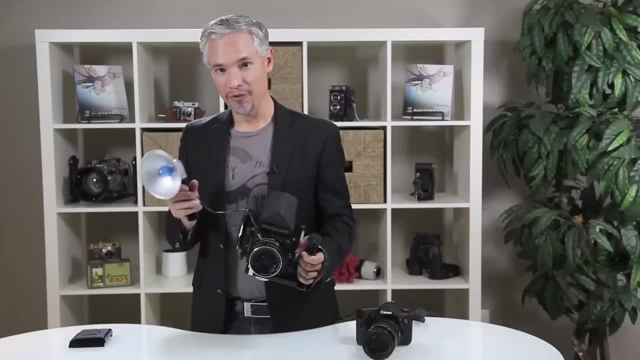 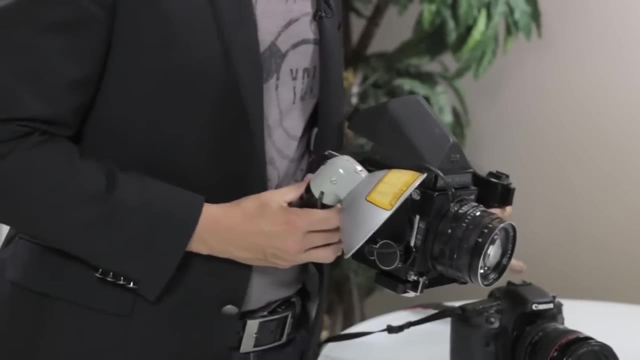 pretty much all the same components of a modern DSLR over here. They're just bigger and easier to view. So let's walk through the parts of a camera one more time. Up first I have this flash here. Nowadays a flash connects directly to a hot shoe. What the hot shoe on the top of the camera does. 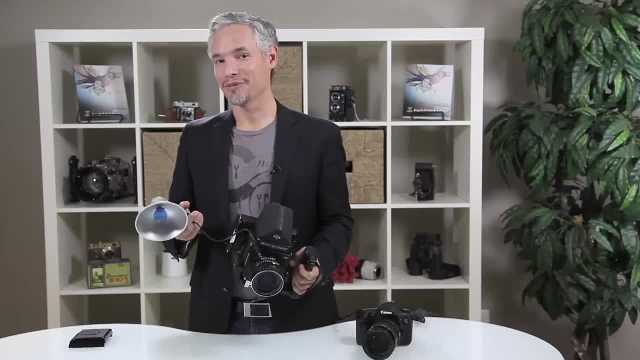 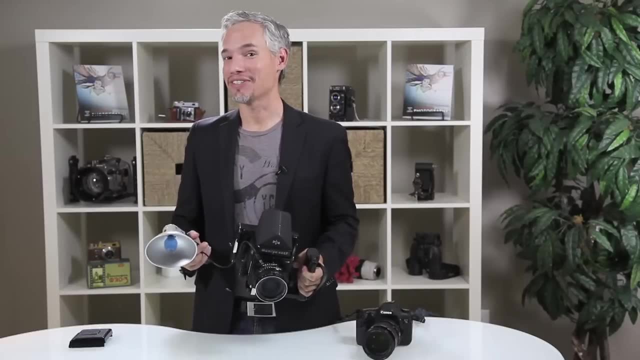 is it simply sends a signal to the flash. Now, with these old flashes, that signal was just: hey, fire. right now, A modern flash is a lot smarter and it can send out messages for metering and exposure and make sure that you get just the right amount of light. 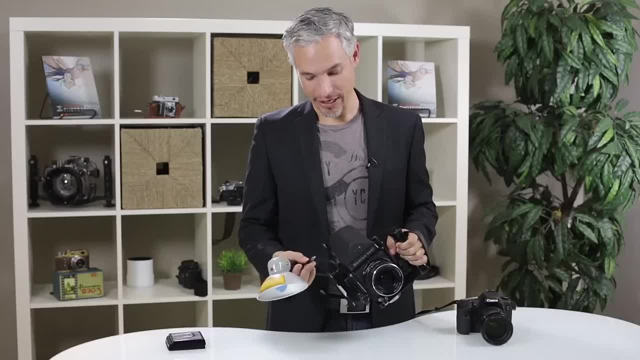 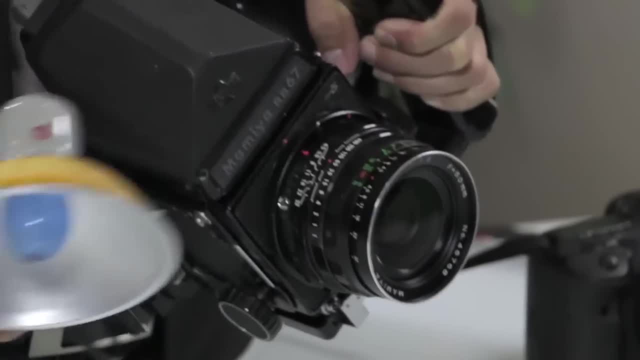 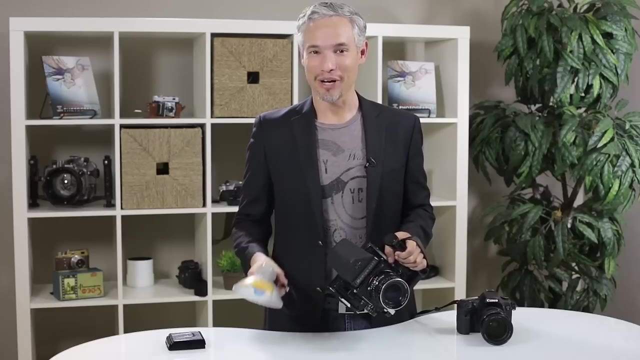 These old flashes connected directly to the lens by a PC sync port, and a lot of modern DSLRs, including pretty much all the professional DSLRs, still have that exact port right on the side. And, yes, you could connect this same old old flash, or just about any flash ever, right to it. 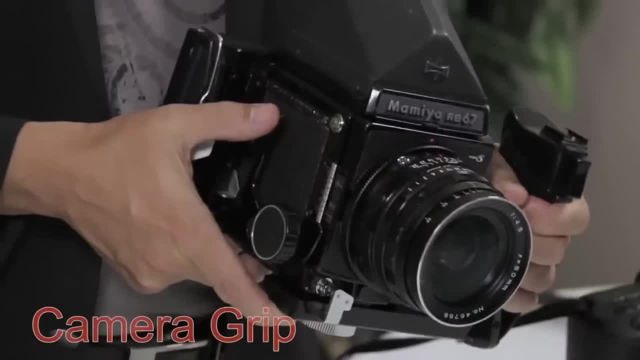 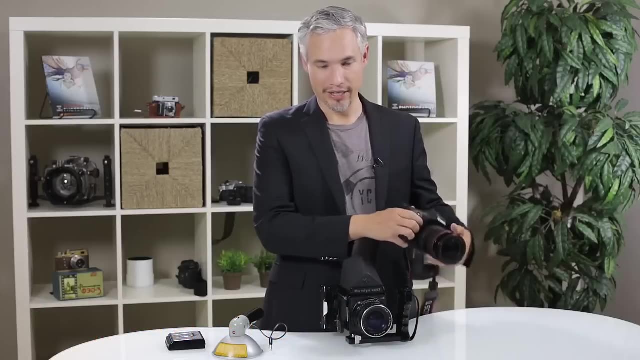 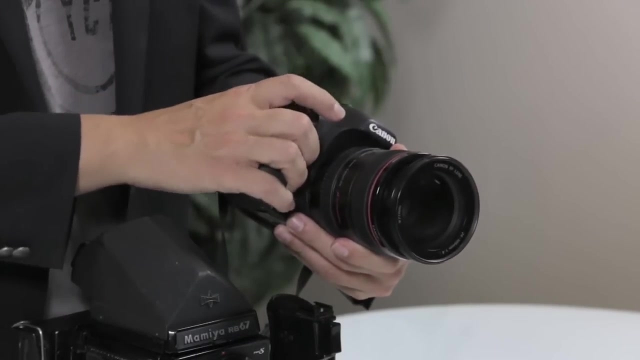 So the next component I'm going to take off is the grip, just because it kind of gets in the way here. Modern DSLRs have the grip integrated into the body, and that's convenient. That makes it a lot more compact, but it also means that you can't easily exchange it for something else Like. 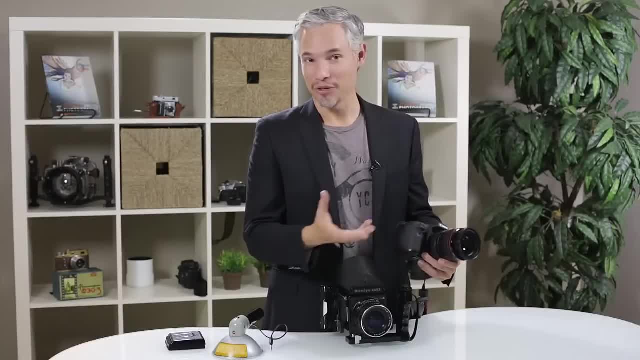 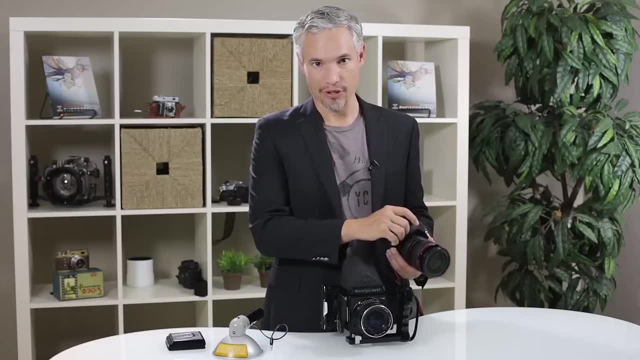 what if you were left-handed? What if you had big hands or particularly small hands? you're kind of stuck with it. You need to pick your whole camera around it, And the grip is a very important part of the camera, Something you really need to think about when you're buying a. 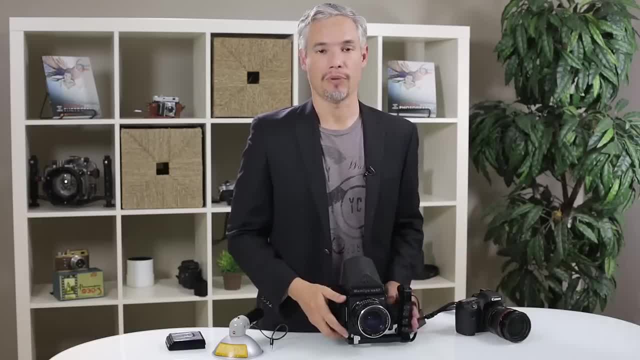 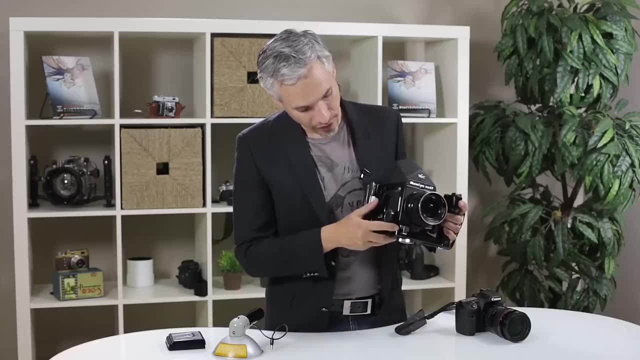 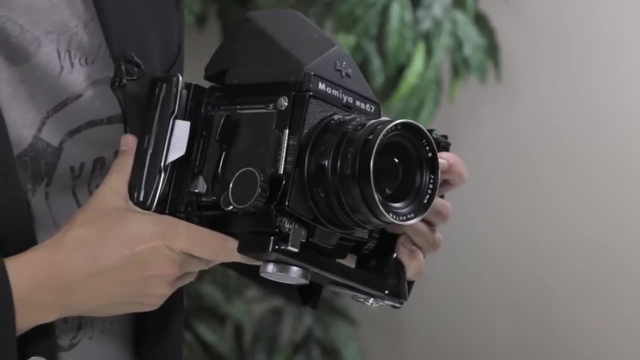 camera, These old cameras. they would have four or five different grips that you could buy This one right off. it just attaches to the tripod mount And I'll point out that if you look right here, it has a little remote shutter. I need to crank it before I can fire it And it just pushes in. 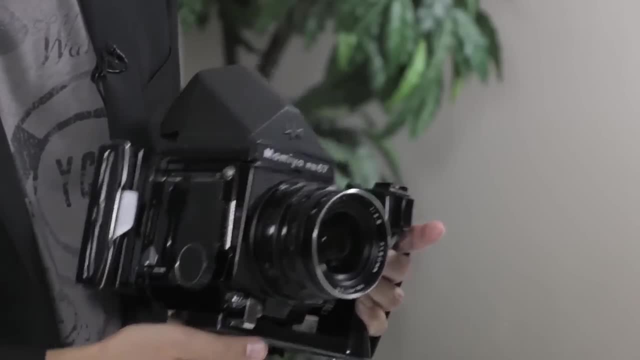 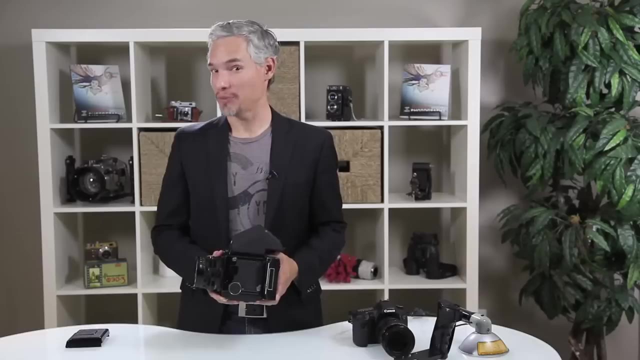 the shutter button. So after I take the grip off, I'll just have to manually push that button Up. next, let's take off the back of this camera. Now, at the back of your digital camera is a digital sensor and it's probably hidden pretty well within the camera, That digital sensor just. 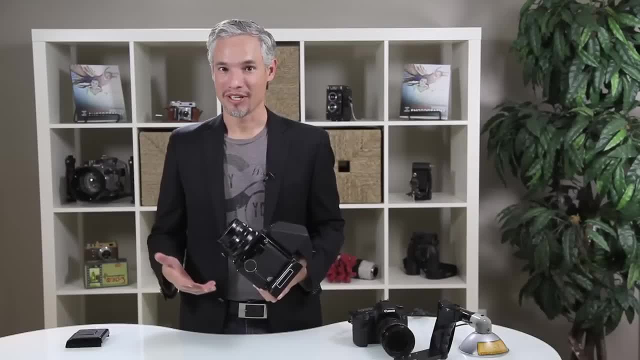 captures light and transfers it into the middle of the camera. Now, if you're looking for a memory on your camera Now, back in the film days we had the same process but of course, the light permanently embedded an image onto your negative or your slide. Now this particular back happens. 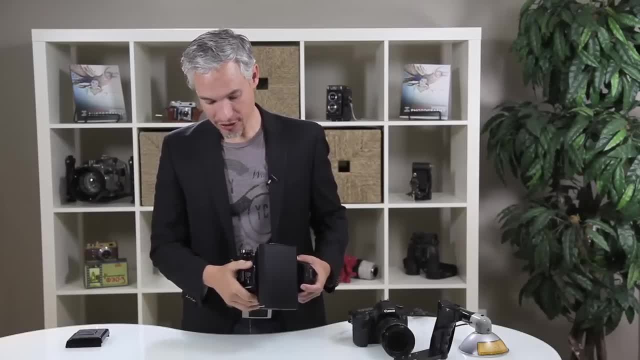 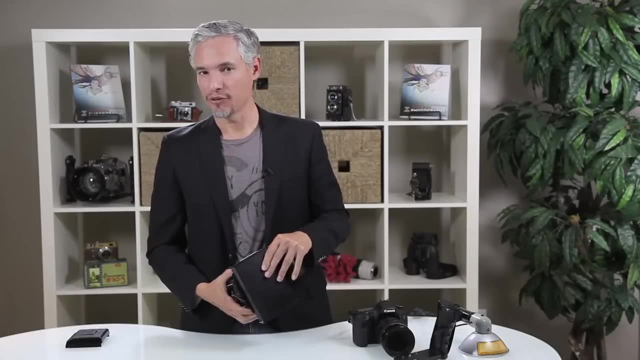 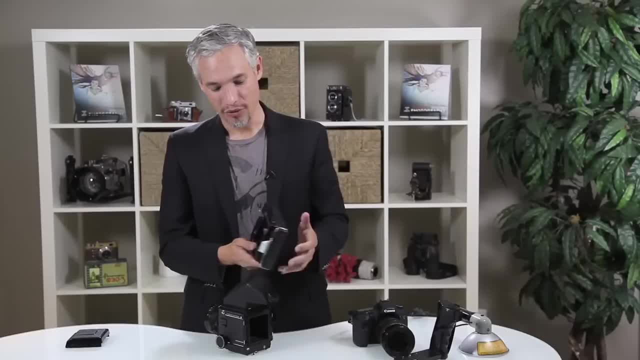 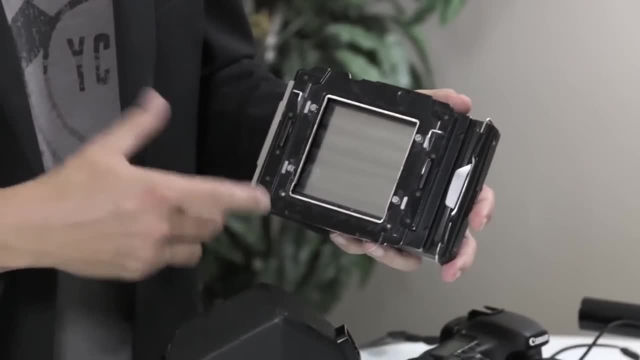 different rolls and then they would put on the next back so they could immediately slide it on. Now, as you look at the back of this, you'll see it has an opening, And this particularly opening is square, but I bet your camera doesn't have a square image. It's probably more long and 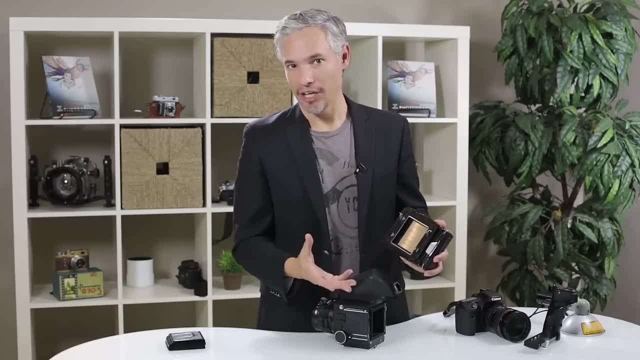 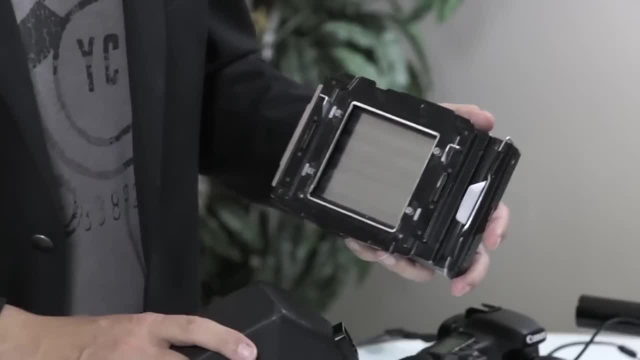 rectangular, This being a Polaroid chap and happened to shoot square, and film can be in many different shapes, but this is the actual size of the negatives that a camera like this produces, which is much, much, much bigger than the digital negative on your camera. The black and black where I've got all this black bed mismo, which is really kind of just one of a kind in your head here. So here's what it looks like. You have four Combat Roomλάai sensors. You can go through all three cameras in one shot, especially. 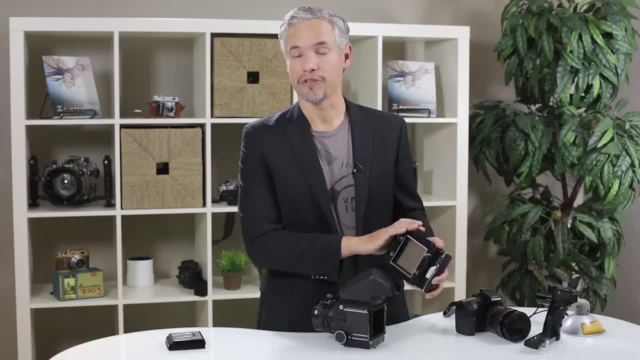 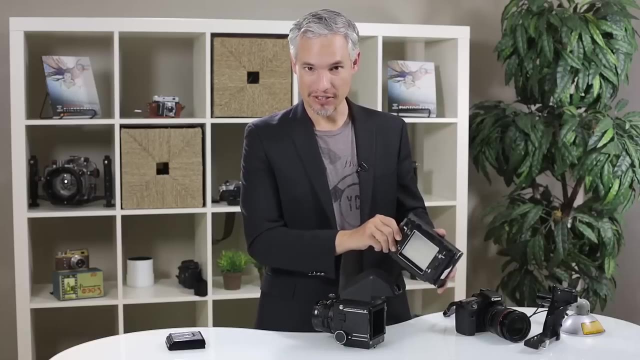 camera. This is about five times bigger than a full-frame 35mm digital camera, or probably about eight or nine times bigger than most compact DSLRs. So that was actually capturing a whole lot more light, and that's part of why this whole gear is so much bigger. So this is basically the 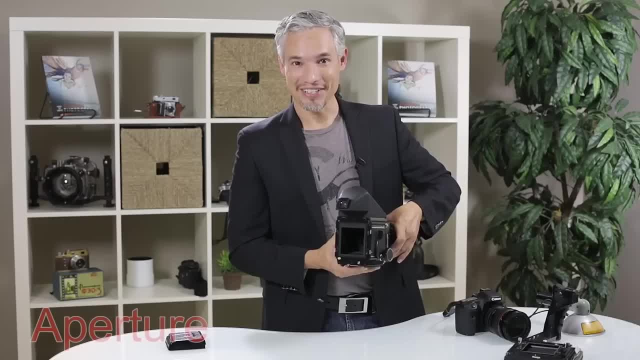 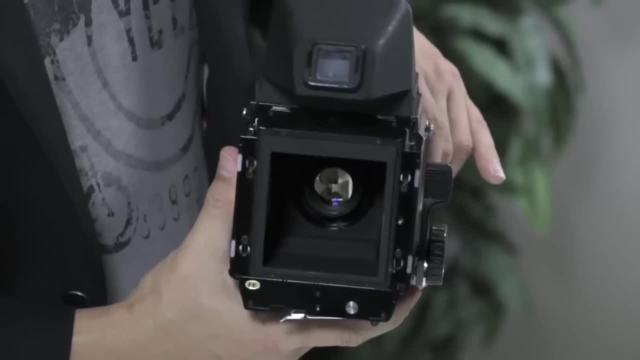 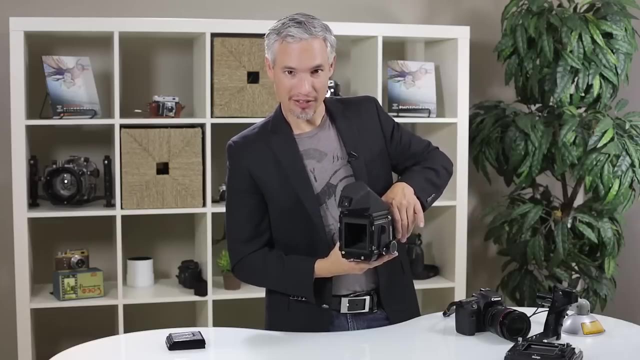 digital sensor on an old film camera. Right now this lens is set to f4.5, but as I push this slide down, the aperture is going to go all the way to f32, so as we look through the lens from the viewpoint of the digital sensor on the camera, we can see light coming in and right now, the aperture. 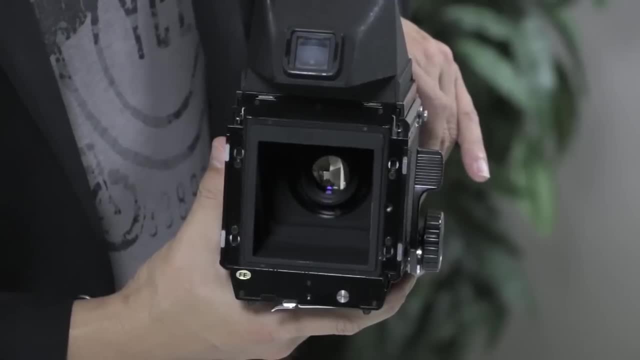 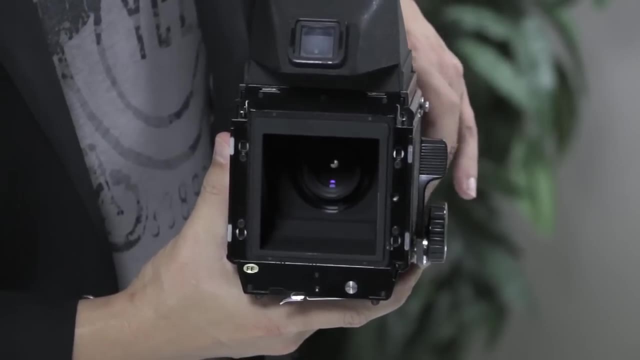 is completely open at f4.5.. So I'm gonna select a higher and higher f-stop number here, and what we'll see is the aperture getting smaller and smaller and smaller. Here it is at f32, and, as you can imagine, this means less light is getting in, just like you were closing off a hose. so we'll 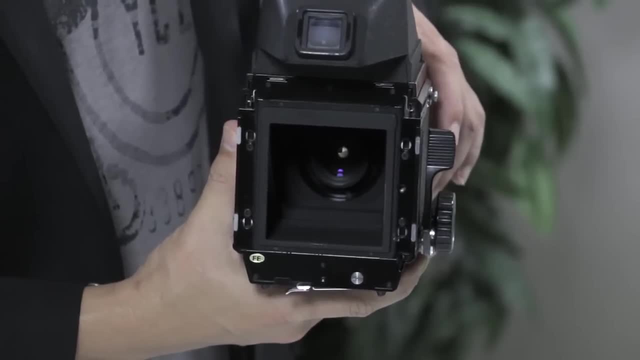 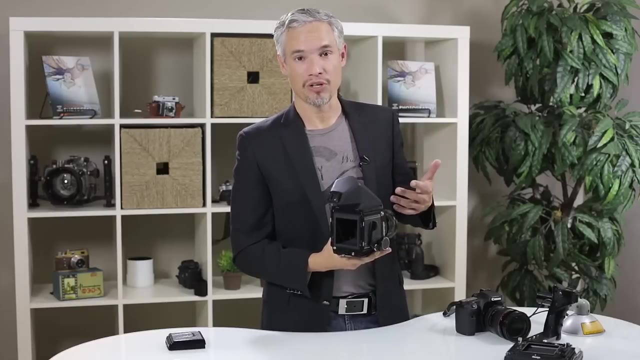 go crazy back to f4.5 here and then all the way down to f32.. This is the exact change that your modern camera and lens makes as you're adjusting the aperture. Of course, it only makes it when you either take a picture for that split second. 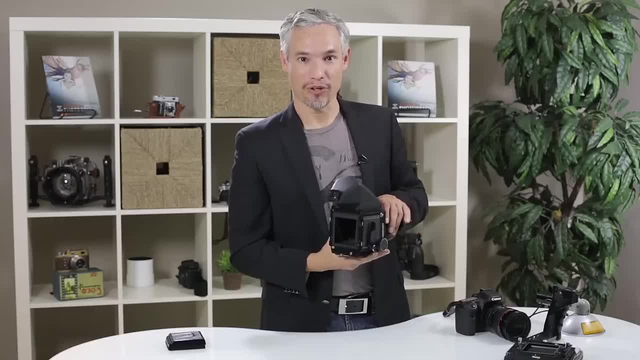 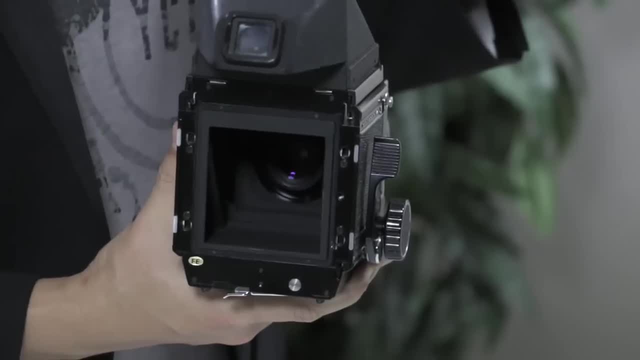 when the shutter is open or when you hold down that depth of field preview button. So, just as an exercise, you might find that depth of field preview button on your own camera and see the effects that it has while you're looking through the viewfinder. Now, since you can see through the lens, you can tell that the 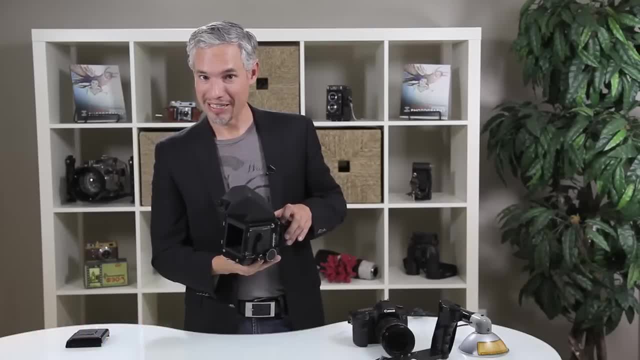 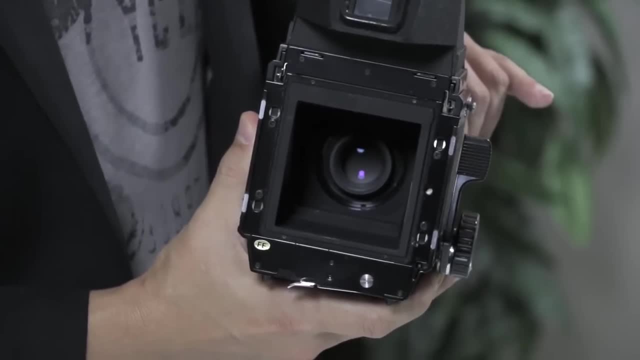 shutter itself is open. These old cameras have the shutter inside the lens itself. it's called a leaf shutter, So I'll just close the shutter so that you can see what that looks like. So, as you can see, now it got completely dark. right, That just. 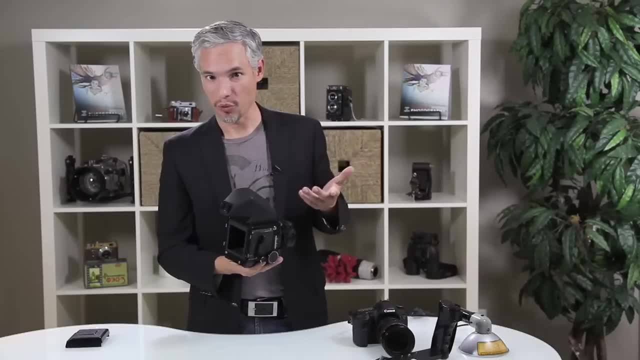 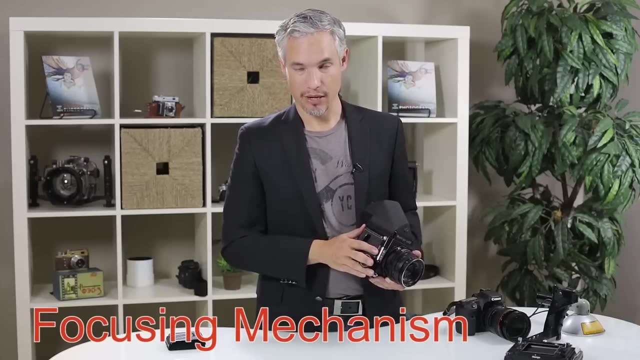 means the shutter is blocking all the light from getting to the sensor or piece of film. Now, before I take this lens off and show you that side of it, I'm going to show you the focusing mechanism on this particular camera. Now, this is going to be different from the lens I'm holding down, and then I'm going to. 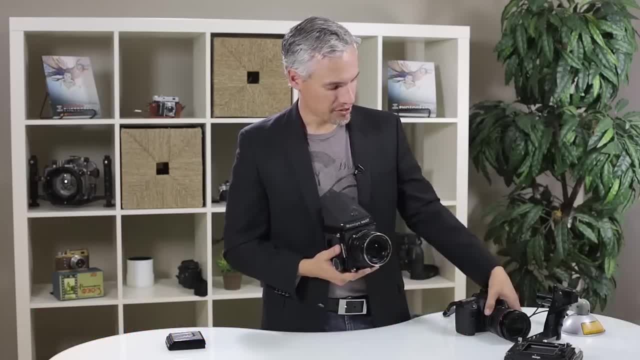 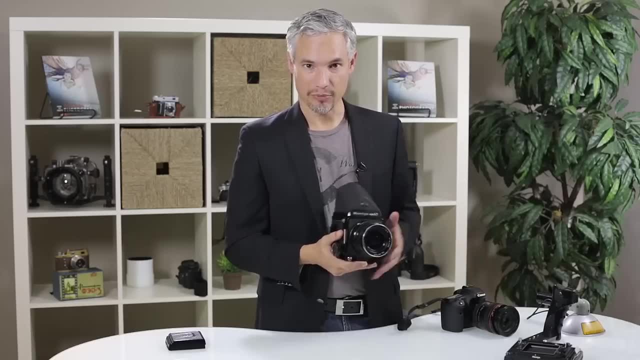 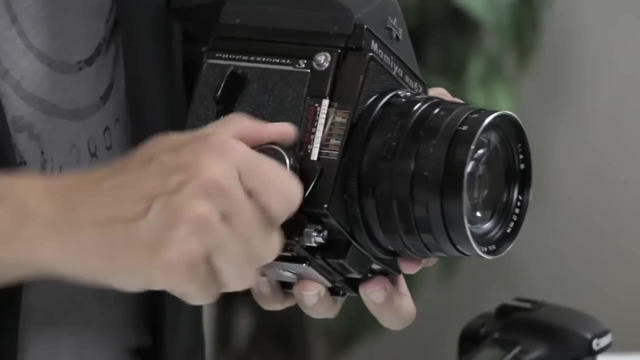 different from your camera. Modern DSLRs have the focusing mechanism built right into the lens itself. These old cameras had the focusing mechanism built into the body, but it worked basically the same way. So right now I'd be focused at infinity and as I twist this dial. 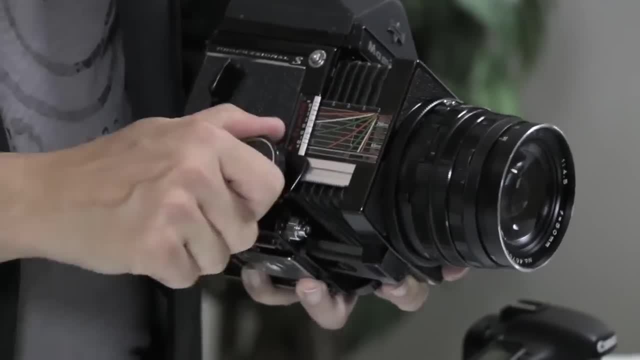 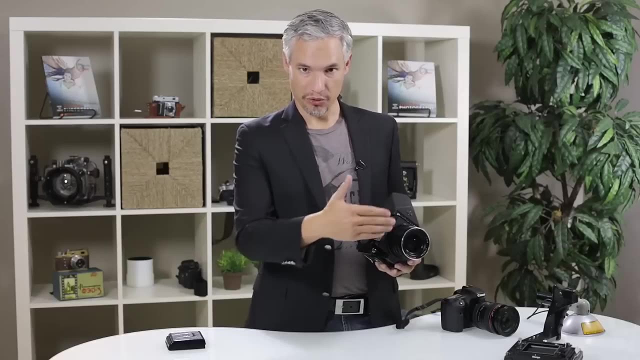 you'll see, the entire camera body extends. This increases the distance from the lens to the body itself and this makes it focus closer and closer to the lens. This works exactly like adding extension tubes to your lens. So basically, the farther I move the. 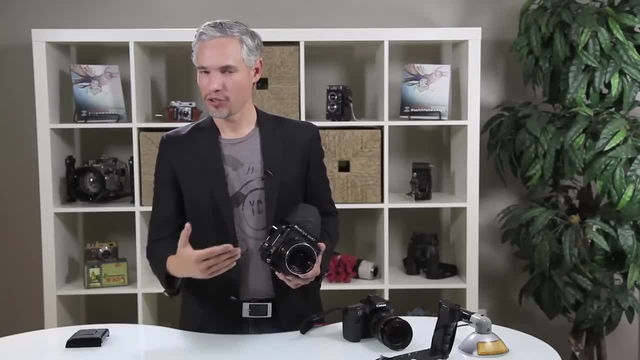 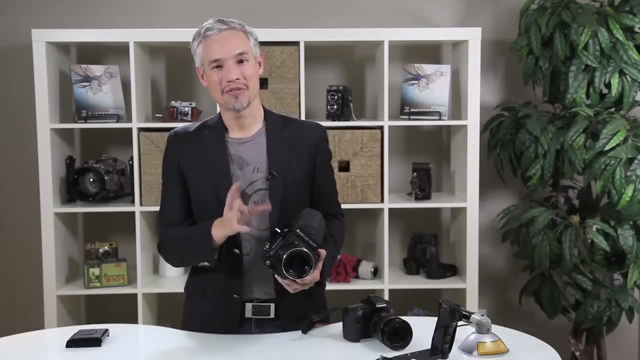 lens away from the digital sensor or film, the closer it's going to focus, And these same adjustments happen in every modern camera. but the adjustments might be made by optics that are hidden inside your lens, so they're not quite as visible. So I'll just pull this. 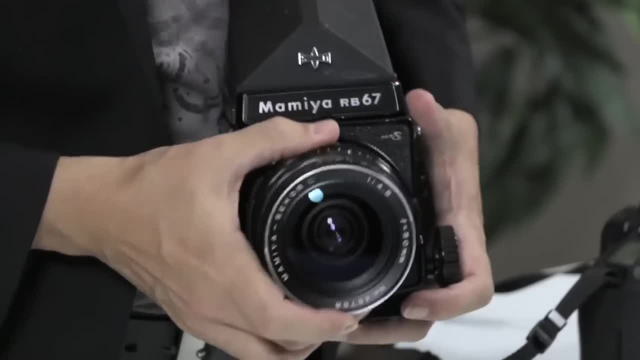 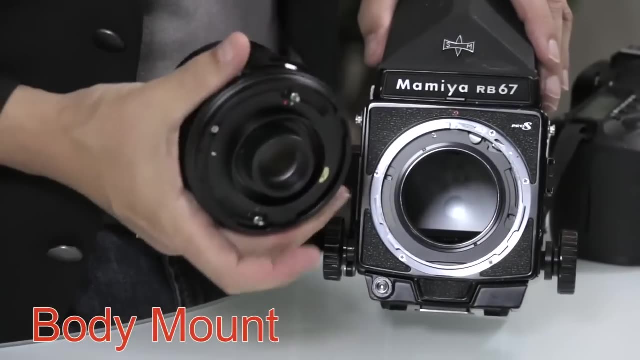 back in and we can take a look inside the lens, And here we can see a couple of common elements. You have the lens mount on the body and then you have the body mount on the lens, and these aren't too much different than you have on. 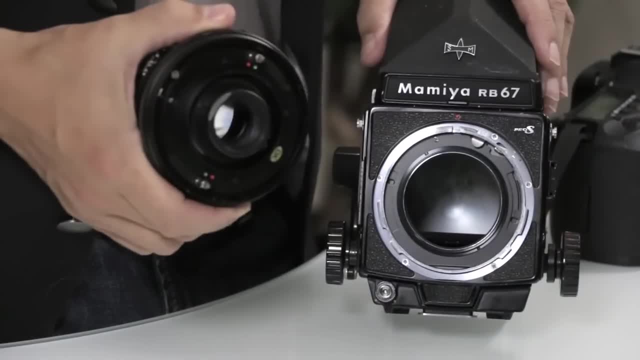 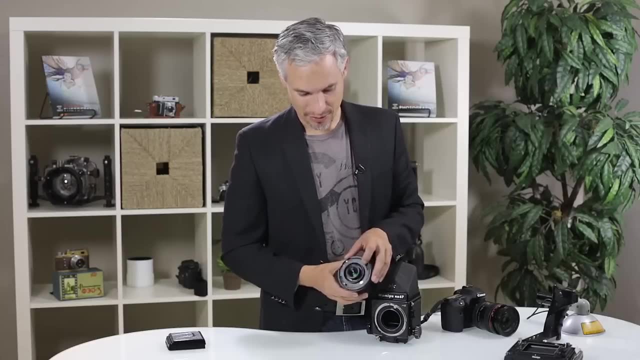 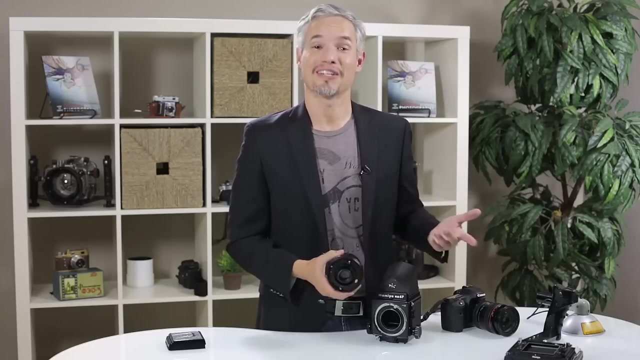 any interchangeable lens camera, including modern DSLRs and mirrorless cameras. You'll notice in this particular model there are a couple of ways for the camera to communicate to the lens. Specifically, there are these two knobs, and your modern camera will have some electrical connectors that allow the camera to communicate to the lens so it can. 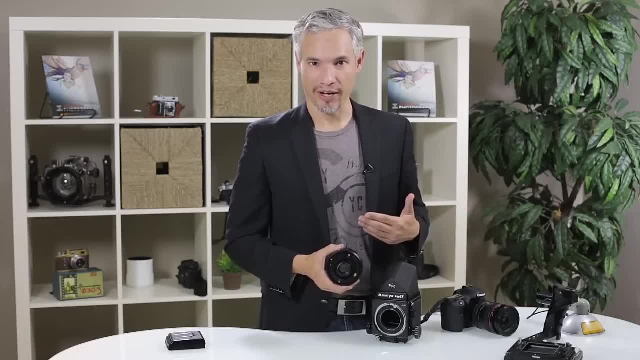 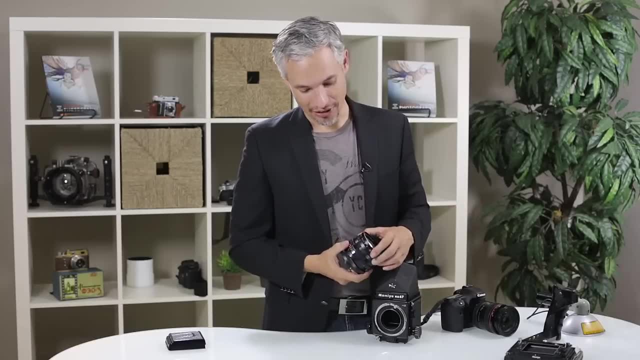 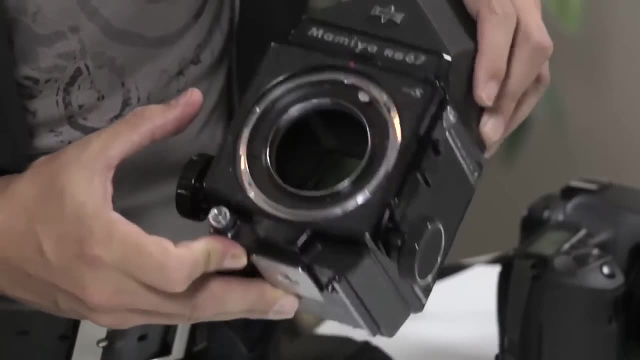 basically set the aperture. These simply allow the camera to tell it when to fire, because the aperture and shutter speed are set on the lens itself using these dials here. So now, as we look in, I will lift that mirror up by firing the shutter and we can see completely. 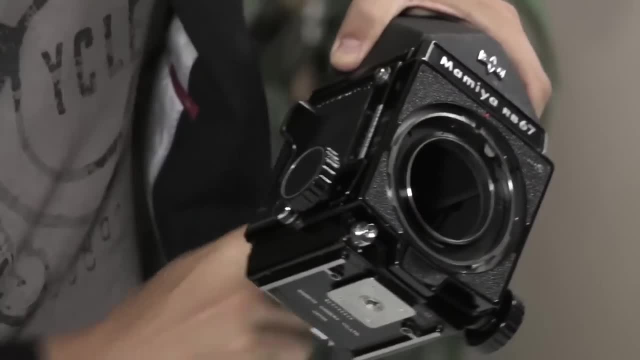 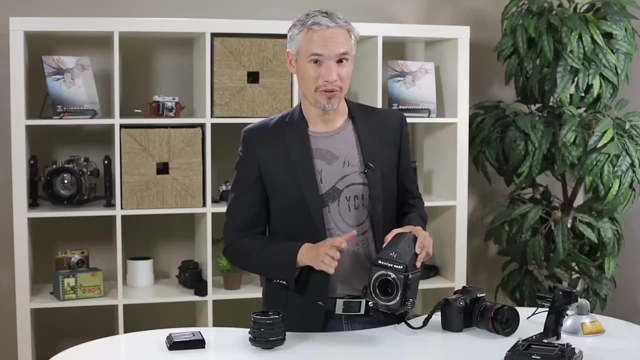 through the back of the camera. There's nothing in there, nothing to hide, and this is the position that the camera would be in when you were taking a picture. This is not, however, the way the camera would be configured if you were looking through the viewfinder, because 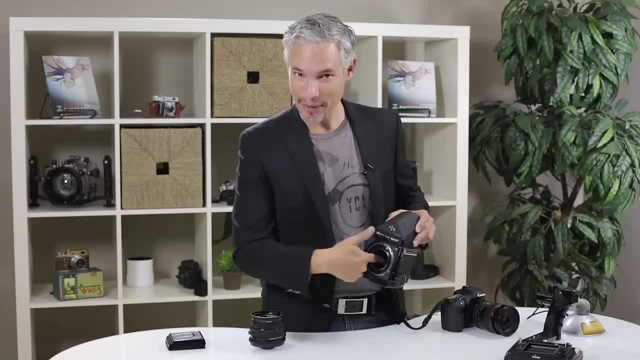 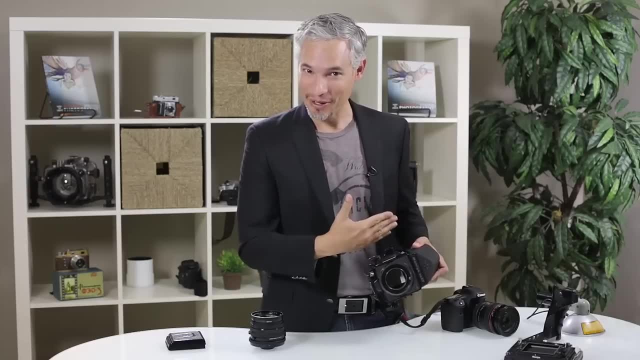 I couldn't see anything through the viewfinder now because all the light is passing straight through back to where the digital sensor would be. If I wanted to be able to look through the viewfinder up here, I'd need to redirect the light some way, right? So the way you? 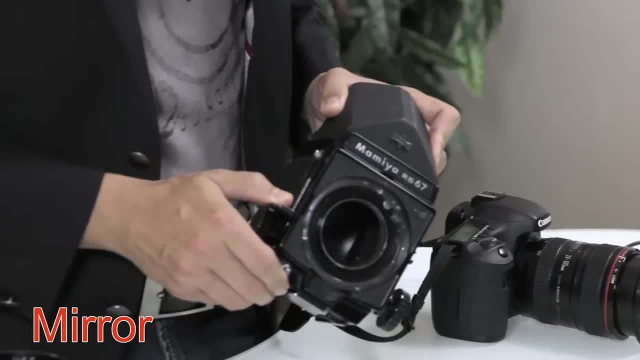 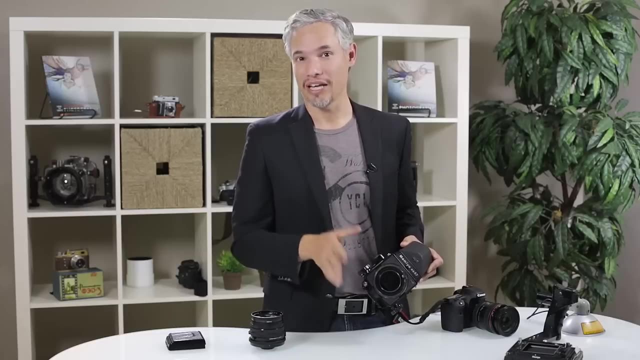 do, that is with a mirror. Now, if you've heard the term mirrorless camera, they're talking about a camera that doesn't have this particular design element. The DSLRs, the digital single lens reflex cameras or anything in the SLR family has. 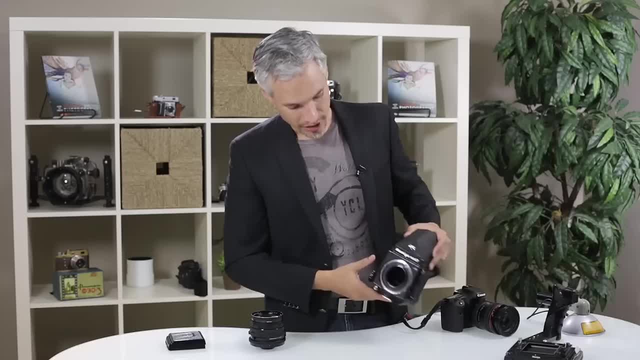 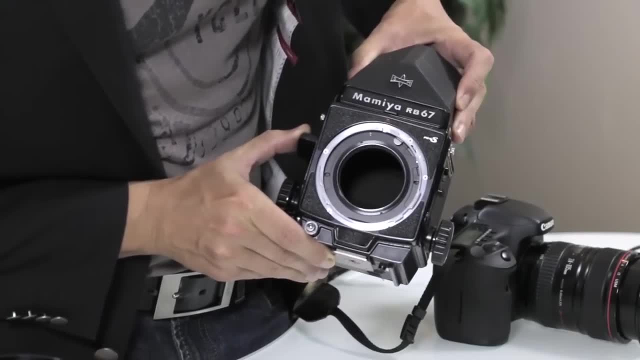 typically comes down at a 45 degree angle- it's just like this right now- and redirects the light upward. So I'll flip that back up and then kind of crank it down slowly so we can see the mirror coming down into place. Oh, there it is and you can see it's kind. 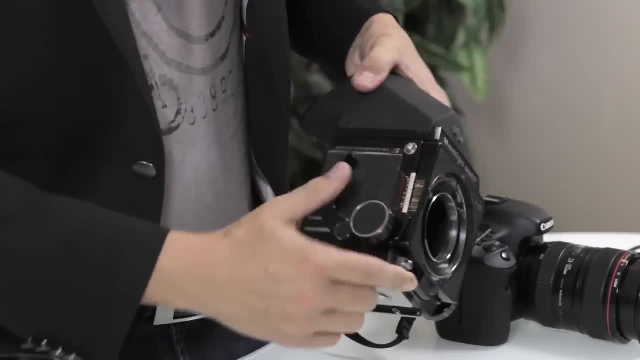 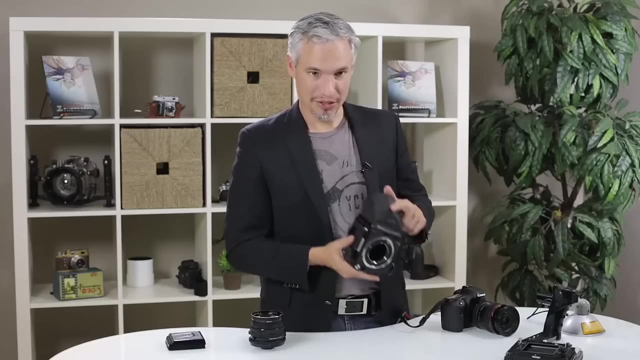 of mirrored. So what that's doing is it's bouncing all the light that's coming in through the lens up into the prism here through the viewfinder, and allowing me to see it. when I hold it up, The mirror is in the down position, like it is now. 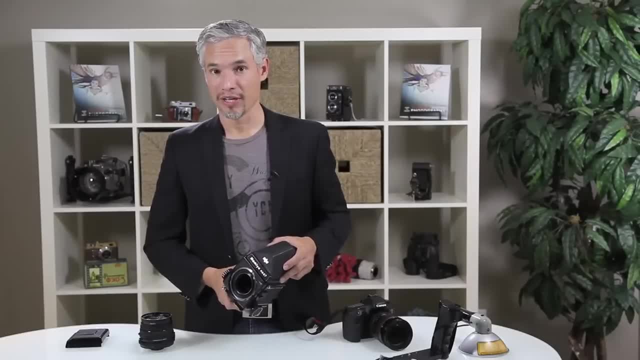 On this camera every time you're looking through the viewfinder, if you have live view on, if you're recording a video or if you're taking a picture, well, the mirror has to flip up to allow light to bypass the mirror and hit the digital sensor. If you see dust when 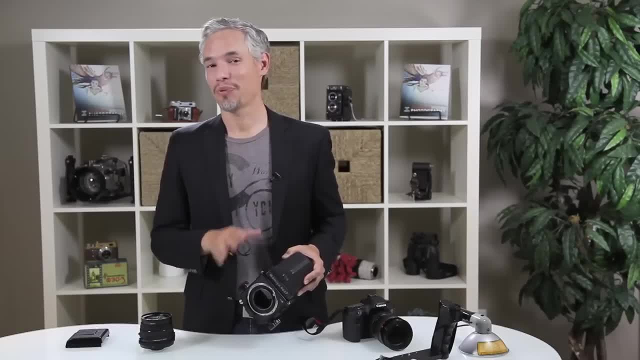 you're looking through the viewfinder but it doesn't show up in your pictures. it's probably on that mirror. It's okay just to take a fine brush to it and very gently clean it off. The only other place that the dust could be would be on the prism itself, and 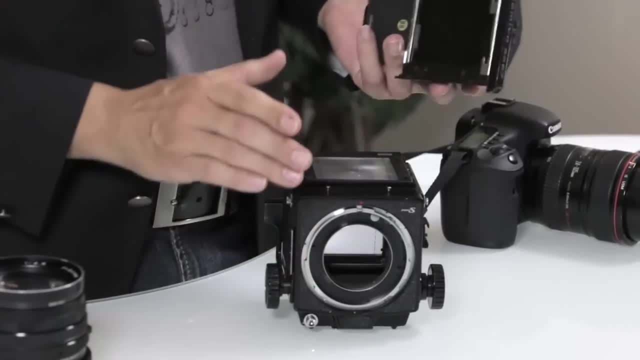 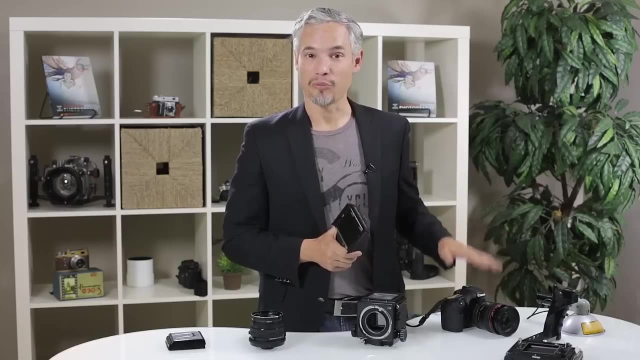 this particular camera has a removable prism, so I'll pull that off, and here we can see the bottom of the prism. Now, on your digital SLR, when you have the mirror in the down position, you can look in there and see the bottom of the prism, and so dust can collect. 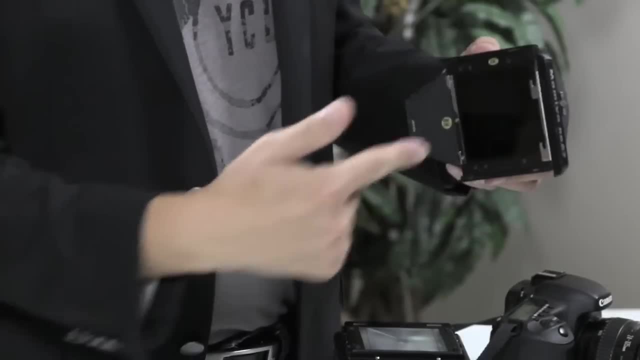 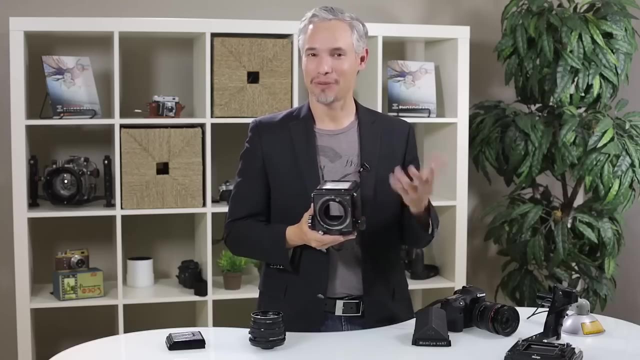 there as well. What this prism does is it takes in light, just like a lens does, and then it bounces it back over here, And that's the way your digital camera records. everything is flipped horizontally and flipped vertically, Of course. it just flips it back for you by. 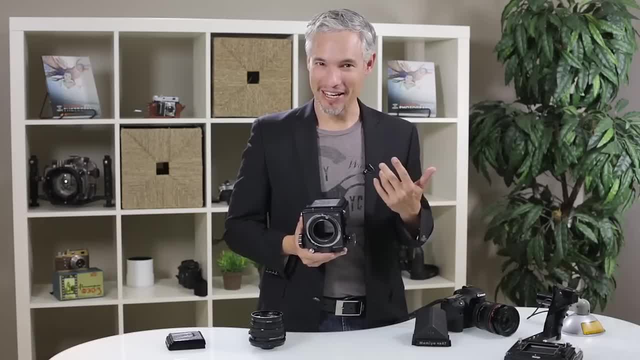 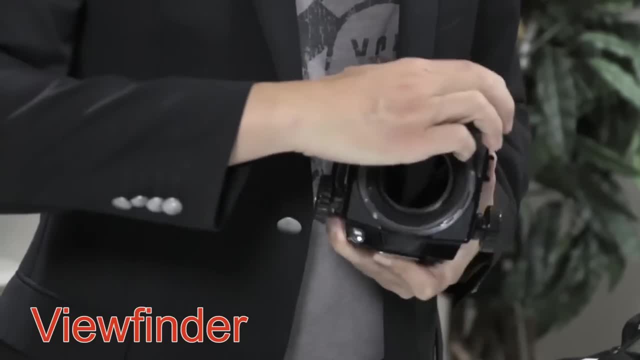 the time you look at it on the camera. but that would get pretty confusing if you were looking at it in a viewfinder- And in fact many of these cameras will use a waist-level viewfinder like this, and I'll just snap this on. And if I look through it like this, everything 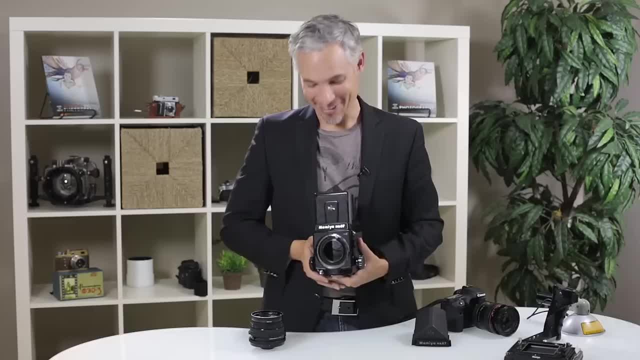 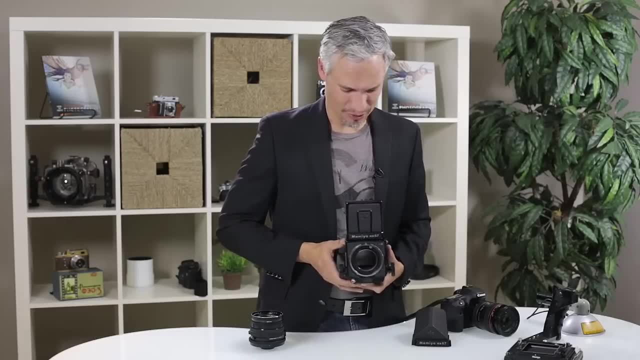 I see is flipped left and right. So the first thing everybody does when they use a camera with a waist-level viewfinder like this is they turn the wrong direction. So they'll try to focus to the right and they'll be moving this way because everything is flipped back. 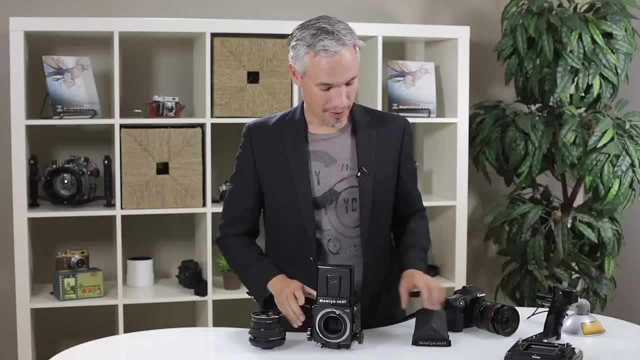 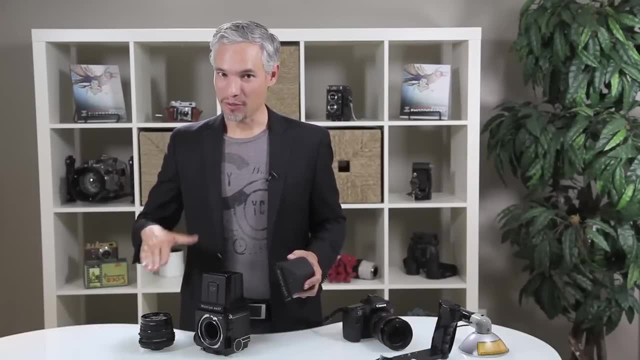 and forth. Well, your prism is doing a very important job and it is flipping everything left and right. So the point I'd like to make with that is that your mirror is fixing the problem of having the image flipped vertically. The prism is fixing the problem of having the 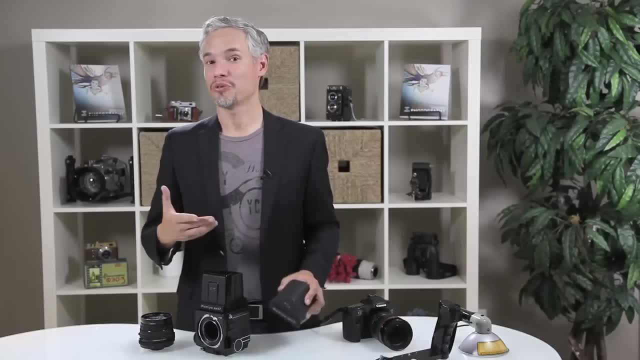 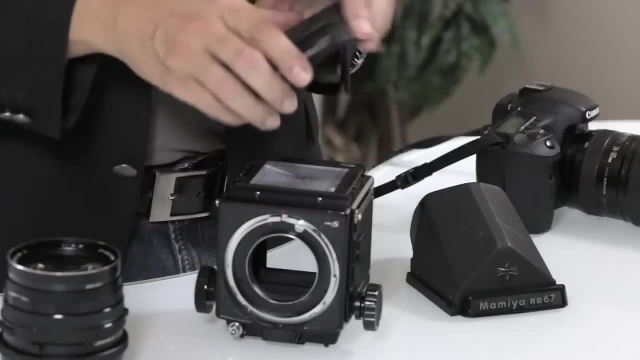 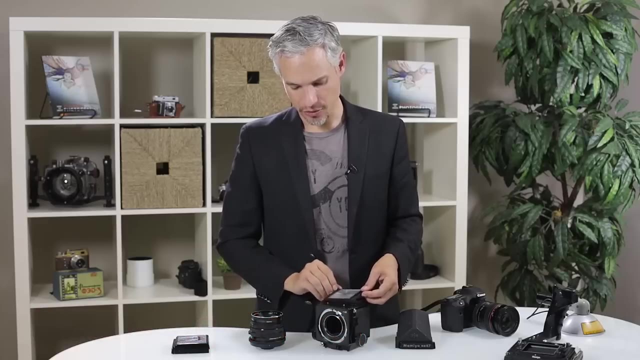 image flipped left and right, And together those two things allow you to look through the lens and see everything oriented correctly. So I'll take the waist-level viewfinder back off so that we can see the focusing screen better. Now your modern camera has a focusing screen like this too. That's the screen. 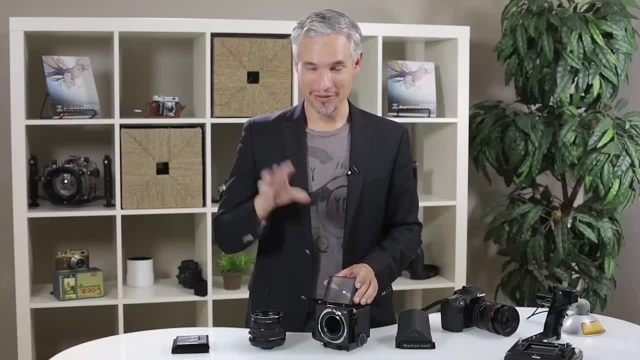 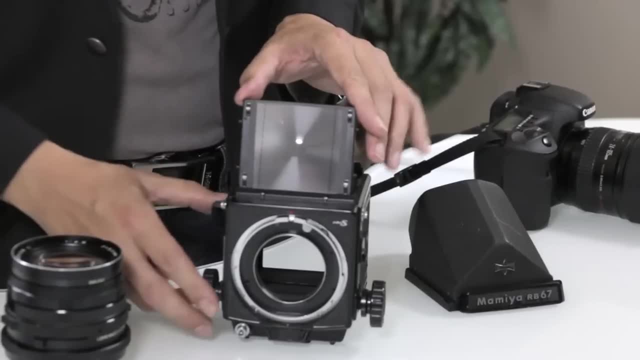 that displays things when you're looking through the viewfinder. It will light up focusing points, maybe show you the number of shots that you have. This focusing screen happens to be the exact distance from the mirror, as your digital sensor or film is. So what the 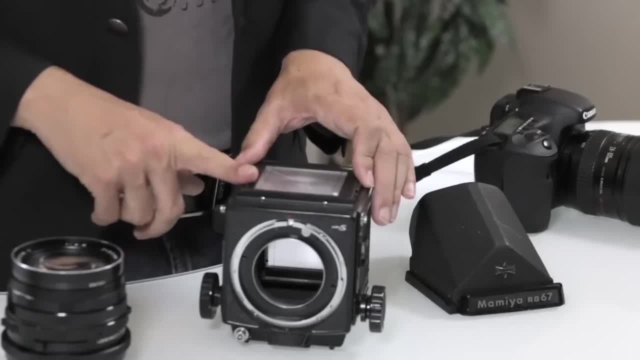 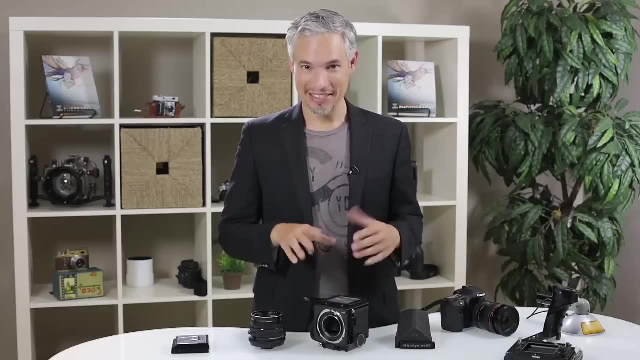 mirror is doing is reflecting the light onto this focusing screen so that it's sharp, And when you're looking through the viewfinder, you're looking through the lens and you're looking at the focusing screen, because this is catching all the light and basically replaying. 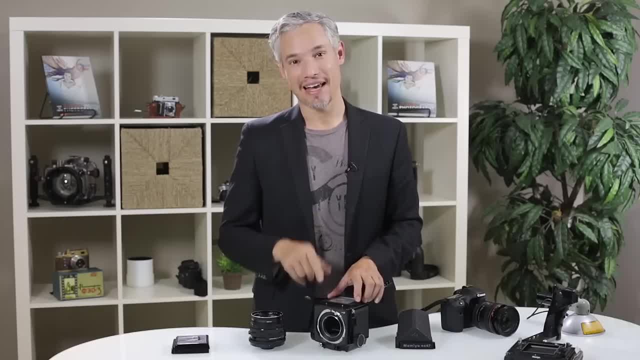 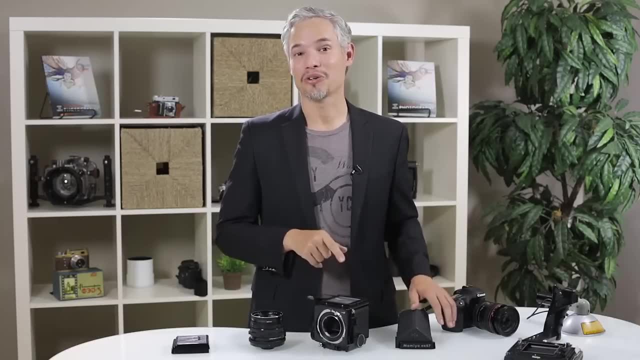 it back through the viewfinder for you, And because it's the exact same distance from the mirror as the film. if the image that you see on the focusing screen is sharp, then you can be sure that the image on the film is also sharp, And that's part of the brilliance. 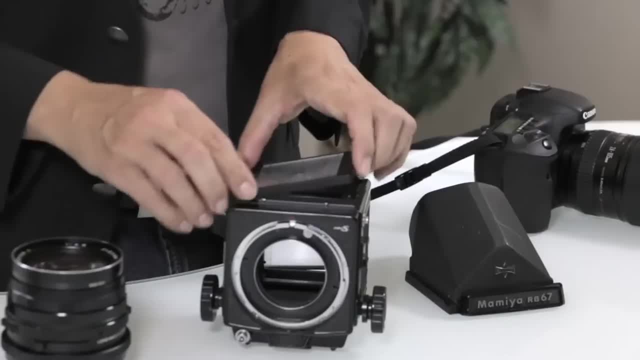 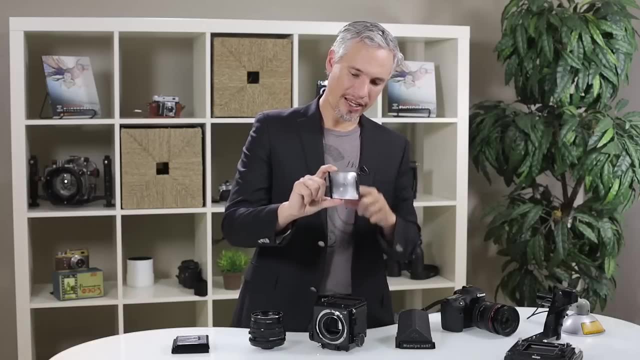 of the DSLR design. So I'll take out this focusing screen, because these old viewfinders used to have many different focusing screens that you could swap out, And I'd just like to show you that it has a special area in the center there and that helps with manual. 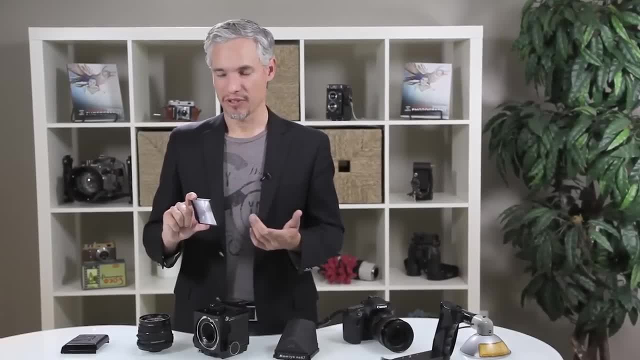 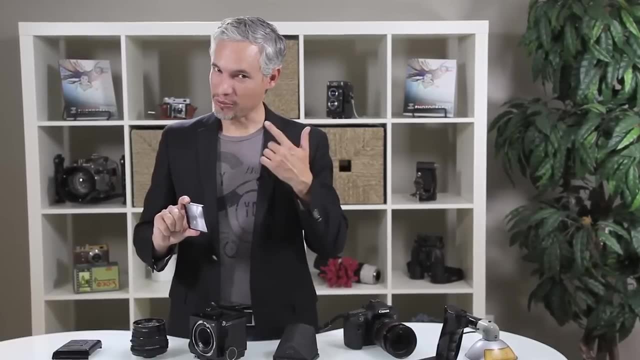 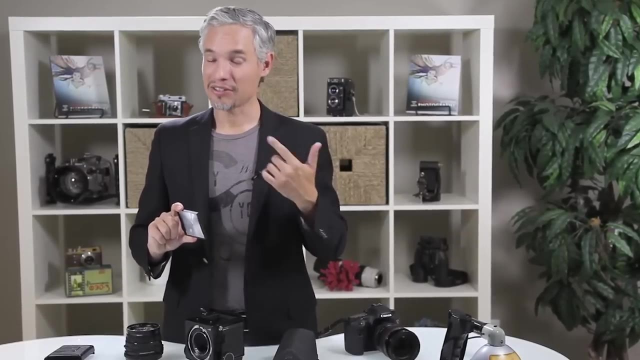 focusing. There are many different designs here: split prism designs- This happens to just be a ground glass design- but these designs all made it much easier to manually focus, because if you just had a regular piece of glass, you just wouldn't be able to easily. 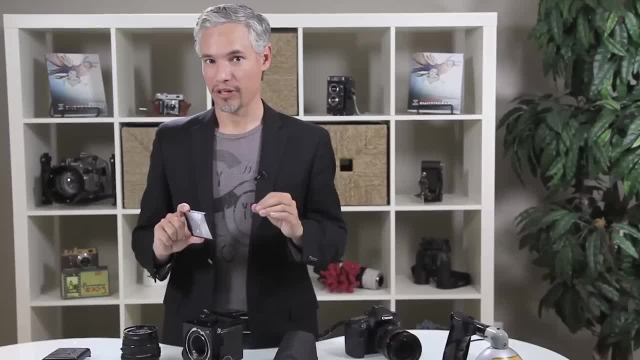 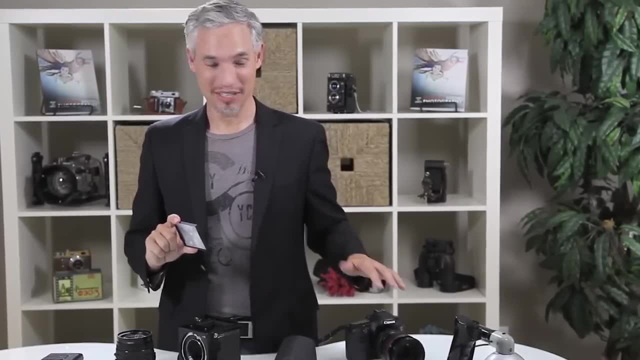 determine whether your image was going to be perfectly sharp or not, because your eye just doesn't have that much resolution. So I know a lot of people who try to manually focus with their modern DSLRs and it just isn't very precise. Your camera has special 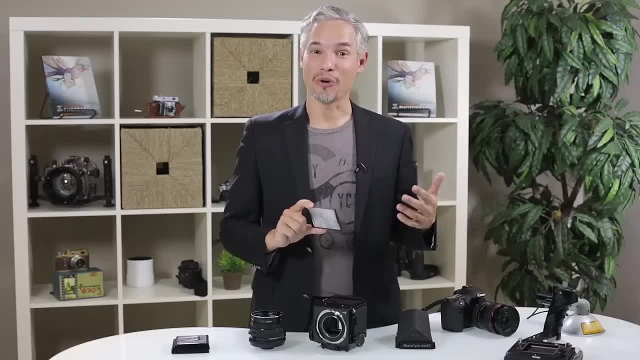 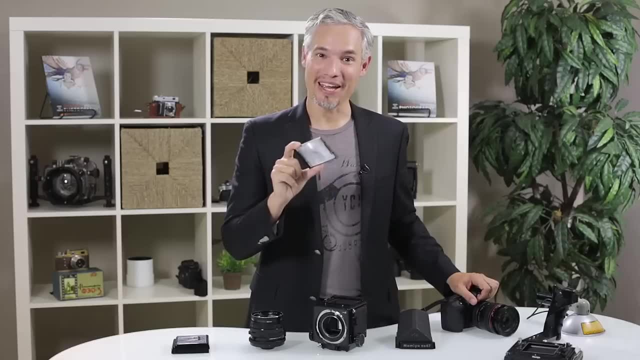 focusing points in it and technology that allows it to focus using basically a split prism technique, but your eye isn't that good at it And they didn't give you a focusing screen in your camera to enable manual focusing And, as a result, manual focusing is really. 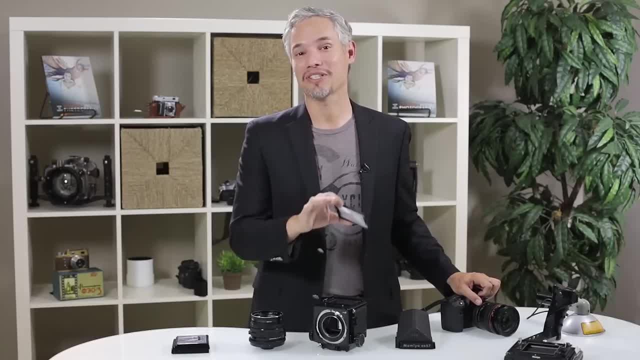 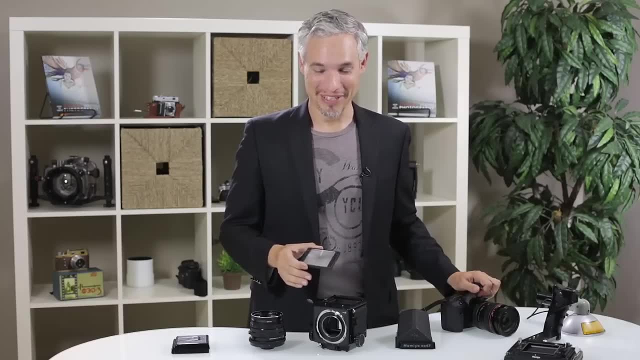 hard on DSLR cameras, So for that reason, I really push people to use auto focus, even when manual focus might be more attractive. Now, if you're using these old cameras, you've got these tools built in and manual focusing is much easier. 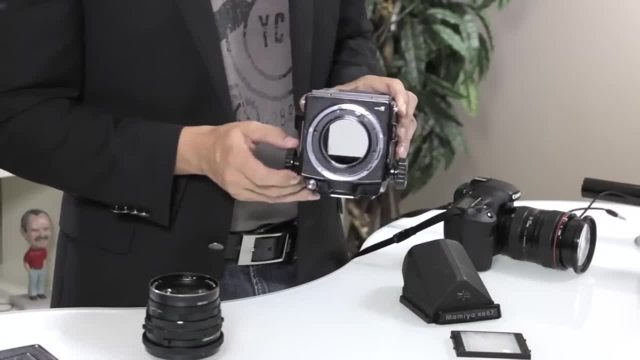 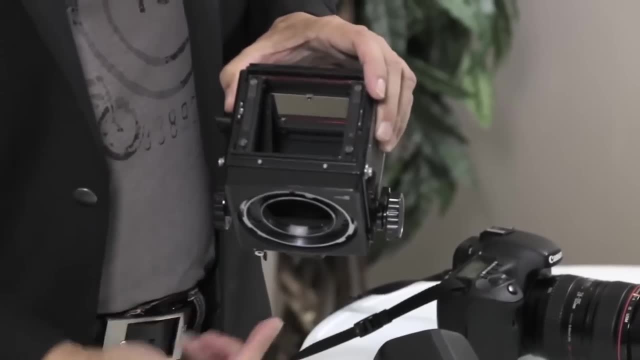 So with that off, we can now see the mirror clearly from here or from the top. So as I flip through, you can kind of see that the mirror is reflecting light that's coming in here and then it's coming back out the top, It's hitting the focusing screen and then 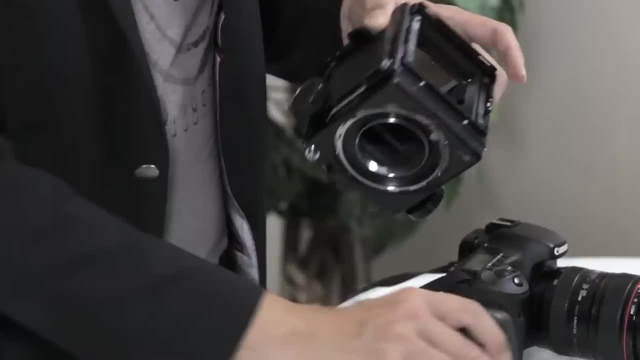 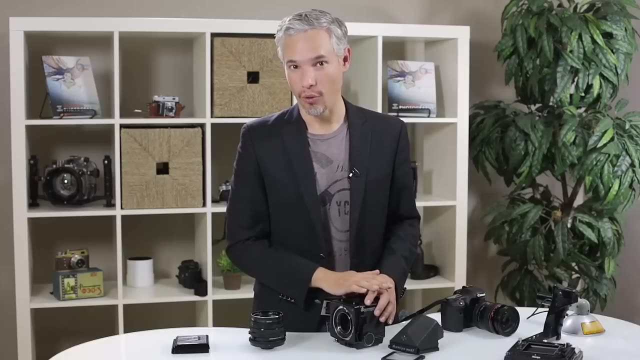 going through the prism and finally to your eye here. So I hope that tour of a really old camera helps you understand the individual components of your modern DSLR or mirrorless camera. Now let's talk about the different focusing types that your camera supports. If you have, 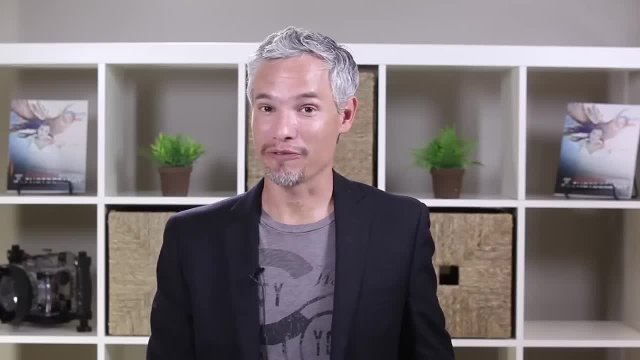 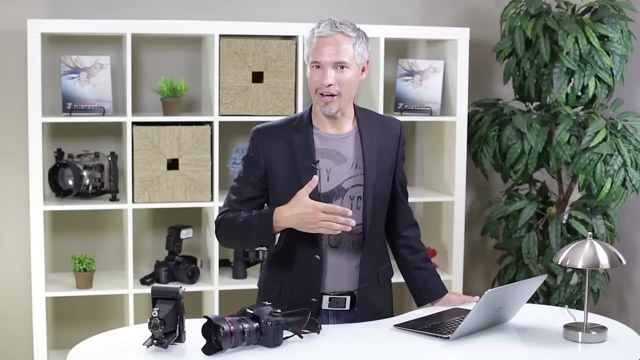 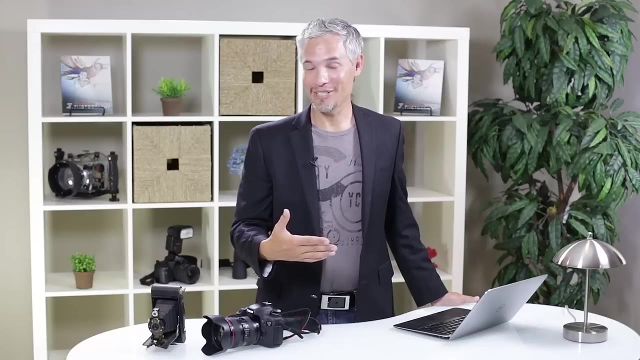 a mirrorless camera or point and shoot camera or camera phone, you have one focusing type and that's contrast based focusing. The way contrast based focusing works is it focuses the motor in or out until it sees things getting sharper And then, when it stops getting sharper and it starts getting blurrier again, it backs. 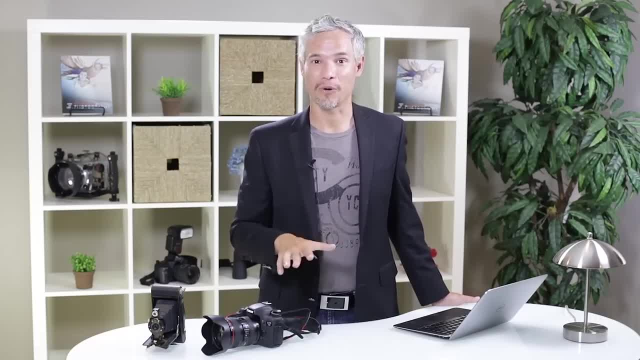 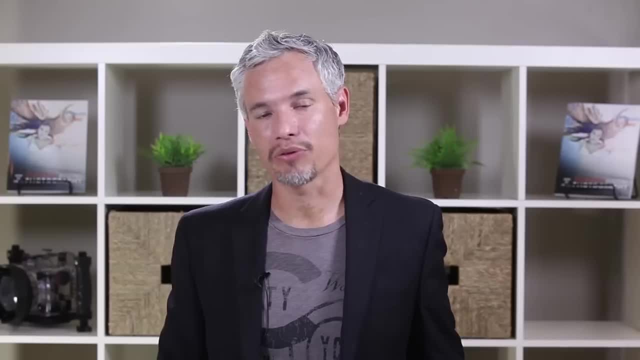 up a little bit and it knows the part of the scene is in focus. Contrast based focusing can be a little slow, especially in older cameras, but some of the most recent cameras coming out in 2013 and later have gotten really fast contrast based focusing systems. So some 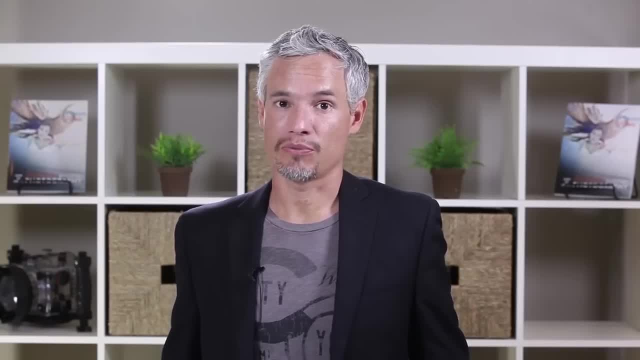 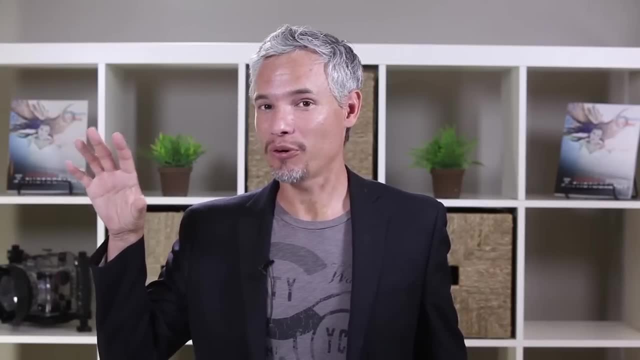 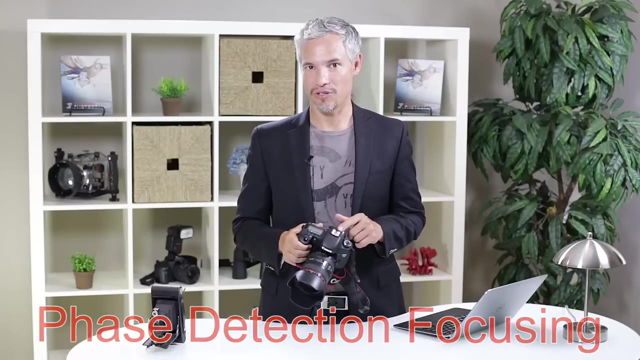 of the disadvantages have disappeared. Contrast based focusing systems also usually allow you to focus basically anywhere in the frame, So you can pick a focusing point right in corner of the frame and it will focus there. That's in distinct contrast to phase detection focusing, which is how SLRs focus whenever you're looking through the viewfinder. Now, if you have a 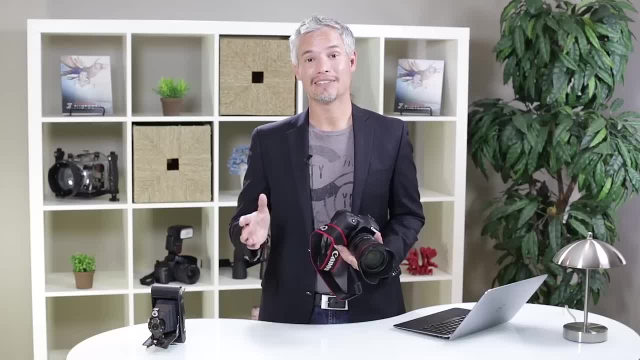 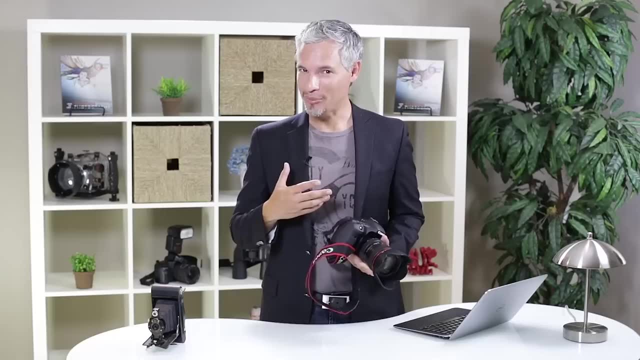 mirrorless camera. well, you don't have phase detection focusing, because phase detection focusing relies on that mirror that I was telling you about. It's not just a true mirror that reflects all the incoming light. No, it sends some of the light through it. It's partially translucent and 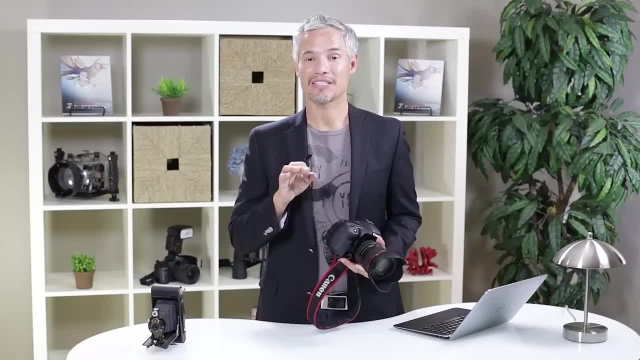 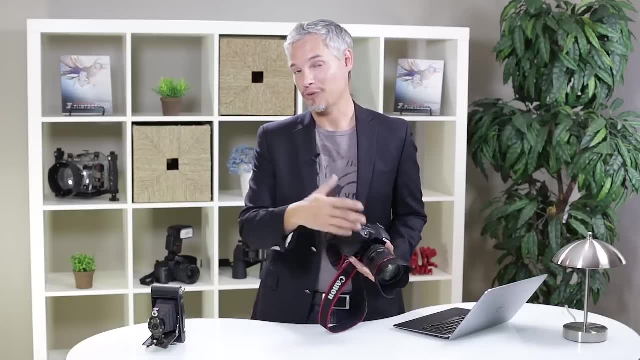 it sends some of that light over to specialized phase detection sensors, and these sensors have the exact format that you see of the focusing points when you look through the viewfinder. So if your camera has nine focusing points, well it has nine little phase detection sensors in. 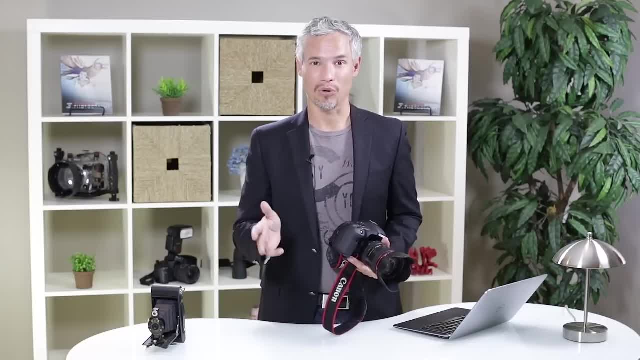 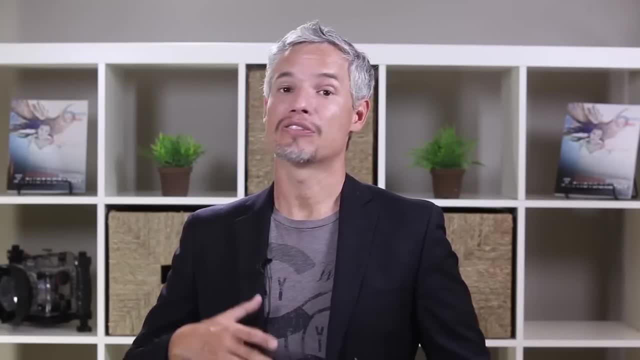 there, And if your camera has 50 something points, well, it has a lot more. So phase detection focusing only works when you're looking through the viewfinder of an SLR, but it's pretty much always faster than contrast based focusing, And if you're shooting moving. 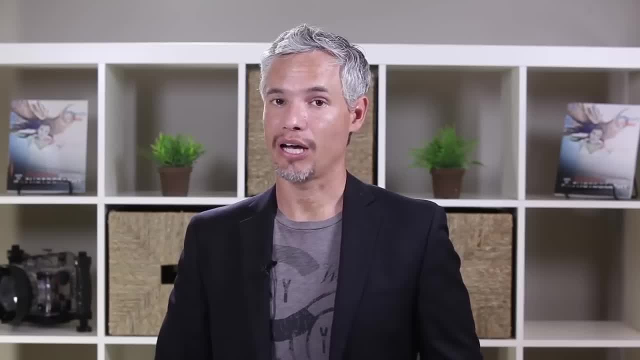 in the background, you're going to see a lot of light coming through the viewfinder And if you're shooting moving cars or flying birds, or even a wedding somebody walking up the aisle, you probably want to be using that phase detection focusing. We'll go into the exact details of 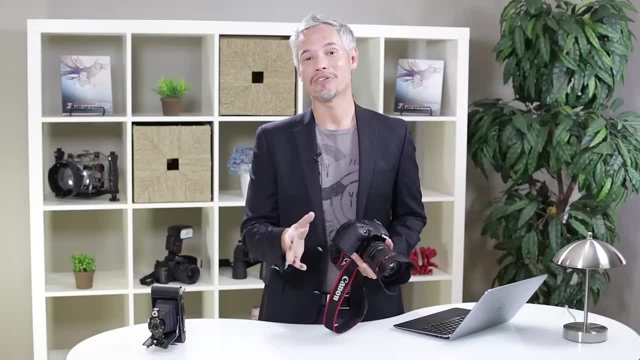 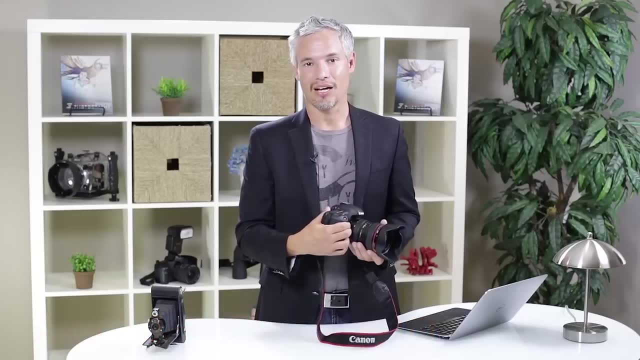 how to use focusing in just a little bit. And of course, the other major type of focusing is manual focus. With manual focus, well, sometimes you're adjusting a button on the camera, but usually you're moving a dial on the camera like this to adjust the focus in or out, just according. 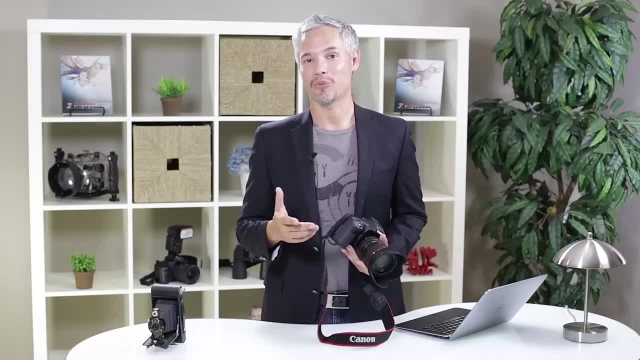 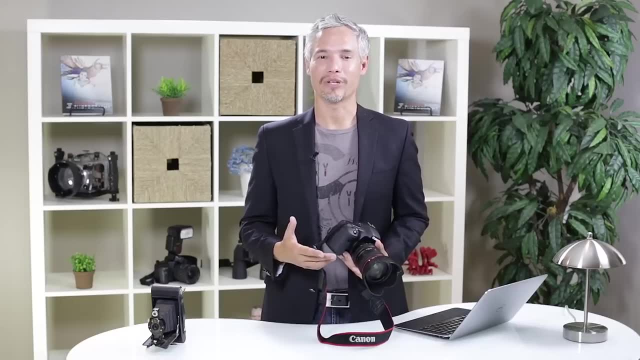 to your own eye. Manual focusing used to be really popular with older cameras, and so some people think: well, you know, because my grandfather manually focused, I should be manually focusing too. But that's probably not true, because your grandfather probably had a specialized viewfinder. 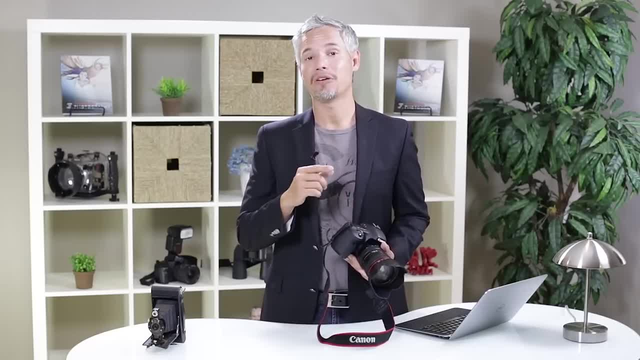 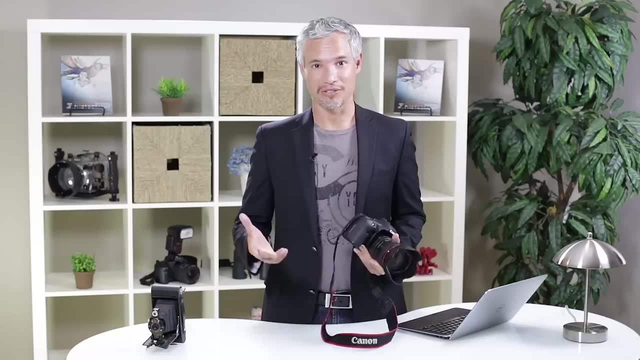 Maybe it had ground glass or a split prism viewfinder that allowed him to very precisely manually focus, And our modern cameras just don't have that. Instead, we have an awesome autofocus system which is more precise and better, So you'll find that I generally 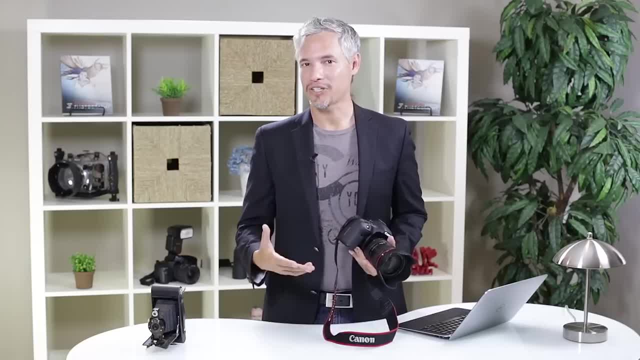 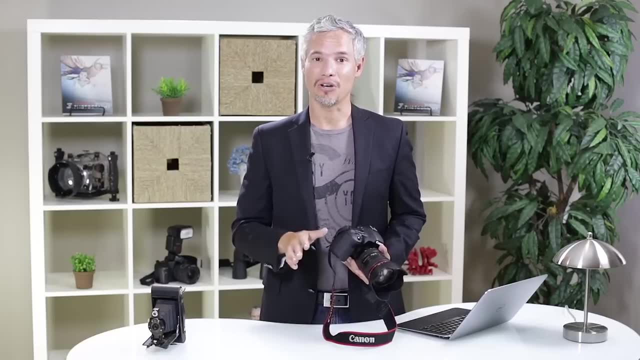 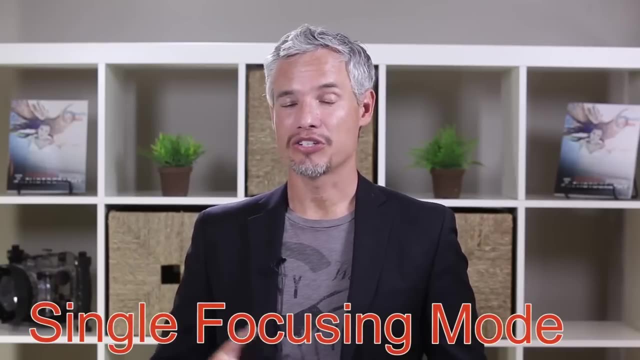 discourage the use of manual focus outside of very specialized uses like night photography and macro photography, Then you'll be using manual focus, But for everything else, get to know your autofocus system. Cameras in general have three different focusing modes. They have single focusing mode, which changes the focus and then locks in on a subject and freezes. there. There's. 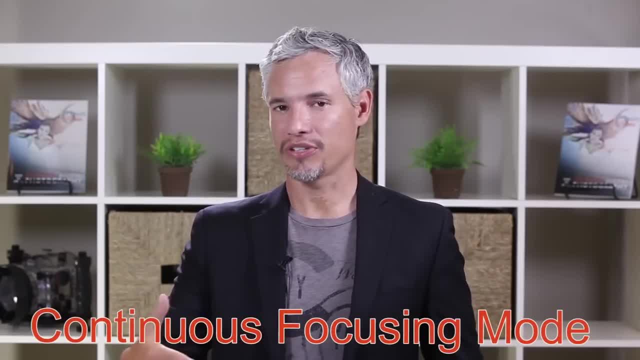 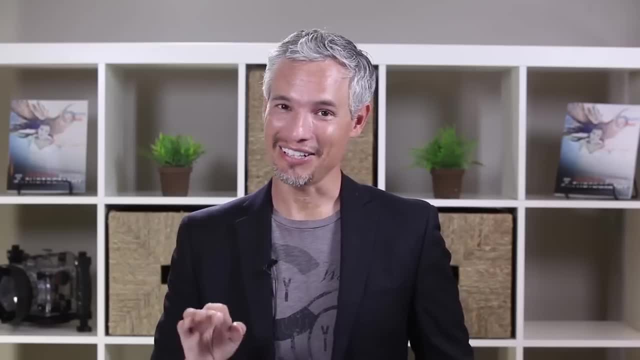 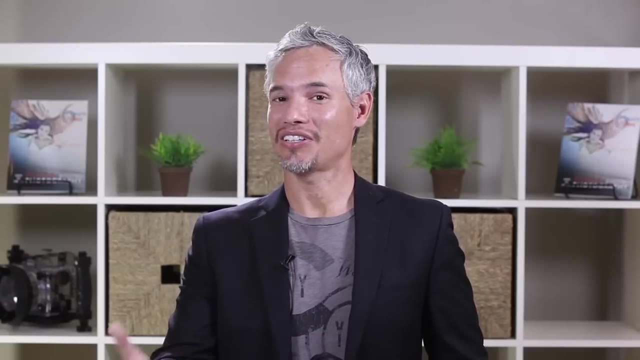 also a continuous focusing mode which tracks a moving subject, Whereas single focus will catch, focus and then stop, even if the subject moves. continuous focus is constantly trying to refocus on the subject. So if you're focusing on the bride and she's standing still and then she suddenly starts walking down the aisle, 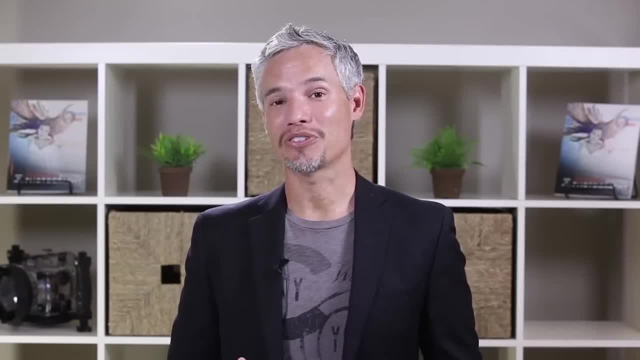 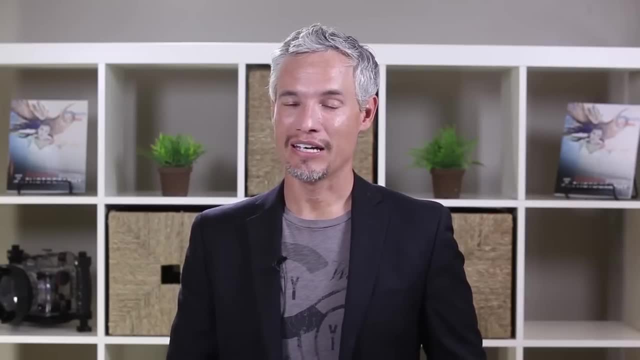 continuous focusing will at least try to keep up with her. Single focusing would just stay focused at the back of the church. The third focusing mode that consumer level cameras have is sometimes called AI servo or some kind of intelligent or automatic focusing, and it's designed to automatically switch between single and continuous focusing modes. You'll find that. 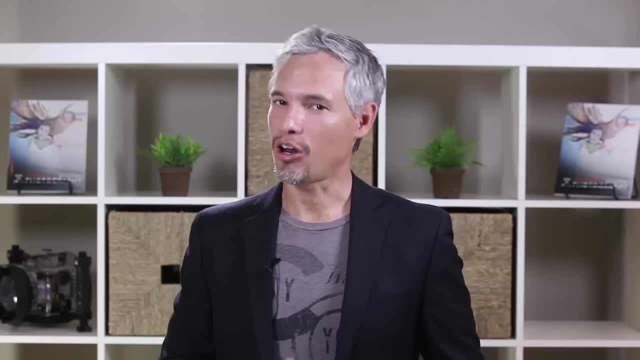 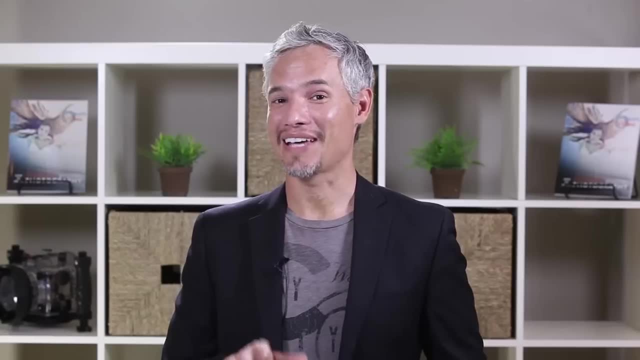 I'll talk a lot about single and continuous focusing, because the automatic mode is more for people who are using the automatic modes of their camera and because you're going through these videos, you're going to know exactly how to use your camera and you'll be switching between automatic 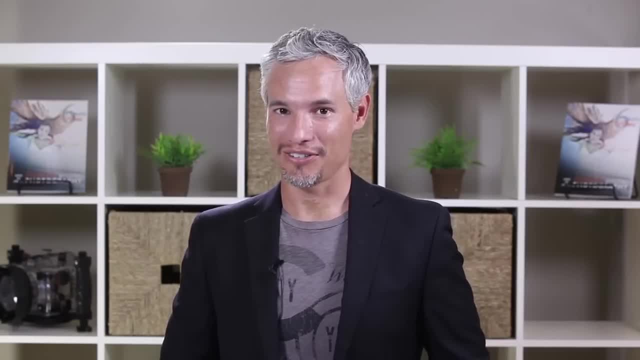 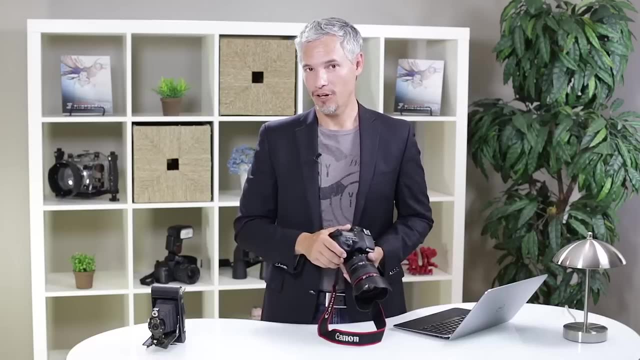 and continuous all the time, but you won't have to use any artificial intelligence. Now, I mentioned earlier that phase detection autofocus has multiple specific autofocus points By default. when you turn your camera on, it will probably pick whichever one it thinks is the one that you want. In other words, 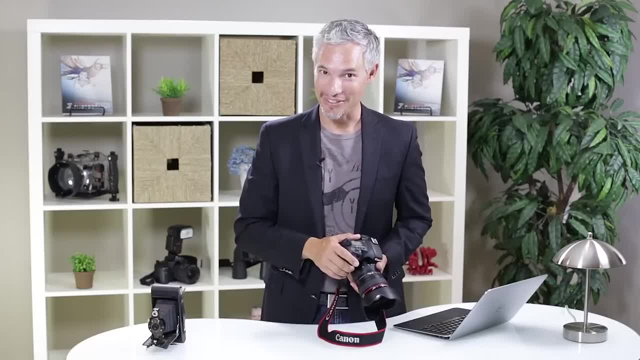 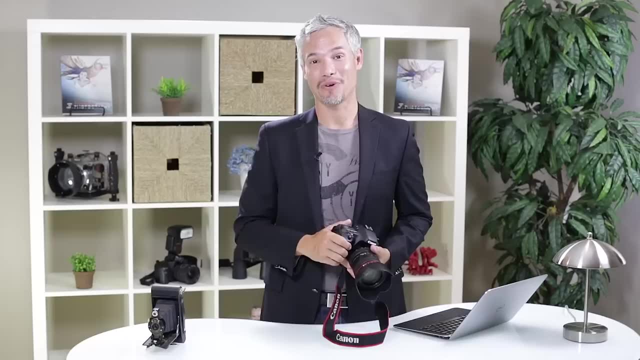 that's a different kind of autofocus. If you're going to be using a camera that's going to be focusing in the picture, that seems like a terrible idea, right? If you have autofocus pictures sometimes it very well might be blamed on your camera's focusing system, just deciding. oh, I'm. 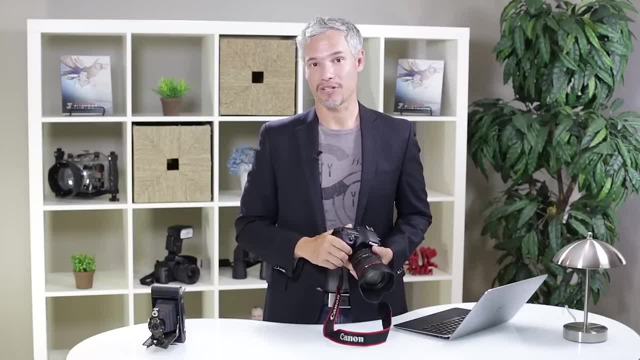 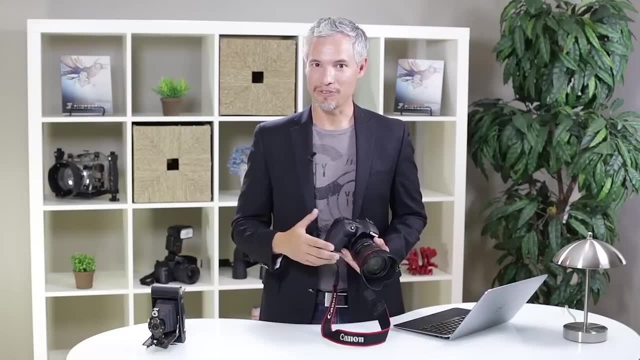 going to focus up here. Usually the way the automatic focus point selection works is it picks whatever is closest in the frame and if you're using a fast lens with a short depth of field, well, it might focus on my camera instead of focusing on my eyes up here, and it would just lead 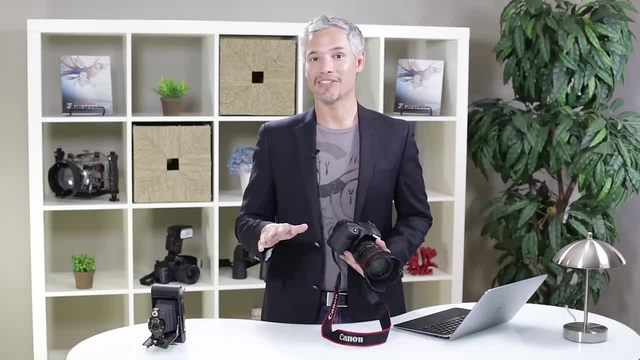 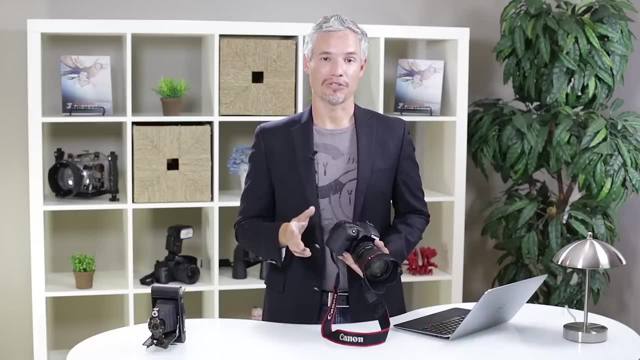 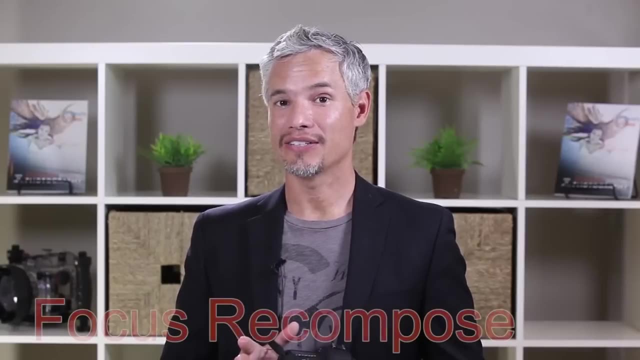 to an unfocused picture. So I always recommend choosing a single focus point and putting it wherever it is you want that focus to be- on your subject. Now let's talk about a few different techniques for getting your subject in focus. The most important technique is focus and recompose, and with focus and recompose, you use any. 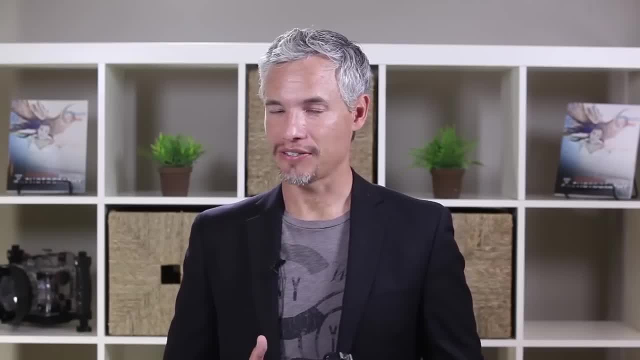 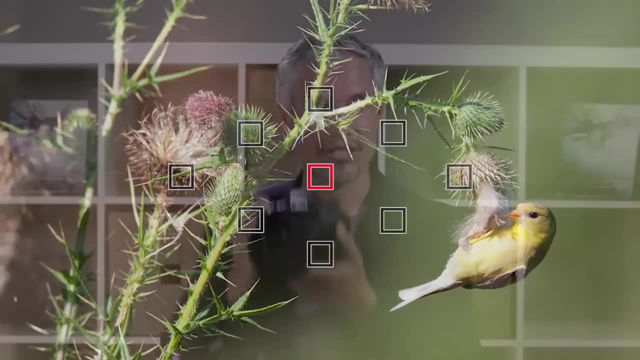 focusing point. It can be the center focusing point, which is almost always the fastest on a camera, and you'll focus on a subject, push the shutter halfway down and then recompose. So if you're using that center focusing point, you'll pull up the camera and put that center. 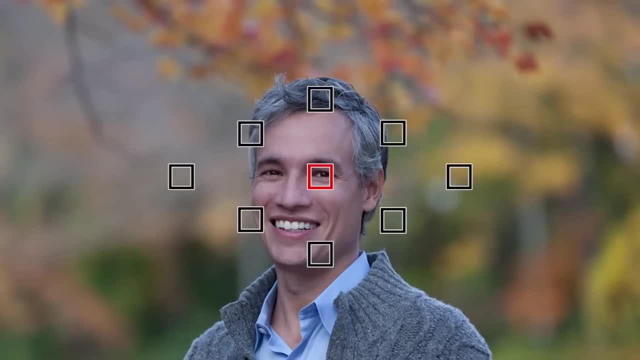 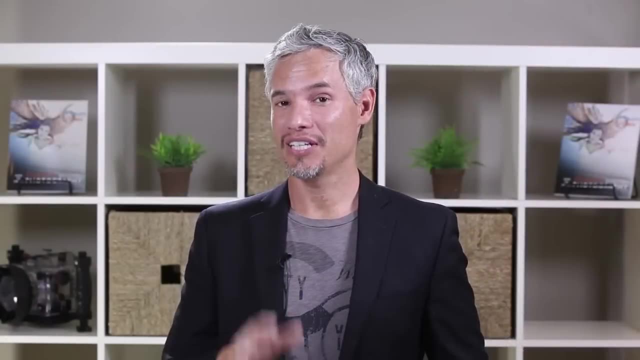 focusing point right on the person's eye. You'll put the shutter halfway down to lock the focus and then you'll recompose the picture. This will only work in single focusing mode. If you're using continuous focusing mode, you'll have to switch over to single for focus recompose to work. 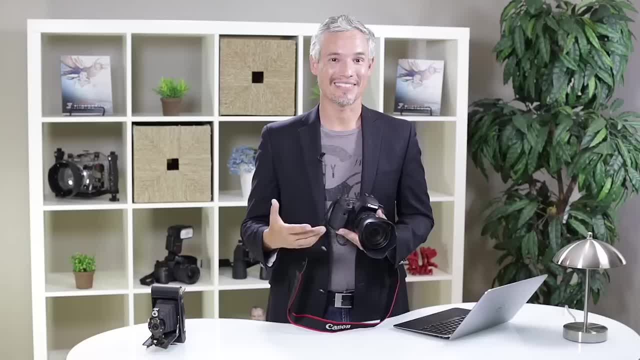 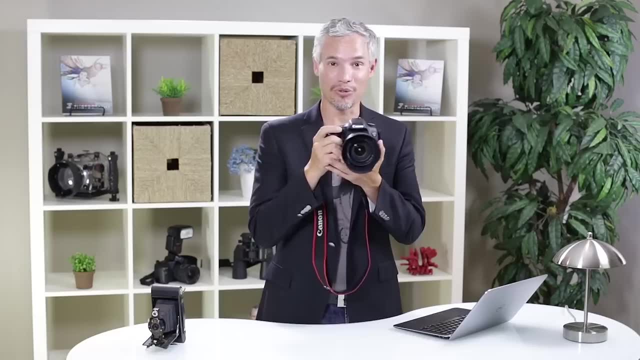 Now focus, recompose isn't an especially precise technique, As you can imagine, when you hold your camera up to your face and then recompose it. well, you're waiting a second before you actually take the picture from the time that you focused. Your body also might move in or out, or whatever you're. 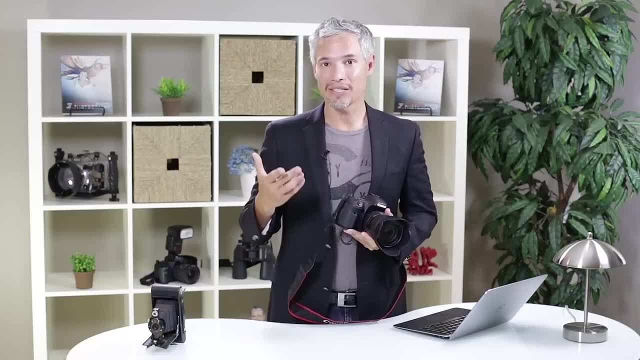 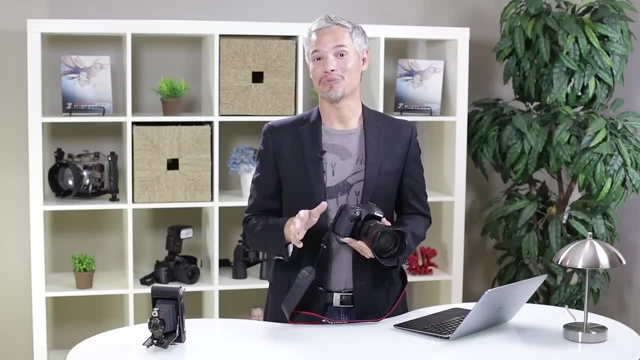 taking a picture of might move in or out, and that's enough to make the eye seem a little bit out of focus at times. Now, you might never notice this with your SLR and your kit lens, but if you buy an expensive professional lens or a portrait lens, you can bet that you'll see the difference. 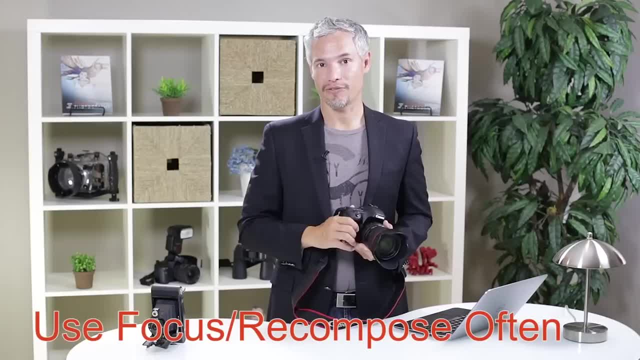 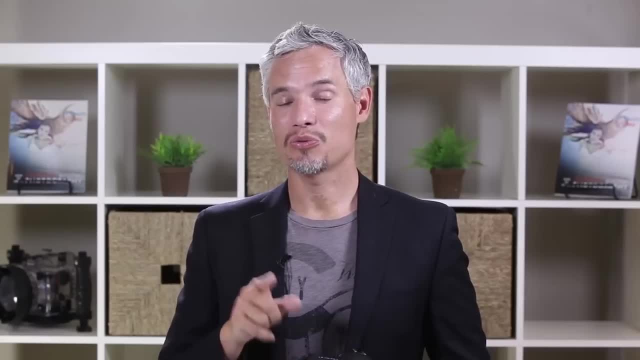 Nonetheless, I still recommend that people use focus recompose often, especially on lower end bodies. If you have that basic kit, that's great, but what I would do is switch over to the focus recompose mode and switch to the center focusing point only and rely heavily on focus recompose. 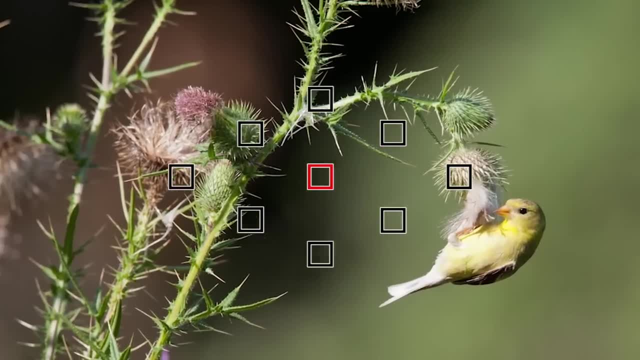 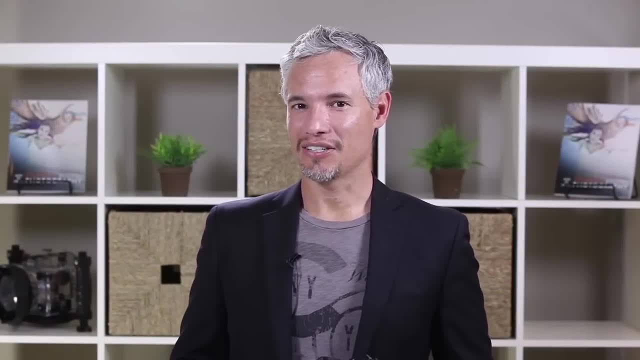 and you'll probably never notice the focusing problems. I really only mention the lack of precision with focus recompose, because a lot of people would otherwise bring it up. They'd say this isn't always the best technique to use, but you know what, with basic cameras, I think it really. 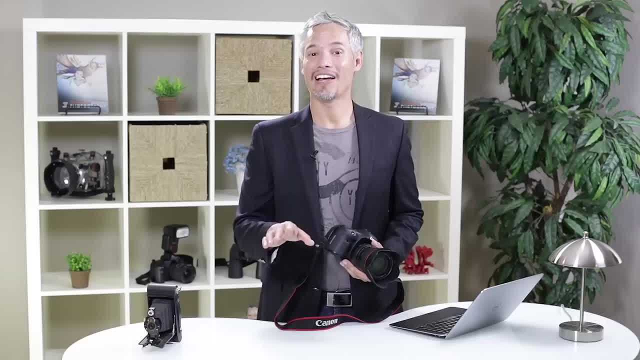 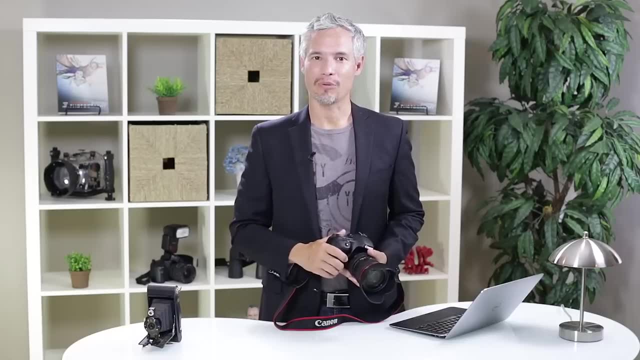 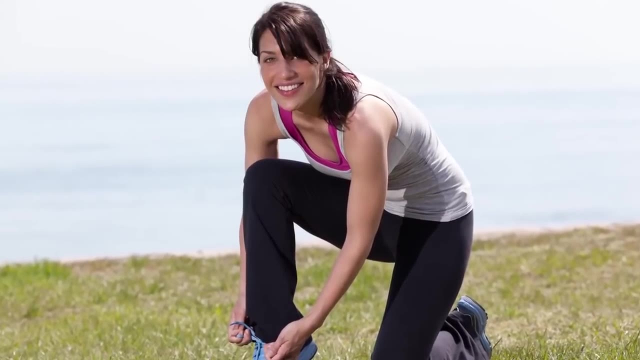 is the best technique to use for most subjects. So now let's head outside and do a fitness stock photo shoot with Chelsea. So there are lots of different scenes in a fitness shoot. Some are still. for example, maybe she's tying her shoe or drinking some water. Others are moving if she's running along in the beach. 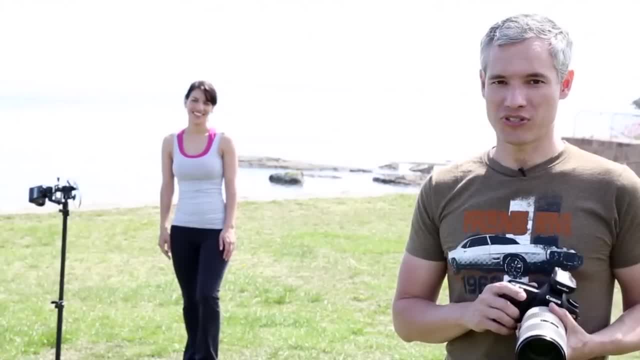 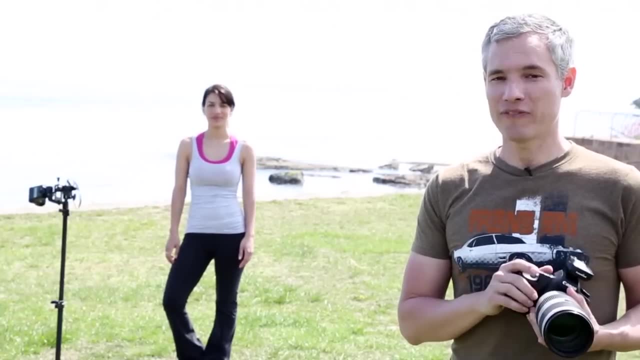 and, depending on the type of shot, you're going to want to change your auto focus system. So we'll start with the simplest, which is most cameras default. It's called a one shot, or AFS. Now, when you have this focusing mode selected, you can push the shutter button halfway. 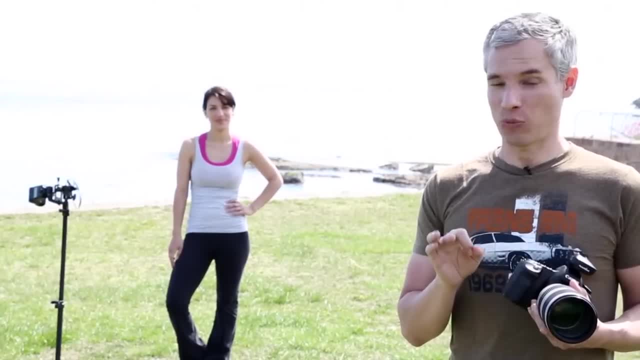 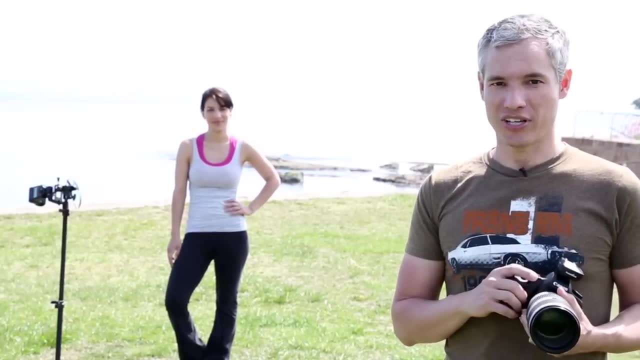 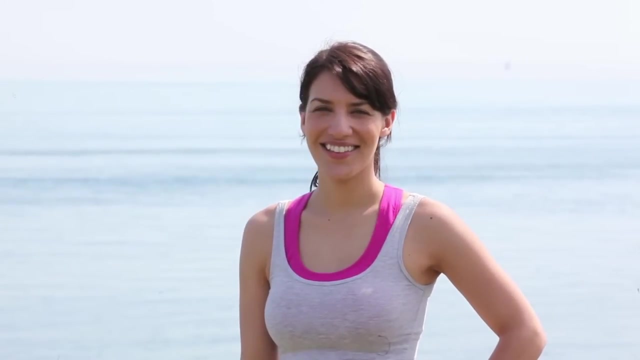 and the camera will grab focus for you Once it gets it, it will stop trying to focus and wait for you to push the shutter button all the way to take a shot. So let's take a shot of Chelsea with one shot selected. One shot is perfect anytime you're photographing a still subject. Now, usually the camera will have 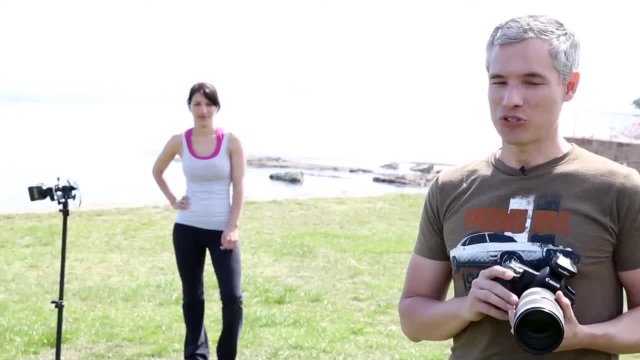 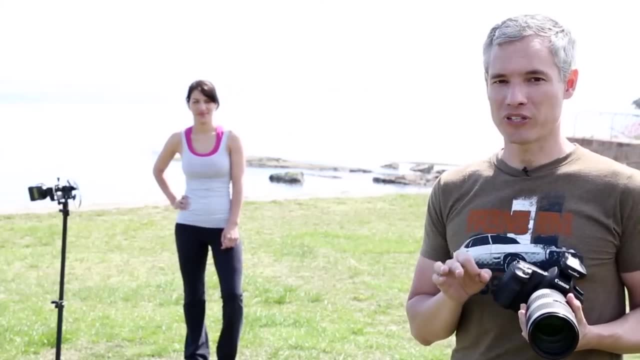 all auto focus points selected. That might not be exactly what you want. It might pick the wrong subject to focus on, So most of the time I select the single center focus point. However, if you read chapter two, you learned that the rule of thirds is one of the most important. 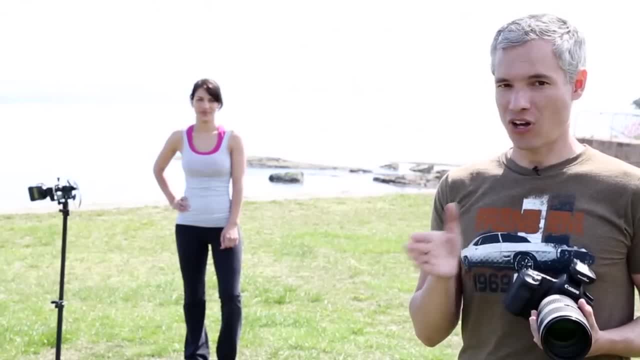 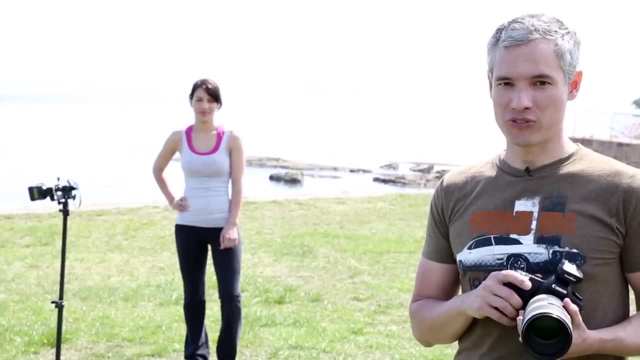 compositional rules. When you use the rule of thirds, you want to place the subject off center. So what do you do if the camera always wants to focus in the center? I use a technique called focus recompose. I hold the shutter button down halfway until it focuses, and then I will shift. 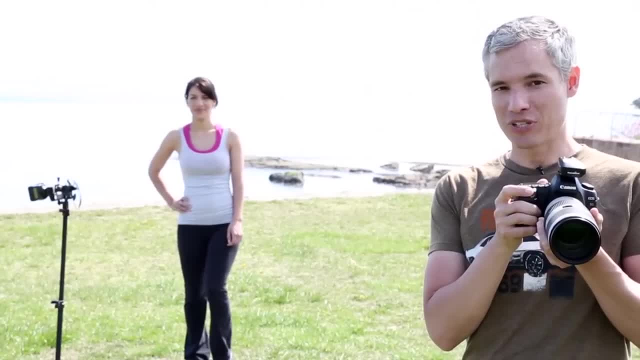 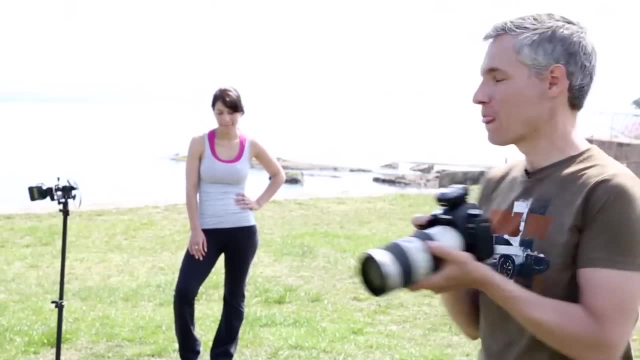 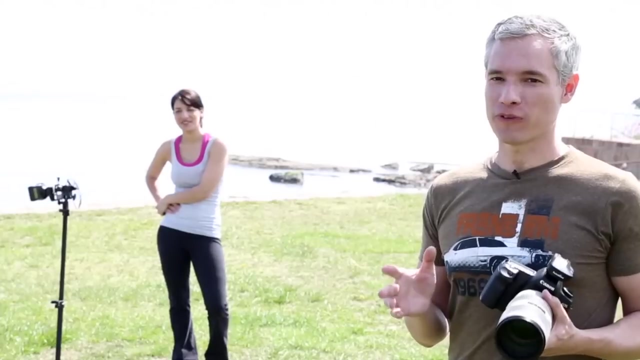 my camera and frame the picture the way I want. Once I've got it framed, I can push the shutter button down all the way, So I'll try that again. to place Chelsea in the right third of the frame. Focus recompose is my preferred technique because every camera focuses the best with. 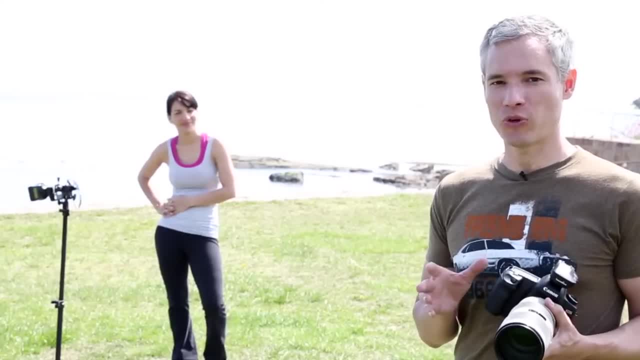 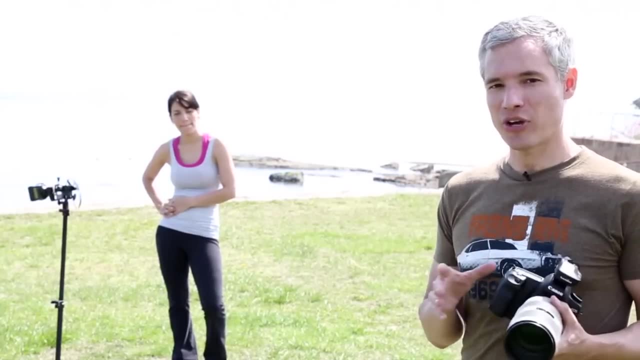 the center focusing point. However, many cameras have multiple focusing points and they all might be very usable. Whether or not you can use these other points effectively depends upon the lighting, the contrast of the subject, the speed of your lens and your camera body. So there are a lot. 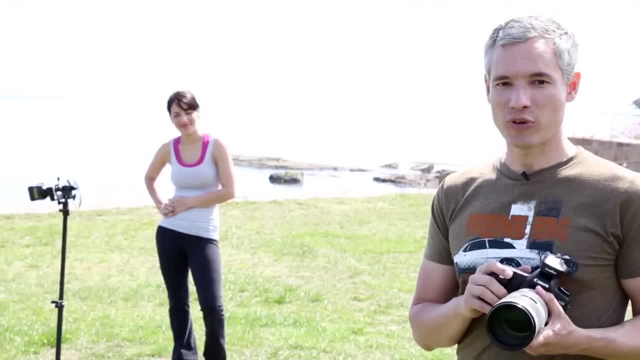 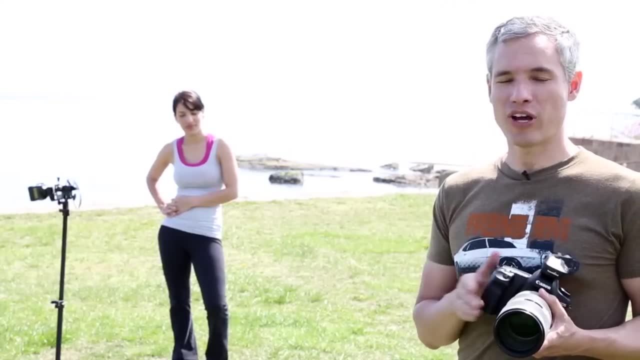 of a lot of factors at play. However, if you want to try out the other focusing points and see how they work, you should do that. If you want the subject to be in the right third of the frame, for example, you can select a focus point that is over there. Then you don't have to recompose. 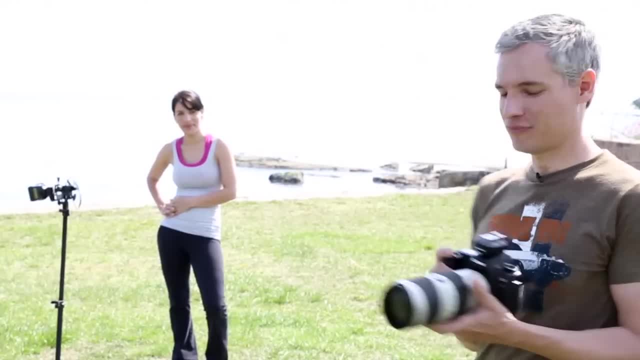 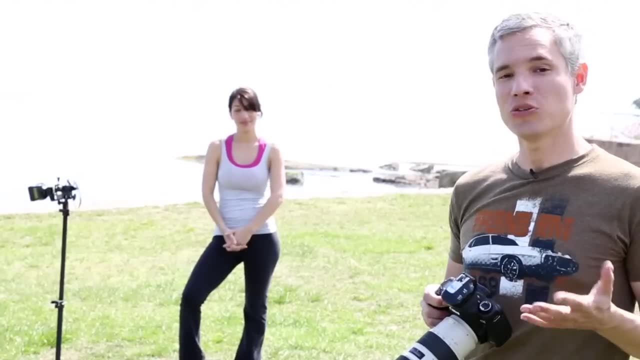 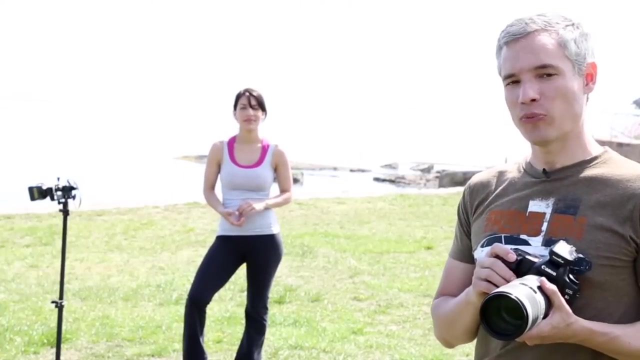 You can simply focus and shoot, So let's try that. When you have a moving subject, you want to use continuous auto focus, which is called either AI focus or AFA. This will continue to focus while you have the shutter button pressed halfway. When the subject moves, your focusing system will try to keep up with it. 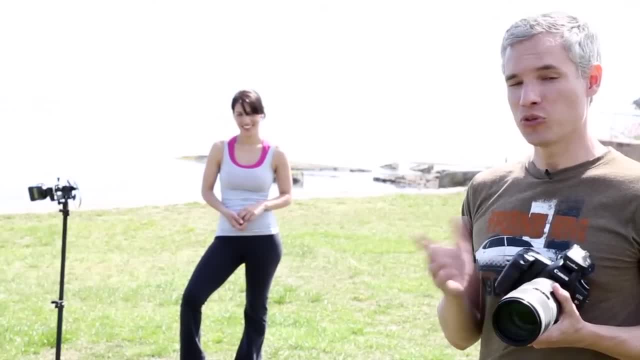 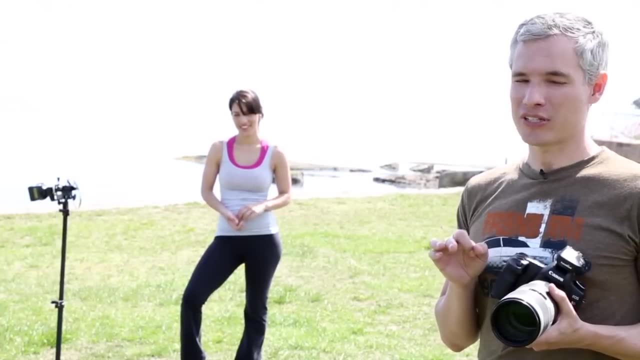 When you push the shutter button all the way, it will take that shot. If you use your camera's automatic modes, you can select the sport mode, and it will usually get it done. This allows you to keep track of a moving subject. However, it's not always perfect. 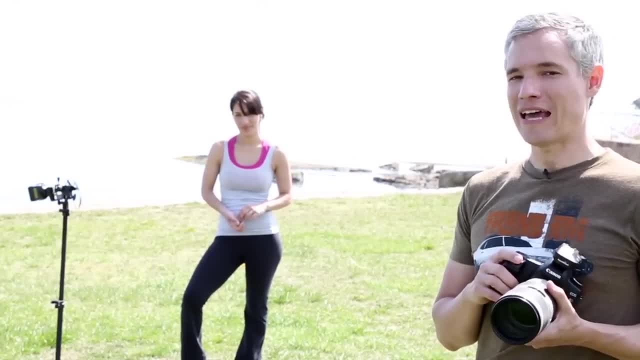 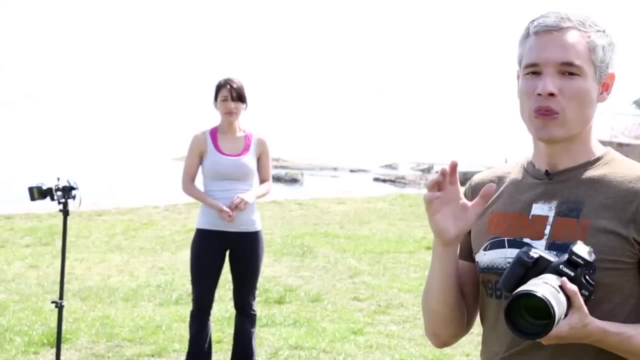 Many automatic focusing systems aren't as good as others and you'll find that you might only get one out of three or one out of four shots. It depends on the lighting, the camera body and the lens and many other factors. So put your shutter on continuous 2 and take lots of shots. 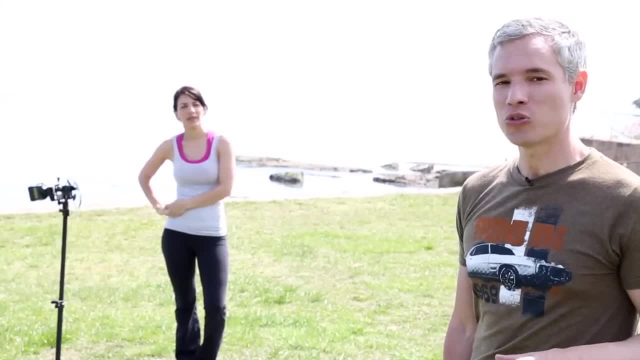 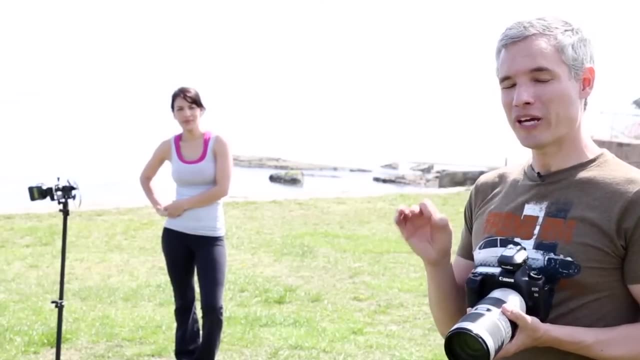 If you find that your focusing system can't actually keep up with a moving subject, you can do something called a focus trap. With a focus trap, you set your lens to manual focus, then you pick a point where the subject is going to be in the future and you manually focus there. 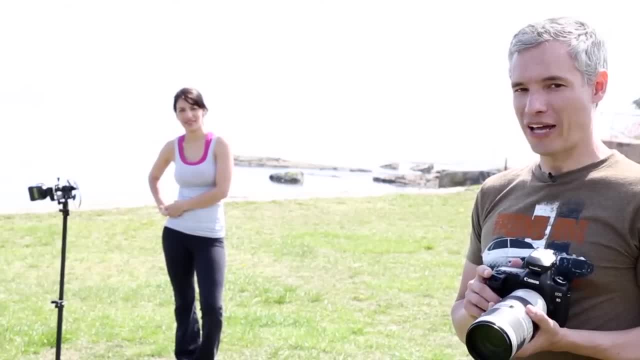 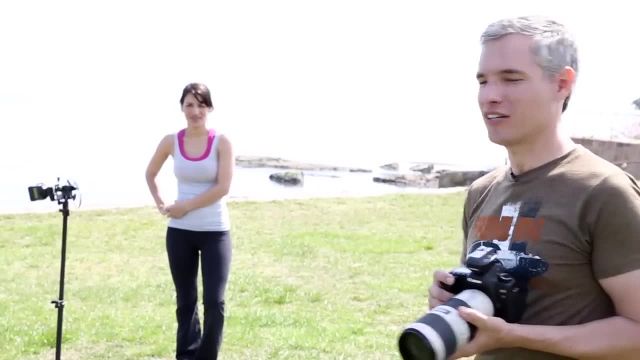 Then you simply wait. So what I'll do is I'll pick a spot on the grass and I'll manually focus my lens, Then I'll ask Chelsea to run, and when she gets to that point I'll snap a shot. Let's give it a shot. 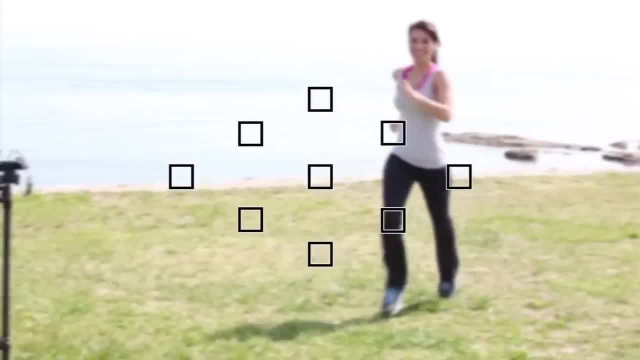 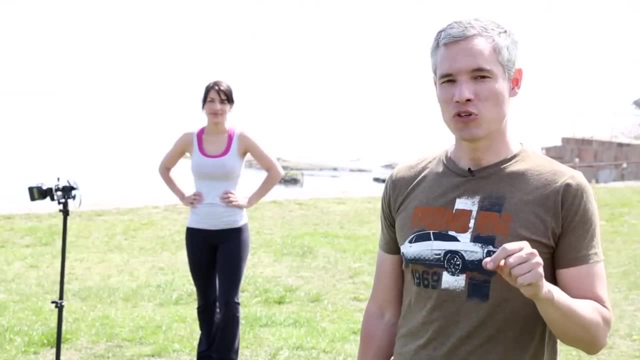 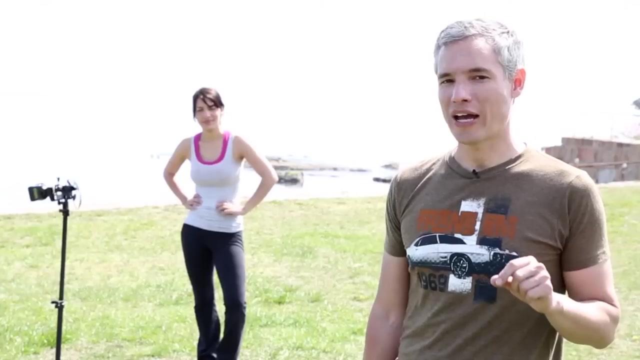 So to wrap that up, use one-shot or AF-S if you're photographing a still subject. If you want the focusing point to be somewhere other than the center of the picture, use your focus and recompose technique. You can also try changing your focusing point, but it doesn't always work that well. 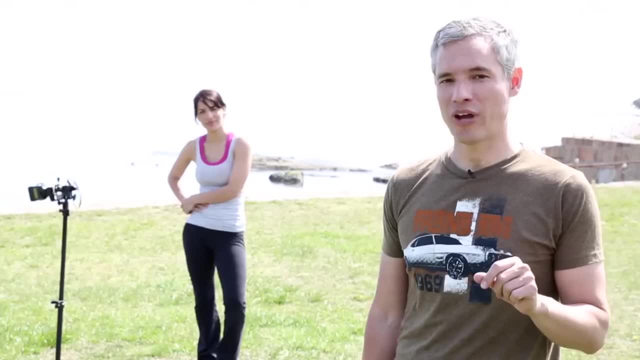 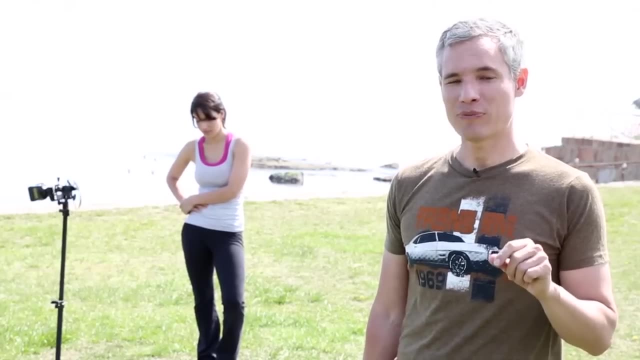 If you're photographing a moving subject, you'll want to use AI focus, also known as AF-A. That will be a little less reliable than AF-A, But it will keep the subject in focus. Just be sure to take lots and lots of shots. 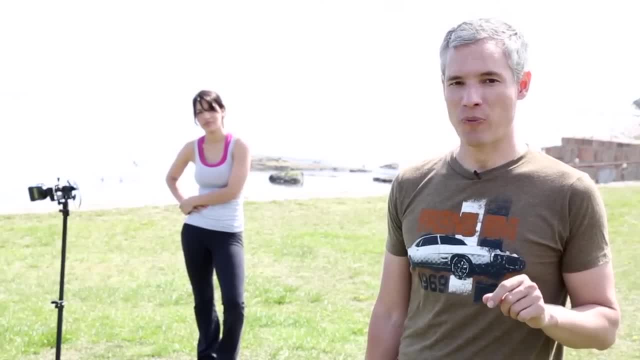 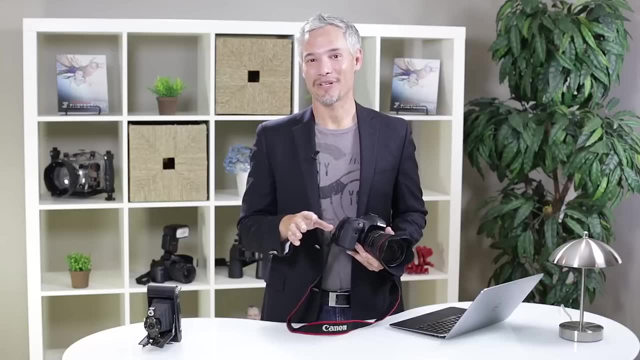 If you aren't getting good results with that, then try creating a focus trap: Manually focus where your subject is going to be and then, when they get to that point, snap a shot real quick. Another technique that I'd like to mention is commonly called back button autofocus. 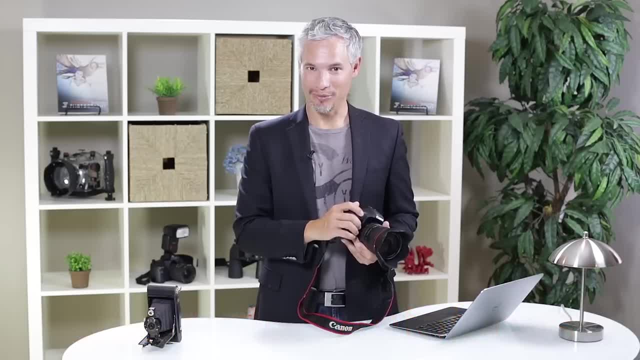 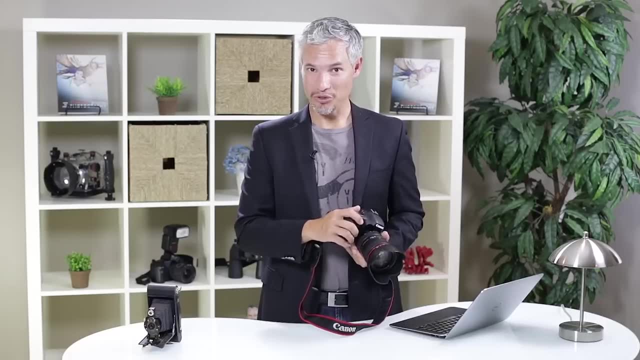 With back button autofocus, it doesn't focus when you push the shutter halfway down anymore. Instead, you have to push a separate button on the back of the camera to make the camera focus. This triggers the camera's exposure system and the shutter itself. 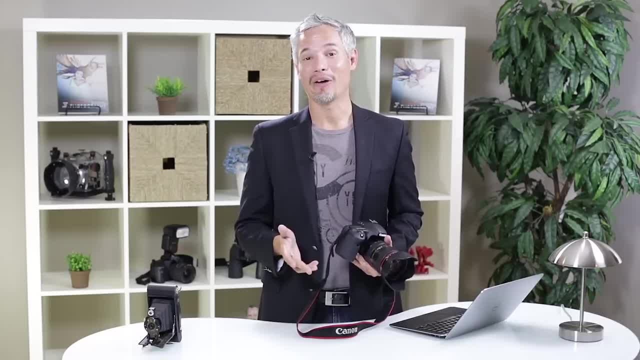 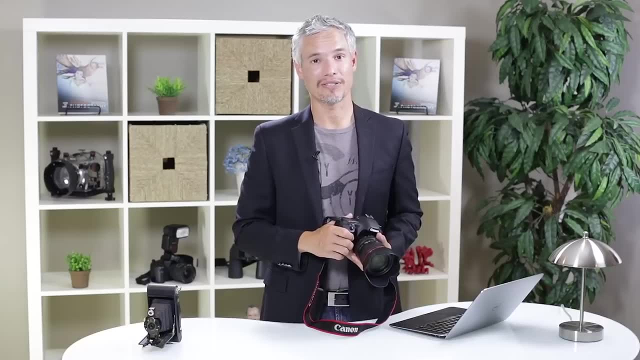 So that seems like you actually add complexity, right. Why would you want to do that? Well, I use it exclusively, as do most professionals. It's a terribly useful feature because it enables you to completely forget about whether your camera is in single focusing mode or continuous focusing mode. 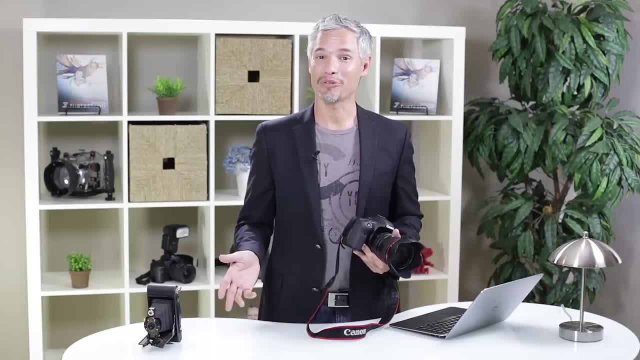 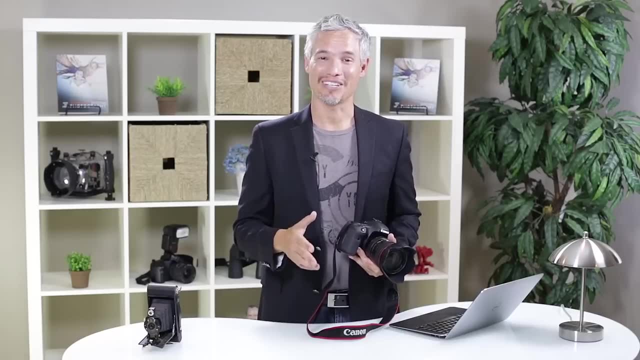 You can continuously focus all the time, and you can focus, recompose whenever you want. It really provides the best of both worlds. It just requires a little bit of practice, A couple of things. You'll have days of using it and you'll get used to it. 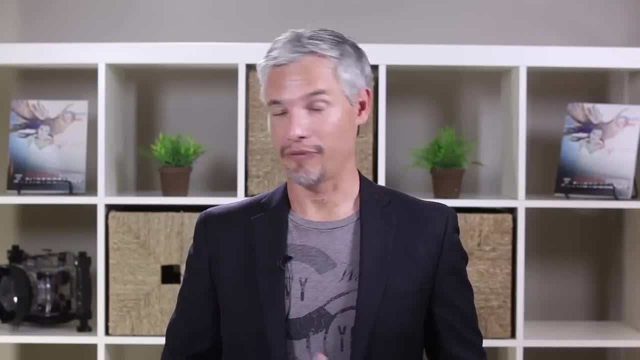 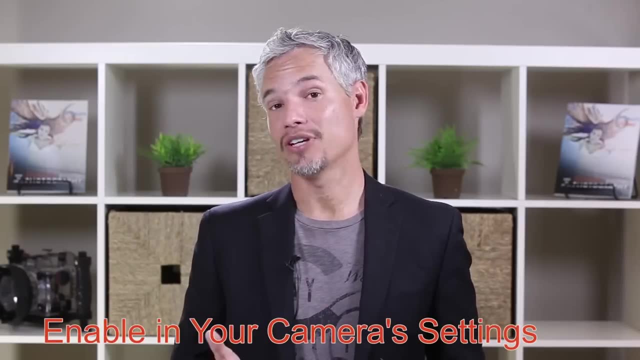 No camera that I know of has back button autofocus enabled by default. Every single camera I know. when you push the shutter halfway it tries to focus, So you'll have to go into your camera's settings to enable it. I suggest looking for the model of camera that you have, like Nikon D3100, and then 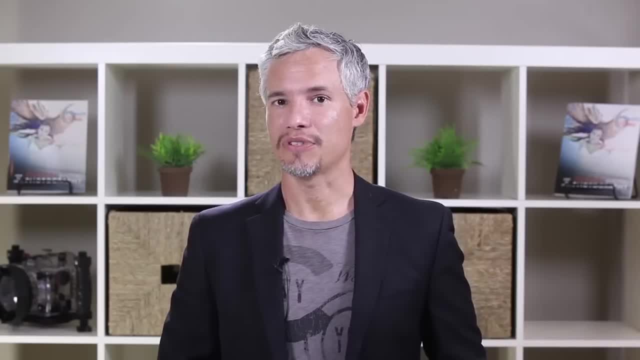 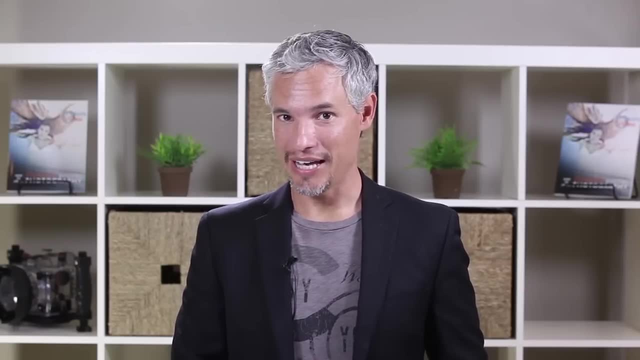 adding the phrase back button autofocus and looking up specific instructions for your camera. Usually it's a two-step process. You need to disable focusing with the shutter button, So you de-tap those two features, And then you enable focusing on some button on the back. 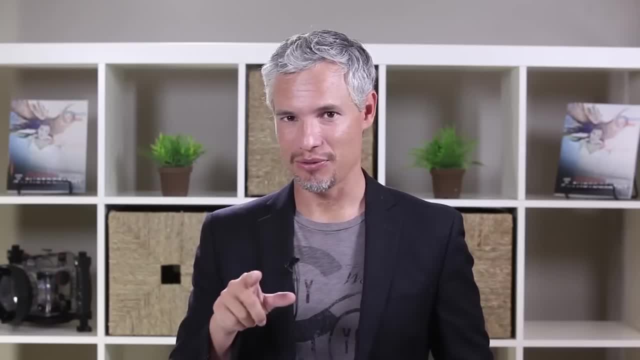 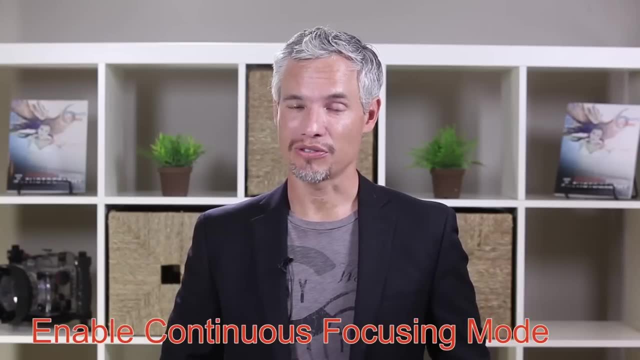 Sometimes there's simply an unlabeled button- maybe it has an asterisk next to it- that you then assign the feature of focusing. Then you'll put your camera into continuous focusing mode because you don't need to use single focus mode anymore. 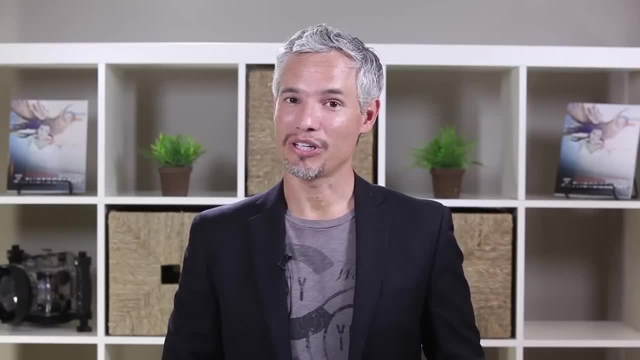 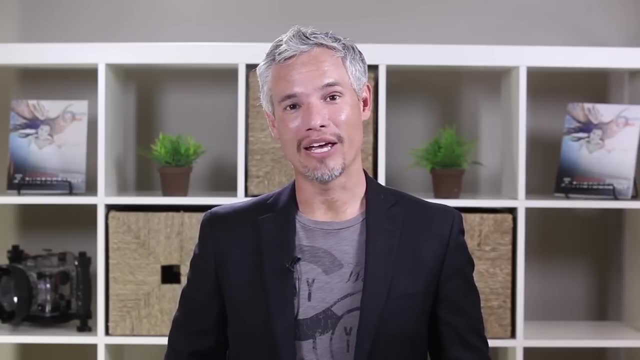 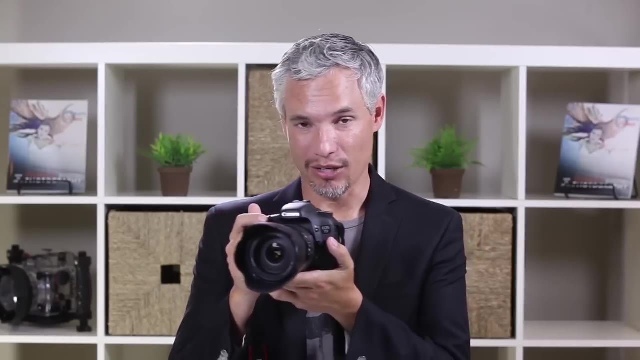 The reason you don't need to use single focusing mode anymore is you can simply release the focus button once continuous focusing gets your picture nice and sharp. So I would hold my camera up And hold down the autofocus button until I see it focus And then, if I want to re-compose, I let go of the focusing button and I can re-compose. 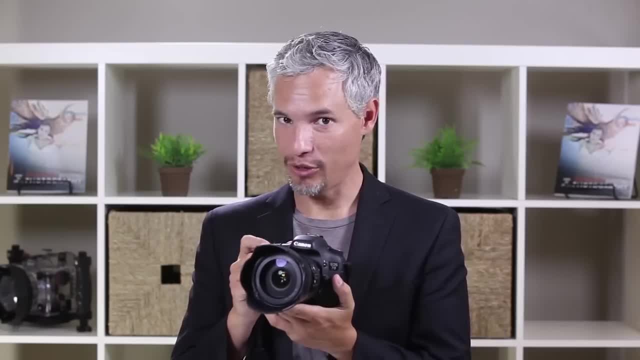 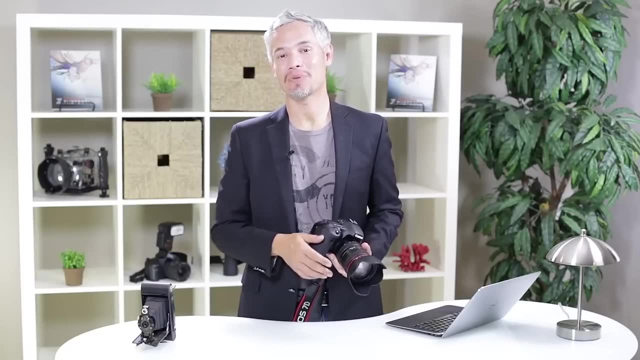 freely, and my camera won't change, focusing on me even when I push down the shutter button. If I haven't yet sold you on back button autofocus, here's an example. Imagine that you're at the beach taking pictures of your kid while he or she builds a sand. 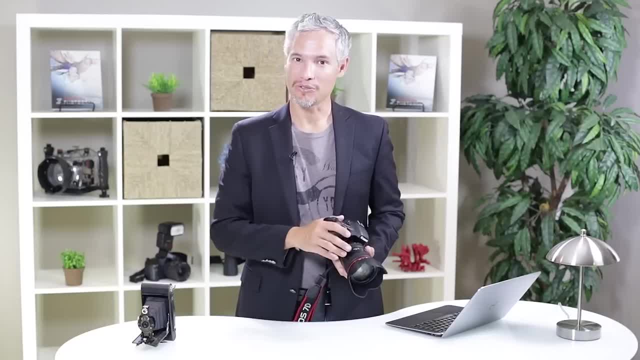 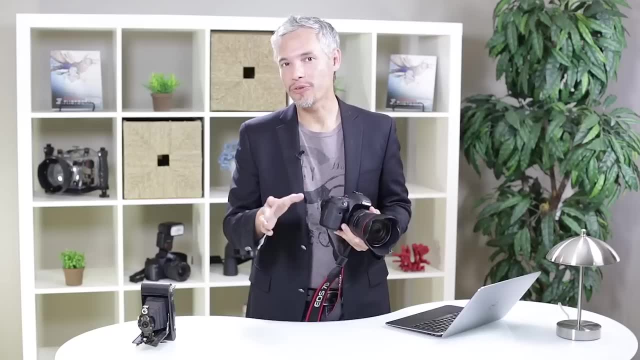 castle. Now, for this sort of still shot, you'd probably want to use single focusing mode and then focus and re-compose, So you'd focus right on her eye And then re-compose the picture. So use the rule of thirds or whatever compositional elements you wanted to use. 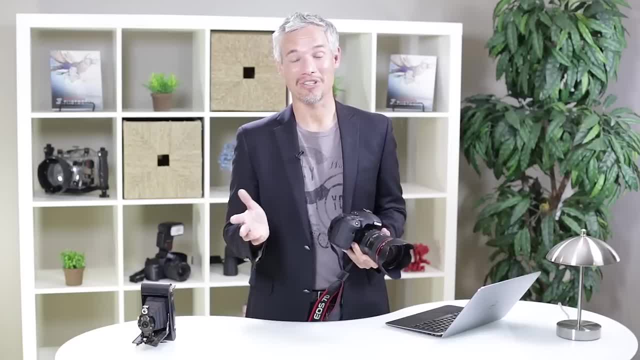 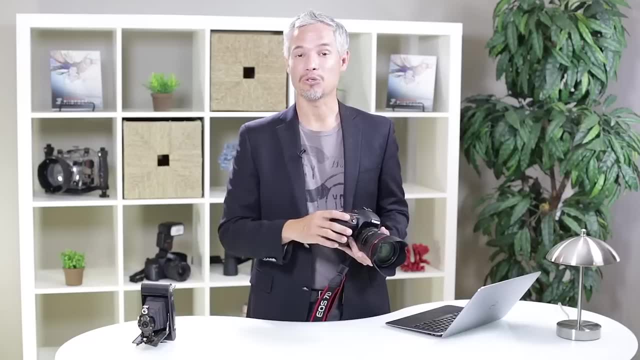 But then, suddenly, your kid sees a seagull and goes chasing after it, and this is a great moment you'd like to capture. If you're not using back button autofocus, you'd have to look at the top of your camera and fumble around until you switch from single to continuous focusing. 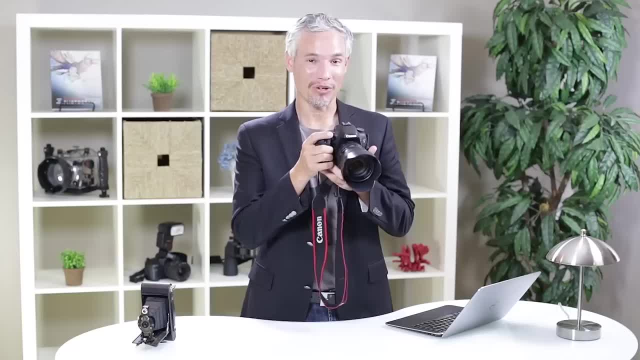 Then you'd have to get the camera back up to your eye, get the child focused and in frame and finally take your picture. And you know what That's going to take you a couple of seconds And the moment's going to be lost. 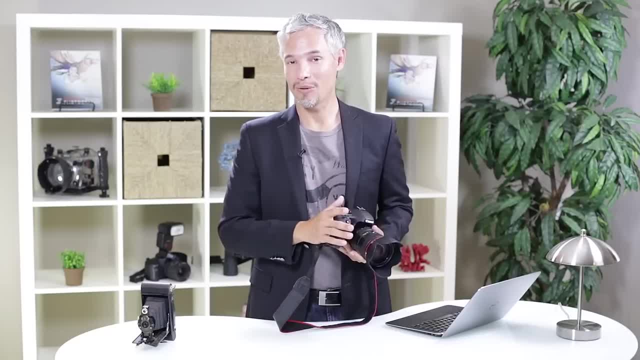 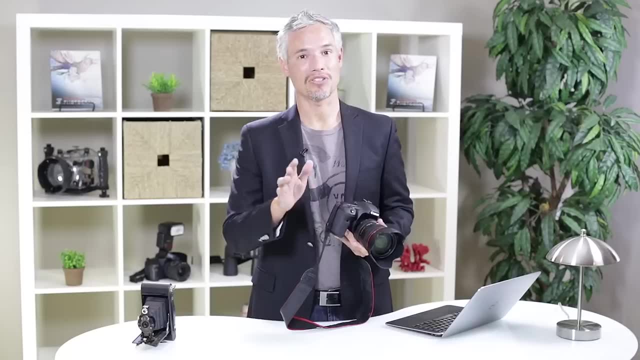 Using back button autofocus. here's how that goes down. You keep your camera in continuous focusing mode While your child is still. you just hold down and then release the focusing button as soon as it's locked in on her eye. Then you can re-compose freely and take as many pictures as you want without re-focusing. 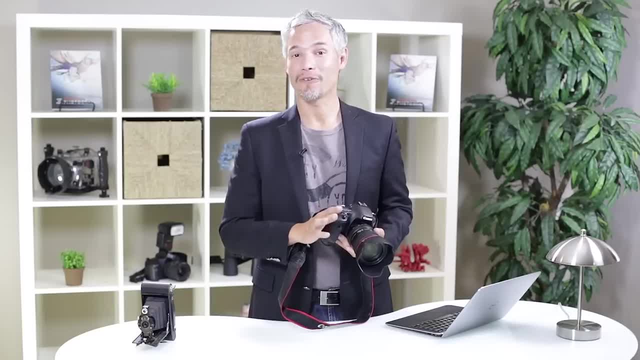 As soon as your child hops up and starts running, you put that focusing point on them and then hold down the back button, autofocus button, and it will keep tracking her as she runs. Then you can just snap away without changing any settings. So the benefit. 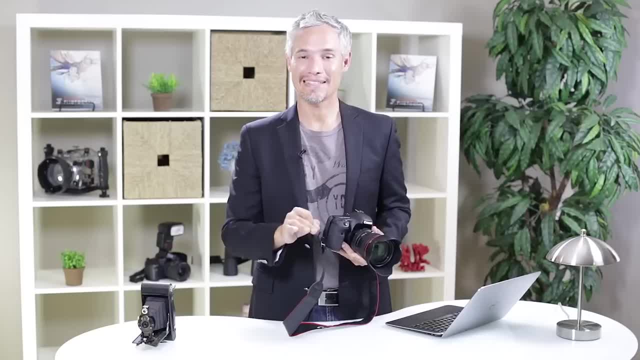 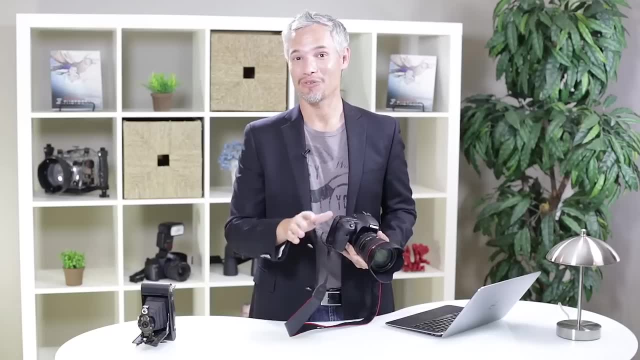 Back button autofocus really gives you is the ability to respond instantly to changing conditions without having to change your camera settings. And it does take some getting used to. it can take several days, but you're going to be a photographer for years, the rest of your life. 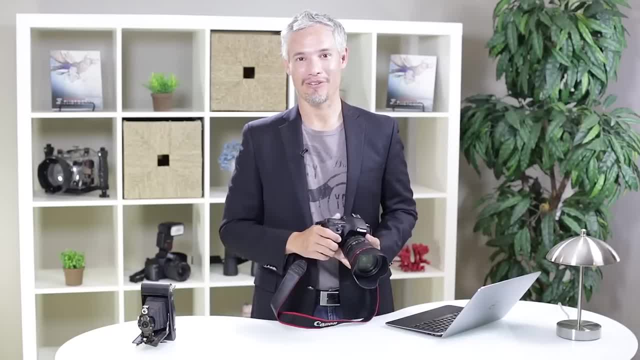 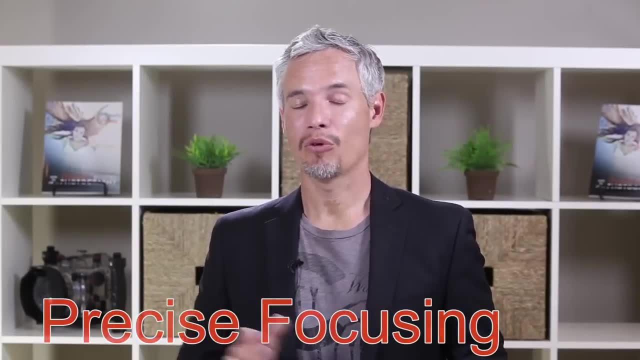 So it's worth going through that kind of uncomfortable learning curve to figure it out. Now let's talk about precise focusing. Precise focusing is a technique that I like to use for still life work when my camera's mounted to a tripod. So it's not good for portraiture and certainly not for sports, but if you're doing a landscape. 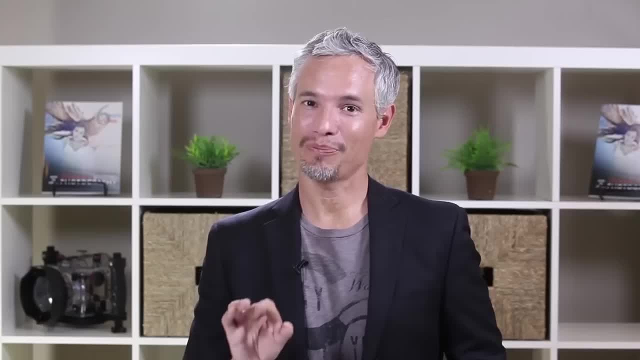 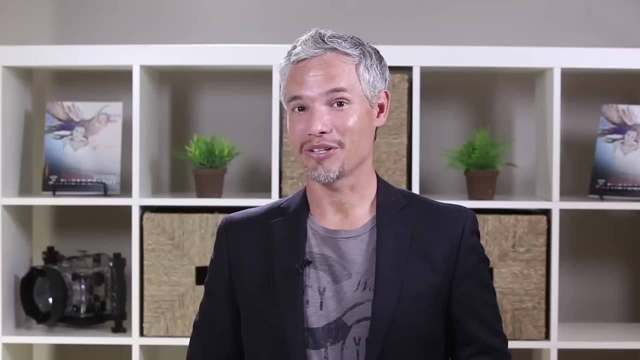 or macro work and you want to make sure that it is perfectly, perfectly focused on the right part of the picture. precise focusing is for you. Precise focusing is also a great way to make sure that your camera and lens are focusing properly, because sometimes people get blurry pictures and they think, oh, my lens is broken. 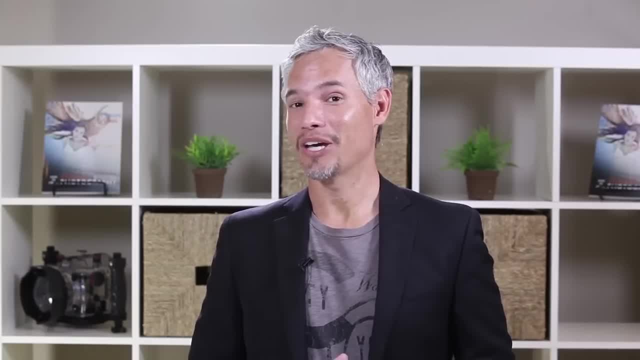 or my camera's broken. Usually it's user error, But if you want to make sure it's your camera and not user error, you can use precise focusing to test it. So, to use precise focusing, just turn on live mode on your camera so that you can see what. 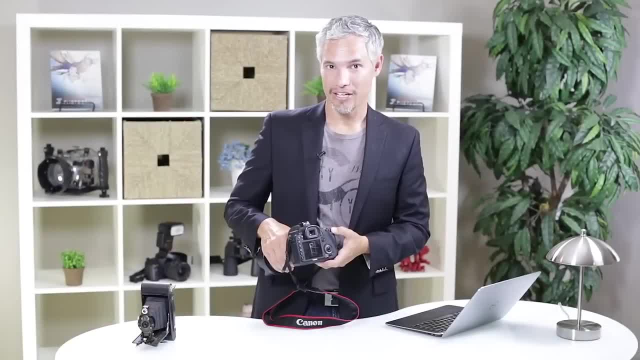 your lens sees through the back of the camera. Now you can use the magnification buttons to zoom in on the live view. zoom in as tight as you can so that you see a very close up part of the frame on the live view here. 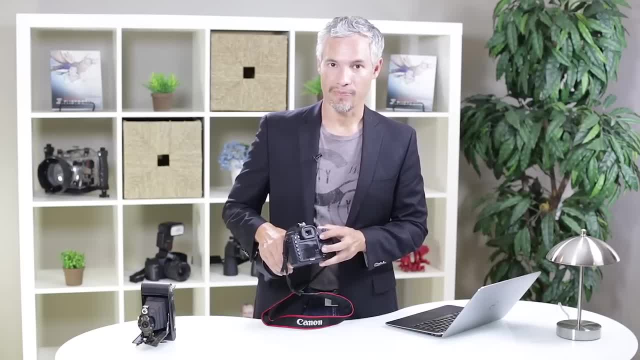 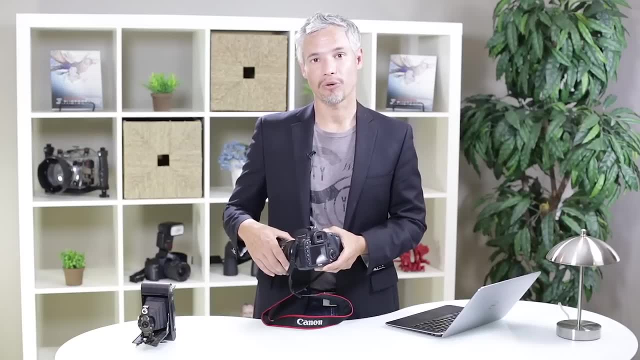 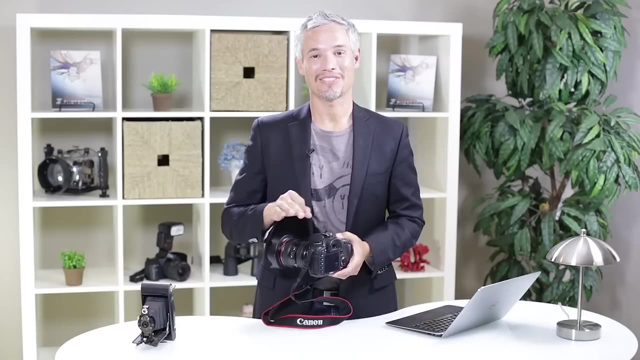 You can move this around as needed to view a different part of the frame. Now you can either use the contrast based focusing system by pressing the AF on button, or you can manually focus using your lens. Either way, this is going to allow you to get extremely pixel perfect focus, and you're 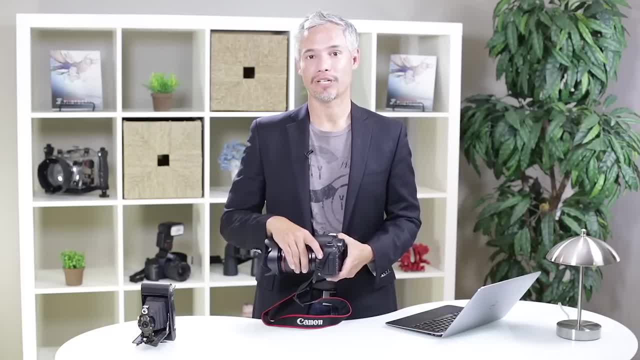 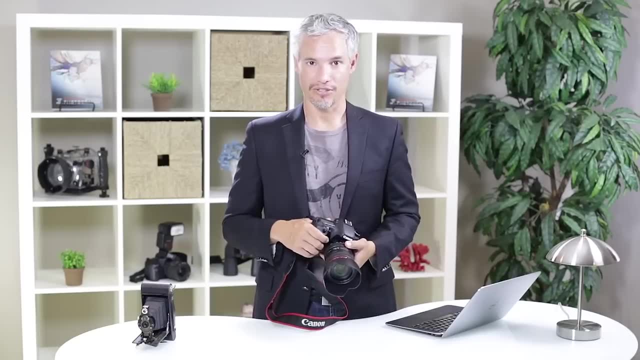 going to be confident that your picture is going to be completely sharp because you're seeing individual pixels on your live view And that's far sharper than you'd be able to see if you're looking through the viewfinder itself, As I mentioned, some people think that their camera's not focusing properly, and I like. 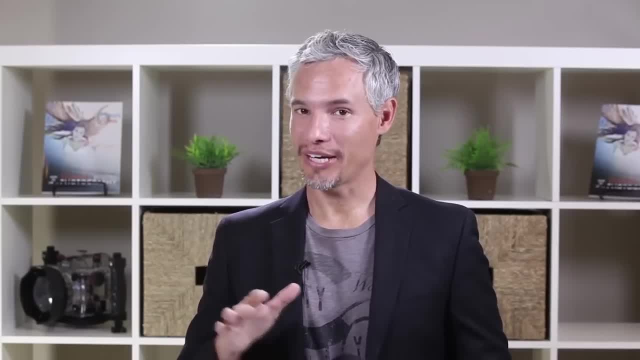 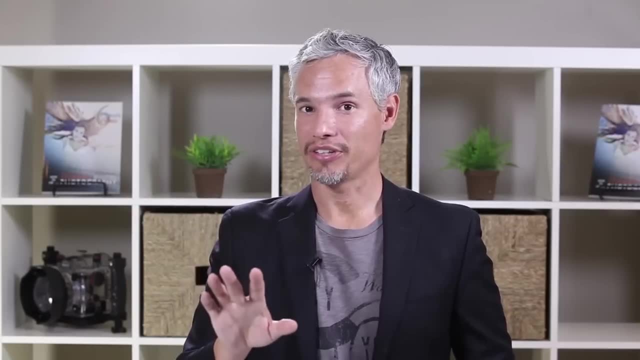 to use precise focusing to test that. So what I'll do is I'll set up my camera on a tripod and then I'll set up a book or something else. I'll set it up a few feet away and I'll have that perfectly still too. 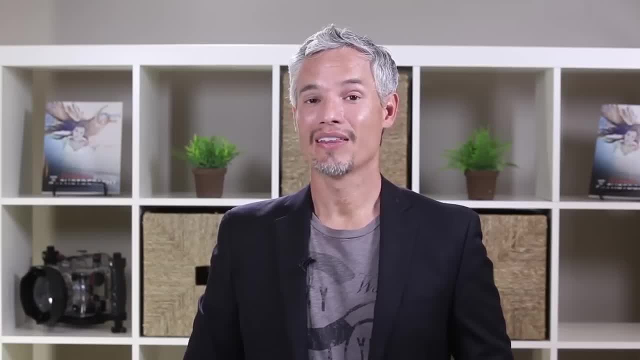 You don't want somebody holding it, so have it resting and still. Then I'll use the camera's auto focus system to focus on the book, and I'll just let it focus as it normally would. What I'll then do is turn on live view and zoom way in, and I'll see if it's actually. 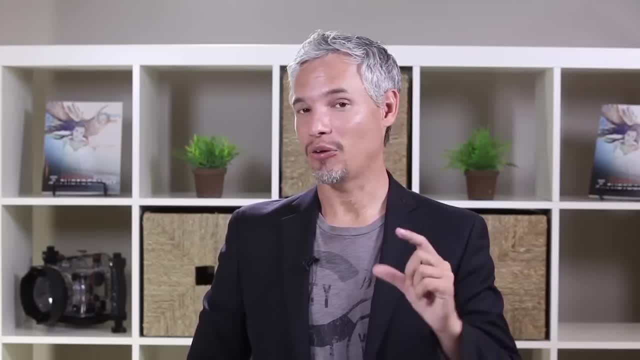 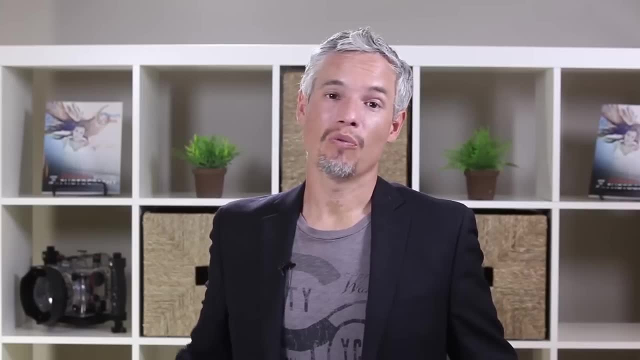 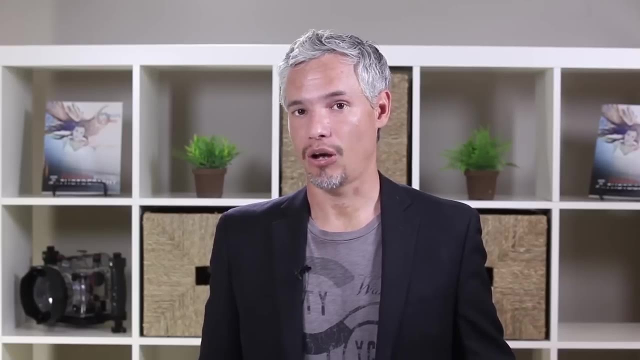 sharp. If it doesn't seem sharp, then I'll manually adjust the focus on the lens until it is sharp. So what this tells you is, If you use precise focusing and the focusing is more sharp than your camera's auto focus system, then you might indeed have a problem with your camera's auto focus system. 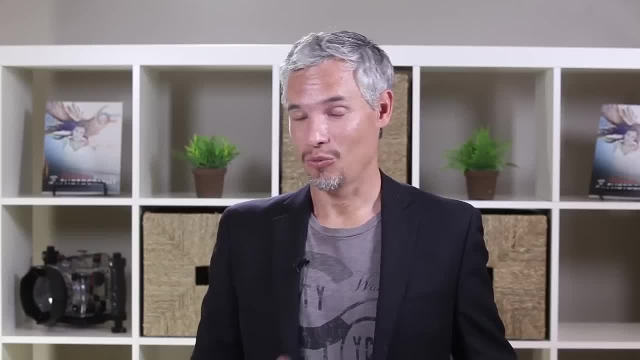 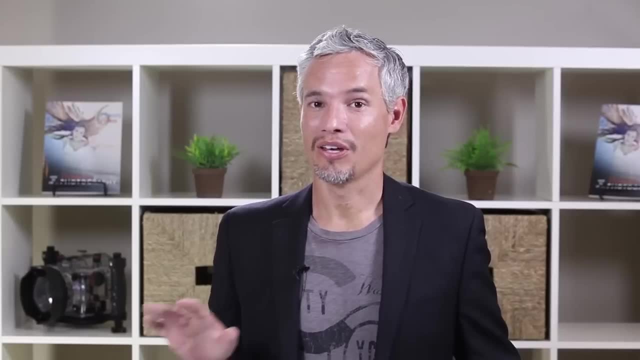 If you focus and then zoom in with live view and it seems sharp, well, the focusing problems might be user error. Now in the next lesson we'll cover some of the common problems with focusing and how you can solve them without having to blame your gear. 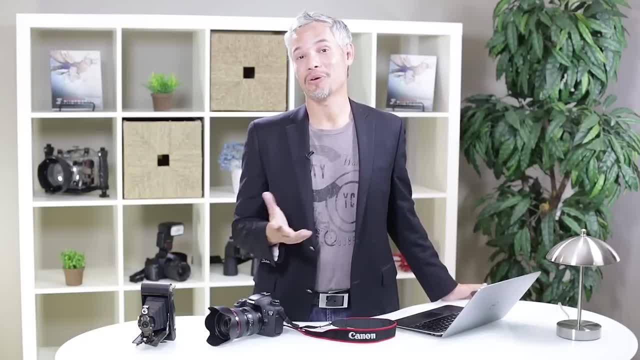 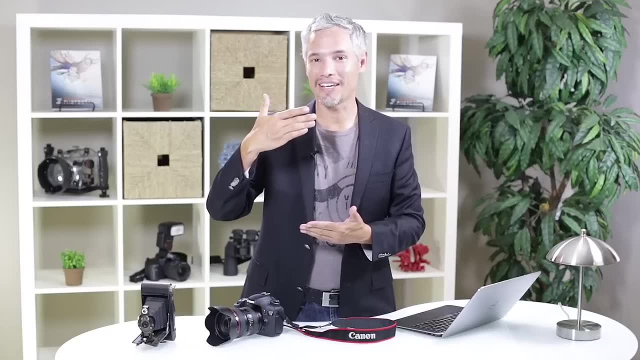 Now let's talk about your camera's shutter and how you can control it. As I mentioned earlier, The shutter is the curtain that is normally blocking your digital sensor, and when you take a picture, well, it slides out of the way and lets the light come in, and then covers. 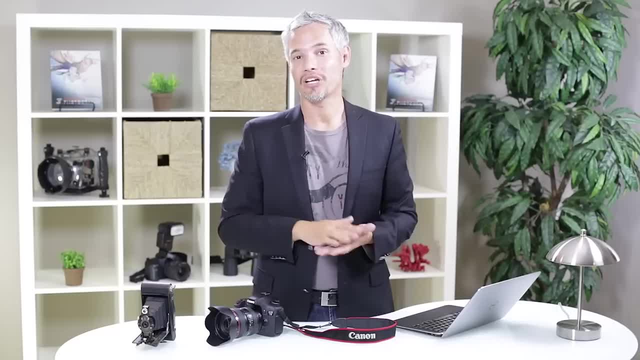 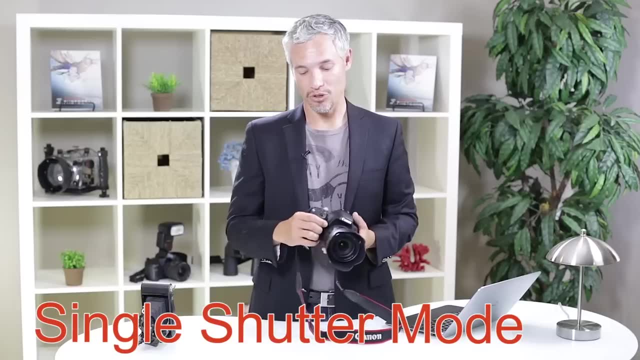 it back up again when your exposure is complete. Your shutter can operate in several different modes, and when you turn your camera on, when it's brand new, it's probably going to be in single shutter mode. That means when you press the shutter release button it takes one picture. 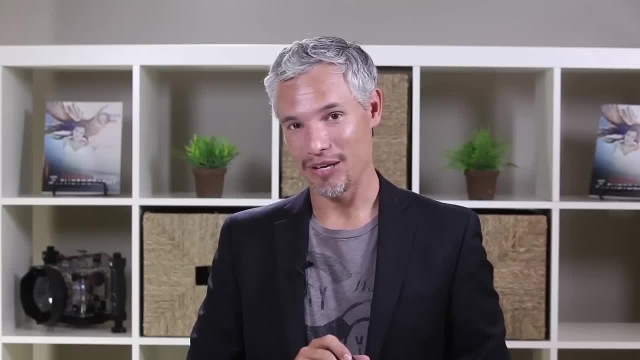 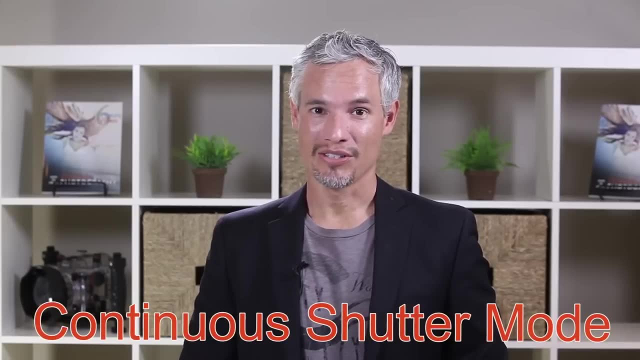 Even if you hold the button down, it just takes the one picture. You have to let your finger up and push it down again if you want to take another picture. The mode that I use for almost everything is continuous, Continuous shutter mode, So I'll switch this camera to continuous shutter by pushing the drive button here and then. 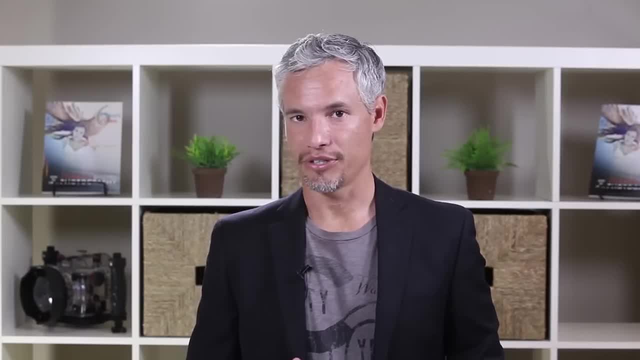 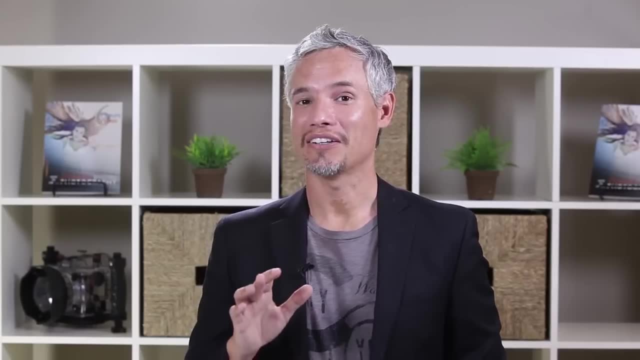 adjusting the main dial, Your camera is going to operate a little bit differently. But when you have your camera in continuous shutter mode, it'll sound something like this: It'll be taking lots of pictures continuously. Some cameras are faster than others, so yours might not make quite such a racket. 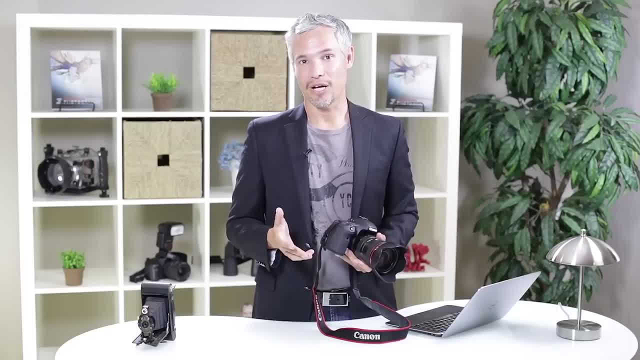 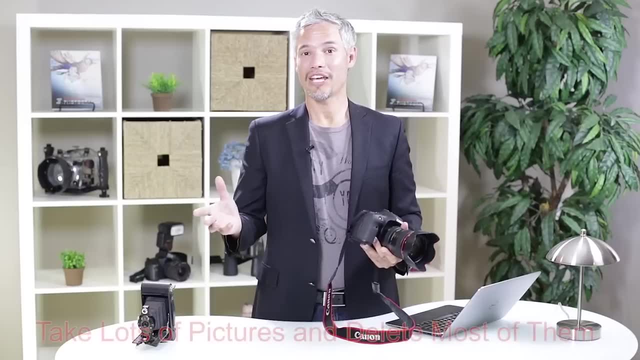 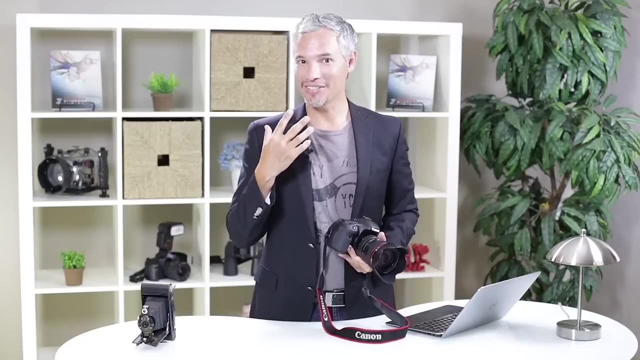 Now, the reason I like to use continuous shutter as often as possible is that it's good to take extra pictures, As I mentioned in the quick tips video, take lots of pictures and delete most of them. So even if it's a portrait of a posed person, well, their expression changes a little bit. 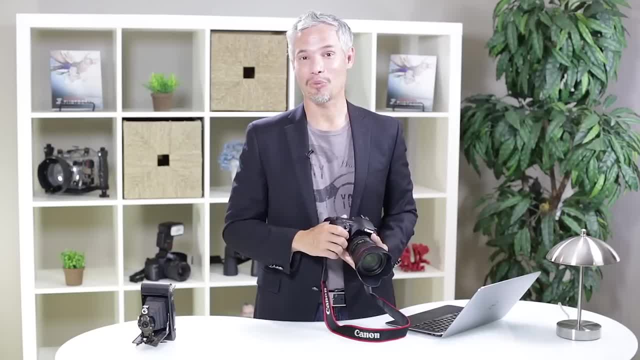 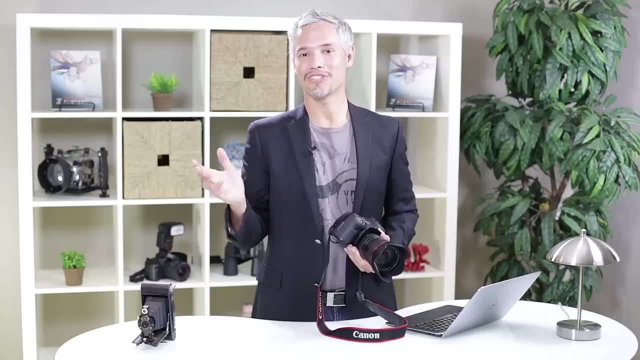 from moment to moment. Maybe they close their eyes when the flash goes off and then they open it up. If you take five pictures continuously like that, chances are good that one of them is going to be great and you can just delete the other four. 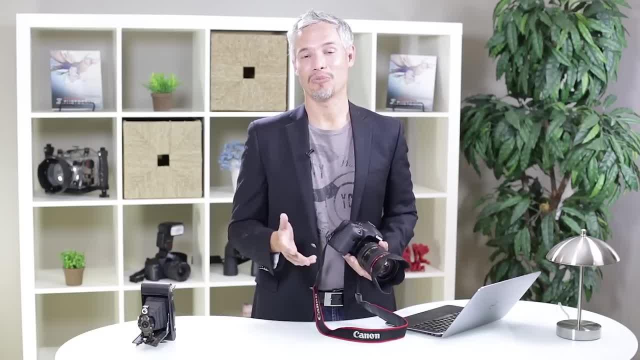 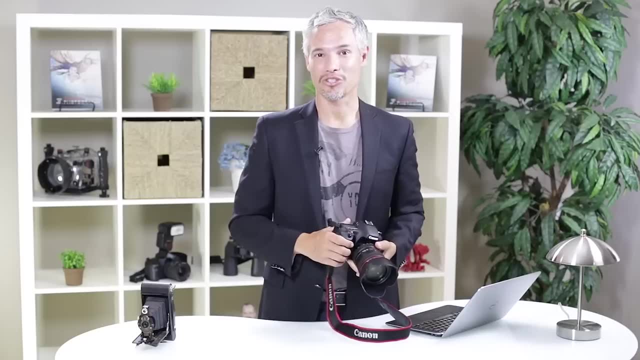 Now, back in the film days, I understand people wanted to use single shutter mode because they didn't want to waste a lot of film. But nowadays, just keep your camera in that continuous mode. Now there are a couple of other shutter modes you should know about. 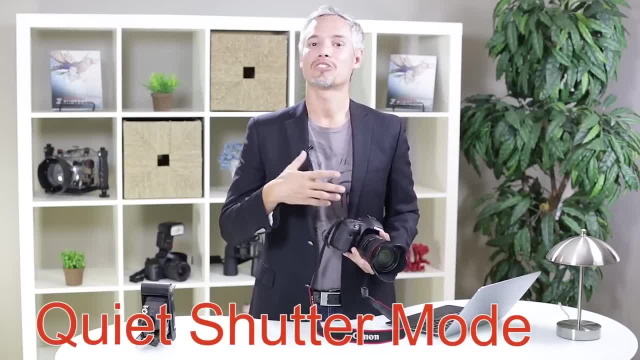 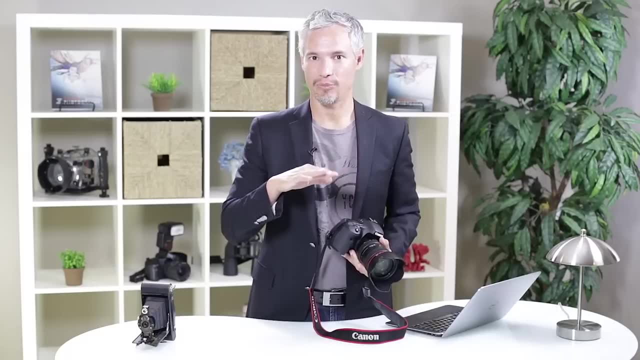 Some cameras will also have a quieter mode, which slows down everything a little bit, Maybe softens the mirror moving out of the way, because a lot of that noise is actually caused when the mirror has to flip up. So check your camera's manual and see if you have a quiet mode. 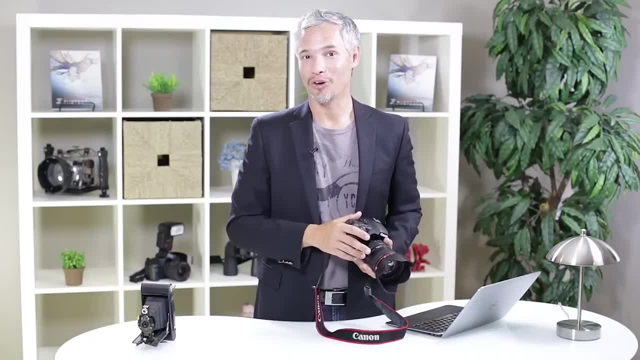 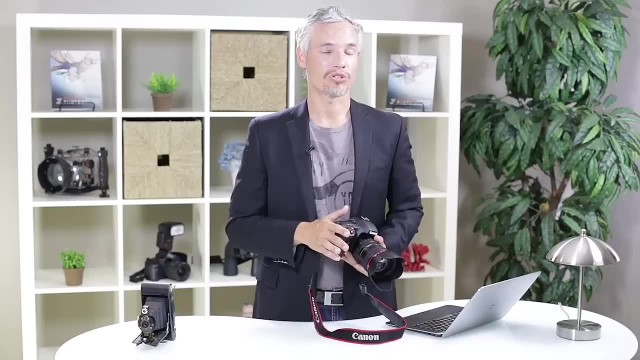 That's great for- well, journalists call it the funeral mode, but it's also great for weddings or any time you don't want to disturb somebody, Maybe street photography. There's usually also one or two delayed shutter modes. These cause the camera to wait a couple of seconds between pressing the shutter release. 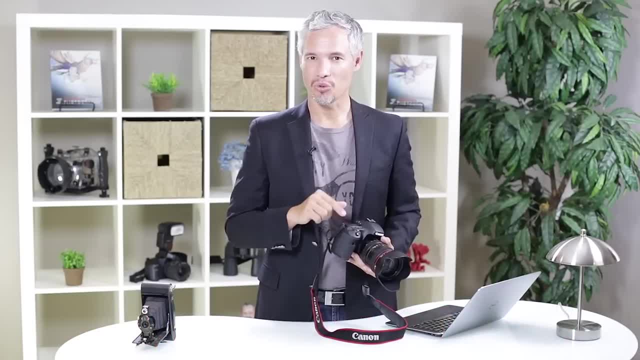 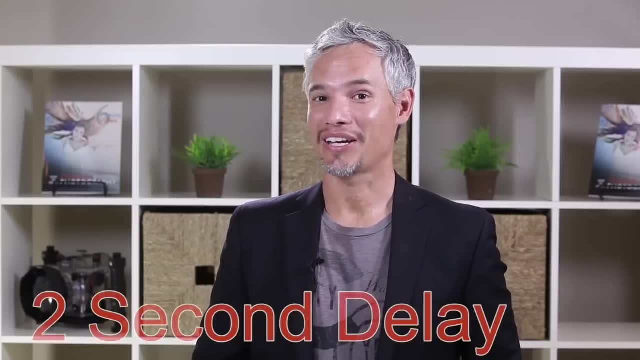 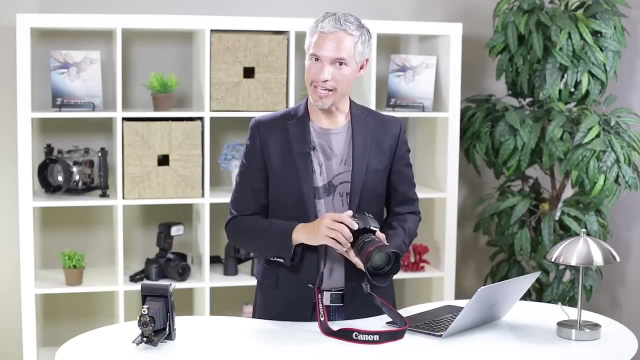 button and actually taking a picture. So I'll turn on the shorter delay mode here. Now, when I push the shutter, there we go, there's a two second delay before it takes a picture. Now this shorter delay is useful when your camera is on a tripod and it can reduce the 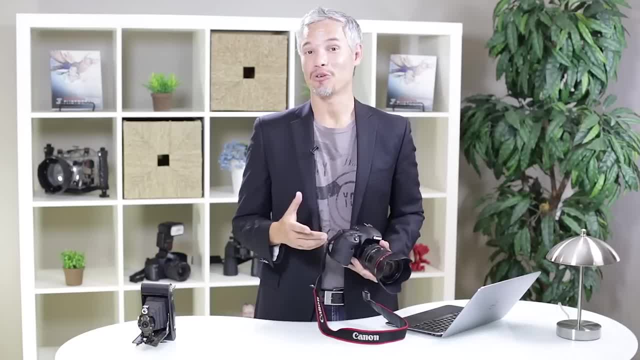 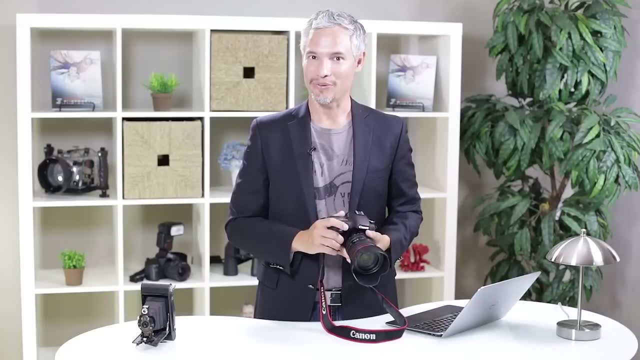 camera shake that's caused by simply pushing the button down. I know you don't feel like you're doing any major damage to the camera when you just push the shutter down, but you are moving it a little and that can cause a little bit of bounce. 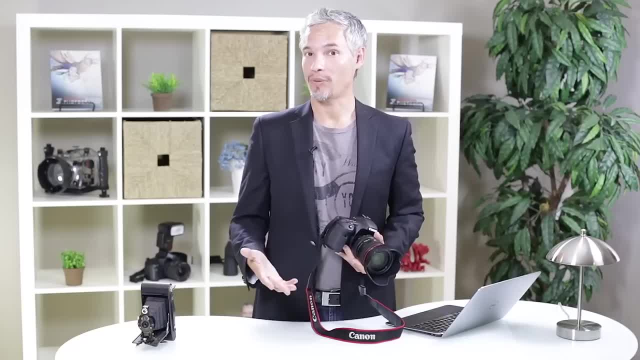 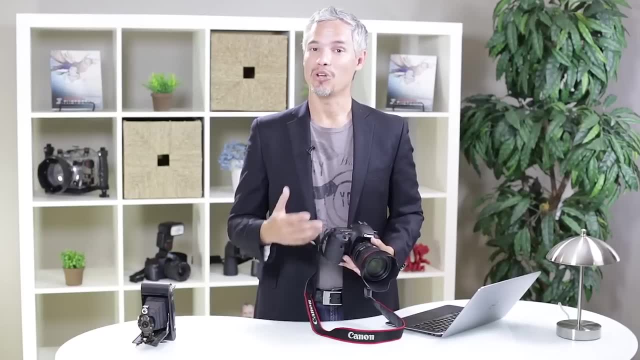 And if you have a long shutter speed- maybe you're taking pictures on a tripod at night and your shutter is one or two seconds. well, pushing that shutter down can shake the camera enough that you notice the problem in the final image and it'll be a little bit shaky. 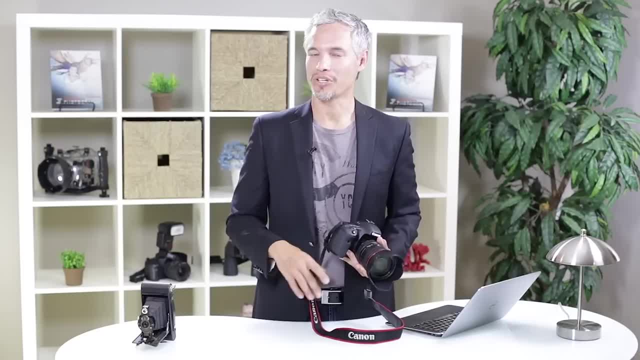 Easy way to solve it: Just set your shutter to that two second delay, or whatever the shortest delay is on your camera And after you take the picture, that's it. That's it. Your camera will steady and then the shutter will fire. 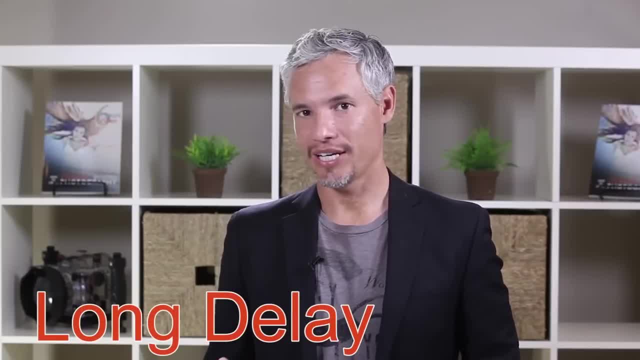 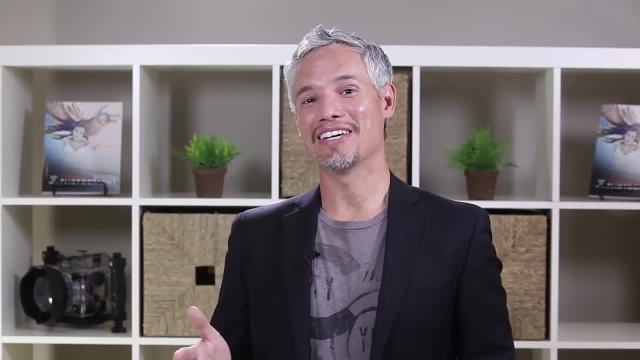 There's also a mode for a longer shutter delay, and this can be eight or 10 seconds after pushing the picture. And I think we all know from our childhoods what this is for right, Those holiday pictures where you stick the camera on a tripod and then everybody runs. 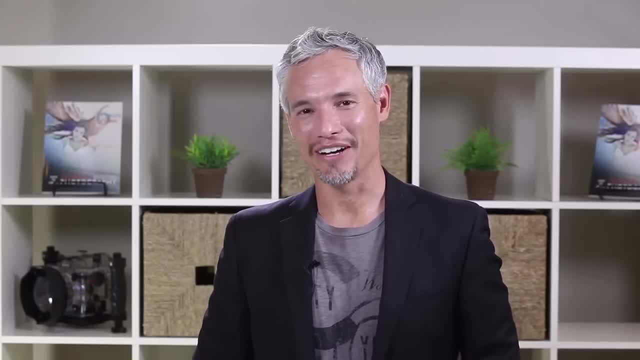 in front of the tree and you try to take a picture after it fires. When you do that, you push the shutter and then you wait eight or 10 seconds and then the camera finally takes a picture. That's useful for what it is. 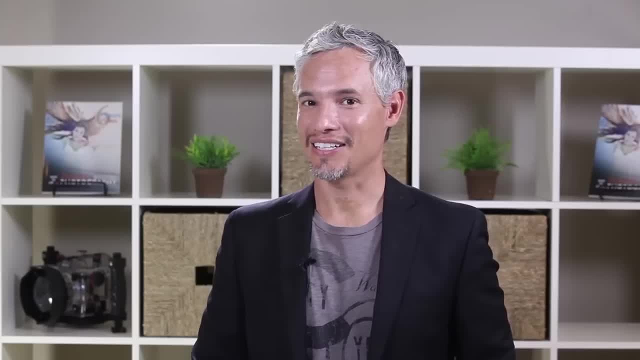 I'll say that instead of using that 10 second delay, I tend to just put a remote shutter release on the camera. That way I can fire it from wherever it is. Those are available pretty inexpensively, so it might be something you should look into. 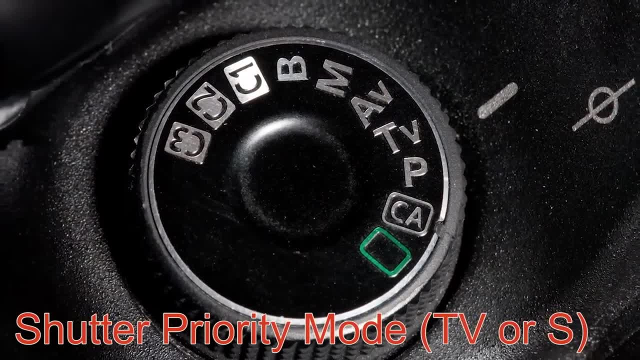 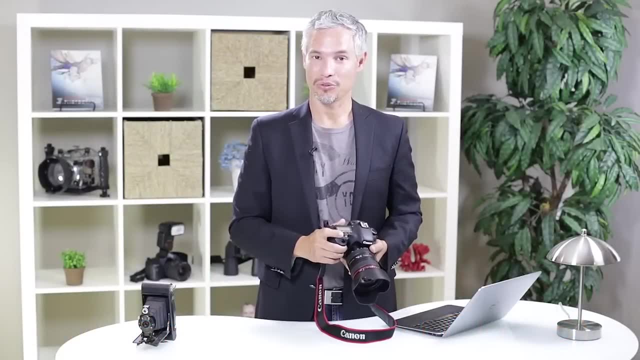 When you have your camera in shutter priority mode- that's TV on Canon cameras and S on every other make of camera in the world- well, you can adjust the main dial to control the actual shutter speed. So you'll see a number on either the back or the top of your camera. 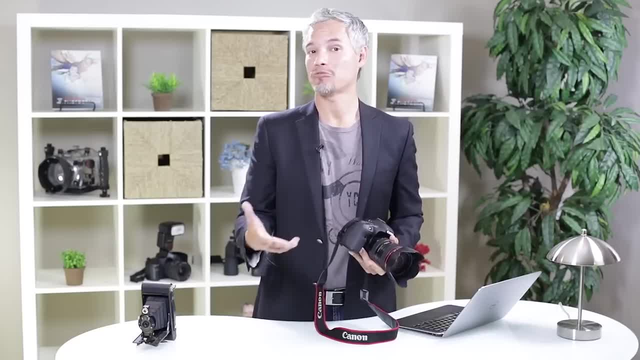 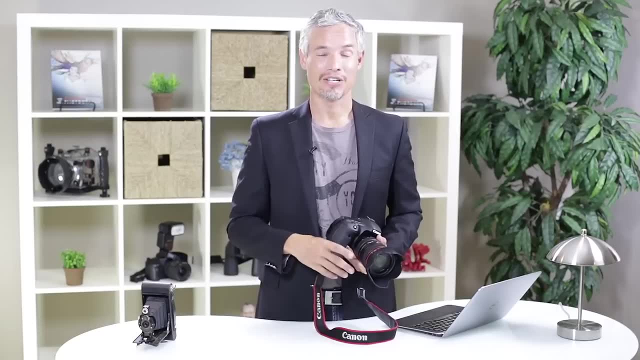 And that's the shutter speed. It's usually displayed at 60 if it's actually 1 sixtieth of a second, or it'll be 125 if it's 1 twenty-fifth of a second. Here's an example picture at 1 twenty-fifth of a second. 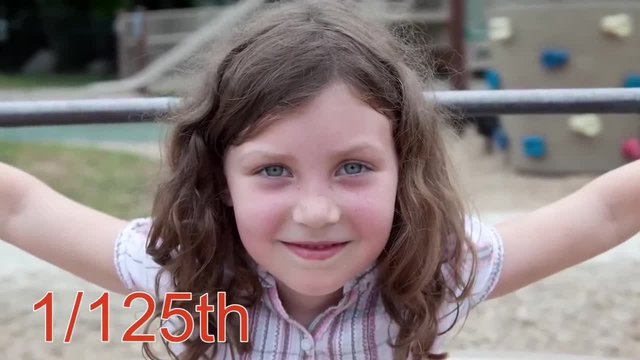 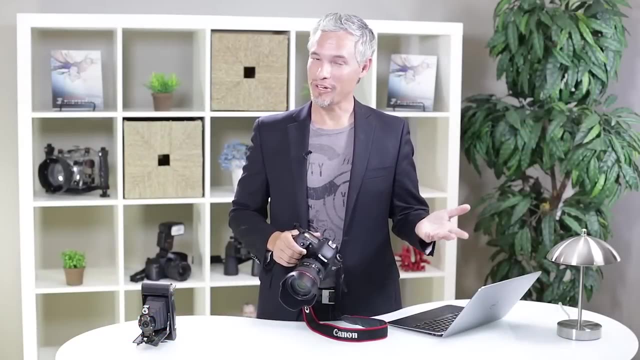 Believe it or not, this is a moving picture. I'm on one of those merry-go-rounds and my daughter and I are facing each other and it's spinning at a good pace. But 1, 1, twenty-fifth of a second is a pretty fast shutter speed and that completely froze. 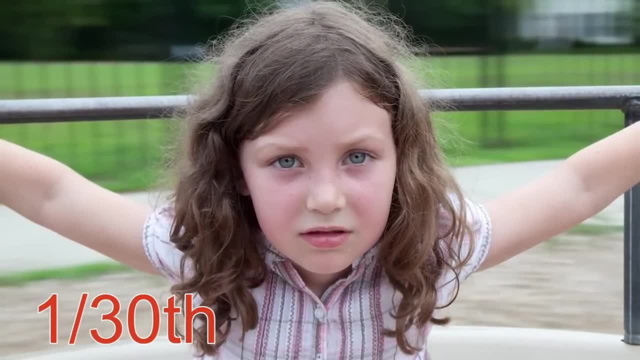 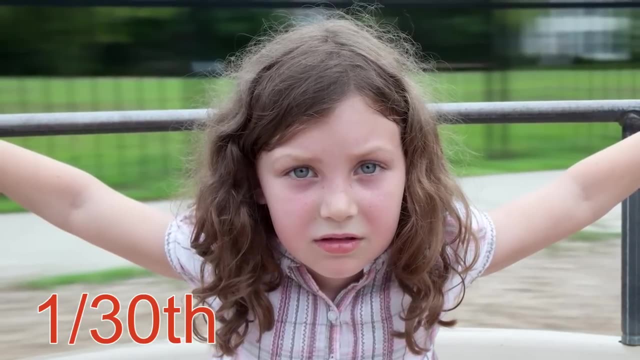 the action. So let's look at a picture with a slower shutter speed. This picture is taken at 1 thirty-fifth of a second and she looks a little terrified and sick there, but, believe it or not, she was actually having a good time. 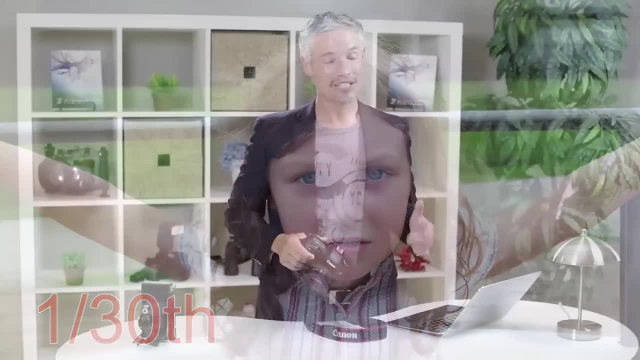 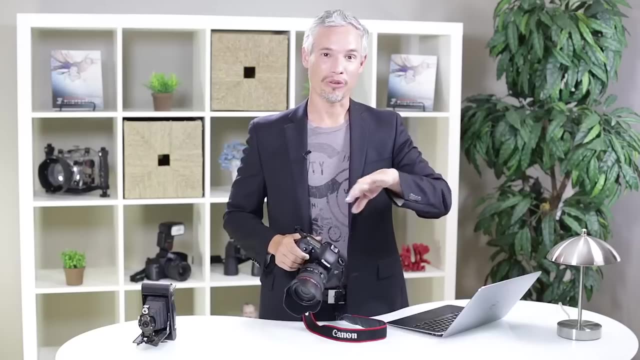 But if you look at the background you can now see a distinct blur. She's frozen because she is moving with me on the merry-go-round, but the background is spinning and at 1 thirty-fifth of a second- a slower speed- you can start to see the panning. 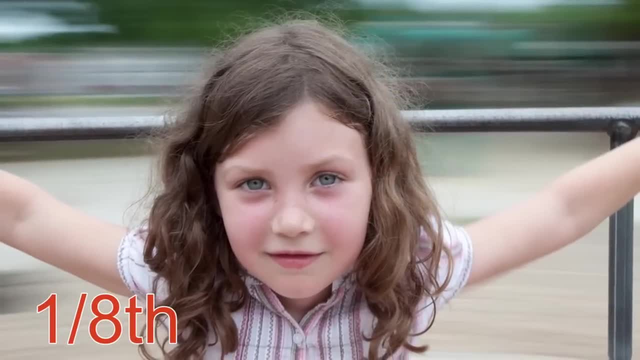 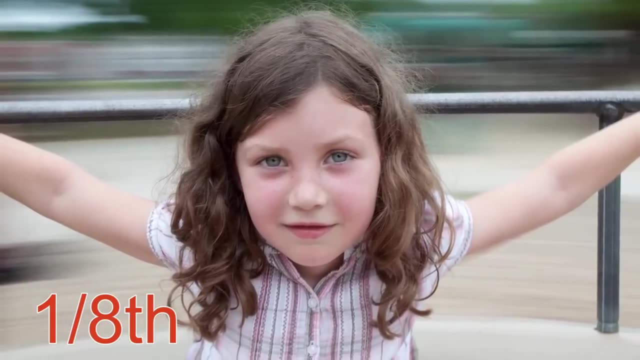 motion from the background. Let's go even slower Here. at 1 eight the background is very blurred. So this is an important lesson: The slower your shutter speed, the more movement gets shown on your camera. You often think that a picture happens in an instant, but it's not. 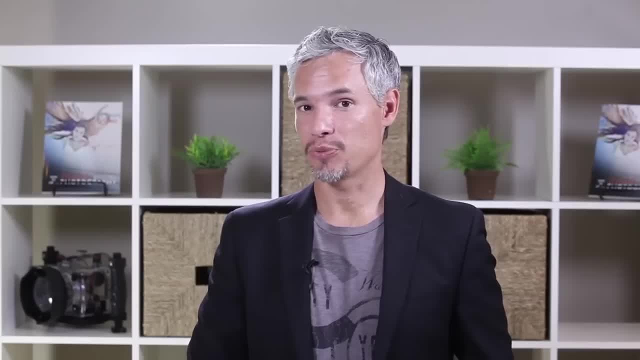 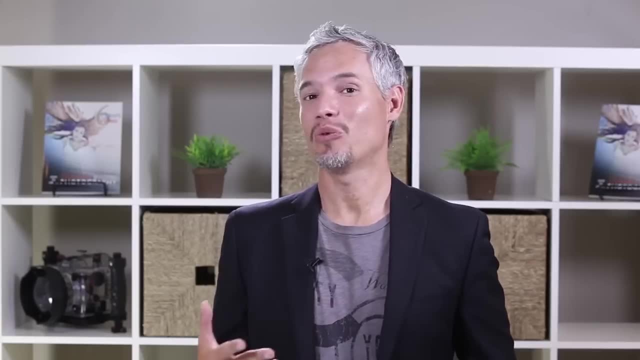 It happens over a period of time, no matter what the shutter speed is. If your shutter speed is 1 four-thousandth, well, that means the shutter is open for 1 four-thousandth of a second. But if it's 1 eighth, well, 1 eighth is a fairly long period of time, and stuff moves. 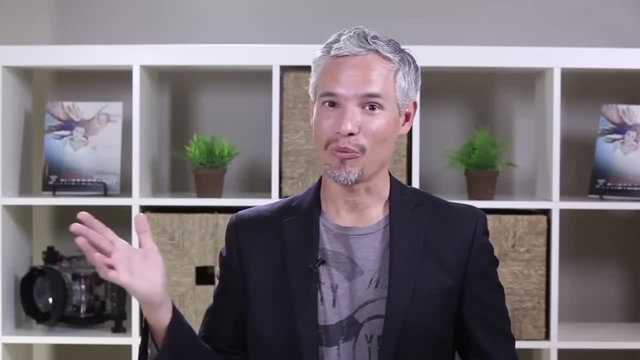 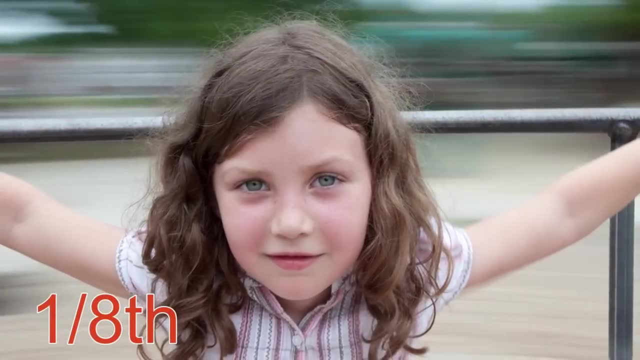 in an eighth of a second and your camera is going to capture light from all points of movement As a subject is inside the frame. So because we were spinning here in this picture, you can see that the background itself is also nicely blurred, And that's the benefit of using shutter priority. 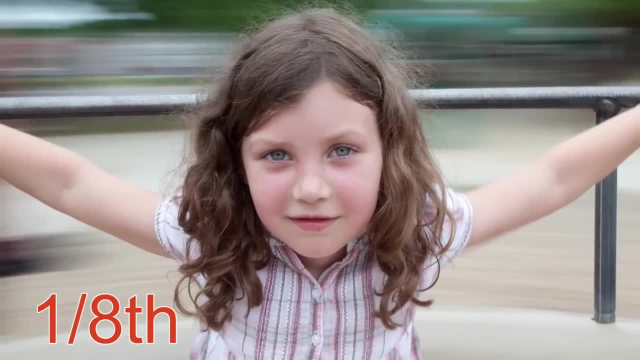 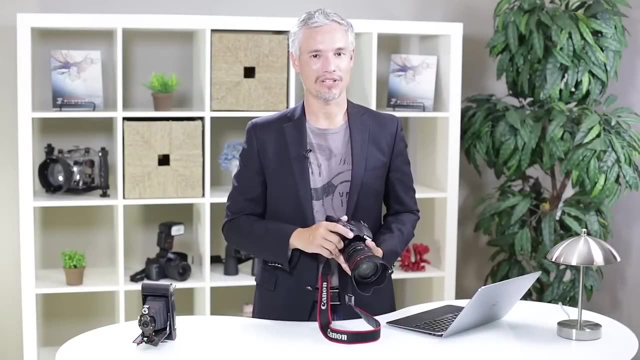 You can control the shutter speed and your camera will adjust all the other settings automatically, Certainly the aperture, but also often the camera's ISO. Those settings we'll discuss a little bit later. If you're shooting a moving subject or the background is moving, shutter priority is. 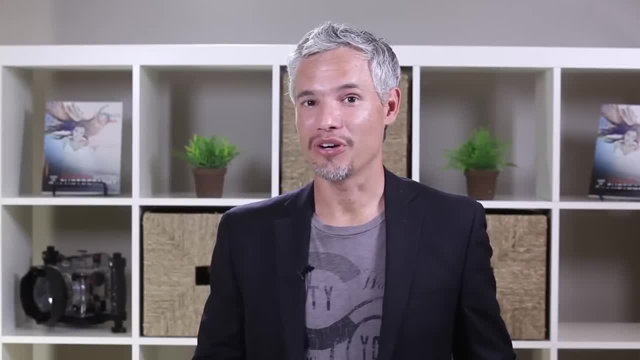 the mode for you. You can also adjust the shutter speed for the camera. I'm going to go to the photo studio and I'll just go through a slideshow of pictures taken at different shutter speeds so you can get a sense for what different shutter speeds. 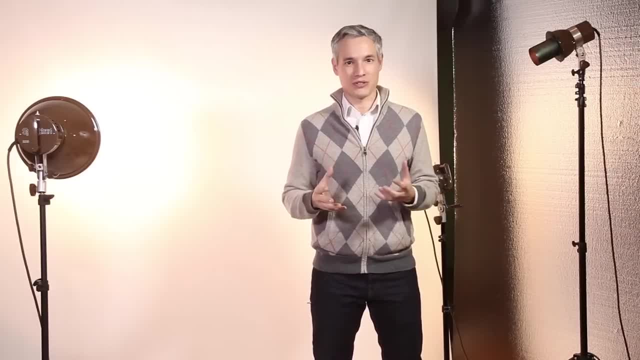 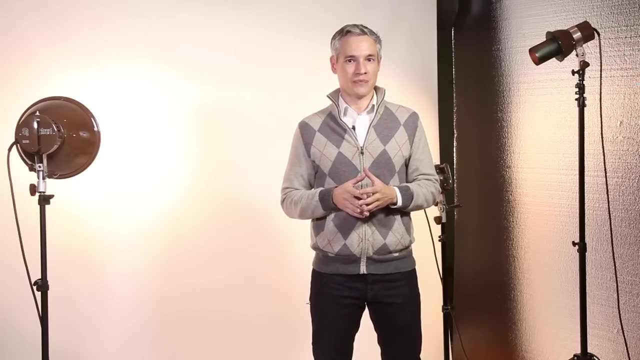 are used for. The best way to really understand how different shutter speeds affect your images is to go out and take a lot of pictures at different shutter speeds. I'm going to try to fast forward you through that process by showing you a series of pictures. 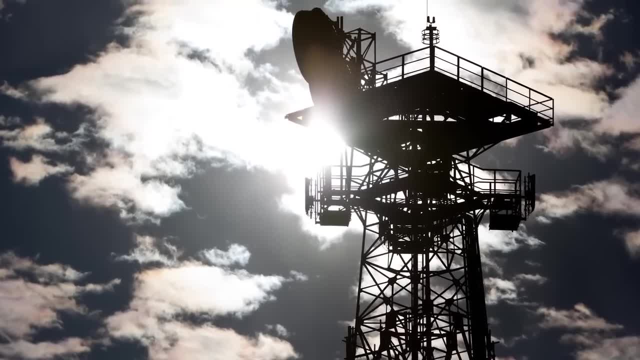 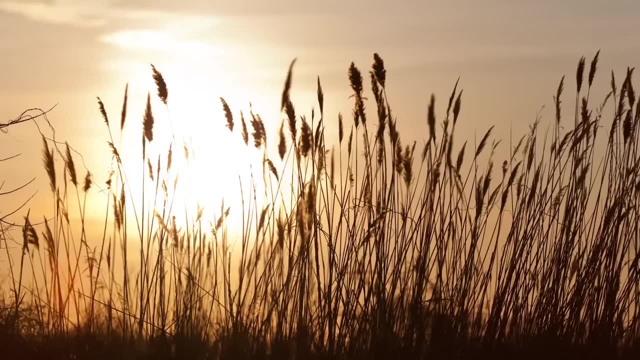 that I've taken at different shutter speeds. My first picture shows 1 eight-thousandth of a second. Now I'm going to zoom into the sun. Anything shorter and it would have been overexposed. Here's another shot, directly into the sun. 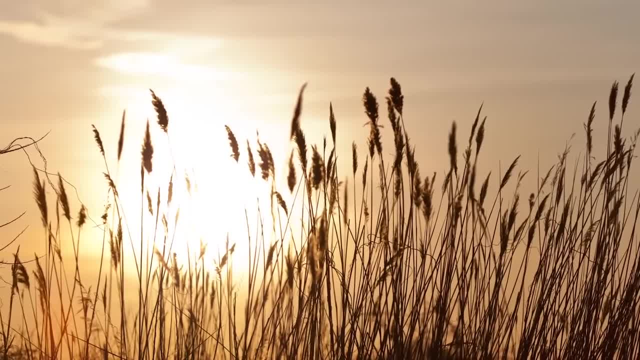 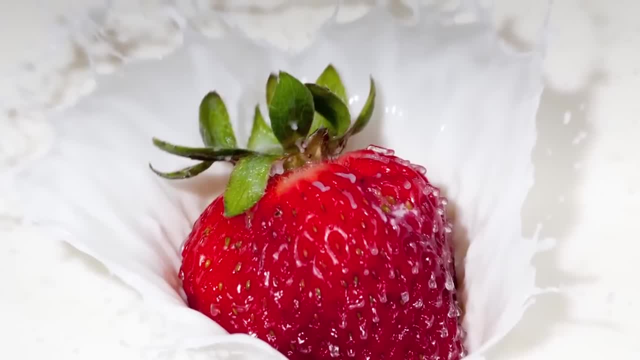 One four-thousandth of a second was the right exposure to silhouette, the reeds in the foreground. Another shot at one four-thousandth of a second, this time taken in this studio using high speed strobes. I use these high speed strobes at a fast shutter speed to freeze the action. 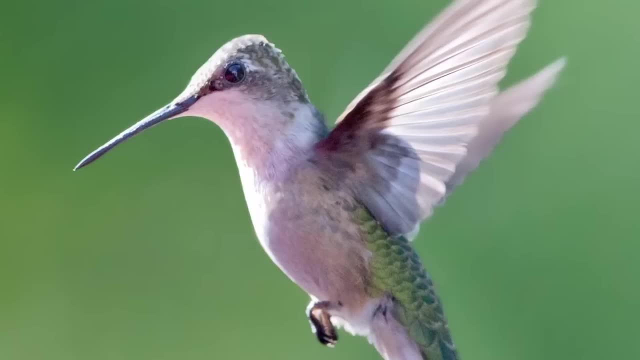 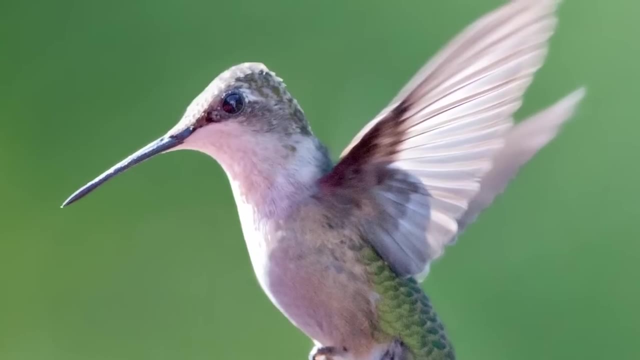 A slower shutter speed would have resulted in blurry drops. Here's a picture of a hummingbird at one fifteen-hundredth of a second. It's a very fast shutter speed, but it's not fast enough to completely freeze the wings of this bird. 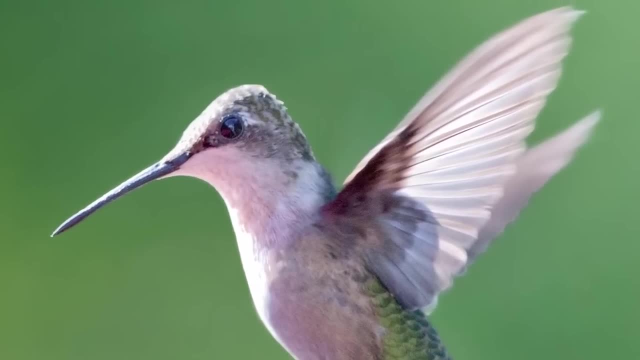 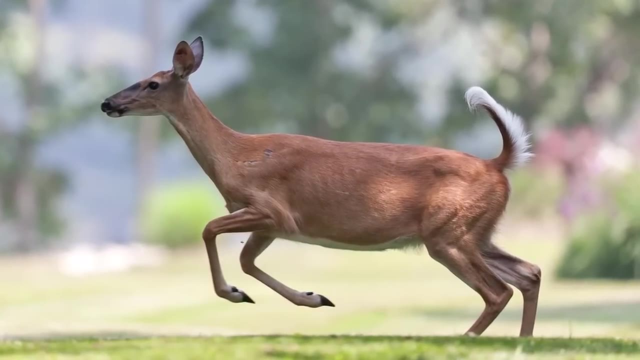 As you can see, just the tips of it are blurred. That's not an entirely bad effect, because sometimes you want a little blur in there to show motion. This deer isn't quite as fast, but the one one-thousandth shutter speed didn't completely. 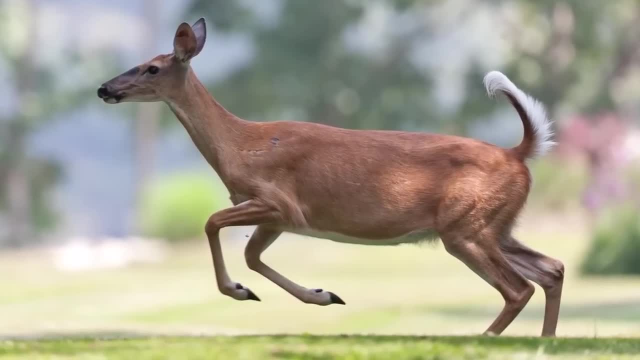 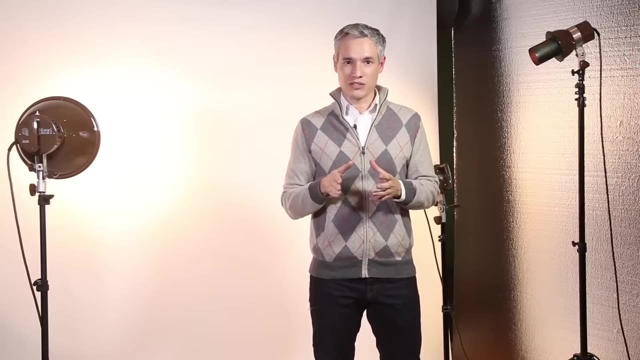 freeze it. Most of the body looks good, but if you look closely at the hooves you'll see just a bit of motion. As I was saying, there's always a little bit of motion in your pictures. The faster the shutter speed is, the less you'll notice it. 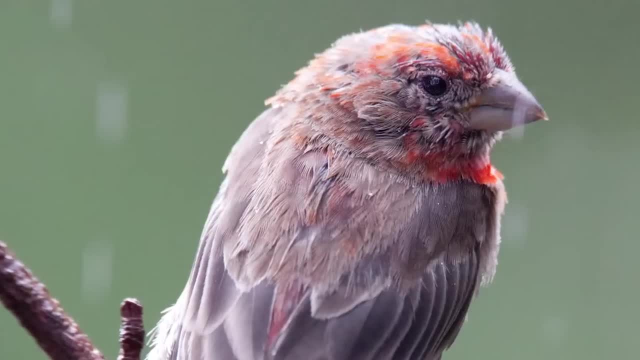 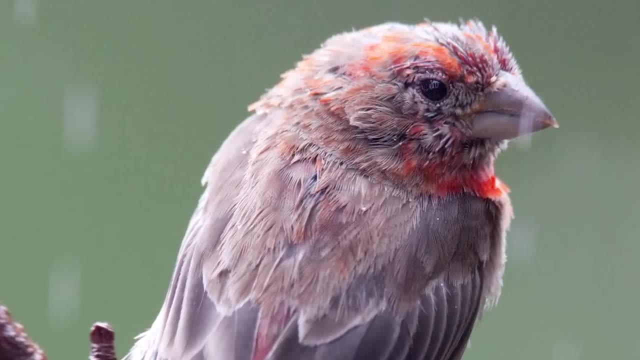 But it's not always a bad thing. One five-hundredth of a second is really good for shooting birds. In this case, you'll notice that it didn't completely freeze the raindrops. I want you to notice just how far the raindrops moved while the shutter was open here, because 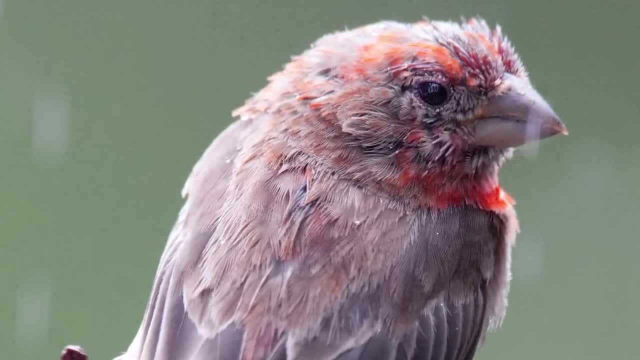 I have another raindrop picture, taken at a slower shutter speed and you'll be able to see the before and after. Here's a picture of my daughter, Madeline, in the playground. I shot this at one three-hundred-twentieth of a second. 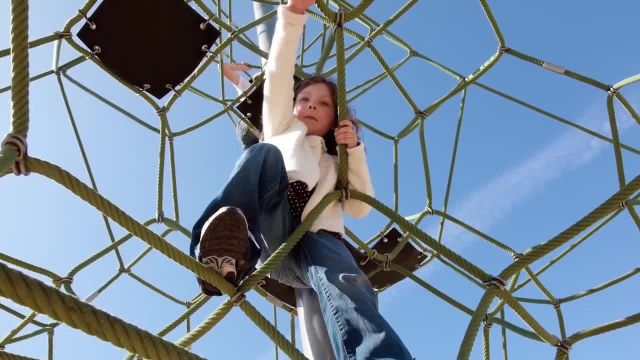 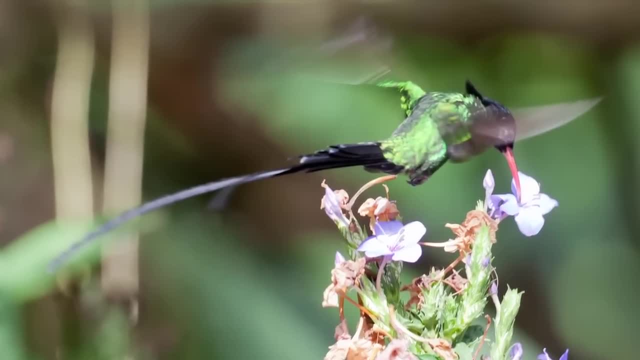 You'll be working with this range of shutter speeds pretty frequently when shooting outdoors in sunlight, And for people that's more than fast enough. Here's another hummingbird picture, this one taken at one two-hundred-fiftieth of a second. 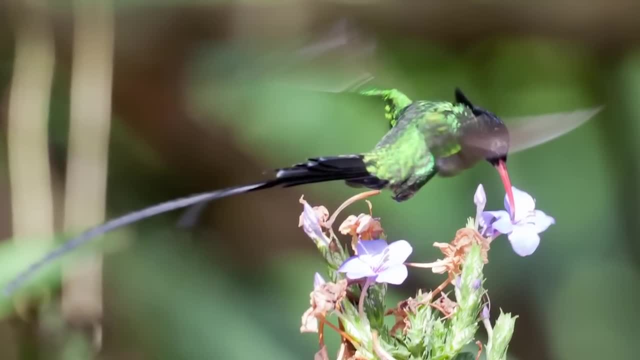 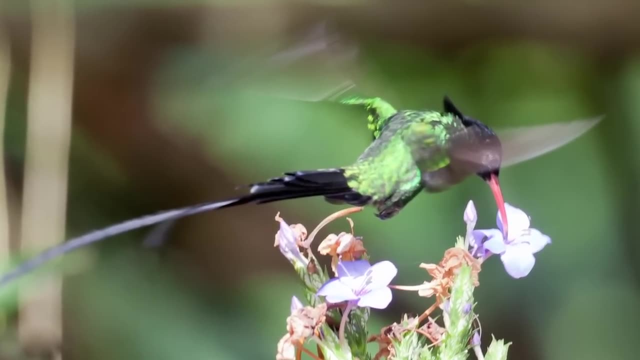 The wings on this Jamaican doctor bird moved so fast that it completed an entire flap while the shutter was open for that very brief amount of time. Notice, though, that the body is frozen still If the wings had also been frozen, which would have required a shutter speed of one four-thousandth. 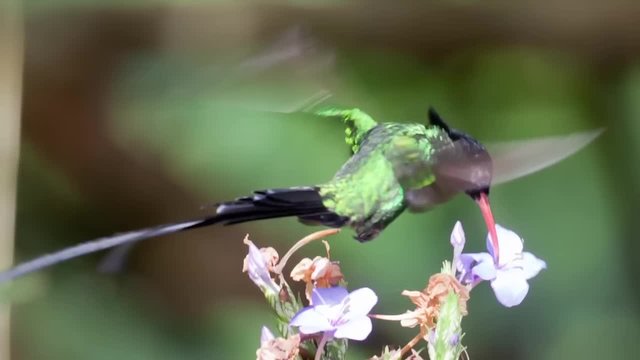 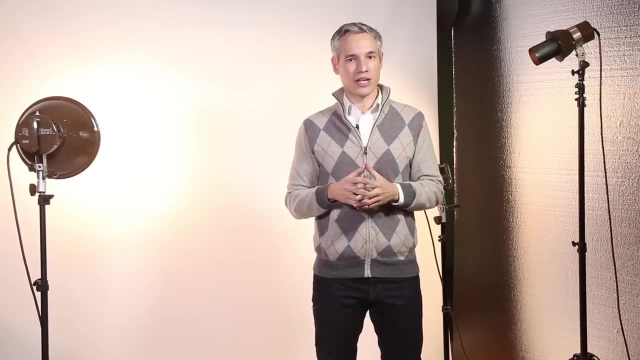 of a second, or maybe even faster. the bird would have appeared to have been pinned in the air, So in this case, one two-fiftieth of a second would actually look better than a faster shutter speed. I photographed this bee at one one-hundred-sixtieth of a second. 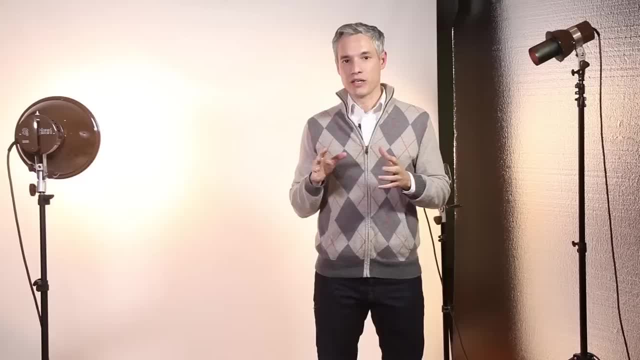 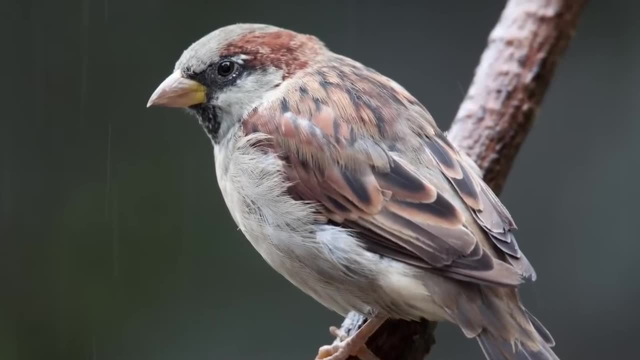 Like the hummingbird. the wings are blurred, but the body is frozen. Here's that second rain picture that I was telling you about, at one-sixtieth of a second. Here you can see that the raindrops appear much longer because they moved farther while. 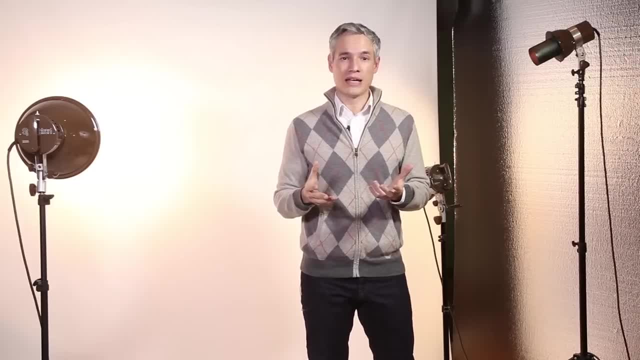 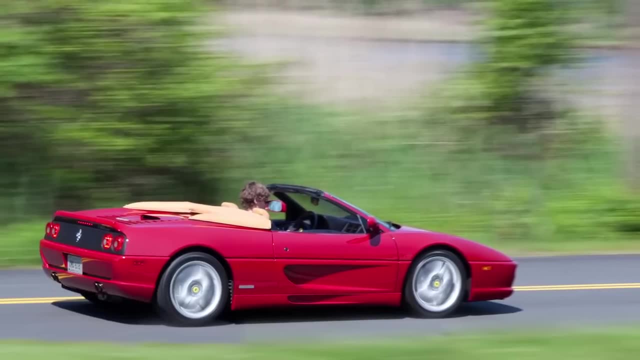 the shutter was open. It's difficult to take good pictures of birds at such a long shutter speed, but with some practice and plenty of shots you can get a few to turn out. I shot this Ferrari at one-thirtieth of a second and panned along with it as it moved. 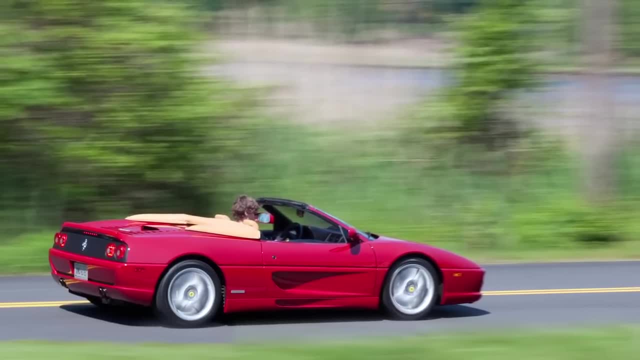 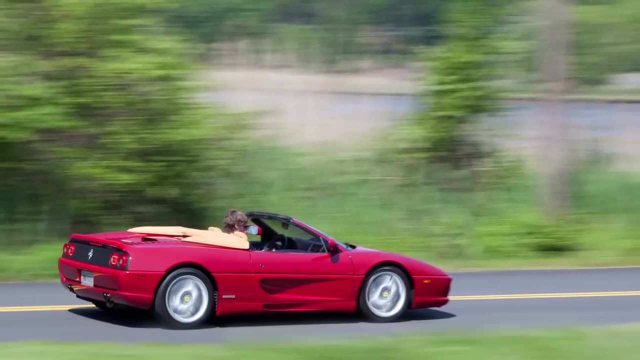 I experimented with different shutter speeds and it turned out that one-thirtieth was about right for the car's speed. This allowed the wheels to rotate about one-eighth of a revolution which completely blurred one spoke into the next. You'll often get pretty slow shutter speeds on dark and cloudy days. 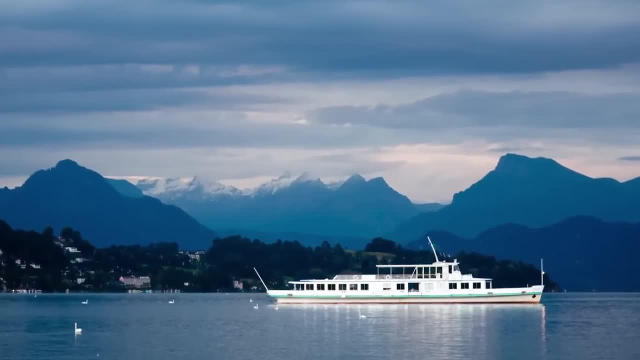 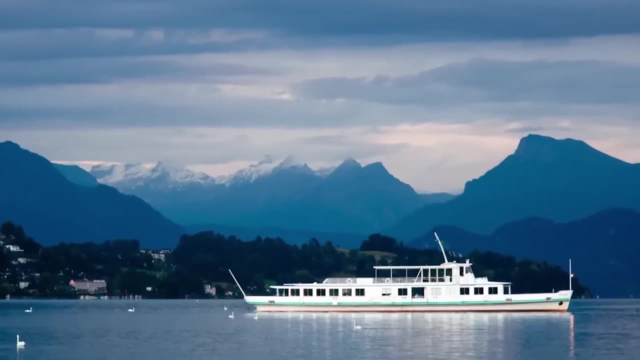 This shot was taken at one-fifteenth of a second at Lake Lucerne in Switzerland. This shot would have been difficult to handhold, except that I used image stabilization. My camera actually cancels the shutter speed. For this next shot, my co-photographer, Chelsea, photographed me in front of the Boston skyline. 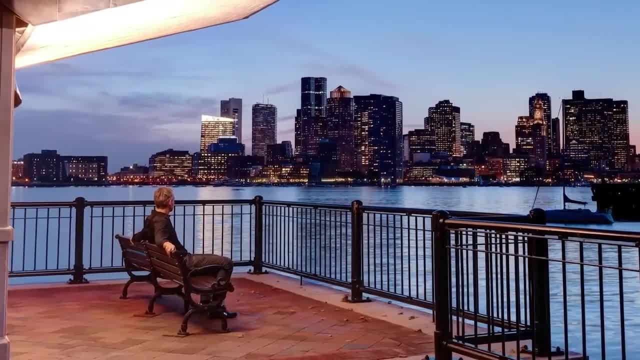 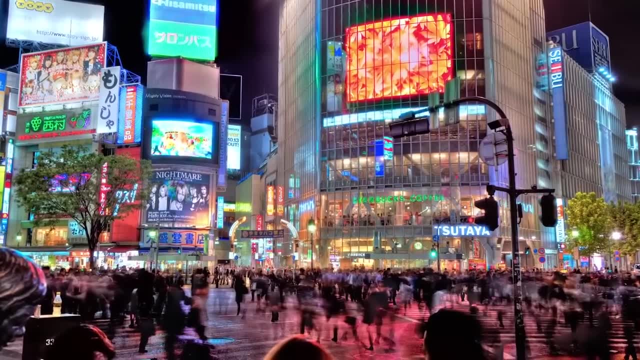 She did it at one-quarter of a second, which absolutely required a tripod. Now here's a shot at half a second of Shibuya Station at night. Shibuya Station in Tokyo is the busiest intersection in the world. You can see that the half-second shutter speed was enough to completely blur people as they. 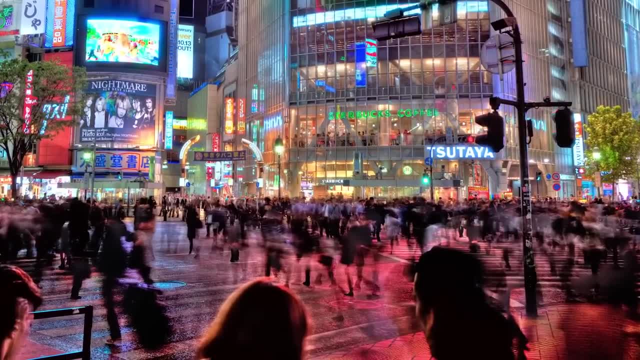 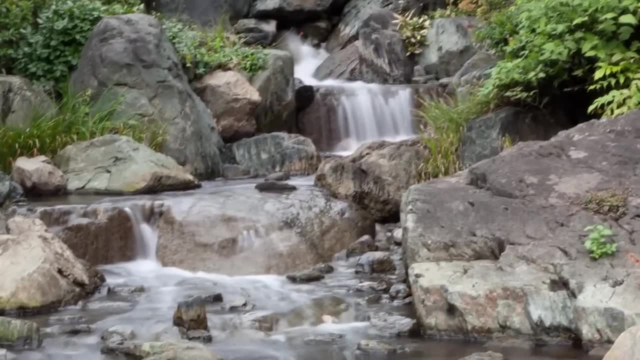 walked across the intersection, Those people who weren't moving appear more solid. Shutter speeds of more than a second are almost the same. They're almost entirely reserved for night photography and waterfalls. So here's a waterfall at one and a half seconds. 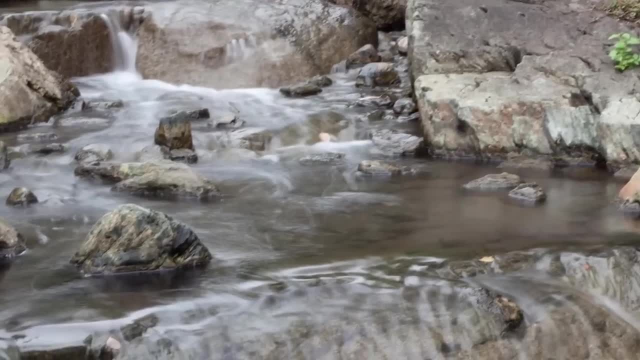 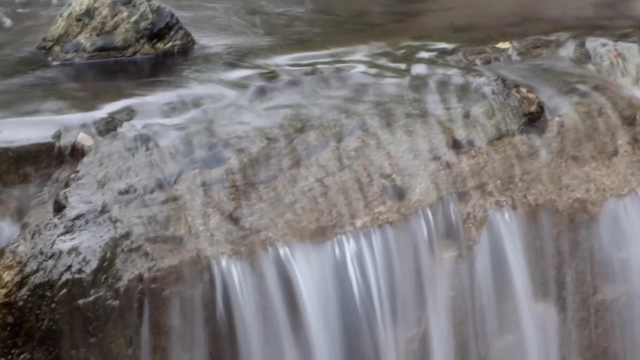 Now, if you shot a waterfall at a faster shutter speed, you would see that individual droplets were frozen. I find the effect of a long shutter speed on waterfalls much more pleasing. It gives a very feathery effect. My favorite shutter speed for fireworks is four seconds. 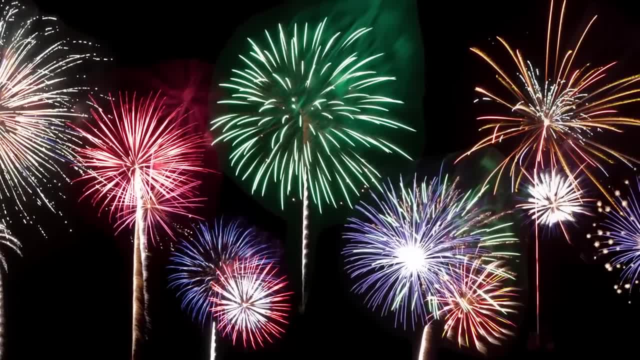 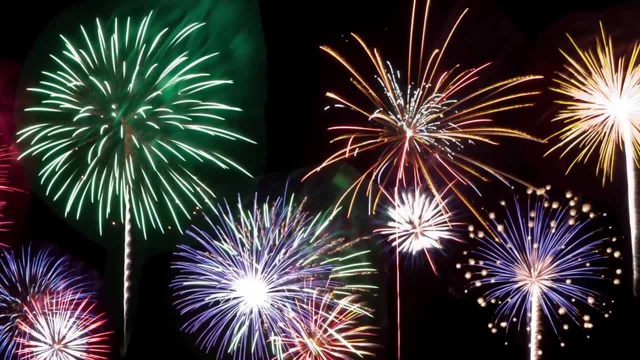 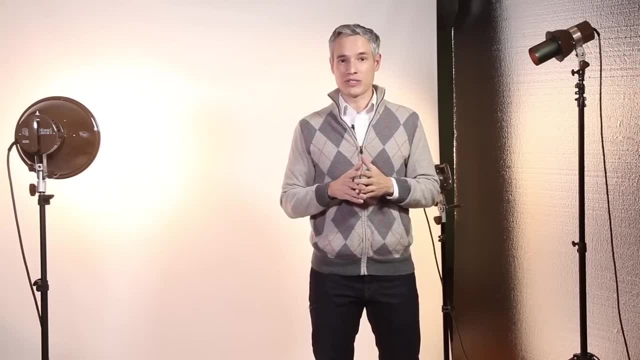 What I do is I set the shutter speed to four seconds and then take shots of individual explosions. I then blend them together into Photoshop, as I did for this shot. Here's another shot by my co-photographer, This one's at eight seconds. 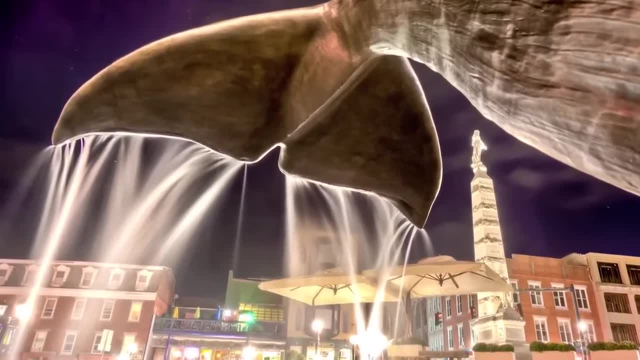 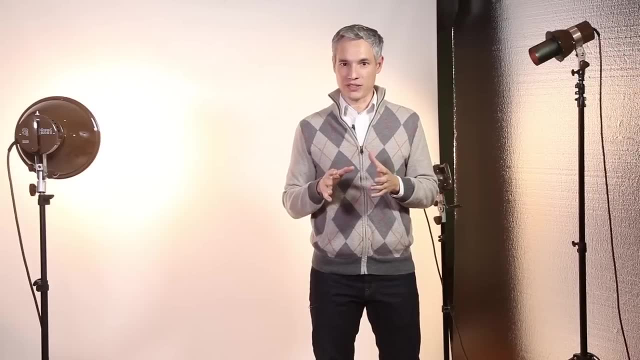 You can see that the eight-second exposure nicely blurred the water. It also allowed some of the stars in the night sky to appear. Now, most cameras only support shutter speeds of up to 30 seconds. If you want to go beyond that, you'll need to attach a remote shutter release with a 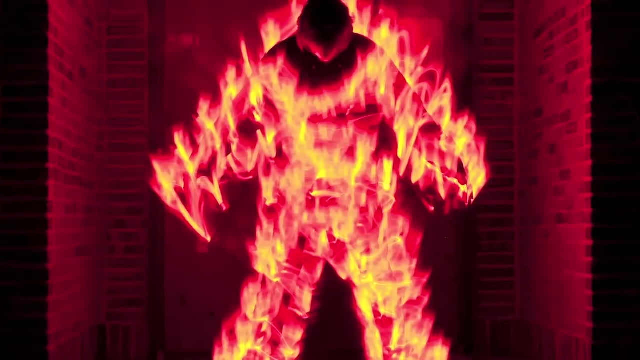 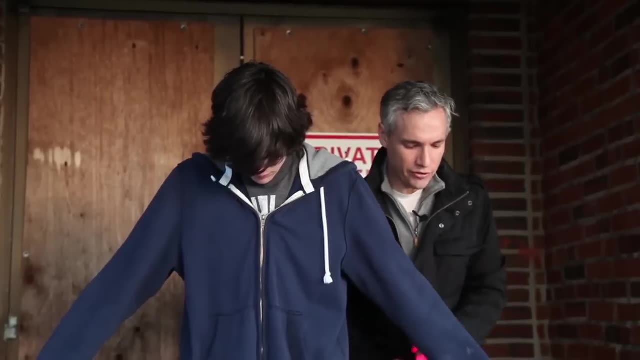 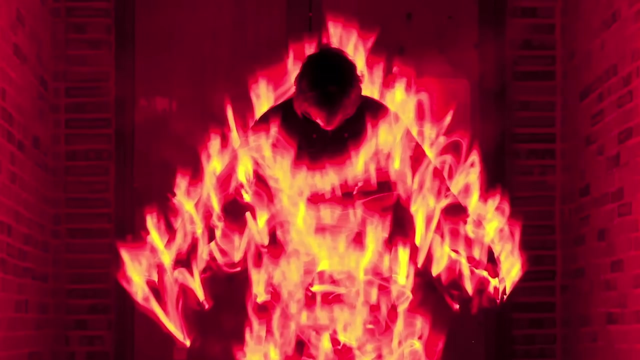 timer. I did that and set it to three minutes in order to take this light painting picture. I then held a glow stick in my hand and waved it around the subject to give the appearance of fire. Because I was moving the glow stick, the light it gave off appeared in the final image. 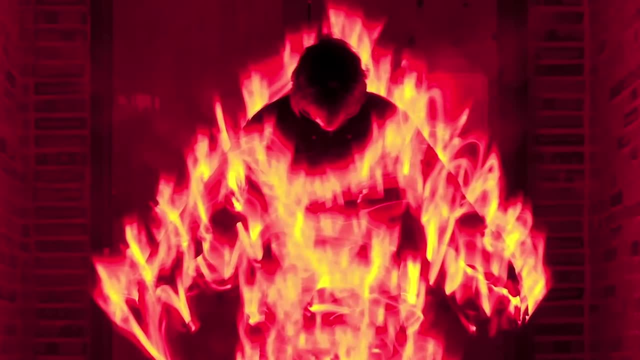 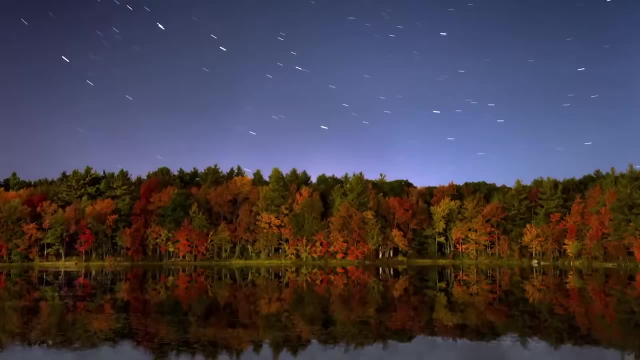 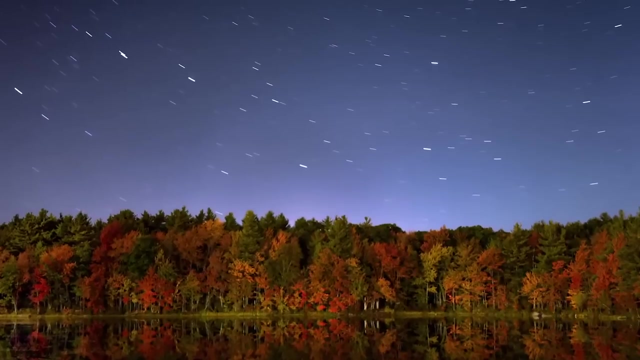 So wherever I held the glow stick during that entire period is where it appeared. It's a technique called light painting, and I go into great detail in my book. Here's a three-minute night shot of fall colors. Now, in rural areas where there are no city lights, you need exposures of three to five. 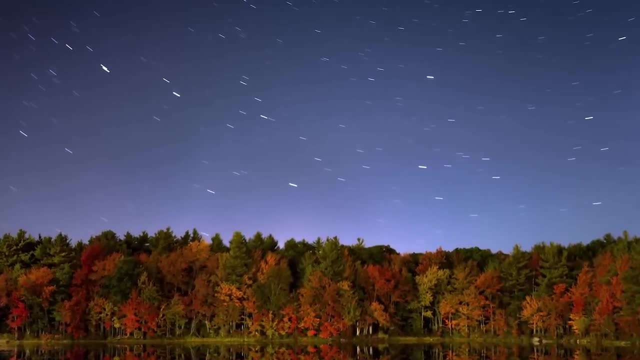 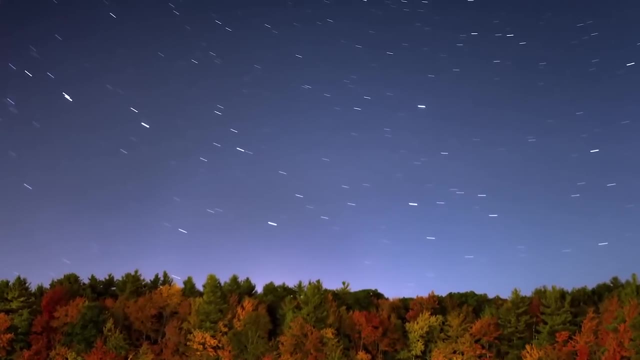 minutes just to expose things properly. As I recall, there was no moon on this night, so I was relying entirely on starlight to light the trees. If you look closely, you can see that the stars aren't dots, but rather lines. 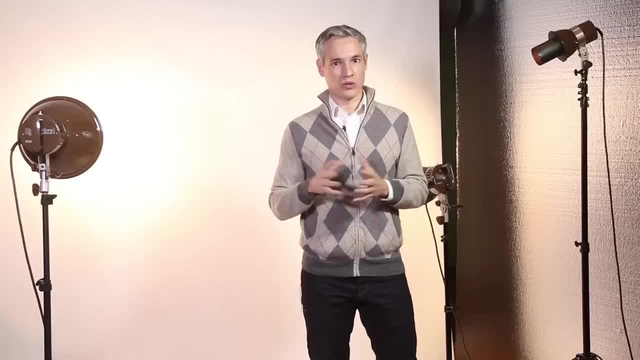 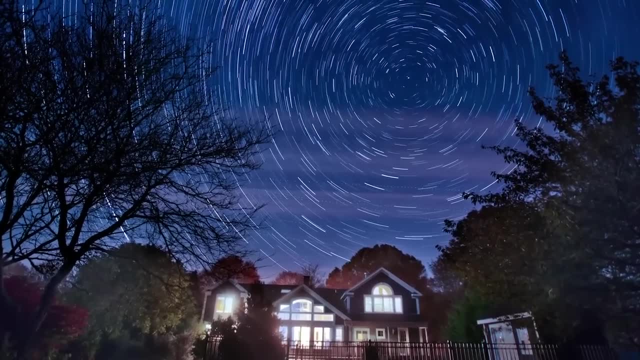 Because the earth is constantly rotating, the stars seem to move around the north star. This next picture, which is about a 45-minute exposure, illustrates that better. All of the stars are rotating around the north star, which appears in the center of that. 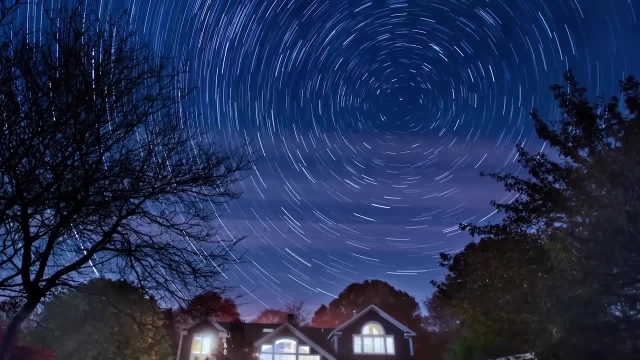 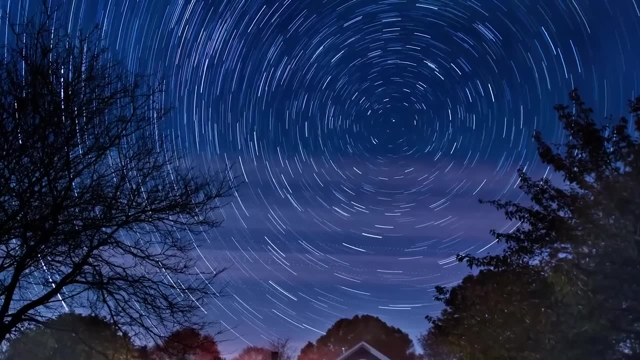 radial point, It's difficult to get a good shot. I'm keeping the shutter open for 45 minutes, so this uses a technique called image stacking. I took about 80 different pictures at 30 seconds each and then combined them on the computer. 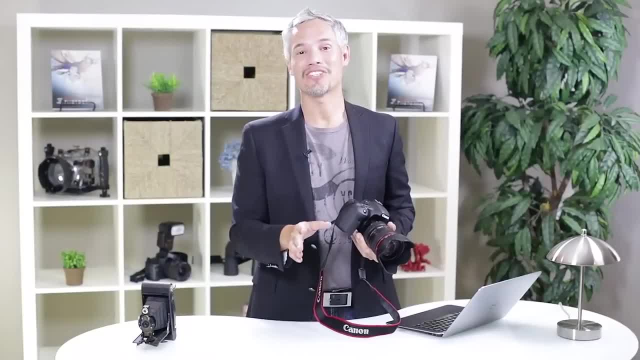 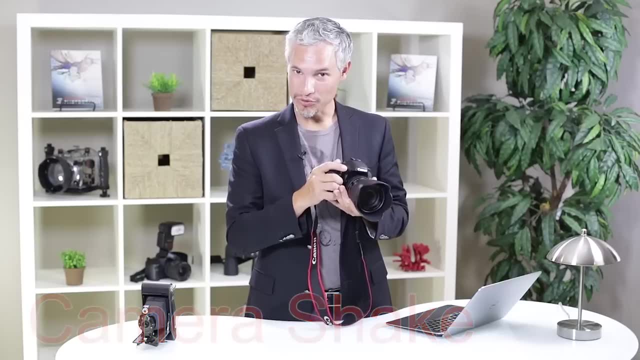 It's the best way to get a really long exposure. One of the biggest challenges of photography is avoiding camera shake. Camera shake is a condition where the camera in your hands moves around while the shutter is open And, of course, if you're looking through the camera and you move it, well, the whole world. 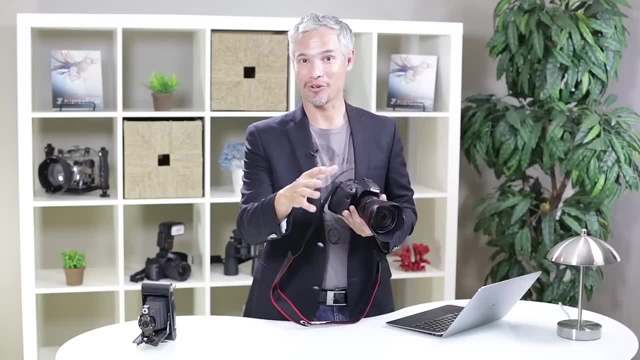 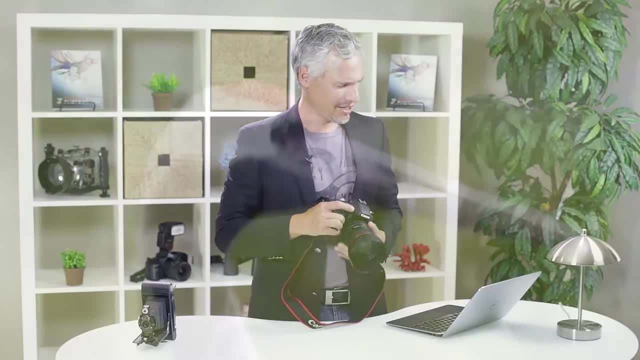 is moving right. Well, If you look at this picture, the whole world is going to be moving inside your picture and everything is going to seem shaky. So let's take a look at this example picture of a crane, And here you can see that it's blurry. 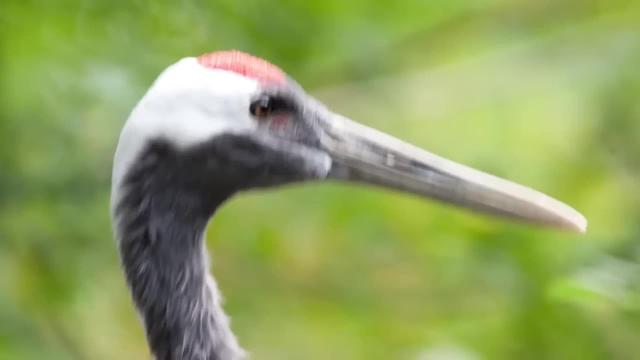 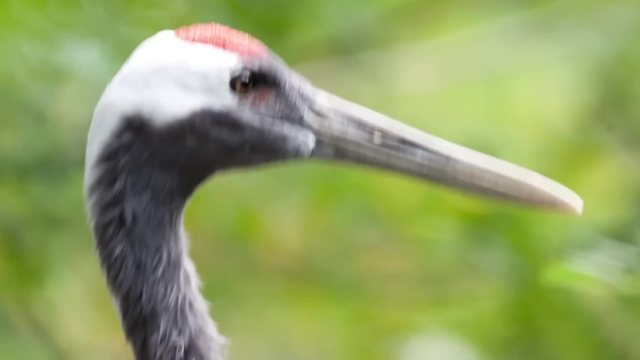 And the crane might have been moving. but I can tell that this is camera shake because if you look at the highlight in his eye you can see that it looks like there's two copies of that highlight. That's because my camera must have moved up or down while the shutter was open. 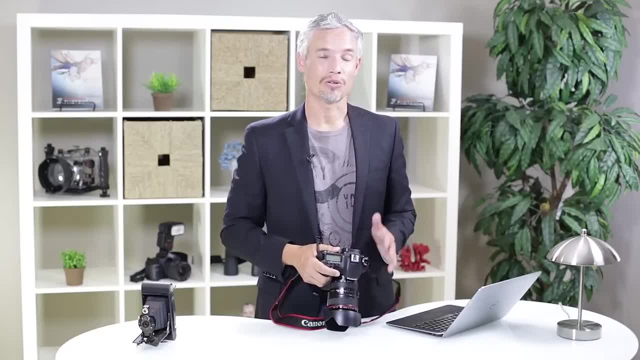 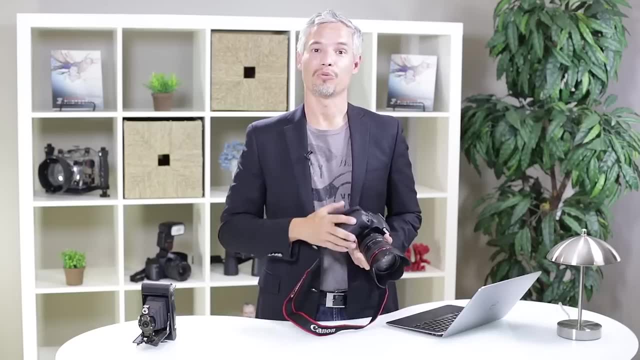 This happened. It was too slow, So what shutter speed should you have while you're hand holding your camera? There's a guideline that photographers call the reciprocal rule, And basically the way it goes is: if you're using a hundred millimeter lens you want. 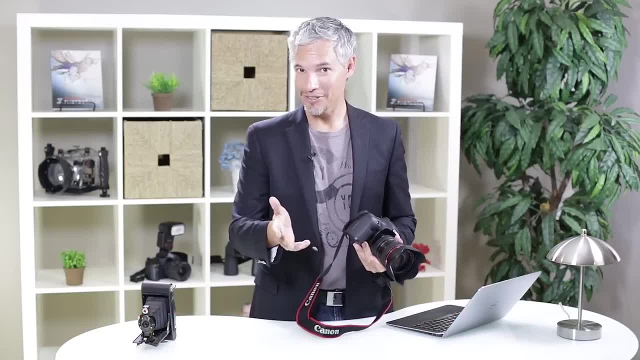 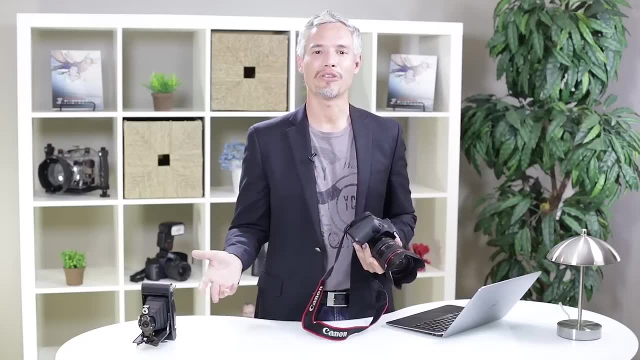 to keep your shutter speed at one one hundredth of a second or faster. So if you have a hundred millimeter lens and you're hand holding it, you could have your shutter speed at one one hundredth or one two fiftieth or one five hundredth as long. 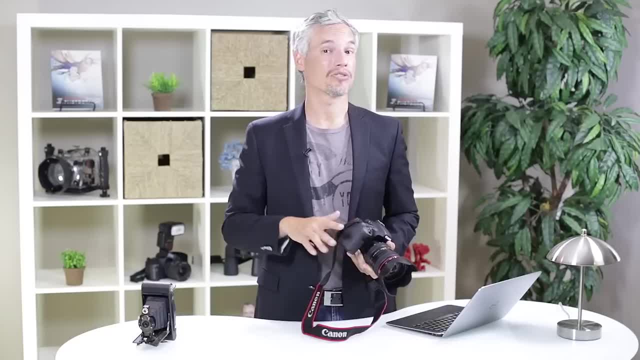 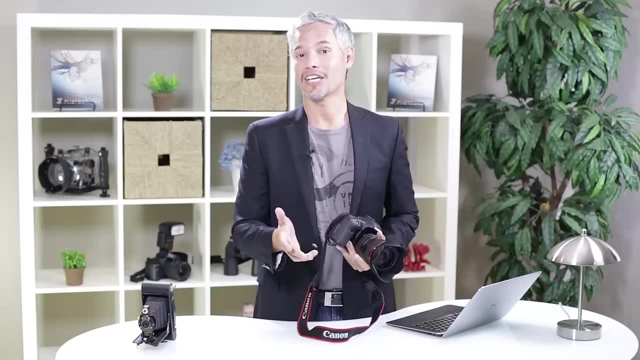 as it's shorter than one one hundredth. But if you started to go down into one Sixtieth of a second, one thirtieth of a second, it would probably start to turn out shaky. If you're using a twenty four millimeter lens, you can go with a much slower shutter speed. 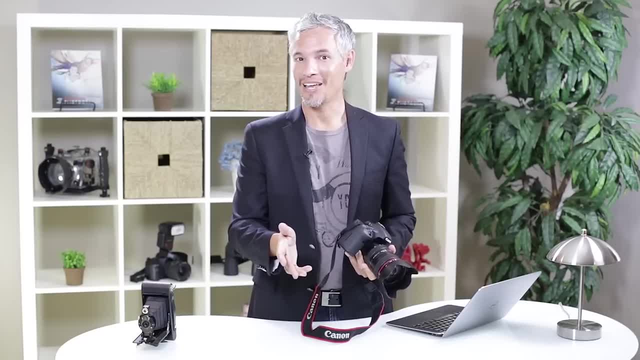 You could shoot at one twenty fourth of a second and you'd probably be OK. if you shot at one thirtieth, You'd be fine, One sixtieth, You'd be fine with wider angle lenses. Therefore, you get away with slower shutter speeds. 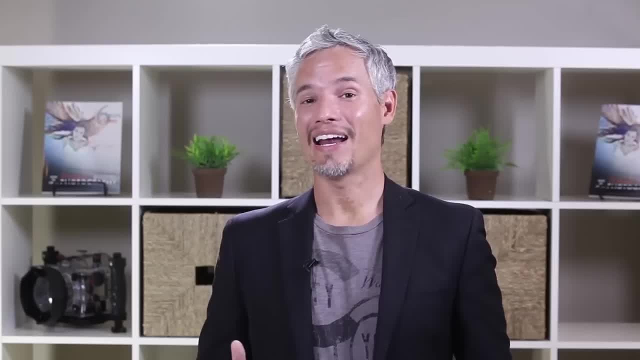 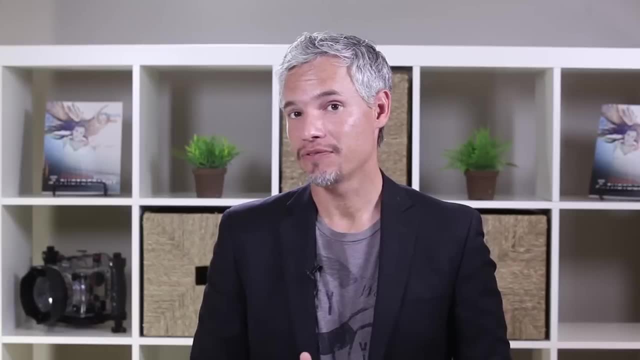 Now, the reciprocal rule is just a general guideline. It's not actually a rule. Some people have shakier hands and they'll have to use a faster shutter speed at any given focal length. Some of us have very steady hands and we can get away with much slower shutter speeds. 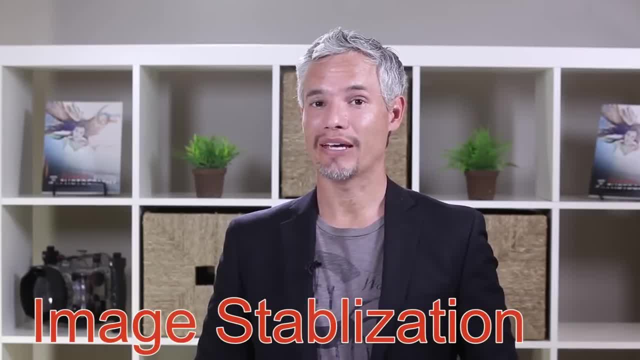 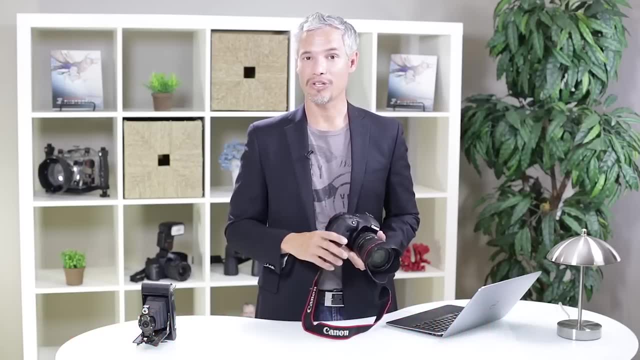 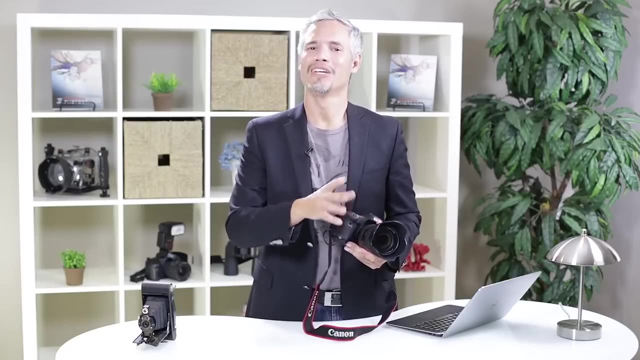 There's also a technology called image stabilization, which can make a big difference with camera shake. Nowadays, many lenses and in fact some camera bodies have image stabilization built in, and image stabilization is this electrically complex system that involves some gyroscopes and little. 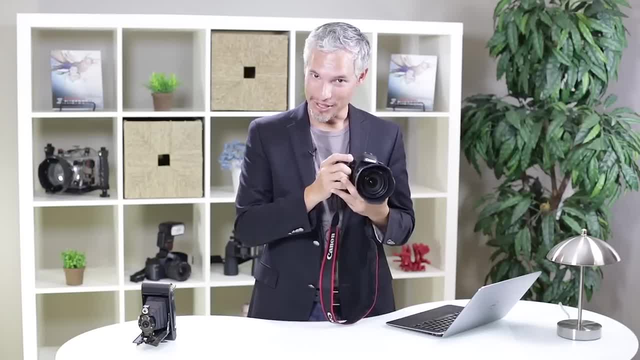 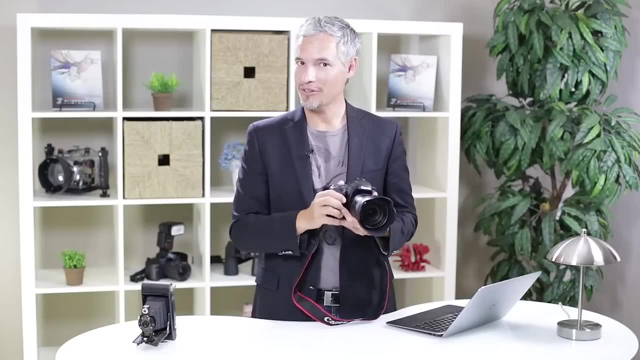 motors And basically what it does is if your hands move the tiniest bit this way, they'll move the other way And they'll counteract it And they will keep the image perfectly centered in your camera even though your hands are moving around. 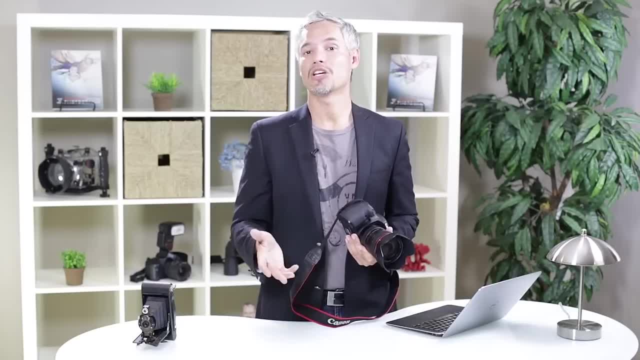 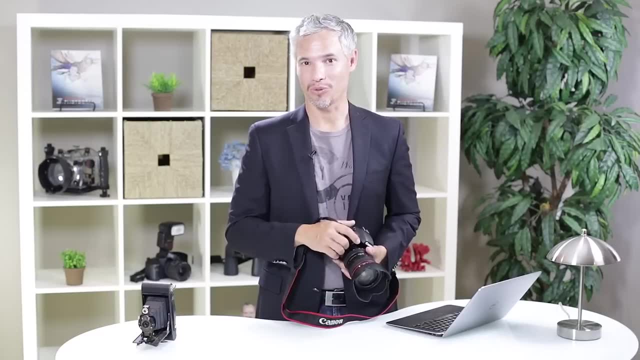 As a general rule, image stabilization lets you use shutter speeds that are four to eight times slower than you would normally be able to shoot with using the reciprocal rule. So if you're using a hundred millimeter lens with the reciprocal rule you'd want to have, 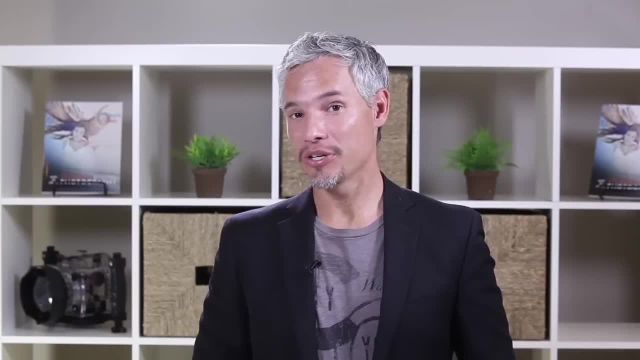 a shutter speed of one one hundredth or faster. But if you had image stabilization you might be able to get away with one thirtieth of a second stabilization. you might be able to get away with 1, 30th of a second, maybe 1, 15th of a second you. 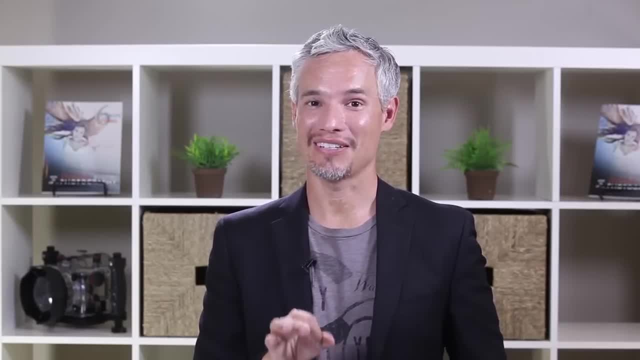 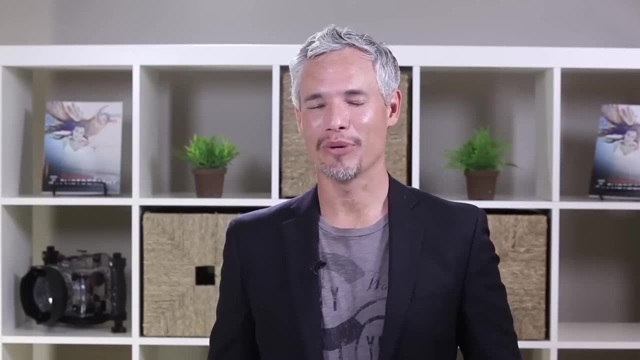 know what. you might even be able to get: 1, 8th of a second, if your subject is still different. image stabilization systems promise different levels of compensation for movement. they'll word it like the number of stops, and a stop is a doubling or a halving of the light, or the shutter speed, or the 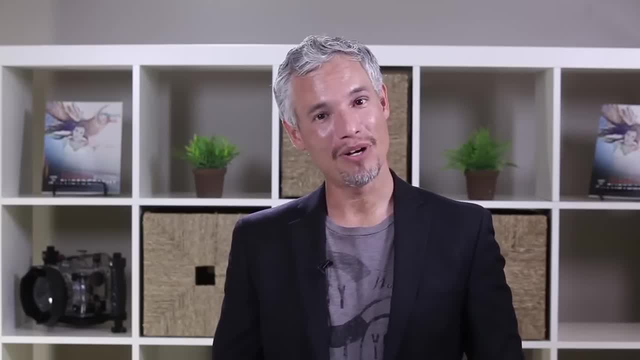 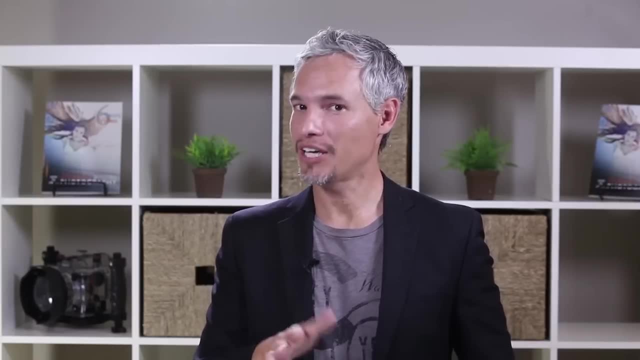 aperture. so if image stabilization offered one stop of improvement, you'd be able to shoot at 1- 50th with your 100 millimeter lens. if it offered two stops of improvement, you'd be able to technically go down to 1- 25th. let's look at a couple more example pictures. i photographed these. 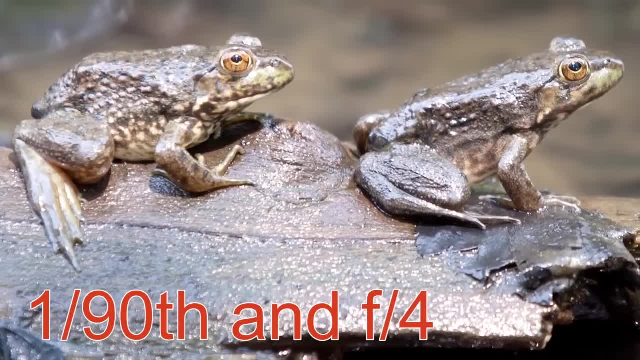 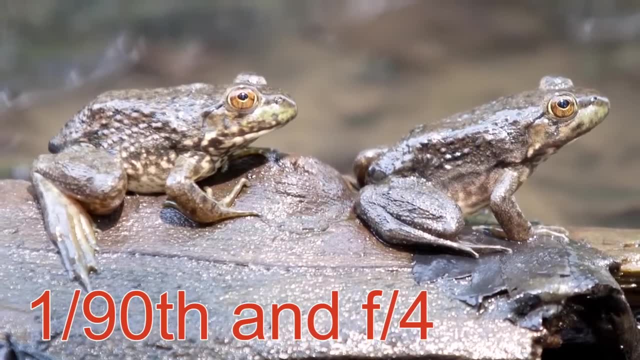 two frogs at 200 millimeters and 1- 90th of a second. this lens did have image stabilization, so as we look at the frogs they're nice and sharp. now, 1- 90th would normally be 2 slow to use with a 200 millimeter lens. i'd want to keep the shutter speed at 1. 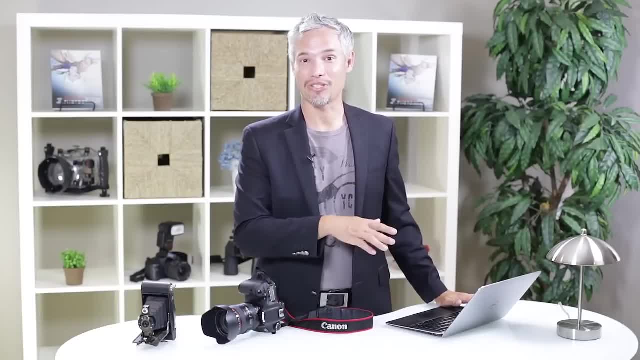 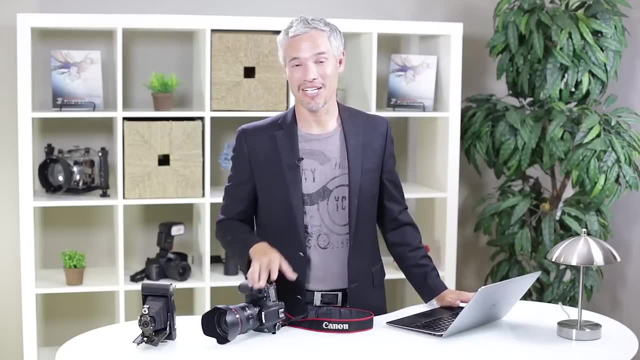 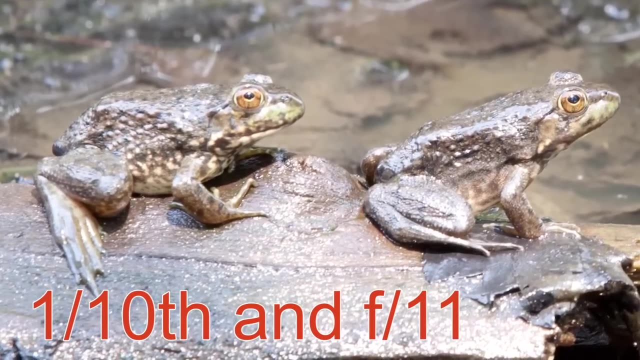 200th or faster right, but the image stabilization allowed me to go below 1 200th of a second to 1 90th and still take sharp pictures. i love image stabilization. now let's go to an even slower shutter speed. this picture was taken at 1 10th of a second, still at 200 millimeters. so here were. 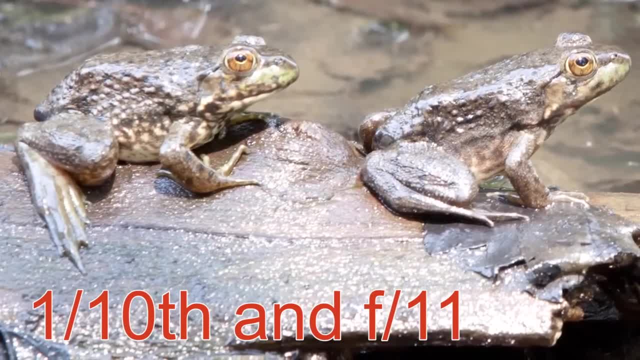 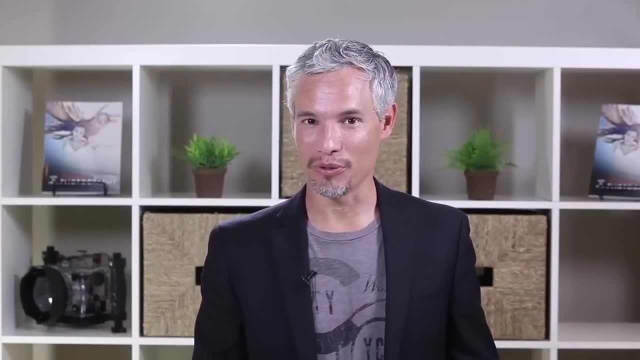 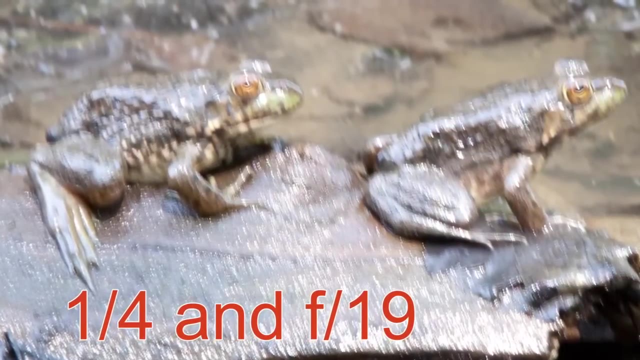 several stops below the reciprocal rule and if you look really closely you'll see it's not quite as sharp. however, i think it's still acceptably sharp for most purposes. let's try to go even slower and see just how slow i can hand hold with that 200 millimeter lens. this shot is taken at 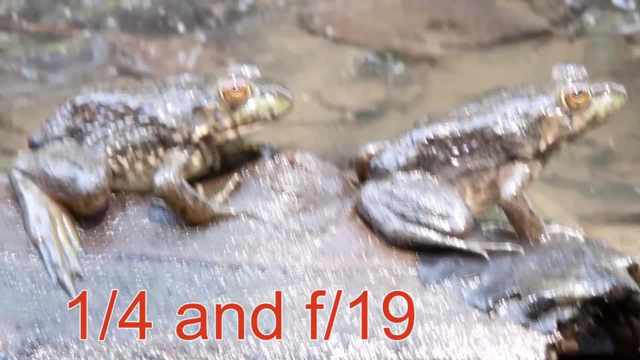 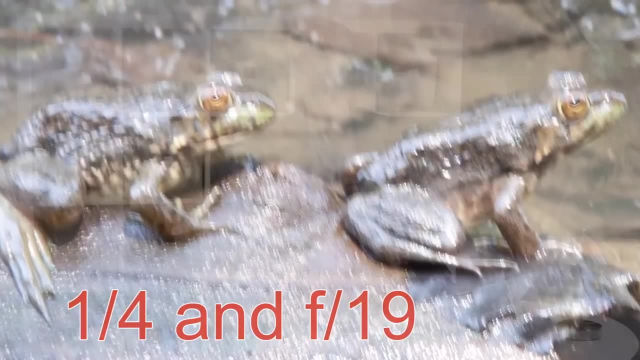 one quarter of a second, so that's something like eight stops below the reciprocal rule and, as you can see, the picture got shaky. i was not able to hand hold that 200 millimeter lens, image stabilization or no, and prevent camera shake. it is a telephoto lens, which means i generally 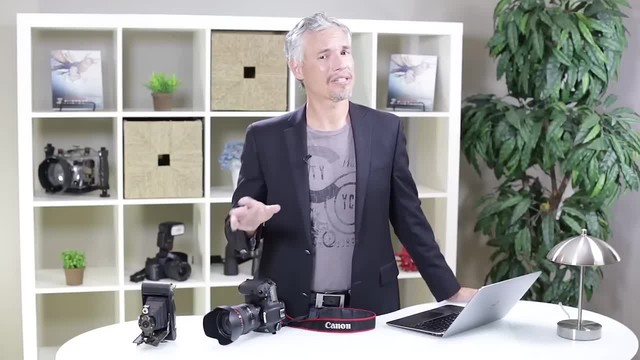 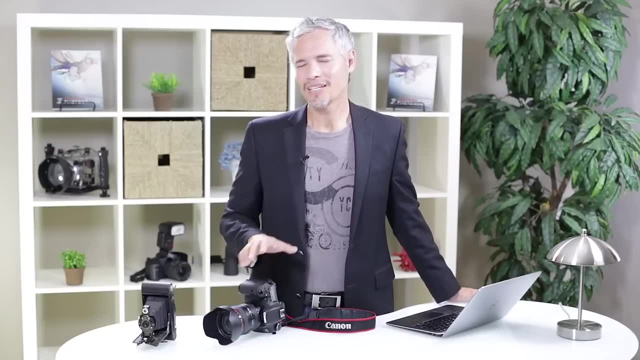 need to keep a pretty fast shutter speed and because of that you'll find that image stabilization is very common in telephoto lenses and less common in wide angle lenses. canon and icon build the image stabilization into lenses. by the way, if you happen to have a sony camera. 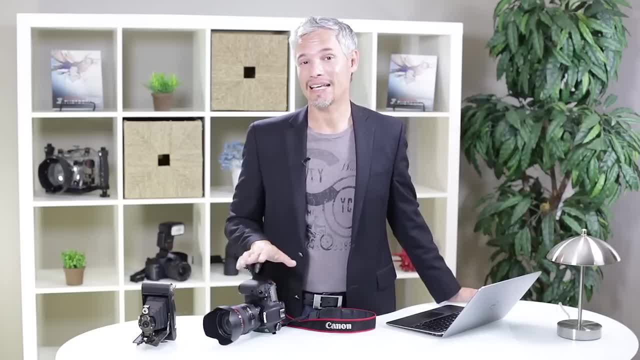 they build the image stabilization into the body. that means any lens that you attach to a sony camera will have that image stabilization built in. i personally don't consider that to be a huge advantage. i kind of like it being in the lens. but i did want to make you aware of that and 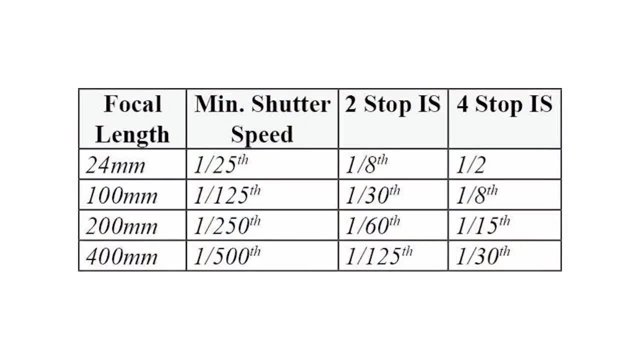 where of that difference? here's a table that simply shows what your recommended shutter speed would be, based on the reciprocal rule, if you don't have image stabilization, and the kinds of shutter speeds that you could hand hold if you had image stabilization that offered either two stops of 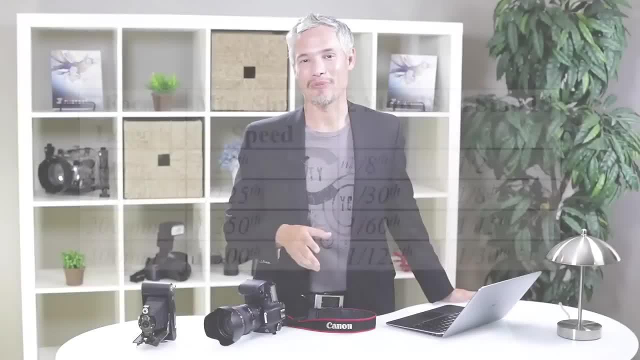 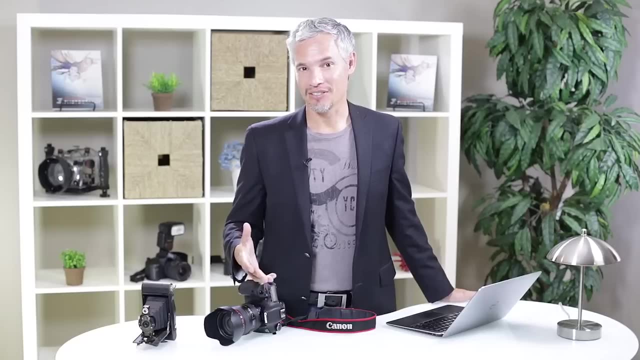 image stabilization, improvement or four stops. by the way, different camera manufacturers use different terms for image stabilization. some of them call it os, like optical image stabilization. some might call it vc, like vibration control. uh, nikon calls it vibration reduction or vr. all these offer exactly the same capabilities, i think. 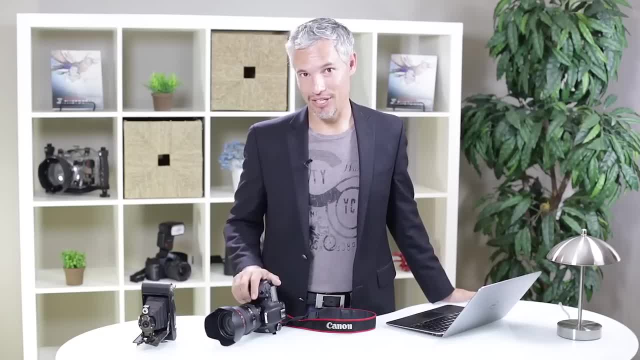 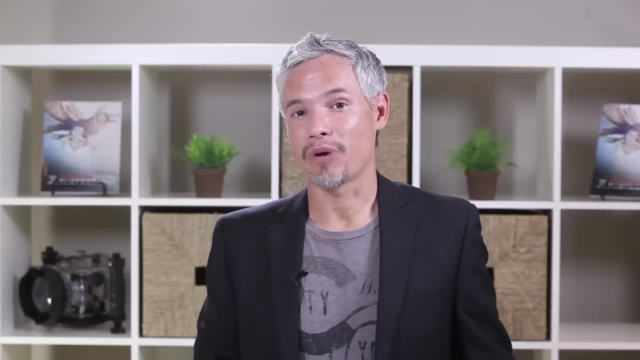 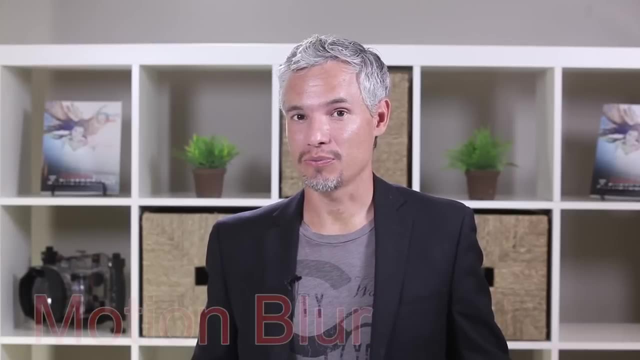 canon was basically the first company to come out and they called it image stabilization, so that's why i tend to call it that. but is os, vc, vr? it's all the same thing. camera shake is probably the most common cause of shaky pictures, but another problem that slow shutter speeds can cause is motion blur. 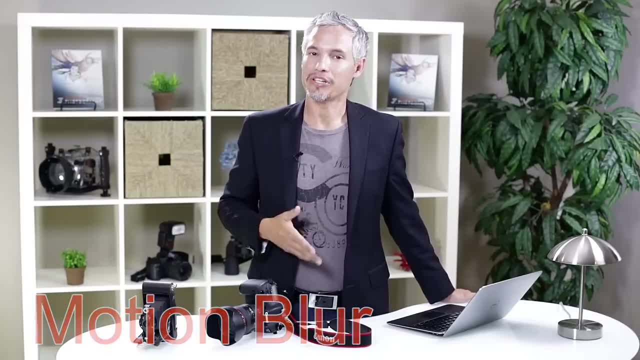 if you're taking a portrait and the subject is standing in front of you and they're pretty still, you can probably take a picture of the subject. and the subject is in front of you and they're pretty still. you can probably take a picture at 1: 30th of a second and it'll seem sharp. but you know what? 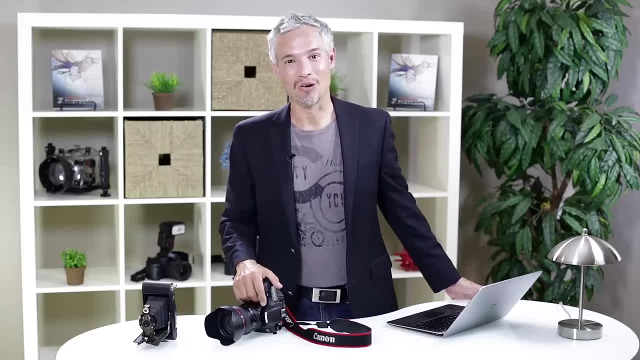 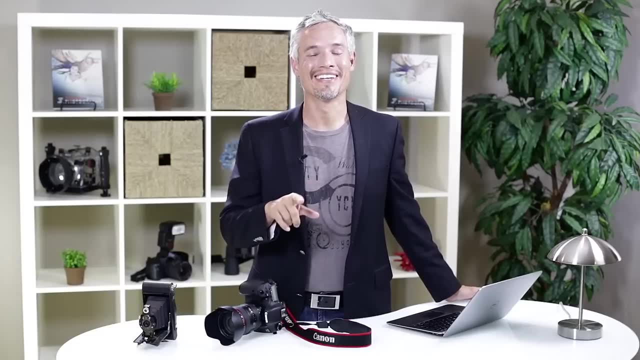 if it's a little kid and they're kind of jumpy and they're bouncing around like this 1, 30th of a second is going to cause them to be completely blurry. it doesn't have to be your shaky hands, it can be that shaky kid. so the way you solve motion blur is exactly the same way that you solve camera shake. 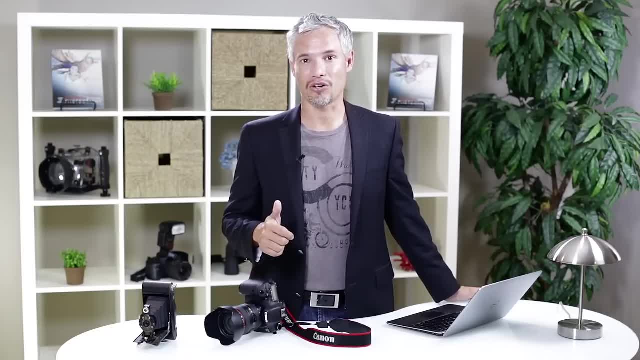 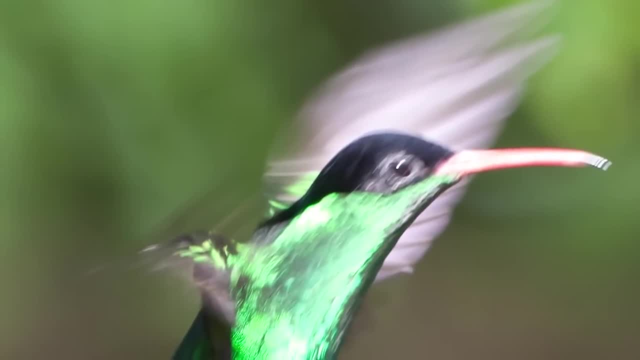 and that's by using a faster shutter speed. you just need to crank that shutter up a little bit. so here's motion blur shown in a hummingbird's wings. and of course hummingbird moves their wings really, really quickly and you need to use a really fast shutter speed to freeze. you'd probably want to be at about one. 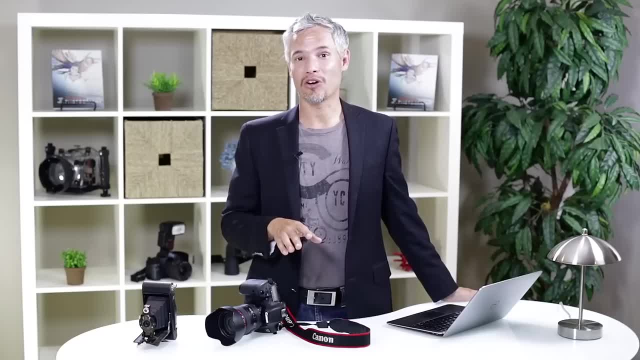 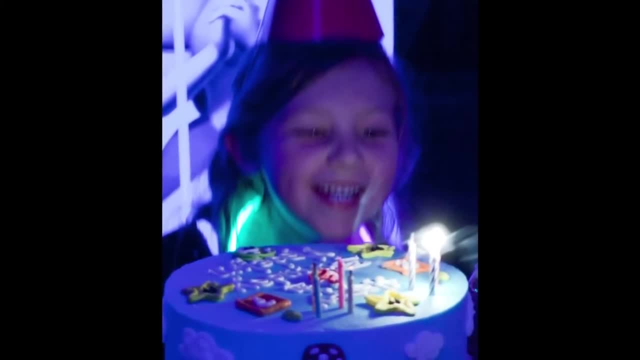 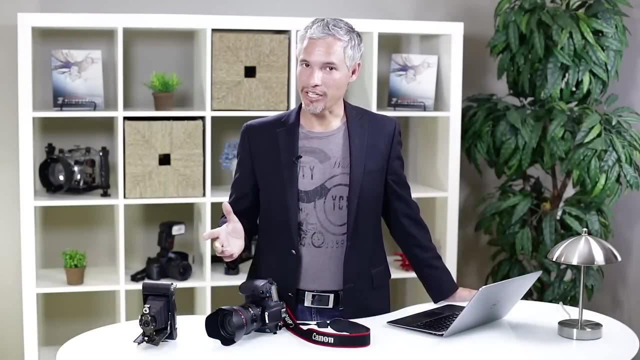 four thousandth of a second. here's a picture of my daughter blowing out her birthday candles, and because it was dark i was required to use a long shutter speed, but she simply moved too much and that caused the picture to be blurry. generally, the way you solve motion blur is by checking. 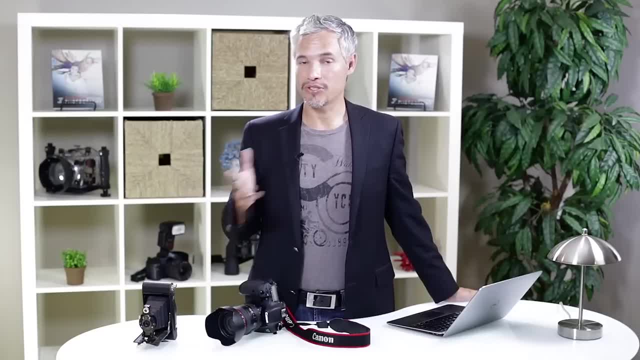 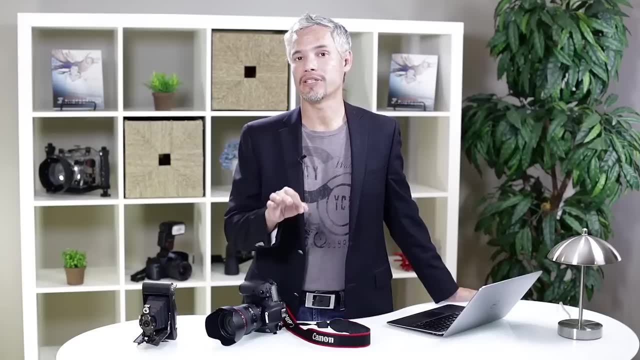 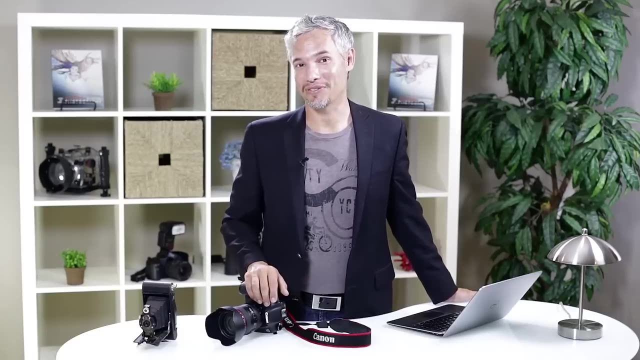 your pictures regularly and if you see motion blur, if you see the subject moving in the image, just adjust your main dial and shut a priority mode to use a faster shutter until you freeze the action. now, as you'll learn a little bit later, you can't just use the fastest shutter speed. you could just set your camera to one four thousandth of a. 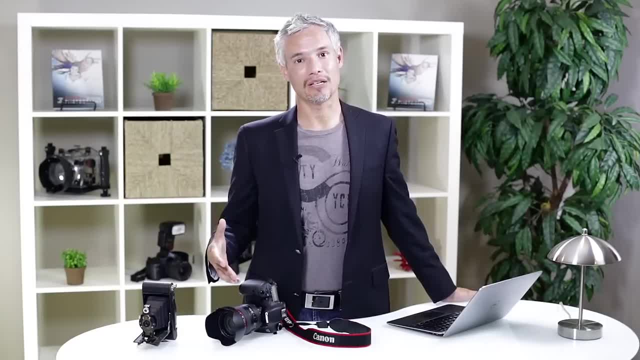 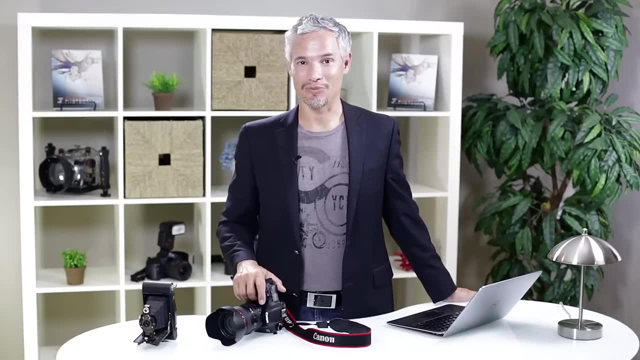 second and use that all the time, but that requires the camera to make some big compromises, like using a really high iso. so what happened is you'll end up with really noisy pictures, but we'll talk about iso coming up soon. so, speaking of low light, let's head over into the 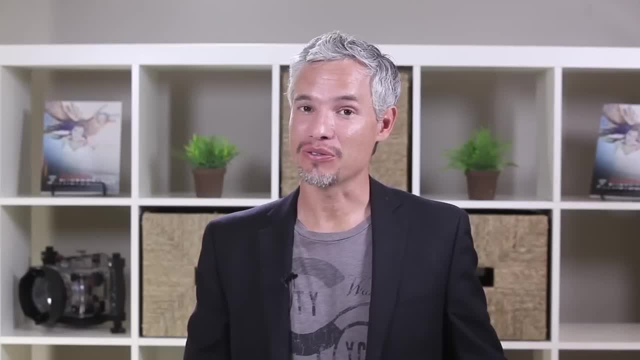 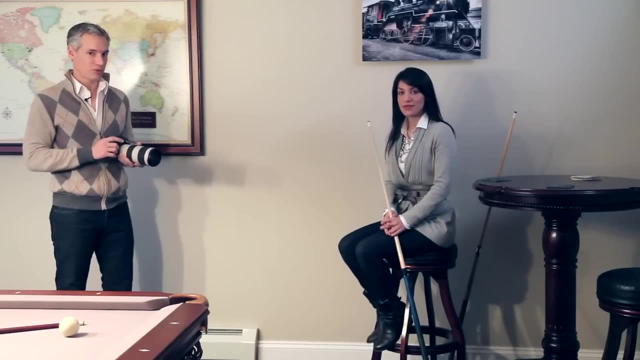 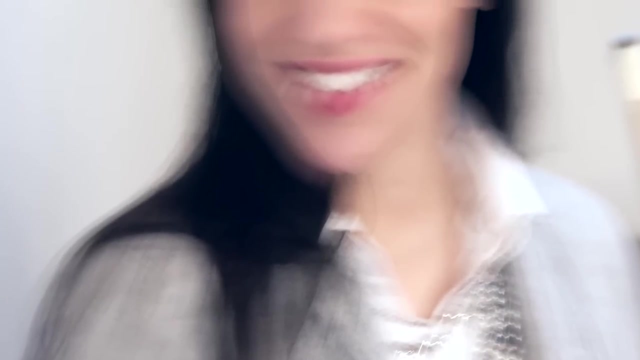 billiards room and i'll show you some of the techniques i use for getting solid pictures in low light conditions. first i'll take a picture of chelsea here using my camera's default settings. now, as you could hear, that was a slow shutter speed. that was about a second and a half. 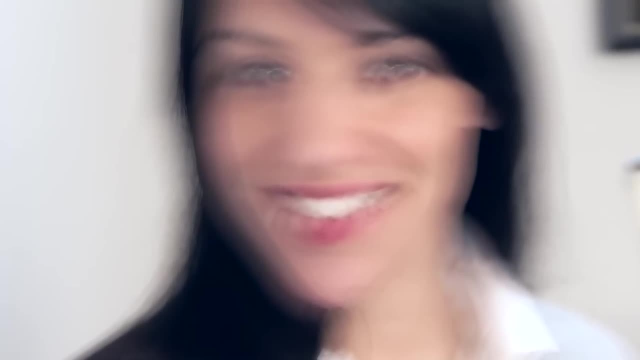 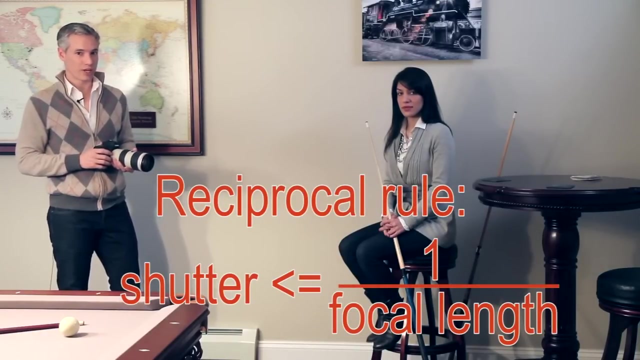 and that gave me a shaky picture. that's a phenomenon known as camera shake. anytime you take a picture that breaks the reciprocal roll, it's going to be shaky to figure out whether you're breaking the reciprocal or not. look at your current focal length. i'm currently at 70. you. 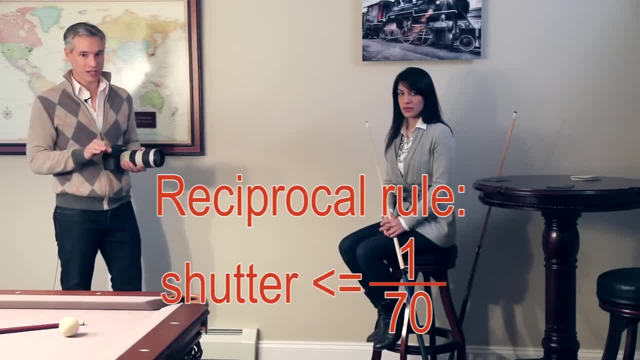 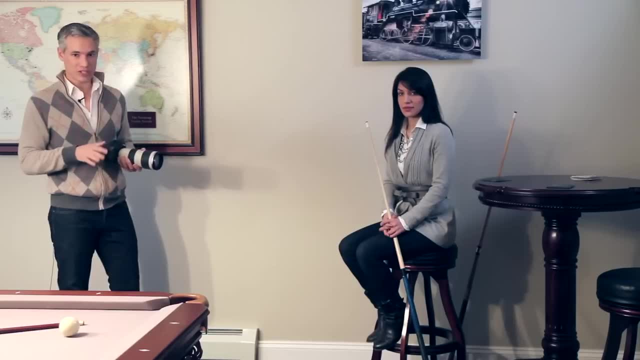 can shoot at 1: 70th of a second or faster. second and a half is much slower than 1: 70th of a second, so it ended up blurry. there are four things you can do to fix that without changing any camera settings at all. the first is just to put your camera on a tripod, but i personally don't like. 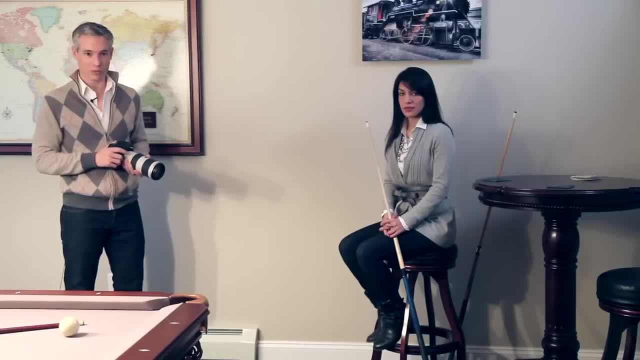 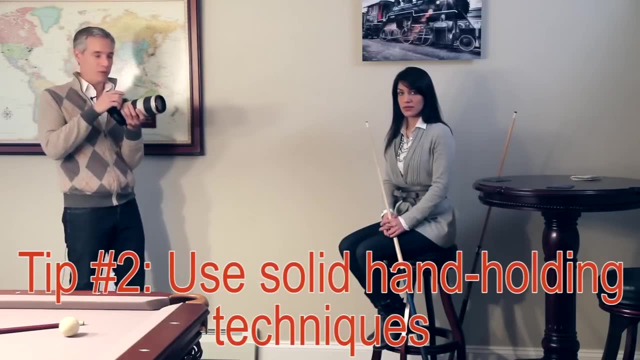 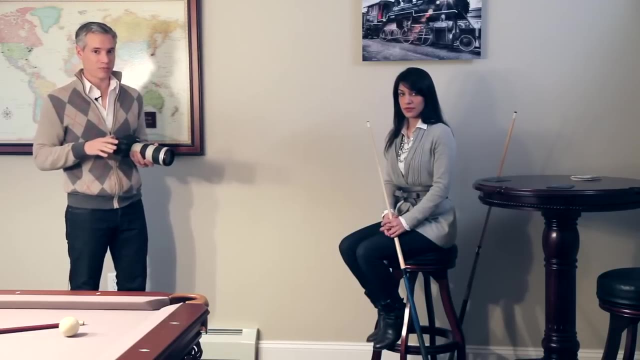 tripods, and if you're in a bar, you probably wouldn't have a tripod with you. the second is that you can use better hand holding techniques. you can do things like bracing your elbow against your body or leaning against the wall. these help stabilize your body and the camera, reducing camera shake. the third thing you can do: 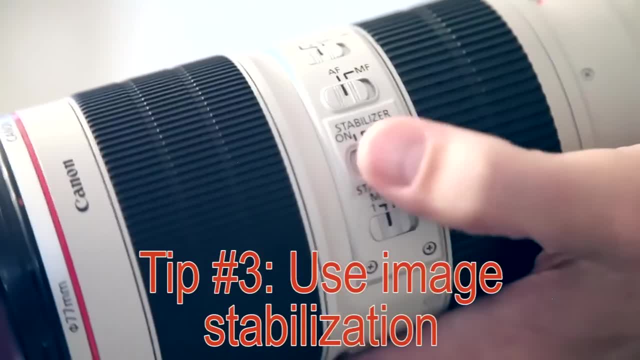 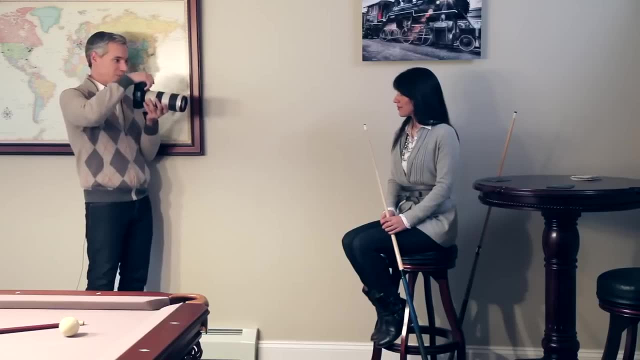 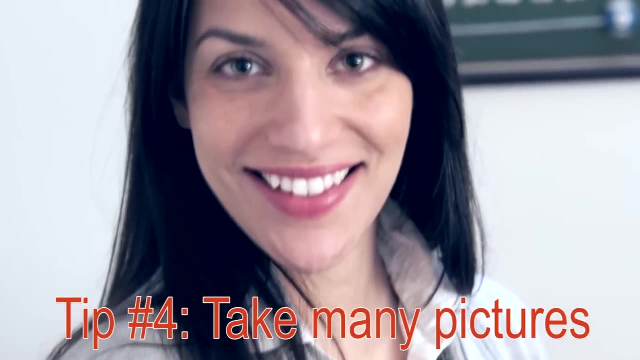 is to turn on your lens's image stabilization. so i'll turn on image stabilization, i'll brace my elbow against my body and i'll lean against the wall. we'll see if the picture turns out any better. well, the more pictures you take, the better they're going to turn out, but sometimes it's. 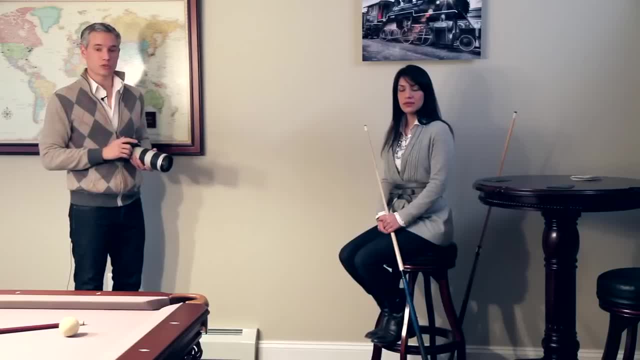 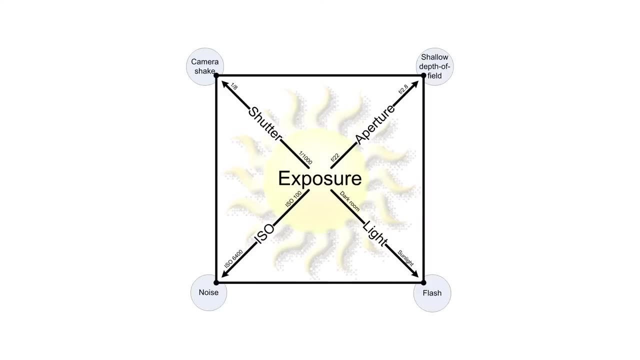 just too dark to do it without changing any camera settings. the exposure square shows you the camera setting that you can use to adjust the aperture and the aperture speed. so you can see from this diagram, when we pull the shutter speed in towards the center, we need to pull one of the other three corners out. that means we can do one of three things. 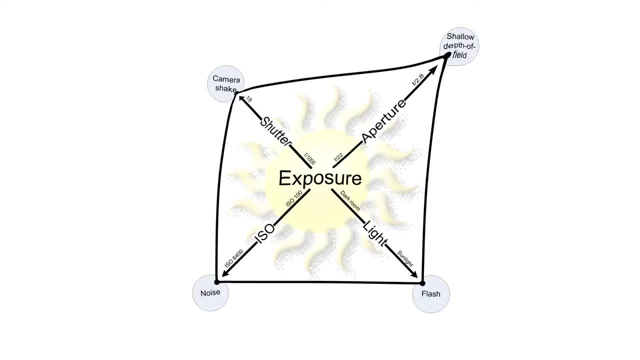 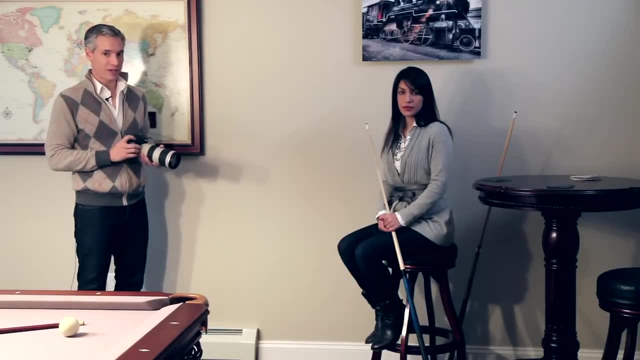 we can use a lower f-stop number that opens up your aperture, allowing more light in. so my camera was at f5.6. i'll set it to f28. not all lenses will support such a low f-stop number. the other two corners are light and 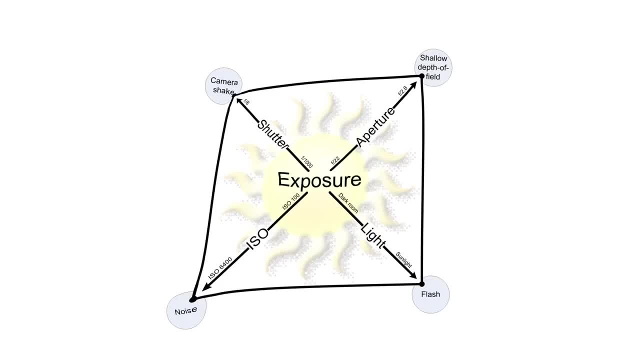 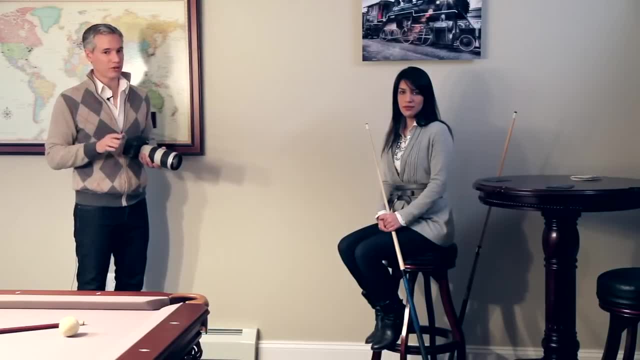 and iso. you can add more light simply by turning on the lights in the room. you can also turn on your camera's flash to up the iso. you sacrifice noise a little bit as you increase the iso. the picture is going to get a little noisier. so i've dropped my aperture down to f28. i'll also buff my iso. 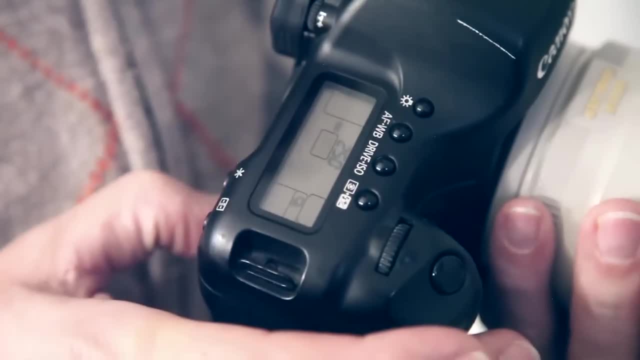 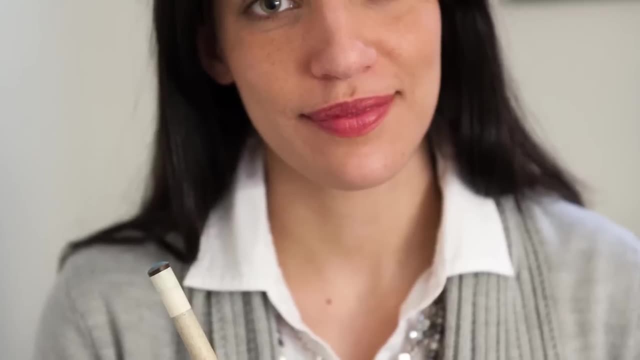 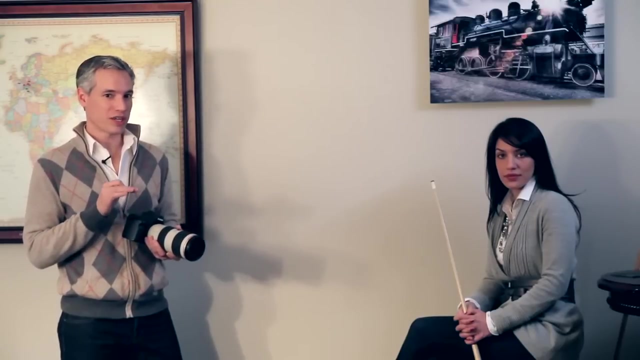 up from 100 all the way to 800, and let's take another picture and see how that turns out. decreasing my f-stop number and increasing my iso gave me a much faster shutter speed. i was at 1 15th of a second which, thanks to image stabilization, was fast enough to get a clear shot. now it's. 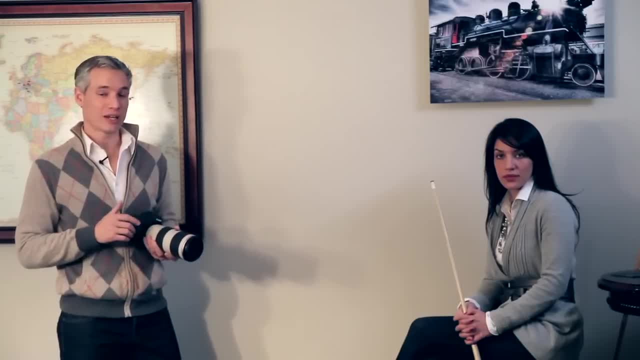 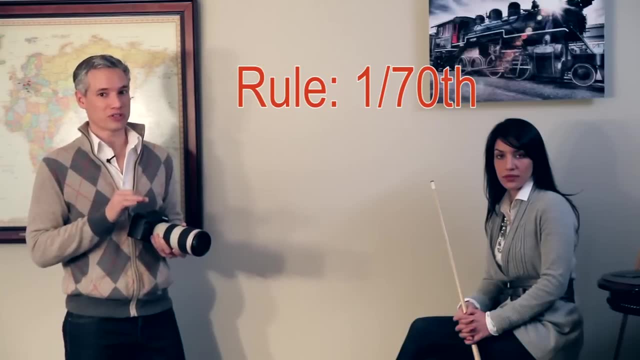 still not within the bounds of the reciprocal rule, which said i needed to be at 170th of a second or faster. this particular lens advertises that it helps out up to four stops with your hand holding, based on the reciprocal rule. so one stop off of 170th of a second. 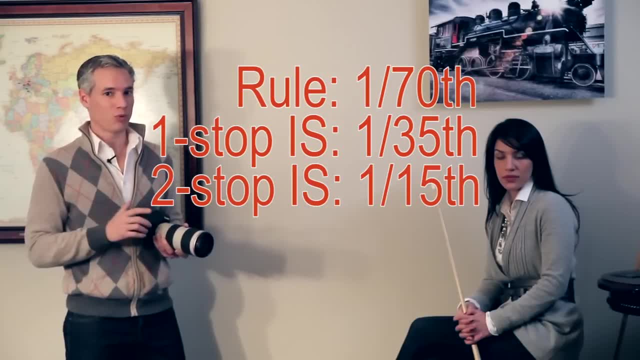 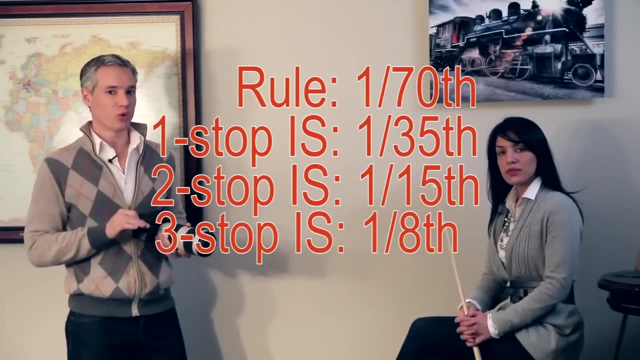 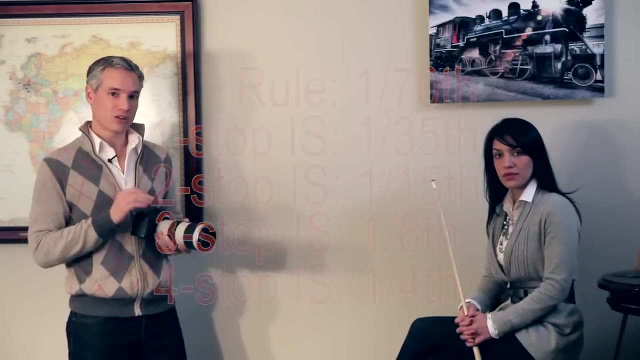 would be 1 35th of a second. two stops would be about 1 15th of a second. if this lens works as advertised, i would actually be able to shoot at about one quarter of a second handheld and get pretty clear shots. so now that we've shown how to take good shots in low light, let's move over to 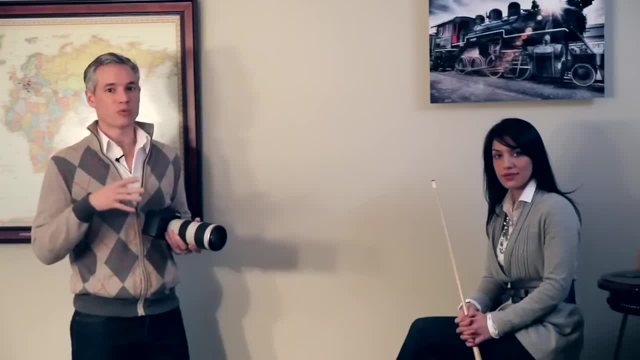 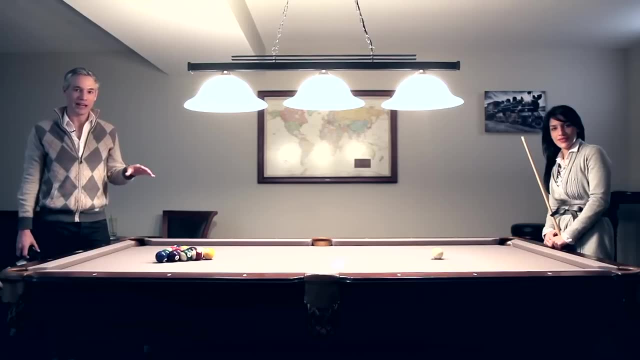 the pool table and we'll have chelsea break the balls so that we can capture some motion even when we're handheld. so i want to capture chelsea breaking these balls and i actually want to be able to capture the movement of the cue ball and the 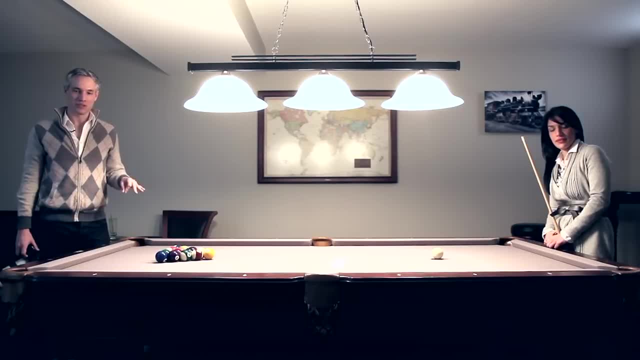 balls breaking. that means i actually need to use a slow shutter. speed flash would ruin it now. normally, you'd want to use a tripod anytime you want to capture motion. if you're in a pool hall, you might not have that as an option, though, so i will show you how you can stabilize the camera as 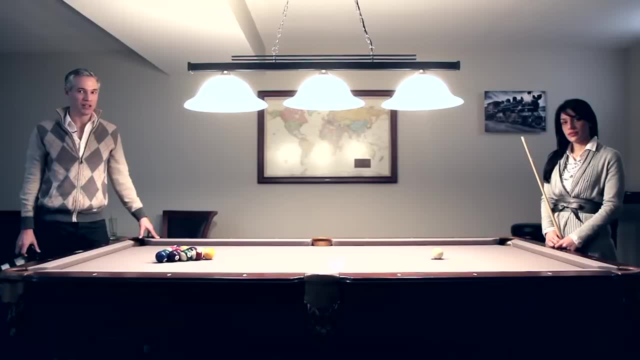 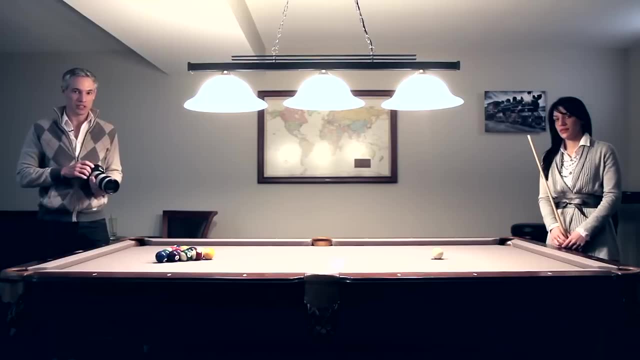 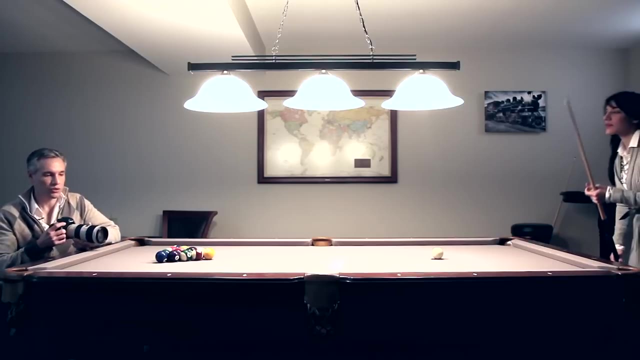 much as possible and still capture motion in a dim environment. so, as before, i'm going to use image stabilization. i'm going to crouch down. the lower you can get, the more stable you're going to be. i'm going to go ahead and use the pool table itself to stabilize myself. 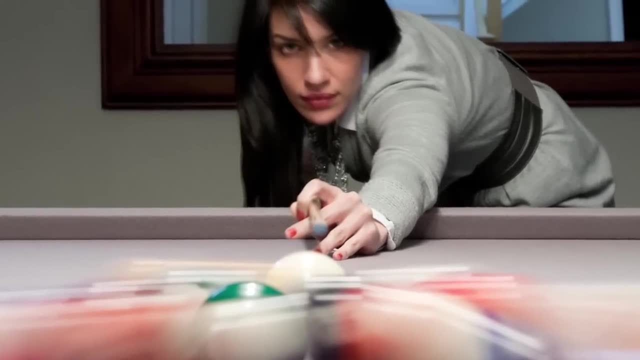 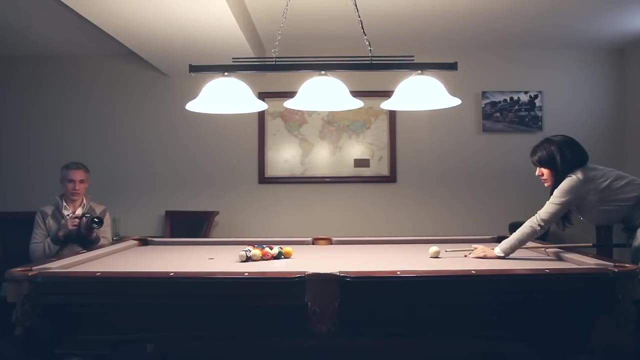 getting the shutter speed. this right always requires some trial and error, so now i'll demonstrate how to take a shot in low light. if you can't brace against something, i'm going to use my body as much as possible. you can see, i'm on the ground. additionally, i'm going to 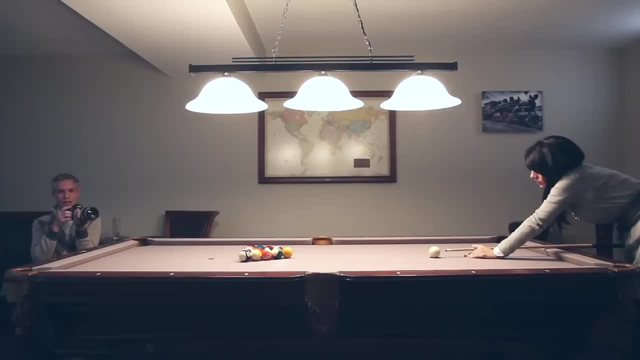 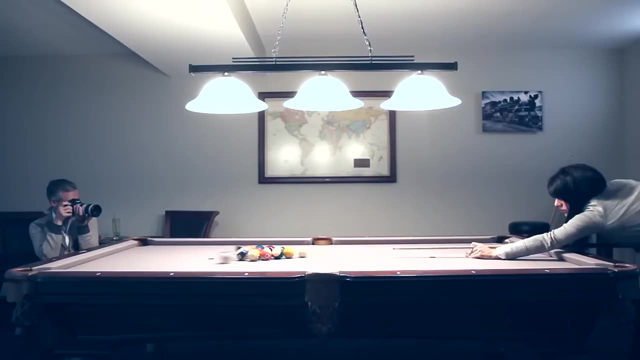 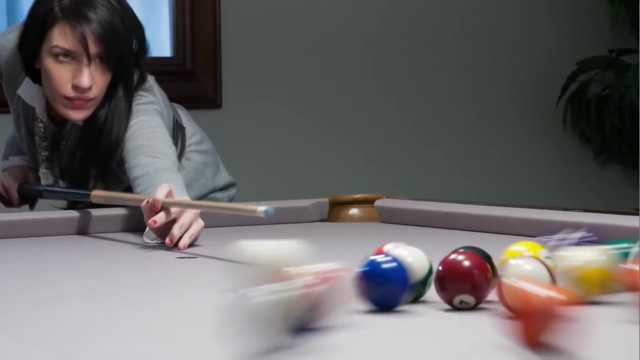 put my elbow right on the ground, and i'm going to put my elbow right on the ground and i'm going to put my elbow right against my chest and lean back against my heels. this makes my body as stable as it can possibly be. so the best shot was at 1, 6 of a second. that's normally way too slow to hand hold a shot at. 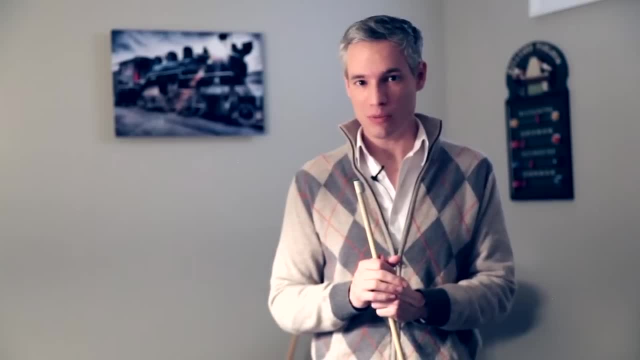 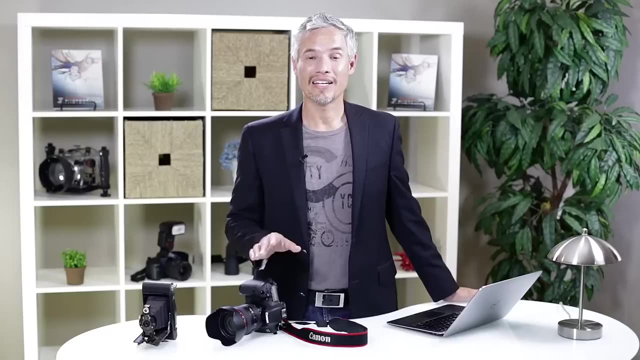 70 millimeters. however, a combination of image stabilization and good hand holding technique allowed me to get a nice, clear picture that still captured the motion. now let's talk about aperture. as i demonstrated earlier, aperture is the opening on the lens. aperture is numbered in a really 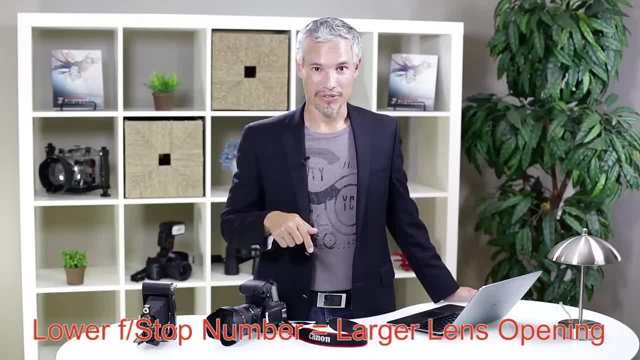 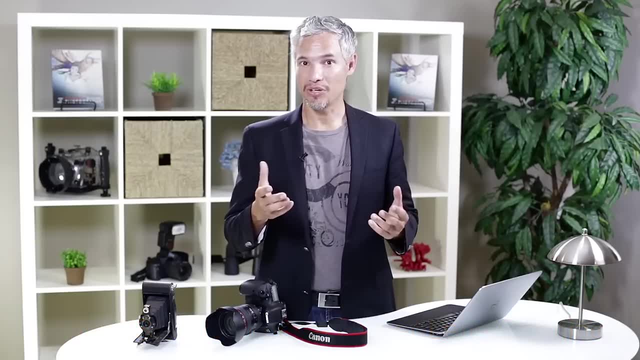 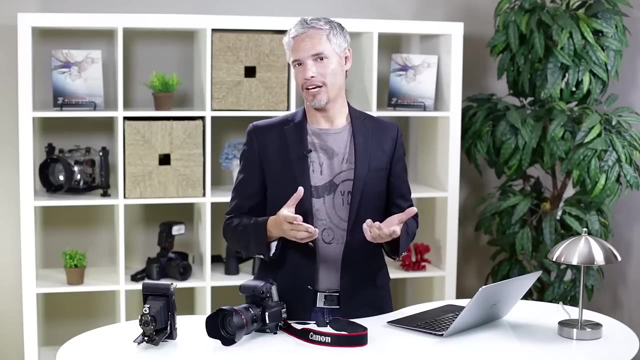 strange way though, with aperture the lower f-stop numbers, such as f 1.4, indicate a larger lens opening. higher f-stop numbers, like f-22, indicate a smaller lens opening. now this clearly impacts the amount of light getting to the lens. if you had a really big hose, a bunch. 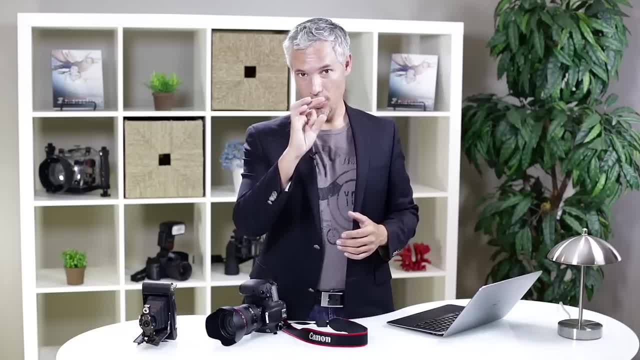 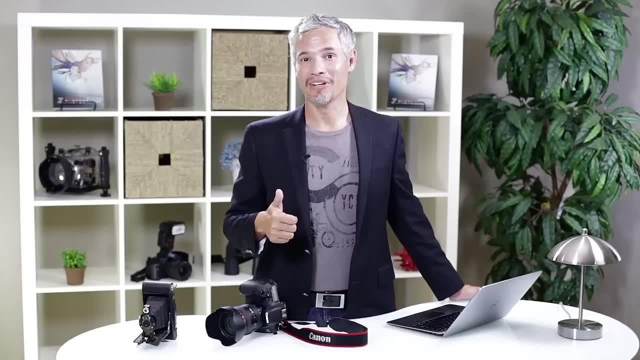 of water could rush through it as fast as it wanted, right? if you had a really small hose, will not have nearly as much water would get through it and light works the same way. if you use a really high f-stop number, well, you're going to end up with a really slow shutter speed because that small. 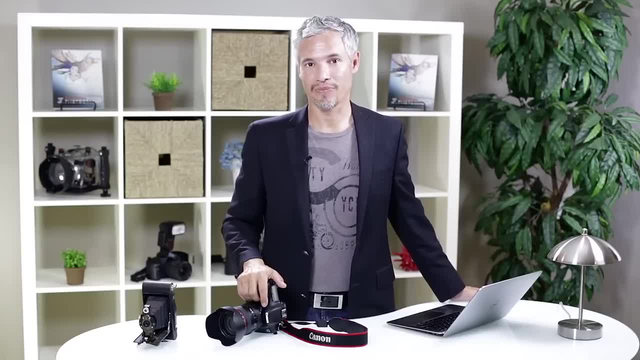 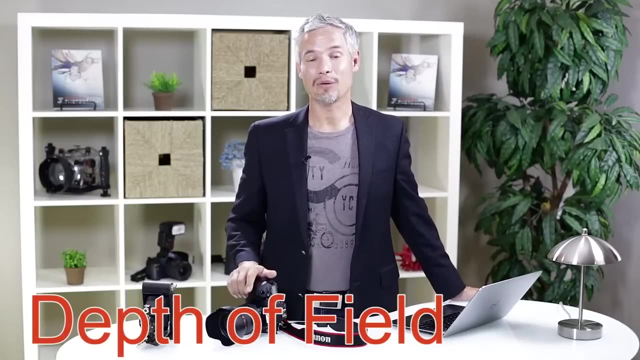 aperture is blocking most of the light from getting to your camera. so aperture affects a couple of different things and obviously it affects the shutter speed by simply blocking the incoming light and requiring your camera to use a longer shutter. but it also affects something called the depth of field, and the depth of field is how much of your 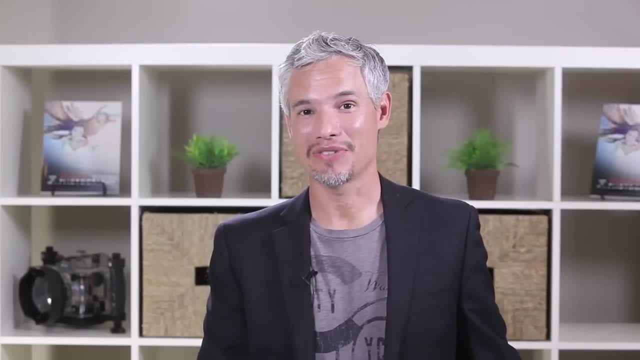 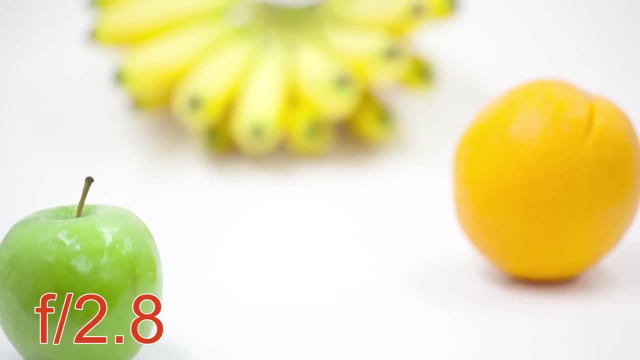 lens is in focus. let's take a look at some sample pictures. here we see some fruit on a white background and i've focused the camera on the apple. i was using a 150 millimeter lens set at f 2- 8.. you can see the apple is quite in focus, the orange quite blurry and the bananas are just. 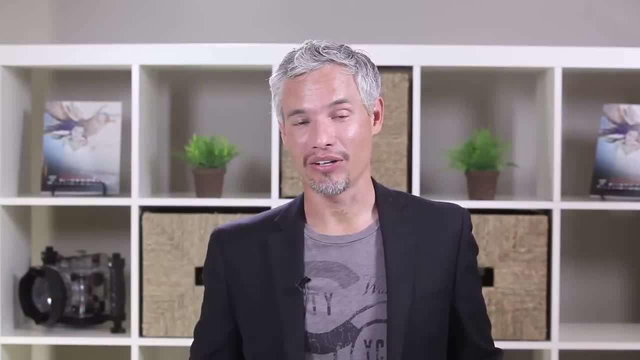 completely blurry. now with my camera in aperture priority mode, i'll adjust the main dial and choose a higher f-stop number. this is f8 and you can see that the aperture is a little bit lower than the f-stop number and the aperture is a little bit lower than the f-stop number. so you can see that. 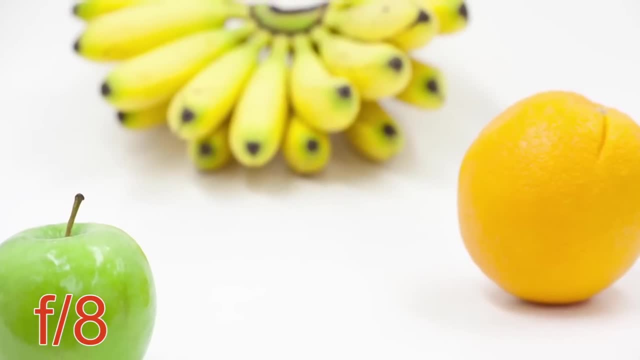 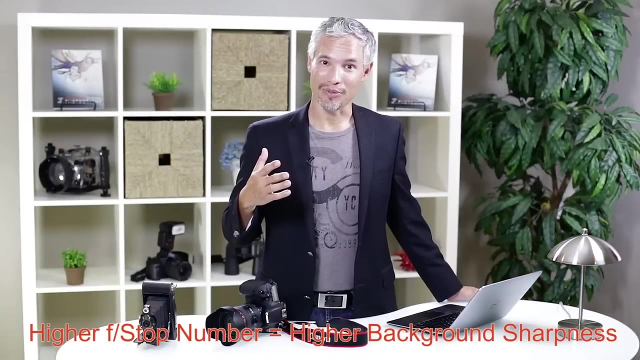 the aperture is a little bit lower than the f-stop number and the aperture is a little bit lower than. as you can see, suddenly that orange seems to be sharp and the bananas are quite a bit sharper. by using a higher f-stop number you increase the background sharpness. this is a really important 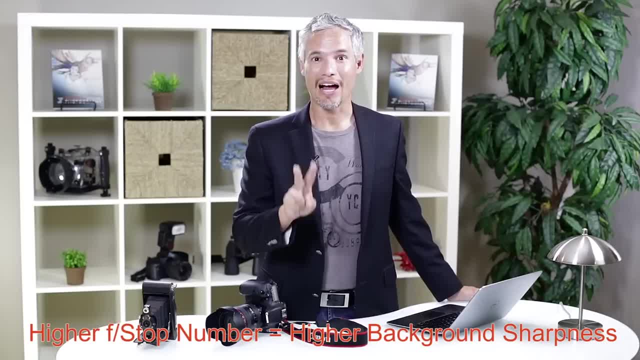 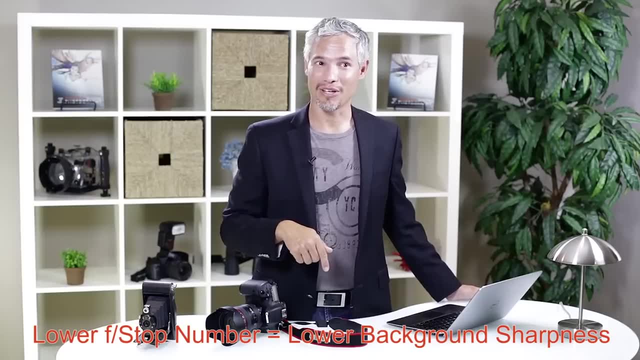 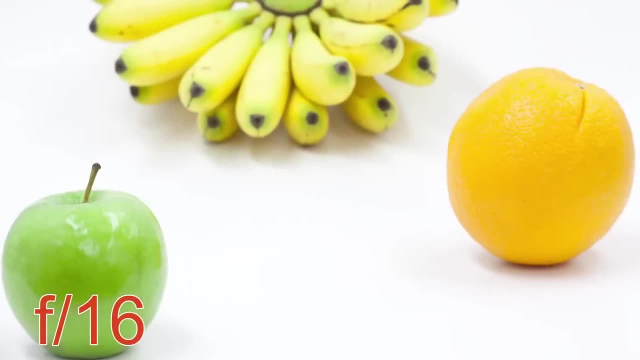 concept. so i'll repeat it: higher f-stop number, higher background sharpness, lower f-stop number, lower background sharpness. basically, the lower the f-stop number, the shorter your depth of field and the more blurry the stuff that's not your focus point is going to get. let's take a look at another picture. this is that. 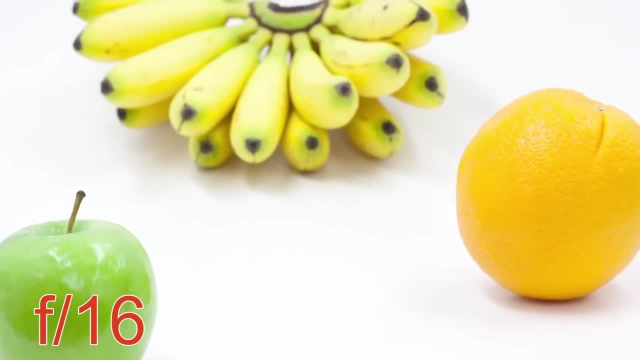 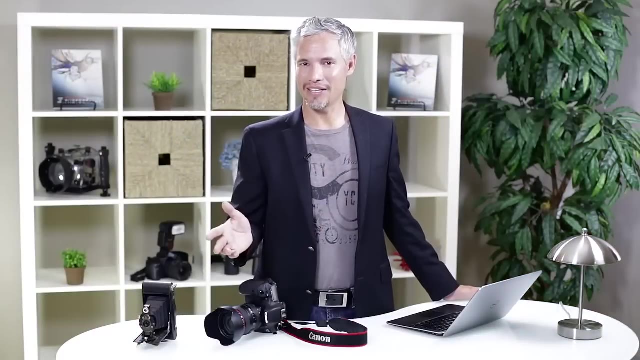 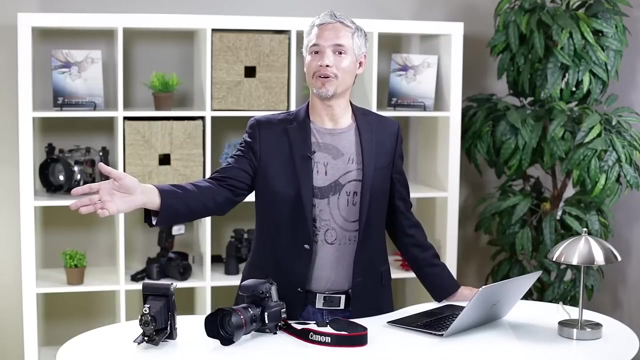 same scene at f16. i didn't change anything. all i adjusted was the camera's aperture and aperture priority mode. as you can see at f16, the bananas suddenly come into focus. in fact, the entire scene is in focus. if you're taking a picture of a landscape and you want everything to be in focus, 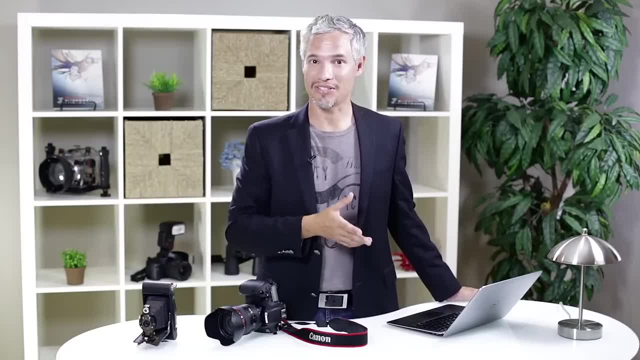 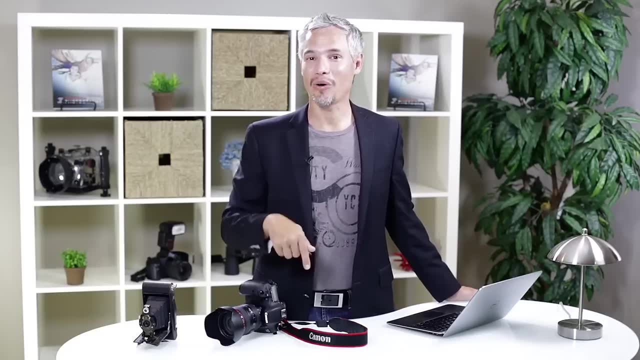 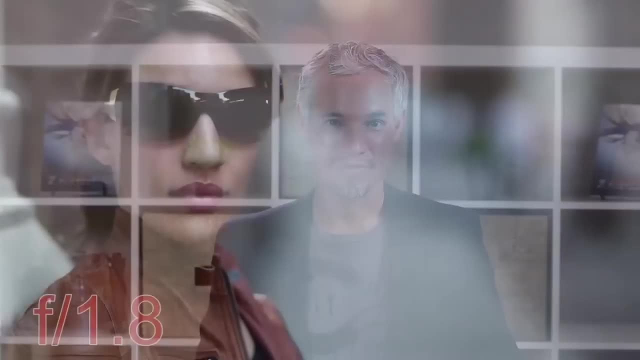 clearly you'd want to use a high f-stop number like f16. if you're shooting a portrait and you want a nicely blurred background, obviously you'd want to use a low f-stop number, because low f-stop number, low background sharpness. here are some more sample pictures. this is chelsea in. 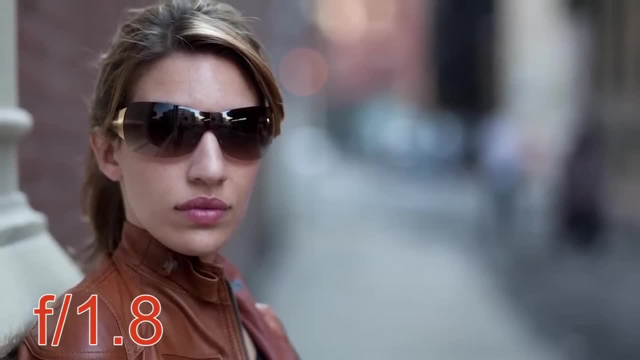 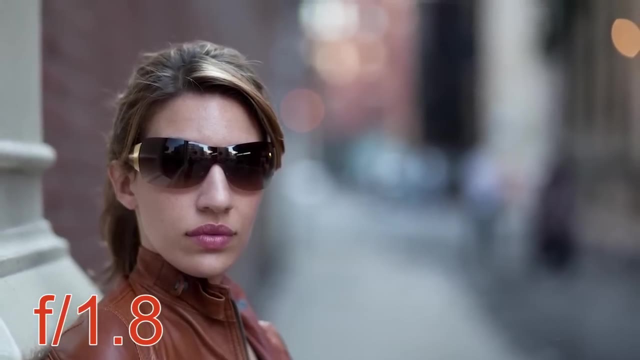 new york city, taken with an 85 millimeter lens at f 1.8, and as you can see, these streets behind her are quite blurry. you can kind of make out street lights and other features, but everything is quite blurred and it's kind of nice for a portrait right. it helps to eliminate distractions, which is 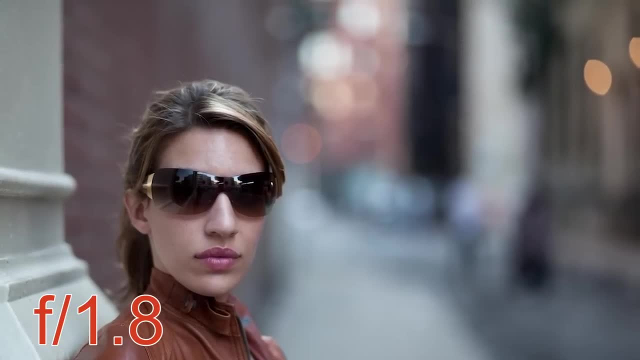 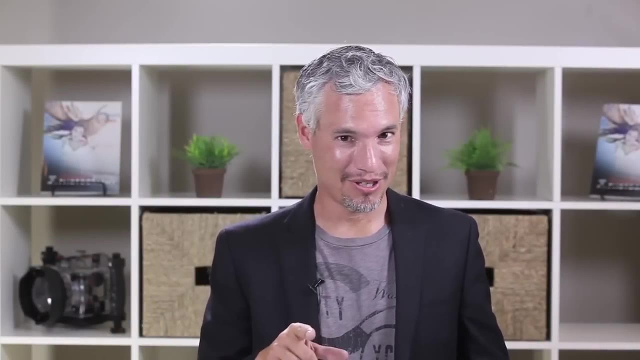 a powerful compositional element. there's nothing competing with the subject. when you have the background blurred like that now in aperture priority mode, you can see that the background starts to come into focus. you can make out the vague shape of a person there and the lines of 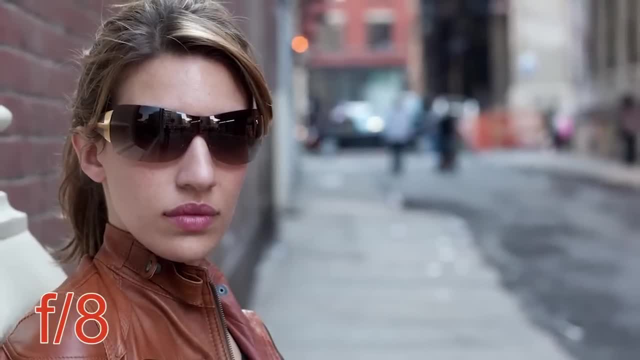 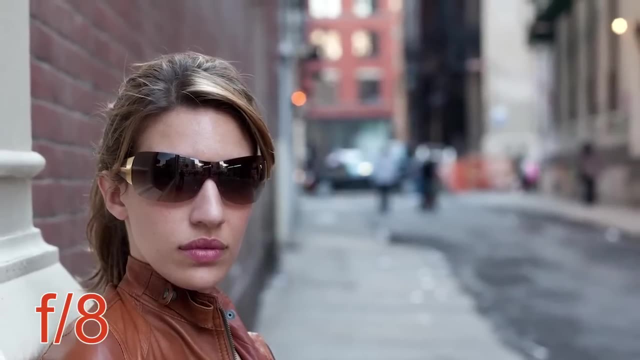 the brick start to become more distinct. so let's raise that f-stop number even higher by moving that main dial in aperture priority mode here. at f22 you can distinctly see a car in the background and even the distant buildings are in focus. so if you're shooting a picture of a car in the background, 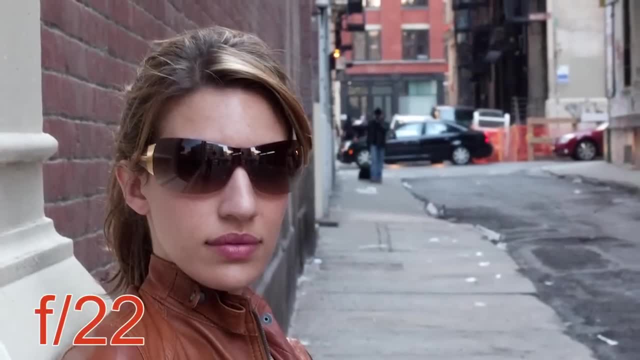 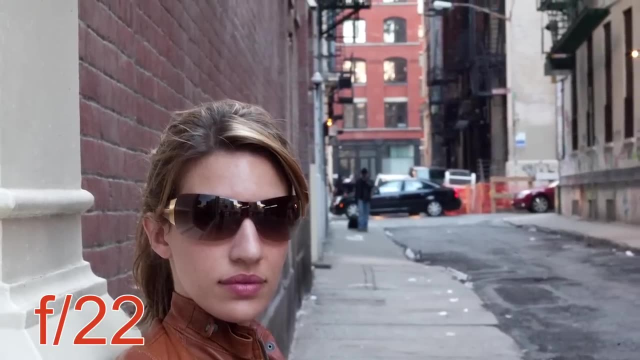 you can see that the background is starting to come into focus and you can see that the background is starting to become more distinct. so let's raise that f-stop number even higher. as you can see, the higher the f-stop number, the higher the background sharpness. i'm saying that. 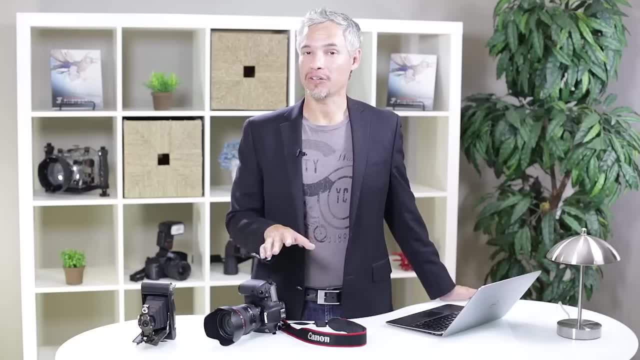 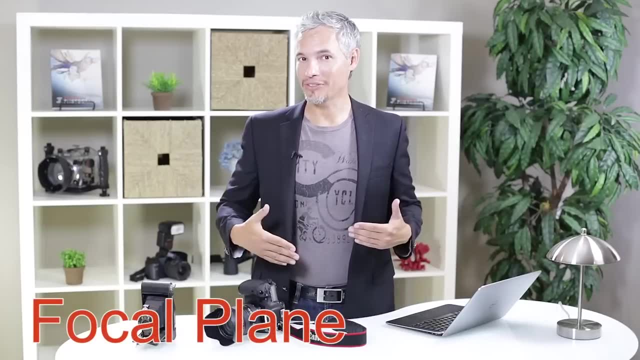 over and over again, because i really want to make that clear now. here's a technical note about how depth of field works. whenever you focus on something, there's a focal plane that is parallel to the camera sensor, perpendicular to the camera's lens. basically, what that means is: 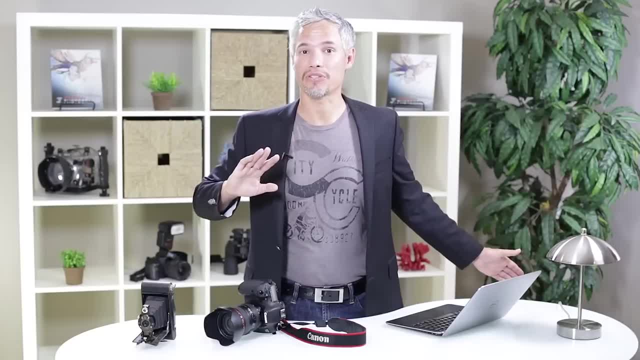 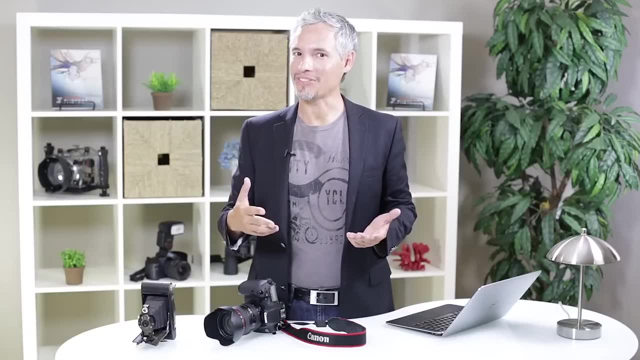 everything side to side and up and down from where you focused, is going to be perfectly in focus, and everything that's in front of or behind the subject is going to be a little out of focus. now, if you're really being precise about what gets into focus, you'll want to 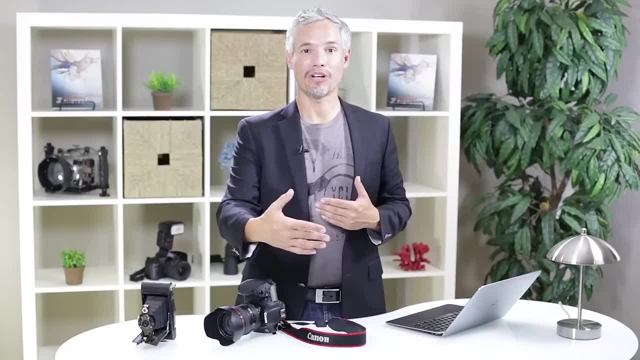 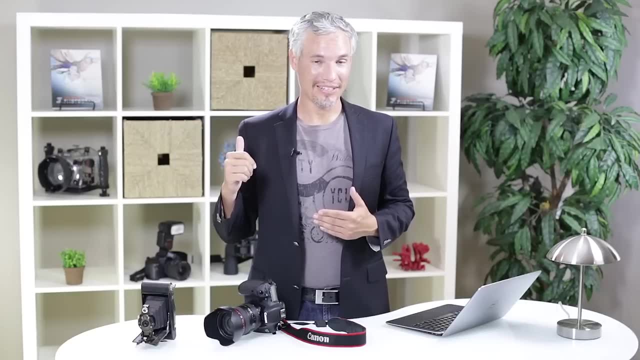 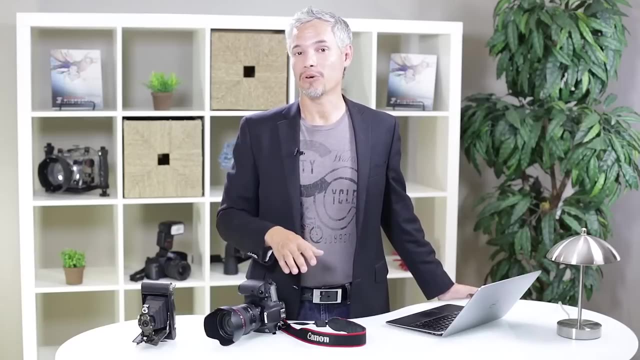 understand that you actually have shorter depth of field in front of your subject and longer depth of field behind your subject. in fact, you have about two-thirds of your depth of field behind the subject. this becomes important when you're trying to get multiple people, for example, in focus in a 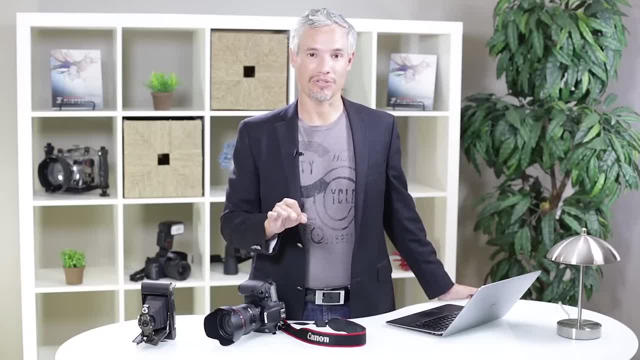 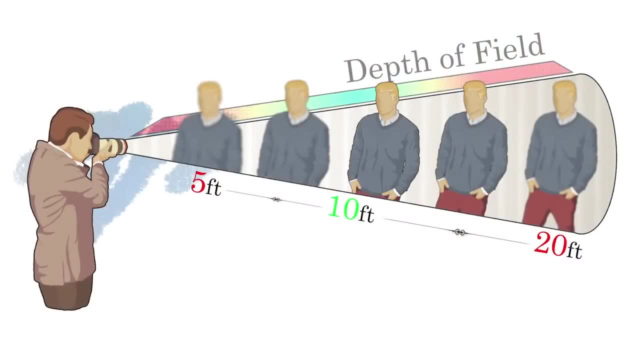 shot. if you're taking a group photo, this is going to be really important to understand. you basically want to focus on the subject and you're going to want to focus on the subject and you're going to want to focus about one-third of the way through the frame. so let's take a look at a diagram to 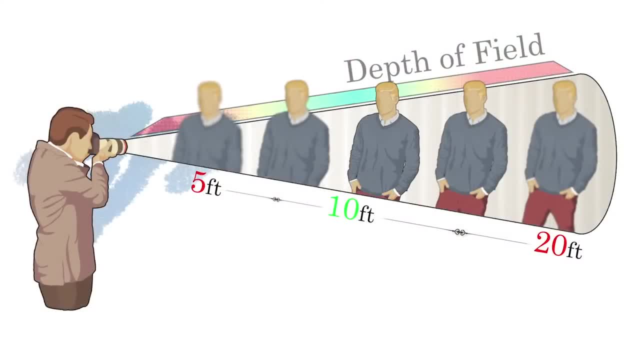 demonstrate depth of field. as we look at this diagram, we can see that if we're focused on this individual, the depth of field might cover a span from about five feet from the camera to 20 feet from the camera. about five feet of that would be in front of the person and about 10 feet of that 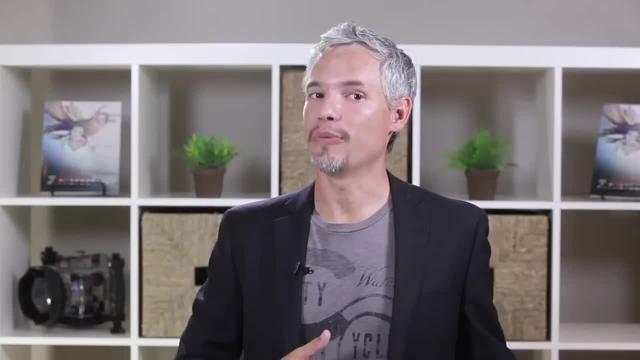 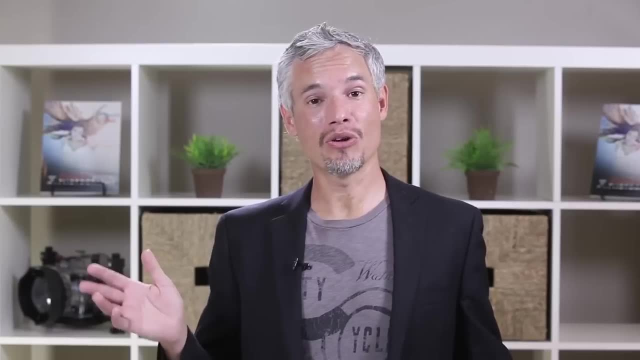 would be behind them. so, basically, wherever you focus is going to be about a third of the way through the total depth of field. now, if this all isn't making sense, don't worry about it. if you're focusing on a specific subject, you can just take a picture, and if you want more stuff to be in focus, 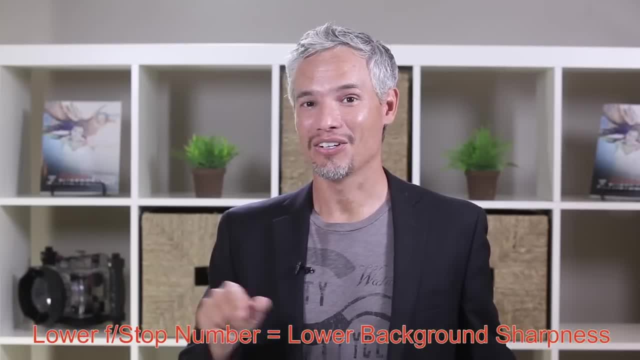 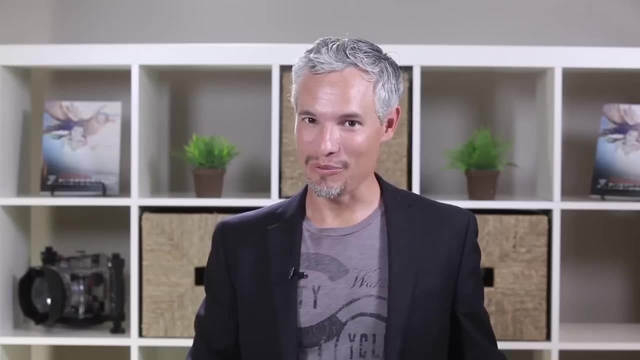 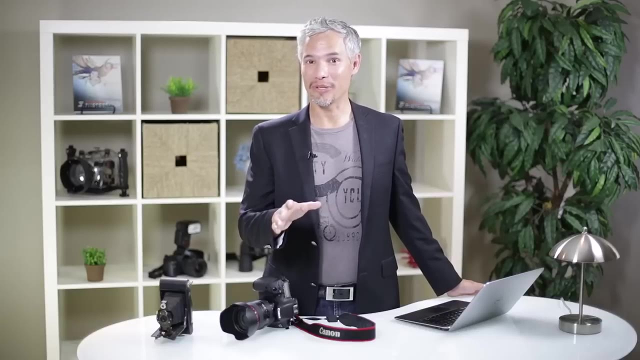 increase your f-stop number. if you want more background blur, decrease your f-stop number. now let's go through a live demonstration using my video cameras and we'll see how the different f-stop numbers make the video camera respond. right now we're filming with a 35 millimeter dslr. it's a. 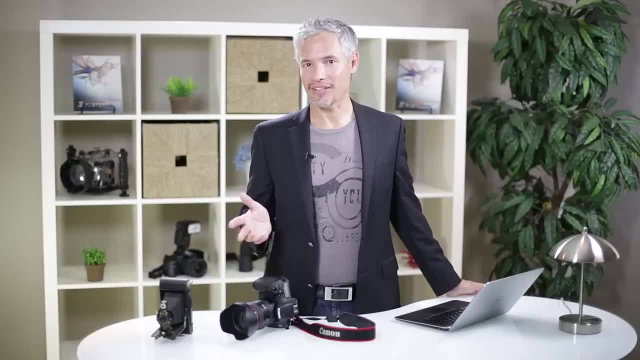 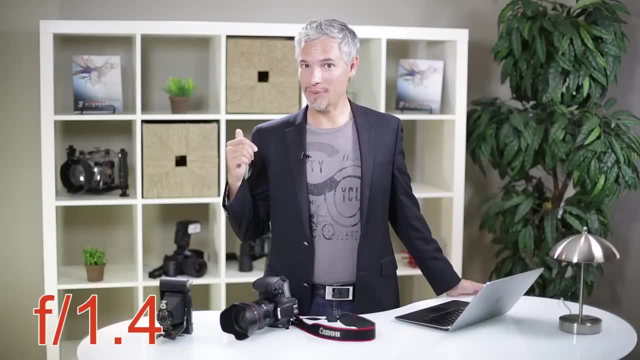 canon 5d, but any full frame dslr would behave exactly the same way. i have a 50 millimeter lens set at f1.4 and, as you can see, I'm nice and sharp. but that bookcase behind me is a little bit. 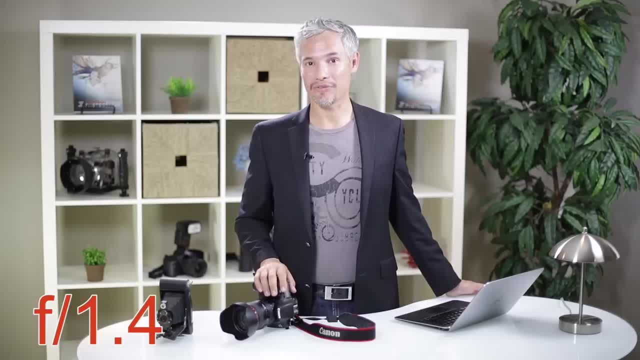 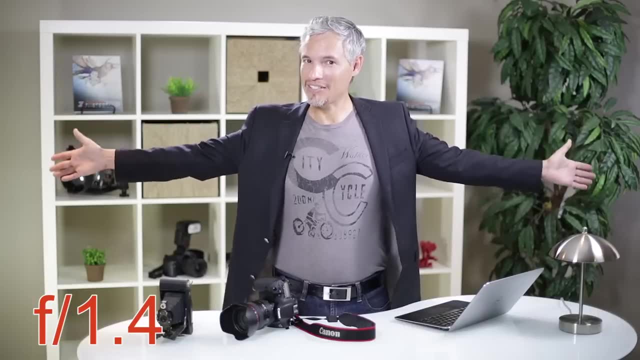 blurred. that's because f1.4 is a really low f-stop number. that means low background sharpness. you also notice, if I hold my hands out directly to the side, they'll stay nice and sharp too, because this is about what the focal plane looks like. as long as I'm facing the camera directly my whole. 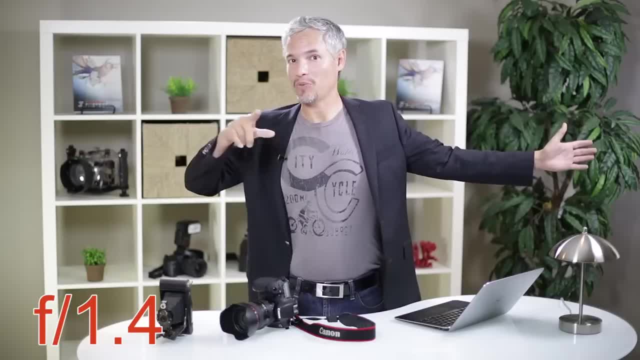 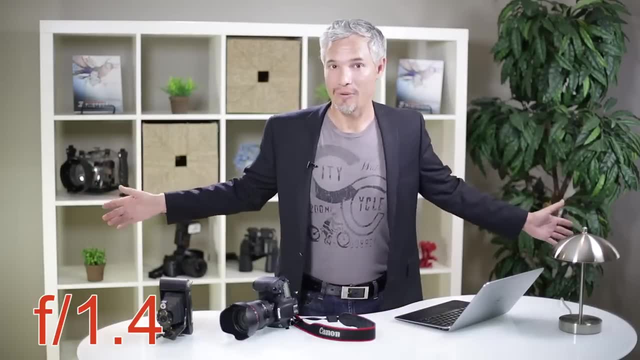 body up and down and my arms side to side will be in focus. but watch, as I step back, I'll become blurrier and blurrier because I'm moving out of the focal plane. the same thing happens as I lean forward. now the entire depth of field here, as I mentioned, is going to be about one third in front. 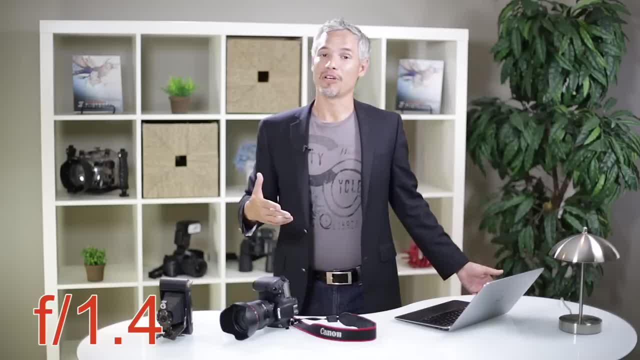 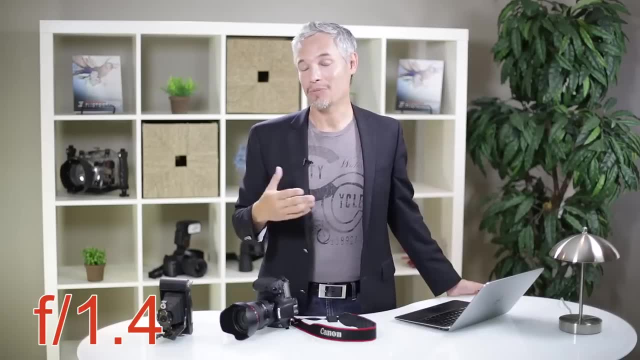 of me and about two thirds behind me. depth of field is never a perfect thing. if you move back just a little bit, you're always going to be a little bit less sharp. depth of field is just kind of a general term that means sharp enough. now let's have our cameraman Tyler adjust the. 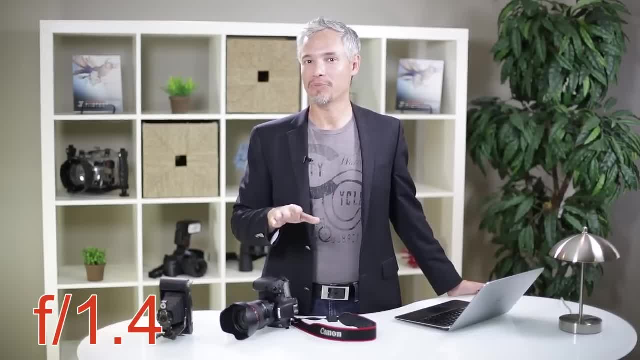 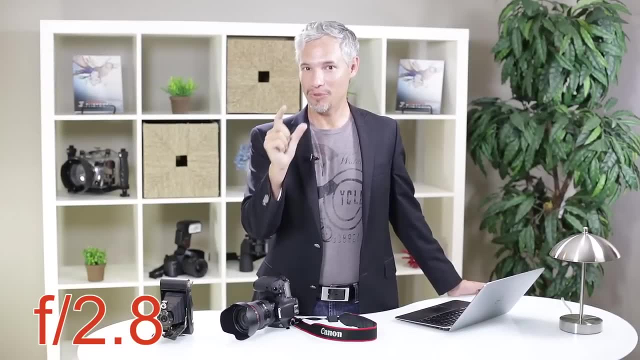 f-stop number to a higher f-stop number. so we're at f1.4. now let's go up to f2.8 and as we can do that, the aperture is getting smaller and smaller. higher f-stop numbers, smaller physical opening, remember, and the bookcase behind me is: 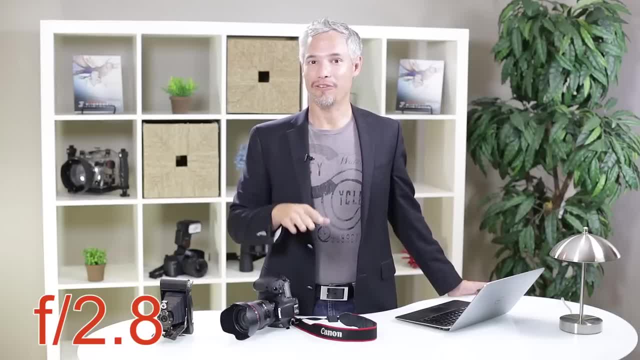 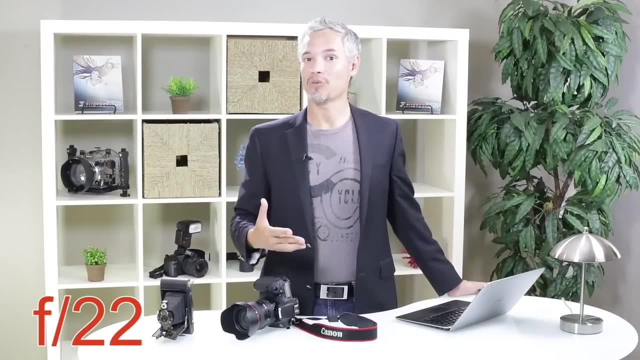 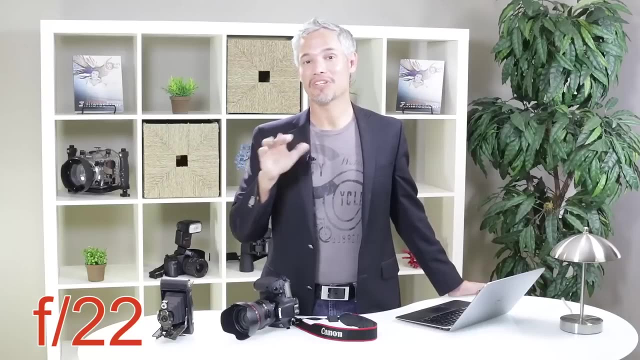 becoming a little more in focus. so let's crank it all the way up to f22. on this particular lens, f22 is the maximum f-stop number, which means this is going to give us the greatest depth of field that we can. and, as you can see, that bookcase behind me got quite a bit sharper, so I'm 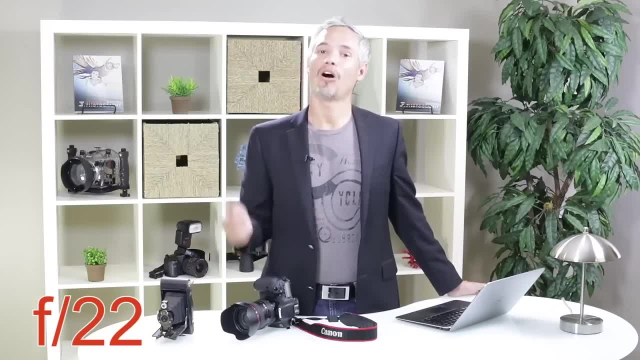 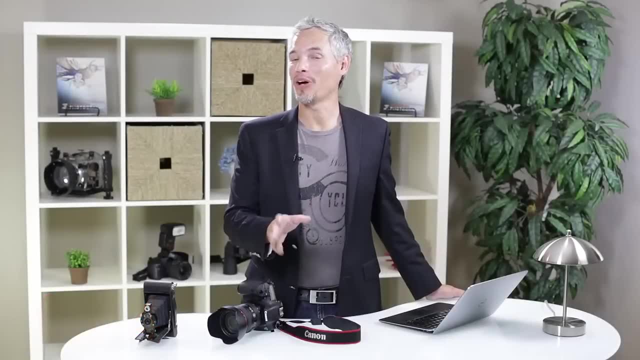 just going to ask Tyler to adjust the f-stop number one more time, this time all the way back down to 1.4, so we can see that bookshelf behind me go back out of focus. aperture is just one way to control depth of field. now it's definitely the easiest way because you can change the depth of. 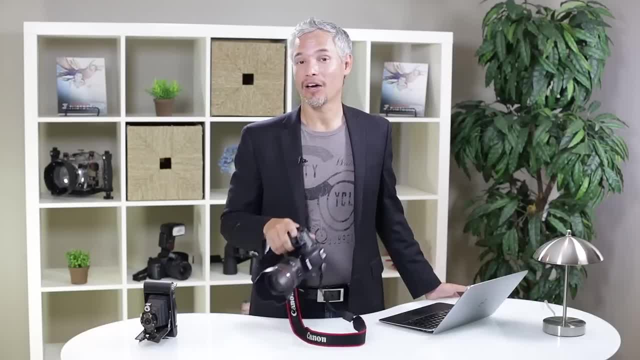 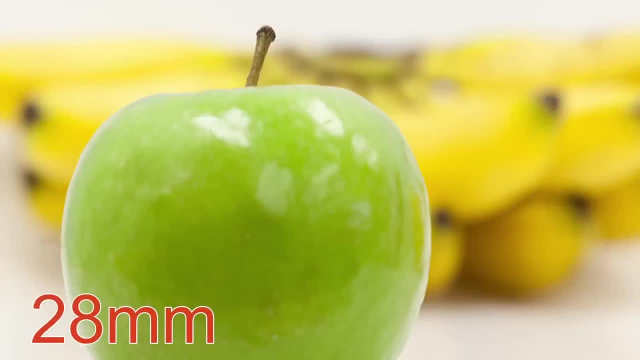 field just by flicking your finger in aperture priority mode. but the other ways you can control depth of field include changing your distance to the subject. so let's look at some sample pictures. breaking out the fruit again for this, here's an apple and a bunch of bananas. obviously, I've 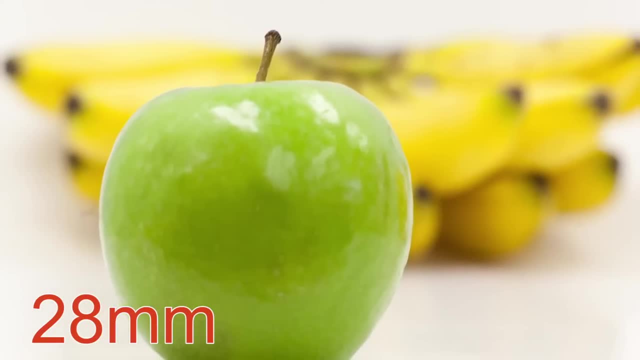 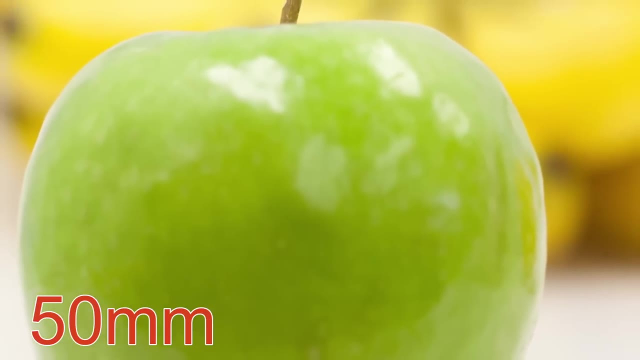 been focusing on the apple. now, without changing the aperture or the focal length or any other part of the camera settings, I'm going to move the camera closer to the apple. as we can see here, the bananas went from being fairly sharp to being more blurry. now I'm going to step even closer. 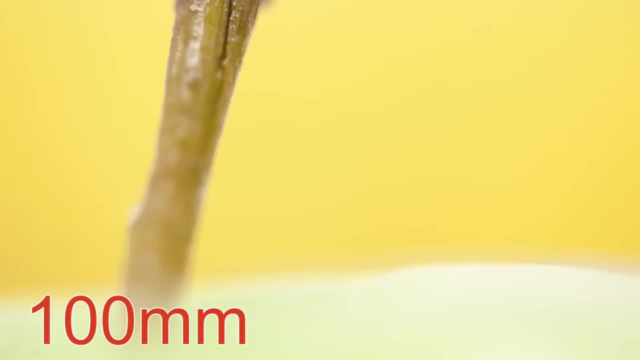 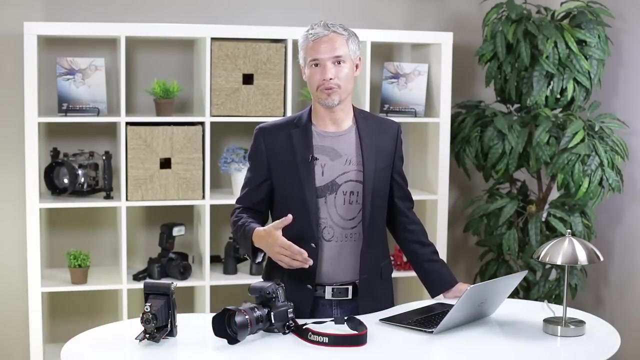 oh, that's really close and, as you can see here, the bananas are a complete blur and you can barely see just one part of the stem is in focus. that's really shallow depth of field and, even though I didn't change the aperture closer, caused the background to be much, much blurrier. this gets to be a real issue with. 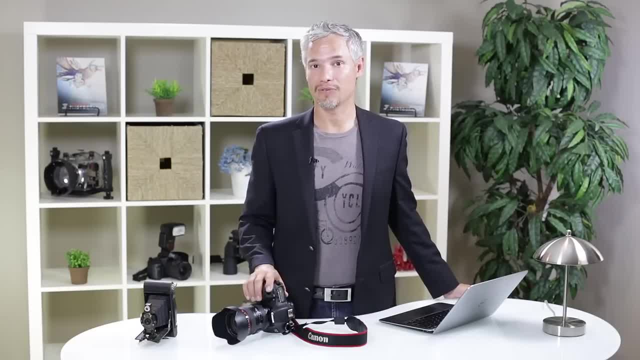 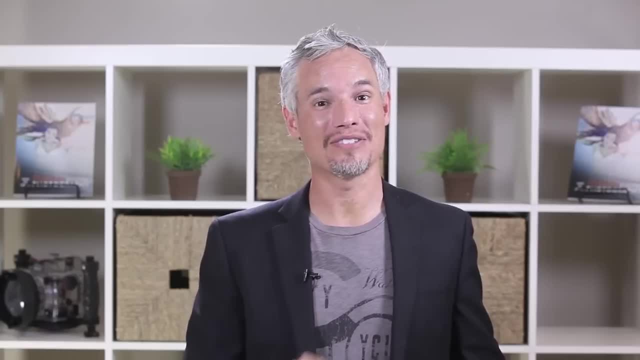 macro photography, which is close-up photography. that's covered in a different video lesson, but let's take a look at a macro shot of a teeny, tiny jumping spider, so we can get an idea of the kinds of depth of field that you have to deal with at these macro levels, as you can see this tiny little. 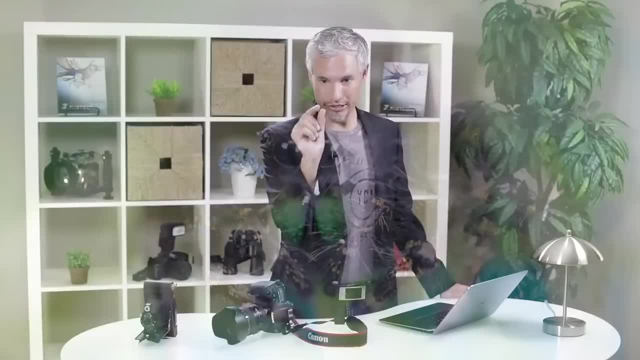 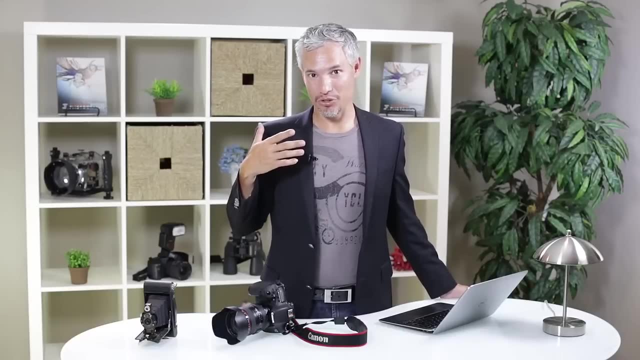 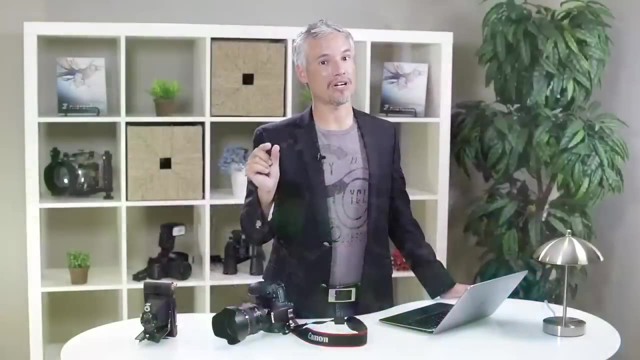 guy has his eyes sharpened in focus, but his body, which is like this far away from his eyes, is not this. if you're trying to do a portrait, you might get the guy's eyes in focus and his eyelashes would be blurry, but when you get really close to subjects, the depth of field gets shallower. 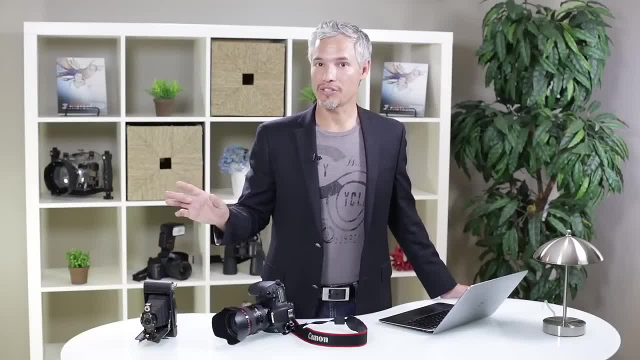 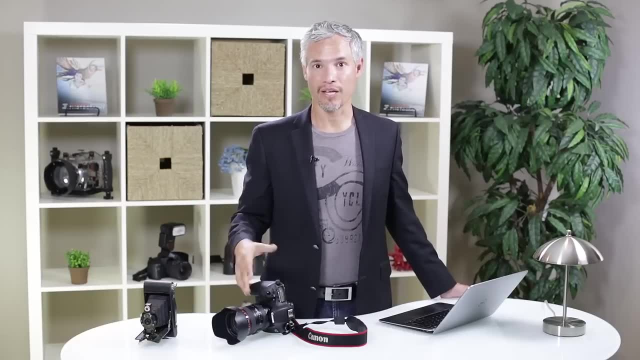 and shallower. if somebody's really far away, you can forget your chances of blurring the background behind them, because when something is far away, the depth of field gets longer and longer. so let's talk about another way to control depth of field, which is changing your focal length. 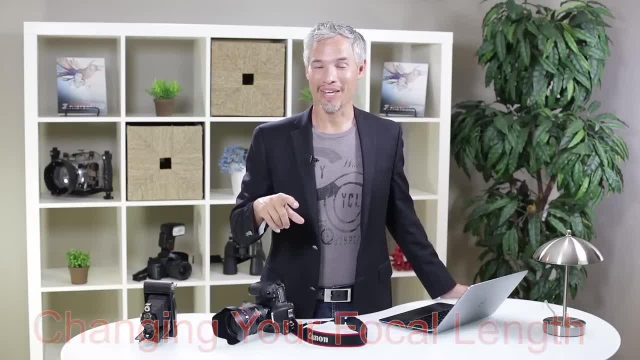 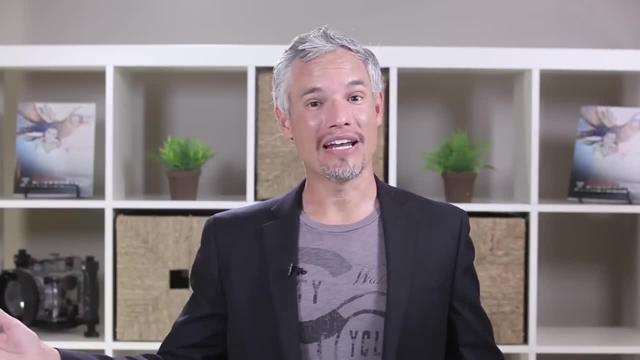 basically zooming from wide angle to telephoto. at wide angles, you have really long a depth of field, which is why you can take a landscape photo with your iPhone and have everything seem nice and sharp. with telephoto lenses, however, depth of field gets to be really. 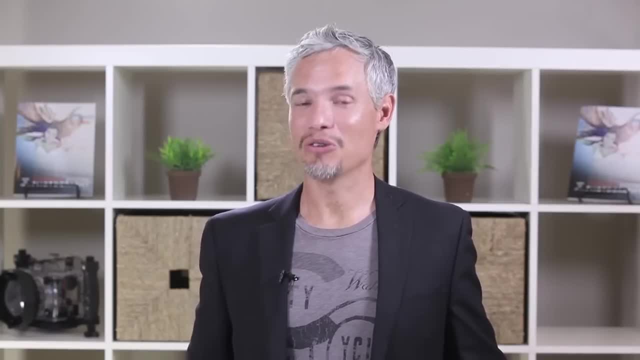 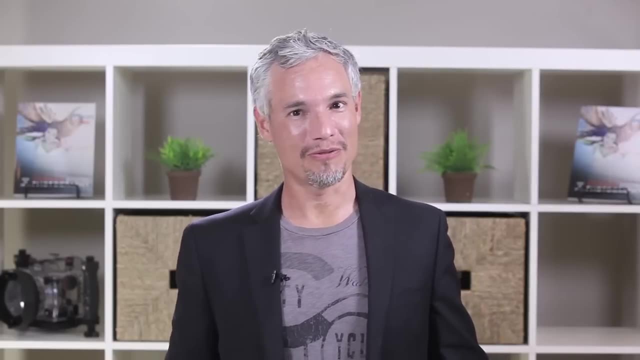 shallow, and that's part of the reason why, if you're taking a portrait of somebody and you want the background nice and blurred, you're going to use a telephoto lens. so let's take a look at some more sample photos of fruit. here we go. here's my Apple, orange and banana. once again, this is at. 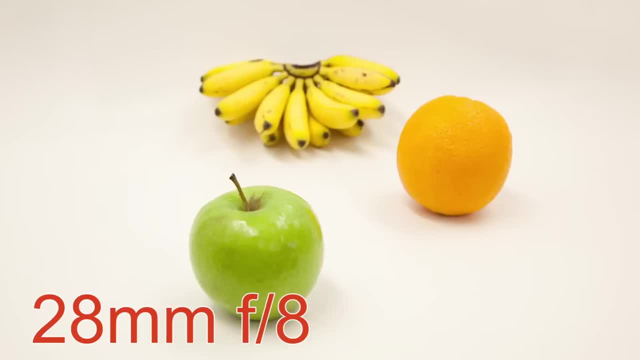 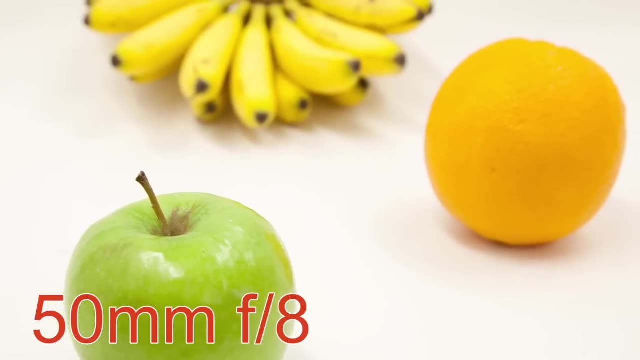 28 millimeters and f8 and, as you can see, they all look nice and sharp, but in fact I'm focused on the Apple. now I've zoomed in from 28 millimeters to 50 millimeters and we can see the bananas start to get a little blurrier. I didn't 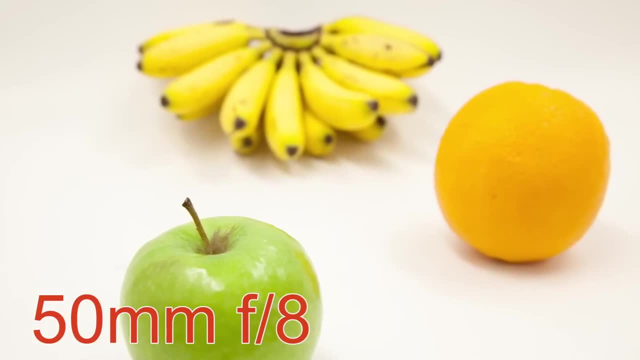 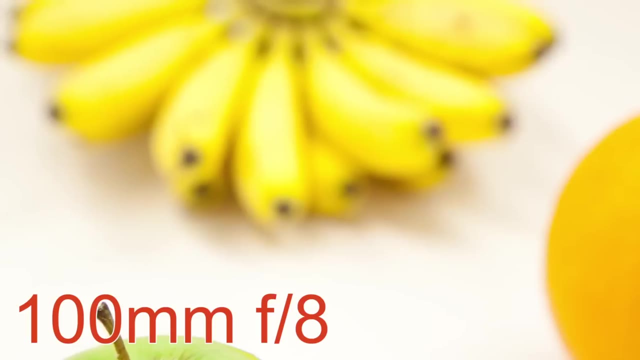 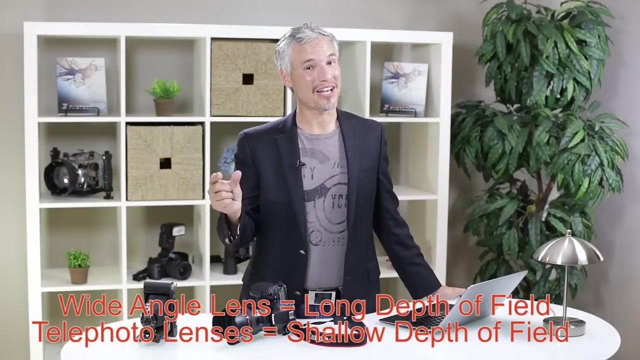 move the camera or change the aperture at all, it's still at f8. let's zoom in even closer here at 100 millimeters. the Apple still sharp, the bananas are now quite blurry and the orange itself is blurry too. wide angles, long depth of field, telephoto lenses: really shallow depth of field. 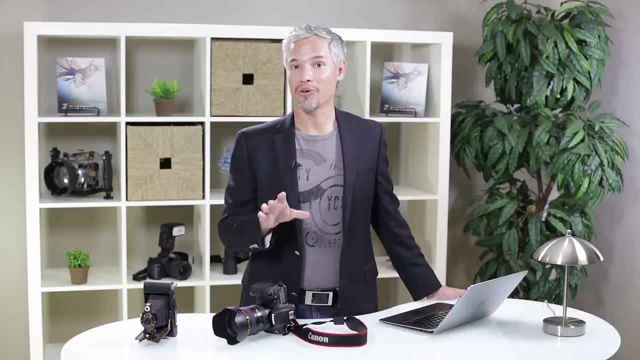 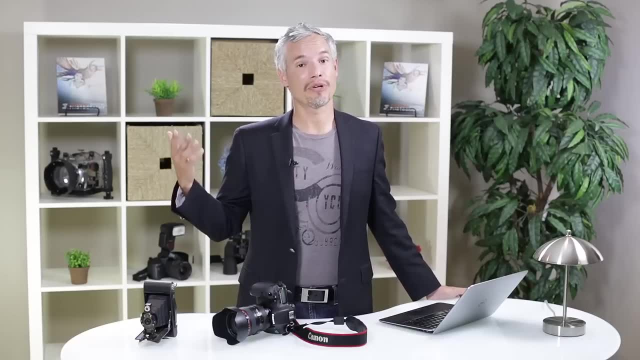 and blurry backgrounds. you can use both to your advantage and you'll find that both will become a challenge in different conditions. you can't use a wide angle lens and take a portrait of somebody and blur the background nicely. you just can't. and if you're using a telephoto lens and you 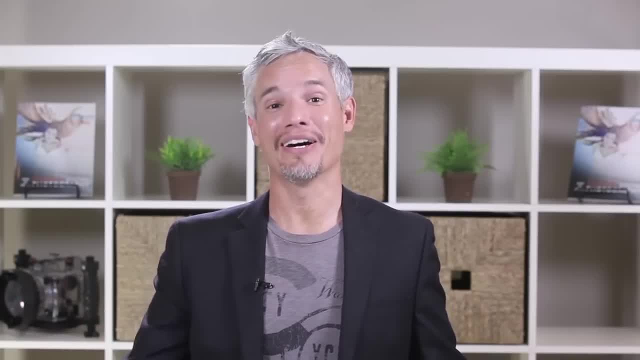 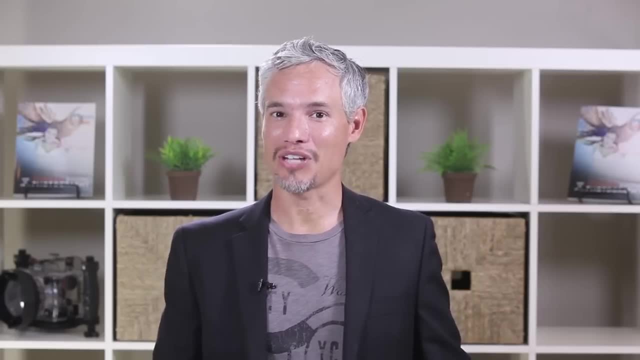 want something in the foreground, sharp and something in the background, sharp. forget about it, you won't be able to do it. let's take a look at a bird picture taken at 500 millimeters so we can get an idea for just how shallow this depth of field is. this house Finch is just a couple. 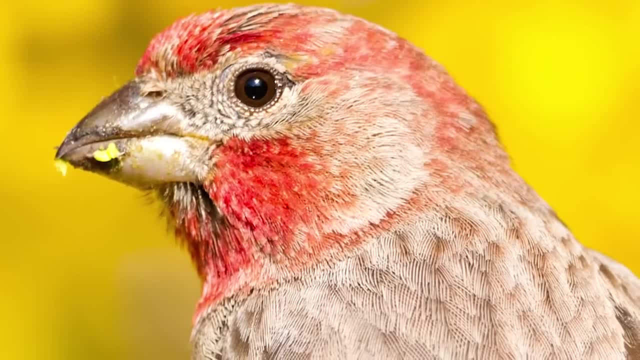 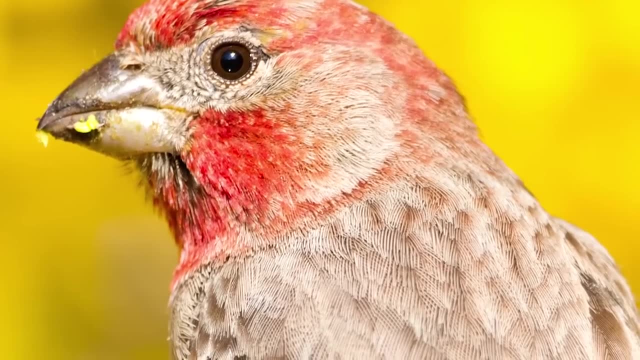 of feet in front of the yellow flowers behind them. but you can see, while his eye is nice and sharp, the background is completely blurred and in fact, if you look closely at the feathers in the foreground there, they're a little bit blurry too, even though the bird is pretty tiny, you can. 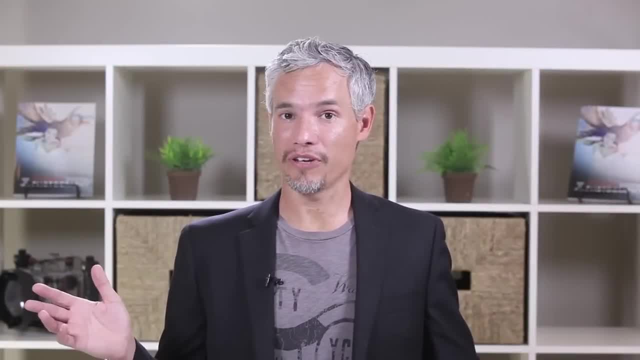 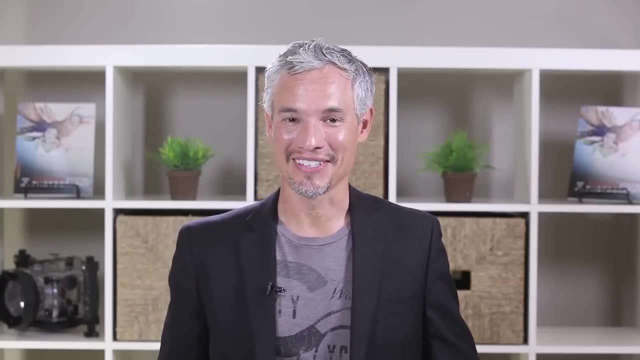 get his eyes nice and sharp and the tail of the bird- the feet of the bird- will be completely out of focus. that's because the depth of field is so shallow that you can't even get a little bird completely in focus. now let's look at a wide angle vacation shot that I took. 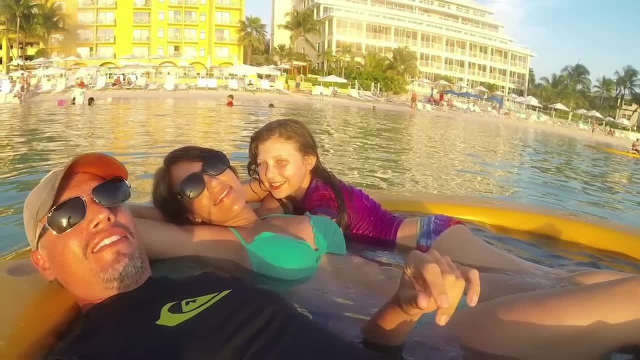 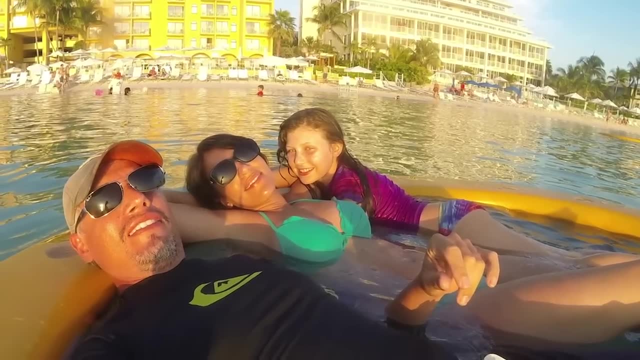 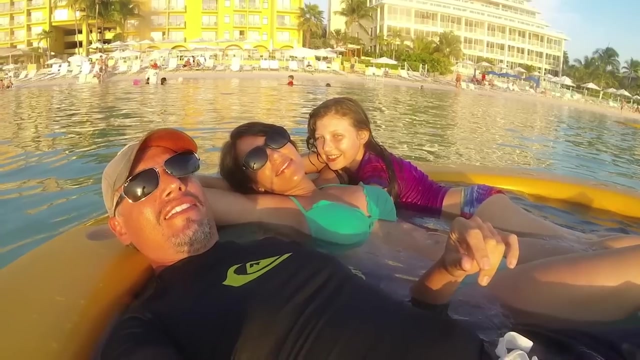 yes, it's just a selfie taken with a GoPro camera, but it's at the 35 millimeter equivalent of 15 millimeters, and at f28. the bird picture was taken at f45 but at 500 millimeters and because of that, the depth of field was just a fraction of an inch. this wide angle lens at 15 millimeters. 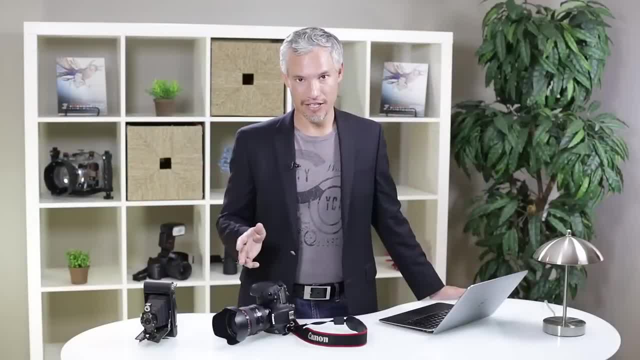 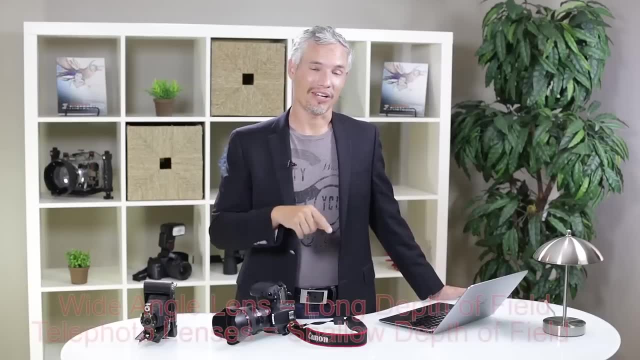 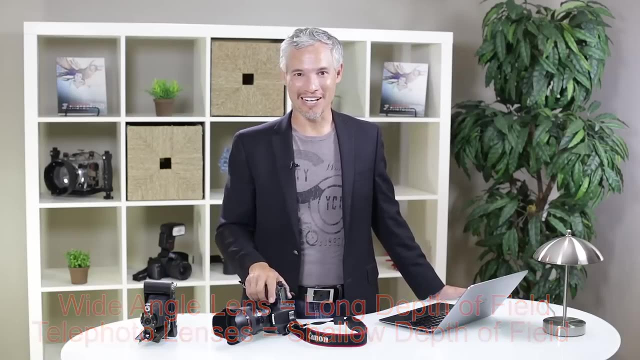 even though it has a lower f-stop number, it seems to have infinite depth of field, going all the way from the people in the foreground to the buildings far, far in the back. remember wide angle lenses, plenty of depth of field, you'll get everything in focus. telephoto lenses: you're going to blur that background, whether you like it or not. another: 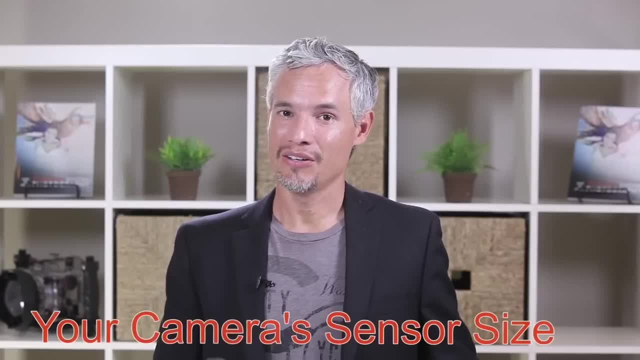 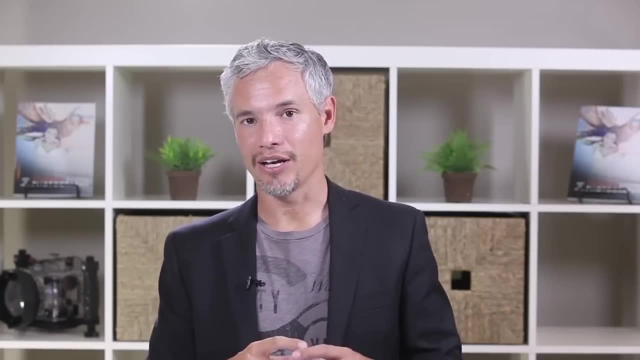 way that you can control depth of field is with your sensor size. small sensors have a really large depth of field and make everything seem to be in focus, whereas the large sensors that you find on expensive professional full frame cameras give you a very shallow depth of field. that's why 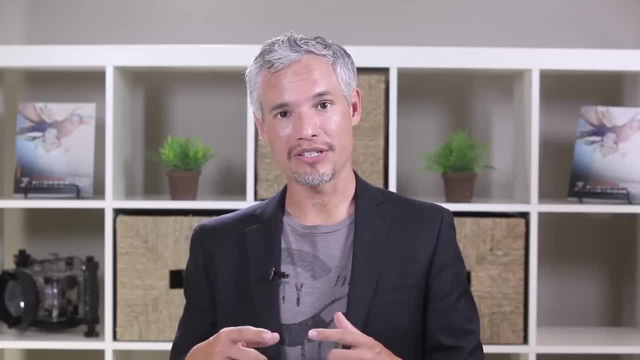 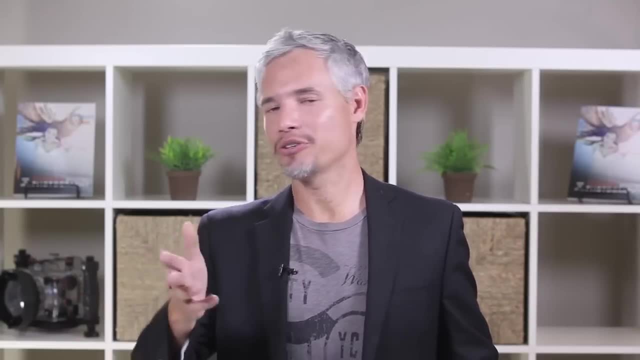 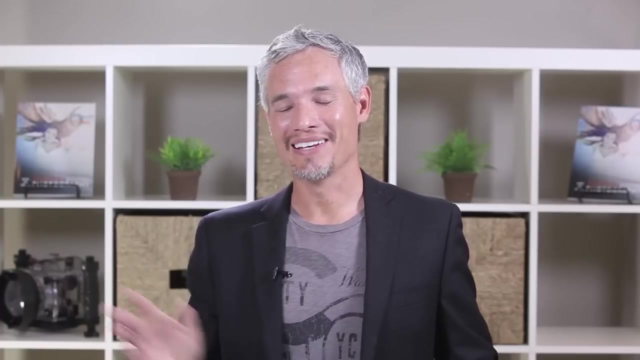 professional movie makers tend to use cameras with really large sensors because they want to be able to throw that background out of focus whenever they want. that's also why, with your iPhone or smartphone or your GoPro camera, those all have really tiny sensors and that's why it seems like everything's in focus all the time. now, sometimes people move up. 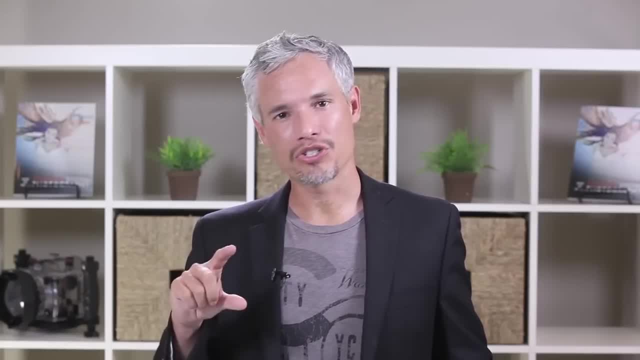 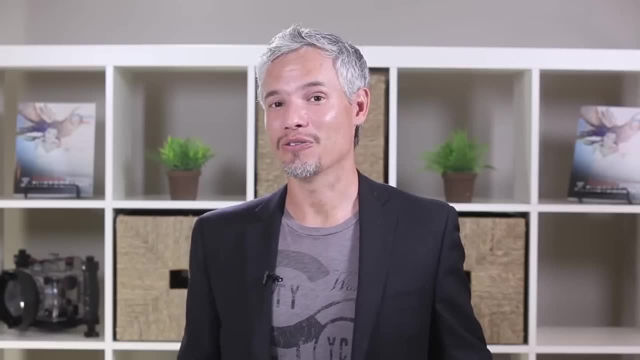 to a DSLR with a large sensor, from a small point and shoot camera or a mirrorless camera or just their camera phone and they're baffled about why stuff is out of focus. well, you know what your phone was, getting things out of focus too, but because that small sensor is out of focus, it's. 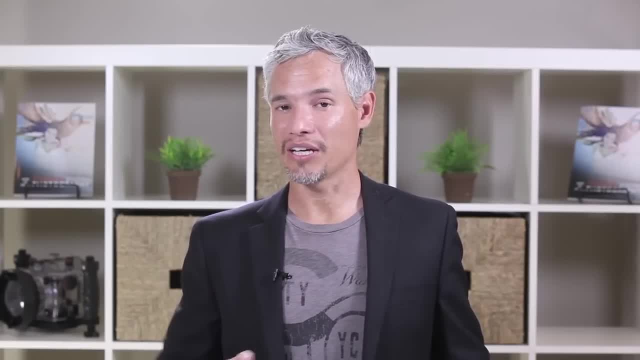 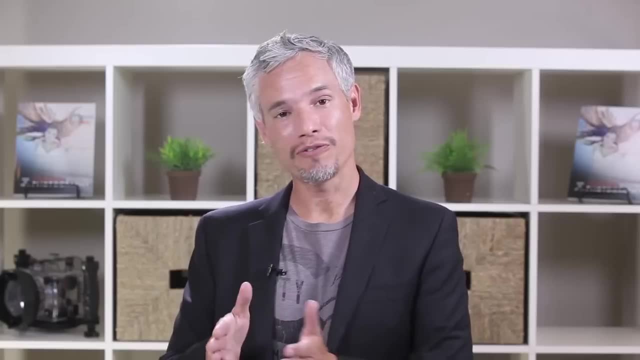 not going to be out of focus for a long period of time. it's going to be out of focus for a long time and that's why it's important to have a large sensor and wide angle lens combined to provide a really large depth of field. it seemed like everything was in focus, but remember realistically. 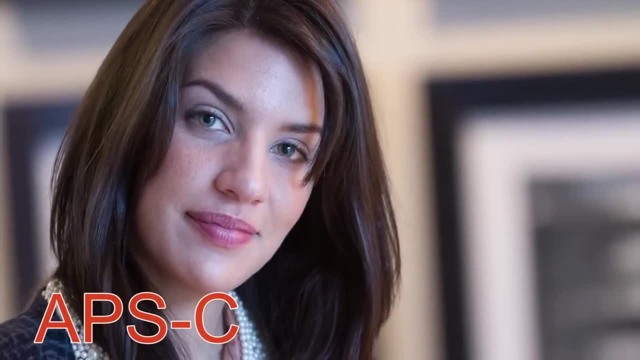 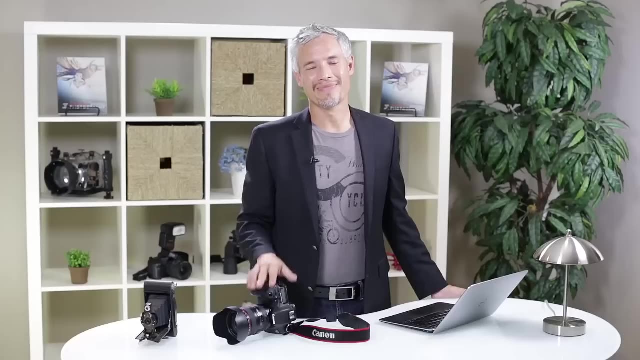 you only focus on a plane, so there's only ever a plane that's truly sharp. let's look at a couple of sample photos. this snapshot of chelsea in the living room was taken with a 200 millimeter lens at f28, but it was done on a compact dslr if you spent less than fifteen hundred dollars on your. 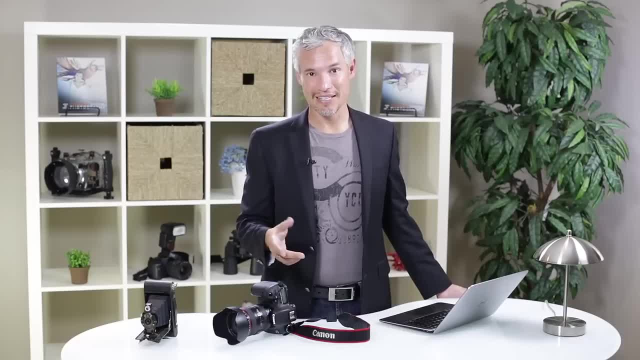 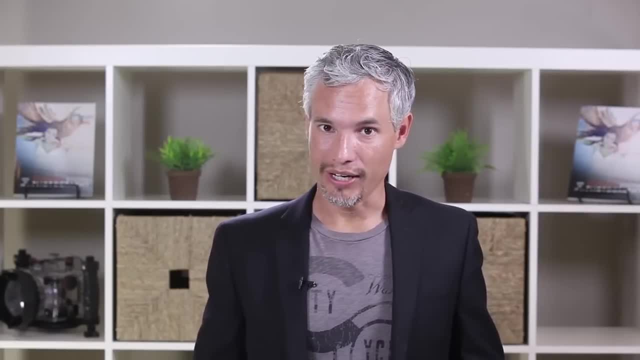 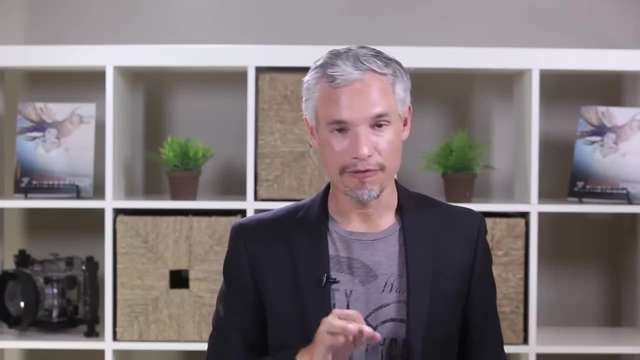 dslr. you'll see a compact dslr. sometimes they call them aps-c dslrs, and they just have a slightly smaller sensor. this means that you have a larger depth of field and the background won't be quite as blurred. now let's look at the same shot, taken from the same spot with the same lens, with a full 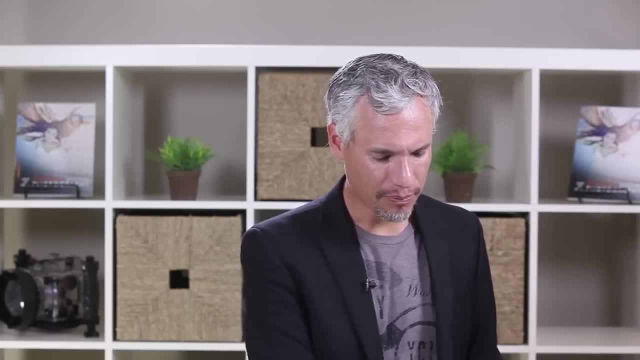 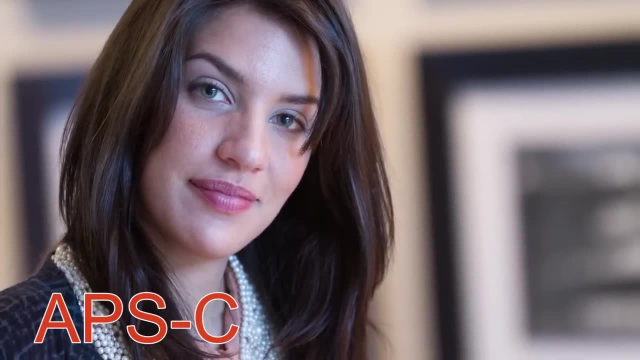 frame camera. but before we switch i want you to look at the picture in the background just off to the right of the frame and notice that you can kind of make out a shape. you can see some dark lines in there. but as i switch to this next picture you'll see that background photo go out of focus even more. 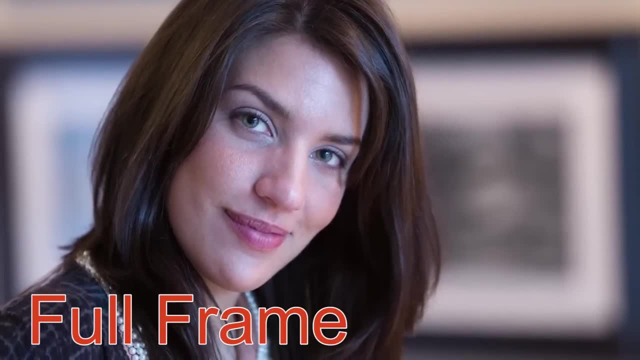 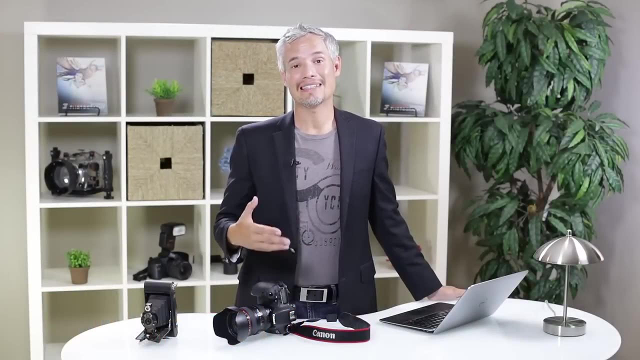 as you can see here, that went from being fairly distinct to being completely blurred. that's because i switched from a compact camera to a full frame camera, and full frame cameras offer about 60 percent shorter depth of field, for better or worse. if you're making portraits and you want to, 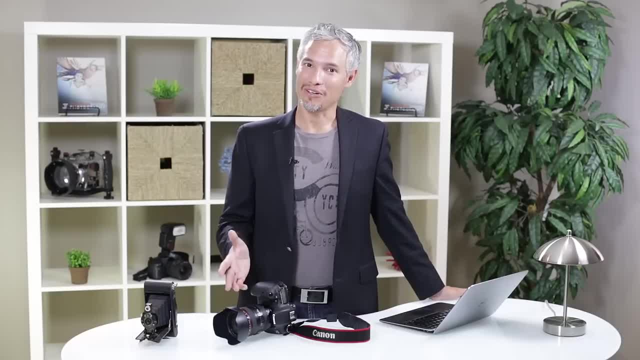 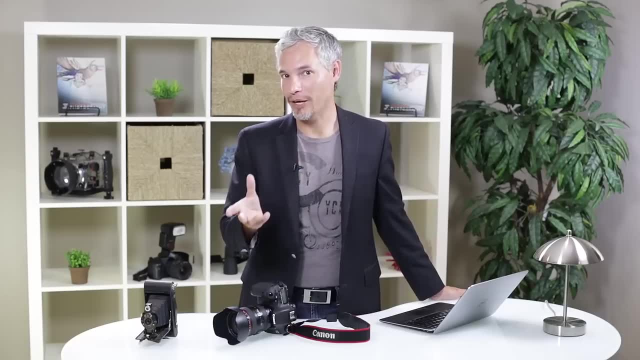 blur the background. that full frame camera might be a good investment for you but honestly, for most of us the smaller sensors on compact cameras are going to be a little bit more expensive than the larger cameras or the even smaller sensors on like micro four-thirds cameras. they're going to be fine. 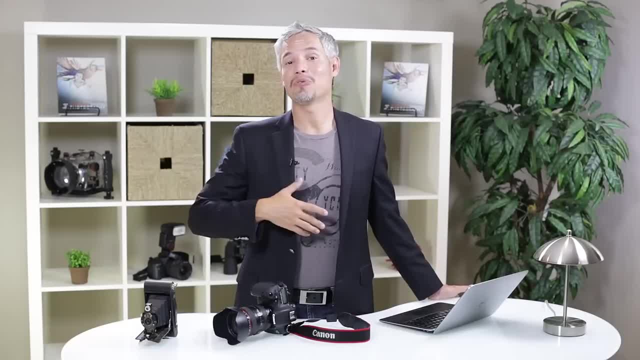 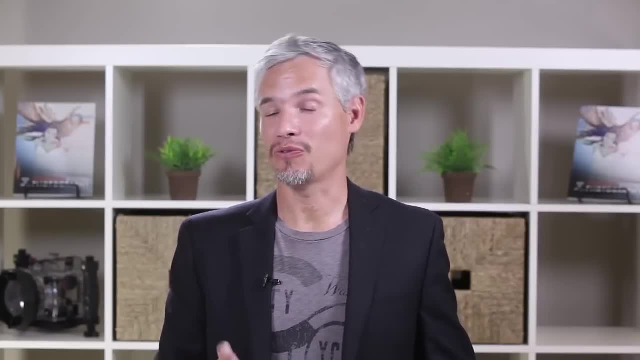 they're especially perfect for still lifes and landscapes and anytime you want everything to be in focus. but if you're into portraiture and you're always trying to blur the background, well, cameras with larger sensors, full frame cameras especially, will make blurring the background much easier. for 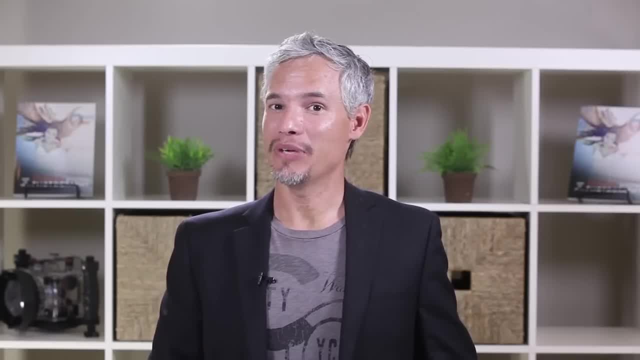 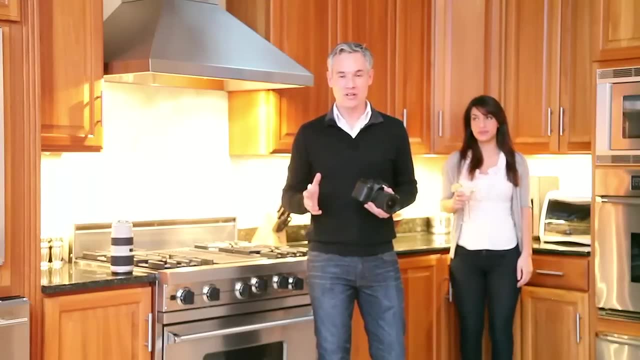 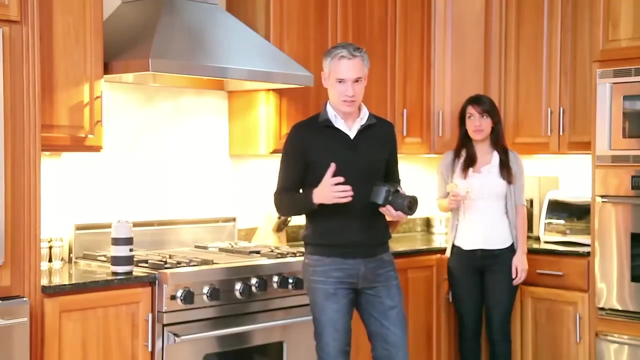 you. now let's go to a six minute video of me and chelsea demonstrating aperture and depth of field in our kitchen and living room. so here's a common scenario: you're at a party and you want to take a picture of somebody. what i always see people do is they take a picture of a person when they're standing right against the back. 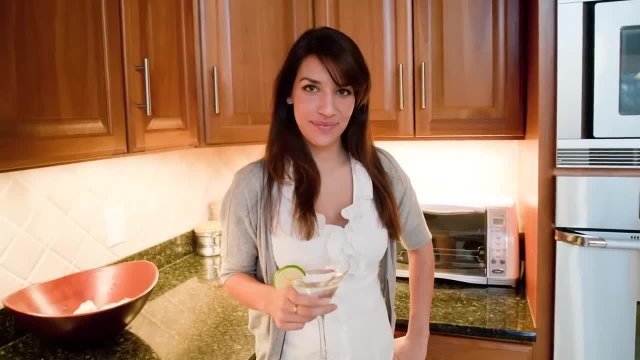 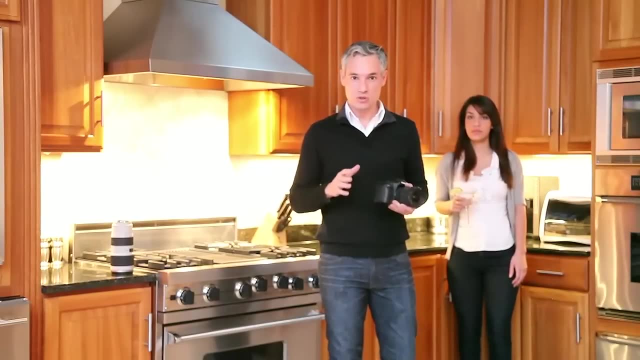 what happens then is the background is so prominent in the picture it distracts you from the subject person. there are a few really easy things you can do to fix that. the first is to zoom all the way in. i'm going to switch to a telephoto lens. you can do it with a lense or you can use a tape measure if you like. 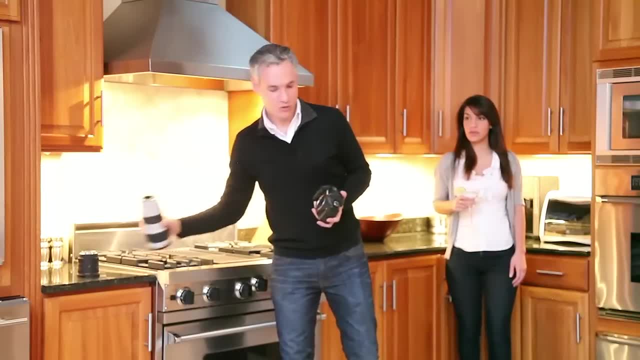 you can do it with a tape measure, if you like. you can do it with a tape measure, if you like. you can do it with a tape measure, if you like, with one lens, just by zooming out to the longest focal length that the lens supports. 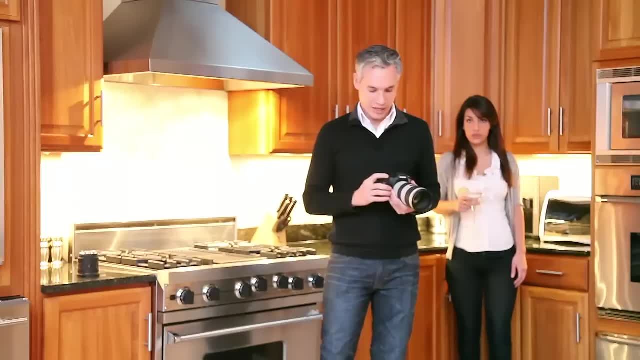 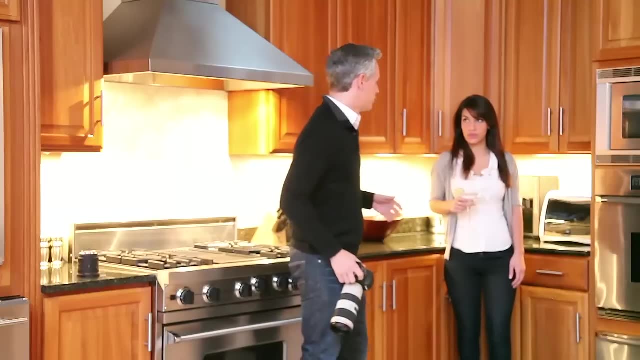 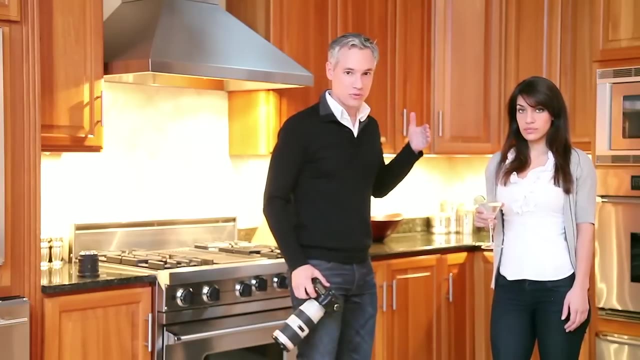 The next thing you can do is to switch to aperture priority mode and select your lens's lowest f-stop. Here's something easy: Just ask the person to step away from the background. So let's have Chelsea step a couple of feet forward. That gives some room behind her for the background blur to take effect and turn what's behind. 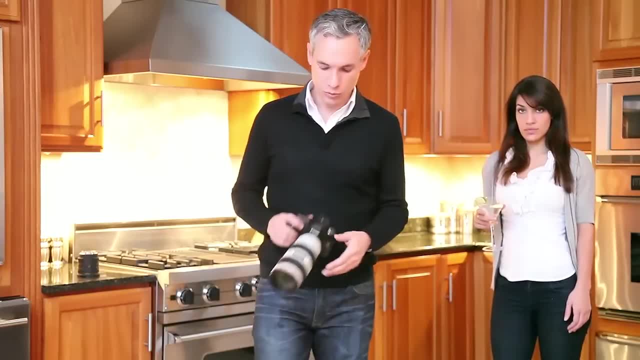 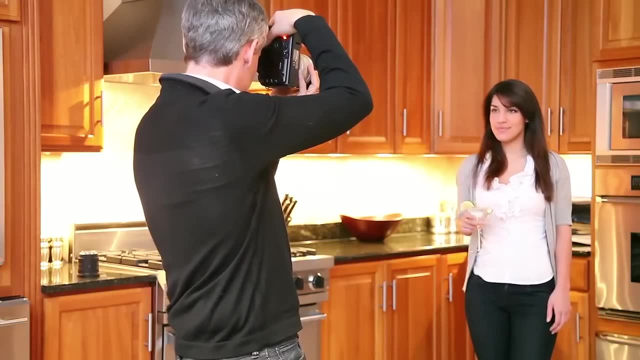 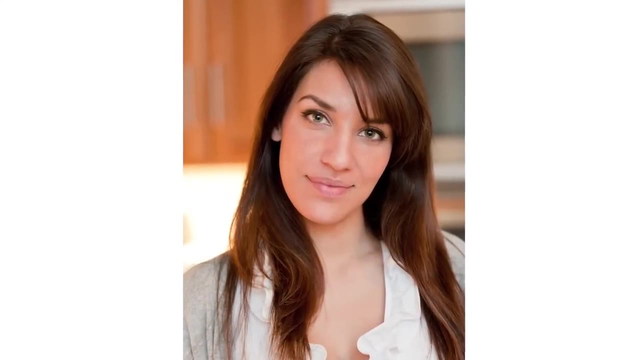 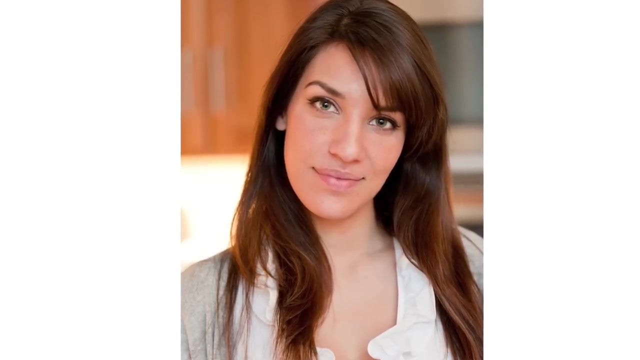 her into a nice blur. So I'll move into position and take a couple more shots. So, as you can see, those are much better portraits. The lighting and everything is the same, and I didn't even have to change the camera that much, but they turned out much better because they focused on the subject and the background. 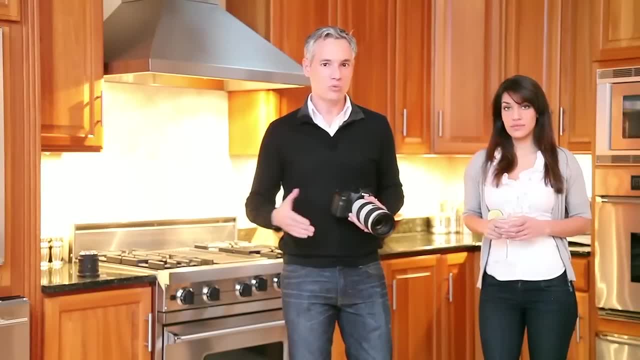 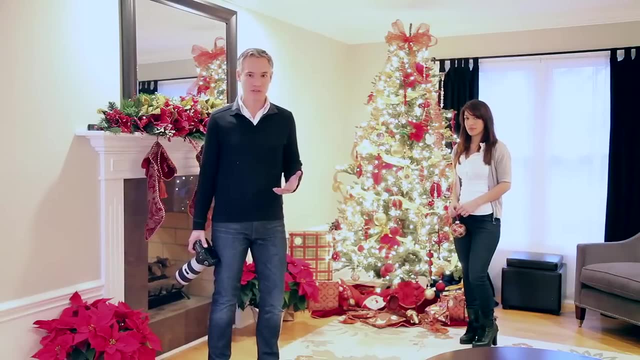 is blurred nicely. Now let's look at what you need to do. if you actually want the background to be in focus, Let's go into the living room. So this is one of those times when you might want as much depth of field as possible. 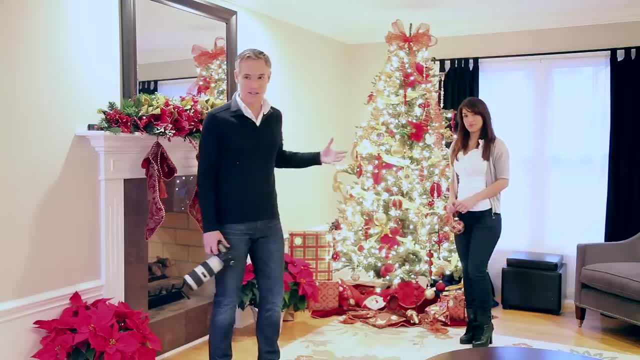 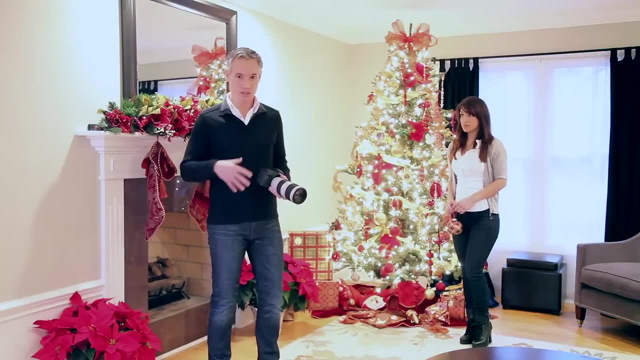 With a Christmas picture, you generally want both your subject and the Christmas tree in the background. So if I were to take a picture of her with the aperture- what they say wide open- wide open means using the lowest f-stop number- what we'll see is that it's actually pretty. 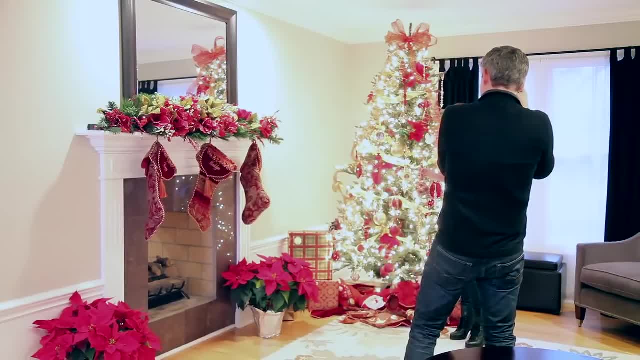 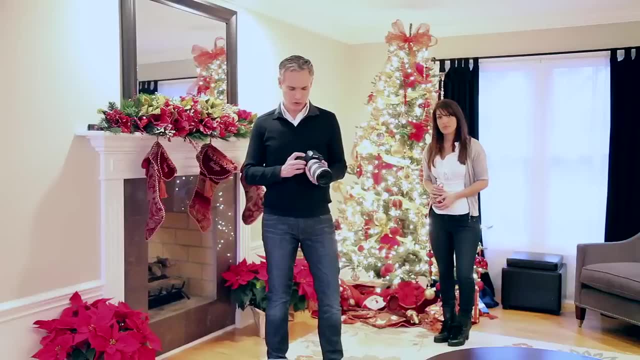 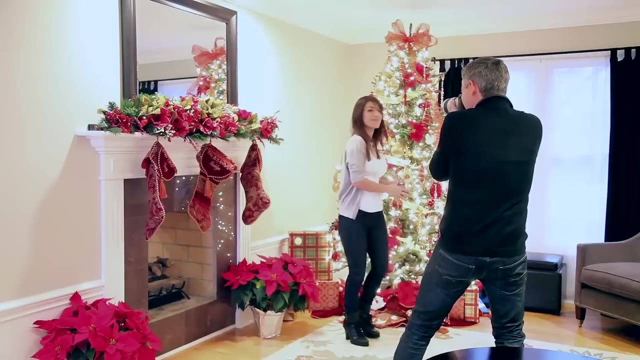 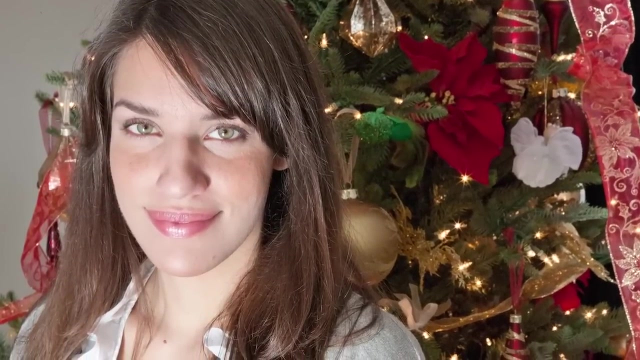 blurred out. I can fix that, though, by choosing a higher f-stop number. I'm in aperture priority mode, So I'll switch from f2.8 to f8 and take a couple more shots. As you can see, increasing the f-stop number increased the depth of field, increasing the 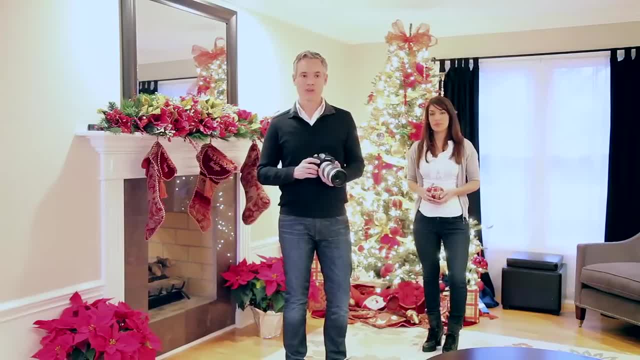 background sharpness, bringing everything into focus. There was a negative side effect, however, and you might have heard it. when the shutter clicked, The shutter speed increased. For every stop you increase your aperture, your shutter speed is going to double, And if it doubles too much, then it's going to be too slow for you to handhold the shot. 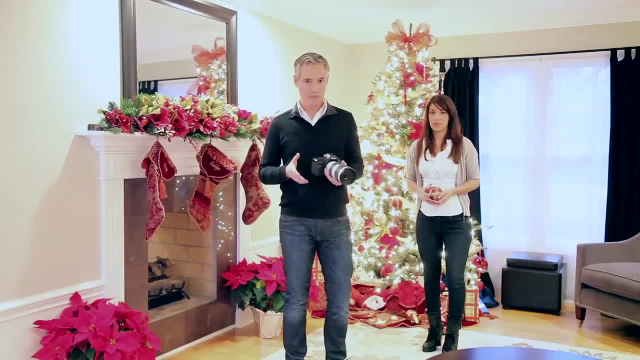 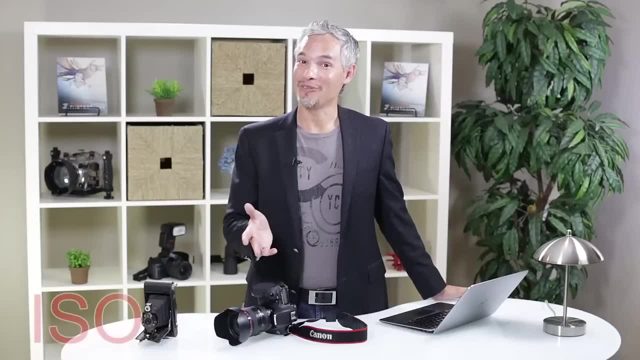 There are a few ways to fix that. You could put your camera on a tripod, You could increase the ISO and continue to handhold it, Or you could add flash. Now I'd like to talk about ISO, spelled I-S-O, but it's actually not an acronym. 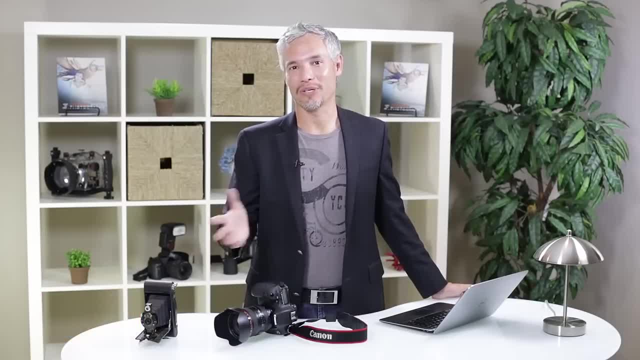 It's the name of an organization that refers to themselves as ISO, because they didn't want to use an acronym That would have been specific to one country. Anyway, ISO. previously, back in the old film days, some people knew it as A-S-A it. 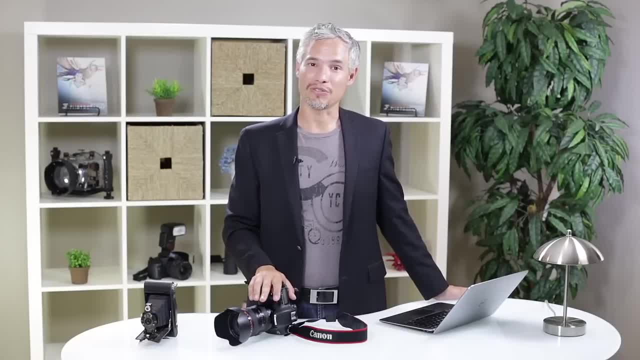 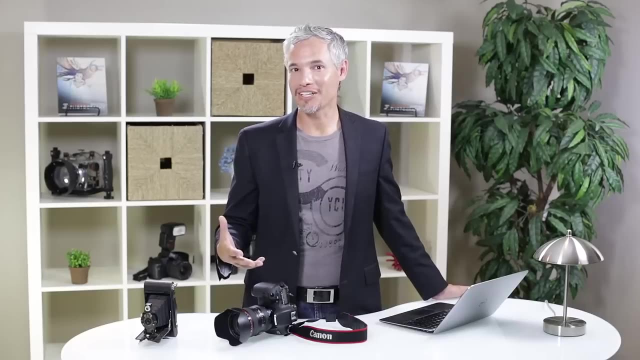 measures basically the sensitivity of your camera's sensor to light. Really it's more like a digital gain in an amplifier. That'll only make sense to my nerd friends. but the way ISO works is it doubles or quadruples the amount of light coming into your camera, effectively increasing the sensitivity to 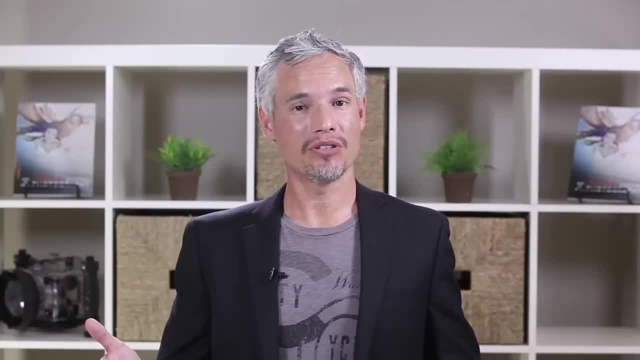 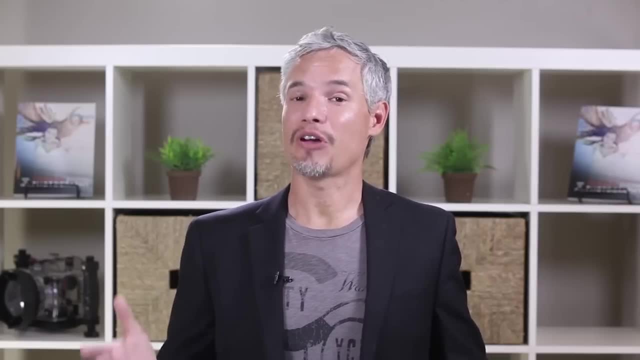 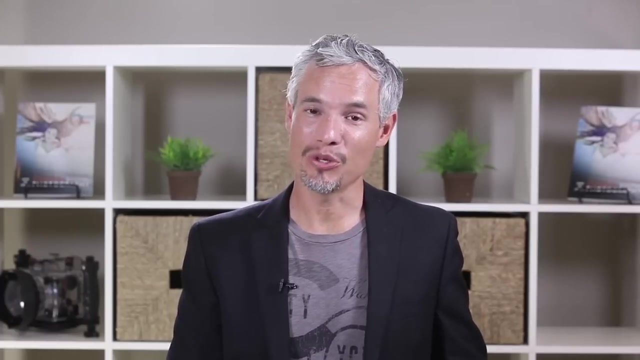 dim situations. ISO 100 is the lowest ISO Most cameras support And that's also the lowest sensitivity, meaning you need the most light. If you're out in bright sunlight, you should definitely use ISO 100.. ISO 100 gives you the best image quality always. 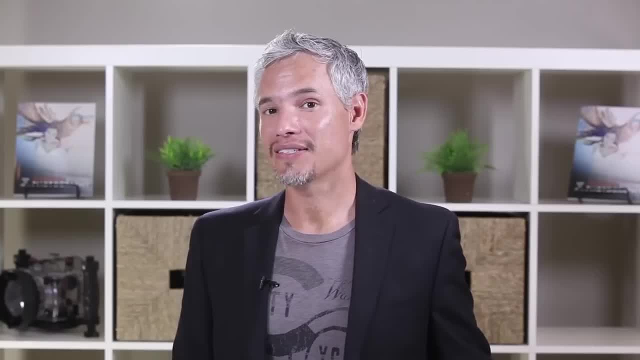 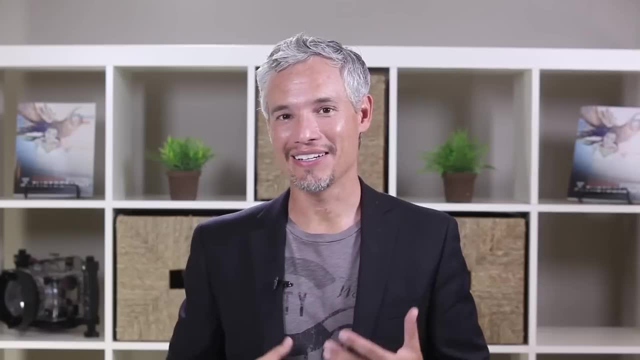 So whenever I can, I use ISO 100. But because it's not that sensitive, you might need to use either a big aperture or a slower shutter speed to make sure that your camera gets all the light it needs. Don't worry, it's not that hard. 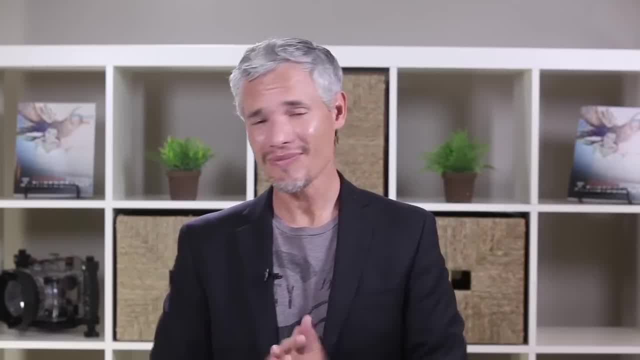 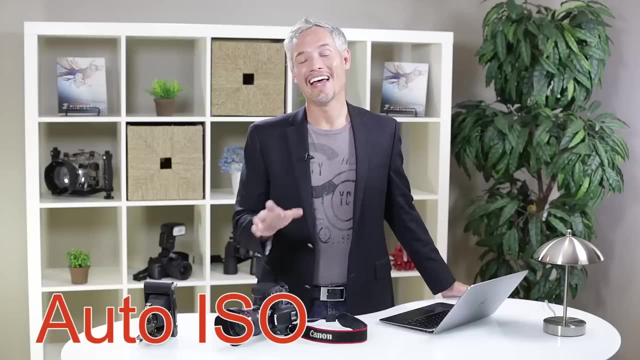 Because your camera handles the exposure automatically, By default. in fact, if you're ever not sure how ISO works, you can set your camera to auto ISO and then it will just set it for you And, in fact, whether you're an experienced pro or a complete beginner, auto ISO is a 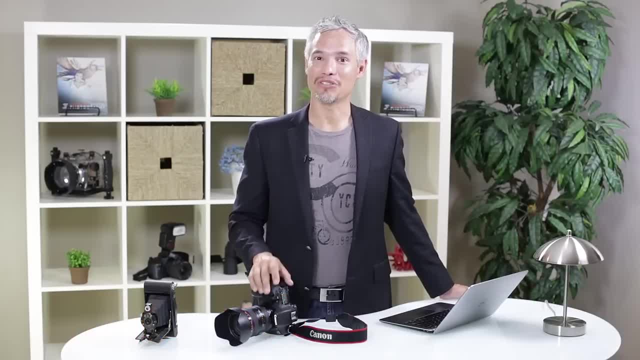 really good idea, because it allows you to instantly adapt to changing lighting conditions without having to change your shutter speed or aperture, which might change the content of your picture. Now let's look at some pictures taken at different ISOs, So I can show you. 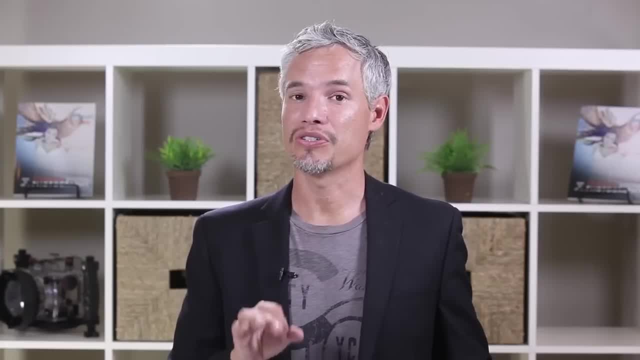 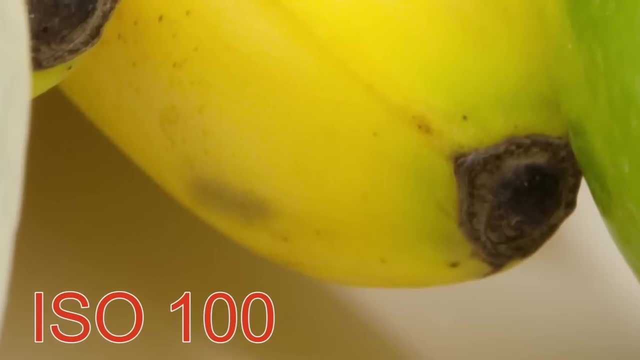 This is a major side effect of using higher ISOs, which is image noise. This first picture, more fruit, is taken at ISO 100.. As you can see from looking at this picture, it seems completely smooth. You don't see any noise or grain in it. 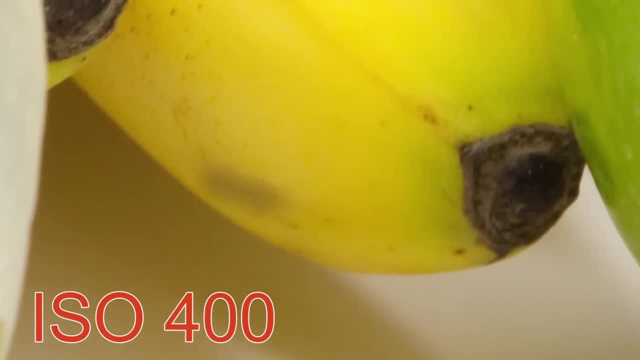 Now let's jump up to ISO 400. And especially if you look in the white areas, the shadow areas, there you can start to see it becomes a little bumpy, There's a little bit of noise there. Jumping up to ISO 1600, you can see that it becomes gritty. 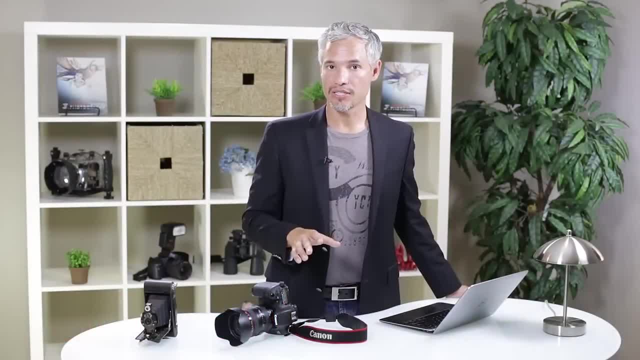 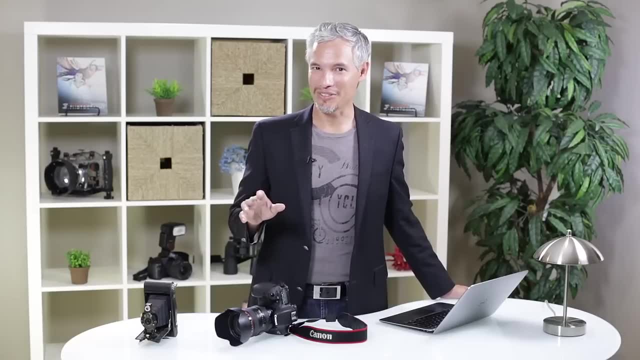 At this point It's not visible And anytime you use these higher ISOs this is going to be a problem. If you've gotten some pictures back and they look all speckled and they were like random colors, Well, that's digital noise. 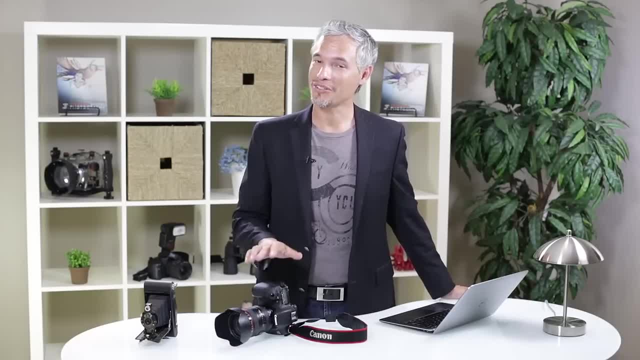 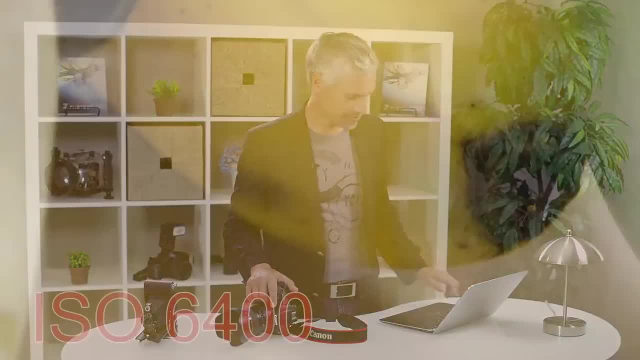 And it happens when your camera uses higher ISOs, And that's why it's important to understand ISO, So you can avoid that side effect whenever it's possible. Let's look at some even higher ISOs. This is ISO 6400.. 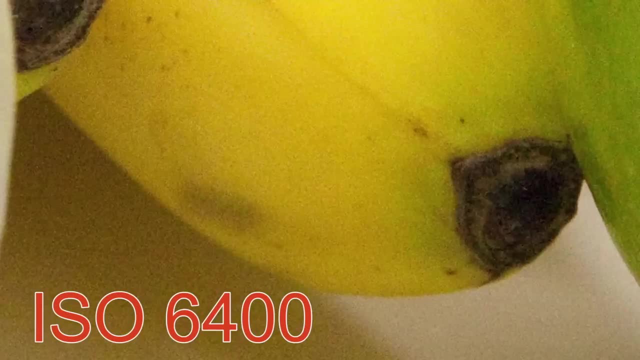 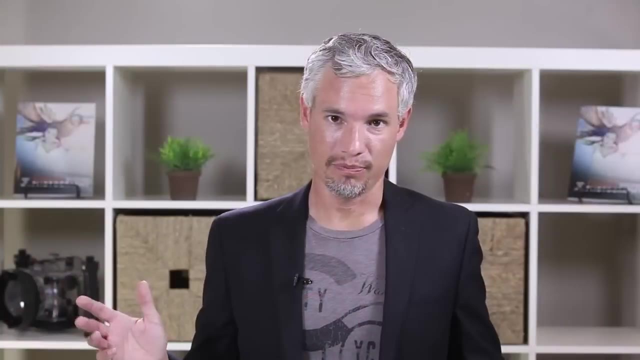 And even if the picture is really small, the noise here is going to be very, very visible, Jumping up to a ridiculously high ISO 25600,. you could see the picture at this point is basically unusable, Like it's really ugly. 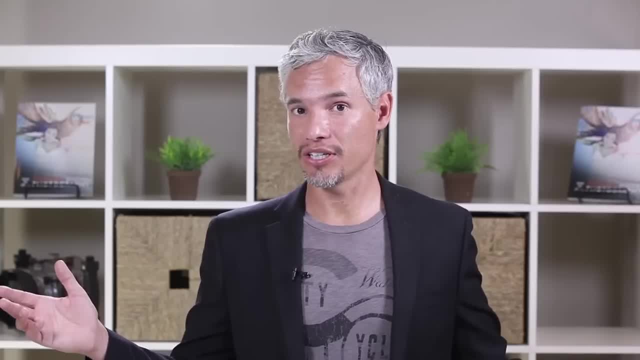 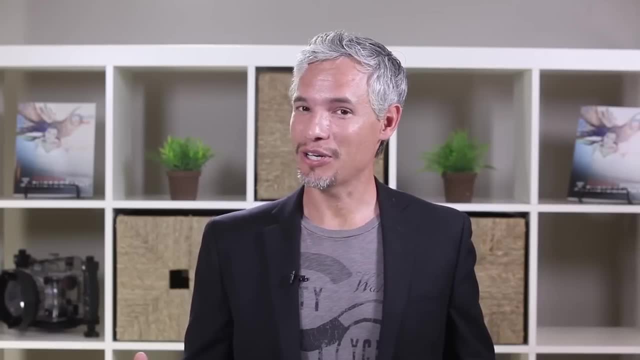 But you might have to use ISO 25000. if you're in dark conditions in a dim bar or a restaurant and you were working by candlelight, You know what. It's better to get some kind of picture, even a noisy picture, than no picture at all. 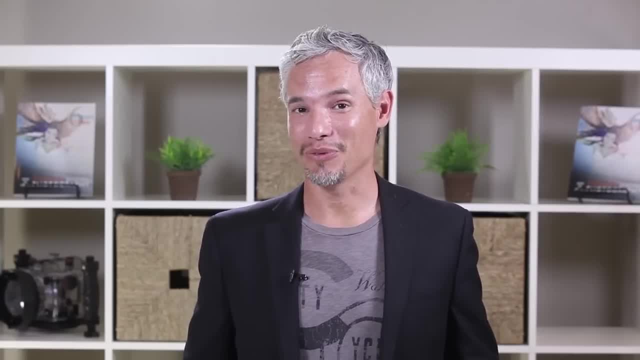 And you can always go to black and white. That's a little trick to visibly reduce the noise. So I know what everybody wants from ISO And that's ISO 2400.. So I know what everybody wants from ISO 2400.. So I know what everybody wants from ISO. 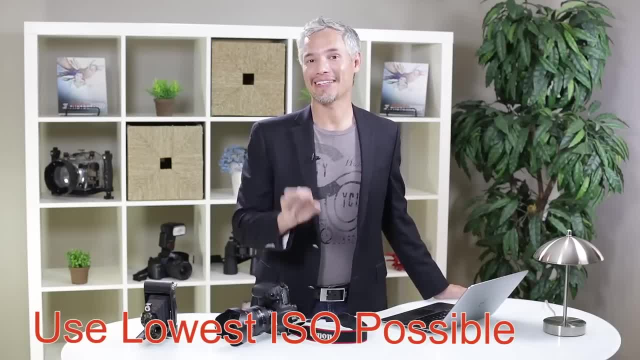 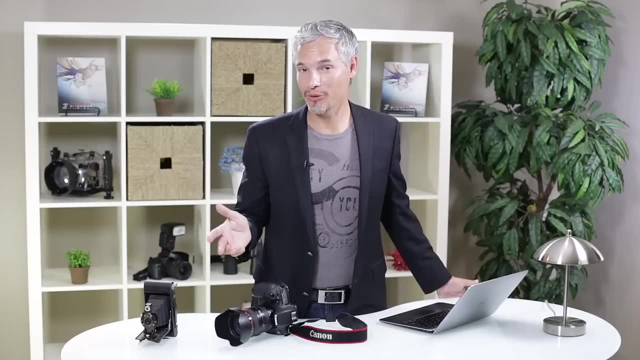 And that's to use the lowest ISO possible so that you get nice, clean pictures without a lot of noise. Well, I've already told you to use ISO 100 whenever possible, and then ISO 200 or 400 whenever that isn't possible. 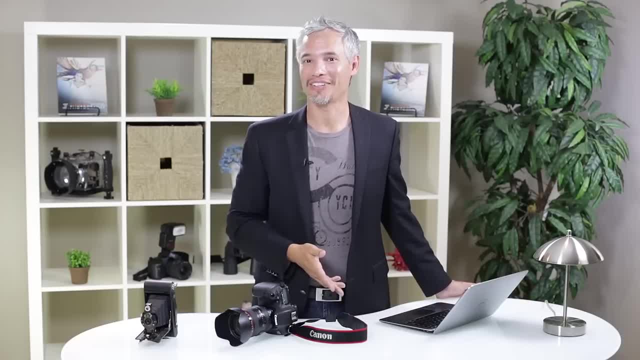 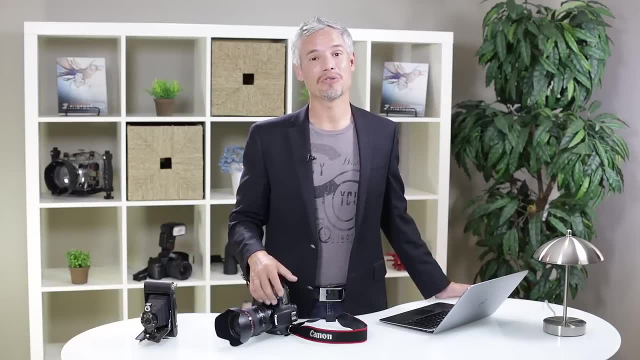 You don't want to just keep your camera at ISO 25600 because you saw what they'll look like, right, But if it gets dark you might not have any choice. Something has to give. Either you have to use a bigger aperture, and your lens only supports an aperture so big. 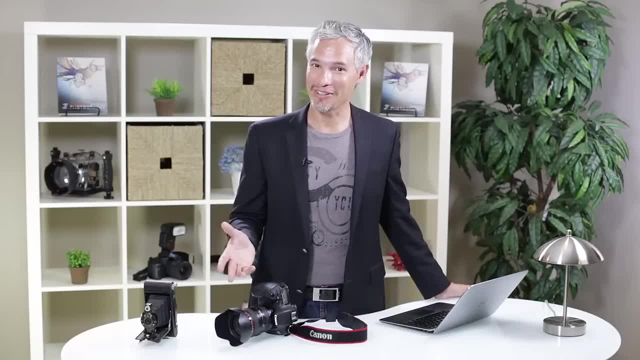 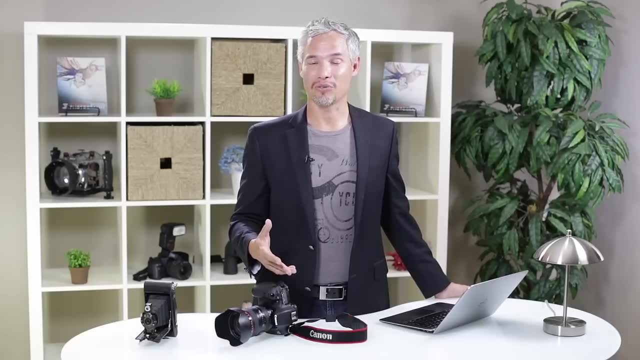 or you have to use a slower aperture. And we know what happens when you use a slow shutter speed right. Everything becomes blurry. You get camera shake or you get motion blur. So you can't always just use ISO 100.. There is another way to help reduce the noise that you get at lower ISOs. 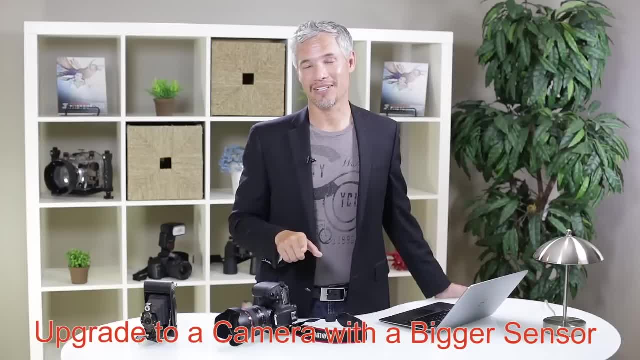 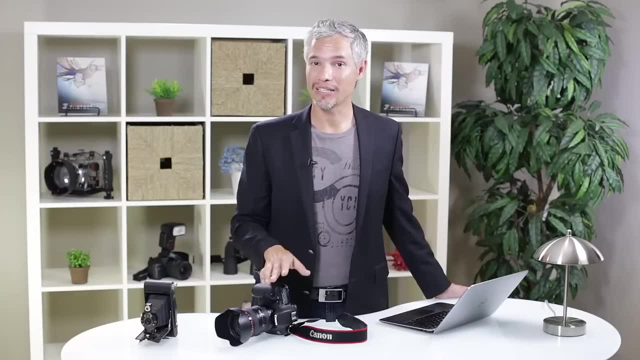 And again it's by getting a camera with a nice big sensor. These cameras are really expensive, so I don't want you to rush out and swap your camera or anything, But if you're completely knowledgeable about using ISO, aperture and shutter speed and you're, 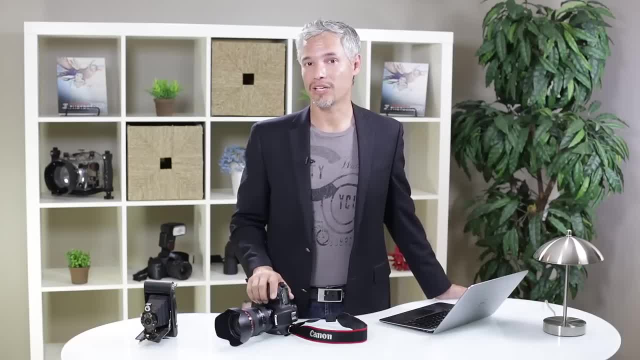 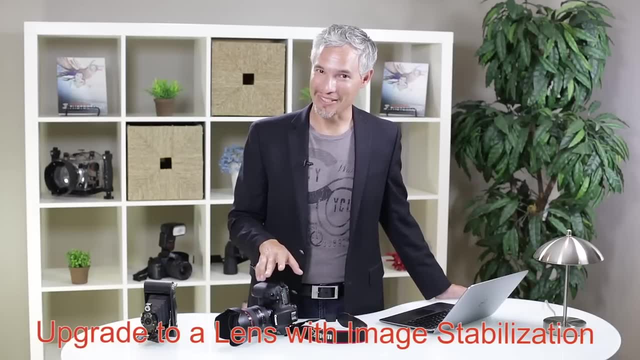 still trying to get less noise, I would recommend looking into getting a full frame camera. Another option for you that might be less expensive is to get a lens that supports image stabilization, As we discussed earlier, lenses that support image stabilization allow you to handhold. 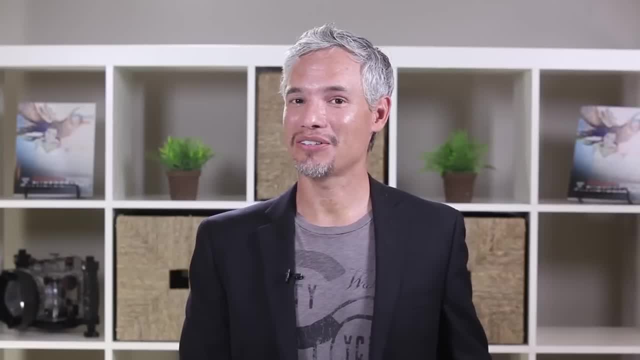 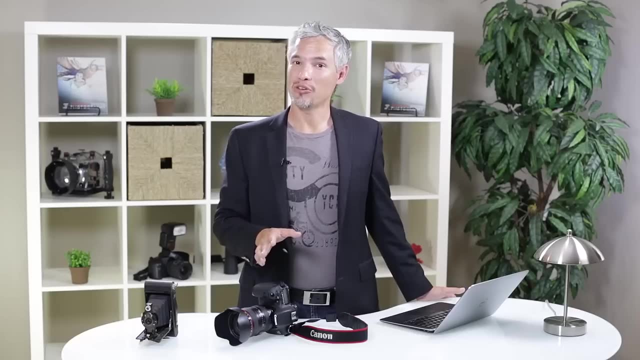 with slower shutter speeds. And with a slower shutter speed you can also use a lower ISO. Don't worry, if you don't understand this yet. I'll give you a more thorough explanation soon. Unless you're in manual mode, your camera is using an auto exposure system. 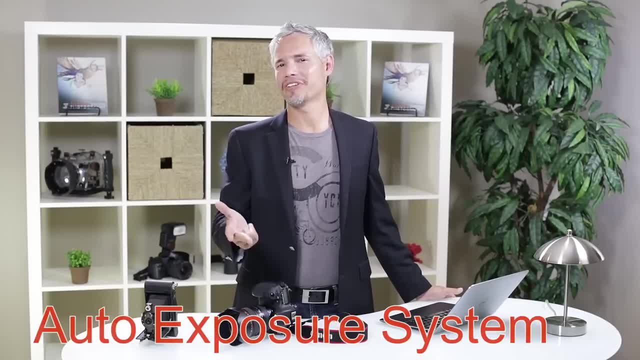 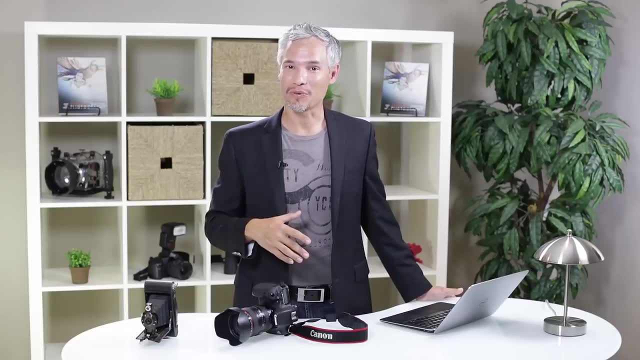 In other words, If you're in aperture priority or shutter priority or program, or you've got it on the green mode or one of those modes with a picture on them, your camera is using auto exposure and it's taking care of the exposure for you. 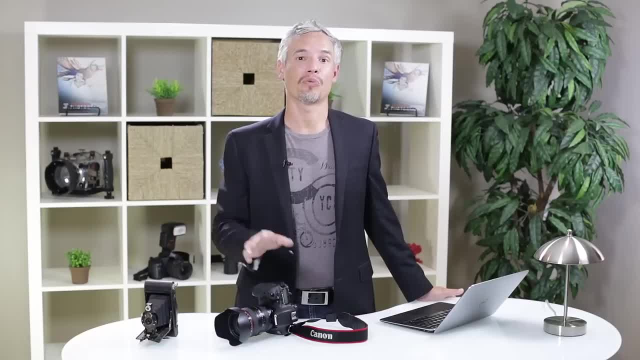 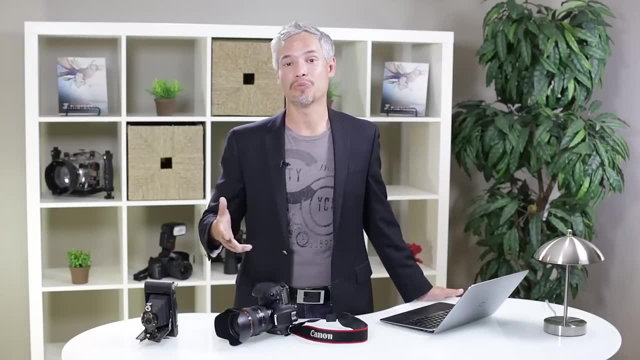 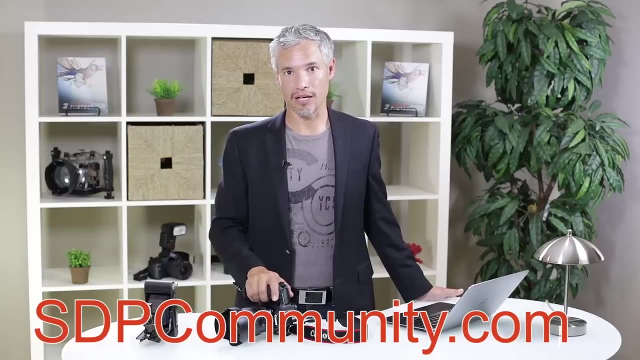 You should use auto exposure almost all the time. no matter how advanced you get, Even if you're a pro, you should use auto exposure. But sometimes the auto exposure is wrong and your pictures come out too dark or too bright. I would say this is the most common problem that I see on our readers group and at sdpcommunitycom. 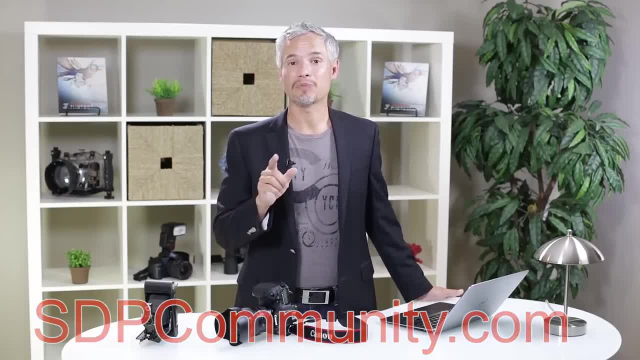 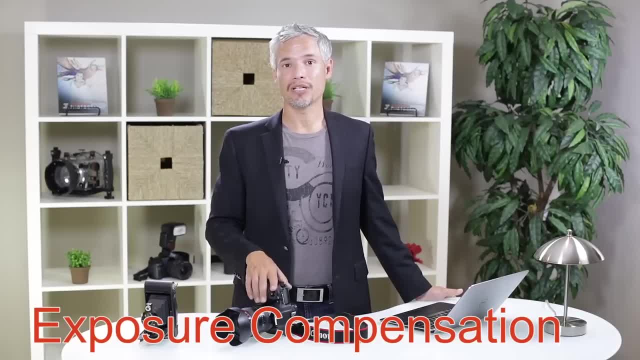 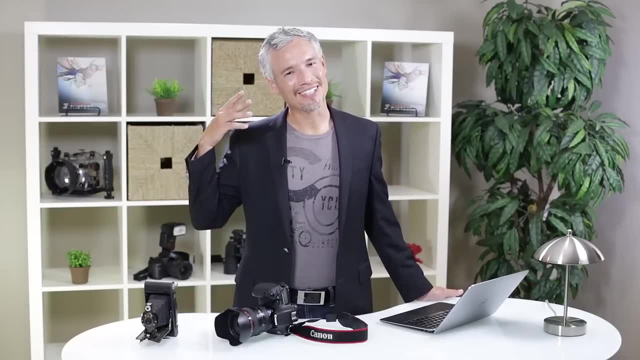 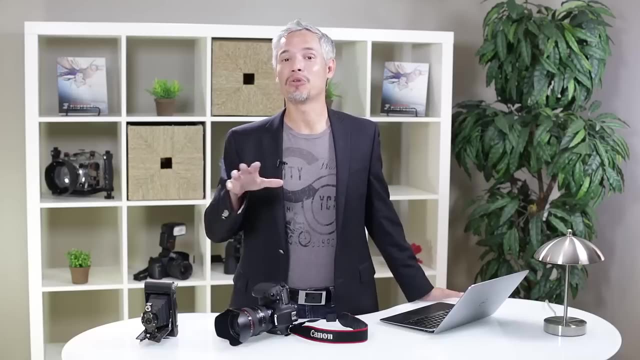 And it's by using exposure compensation. Exposure compensation simply adjusts your camera's default exposure settings. Your camera will evaluate the scene and make a guess about how bright or dark it should be, and usually your camera does a pretty good job at guessing, but it can't read your mind. 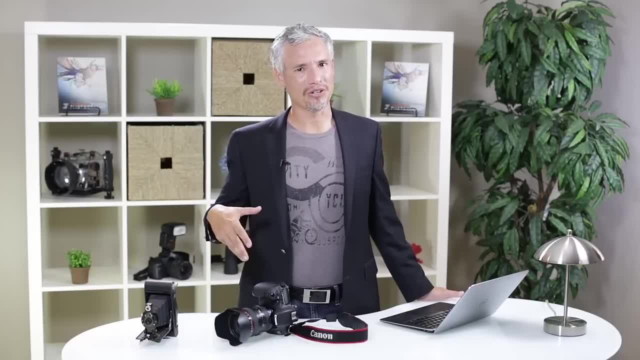 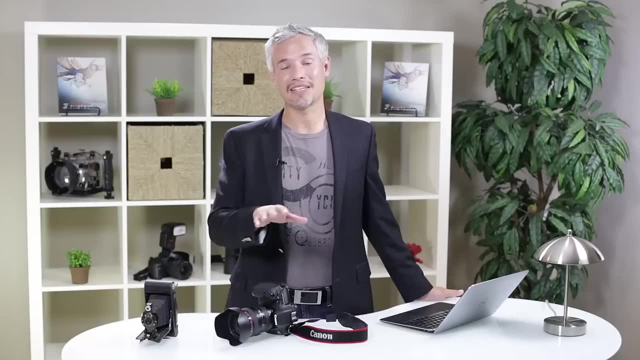 it doesn't know the most important part of a subject. If there's a guy there with a bright white shirt, okay, you want that shirt to be bright white as opposed to just gray, so you might have to take a sample picture and adjust it based on that, and that is what i usually do, because it's just not that hard. 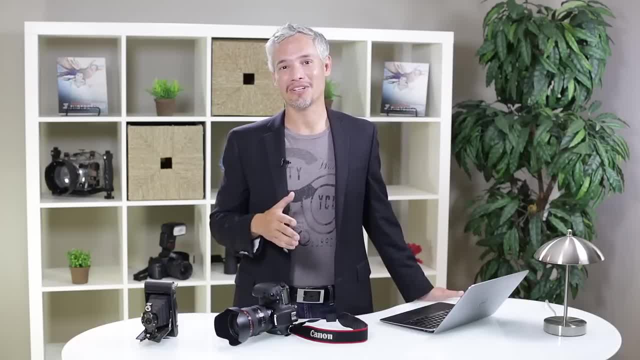 i'm going to go into detail about exposure compensation, but here's all you really have to know. take a picture, look at it and look at the histogram and, if it's not right, adjust the exposure compensation up or down. don't worry, i'm going to go out in the field and show you exactly. 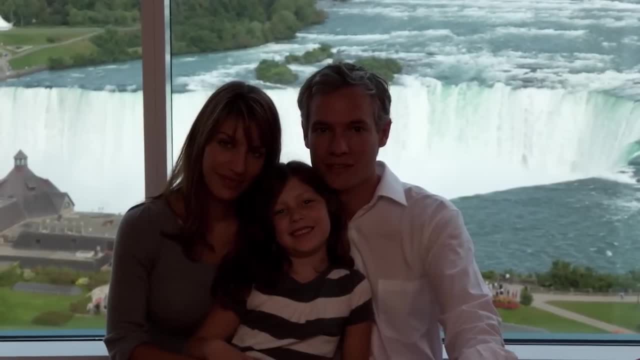 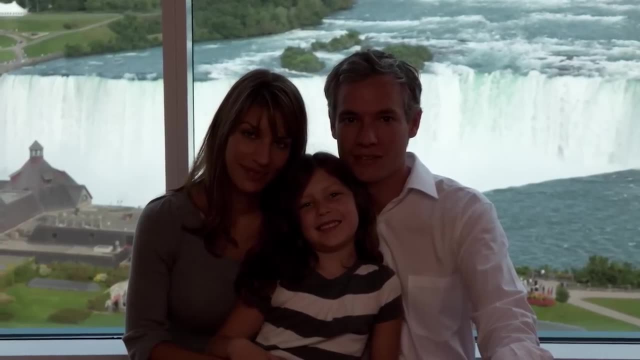 how to use that in a moment. so here's a snapshot of chelsea and i with our daughter and a hotel room in front of niagara falls. and niagara falls is bright and white and it was catching all the sunlight, but we were in a dark hotel room with just the ambient lights in the hotel and, as a 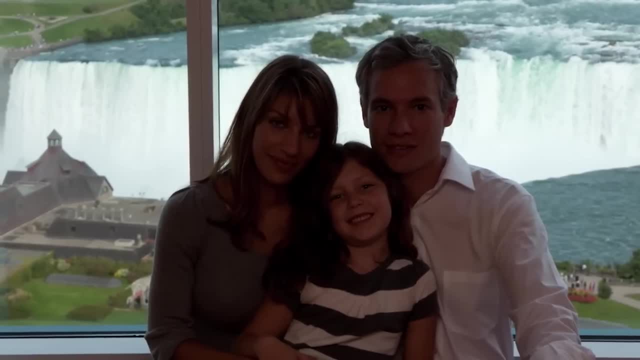 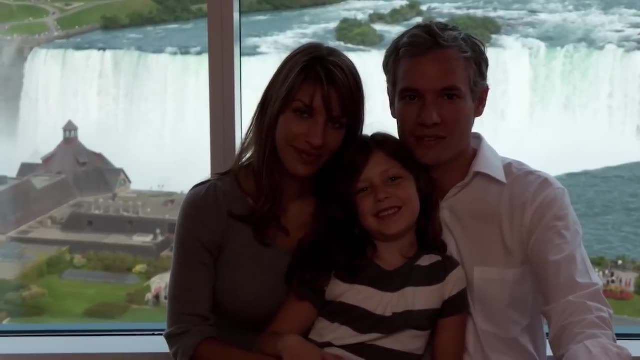 result: the background is really bright and we're very dark. so to fix this, i just dialed in a couple of stops of exposure compensation. there's a dial on the back of my camera that does it, and i added two stops, so let's look at the after picture. there we go now. in this picture we are correctly exposed. 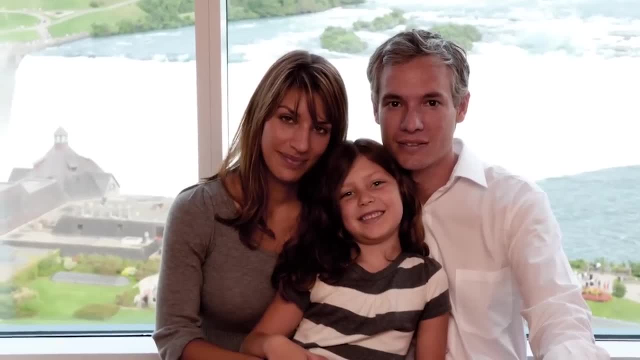 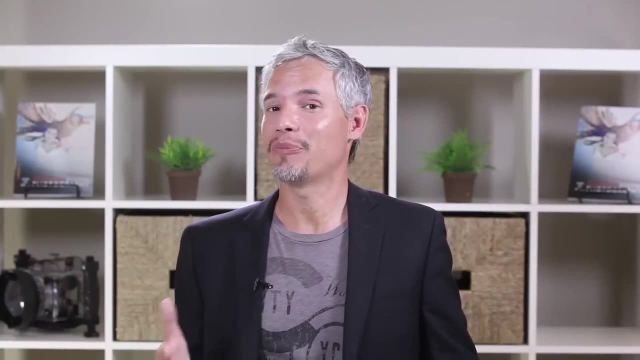 but the background itself is way overexposed. that's better than the first picture, right? because the most important thing is to get your subject properly exposed, and if the background gets blown out, well, might not be ideal, but it's better than the alternative. let's take a look at a couple more pictures. here we see a red-tailed 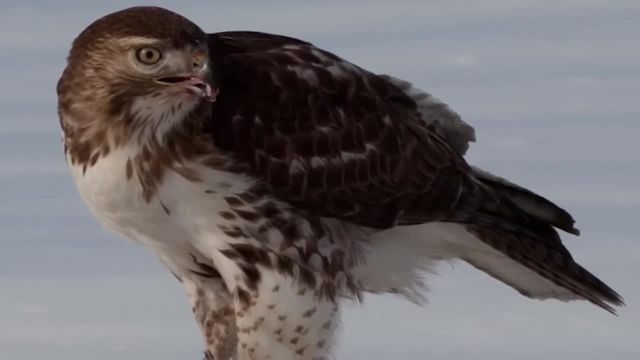 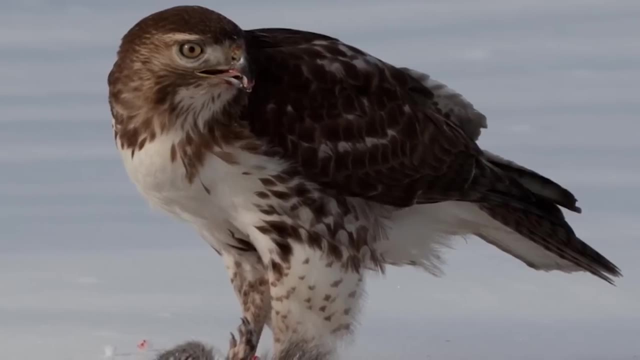 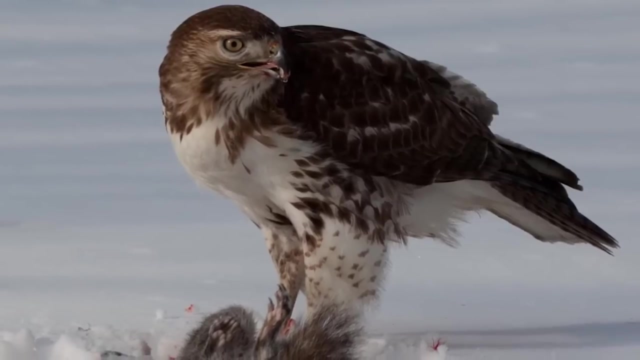 hog. it's kind of a gruesome scene. he caught himself some food, but the picture itself is actually pretty dark. it looks okay, but the snow should be bright, white, and instead the snow is kind of a middle gray. and this, like the niagara falls picture, is because the background is nice and bright but the subjects are dark. so to fix this, i just 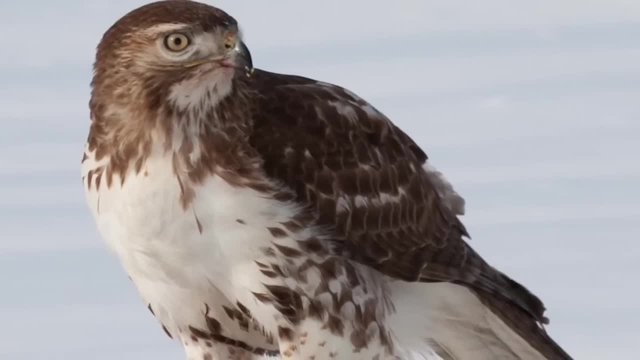 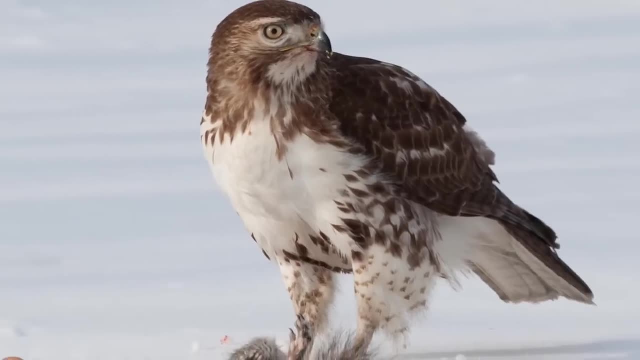 dialed in a stop or two of exposure compensation and, as you can see, the after picture is much better. here we have nice and bright snow. the whites and the bird are nice and white, but they're not overexposed. let's look at yet another picture. this is a picture of a cedar waxwing and 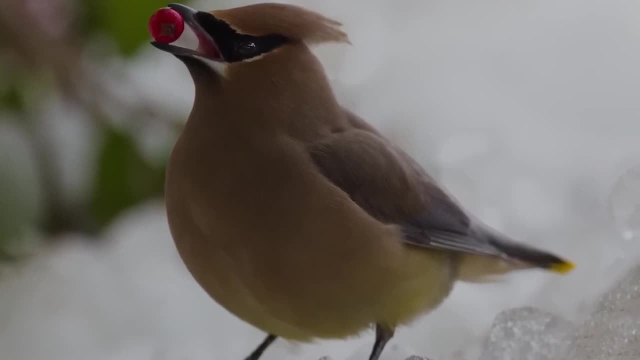 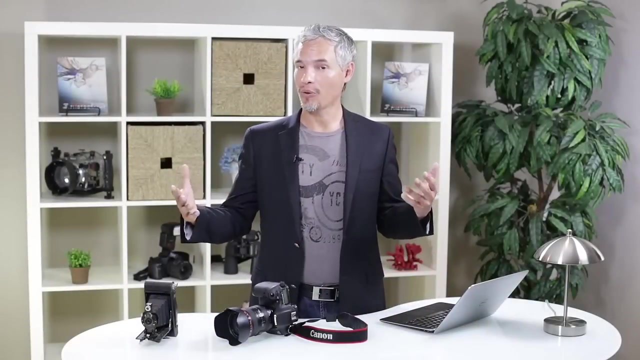 he's in the snow again. all these pictures so far have had bright backgrounds and dark subjects, and that's one of the situations that you really need to keep an eye out, for anytime the background is brighter or darker than the subject, you need to really be careful to check your exposure and 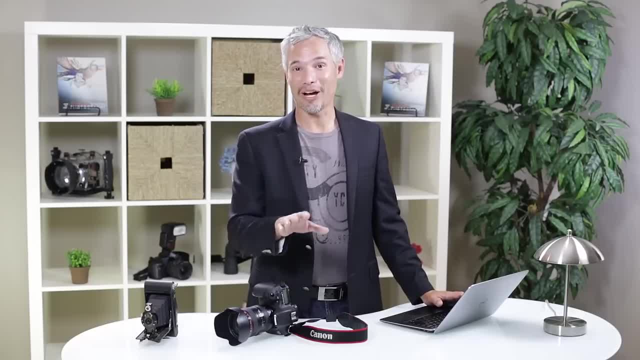 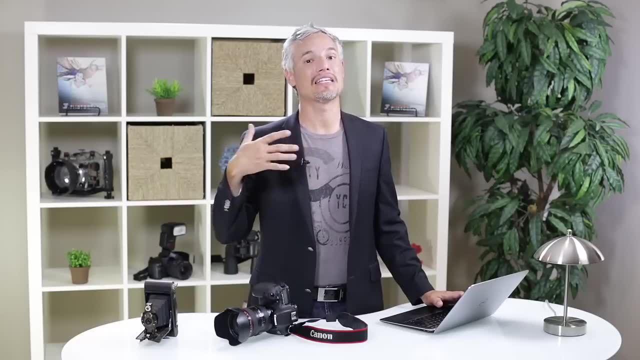 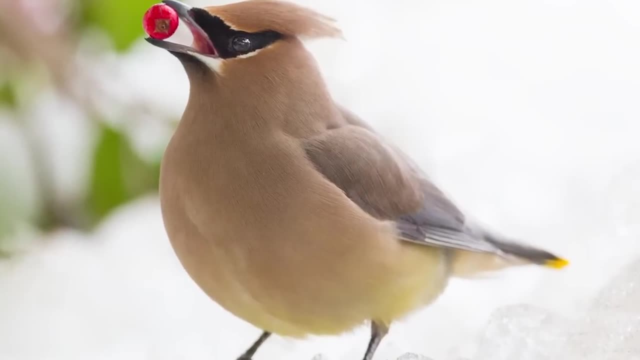 dial in exposure compensation as necessary. so with a bright background it's a little counterintuitive, but you need to add exposure compensation. you need to make your camera adjust the scene even brighter. so this is what my camera metered the picture at, and, and here's how it looked with exposure. 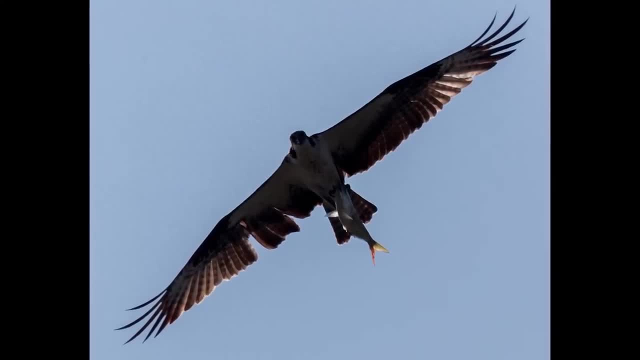 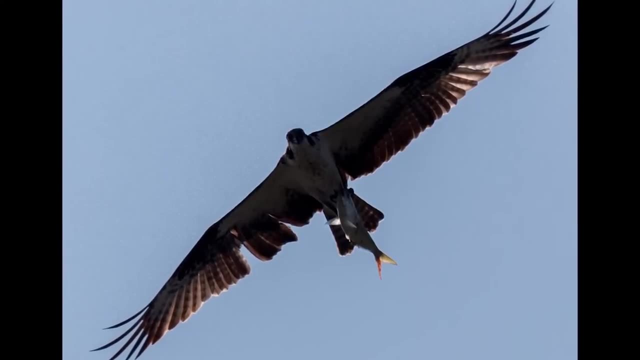 compensation. i have another shot here for you. this is an osprey with a fish flying through the air, and the sky, of course, is nice and bright because the sun was out that day and the osprey is in his own shadow. as a result, the osprey is way too dark and you don't get to see any of the details. so when i'm in that situation, 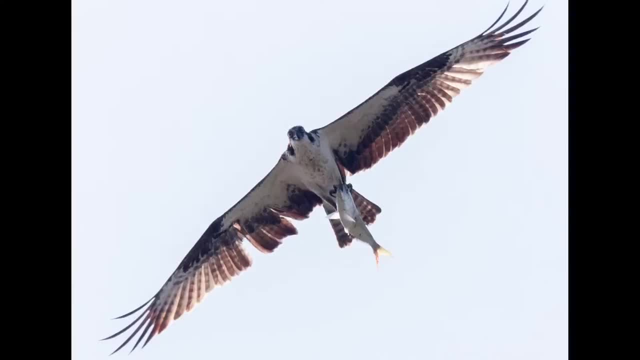 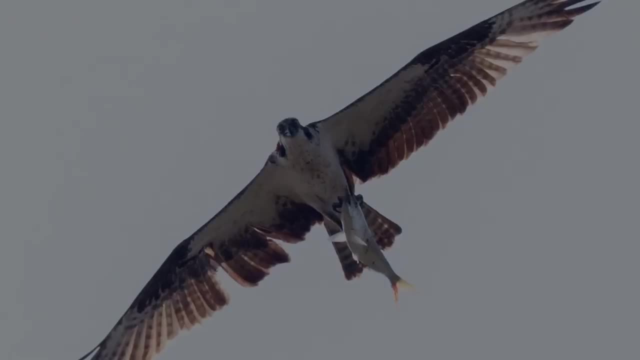 i know to add a couple of stops of exposure compensation. so with two stops of exposure compensation here, the sky is blown out but the osprey is properly exposed, and the most important thing is that you get your subject properly exposed, even if the background has to be over. 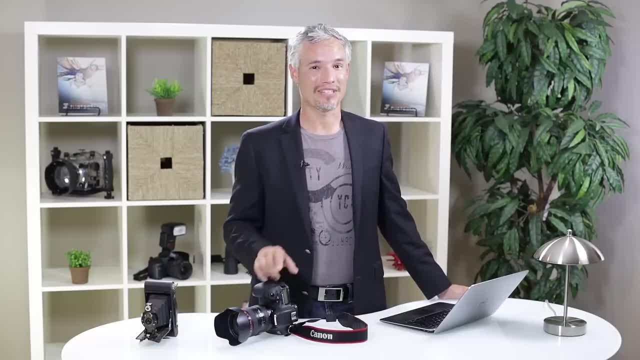 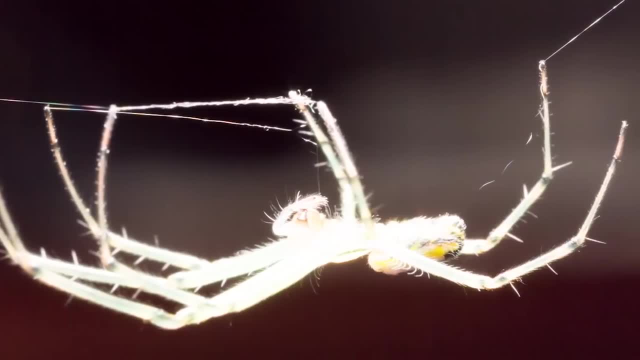 or under exposed. now let's look at a different type of picture. let's look at one with a dark background. this is a little orchard spider on a dark background. you can see he's weaving a web and he's completely overexposed. that's why he looks all white. the 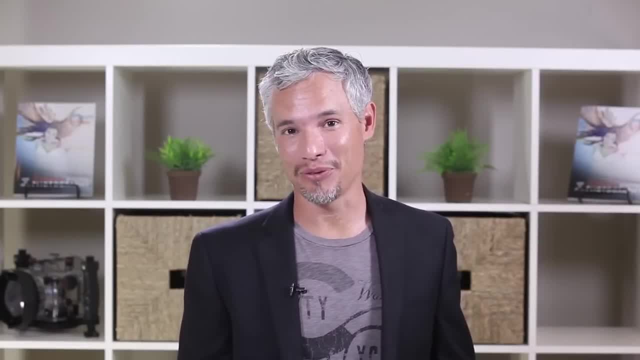 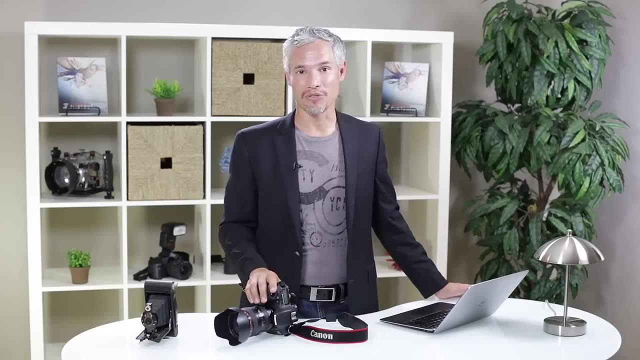 background, of course, is nice and dark. so the camera tried to expose the background properly. it tried to make it a gray color, basically, but i want the background to be black and the spider to be properly exposed. so i dialed in negative two stops of exposure compensation. i just turned that. 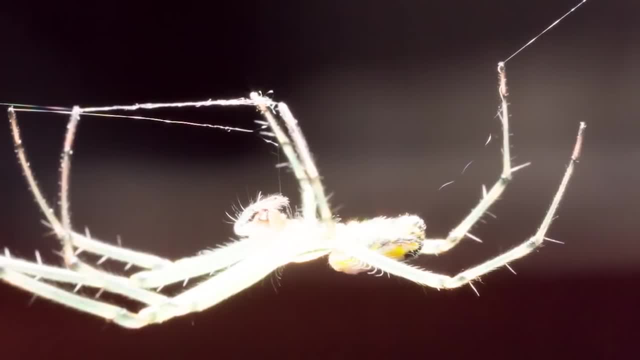 dial on the back of my camera counterclockwise over to the left, and then i'm actually going to and, as you can see, with the after picture, came out to be much more pleasant. You can see every detail of the spider and the background, which we don't care. 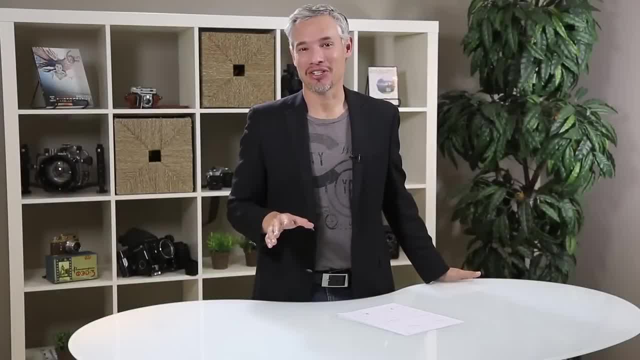 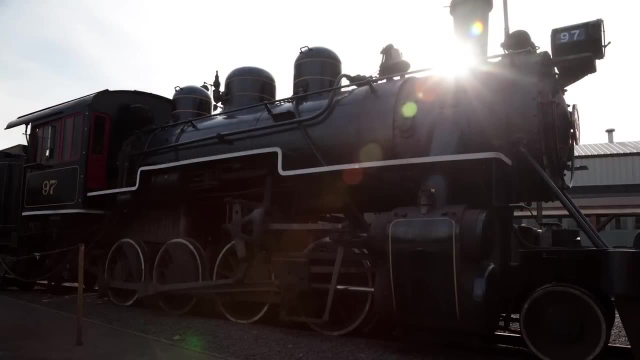 about is black. Now I'd like to talk about dynamic range. Dynamic range in a scene is the difference between the darkest, shadowiest part of the scene and the brightest to highlight in the scene. So if you're looking at, say, this dark train with the Sun behind it, the Sun obviously forms the brightest part of. 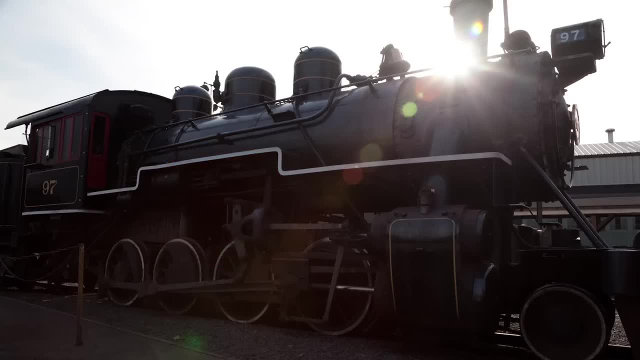 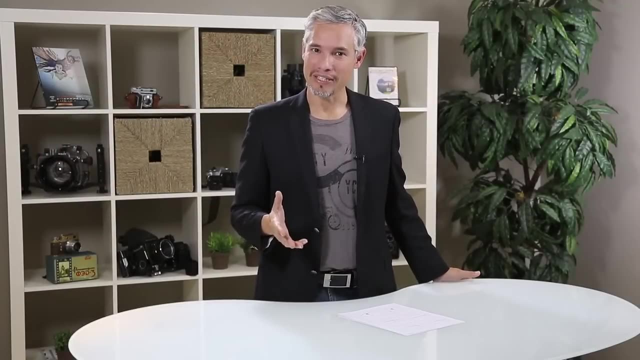 the scene and the train forms the darkest part of the scene. Now your eye and brain have a limited dynamic range. Your eye and brain can see about 20 stops of difference. So there's about 20 stops of difference between the brightest thing your eye can perceive detail in and the darkest thing So you can make. 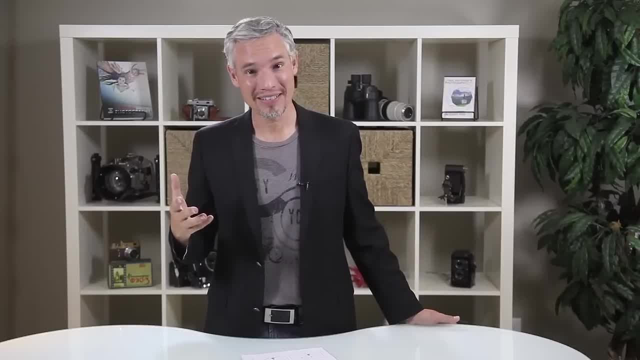 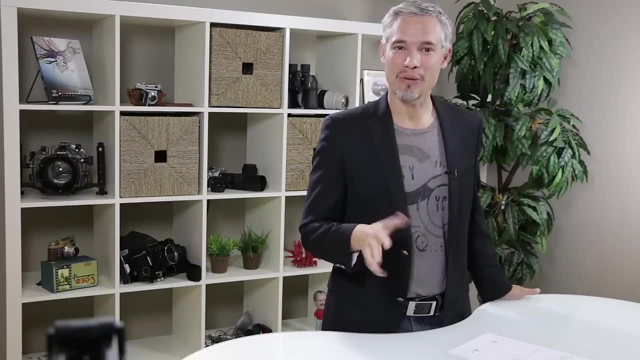 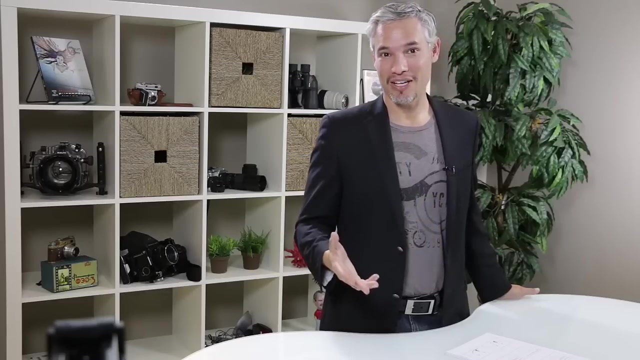 out detail in a shadow and detail in a highlight that's a million times brighter. Your eye is pretty amazing that way. Your camera is good, but not nearly as good. Your camera can make out about 10 seconds, So that's a big difference between what your eye can see and what your camera can capture. 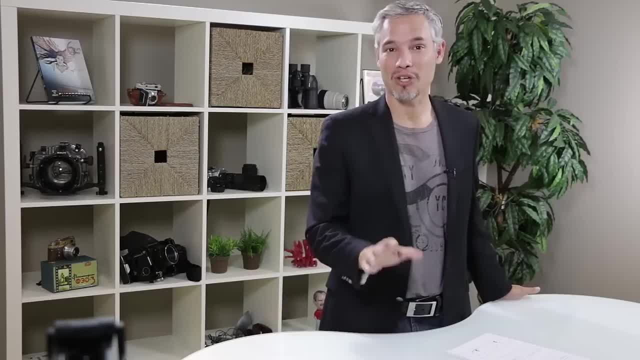 And this is one of the biggest challenges in photography and that's why I'm talking about it- because you need to understand the dynamic range of your camera and how you can control it to best capture a scene. Now, some scenes that you're in will have a very limited dynamic range. 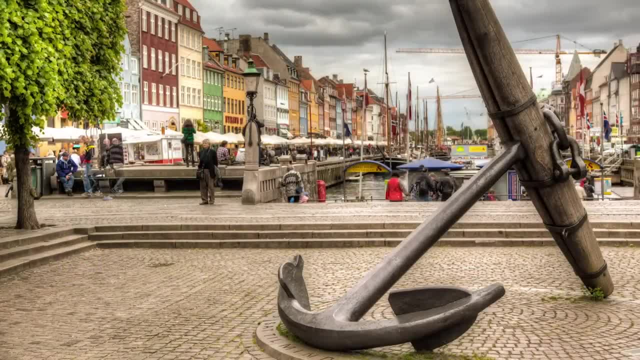 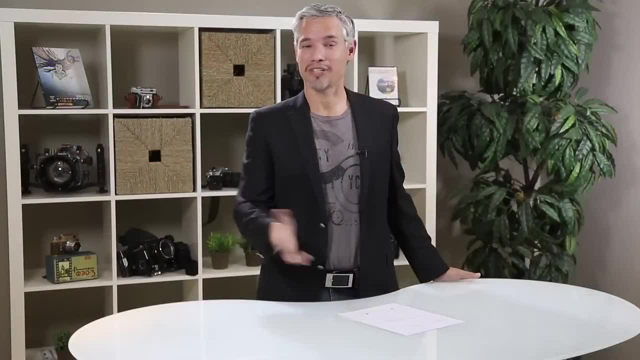 If you're outside and it's an overcast day, the lights gonna be very. even then you might only have four or five stops of dynamic range, So your camera's auto-exposure system will capture it just perfectly and you don't have anything to worry about. However, if you're in a scene that has 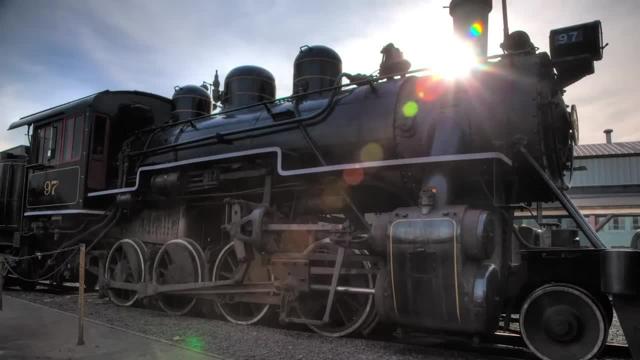 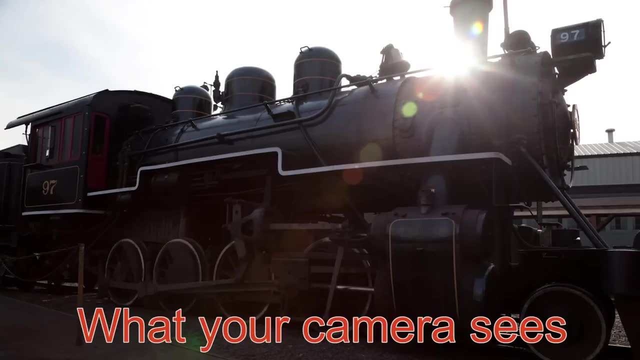 a great dynamic range- say, 20 stops of dynamic range- here I will be able to see everything just fine, but your camera is only going to be able to capture about 1% of that dynamic range. therefore, you need to make some adjustments, Your 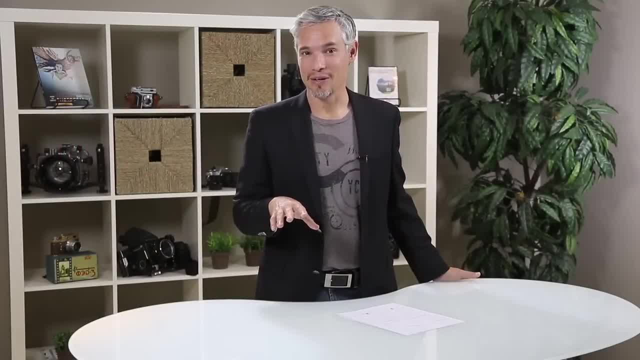 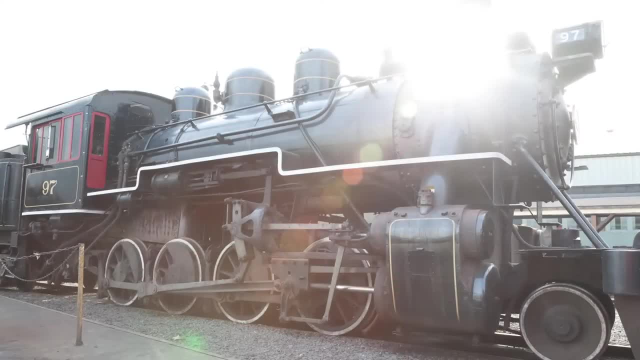 camera will try to expose some part of the scene correctly, but what might happen is the foreground could be underexposed and the background could be overexposed, or vice versa, and you might not be able to make out the most important part of the scene. So in situations like this, you need to be able. 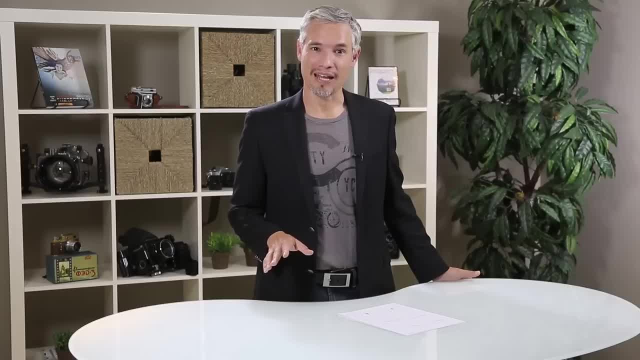 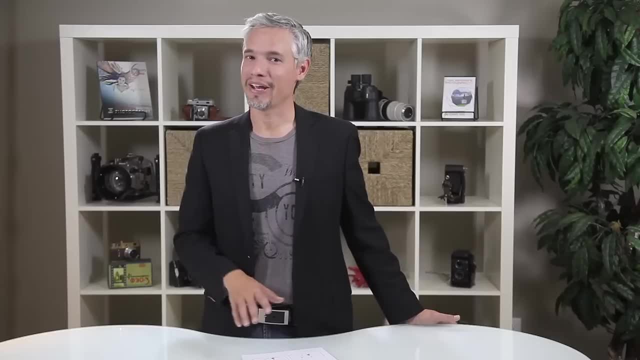 to understand your camera's exposure system and how you can select which part of the scene you want the camera to capture correctly. So we'll talk more about metering and exposure compensation in a minute and we'll look at some more examples. but I also want to add that you can kind of control the dynamic range. 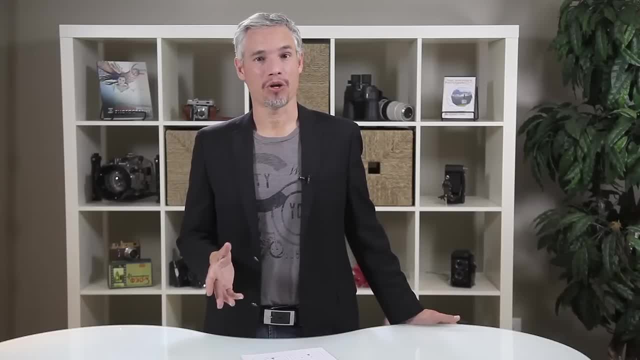 You can add light to the shadowy parts of an image to reduce the overall dynamic range of a scene and make it easier for your camera to capture. The easiest way to do this is just to add fill flash If you're taking a picture of. 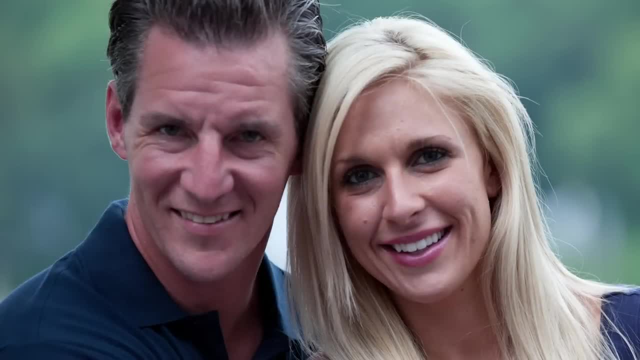 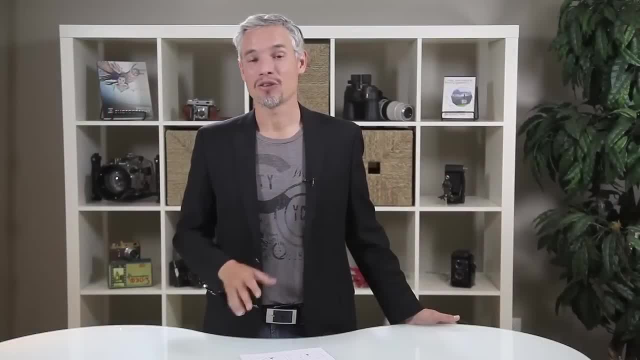 bringing up the light in the shadows. Another way to overcome the limited dynamic range of your camera is by using HDR. That stands for high dynamic range, and with HDR you set bracketing on your camera and you capture three or five or more pictures at different exposures, So you'll take a really dark picture and a 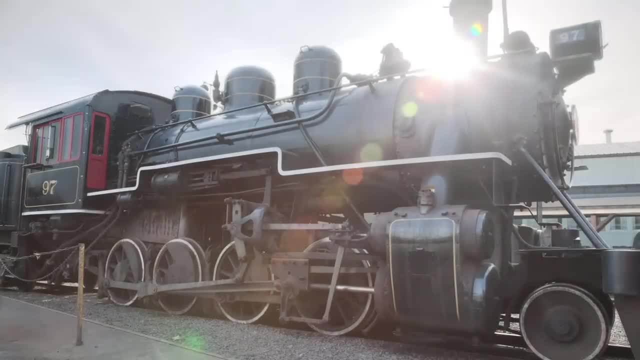 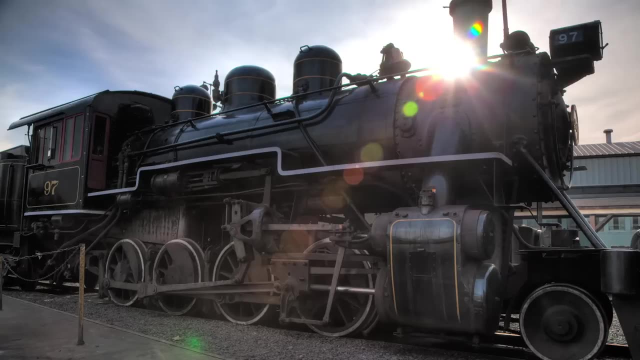 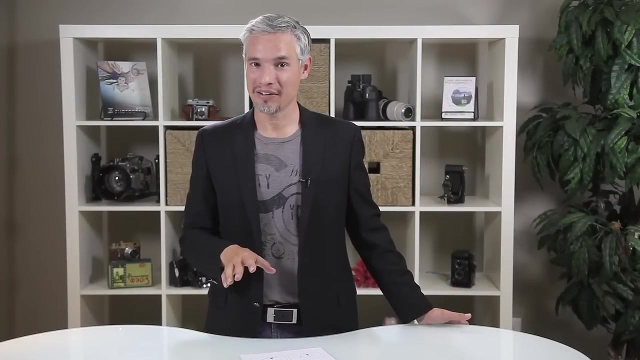 normally exposed picture and then a really bright picture. Then you'll blend the best parts of each image to virtually extend the dynamic range of your camera beyond 10 stops and maybe to 15 or even 20 stops that your eye can see. I'm not going to cover HDR in complete detail now, but you can check. 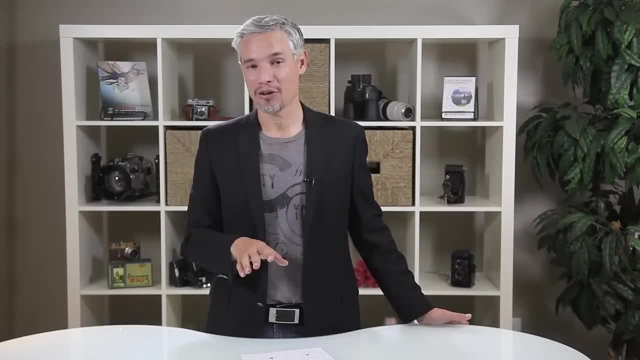 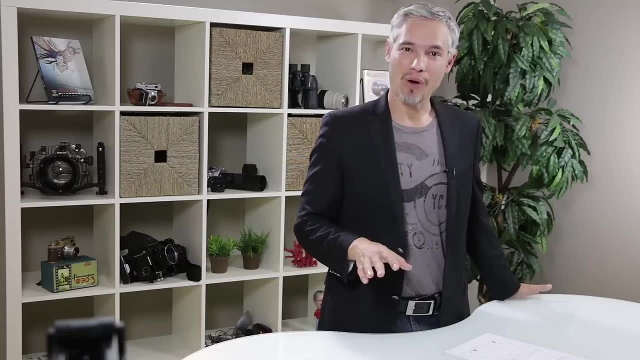 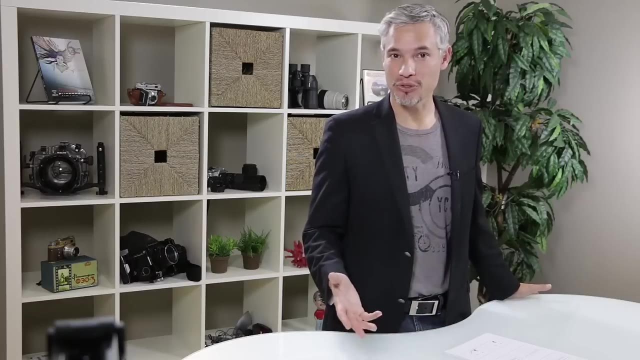 out chapter 11 of my book Stunning Digital Photography, or check out the videos at SDP Community for more detail. Now I mentioned metering, and metering is the process that your camera goes through to determine the proper exposure, The exposure being which aperture and shutter speed and ISO it's going to use. 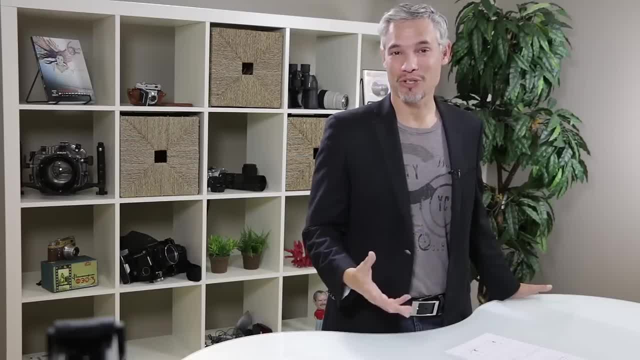 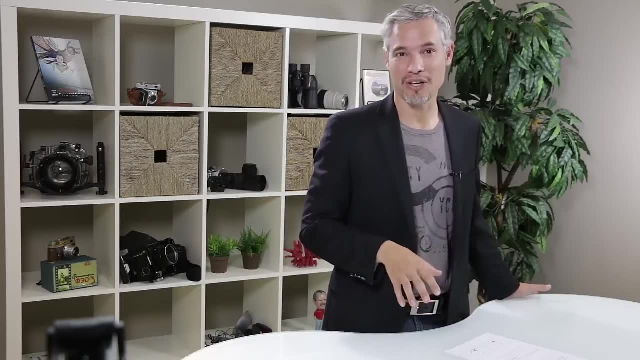 Metering determines how bright or how dark a picture is going to be. Obviously, your camera kind of looks at the scene and decides: hey, this is a really bright scene so I can use a really fast shutter speed, or this is a pretty dark scene, I need to use a really slow shutter speed Any time your camera is making important. 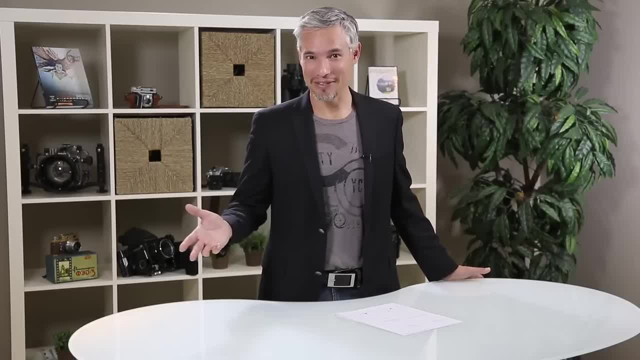 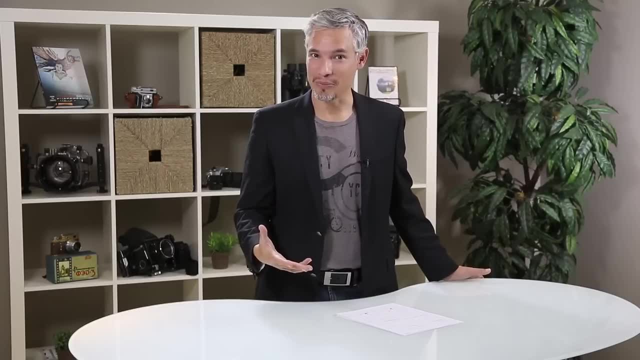 decisions like that. you kind of need to understand it, because your camera is going to make some mistakes. After all, you're going to have a camera that's going to take a picture. After all, your camera can't necessarily determine whether you're trying to take a picture of the really bright subject in the background. 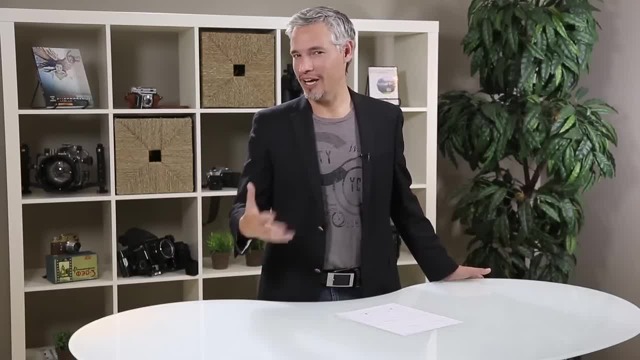 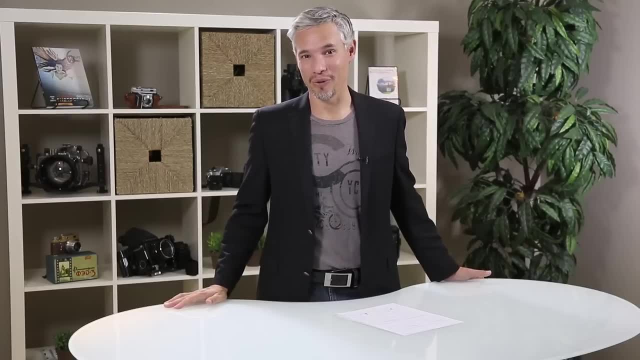 or the really dark subject in the foreground. Therefore, it might pick the wrong one to expose properly, or it might just pick some exposure in the middle which exposes neither the foreground or the background correctly. Generally, however, you can just use your camera's built-in auto exposure system and things. 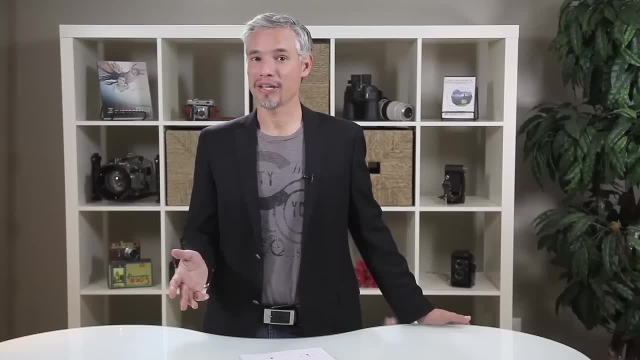 will go well. Now, in the digital era, what I usually recommend is just relying on your camera's auto exposure system and taking a shot. Then take a look at the picture you just took and look at the histogram specifically. Usually you can view the histogram by just hitting the info. 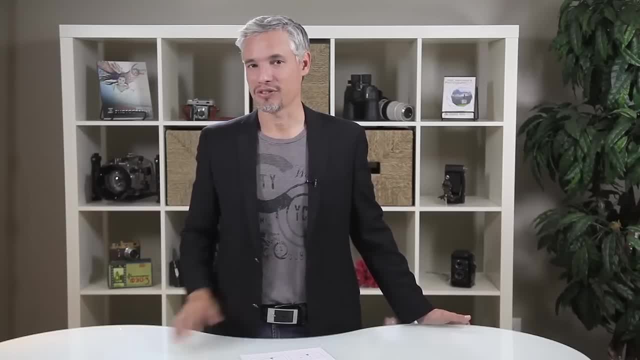 button on the back of your camera a couple of times until you see that little chart. We're going to look at some more examples of that later. But if your picture is too dark, you add a stop or two of exposure compensation to brighten it up, and if your picture is too bright you use exposure compensation to reduce. 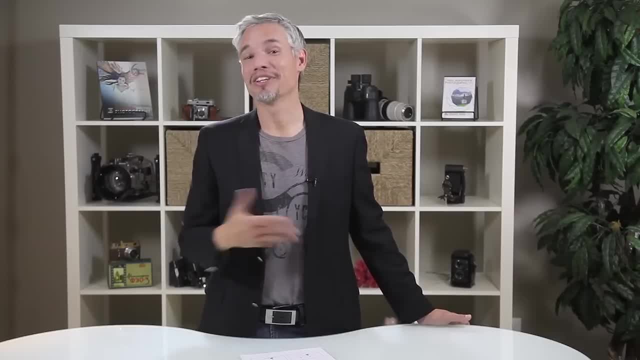 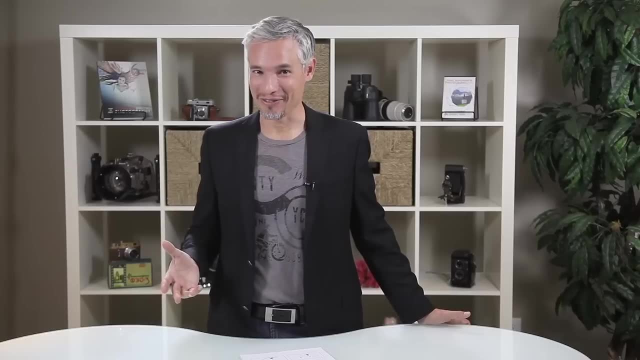 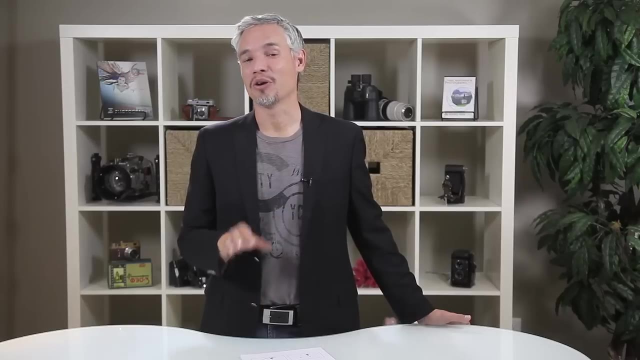 the overall exposure until the subject looks right. So in the digital era, I really recommend trial and error. Now, when I was shooting with film cameras back there, I didn't have the luxury of trial and error, because it would have taken me hours of developing and printing to determine whether or not I had exposed something properly. So then, 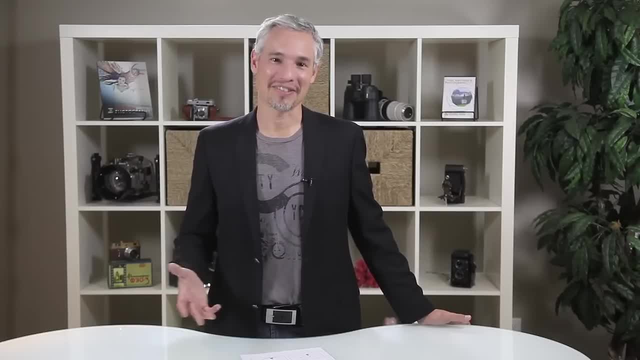 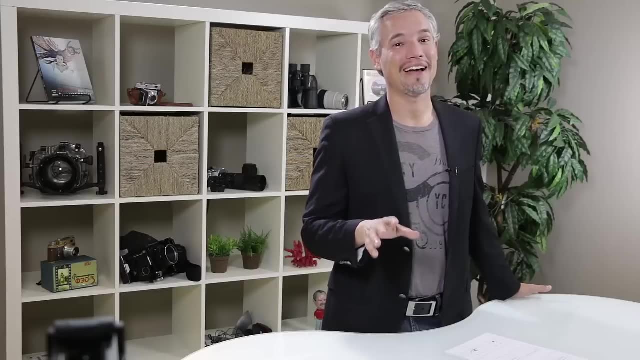 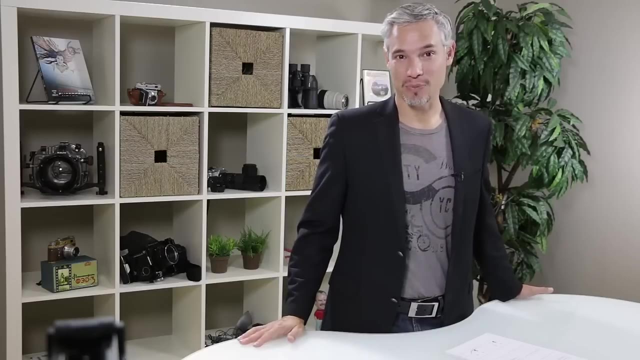 I had to be a little more precise about it, But nowadays, digital, the fastest thing to do is just to take a sample shot and make adjustments based on that shot. So now I'm gonna grab Chelsea and drag her outside into the bright white snow so we can go hands-on with exposure and exposure compensation. 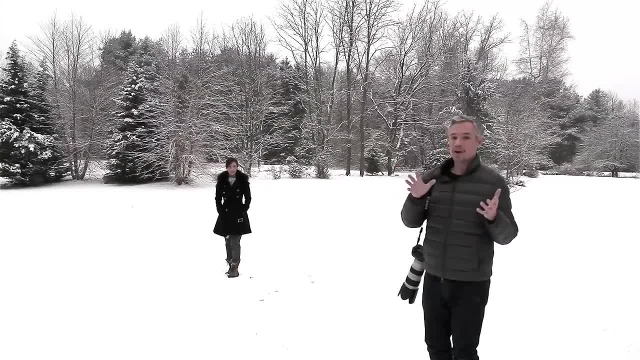 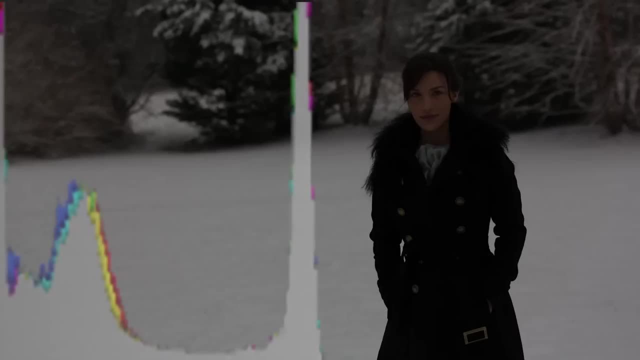 Snow is one of the like perfect examples for a situation that requires you to change your camera's default metering. So to explain this a little more, I'll take a couple of sample shots of Chelsea. Now. take a look at that picture, and especially the histogram, because it's really important that you review the 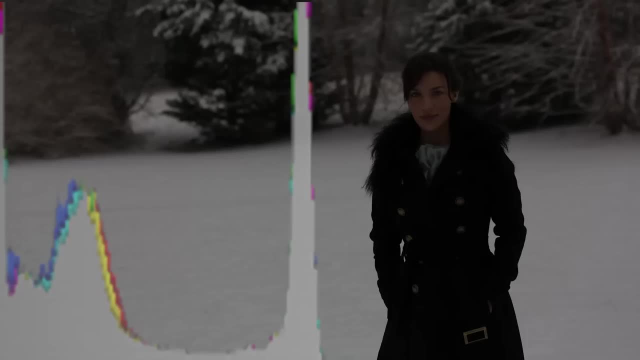 histogram anytime that there's an exposure challenge, like a bright environment or a dark environment. This histogram is almost entirely in the left half of the frame and that's no good at all. That means our picture is underexposed. Now you can't just trust your eye here. 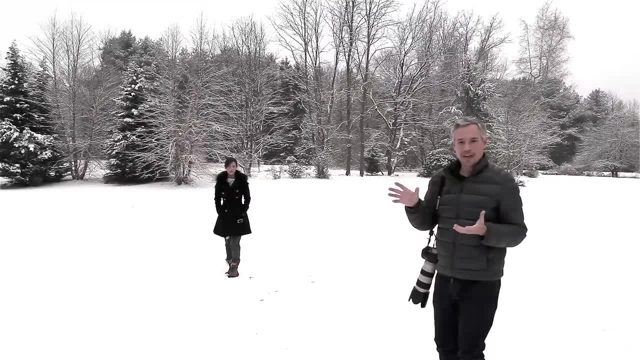 because a million times I've looked at the preview of an image on my camera when I'm out shooting and thought it was okay. Then I get it back on my computer and see the histogram and realize it's wildly underexposed. You can't trust your. 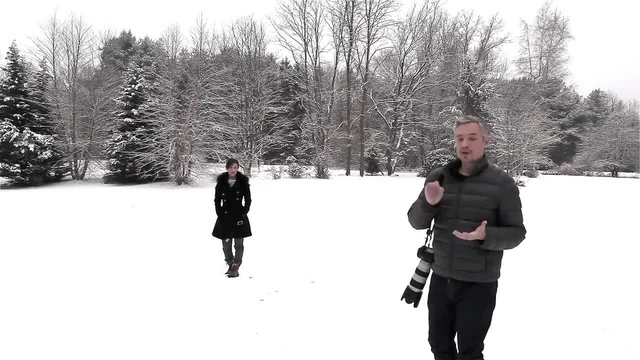 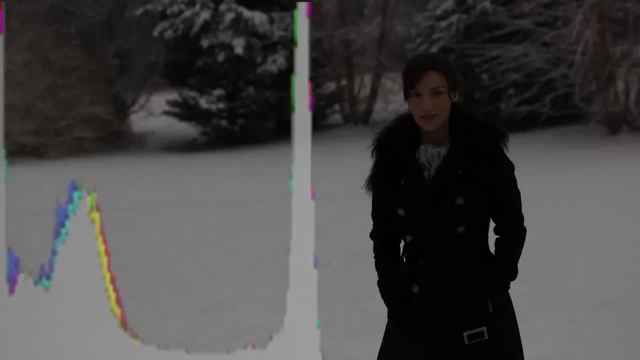 camera's LCD, You always need to look at the histogram. So when you see a histogram like this that doesn't touch the right side, that means the photo's underexposed And, as a rule of thumb, when you're in a bright environment like this, 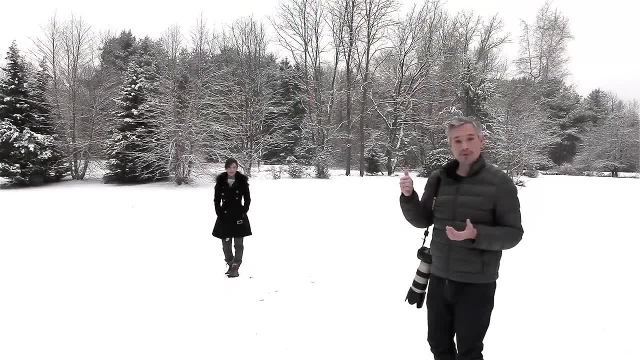 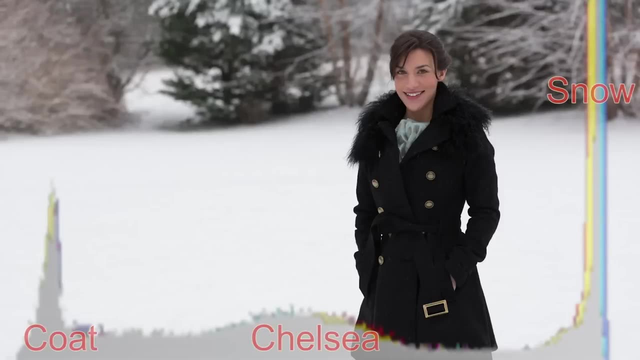 you need to add at least a stop of exposure compensation. But when it's mostly snowy like this, you need to add a couple of stops of exposure compensation. So I will add two stops of exposure compensation and shoot again. That turned out much better. Now, that's really all you need to understand about. 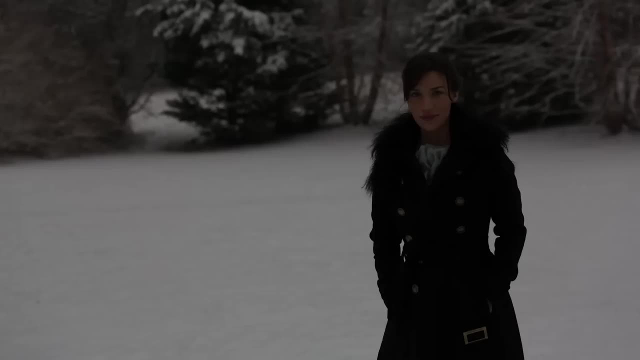 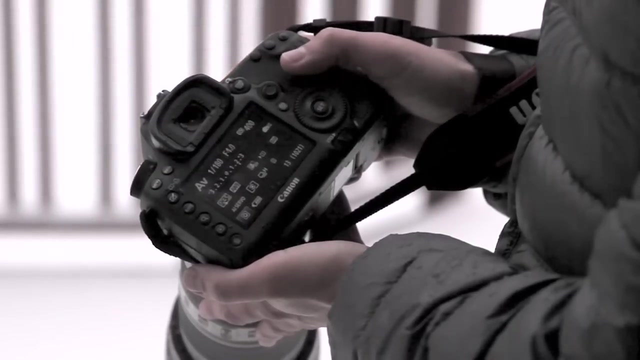 metering and exposure compensation. Take a shot, look at the histogram. If it doesn't touch the right side of the frame, then you need to add one or two or three stops of exposure compensation. Shoot again and if the histogram is perfect, then you're good. Back in the olden days when we shot film. 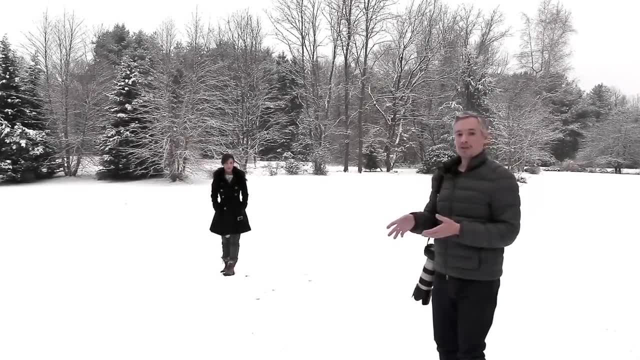 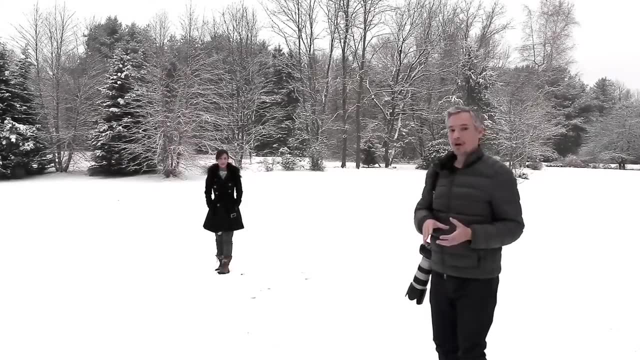 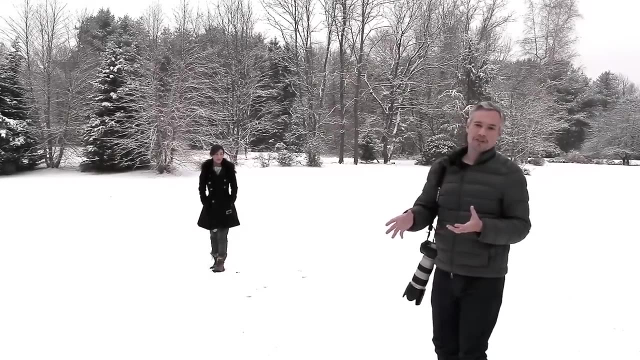 you didn't get a chance to immediately review it and then reshoot And, as a result, cameras developed these really complex and flexible metering systems and they're still in our modern cameras And, in fact, the camera manufacturers often use them to advertise advantages of their models versus competing models. 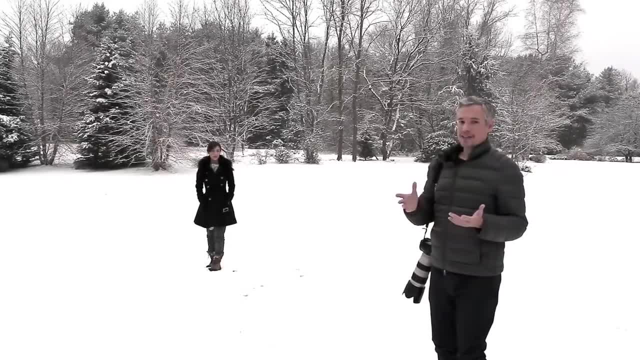 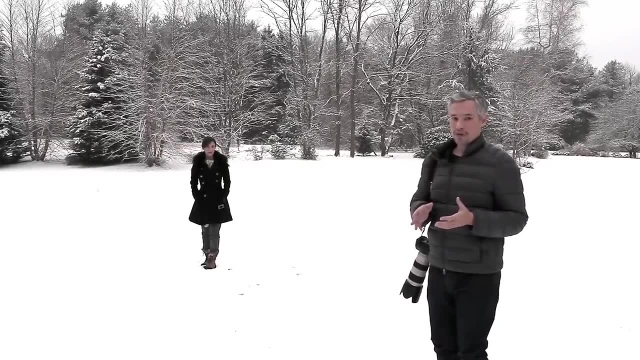 But I don't think they're that important because nowadays, I think the easiest thing to do is just to take a shot and make an adjustment based on what you see. However, I do want to give you an overview of your camera's different metering modes. 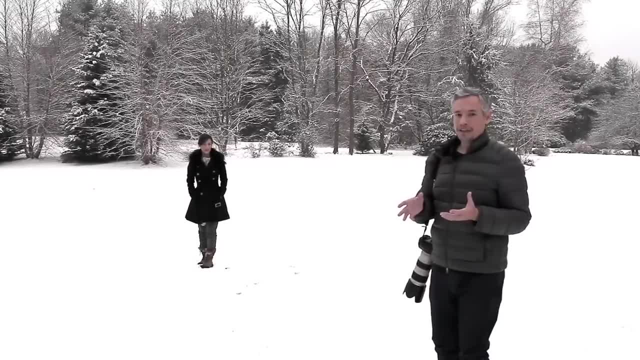 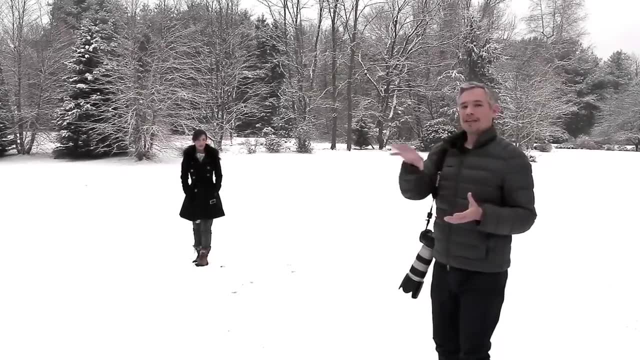 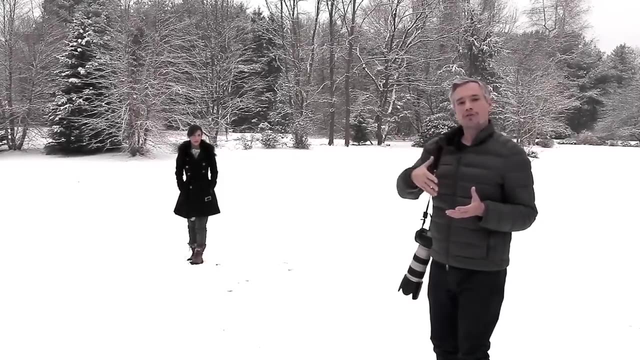 Now the one that your camera is probably set up with by default is they have different names. Some companies call them evaluative metering, some are zone metering, But they look at the entire frame and intelligently decide what the exposure should be. So they'll look at your foreground subject and the 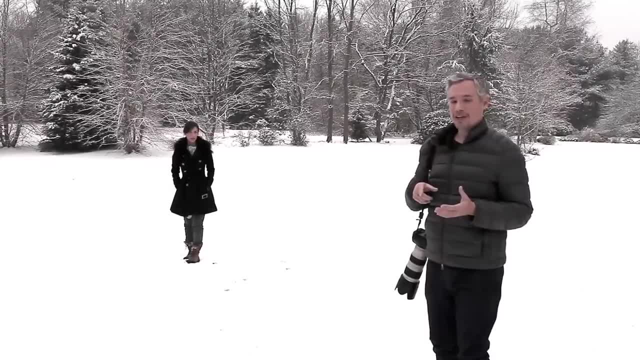 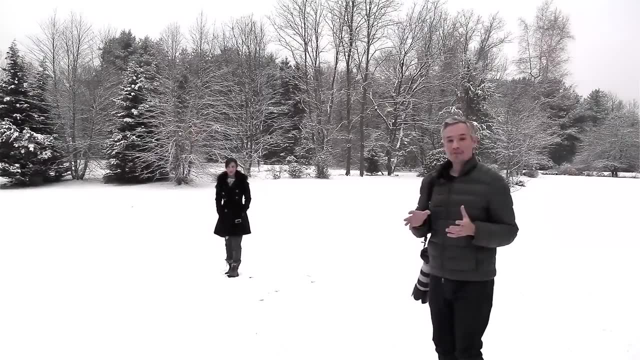 background subject and try to guess. That's what my camera was set up with when it managed to underexpose that shot by a couple of shots, So it doesn't work perfectly. The way your camera's metering system works is that you can set up a camera. 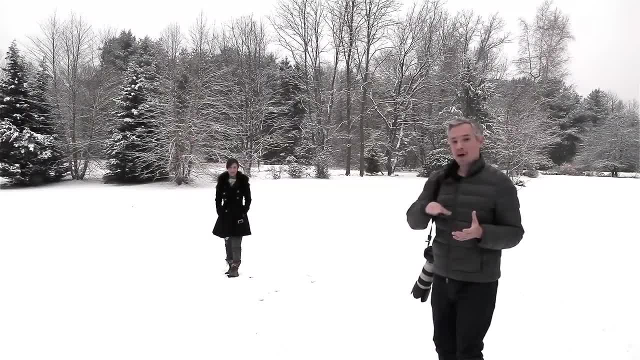 in the middle of the frame and then make that a middle gray right in the middle of the histogram. Now in the olden days you'd even hold up a gray card and meter off of that gray card and you'd feel pretty good about it. But it doesn't work well in an 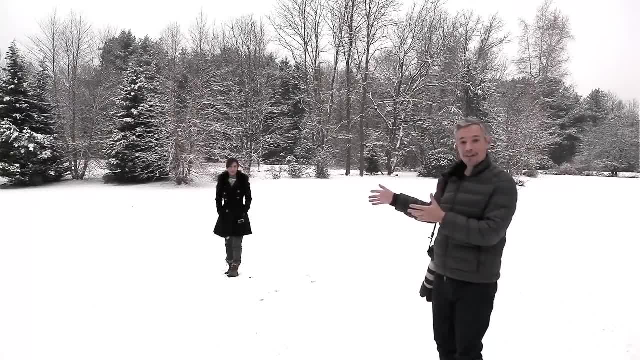 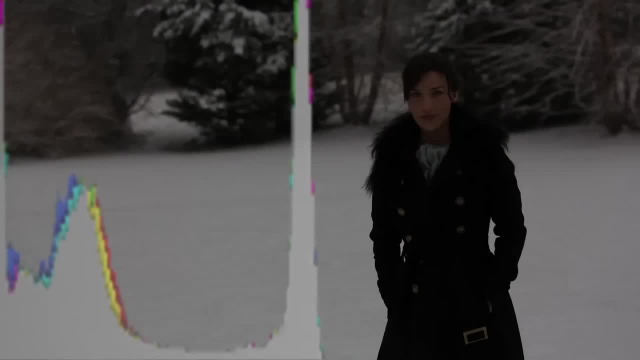 environment like this, where everything is white. You see the snow. I don't want it to appear gray, but that's the way it appeared in the first shot. I want the snow to appear white because that's how it looks. to my eye, It should be almost all the way to the right. 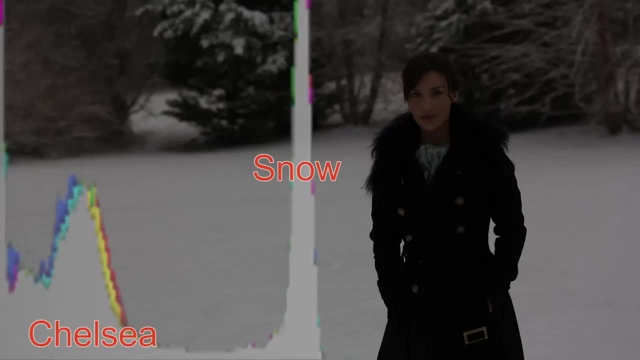 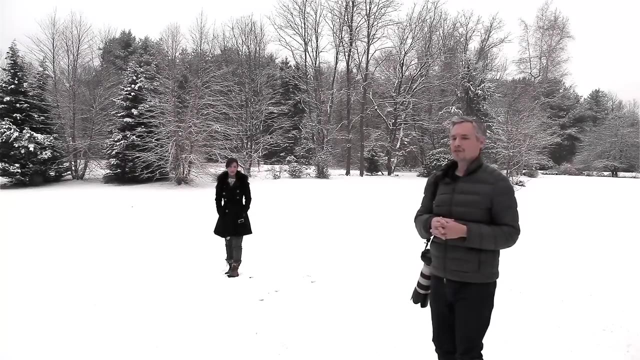 side of the histogram. This exposed it, and that's why I had to adjust it with exposure compensation. Now another way to fix that, besides using exposure compensation, is to use spot metering. Now, many cameras have different types of spot metering. They might call it center weighted or partial metering. 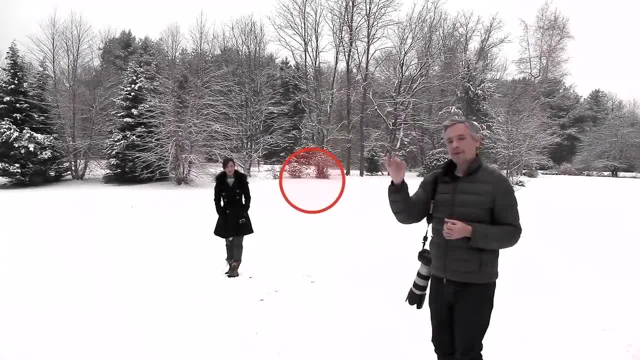 True spot metering takes a very small part of the frame and meters off of just that. Sometimes it's linked to the focusing point, but usually it's right in the middle of the frame. So I'll take a shot with spot metering on and 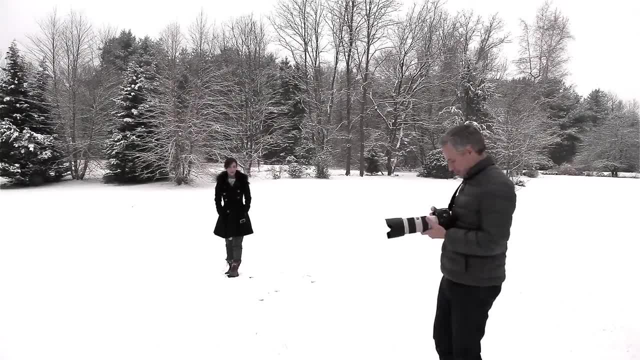 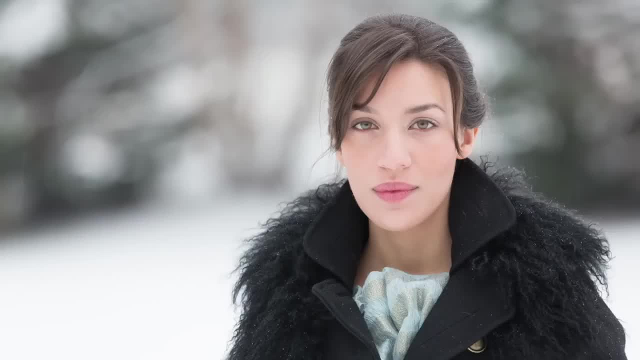 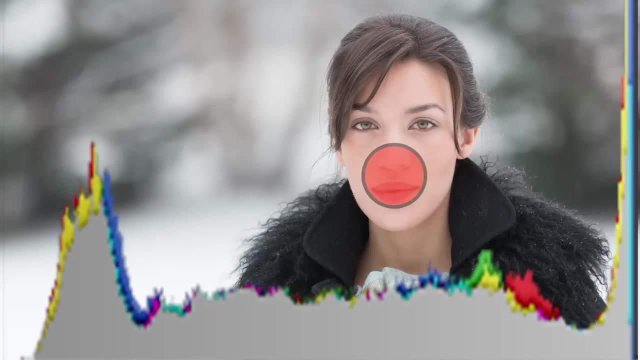 no exposure compensation and we can see how that works Now. you can see in that shot I metered off of Chelsea's face which, because of her darker skin tone, is about what middle gray should be. The background is brighter So the camera actually adjusted the exposure. so where I put the spot metering sensor would be in the 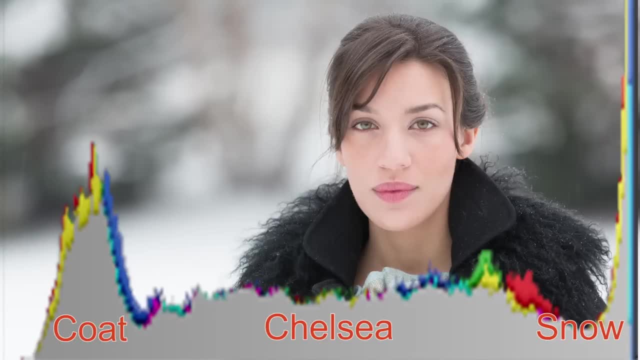 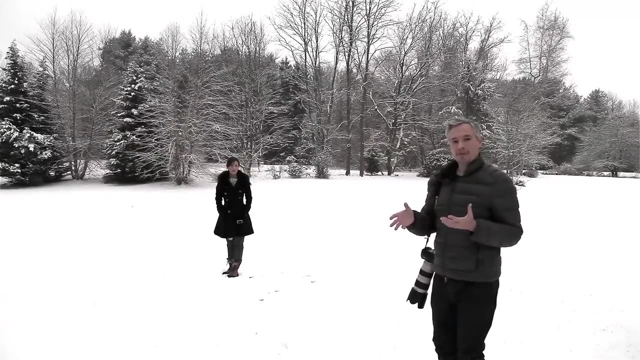 middle of the histogram. The snow, being brighter, ended up on the right side of the histogram for a perfect exposure. I don't really like spot metering, though. First, it works differently in different cameras, so you really have to learn how your camera works and experiment with it to get it to. 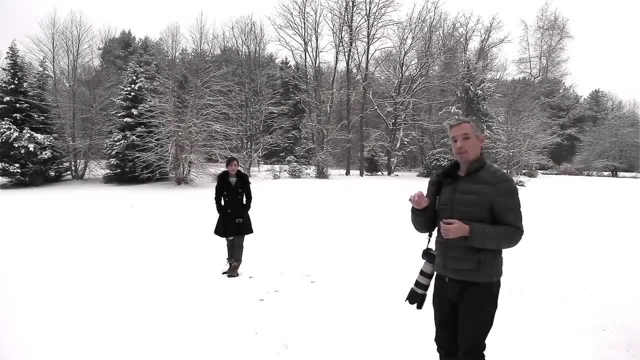 work right. Second, it meters off of a very small part of the picture and with moving subjects where this might be particularly useful, it's really easy to move to a dark or light part of the subject. So, for example, I try spot metering with flying birds- What? 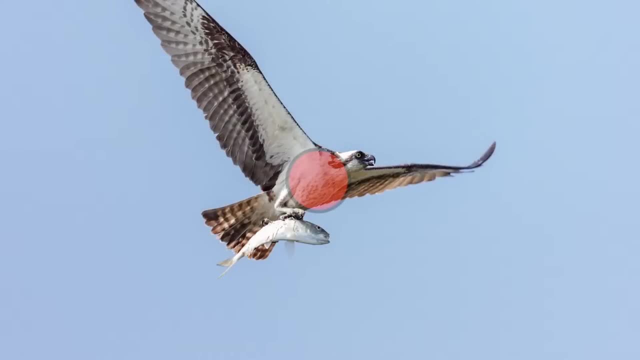 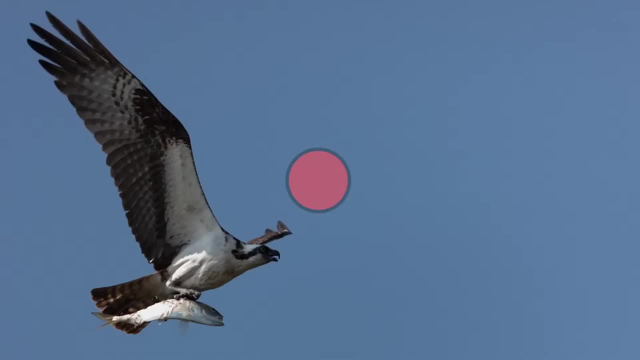 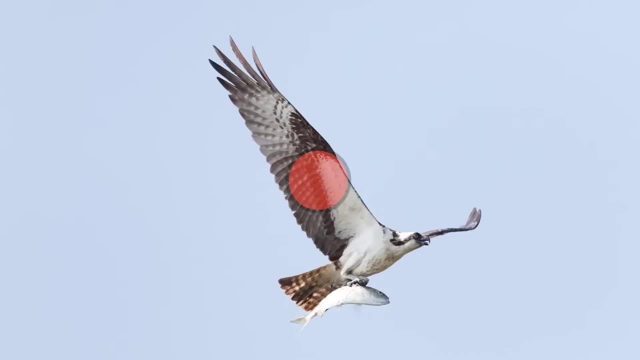 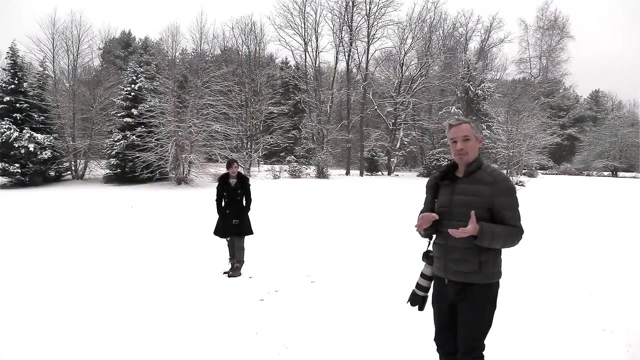 to make the sky grey, Maybe then meters off of a dark part of the bird, and it moves the exposure way up. Now I'd like to illustrate what happens when you have a dark background. So let's take Chelsey and move her in front of some dark trees, and we'll repeat this experiment, This. 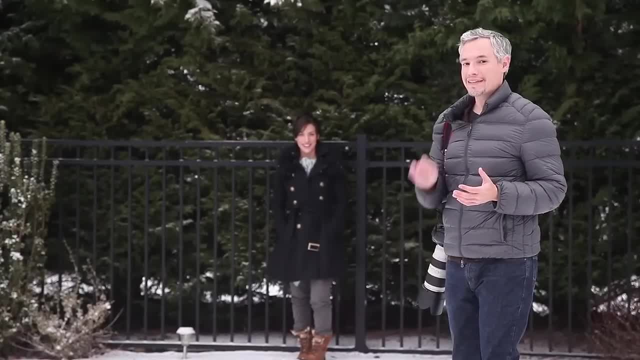 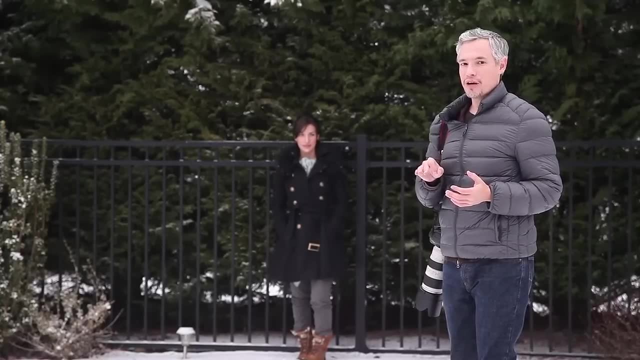 isn't the most scenic spot for a portrait, but it will serve for an example here because it's got a nice dark backdrop. Now I'm going to take this photo again, but I want to remind you to please read through chapters 3 and 4 in Stunning Digital. 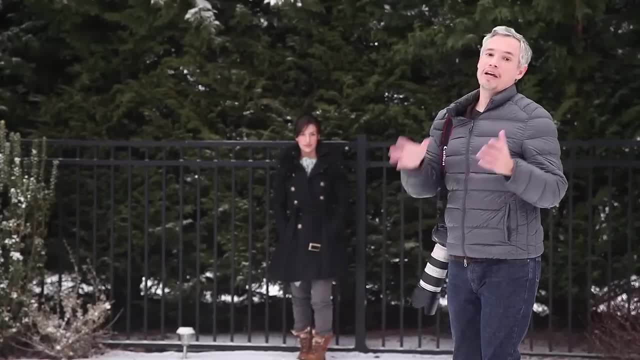 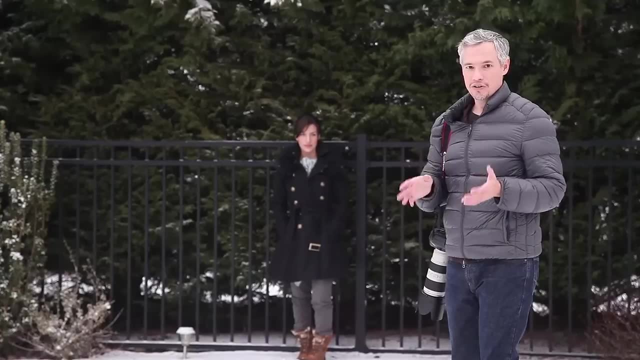 Photography because it has a ton of detailed information about exposure and the exposure square, which includes aperture and shutter speed and all the camera settings that you need to understand to be able to work it properly. So, with my camera set to evaluated metering and no exposure. 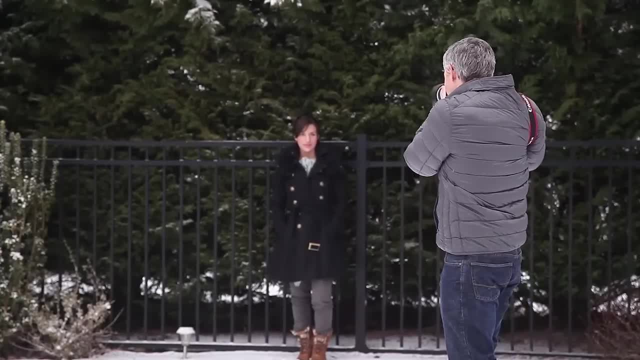 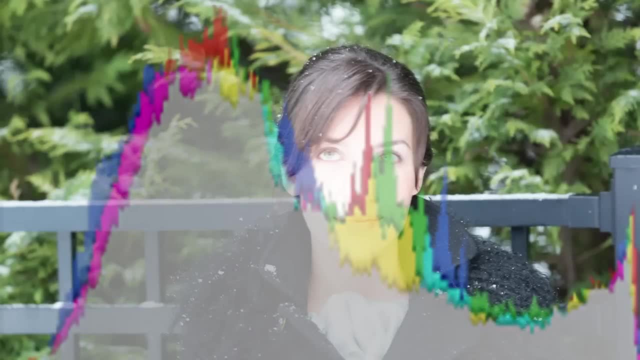 compensation. I'll take another sample shot. If you look at that, Chelsea's face is now overexposed and the reason for that is the camera included the dark background in the metering and it tried to bring the background up to middle gray. Chelsea's face is now brighter than the background, meaning it pushed that. 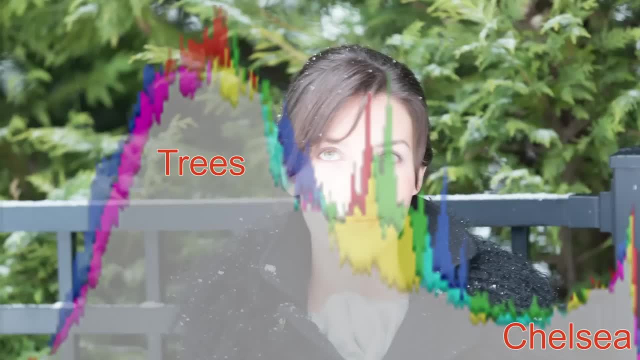 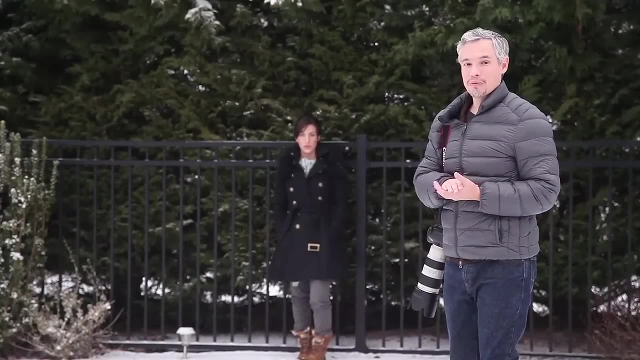 exposure up beyond the right side of the histogram, causing it to be blown out. Now it's really easy to detect if you look at the preview and you enable blinkies, which I described in the book. So because I could see it blinking, I immediately knew that I needed to adjust the exposure compensation. 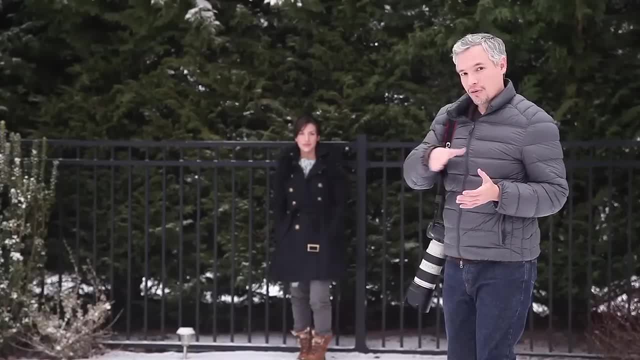 down here. So I'm going to go ahead and do that. So I'm going to go ahead and down. I can also look at the histogram, and if I see the histogram climbing up the right side there, that means I need to dial down one or two stops of. 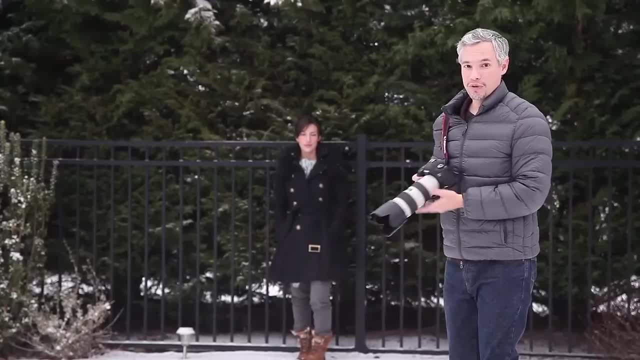 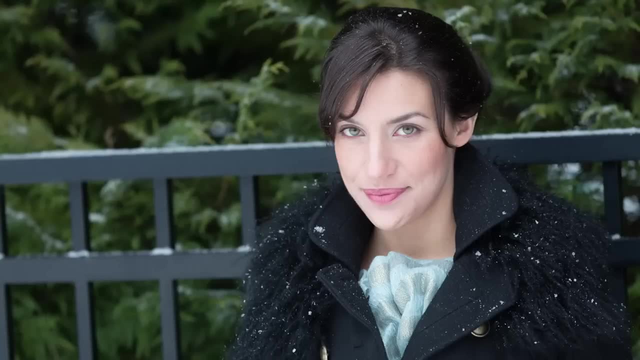 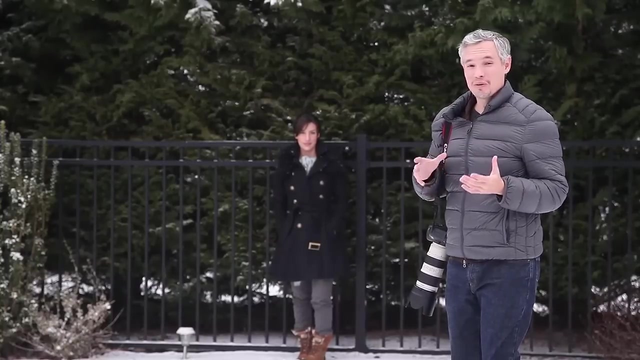 exposure compensation. So I'll just dial in a couple of stops and retake that picture. That was enough to fix it. So remember, when you have a bright background you need more light. If you have a dark background, dial your exposure compensation down. It works exactly the opposite of the way you. 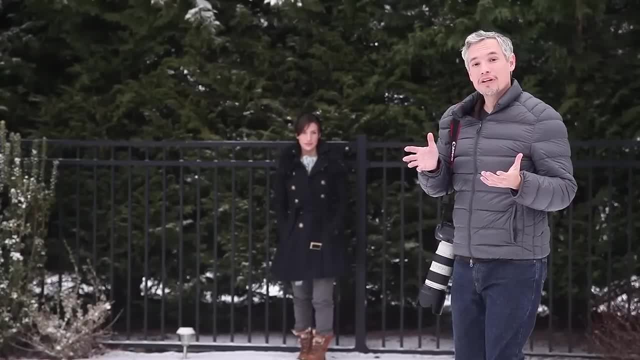 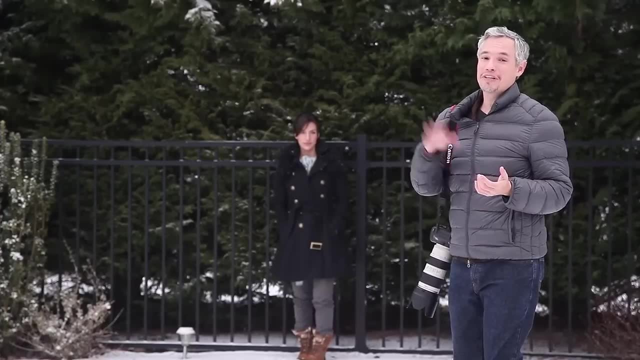 would think it would. But you don't need to memorize anything. All you need to remember is look at your picture after you take it and examine the histogram, Then adjust the exposure compensation, even if you get it backwards. you'll figure it out after you take your next test shot. Now we'd like to talk a little. 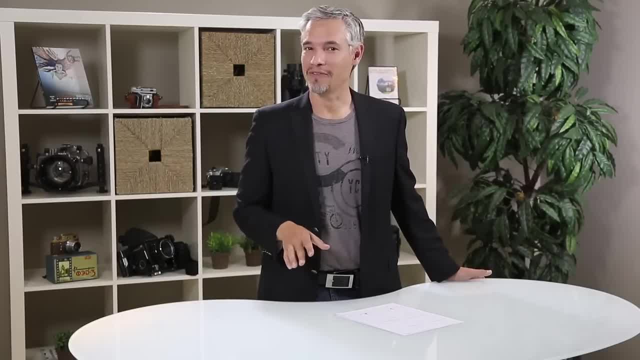 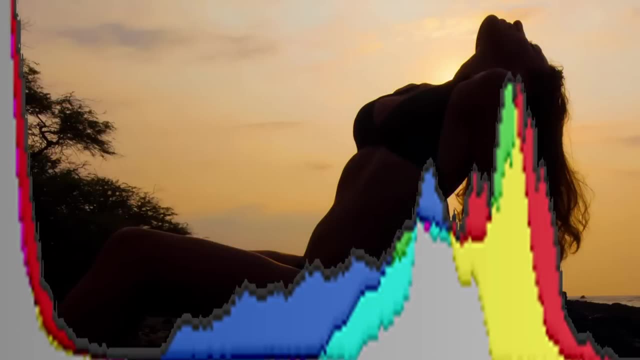 bit more about histograms. I mentioned them a little bit in that video, but I want to go into a little more detail. The histogram is basically the bar chart that visually represents the brightness of your picture, And if it has a bunch of detail over in the left side of the picture, that means that there's a bunch. 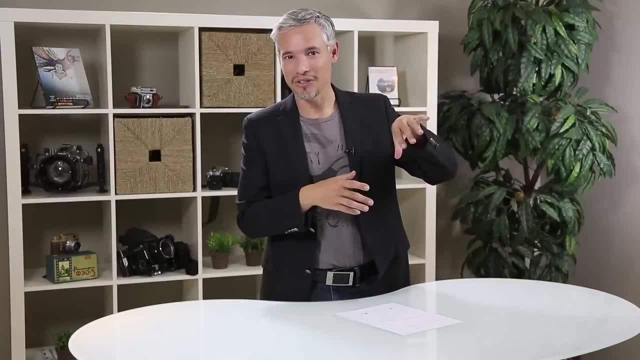 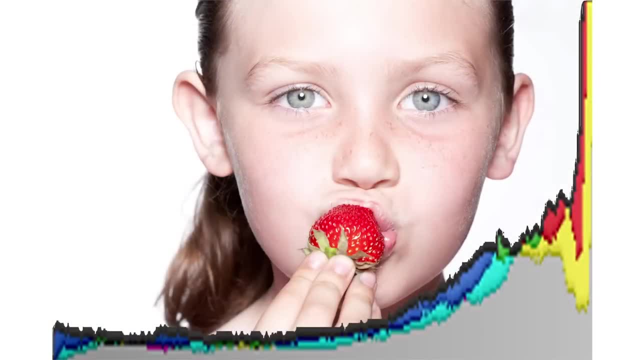 of dark In your picture and if it has a bunch of detail on the right side of the picture, that means that your picture is kind of bright. So let's look at some sample photos. This is a high-key photo of my daughter eating a strawberry, and by 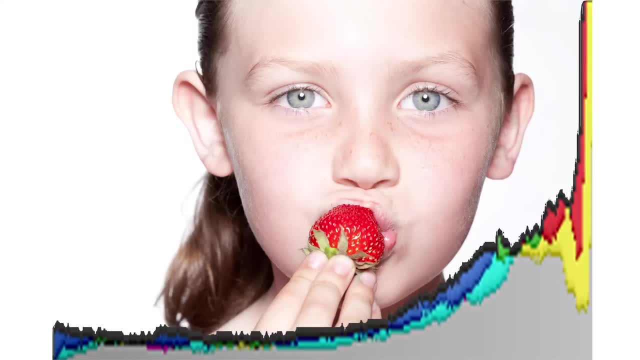 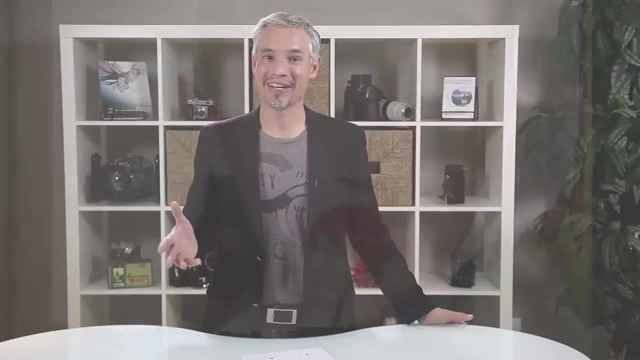 high-key. I mean it's mostly white. When we look at the histogram, we can see that the histogram is creeping up the right side of the picture. That's because the picture is bright and it's mostly white. Anything that's completely white in the 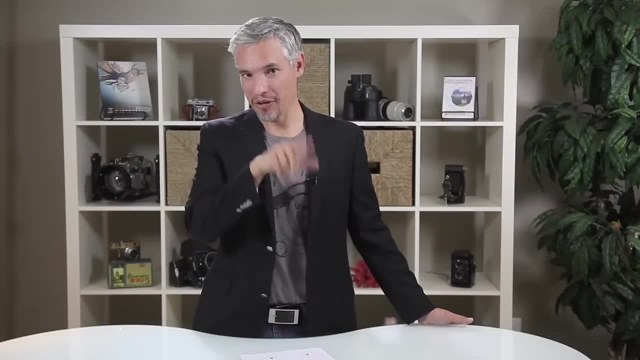 picture is gonna cause the histogram to touch that very right side. That means it's a little bit overexposed. With this photo that overexposure was done deliberately. Now you can look at the histogram alone and see that this picture doesn't really have any areas of black, of darkness, And though I did it. 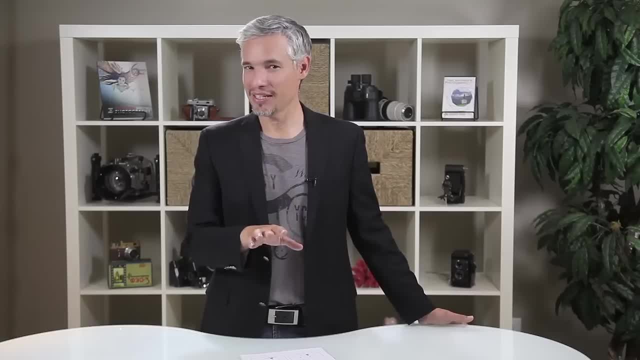 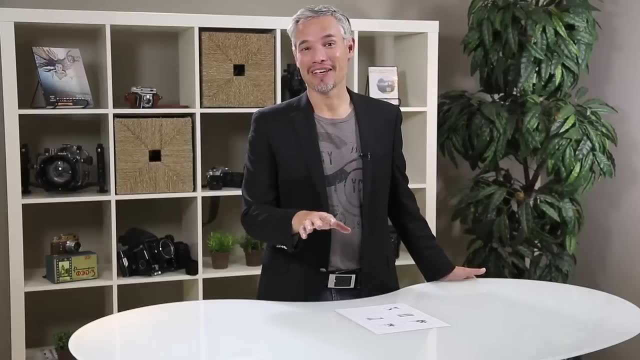 deliberately this time. usually that's something you want to avoid, And if you were to see a histogram that looked like this, you probably use your exposure compensation to drop it down a stop or two. This picture of a sunset has an extreme dynamic range, because I'm shooting right into the sun. That's the 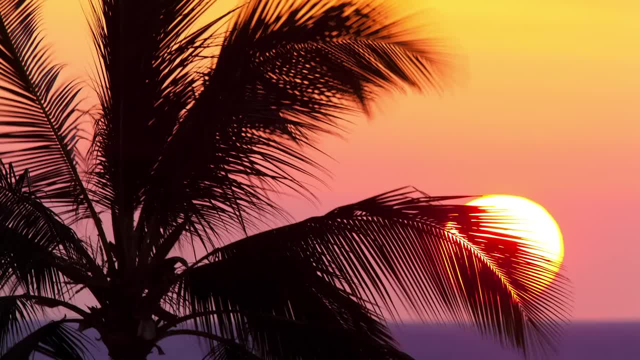 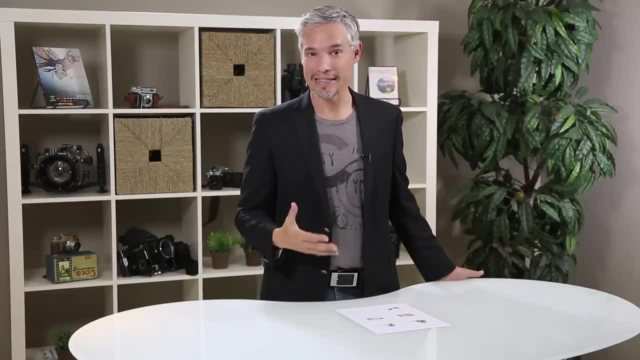 brightest thing in our solar system. There's nothing that's gonna be any brighter than that. And those palm trees in the front are a perfect silhouette, and they form a silhouette because the camera couldn't capture any detail in those shadows. As we look at the histogram, what we see is that the histogram is climbing up the 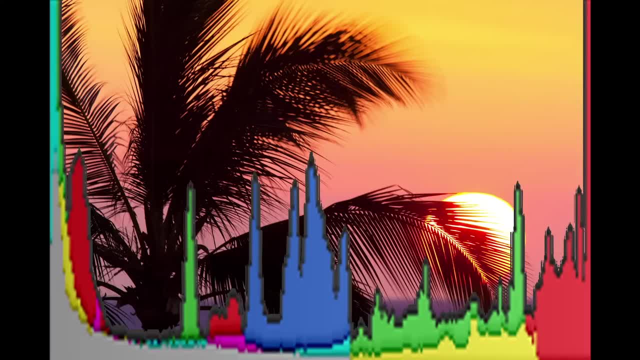 right side, where the Sun has overexposed in the picture and all the shadows of the palm trees are on the left side. Now we do see some detail in the histogram in the middle there, and that's because there are some parts of the sky that are 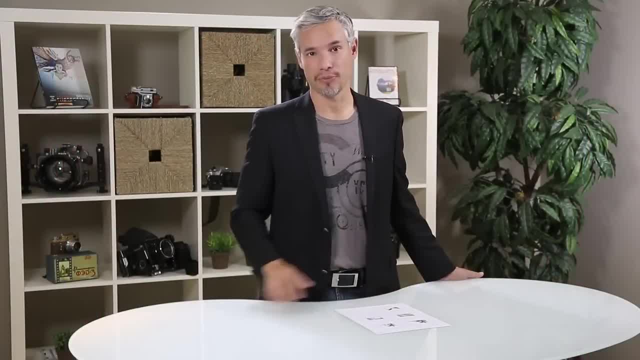 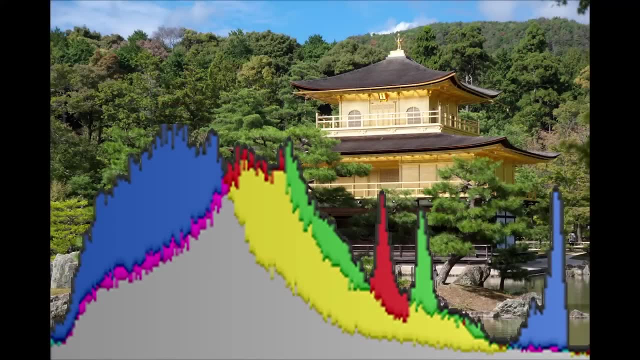 properly exposed that the camera was able to capture in the camera The camera's limited dynamic range. Now let's go to Japan and look at the Golan Temple. This scene had a very reasonable amount of dynamic range and therefore, when I took a picture of it, the camera was able to capture the entire dynamic. 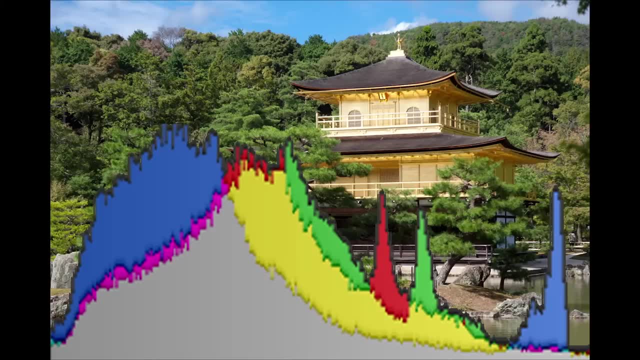 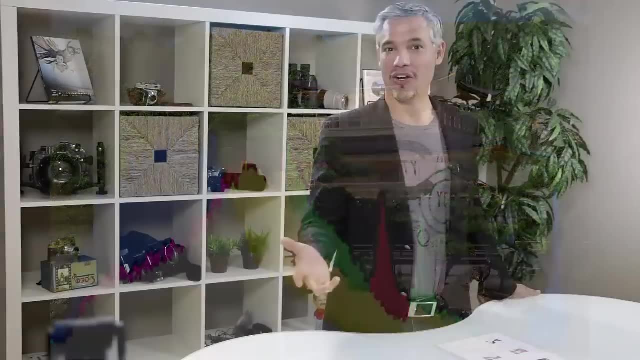 range. As we look at the histogram, we don't see anything creeping up the left or right sides of the histogram. That means the picture is well exposed. This particular scene wasn't challenging at all, and in fact I could just rely on the camera's auto exposure system. Here's another picture with an extreme dynamic. 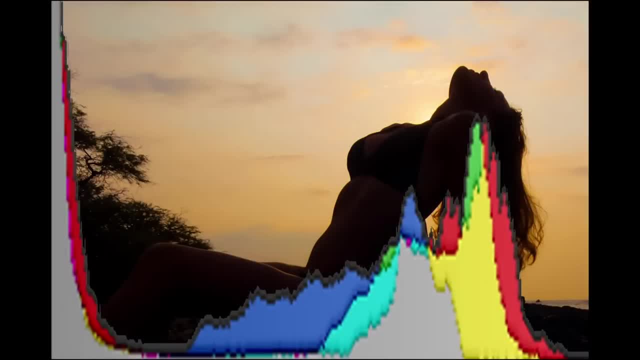 range. This is another sunset picture. I'm shooting right into the Sun and my subject in the foreground is forming a complete silhouette because there's no front lighting on her. You can see from looking at the histogram that the sky itself is well exposed, but the foreground subject is almost completely. 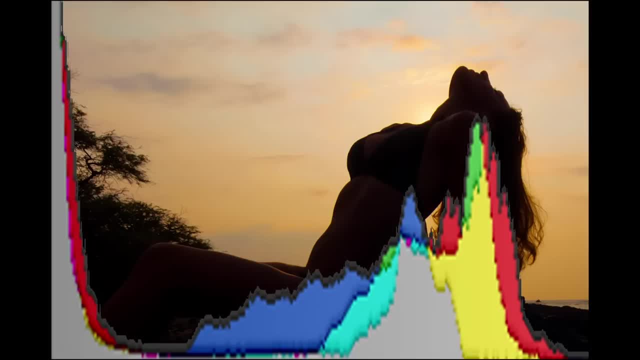 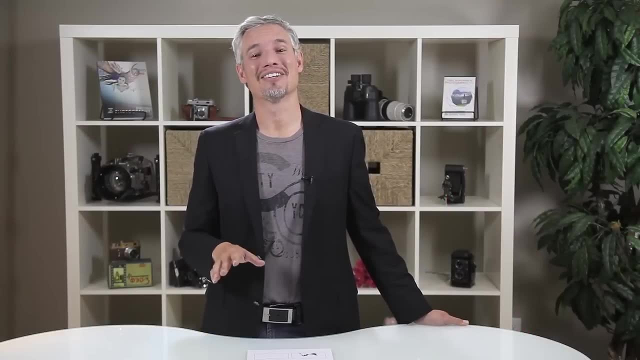 black. That's why that histogram is creeping up the left side of the picture. That relates to the darkest parts of the picture. Now, in this case, I was going for a silhouette. That's what I wanted, So I didn't have to adjust the camera's auto. 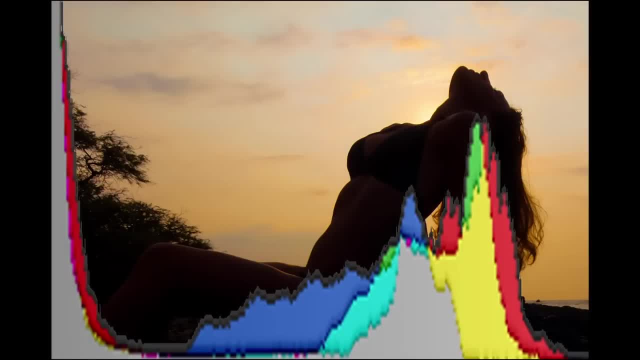 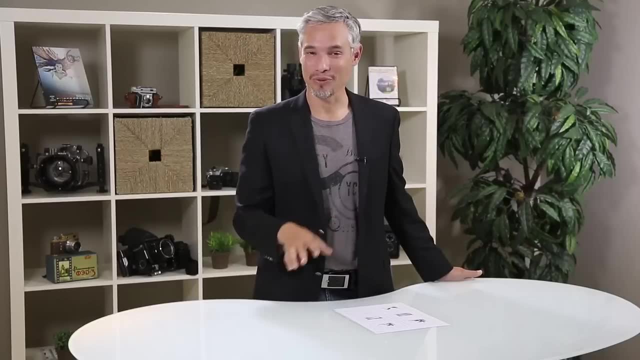 exposure any further. but if you wanted to properly expose the foreground subject, you'd want to add several stops of exposure compensation. Now let's head into my pool room in the basement where I've set up a couple of items so that we can experiment with different camera modes, including manual mode, and 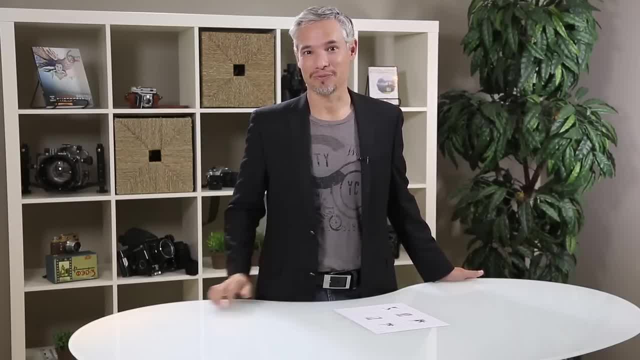 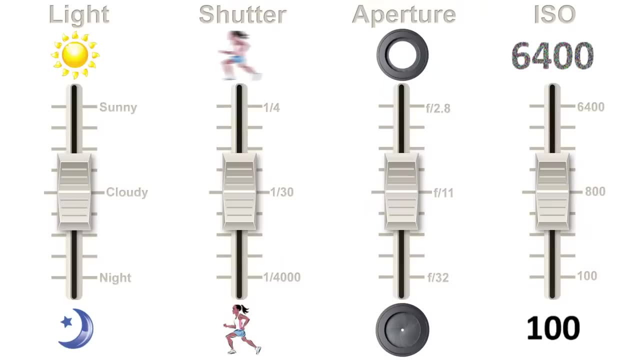 different settings for aperture, shutter speed and ISO. I'd like to explain to you the relationship between shutter speed, aperture, ISO and light. They are all connected to each other and they're all connected to each other. So I'm going to. 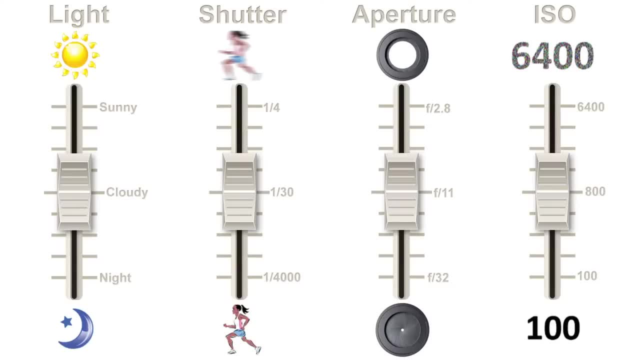 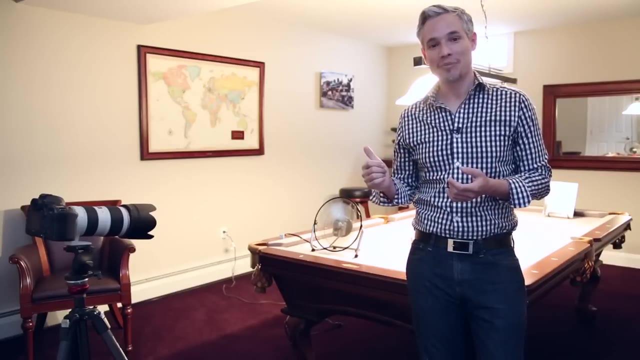 show you how to adjust the shutter speed, and adjusting any one of them can be compensated for by adjusting any other. In other words, if you make the room brighter by raising the lights, you'd have to make your shutter speed faster to compensate for it. I'm going to walk you through a series of tests with my 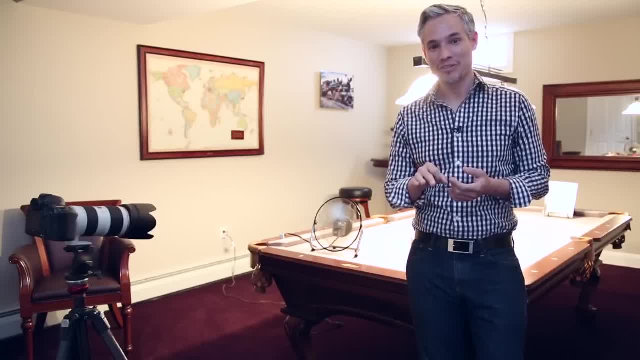 camera here and this little lab setup that I've made to show you exactly how everything works. What I'd like you to do is to watch this video from start to finish and then set up something similar in your own home. Once you get some hands-on practice with it, you'll start to make more sense. 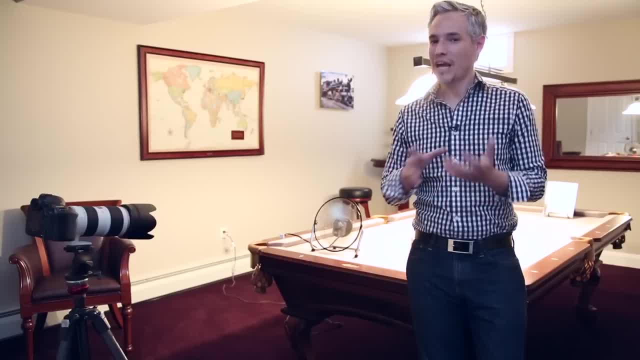 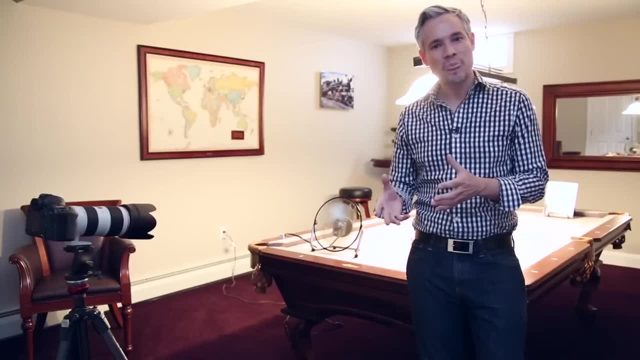 Now, understanding these is important, because not understanding them can cause a lot of problems with your photography: Shaky pictures or not getting everything in focus that you want to- and once you get an understanding of it, you'll be able to fix those problems. Noisy pictures, too. So let's get started by. 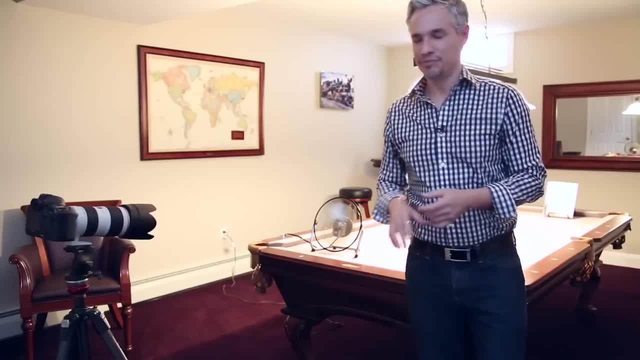 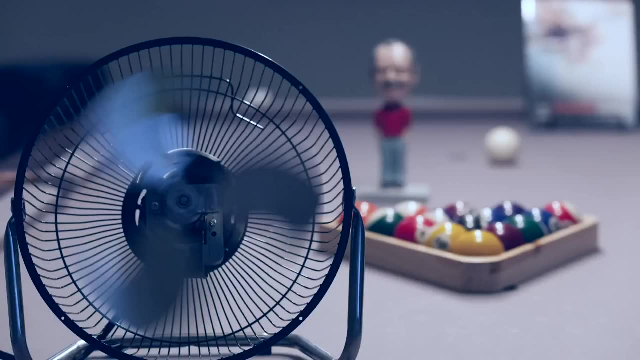 taking our first picture on totally automatic mode. The mode I'm using now is the program mode, which is P1. P on most cameras and it lets the camera make all the decisions for you And if you're ever unsure about the settings or you're giving your camera to, 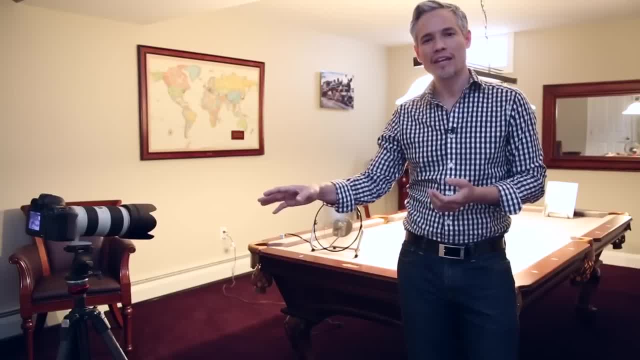 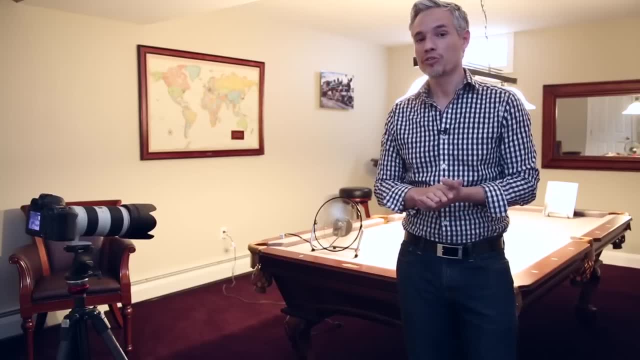 somebody who isn't a competent photographer, set it on P mode and it'll take care of everything for you. It's a great way to go when you're feeling a little bit nervous about your photography. However, for those of us who master shutter speed, aperture, ISO and light, it's a mode that you won't ever. 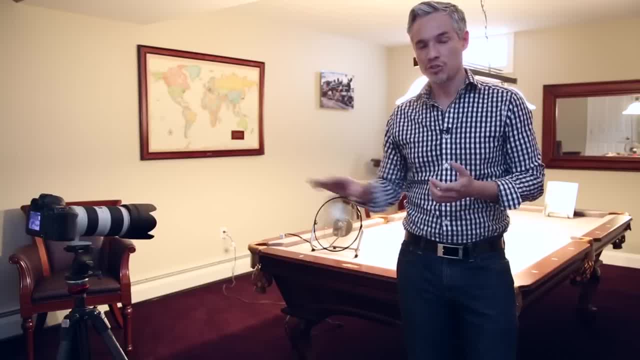 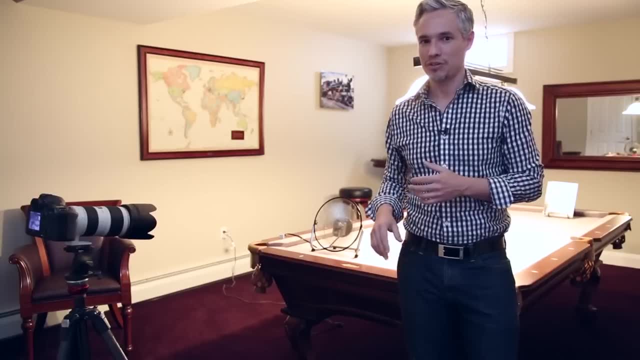 want to use, because you'll always want to be able to control those conditions. So you can see, the camera does just fine. What I'm going to do now is to cut the lights in the room by about half and I'll take another picture. 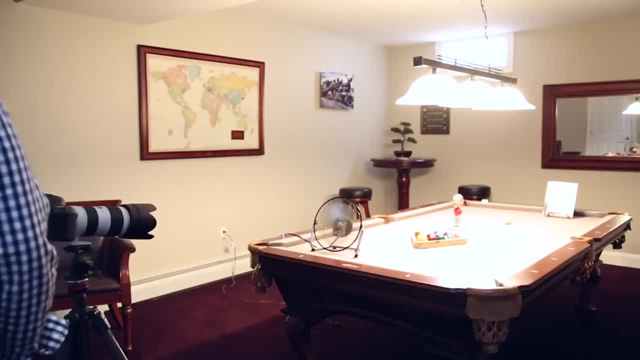 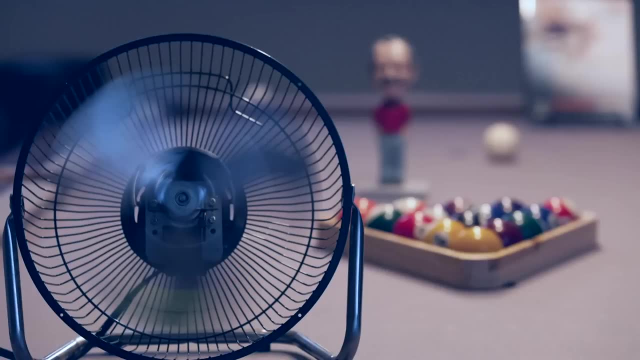 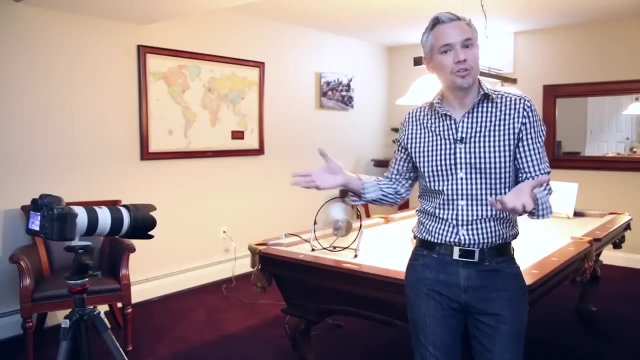 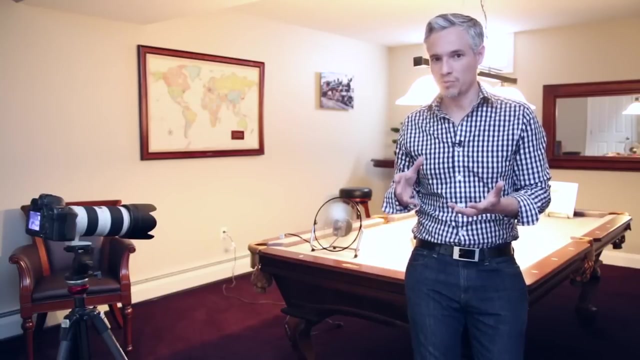 Now, as you can see, the exposure didn't really change between those two pictures. The brightness of the picture is exactly the same and that's because the camera auto exposed it. It looked at the light in the room and adjusted the ISO aperture and shutter speed in order to get a well exposed picture. However, those had a side. 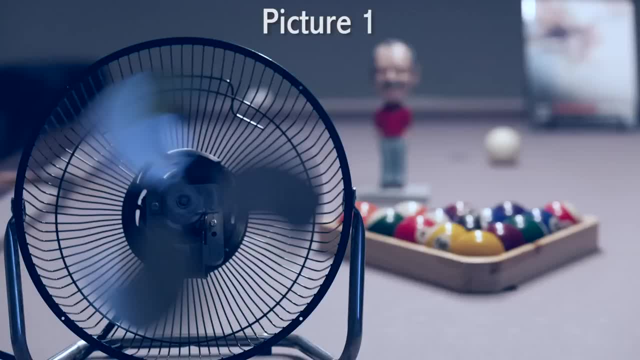 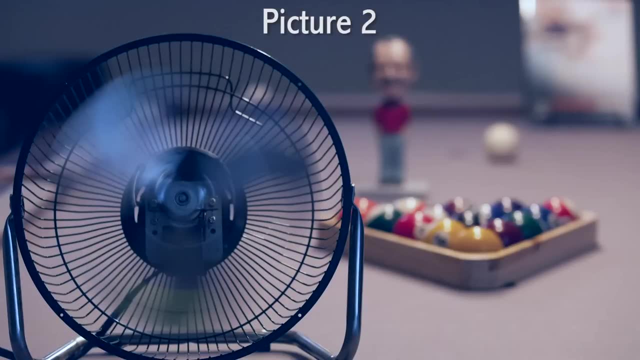 effect. As you'll notice, the fan is a little more blurred than it was in the previous picture, and that's because it had to use a longer shutter speed to expose the picture properly with even less light. That's one of the reasons you need to understand these, because you might or might not want that extra blur. 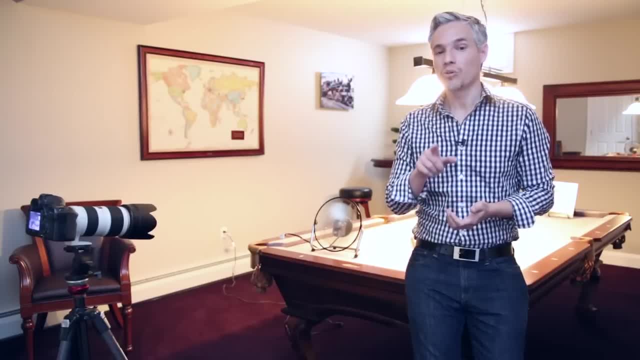 in there and you do have total control over it. Now you also notice that the brightness didn't change, and a lot of people think they can change any one of these settings and it will adjust the brightness of the picture in automatic mode. It's not true. 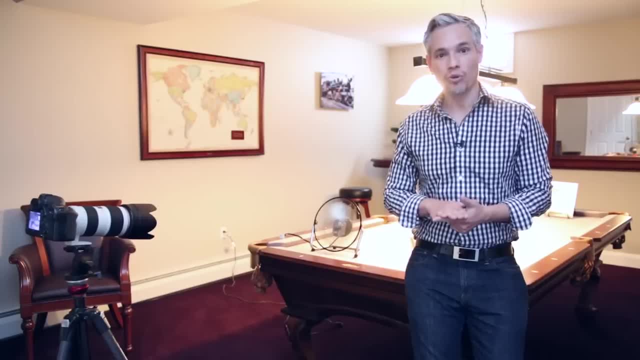 You can adjust the brightness of the picture in automatic mode. It's not true. You can adjust the ISO or the shutter speed, or the aperture or the light in the room, and the camera is always going to adapt to it. So, changing any of one of 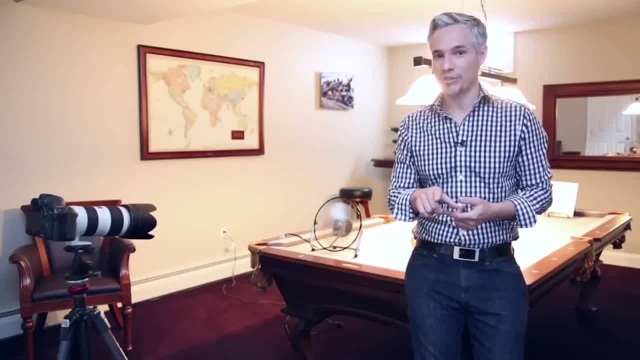 those won't change your brightness. If you want to change your brightness, use exposure compensation, and on most cameras that's controlled with a dial on the back, Though sometimes you need to press an extra button or go into a menu system. So, just for an example, I'm going to add a stop of exposure compensation. 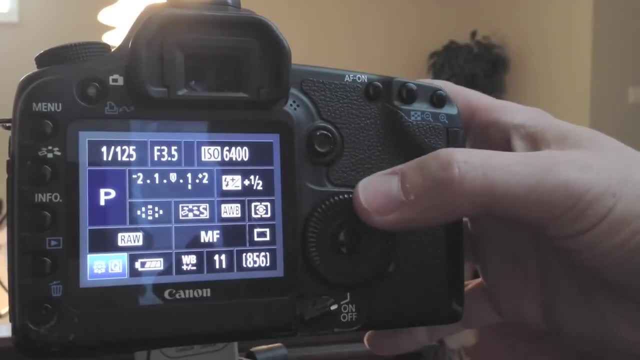 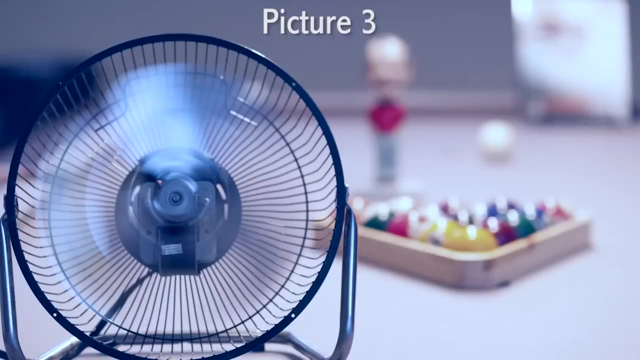 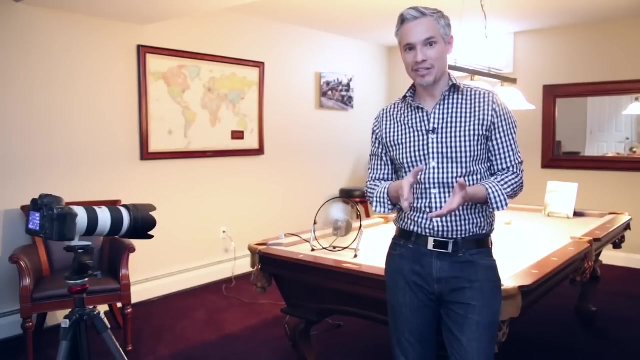 so we can see the difference. As we can see there, the picture did get brighter. It got one stop brighter, to be precise, because I adjusted the exposure compensation by one stop. Now a stop in photography is a doubling or a halving of the light If you double the. 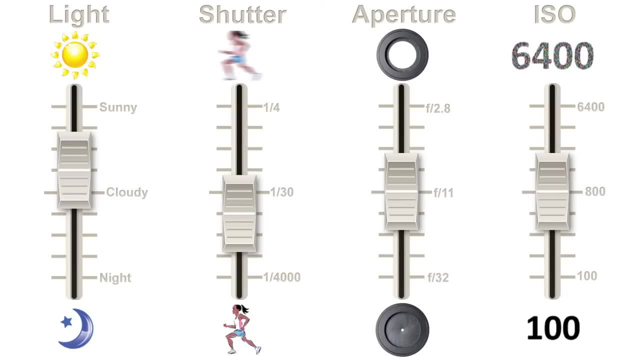 amount of light in room. you've added one stop of light. If you cut the shutter speed in half, if you go from 1 to 50th of a second to 1 500th of a second, you've increased the shutter speed by one stop. Now I'm going to move the camera. 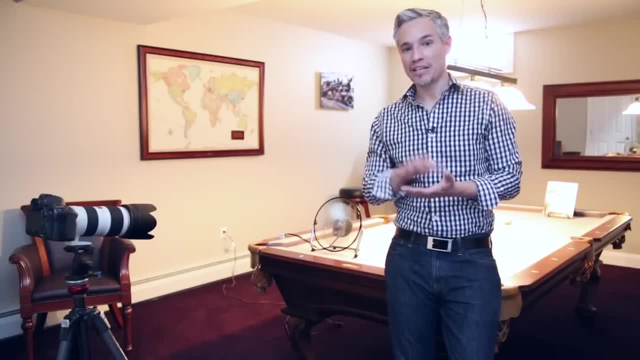 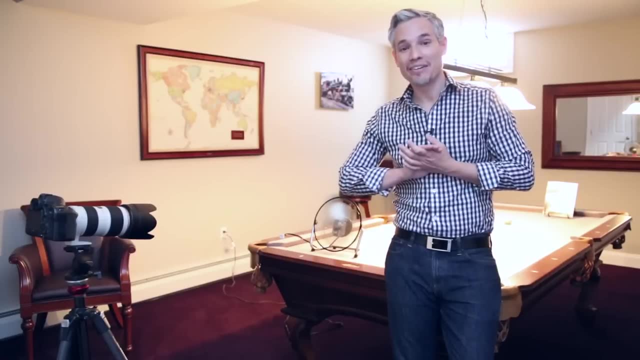 into manual mode, whereas the ISO, aperture and shutter speed were all unlocked so that the camera could adjust any of them when I have it in program mode. In manual mode, I can lock down everything and prevent the camera from making any automatic decisions. It gives me complete control. So that's what. 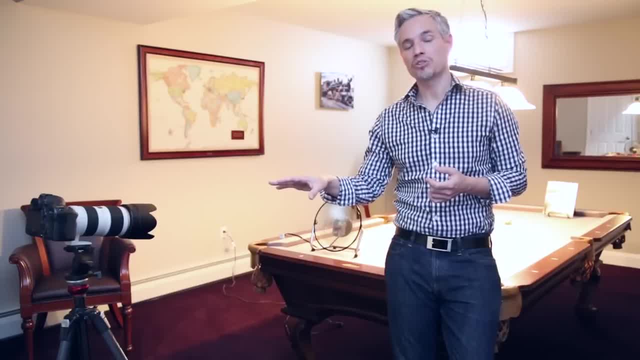 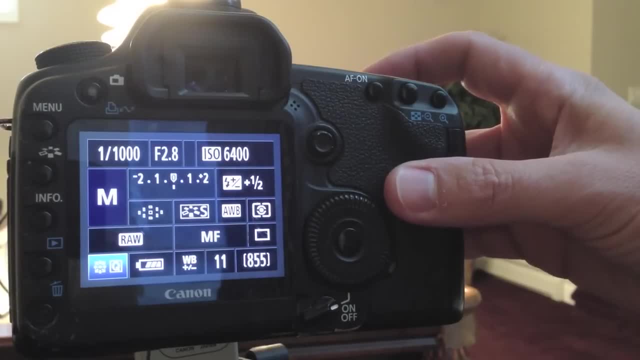 I'm going to do, and I'm going to set it in manual mode and then configure it so that it will expose the picture properly and we'll take a test shot. What I did there was I set the camera to manual mode, a shutter speed of 1 1,000th. 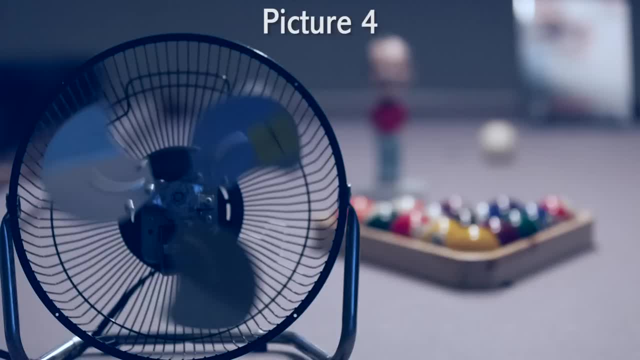 of a second, F28 and ISO 6400.. Those settings together allowed the camera to expose the picture decently and you can see that blade of the fan is just about frozen, because 1 1,000th of a second is pretty fast. You can also see that the 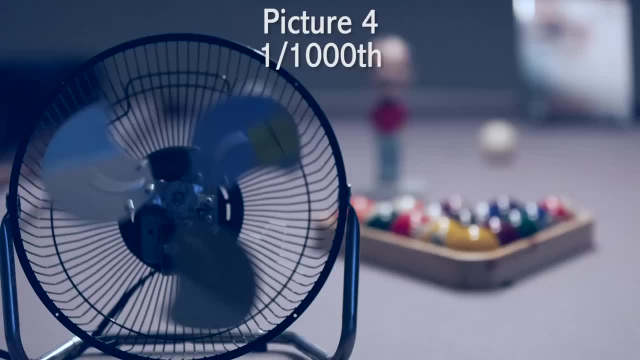 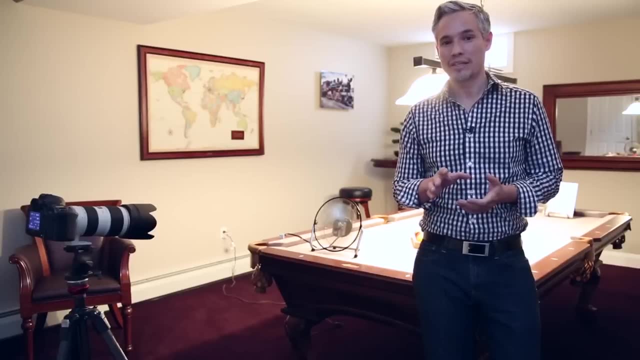 objects in the background: my dad, the cue balls and my book. they're all pretty well blurred. You'll see in some later pictures those will get sharper and sharper. The first thing I'd like to do is experiment with changing the ISO, ISO. 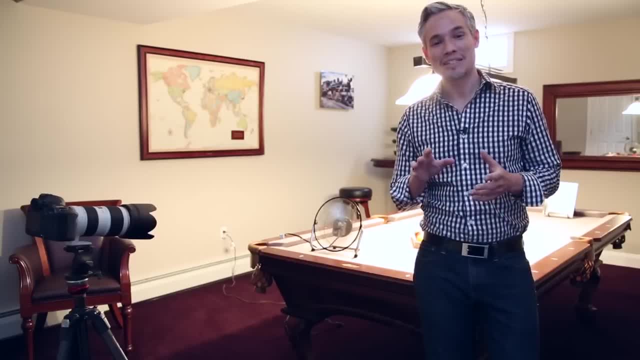 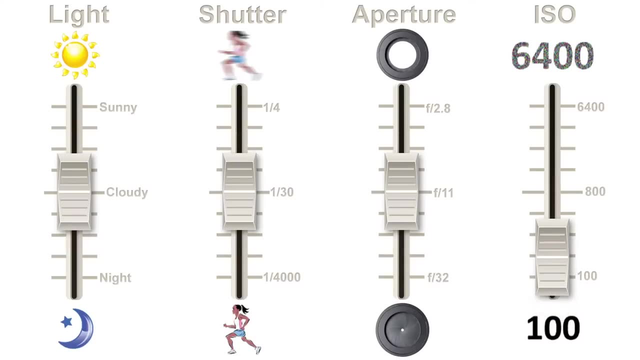 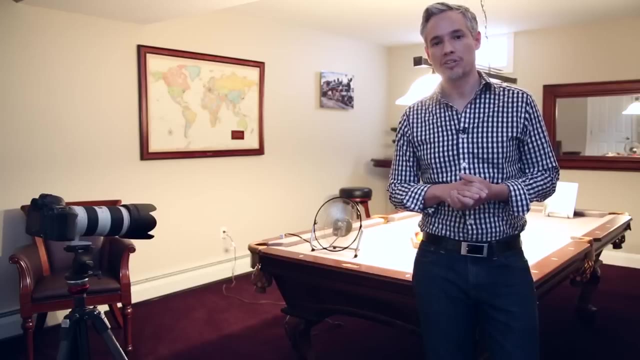 which, by the way, is not an acronym. You can look it up. ISO is the sensitivity of the camera's sensor. If you increase the ISO from, say, 100 to 200, you're increasing the ISO one stop and that's doubling the sensitivity of the sensor. The typical usable range. 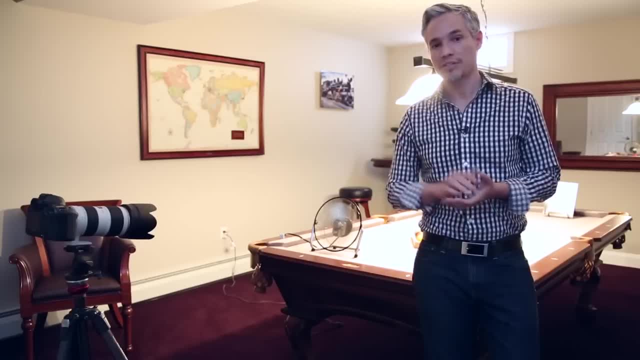 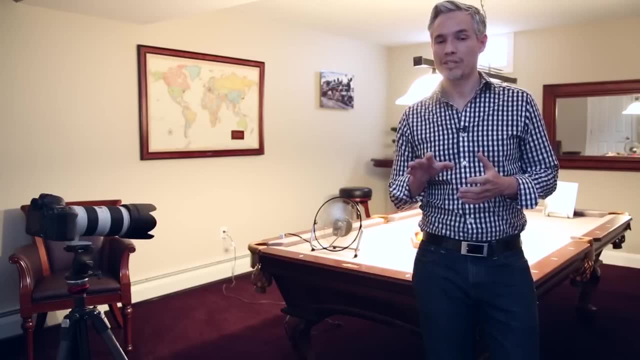 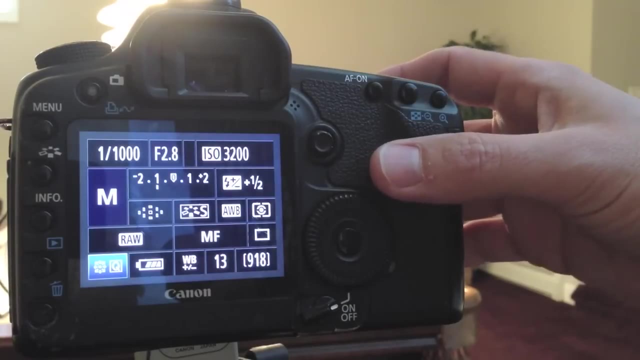 goes from about 100 to 6400.. So this was at 6400, which is a pretty bright ISO, because this room is pretty dim. So I am going to drop it down to 3200 and we'll see the effects. As you can see, the picture got darker. As your ISO gets lower, the camera gets. 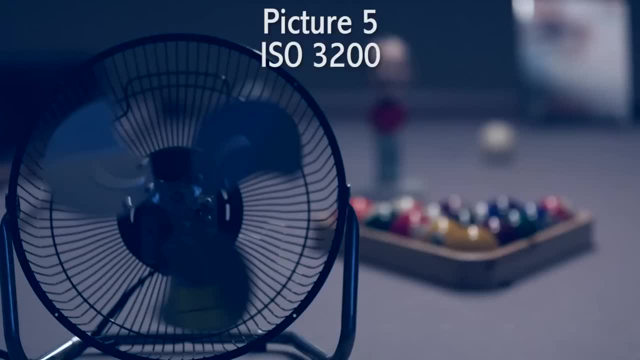 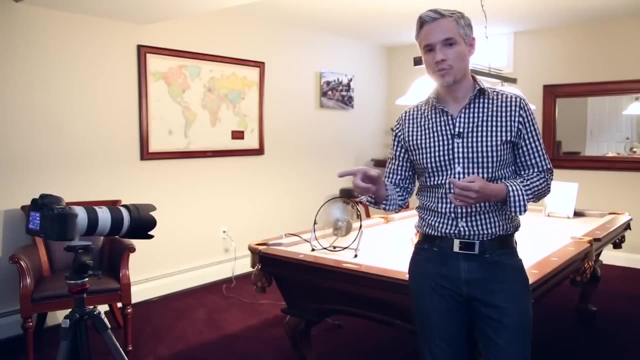 less sensitive, and if you don't let the camera adjust the other elements- the aperture or the shutter speed- automatically, then the picture is going to get darker. So let's move the ISO up two more stops to 12,800, and see what the 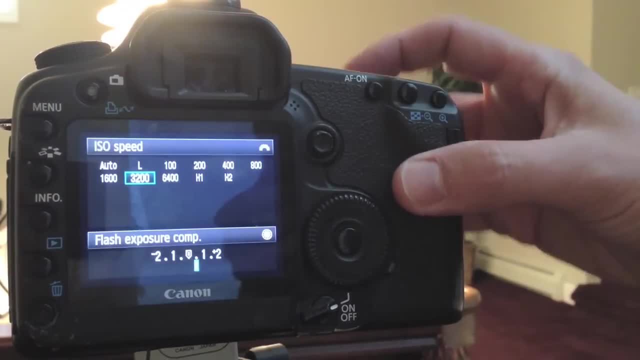 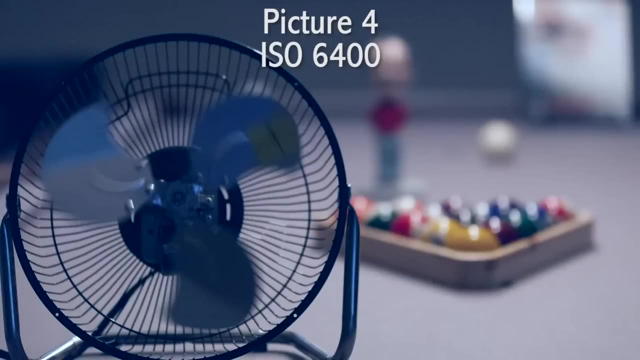 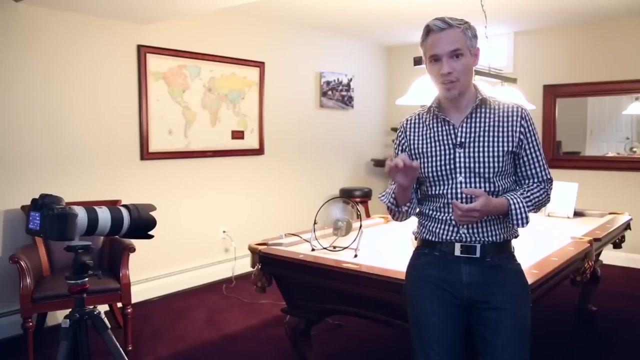 effect is, As you might have guessed: the picture got brighter because we increased the sensitivity of the camera without changing any of the other settings. Now we've been in manual mode, where we locked all of the settings except for the one that we were controlling Now. 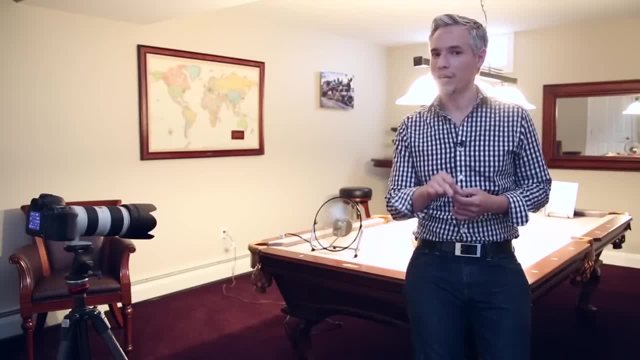 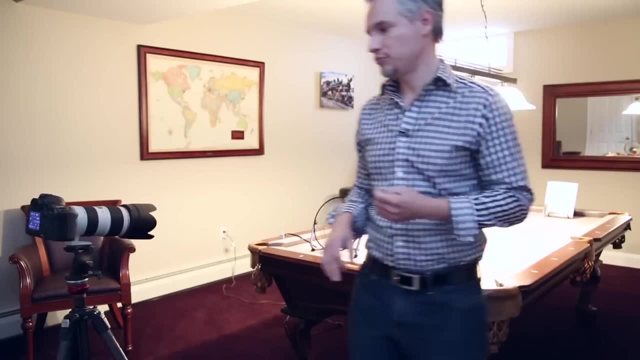 I'm going to switch back to program mode, which will make everything but ISO automatic, And I'm going to take a couple of shots at different ISOs so you can see the effects. You can see here that the ISO is a little bit lower, So I'll just move it up a little. 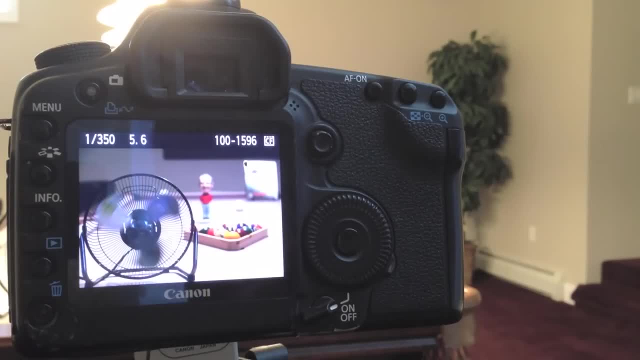 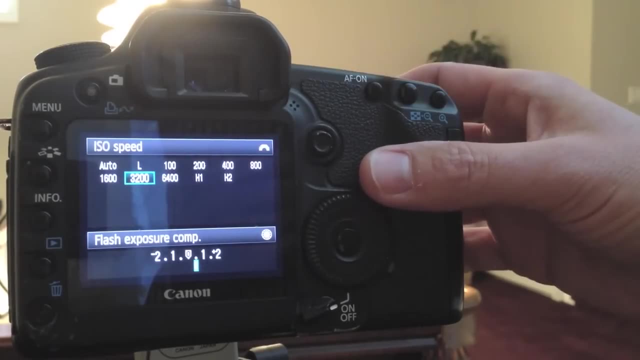 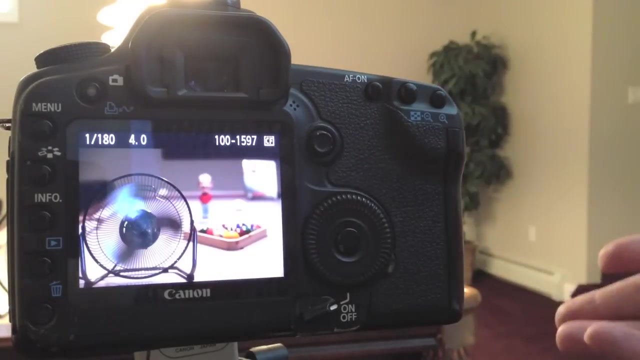 bit. You can see here that the camera exposed the picture at 1,350th of a second in f5.6 and it was well exposed. Now I will drop the ISO to 3200.. That's dropping it two stops. so the camera will need four times as much light And, as you can see, the 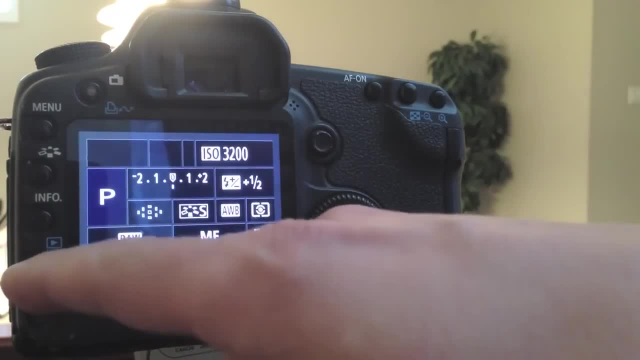 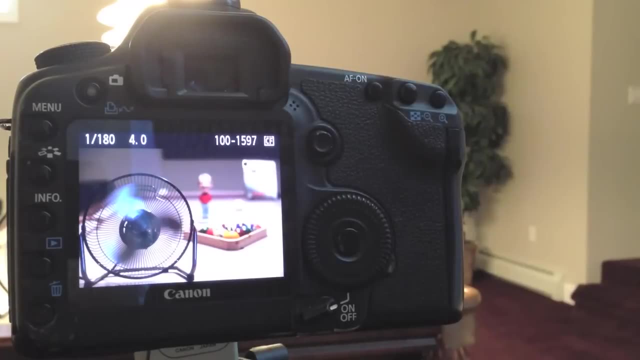 picture is still well exposed, but the camera had to change the settings to 1,180th of a second and f4,, increasing the amount of light using the other factors And, as you can see, as a result of the longer shutter speed, the blades got more blurred. 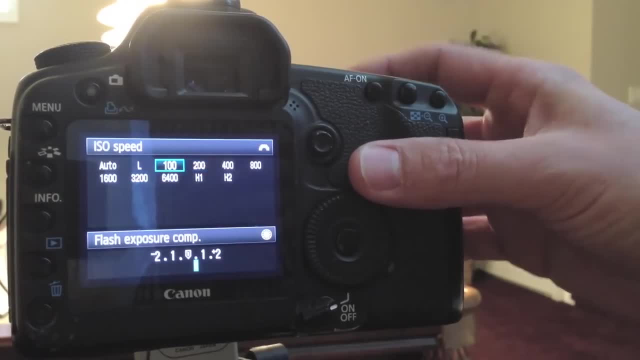 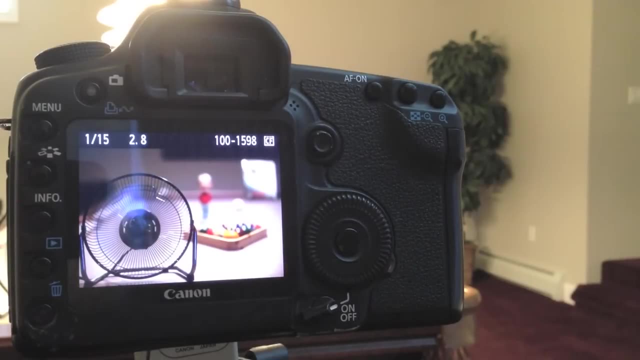 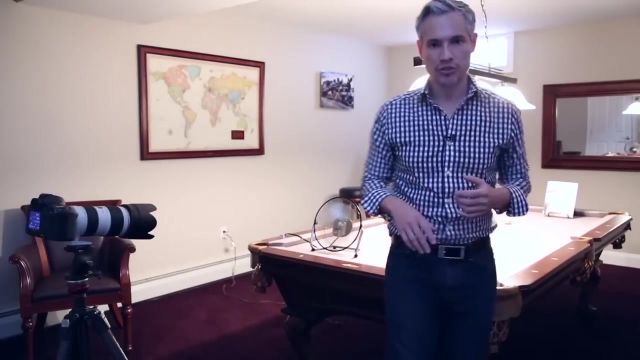 Now I will drop the ISO way down to ISO 100.. And, as you can see, because it's in automatic mode, I can change the ISO to anything and the picture is still properly exposed. But let's take a closer look at those pictures and we'll see some really important differences. 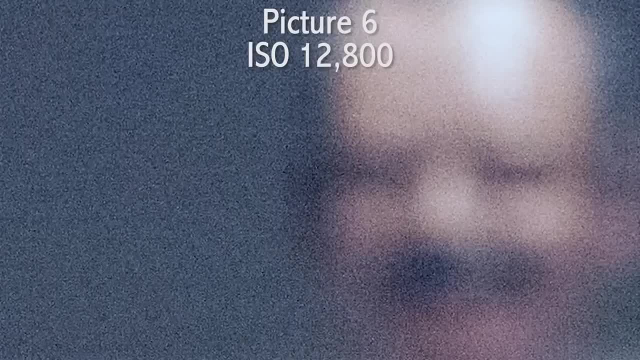 As we get really close to those pictures, we'll see that the pictures at the high ISOs are really what they call noisy, And noise is the digital equivalent of film grain, and it's not pleasant. It's something to always be avoided. Now, if you look at that ISO 100. 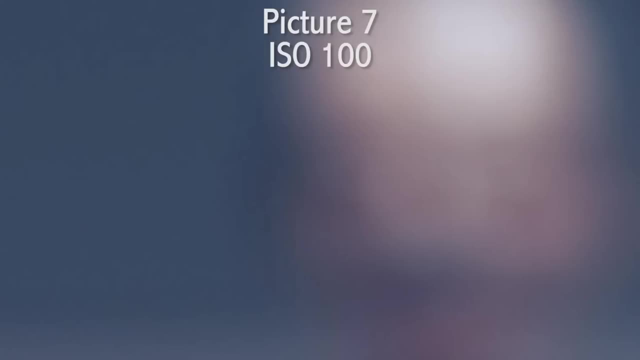 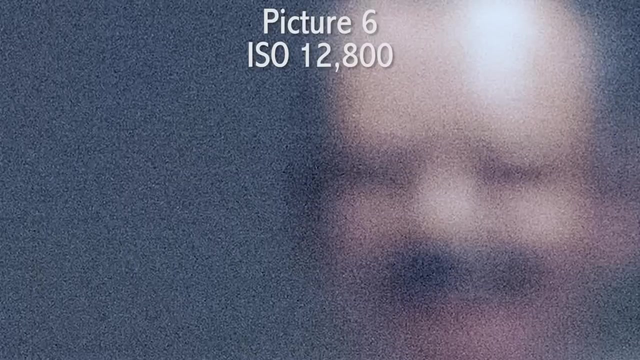 picture. you can see that it's nice and clean and beautiful. ISO 100 is almost always better than the higher ISOs, But one of the challenges of photography is that when you choose a low ISO, you're going to have to change some of your other settings, such as the shutter speed. 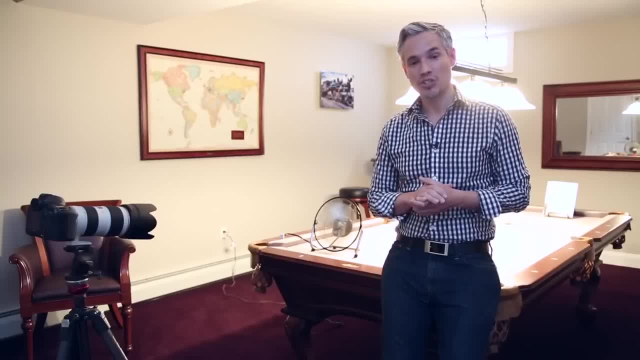 and aperture as well. Now let's take a look at the shutter speed. You can control the shutter speed by putting your camera into shutter priority mode. On almost all cameras that's marked by an S. On Canon cameras, though, it's marked by a TV. Now, when you put your camera into shutter, 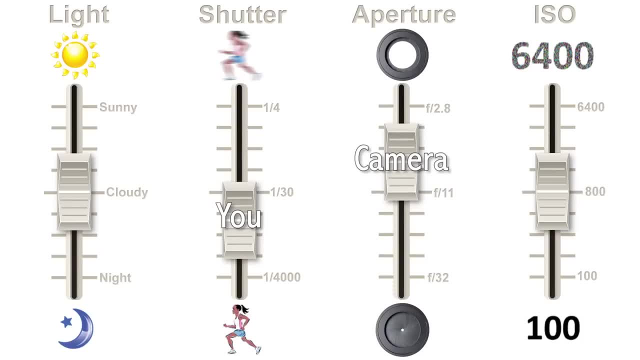 priority mode. it gives you control over the shutter so you can specify how slow or how fast you want it, And the camera will change the other settings for you, most notably the aperture and perhaps the ISO, if you have it set to auto ISO to allow the picture to be. 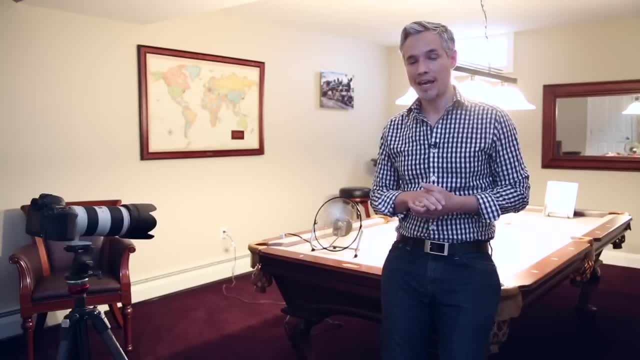 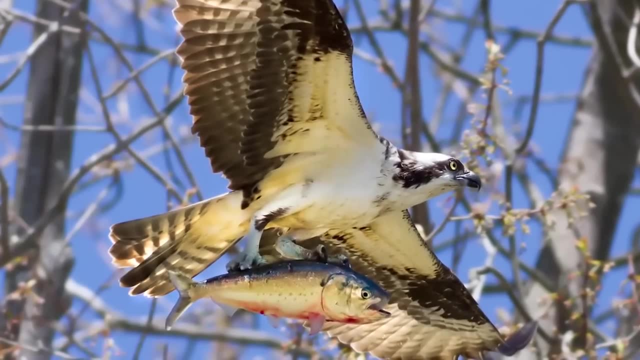 exposed properly. You want to use shutter priority mode any time. the speed of the picture is important to you. If there's a moving subject in your picture, you want to switch it to shutter priority mode. So yes, at your kid's basketball game if you're taking pictures of your dog. 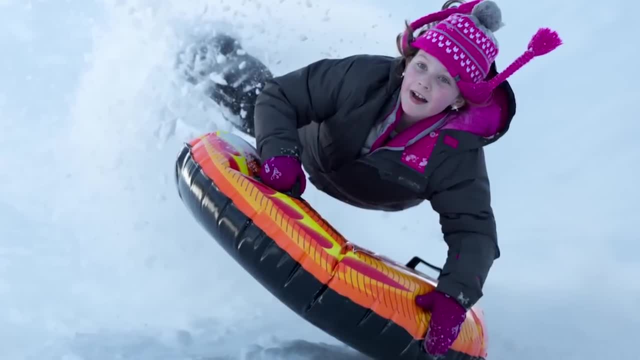 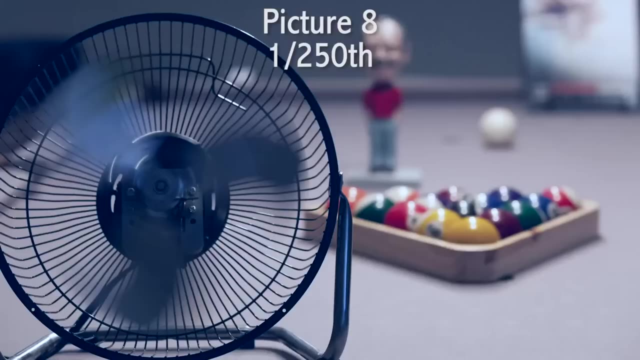 running or a bird flying. those are all times you want to be in shutter priority mode. So let's take a picture with the default settings in shutter priority mode. So at 1, 2, 50th of a second, the fans on that blade are pretty well blurred. Now let's imagine 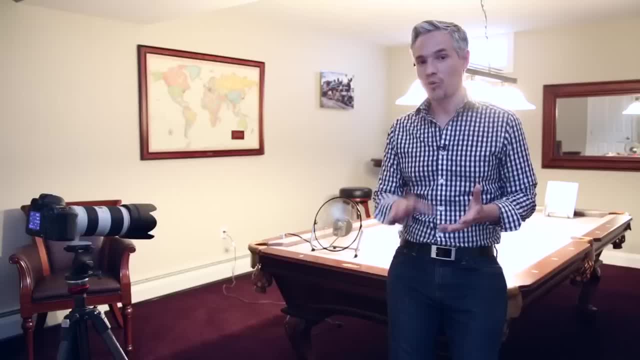 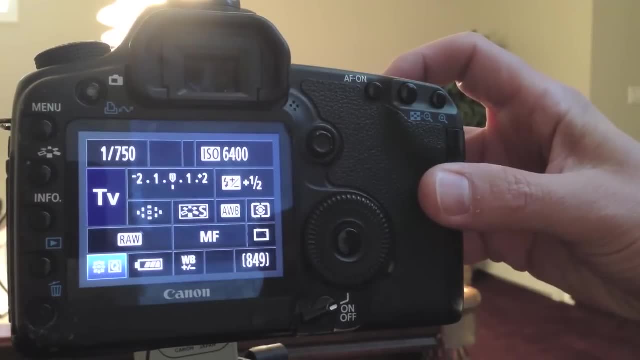 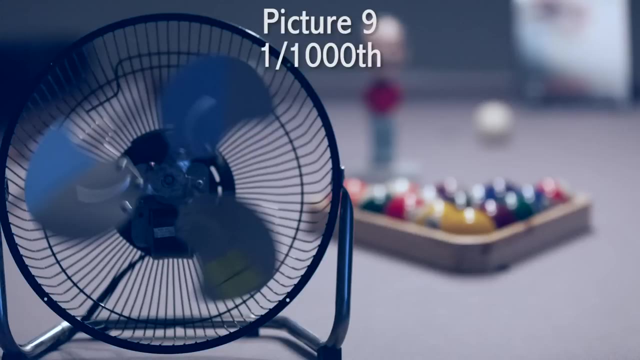 we're shooting a moving car. We're going to show those fan blades nice and crisp. We're going to crank that shutter speed even faster. So let's jump up to 1 1,000th of a second. That's better. They look nice and sharp. But what if that isn't the effect you want? What 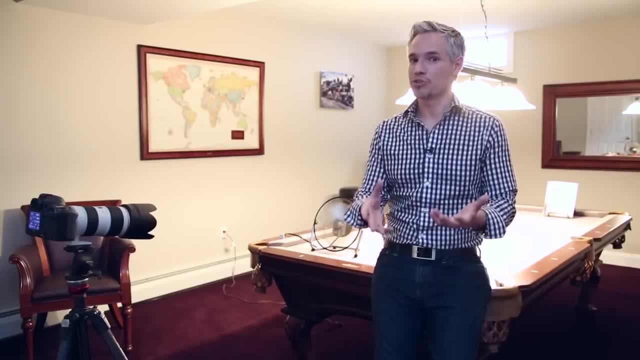 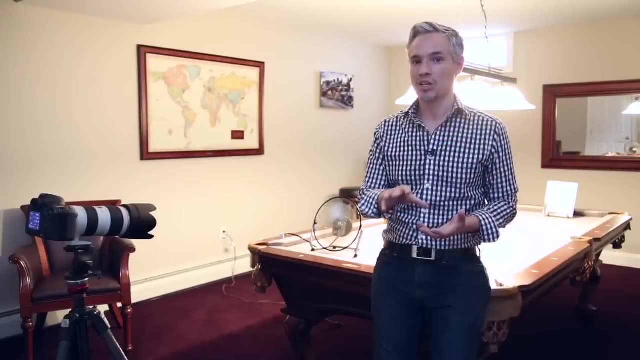 if you want to show motion blur. This is really common. if you're shooting a moving car, for example, You've got to get some spin showing in those wheels, and if your shutter is too fast you're going to freeze too much motion Intentionally. showing blur is what You're. 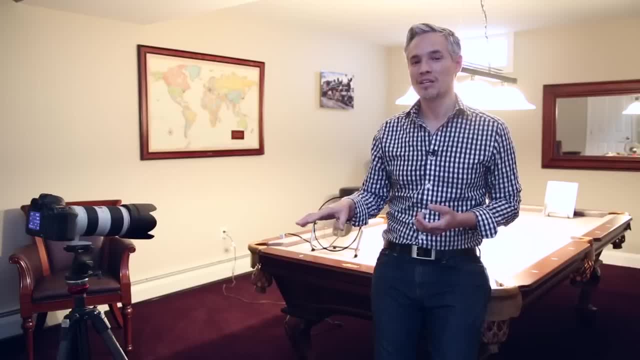 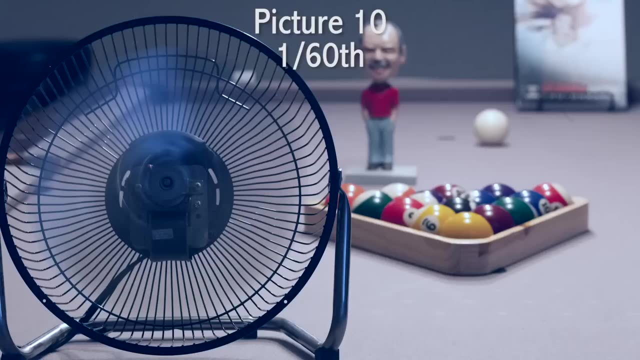 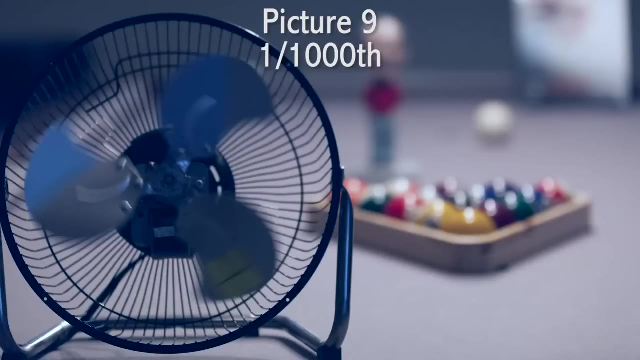 going to get a lot of blur. So let's drop that down to 1 1,000th of a second and see the effect. There's that nice blur I wanted At that speed. the fan blades are a complete blur. Shutter priority gives you a control over just how much motion your pictures show. 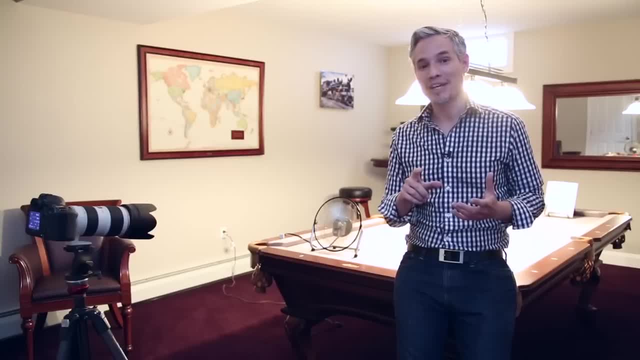 There's also motion in your own hands, and if you're hand-holding a picture and it's ending up blurry, it's probably what they call camera shake, And you can control that by using shutter priority and specifying a shutter speed that's fast enough for you to hand-hold. Now I will show you what happens when you change. 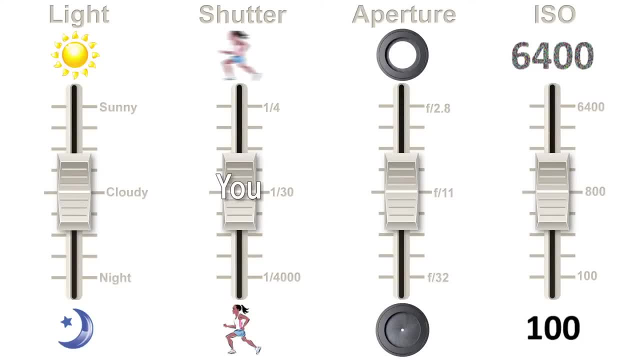 the lights. Shutter speed gives you control over the shutter and the camera will not change it. The camera will change the aperture and if you've chosen auto ISO, it will change the ISO as well, But it will never, ever change the shutter. You have control over that, So. 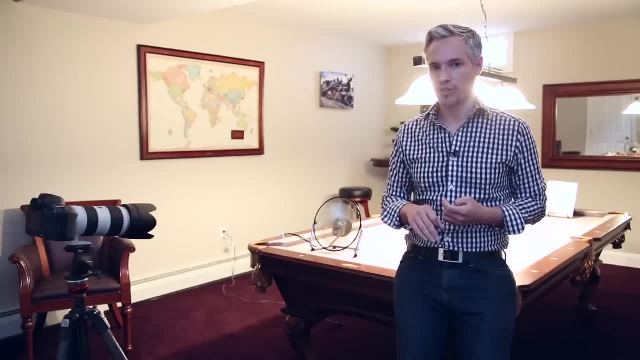 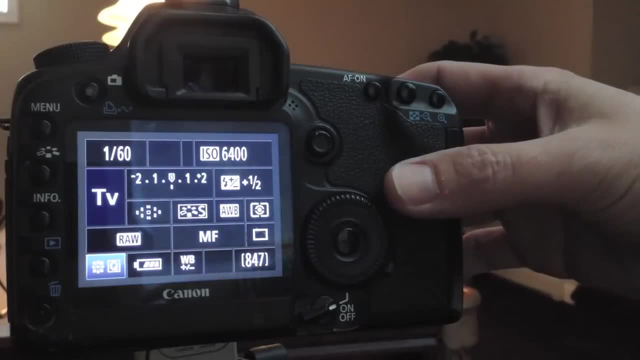 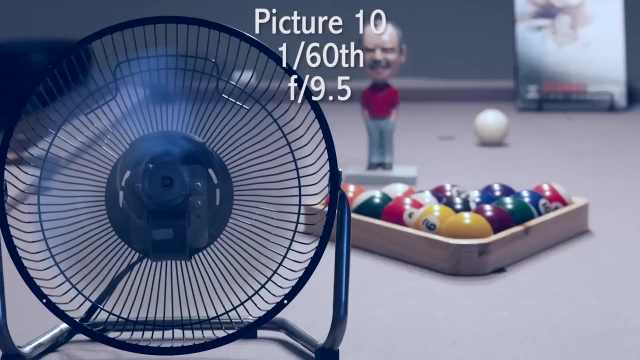 I'm going to drop the lights in half and we'll see what the camera does differently. As you can see, when I lowered the lights in the room, the camera compensated for that not by changing the shutter, but by lowering the f-stop number, Choosing a lower f-stop. 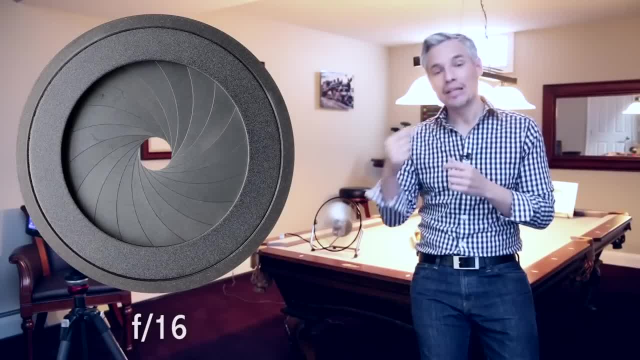 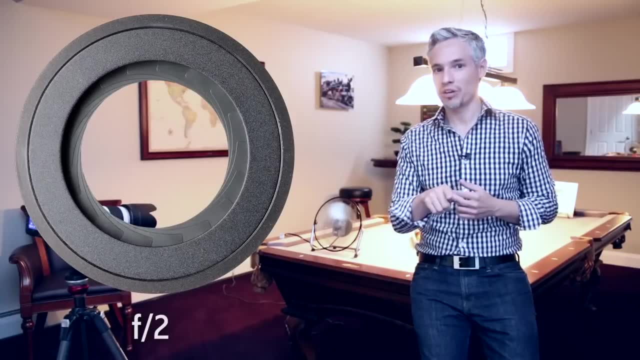 number opens up the aperture- the iris of the camera letting more light in. It had to do that in order to get the picture properly exposed. but in shutter priority you control the shutter, the camera controls the aperture. So let's take a deeper look at aperture. 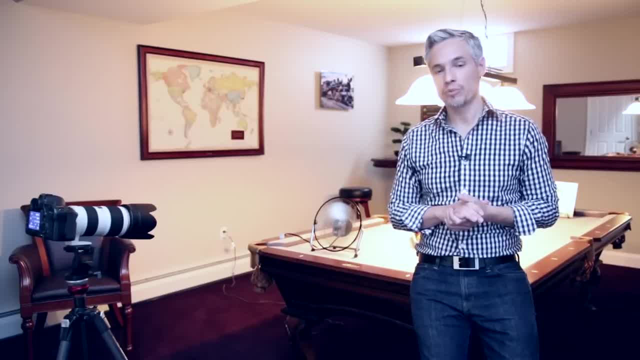 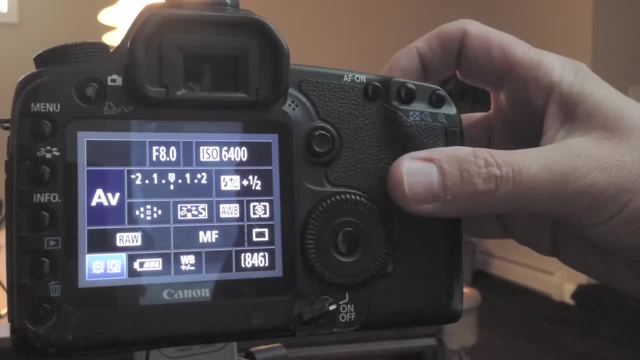 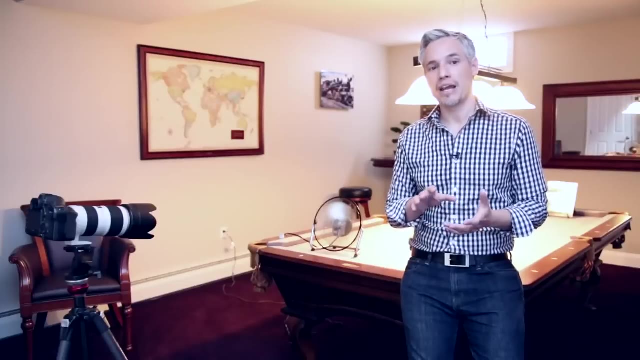 Now I'll switch the camera into aperture priority mode and take my first picture. I took that first picture at f8, which is a pretty moderate f-stop number. Now, one of the things that aperture controls besides the amount of light that gets in through the 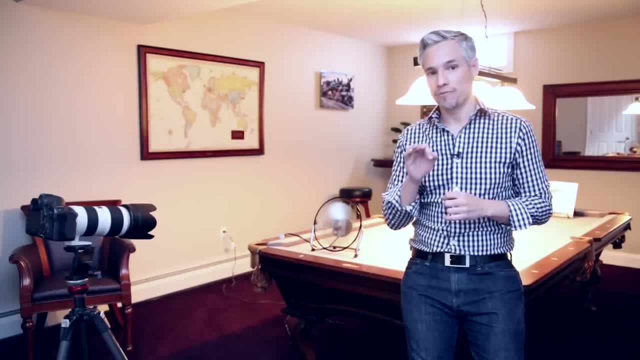 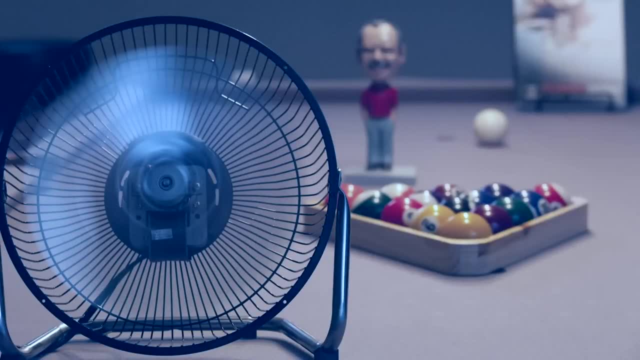 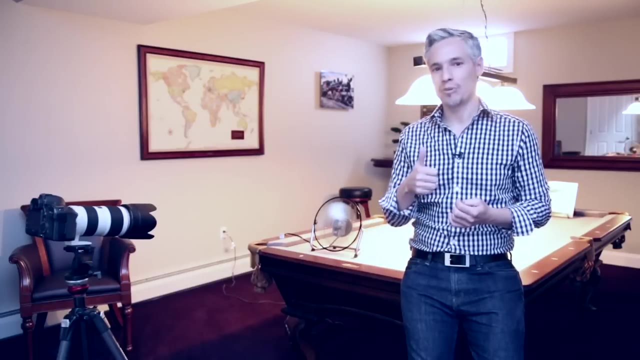 iris is the depth of field At f8, I got the objects in the background kind of in focus. But let's say I want them nice and sharp. What I'm going to do is to choose a higher f-stop number. so let's crank that f-stop number up and crank up the background sharpness. 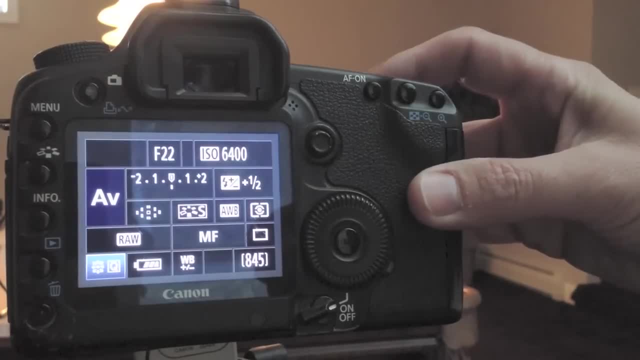 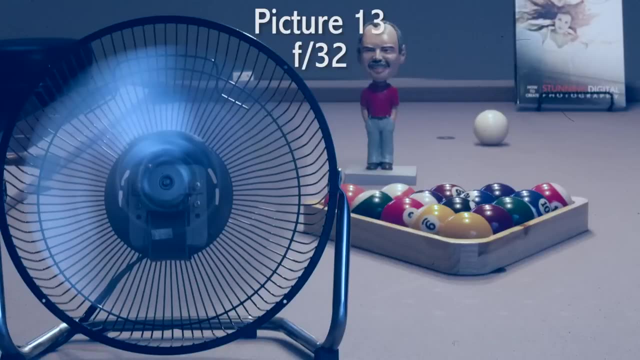 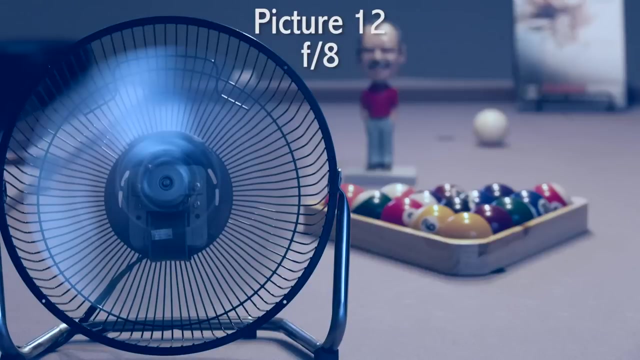 too. Now at f32, I have enough depth of field that you can read the title of my book in the background. I control the aperture in aperture priority mode. The camera doesn't do it, So let's imagine that I don't want to see the background sharpness and I want to see 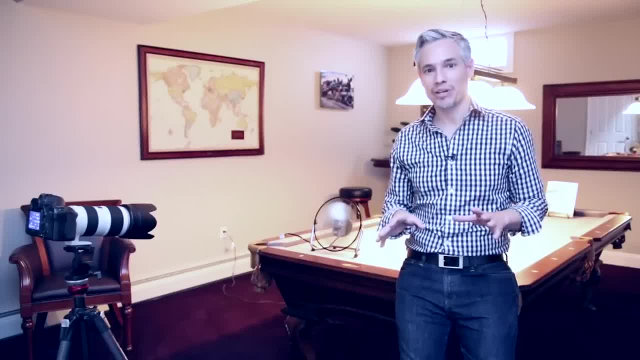 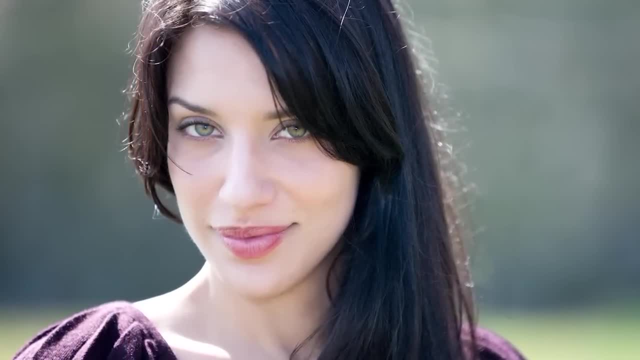 the background in focus. Let's imagine I want a nicely blurred background. This is really popular in portraits, where having a nice blurred background helps to eliminate any distractions. To do that, I'm going to choose a low f-stop number, because a low f-stop number means low background sharpness. Let's crank that. 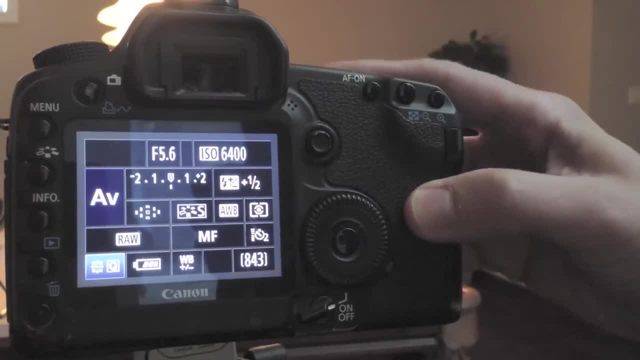 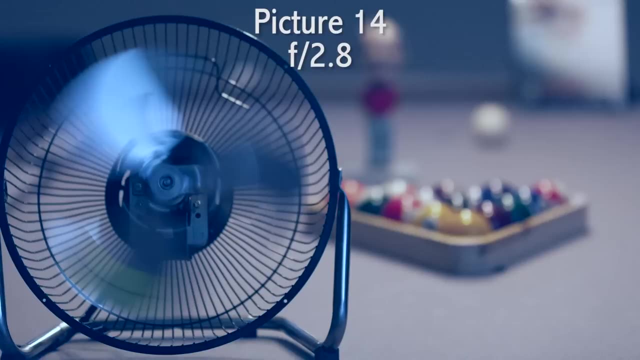 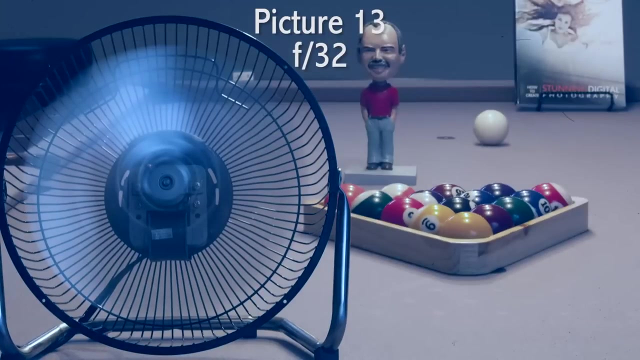 down to f2.8 and take another picture At f2.8, that book is completely blurred and even my dad in the middle is pretty blurry. Now you also notice those fan blades got a little more distinct. That's because the camera chose a faster shutter speed, because it was using a 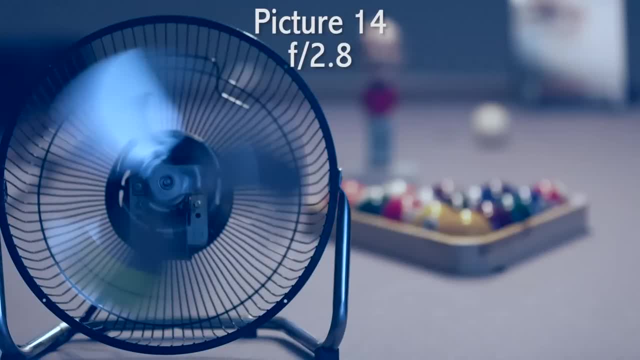 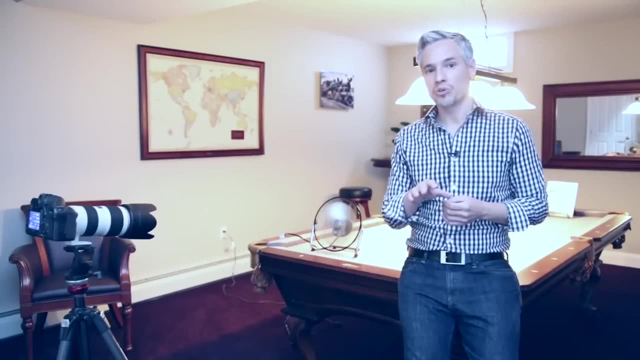 larger iris, a larger aperture which let in more light, And that's how aperture works. Now there's one other thing that I'd like to show you, and that's how a flash can control the amount of light in the room totally automatically. So I'll 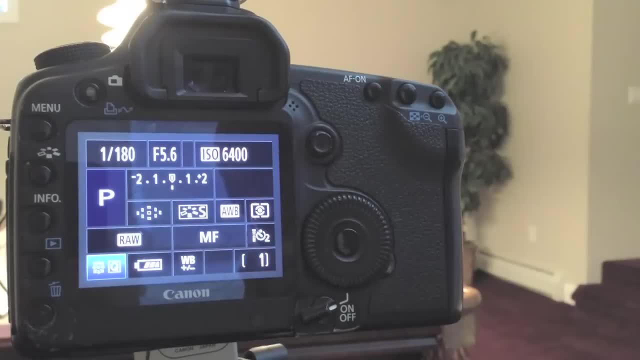 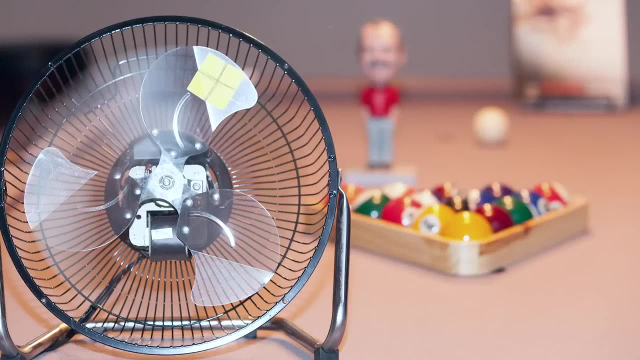 attach a flash to the camera now. Now, as you can see, the flash had an interesting effect on the fan blades. It kind of froze the motion, but then you can still see some blur. When the flash actually fired, the imprint of the blades at that current position were burned. 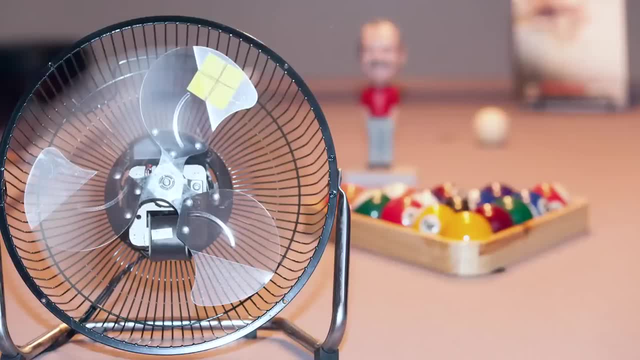 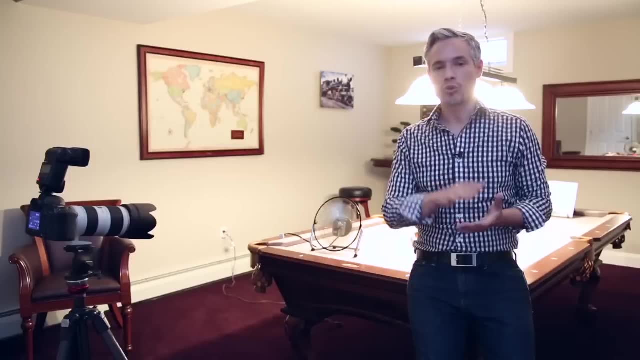 into the sensor, But because they were moving the rest of the time the shutter was open. you see this kind of interesting effect where they're blurred and then frozen, almost like a ghost moving into position. It's one of the cool tricks that you can do with flash. Now, why might you want to use a flash? 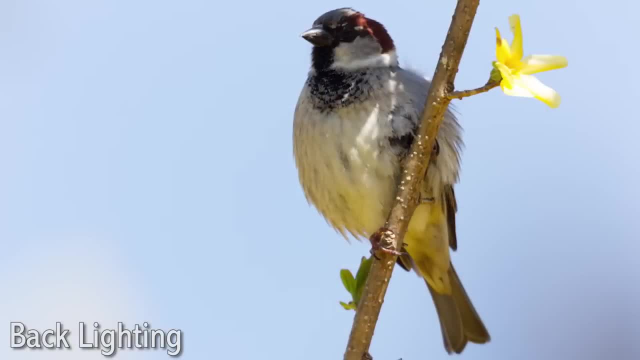 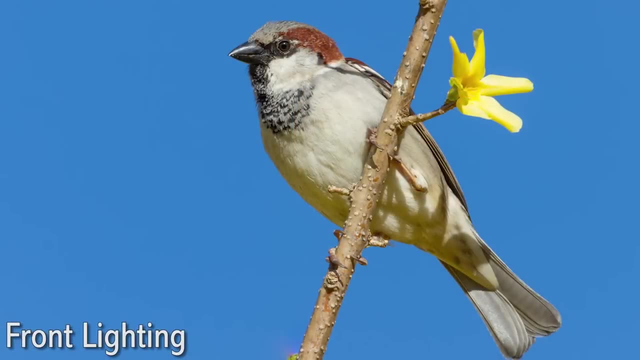 and add light. Well, first you might want front lighting. If the subject is backlit, a front light would help fill in any shadows. So check chapter 3 for detailed information about controlling your light. You might also want it because you're. 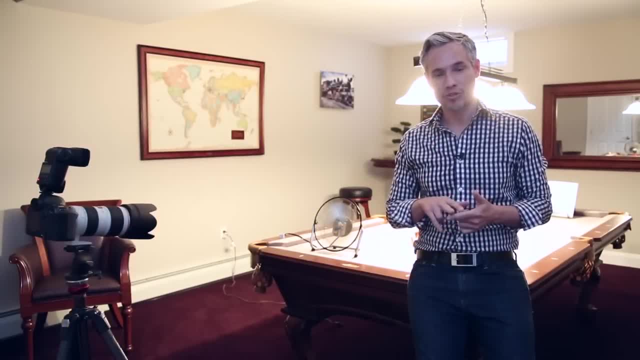 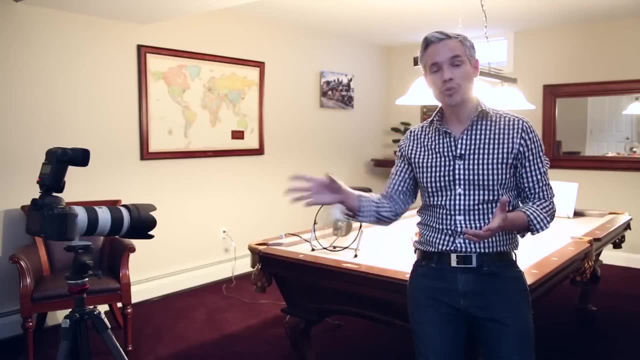 not happy with the compromise of ISO aperture and f-stop, given the amount of light. If you're forced to use ISO 6400 and you just hate how noisy it is, put a flash on. Add a little light to the room and that'll let you use a lower ISO. 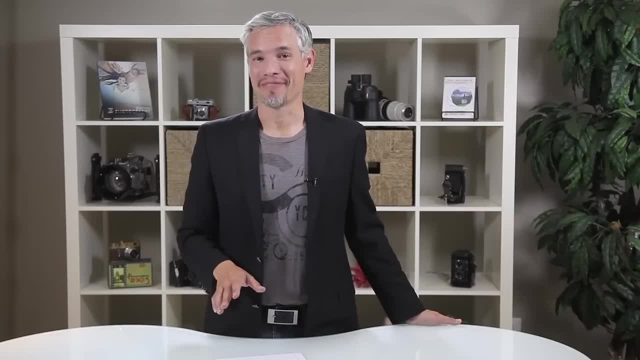 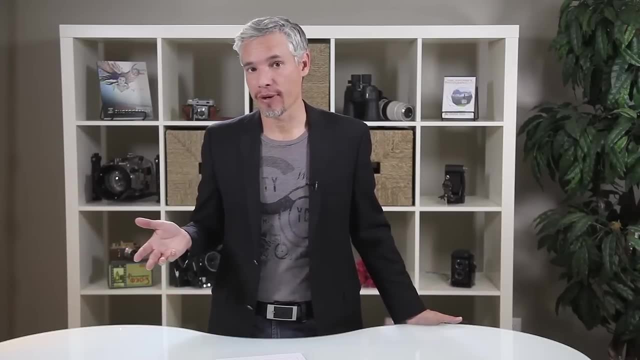 Now I'd like to talk about RAW vs JPEG. JPEG is the standard format for just about every picture that you see on the internet. In fact, it's the standard format for the pictures that almost every camera takes, But it's not the best. 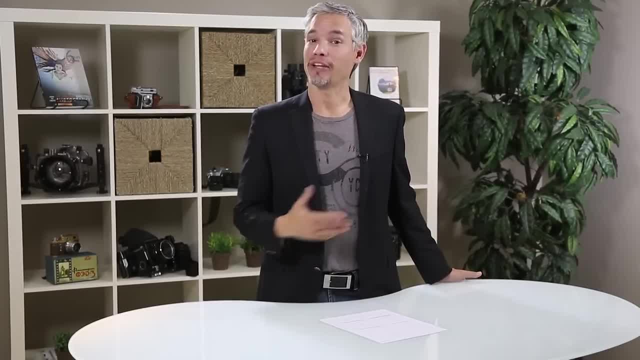 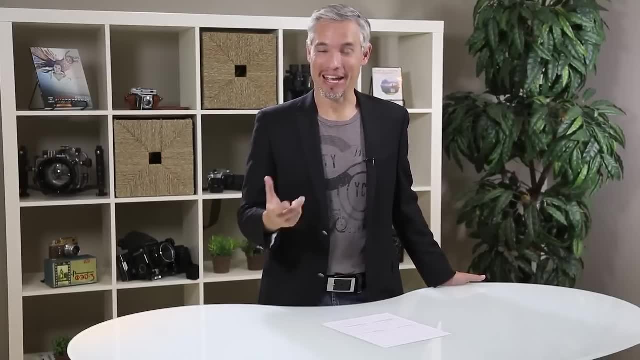 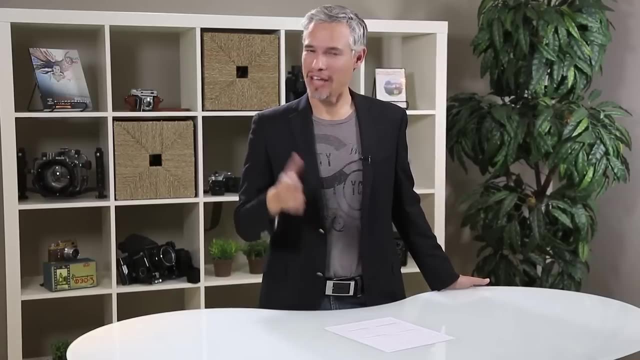 format. The best format is actually a format that's generically known as RAW. RAW files capture all the data that your camera sensor captures when you take a picture. It doesn't throw out anything, by contrast, is actually just a compilation of the data that's been processed by your camera. 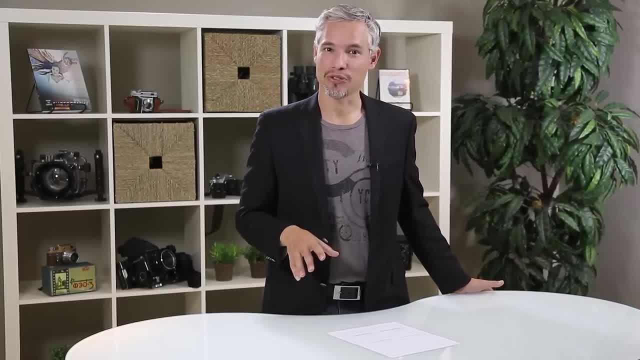 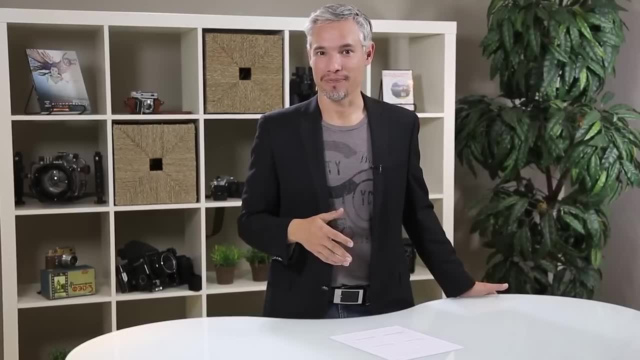 Now, one of the things that your camera does when it converts all that data that it captures into the JPEG file that most people work with is it throws away the brightest and the darkest parts of the picture. So that's right. you're actually losing some of that really important dynamic. 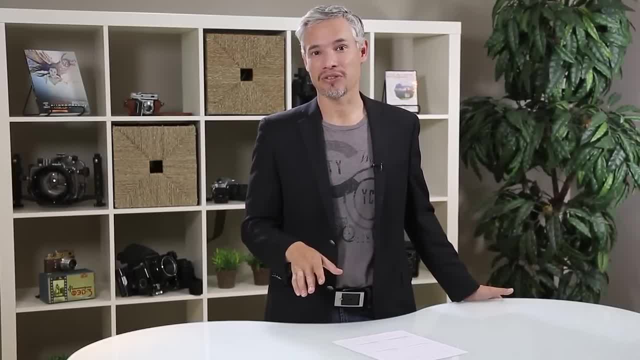 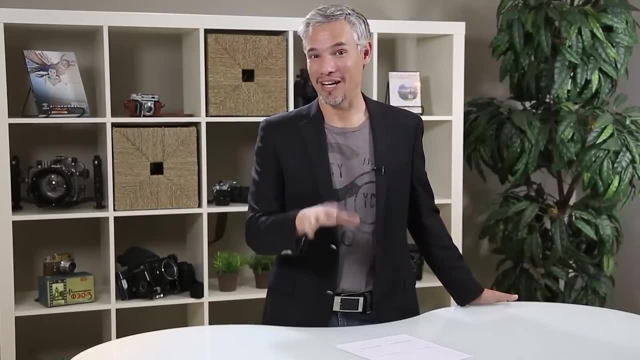 range. You're losing some of the details and the highlights and the shadows, and you're getting this highly compressed JPEG file. And if that doesn't sound ideal to you, well you're right, Because the RAW file captures all the data that your camera collected. it gives you a lot more. 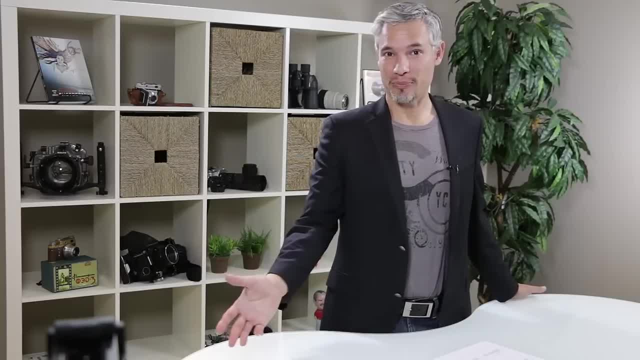 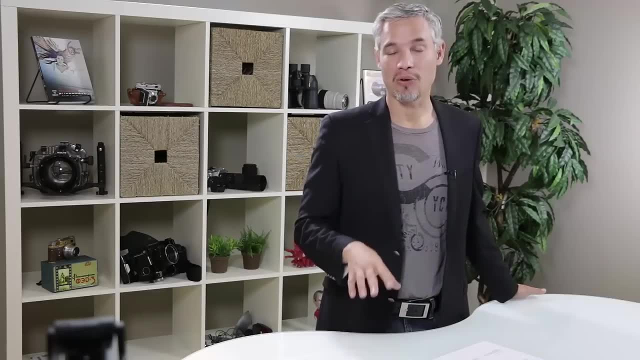 flexibility in editing. So, while you're going to need to convert the picture to a JPEG before you share it, while you're editing it, while you're adjusting the exposure and the white balance, that data that's included with the RAW file will allow you to do a lot more powerful editing than 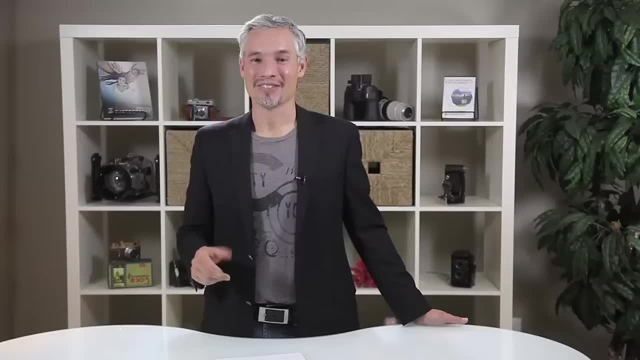 you would if you were working directly with a JPEG. So here's a quick recommendation: Just shoot RAW, Just shoot RAW all the time. Set your camera to RAW and forget about it. You might need to buy a little bit bigger memory card, but five, ten years. 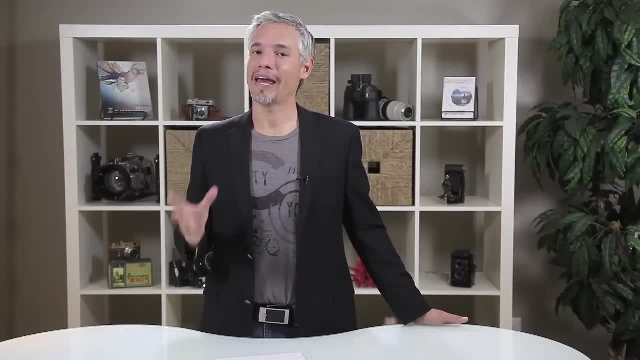 from now you'll be really glad you did, Because even if you don't edit your pictures now, you probably will in the future. if you continue to be serious about photography And if you're looking at pictures of your kids or other important moments and all you have are JPEG files, you are 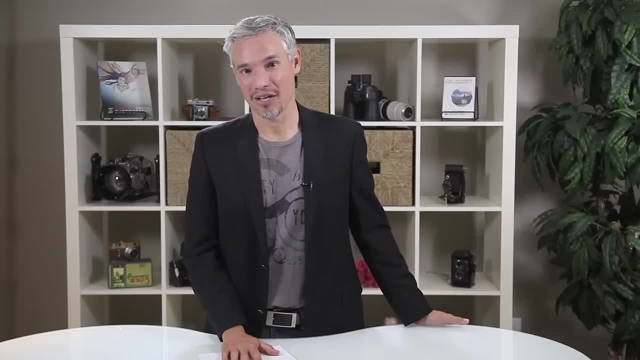 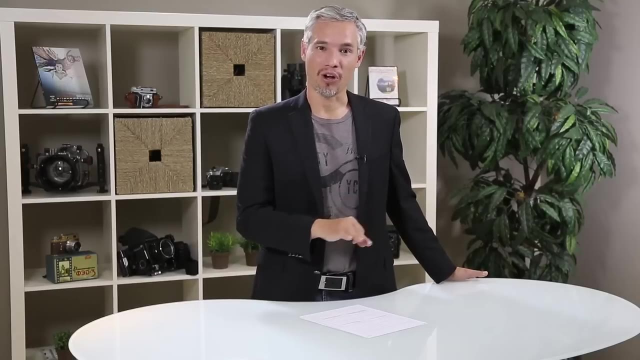 going to be kicking yourself about all the detail that you lost. So start shooting RAW now and when you start editing your pictures, I promise you'll appreciate it. Let's head over to the computer so that I can show you exactly what a difference shooting RAW makes. 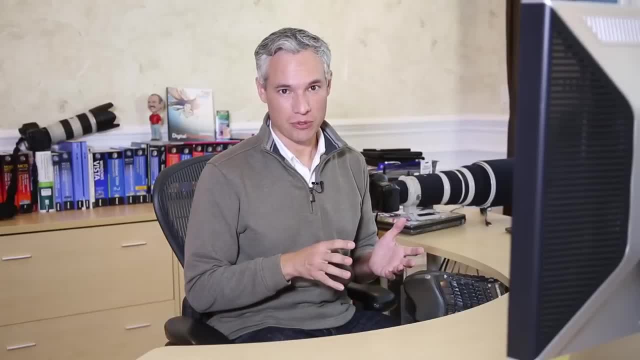 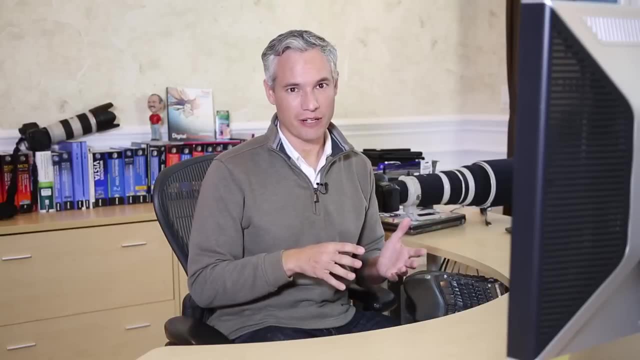 versus shooting. JPEG RAW files take all the data captured by your camera's sensor and put it into a really big file that you can process later. Now, that's distinct from a JPEG file. If you use JPEG files, your camera takes all that RAW data and processes it. 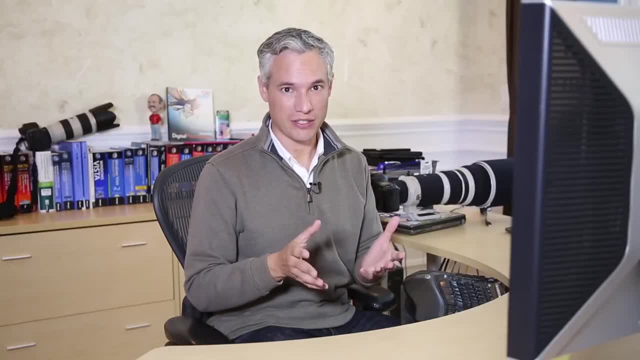 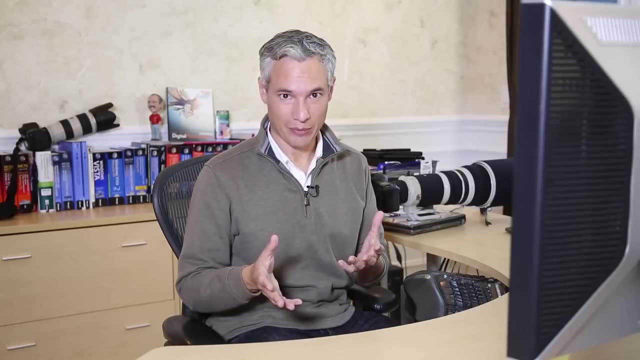 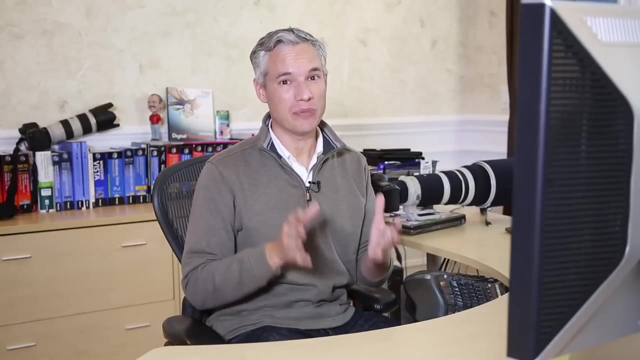 in camera and then you get to work with that processed file. Now you might notice that a JPEG file tends to be about three megabytes, whereas the RAW file might be 25 megabytes. The difference is important. The RAW file is giving you way, way, way more data. In fact, it's giving you every bit of data. 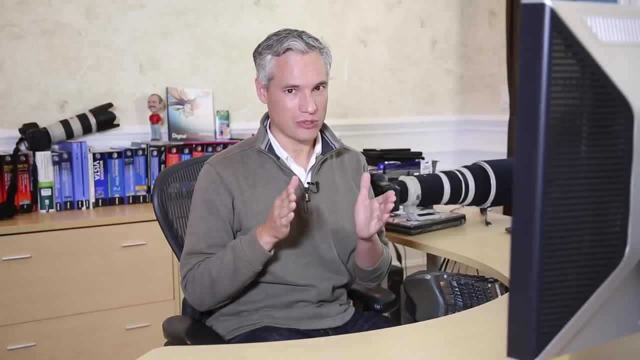 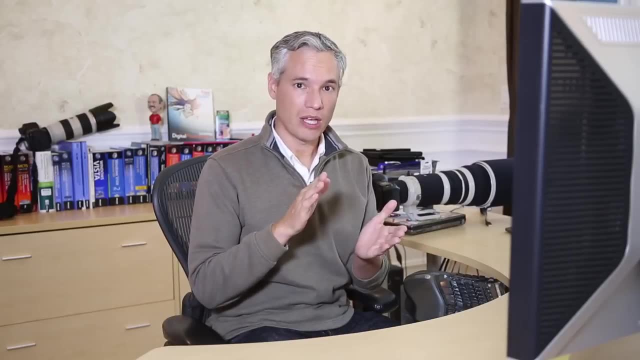 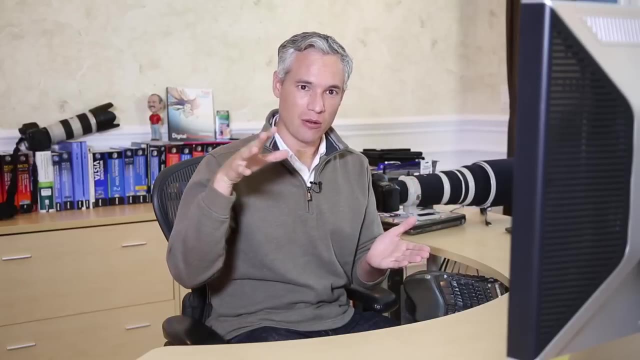 that the sensor captures The JPEG file drops an awful lot of that data. Your JPEG pictures might still look good, but they don't have all the data in them. For example, a RAW file will capture, let's say, 10,000 different bits, different gradients from black to white, and it will store. 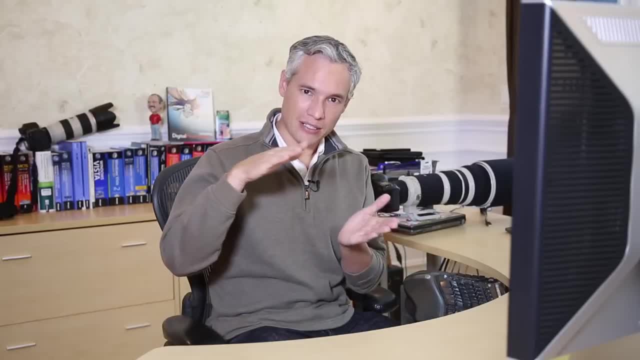 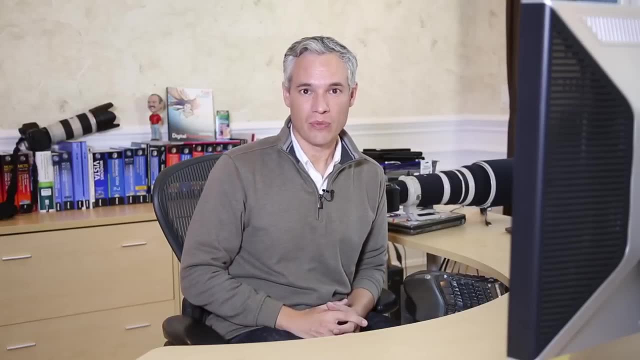 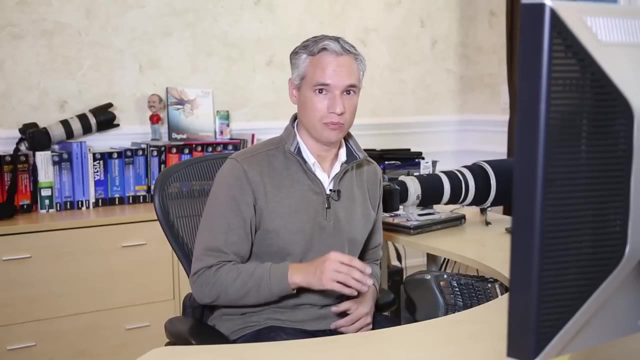 them all. When you save it as a JPEG file, it has to clip the top and bottom part of that. It clips some of the shadows and some of the highlights and that means you're losing detail. To demonstrate that, let's look at some JPEG files and RAW files. in my photo editing app, Lightroom, Here I have a picture. 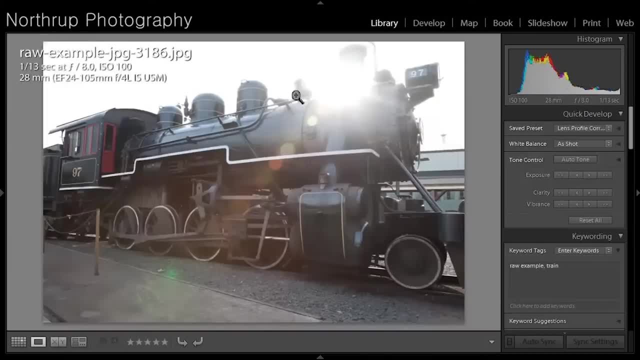 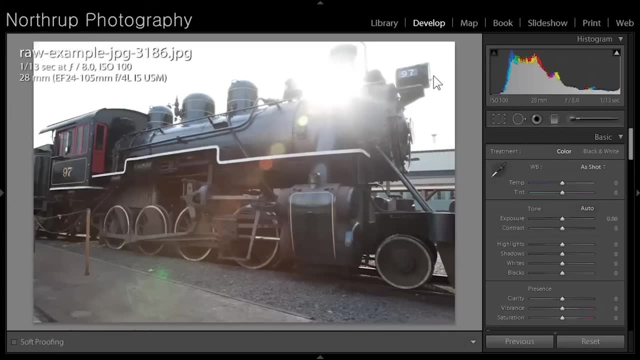 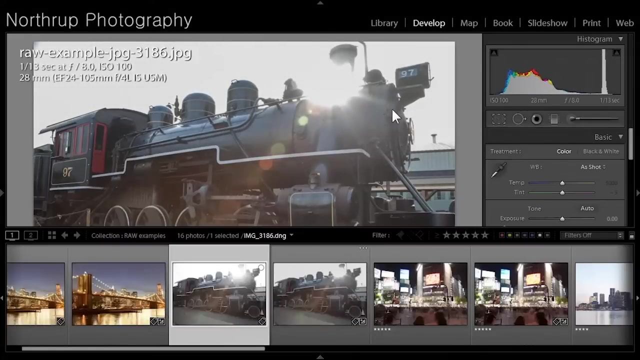 of a train, shot in both RAW and JPEG, And you can see that this is a pretty challenging scenario. I'm shooting directly into the sun here. I'll switch over to the Develop module and try to recover some of the highlights. You can see I am able to retrieve some of the information. Now let's look at the RAW file instead. 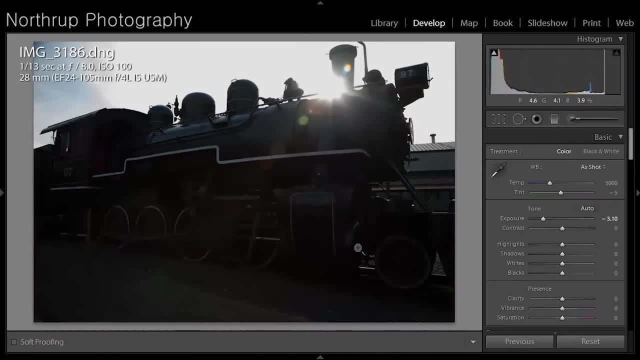 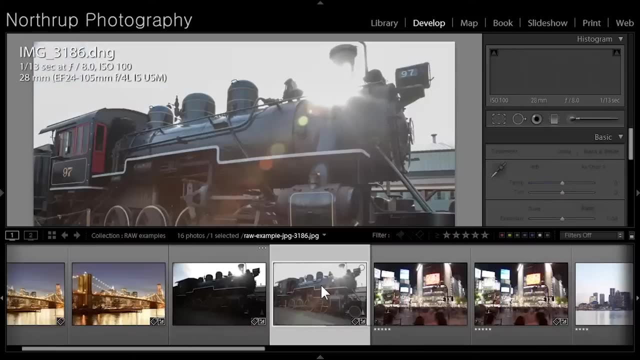 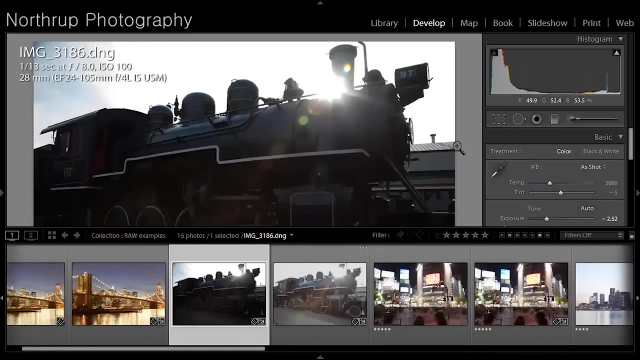 Now you can see how much more information I was able to recover there. I was able to see quite a bit more of the train in that one than in here. You can see how much more that sunburst covers up. Now I'll switch over to the RAW file one more time and bring up the shadows a little bit. 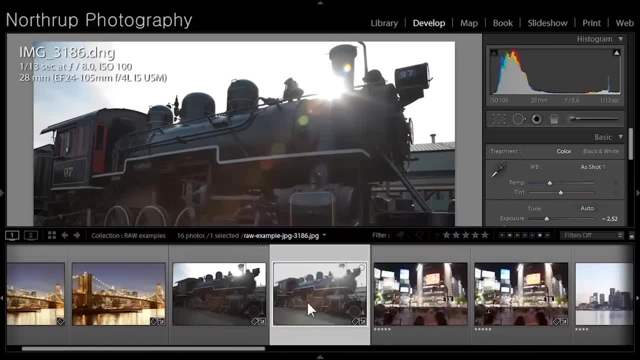 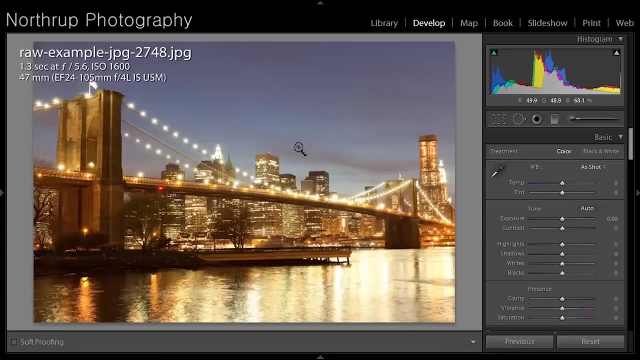 And you can see that I'm able to get a much clearer picture from the RAW file than I could from the JPEG file. Another good use of RAW files is white balance. In this night shot of the Brooklyn Bridge you can see the white balance is terrible. With a JPEG file you can adjust the white balance. 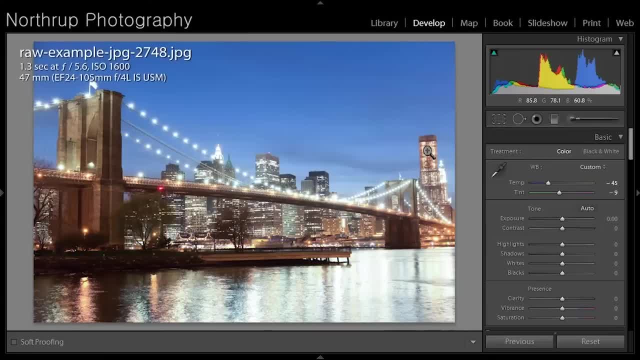 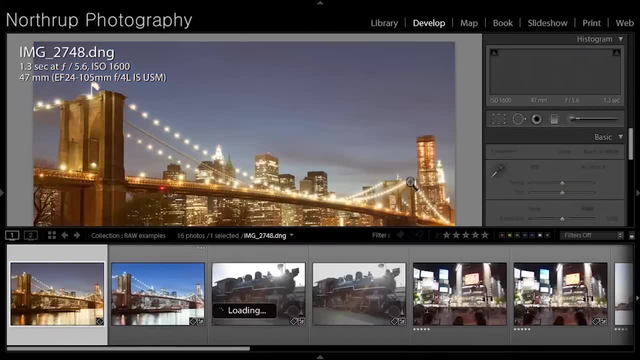 but it's not quite as perfect because your camera has already decided upon the white balance in camera and set that permanently for you. With a RAW file you have quite a bit more flexibility and you don't have to worry about any data loss. So you can fix the white balance and you will. 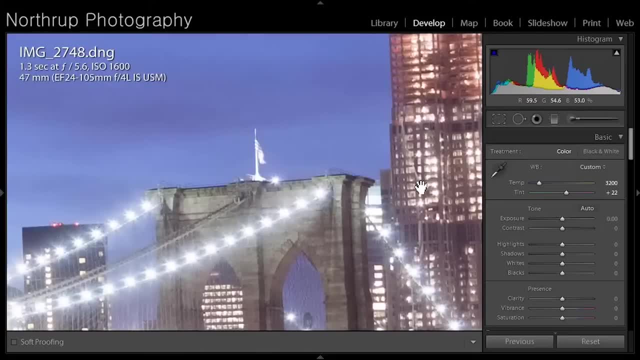 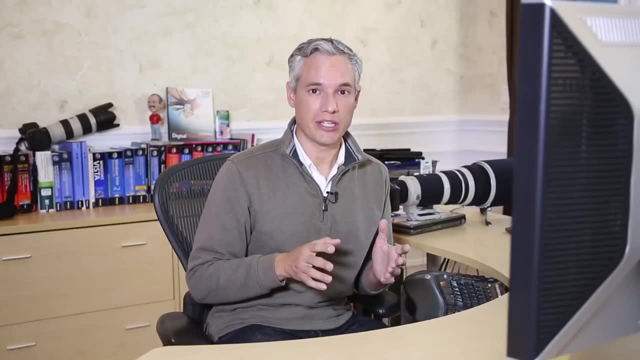 still retain perfect detail, as if you had set the white balance correctly in the first place. Of course, it's always ideal, but you don't have to make those decisions at the time you're shooting the RAW file. You get to make those decisions later, which means if you happen to make a mistake. 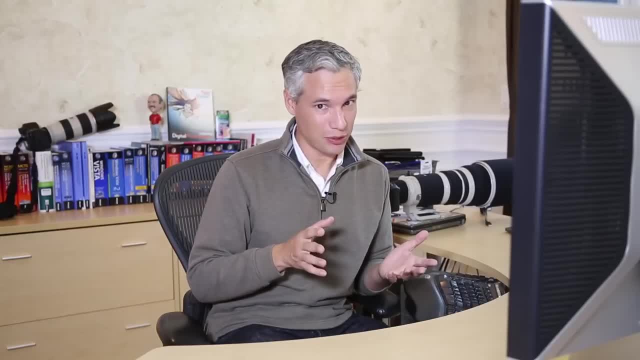 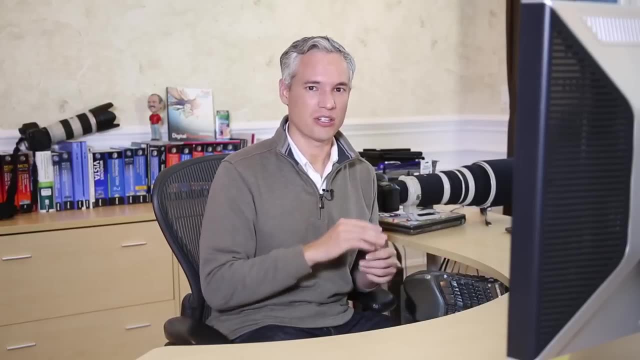 or if the lighting situation is such that it would be impossible to pick one right answer, you can fix it in post. as long as you shoot RAW, It just gives you more power later on. Let's look at a couple more examples. This is Shibuya Station in Tokyo, Japan. 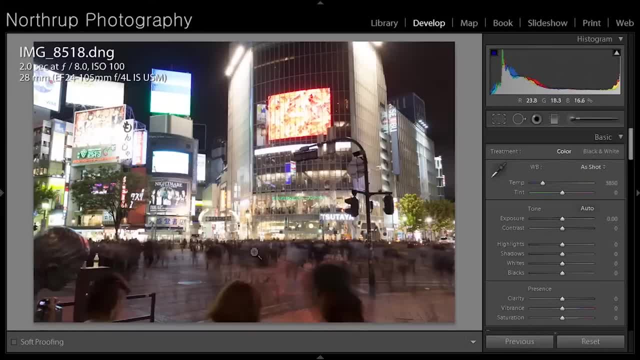 and it's the busiest intersection in the world, which means I couldn't necessarily bracket shots because you can see just how much movement there is here. So HDR wouldn't work to capture this huge dynamic range between the darks and the blown-out highlights here. Look at this. sign up here. 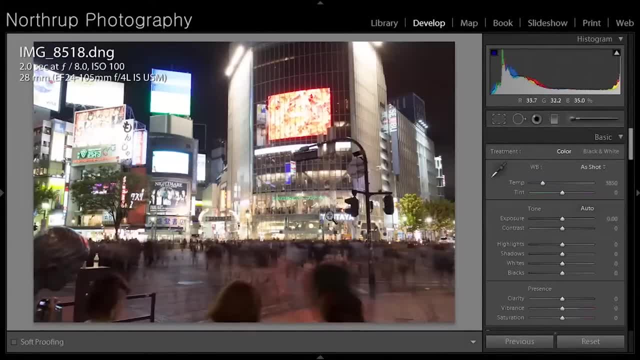 and you can see you can't read those words at all. This is completely white. With RAW I can drag these highlights down and suddenly this sign is completely readable. Take a look at this area of this sign over here and how much is lost versus how much can be recovered. 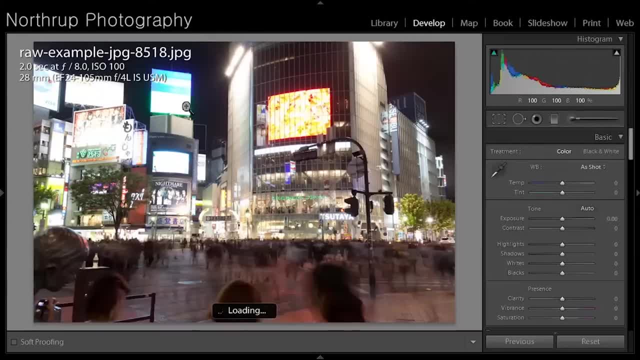 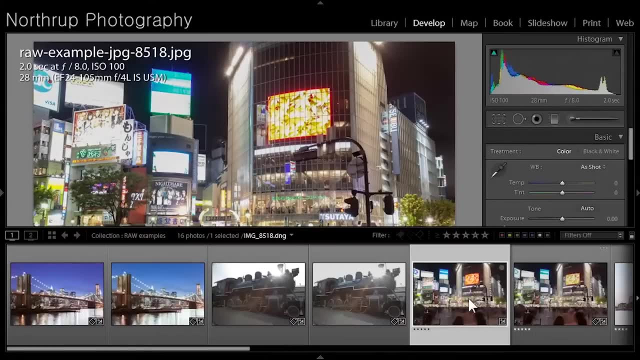 Now I'll switch over to the JPEG file and we'll look at the same blue sign up here. I'll try to recover the highlights and you'll see it's just not as good. Do a before and after with the RAW file. That's the RAW file and that's the JPEG file. 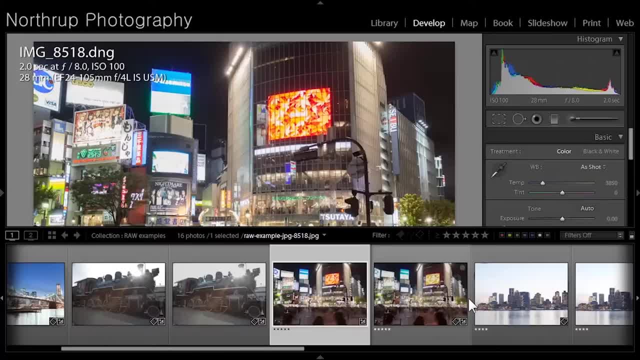 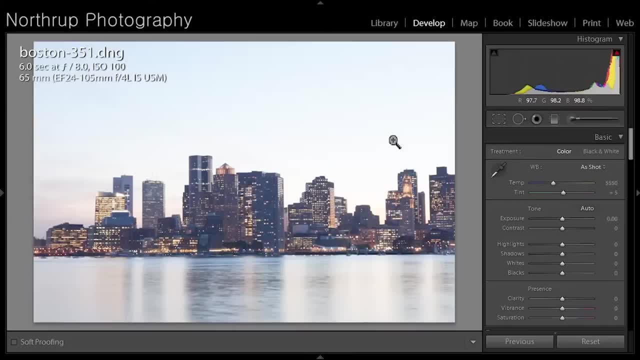 Once again, the RAW file shows far more detail and the JPEG just has more and more blown out. Here's another example. This is a sunset shot of the Boston skyline and you can see it's at dusk, but the sky is completely blown out. This is actually a great. 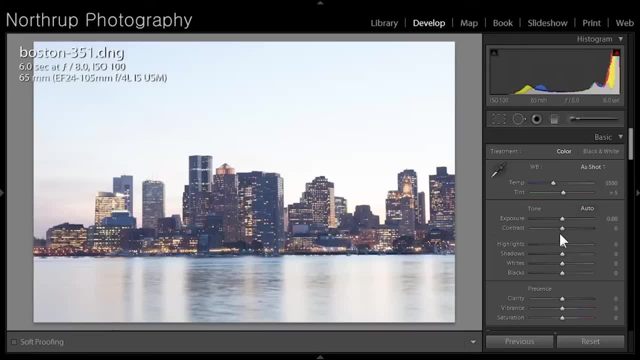 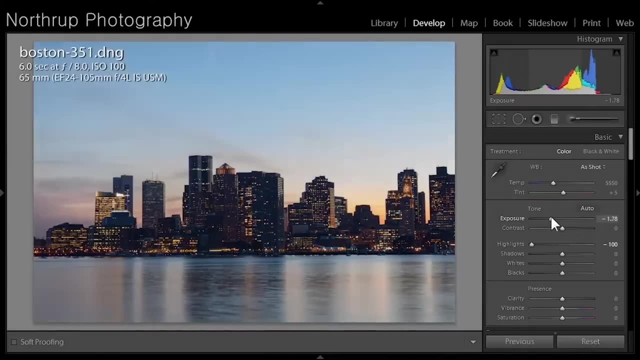 exposure for a night shot, because I'm capturing all the detail in the shadows here and if it were a JPEG the shot would just be a loss. But with a RAW file I can drag those highlights down and you can just see a ton of detail in the sky. You can see, even though the sky looked overexposed. 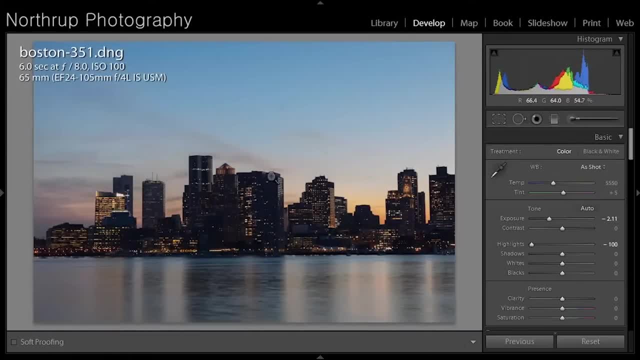 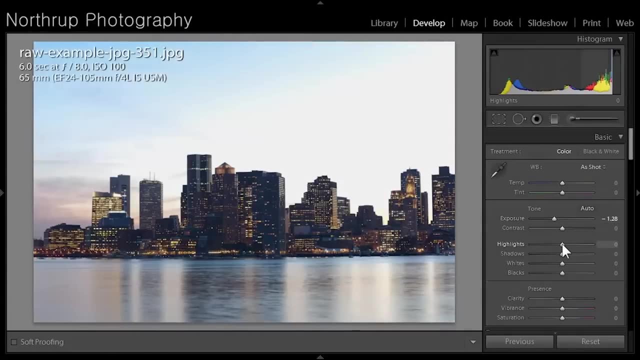 initially there's absolutely no detail lost. Lots of dust here, but you can see these wispy clouds. Now let me switch over to the JPEG file and I'll drop the exposure down. I'll recover the highlights and you can see what happens. 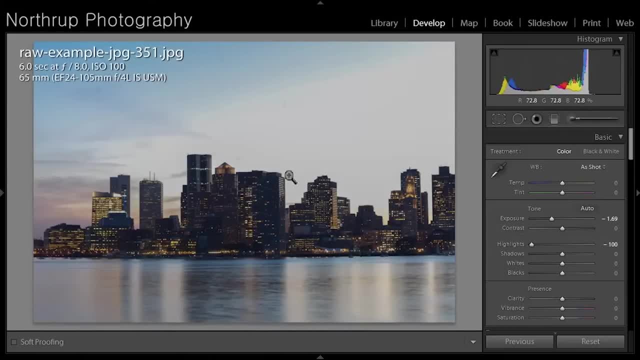 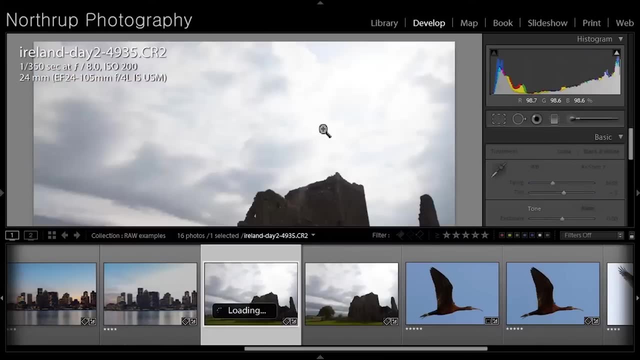 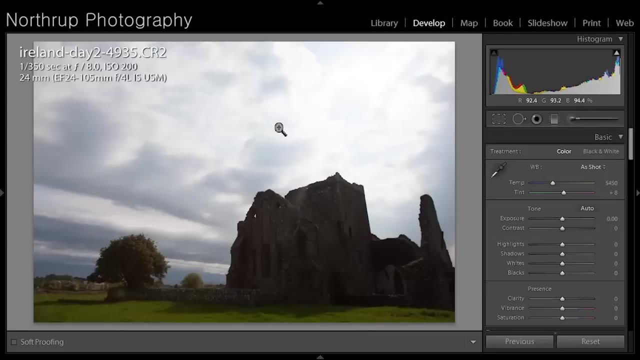 There's a little bit of detail that can be recovered, but you see these terrible lines up here. Switching back to the RAW file, it just looks so much better. Here's another high dynamic range situation, this one in the day You can see this ruin in Ireland is completely in shadow because you have these overcast skies here. 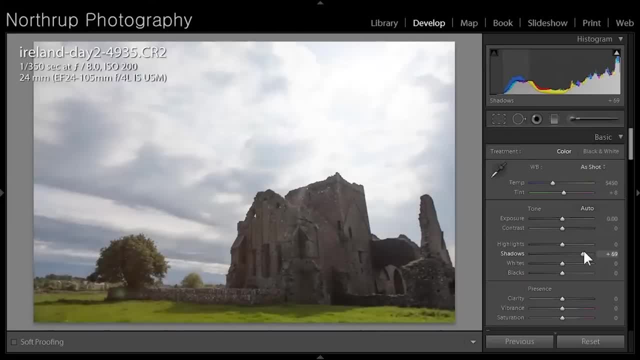 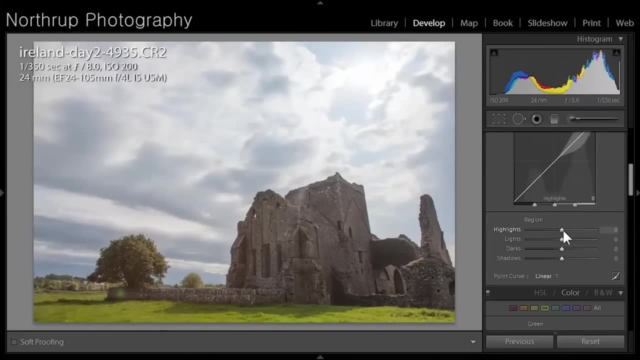 but there's a great deal of detail in both the shadows and the highlights here. So with the RAW file I can drag up these shadows and drag down these highlights and just overall reduce the contrast of it. Now let me pull the blues down a little bit to show some more detail in the sky. 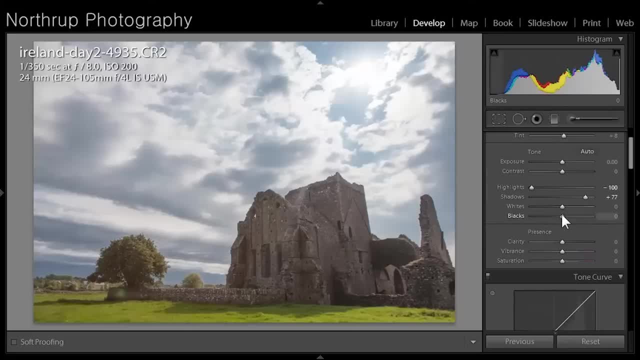 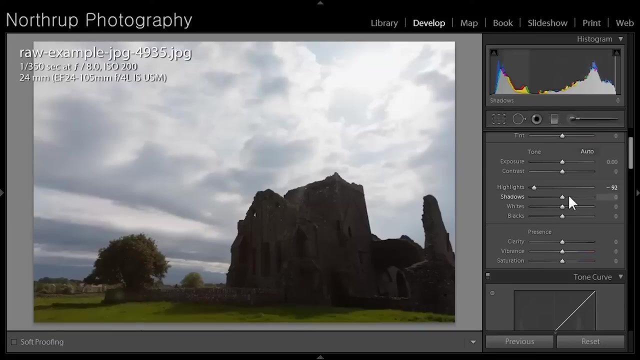 And wow, that's just amazing. Just a lot of detail that was recovered in that picture. Now let's take a look at the JPEG file. That's the JPEG file and this is the RAW file edited. Now I can try to do that same editing here in the JPEG file and you can see I'm able to recover some of it. 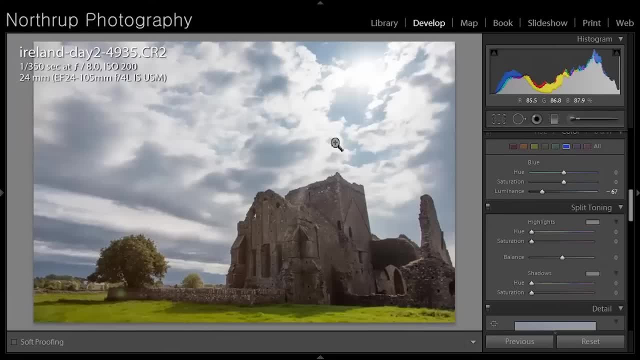 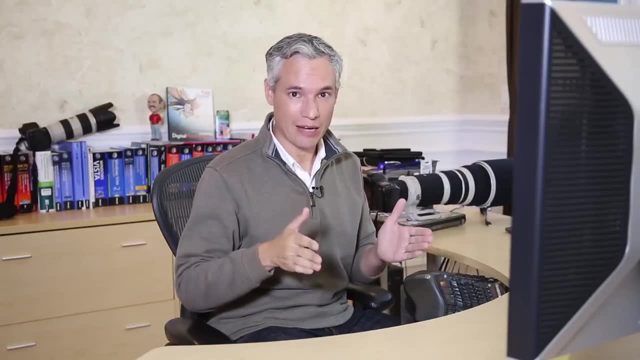 Drag the blues down. You can see, after processing, the RAW file just looks much, much better because you have all that extra information. When you choose JPEG files, your camera processes it, It processes it in the camera and just throws away that information forever. 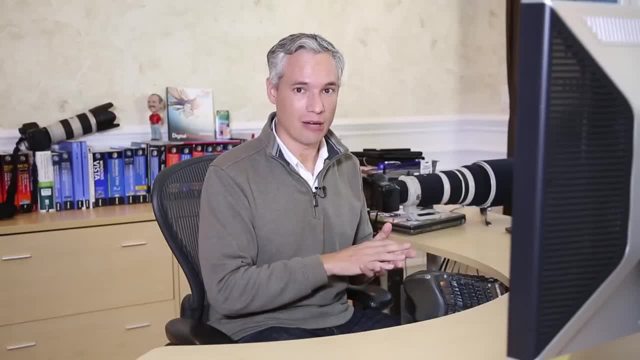 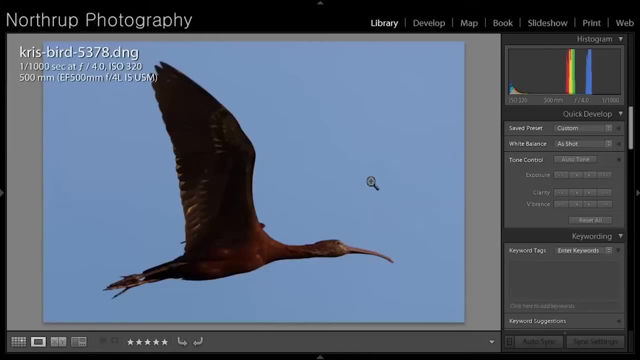 When you pick RAW, you can always go back and save it and you have all the detail that your camera sensor was able to capture. Wildlife shots can be really challenging because you don't necessarily get to make adjustments and shoot later. Here I saw this. 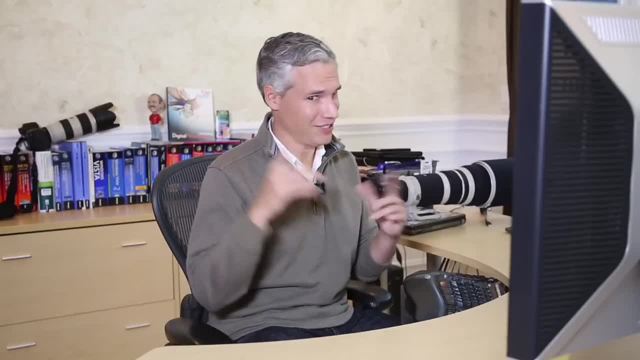 I was flying and I had to capture it with whatever settings I had. I didn't get to take a picture and then look at my settings and think about it, and I did a pretty good job, But you can see it's a little bit underexposed. 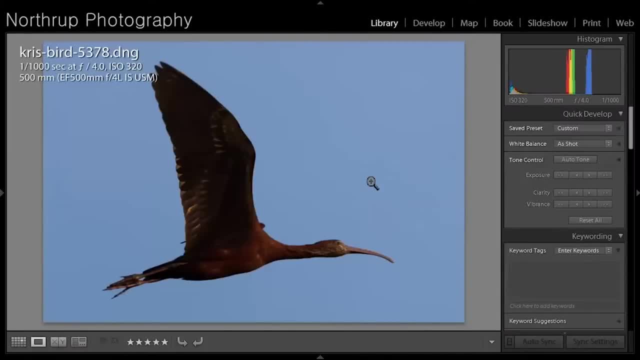 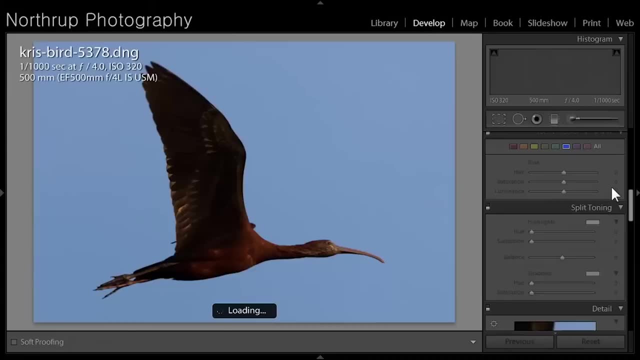 The detail that we want to see are these gorgeous colors in the bird's wings, and in the JPEG file they would be lost, But look here in the RAW file and you'll see that we can recover a great deal of detail in this picture. 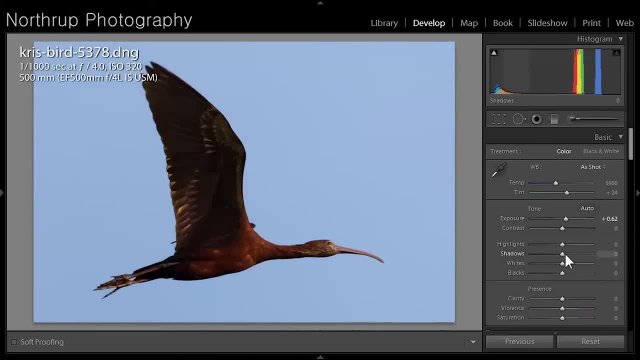 I'll drag the exposure up and then pull these shadows up and you'll see what happens. Now that's just amazing. You can just see all this metallic color in this ibis. Just really beautiful, and with the JPEG file, all that would be lost. 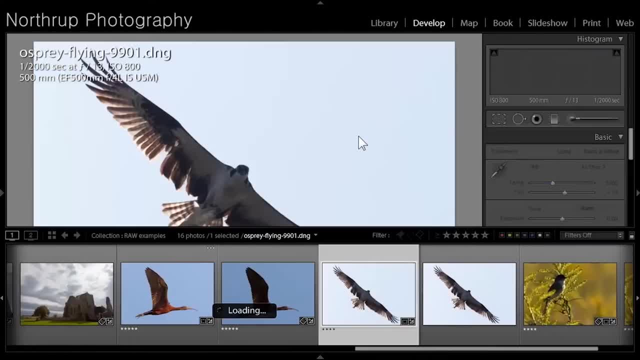 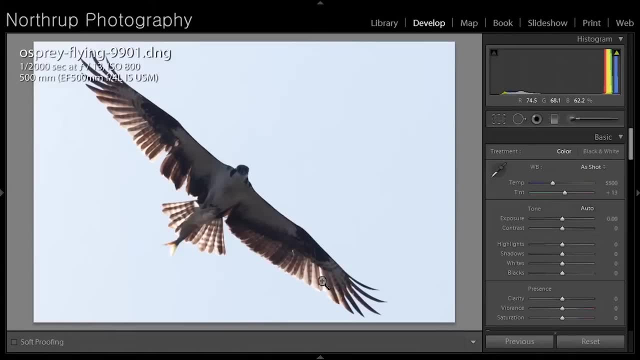 Here's a little more extreme example. This osprey had caught a fish, but because the sky was overcast, it's completely blown out and he's completely in shadow. Now here's an answer. Wait around for better lighting, right? 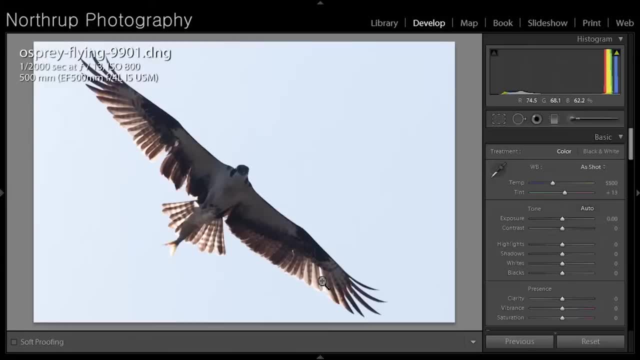 But you don't always necessarily want to waste a whole day of shooting because I had bad weather that day. But with RAW this file can be recovered. So the first thing I'll do is pull the highlights down to recover some blue in the sky, and then I'll just drag the shadows up some. 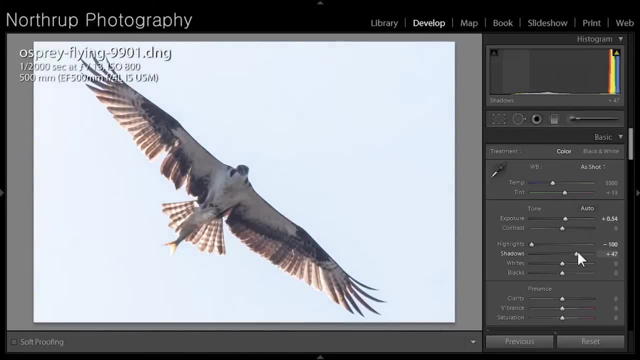 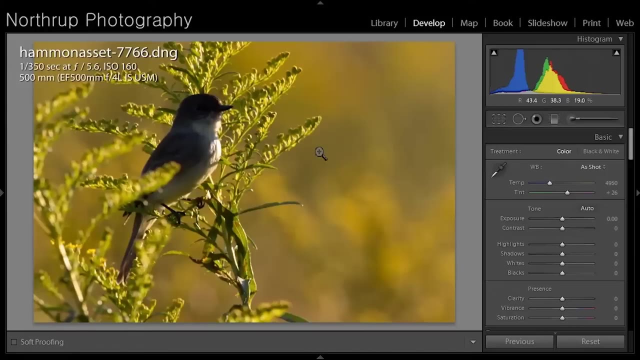 Pull the exposure up a little until the bird is well exposed, And then I'll just drag the shadows and then drop the blacks down and you can see I ended up with a pretty good picture. Another wildlife picture. I shot this flycatcher at sunset and it was just beautiful and the lighting is beautiful. 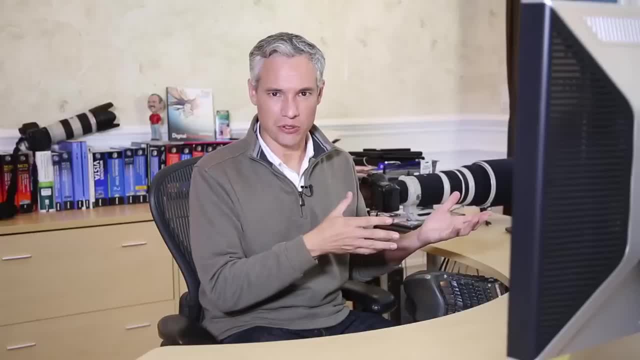 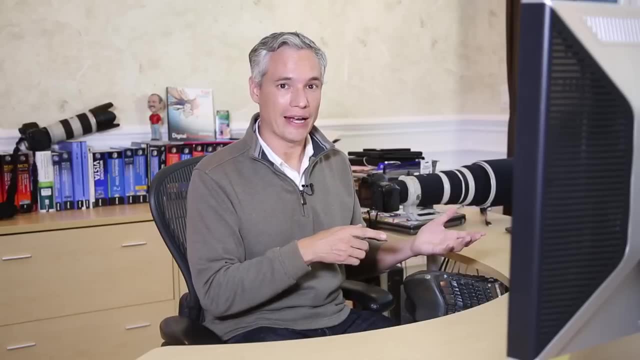 You can see, because the reeds are backlit, that they're kind of glowing With wildlife. you usually want the subject to be frontlit, but I wouldn't have had the beautiful lighting on the reeds if I did that With RAW. however, I can expose it properly for the reeds and then recover some of that. 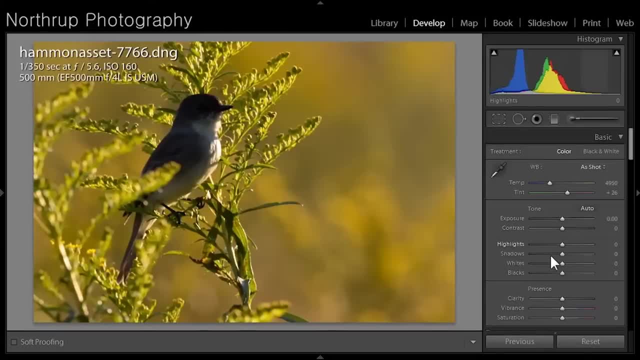 But this is just so much of the shadow detail that you'll be able to see the bird nicely. So I'll pull out the shadows here And I'll bump the exposure up just a little bit And you can see. it ended up being just a really nice picture. 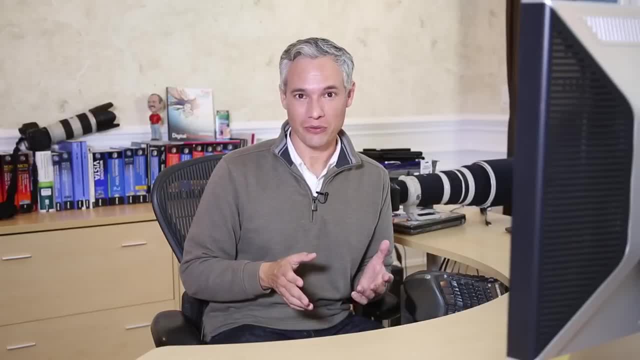 So I hope you'll check your camera's manual and learn how to turn on RAW files for it. There are a few disadvantages that you should know about. RAW files are way bigger, and that's where the disadvantages come from. You can fit fewer pictures on a single memory card. 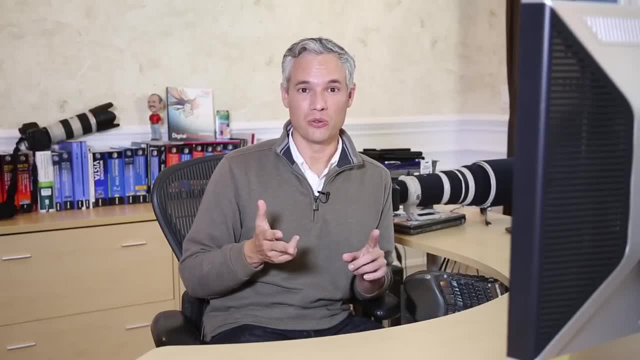 bigger memory cards or more of them, You run out of buffer faster. So if you're, say, shooting wildlife or sports and you're holding down that shutter on continuous, you might find that you run out of buffer in six or seven pictures Depends on the camera. but after you run out of buffer, the number of pictures you 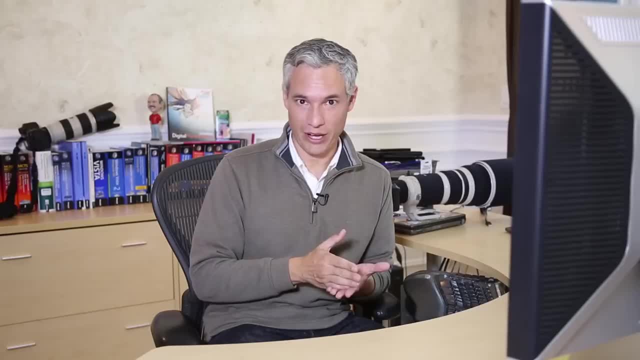 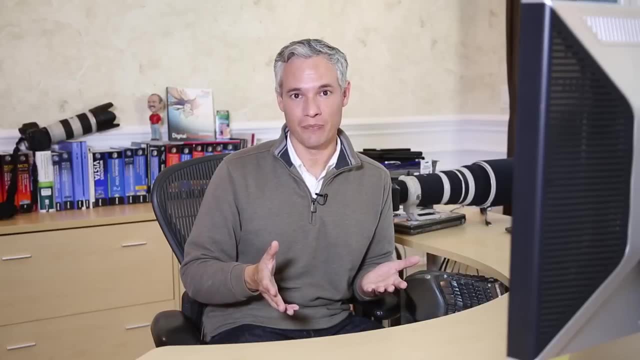 can take is gonna slow down a lot Like it's gonna go from being four or five pictures in a second to one picture in a second. So if you find that you're running out of buffer all the time, might be better to switch back to JPEG. It also. 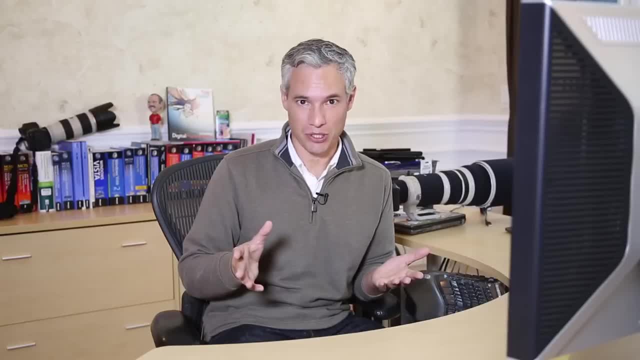 takes up a lot more disk space. If you take thousands of pictures a week, you could find yourself buying a new hard drive pretty soon. But nowadays hard drives are so cheap I say: go for RAW, delete the pictures you don't need and 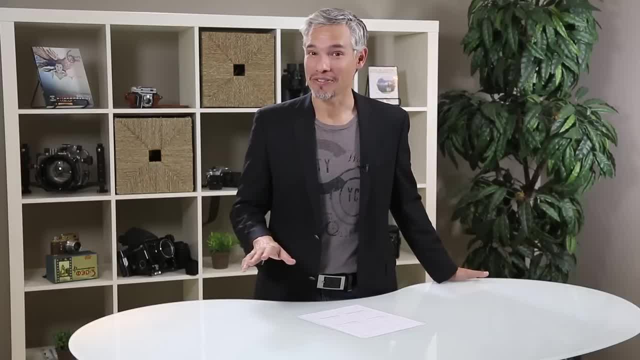 you probably won't have any problem with it at all. Even if you're not editing your pictures now, you know, if they just go straight on Facebook, you in the future might want to edit your pictures, Or, who knows, maybe your kids or grandkids. 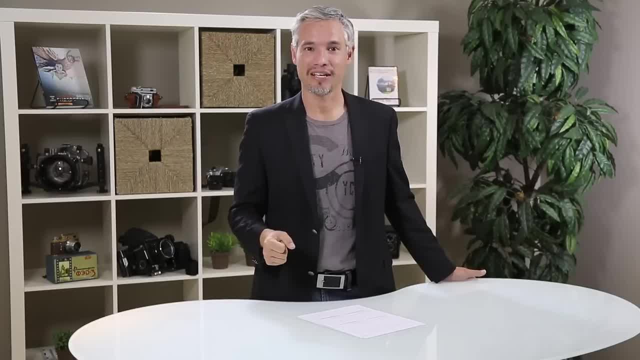 will look back in these pictures and they'll want to be able to extract all that detail out of it. If you store all your pictures in a highly compressed JPEG format, sure you'll save a little disk space, but you're losing important parts of. 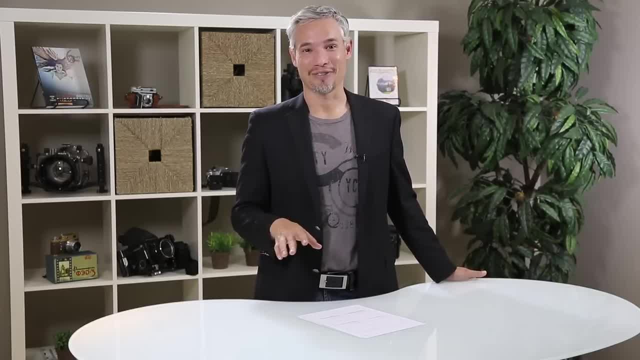 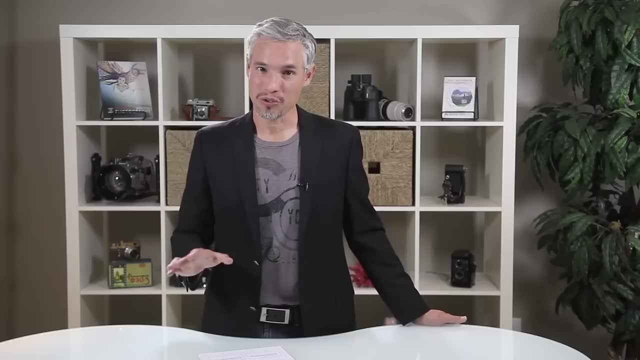 your memories. Anyway, shoot RAW. that's the quick answer. Now I can talk all day about camera settings, but it's not gonna make any difference to you until you actually start to apply these techniques. So here are some practices that you can. 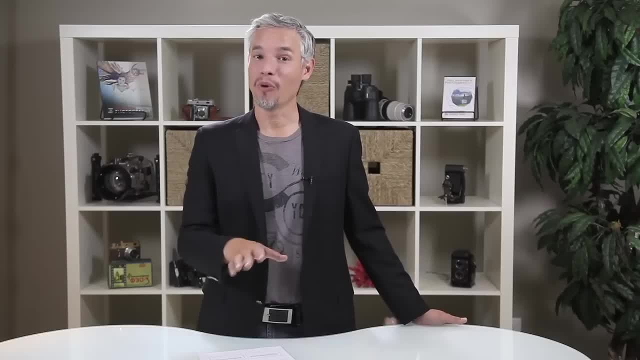 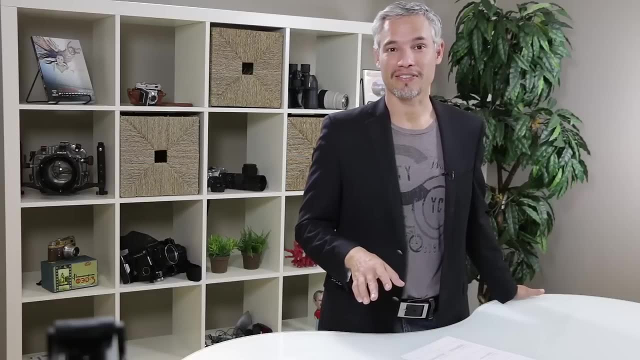 do to get better at controlling your camera. before you need to actually take great pictures. The first thing I like you to do is to practice your auto focus techniques in different ways. Let's say you're using your camera in well-lit environments, So you've probably 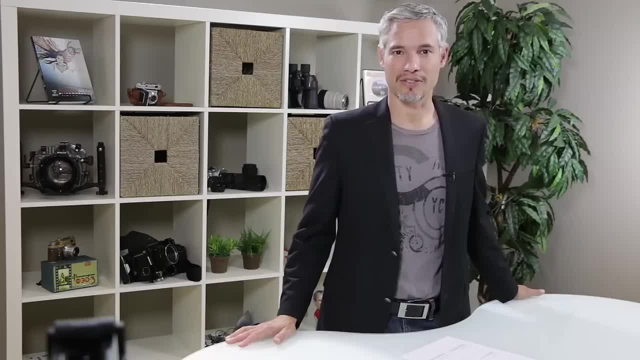 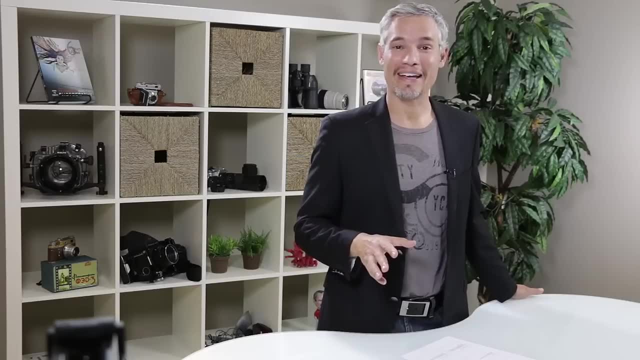 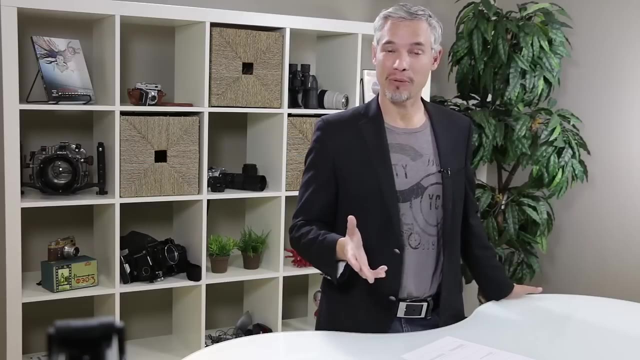 already used your camera in well-lit environments and maybe you've even seen your auto focus fail in some circumstances, but now we'd like to deliberately induce the failure. So take your camera and point it at a completely blank wall and try to focus it. What happens, You know, your camera might. 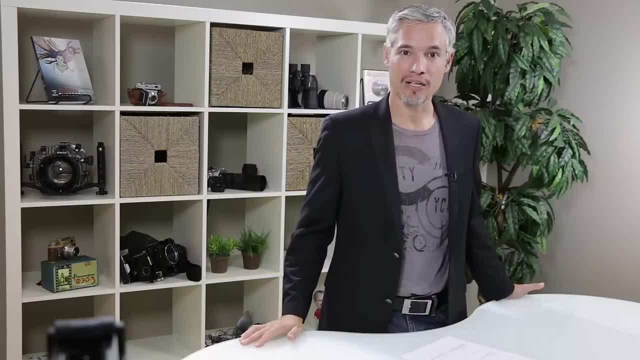 actually be able to focus. Maybe it finds little bumps on the wall or something that it can focus on, or maybe it fails. If it does succeed, well, just turn the lights on. If it does succeed, well, just turn the lights on. 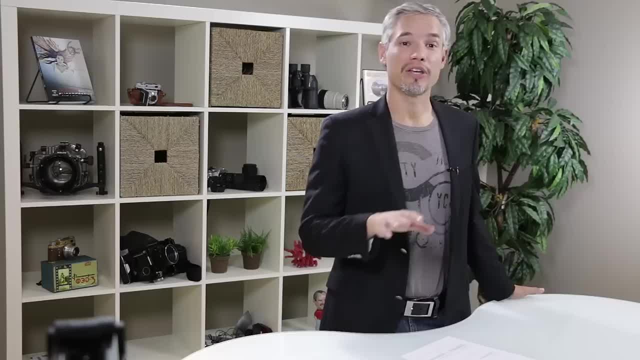 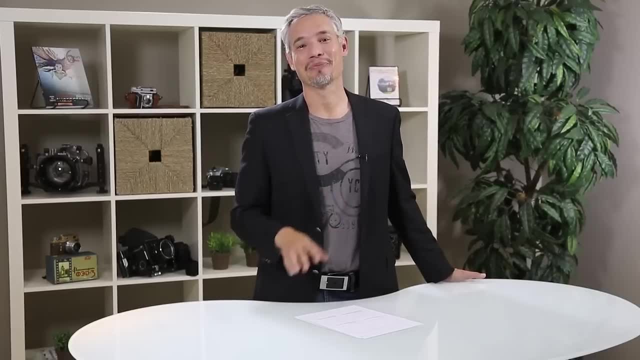 Or go to a darker room At some point, with darkness and a completely plain subject, you're gonna find that your camera will be unable to focus. And that's gonna be a really important concept for you to understand, because no matter how much you spend on your camera, there's gonna be some point when auto focus is. 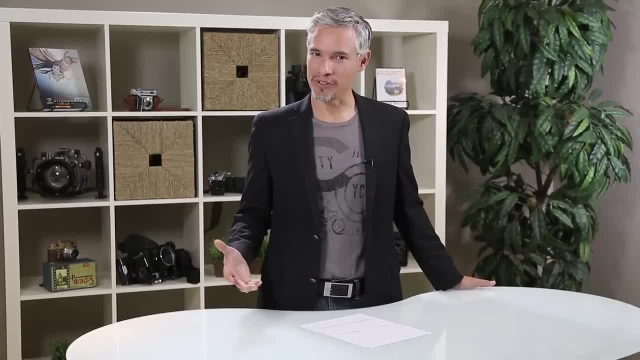 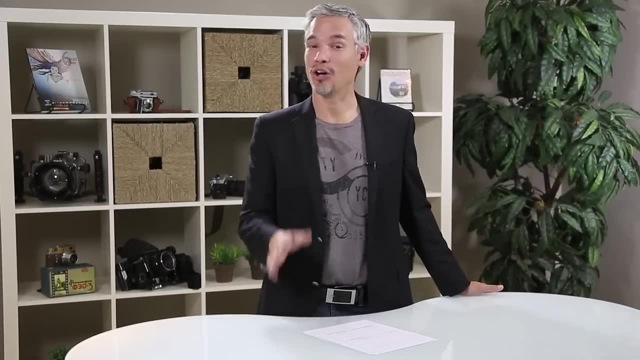 going to fail you, And usually with modern cameras, manual focus isn't gonna be a great replacement either, because it's also gonna be so dark that you can't see enough detail with your eye to properly focus. So you know what to do, right, Because you were listening earlier. 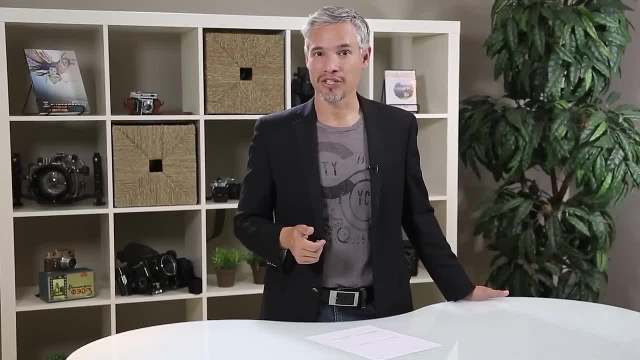 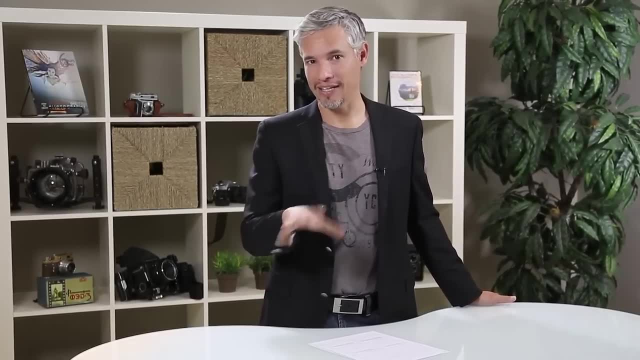 You can turn your flash on or connect an external flash. Often the flash will flicker to allow your camera to focus a little bit better. Or maybe it has an active focusing system where it will broadcast out some infrared beams that your camera can pick up and focus on. You could also focus on an area of 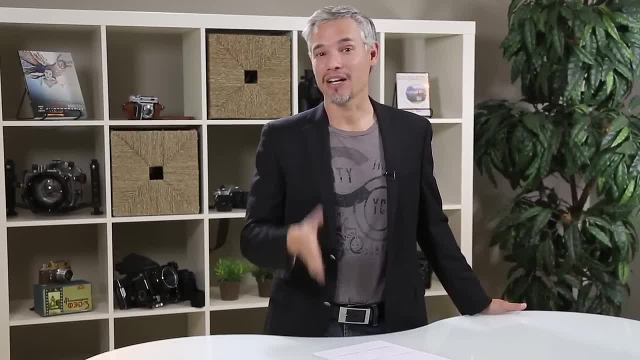 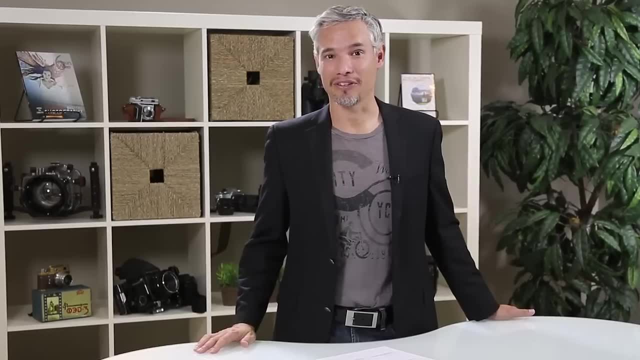 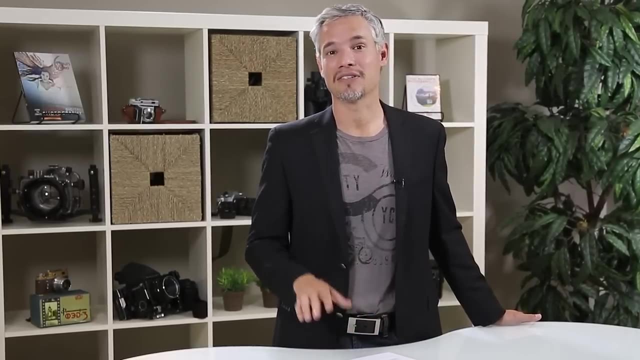 contrast, Like, instead of focusing on that blank wall, focus on a beam or a point of color, Or you could simply turn the lights up. That's something I do a lot with night photography when I'm having a difficult time focusing. So grab your camera and get out there and push it to its limits. Get some practice. 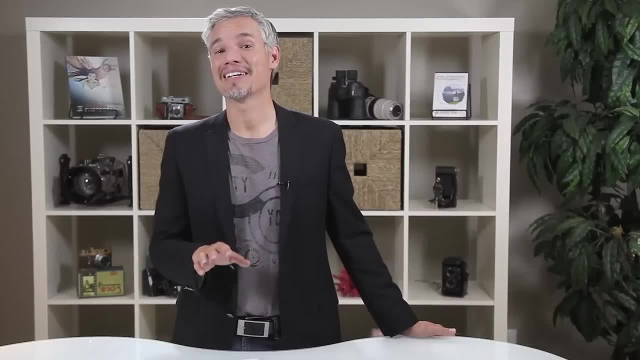 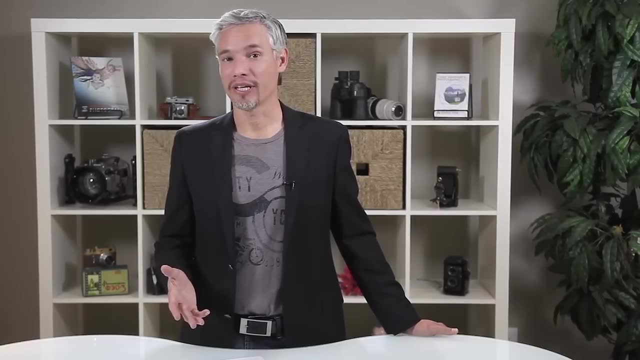 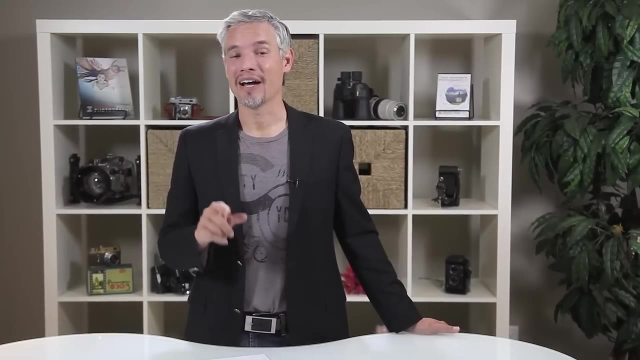 dealing with autofocus when it fails. Now I'd like you to get some practice manually focusing. So take the fastest lens you have, preferably a telephoto lens. By fast, I mean a lens with a really small f-stop number. If you just have your kit lens, that's fine too. Now, if it's a zoom lens, I want you to zoom. 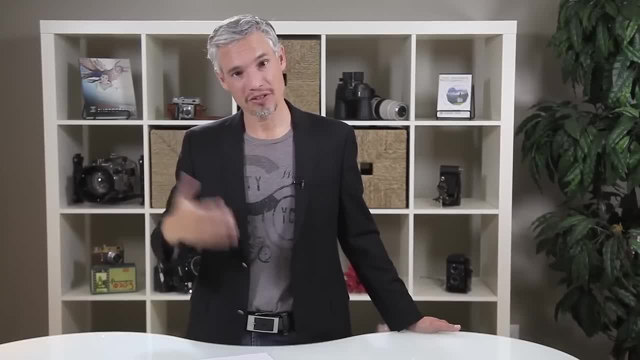 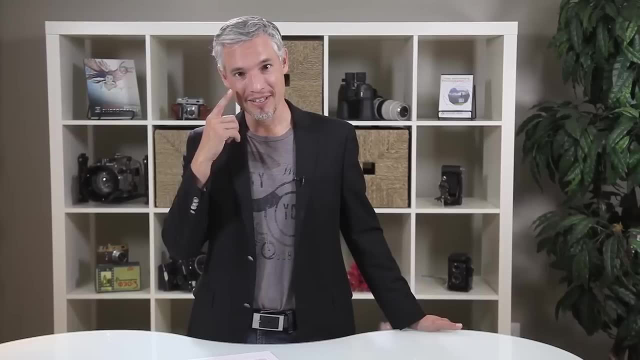 all the way out to the longest focal length and focus on a subject that's pretty close to you, Maybe a few seconds, maybe a person. Use autofocus and focus right on their eye, using a single focus point, and take a picture. Now focus on something in the background. 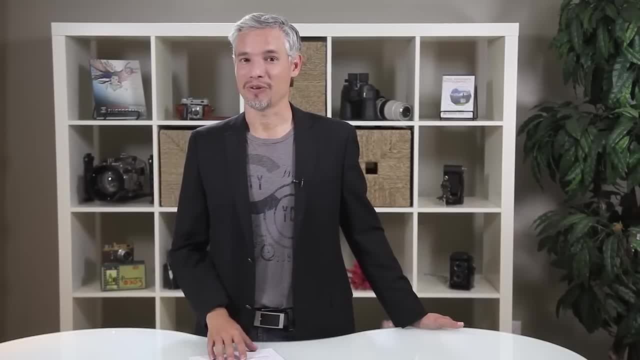 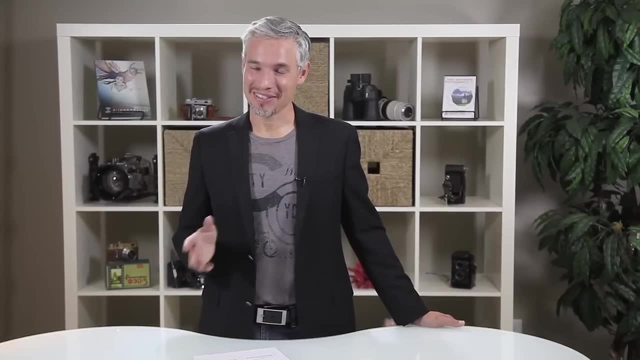 Now I want you to repeat that exact same picture using manual focus. So turn your camera's autofocus system off- there's usually a switch on the lens- and try to manually focus and take a couple of pictures. Now load those pictures on your computer and take a look. 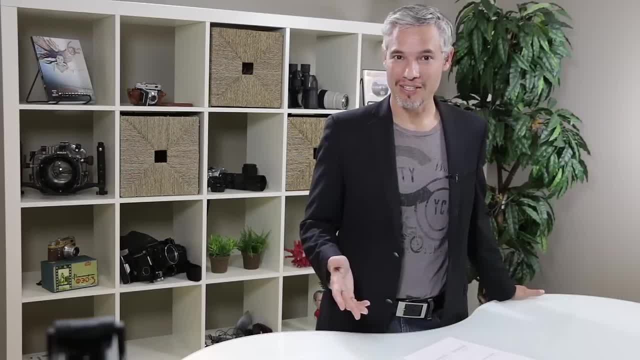 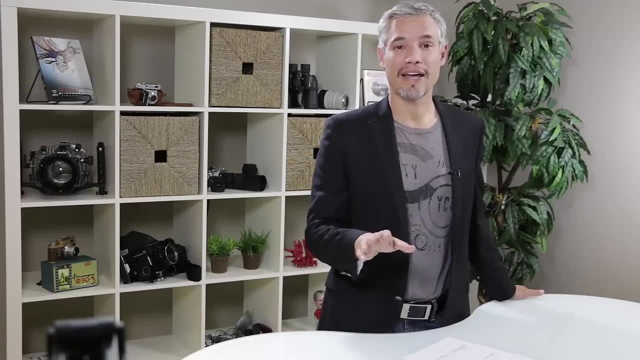 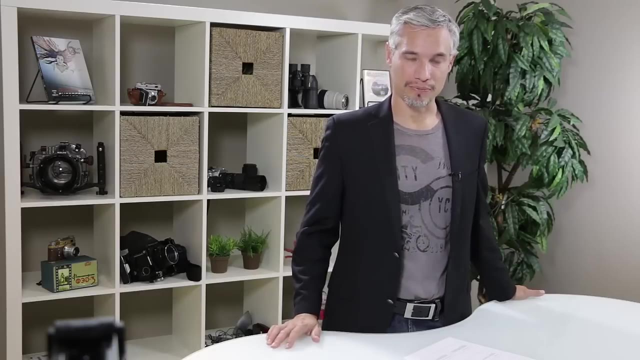 What did better, your manual focus or the autofocus? Well, if you did everything properly, the autofocus is usually going to do better, But I want you to understand the differences and I want you to get some practice switching between autofocus and manual focus. 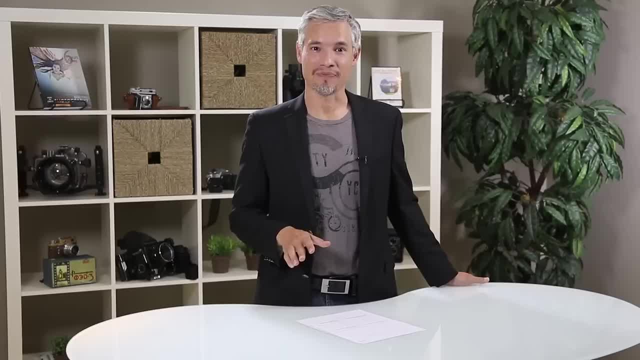 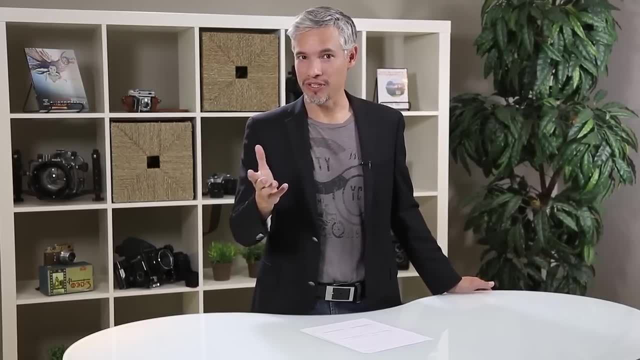 Now I'd like you to practice the focus recompose technique. So, using just the center autofocus point on your camera, focus on a subject, for example a person, and then recompose the picture so that they're in the right or left. third of: 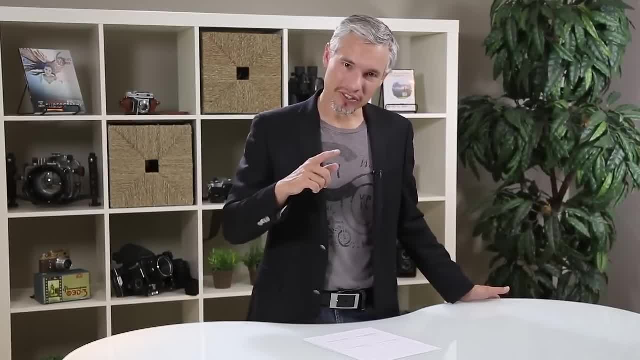 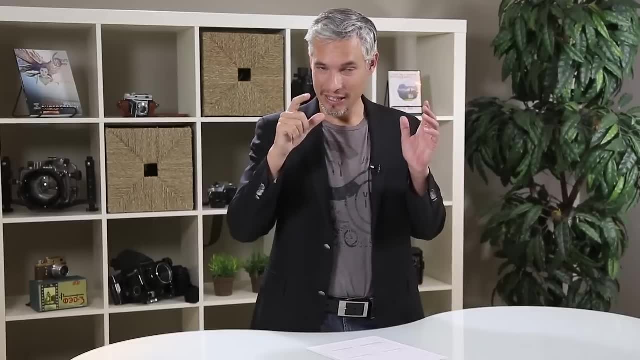 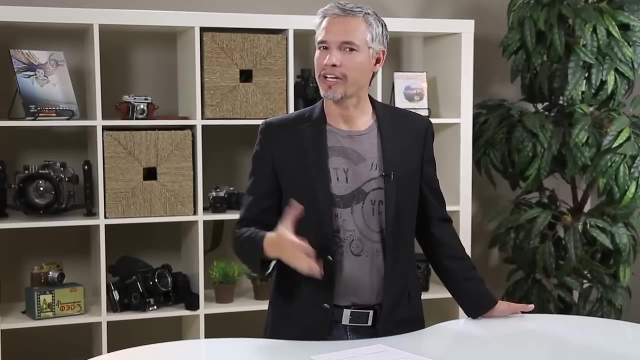 the frame, Go around and pick a few different subjects, Focus and then recompose. Remember to focus. you'll usually put the shutter button halfway down and then keep it held down while you recompose- Focus. recompose is a really important technique for getting more creative with your composition. 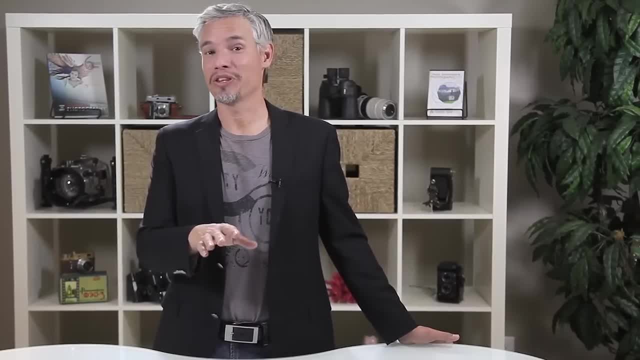 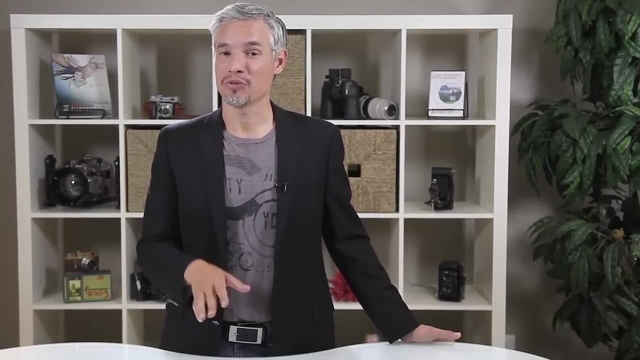 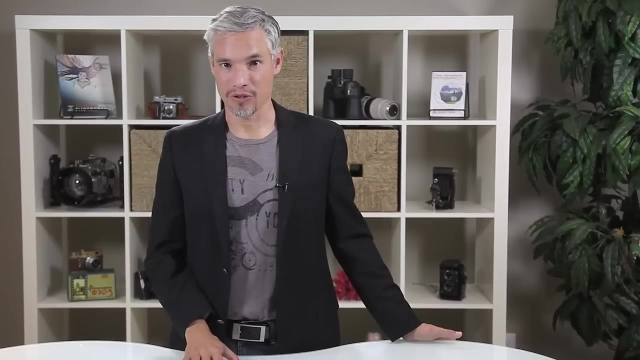 Now I'd like you to get some practice using continuous focus. So, with the focus recompose, you had to be using AF-S or one-shot focusing. With continuous focus, you're going to use AF-C or the AI servo focusing on Canon cameras. Continuous focus will track whatever is in front of it and try to focus as fast as possible. 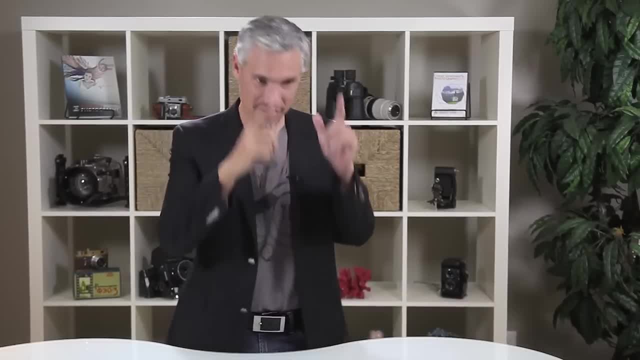 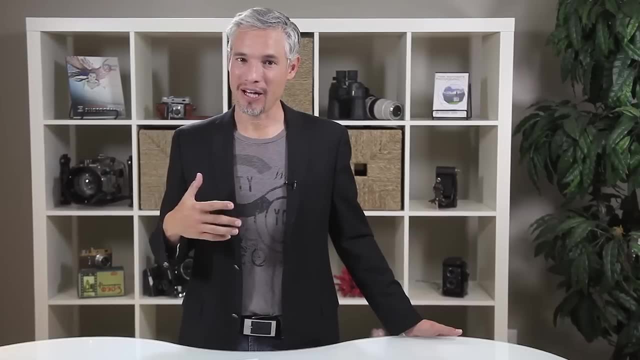 on it. So just turn it on and kind of move, focus on subjects at different distances in the room and the world outside and see how fast your camera responds. You should be able to focus on something close and then focus on something far away without even lifting your finger off the shutter. 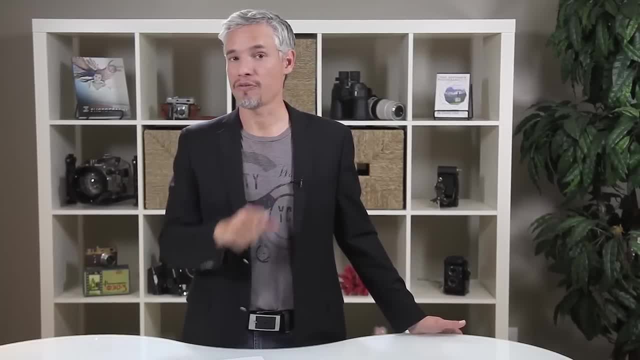 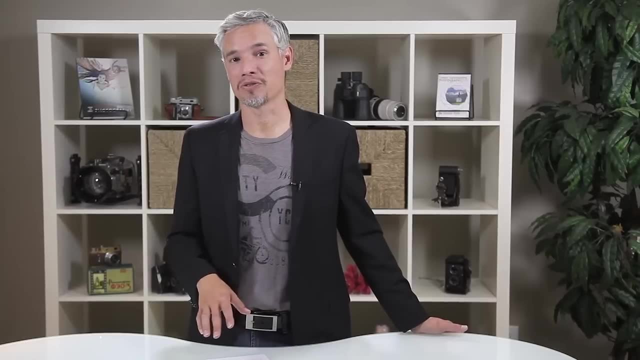 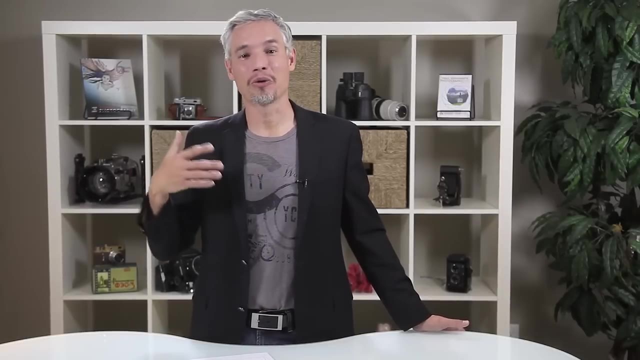 That's a great tip. You might also want to take your camera out and practice with a moving subject. You could even just go down to the street and focus on cars that are coming towards you, Or maybe you could corral your kid and get them to run towards you so that you could. 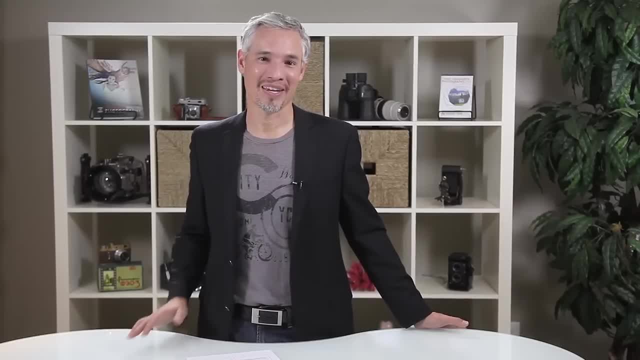 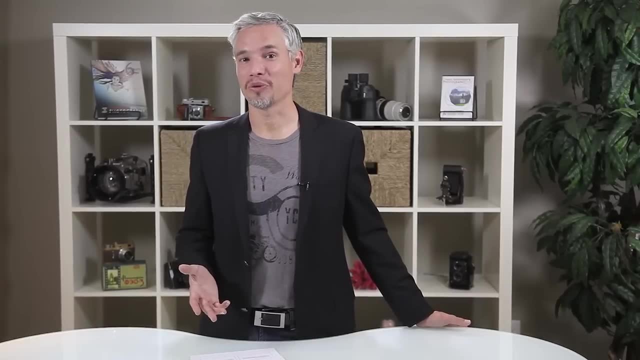 practice working with continuous focus and taking pictures with it. Now I will note: don't be disappointed if some of your continuous focus pictures don't work Or if your camera seems to struggle with continuous focus. depending on the camera you have, the lighting conditions and the amount of contrast in your subject. continuous 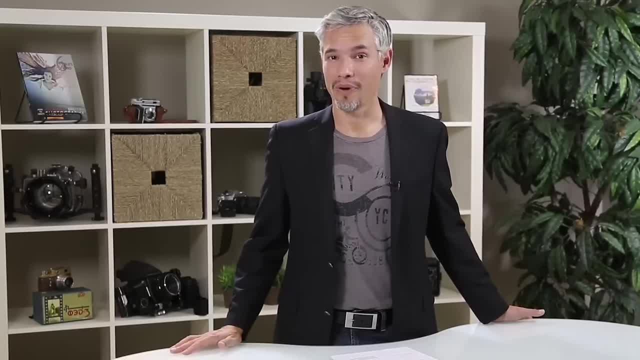 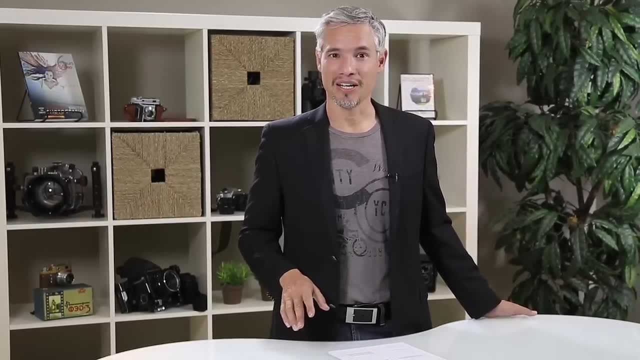 focus can be a real challenge for cameras, So let's get some more practice with moving subjects, Again using continuous focus. I'd like you to take two sets of pictures. Find a kid or friend or person, or just go out to the street and find some cars that 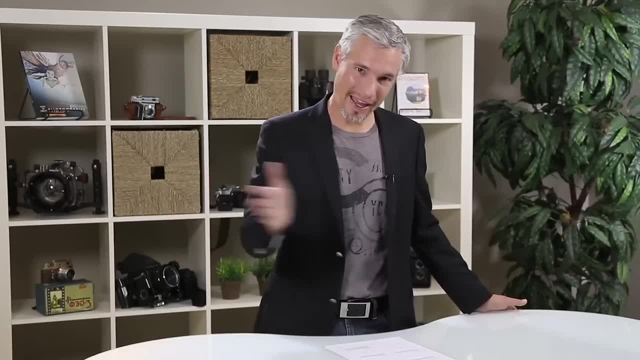 are driving past First. I'd like you to kind of pan with the subject. I'm going to take a picture of a car. I'm going to take a picture of a car, Or I'm going to take a picture of a person driving past. 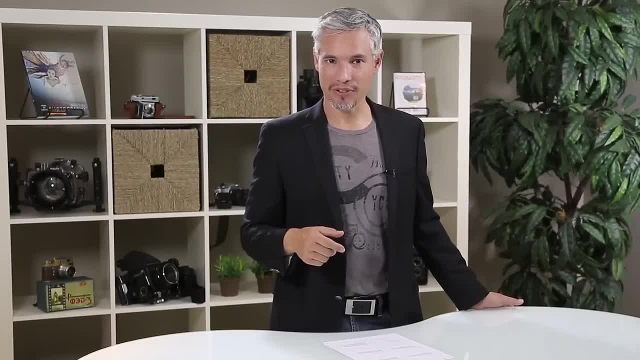 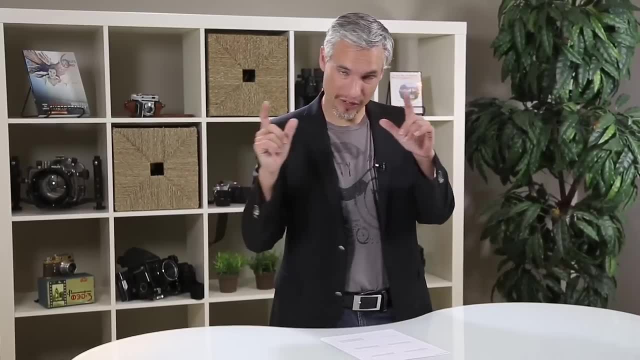 And finish it off with the subject moving from left to right. So set your camera to continuous focus and keep your finger half-pushed on the shutter button and keep the subject in focus as it goes from left to right. So set your shutter in to continuous and take as many pictures as you can. 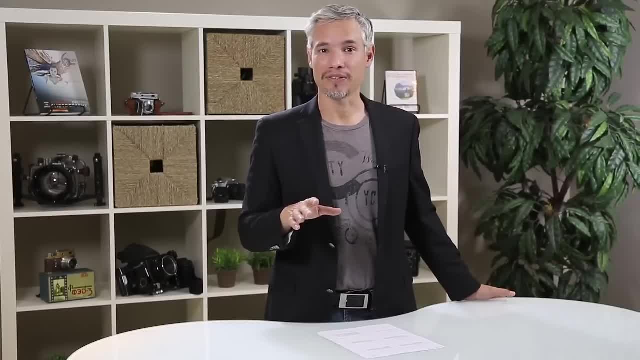 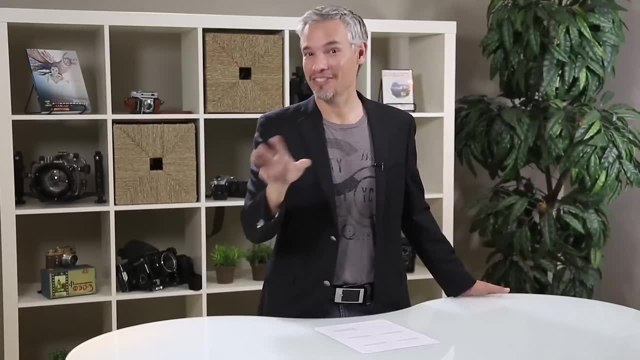 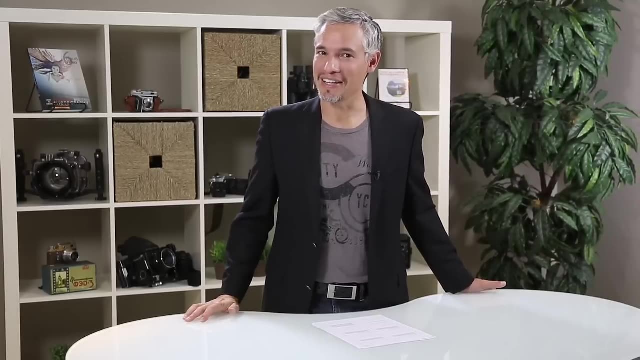 Do this a couple times Now. I'd like you to repeat that process with the subject coming towards you. So get your kid to go a little bit away and then run towards you or stand near traffic so that it's coming towards you, towards you. and I want you to go back to the computer and unload those pictures and 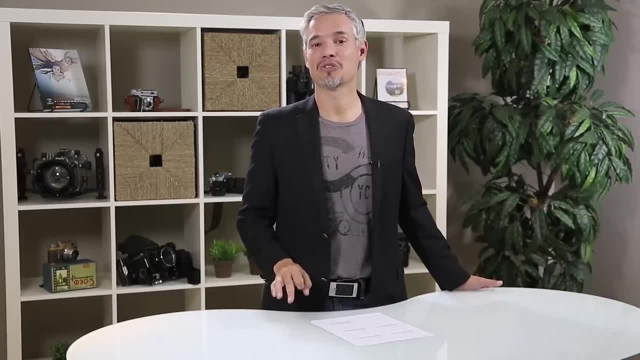 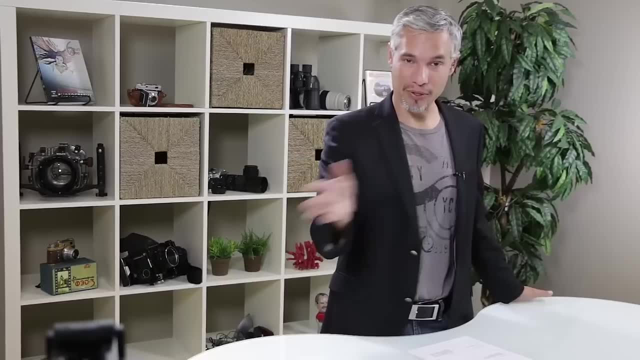 then look carefully and see how many of each were in focus and out of focus, For example. find out whether you got more pictures in focus, panning from left to right or when the subject was coming towards you. Now let's get some basic exposure practice. 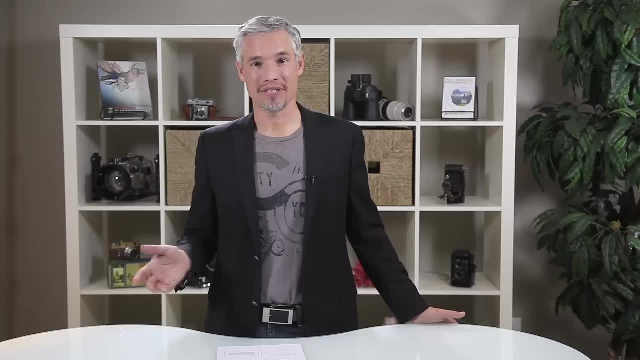 I'd like you just to put your camera in completely automatic mode and take a picture of something indoors Now go outside during the day and take a second picture and just look at the settings. Usually you can just review them in camera and hit that info button a couple of times. 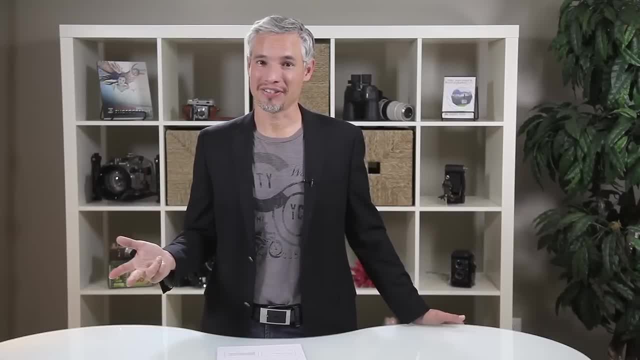 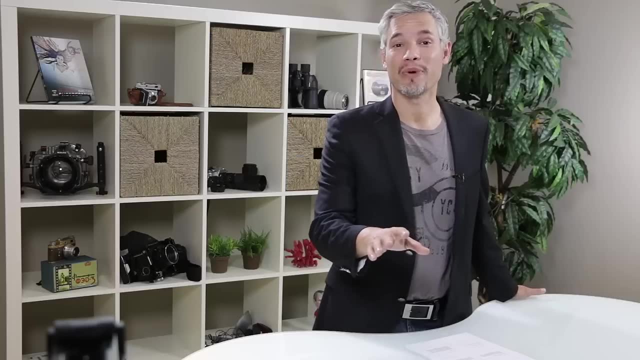 until it shows you your shutter speed, aperture and ISO. What were the differences between the different settings and are they what you'd expect? Here's another exposure practice. I want you to take a picture with your camera in fully automatic mode, then review that. 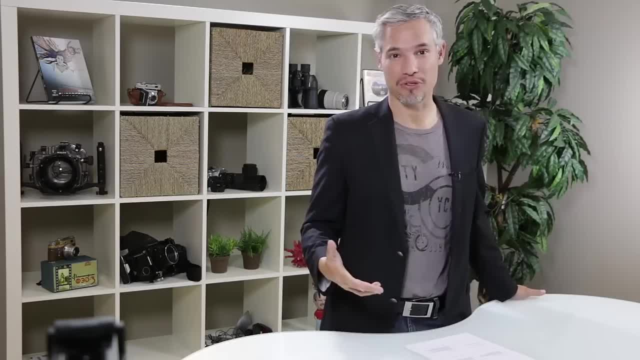 picture and hit that info button until you can see the shutter speed, aperture and ISO. Make note of those. Now switch your camera to manual mode and set the ISO, aperture and shutter speed to those exact same settings. Now take another picture of the same subject. 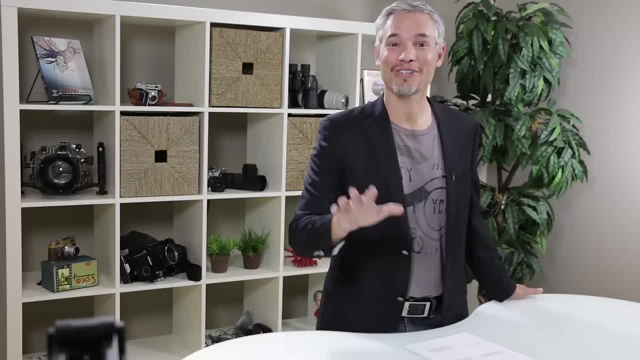 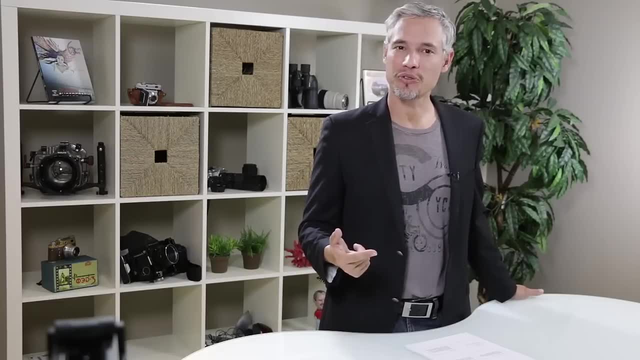 It should turn out properly exposed, right. So congrats. you took your first manual picture and you're well on your way to understanding how to manually control your camera. Now I want you to cut that shutter speed in half and take another picture. 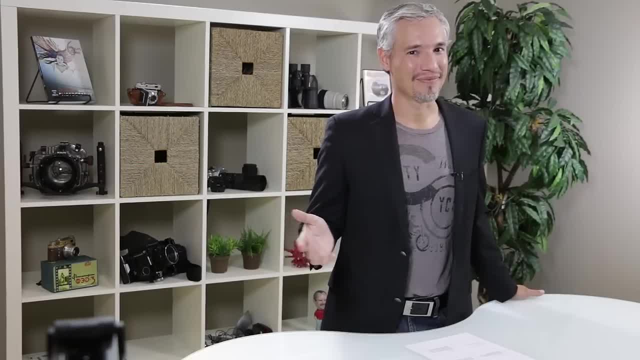 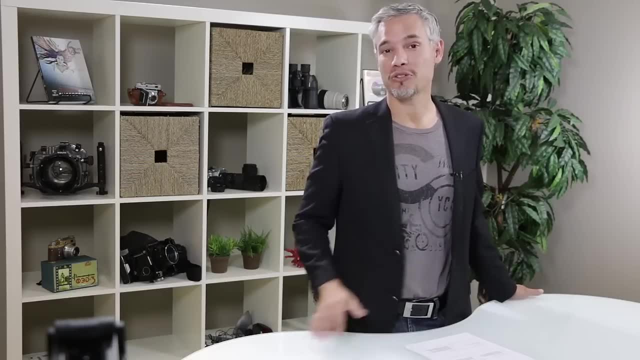 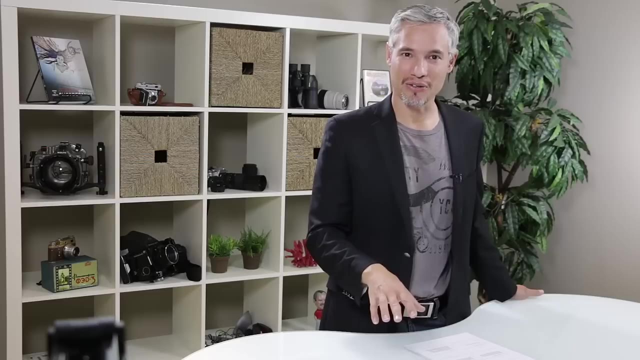 What happened? Did it come out darker or brighter? Now move the shutter speed the other way and determine whether it came out brighter or darker. You can set your settings back to the original set of settings and do the same practice with your aperture and ISO, determining whether your pictures get darker or brighter as you. 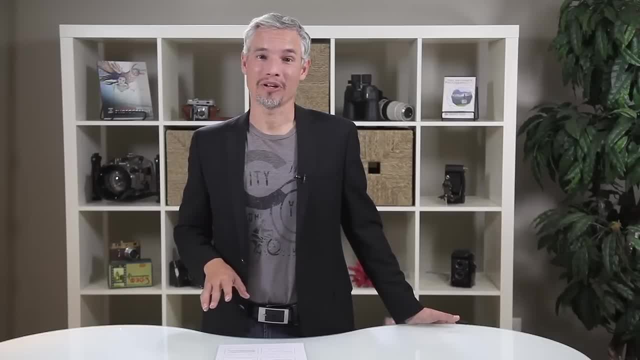 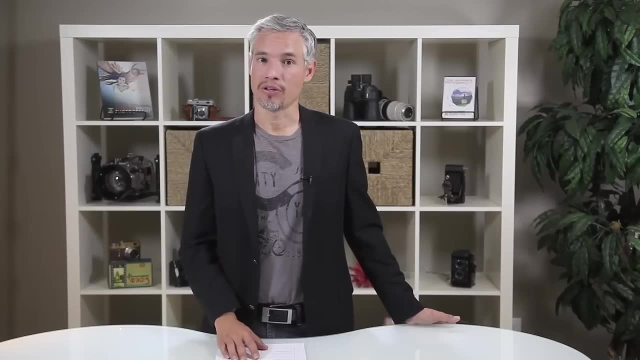 go Now. set your camera to shutter priority mode. In shutter priority mode your camera controls the aperture and the ISO. if you set it to auto ISO and you control the shutter speed, So you make that one decision- how fast that shutter is going to be and your camera can. 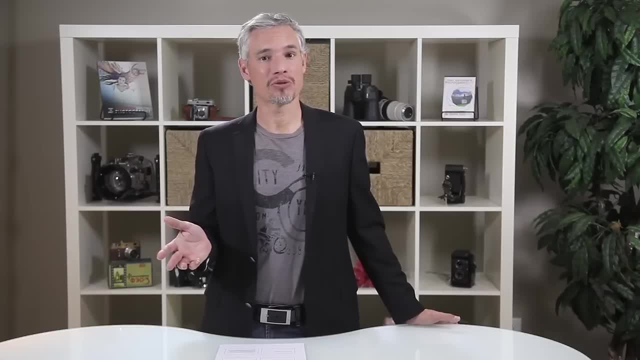 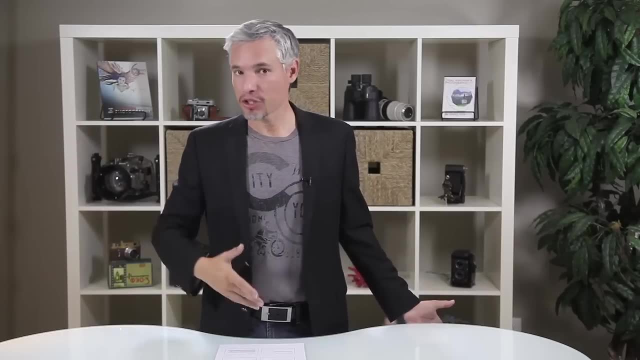 decide everything else. So try just taking pictures of moving subjects whatever you like, at different shutter speeds. A fan is good, or you could have your kid wave like this. You know, take a picture at 1, 30th of a second, 1 1,000th of a second. 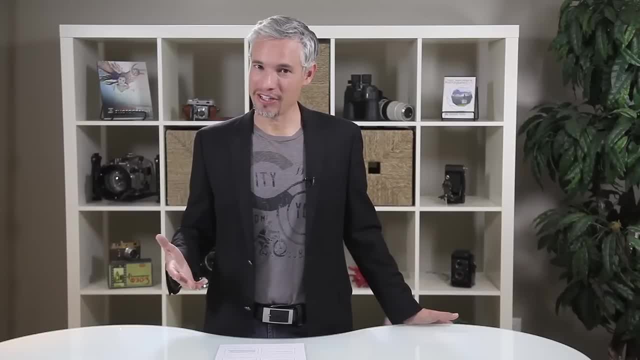 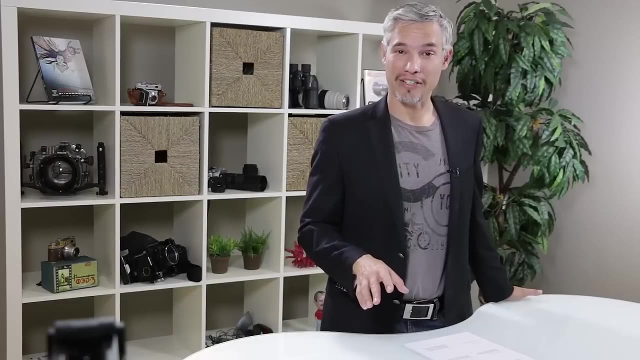 Think about how fast something is moving and try to find that shutter speed that freezes it and that shutter speed that shows just a little bit of motion, and how much shutter speed you need to control. Anyway, play with your shutter speed. I'd also like you to perform the same practice using aperture priority mode. 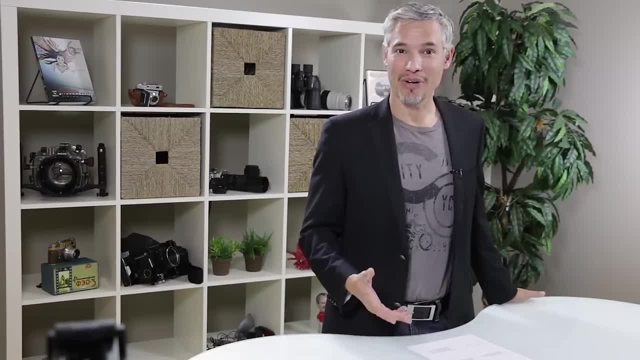 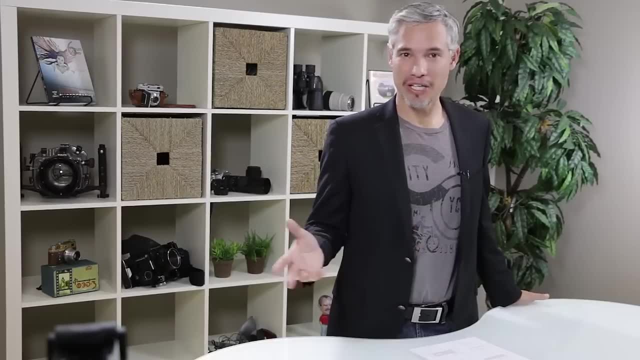 Set your camera to aperture priority mode and set your ISO to auto ISO. Now use that main dial and use the lowest f-stop number you can and take a picture of something fairly close up. You should see stuff in the background that's a little bit out of focus. 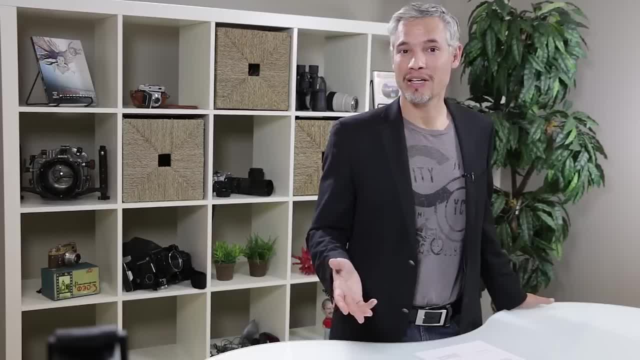 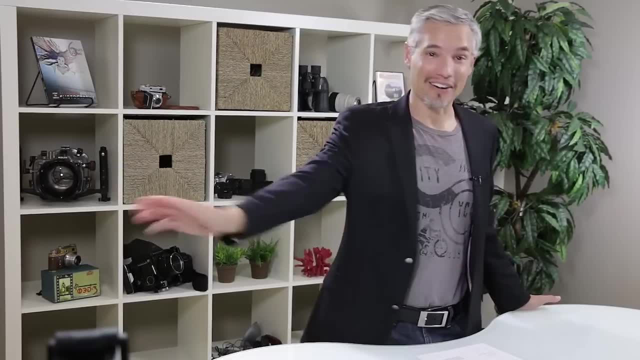 Now try using a higher f-stop number and see what happens. Experiment by zooming in and zooming out, being close to subjects and far away from subjects. Try to get an entire scene in focus, using the depth of field practices that we talked about earlier. 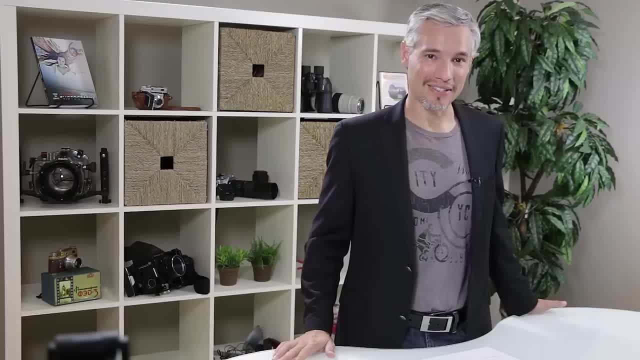 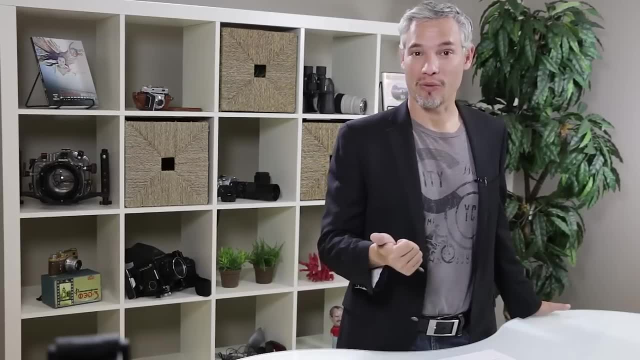 Also specifically try to blur the background, to isolate the subject. Remember the different techniques that we used: using a low f-stop number to blur the background, zooming all the way in tight using a long focal length or a telephoto lens and getting just as close to your subject as possible. And again you can see a lot of action there, with just a little bit of ambient noise. So I'm going to switch back to shutter priority mode And again we're going to try and do this with auto or auto-focus as your camera's. 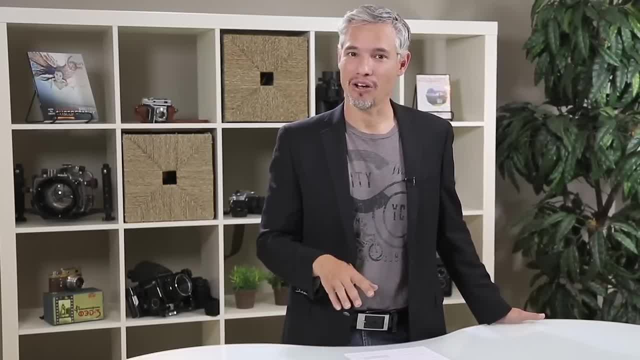 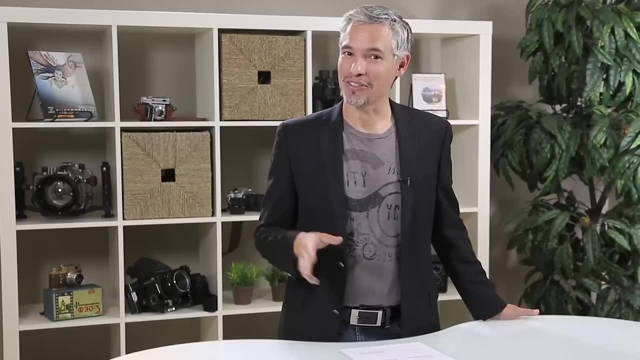 focusing will allow Switching back to shutter priority. I'd like you to again use auto ISO. This time. we're going to practice hand holding your lens and seeing just how slow you can get and get a good picture. So if you have a lens with image stabilization or VR- whatever it calls it- go ahead and 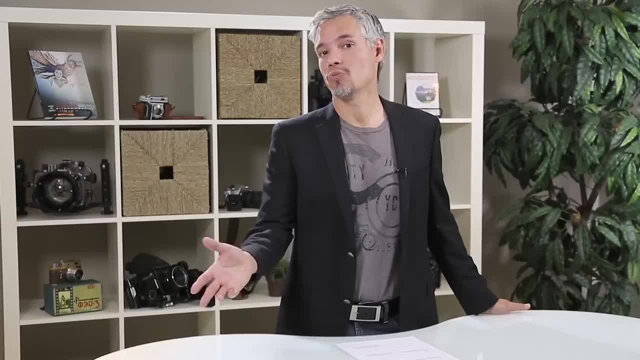 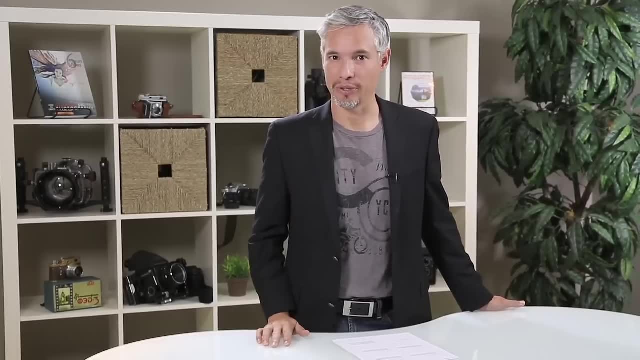 turn that on Now. start out at, say, one 250th of a second and take 10 pictures of a fairly close up subject. Okay, here we go. if you zoom in a little bit, Then drop that shutter speed in half, So go down to 1, 1, 25th. 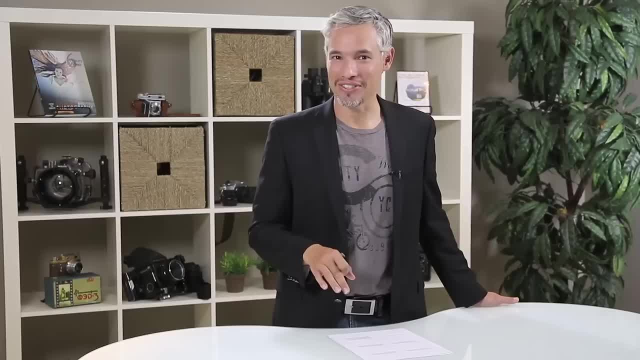 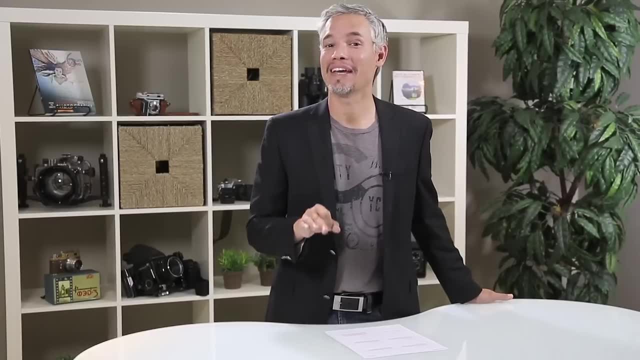 and take 10 more pictures, Go in half again down to 1, 60th- 10 more pictures and just keep cutting the shutter speed in half and taking 10 more pictures until you get down to a quarter of a second. Now I want you to unload all those pictures. You'll probably have like 100 pictures. 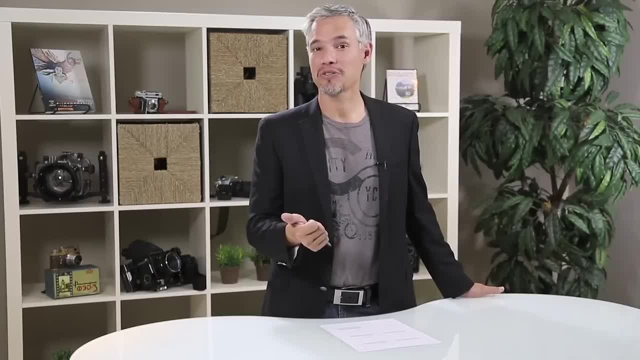 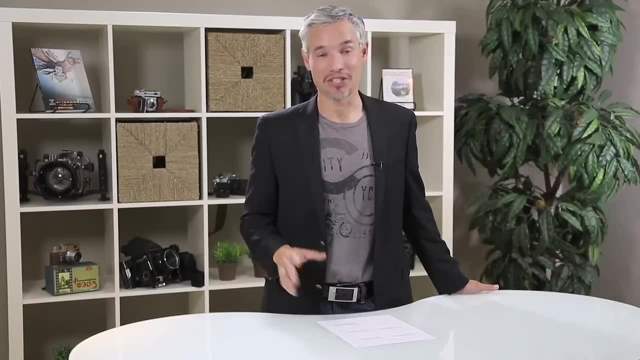 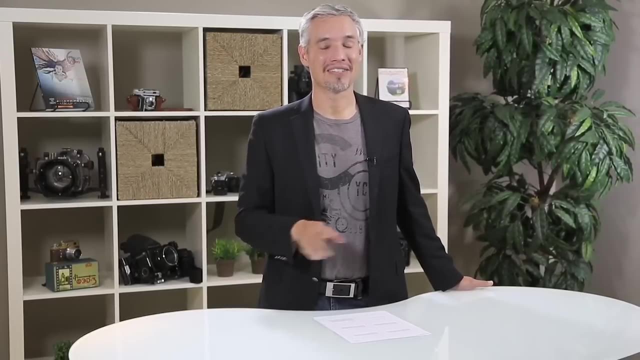 and go through each set and count. How many pictures did you get nice and sharp at 1 250th of a second? How many did you get at 1 125th of a second? Did you get any sharp at one quarter of a second? How slow can you handhold a picture? This is a great way to practice your handholding. 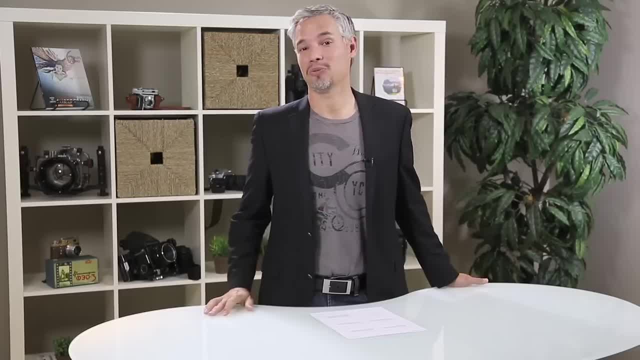 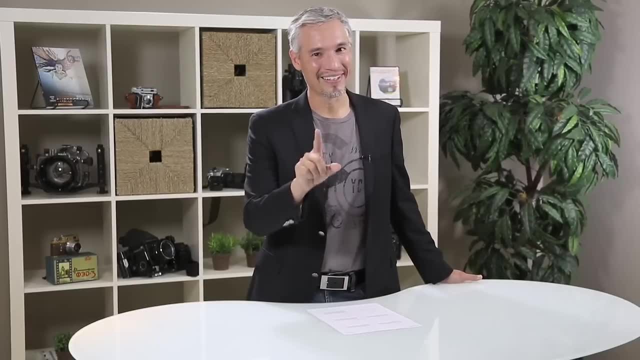 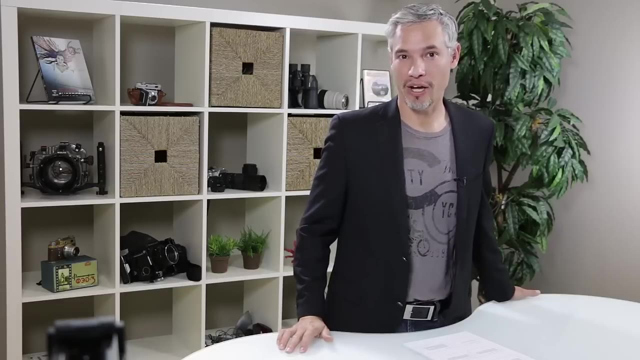 techniques, but it's also really good just to know what the slowest possible shutter speed is, that you can handhold a picture and how many pictures you need to take to get that. Now I want you to use either the free Picasa or Adobe Lightroom, which has a 30-day free trial. 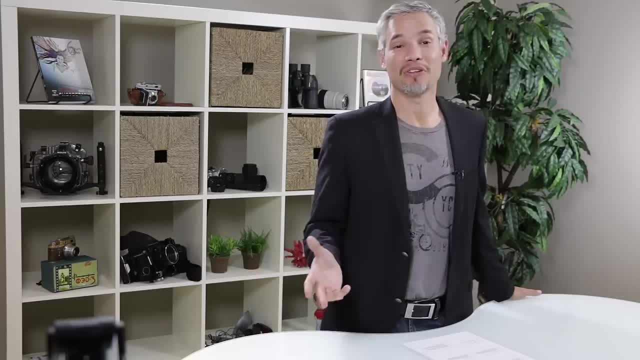 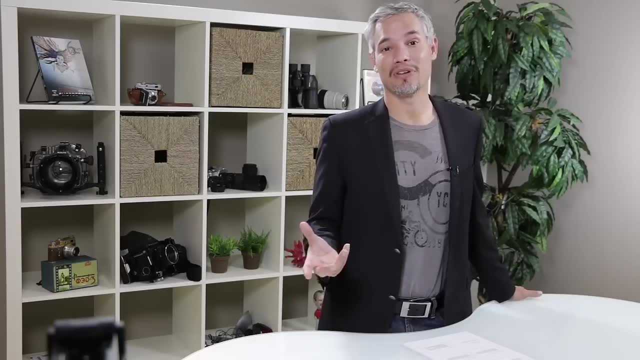 and copy those raw files and process them. Now, if you've been working with JPEG, you'll notice that those raw files are way, way bigger and they probably take longer to load onto your computer. Maybe your computer even works a little bit harder as it's processing them. 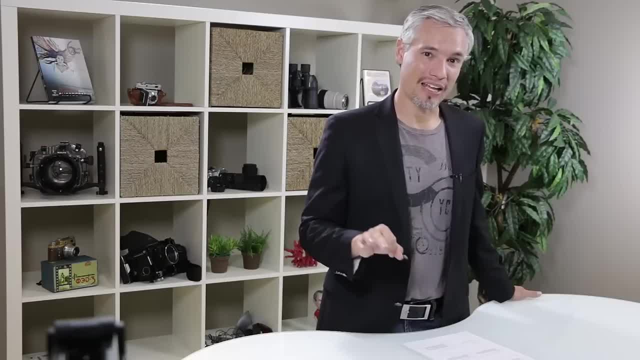 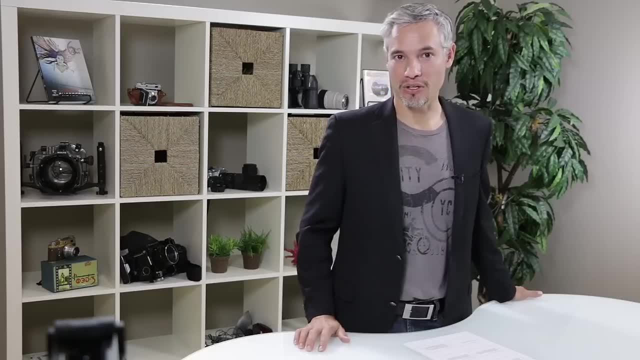 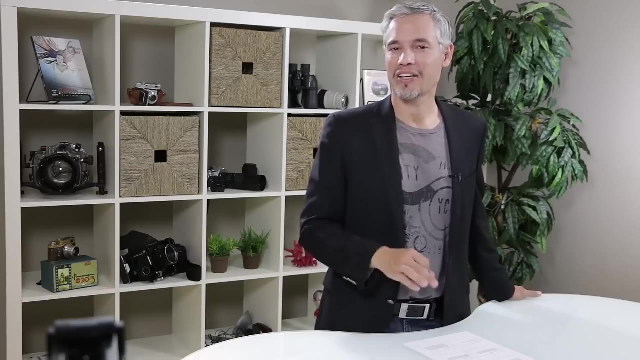 If you get the chance, take some pictures with JPEG and RAW both and see if you can spot any differences. I'd also like you to get some practice working with RAW files, so you kind of know what to expect. I'd also like you to make note of how many pictures your camera reports that. 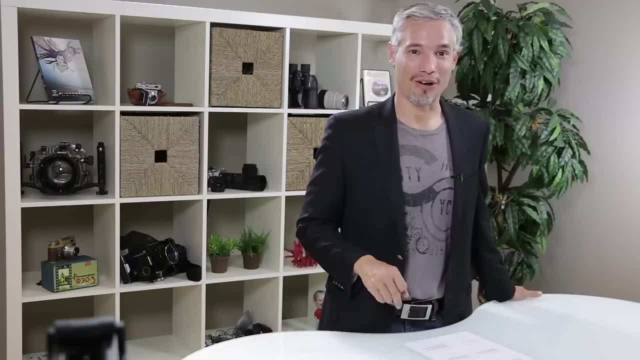 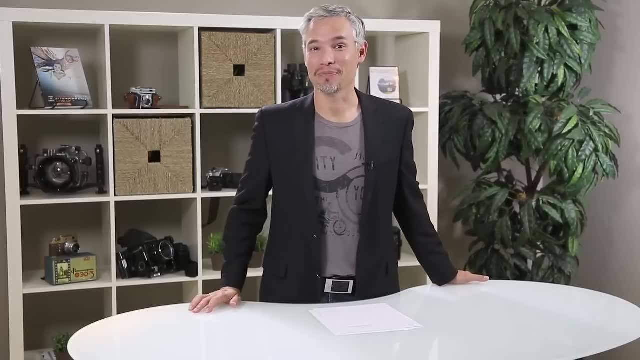 you can take on your memory card in both JPEG and RAW mode, because I bet it's going to be a smaller number when you're shooting RAW. Here's a really fun way to get to know the parts of your camera, and it's going to only 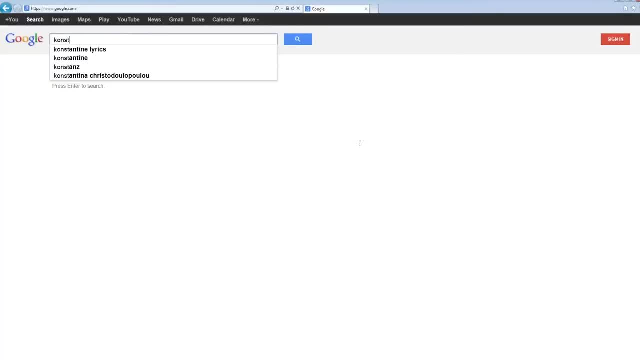 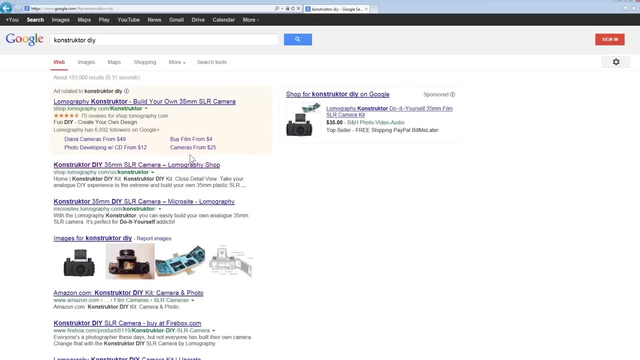 cost you $35.. There's this little link in the description below. I'll put a link in the description below. It's this constructor with two K's DIY do-it-yourself kit that you can buy. It's a full-blown SLR that you build and it takes film pictures. but it works and 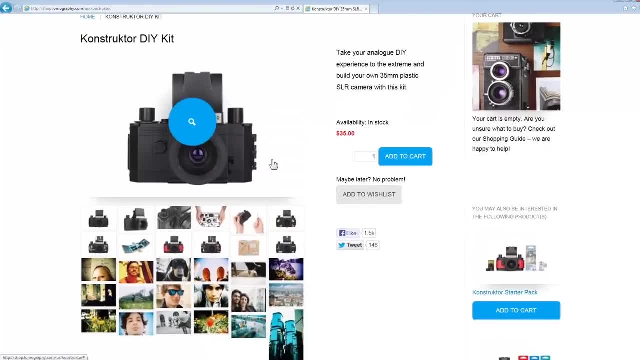 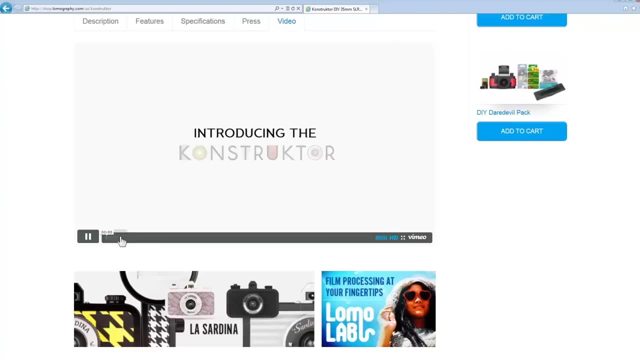 you can still get your film developed. You can send it in to mpixcom and they'll even scan it for you. When you build your own camera, you're going to absolutely master every part of it, from the mirror to the viewfinder and the grip and the shutter and the motion of it. 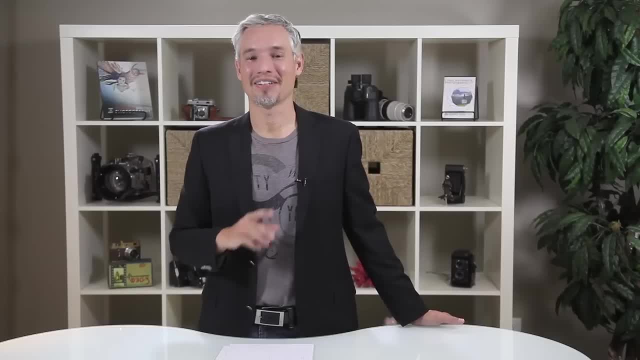 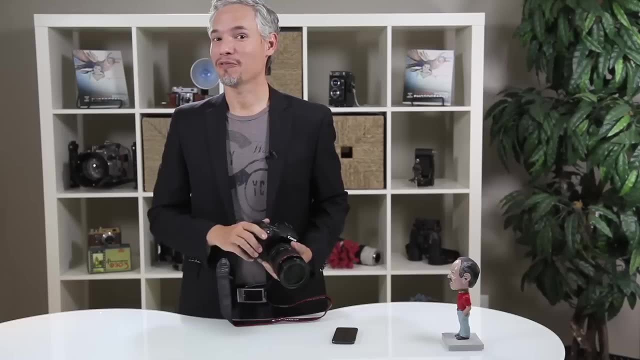 Anyway, it's certainly not. It's not a mandatory practice, but it's a lot of fun. Here's one last practice that might seem a little extreme, but I promise if you do this and keep at it for a week, you will master manual mode on your camera as well as aperture. 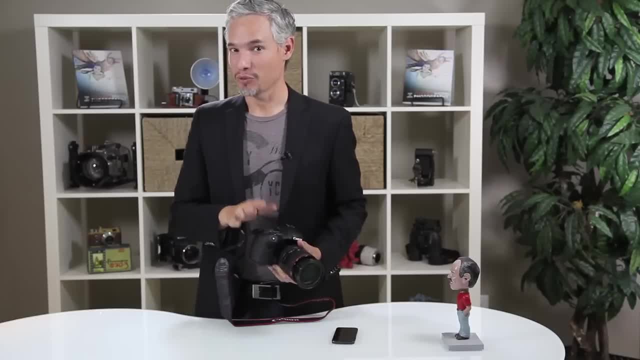 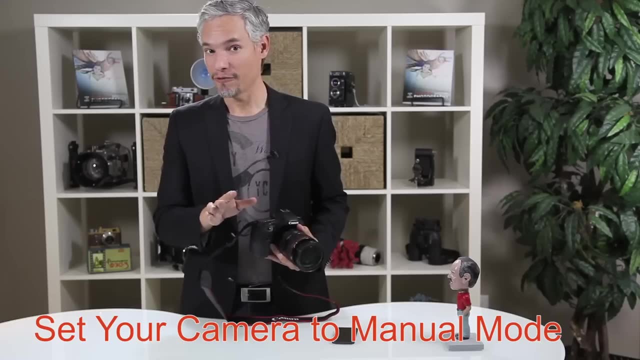 shutter speed and ISO. What we're going to do is we're going to put our camera into manual mode and then we're going to leave it there. So I'll switch my camera over to manual From now on and for the next week, we are going to manually determine the metering for 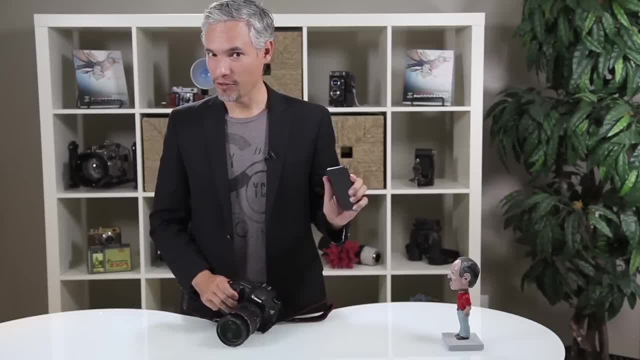 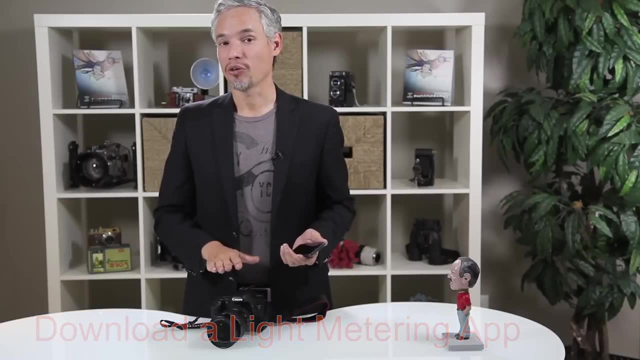 a scene using a smartphone. If you don't happen to have a smartphone, you can use any external light meter, But we're decoupling the metering from your camera, So we're no longer going to use your camera's auto exposure system. 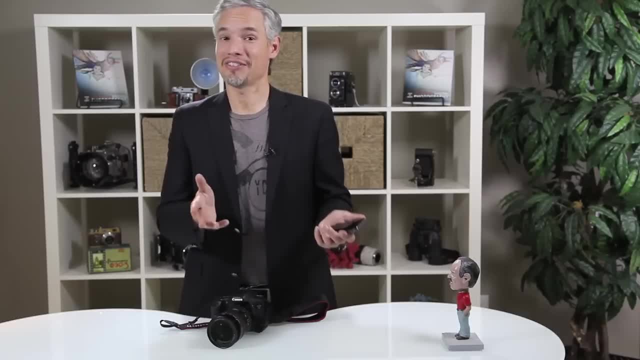 iPhone apps are available for free, as well as Android apps. I'm going to use one that's just called Light Meter, but I promise if you search your app store you'll have an app that can do it. A tablet can work too. 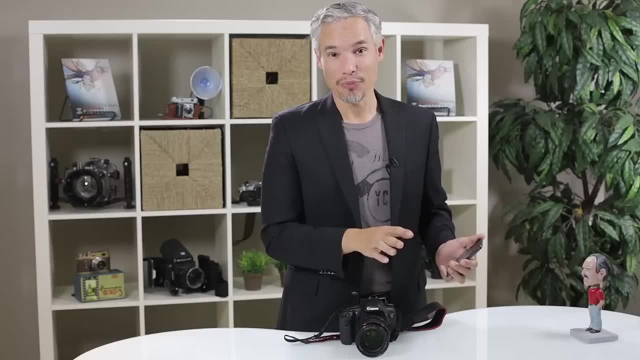 Anything that has a built-in camera will probably have an app available for it. So the first step will be to just pick a general ISO. So I'm indoors here under decent light and ISO 800 is good for that. If I were outdoors in shade, I'd pick ISO 400.. 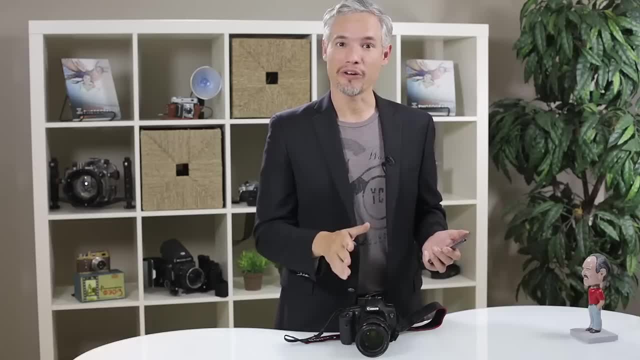 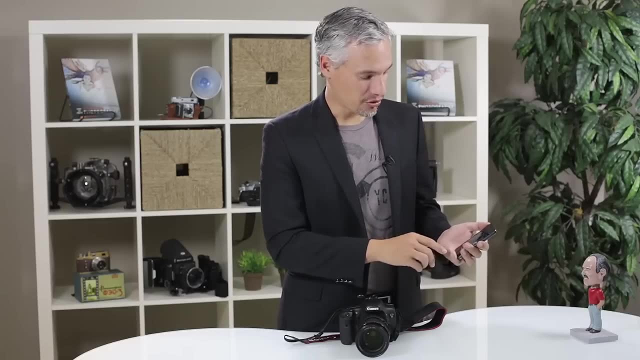 If I were outdoors in full sunlight, I'd go ahead and pick ISO 100. And if you're in a dark room, a bar or a restaurant, go ahead and go for ISO 3200. But for me ISO 800 is going to work well. 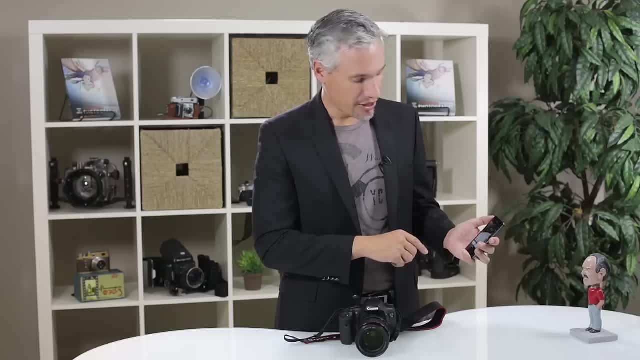 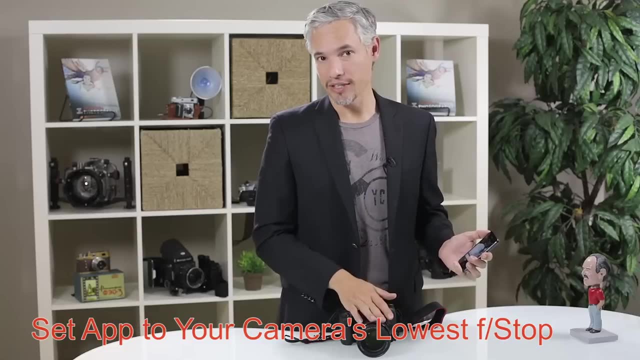 So I'm going to go ahead and pick ISO 800 here, Then for my aperture I'll go ahead and shoot at the lowest f-stop number that this lens supports. For me that's f4.. For your lens it might be f5.6.. 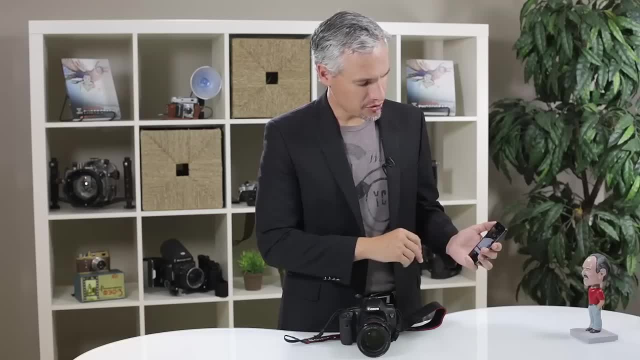 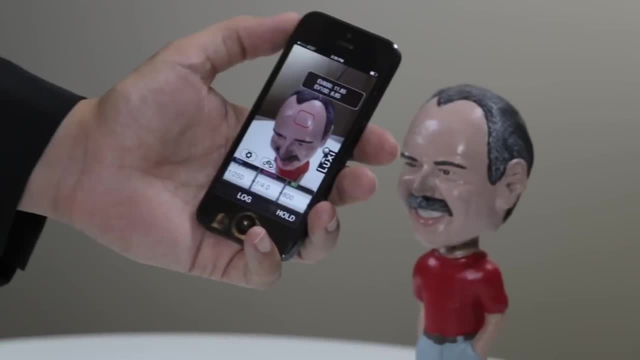 So I'll dial in f4 there and then I'm just going to use this app to tell me the shutter speed that I need to use. So I'm going to go ahead and point the app- it's metering- off the red square there at. 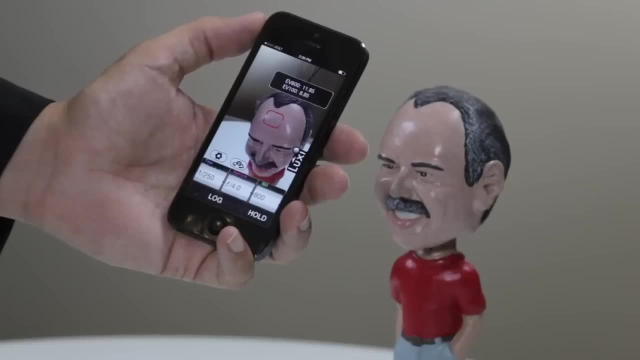 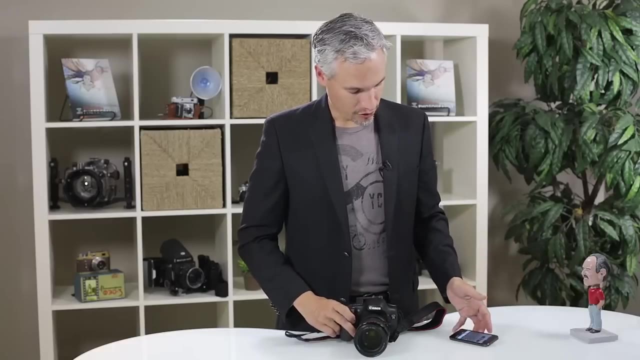 my dad's forehead And you can see it's telling me the right shutter speed is 1, 2 50th of a second. So I'm going to copy these settings into my camera here. So I've got it in manual mode. 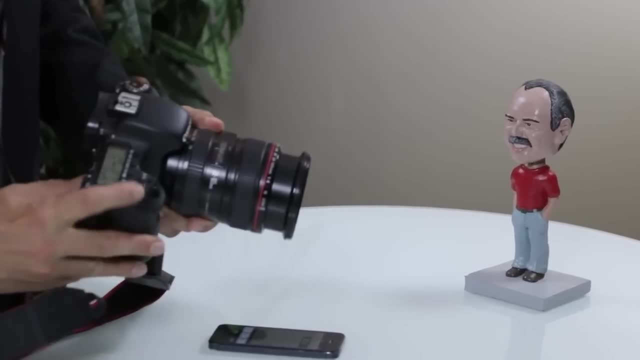 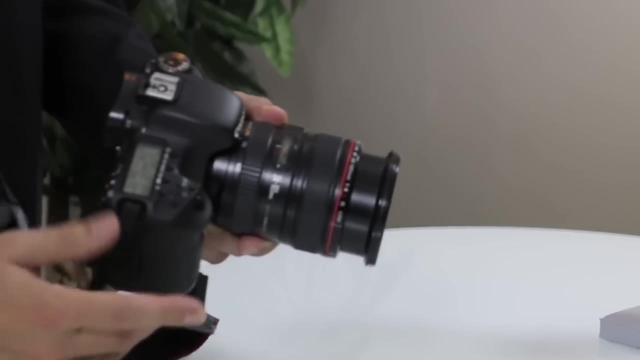 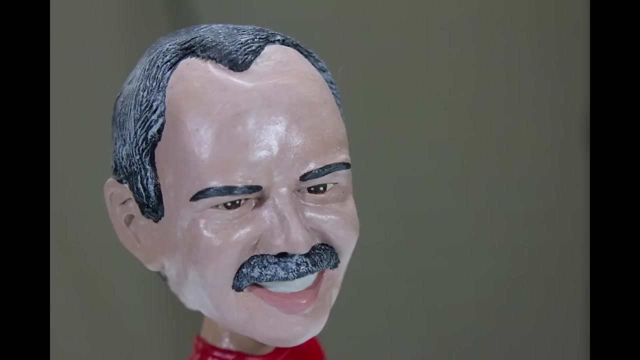 And I'll set it to f4.. 1, 2, 50th of a second And I'm going to manually dial in the ISO. I had it on auto ISO, So now I'll take a picture So you can see that turned out a little underexposed. 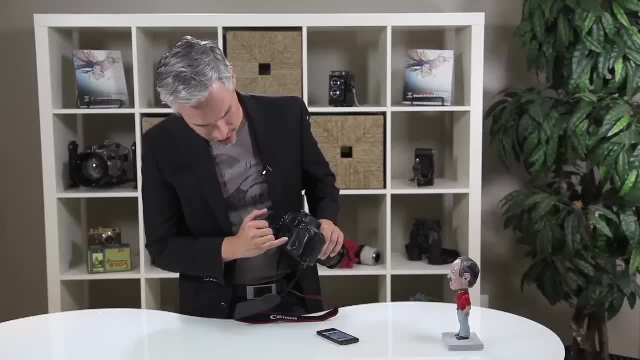 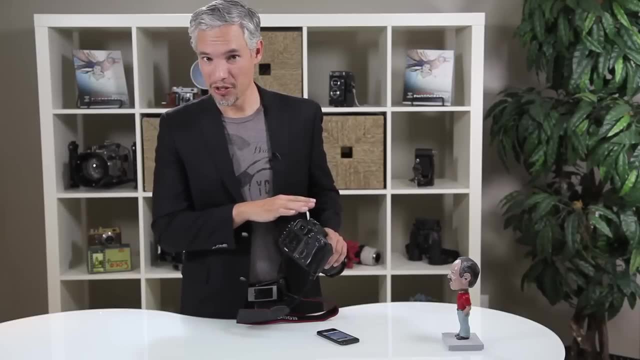 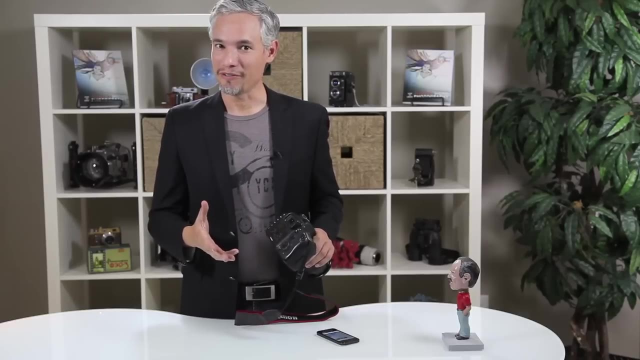 I'll look at the histogram here And we can see the histogram is all in, like the left side here. The reason that it came out underexposed is that my dad's skin tone is a little brighter than middle gray And when your camera meters it kind of assumes whatever you're metering off of is some sort. 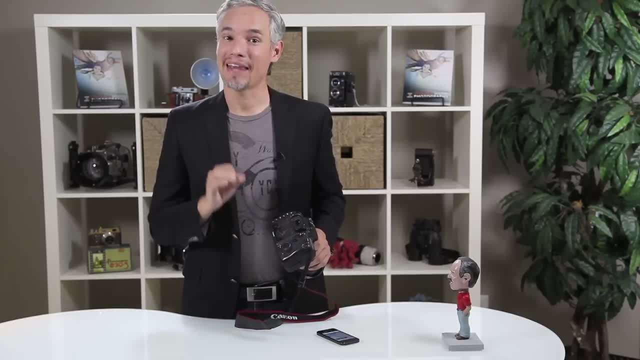 of mid-tone- Middle gray basically- And it tries to make that the center of the histogram. So anything that is more reflective, brighter than whatever you meter from, is going to show up closer to white. Anything that's darker or less reflective is going to show up closer to black. 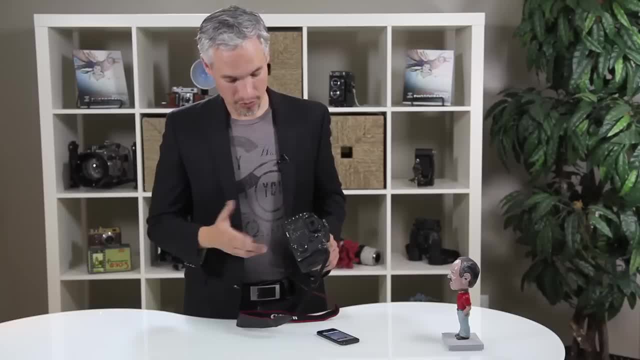 So it just so happens that I don't want my dad's skin to be middle gray, because it will appear too dark. Instead, I need to meter off of something a little darker in the scene. Now it doesn't have to be a skin tone or a shade of gray. 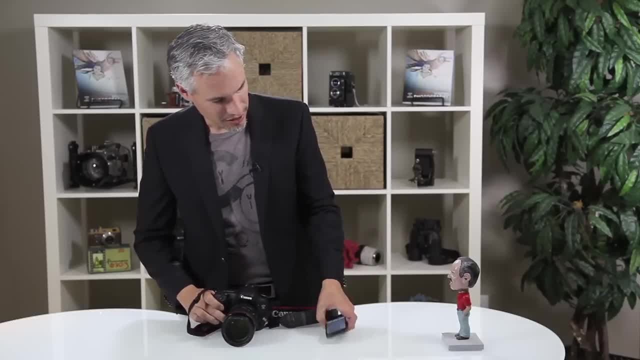 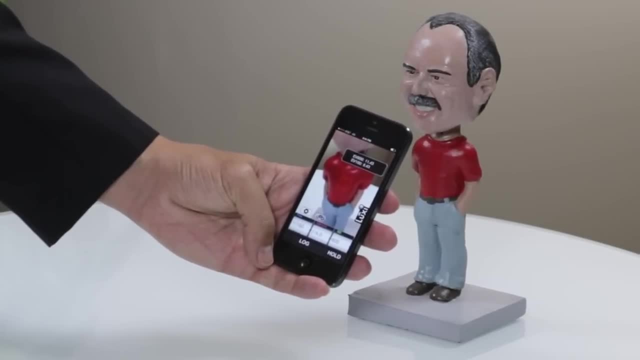 It can be a color too, And so, looking at my dad here, his red shirt looks a little darker, So I'm going to go ahead and take a metering off of that. And wouldn't you know it, the shutter speed is getting longer and longer. 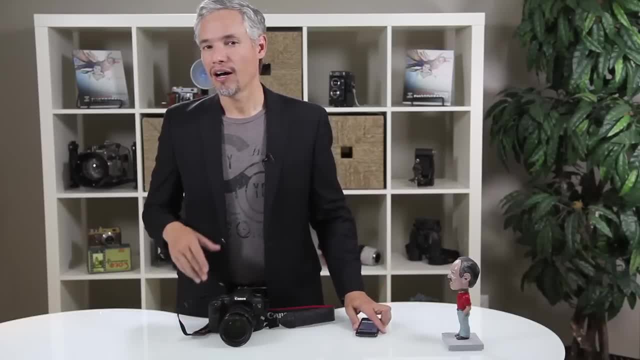 Now it's saying 1, 60th of a second. So I took a sample shot and realized I was metering off of something too bright. Now I'm metering off of something a little darker and I'm going to go and adjust the. 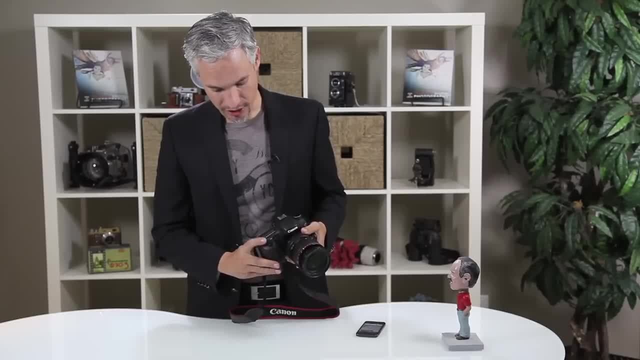 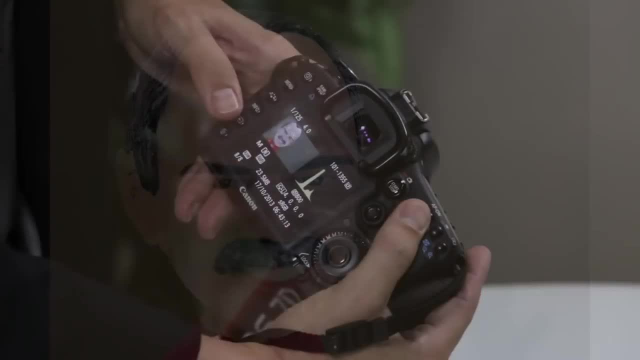 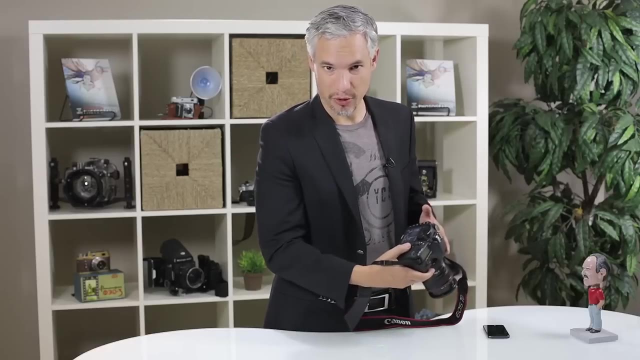 shutter speed to that 1, 60th of a second and we'll try it again. So that's looking much better. My dad's face is closer to the right side of the histogram. If I wanted to make the whole thing a little bit brighter, normally I would just use exposure. 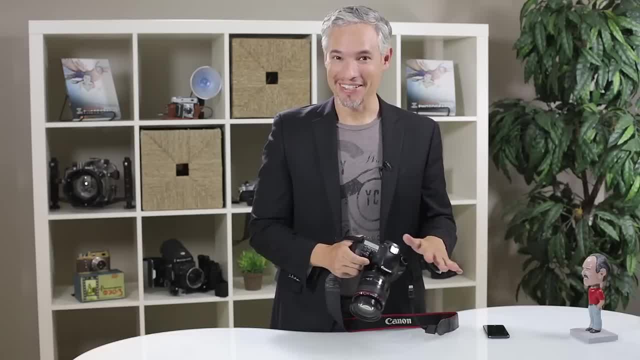 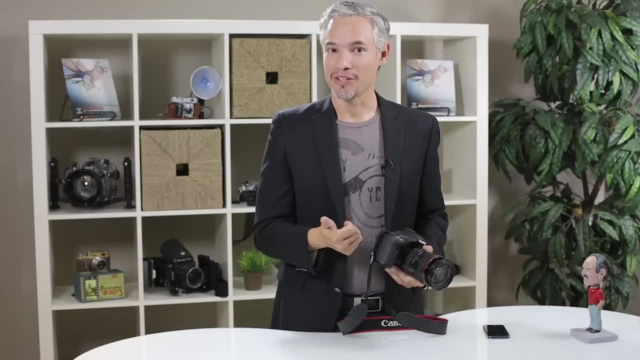 compensation on the camera itself, But we're doing this manually, right. So I need to think to myself: what can I do to make the shot brighter? I could Maybe use a slower shutter speed, I could use a smaller f-stop number, or I could use a higher ISO. 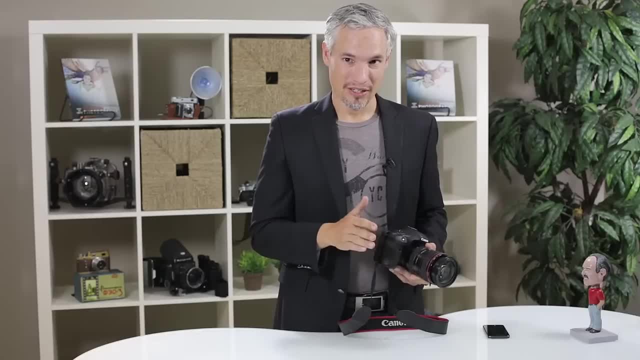 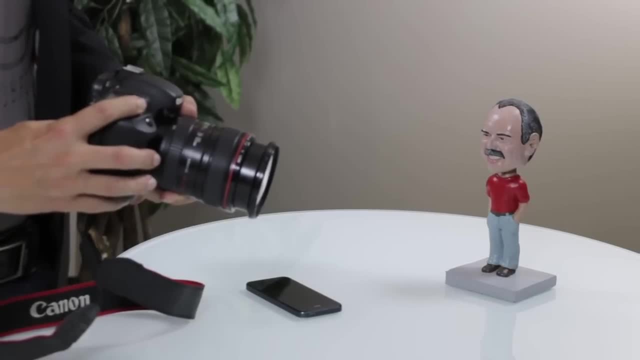 So I need to pick from one of those three and then dial it into the camera. So for me, I think I'm going to use a slower shutter speed, So I'm going to just go down a full stop from where I was and I'll go all the way down. 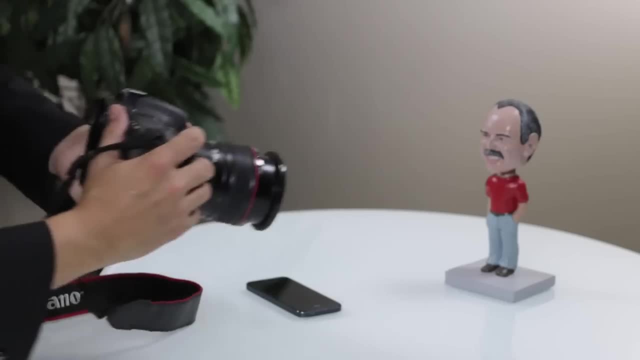 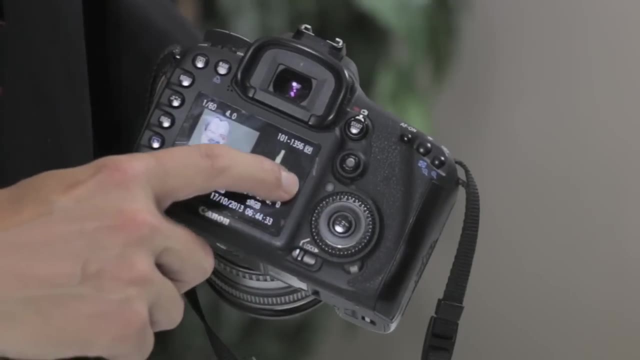 to 1, 60th of a second and take another shot. So looking at the histogram, I can see nothing really is blown out. My dad's face is close to the right side of the histogram and I can see from the blinkies. 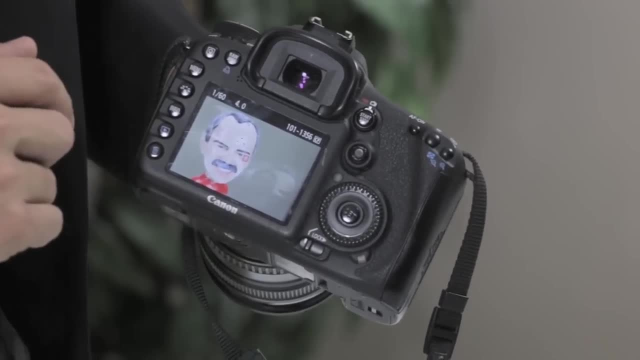 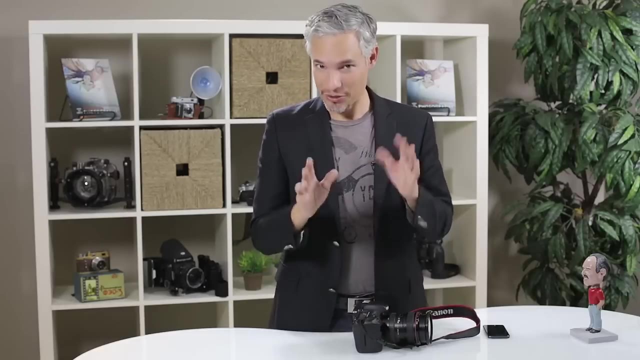 that I have going, that just a few highlights in his head are blinking, So that's a pretty proper exposure, And this is the kind of process that you're going to have to go through for the next week while you're using decoupled metering. 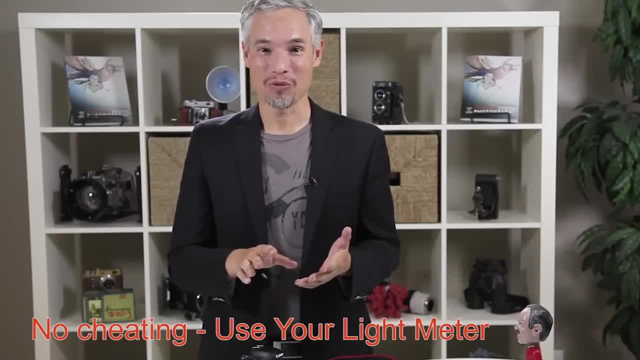 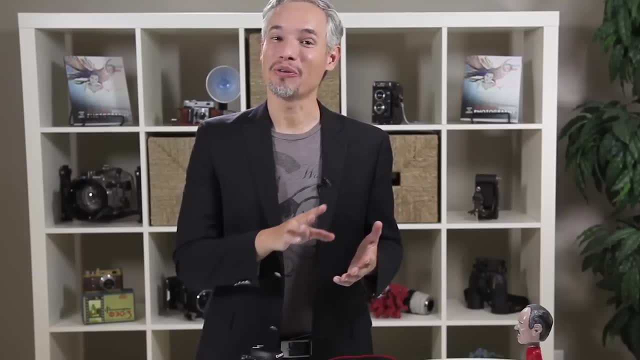 And I don't want any cheating. I know your camera will give you a hint and it will tell you whether it thinks you're underexposing or overexposing. Don't pay attention to that hint. I want you to use only your eyes. 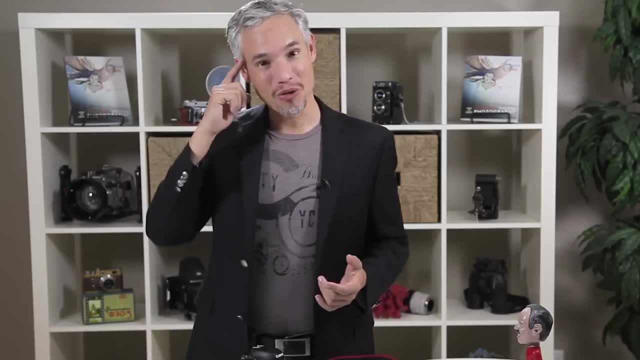 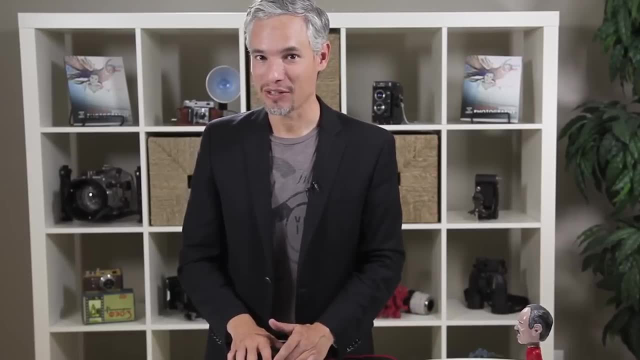 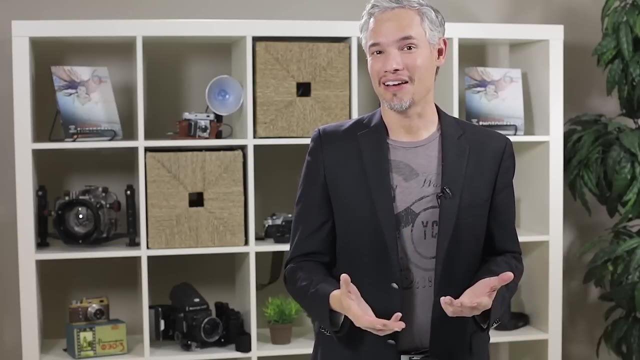 Only your smartphone app or whatever it is you're using to meter And your own head. I need you to manually copy all the settings from your meter over to your phone, and that process of copying those settings will make you think about them. You'll start to really understand what f4 and f5.6 are and what 1- 60th and 1 60th of. 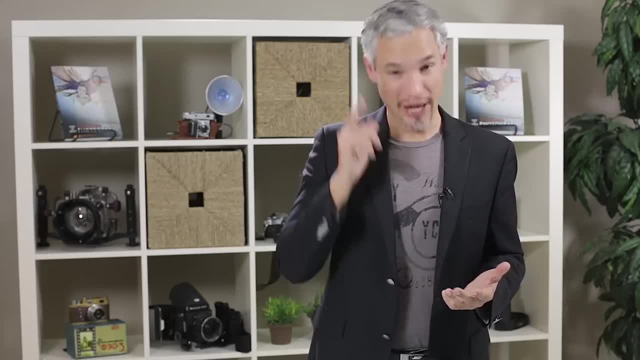 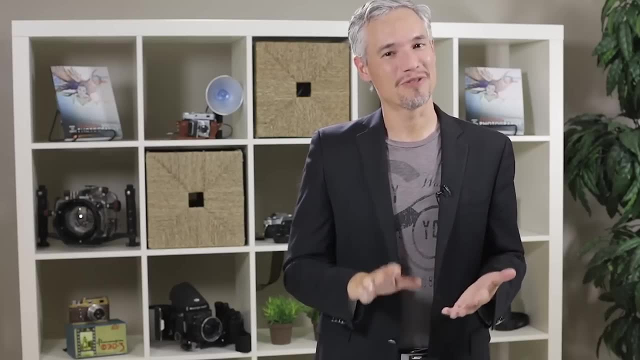 a second are, And whenever you start to have a problem and you have to manually decide which of those settings to adjust. well, you're going to be learning at the same time, So you might miss a few shots as you go about, But I promise it will make a difference for the rest of your life as you're taking pictures. 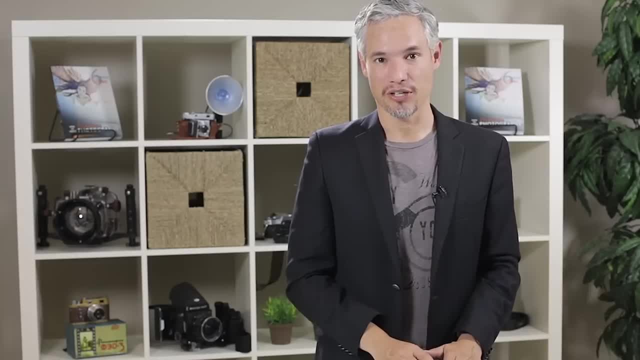 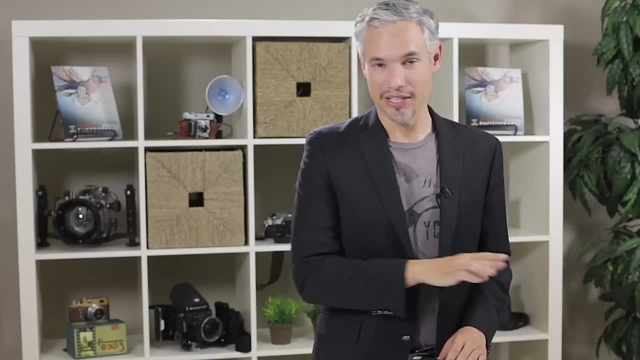 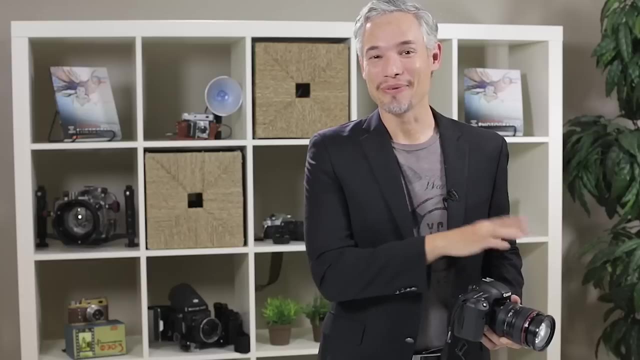 no matter which camera you're using in the future. I do want to show you a couple other things that can happen. I'm going to try metering off of this white table and then taking a picture of my dad. So metering with my app told me I needed to shoot at 1 750th of a second because this: 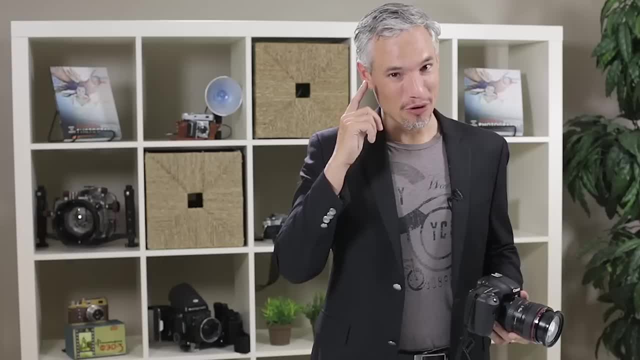 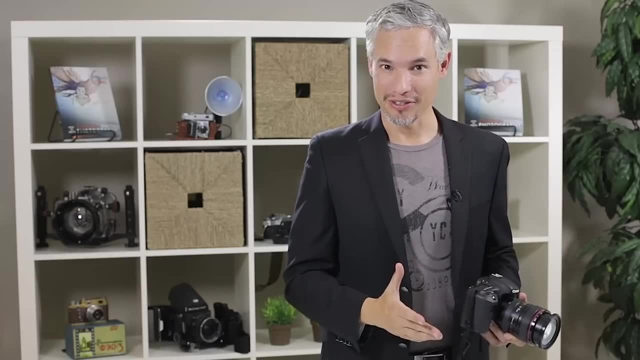 bright table is pretty bright and I already know what the proper exposure is, so I'm going to try it. And this is a faster shutter speed. So what do you think? Is the picture going to come out too bright or too dark? 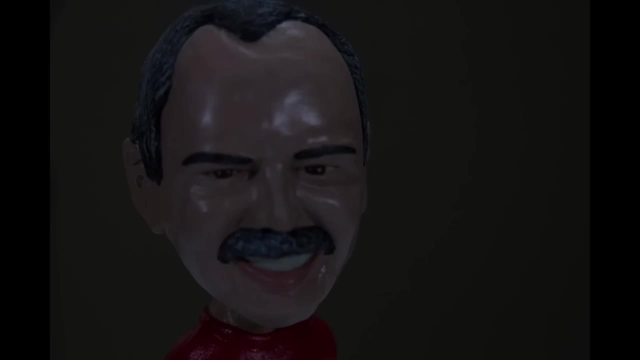 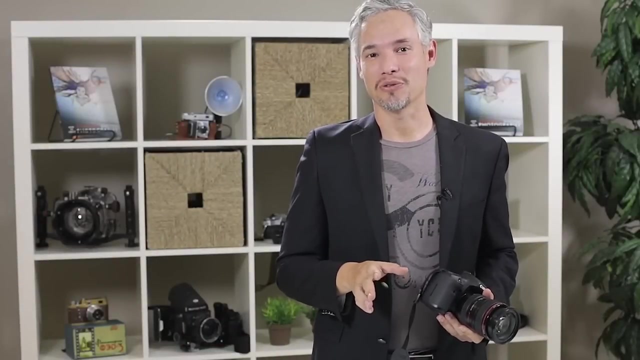 Well, let's find out. Wow, Way too dark. He's still a handsome devil in there, but I'm going to have to use a much slower shutter speed to expose it properly. And the lesson I'd like to show you is the same one we talked about earlier. 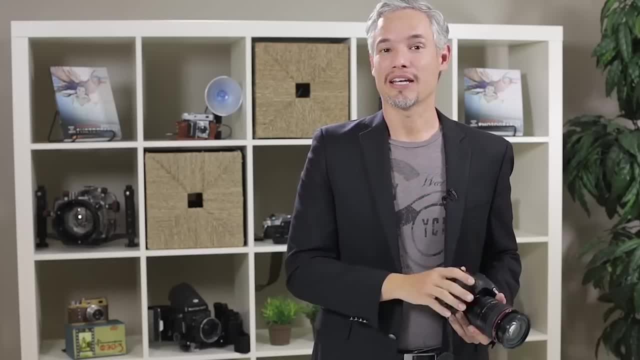 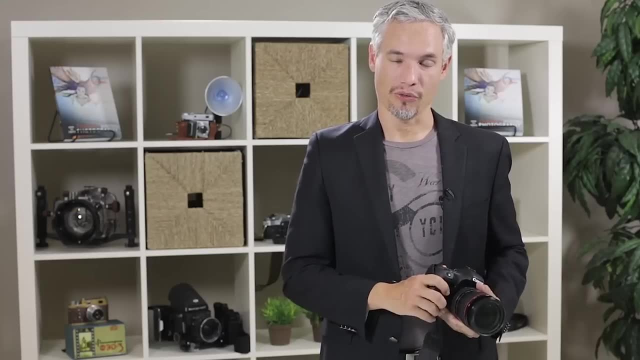 If you meter off of something bright, then you're going to get a dark overall picture and you need to adjust for it manually. If you meter off of something dark, your picture is going to be better. I really hope this video has helped you understand exactly how to control your camera and that 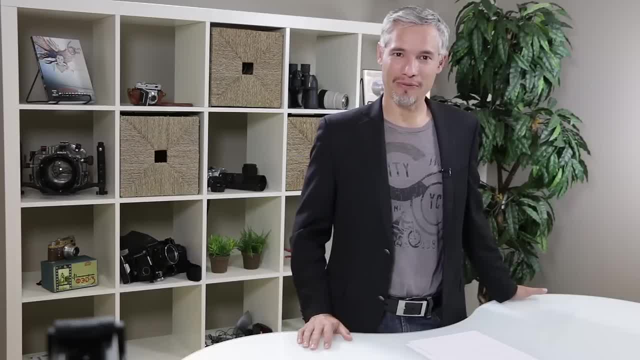 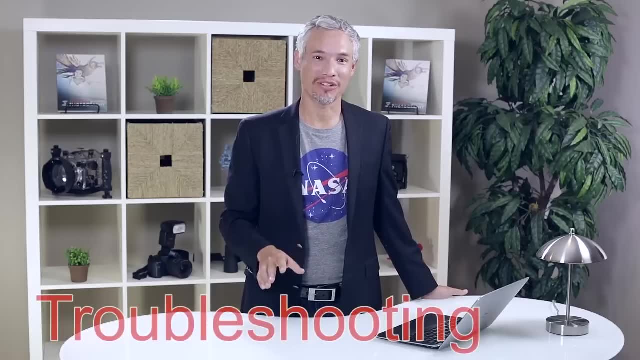 it helps you overcome those technical challenges that so many people have with their cameras. Hi, I'm Tony Northrup, and for my stunning digital photography video training series, I'm going to talk about troubleshooting your camera problems. So all those pictures that you get where they're blurry or there's weird shakiness to it or 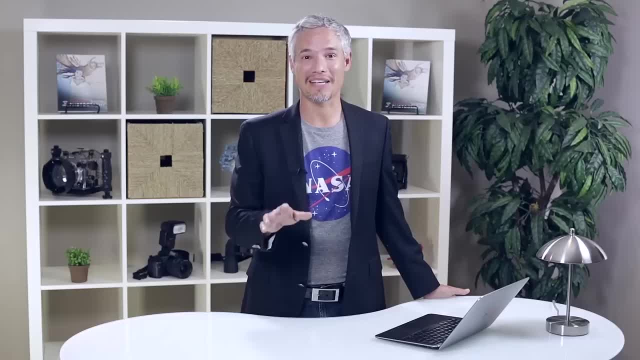 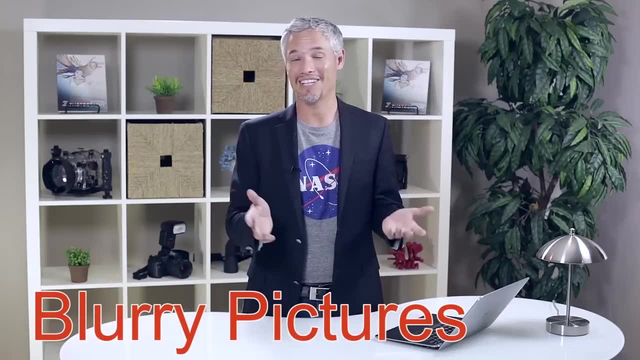 the colors are completely wrong, all those pictures you hate. I'm going to show you exactly how to fix them And up. first I'm going to talk about blurry pictures. Now, blurry pictures can be caused by like 10, 15 different things. 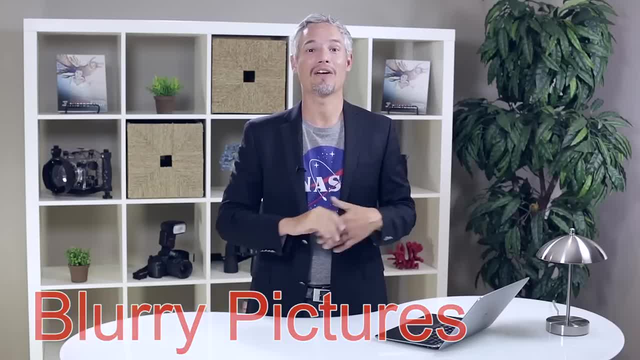 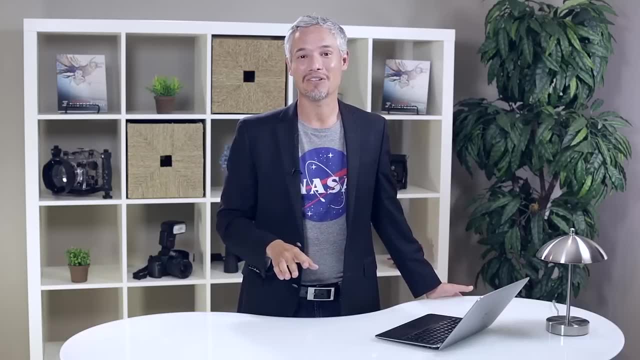 And in the time I've been taking pictures, I've managed to screw up every single way you can possibly screw up, So I'm going to look at a lot of bad pictures today. Let's take a look at one of the most common causes of blurry pictures, which is just mis-focusing. 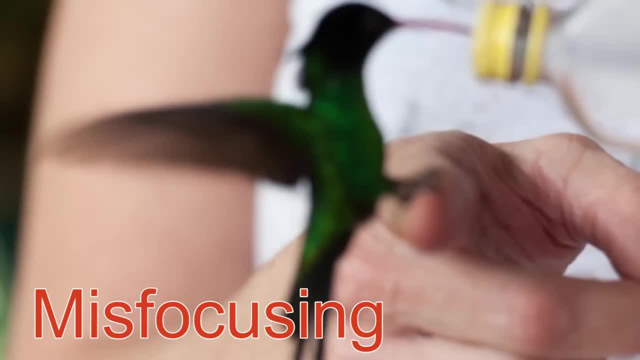 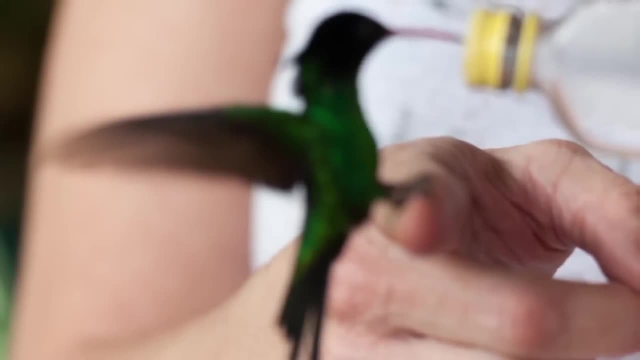 If you look at this picture of a hummingbird drinking from a bottle- here you can see the bird is completely blurry, But you know that this is caused by mis-focusing, because you can see that the woman's hand is sharper than the bird. 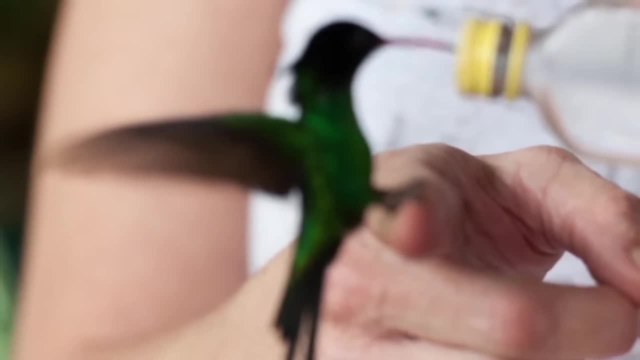 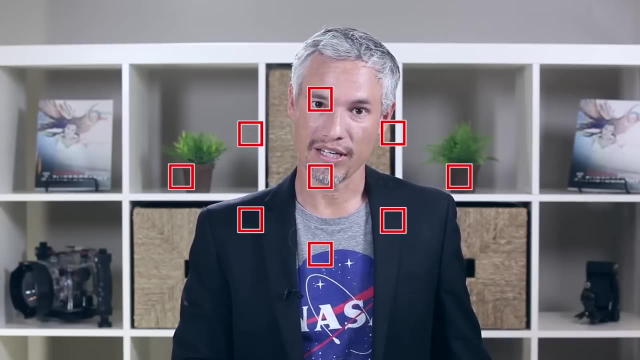 What happened here is the camera back-focused. It focused behind the subject, and it can happen for a lot of different reasons. In this case, I suspect the camera had multiple focus points selected and the camera simply decided to focus on something other than what you wanted to focus on. 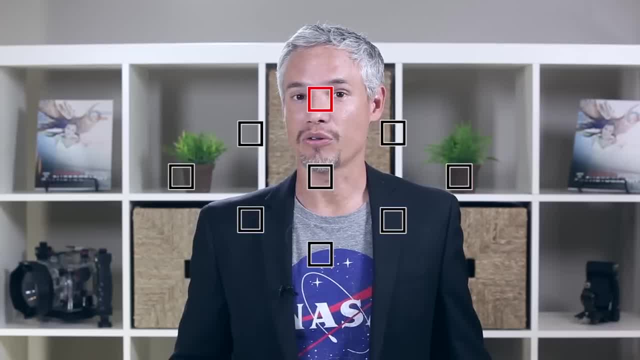 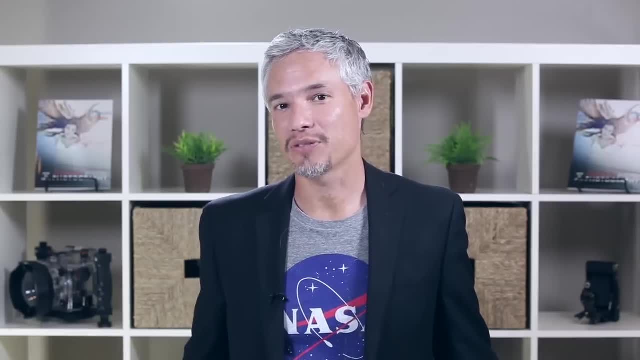 How would you solve this? Well, you'd set your camera to use a single auto-focus point- I almost always recommend using a single auto-focus point- and then you'd put it right on your subject. Another way you'd solve it is just by taking a whole lot of pictures and regularly refocusing. 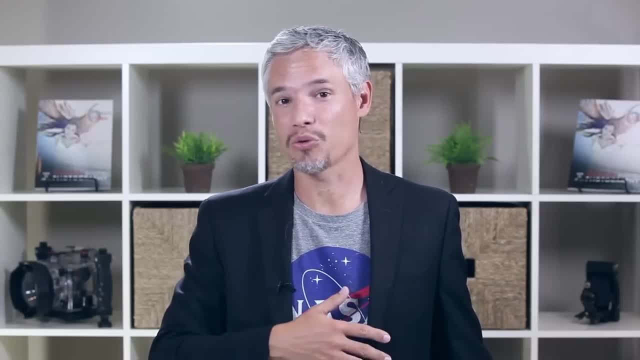 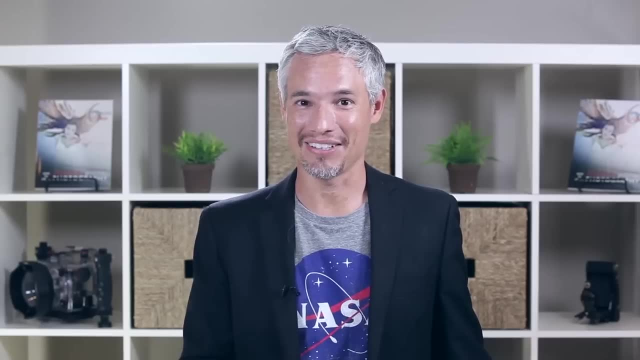 because no camera's auto-focus system is perfect. They're all going to screw up sometime. So remember: the very first thing I tell you in the Quick Tips video is: take lots of pictures and delete most of them. Let's look at another picture. 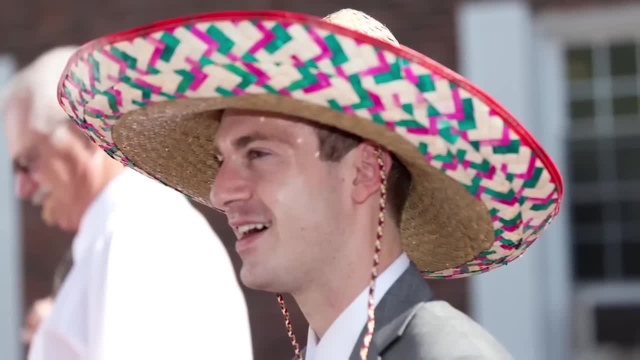 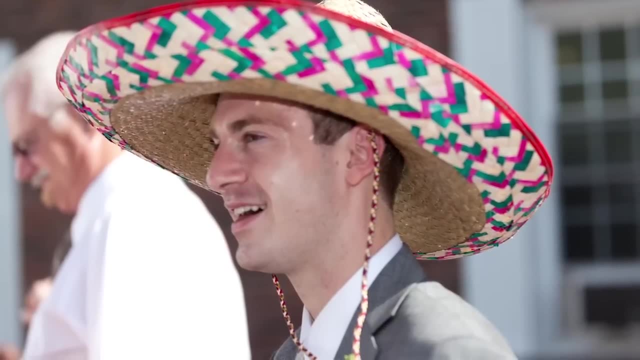 This is my friend Justin at his wedding, and if you look at his face it's not quite sharp. So of the different things I can tell you about him, one of the things I can tell you about him that can go wrong. the way you can diagnose this one is by looking at his sombrero there. 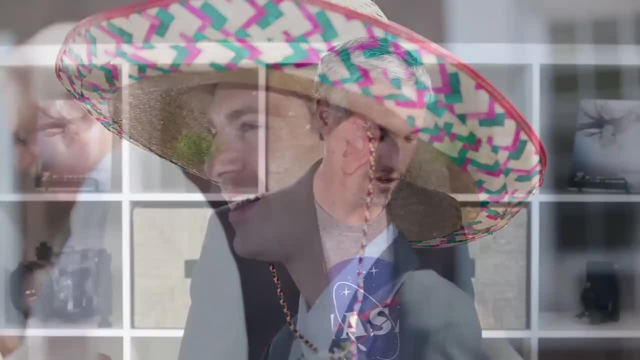 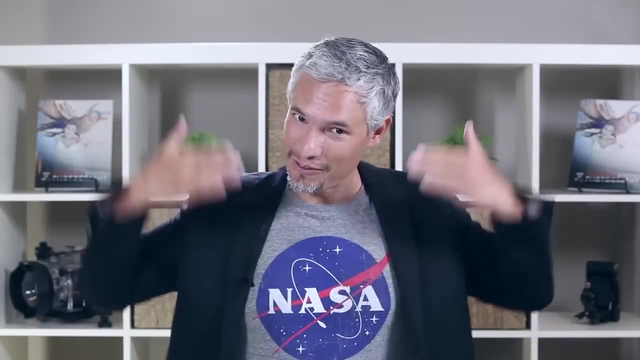 You can see that, a little bit past his face, his sombrero gets nice and sharp and that just means that the camera focused a little bit behind him, causing his face to be out of focus, Because, remember, the focal plane is a big flat space like this: 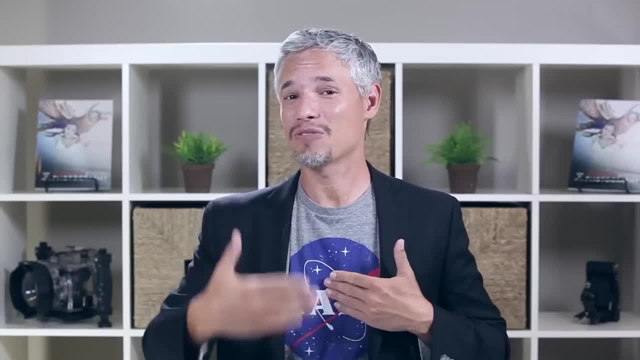 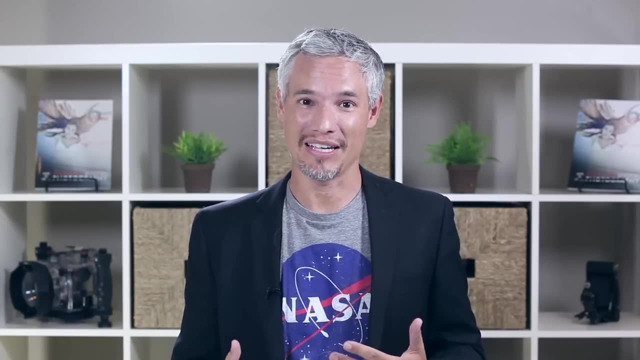 It's a two-dimensional space parallel to the sensor, So anything that's in front of or behind that space is going to be a little bit blurry, And the farther it is away from that focal plane, the blurrier it's going to get. 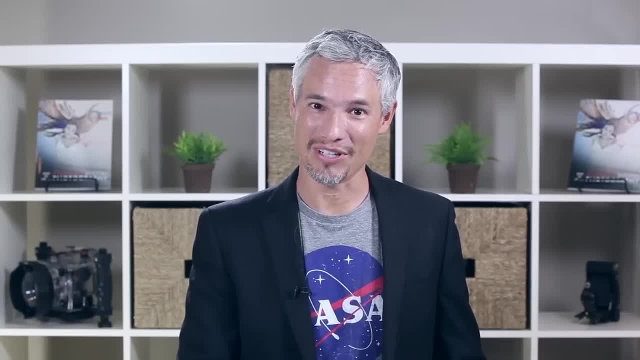 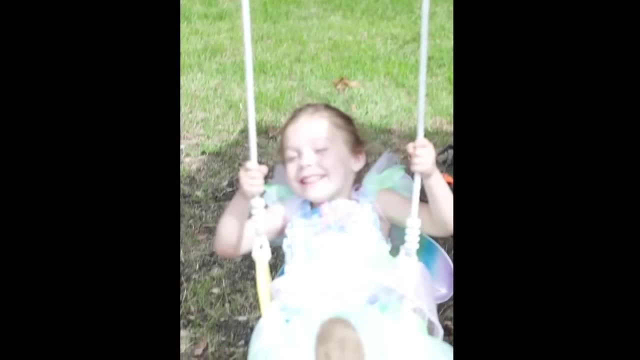 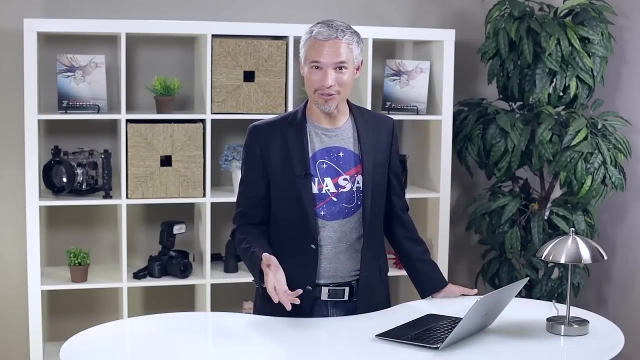 So, of the many things that can go wrong, we know that in this case the camera just missed focus. Let's look at another picture With this little girl on a swing. you can see that she's completely out of focus there. So how do we know if it's motion blur or camera shake or a bad lens or a bad camera? 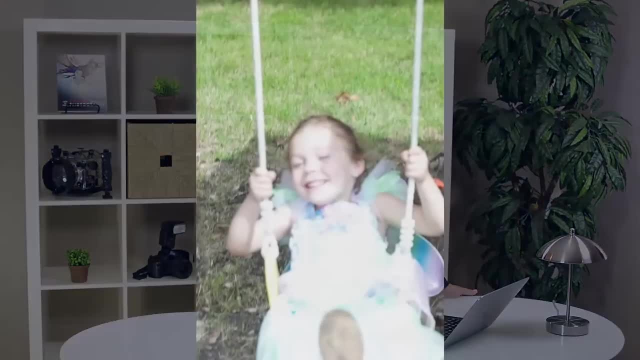 Well, we just look at the rest of the picture and we can see in the background there's some grass that's nice and sharp, And that means the problem is just as simple as the camera focused on something else. Let's look at another picture. 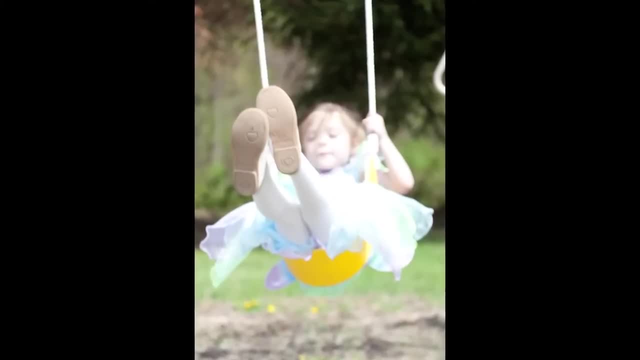 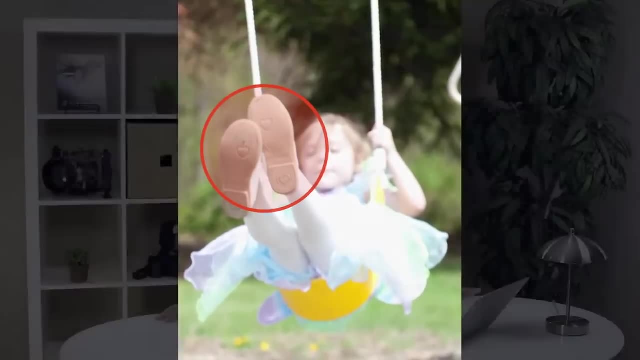 This is Justin. Here we can see the same little girl on the swing set and the camera missed focus again, And this is another common scenario- The camera just focused on her feet. Now, with a moving subject like this, it can be hard to keep your focus point exactly on. 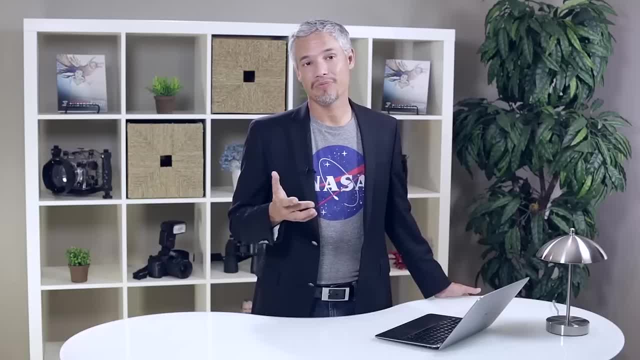 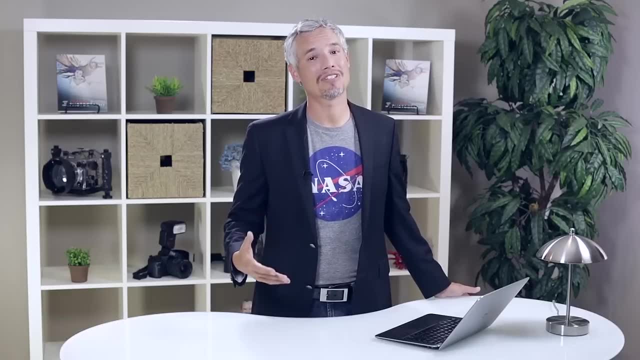 the person's eyes, where the focus should always be, The camera probably just focused on her feet, and that's going to happen sometimes. There's no real way to get it perfect 100% of the time. So, again, the way you fix this is by taking lots of pictures and refocusing and refocusing. 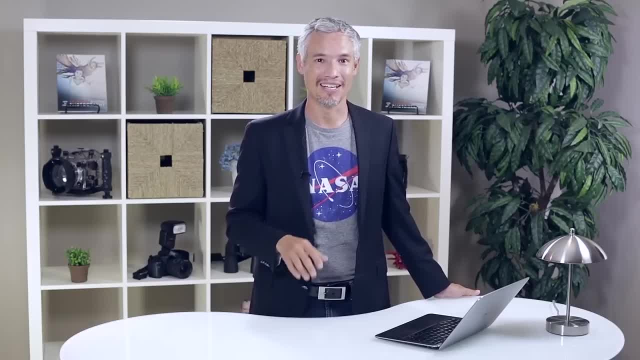 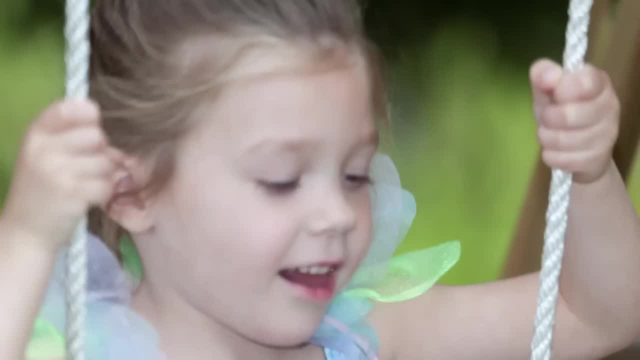 and you just hope that some of them turn out, Because you'll never get 100%. Let's look at another picture. There's the girl again And again looking at this picture. she is moving. so it could be motion blur or it could. 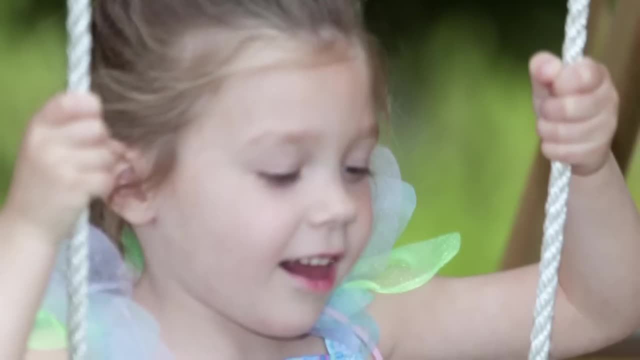 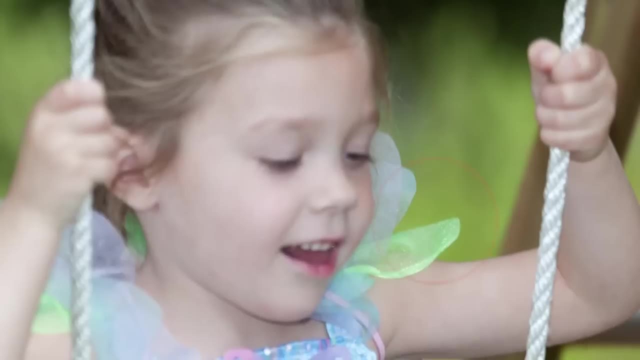 be camera shake, But if I look closely at it I can see that if you look at that rope that's in her hand, that looks nice and sharp, And I can also see that the dress that she has on the sort of frilly lace around her. 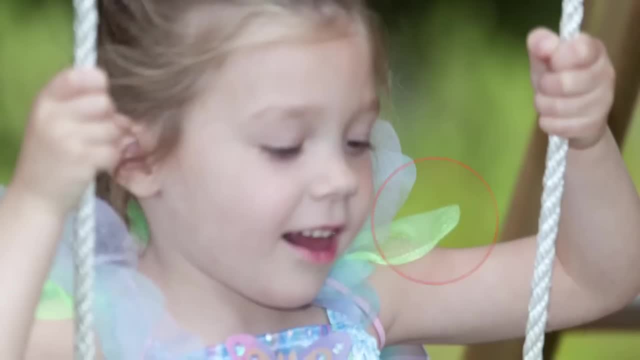 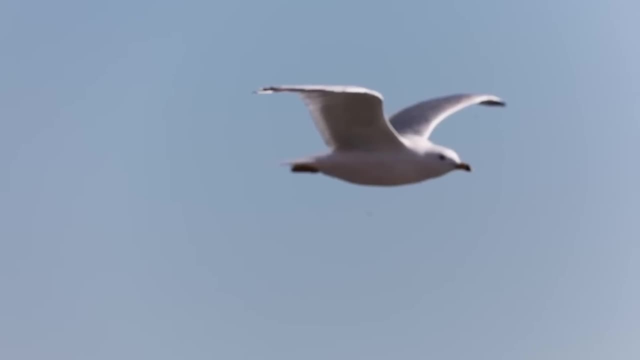 neck looks nice and sharp, even though her face is out of focus. So I think the camera here back focused, Which means it focused behind, Where I actually wanted it to focus. This is a picture of a seagull and there's nothing in the background but the seagull. 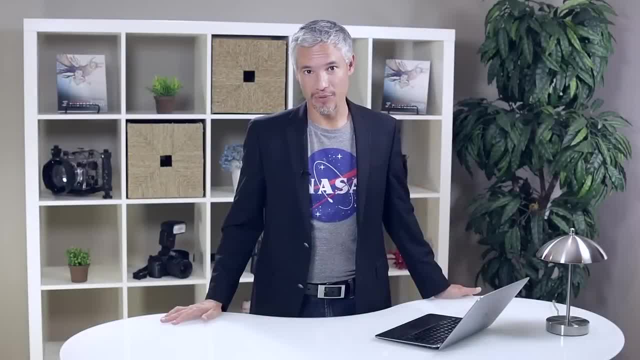 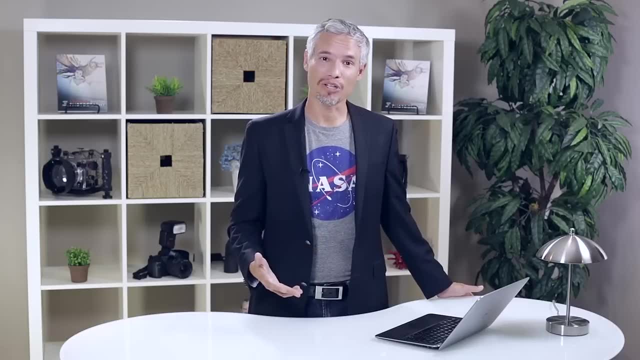 itself is blurry, And this is just going to happen, especially with moving subjects. Your camera isn't going to keep up perfectly with moving subjects. so it's not something wrong with your camera. It's not even something necessarily wrong with your technique, but good technique can. 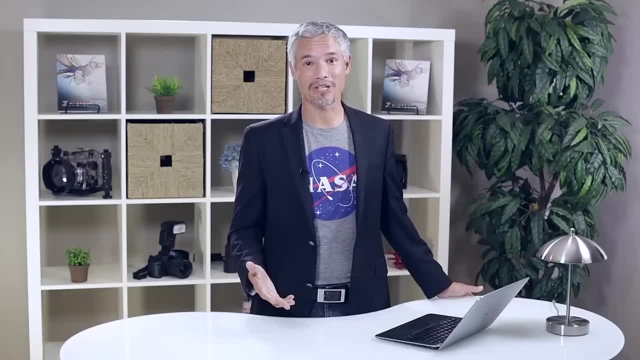 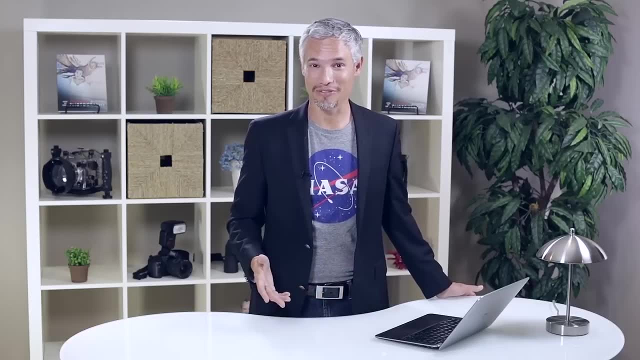 give you a higher percentage of results. You're always going to get some blurry pictures, including the seagull picture, And keep in mind I've had a lot of practice at this and these are all pictures that I've taken in just the last couple of years. 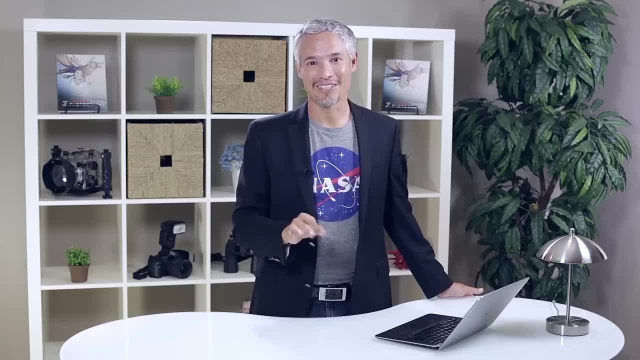 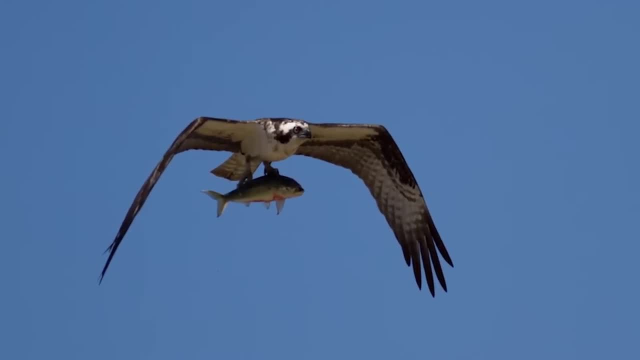 Nobody gets 100% of the pictures perfect all the time. So let's look at another picture. This is another flying bird picture. This is an osprey with a fish And if we zoom in nice and tight on this picture, we can see that it's just not perfectly clear. 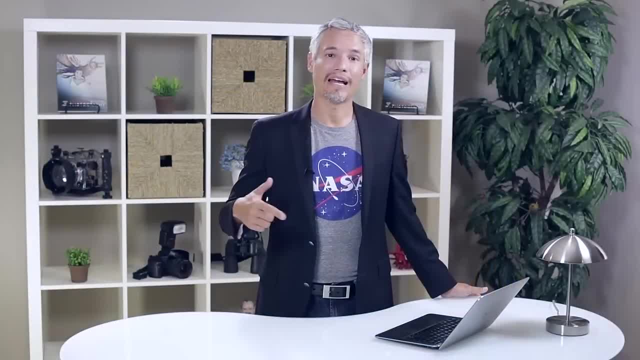 It's just a little bit out of focus. It's a moving subject. The camera has to track that moving subject and constantly adjust the focusing distance. It's moving a little motor in the lens and it's not perfect. No camera is completely perfect. 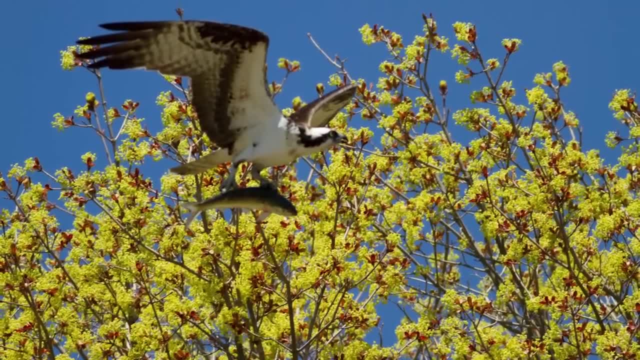 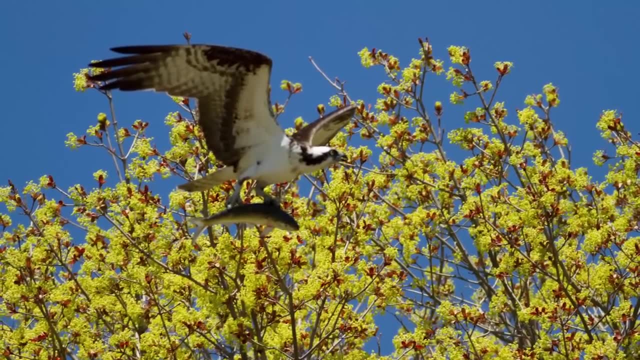 Let's look at another picture, Same osprey, and this time the focus problem. it's mis-focusing, but the cause of it is a little bit different. The previous picture didn't have anything in the background, but this picture has a. 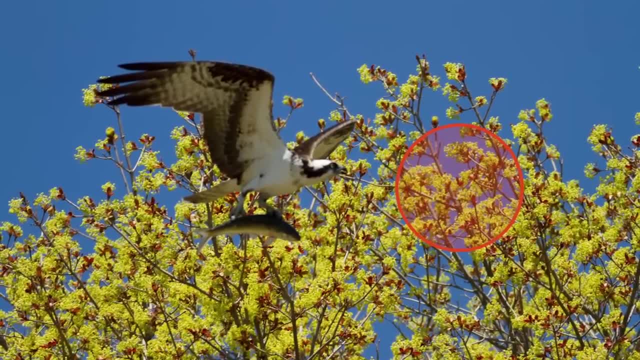 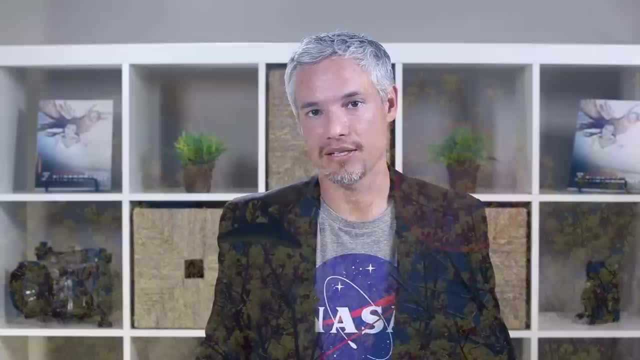 tree in the background- and this happens all the time- The camera decided to focus on the tree instead of the moving bird. When you're hand-holding a telephoto lens like this, it's really hard to keep that center focus point right on your subject, because you'll move the camera around a little bit. 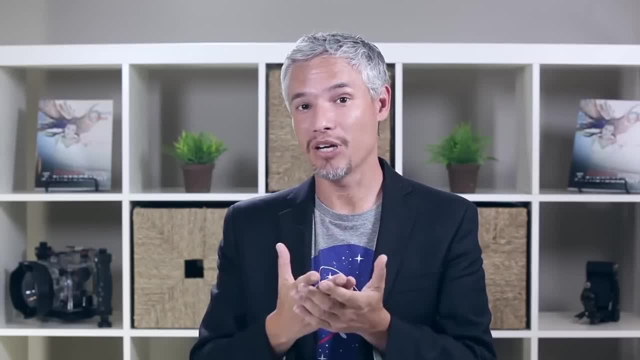 and at some point, if the focus point happens to be out of focus, it's going to be out of focus. If you put it in front of a tree instead of your subject, it's going to focus on the tree. if the camera is doing what it's supposed to do, 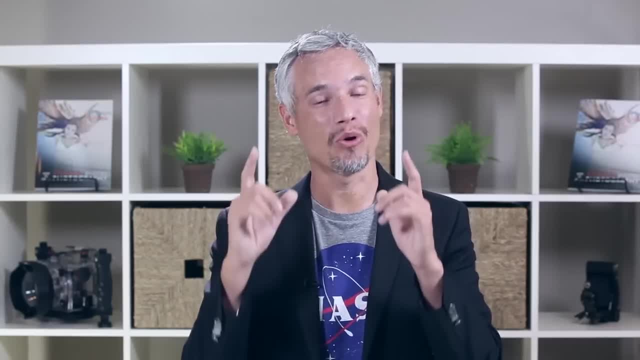 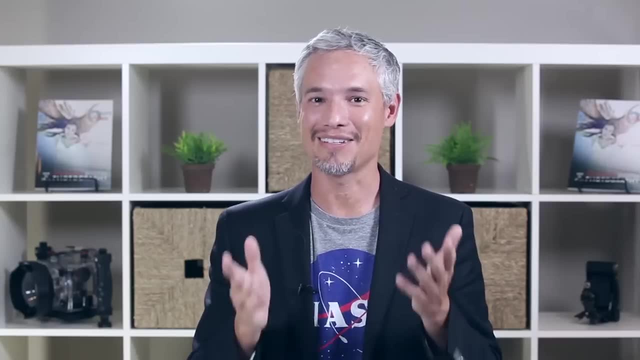 You basically are telling it to focus on the tree by not keeping the camera perfectly centered on the bird. Anyway, it happens, You solve it by just practicing, steadying your hands and, of course, taking lots of pictures. Let's look at another shot. 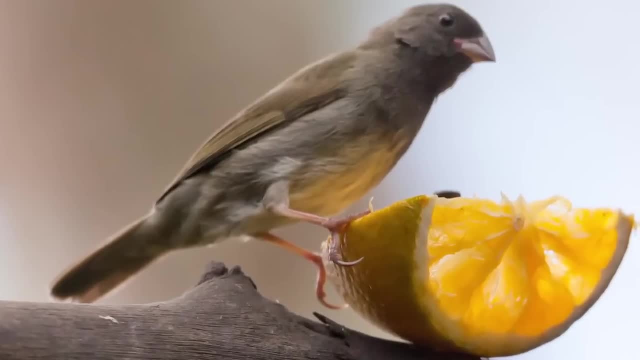 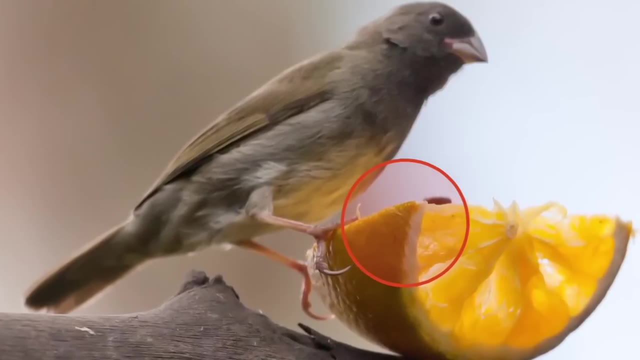 This is a still bird and he's perched on an orange, but you can see that the camera focused on the orange rather than on the bird. This is a really common problem. Most cameras focus on the orange. Most focusing systems are configured to focus on the very first thing that registers as 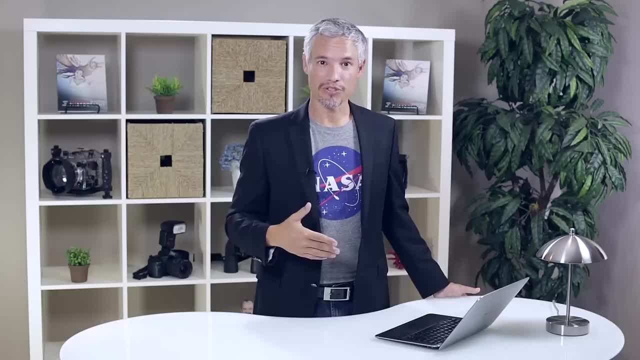 sharp, so if there's something in the foreground in front of your subject, it's very likely that your camera is going to try to focus on it. You just have to be careful about it and try to move any obstructions out of the way. 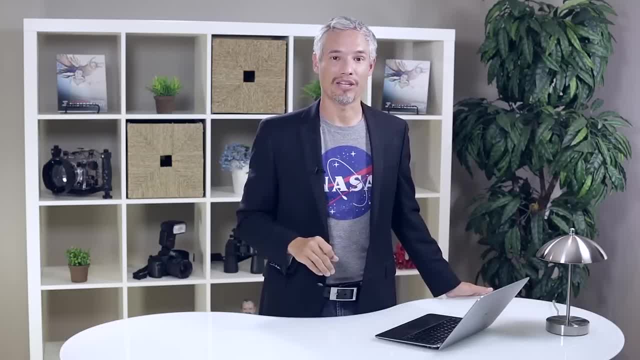 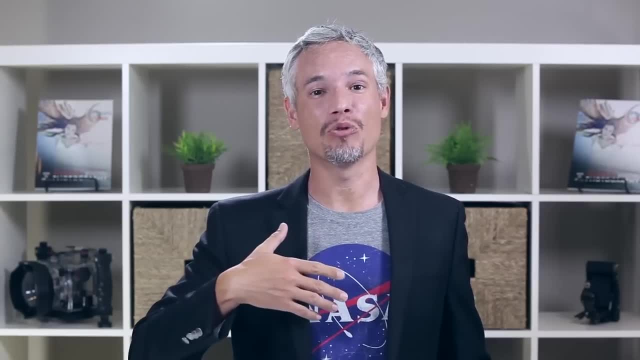 Move yourself so that the obstruction isn't between you and the subject. Sometimes, when you're trying to take a picture, your camera just won't focus. It'll start to focus and then it will move past your subject and then it will come in. 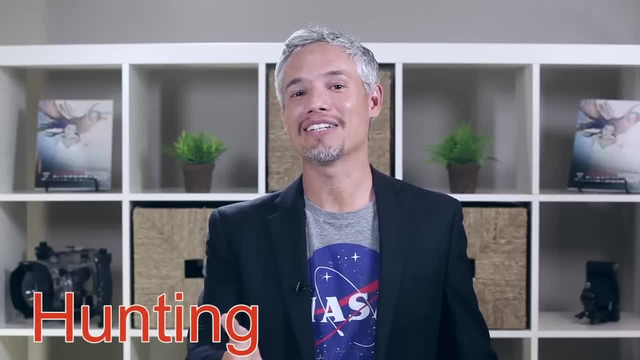 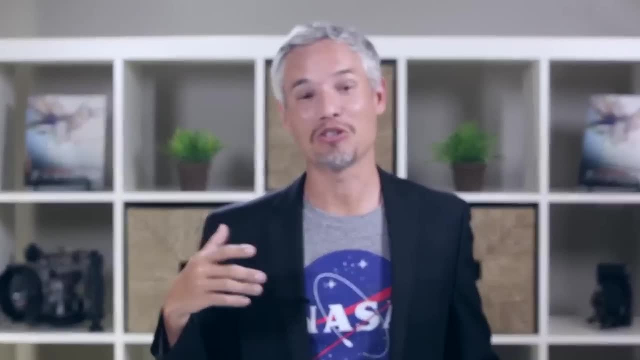 and out. This is a process called hunting, and my camera guy, Tyler, is going to demonstrate that now. As you can see, it will just keep moving back and forth and it'll move past your subject. You'll be like stop, you got it almost, but then it will just keep going. 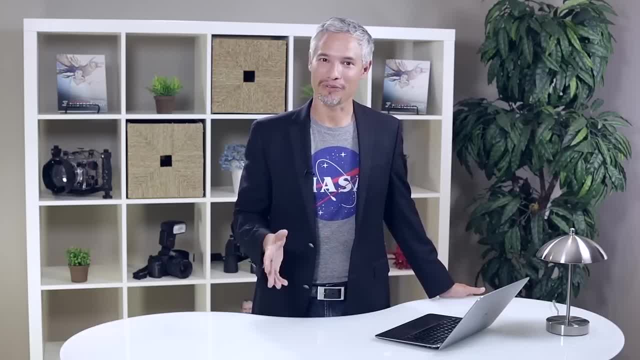 There are lots of different causes for this, but often it's a combination of multiple different factors. One of the biggest factors is not having enough light. If you're indoors, or you're in the shade, or it's particularly dark, well, your camera's. 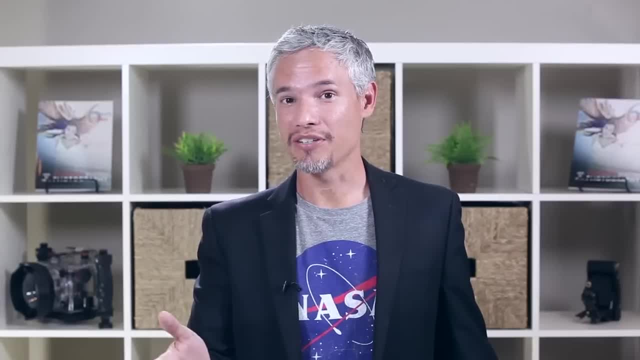 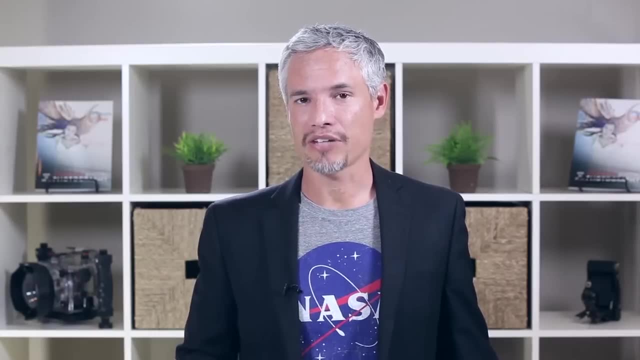 focusing sensors need lots of light. Of course you can solve that problem by just turning the lights up. Another way to solve that problem is by connecting an external flash. External flashes- most of them- have an infrared transmitter on them. that will help with the 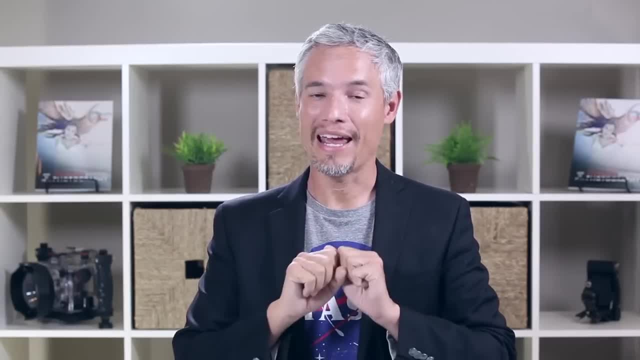 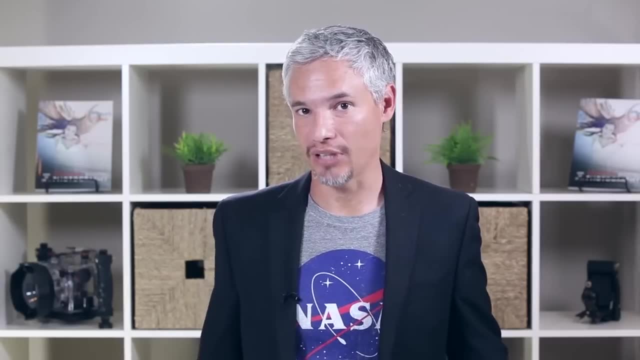 hunting problem. What that transmitter will do is transmit an infrared pattern on your subject and that pattern will add contrast to the scene and your focusing sensors will be able to latch onto that contrast. So, speaking of contrast, another common problem with focusing is that there's just not enough. 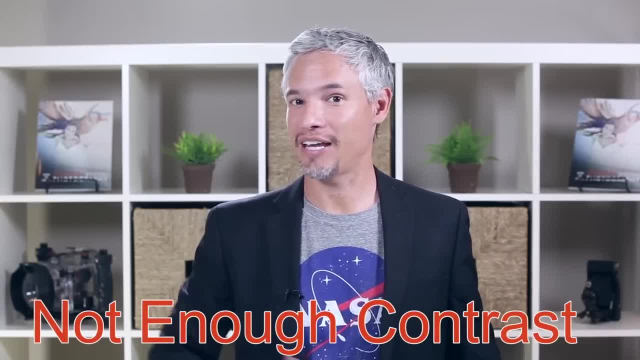 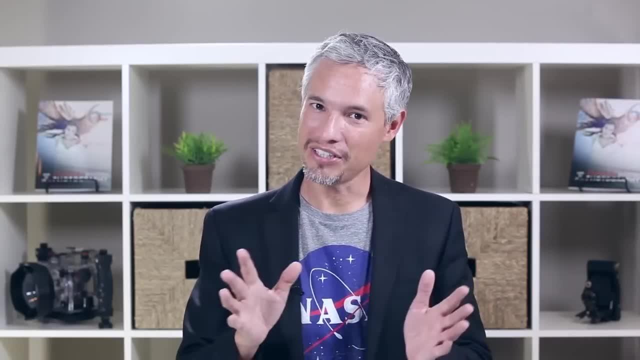 contrast on a scene. If you take out your camera and you try to focus at a completely blank wall, there's a good chance that it's not going to be able to do it, because your sensors are looking to see that multiple different versions of the same image match up and line up perfectly. 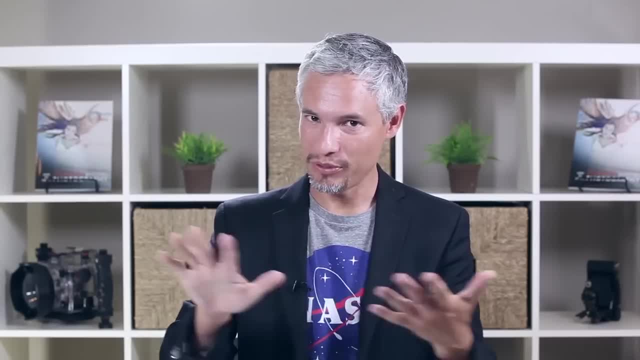 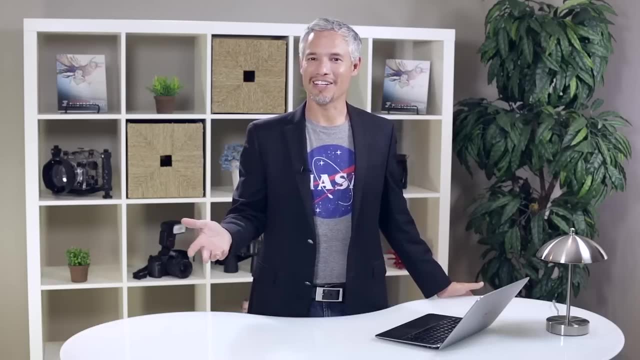 and if there's no detail in the scene, it won't be able to match up those two copies of the image and it will just keep looking. So the easiest way to solve this problem is just to focus on an area of contrast. If you were trying to focus on this spot on my jacket here, it would be fine. 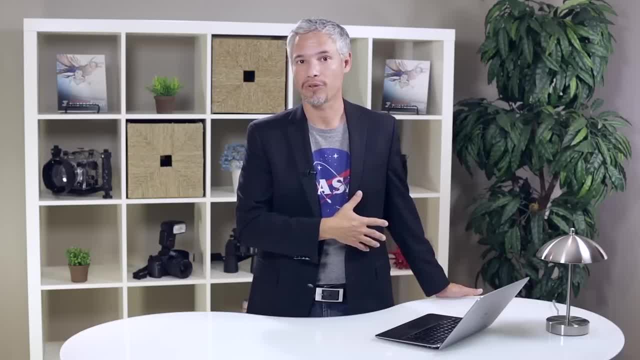 It would just be like: oh, it's just this area, completely solid black and the camera probably wouldn't be able to focus. But I bet you'd get much faster results if you focused on this contrast between my dark jacket and my blue, because the camera will be able to latch on to that. This is 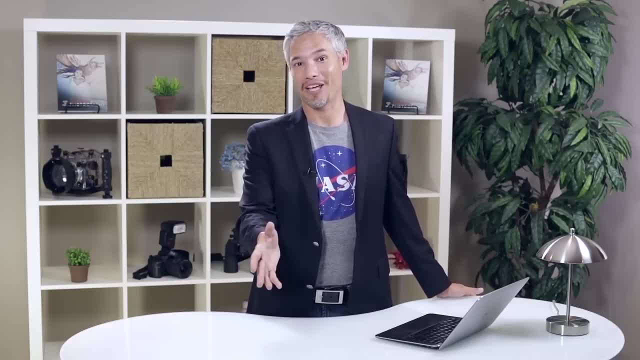 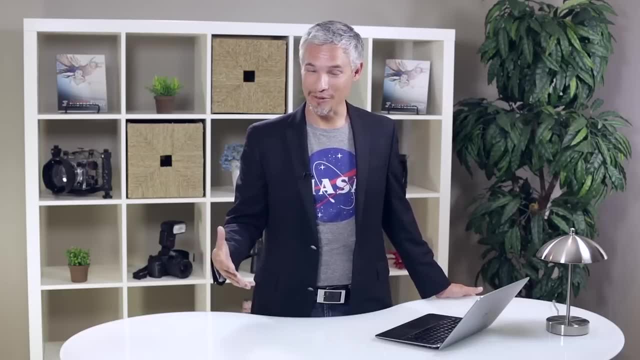 especially important if, for example, you're taking pictures of an indoor basketball game, one of the most challenging focusing situations, because you have low light, which we already know is a problem. You have moving subjects, which makes everything challenging. Well, the way you can improve that is by 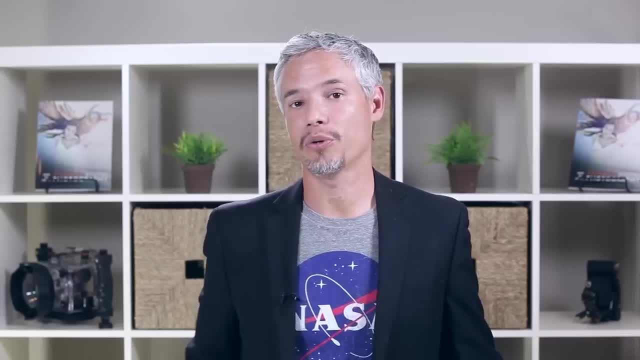 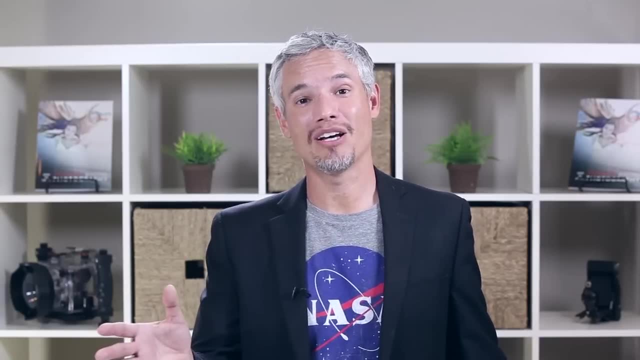 making a point of using a single autofocus point, your center autofocus point specifically, because it's the most powerful, and putting that autofocus point on an area of contrast. So in the example of an indoor basketball game, I think the most contrasty area is usually the number on the jersey. So keep it on. 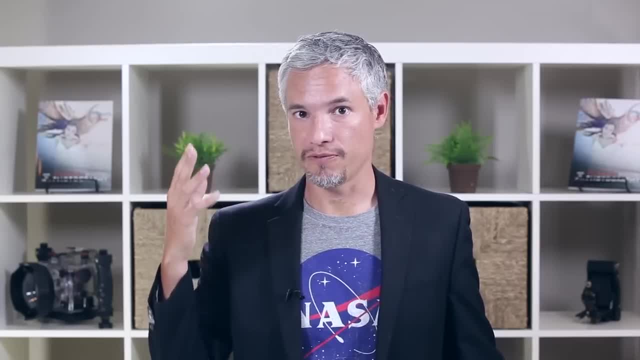 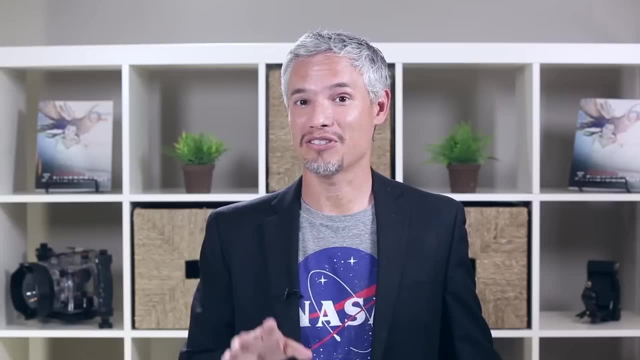 the number. That has a lot more contrast than just a person's face and that will allow your camera to keep up much better. Again, you're never gonna get a hundred percent perfect results. You're still gonna miss some shots, especially with 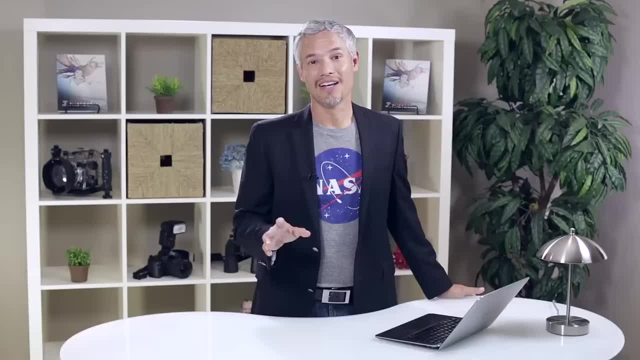 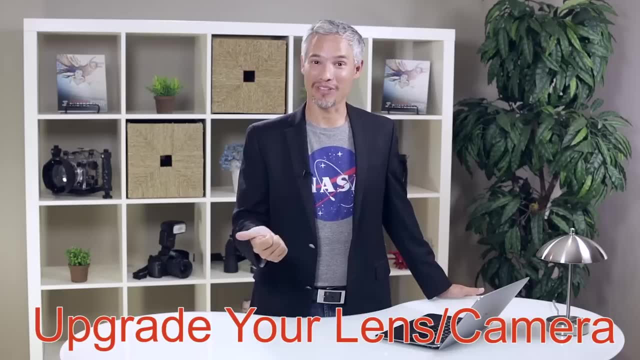 moving subjects, But that's the way that you get the best results. Another way to solve the focus hunting problem: it gets a little bit expensive, but you can upgrade both your lens and your camera. Higher-end cameras tend to have more sophisticated focusing. 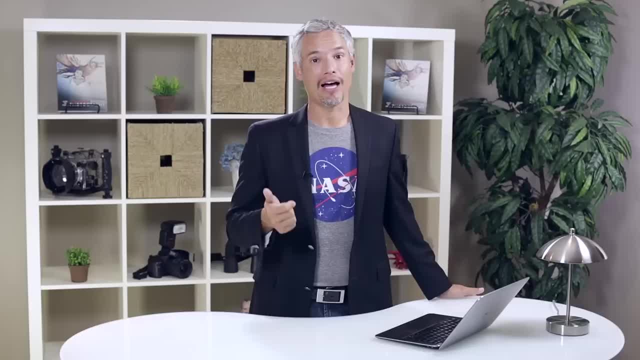 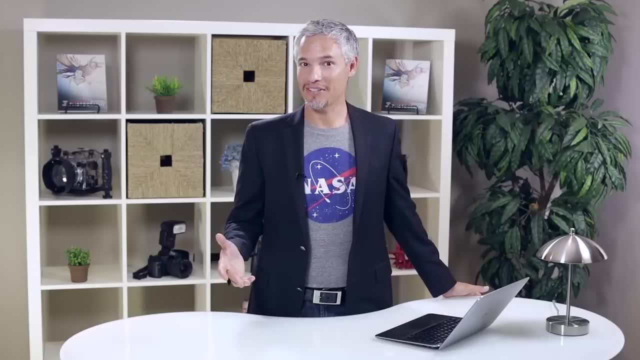 systems that can work in lower light and work with lower contrast. Higher-end lenses, specifically what they call faster lenses, let more light in. If you have a lens that's twice as fast as another lens, well, that lens is letting in twice the light and the focusing is much faster. 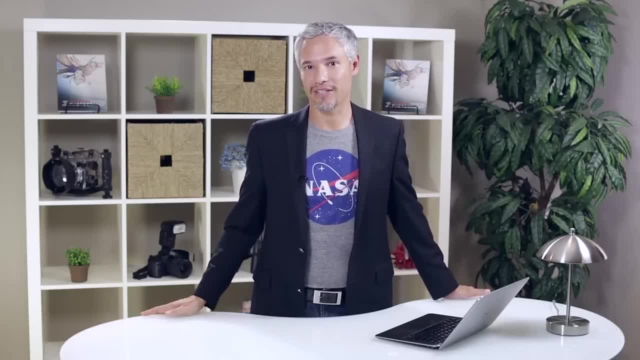 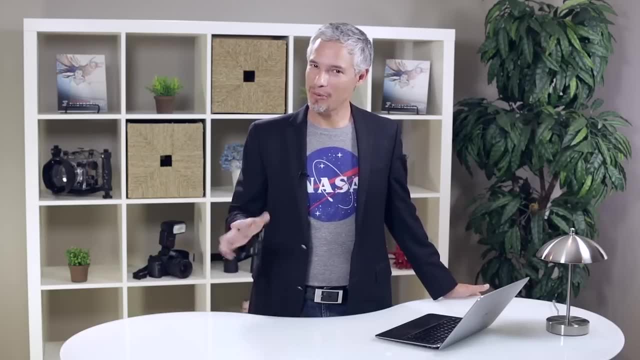 You're going to get a lot more results with the right lens. So the way you tell a fast lens is by looking for a lens with a low minimum f-stop number. For example, the kit lens that came with your camera probably has a minimum f-stop number of 4.5, or 5.6, or some range like that. That's a pretty 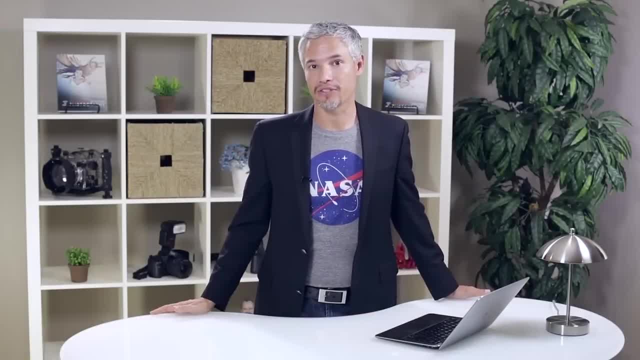 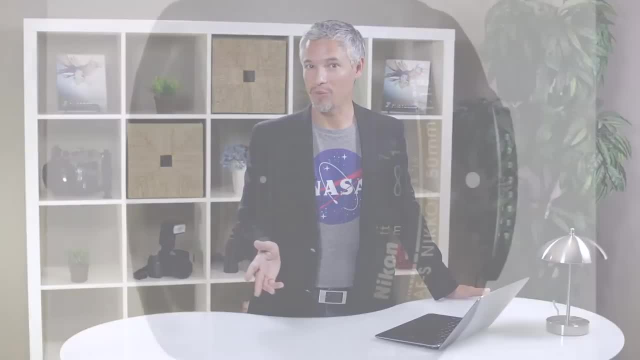 high number. That means that it requires just a whole lot of light if it's gonna focus properly. really need to be outdoors. If you were to go out and pick up, say, a 50mm f1.8 lens, that's going to be letting in like eight times more light. 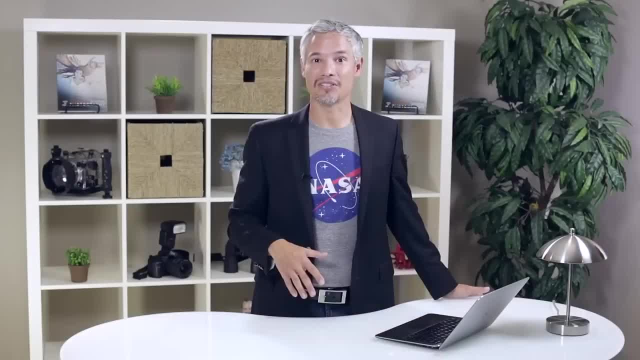 more light than your kit lens. that means you'll be able to work in lower light conditions and you'll be able to focus faster, even in bright light. You can also get one of the like pro series lenses. Usually these are like the 24-70mm f2.8 or the 70-200mm f2.8.. That f2.8 is a pretty low. 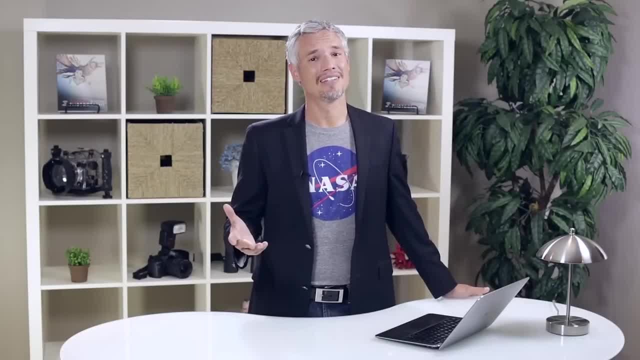 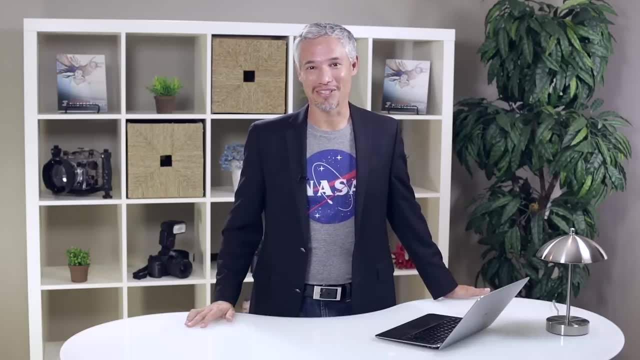 number and it's going to let you focus in much lower light conditions. Of course, I'm telling you that you can solve your focusing problems by spending thousands and thousands of dollars, and that might not be worth it to you. I mean, if you're a super rich guy, by all means go buy the. 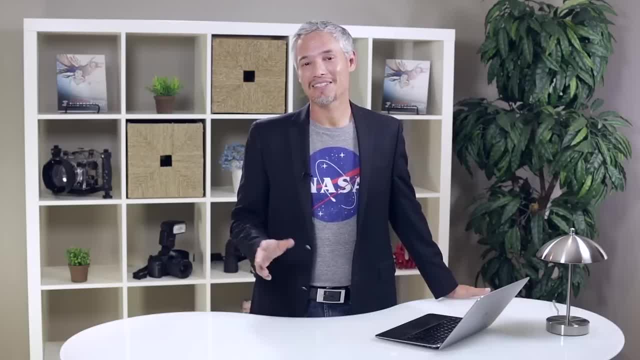 top-end camera and buy some expensive lenses, but that's not right for everybody. You can get around that with a lot of practice, though, which is why I'm spending most of my time preaching technique. Another common problem I see with people's focusing isn't really a problem, it's more of a feature. 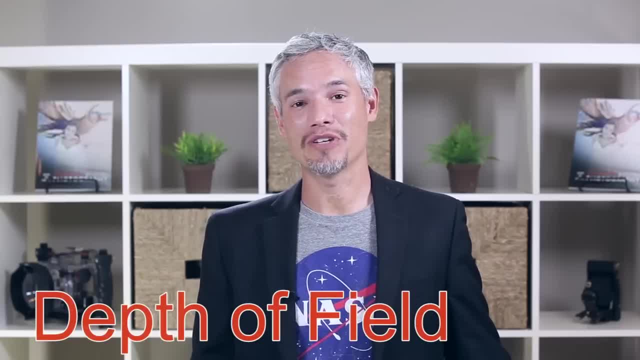 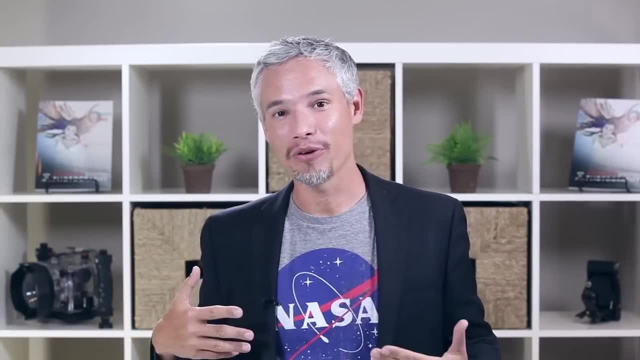 That's what we say in the software world anyway. It's really just shallow depth of field. As I was mentioning earlier, when you focus on something, there's one single focus plane and if you're in front of or behind that focus plane, you're out of focus. 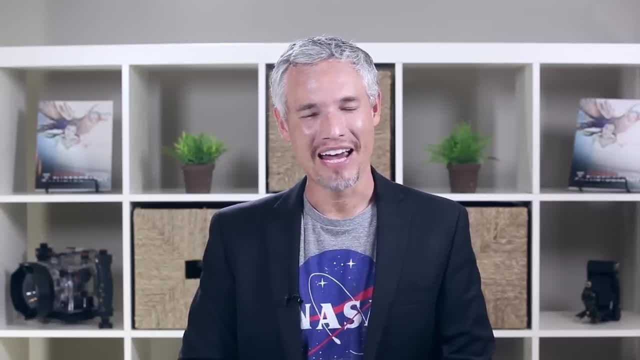 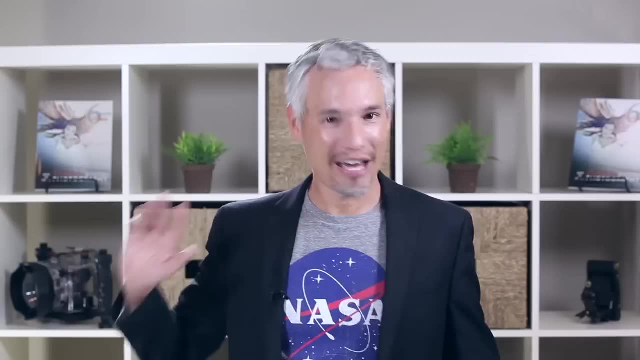 So people will use a lens that has a shallow depth of field, and then they'll wonder why the entire scene isn't in focus. Sometimes you want a nice blurred background, but sometimes you want to capture the Statue of Liberty behind you and you're frustrated that your camera didn't focus. 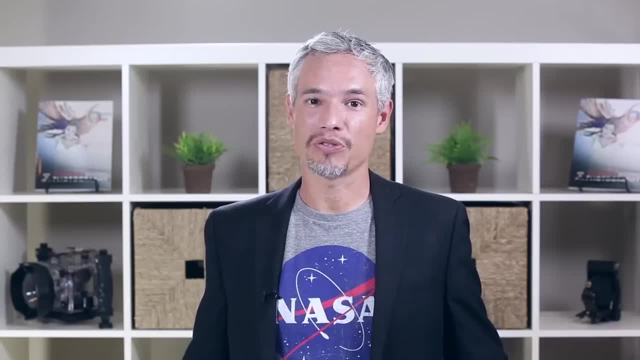 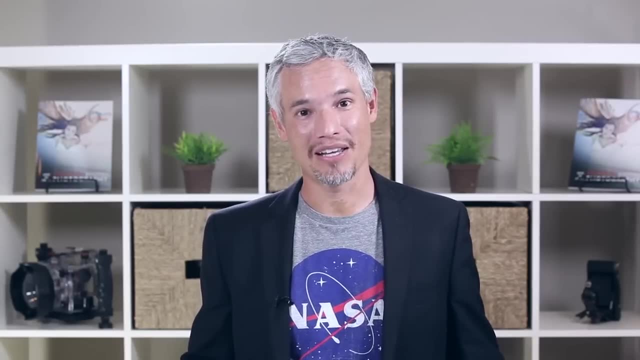 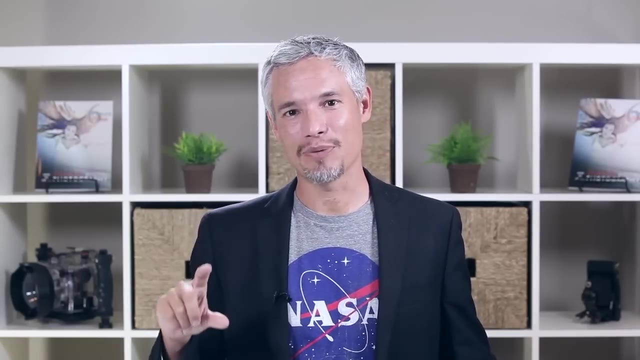 on everything. Here's what happens. People will get comfortable using an inexpensive point-and- shoot camera or a camera phone, and these cameras, because they have inexpensive, inexpensive lenses on them, tend to capture everything in focus because they have a high minimum f-stop number. So you get used to using these kind of inexpensive wide-angle lenses. 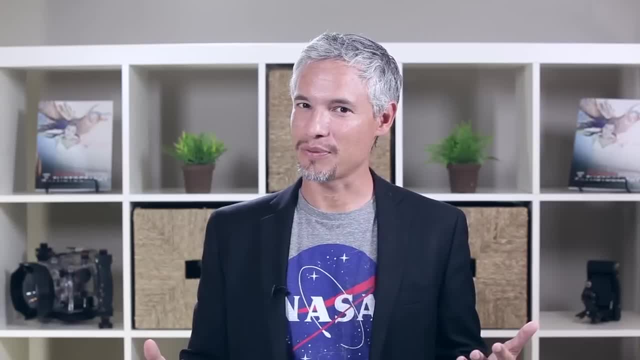 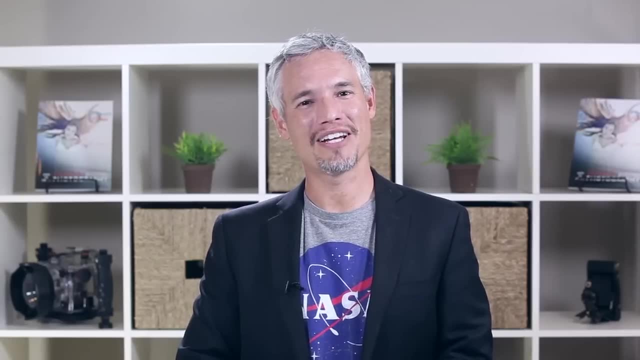 and everything's in focus all the time. You don't really worry about whether you're focusing as precise or not. and then you switch to a DSLR. Maybe you get yourself a nice fast lens and suddenly it's really frustrating that your daughter's face is in focus, but her friend's 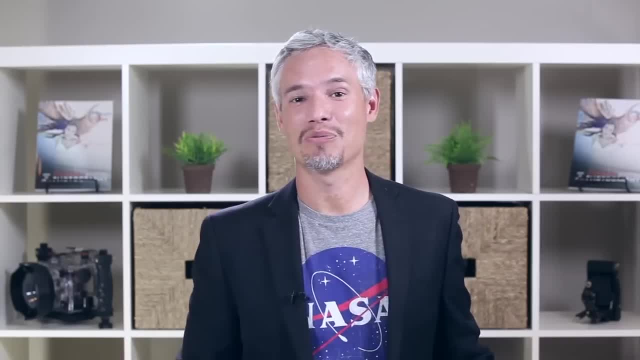 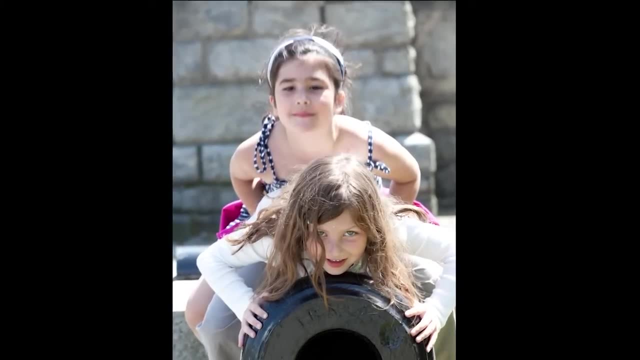 face is completely out of focus. I'll show you some sample pictures so you know exactly what I'm talking about. Here is a picture of my daughter and her friend and, as I was saying, my daughter's face is perfectly in focus and her friend is completely out of focus. It's not the camera's fault. 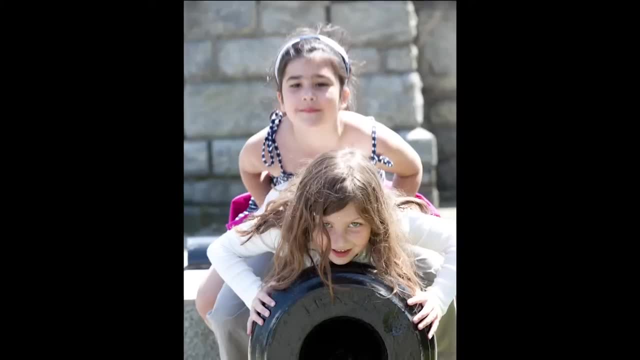 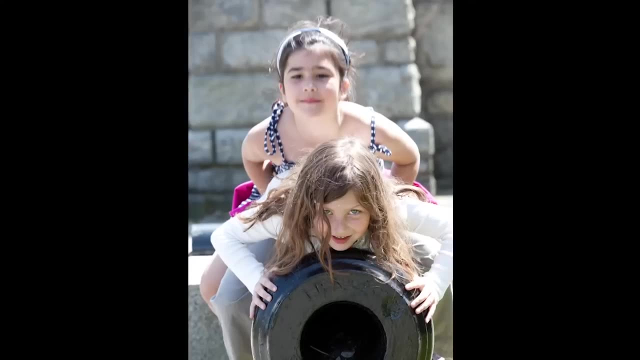 it was my fault because I chose an f-stop number that was too low. I shot this at f4,, but if I wanted to get both their faces in focus, I should have increased the f-stop number to f16.. So in these cases you want to put your camera into aperture priority mode. 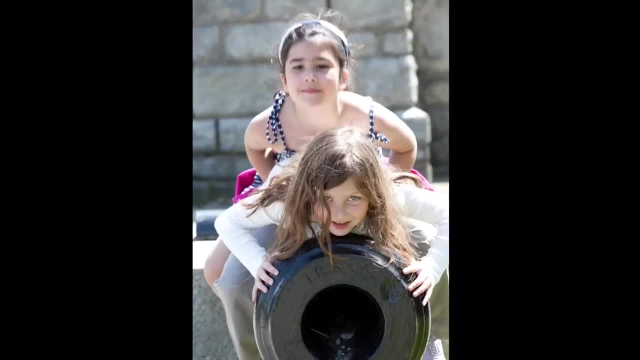 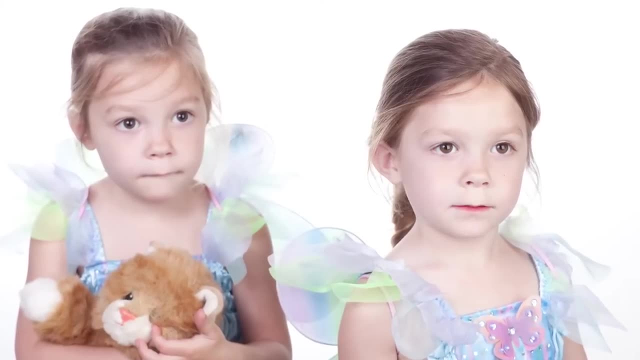 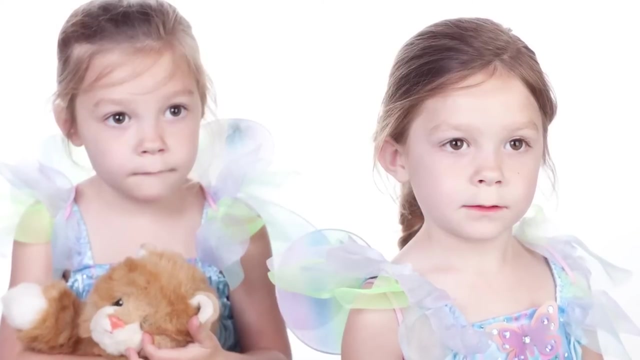 select auto iso and then use the main dial to select a high f-stop number Again, f16 or f22.. Here's the exact same problem, but in a studio Now, with group portraits like this or couples portraits, you need to use a high f-stop number. If it were an individual portrait, I could. 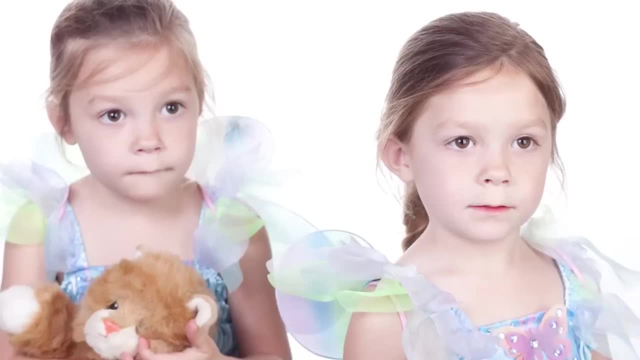 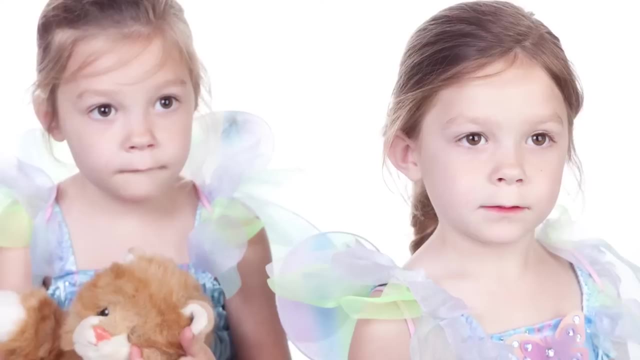 just focus on the person's closest eye and the rest of the scene would just fall into place perfectly. But with multiple people I need to get every eye sharp, all of them, and you can see the girl on the left there. her eyes are completely out of focus because the other girl isn't lined. 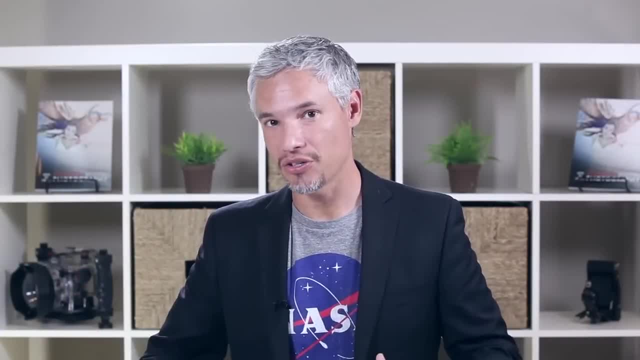 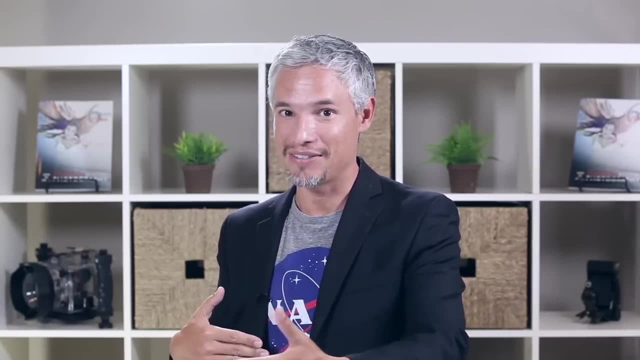 up with her. She's a little bit in front and remember that focal plane: it's two-dimensional and if you're behind that focal plane you're going to be out of focus. So we extend the depth of field, We make that focal plane bigger, in essence by using a higher f-stop number For 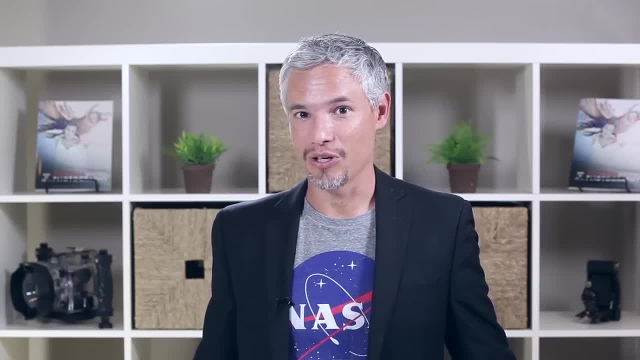 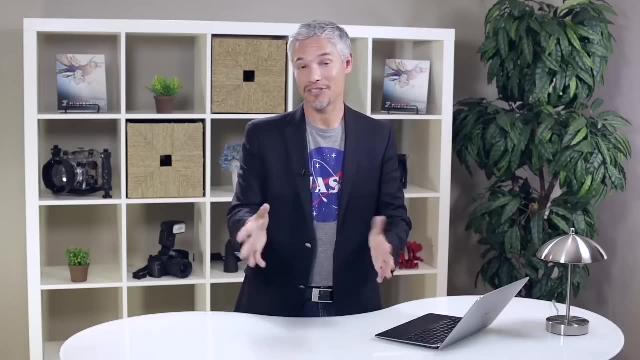 detailed information about that, refer to the controlling your camera video. Shallow depth of field can be a problem in landscapes too, especially if you put something in the foreground and something in the background. That's a good compositional technique. It adds depth to the 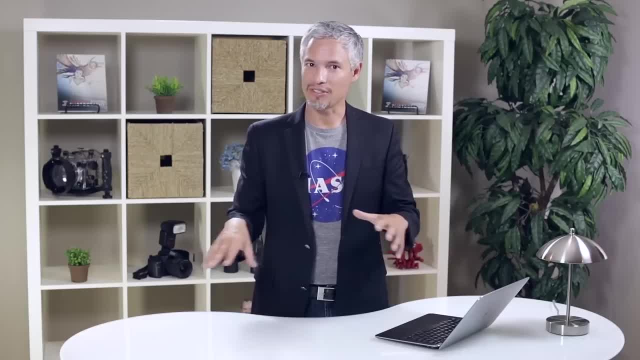 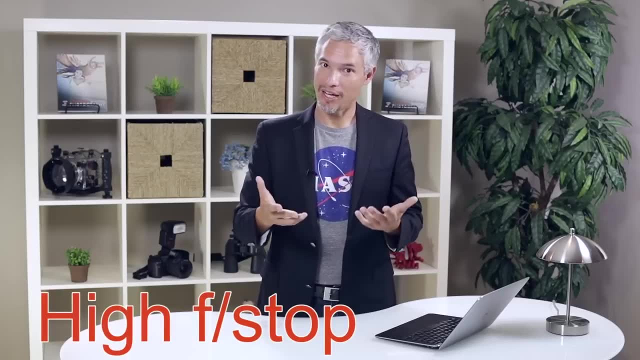 picture, but it's very difficult to get some grasses in the foreground in focus and get the mountains in the distance in focus. So if you're behind the focal plane you're going to be out of focus. The way you can do this is, of course, by using a high f-stop number, even the highest f-stop. 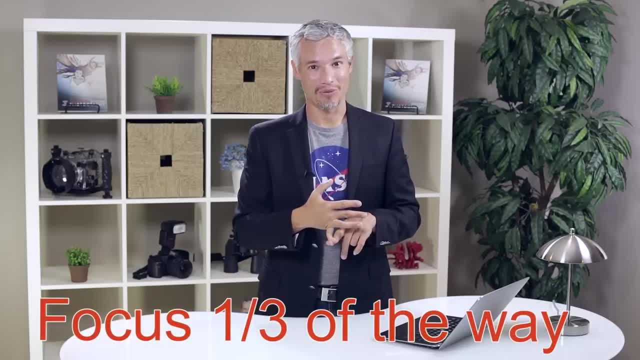 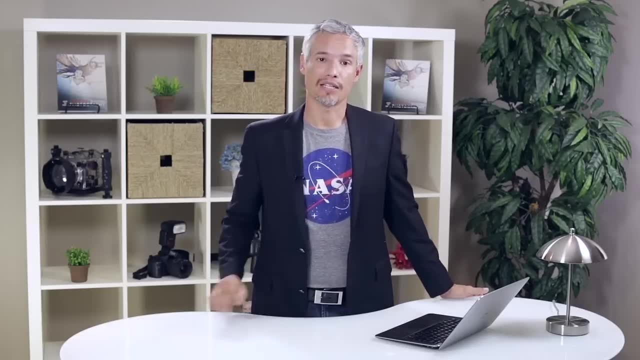 number. You can also try to focus one third of the way through the scene. Focusing one third of the way through the scene maximizes the depth of field. If that's still not enough, you can use a technique called focus stacking. With focus stacking, you take a picture of the foreground, you take a 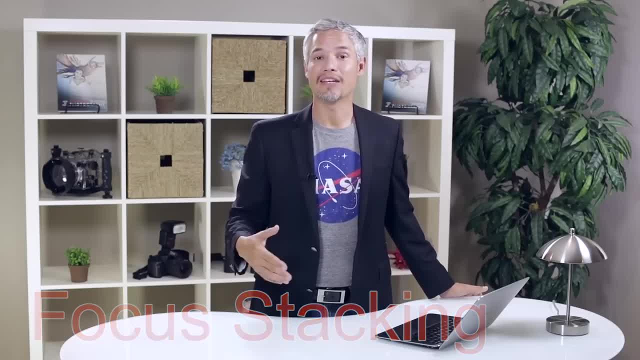 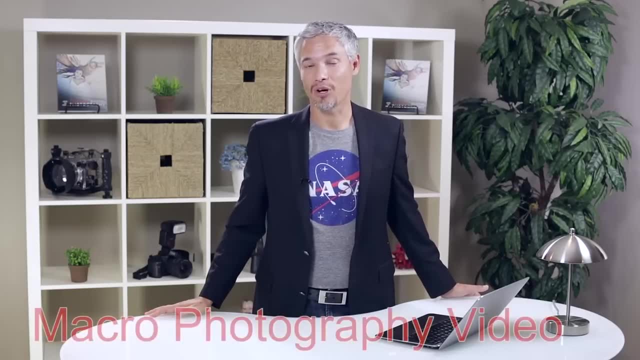 picture of maybe the middle ground and then you take a picture of the background. Then you can blend those pictures together and get basically infinite depth of field. For more information about focus stacking, watch the macro photography video. Now I've covered a lot of different reasons. 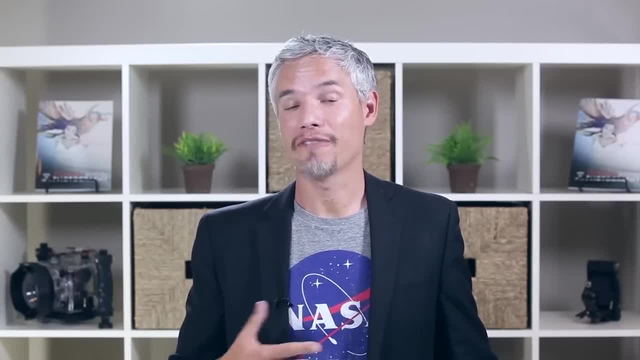 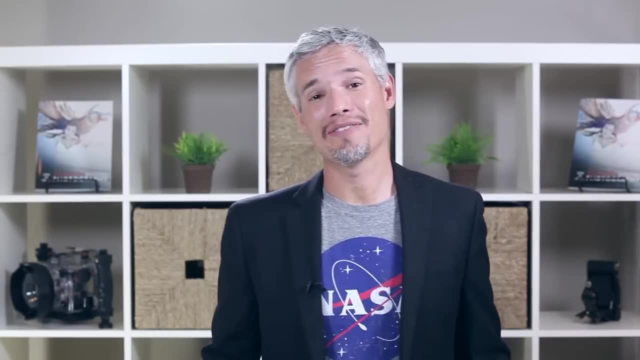 that your pictures can be blurry or out of focus. I find that a lot of people still think it's the camera's fault. It's rarely the camera's fault, It's rarely the lens's fault. I would say in 95% of the cases it's user error of one type or another. That's good news and bad news. The good: 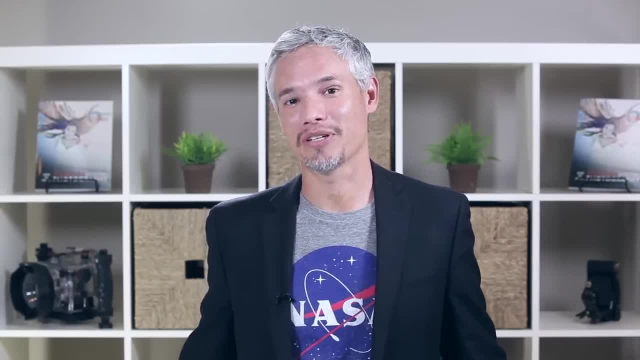 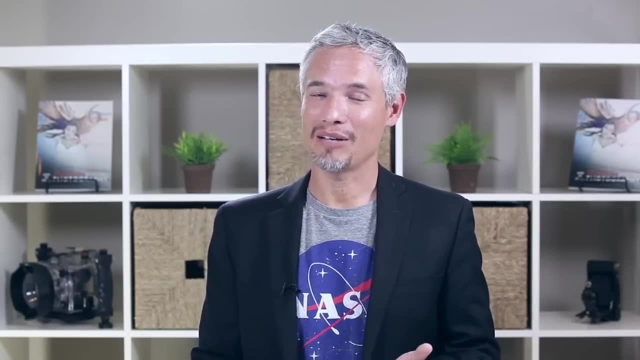 news is you don't have to send your camera in for repair, which would be really expensive. The bad news is you only have yourself to blame. You don't have to send your camera in for repair, which would be really expensive. It's usually some technique issue that you need to work on, but I'd rather do 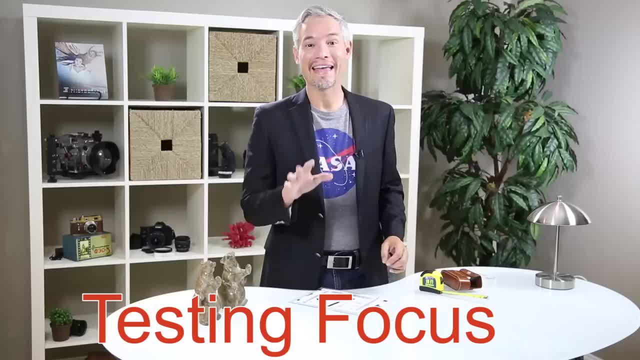 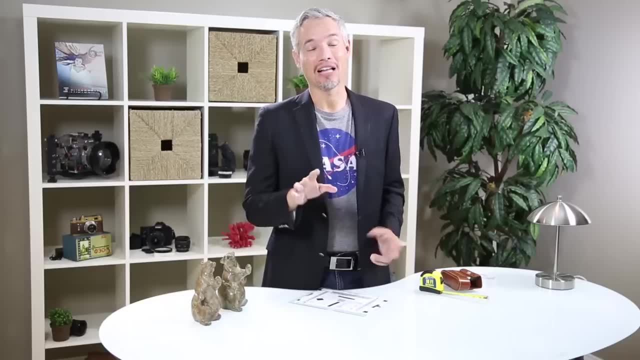 that than send my camera into Canon or Nikon. If you think your lens or camera might actually have a focusing problem, I'll show you how to test it. Now, a lot of people just kind of willy-nilly test their camera and it doesn't focus right and they think they've identified the problem. But as we've 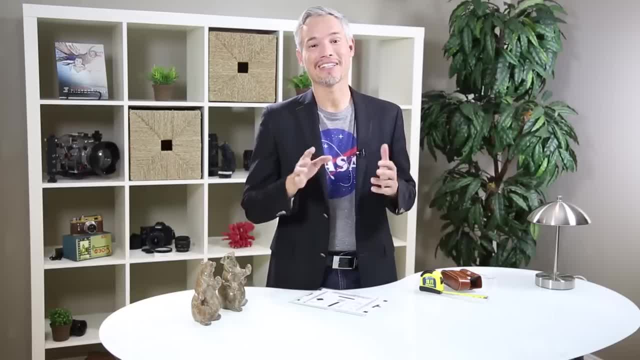 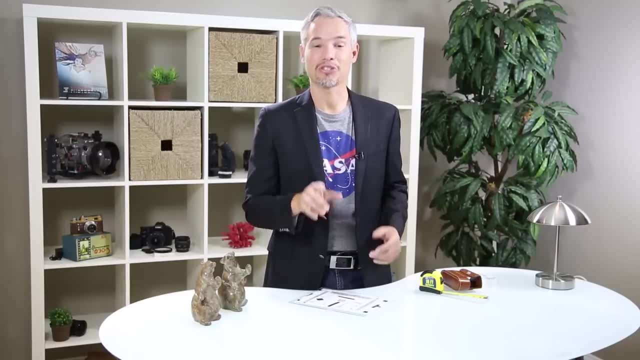 learned focusing. problems can be caused by so many different conditions that it's almost certain that you're just diagnosing the problem. It's usually not a hardware problem, but I'll show you how to identify exactly if it really is a hardware problem, And you're going to start by making yourself a 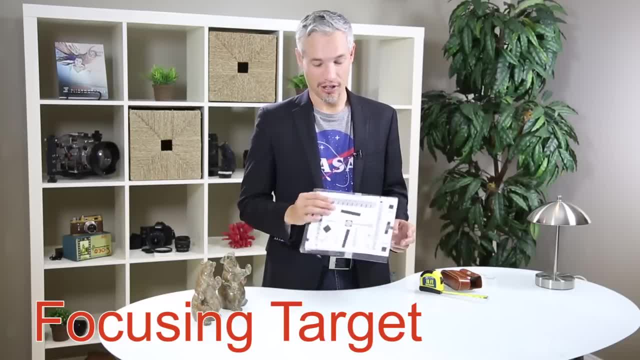 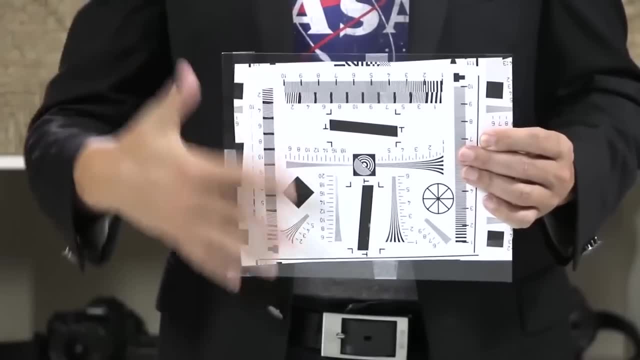 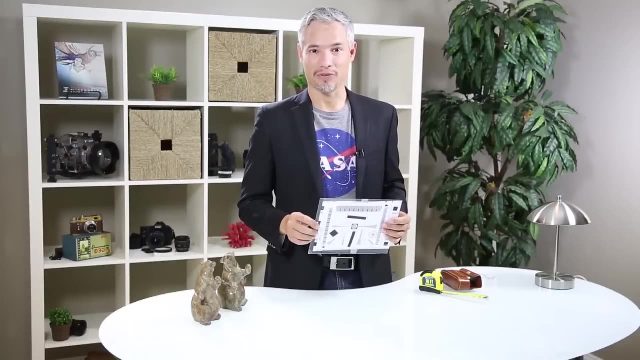 focusing target, And all I've done is I've gone online and printed out a random focusing target. You don't need anything in particular, so as long as it's black and white, I mean, you could use any piece of paper that had black and white writing on it. And then you want to steal a piece of glass. 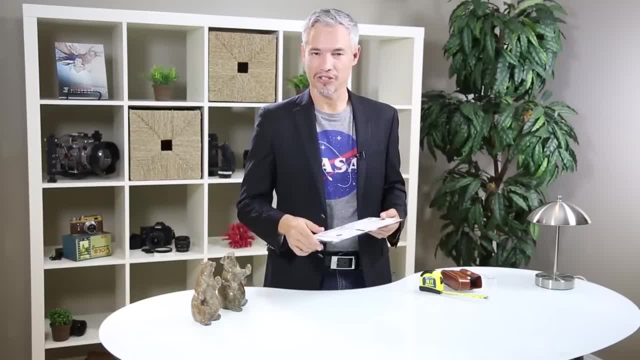 from a picture frame and tape it into a paper, And then you want to take a piece of paper and tape it to the glass just as flat as you can. Now, the reason you're not taping it to cardboard is cardboard might move or might flex. Glass is always perfectly flat, And when you're talking, 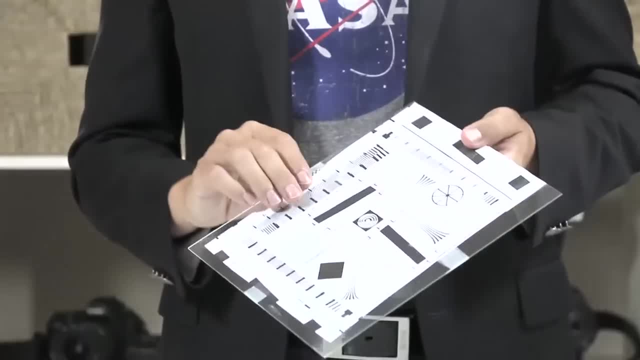 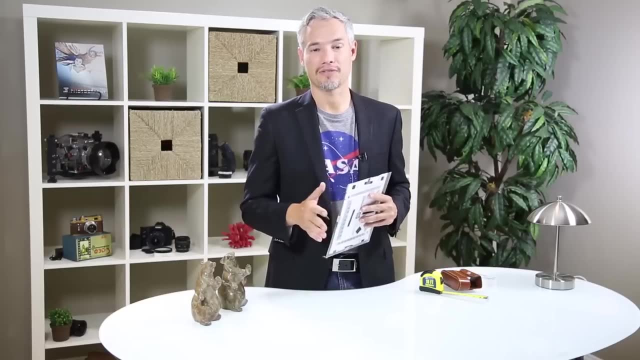 about measuring focusing problems. we're talking about millimeters here, So even if the paper were to peel off from the side a little bit, that little millimeter could show up as a focusing error. So you really want this to be just as flat as you can possibly get If you were to print it. 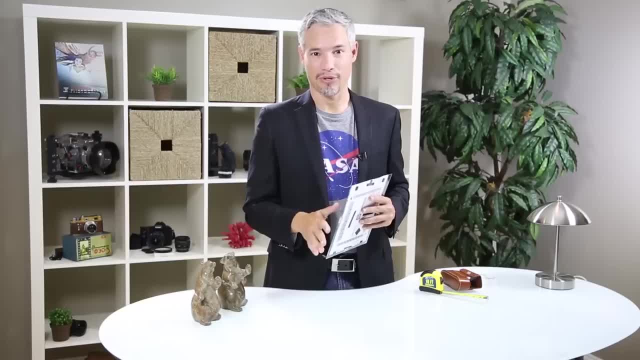 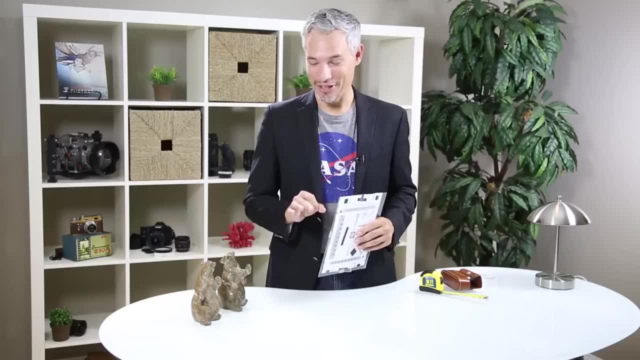 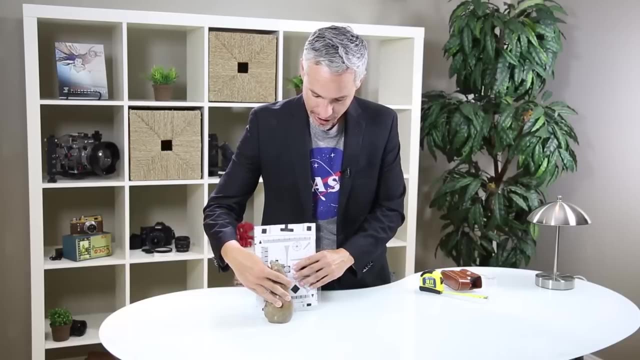 on a sticky label. that would be even better than taping a piece of paper to it. Now we need to make sure that the focusing target is held perfectly upright, And this needs to be really, really vertical. So I'm going to have my bear friends here hold it up And I suggest that. 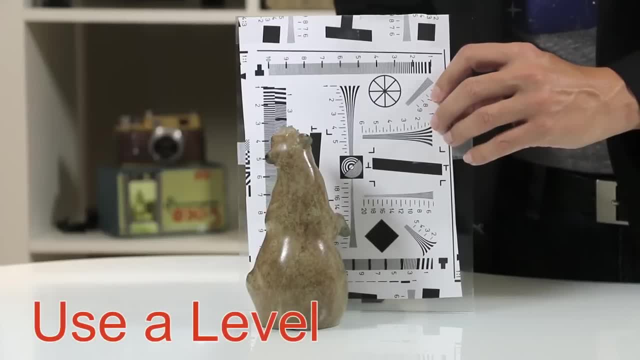 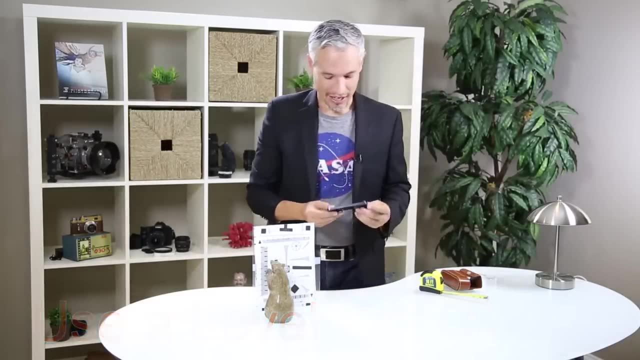 you grab a level and make sure that it's perfectly vertical. I don't happen to have a level, But I do have my phone here And I know that the edges on it are a perfect right angle, So I'm just going to push it against it and make sure that it's completely straight. 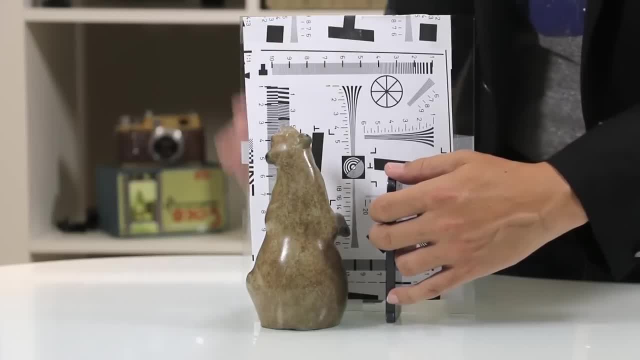 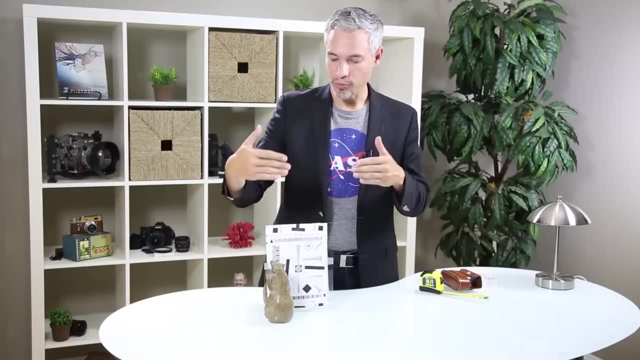 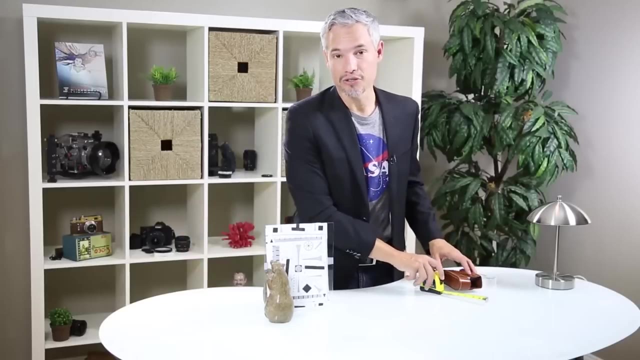 So now I know I can focus my camera on this focusing target And the focal plane will be completely parallel to the sensor, heading off in all directions here. So what I need to do to measure if there's a focusing error is put something that has measurement markings on it. 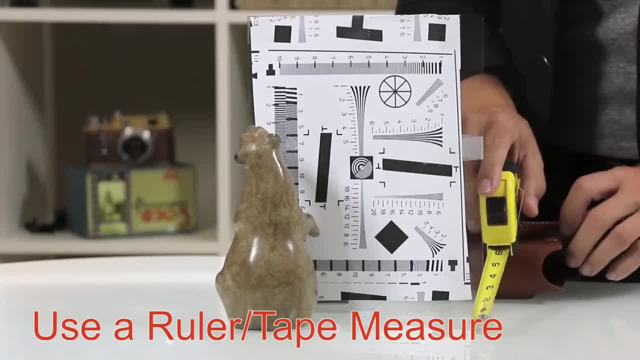 like a tape measure. A wooden ruler or metal ruler works even better. I'm just going to tilt this down at an angle because if I were to lay it flat it would be a little bit more difficult. So I'm just going to tilt this down at an angle because if I were to lay it flat it would be a little bit. 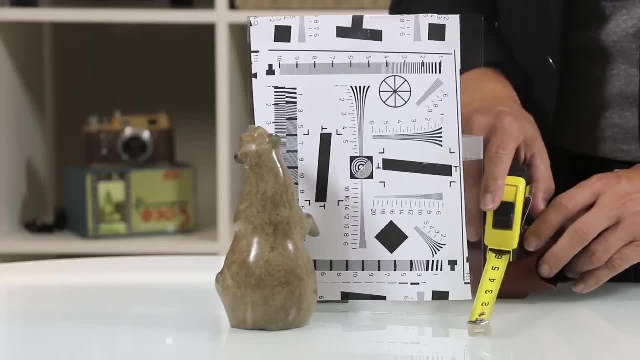 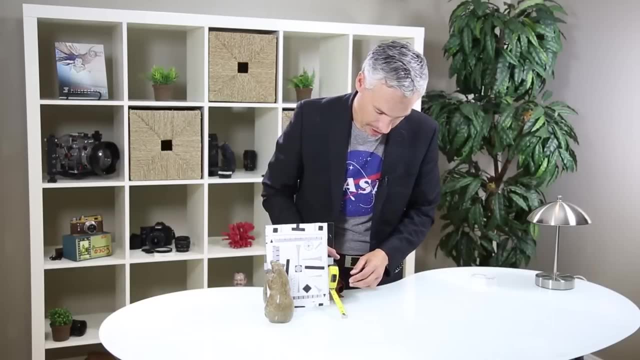 more difficult. So I'm just going to tilt this down at an angle, because if I were to lay it flat, well, I wouldn't be able to read the numbers on it from where I'm going to put my camera. So for my purposes, I'm just going to put this ruler right against the glass there, right on the number four. 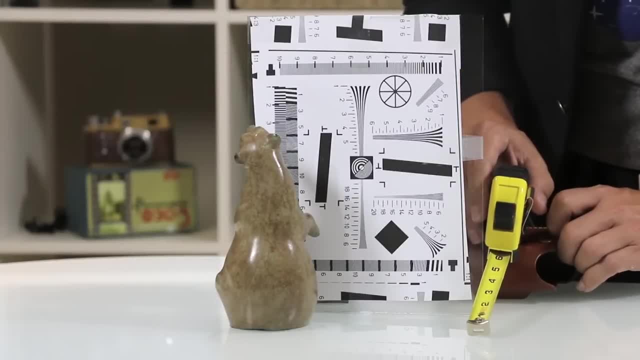 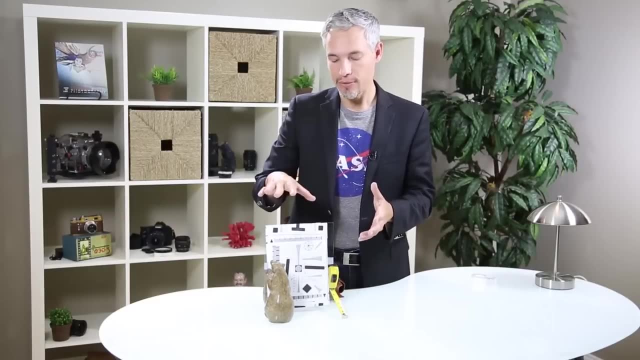 You actually want to line it up with the front of the glass, like wherever the front of your paper is, because we're measuring with as much precision as possible here. So this is going to be my focusing target And I'm going to line my camera up at exactly the same level as this and focus. 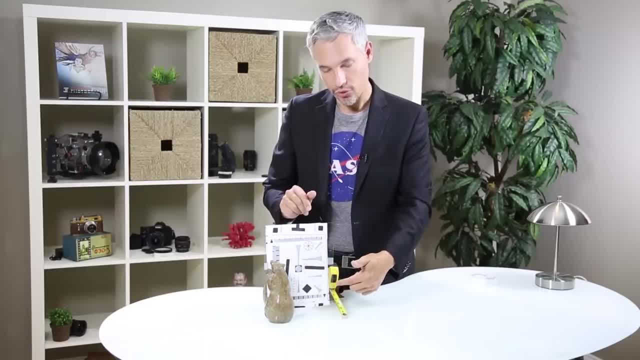 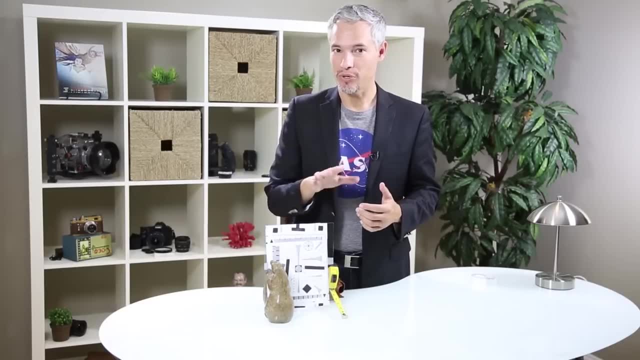 somewhere on the contrasty area of the camera. So I'm going to line my camera up at exactly the same area of the camera of the target. then I'll be able to look at the ruler and see exactly where on the ruler it focused on And if it's front focusing or back focusing it'll be pretty. 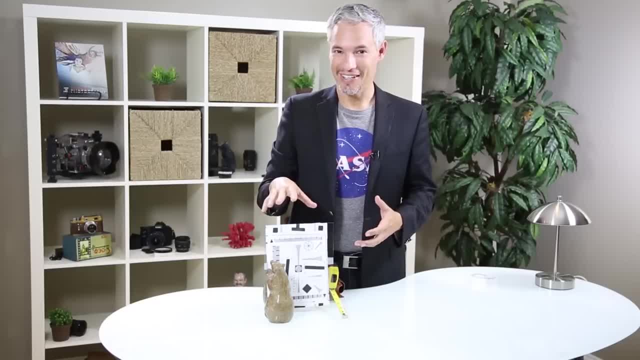 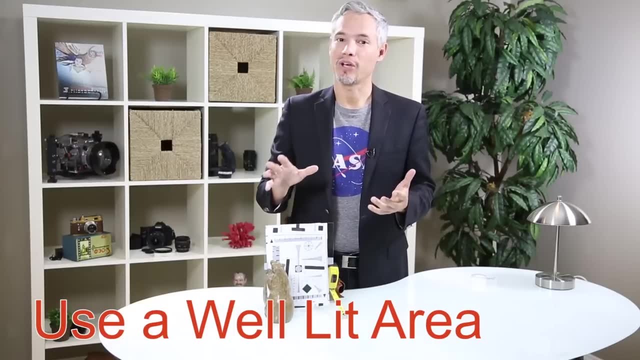 obvious. at this point. I'd also like to point out that I have bright lights shining on this. you don't want to do this in dim lighting, because dim lighting reduces your camera's ability to focus. We really want to create a scenario that allows the camera to focus in the 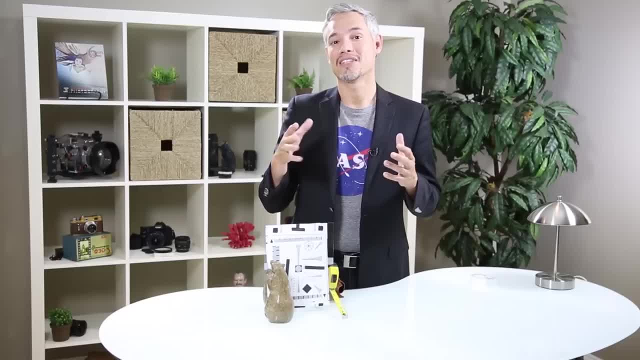 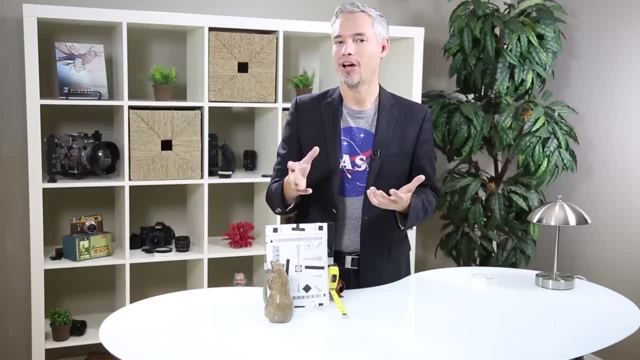 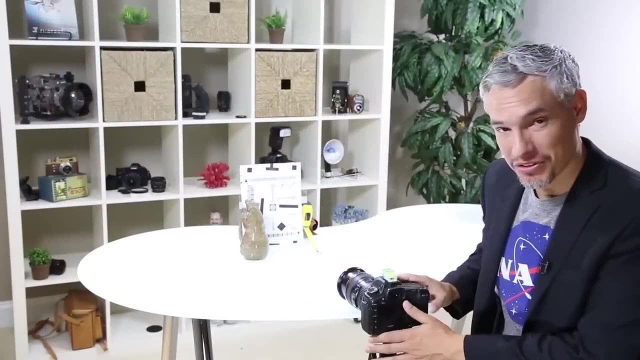 best possible scenario, because this will ensure that it's as accurate as it can be and eliminate the possibility that the focusing problems are caused by some other source. So this looks pretty good to me. Now I'm going to set up my camera. Now you'll notice that I have my camera on a tripod. This is because so many 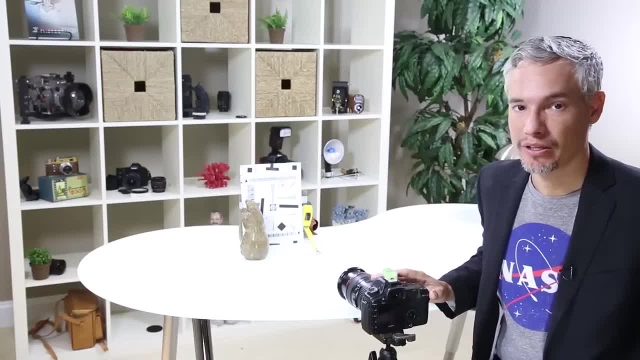 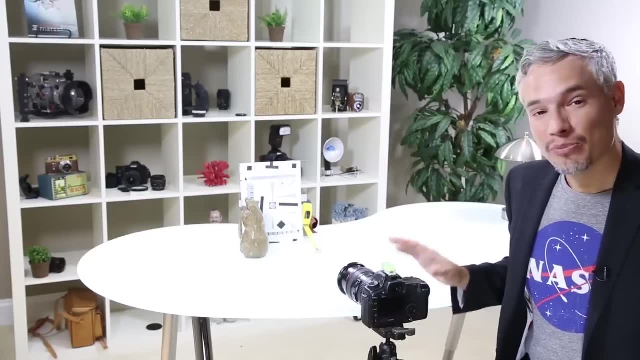 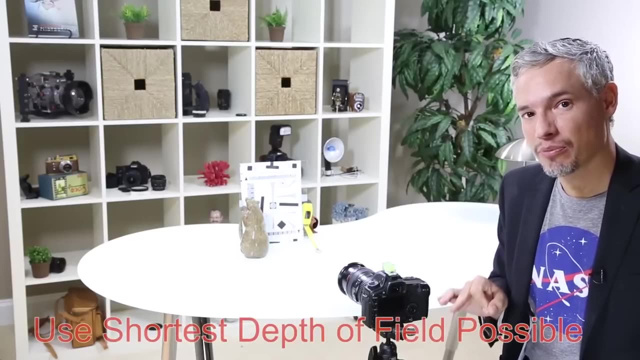 problems with non-clear pictures can be caused by camera shake or a moving camera, so the tripod is really important if you want to eliminate all other problems. To make any focusing problems as prominent as possible, I want to set up my lens to use the shortest depth of field possible. The depth of field is the 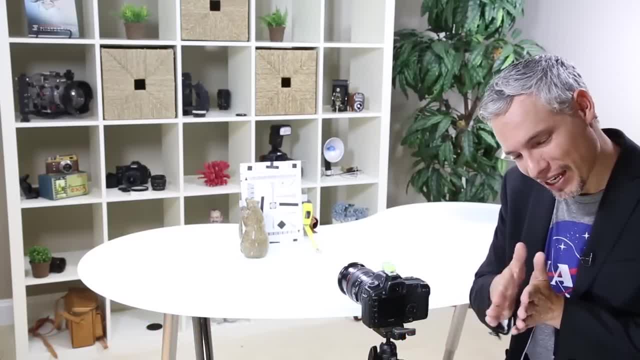 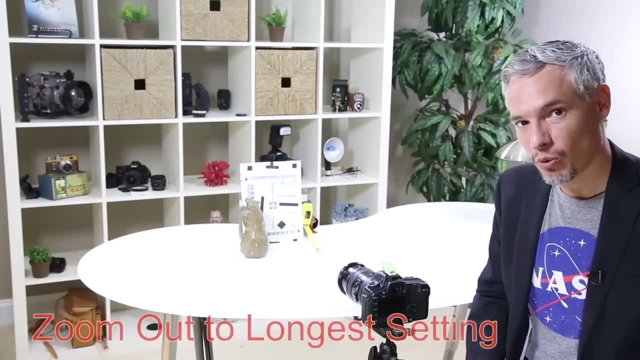 total range that will appear to be in focus. so by making that really nice and shallow, any mis-focusing is going to be really, really obvious. So to get the most shallow depth of field possible, I'm going to zoom out to the longest setting. 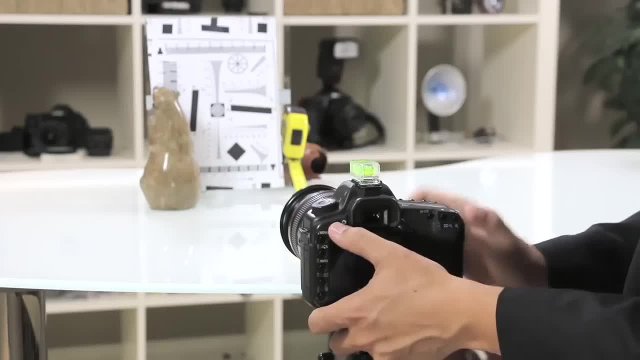 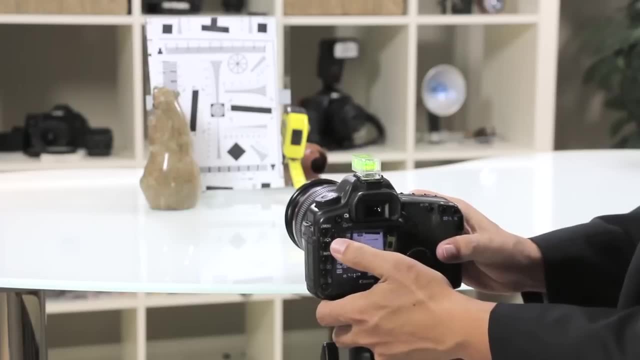 On this camera. it's a hundred and five millimeters. Next I'll move the camera until it's almost in focus, but not quite. I still want the camera to have to auto focus on it. Alright, that's pretty good. Just make sure you're about close to the minimum. 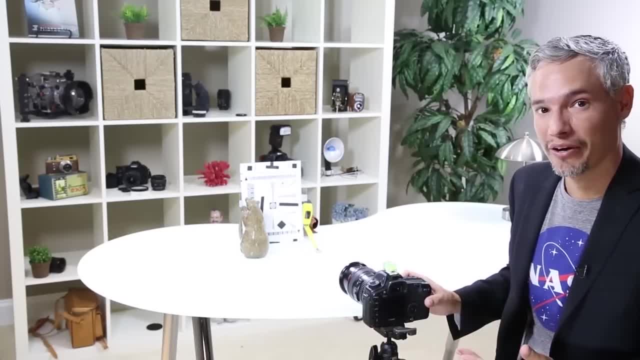 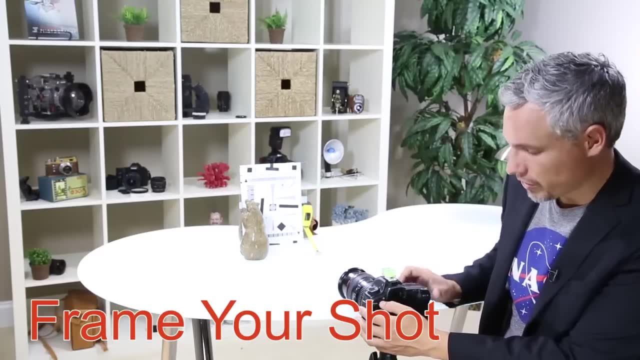 focusing distance on the lens and that you're zoomed all the way out. Now I need to go ahead and frame it so that I can see both the focusing target and the ruler here. So for convenience, I'm going to turn on live view, even though I won't. 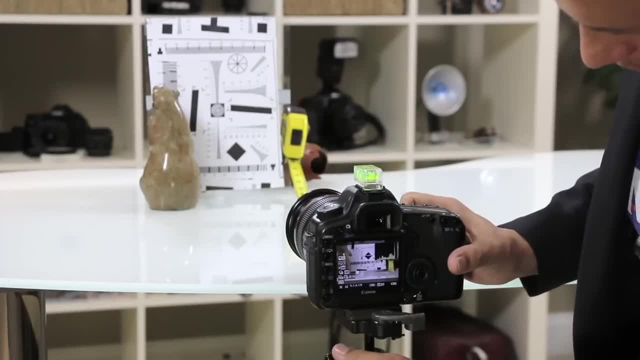 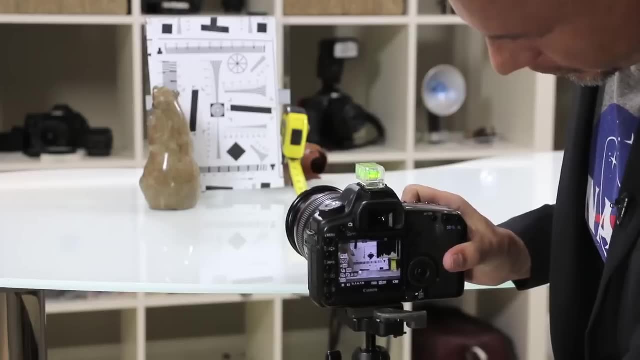 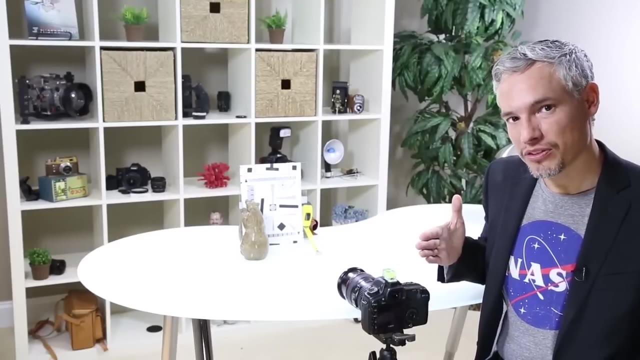 do my shooting in live view And that actually looks pretty good. I'll adjust the height of it up just a little bit. There we go, that's good. Now, the way the focal plane works is it's always completely flat and completely parallel to the camera sensor. So I need the 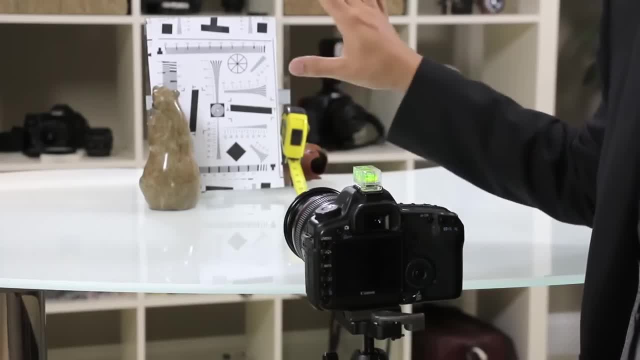 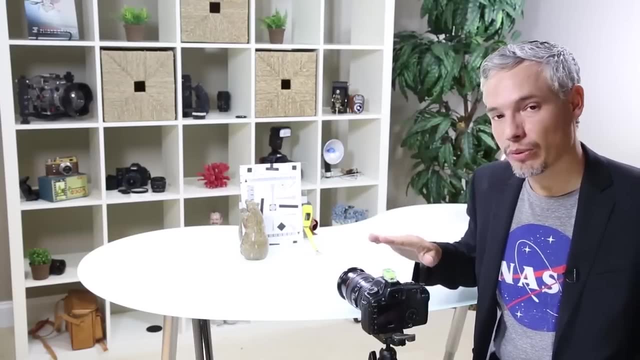 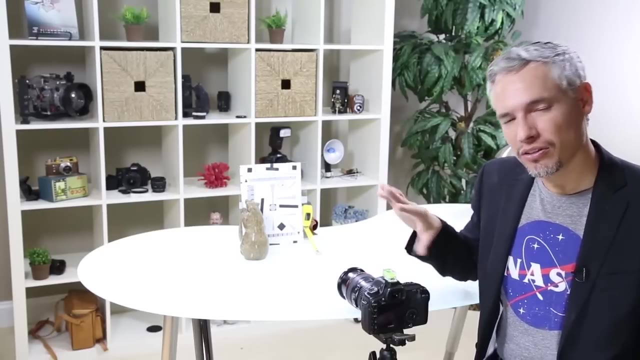 camera's digital sensor to be perfectly parallel with my testing target there. And because I made sure my testing target was perfectly vertical, perfectly upright, I need to make sure my camera is perfectly vertical too. Most modern cameras happen to have a digital level built into them, So check your camera's manual, see if you have that. 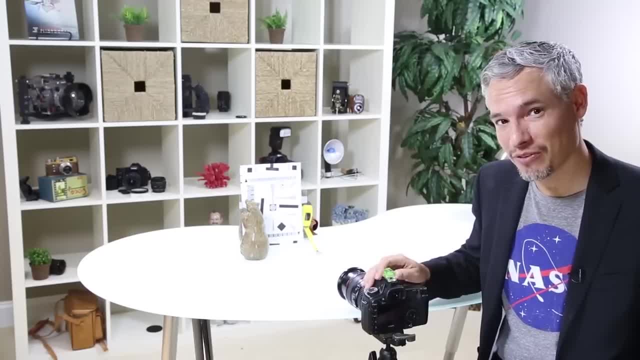 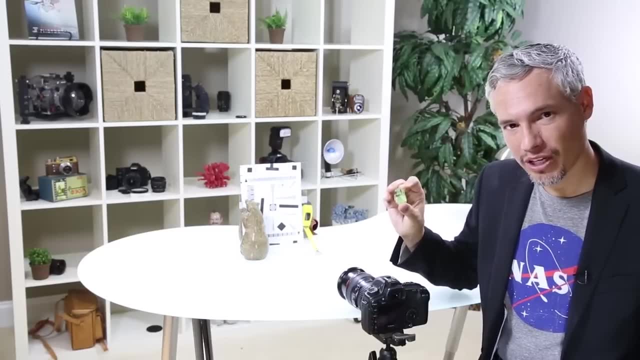 feature built in. Sometimes you can just hit the info button enough in live view and it'll. it'll show you that level. If yours doesn't have it, you can pick up a bubble level for just a couple of dollars. Amazon sells them, V&H sells them, and 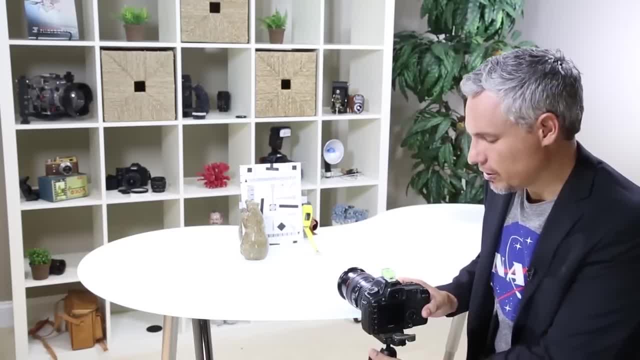 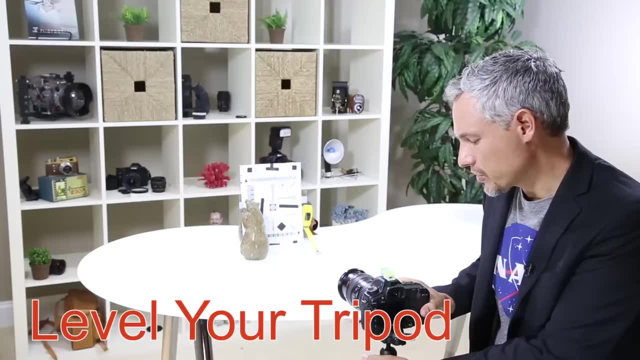 they go right in the flash hot shoe. So I'll put that in there and then I'm gonna adjust my tripod to make sure that it is perfectly, perfectly level. Now I don't care if it's twisted left to right, we just need to make sure it's tilted. 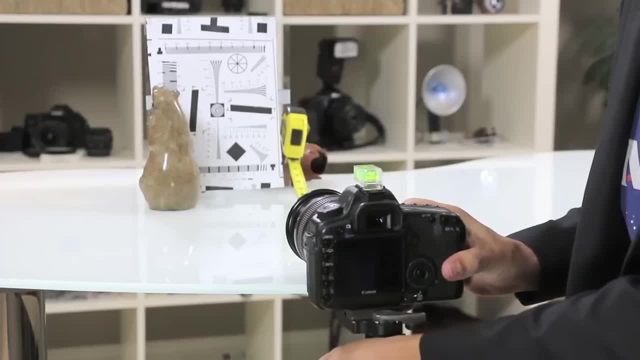 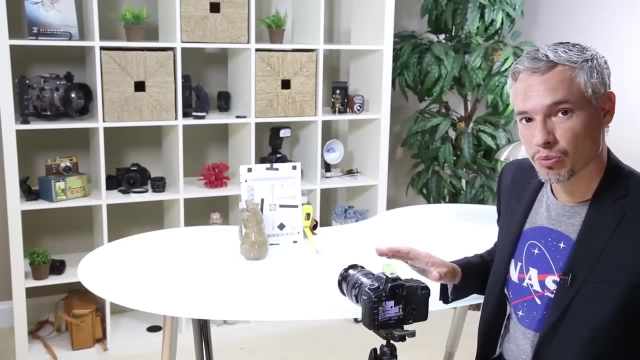 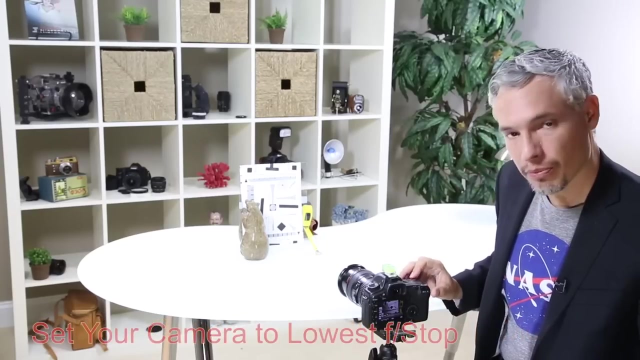 up and down to be perfectly level. So my camera positioning is all set. Now I'm going to put my camera into aperture priority mode. I'm going to select the lowest possible f-stop number by moving my main dial On this camera. it is 4.5, on. 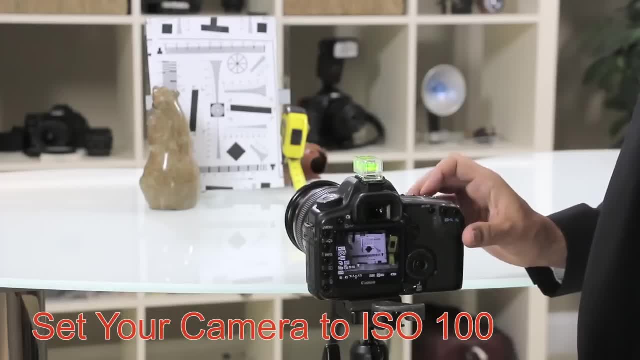 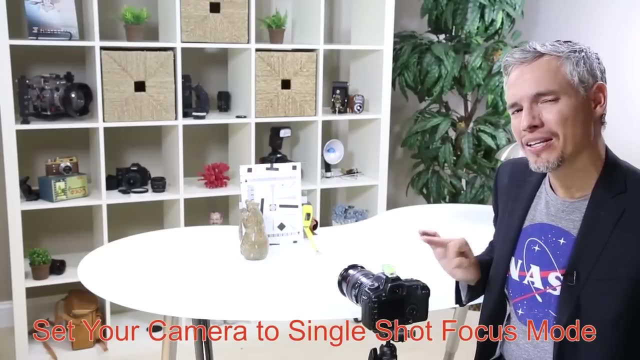 this lens, rather. And now I'm going to select ISO 100.. And now I'm going to set the focus to 100.. And now I'm going to set the focus to 100.. And now I'm going to set the focusing type to the single shot focusing mode. This is going to be called. 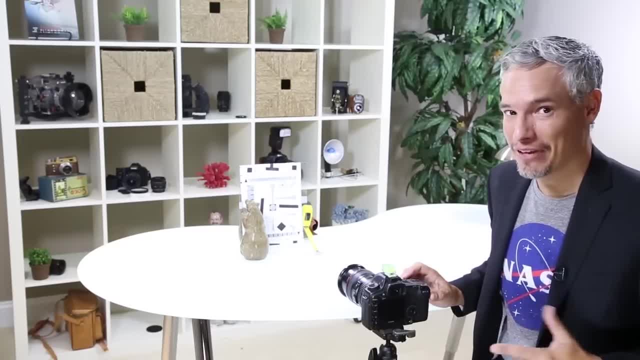 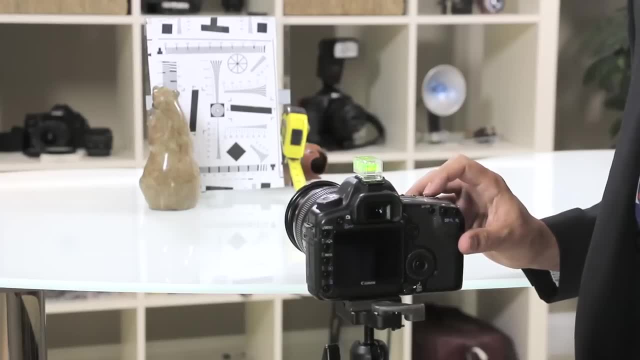 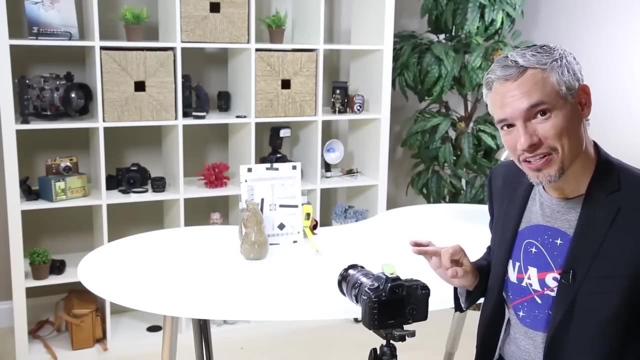 something different on different cameras. Most of the camera world calls it AF-S, including Sony and Nikon. In the Canon world it's called one shot. The single focusing mode causes your camera to focus until it achieves a focusing lock. Sometimes it doesn't happen instantly, it might have to hunt. 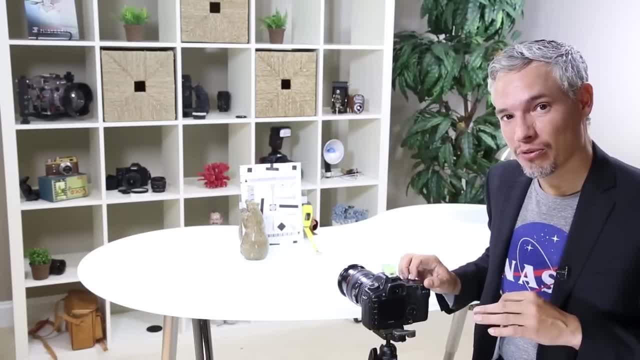 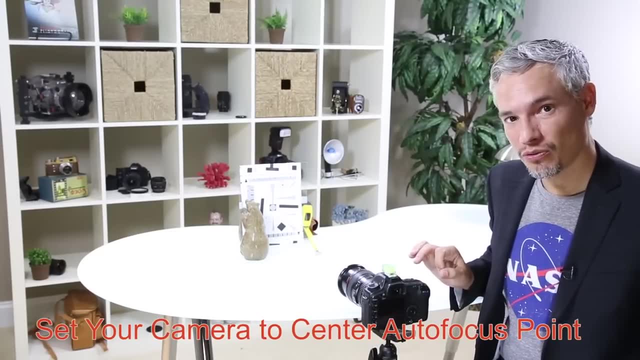 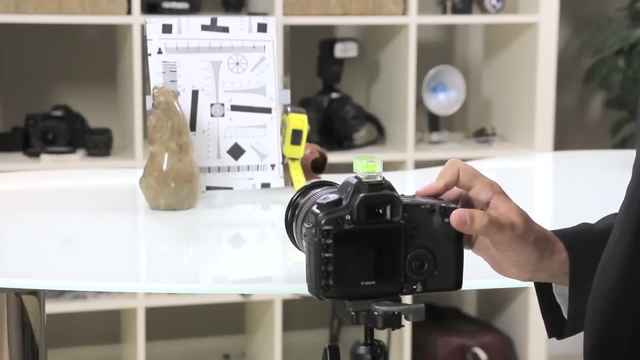 around a little bit, But it's the ideal way for your camera to focus, and that's why we want to use it for this test. Next, I'm going to select only the center autofocus point. Now, before I actually take a picture, I'm going to just mess up the focusing on. 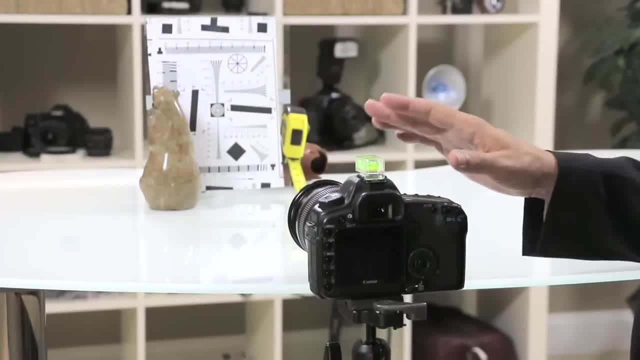 the lens because I want it to actually work, So I'm just going to give it a twist so that it will have to focus. Now my camera is all ready for the test. I need to make sure that live view is turned off and then look through the 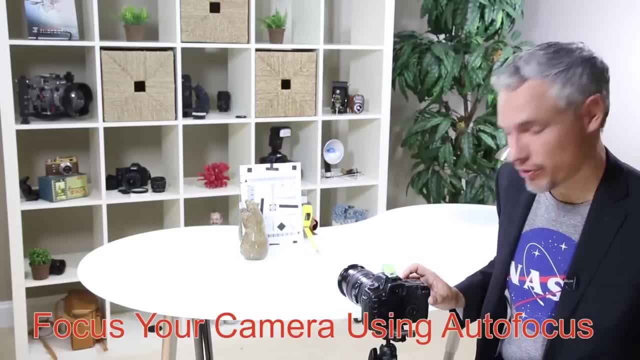 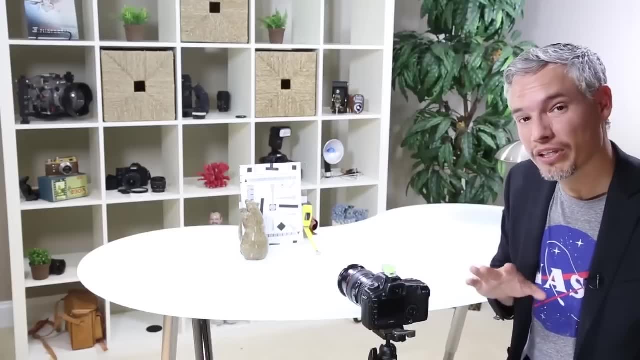 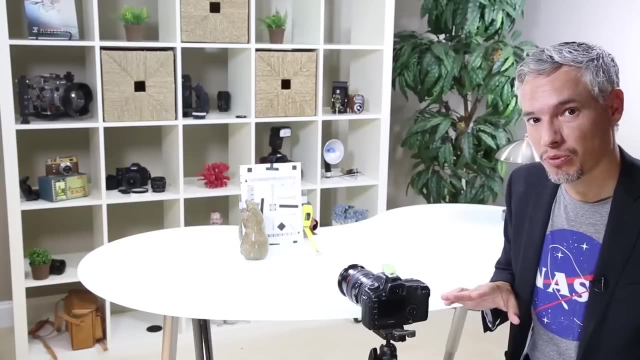 viewfinder and focus the camera Using the autofocus system. Now one last thing: before I take the picture, I'm going to set my camera to a shutter delay. I'm just going to configure it to wait two seconds after I press the shutter. The reason for this is that when I push the shutter button, it 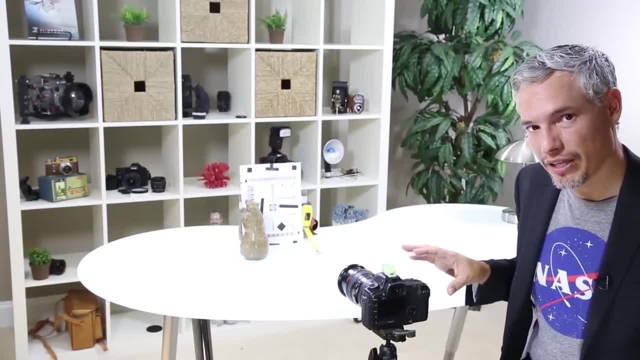 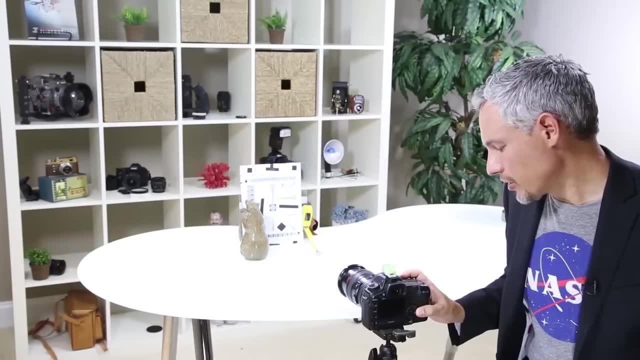 can introduce a little bit of camera shake. I can twist the camera just a little bit and that can cause the picture to be blurry. So by setting a delayed shutter, I can be 100% confident that the shutter is working. I'm not shaking the camera at all. Now I'm ready to push the shutter button. 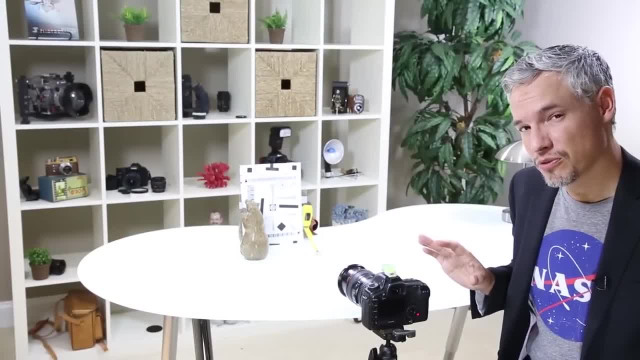 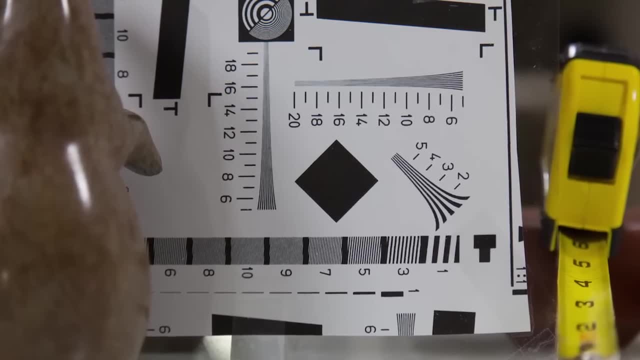 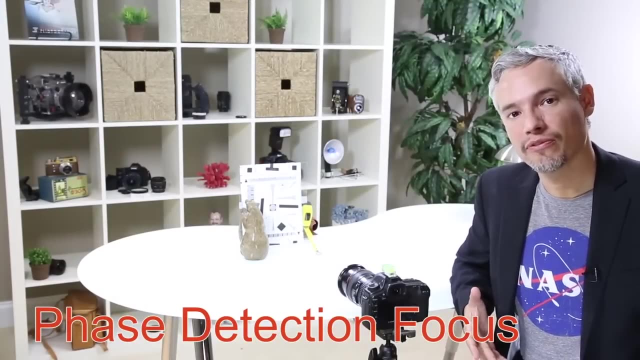 Now go ahead and take a few more pictures, just to have a few to compare to in case something went wrong. Up until now, we've been testing our SLR's phase detection focusing system, and this is your camera's primary focusing system Whenever you're looking through the viewfinder. 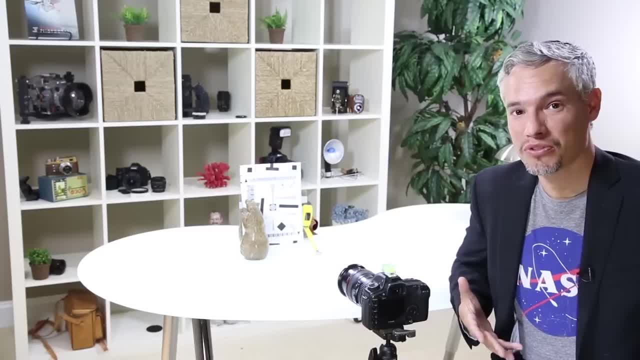 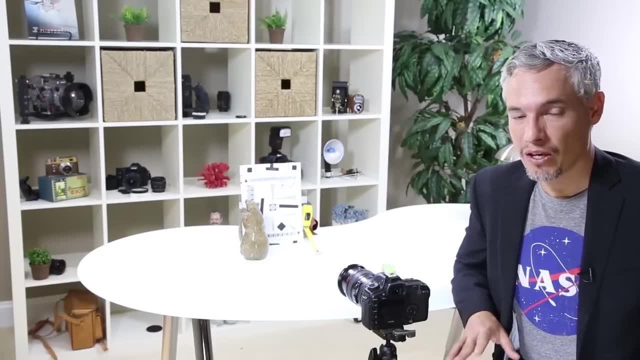 it's using this phase detection system because it's the most effective way to focus And if you do have a focusing problem, either in the lens or the body, this is where it's going to show up. Your cameras other focusing system is a contrast based focusing system, and that's what it relies upon anytime. 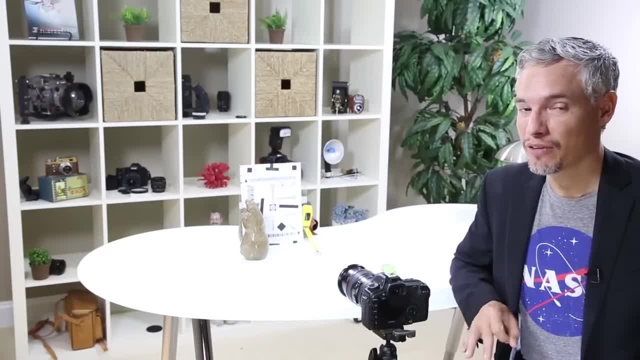 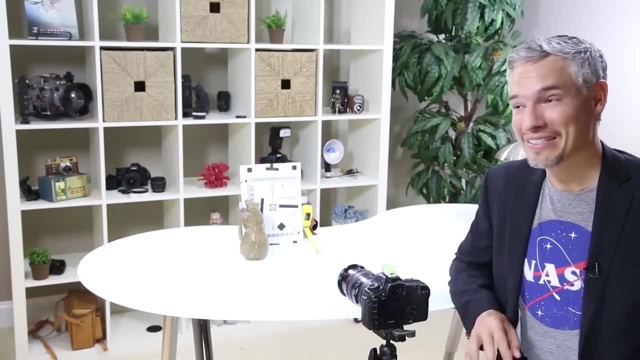 you're in live view mode, So I do also want to take a few pictures with the contrast based focusing in live view mode, because the contrast based focusing isn't prone to any sort of problems. That's because it's actually reading the information in from the sensor itself. 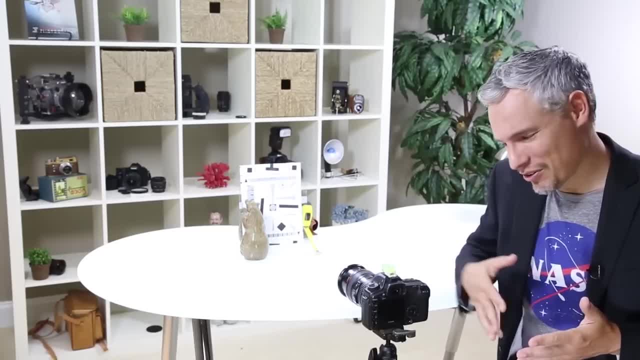 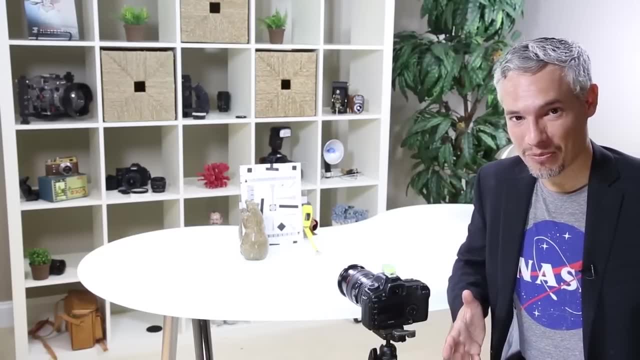 Your phase detection focusing sensors are off the sensor and sometimes they get a little misaligned and that's where your focusing problems can come from. But the contrast based system, because it's using the actual image data, it's basically foolproof. So we're going to take a couple of sample shots with the. 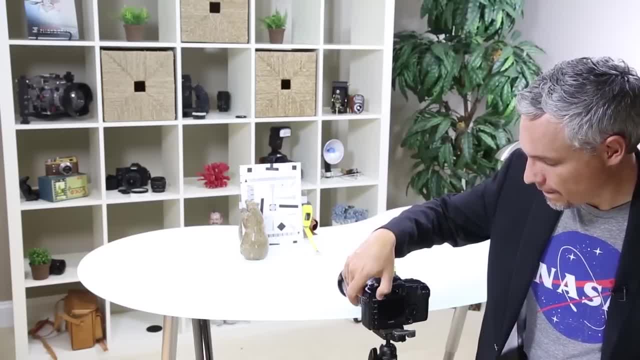 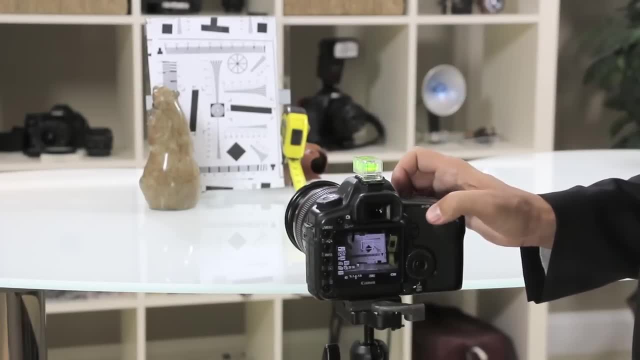 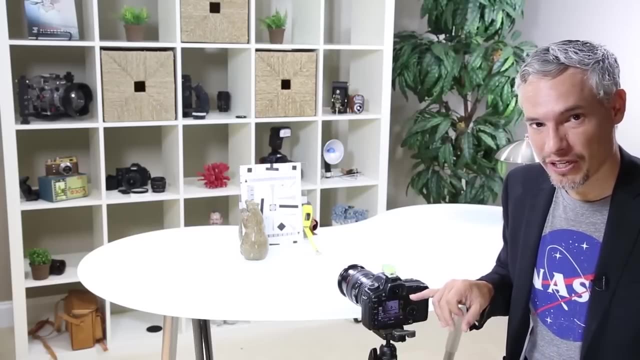 contrast based focusing system just by using live view and then focusing the image. I'm just going to push the AF on button here to allow it to focus. Ah, notice that the image on the live view disappeared for a second and I could. 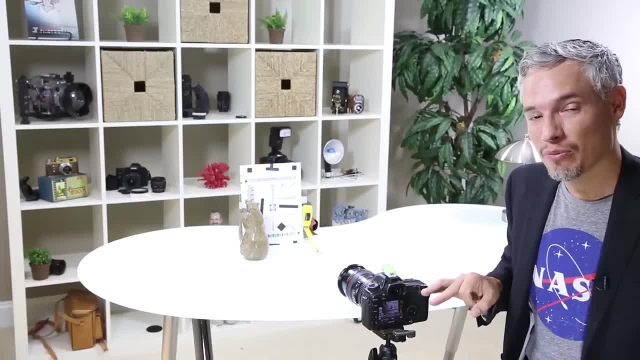 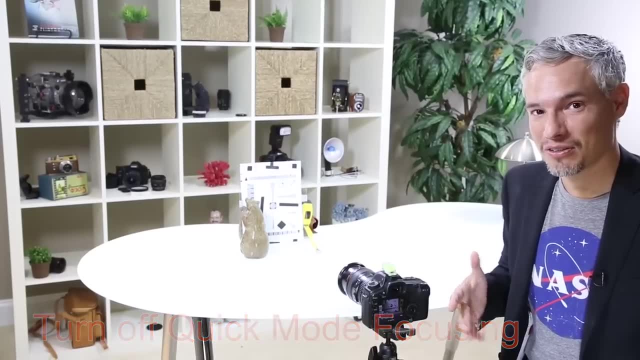 hear the mirror flipping up and down. That's because this camera is in quick mode focusing for live view, and that means that it's still using the phase detection focusing system even though I have live view on, So I want to be sure to turn that off. 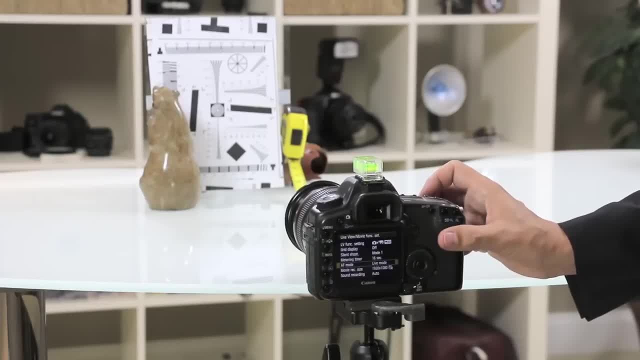 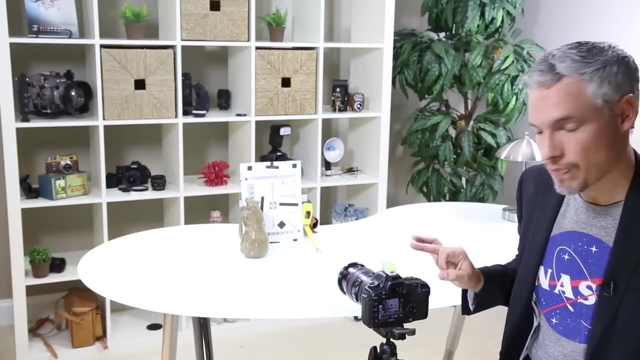 I'll do that now. Now I should be able to focus in live view, so I'm going to press that AF on button so it focuses and that green icon means that it worked properly. and because I didn't hear the mirror, I'm confident that it's using contrast based focusing. Now I'm ready to take. 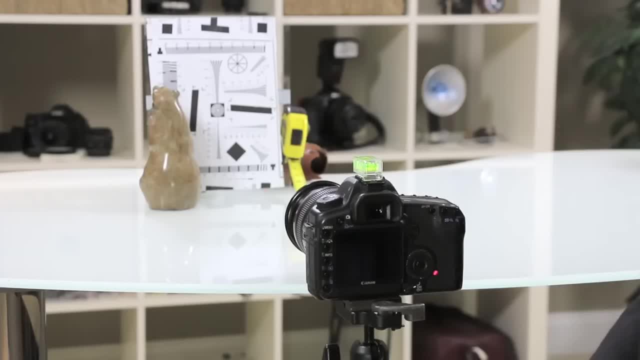 another shot. There's that two second delay and I'll take a couple more shots just to be sure. Looking at the LCD screen isn't going to be ideal. I mean you can zoom in and get some general idea, but for the best results go ahead and load the pictures. 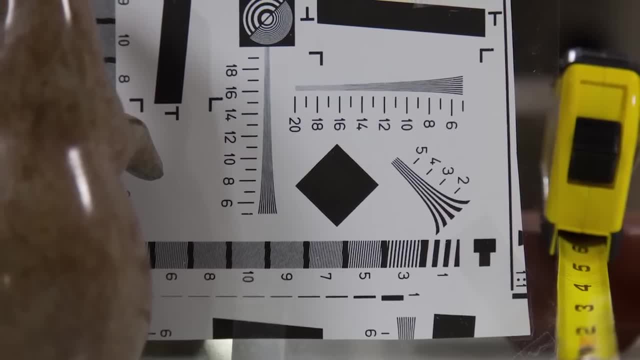 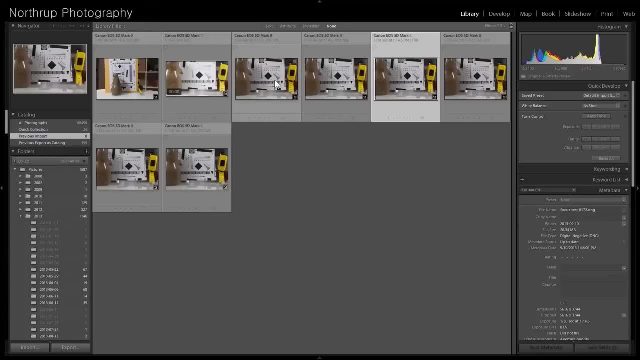 on your computer. So let's go check out my results. Here we are in Adobe Lightroom, which is the app I use to preview and organize my photos. I took three pictures with the phase detection focusing system and then three with the contrast based focusing system in live view. so I want 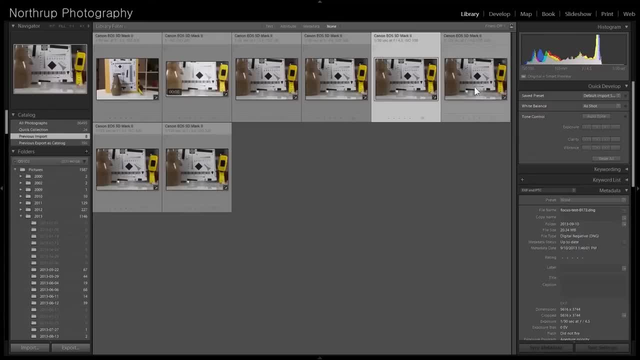 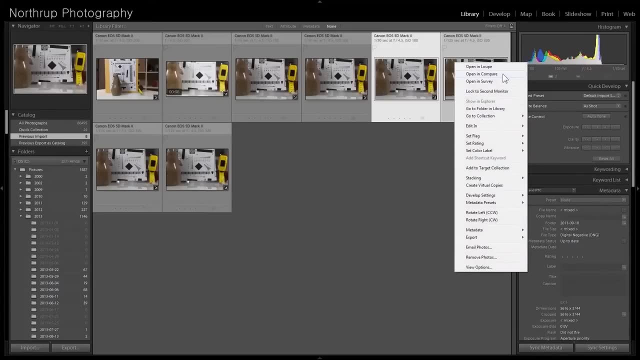 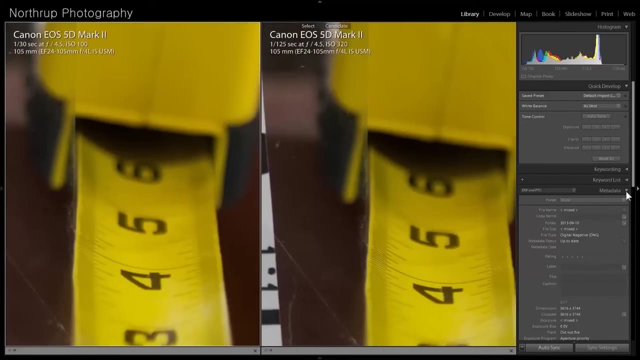 to compare two of these pictures. So I'll take this phase detection one and this contrast based one. I just control clicked them both. Now I'll right click them and then click open and compare. Compare is just a tool that lets you see the pictures side by side. So let's get in nice and close on those pictures and 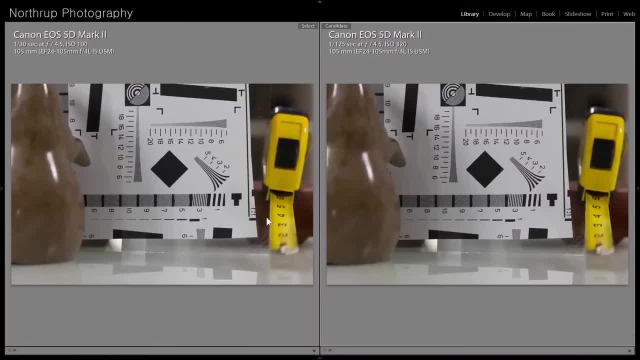 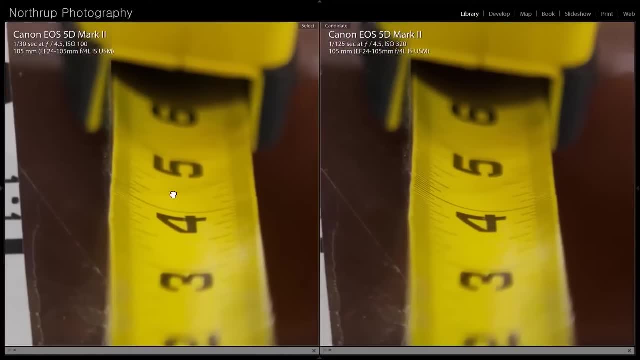 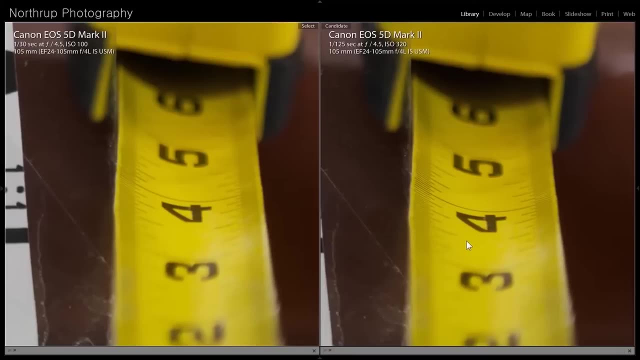 this is the full picture, So I'm going to zoom right into where the numbers on the ruler are. I'm going to use the contrast based focusing picture as my benchmark. So even if I've done something wrong in the testing system, if things aren't, 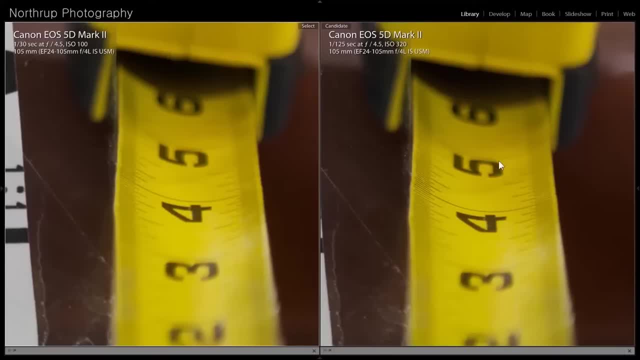 aligned quite the way I thought they were. it'll show up on the contrast based focusing system, So I just want to make sure that the phase detection system is focused on about the same spot as the contrast system is, and indeed it does look like. 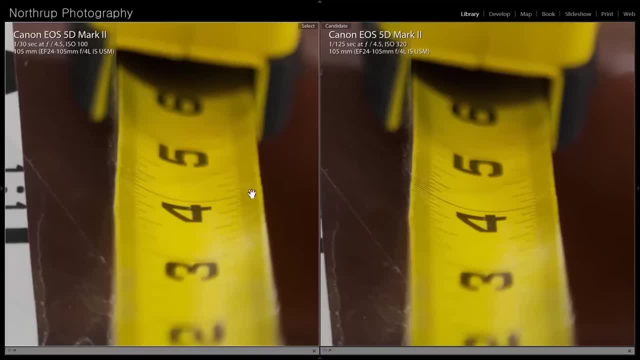 they both focused right about on the four, which is about what I expected. I'm looking at these little lines to see exactly where they blur in and out. Now, an interesting bit of trivia: depth of field extends both in front of and behind your focusing point, but only about one-third of it is in front of the. 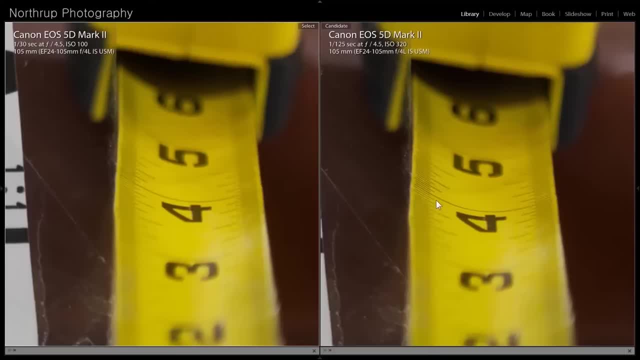 focusing point. So that's a little bit of trivia but it's a little bit of a surprise. So I'm focused right about on the four here and you can see you get it pretty clear for about four or five of these lines here. But as you move back, 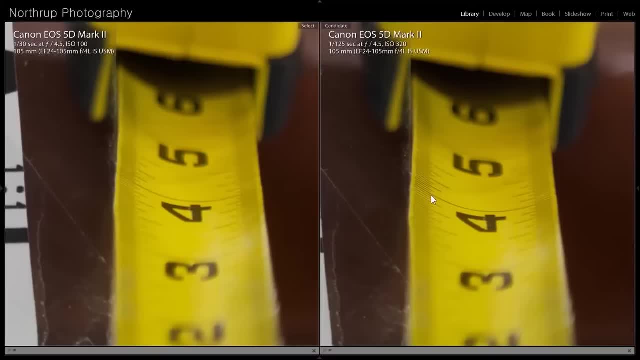 there's about twice as much in focus. This is just an easy way to illustrate a concept: that if you want to get as much of your picture in focus as possible, focus about one-third of the way back from the very first subject that you want to be sharp. Anyway, comparing these two pictures, they do seem to be focused. 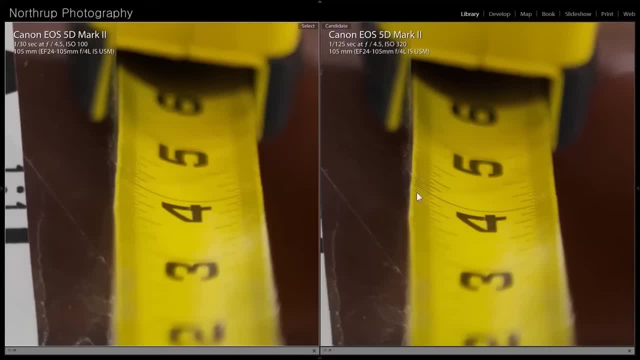 at about the same distance. so I feel like this lens and camera combination are focusing properly. But looking closely, you'll notice that the picture on the left here isn't quite as sharp as the picture on the right. So why would that be? 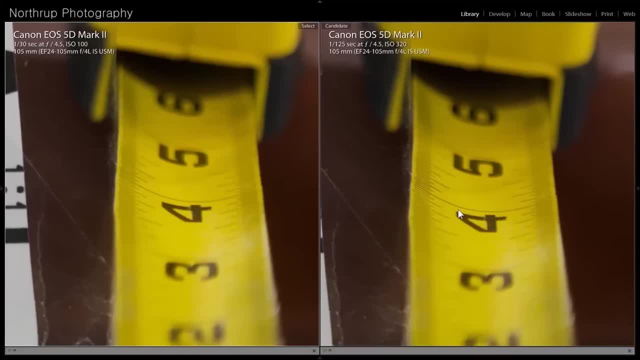 Because I was using good techniques for everything. Well, there was one thing that was different: For the contrast-based focusing picture. here I was using live view and in live view the mirror is up When you press the shutter and you're. 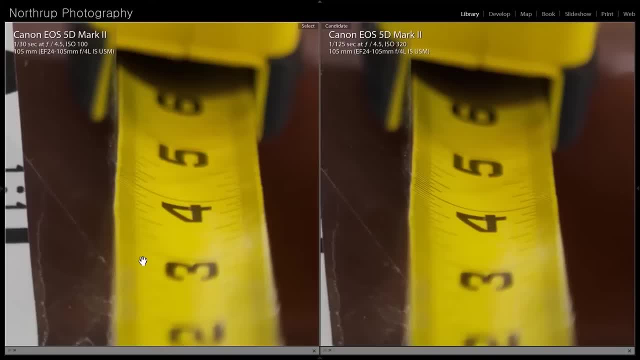 looking through the viewfinder, the first thing that happens is the camera flips that mirror up. Even though I had the shutter on a delay, I didn't have mirror lock up turned on. I probably should have, because the mirror slapping up shook the camera just. 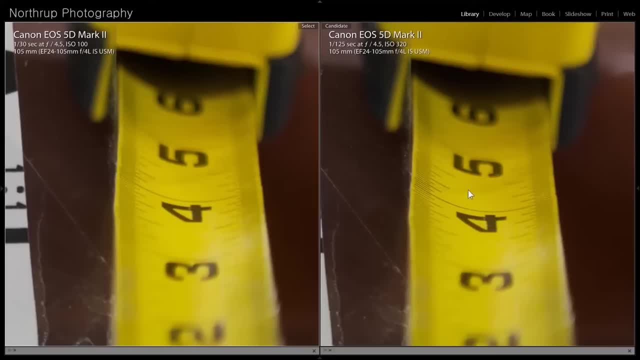 a little bit, and that's why this picture is just a tiny bit less sharp than this one. Nonetheless, it's good enough for me to tell that the focusing system is working properly, and next time I have it on a tripod, I'll have to remember to use the 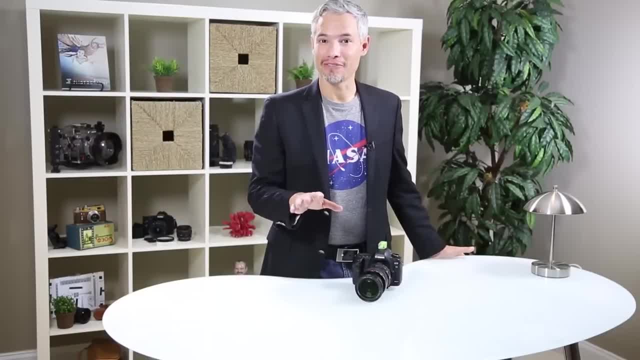 mirror lock up. Now, no matter what your result was, you have a little bit of work to do. If your camera did focus properly in these ideal situations, then you know that you have to update your technique a little bit Now. just the process of testing taught. 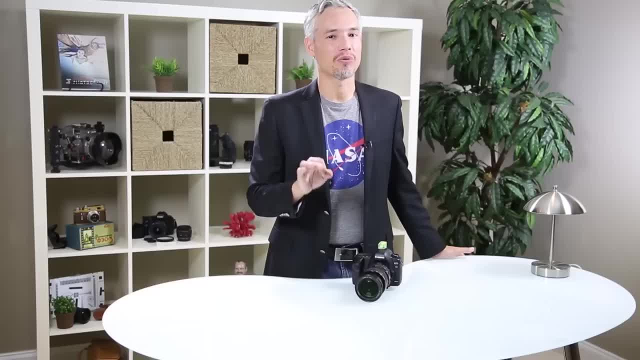 you a lot of the different techniques that you want to use to get really great focusing. You want to use a tripod, you want to put your shutter on a delay and ideally both the camera and the subject are nice and contrasty, well-lit and. 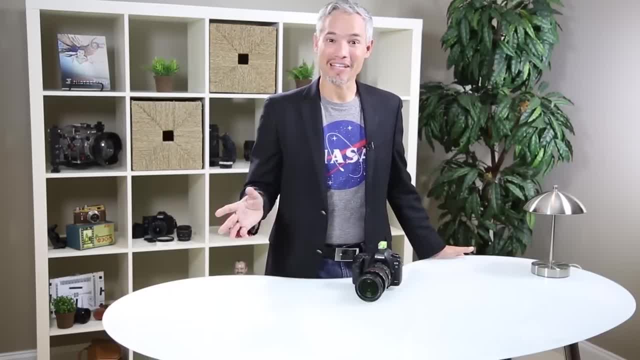 stationary. Anytime you vary from that, anytime things get a little dim or subjects aren't contrasty like they're just grays or nice fading colors, focusing is going to be much more difficult and a lot less breathable, So it's going to be a lot less precise. 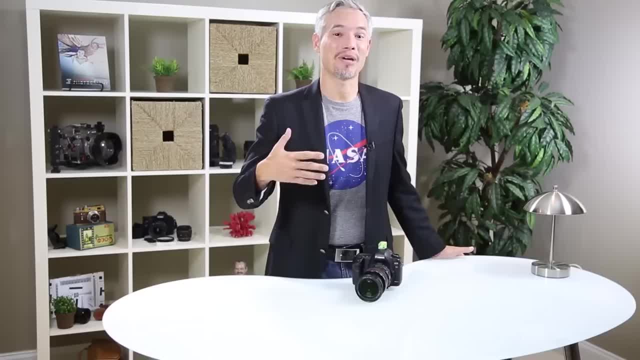 It also happens when your subject doesn't have to be completely flat, because your focus system might pick up on the tip of somebody's nose or their ear or something in the background, and so that causes all sorts of imprecision. There's no camera that's perfect at all of these things. It's really just. 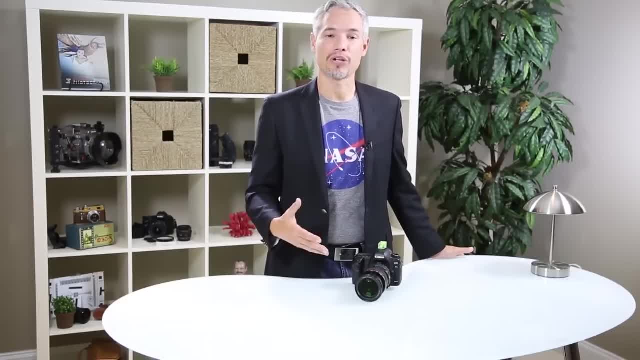 something that takes practice and kind of getting to know your camera and knowing situations where it might miss focus. So just keep at it and it'll get better with practice. Now, if you determine that your lens or camera is indeed miss focusing, then you can probably fix it with some camera settings. Now the 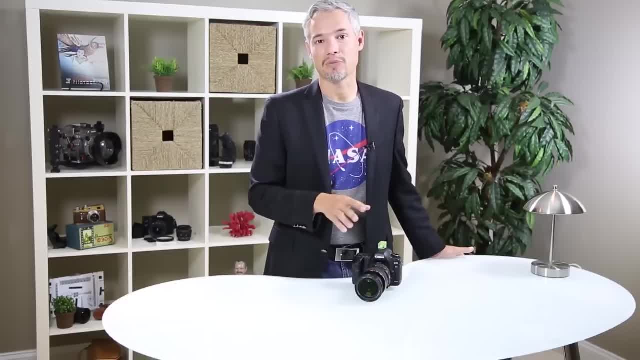 worst case is you might have to send something back for repair, but many times you can just make a few adjustments to your camera's menu system and get it working perfectly for yourself. Now, the focusing problem could be in the lens or the body. 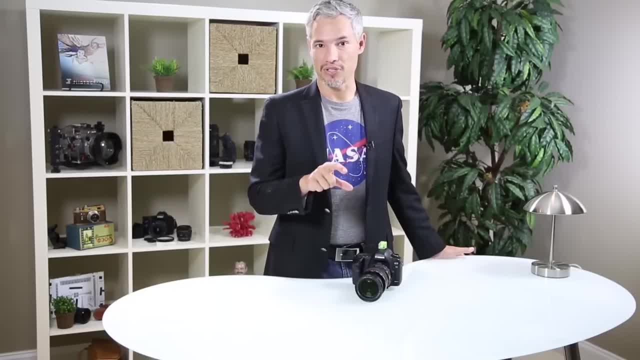 Usually it's going to be in the body because that's where the focusing sensors are held and sometimes they just get misaligned a little bit. If the focusing problem is with your lens, you can identify that by repeating the same test with different lenses, If you. 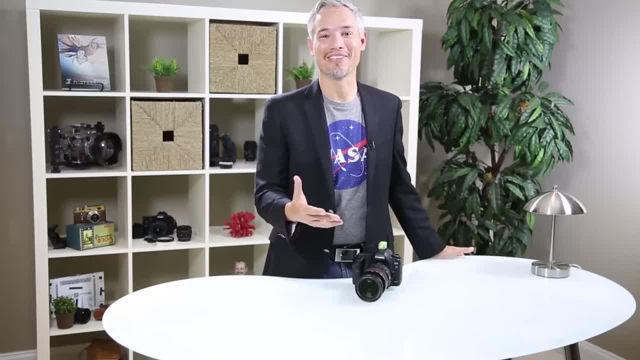 only have the one lens, well, it doesn't really matter. but if you have more than one lens, go ahead and test them all out and see how they do. And if you find that all of them are front focusing a little bit or all of them are back focusing a, 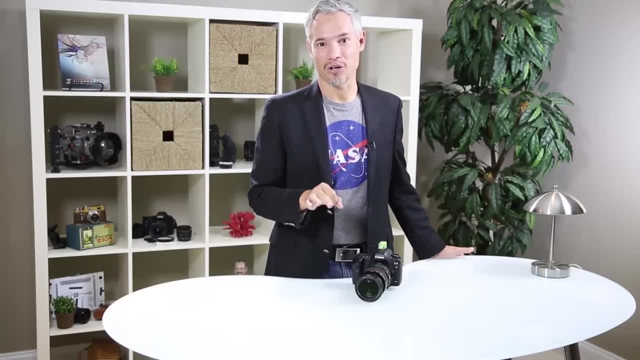 little bit. then you can be confident that it's your body that's causing problems. If it's just one lens, then you'll just make the setting to that particular lens. Now most modern cameras- at least the higher-end cameras- support 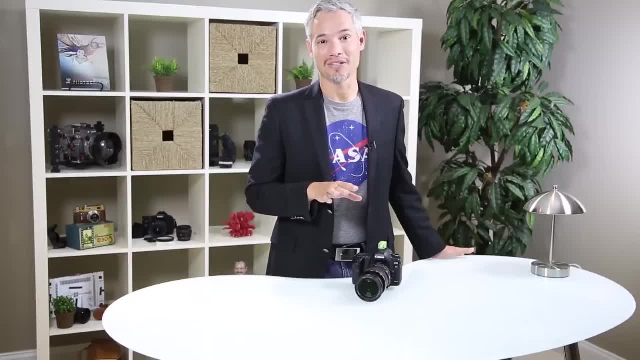 lens micro-adjustments. So what I would do is to go to Google or any browser and search for the name of your camera- like 60D or D3100, and lens micro-adjustment and see what comes up, Because there's probably somebody out there who's documented the. 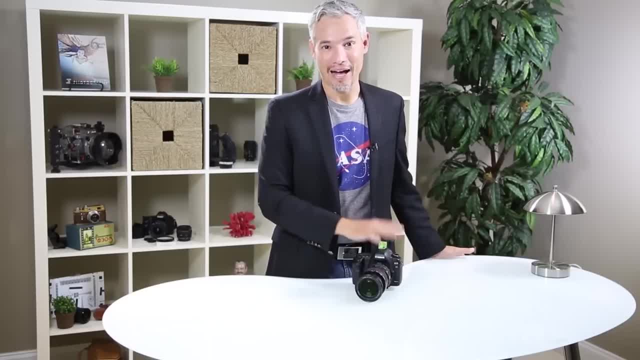 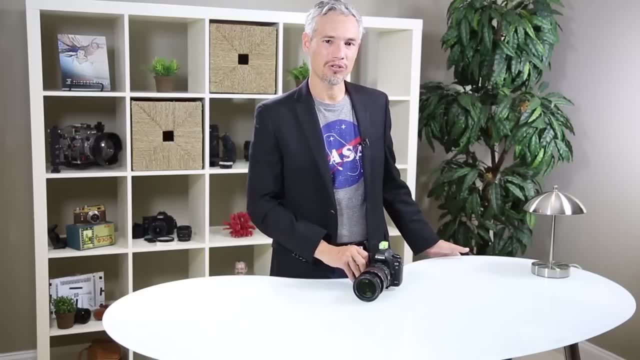 exact steps that you can follow to fix the problem. I here happen to have an old Canon 5D Mark II and it does support lens micro-adjustment, So I'll show you what I do for it. So in the menu system there are custom functions and one of them is for: 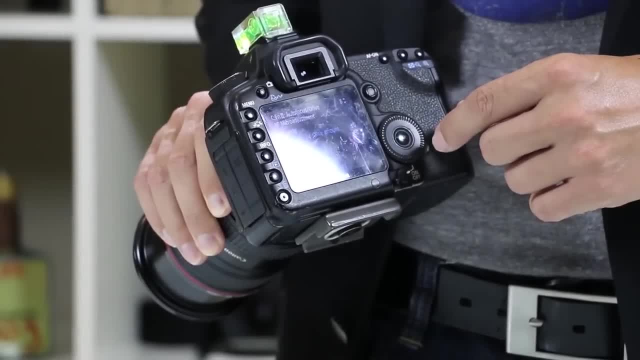 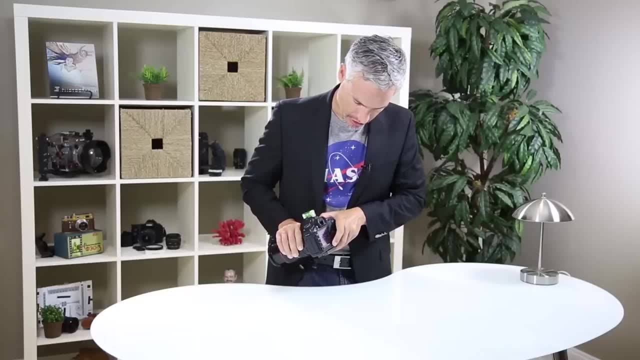 autofocus and drive, And there are lots of little tweaks in here that you generally don't need to change. but for this one- the AF micro-adjustments you'll see- I can choose from: either adjust all lenses by the same amount or adjust. 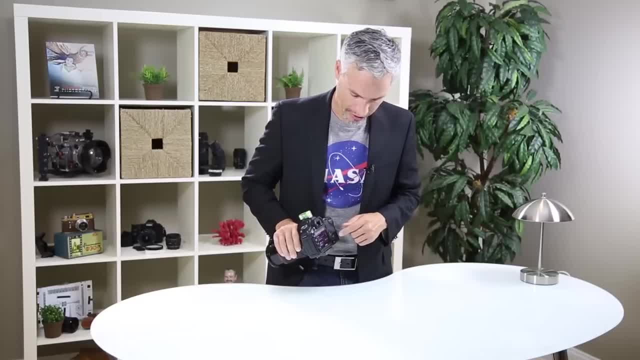 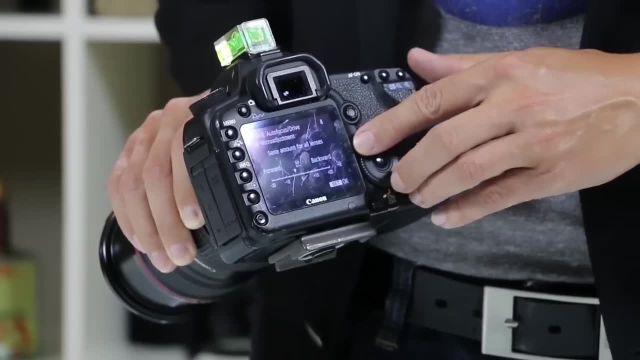 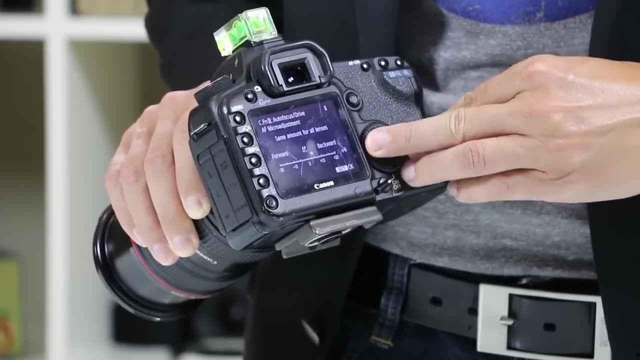 individually by the lens, So I'll choose to adjust them all by the same amount if I were to determine that it was a problem with the body, And then by pushing this button I can adjust it up or down. Now there's no particular measurement for these numbers, like positive 5 or 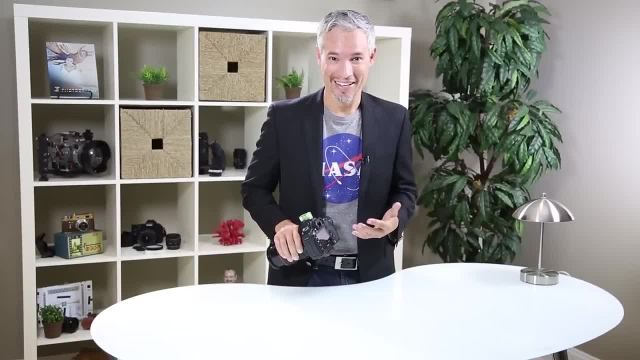 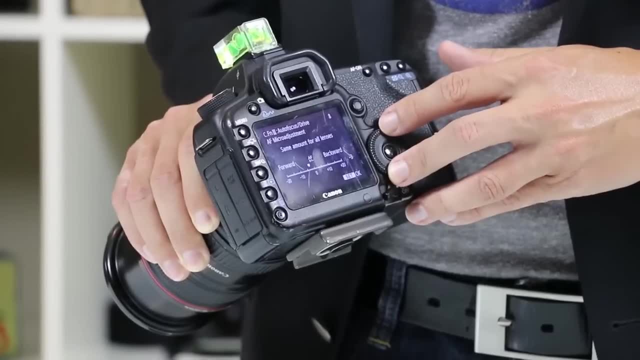 negative 5. They're not in millimeters or anything like that. You basically have to perform a series of trial and error, So you might drop it down by 2 or 3 the first time and go ahead and lock that setting in and then repeat the test and 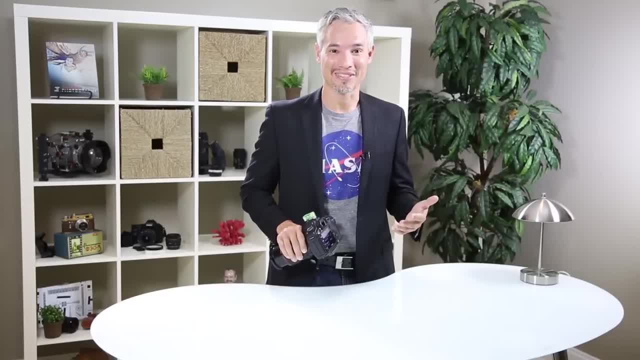 find out if it fixed the problem or if it made it worse. If it makes it better, not quite enough. you can increase the number a little bit more If you went past it. if you're now back focusing instead of front focusing, you know to. 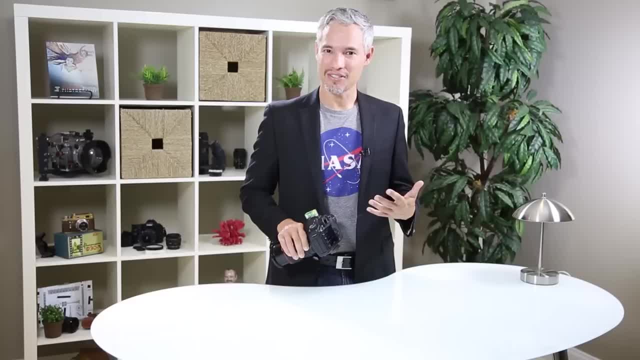 dial it down a little bit. If you find you don't get consistent results between the different tests, well, it just means your focusing system isn't precise. It's not perfect, and that's true of every camera. It's particularly true of the. 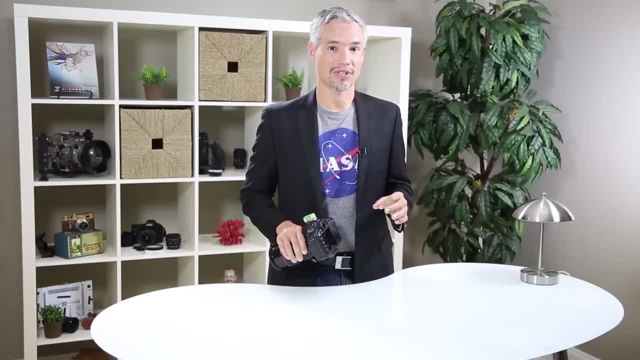 less expensive cameras. The higher-end cameras tend to have a more precise focusing system. So what you might have determined is just that your particular camera model doesn't have enough precision for the short of the sort of short depth of field that you want to work in, and it might be time to 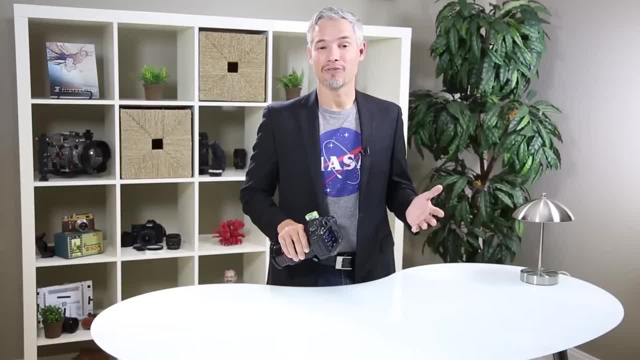 consider an upgrade, But I honestly I rarely see these focusing problems as being very serious. So again, make an adjustment to the micro adjustments. Repeat the test If it doesn't get better. set it back to zero If it does get. 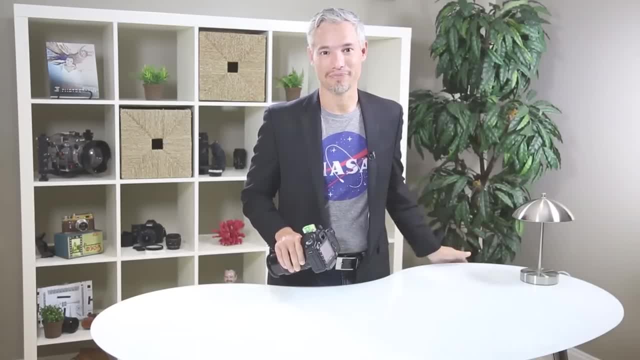 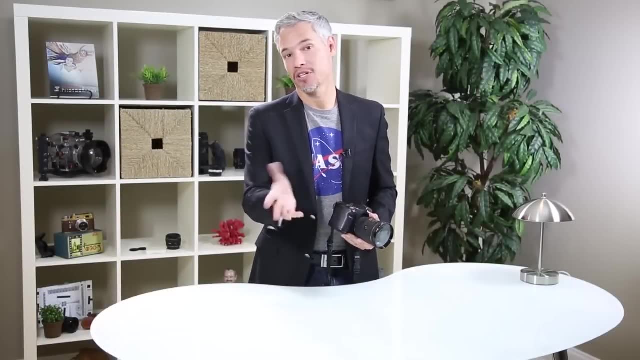 better, then. congrats, You're done and you've solved your focusing problem. Here's a problem that one of our friends had over at the private sdpcommunitycom forums, which you're very entitled to do, and I'm sure you've all seen it. It's a 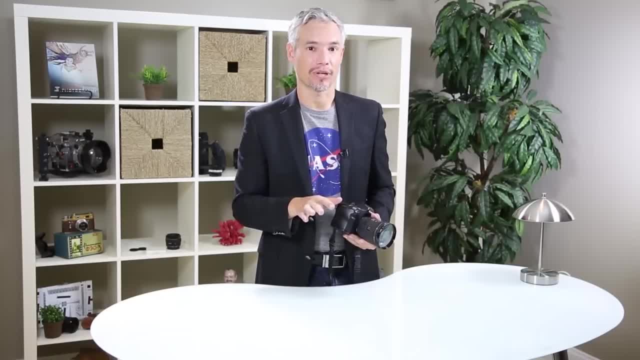 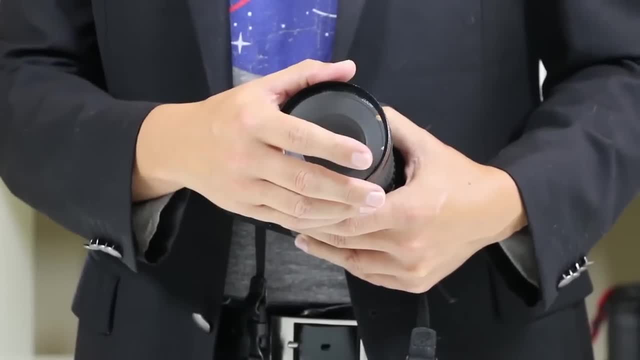 great place to get more troubleshooting help if I haven't answered your question here, But he had a filter stuck on the front of his lens and this can happen for a couple of reasons. You might misthread it as you're trying to put the filter on. 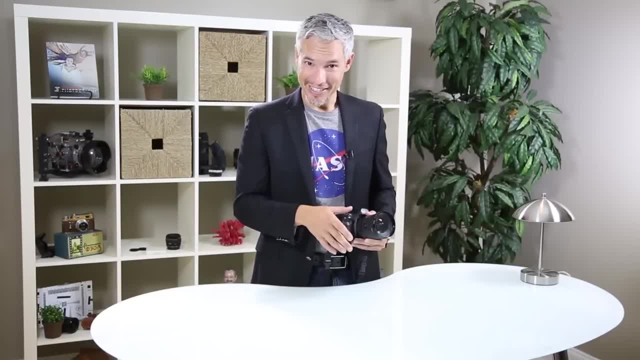 and then it just gets stuck. Or you might just over tighten it and then it won't come loose. Or maybe you leave it on there for a long time and a little bit of rust builds up. It can be really difficult to get off, and if you twist it too hard, 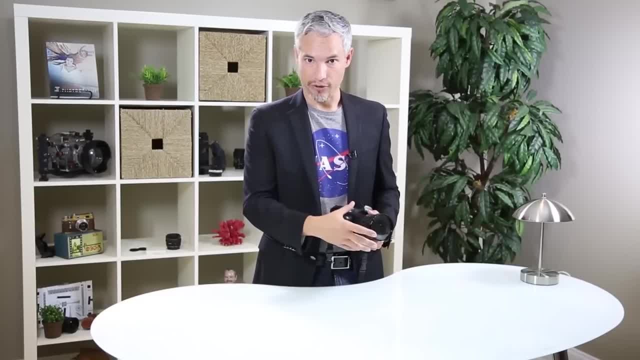 with your hands, you might cut your fingers, You might break the front of your lens or crack your filter, And these filters can be pretty expensive, so you want to be careful with them. I'll show you how I've gotten a few filters unstuck. The first thing to do is to take 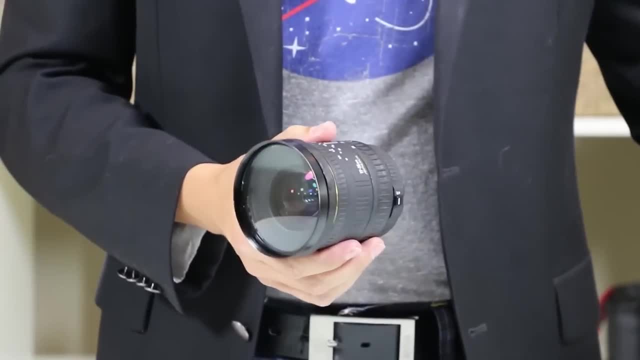 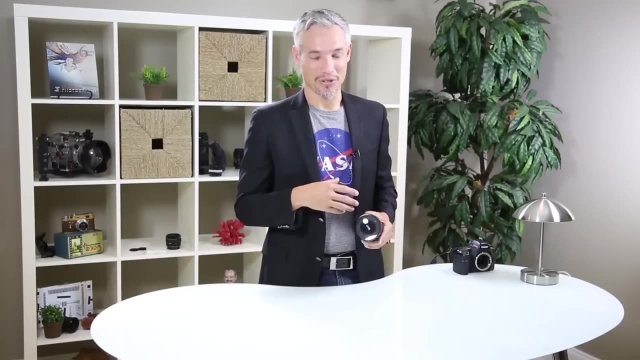 that lens off of the body and by doing that you're going to reduce the risk that when you actually put enough torque on that thing to come off that you're going to twist the body mount too. So it's better just to grab the lens by the outside, but not where the 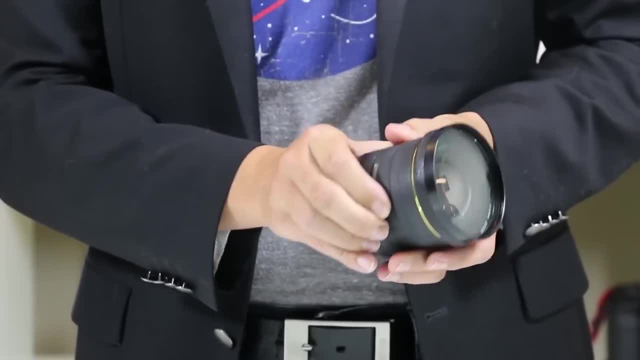 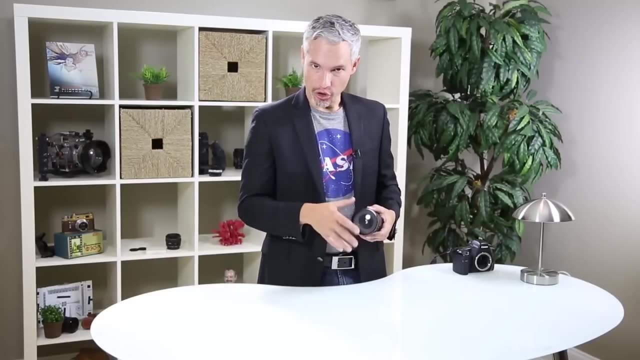 rings are You want to be sure to grab it where it's nice and stable. If you happen to have a rubber jar opener, those work awesome. Those are absolutely the best. One of those things that you can just grip it and turn it really good. Don't use the kind with the teeth, though, because that'll cut right into. 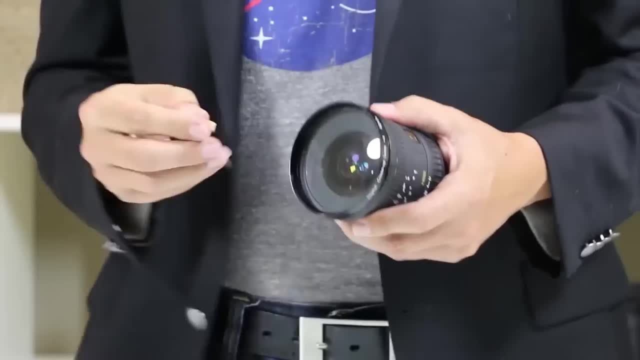 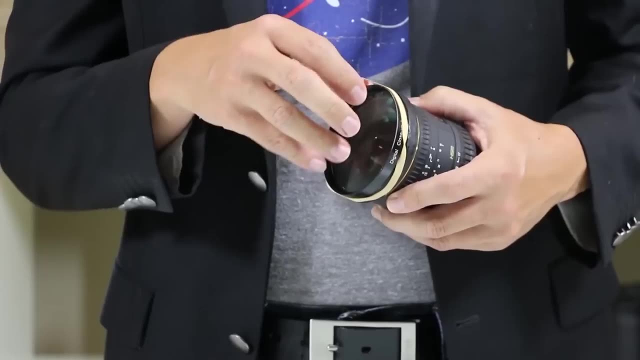 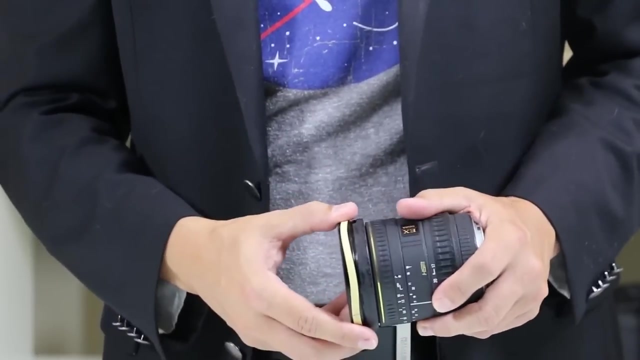 the metal. Otherwise you can just grab yourself a rubber band and stick that rubber band right around the filter like that, And the rubber band is just going to give you a little better grip than the metal would. So now, with that rubber band on there, I can apply a little more torque to it. I get a. 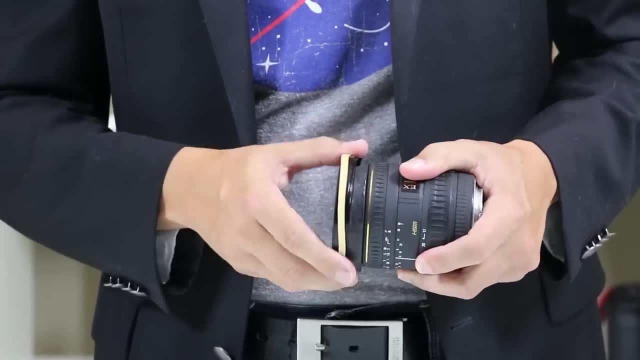 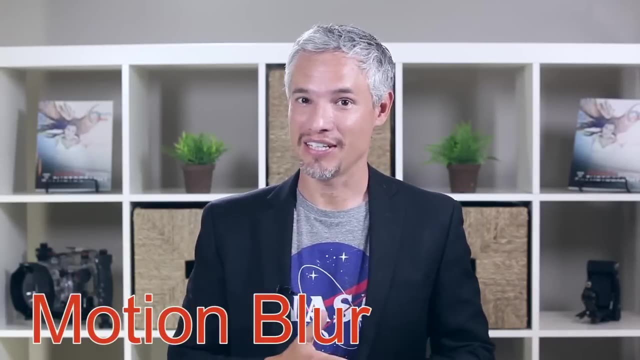 bit of grip and now I can get it to come off without breaking anything. Now let's talk about motion blur. I know it seems like when you take a picture that it freezes an instance in time, but your shutter is actually open for whatever period of time. 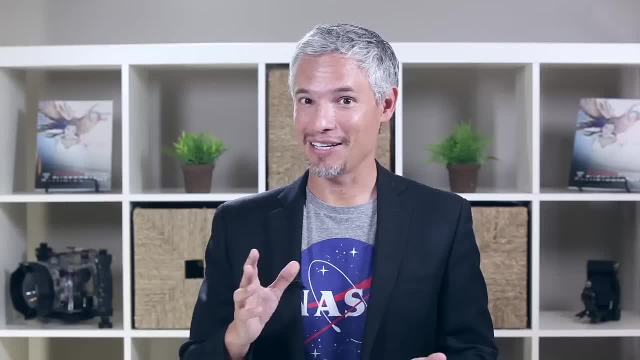 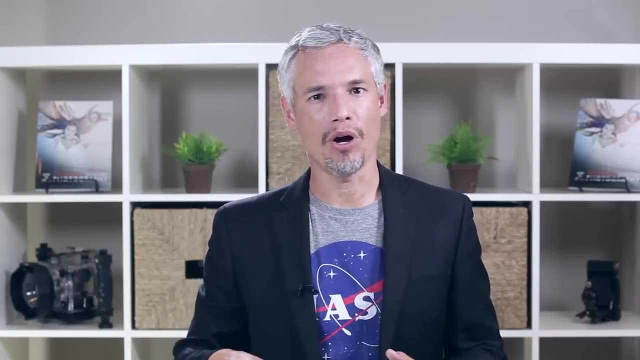 the shutter speed is And 1, 60th of a second seems like the blink of an eye. Maybe it actually is, but that's plenty of time for a moving subject. a person throwing a ball or a bird's wings flapping- It's plenty of time for that to move in the course of 1, 60th of a second. 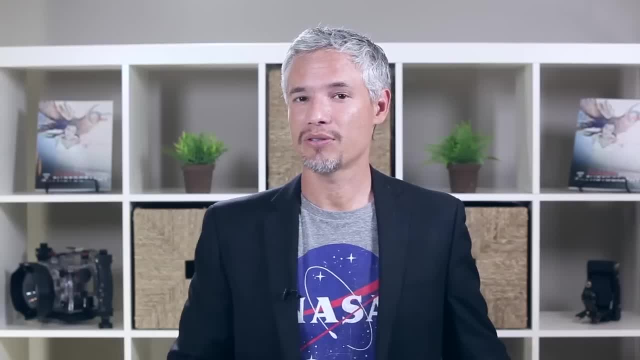 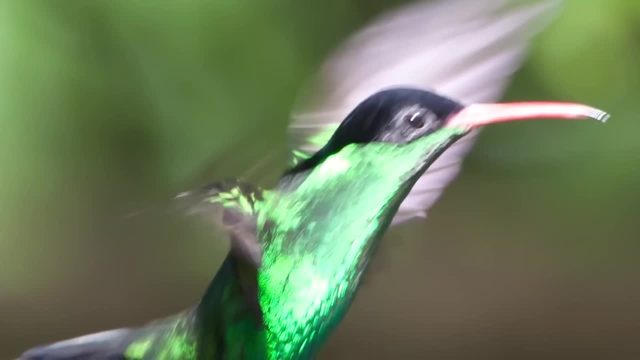 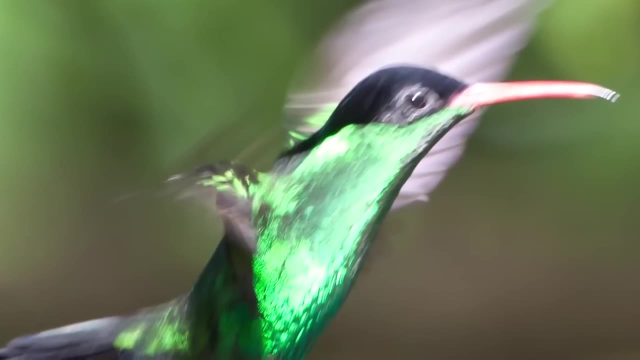 and that will always result in a blurred image. So let's look at some examples of motion blur. Here we see a hummingbird, a Dr Bird in Jamaica, and its wings are just completely blurred And in fact, its eyes blurred too. Look, hummingbirds are really fast and if you're going to freeze, 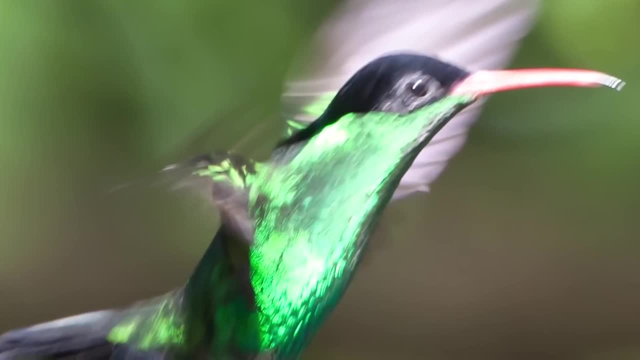 them properly. you need a shutter speed of like 1 2000th or 1 4000th And I had this at 1 500th of a second, so that wasn't nearly enough to freeze the action, To solve it. 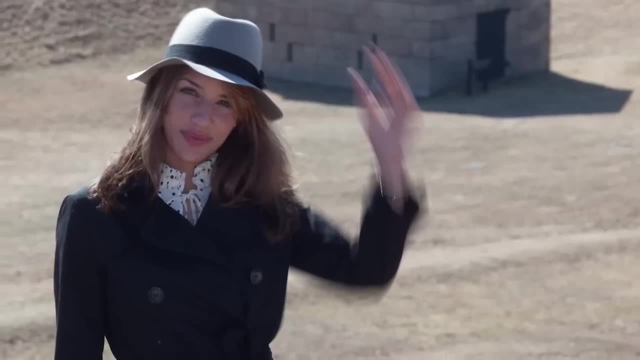 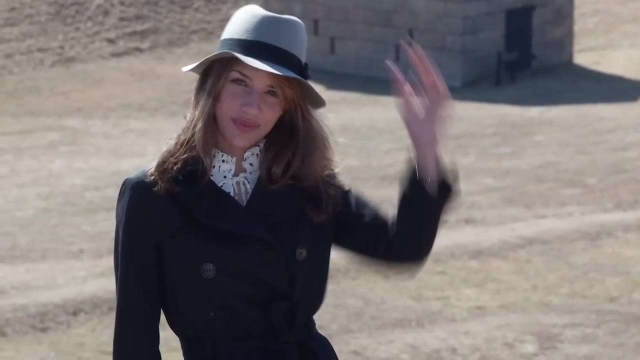 I simply need to use a higher shutter speed. Here's a picture of Chelsea. As you can see, her hand is completely blurry, but because her face is sharp and the background is sharp, I can tell that this is a case of just motion blur, And you know the reason. 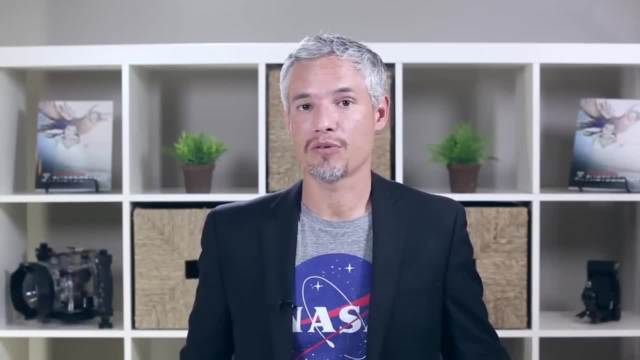 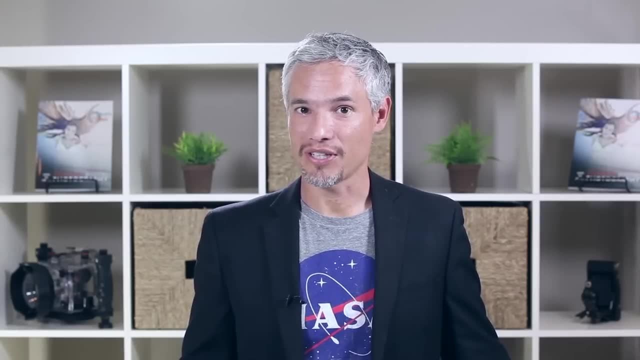 we're spending some time diagnosing the specific cause of the problem is so you also know how to fix it. If this were just out of focus, well, I would solve it by using one of my focusing techniques. But because her face is sharp, but her hand is blurry, that tells. 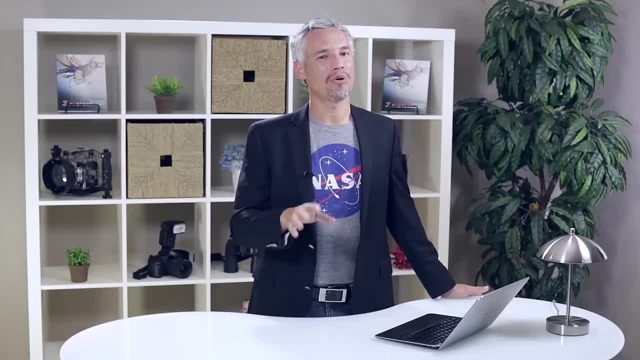 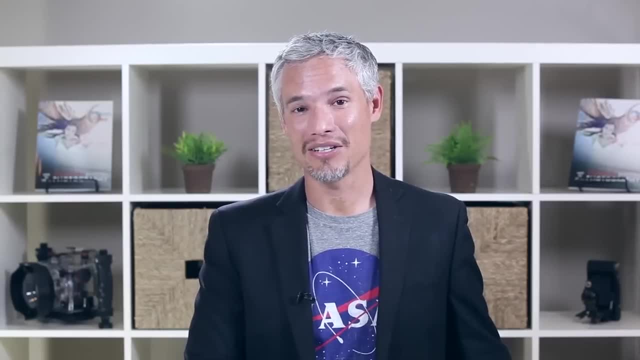 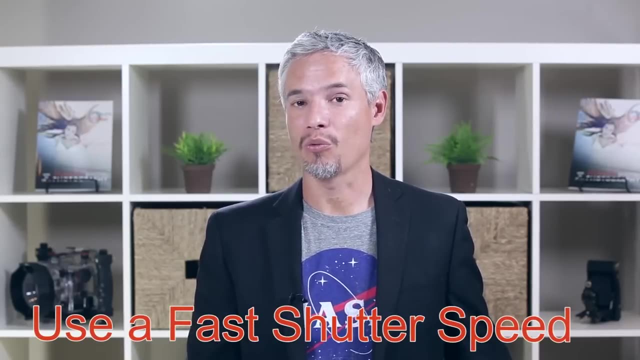 me it's a motion blur problem. To solve motion blur problems by adjusting your lens, you do it by adjusting your shutter speed. So in this case, if I wanted to capture her hand sharp, I'd put my camera into shutter priority mode and select a faster shutter speed, maybe 1 500th or 1 1000th of a second. 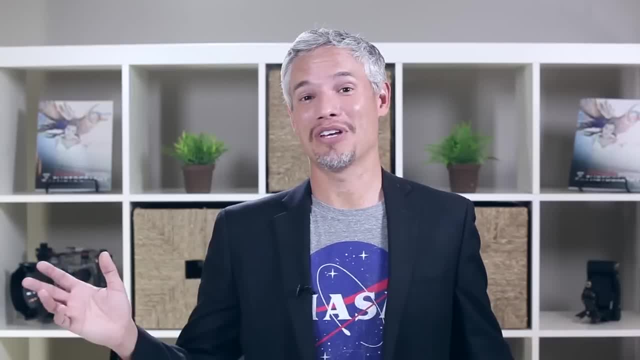 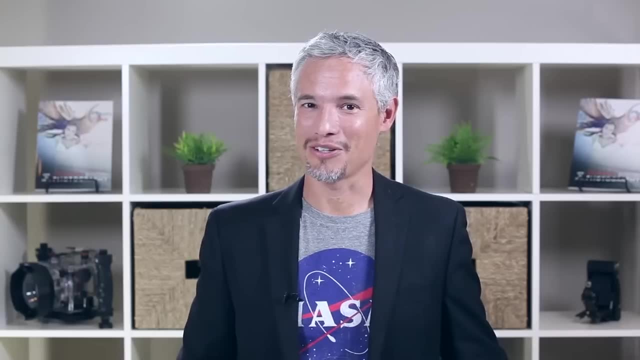 It can be easier said than done, though, right, You can't always just use a super high shutter speed, because your camera just wouldn't be getting enough light to the sensor and you'd have a bunch of other negative side effects. So generally you use the slowest shutter speed. 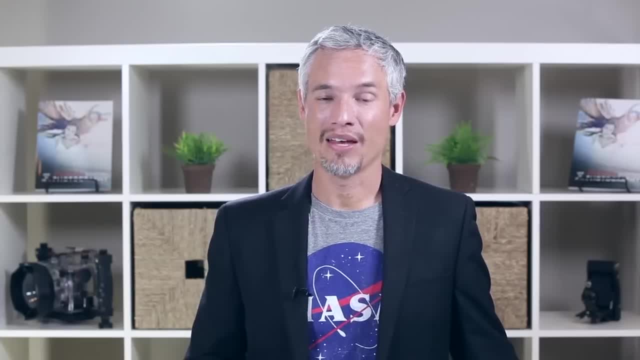 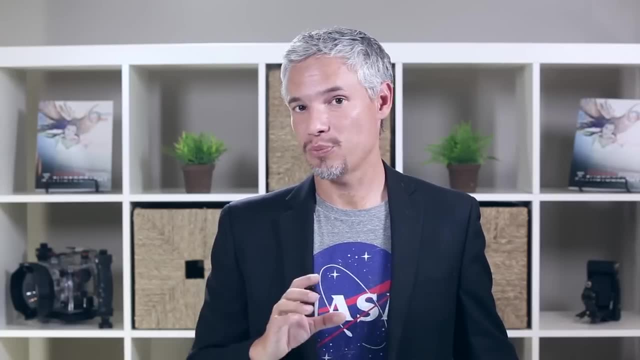 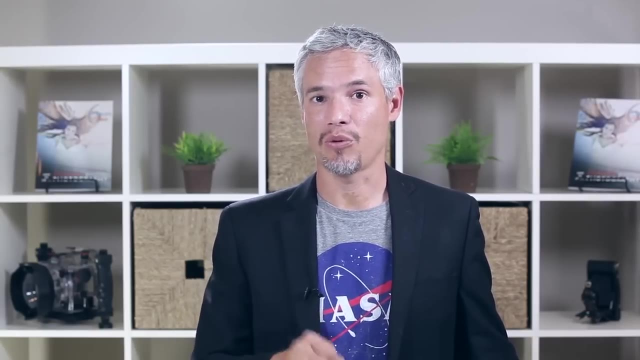 That will allow you to freeze the action in the frame. The way you do that is by using shutter priority mode and perhaps auto ISO. Then your camera will shoot with the largest possible aperture, the smallest f-stop number, and it will adjust the ISO as needed to get the shutter speed that you require. 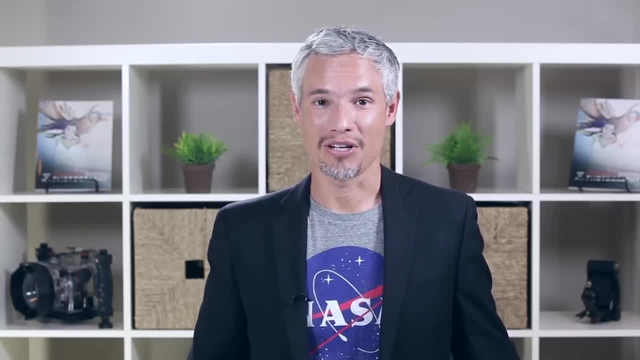 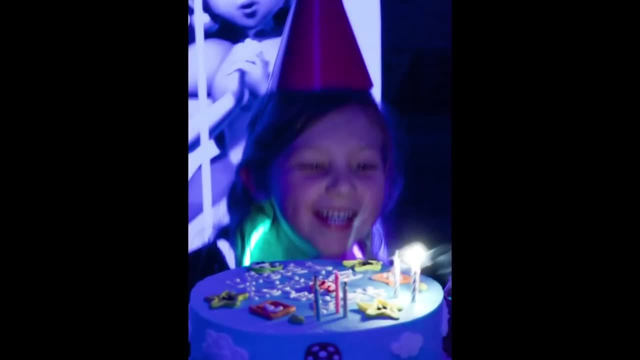 For more information, check out that controlling your camera video. Let's look at another picture. This is my daughter, Madeline, on her fifth birthday and she's blowing out some candles and it was really dark in the room And you can see her face is completely blurred. 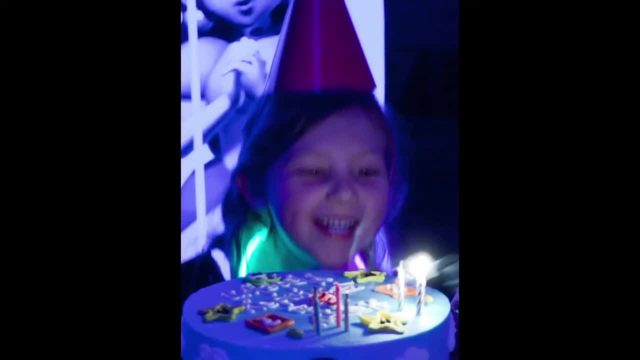 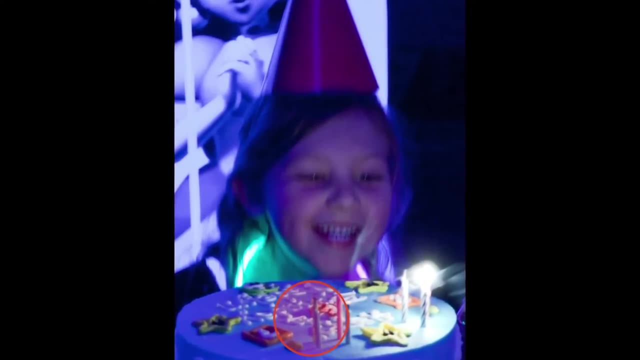 Now, how do I know that this is motion blur and not camera shake or a focus problem? Well, I can see by looking at the cake that the cake is nice and sharp and that means that it's not camera shake. However, her face is moving and everything else in the picture is sharp. 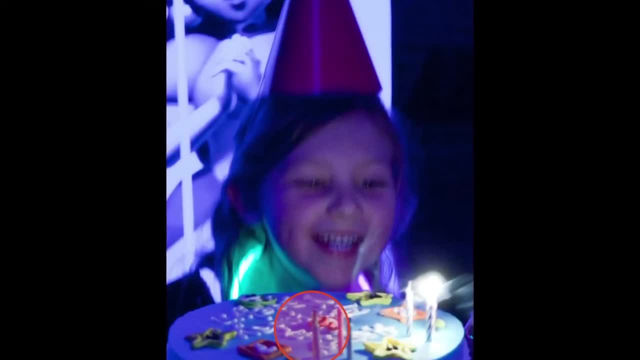 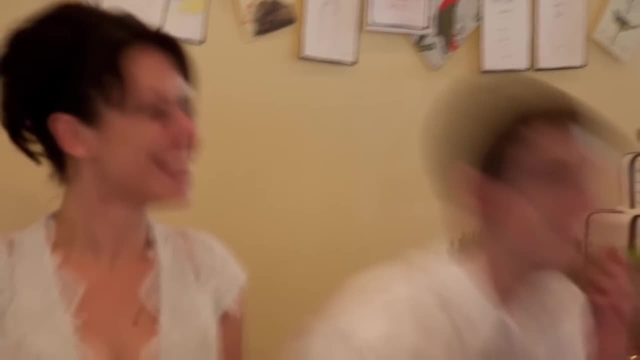 That tells me that she was moving during the course of the picture, and the way I would solve this particular problem is by using a faster shutter speed. Here's another picture taken at a wedding, And if you look At the background you can see that the cake and the cards on the wall are mostly sharp. 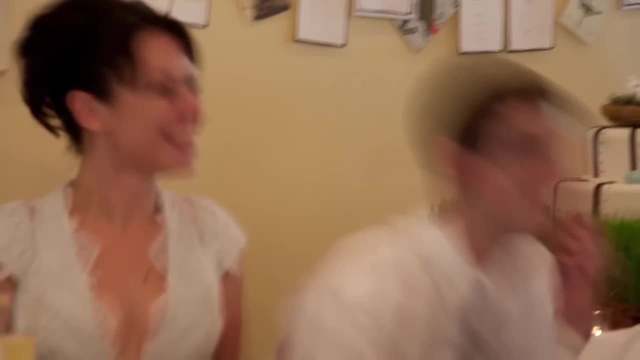 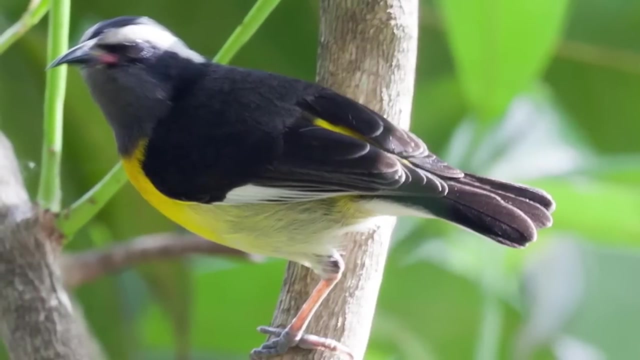 Again, that's what tells me that it's not camera shake, It's not a focus problem, but you can see the motion in the people themselves that indicates motion blur. This picture: once again we see that the tree branch is completely still and sharp. 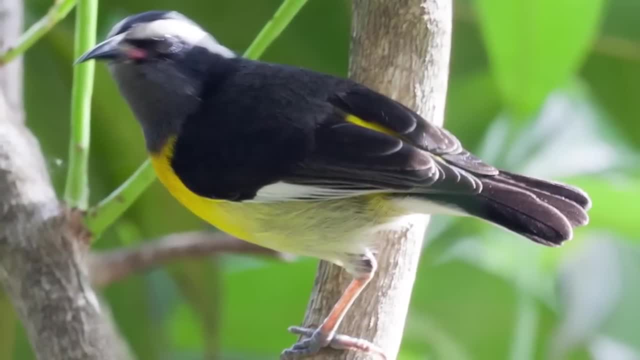 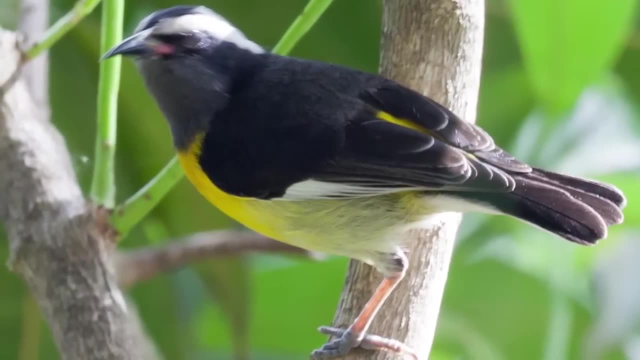 but the bird's head is nice and blurry. You can even see that the bird's body is sharp. The bird was just moving its head. So the way I would solve that is by again increasing the shutter speed or using the technique of just taking lots of pictures and deleting most of them. 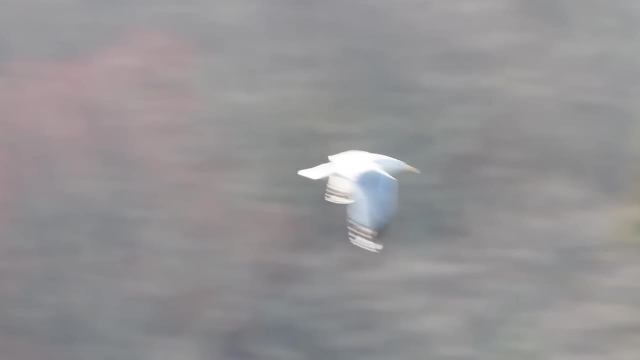 This is a picture of a flying bird, And if you want to freeze the wings of a flying bird, you really need to be shooting at about one two thousandth of a second. This one was shot at one two fiftieth of a second. 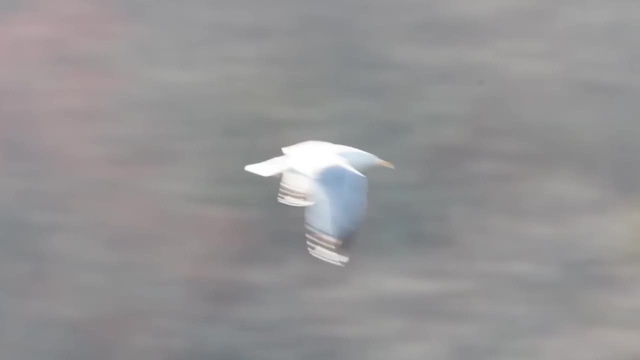 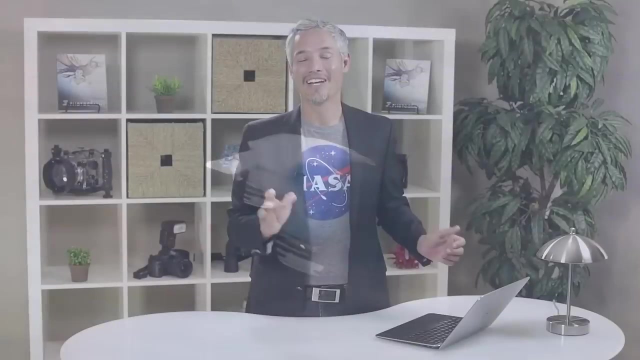 You can see that was not nearly fast enough. The background is panned, My shutter speed was so slow and the wings are completely blurred, So in this case I would have no choice but to raise the shutter speed. Another common cause of blurry pictures is camera shake, and with camera shake, your subject. 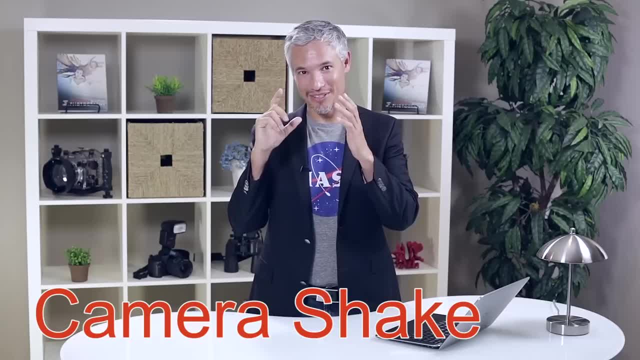 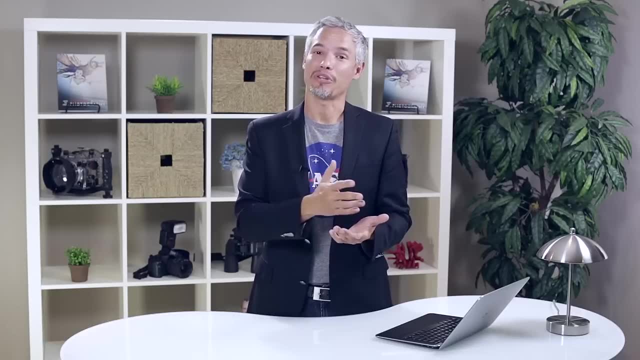 might be completely still, But your hands aren't completely still. It happens when you're using a shutter speed that is slower than what they call the reciprocal rule. So if you're shooting with a hundred millimeter lens, if you're following the reciprocal rule, 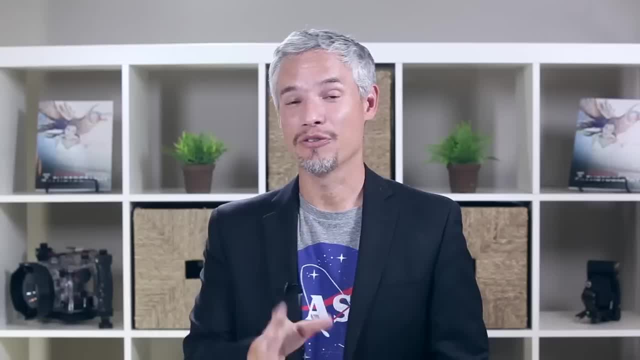 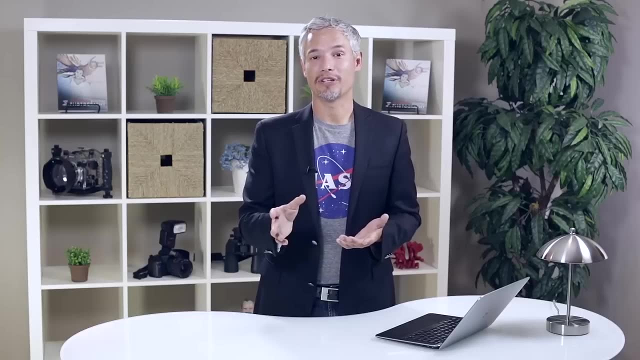 you'll shoot with a shutter speed of one one hundredth or faster. If you're shooting with a 50 millimeter lens, you'll shoot with a shutter speed of one fiftieth of a second or faster. Of course, as I described in the controlling your camera video, other factors like a tripod. 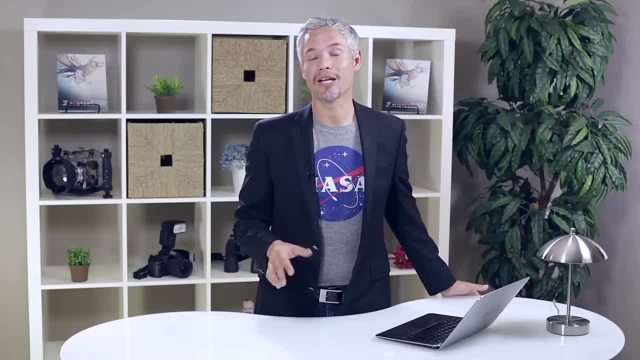 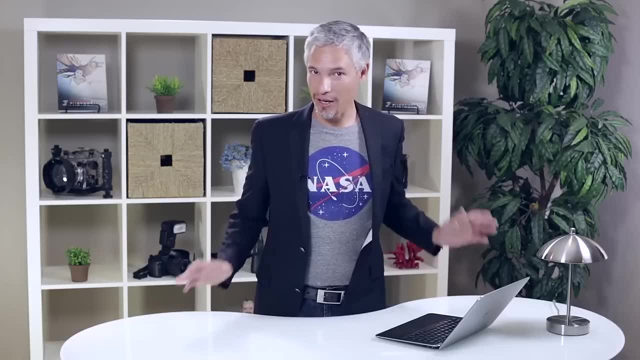 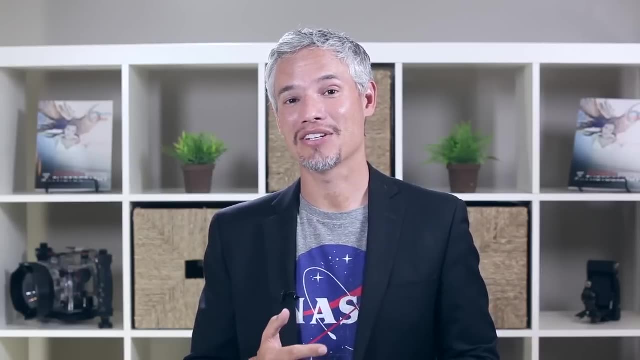 or image stabilization can allow you to use slower shutter speeds. If you diagnose your problem as being camera shake, you either need to use a faster shutter speed to cancel out your shaking hands or you need to add some sort of support to your camera, either by enabling image stabilization in the camera body or lens, depending on the 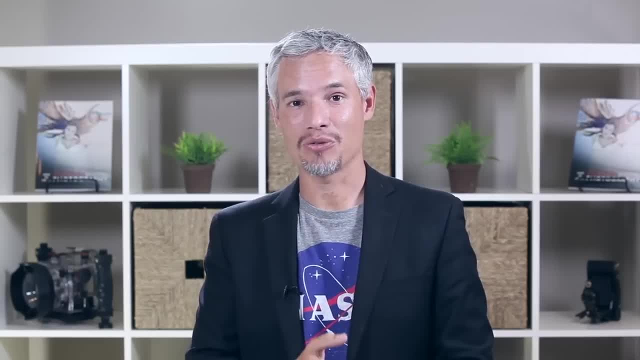 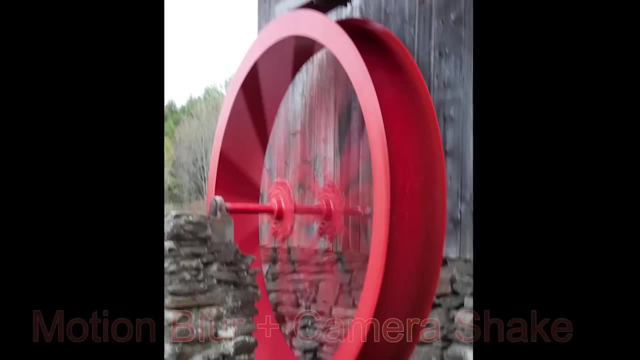 model that you have, or by attaching your camera to a tripod. So let's look at some examples of camera shakes so that you'll know exactly how to diagnose that problem. Now, this picture actually has both motion blur and camera shake. I'm going to zoom in a little bit to see if I can get a better picture. 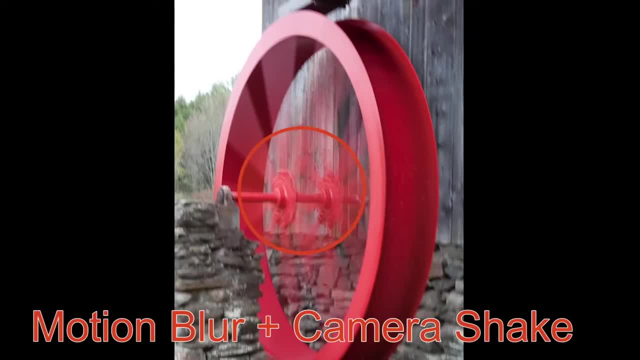 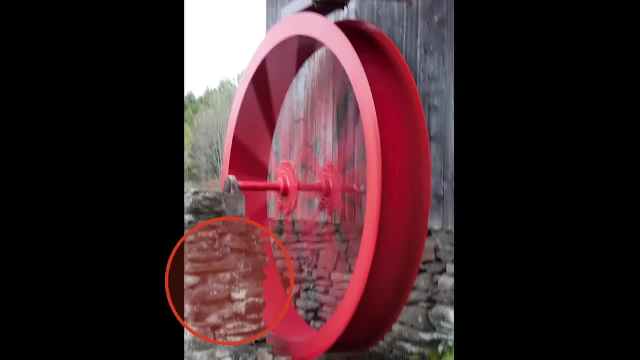 I wanted the motion blur, which is why I was using such a slow shutter speed. I wanted to show the motion of that wheel, But if you look closely at the stones and the wooden wall behind it, you'll see that they're completely blurry. 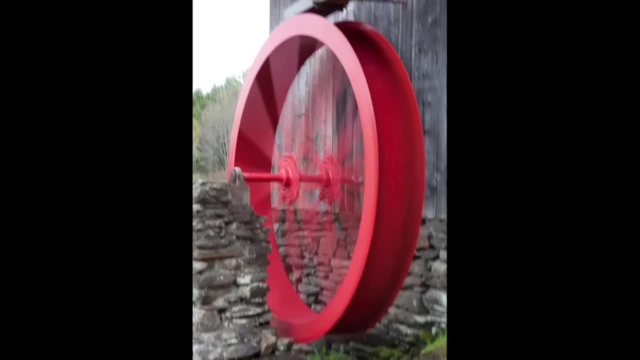 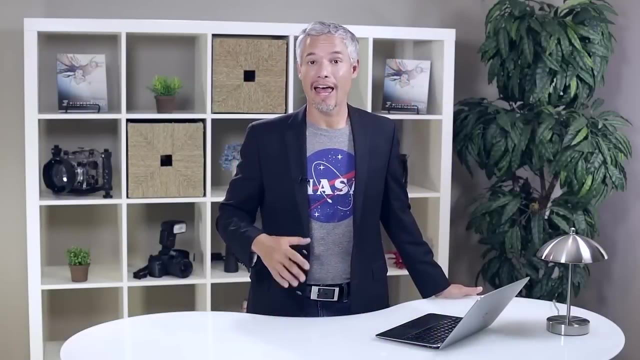 It feels a little bit different than simply being out of focus. You can see that it's sharp, but it's almost like there's a ghost copy of everything. So the way you're going to recognize camera shake is that everything in the photo is going. 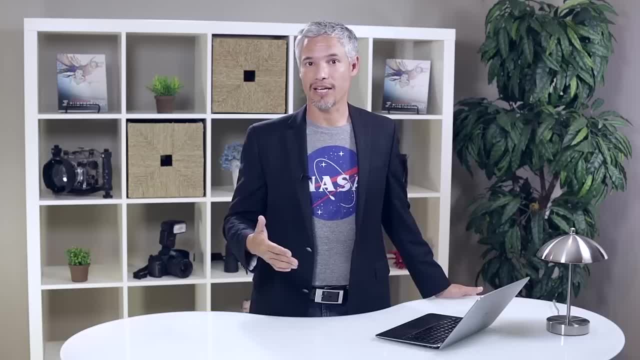 to be a little bit blurry. If you're miss focusing on something, you'll see that the wrong part of the picture is sharp. If there's camera shake, the entire scene is going to be blurry. If it's motion blur, only the moving subject will be blurry and everything else will be. 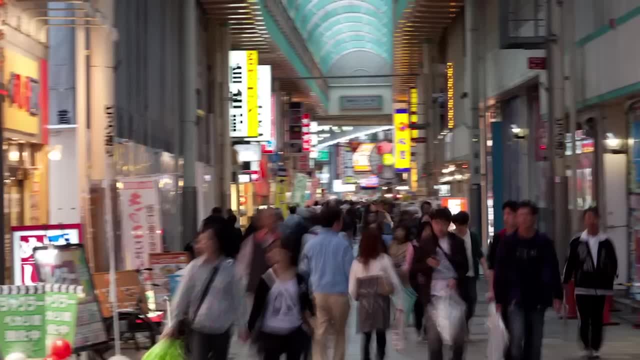 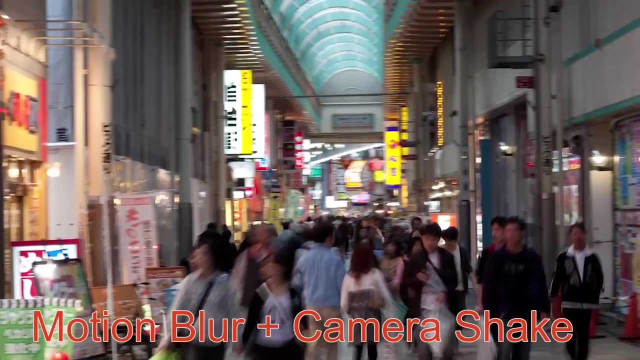 sharp. Let's look at another example of camera shake. Now. in this scene we can see that there are moving people in the scene and they are blurry And that's because of motion blur. The way we're going to identify whether there's camera shake or not is to look at these still. 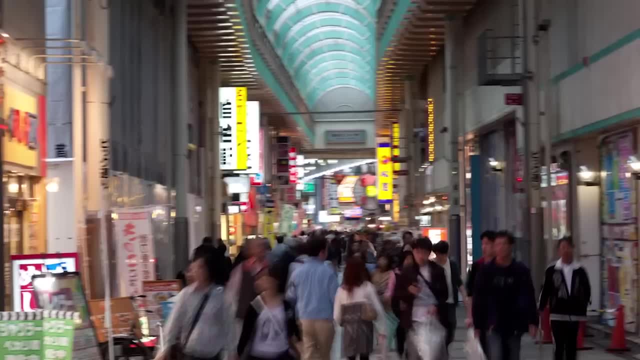 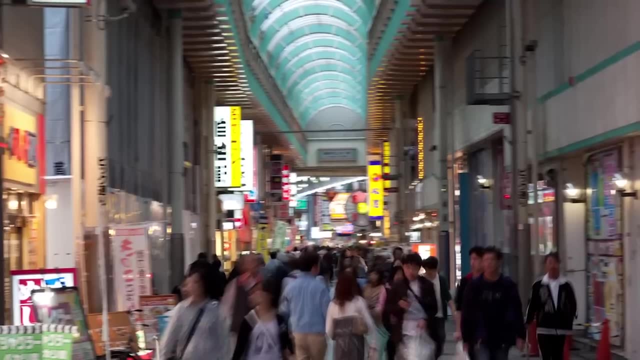 subjects in the photo. So we'll look at the background, the walls to the left and the right and specifically the areas of contrast, the lettering on them, And if we look at that we can see that they're not sharp at all. 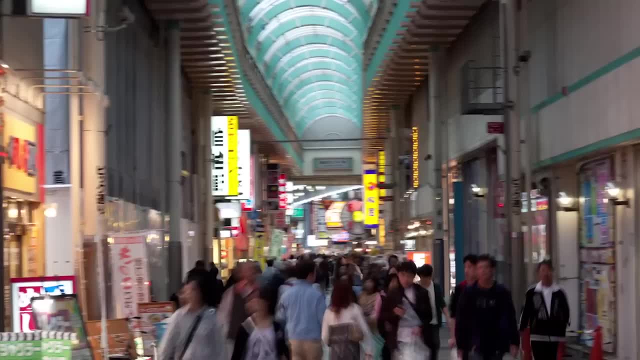 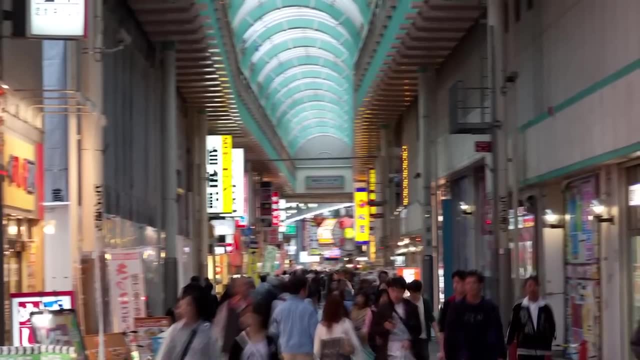 And indeed we kind of see that ghosting that occurs with camera shake. So I was going for a low shutter speed because I wanted to show motion, but I also got camera shake. I should have just attached my camera to a tripod. Now let's look at that same scene without the camera shake. 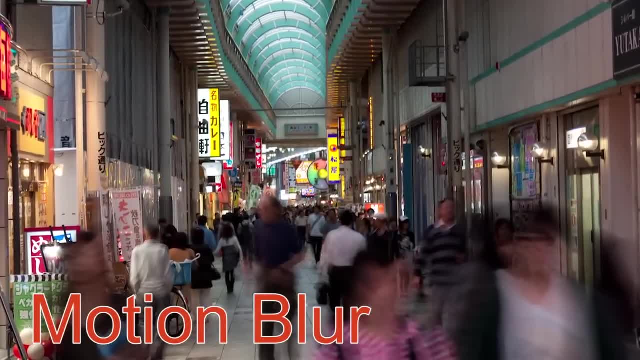 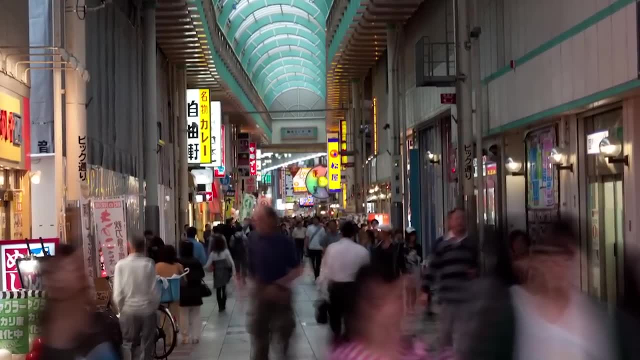 As we switch to this picture, we can see motion in the people, but the background is nice and sharp. So this is motion blur without camera shake. and the other picture was motion blur with camera shake. If you have your camera on a tripod, it's still possible to get camera shake. 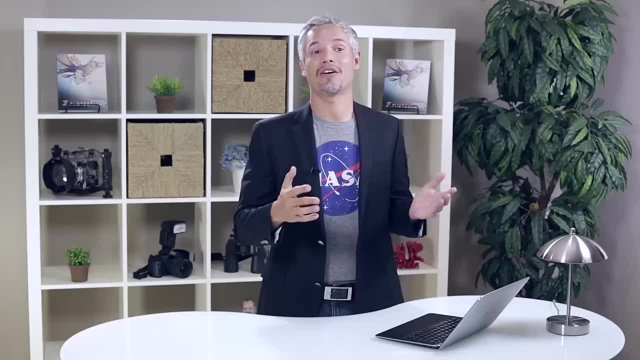 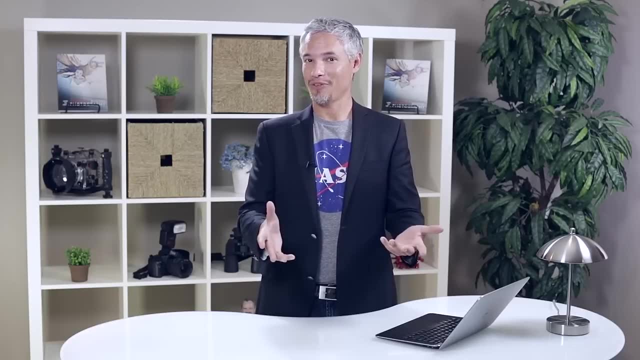 And this comes up a lot with night photography- When you're taking pictures that are one second, five seconds, 30 seconds long, you can still get camera shake because your tripod isn't perfect. It's not a rock right. Some wind can come along and shake it from side to side. 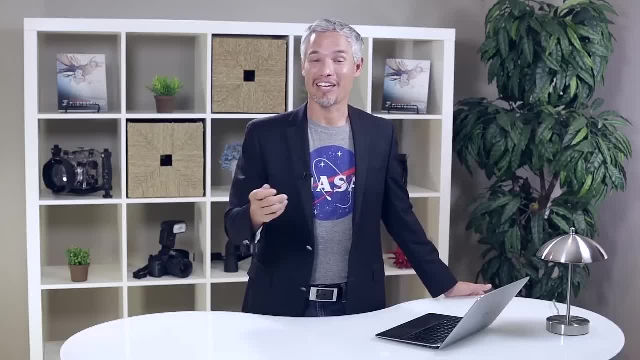 You might bump it with your arm, You might trip over the cable, release something like that, and it will shake the camera, and you'll see the camera shake in there. So the way you solve that, of course, is by looking at the camera. 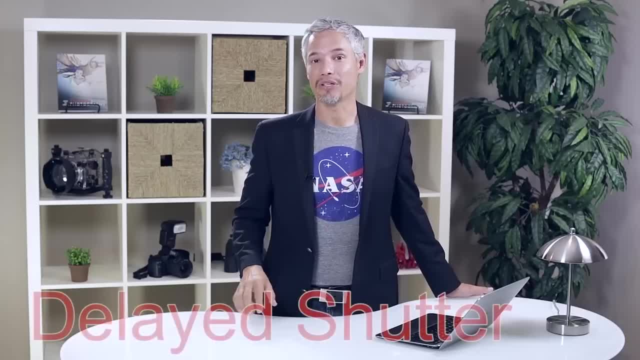 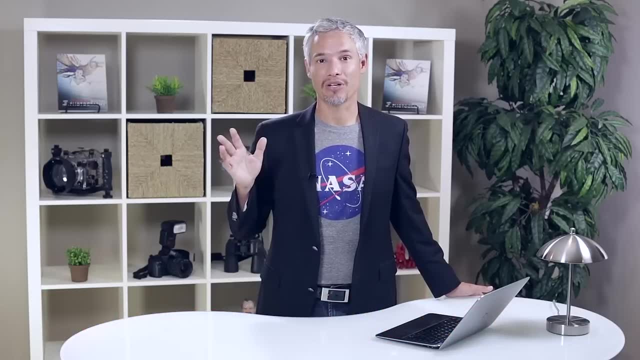 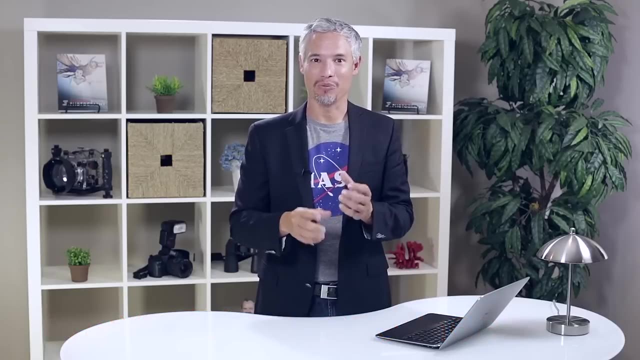 It is by staying farther away from your camera. You might also set up a delayed shutter, so that after you press the shutter button, the camera has a chance to stop shaking before it actually opens the shutter. You also get yourself a nice big, heavy tripod and a heavy head and you lock them down really. 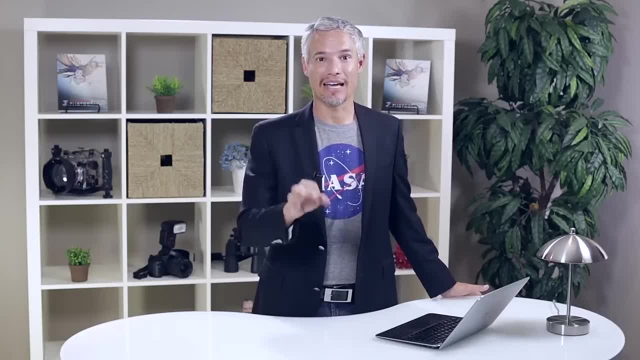 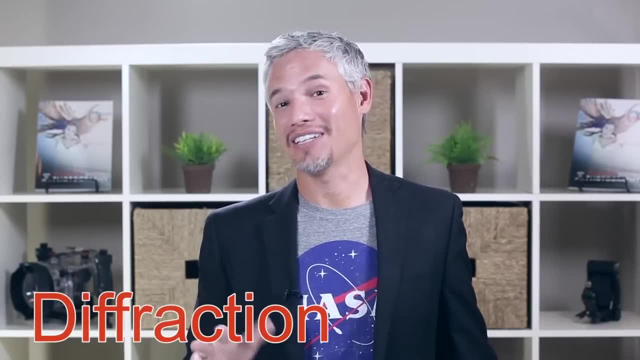 tight. So for more information on tripods, check out the night photography video. A less common cause of blurry pictures is diffraction. To understand diffraction, you'd have to understand like the quantum mechanics Photons use as they travel through the lens. 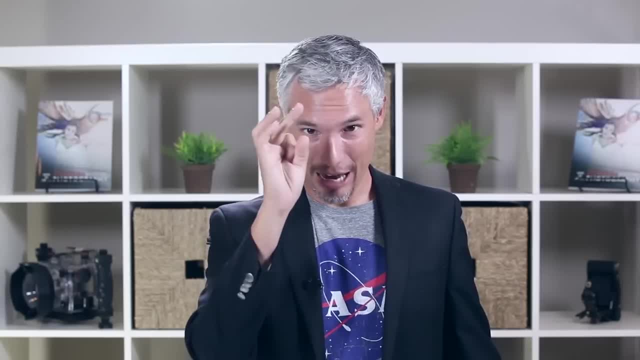 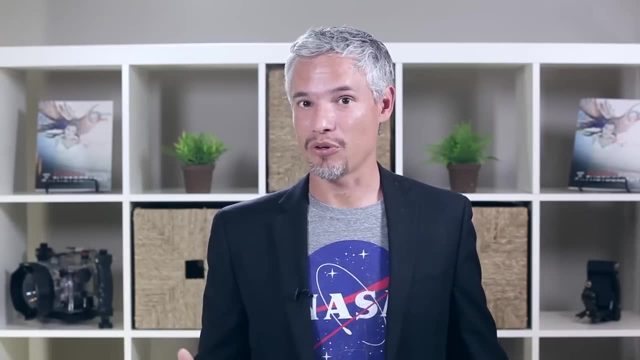 But basically what happens is when you use really small apertures, that's apertures with a very high f-stop number, especially at high magnifications, the picture is never going to be sharp. That small aperture actually changes the path of the photons a little bit. 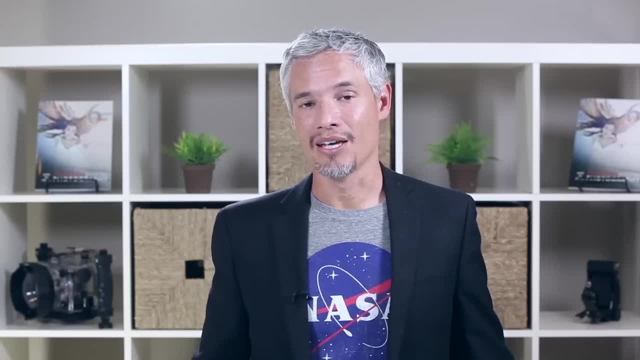 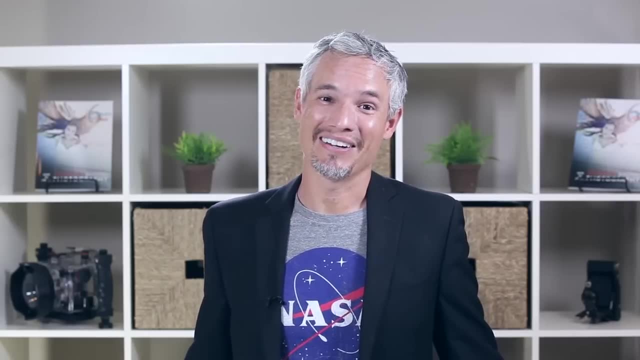 And it means that your pictures are never going to be sharp at near magnifications. This really gets to be a problem with macro photography, so you probably can't blame your blurry pictures of your kid on diffraction. It's not a problem, It's a distraction. 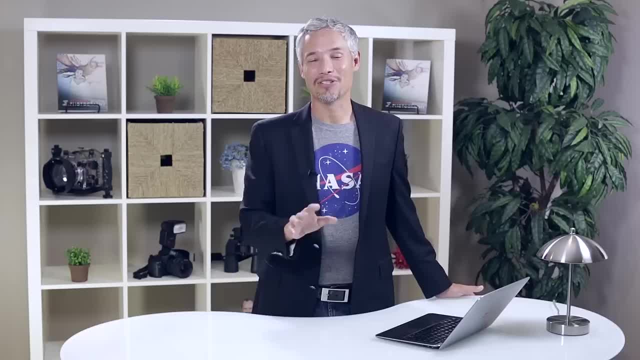 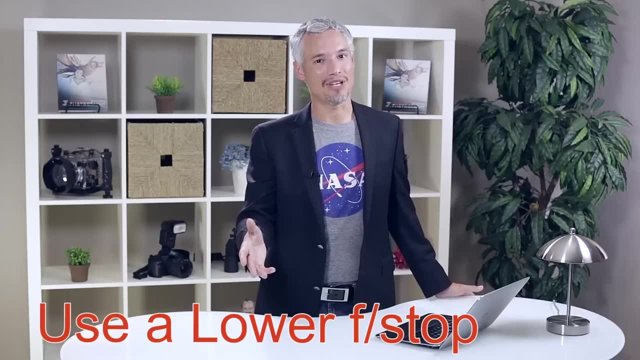 But when you get into macro photography, it's something to look out for. So the way that you solve diffraction problems with macro photography is to use a lower f-stop number, For example, instead of using f22 to get lots of depth of field, you might end up using 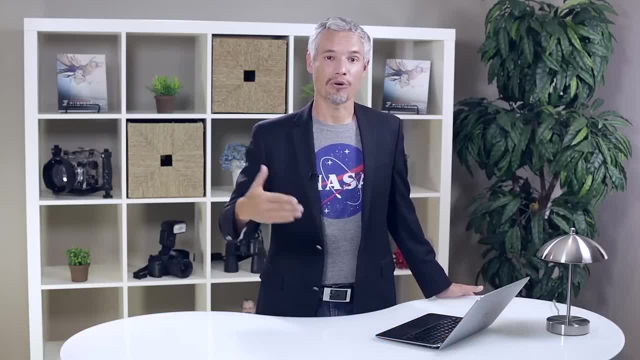 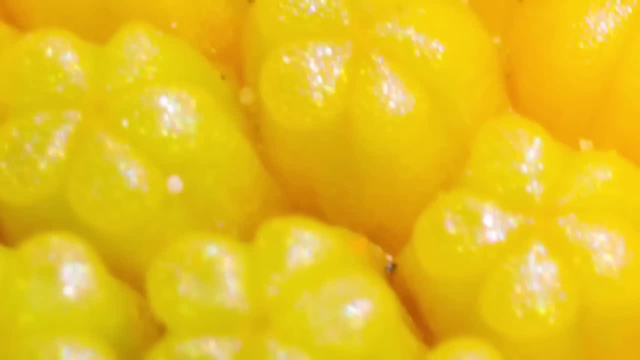 f4 or f5.6 and then using focus stacking to get the depth of field that you need. For more information, check out the macro photography video To demonstrate that. here is a very close-up picture of a flower. This is taken at 5x magnification. 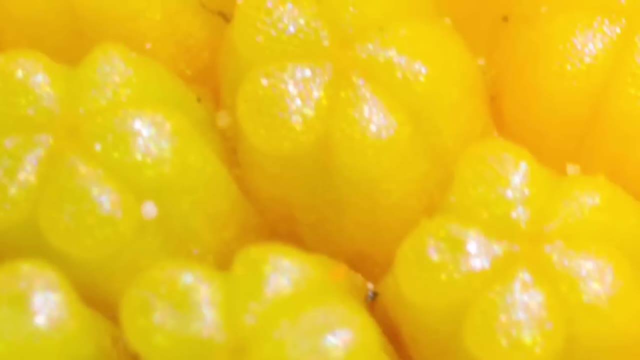 It's like near microscopic levels of magnification And it's taken at f16. And you can see it's just not sharp. Now, the technique here was perfect and the focus was perfect, But at this level the picture is just never going to be sharp because of diffraction. 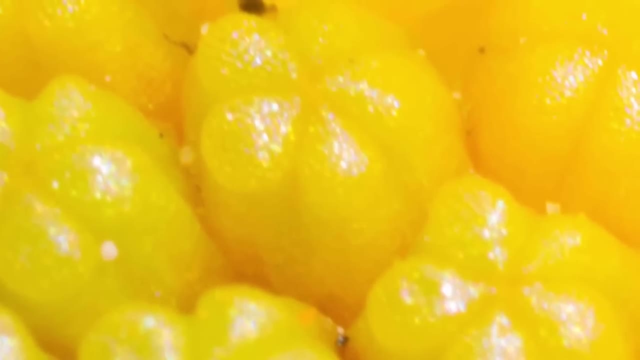 If I were to use a lower f-stop number, such as f2.8, what we'd see is perfectly crystal clear sharpness, because the larger aperture associated with the smaller f-stop number will allow the picture to be much sharper by eliminating diffraction. 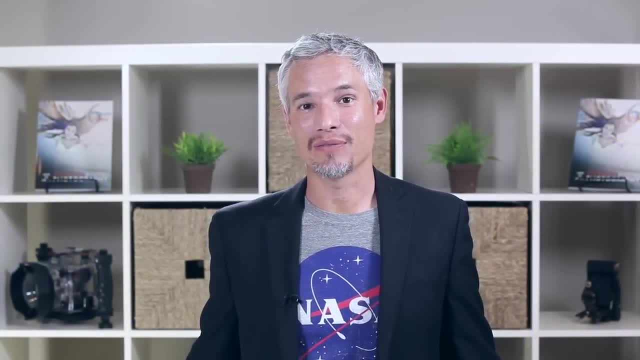 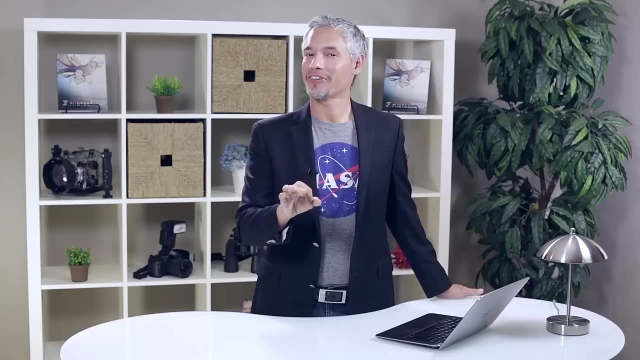 Another common question I get asked is: how do you know if a flower is sharp? Another common cause of blurry pictures is simply using a low-quality lens or filter on your camera, If your pictures are just very slightly blurry and you've determined that they're in focus. 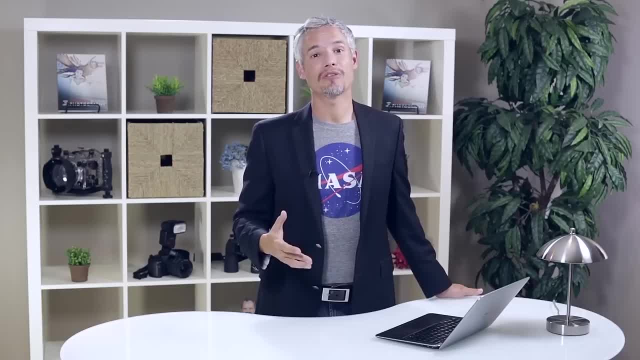 and there's no camera shake and there's no motion blur. it could be the fault of either your lens or a filter that's attached to the front of your lens. The kit lenses that come with cameras tend not to be of the most perfect quality. 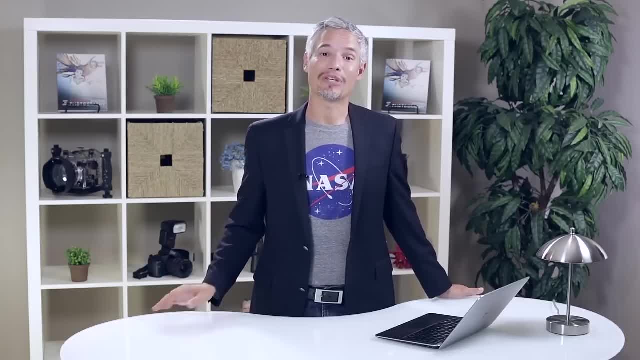 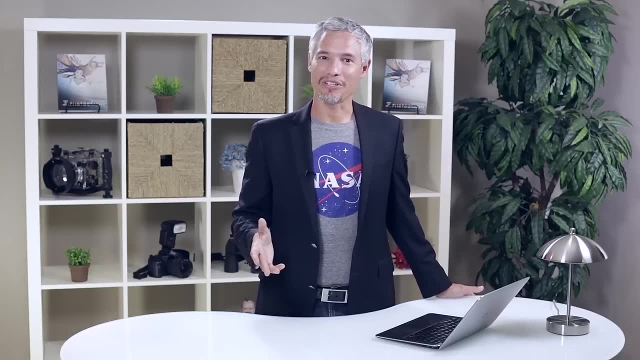 Now they're good enough for the average person's family photos, But they might not be commercial quality sharp, So you could upgrade your lens or you could just set the bar a little lower and decide that you're going to be satisfied with that little bit of blurriness. 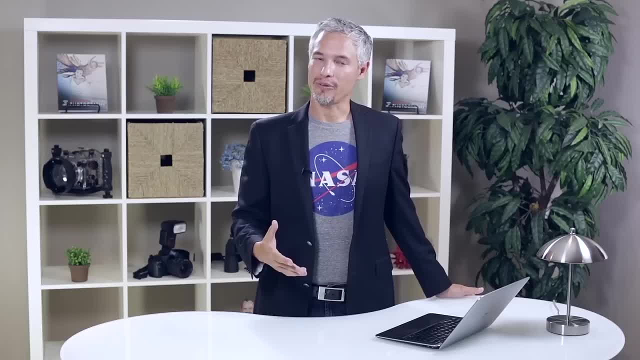 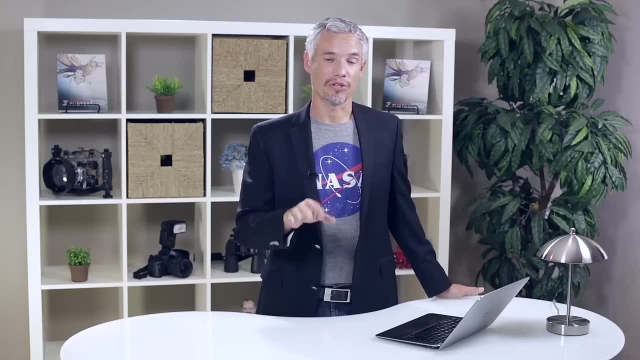 Now it can be difficult to determine which lenses are sharper than others, because sharpness is really important to a lot of people. So the way I determine this is by looking at lens reviews. These are very analytical lens reviews that just check out sharpness on different camera. 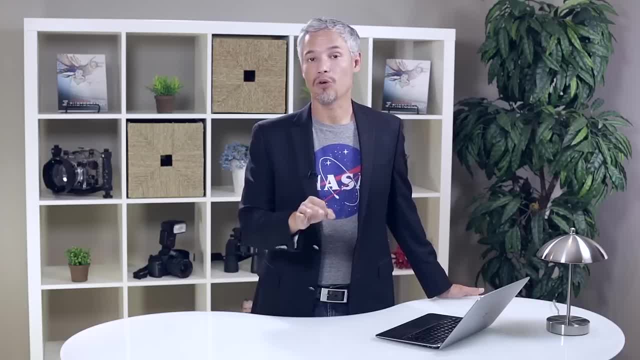 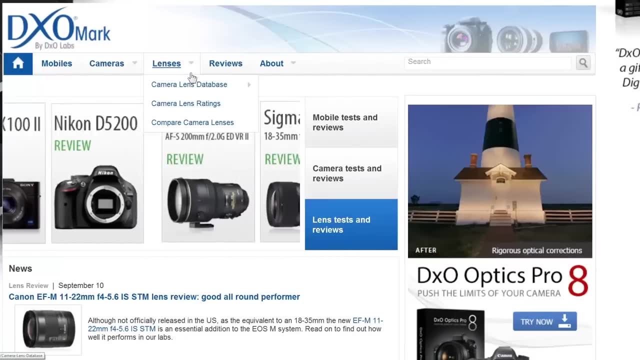 bodies. So let's open up a browser and head over to DxOMark, just so I can show you how to compare different lenses. Here we are at the DxOMark website. I'm going to go to the lens menu here- camera lens database- and then I'll select Nikon. 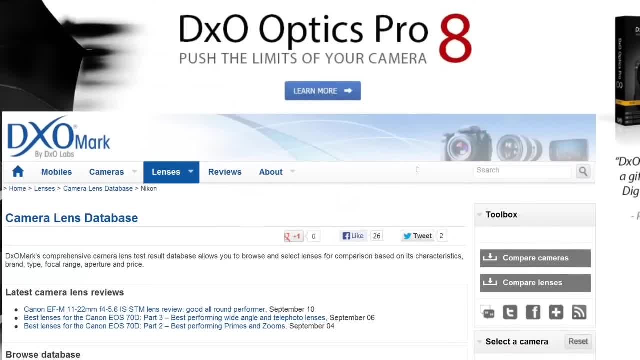 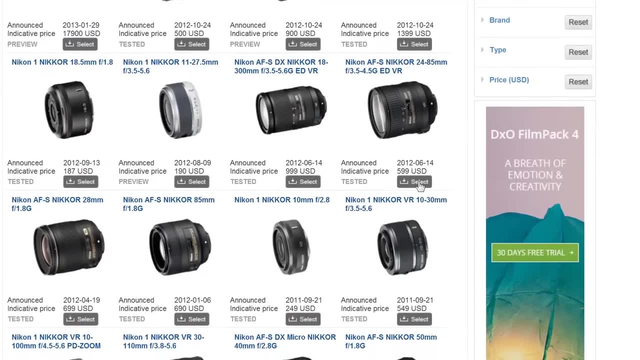 so we can compare some common Nikon lenses. This will list every Nikon lens, basically ever at least stuff they have in their database. So let's compare a few lenses at different price points and different quality levels. This Nikon 18-300mm. 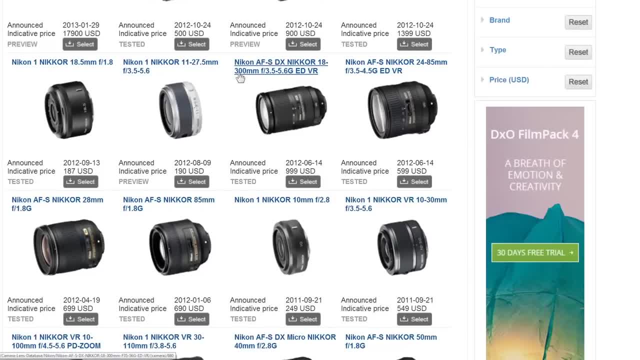 It's what we call a super zoom, So it has this huge zoom range. As you can see, most zoom lenses are more like this one: 24-85mm. that's a fairly small zoom range, But 18-300mm is a huge zoom range, and these super zooms are known to have poor quality. 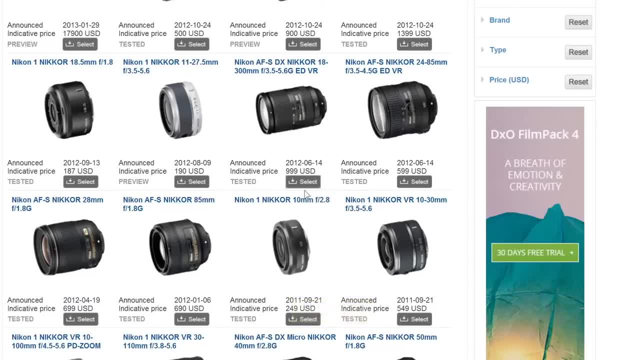 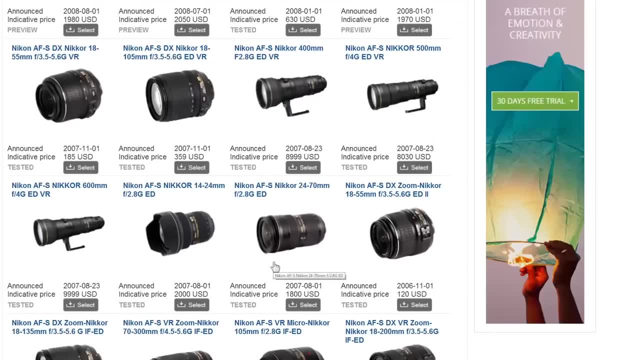 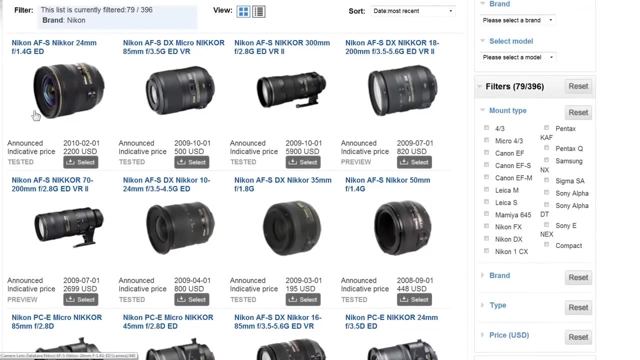 So I'll click the select button here to add it to my list of selected lenses for later comparison. Now I'm going to go to the next page and let's select a prime, because prime lenses are almost always sharper and faster than comparably priced zooms. 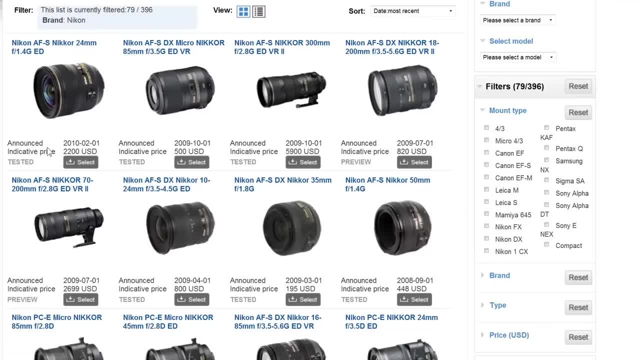 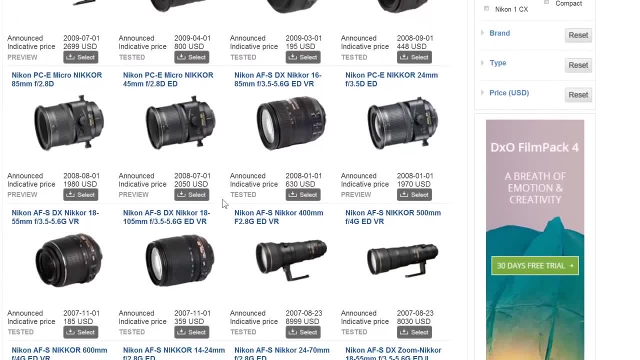 And this: well, this is a really expensive prime, but just for the sake of these, but just for the sake of this comparison, I'll go ahead and select that too. Now let's see if we can find their professional zoom lens, their 24-70mm, which every camera. 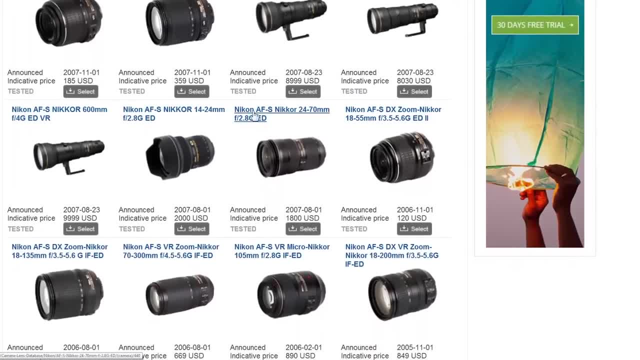 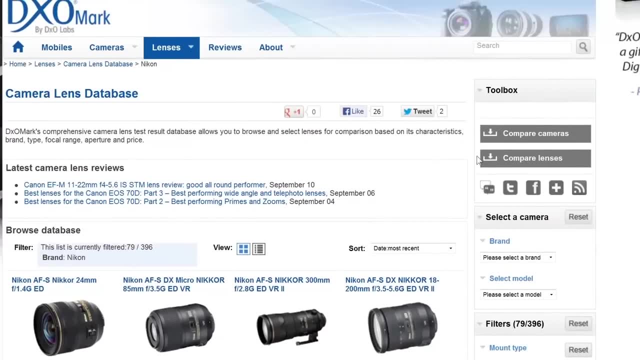 manufacturer has one of these 24-70mm f2.8s and they're always very expensive. You can see this one's 18-100mm, so I'll select that too. Now I'll scroll back up to the top and click compare lenses here. 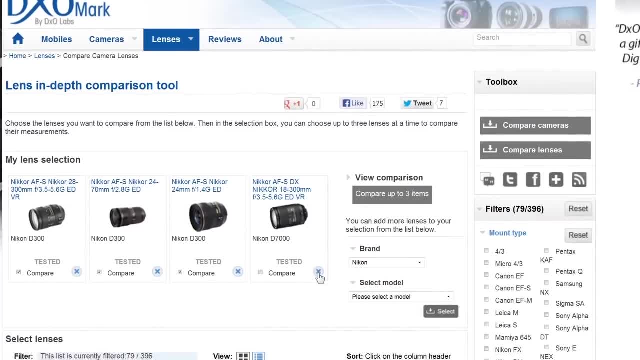 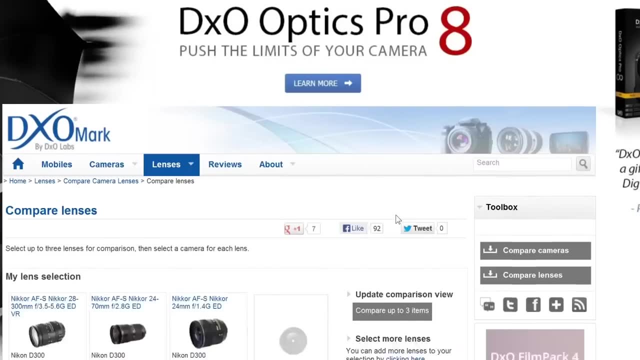 Looks like I had an extra lens from a previous comparison, so I'll just drop one of these and click compare up to three items And this is going to show me their test results for the different lenses. So on the left we have the super zoom and in the middle we have their professional zoom. 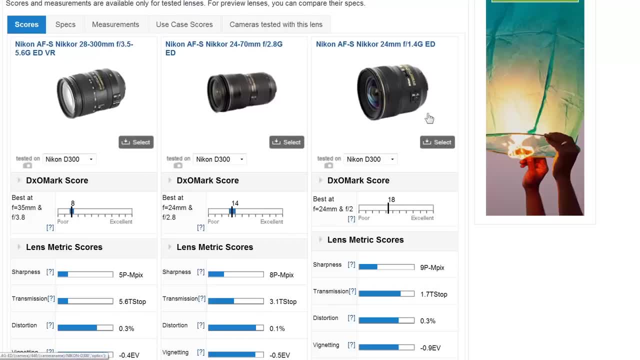 the 24-70mm, and on the right we have this very expensive prime lens. The DxOMark score gives you a good overview of generally how sharp the lens is, So you can see the super zoom. it's a good quality lens. 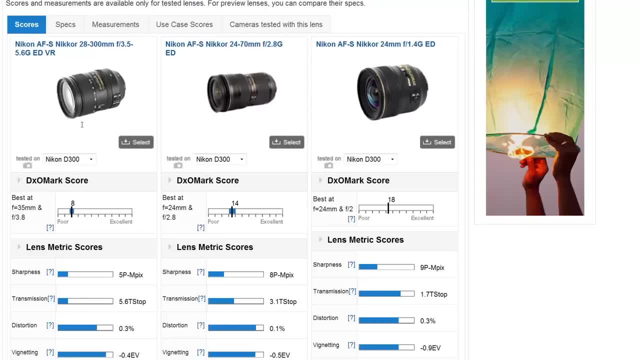 But I warned you that super zooms are never extremely sharp, because they're more of a jack-of-all-trades than a master of any, And the sharpness is coming in at an 8, and that's just an arbitrary score that they provide. 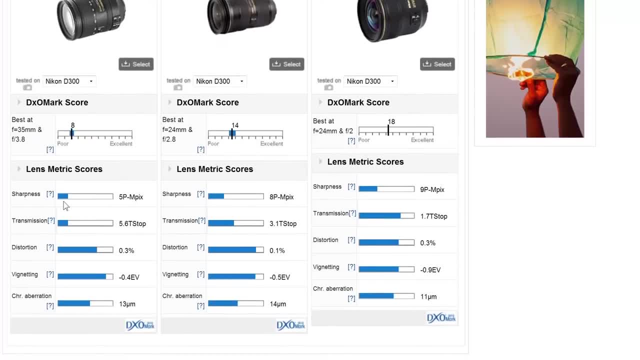 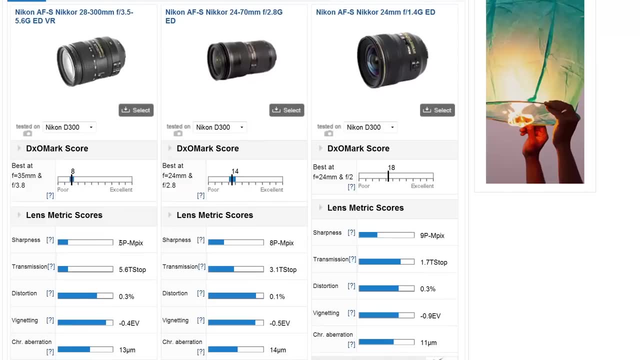 It's not a measurement of anything specifically. We can also see the sharpness measurement here. They also provide this. what they call the PMPix is coming in at a 5. So it's roughly 5 megapixels of data transmission. 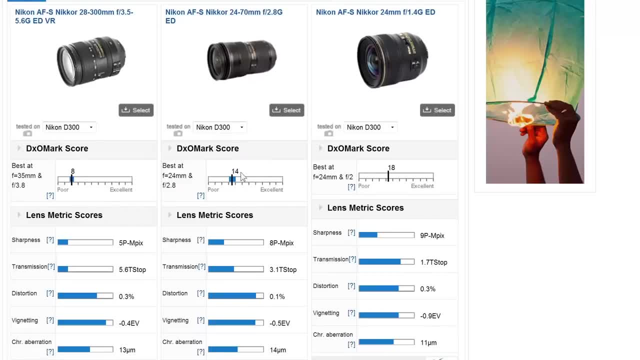 The professional zoom, the 24-70mm f2.8, is coming in at a sharpness level of 14. So a 14 compared to an 8. Pictures taken with this lens are going to be much, much sharper than pictures taken. 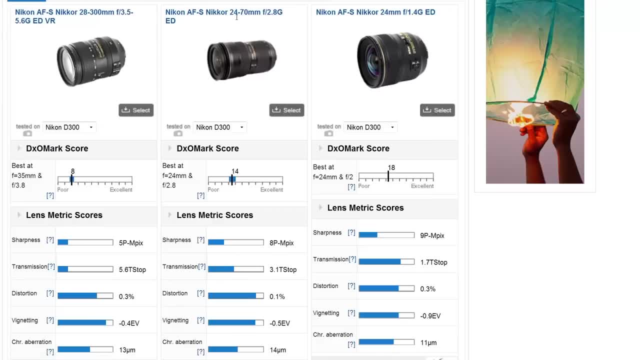 with the super zoom, However, you have a range of only 24-70mm instead of 28-300mm, So there's a trade-off there. This lens is also much more expensive because it's a professional lens. Now, on the far right, we have this high-end prime lens. 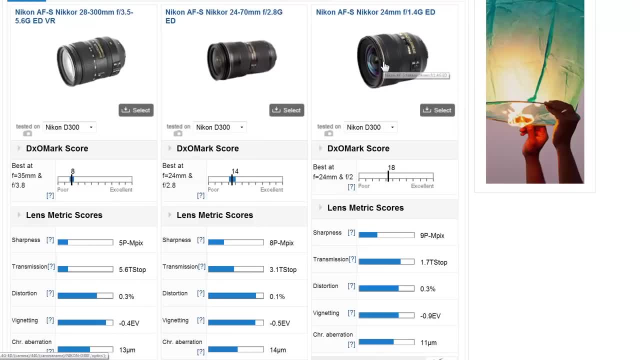 This is not a zoom at all. So you're stuck at this one focal length And if you zoom in, you can see that it's not a zoom at all. If you want to zoom in, you get to change lenses and buy another lens. 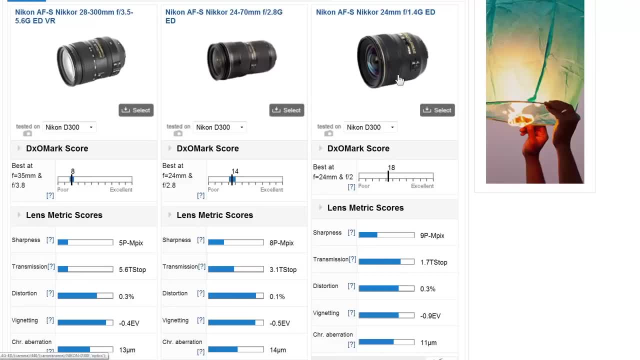 You can see that this is rated at 18.. So this is sharper than this professional zoom lens substantially, And these are both sharper than the more consumer-level super zoom. Now, one other thing to check is the camera that it's being tested on. 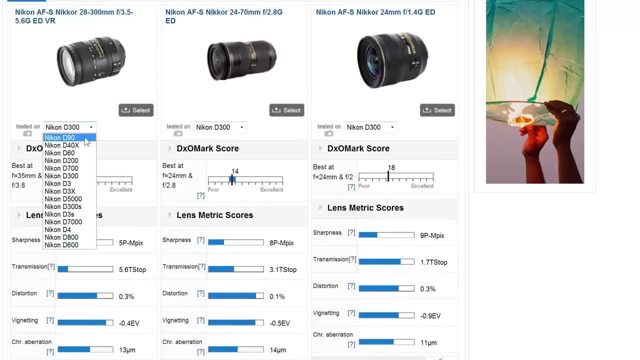 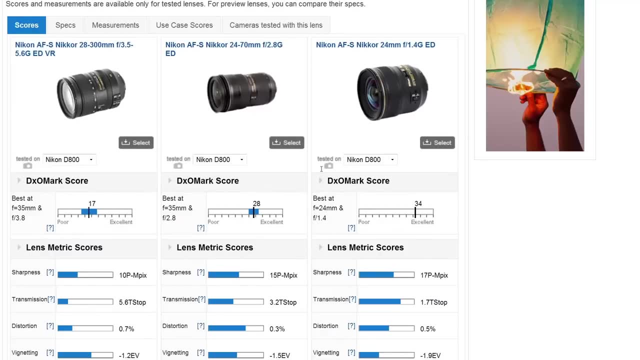 If you do have a camera body that's on the list, I would go ahead and select that. DxO tests their lenses on different bodies, because a body with very low megapixels might not be able to realize the difference between a super zoom and an expensive prime. 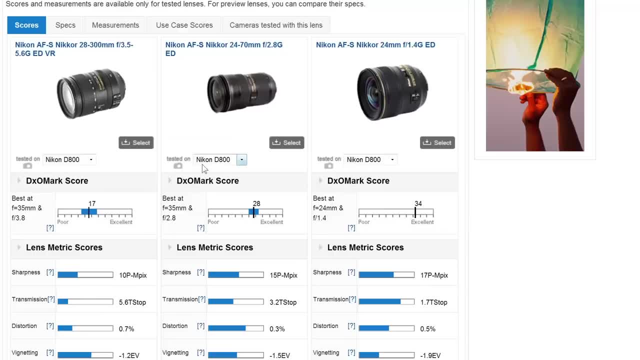 Therefore, you can see how these score on your actual body to know if it's even worthwhile. If you had a 6-megapixel camera, you'd get the same results with either lens most likely. However, if you have a monster like the D800, which has a ridiculous number of megapixels, 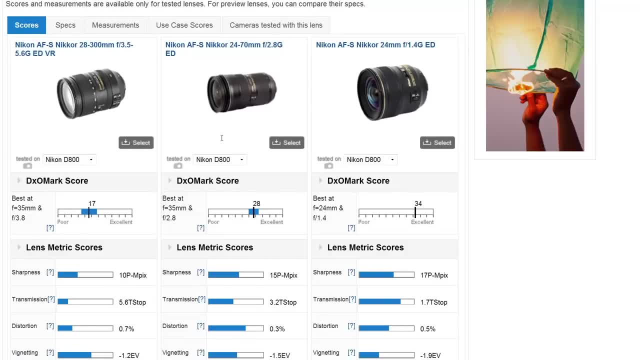 you're going to realize much more of the improved quality with these higher-end lenses. So you can see on this very high megapixel D800,. suddenly the DxOMark score of this super zoom jumps up to 17, and we can now extract a total of 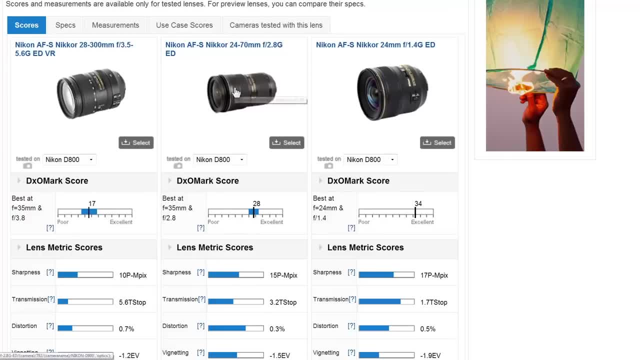 about 10 megapixels from it On their professional zoom to 24-70, on the higher-end body with plenty of megapixels. we can now extract a total of 15 megapixels, and this score is at 28.. 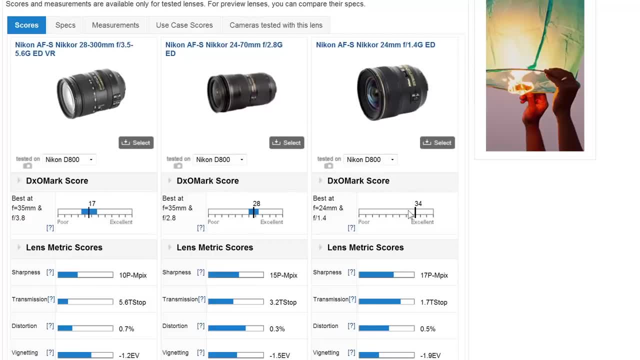 And once again, the prime is still way, way ahead because, like I said, these primes are always sharper than the zooms. they're just kind of a pain to use And the total sharpness extracted is about 17 megapixels, according to DxOMark. 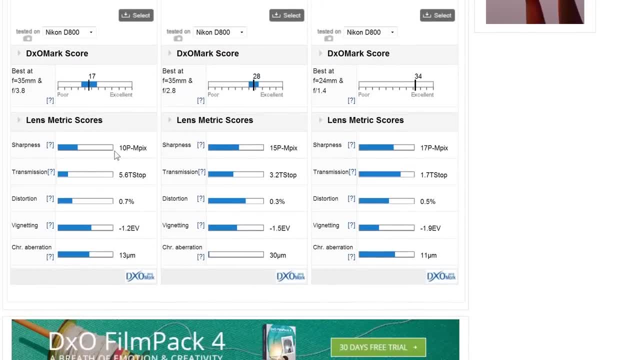 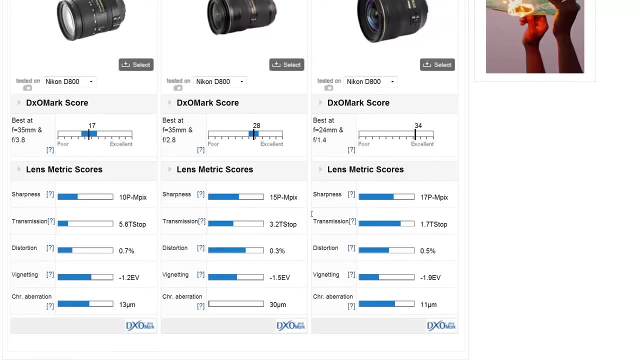 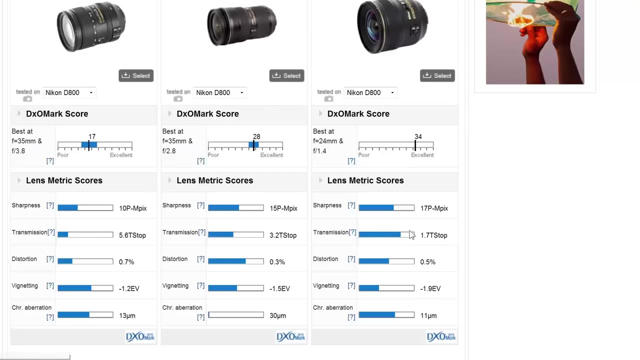 Now, below that, you can see some other data which is probably not as important to most people as the sharpness. The transmission tells you basically how much of the total light entering actually gets through to your camera's sensor. Once again, prime lenses transmit much more of the light, and this means that you'll be 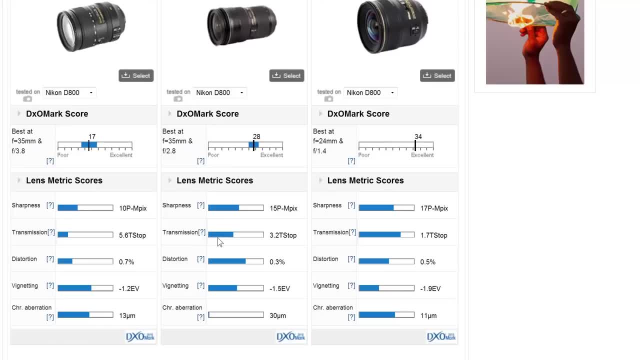 able to use a faster shutter speed even at the same aperture. Many people don't realize that lenses, even at the same aperture, will transmit different amounts of light. Where you're focused makes a difference, and how you're zoomed in can make a difference. 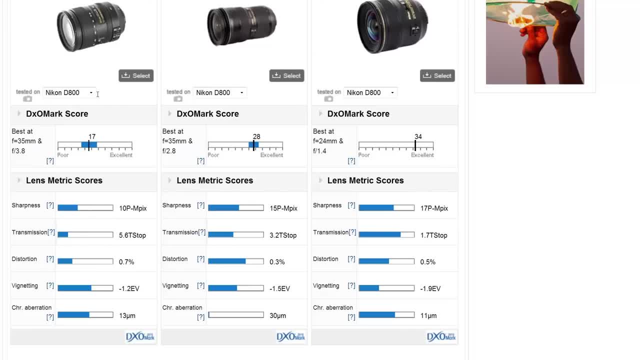 as well as the actual construction of the lens. Sometimes light just gets lost and doesn't make it all the way to the sensor. As you can see, the very simple prime lens design allows much more light to get to the sensor. Distortion is a measurement of how much curving, pincushioning and several other factors gets. 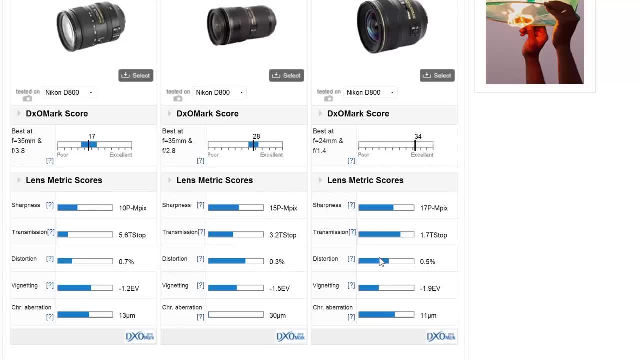 transmitted into the final image And once again, the prime lens is by far the best here, with the super zoom being the worst. The fuller these bars are, the better it is. Vignetting is the darkening of the corners of the images, and wide-angle lenses are always. 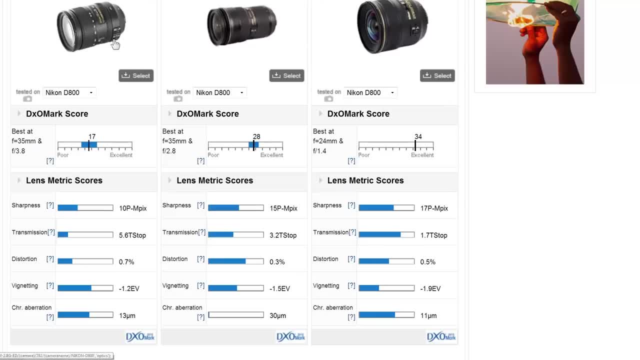 worse at vignetting than the more zoomed-in telephoto lenses, and I think that's why this prime didn't score as well there. One nice thing about distortion and vignetting and chromatic aberration is that these can all be corrected in post, and in fact Adobe Lightroom will automatically correct for distortion. 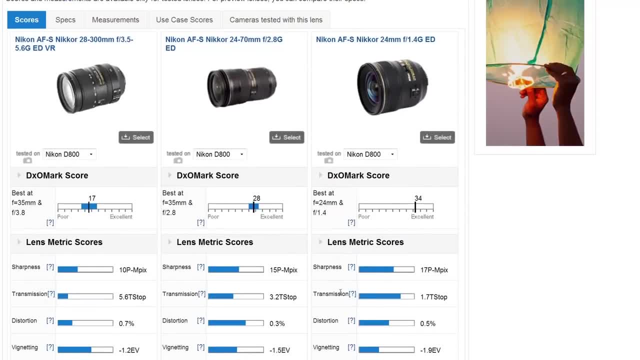 and vignetting if you select that option. Once again, I'll mention that I think most people overestimate the importance of sharpness when choosing a lens. Sharpness doesn't matter as much as most people think it does, but for some of us it really. 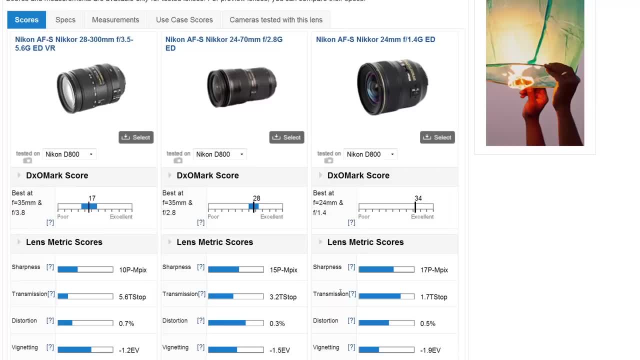 is important. For example, when Chelsea and I shoot commercial photography, I know the commercial buyers really scrutinize the sharpness and for that reason it's very, very important for me to have the sharpest lenses for my work. But if you're just putting up pictures on Facebook, you know they're only going to 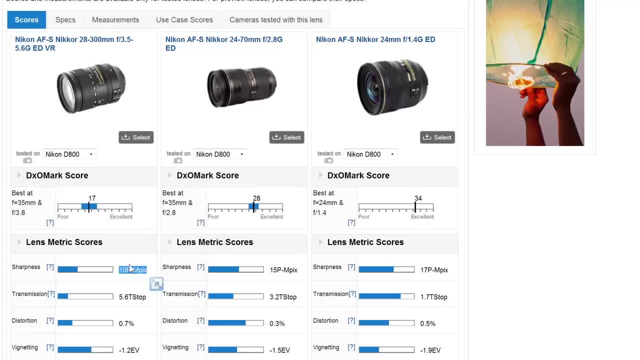 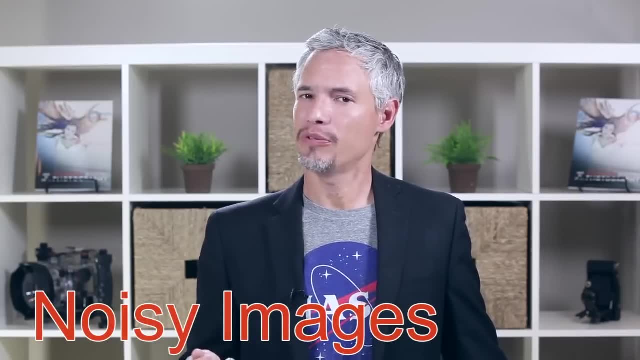 be a couple of megapixels. so even if this can transmit 10 megapixels, that's still a little far more than you'll ever need. Now let's learn how to diagnose noisy images. Your images will be noisy if you're using a high ISO number. 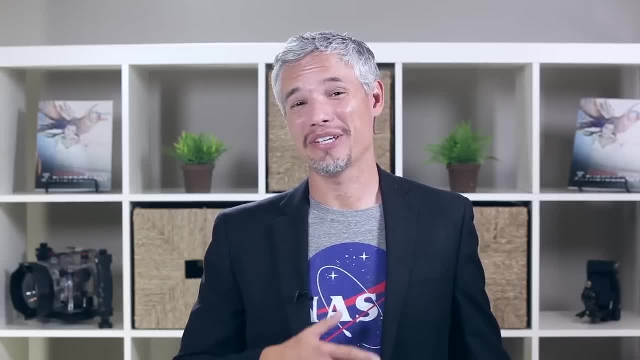 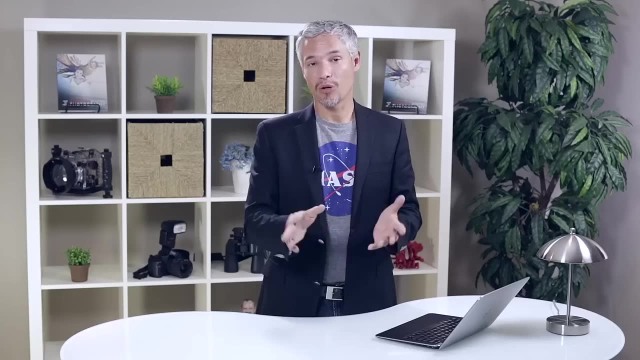 Now, different cameras have different levels of noise. Some cameras will be completely unbearable at ISO 800, and other cameras you might be happy with pictures taken at ISO 3200.. But one fact is always true: The higher the ISO number, the noisier your pictures are going to be. 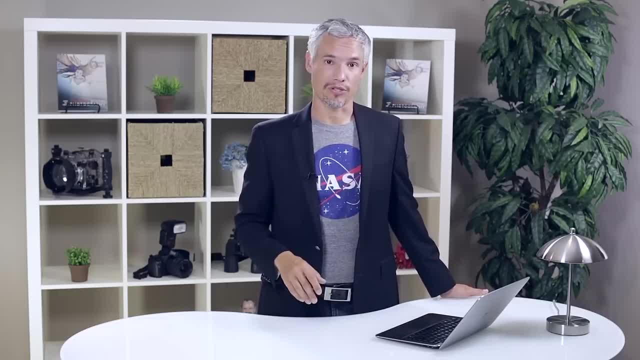 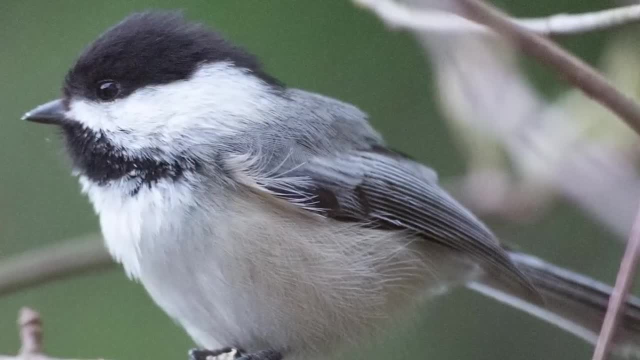 So let's look at a couple of pictures taken at high ISO so you'll know what noisy pictures look like. This picture of a chickadee was taken at ISO 6400, and you can see it's not that bad. But if you look at the background and especially if you zoom in real tight, you'll see that 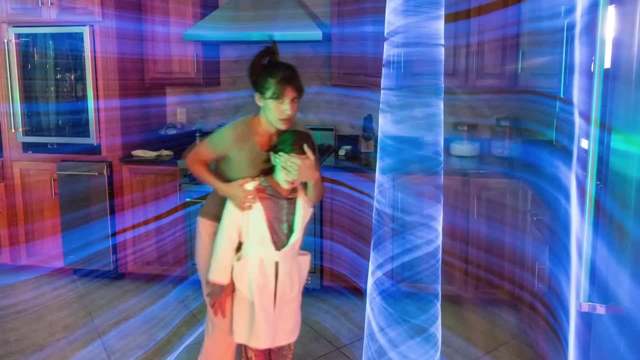 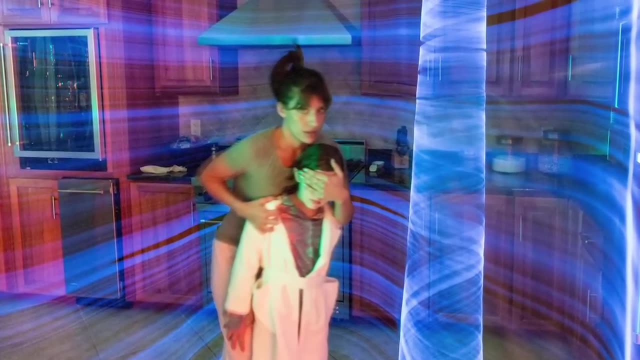 it's completely speckled. This light painting picture is also taken at ISO 6400. And if we zoom in nice and tight here we can see that everything is a little bit speckled. That's a sign of digital noise and, again, a side effect of using a high ISO. 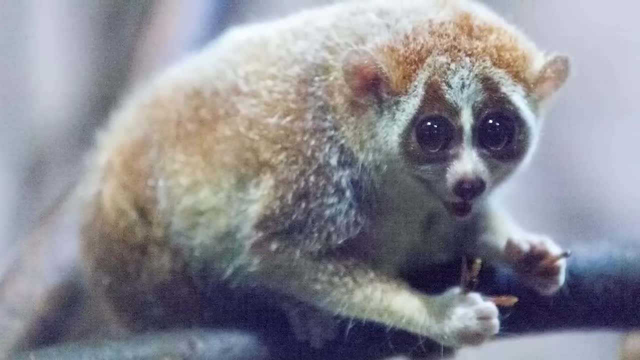 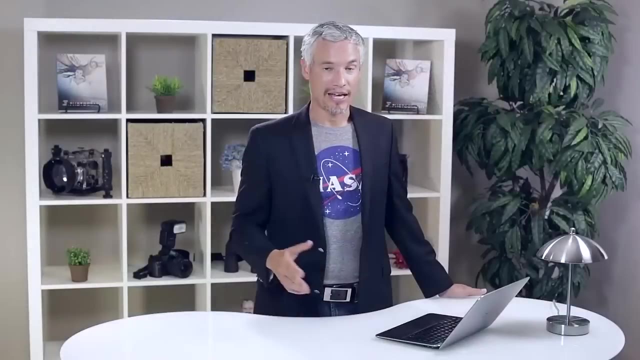 Let's go even higher on the ISO scale. This picture of a slow Lowry. It was taken at ISO 25600.. This is a night animal, So the zoo exhibit that they have has them in very dim conditions and I had no choice. 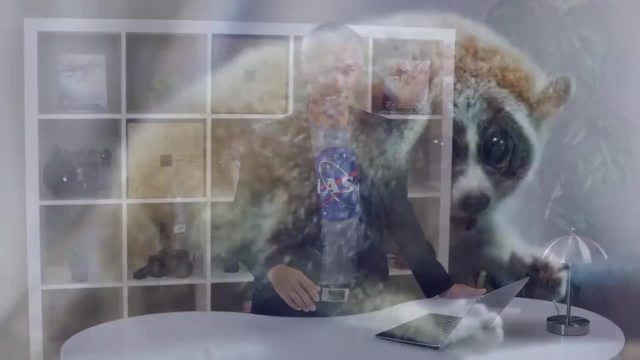 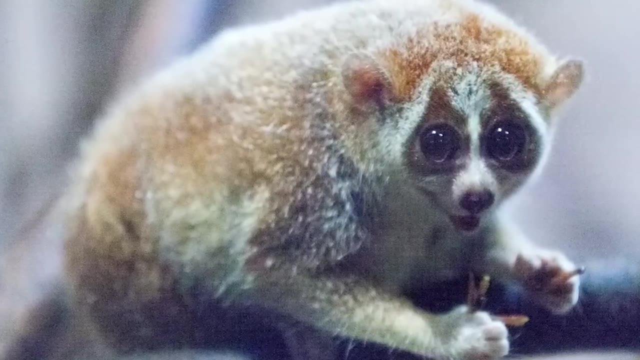 but to use a really high ISO and you can see. the necessary side effect is that everything is very kind of speckly and you'll see just random spots of red and green If you get zoomed in enough. there's no eliminating this. 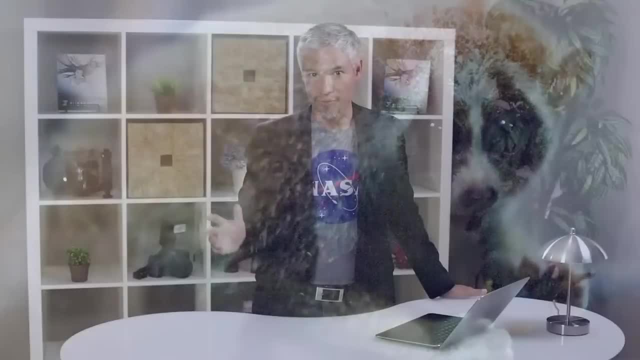 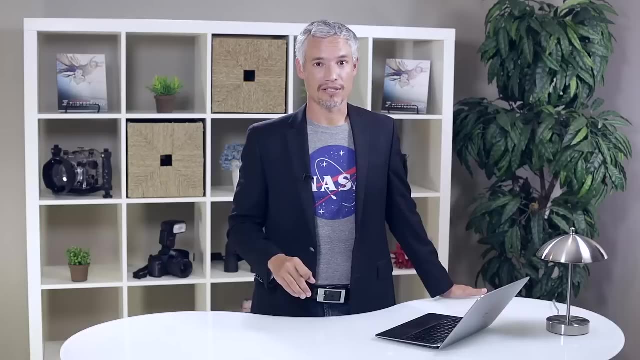 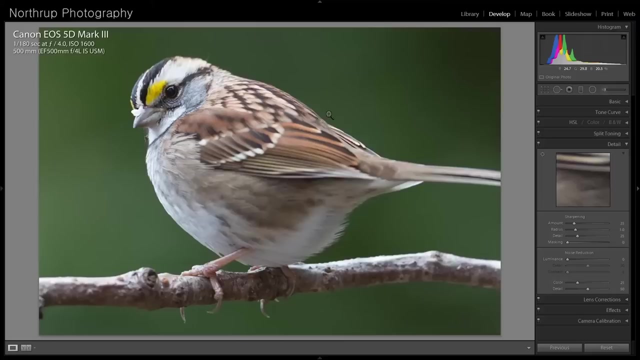 Noise is going to be a factor in digital images forever, as far as I can tell. I would like to, however, show you how you can reduce this, The noise, using post-processing techniques. So let's look at an application. This is Adobe Lightroom, the app I use to organize and do light editing on my photos. 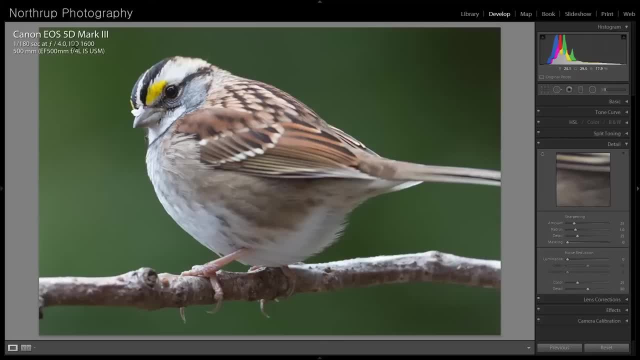 This is a cute picture of a chipping sparrow and you can see up here that I shot it at ISO 1600. And I know with any camera at ISO 1600, we're going to see some noise, but especially in 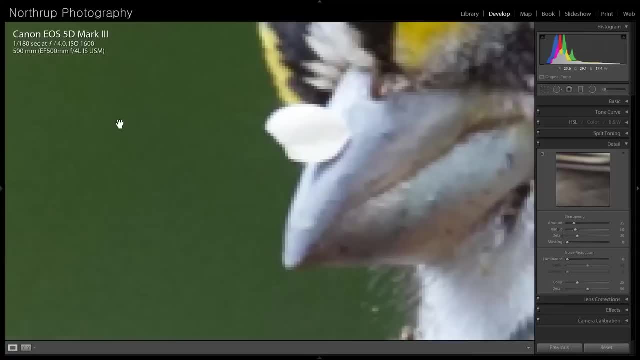 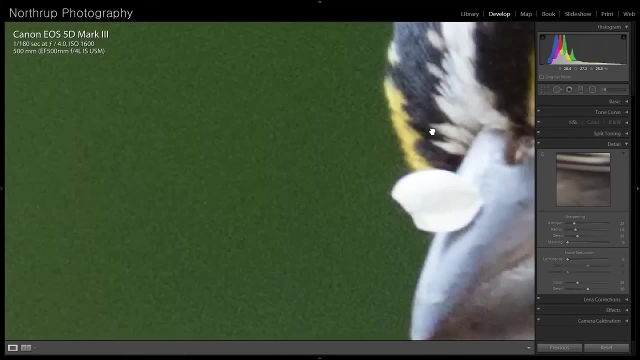 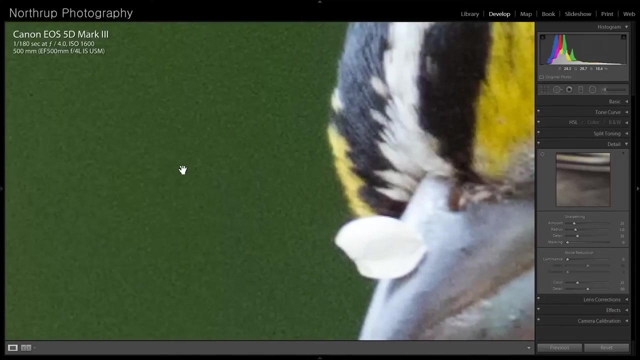 solid colors, So I know to expect some noise in the green here. especially solid primary colors are bad. I'm going to show you how my camera sensors work, So I'm zoomed way in here at about four pixels to one pixel, so at about 400%. 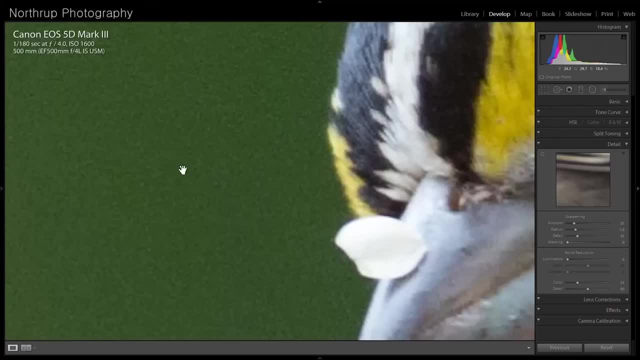 And I know on video noise and still images doesn't always show up, But what I want to see here is a solid, just nice wash of green, because the background is completely out of focus and it should be completely silky smooth, But instead what I see is green speckles everywhere, and if you're not seeing it in the video, 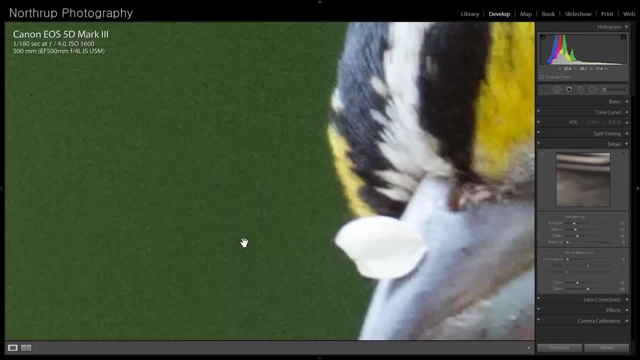 clearly. So go ahead and take a look at one of your pictures that has a nice solid colored out of focus background and you'll see exactly what I mean. You might have to zoom in to four, to one or so, but my camera has a pretty good quality. 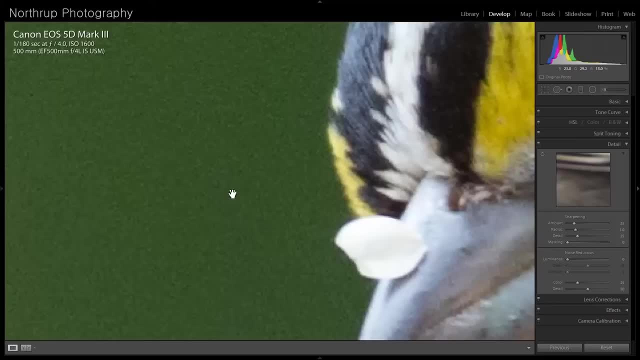 camera. It's a professional level camera, but you can still see that it has quite a bit of noise. There are a couple of ways to get rid of this. In the detail pane here I'll see the noise reduction slider, specifically the luminance. 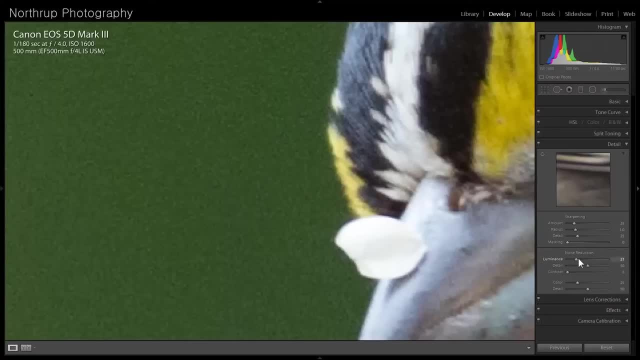 slider here and I can just drag this up, And the more I drag it up, the more the noise disappears. Most image editing apps have some noise reduction feature. Photoshop has it built in, of course, if you go for the big guy. 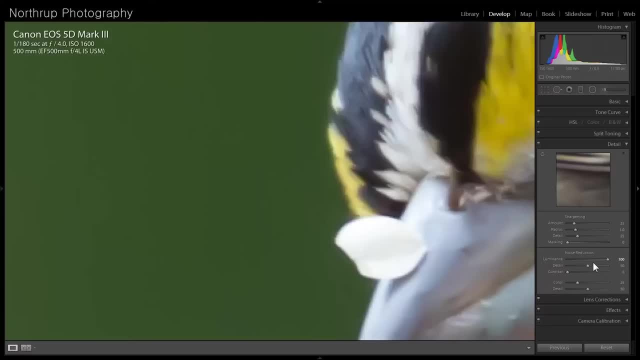 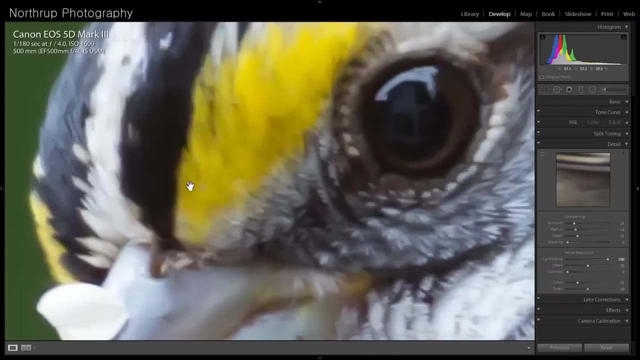 But Google Picasa is a free app that has noise reduction built in. Now there's a downside to cranking the noise reduction way up. As you might imagine, there's always a trade-off right, And that's loss of detail. 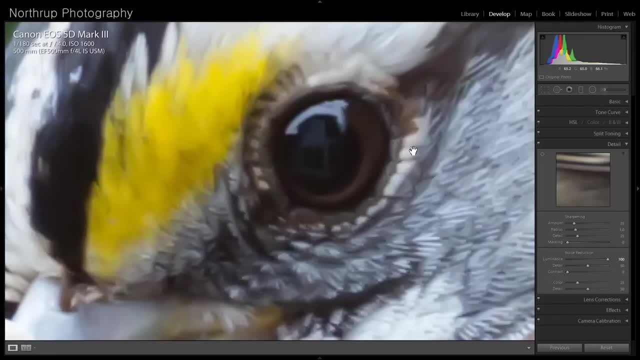 So if we look at the bird's eye here, we can see now it has this almost painterly effect. If I turn the noise reduction back off, we see it much more clearly. So that's a great way to get rid of the noise reduction. 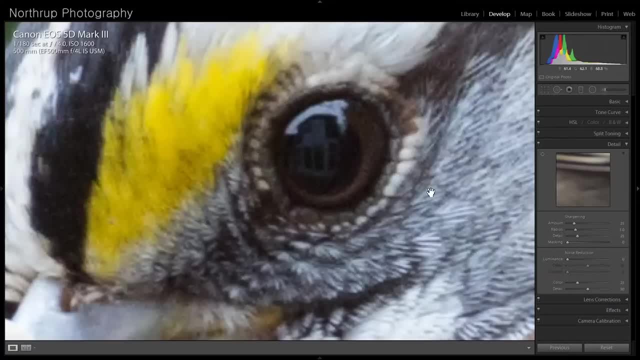 And that's a great way to get rid of the noise reduction. It's a much more natural-appearing photo. You can see all the details in the feathers here and it all looks very normal. But crank it way up and it starts to look a little like Gary Busey- a little crazy-looking. 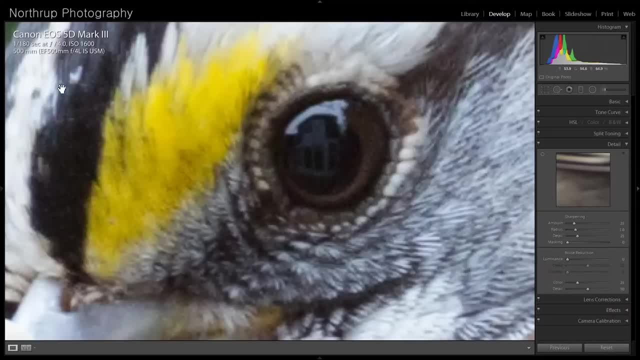 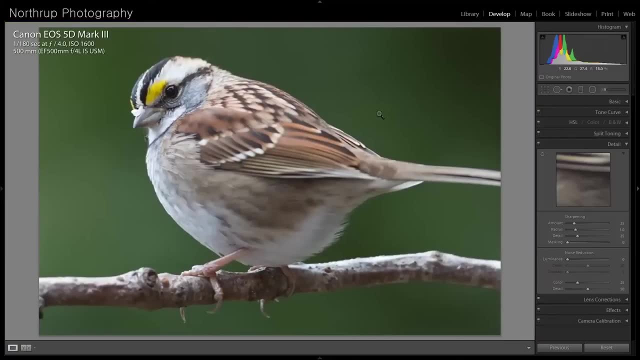 There's an easy way to fix that, and that's to select the background and apply the noise reduction only to one specific part of the picture. So you can do this pretty easily in Lightroom. You used to have to go into Photoshop, but now you can just use the adjustment brush. 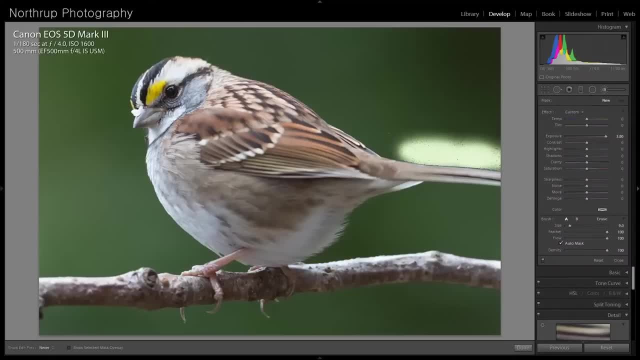 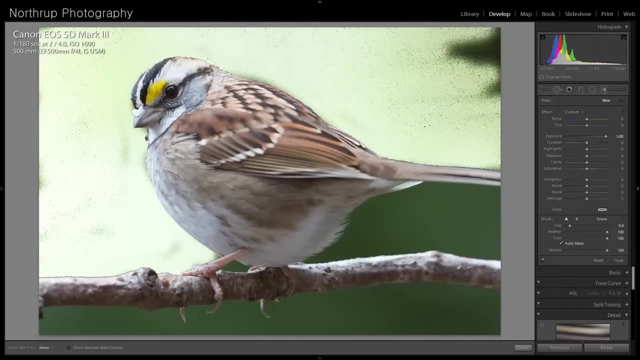 here You can do this and then I can just paint in the edges and it does a pretty good job of just picking up the background that needs to be modified In Lightroom. this isn't the most exact process, It's more of a general process and it's not going to do a perfect job. 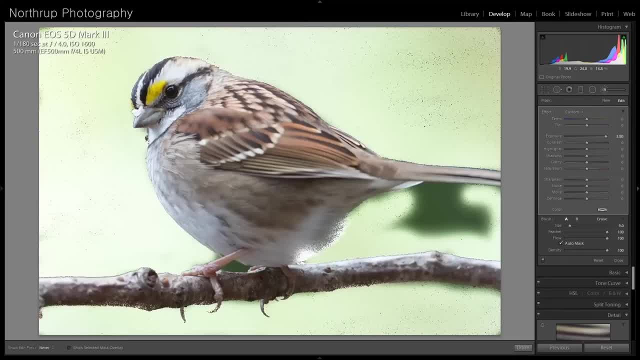 But for the sake of noise reduction, where you're not actually destroying anything, you're just making it a little silkier. it's not usually a major problem if you have a little bit of the subject itself highlighted. However, if you do go over, you can hold down the Alt key. 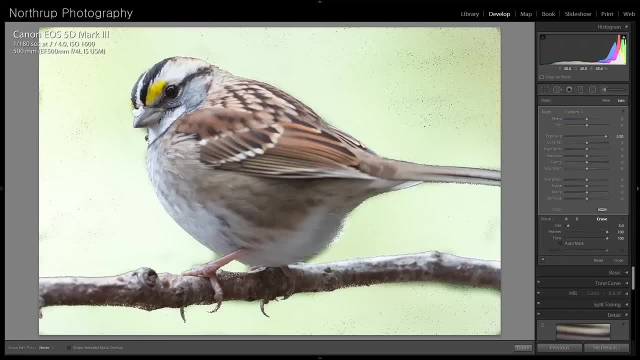 And this allows you to subtract parts of the selection. So you can see I went over here a little bit so I'll just subtract that out. to too much noise reduction on this branch here. So I'll even that out a little bit. Now, with this area selected, I can go into the adjustments here to fix it. 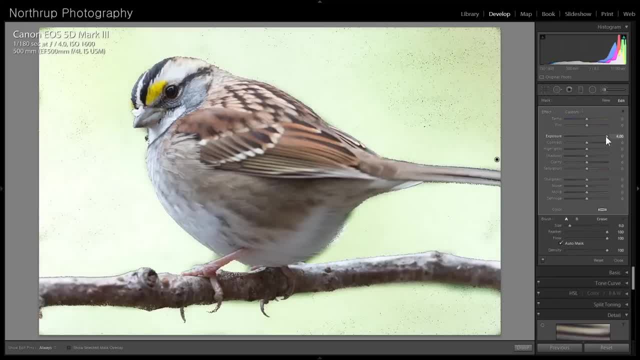 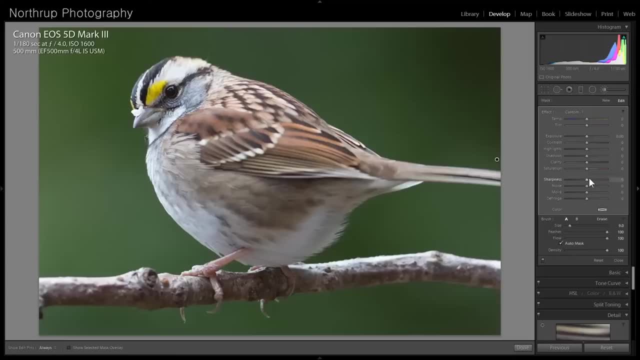 Now, by default, it cranks the exposure way up to three. This pretty much just allows you to see what you've selected. So I know I've got it selected and I'll drop the exposure back to where it belongs. Now I can crank the noise. 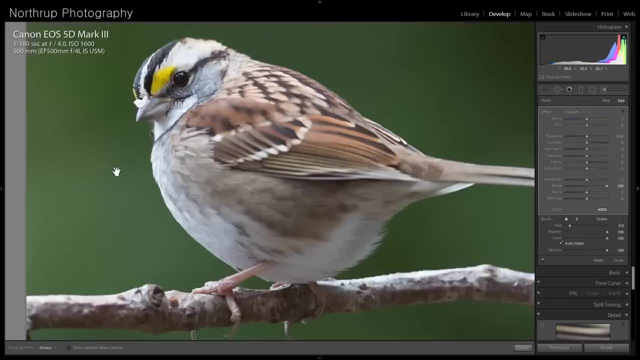 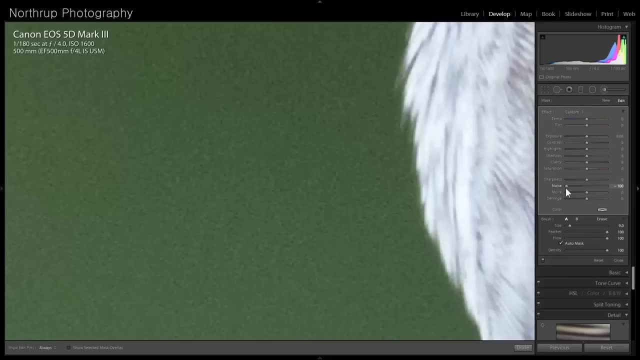 Here way up, And if I zoom back in now, I'll see nice and silky colors here. So just for comparison, that's what we started with and here's the noise all the way up. You can also adjust the sharpness down, because sharpness is basically the opposite of noise. 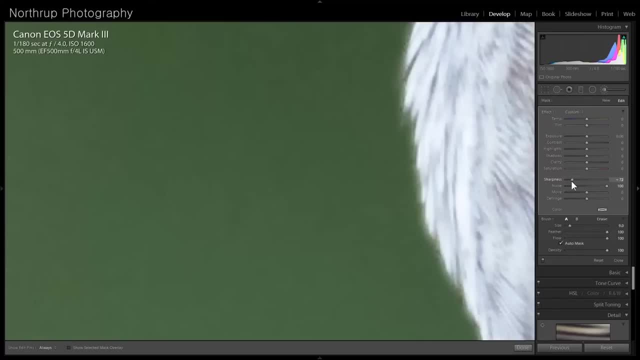 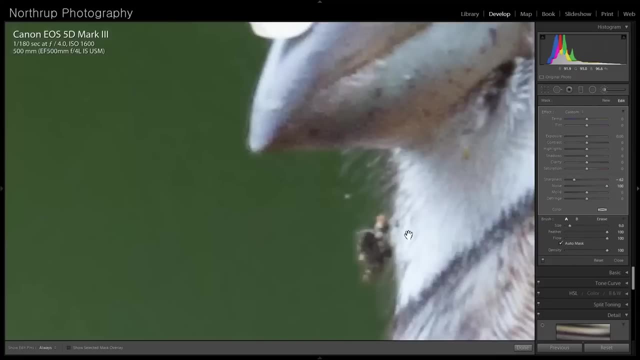 reduction. So I'm just going to drag the sharpness down to the point where I don't see any artifacts along the edges here. I always want to check the edges of your selection. In my experience, Lightroom does a really good job of selecting it. 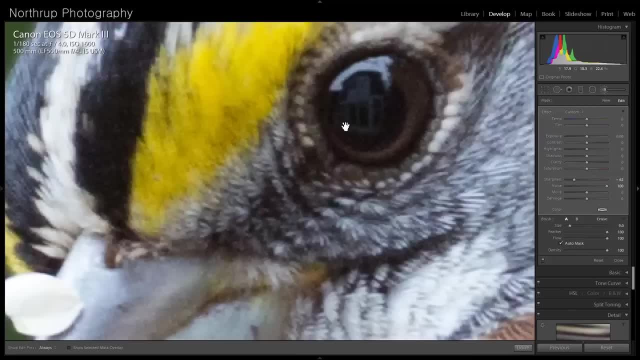 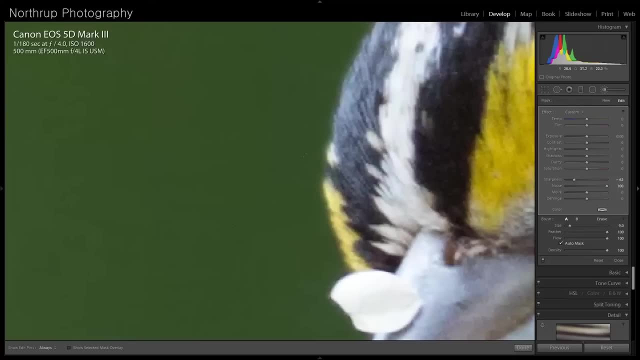 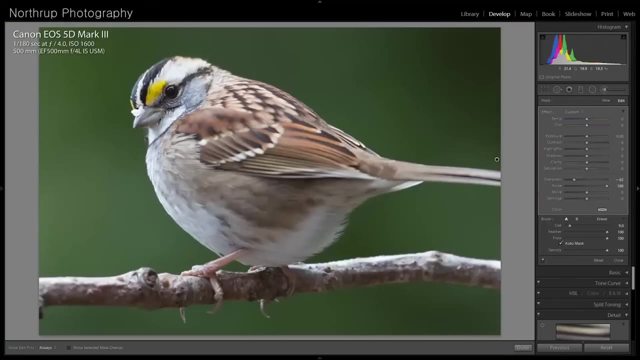 So you can see what we have now is the original, untouched eye, with all of its details still intact and silky, smooth background greens. Now, this looks good on screen in close up, but it will also look much, much better in a print, because digital noise doesn't look great in prints. 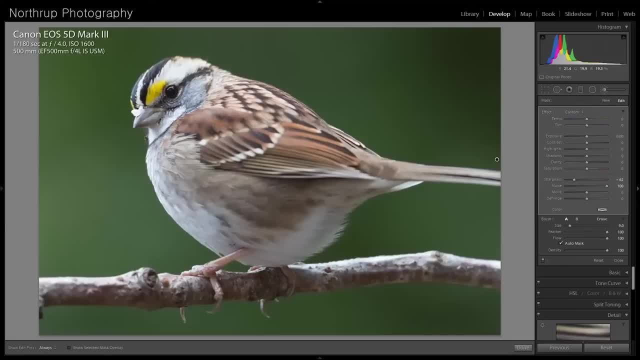 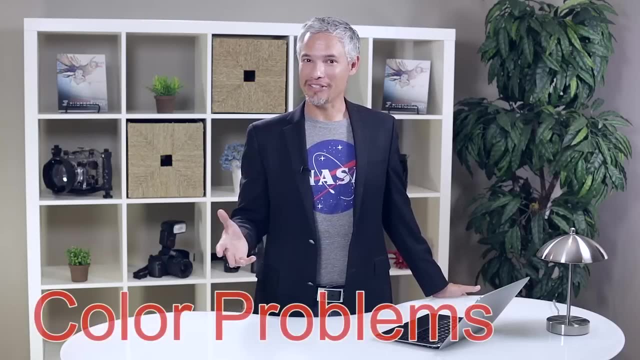 You know, we all kind of learn to love film grain. but that's one of the drawbacks of shooting with digital is fairly ugly grain. Now let's talk about color problems. It's really common that you take a picture of something and then you find out: oh it. 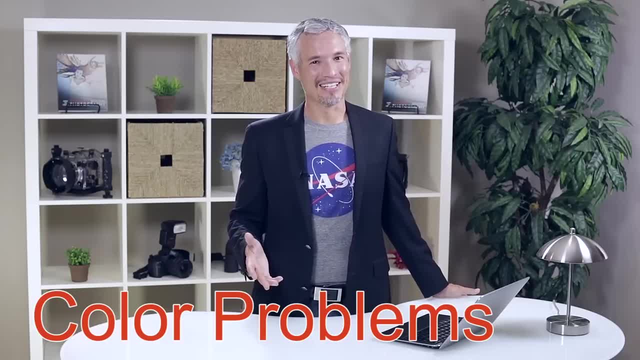 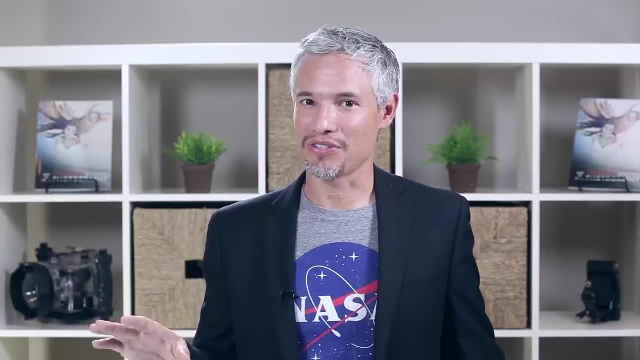 has this weird orange tint or it has like a weird green tint. The most common cause of color problems is white balance. You see, our eyes see most light sources as white. whether it's the sun or that incandescent bulb or an LED bulb, our eye kind of makes it out to be white. 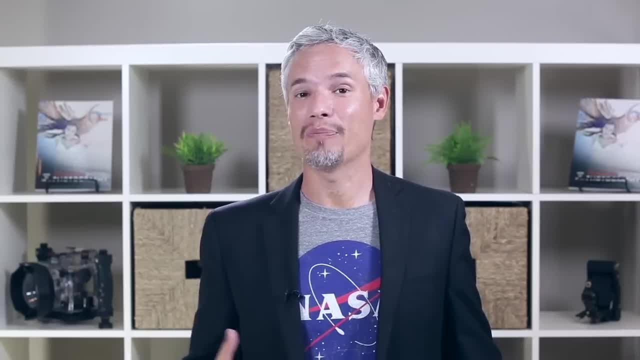 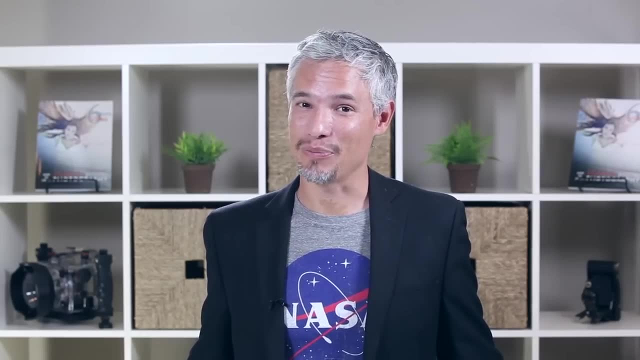 Our camera does its best to make all of that white, but it might not be as perfect as our eye. So if you're shooting outdoors in natural light a lot of times it ends up a little bit tinted brown. Let's look at some examples. 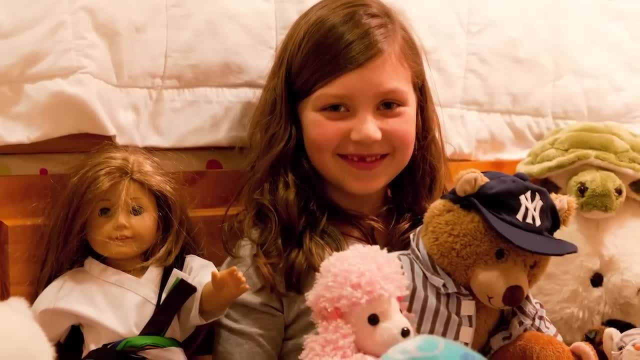 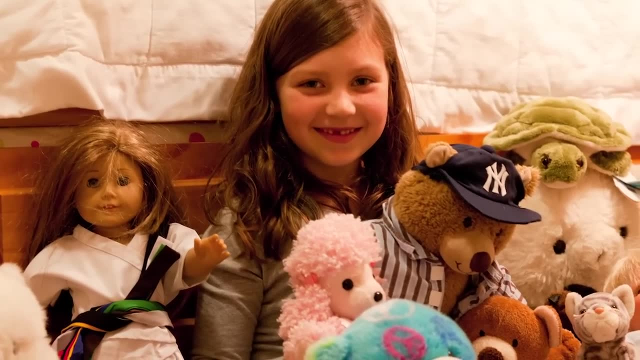 Here's a picture of my daughter in her bedroom with all of her favorite toys and you can see it has this like warm color cast and it might not be a bad of this, but I really prefer a more neutral color balance. So this is easily solved either at the time you're taking the picture or in post processing. 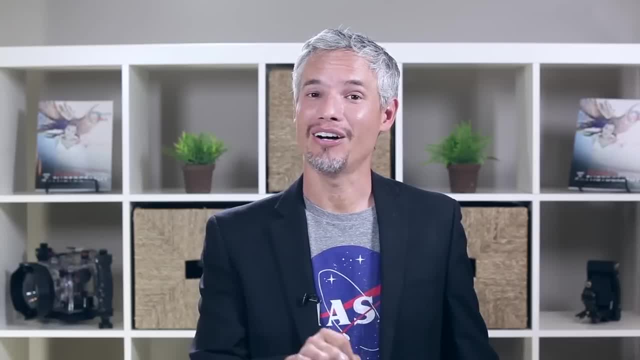 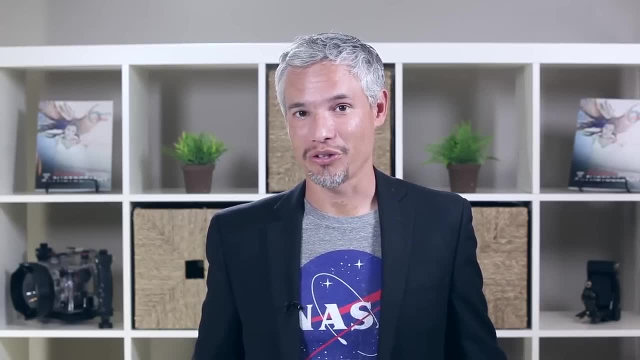 Now I usually leave my camera set to auto white balance, but I shoot raw instead of JPEG. This allows me to easily change the white balance later. For more information, check the controlling your camera video. Now you can also solve it at the time you're taking the picture by changing your camera's. 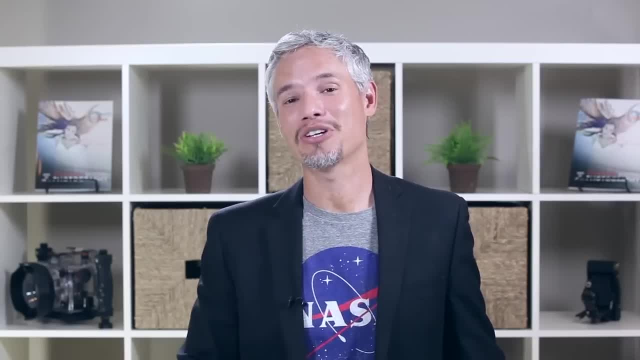 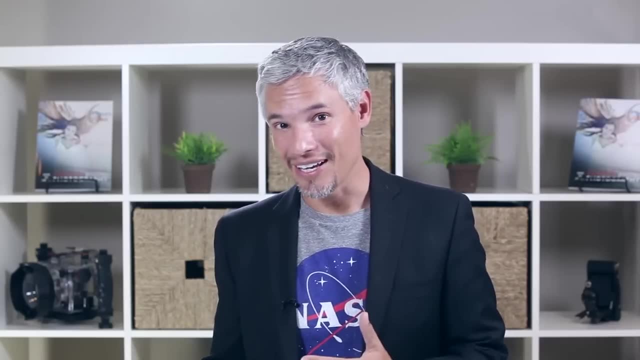 white balance setting to match what the actual light is. So if you look at your camera's white balance setting you'll see it has a setting for sunlight and cloudy and shade and probably tungsten lights and incandescent lights. Just pick the one that matches your environment and you're going to get the closest possible. 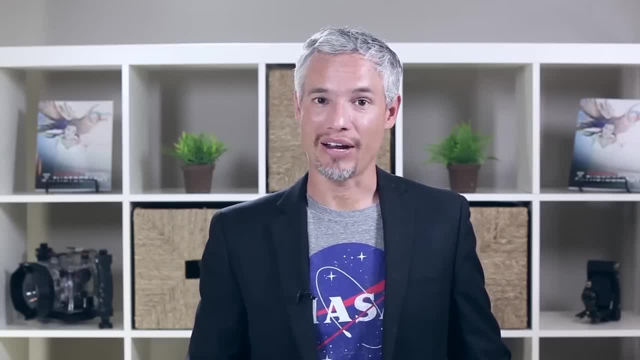 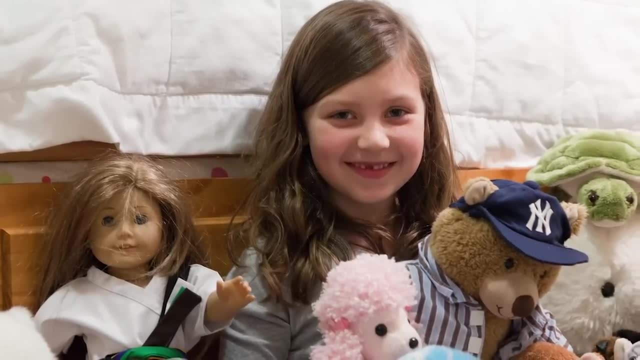 white balance, But This particular picture turned out after I edited it in Lightroom. There we go: We have nice, natural, perfect color, And fixing this is as simple as using the auto white balance tool in Lightroom and then selecting a white part of the picture. 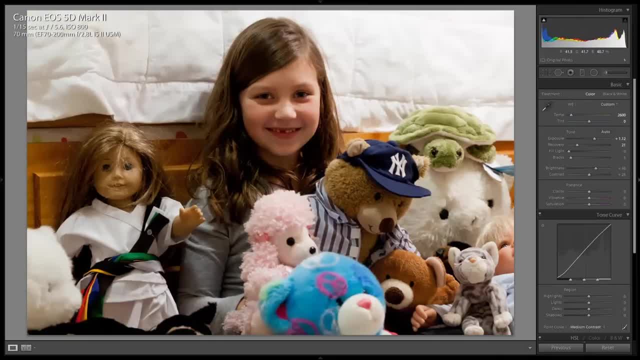 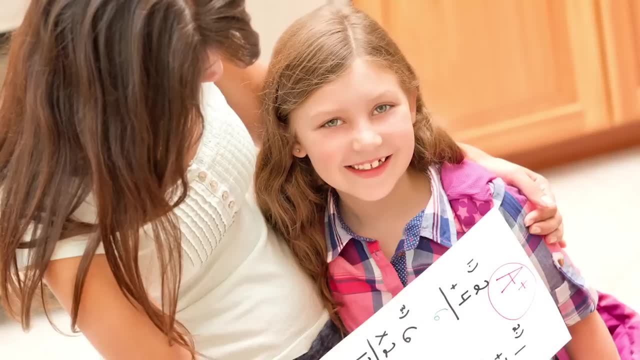 Maybe the gi on the karate doll off of her right shoulder there. Here's another picture of my daughter with Chelsea and you can see again we have that signature like warm kind of orangey tint to it. I can fix this in post processing with auto white balance. 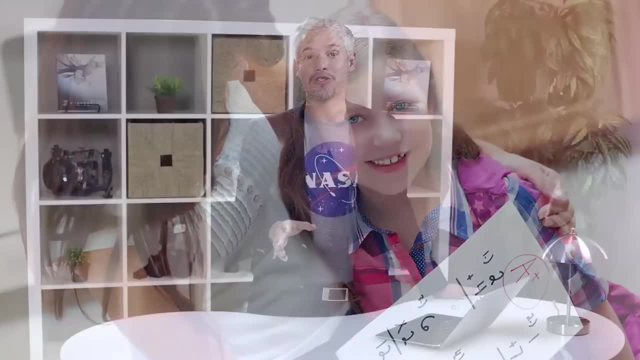 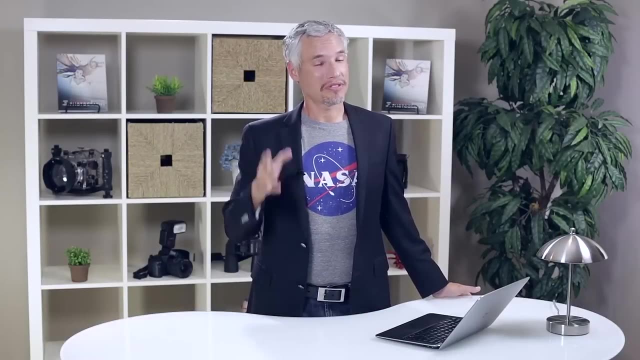 And there we go. That looks much better. Failure to adjust the white balance is probably the most common problem that I see on the readers group. So just when you're going through your pictures, just ask yourself: is it tinted orange or blue? 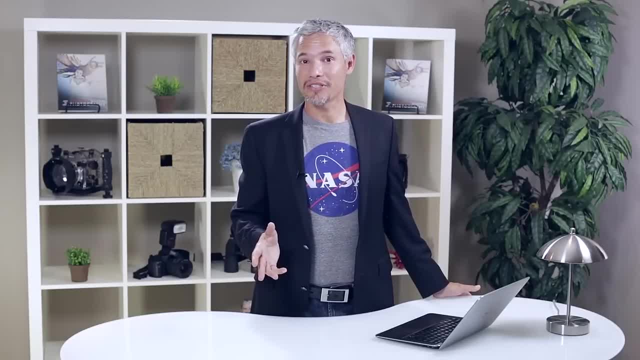 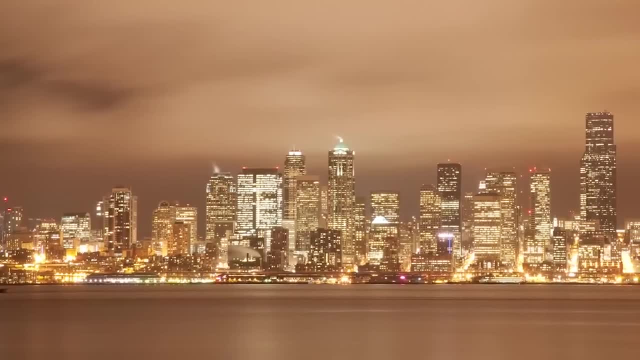 Could it be more natural and maybe decide to leave it with a nice warm tint because you like it. But I want you to do it deliberately and not accidentally. Let's look at another picture. This is a picture of the Seattle skyline, obviously taken at night, and night photos. 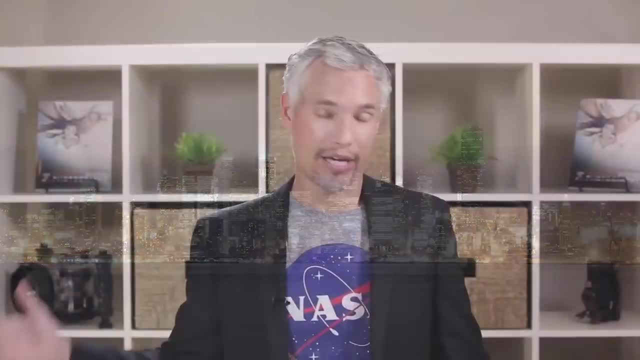 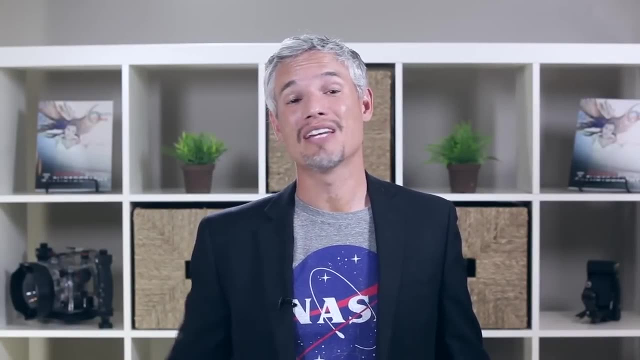 and cities. It's notoriously difficult to white balance because the city has just dozens of different types of light sources in it and they all have a little bit of a different white balance. So there's never going to be one white balance setting that perfectly matches the entire. 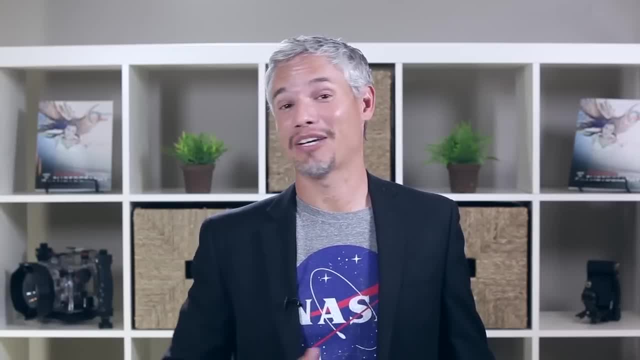 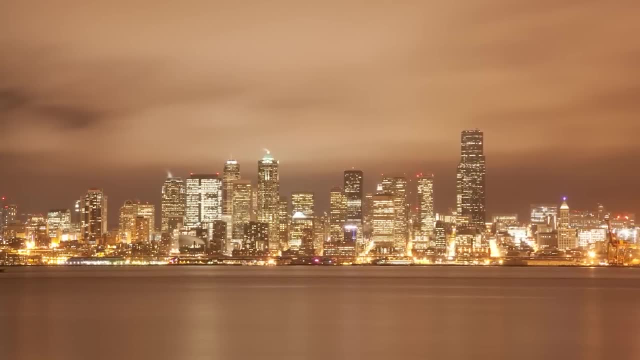 environment. But you know what Your camera- at least my cameras- always tend to pick completely the wrong white balance setting. So this was set to automatic white balance and you can see it's completely brown. That's not the way my eye saw it. 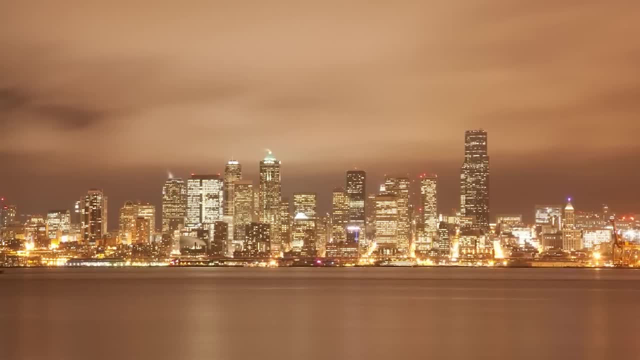 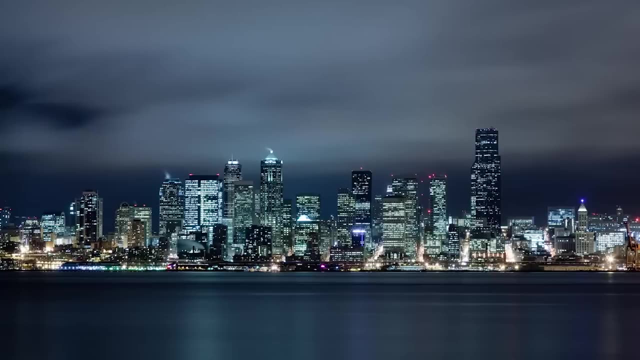 So in post processing I adjusted it So it was the way my eye saw it. Okay, There you go. I just changed it. so it was nice and cool blue. But if you look at those city lights, you still see that some of the lights are blue. 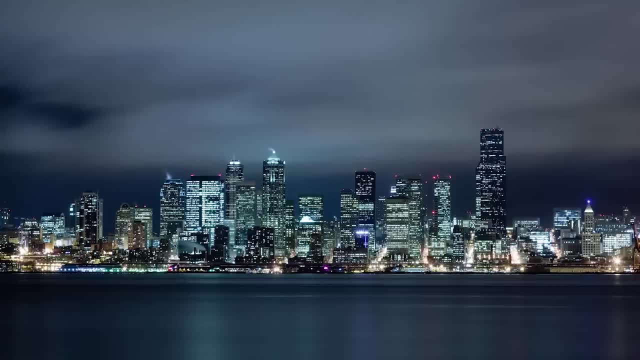 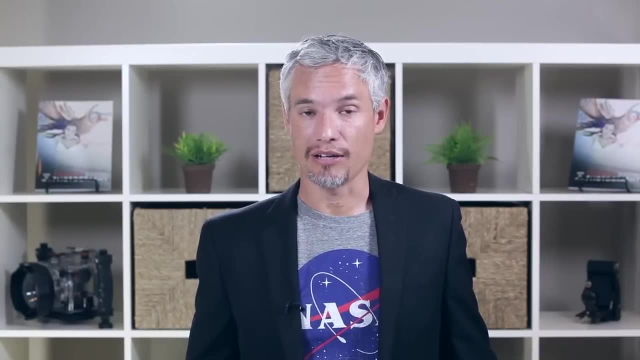 and some of them are orange And really with my eye all the lights kind of looked more white than that range of blue and orange. But like I was saying, because there are different light sources, you're not going to be able to easily get one setting that makes them all perfect. 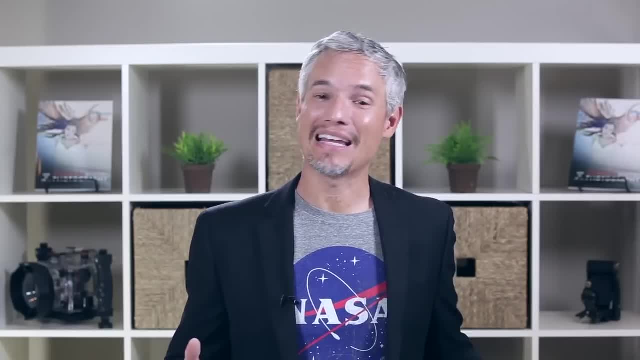 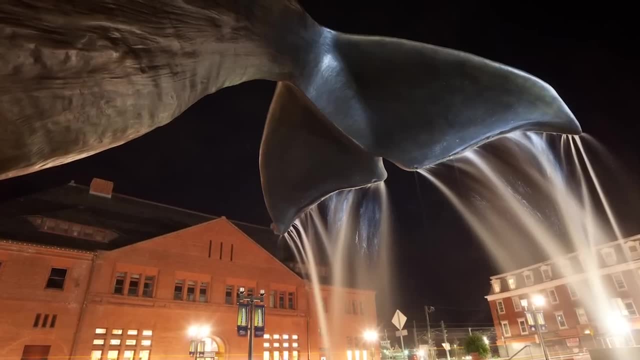 So what you end up doing is you find that one white balance. That's the best balance that gets you as close as you possibly can. Let's look at another picture. This is a picture of the Whale Tail Fountain in New London, Connecticut. 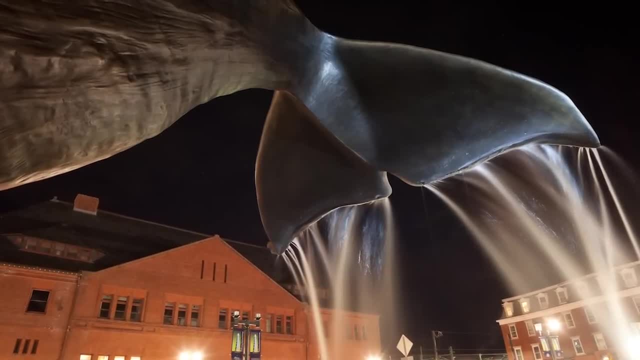 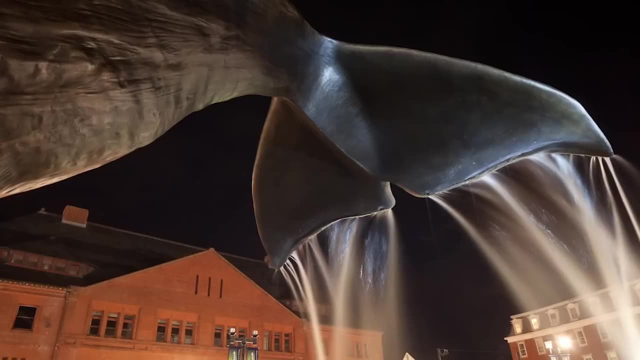 And the white balance isn't too bad here. This was using auto white balance, But if we look around because of the unnatural streetlights they're a little bit warm. I adjusted the white balance here And you can see this provides a much more natural white balance. 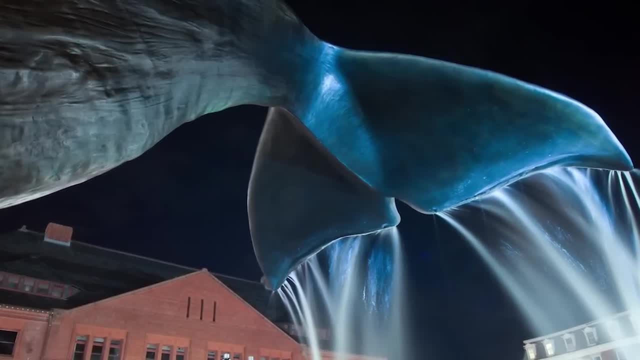 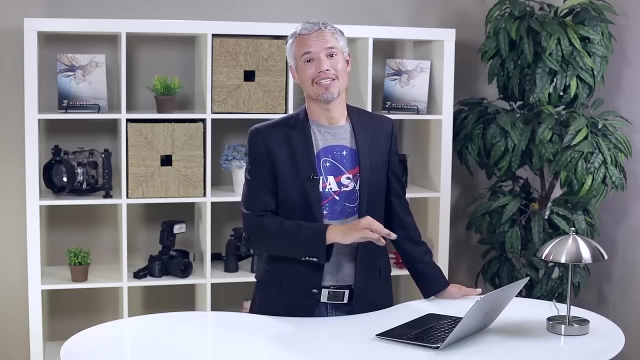 Now, this is an example of light painting. I took an LED flashlight and illuminated the white balance. This is an example of light painting. I took an LED flashlight and illuminated the tail. That LED flashlight has a very blue white balance to it compared to the orange slash. 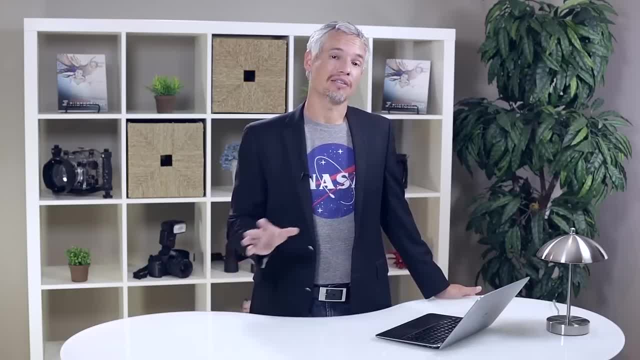 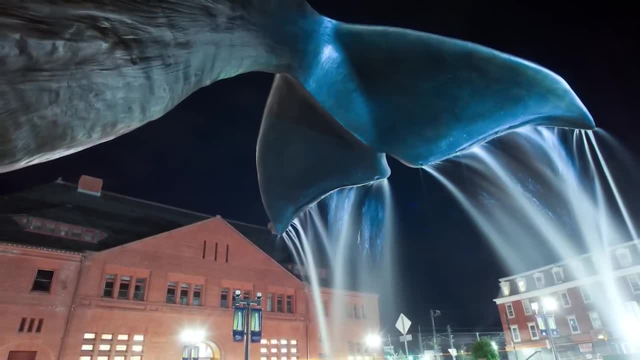 green white balance on the streetlights. So, as you can see, the white balance here is better than in the previous example, But the Whale Tail still has a little bit of a blue tint and the city has a little bit of an orange and green tint. 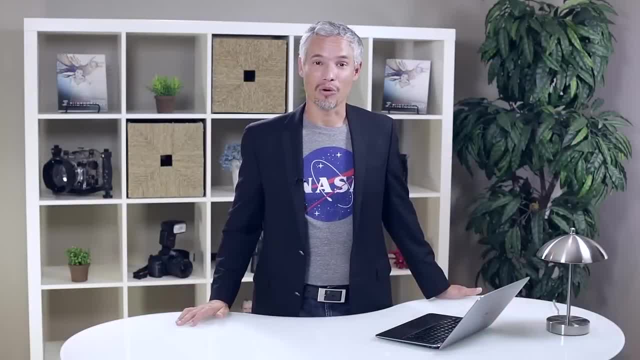 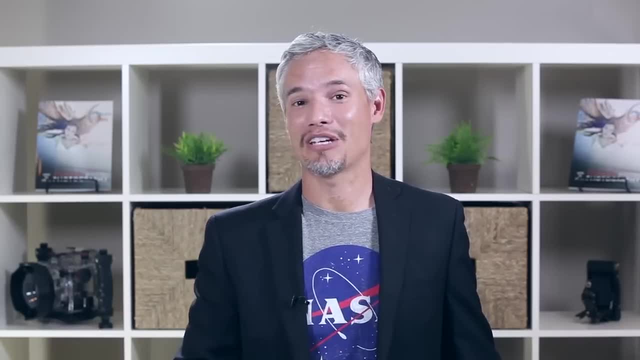 I think it's the best compromise, but you can use your own judgment in your own pictures. Another really easy way to solve the color balance problem is to convert your picture to black and white. Black and white pictures can be very artistic and little differences in color like that. 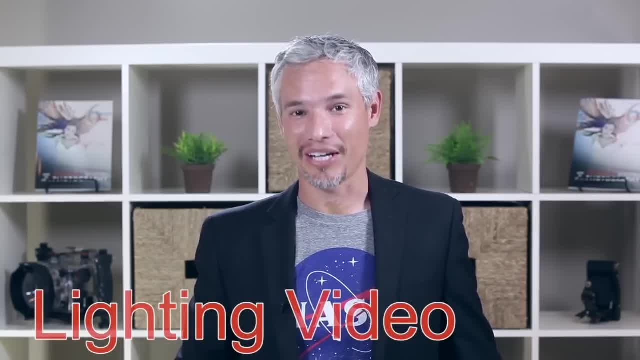 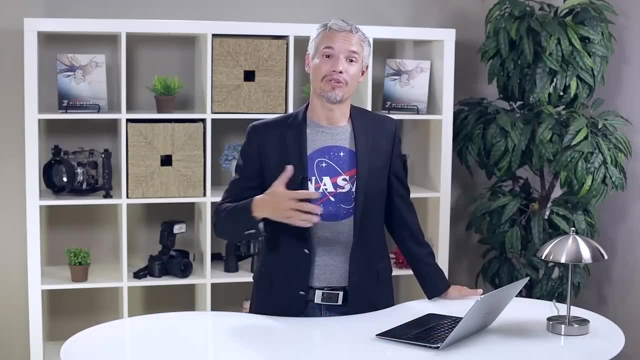 are obviously completely eliminated. So for more information, check out the lighting video. Another common problem is that pictures are washed out. Now, more technically, I would call that a picture with very little contrast. If you look at the histogram, the histogram will look like this: 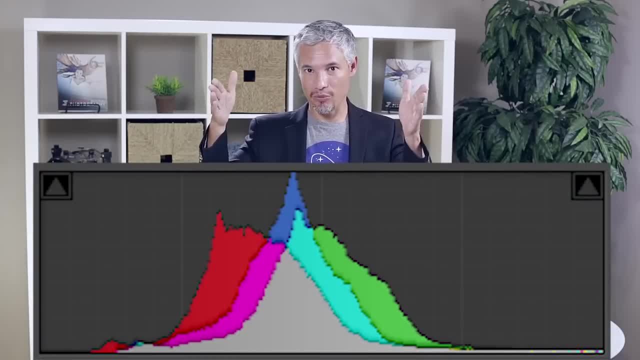 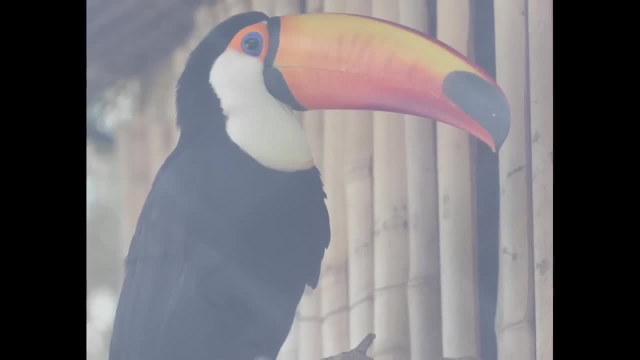 It'll be one big bump in the middle that doesn't come anywhere near reaching the sides of the histogram. So let's look at a sample picture that is washed out. And it is completely washed out because I was shooting through a glass enclosure and the glass was reflecting a bunch of light. 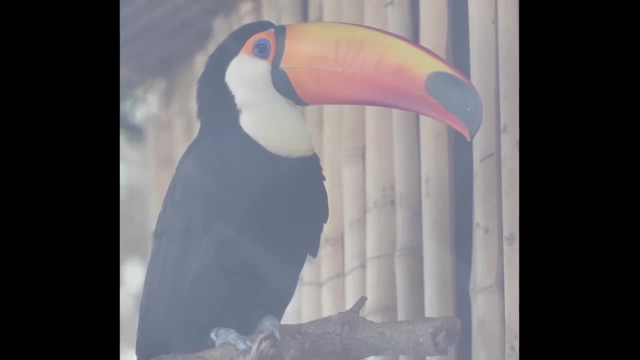 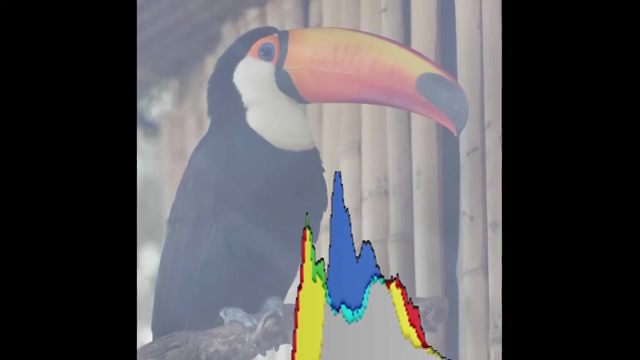 So what happens is that even in the dark parts of the bird, I'm getting a bunch of light bounce back into the camera and it's picking that up And, as a result, this is what the histogram looks like. Now I can improve this in post processing. 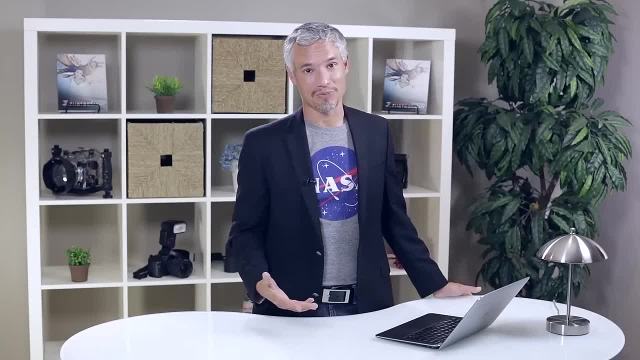 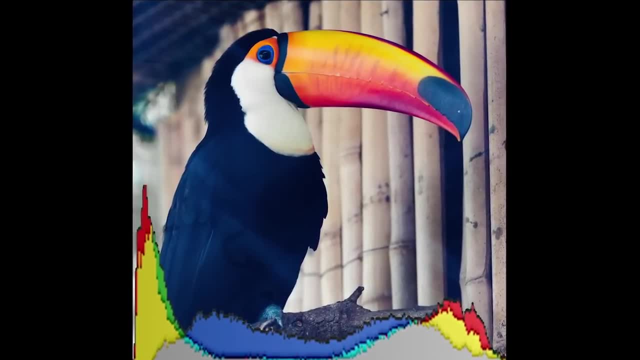 Of course, at the time I was taking a picture, the best thing to do would be to get rid of the glass, but I don't think the zookeepers would have liked that. So instead I brought it into Lightroom and adjusted the black point and the white point. 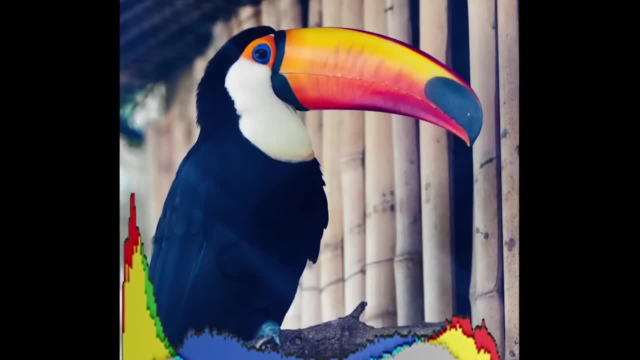 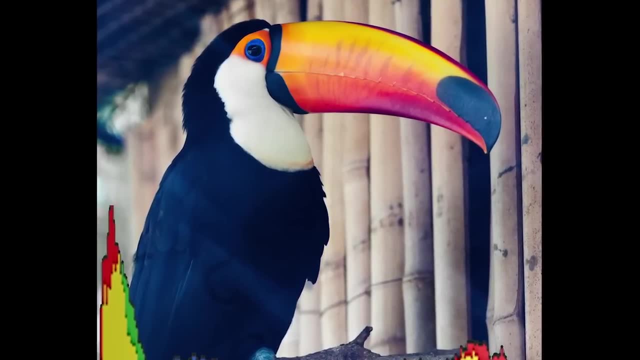 To get the best compromise. Now it's still not a perfect picture. Anytime you have to do that much post processing, it's not going to be great, But you can see the histogram is more spread across the entire frame and the bird does. 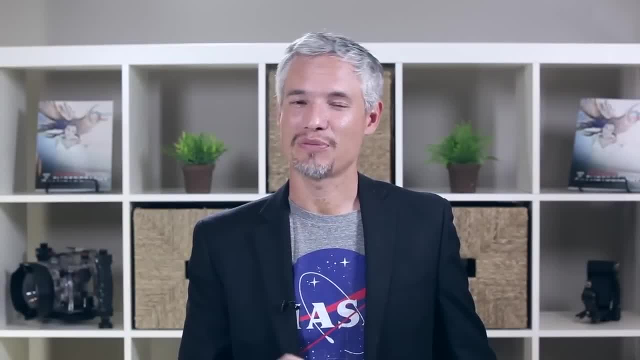 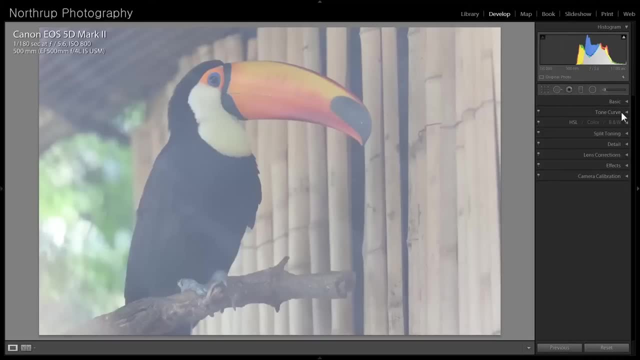 look much better. This is a really easy change to make, So let's spend just a second in Lightroom and I'll show you how to make that same adjustment. I'm demonstrating Adobe Lightroom, but the free Google Picasa has all these same features. 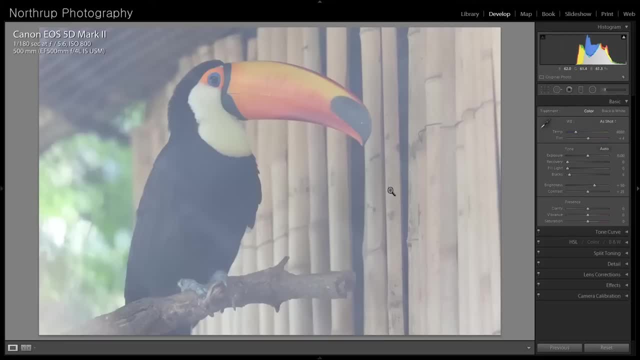 I'll expand the basic panel here which allows me to adjust The exposure and the contrast and common things like that. And where I usually start is by adjusting the exposure so that the widest parts of my subject are pretty close to the right side of the histogram here. 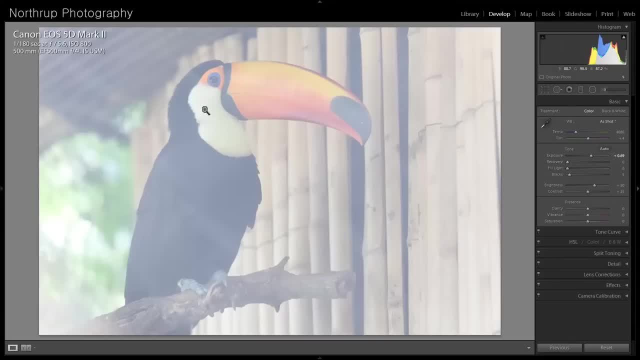 This visually represents the brightness of the photo and this is the widest part of the subject. So I want to make sure that it's right about 100% white. If you look at the histogram here, we see we have big open space here. 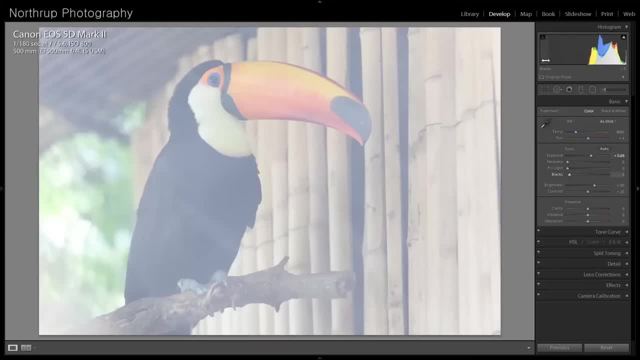 The whole left half of the histogram is blank. There's no information in there And that's why it looks all washy. It's all washed out. Everything's in this right side of the histogram. So to fix that I can drag the blacks up. 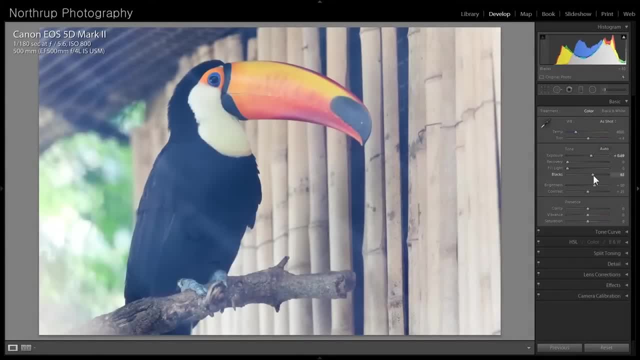 And you can see that histogram moving to the left and the picture is looking better and better and better. The blacks slider basically defines where the left side of the histogram is going to be, So I'm really just squeezing everything in from the left side which spreads the rest. 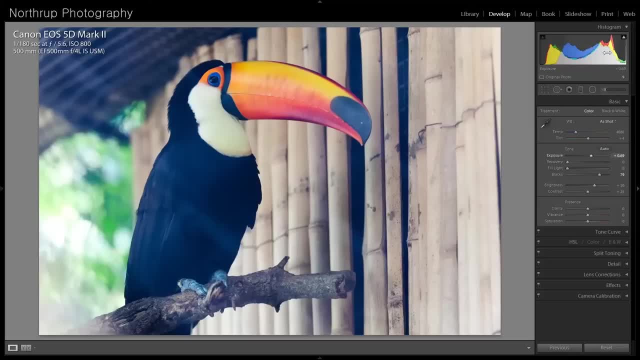 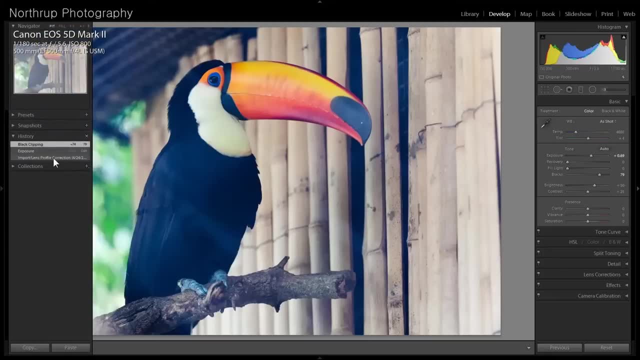 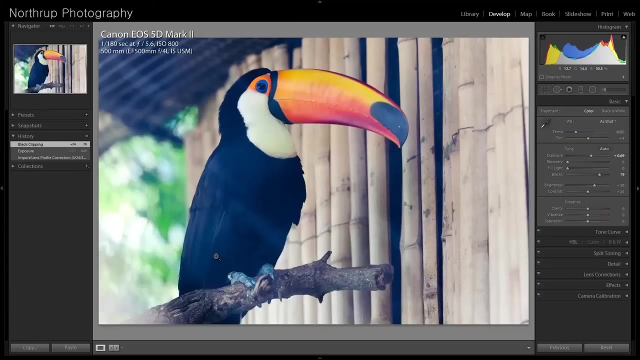 of the information out over the entire histogram instead of just that right half, And we can see that we have a much nicer looking picture than we started with. Just to go back to the original import, that's before and this is after. This would be a much better looking picture if I hadn't had to shoot through the glass. 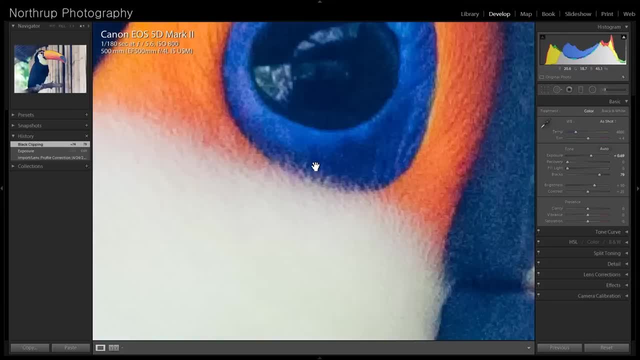 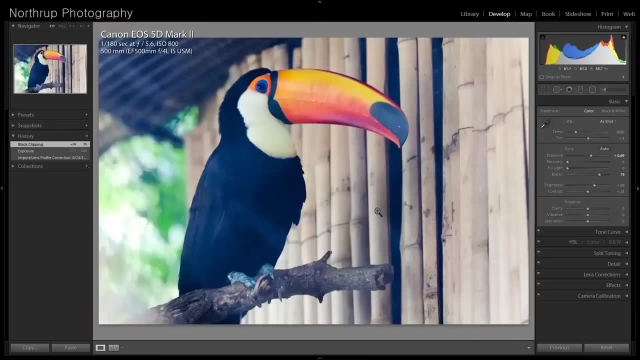 but sometimes you have to shoot through glass. It's out of zoo And if I zoom way in here, the sharpness is okay. but the sharpness would certainly be much better if the glass hadn't been in the way, because a little contrast situation like 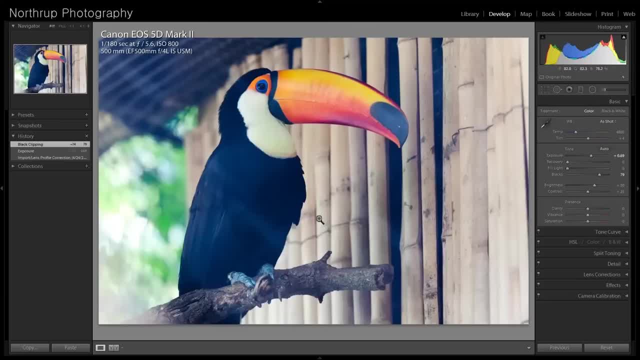 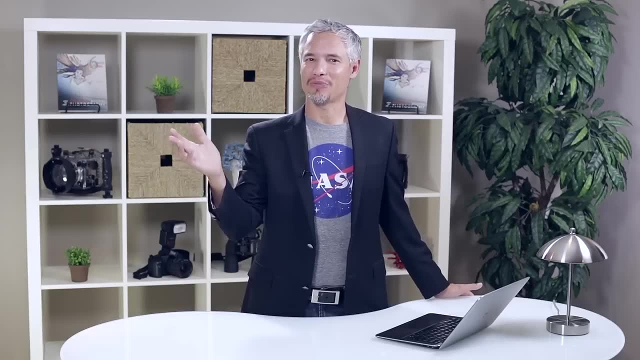 that definitely overall reduces sharpness. Okay, So avoid it when you can and when you can't know that, you can improve it with post-processing. Another common question I get is why does my picture have these weird like blue and green edges? 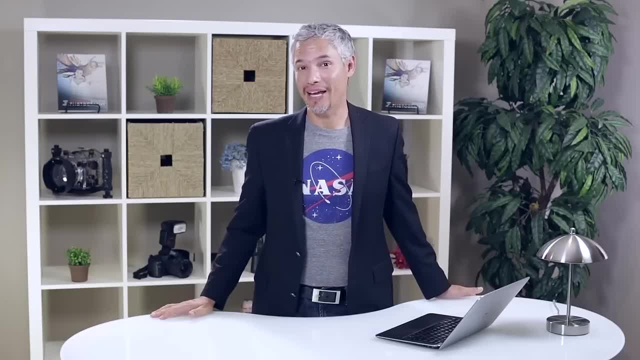 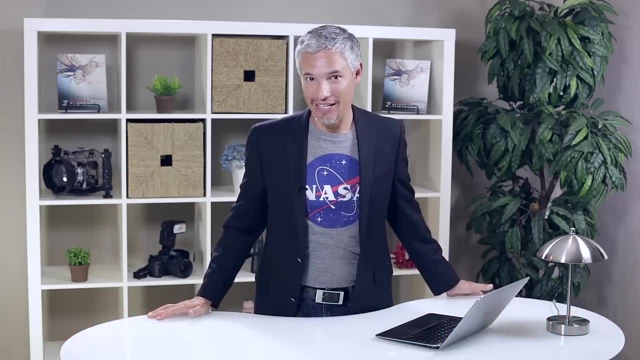 Sometimes they're red or yellow edges. This is a condition called chromatic aberration, and it's another thing that we're not going to get rid of because it is a property of the physics of light. It has to do with the behavior of photons as they pass through your lens. 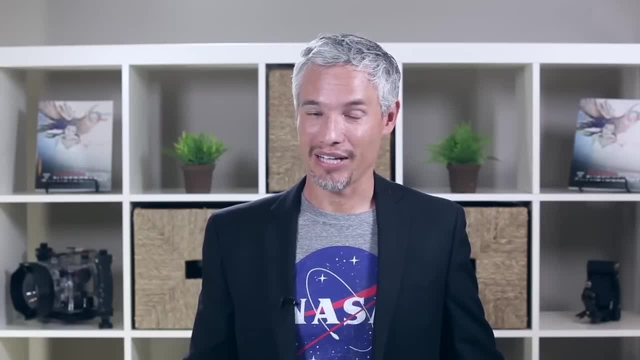 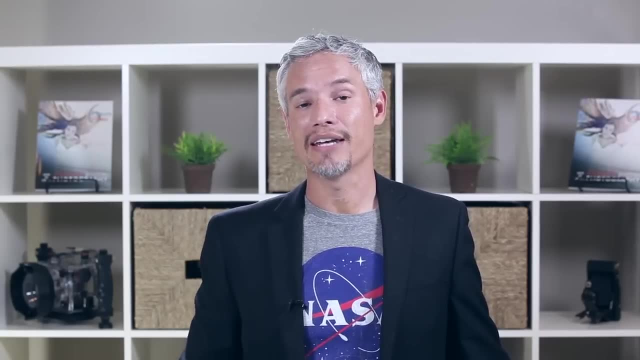 Photons of different wavelengths have different properties as they travel through the glass. So what will happen is some of the blue photons will creep into a dark area of the picture, or some of the green photons will creep in and at areas of contrast between very bright 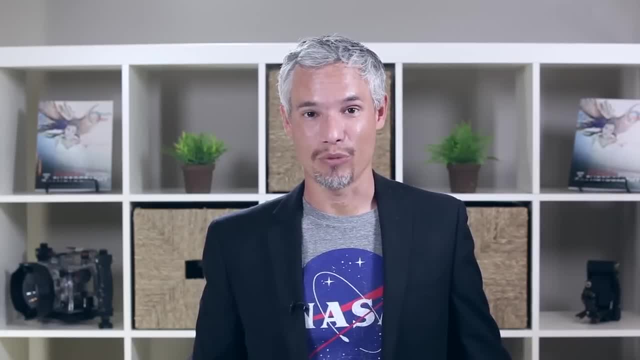 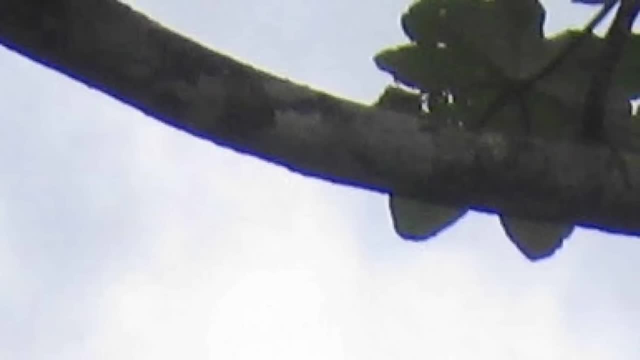 and very dark, we'll get this fringing. Let's look at an example. This is an extreme closeup of a branch against the white sky And even though this is taken with high quality professional camera and lens, you can see these like deep, disturbing blue lines along the edge of it. 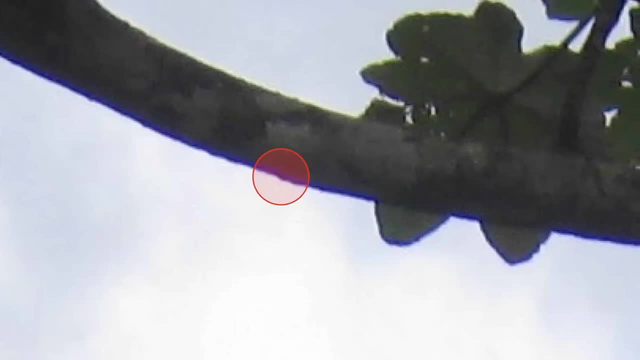 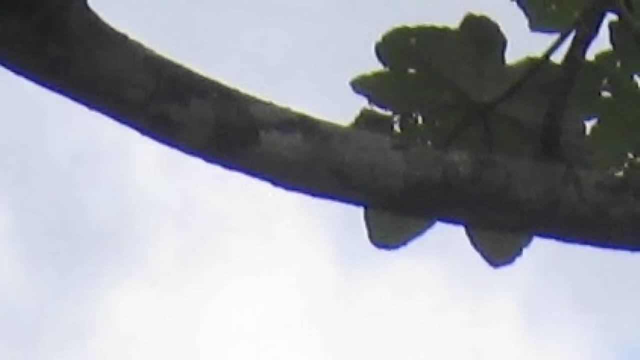 And, like I said, no camera lens can fix this. This is just how light it is. Light works. However, you can fix it in post-processing. If you look in Lightroom or Picasa, you'll see little sliders for helping to fix chromatic. 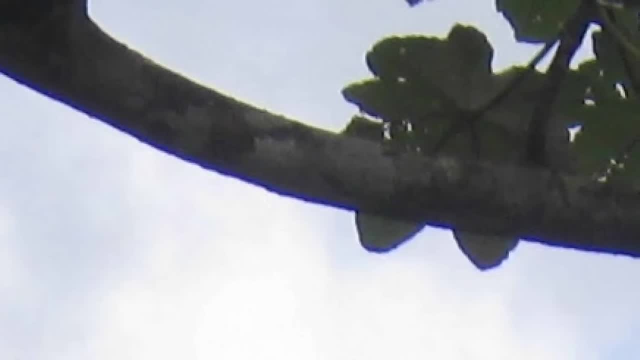 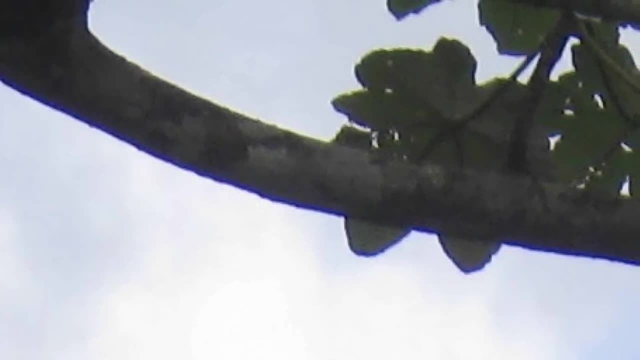 aberration, and none of them are perfect, But play with them. It's different for every picture and often you can significantly reduce them Again. you can always go to black and white and it will eliminate it completely. Now let's talk about how to solve dust spots. 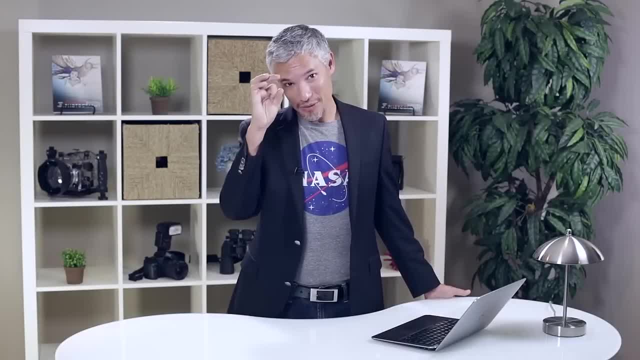 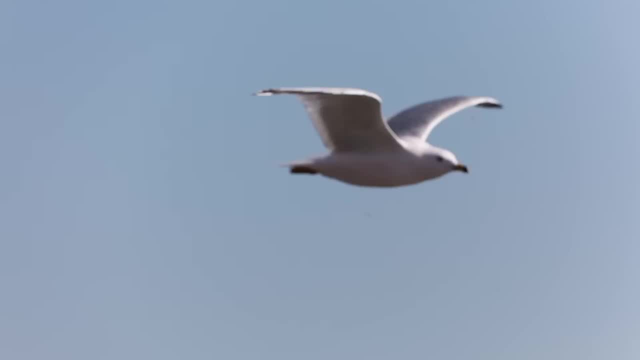 If you ever see like a weird kind of shady area, a little spot on your camera, well, most people think that's something on the front, Because that's the part of the camera that you can most easily see, right, But usually it's a spot of dust or hair or something else on your camera's sensor. 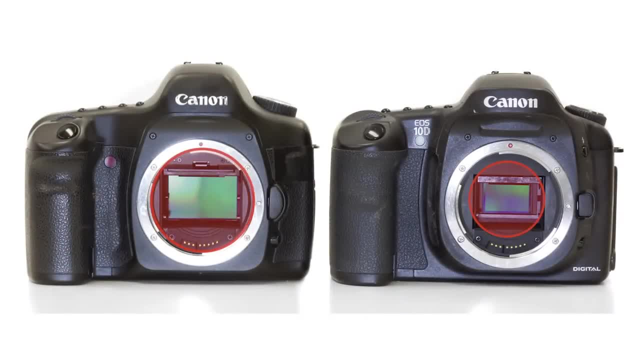 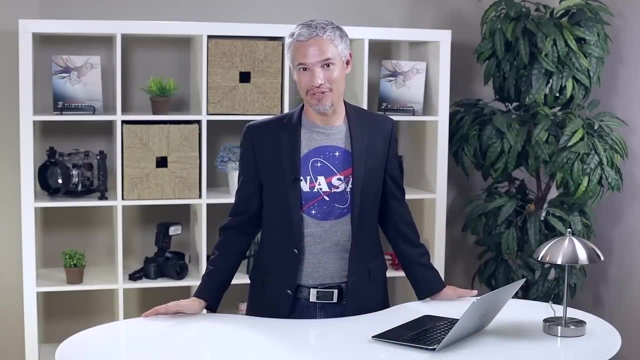 The sensor is, of course, hidden behind your lens and you wouldn't think so many things would get attracted to it. But these things get dust on them all the time and they can be a real pain to clean. in post You can go into Lightroom or Picasa or any post-processing tool and just really easily. 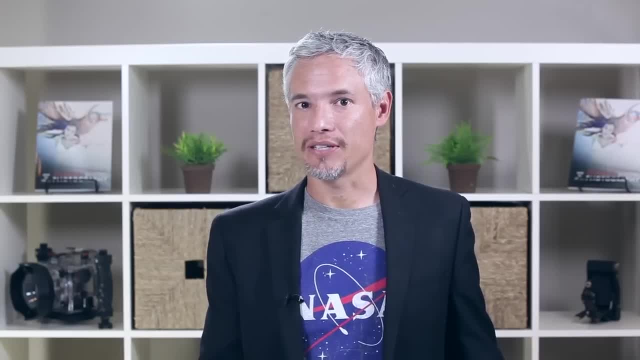 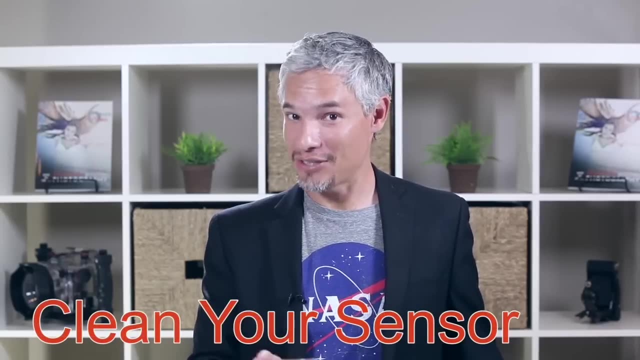 clone over it or use a bandaid or healing tool to fix these problems. But of course, the best way to do it is to actually clean your camera's sensor And while I never recommend taking your lens apart or taking your camera apart, this is 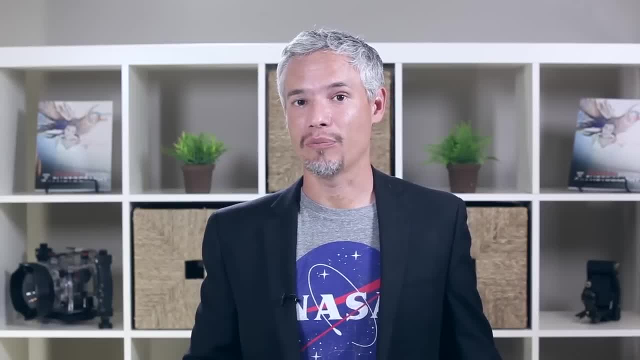 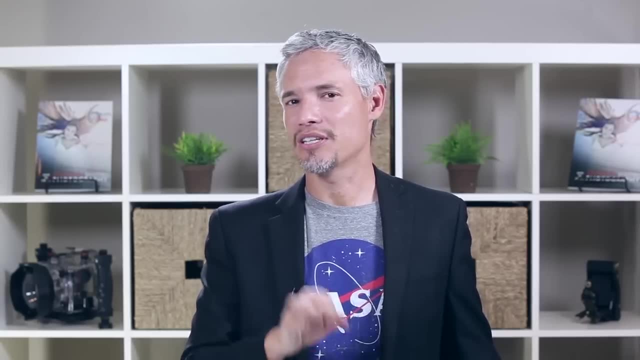 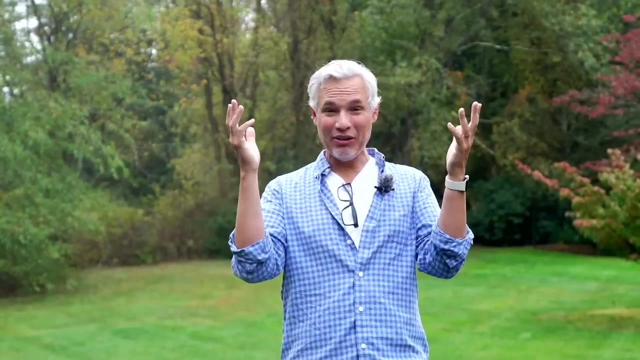 something you can do yourself at home and save yourself a lot of money. So let's head upstairs into my kitchen and I'll show you exactly how to clean your own sensor using the tools that I've found work best: Sensor and lens. dust can ruin your pictures, require post-processing or just completely. 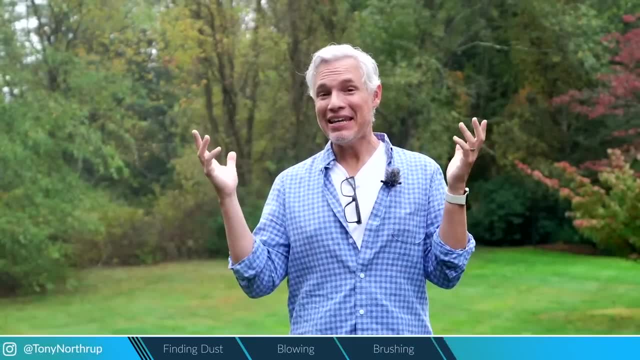 ruin your video, And it happens all the time. In fact, this scene is one of them, So let's take a look. This scene is filled with sensor and lens dust. If you can't see it, it might be hiding in the background. blur. 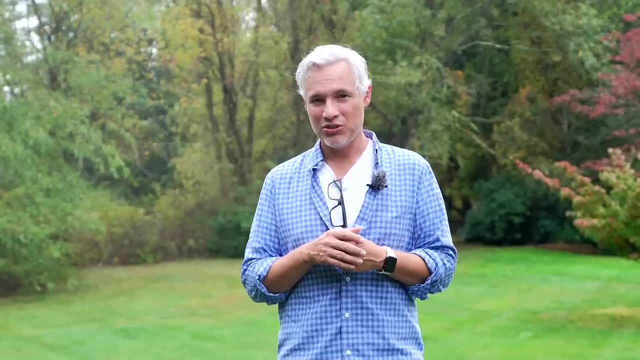 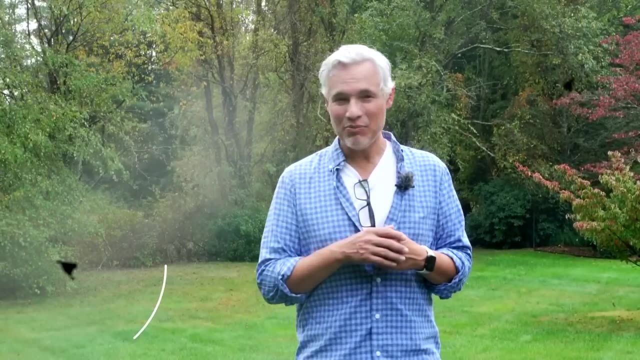 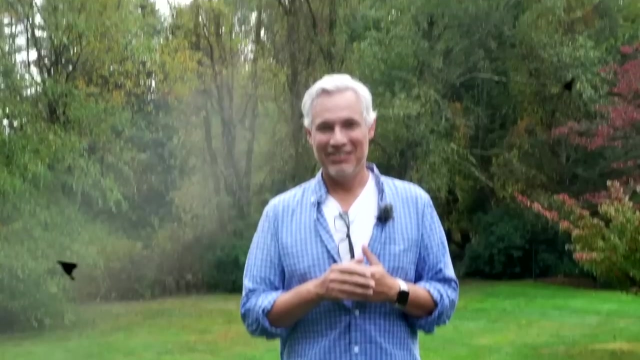 So, Chelsea, raise the f-stop up to f22 so we can see some of the hiding dust. And if you still can't see it, maybe it's hiding in all this detail in the scene. So let's pan up to the empty gray sky. 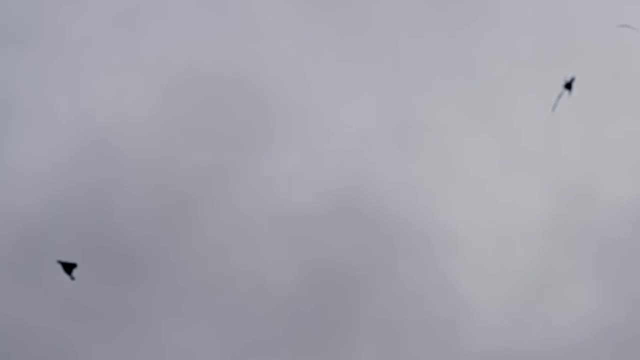 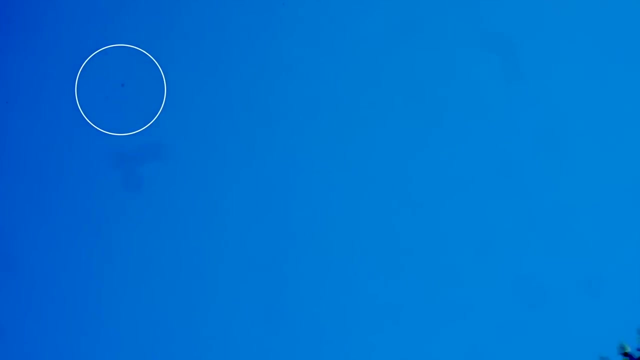 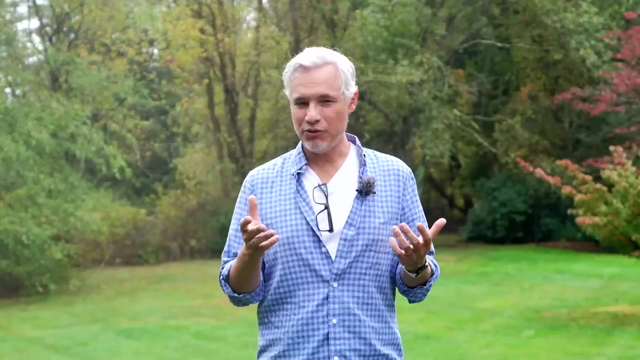 I bet you can see some more of it now. right, If you want to distinguish between sensor and lens dust, try zooming your lens. The sensor dust stays in one place while the lens dust moves in and out. You might also see spots in the viewfinder that don't appear in your final photos. 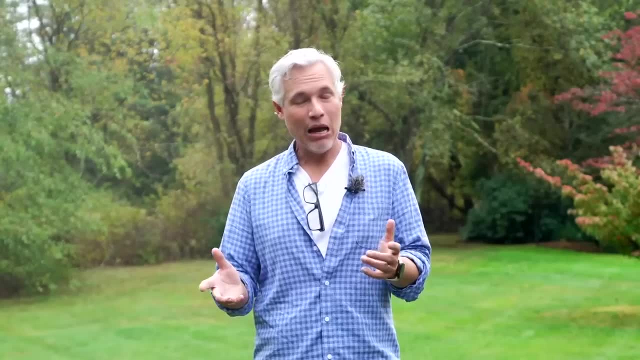 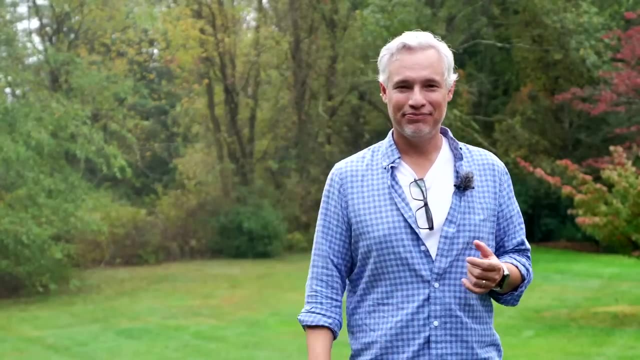 And that can be in several different places depending on the type of camera you have. I'm going to show you how to clean all of that quickly, easily, inexpensively, at home. So let's go inside. My first step is to bring my dirty camera into a dim room. 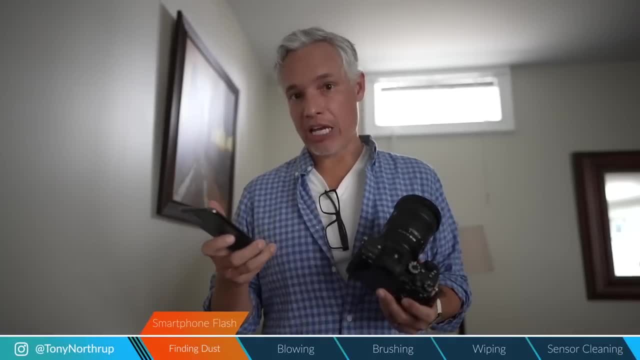 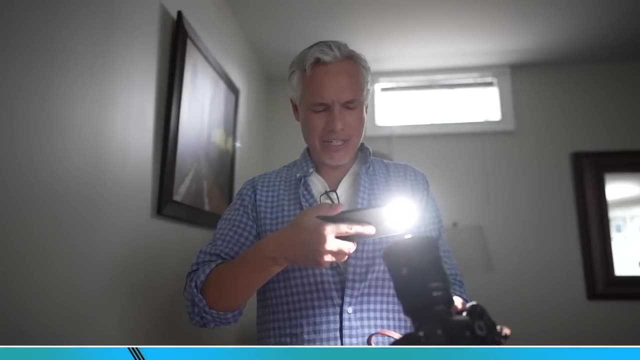 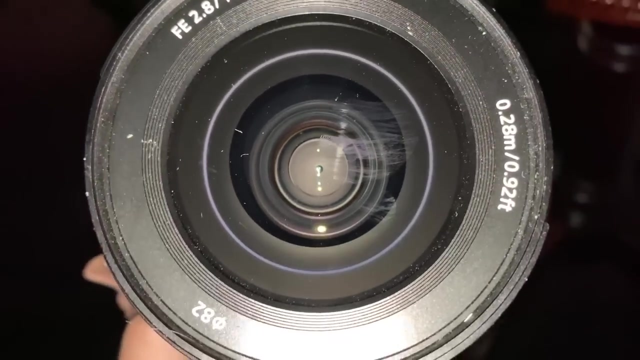 Put my smartphone into video mode, turn the flash on and then start recording. Now, if I look at the camera itself, all that dust and dirt and every smear suddenly glows in the light of the smartphone flash. I'll look at the front element and then I'll also look right in the viewfinder. 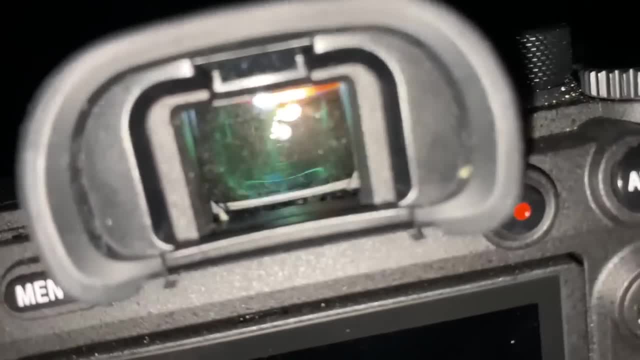 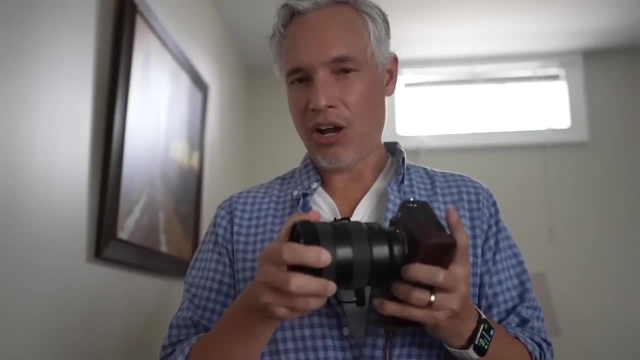 And this sort of tells me exactly where the problem areas are. So I know what I need to do. I need to pay attention to during the cleaning process. Don't forget to take the lens off and inspect both the back of the lens and the sensor itself. 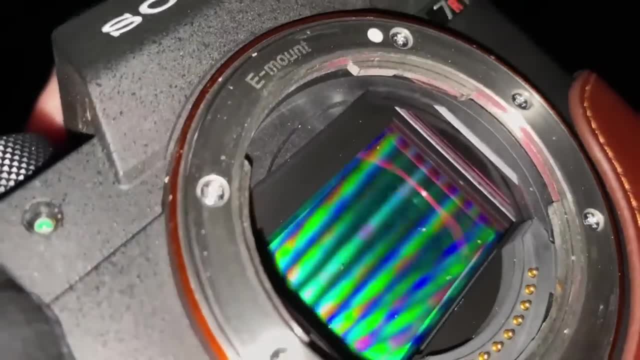 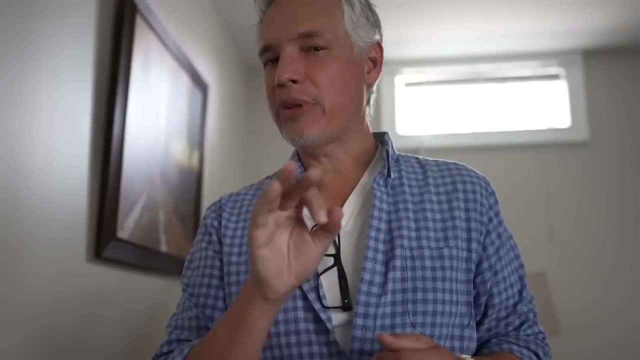 In front of all those pretty colors, you can actually see a ton of dust if you turn the camera at an angle. I'm going to pay attention to each of the four corners, especially If you have a DSLR. there's something else you should take a look at. 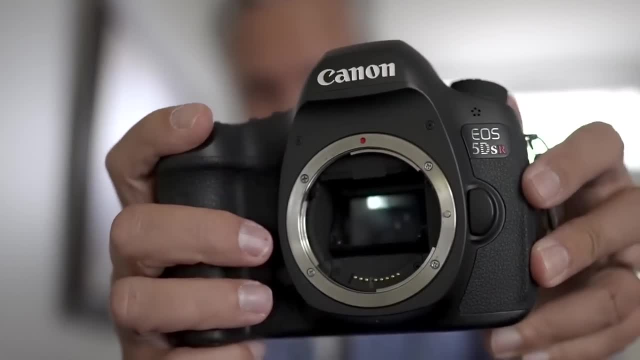 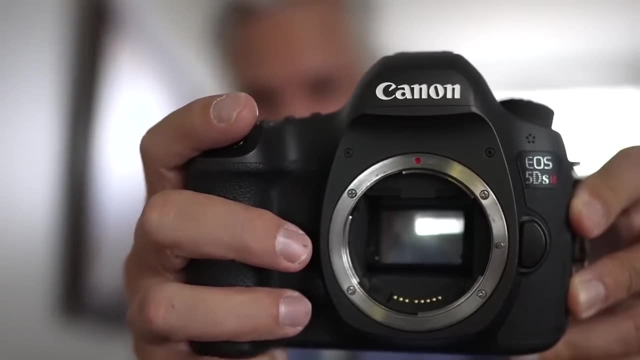 Let me, let me grab one. This is my Canon 5 DSR. It's a DSLR. Note that it has a mirror there. I see it flip up and flip down as I put it into live view. The presence of that mirror is why they call mirrorless cameras mirrorless, because they 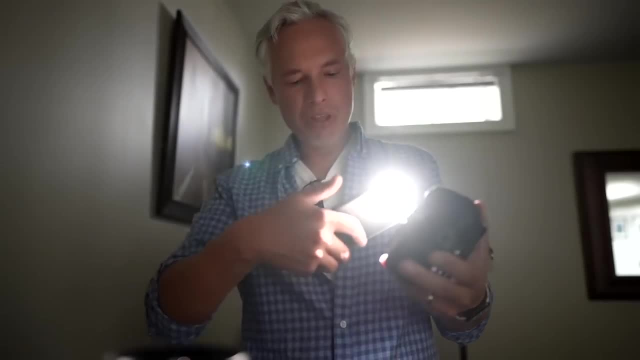 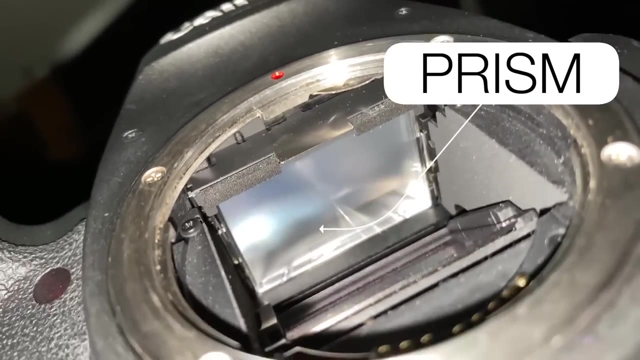 don't have it, But DSLRs do With the DSLR. I'm also going to look with the mirror. down at the mirror, That's a lot of dust, And then also at the prism, because dust gets stuck on the bottom of the prism. 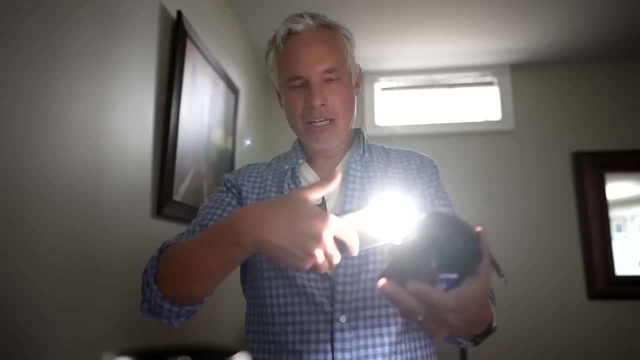 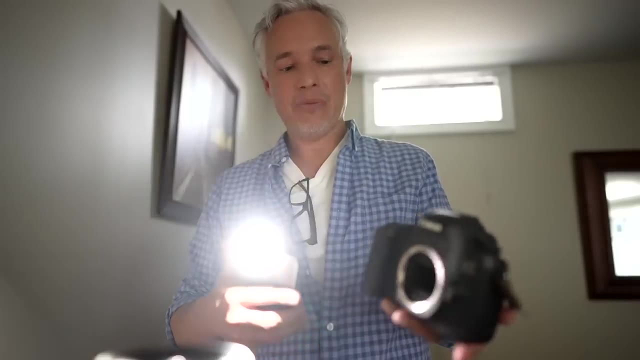 And you can see that in the viewfinder, even though it does not show up in your pictures. And, of course, with the DSLR, if you want to look at the sensor, you can put it into live view mode or go into the menus and put it into sensor cleaning mode, especially with 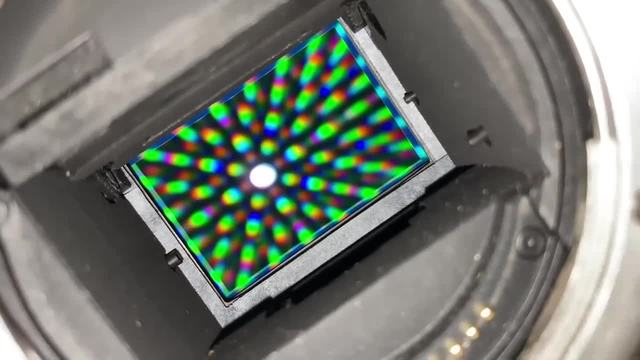 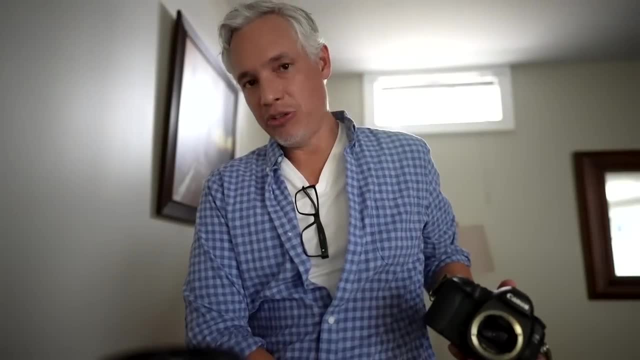 the DSLR, You might not actually see any dust on the sensor because that mirror is almost always flipped down over it, protecting it from dust. It's just one of the ways that DSLRs are a little easier to maintain than mirrorless cameras work. 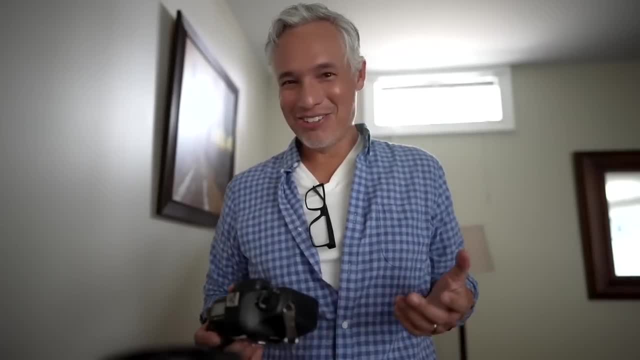 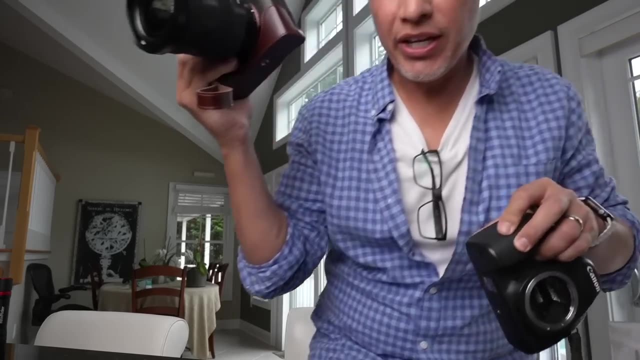 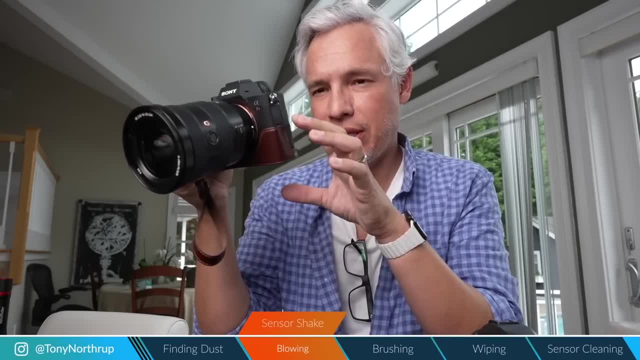 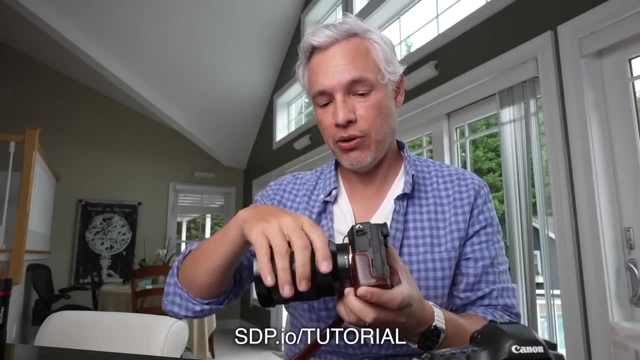 You want to go from low impact to high impact, So we're going to start by using the cameras built in sensor cleaning algorithm, which you'll find somewhere in the menu system. If you aren't sure what it is on your camera, check our free tutorials here. 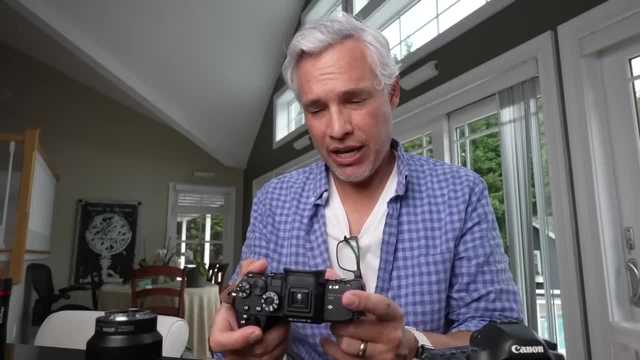 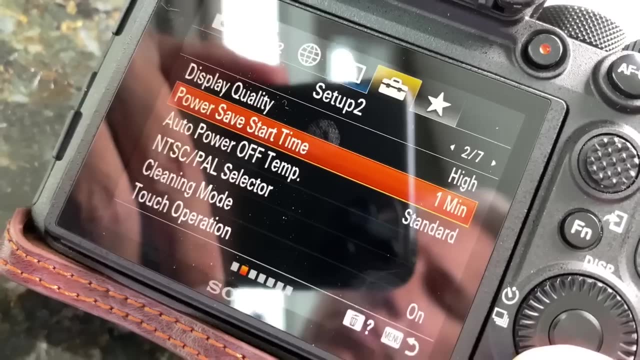 What I usually do is turn the camera upside down, take the lens off. This way, gravity is kind of working with us. If it happens to shake loose any dust, some of it will at least go down, even though it's not necessarily heavier than air. 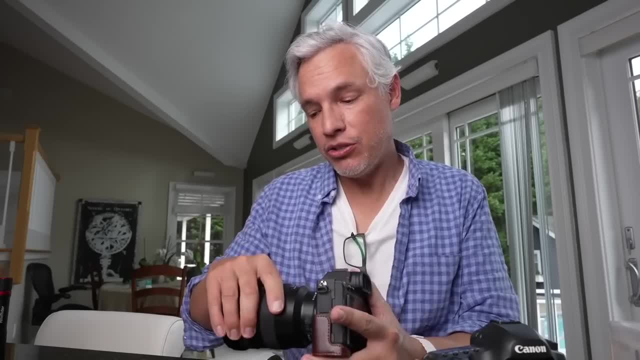 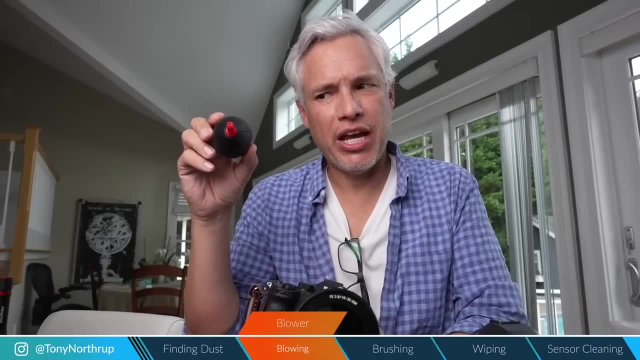 Then turn your camera off For now. I'm going to put the lens back on to do the next stage of cleaning. For this you'll need some kind of blower. A blower simply pushes air And you can imagine that might be a little dangerous because the air might have dust. 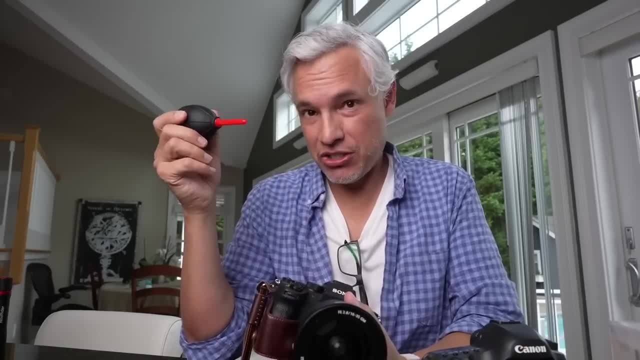 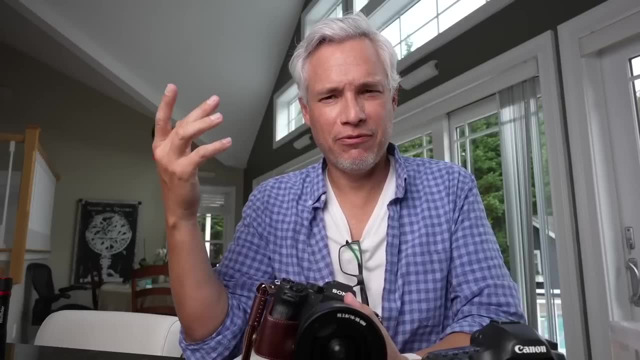 or some kind of contaminant in it, and you might actually be projecting dust onto the area that you're trying to clean, And that's why it's important not to just use whatever cheap blower you happen to get free with your camera And instead pick up a high quality product. 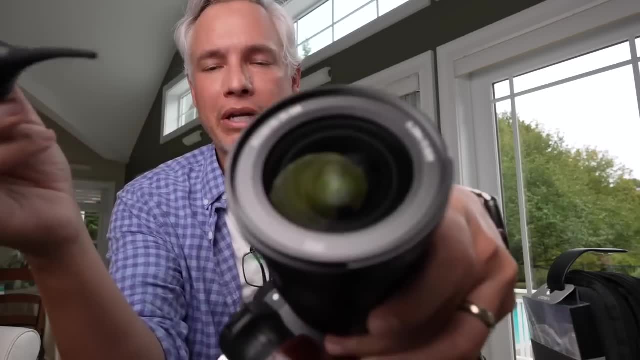 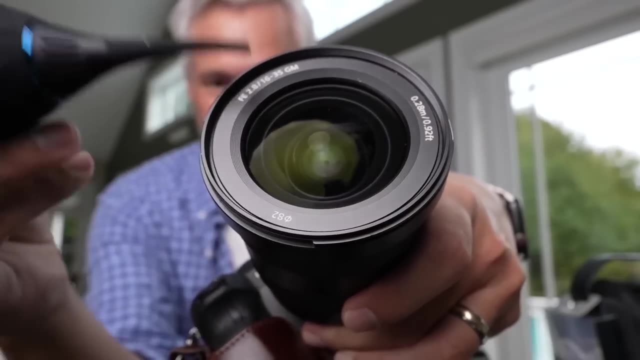 The first thing I'm going to do is actually use a blower to clean the big dust off of the front element here. Just do it like that and you should see some dust blow away. Then I'm going to repeat that process on the viewfinder and I'm going to take the lens. 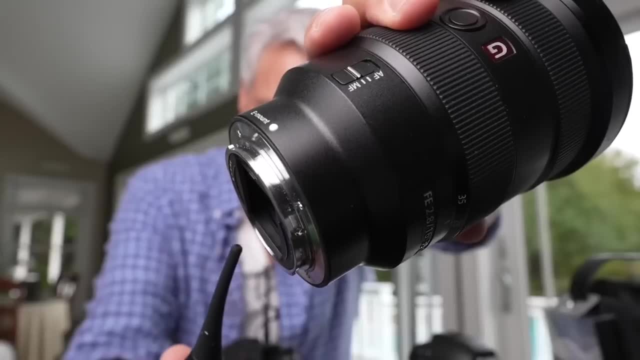 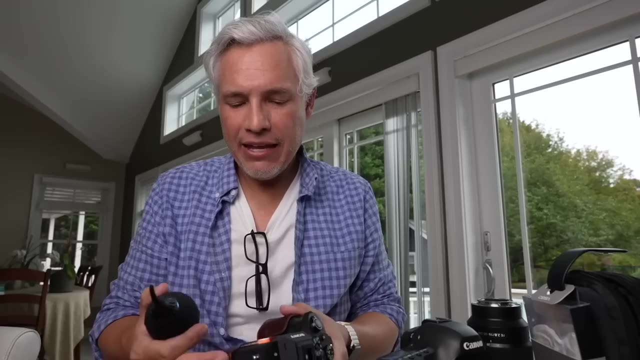 off and get the back element here. I'm going to try to use gravity to help me here by turning the lens upside down and blowing in there just as much as I can. If I still see dust on the sensor here, I'm going to turn the lens upside down and blow in there just as much as I can. 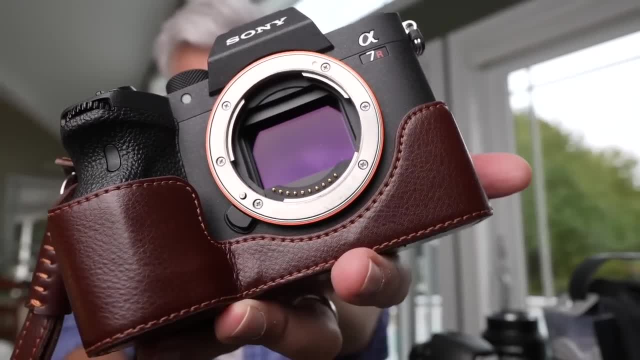 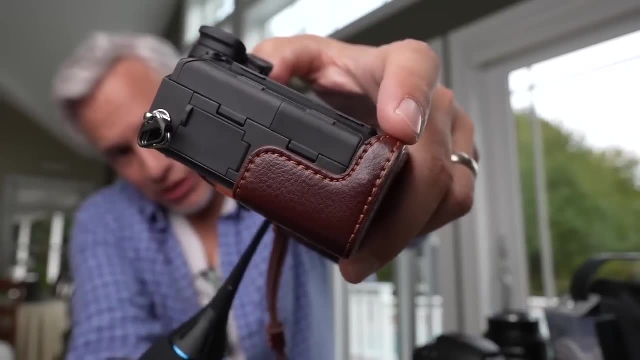 If I still see dust on the sensor here, Then I'm also going to use the blower on the sensor itself. Once again, I'm going to do this by turning it upside down so that gravity works with me as much as possible, and then blowing this in there, hitting it as much as I can from. 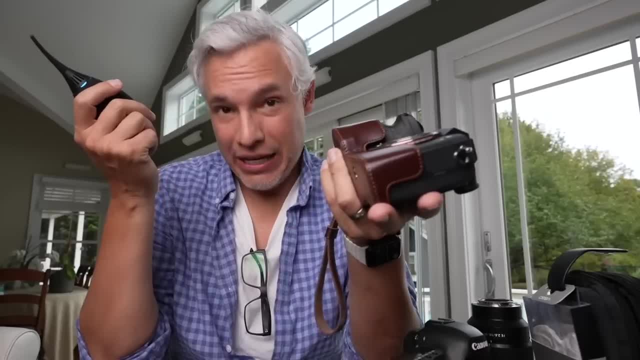 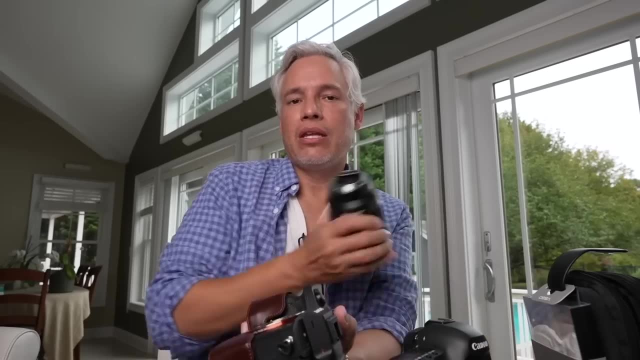 the side. At a glance I can see I got rid of like 90% of the dust, but I do still see a speck, So I can see we're going to need to get a little more intense. with that, The next step. I'm just going to replace my lens here so I don't expose the sensor too. 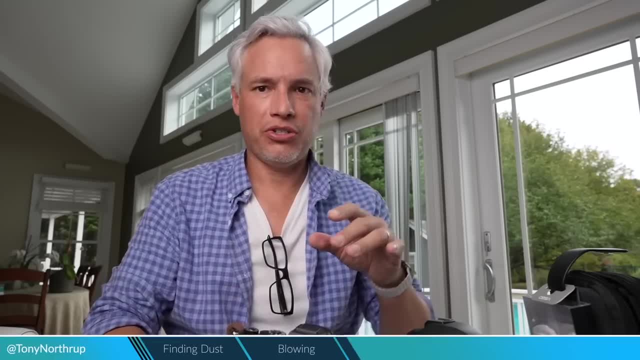 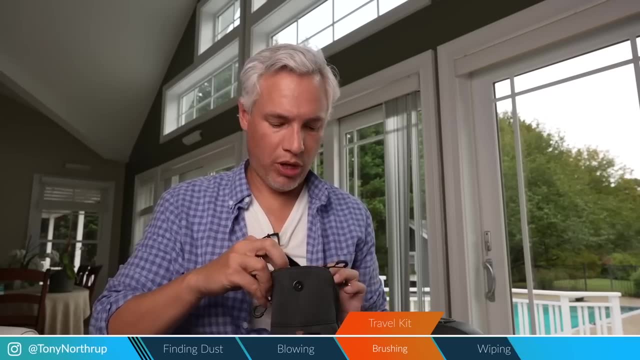 much. I'm going to go to a brush, So I have a couple of brushes to show too. This travel camera cleaning kit that VSGO sent does have a nice little portable brush inside of it, because when you're in the middle of a trip you don't want half your pictures. 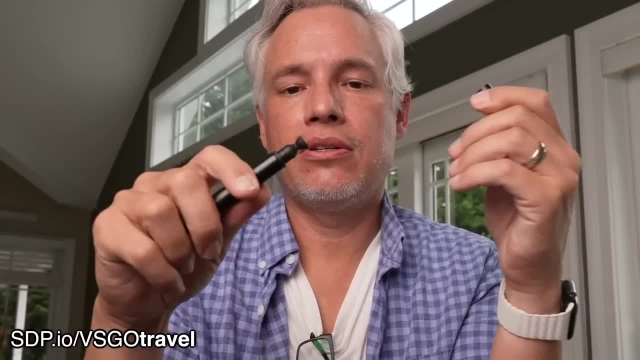 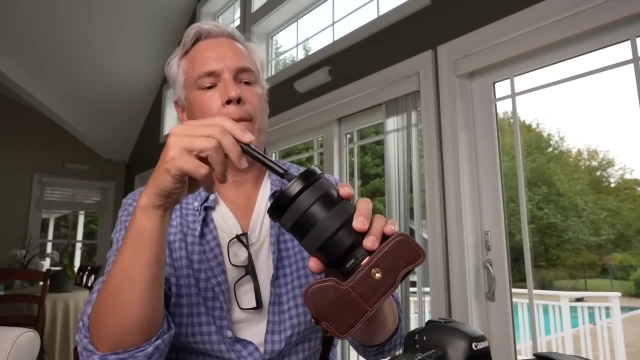 to end up dirty. So it really is important to travel with something And you can see it has a swab, and then I can also extend a little brush like this. This is really useful for getting out bigger particles that the blower didn't get. 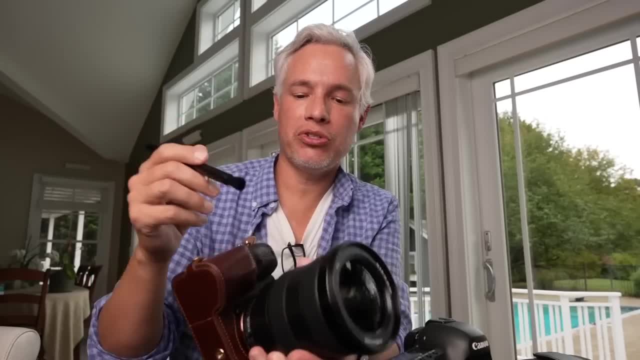 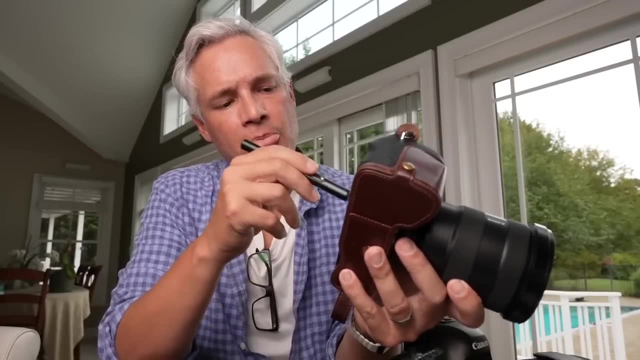 And you know, rather than just kind of randomly swabbing around, I'm actually going to look for visible dust that remains and try to get in there and selectively remove it. And again, if you have trouble seeing it with your naked eye, then go into a dark room and 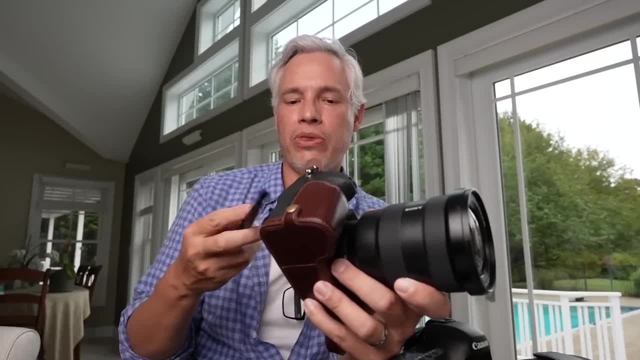 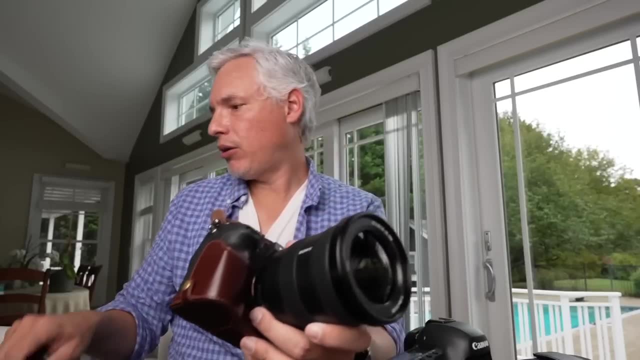 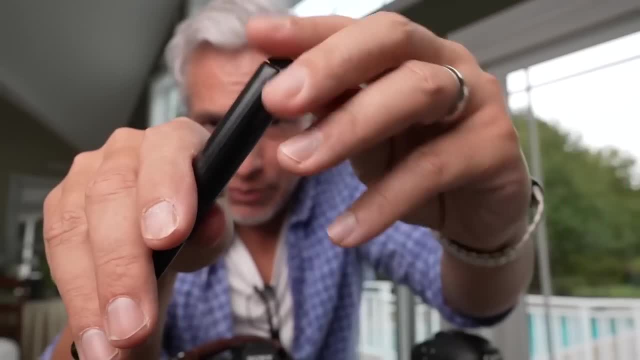 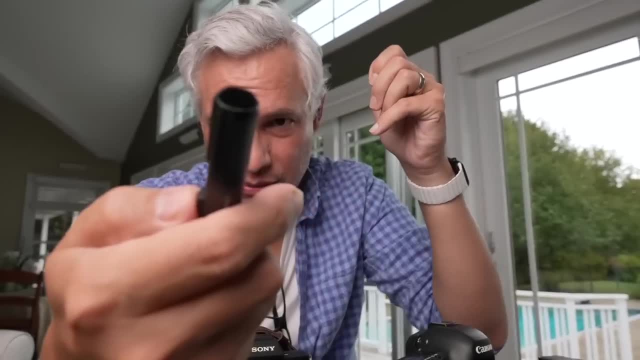 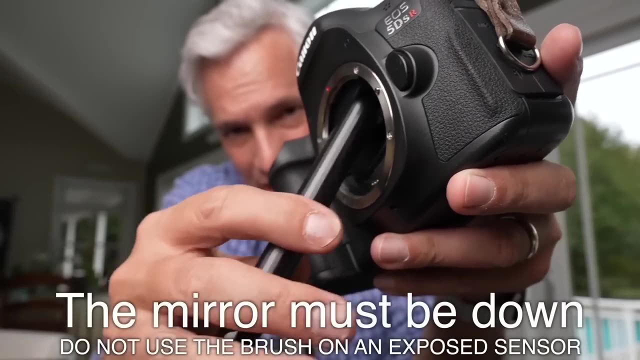 it's not in use. Let's take that cap off and then we can slide to extend the bristles here. If you have a DSLR, be sure you get in there and clean the dust off of the prism at the top of the camera and the mirror- just anything that you could see. 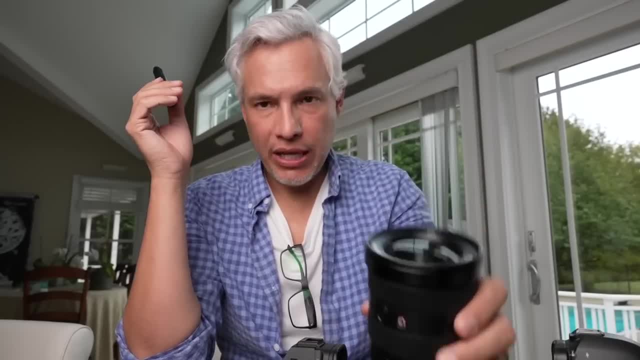 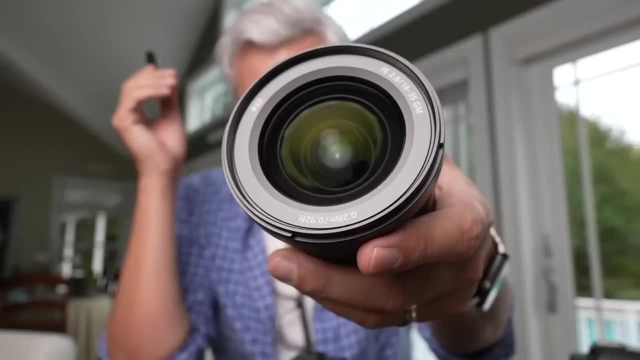 So far everything has been very low-contact, but I still see a smudge on this lens. I don't know if you can see it there. it's definitely there and i'm just gonna have to rub to get rid of that. but i'm not gonna like. 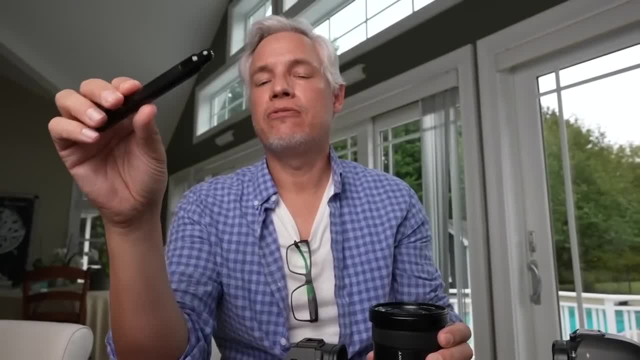 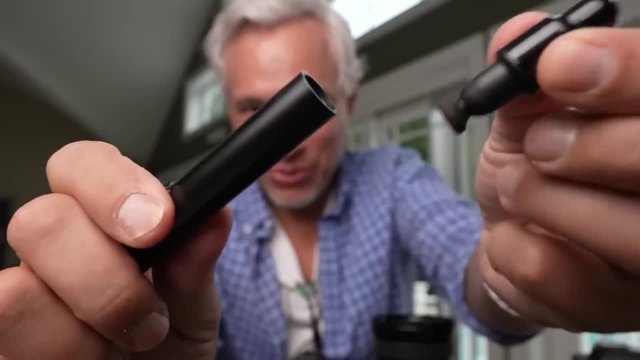 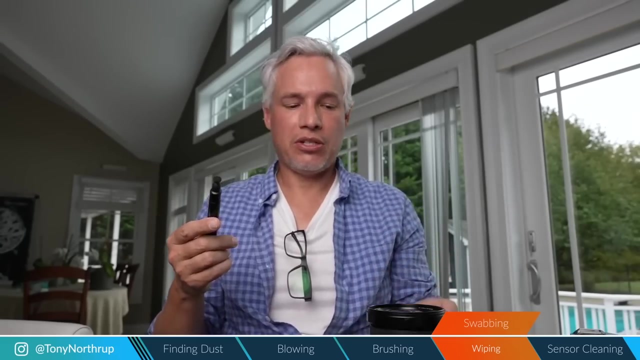 breathe on it and use my t-shirt on it. instead, i'm going to use the flip side of this vsgo power switch. it's magnetic, so i can pull this out and flip it around, and now you see a little swab there. that flipping action makes sure that it's protected all the time, so i wouldn't don't use. 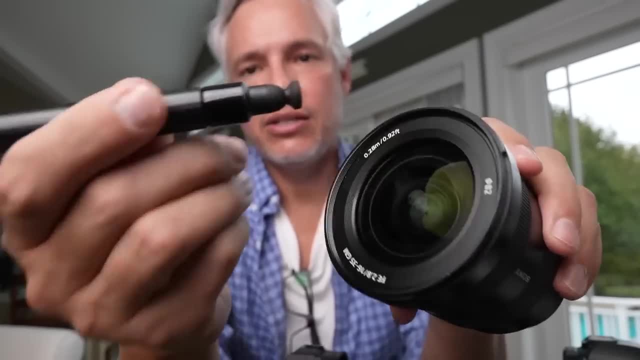 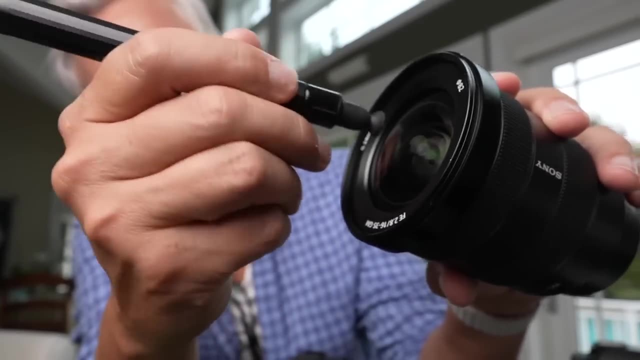 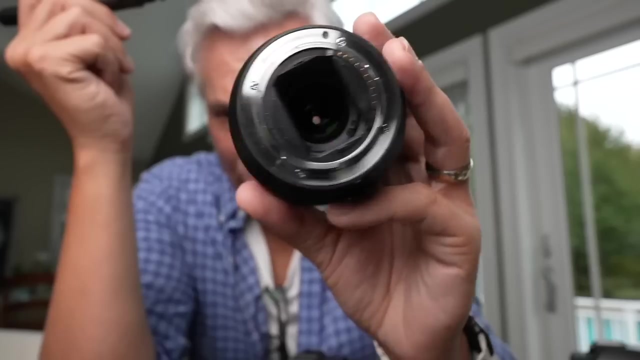 this on a sensor. this is for, like, cleaning lenses and stuff, and what i'm going to do is to put this in the middle of the lens and just gently push out, while my own experimentation produced better results moving from the inside out. vsgo recommends using a circular motion, the back element of your 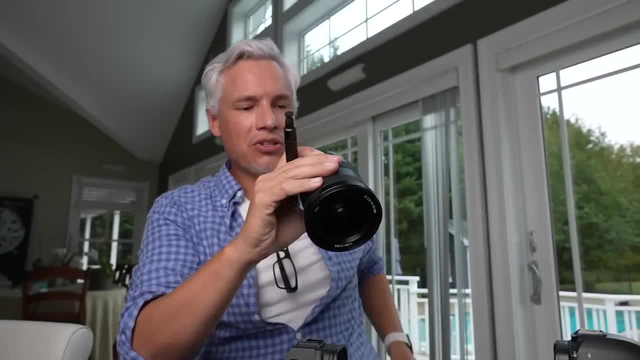 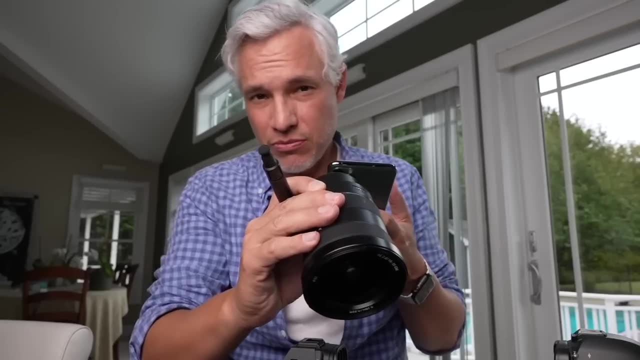 lens might also need something like that. so it's a good time to pull out your smartphone flashlight again and really just look in there and see if anything is catching your eyes, because if there is nothing you can see, then don't do it. my back element is good, so i don't need to get in there and to help protect. 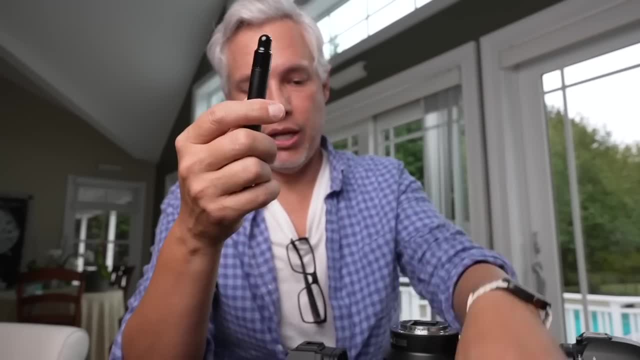 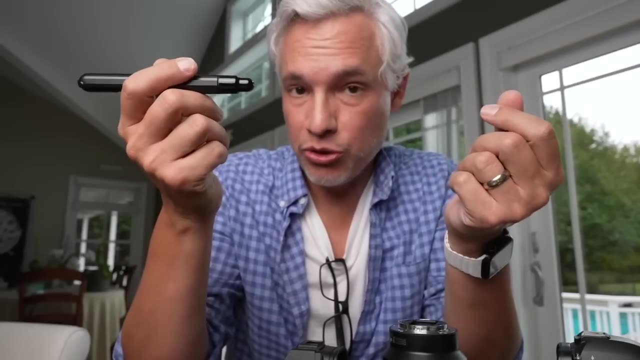 this. i can flip it around and let it get pulled back in there, but it also comes with replacement tabs. problem is: any cleaning product can pick up little abrasives. that's what they're supposed to do. but if you were to continue to use it, then those abrasives could scratch the elements or 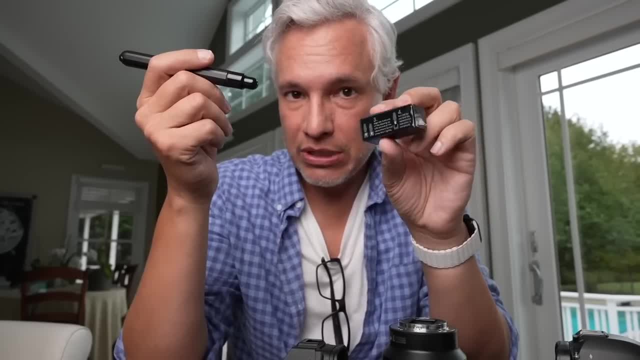 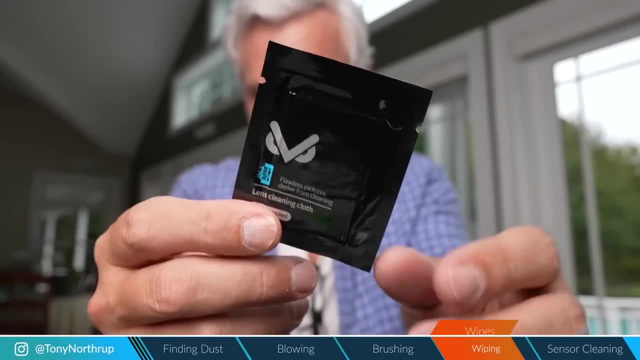 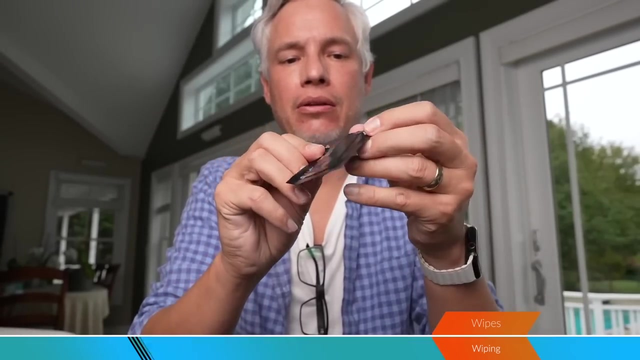 remove some of the coatings, and so that's why regularly replacing the tips or anything that's touching delegate camera stuff is really, really important. vsgo also makes disposable sealed cloths that are guaranteed clean if you just prefer something a little more compact instead of carrying a pen. these are one-time use. 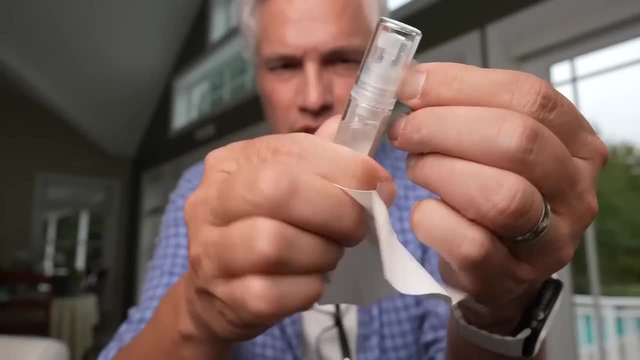 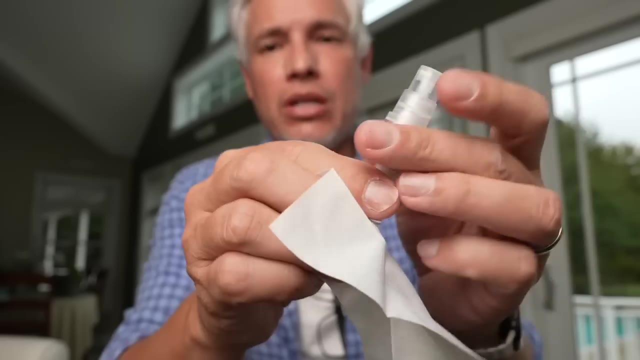 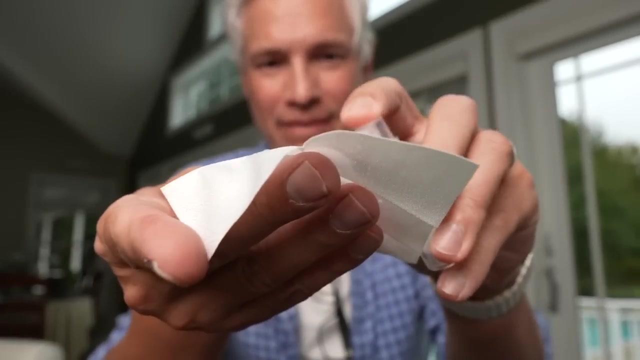 so use them, throw them away. you can use their cleaning spray. don't spray this on the lens itself, but instead put just a little dab onto the cloth to moisturize it and this helps remove the excess oil from your skin for cleaning the mirror and prism. it's kind of hard to get in there with. 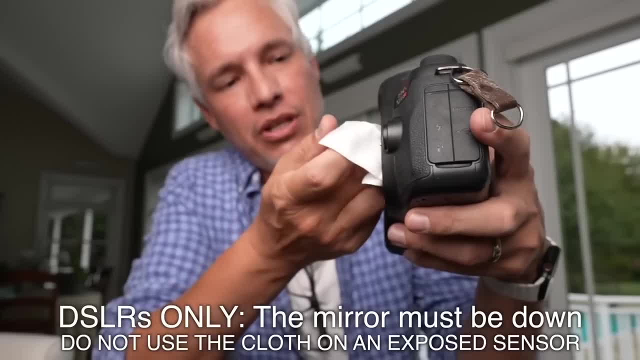 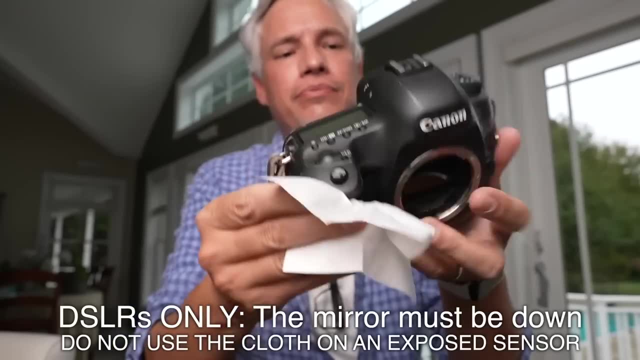 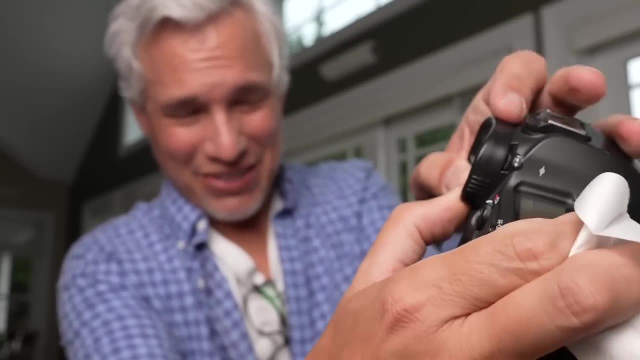 pens so you could use a swab or just a cloth with your finger. it's crucial that you are delicate with these internal components, because any misalignment could alter your autofocusing for the worse. this is also an excellent way to clean the viewfinder: pop the eye piece off it. 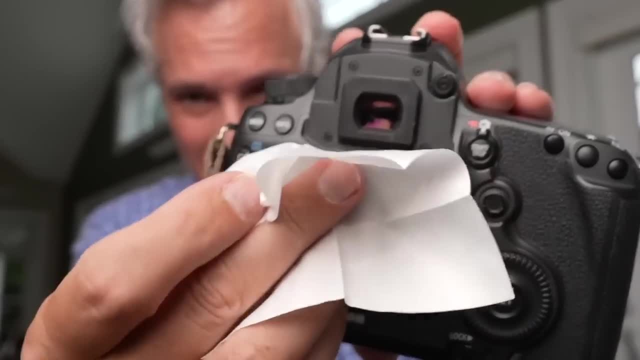 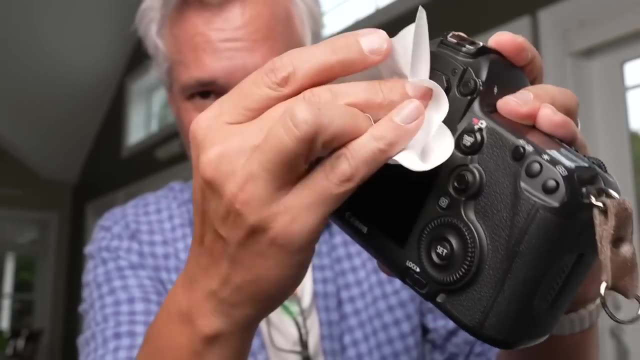 usually comes up just to make it a little easier to reach in there and then take your moistened to off and really get in there if you can't reach it any other way. okay, we've gotten through almost all of it and our camera is mostly clean, but there's still some dust on the sensor. 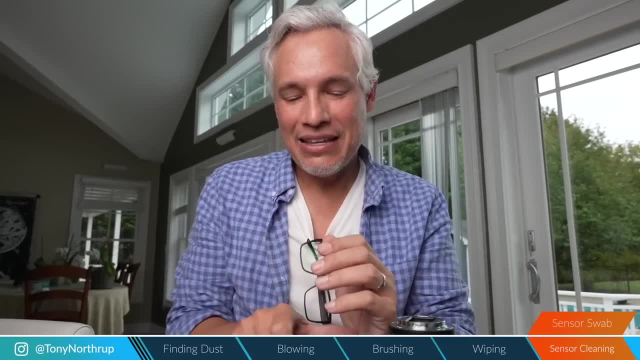 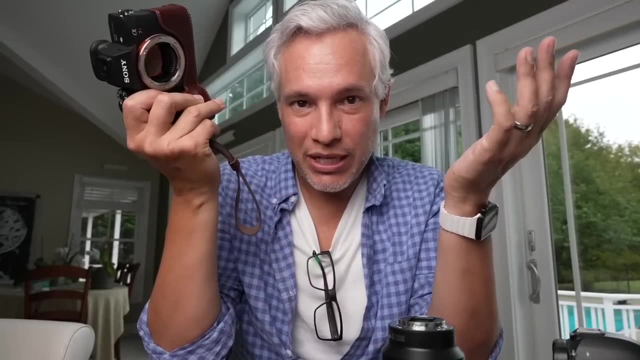 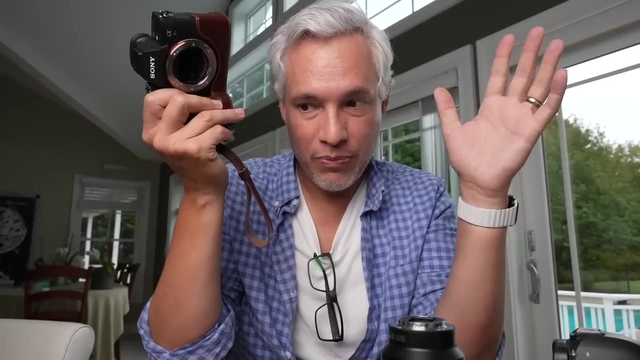 this is really delicate. a lot of people insist on sending their cameras off to the manufacturer for an expensive sensor cleaning that makes them without their camera for multiple days and i just find that completely unacceptable. but i have been cleaning my sensor with vsgo products for years, before we were ever sponsored by them, and i've never had any problem. it's 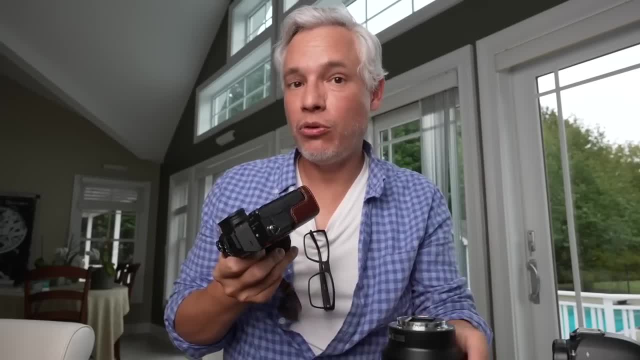 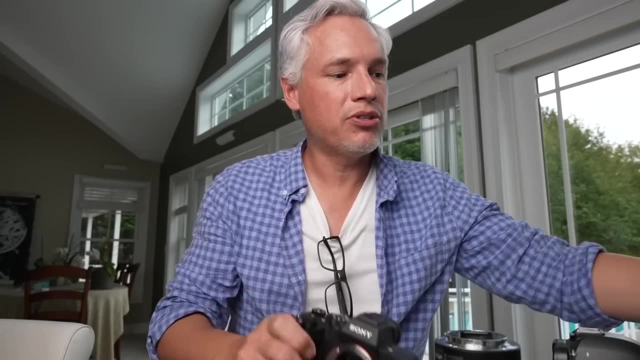 super easy to do. it takes just a couple of minutes, and i always travel with a vsgo sensor cleaning kit too, because it's day three, you get some sensor dust and you don't want to ruin all your other photos, right? so the sensor cleaning kits come in multiple different sizes for different size. 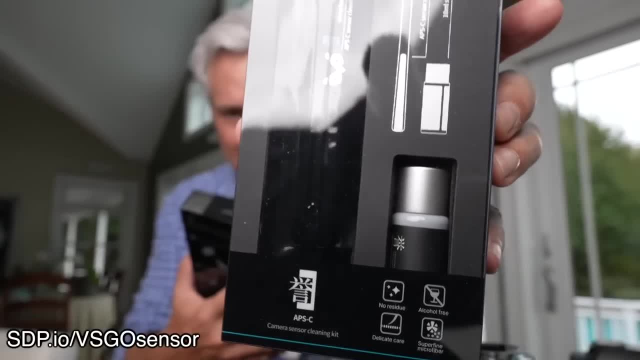 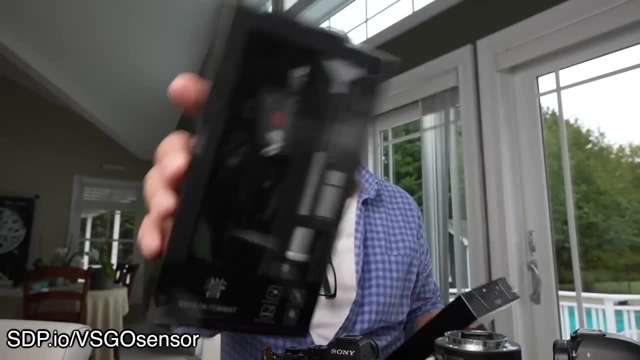 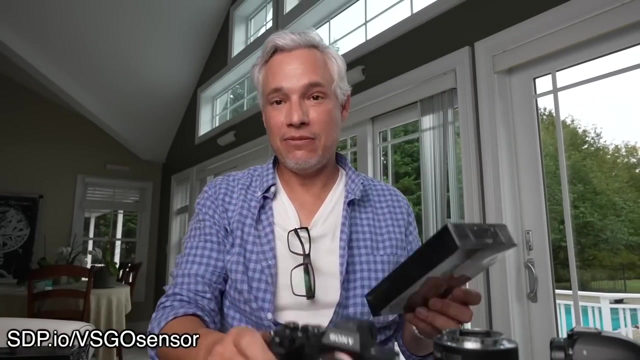 sensors like this is their apsc sensor cleaning kit. this is their full frame sensor cleaning kit. and then they have a medium format sensor cleaning kit for you: hasselblad sensor cleaning kit for your shooters or your fuji shooters. this is a full frame camera, so i'm 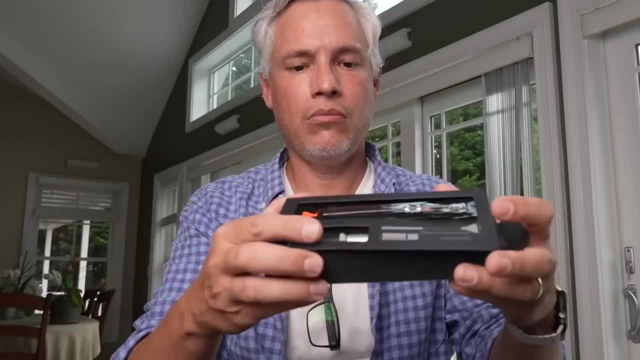 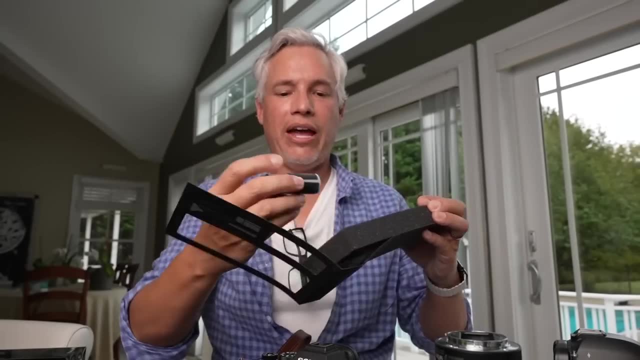 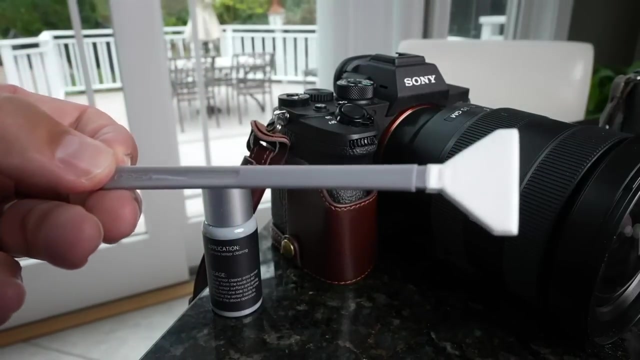 going to use their full frame sensor cleaning kit here. it comes in two parts. you get a whole bunch of swabs that should last you a little while, and then you also have the sensor cleaning fluid, and what i'm going to do is to open up one of these swabs, put a few drops on it and then 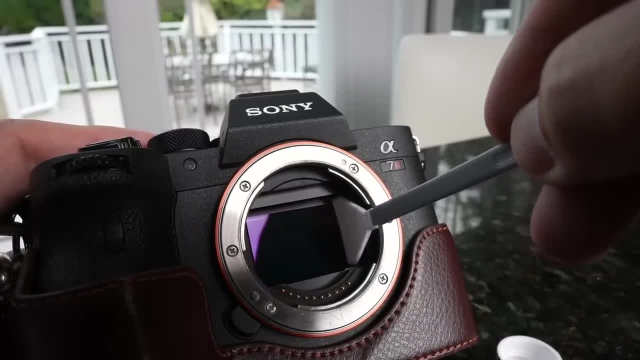 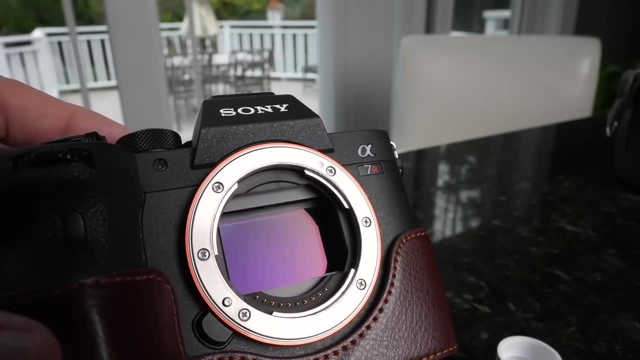 drag it one way across the sensor and then back up back across the other way, and when i'm done i have an absolutely pristine sensor with no dust on it, no damage to it, and i can put my lens back on and go shooting one of the most. 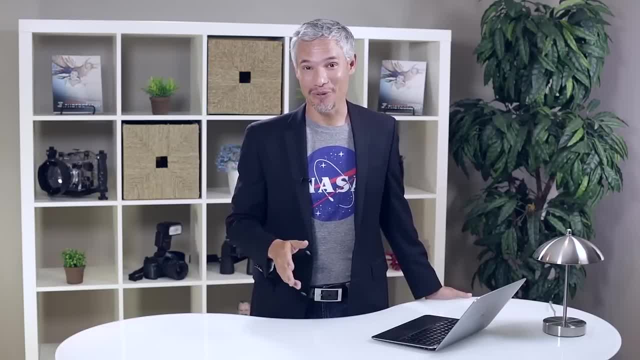 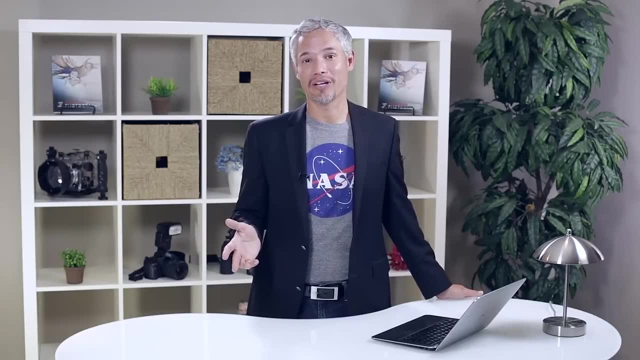 common problems i see, even from my more advanced readers, is a crooked horizon. this is completely unavoidable as far as i can tell, because it happens to me all the time and i really try to avoid it. but if you have straight lines in your picture, for example the horizon at the ocean or 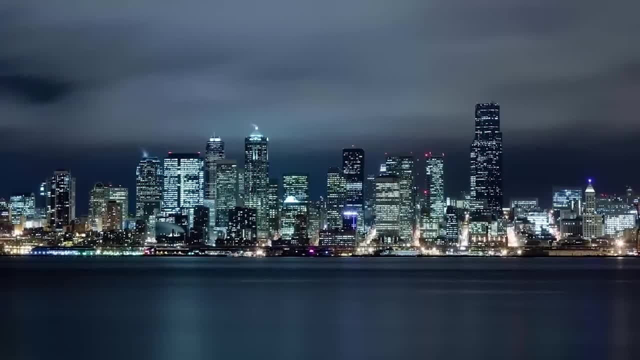 vertical buildings, it's really hard to see the horizon and you can't see the horizon when you're taking a picture. it's really important to make sure that your camera is completely level, and you should do your best to level your camera while you're taking a picture. what i do to help when 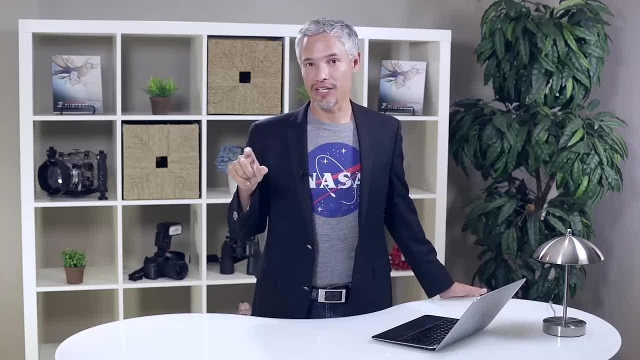 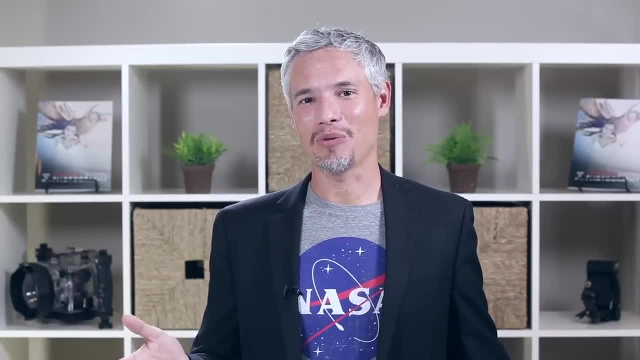 i'm taking a picture is to line up the focusing points in the viewfinder with the horizontal or vertical lines in the scene. but if you're hand holding a picture, it's never going to be quite perfect. now, if you have your camera on a tripod, by all means you can use your camera's electronic 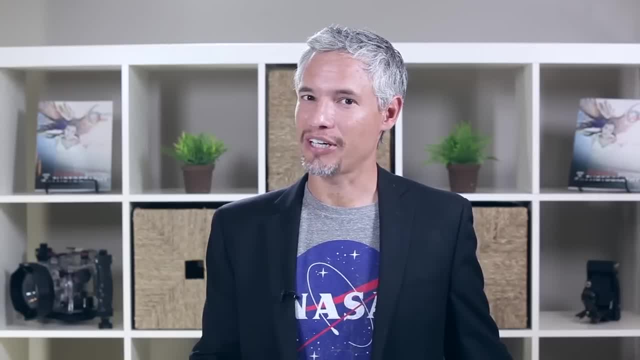 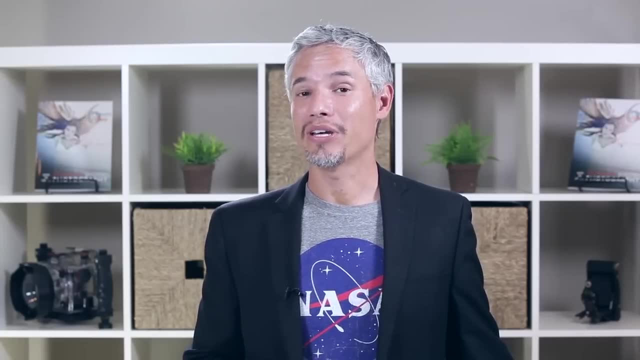 level to make sure that it's completely level. most new cameras have an electronic level, some older, so check your camera's manual. if you don't happen to have an electronic level, you can add a bubble level to your camera's hot shoe. these only cost a couple of dollars but honestly i kind of hate them. 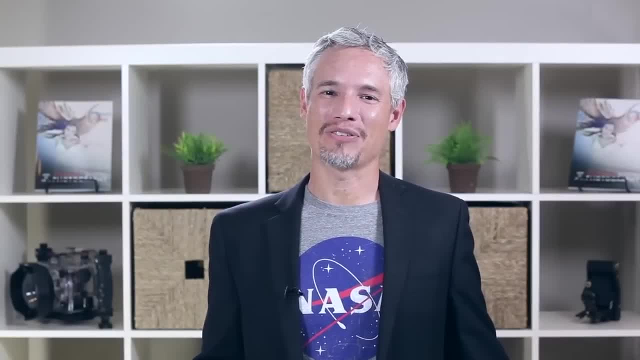 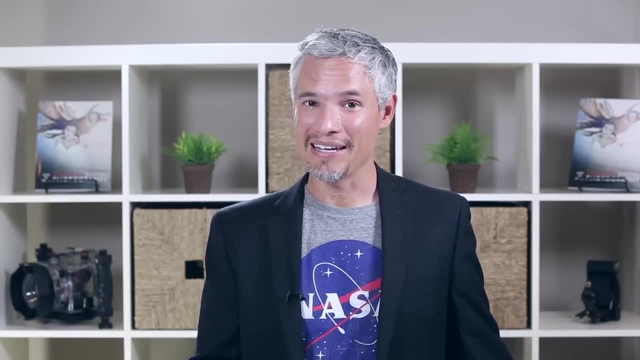 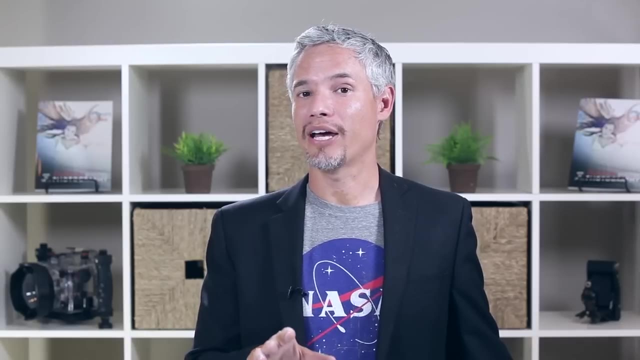 they never really stay in place and you'll be fumbling through your bag trying to find this stupid thing and you'll be losing it all the time. so forget the bubble level. just get it as level as you can, and in post you can rotate it a little bit more if you need to. i always like to shoot my 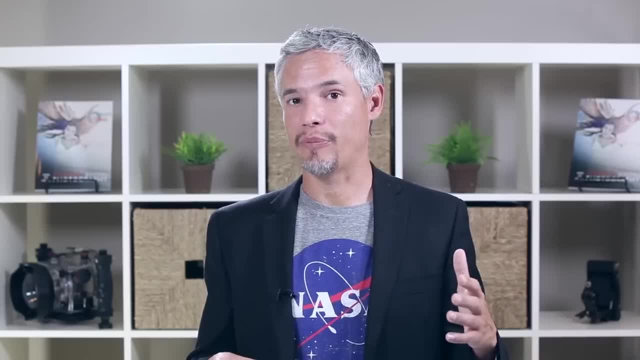 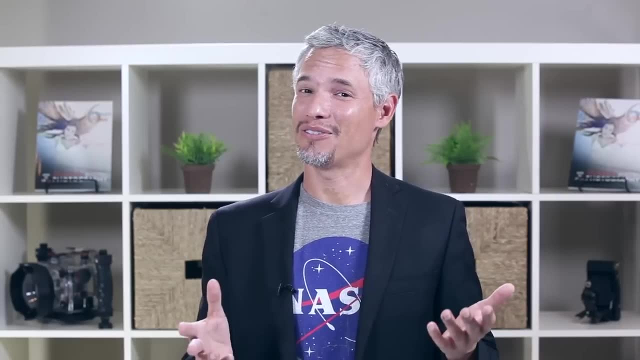 photos, especially a little bit wider angle and give myself room to crop, and one of the reasons you do that is when you rotate a picture in post you're going to have to cut some of the edges off. let's look at a couple pictures that aren't quite level, so you'll know how to recognize the problem. 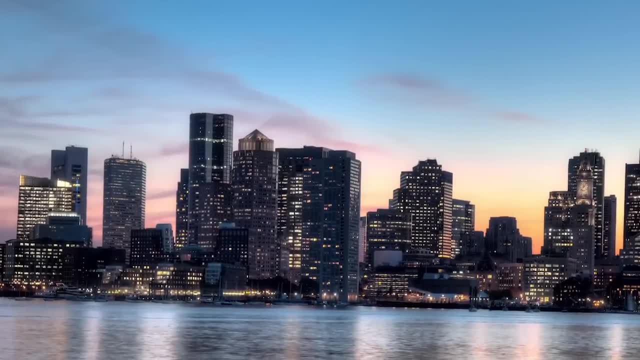 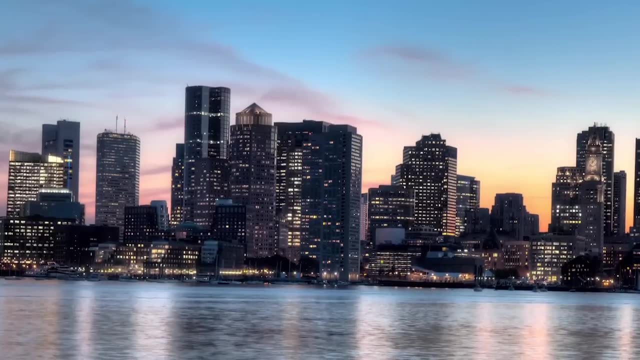 this is a picture of the boston skyline and because of all those vertical edges and the horizontal line of the water, it's really important that it be completely level and you can see it's tilted a little bit clockwise. all i got to do is to bring it into lightroom or picasa and just 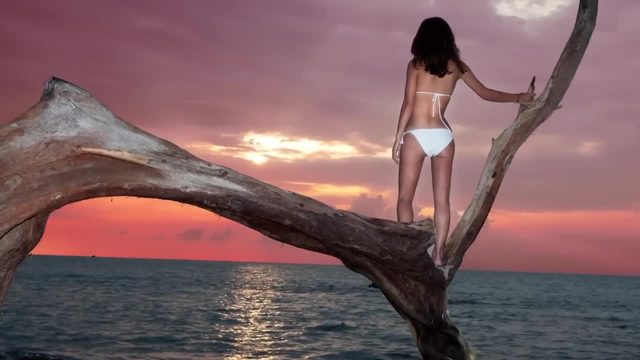 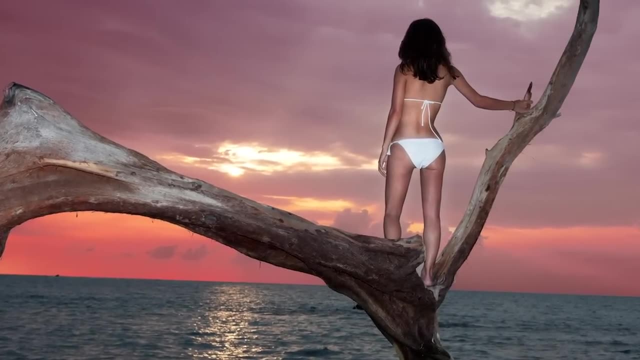 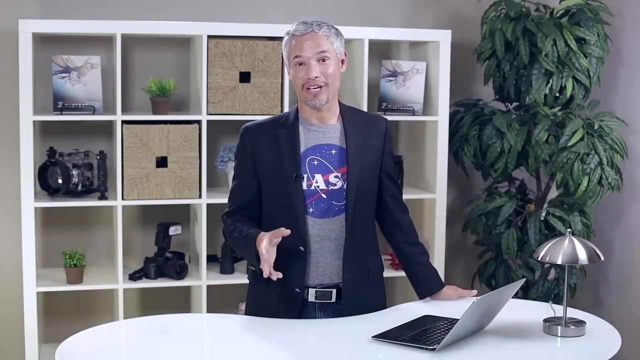 straighten it up. this picture of chelsea also includes the horizon, and because the horizon is so perfectly straight, it's really critical that it be completely level, so i need to level this in post to make it perfect. here's another common problem that i run into when i'm out shooting, and that's low camera batteries. 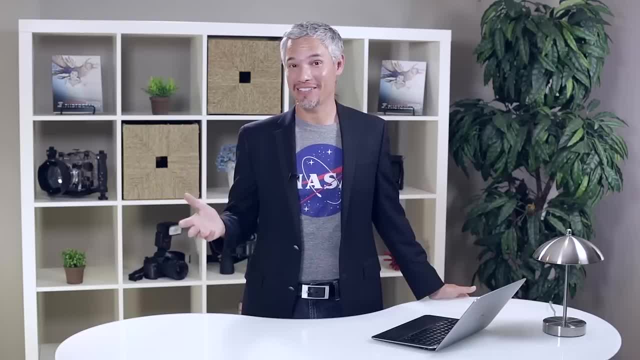 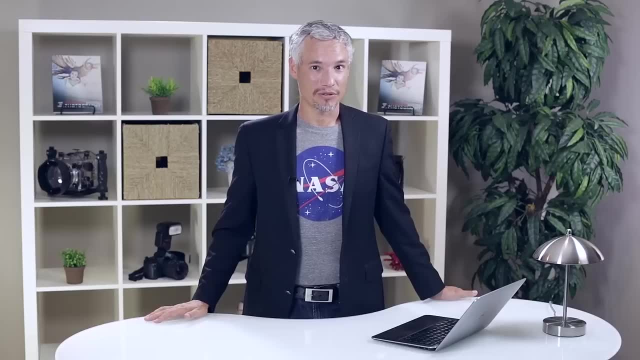 i'm always running out of batteries, and then when you start to run out of batteries, it can't take any more pictures, right? so if you see that your battery is starting to run out and you think you're going to run out before you are done taking pictures, there are some things you can do to 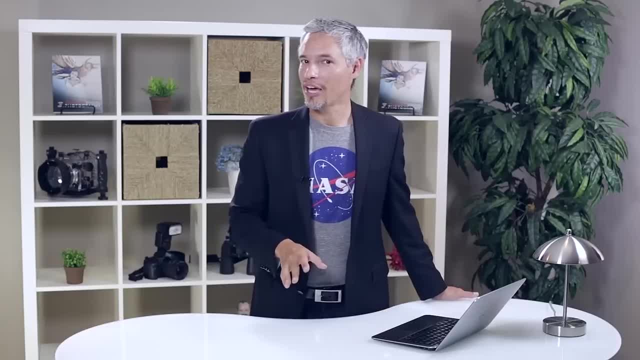 reduce the amount of batteries that you're going to run out of. so i'm going to run out of batteries. here's another common problem that i run into when i'm out shooting and i'm running out of batteries. now, a lot of new cameras nowadays, like the canon 6d, will have a built-in gps and or built-in. 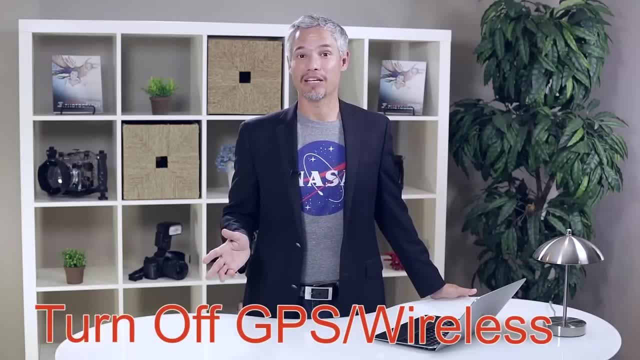 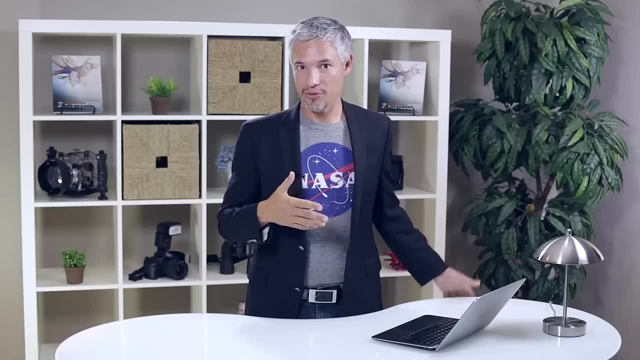 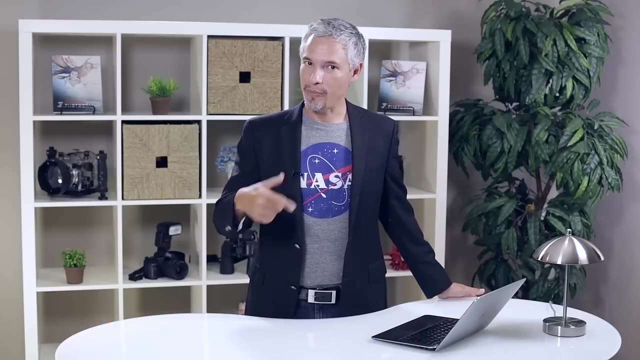 wireless capabilities. turn that off if you don't absolutely need it, because those things really go through batteries. another problem is the live view display. if you're using your camera's lcd screen to frame pictures, turn that off and hold the viewfinder up to your eye. if you are using the viewfinder already, you can turn off that automatic review. 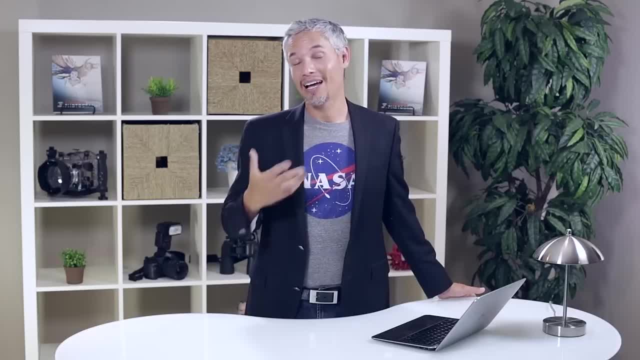 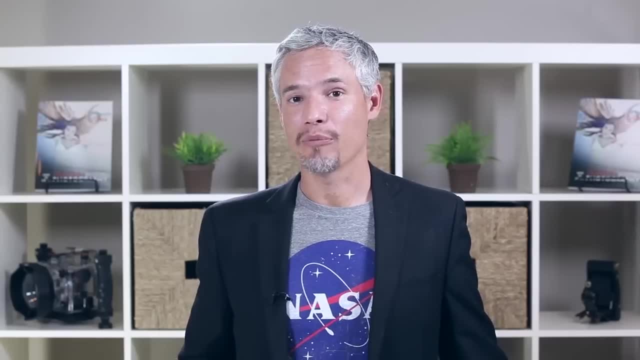 you know, when you take a picture and then it shows you the picture that you just took, i know i like it to look at that automatic review, but that burns a lot of batteries when it's got to light up the screen. if you're using your camera's built-in flash, that's going to drain your camera's batteries. 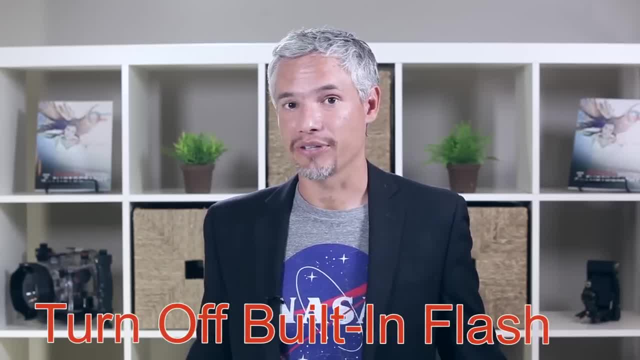 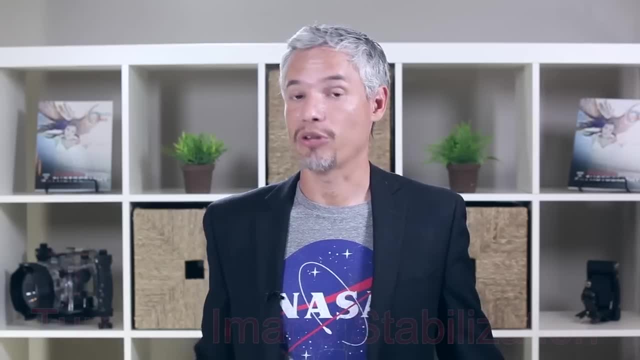 really really quickly. and external flash will have its own battery, so you don't have to worry about draining your camera's batteries quite as fast. image stabilization will also drain your camera's batteries, whether the image stabilization is in the lens or in the body, because either way it's. 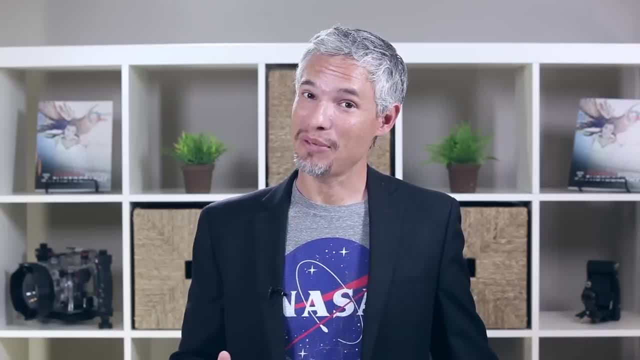 pulling the power from the camera battery. so if you don't need the image stabilization, turn it off and you'll find your battery will be able to run out of batteries and you're going to run out of batteries and it will last much longer. there are a couple of options for extending your battery life. 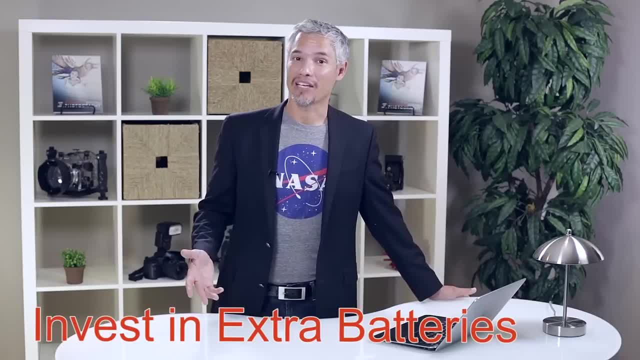 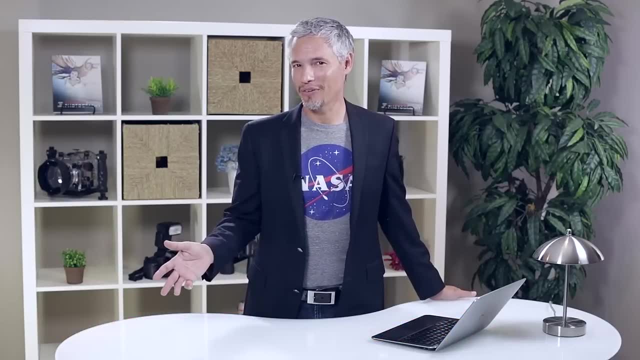 of course one is just to buy an extra battery and keep it charged and carry it with you. now you'll see, if you go shopping for batteries, that those made by your camera manufacturer- canon, nikon, sony, whatever- are outrageously expensive. i know batteries my camera like 65 bucks and i don't. 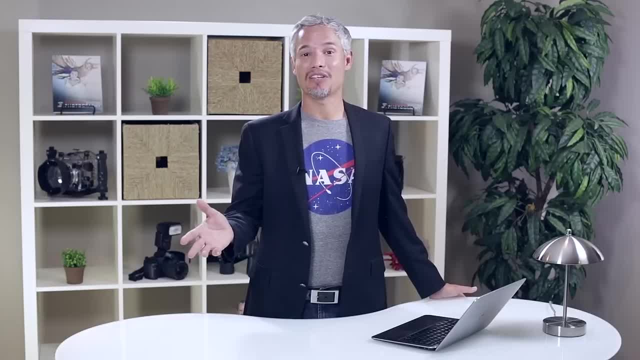 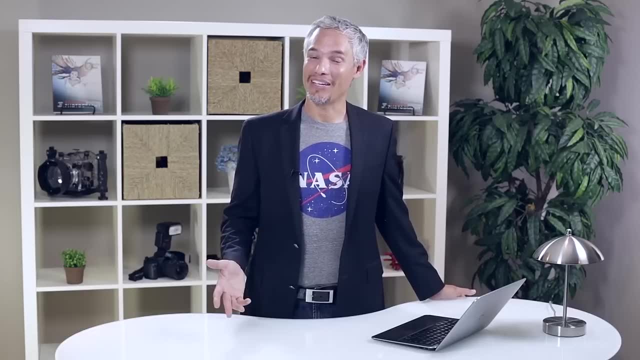 know why any battery would be 65 bucks, um, and then you'll see some generic batteries and they'll be like 12 bucks, so that i bought the generic batteries. i bought the name brand batteries. i'll tell you what i'm always happier with the name brand batteries. they just 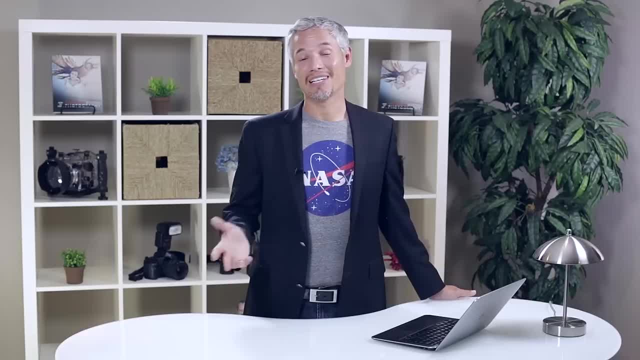 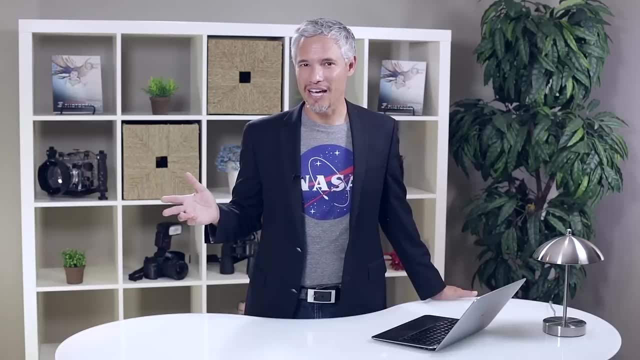 last longer, i still feel like i'm being overcharged. now i also have some cheap knockoff batteries that i use sometimes, but you know what they get like: half the battery life on a good day and then after a year they're completely useless, and you know what does it cost you when you can't take pictures. 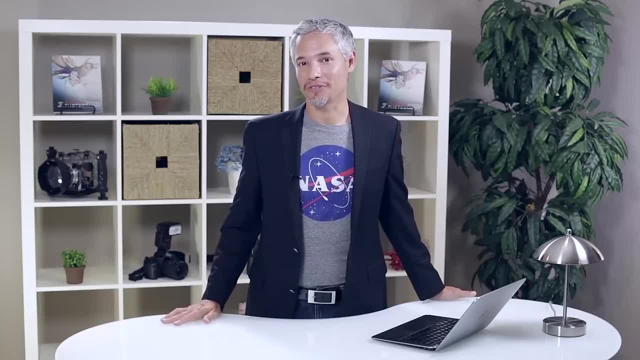 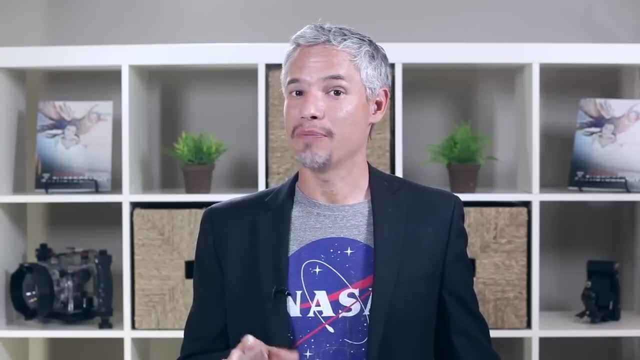 when you need to. so anyway, go ahead and give those knockoffs a try. i know i did, but just be warned that you'll probably be happier with the name brand batteries. another option is to get a battery grip or a vertical grip for your camera, if you have an. 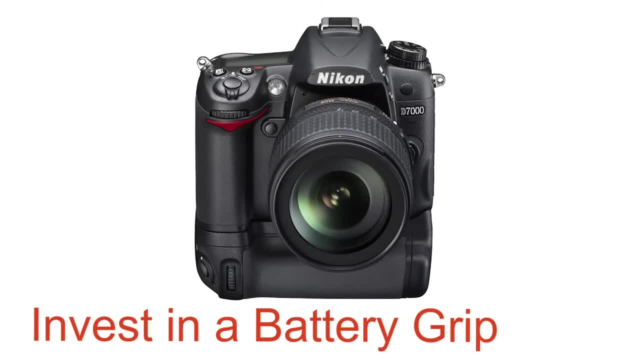 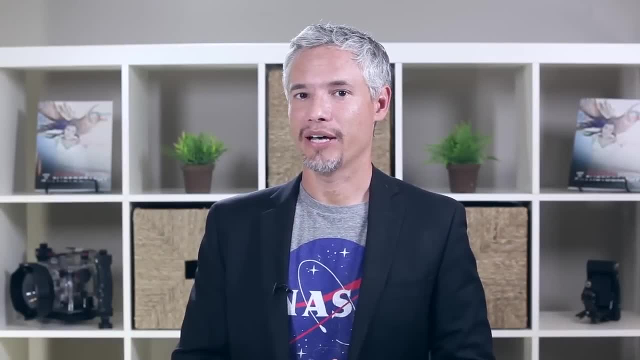 slr. sometimes you can cram on this extra grip that allows you to store two batteries or allows you to use double a batteries inside of it, and in particular, double a batteries can be nice because you can stop at any pharmacy or grocery store and buy more batteries and swap them out. so 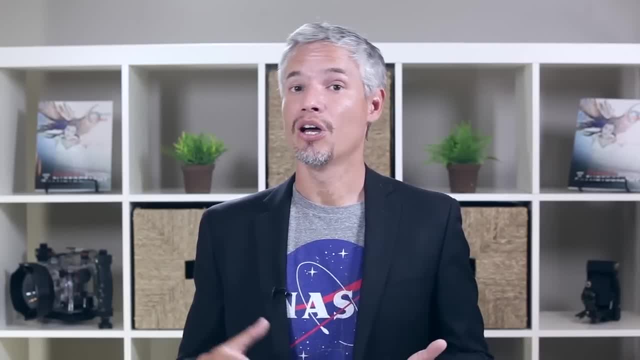 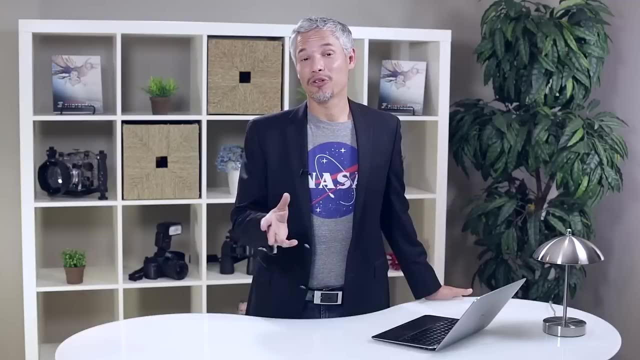 you don't have to worry about using these specialized batteries, and if you put in two of the normal batteries, of course you'll get twice the battery life, and you will have to change the battery life a lot more often. the vertical grips add a lot of weight to your camera, though, and they 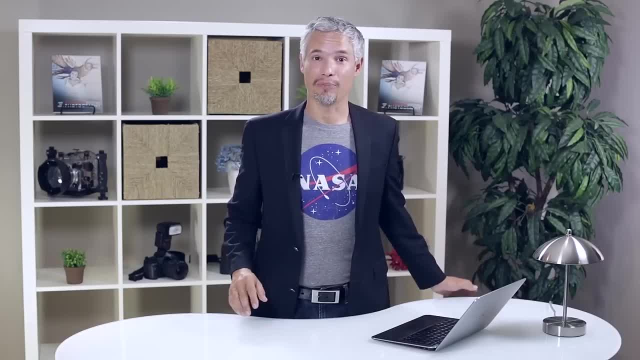 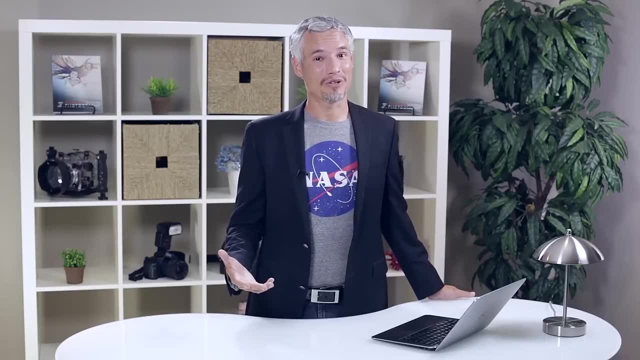 also add a lot of bulk, making it a little more difficult to travel with, but if you want to be sure you don't run out of batteries, it's something to consider. once again, you have the option of the name brand vertical grips or the cheap knockoff vertical grips, and you know, check the reviews on. 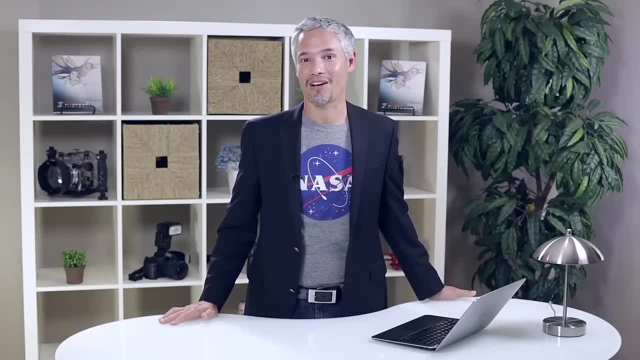 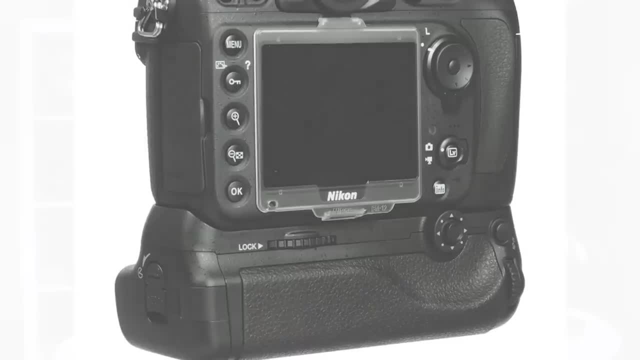 amazon, the knockoff ones aren't that bad. in this case, i do often nudge people towards the knockoff ones, unless they're a pro and they absolutely need the original equipment. manufacturer quality problem is running out of memory space in your camera. i like to carry a couple extra memory. 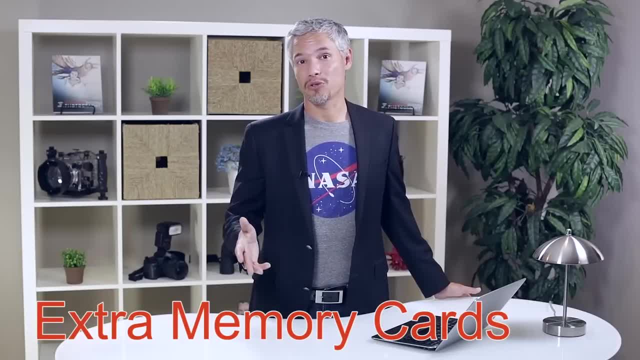 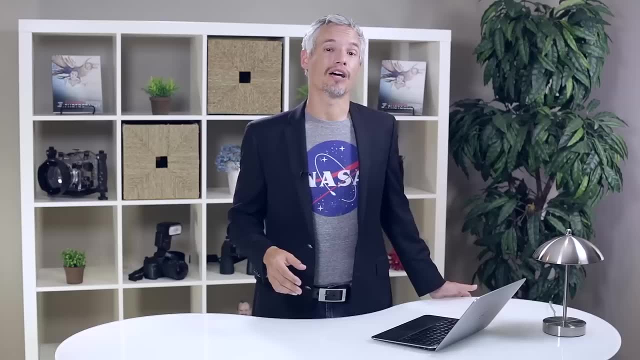 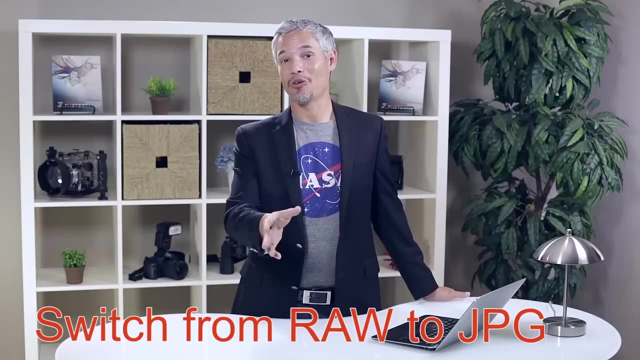 cards. you can also stop by most pharmacies or grocery stores and buy an extra memory card in case you're completely filling up your memory card on vacation. if you find yourself almost running out of memory, one of the things you can do is switch from raw to jpeg recording. now i saw raw. 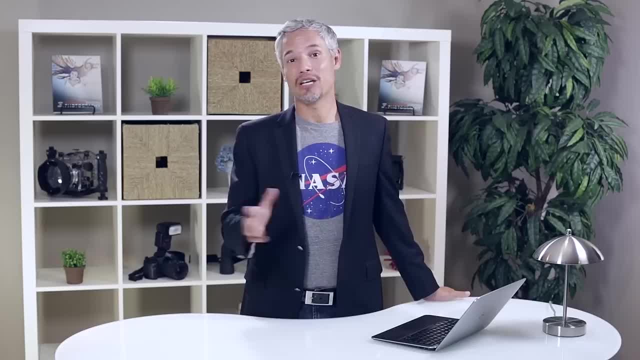 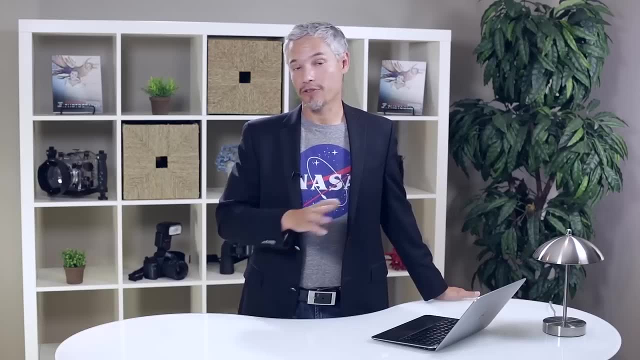 hard because i really like shooting in raw, but jpeg takes like one tenth of the space. i also tend to use a little bit more space in the camera than a lot of other cameras. so if you're going to start scrolling back through my pictures, and first i'll delete any bad videos that i have- 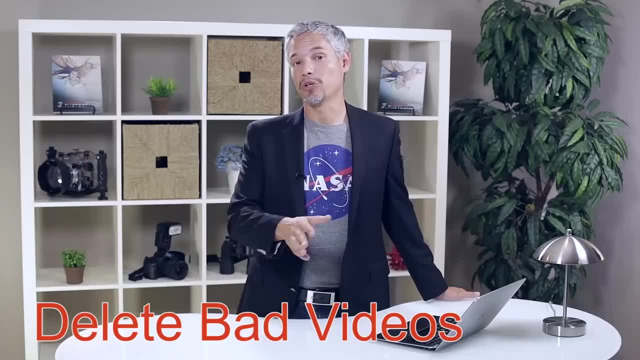 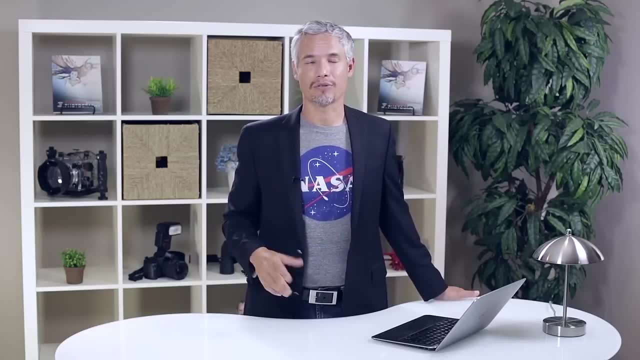 because videos take up far more space than individual pictures. but if i'm really hard up for space, i'll start reviewing my pictures and deleting anything that's blurry or out of focus or just isn't the best of the set. so go back and clean up your memory card once in a while. 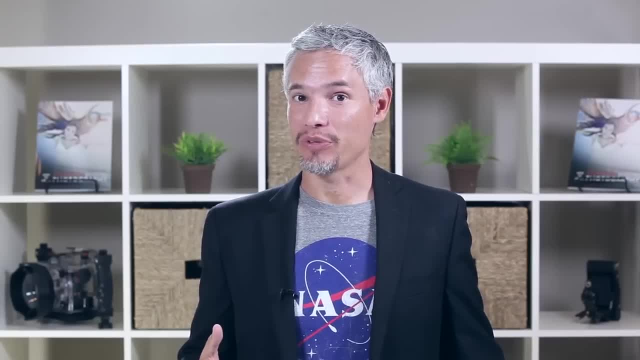 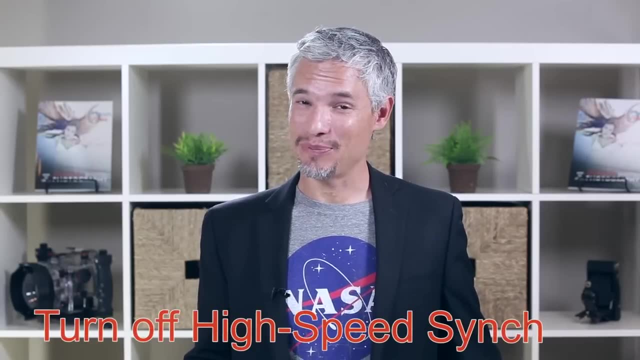 another common complaint is a flash that takes a long time to recycle or that burns through batteries too quickly, and there are a bunch of easy ways to fix this. probably the easiest is to turn off hide speed sync if you're not actually using it. if you're shooting with a shutter speed of below. 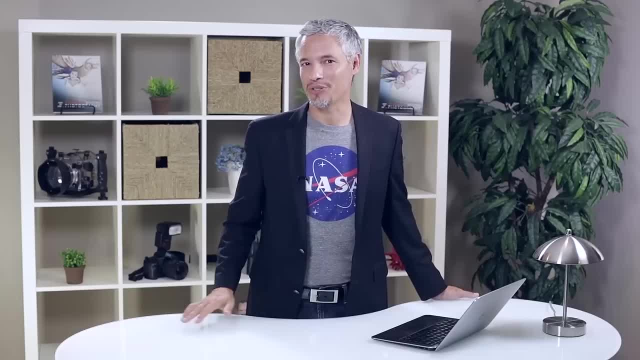 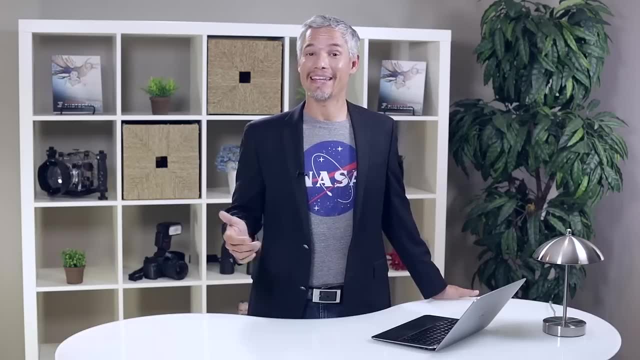 about 1 200th of a second or whatever your camera's sync speed is. you can look it up, but usually it's about 1 200th of a second. you don't need to use high speed sync. some people just turn on high speed sync and use it all the time and that uses like 5- 10 times more batteries. so it's going to. 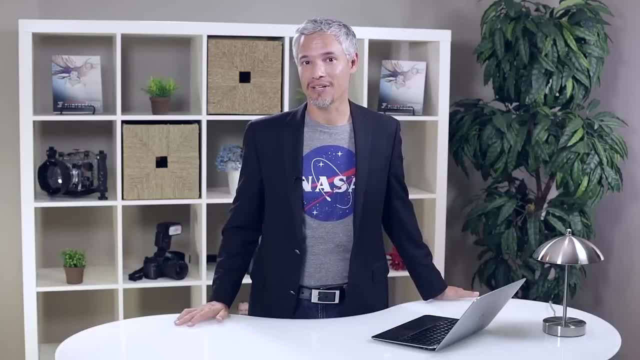 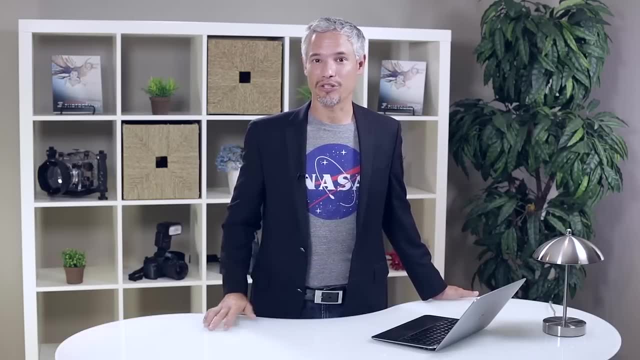 make your flash much, much slower to respond. it's going to burn through your batteries much faster. if you are using high speed sync and high shutter speed, maybe find a way that you can get the shutter down below 1 200th of a second so you can turn off high speed sync whenever possible. use a flash. 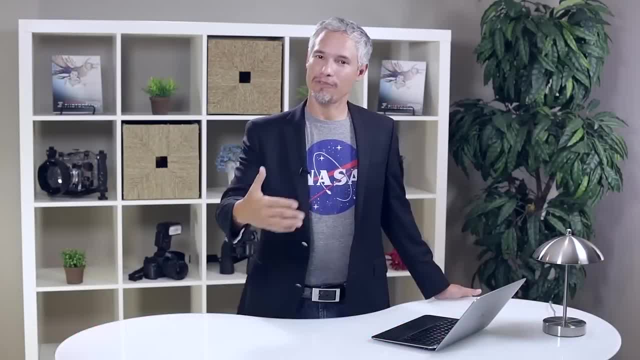 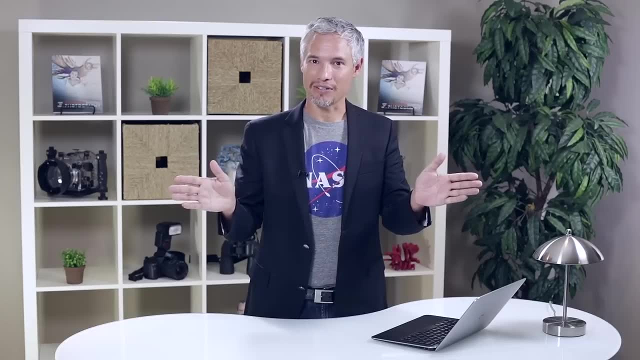 that has a zoom head. zoom heads adjust their focal length to match the length of your lens. so if you're shooting with a wide angle lens it'll send light out so that it covers the entire scene. but if you're shooting with a telephoto lens, it'll zoom the flash head in and just cover that narrow field. 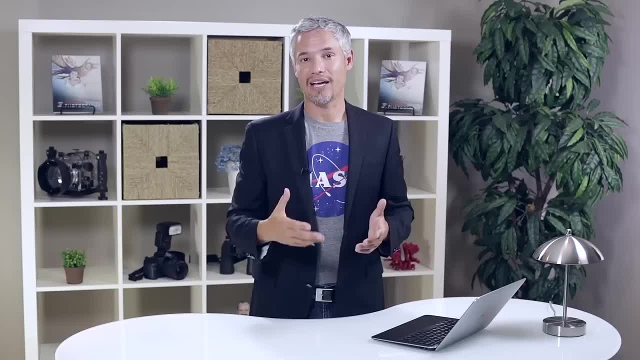 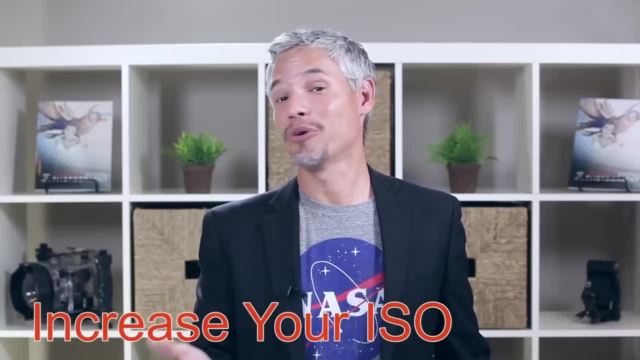 of view with light. that allows the flash to put out much less light and thus use batteries much more. you can also increase your camera's iso now. i've warned you earlier about increasing your camera's iso and all the side effects of that. you're going to get noisy pictures right, but by increasing the 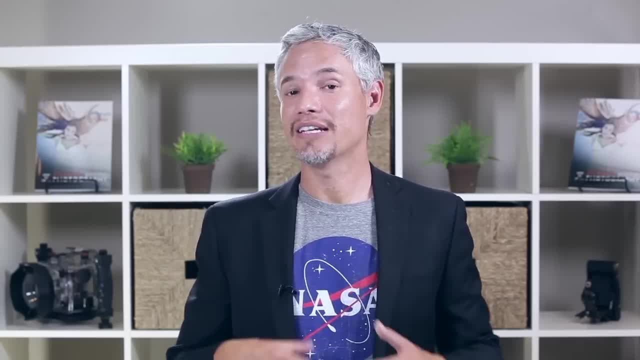 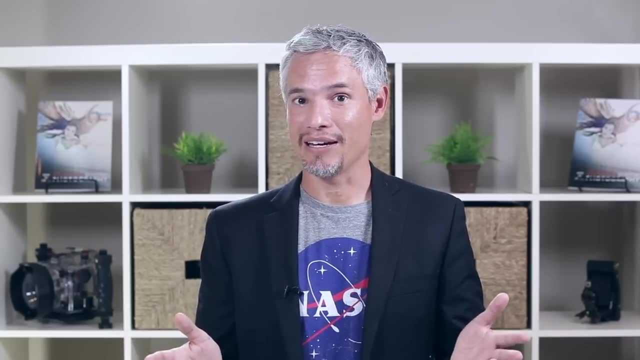 camera's sensitivity to light, the flash doesn't need to output nearly as much power. if you go from iso 100 to 200, your flash needs to output just half as much light, meaning your batteries are going to last about twice as long and your flash will recycle about twice as fast. so, as you can, 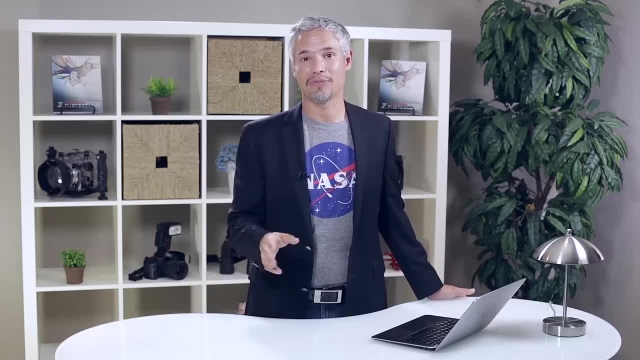 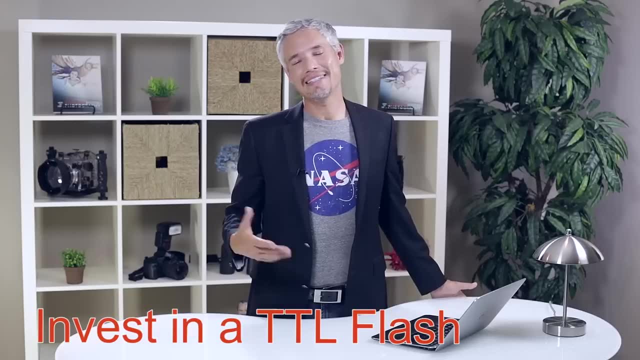 see here, the flash is going to be barely working at all and your batteries will seem to last forever. i'd also suggest getting a flash that supports ttl, that's through the lens, metering ttl just allows your flash to figure out the exact amount of light that's needed in the scene, and not put out. 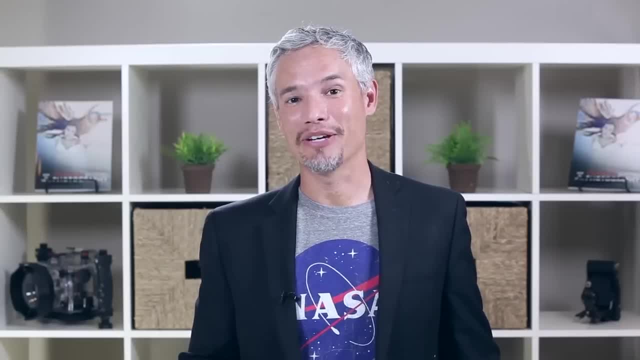 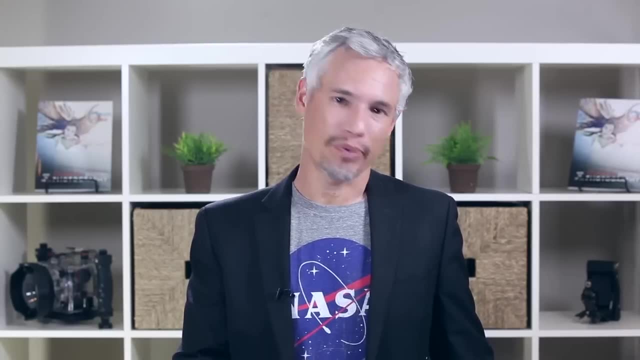 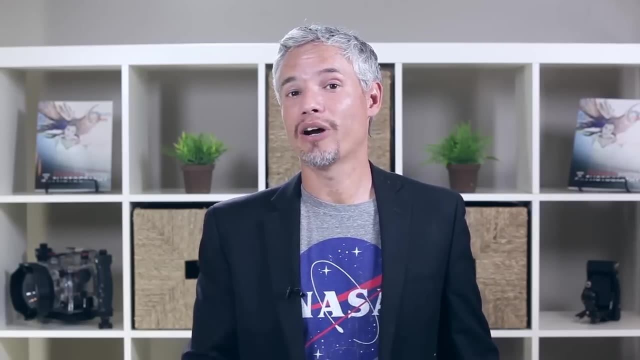 any unnecessary light. just about every flash made by your camera manufacturer- sony, canon, nikon- will have ttl enabled by default. if you get one of these third party flashes, like a mets flash or some brand of it might not support ttl. now i do recommend generic flashes, those that support ttl, and 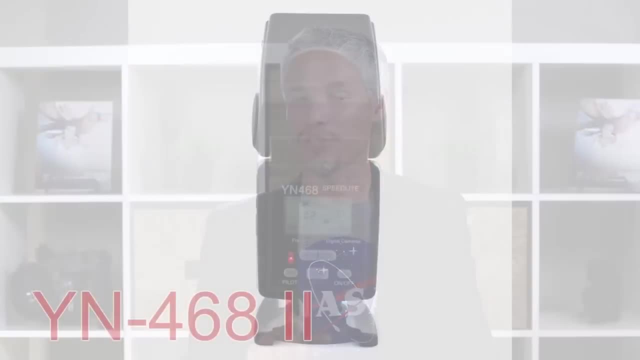 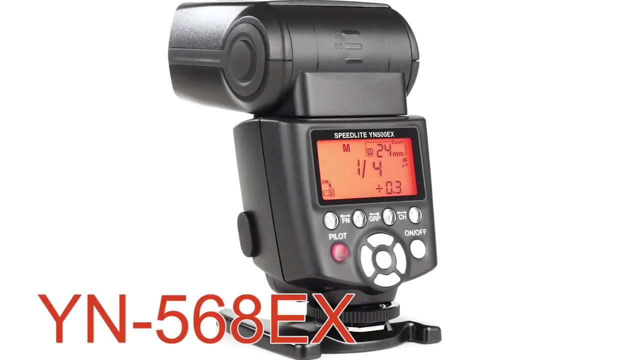 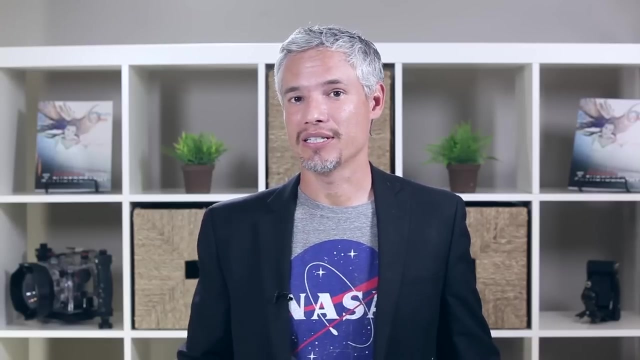 specifically the yongno yn 468 2 for both canon and nikon, or the yongno yn 568 ex. the model 1 version of that works for nikon and then mach 2 works for canon and they both support ttl and they 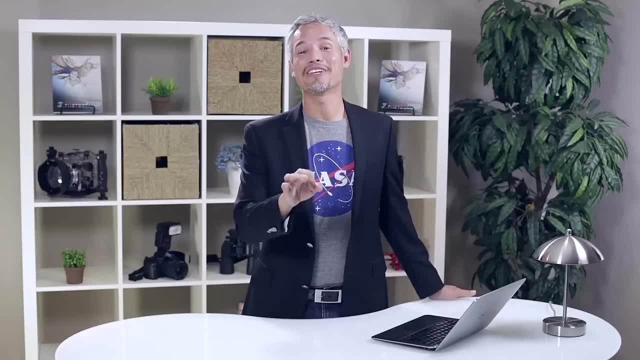 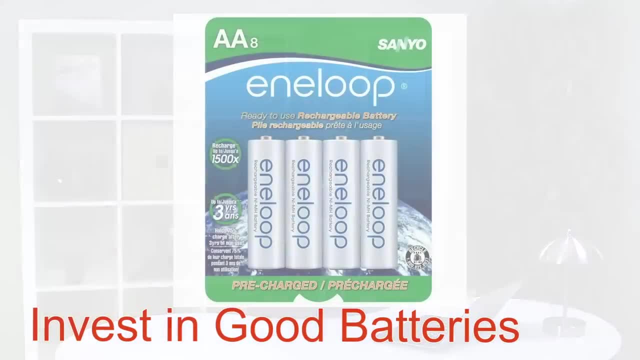 work just as good as the name brand flashes. another thing you can do to make your flash last longer is to use good quality rechargeable double a batteries. i specifically recommend the eneloop batteries. they cost about 10 bucks for four, so that's actually a pretty good price, but they outperform all the other. 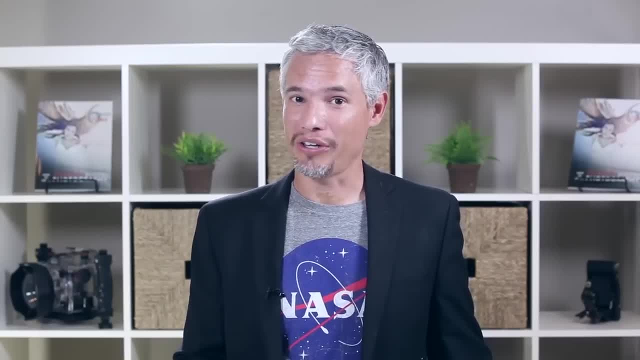 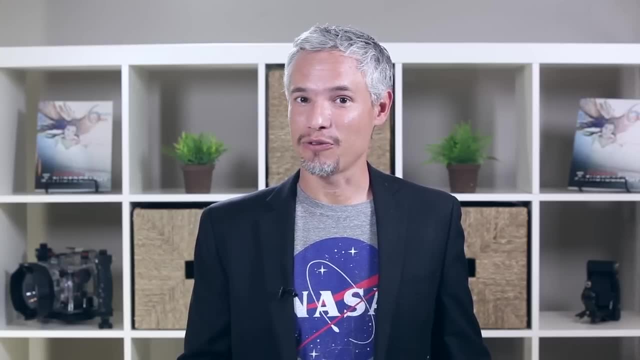 batteries by far. i also suggest getting a good quality charger, because some chargers don't charge all your batteries all the way up, like they'll keep charging a set of four batteries until they see that one of them is completely charged and then they'll stop charging all of them as a result. 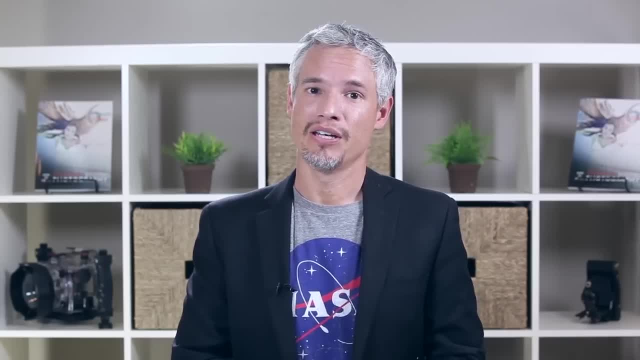 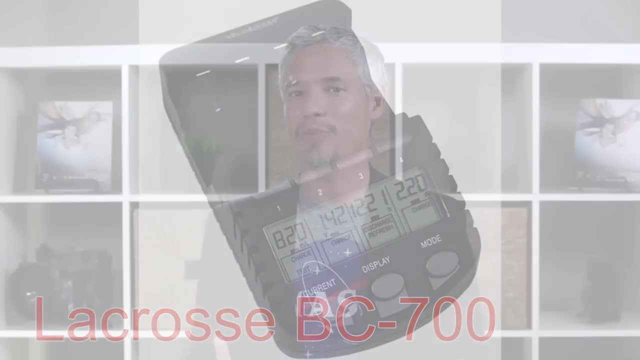 the other three batteries might not be able to charge all of them at the same time, so you can not be completely charged. so you want a high-end charger like a lacrosse bc 700. that's what i use. they cost about 40 bucks, not too bad, and i think you'll get your money's worth out of it when you. 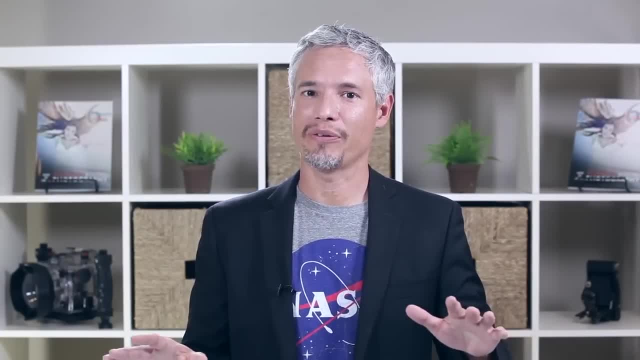 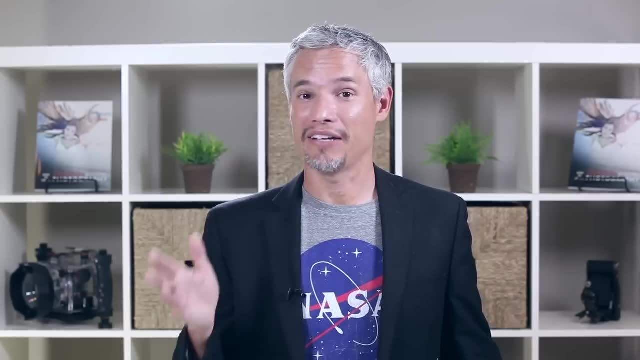 run a few sets of batteries on it, because it'll just make sure that all four of your batteries are completely charged. if you are still running out of batteries- and it happens if you're like shooting a wedding or taking just lots and lots of flash pictures- you can get an external battery. 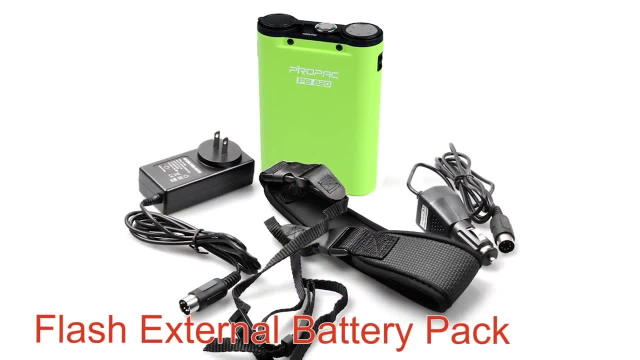 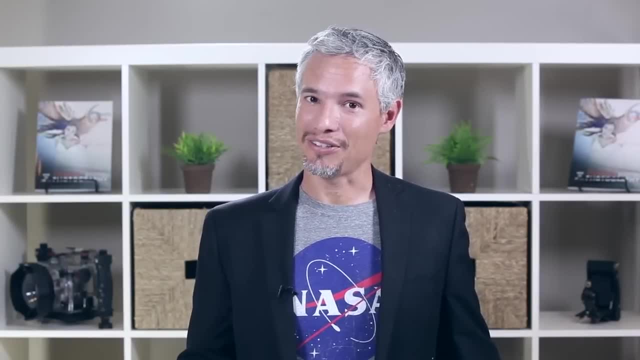 pack for your flash. this does two things. first, they'll usually have like room for eight to ten double a batteries, and all those will power your flash, so of course it will last longer. you can also reduce your flash's recycle time, but just having more juice to pump in there allowing you to 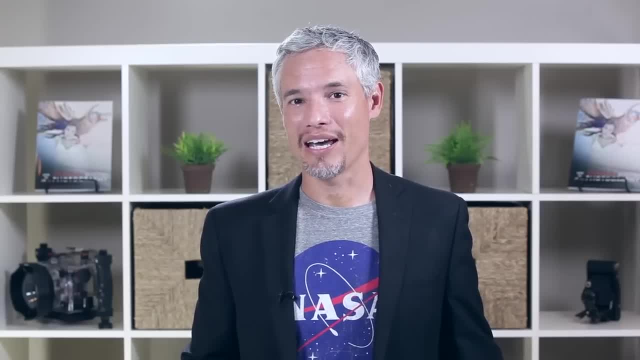 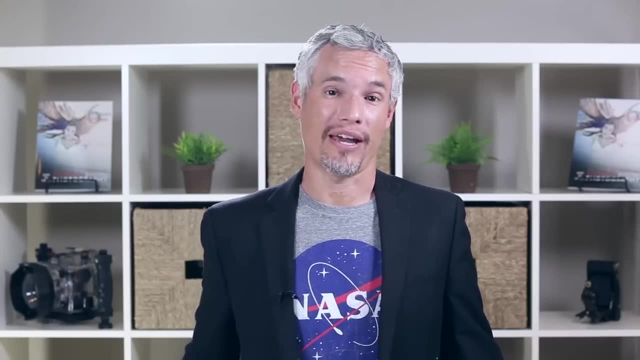 take flash pictures more quickly. not all flashes support an external battery pack, so check your flash's manual to see if that's available and, if possible, pick up a generic external battery pack for it, because canon and nikon make name brand ones, but this isn't one of those times. 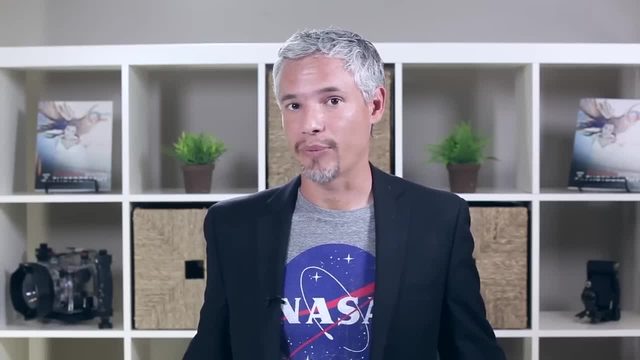 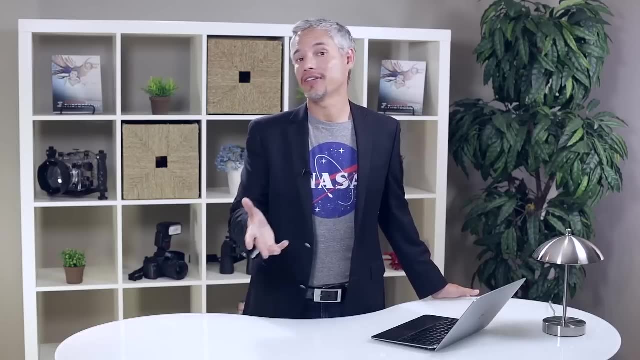 where you actually get any value for your money. so i use a generic battery pack and it works great. now let's talk about flash sync problems. your camera has a sync speed with the flash and, as i mentioned earlier, it's usually about one two hundredth of a second. what this means is you can 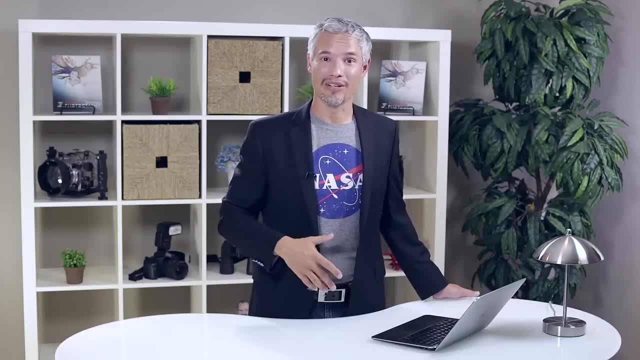 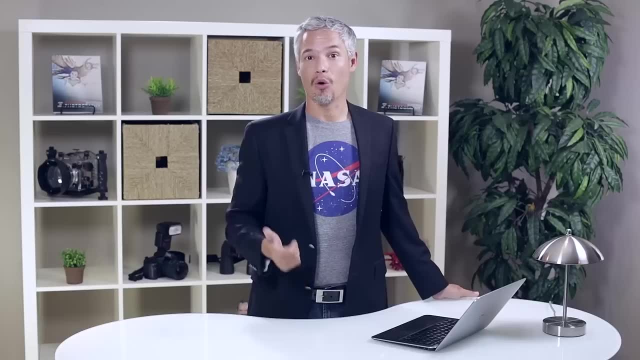 take flash pictures at one two hundredth of a second or slower, but if you were to take a picture at one one thousandth of a second, either your camera would stop you from selecting the faster shutter speed or your picture would be messed up. so let's look at a picture that is messed up. 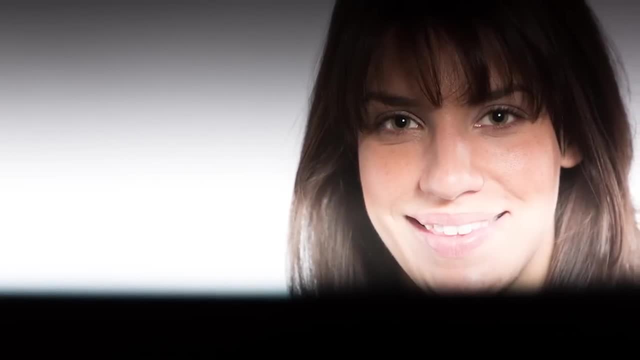 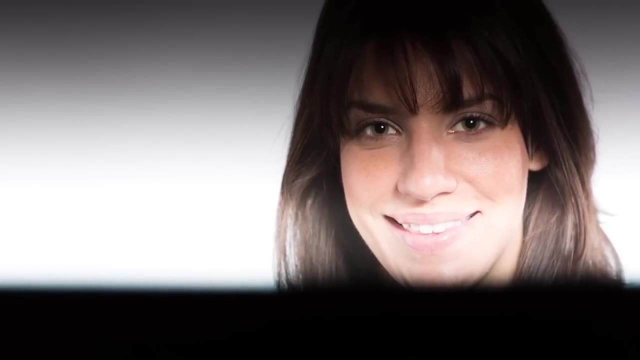 because of flash sync problems. the middle of the picture is bright and well lit and then suddenly we have this dark band at the bottom, and at the top you can see it just gets darker and darker. that's because, as you're taking the picture, your shutter actually. 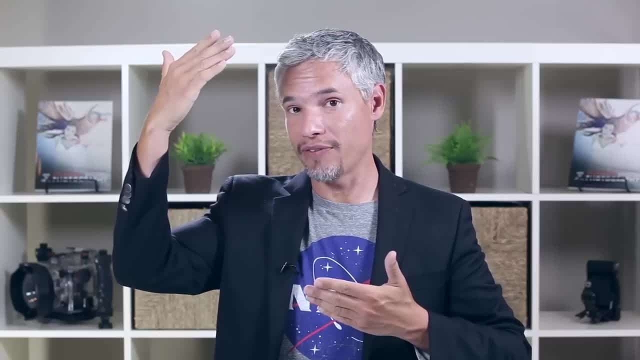 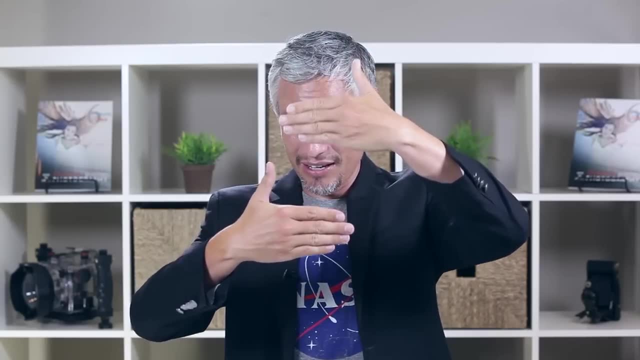 has two curtains. so if you're taking a high speed picture at, say, one five hundredth of a second, that top curtain starts moving down, exposes a little slit of the shutter, and then the other curtain follows it, exposing a little portion of the sensor at one time. now, if you select a shutter, 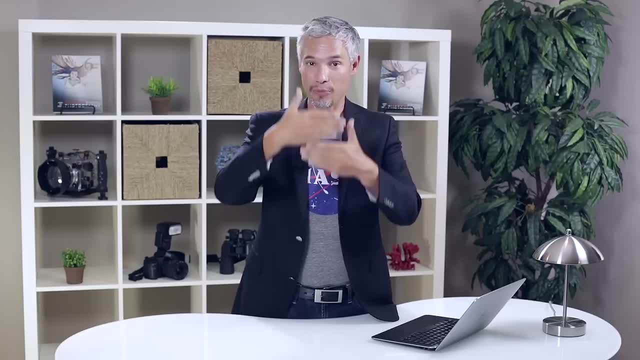 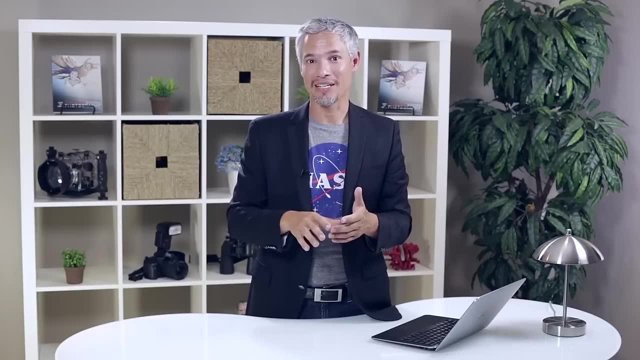 speed of, say, one, two thousandths of a second. any given part of the sensor will be exposed for that amount of time, but it's not exposed at the same time. so the reason we see sync problems is that your flash doesn't fire an even output of light for 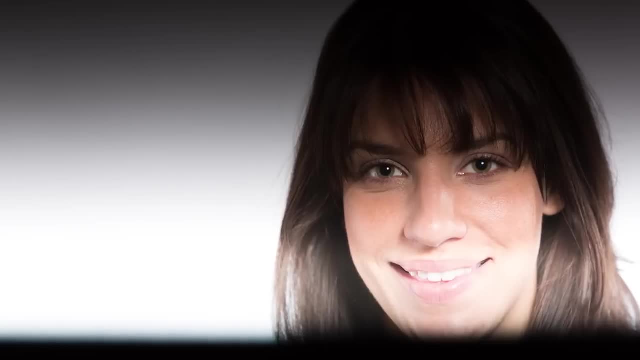 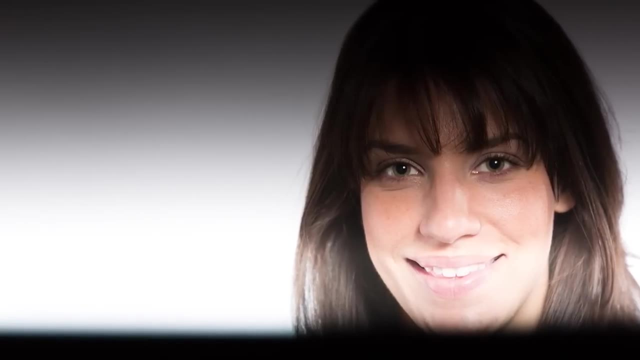 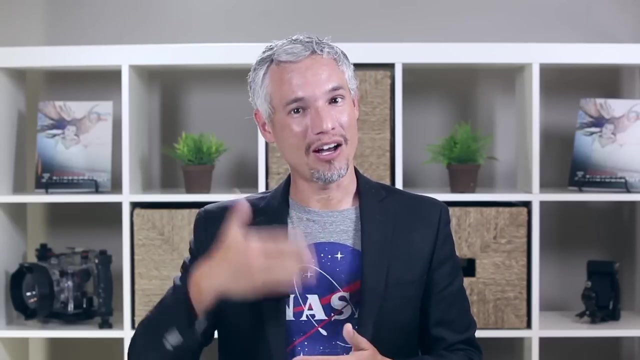 that entire period of time. so the reason we see the bottom of this picture black is that's actually the top of the sensor and it's also the first part that gets covered by that second shutter curtain. therefore, by the time the flash started to fire, part of the sensor was already covered. 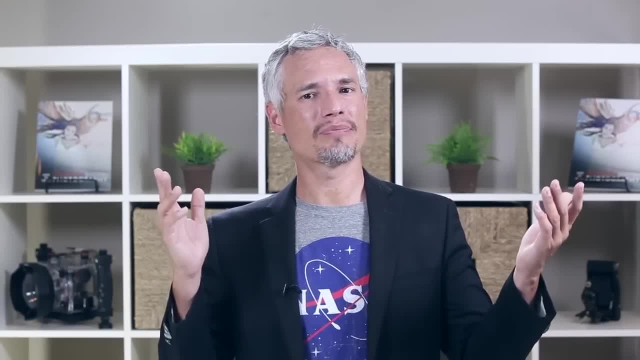 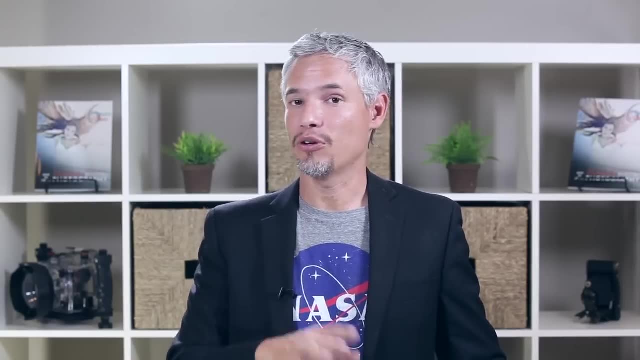 by the shutter and therefore it didn't receive effect. the sensor is now fully breathable, and so any light. You solve this just by turning on high-speed sync and using a flash that supports high-speed sync. Now, not all flashes, even those made by your camera manufacturer, support high-speed. 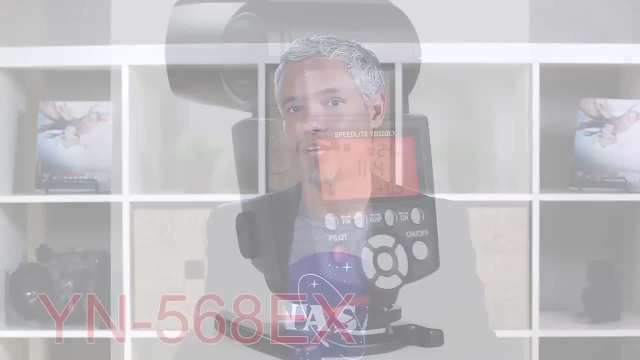 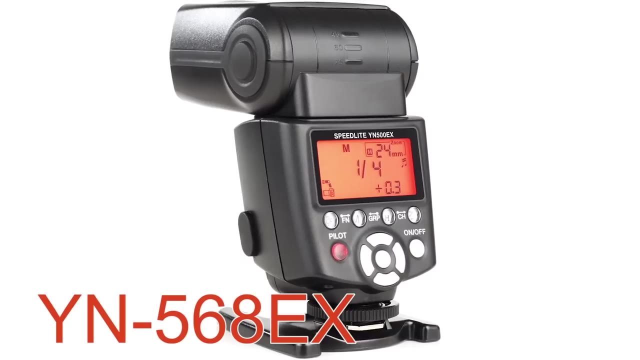 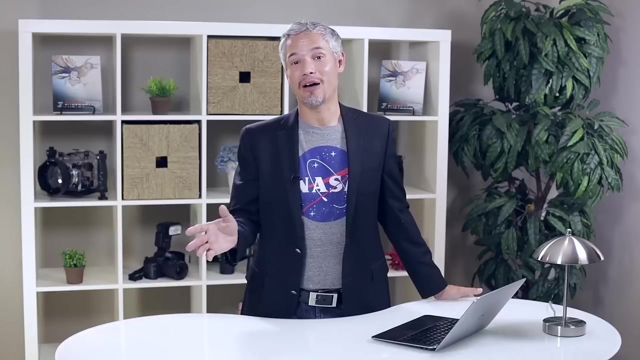 sync, so look for that as a feature In the generic flash realm. the Yongnuo 568EX- both the Mark I and the Mark II models- supports high-speed sync and it's far less expensive than the name-brand models that will work with either Canon or Nikon. Another common flash problem is red-eye and this: happens when you use your camera's on-camera flash, and it happens because the flash is located so close to the lens. What happens is light comes in, bounces off the retina and then bounces right back into the eye and, well, it seems like it reflects that red wavelength more than anything else. 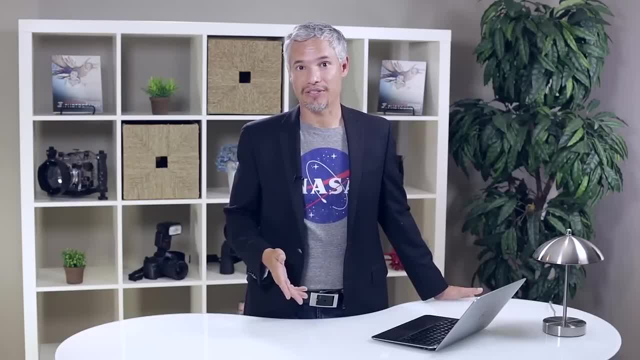 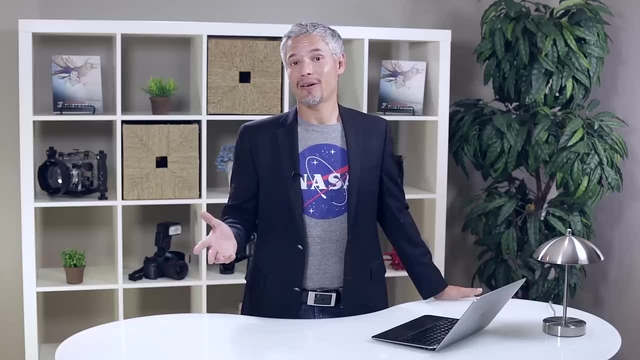 There are a couple of ways to fix red-eye. First, you can go into any post-processing app and fix it. Some cameras even have software that will eliminate the red-eye in post automatically, but I think a better way to eliminate red-eye is just. 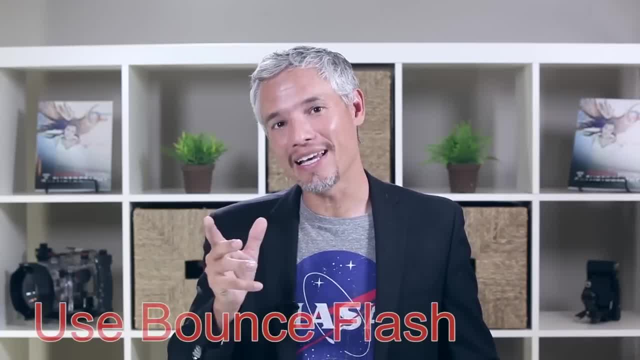 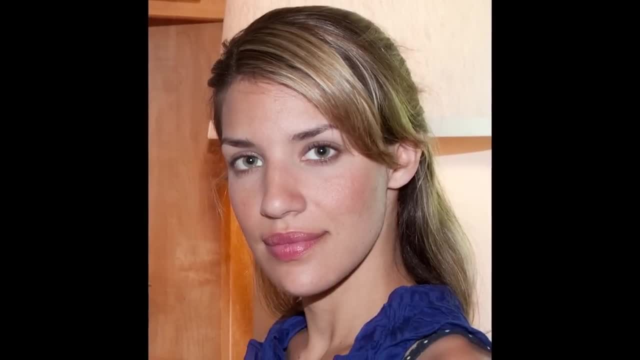 use a bounce flash. Just put an external flash on your camera, rotate that head up and bounce it off the ceiling. This lights up the whole room and lights up your subject much more nicely. so for more information about that, check out the lighting video. Another common flash problem is just too. 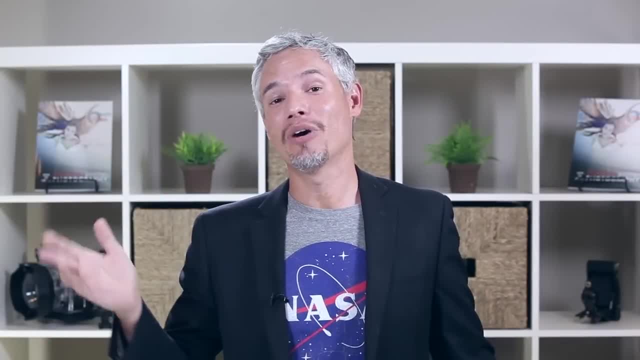 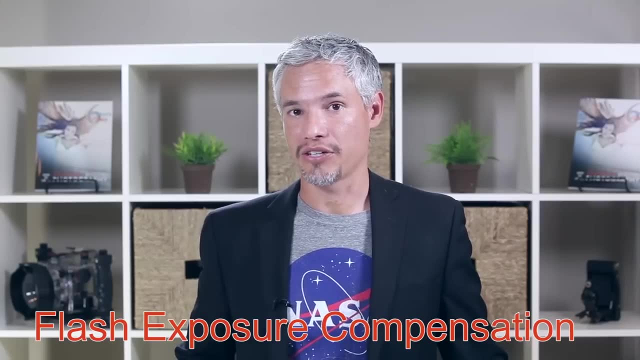 much flash. Sometimes your camera just puts out too much flash. Well, here's an easy way to fix it: Use flash exposure compensation. Your camera certainly has a feature that will allow you to control the flash output. so check your camera's manual for how to do it. Usually there's a button. 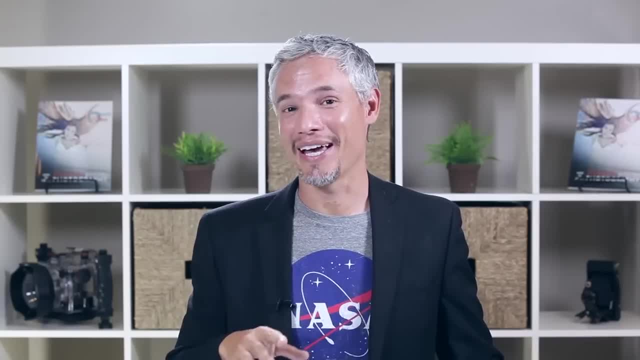 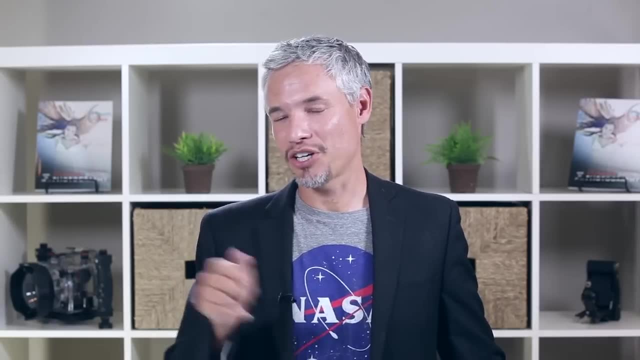 that has like a lightning bolt and then a plus and minus next to it. so look for that. Some flashes, if they have buttons on them, will allow you to control the flash exposure compensation from the flash. so just check your flash's manual to see how you can dial it down a little bit. We'll. 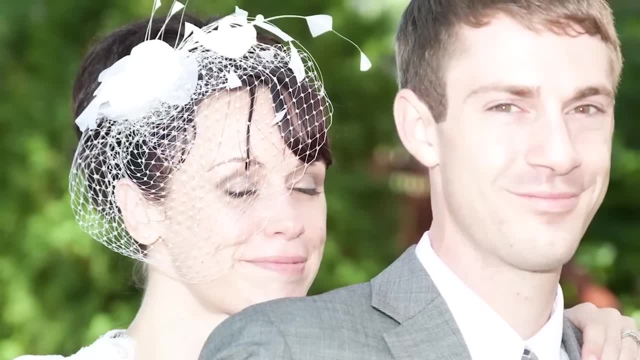 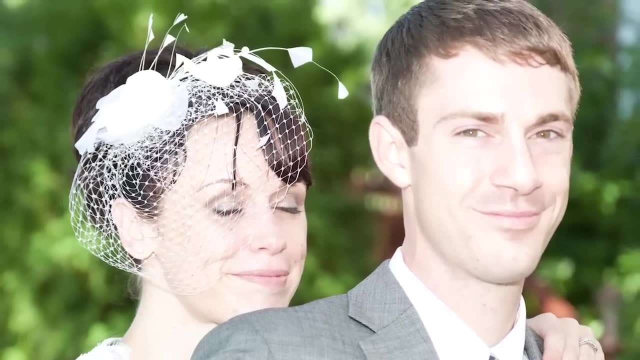 look at a sample picture here that just shows a picture with far too much flash. As you can see, the background seems properly exposed, but the subject's faces are just completely blown out by the flash. so to solve that, I would dial in about negative two. 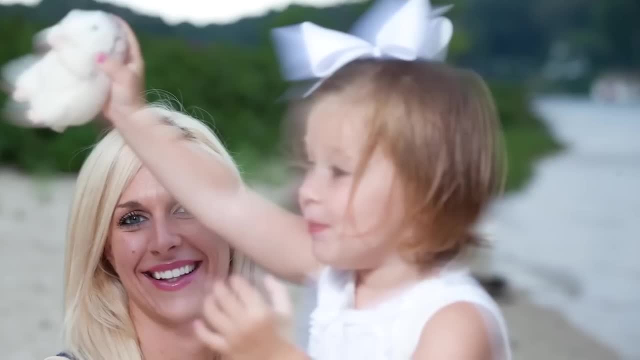 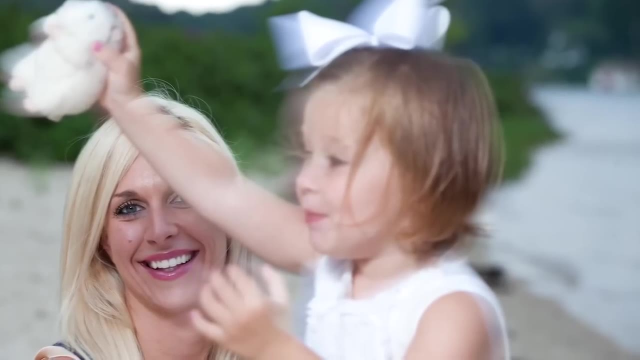 Two stops of flash exposure compensation. Now I'd like to look at an example of motion blur with flash. What we see here looks almost like ghosting. We can see the motion in the little girl, but at the same time she's kind of frozen. I'm just showing this to you so you'll recognize it. 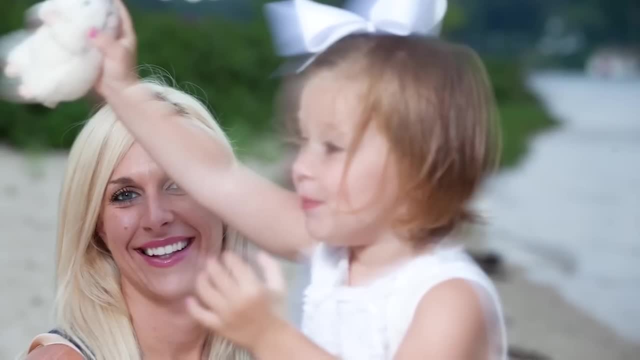 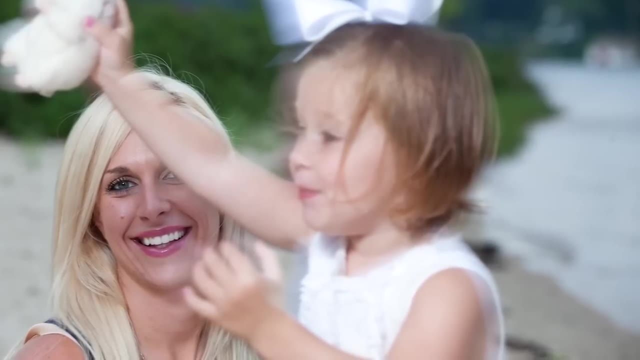 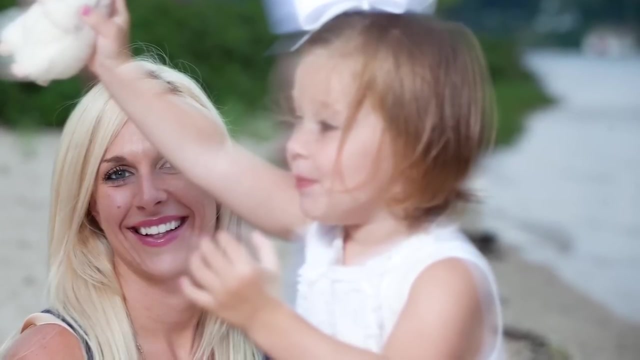 in your own pictures. This happens if you have your camera in shutter priority mode, aperture priority mode or manual mode and you're using the flash and your shutter speed is too slow to freeze motion. So while flash can help to freeze motion, you really can't rely on it because you'll get this ghosting If you want to freeze. 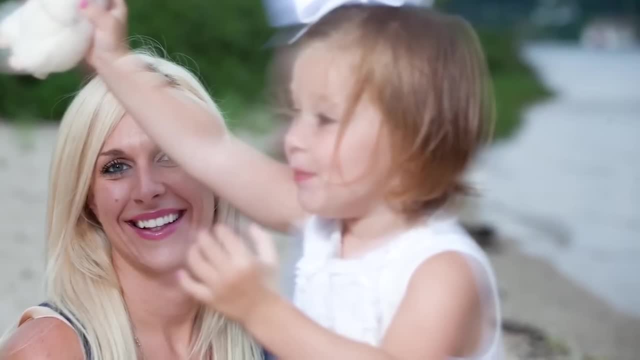 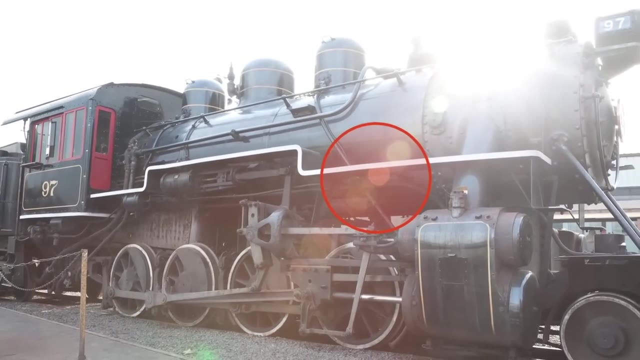 motion, you need to use both a high shutter speed and flash. Flare is another common problem. With flare, you'll see all these weird spots in your picture, even though they weren't there in the scene, like your eye didn't see them. Flare is caused by light coming into the lens and 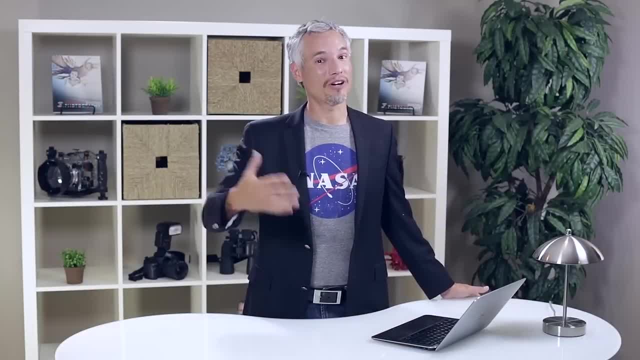 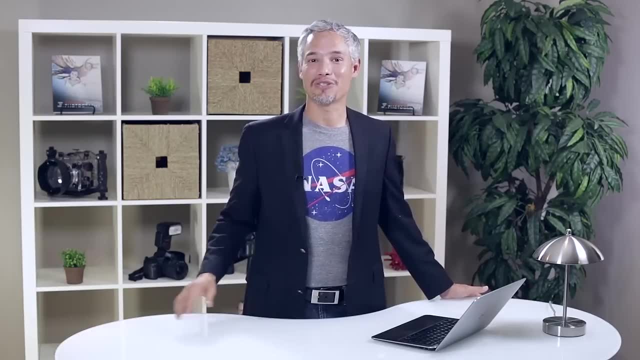 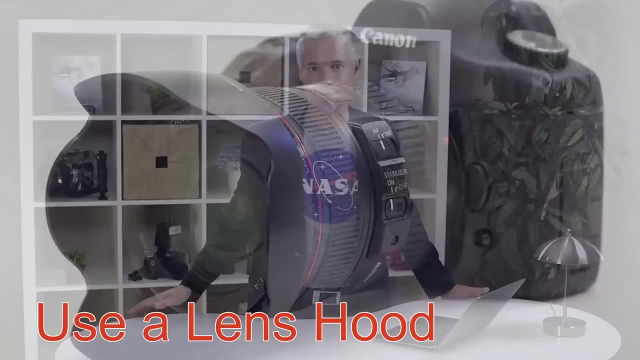 reflecting off of either the lens's internal elements or dust on the front or inside of the lens. Some lenses will just always have flare because they're inexpensive lenses, but there are other options you can do to reduce flare. You can put a lens hood on your lens. That helps stop the. 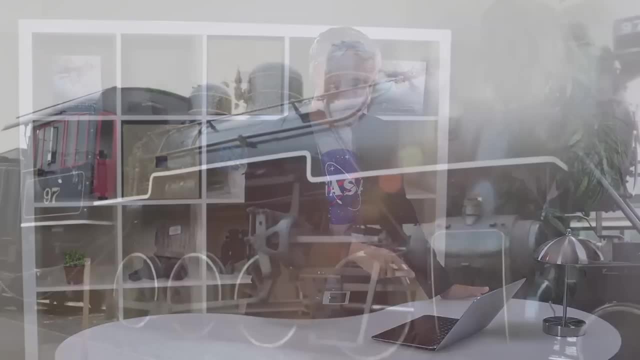 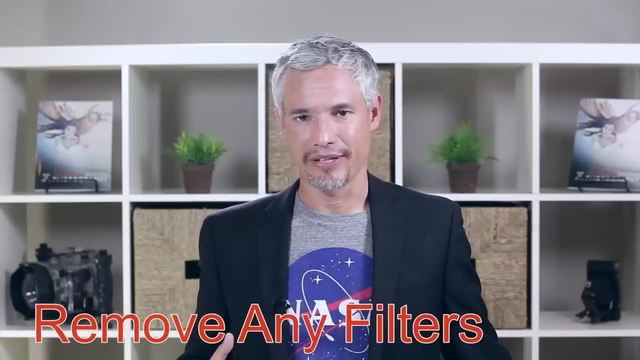 stray light that might be coming into your lens, but if you're shooting into the sun, as I am in this picture, the lens hood isn't going to do you any good at all. Another thing you can do is to remove any filters that you have on your lens. I don't really 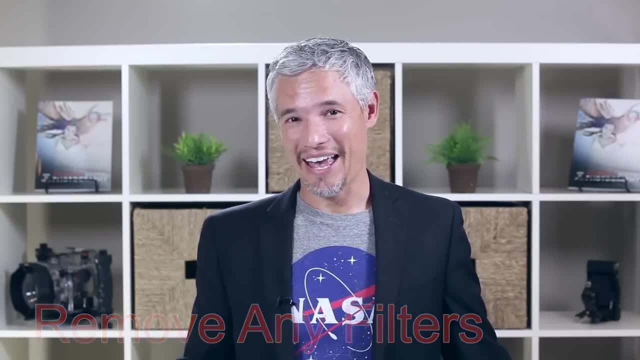 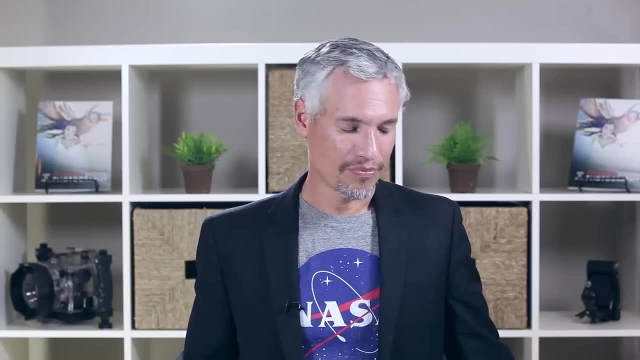 recommend using filters at all, even those UV filters meant to protect it. They're just going to add flare and mess up your pictures, so they're not really worth it. You can also avoid shooting bright lights. Now, this is a rather expensive solution, but if you can drop a grand on a 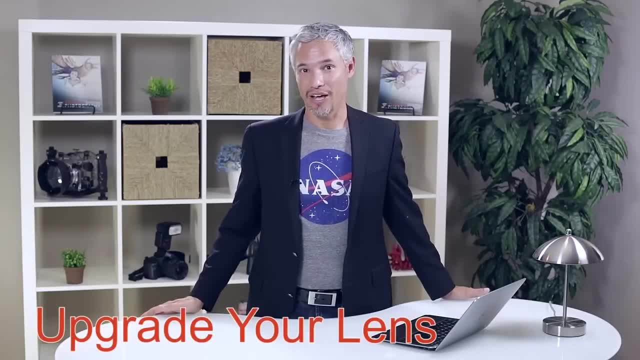 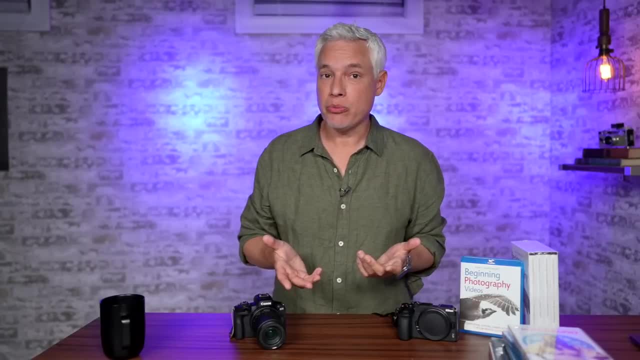 professional quality lens. well, the professional quality lenses do have much less lens flare than the consumer-level lenses. Thanks so much for watching this Again, please do share it with other people so that they can benefit from it. Comment like, subscribe: Those are things that. 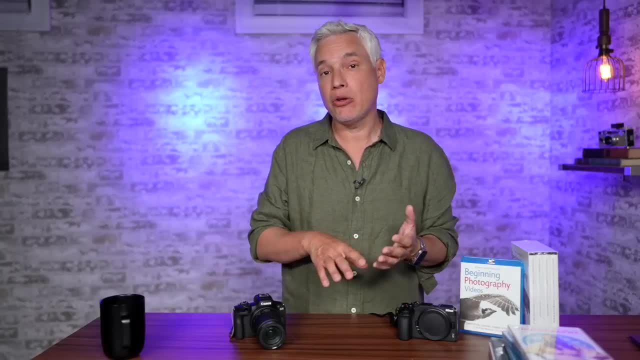 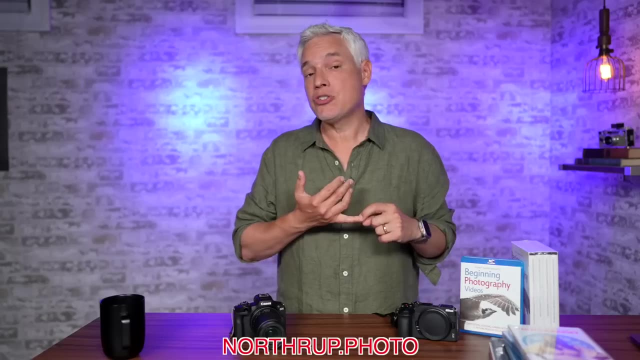 will tell the algorithm that they should share it with other people. And if you want more detailed photography instruction, head to Northropphoto. That's where we sell all of our educational content, including stunning digital photography. That's our award-winning, winning video book. It's a full book, but it also has 20 hours of video and lots of hands-on.